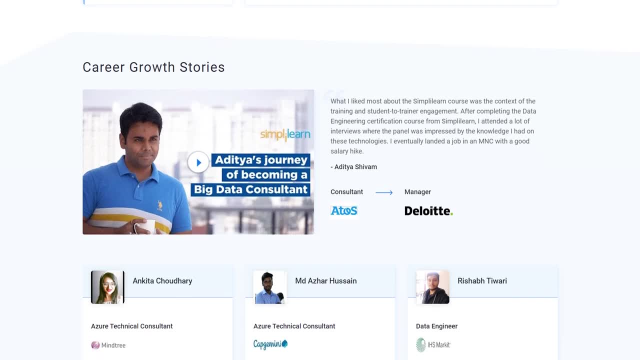 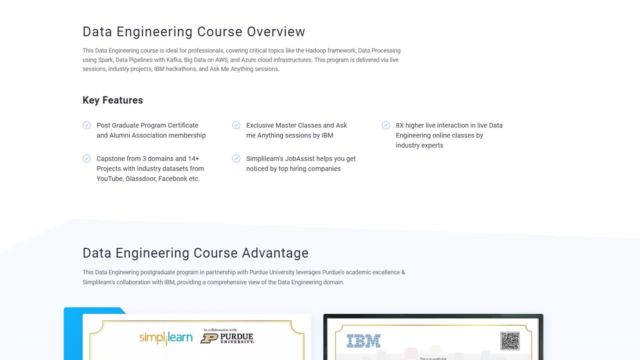 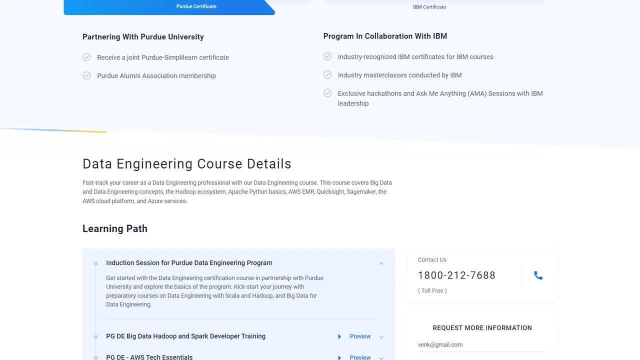 needs. This program offers an exceptional opportunity for professional growth and exposure. with a focus on practical learning and in alignment with industry-leading certifications from AWS and Azure, This program equips participants with essential skills required to excel in this field of data engineering. By enrolling in this applied learning program, individuals can gain master of crucial data. 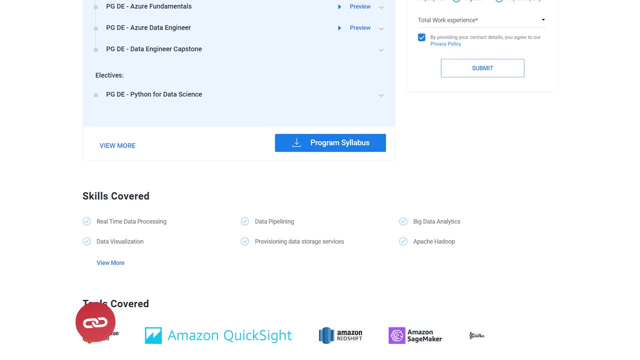 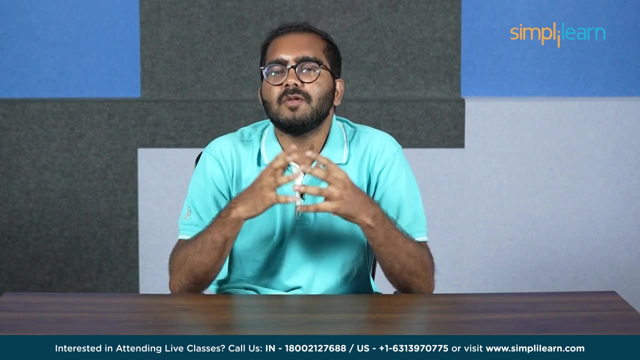 engineering techniques and technologies. Enroll today and take the next step towards becoming a proficient big data professional. Check out the course link in the description box below for more details. This course will explore big data and its challenges, exploring use cases and tools for processing and analyzing massive datasets. 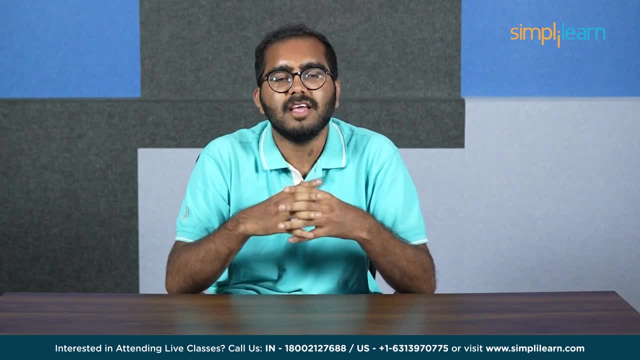 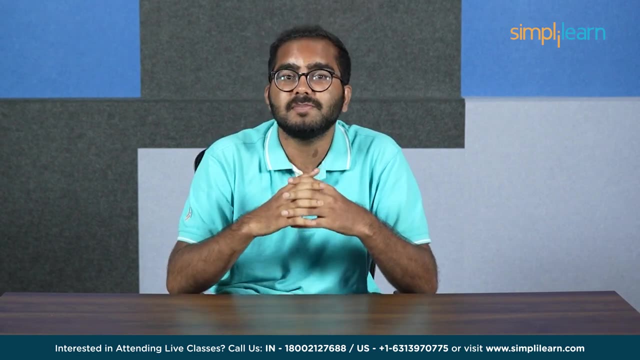 The course covers the Hadoop ecosystem, big data analytics using Python, data science concepts, processing analytics and the three V's of big data. Additionally, we will provide Hadoop interview questions by the end of this course. But before we begin, let's take a minute to hear from our learners who have experienced. 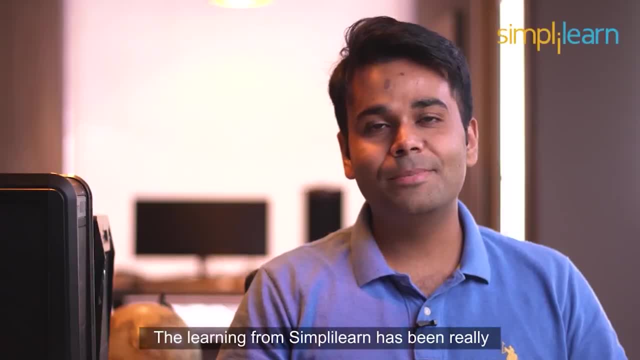 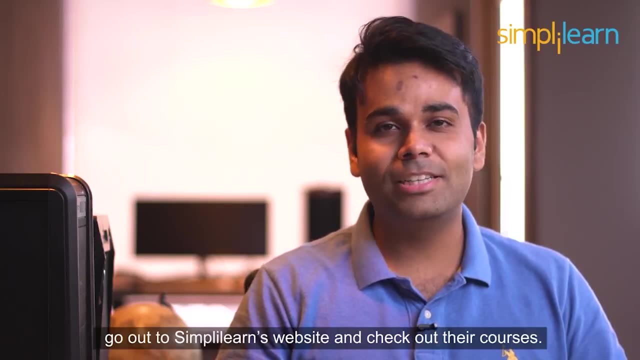 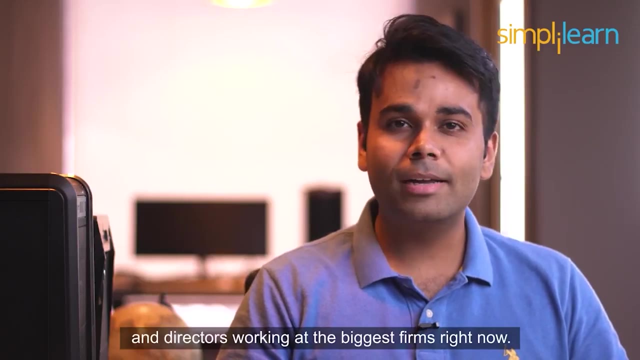 huge success in their careers. The learning from Simply Learn has been really amazing and extremely helpful. Whoever is watching this video, I recommend you go out to Simply Learn's website and check out their courses. They have brilliant instructors who are industry-wide solution architects and directors working. 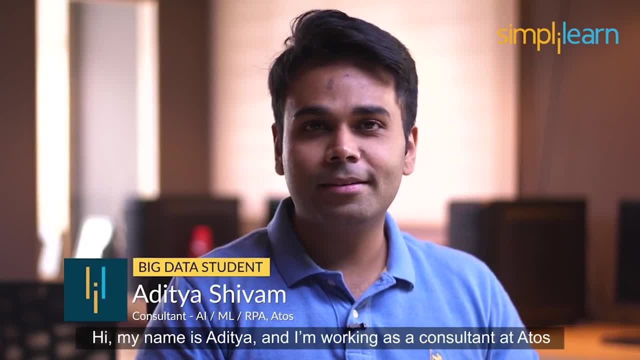 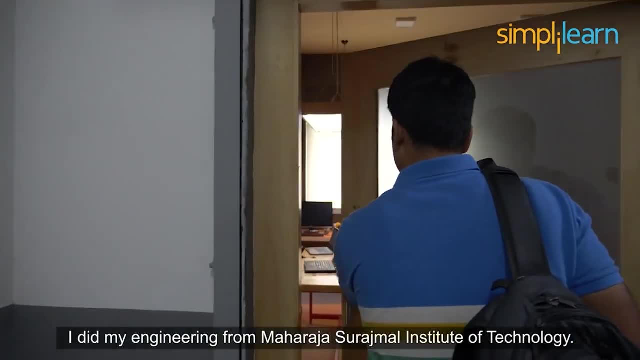 at the biggest firms right now. Hi, my name is Aditya and I'm working as a consultant in Atos in the field of AI, machine learning and RPA. I did my engineering from Maharaja Suraj Mal Institute of Technology. 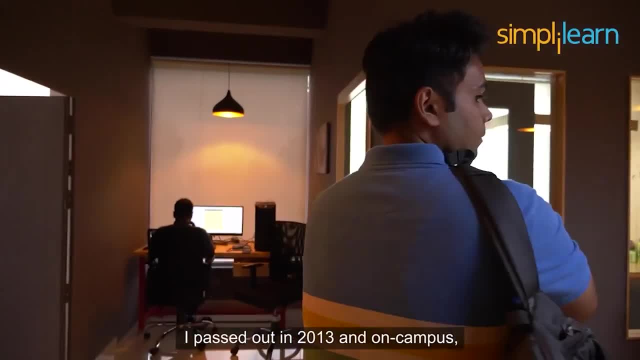 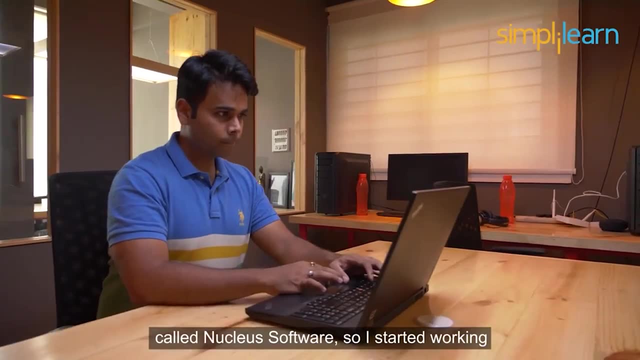 I majored in electronics and communication engineering. I passed out in 2013.. And on campus I got placed into a company called Nucleus Software. So I started working in software engineering team. The team was involved into application development using Oracle forms, SQL and database language. 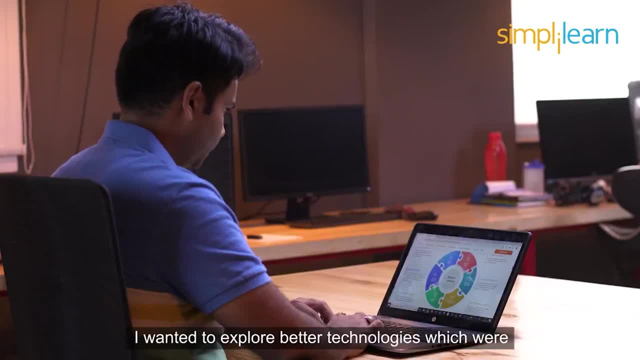 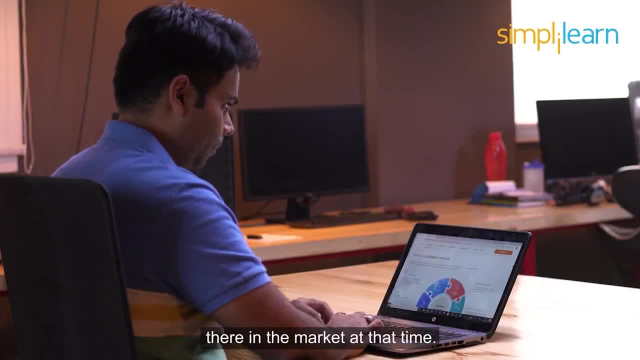 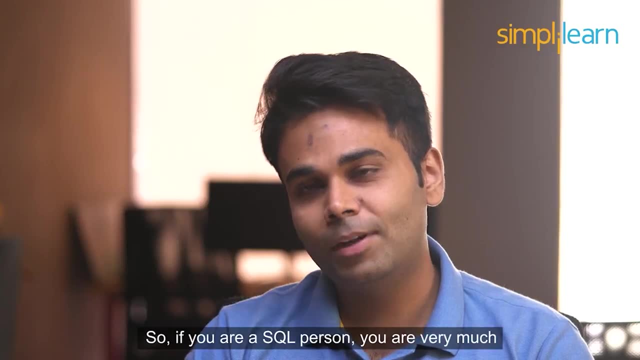 I wanted to explore better technologies which were there in the market. at that time I got to know that machine learning and big data- they revolve around SQL. So if you are a SQL person, you are very much comfortable with learning new machine learning. 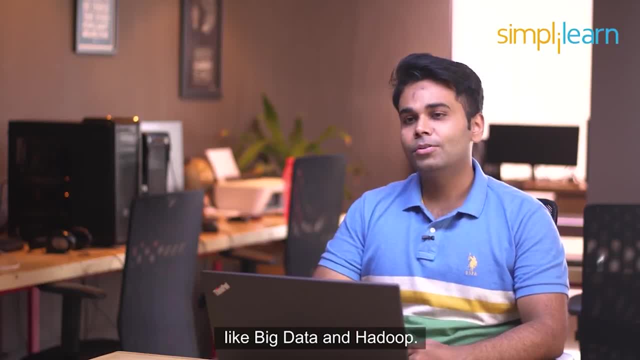 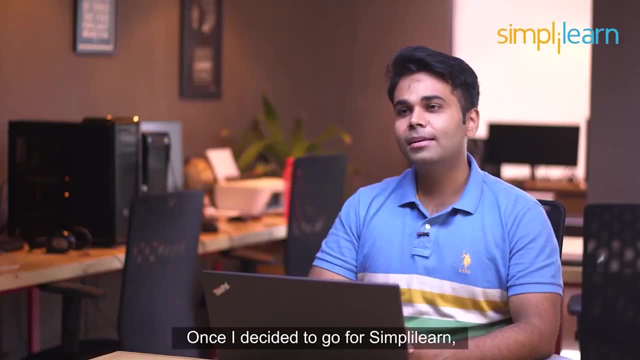 techniques and database technologies like Big Data, Hadoop. So that is when I started looking out for the training institutes And then my relative referred me. Once I decided to go for Simply Learn, I had one course in my mind, which was the content. 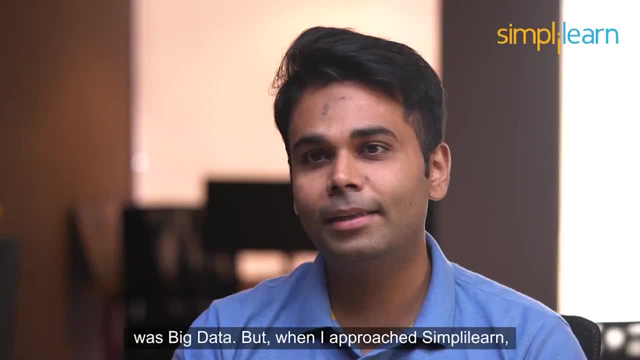 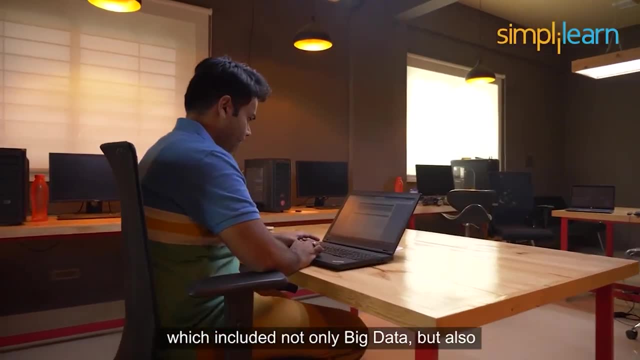 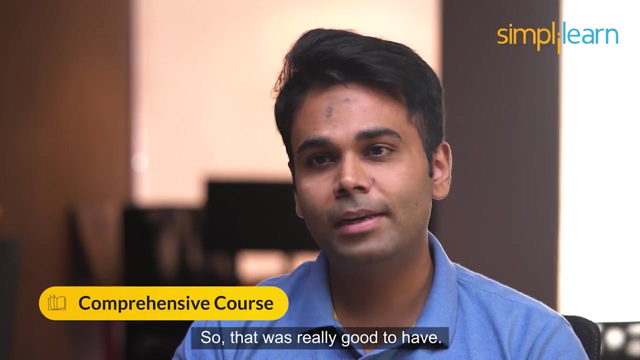 was big data only, but when I approached simply learn, they offered me a bundle of courses in one master program which included not only big data but also machine learning and Python basics- our basics, data science with Python- and some Java fundamentals as well. so that was really good to have. what I liked most. 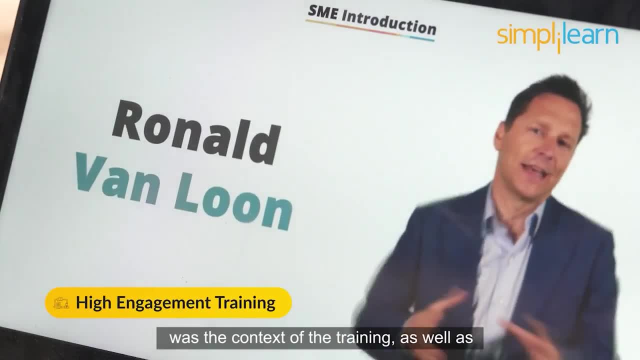 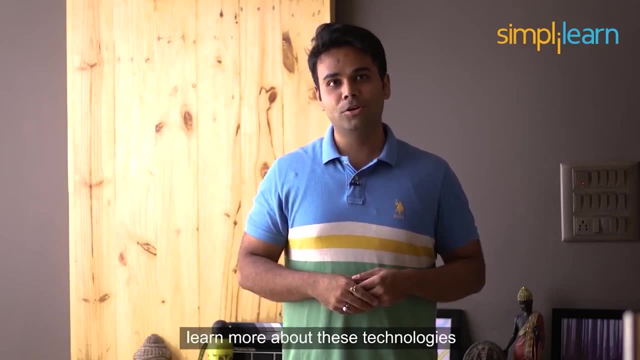 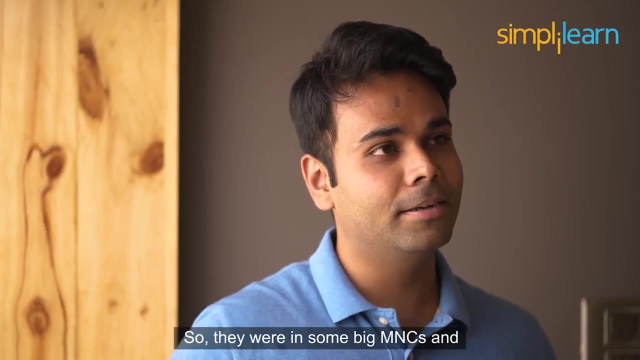 about the training was the context of the training as well as the instructor to student engagement. after the training, I got an opportunity to learn more of these technologies and once I was done learning, I attended a lot of interviews. so they were in some big MNCs and the interviewers were real-life big data. 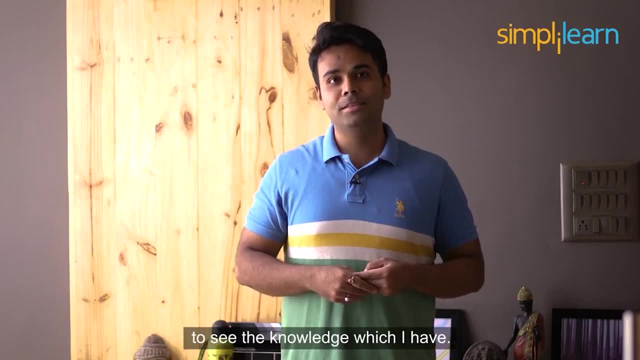 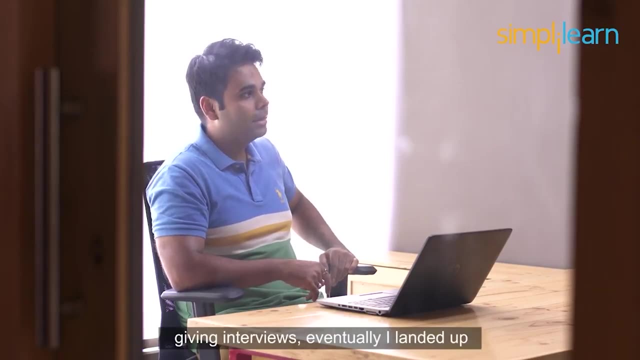 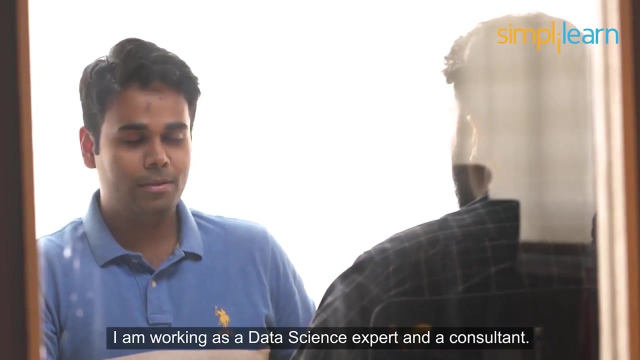 architects and data science experts and they were really happy to see the knowledge which I have so simply learn, definitely set up a base for me on that and, once I started giving interviews, eventually I landed up in a MNC in Chennai where I'm working as a data science expert and a consultant simply. 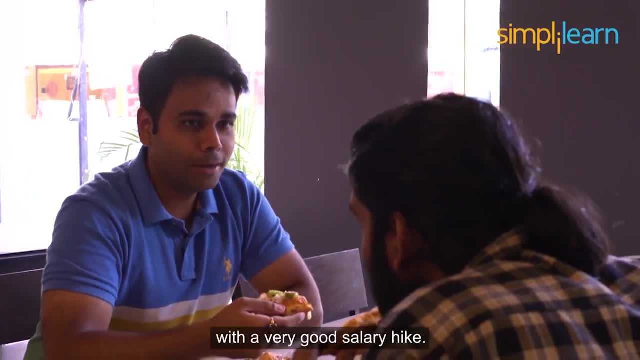 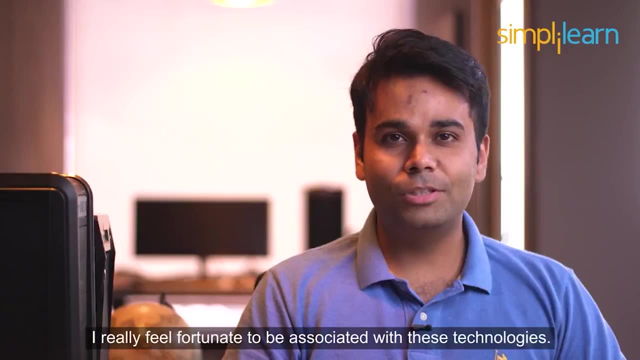 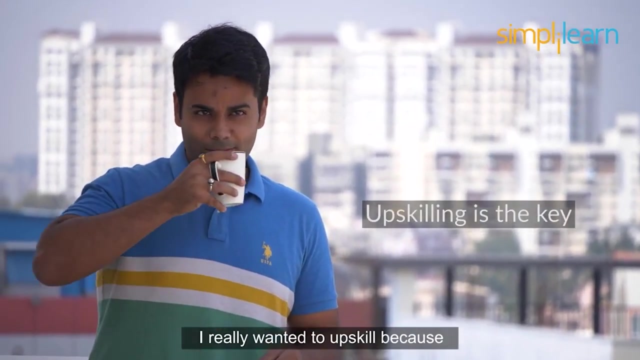 learns. big data master program helped me to get a new job with a very good salary hike. a very big thanks to simply learn for making me who I am. I feel really fortunate to be associated with these technologies. now I can lead different teams and drive different business transformation programs using my skill set. I really wanted to upscale. 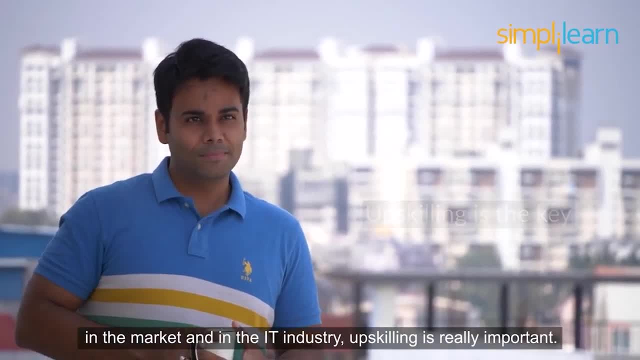 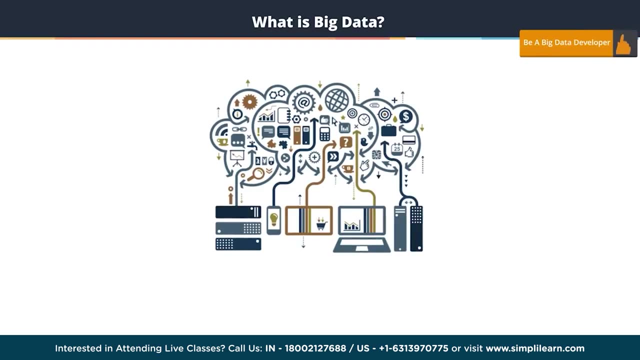 because in the market and in the IT industry, upscaling is really important. what is big data? big data is extremely large or complex set of data and it's so large that it's difficult to process it using traditional database and software techniques. every day we're creating 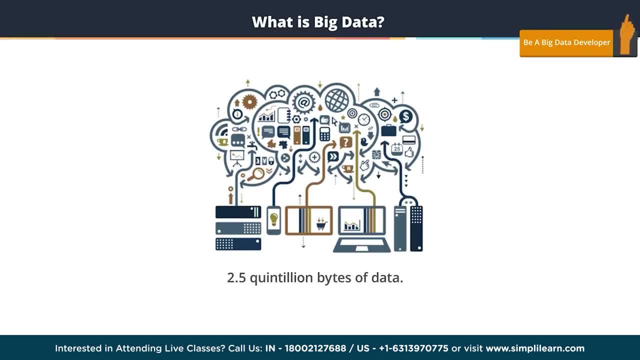 approximately 2.5 quintillion bytes of data. so where is this huge amount of data getting generated? from earlier, we had mobile phones with the functionality of calling and text messages, or clicking some pictures maybe. but with the new technologies like smartphones, we have a lot of applications for music, sports. 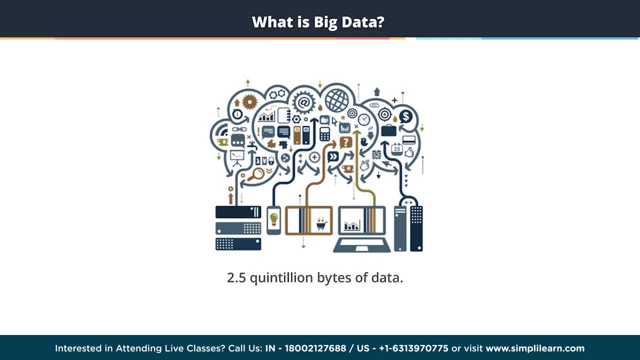 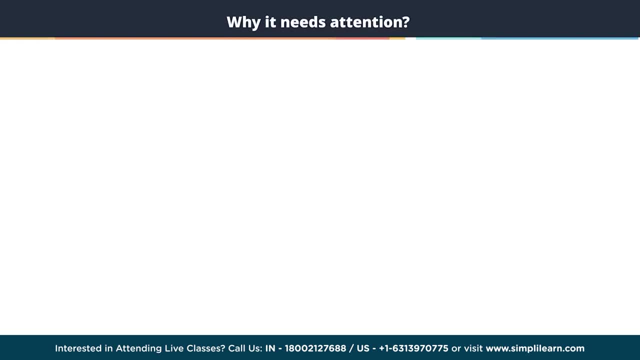 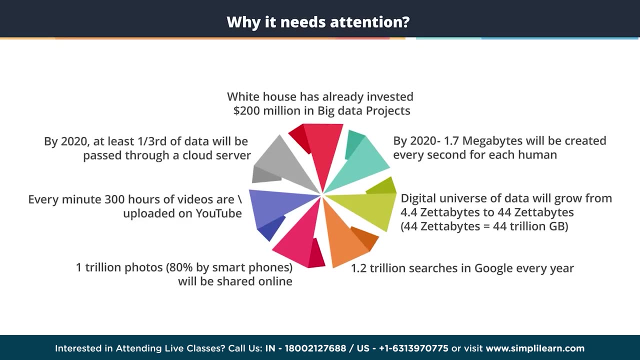 social media like facebook, twitter, linkedin and many more. also, data is getting generated when we shop online. so why does it need attention? as the data is growing, companies are capturing the data that streams into their businesses. they can apply analytics and get significant value from it with better speed and efficiency. companies are leveraging the 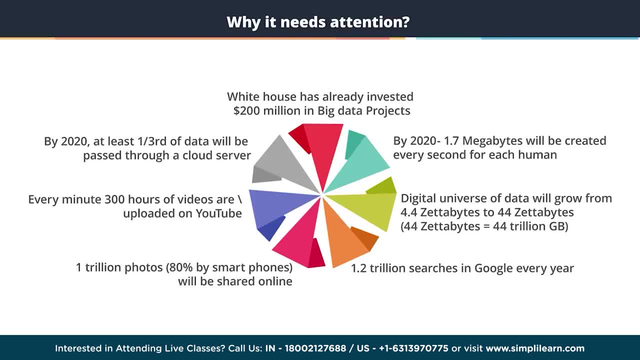 benefits of big data by analyzing the patterns and trends and predicting something useful out of it. for example, companies like Amazon and Netflix use big data to improve customer experience. as we see here from the statistics shown, by 2020, 1.7 megabytes of data will be. 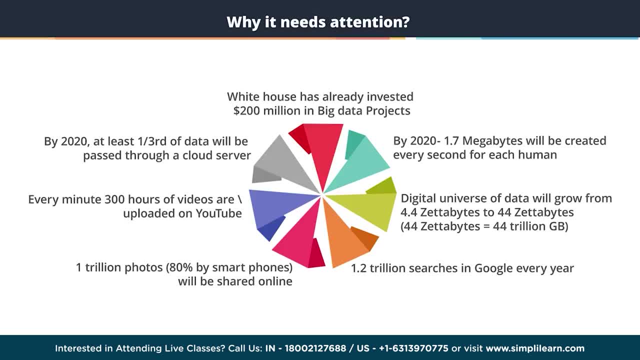 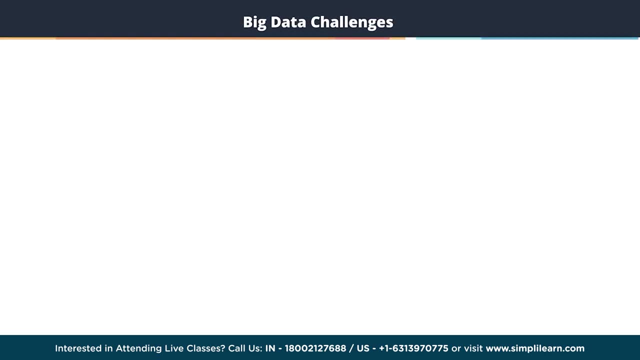 created every second for each human. this needs immediate attention because this data can't be just thrown away. it's going to give profit to the businesses. big data challenges. big data is not just about the volume of data. it poses other challenges as well, like velocity and variety. as a volume: 4d. 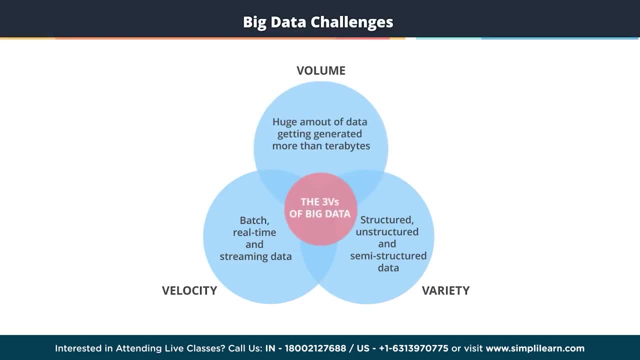 zettabytes of data will be created by 2020. this huge volume of data is either human-generated, like from social media, YouTube, or can be machine generated, like through sensors and personal health trackers, and can also be generated with organizations like credit card details, commercial transactions and medical 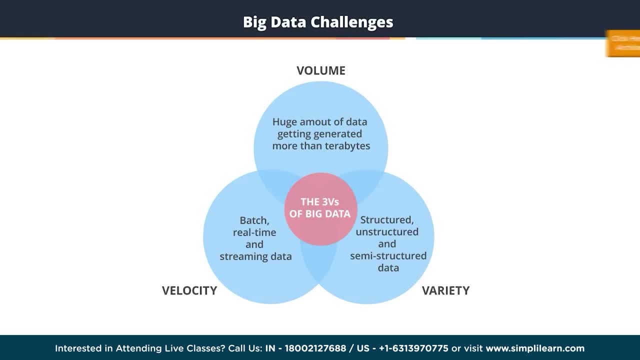 records. Another challenge is velocity, The speed at which data is coming into the system. the data needs to be processed with faster speed. And then there is variety of data. Data is not only structured, but unstructured and semi-structured data like images, videos and tweets. 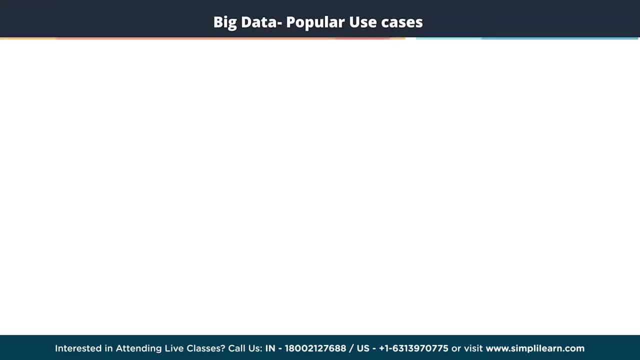 So how are enterprises using this big data today? Let us see big data popular use cases, Internet of Things: These are numerous ways in which analytics can be applied to Internet of Things. For example, sensors are used to collect data that can be analyzed to achieve actionable insights: tracking customer or product movement, etc. 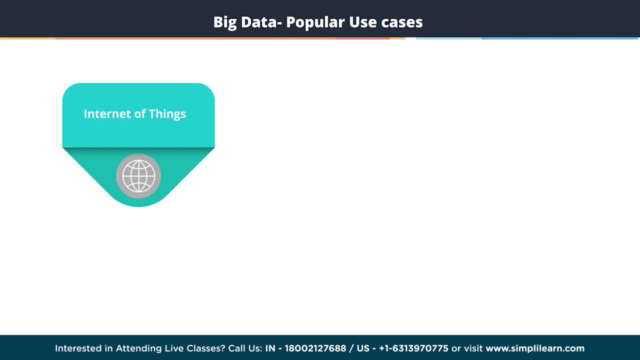 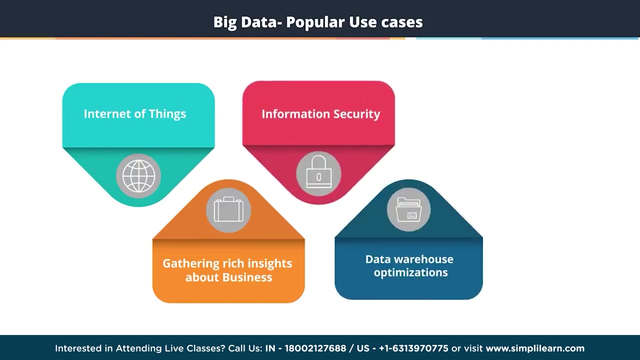 Many enterprises are creating a dashboard application that provides a 360-degree view of the customers, that pulls data from a variety of sources, Analyzes it and presents it to customer service So that allows them to gather the rich insights about businesses. Big data- popular use cases are related information security and data warehouse optimizations. 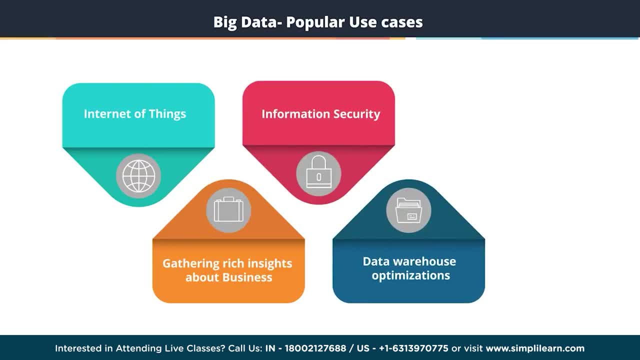 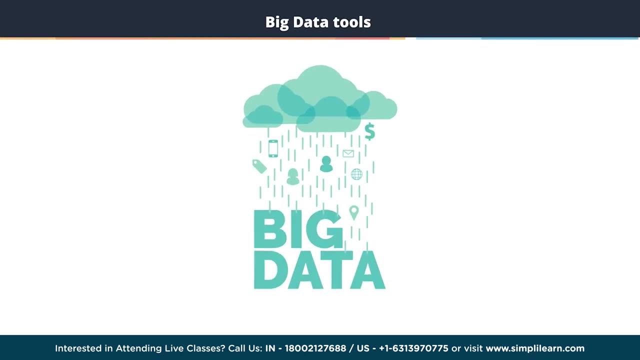 Big data tools are being used to remove some of the burdens from the data warehouses. Even the healthcare industry is looking for patterns in treatment that lead to the best outcomes for patients. The main purpose of big data: popular use cases. The main challenge of big data is storing and processing the data at a specified time span. 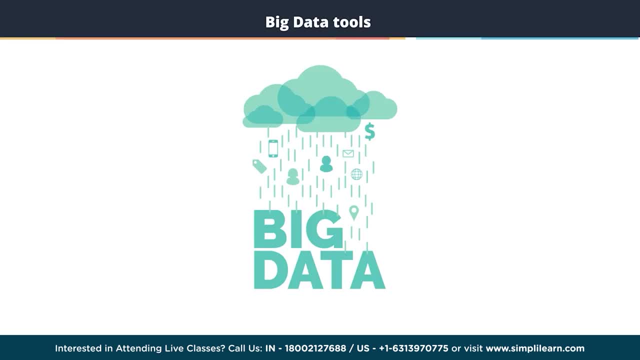 The traditional approach is not efficient in doing that, So Hadoop technology and various big data tools have emerged to solve the challenges faced in the big data environment. So there are a lot of big data tools and all of them help the user in some or another way in saving time, money and uncovering business insights. 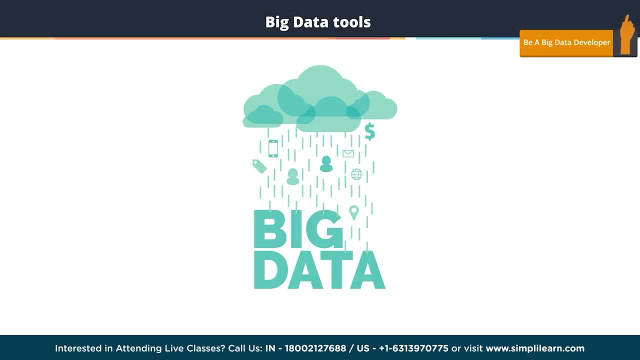 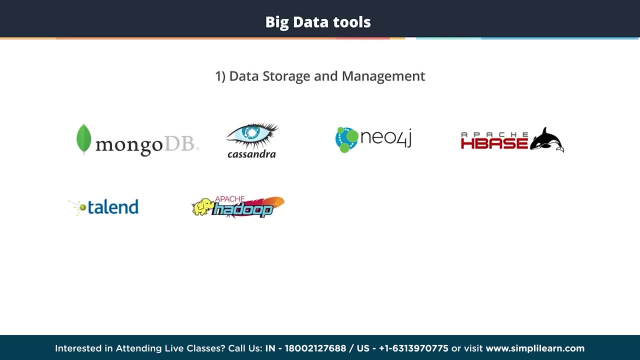 These can be divided into the following categories, like data storage and management. For example, the NoSQL databases such as MongoDB, Cassandra, Neo4j and HBase are popular NoSQL databases. The Talend, Hadoop, Microsoft HD, Insight and Zookeeper are popular for data storage and management tools. 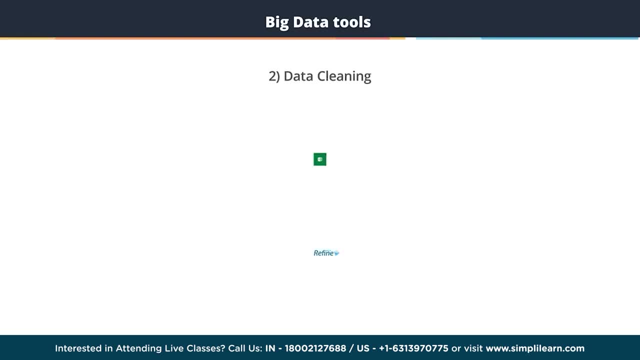 Next broad category is data cleaning. Data needs to be cleaned regularly. Data needs to be cleaned up and well structured. Examples of such tools, which help in defining and reshaping the data into usable data sets, are Microsoft Excel and OpenRefine. Data mining is a process of discovery insights within a database. 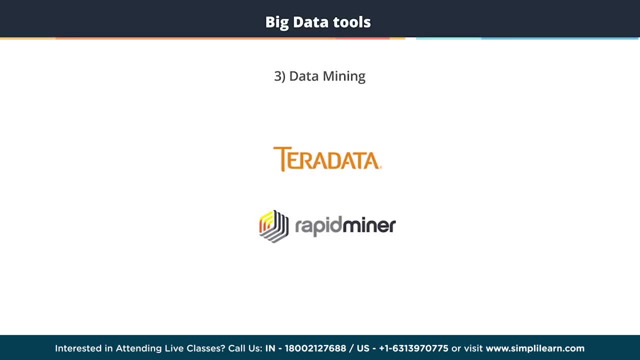 Some of the popular tools used for data mining are Teradata and RapidMiner. Data visualization tools are a useful way of conveying the complex data insights in a pictorial way that is easy to understand. For example, Tableau and IBM Watson, Analytics and Plotly are the common tools. 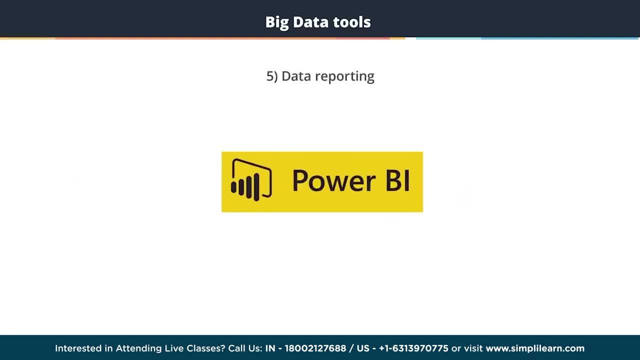 For data reporting, Power BI tools are used. Data ingestion is the process of getting the data into Hadoop Forward, which can be done using Scoop, Flume or Storm. Data analysis requires asking questions and finding the answers in data. The popular tools used for data analysis are Hive Pig, MapReduce and Spark. 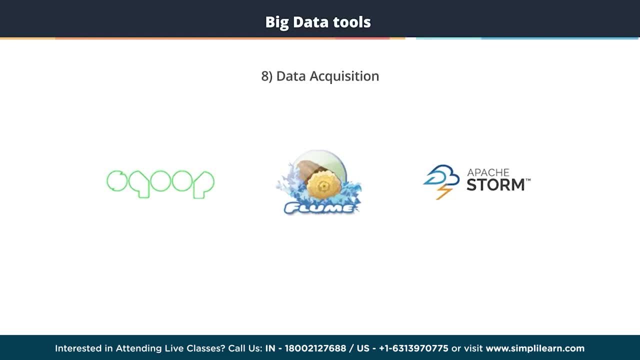 Data acquisition is also used for acquiring the data, for which Scoop, Flume or Storm tools are quite popular. The popular big data tools offer a lot of advantages, which can be summarized as follows: They provide the analyst with advanced analytics algorithm and models. 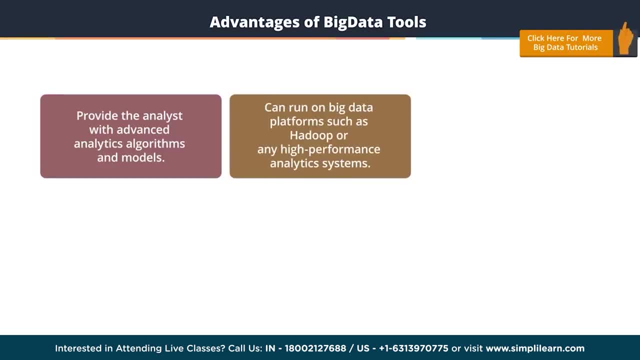 They help the user to run on big data platforms such as Microsoft Office, Google Docs and Google Docs. They help the user to run on big data platforms such as Hadoop or any high performance analytics systems. They help the user to work not only with structured data, but unstructured and semi-structured data coming from multiple sources. 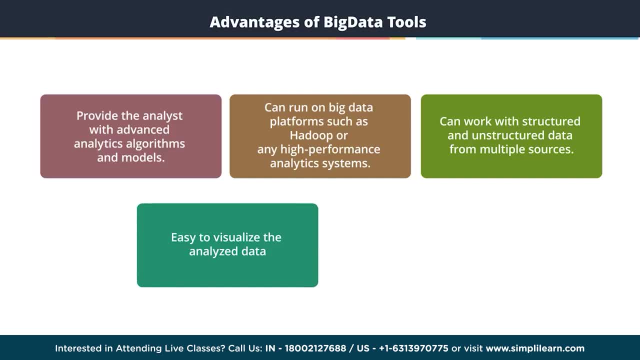 And it's quite easy to visualize the analyzed data in a form that helps in conveying the complex data insights in a pictorial way which is easy to understand by users. Big data tools help you to integrate with other technologies very easily. Thank you so much for listening to the video. 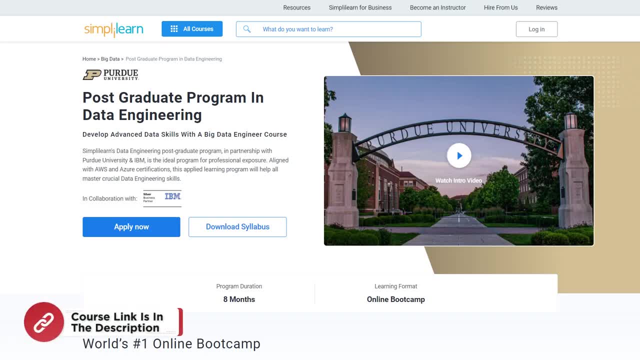 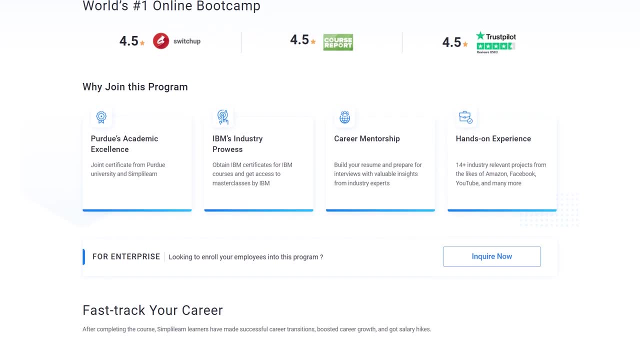 Now. whether you're an aspiring data analyst, a seasoned IT professional or a business leader looking to leverage the power of big data, the Data Engineering Postgraduate Program by SimplyLearn, in collaboration with Purdue University and IBM, is tailored to meet your needs. 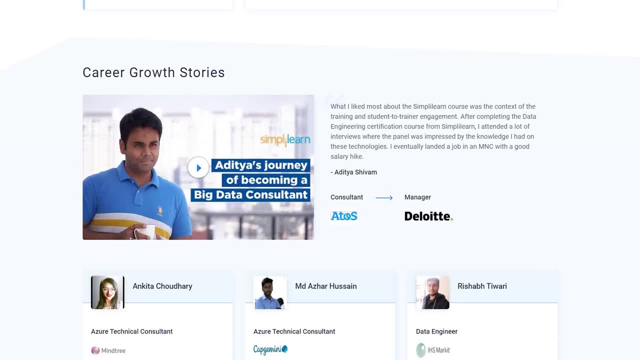 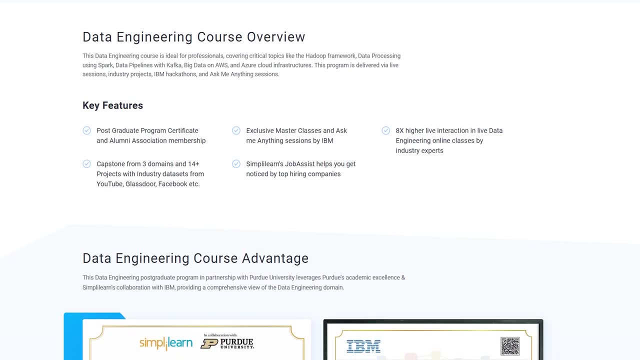 This program offers an exceptional opportunity for professional growth and exposure, with a focus on practical learning and in alignment with industry-leading certifications from AWS and Azure. Thank you so much for listening to the video Now. this program equips participants with essential skills required to excel in this field of data engineering. 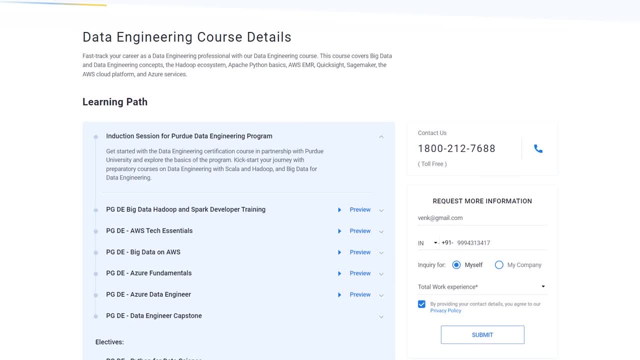 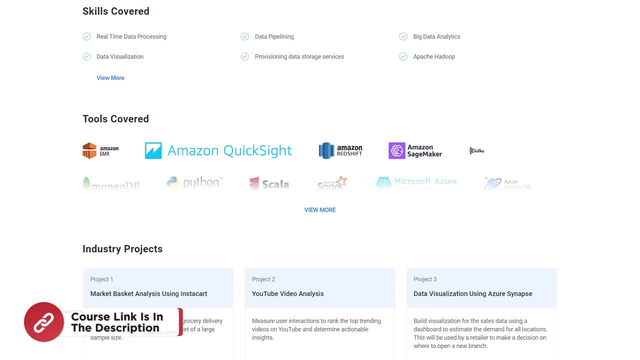 By enrolling in this applied learning program, individuals can gain master's in crucial data engineering techniques and technologies. Enroll today and take the next step towards becoming a proficient big data professional. Check out the course link in the description box below for more details. 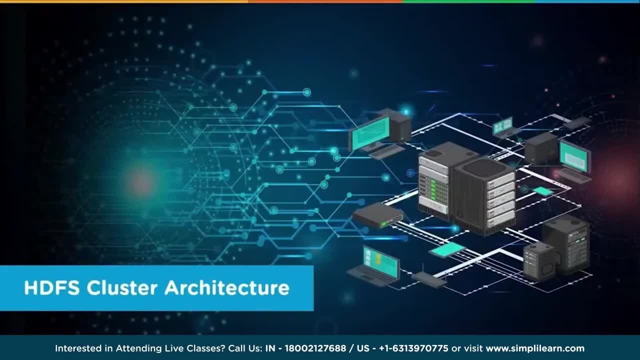 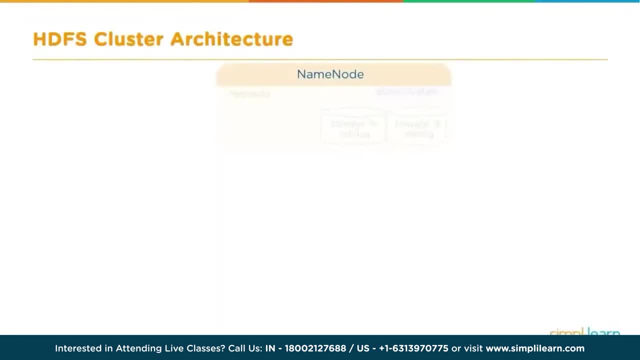 So we took a look at the master node and the name node and the secondary name node. Let's take a look at the cluster architecture of our Hadoop file system, The HDFS cluster architecture. So we have our name node and it stores the metadata and we have our block location. 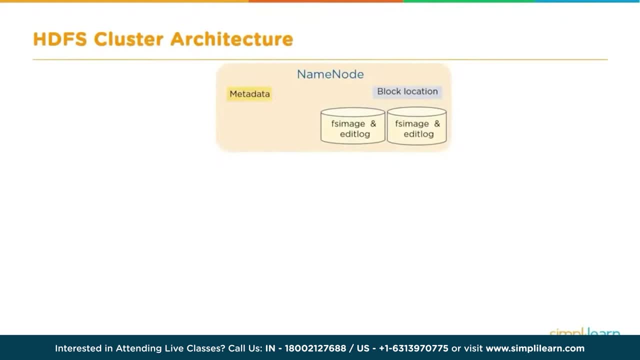 So we have our FS image plus our edit log, and then we have the backup FS image and edit log And then we have. so you have your rack, we have our switch on top- Remember, I was talking about the switch. That's the most common thing to go in the rack is the switches. 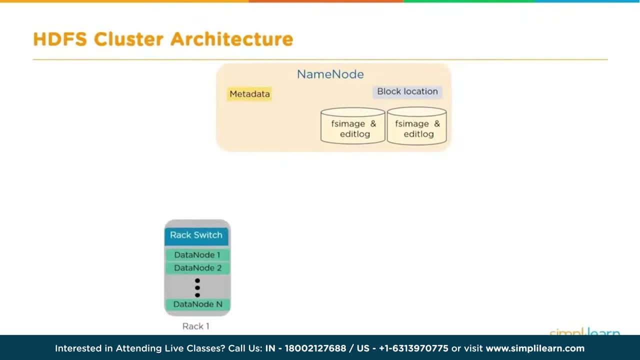 And underneath the rack you have your different data nodes. You have your data node 1, 2, 3, 4, 5, maybe you have 10, 15 on this rack. You can stack them pretty high nowadays. 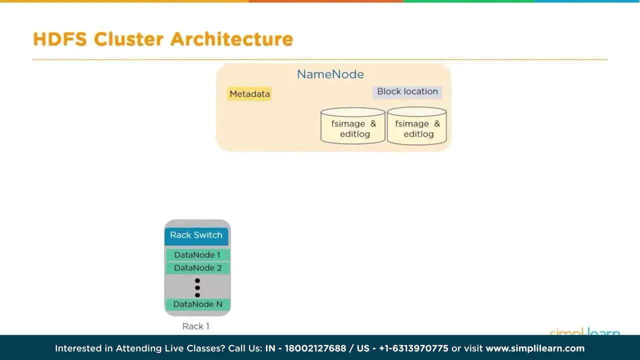 It used to be, you'd only get about 10 servers on this rack, But now you see racks that contain a lot more, And then you have multiple racks, So we're not talking about just one rack. We also have, you know, rack 2,, rack 3,, 4,, 5,, 6, and so on until you have rack N. 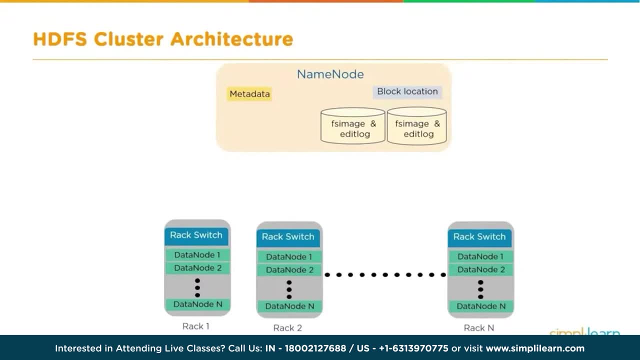 So if you had 100 data nodes, we would be looking at 10 racks of 10 data nodes each, And that is literally 10 commodity server computers, hardware, And we have a core switch which maintains the network bandwidth and connects the name node to the data nodes. 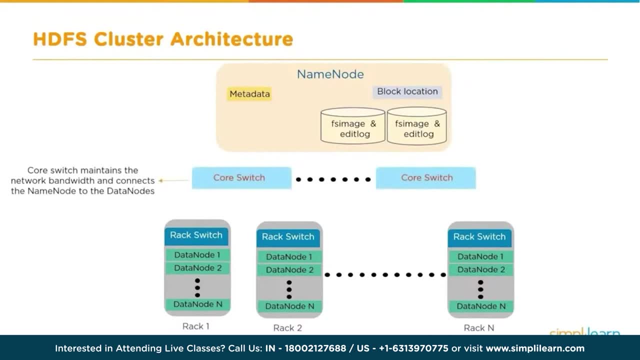 So, just like each rack has a switch that connects all your nodes on the rack, you now have core switches that connect all the racks together And these also connect into our name node setup. So now it can look up your FS image and your edit log and pull that information, your metadata, out. 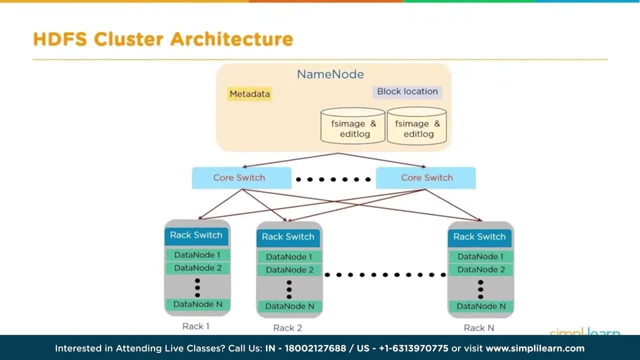 So we've looked at the architecture, from the name node coming down And you have your metadata, your block locations. This then sorts it out. You have your core switches which connect everything, all your different racks, And then each individual rack has their own switches which connect all the different nodes and to them. 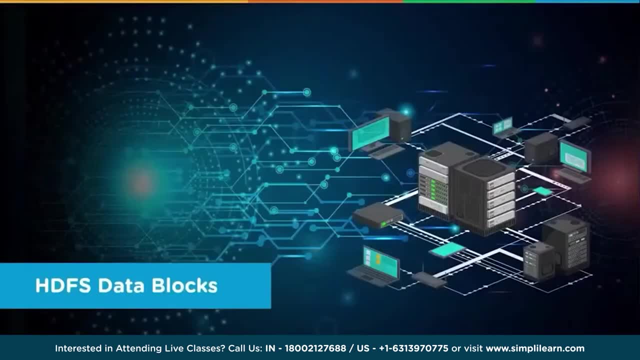 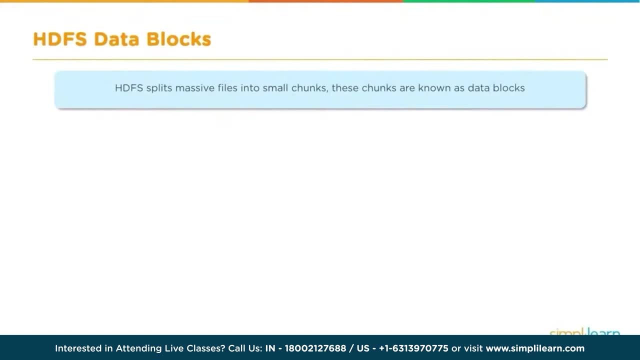 So these are the core switches. So now let's talk about the actual data blocks. What's actually sitting on those commodity machines? And so the Hadoop file system splits massive files into small chunks. These chunks are known as data blocks. 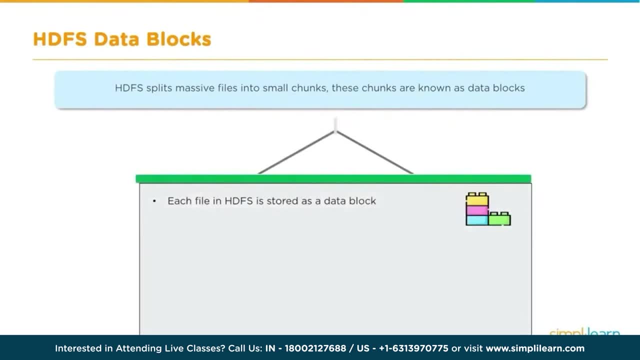 Each file in the Hadoop file system is stored as a data block And we have a nice picture here where it looks like a Lego. If you ever played with the Legos as a kid, it's a good example. We just stacked that data right on top of each other. 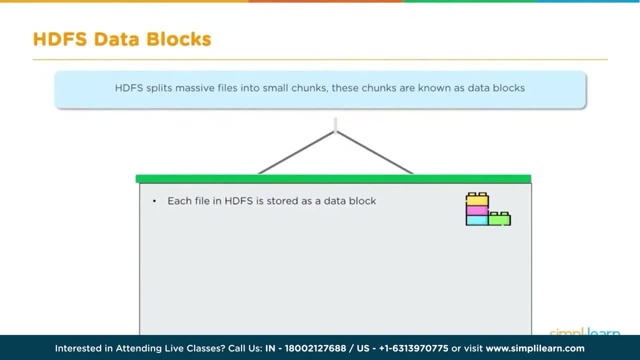 But each block has to be the same symmetry. It has to be the same size so that it can track it easily, And the default size of one data block is usually 128 megabytes. Now you can go in and change that. This standard is pretty solid as far as most data is concerned, when we're loading up huge amounts of data. 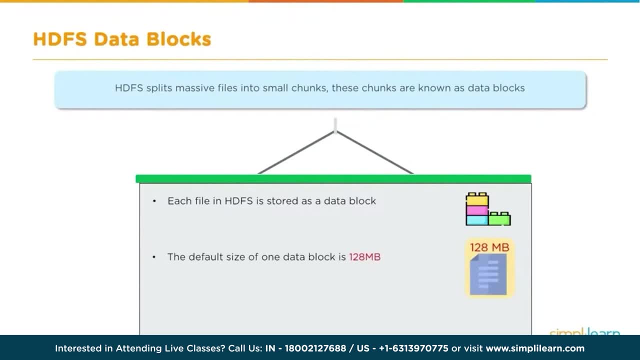 And there's certainly reasons to change it, But 128 megabytes is a pretty standard block, So why 128 megabytes? If the block size is smaller, then there will be too many data blocks along with lots of metadata, which will create overhead. 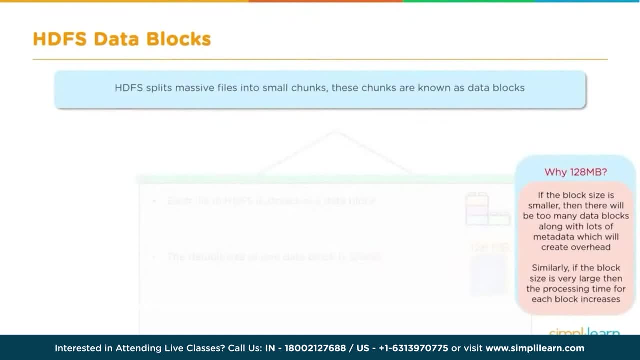 So that's why you don't really want to go smaller on these data blocks, unless you have a very certain kind of data. Similarly, if the block size is very large, then the processing time for each block increases. Then, as I pointed out earlier, each block is the same size, just like your Lego blocks are all the same. 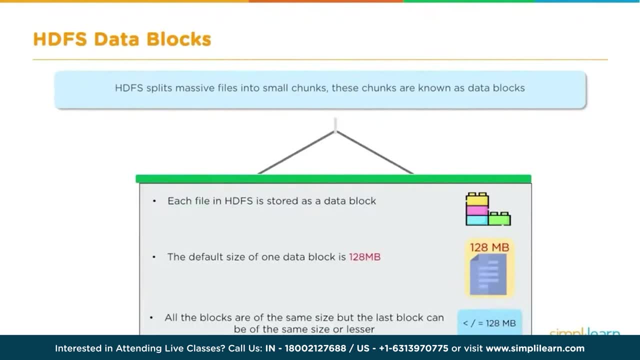 But the last block can be the same size or less, So you might only be storing 100 megabytes in the last block And you can think of this as if you had a terabyte of data that you're storing on here. It's not going to be exactly divided into 128 megabytes. 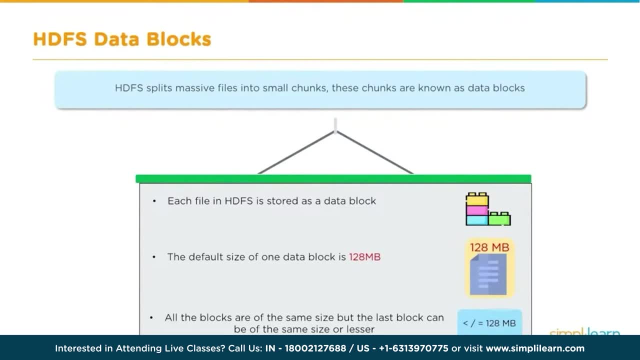 We just store all of it at 128 megabytes, except for the last one, which could have anywhere between 1 and 128 megabytes, depending on how evenly your data is divided. Now let's look into how files are stored in the Hadoop file system. 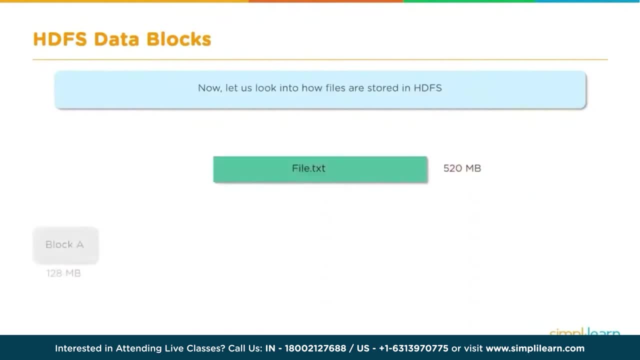 So we have a file text- Let's say it's 520 megabytes. We have block A, So we take 128 megabytes out of the 520 and we store it in block A, And then we have block B. 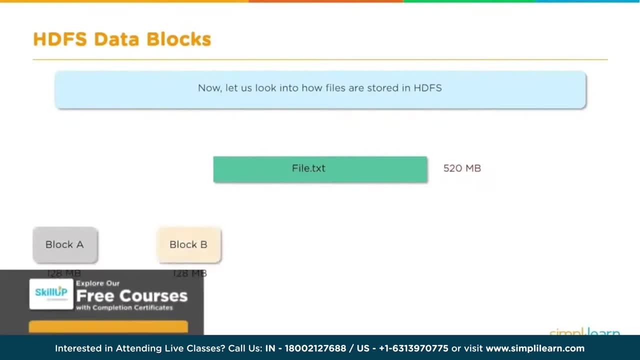 Again, we're taking 128 megabytes out of our 520 and storing it there, And so, on Block C, Block D And then block E, we only have 8 megabytes left. So when you add up 128 plus 128, plus 128 plus 128,. 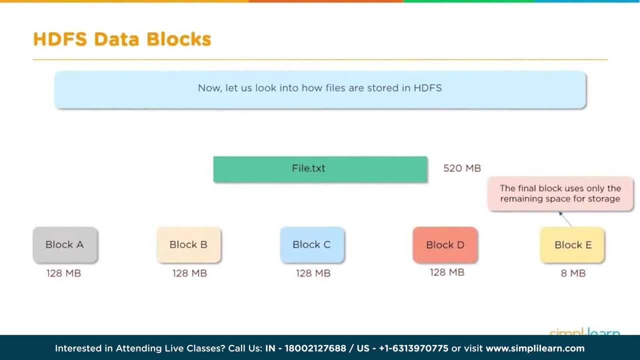 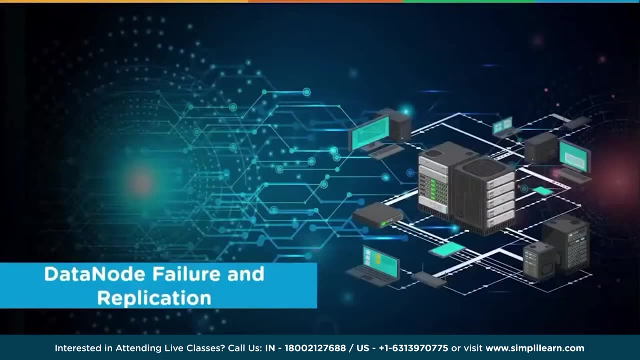 you only get 512. And so that last 8 megabytes goes into its own block. The final block uses only the remaining space for storage, Data node failure and replication, And this is really where Hadoop shines. This is why you can use it with commodity computers. 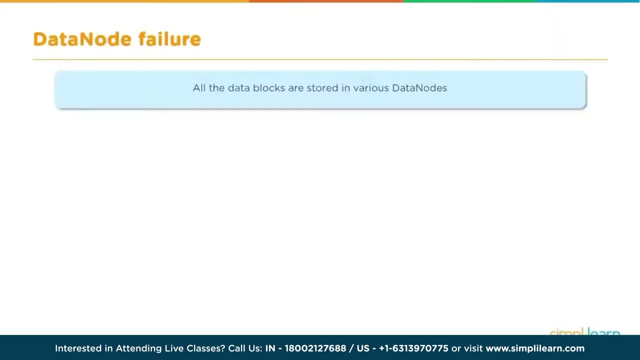 This is why you can have multiple racks and have something go down. All the data blocks are stored in various data nodes. You take each block, You store it at 128 megabytes And then we're going to put it on different nodes. 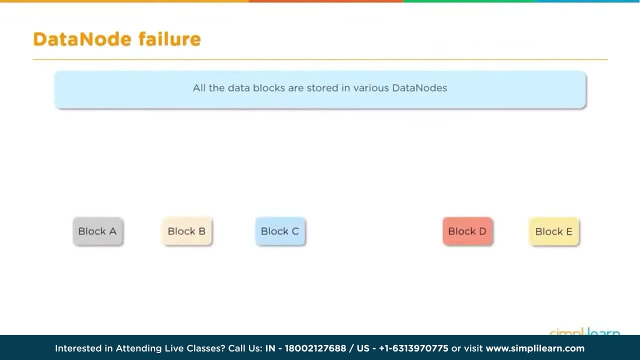 So here's our block A, block B, block C from our last example, And we have node 1, node 2, node 3, node 4, node 5, node 6.. And so each one of these represents a different computer. 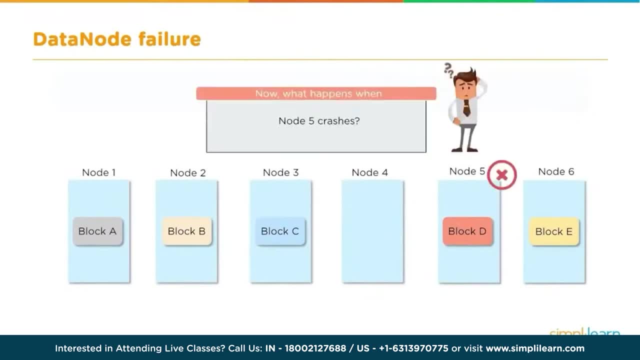 It literally splits the data up into different machines. So what happens if node 5 crashes? Well, that's a big deal. I mean, we might not even have just node 5. You might have a whole rack go down, And if you're a company that's building your whole business off of that. 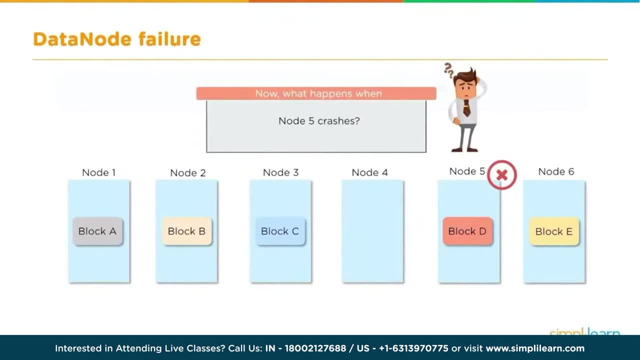 you're going to lose a lot of money. So what does happen when node 5 crashes? When node 5 crashes or the first rack goes down, the data stored in node 5 will be unavailable, as there is no copy stored elsewhere in this particular image. 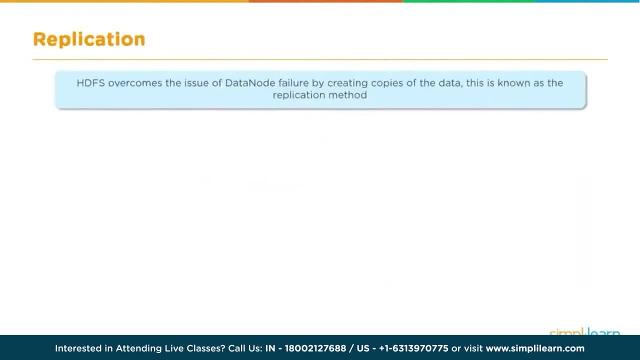 So the Hadoop file system overcomes the issue of data node failure by creating copies of the data. This is known as the replication method, And you can see here we have our six nodes. Here's our block A, But instead of storing it just on the first machine, 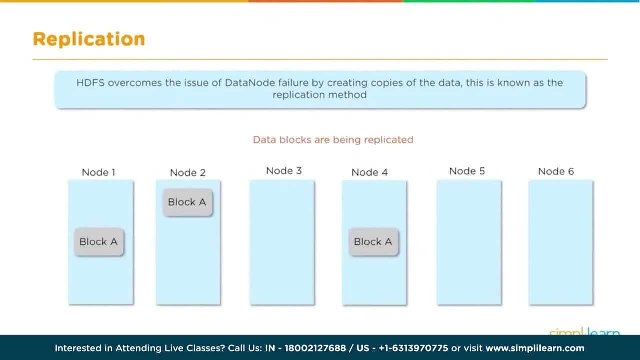 we're actually going to store it on the second and fourth nodes. So now it's spread across three different computers And in this, if these are on a rack, one of these is always on a different rack, So you might have two copies on the same rack. 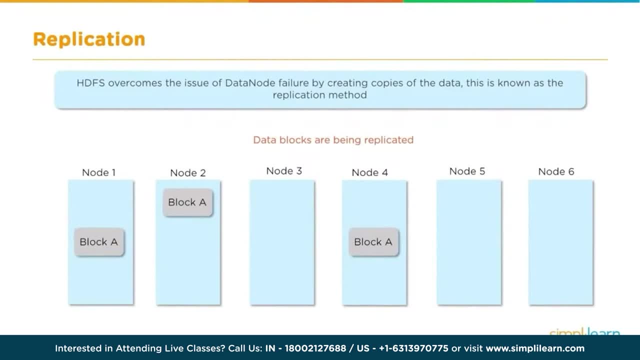 but you never have all three on the same rack And you always have. you never have more than two copies on one node. There's no reason to have more than one copy per node. And you can see we do the same thing with block B. 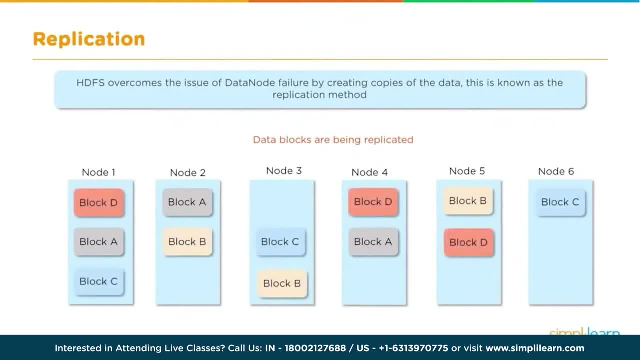 Block C is then also spread out across the different machines And same with block D and block E. Node 5 crashes. Will the data blocks B, D and E be lost? Well, in this example, no, Because we have backups of all three of those on different machines. 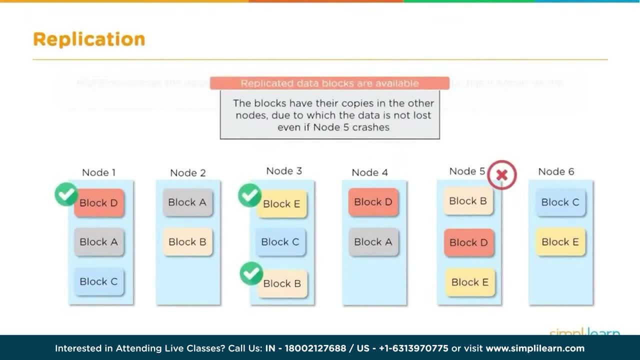 The blocks have their copies in the other nodes, due to which the data is not lost even if the node 5 crashes, And again because they're also stored on different racks. even if the whole rack goes down, you are still up and live with your Hadoop file system. 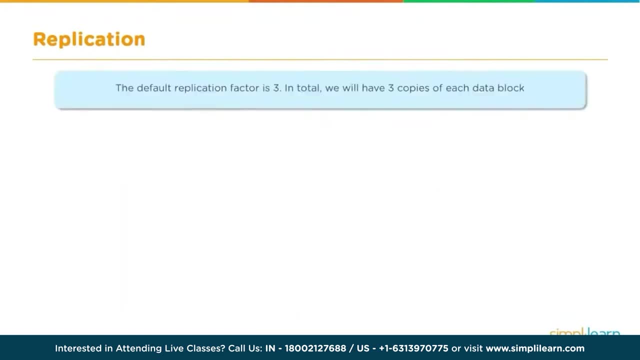 The default replication factor is three. In total, we'll have three copies of each data block. Now that can be changed for different reasons or purposes, But you've got to remember when you're looking at a data center. this is all in one huge room. 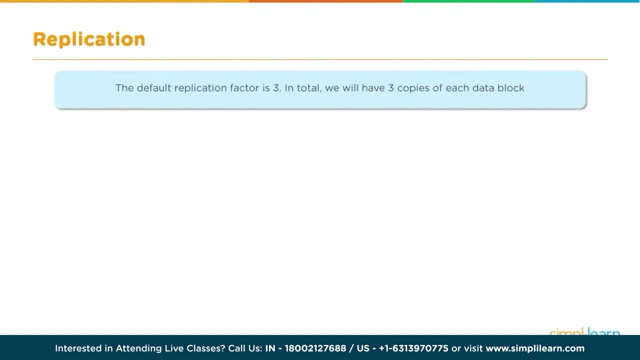 These switches are connecting all these servers so they can shuffle the data back and forth really quick, And that is very important when you're dealing with big data. And you can see here each block is by default replicated three times. That's the standard. 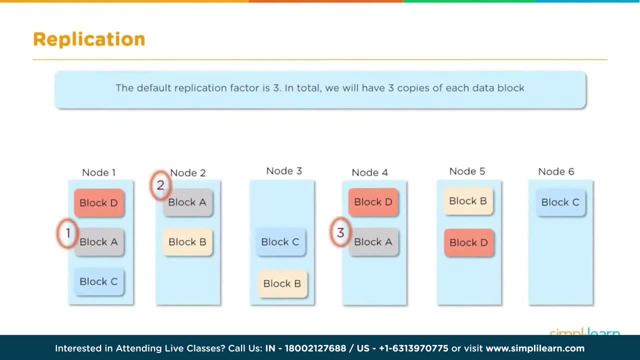 There is very rare occasions to do four, and there's even fewer reasons to do two blocks. I've only seen four used once, and it was because they had two data centers and so each data center kept two different copies. Rack awareness in the Hadoop file system. 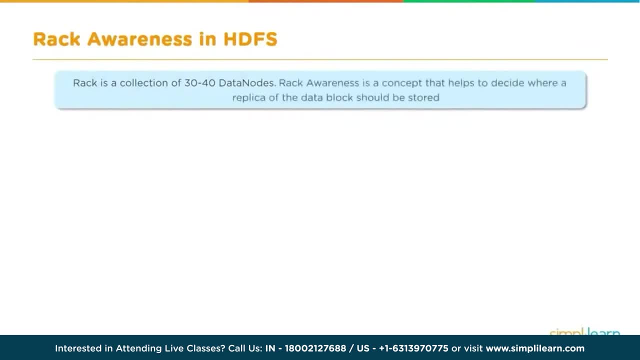 Rack is a collection of 30 to 40 data blocks. Rack awareness is a concept that helps to decide where the replica of the data block should be stored. So here we have rack one, We have our data node, one to four. Remember I was saying that it used to be: you only put 10 machines. 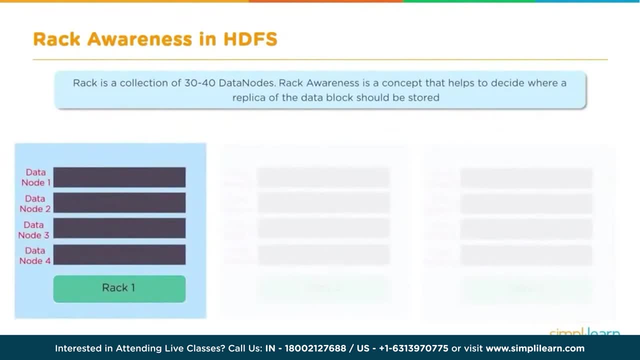 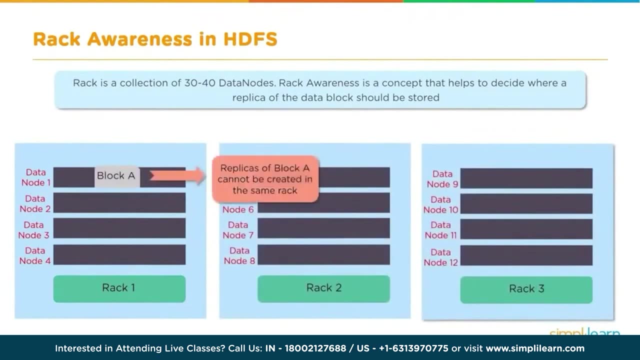 and then it went to 20, now it's 30 to 40. So you can have a rack with 40 servers on it. Then we have rack two and rack three and we put block one on there. Replicas of block A cannot be in the same rack. 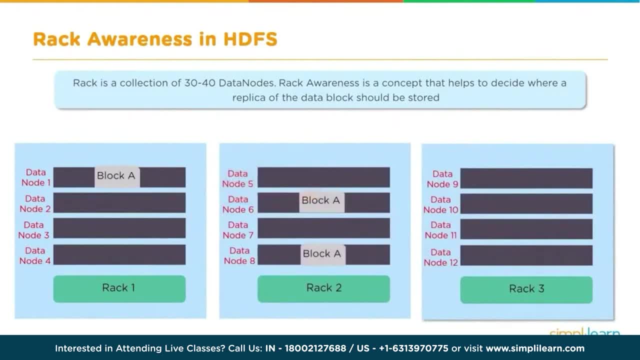 and so it'll put the replicas onto a different rack And notice that these are actually. these two are on the same rack, but you'll never have all three stored on the same rack, in case the whole rack goes down And replicas of block A are created in rack two. 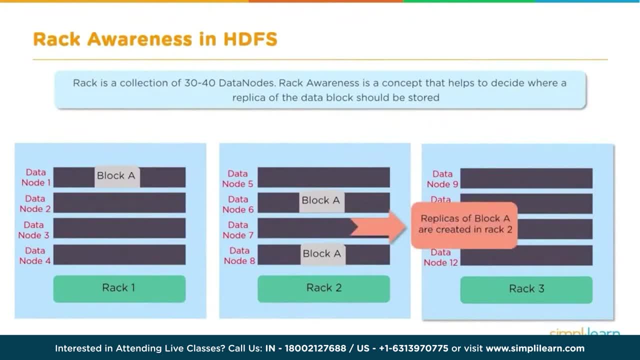 And they actually do. They do, by default, create the replicas onto the same rack, and that has to do with the data exchange and maximizing your processing time. And then we have, of course, our block B, and it's replicated onto rack three. 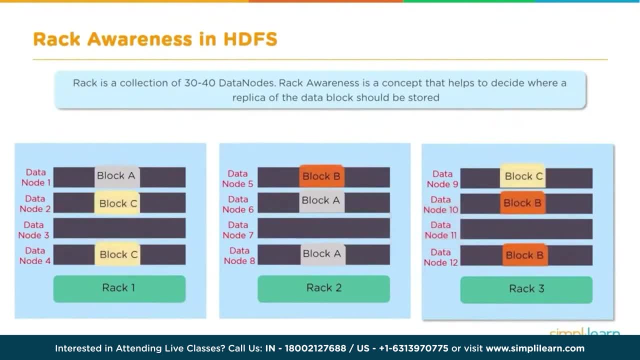 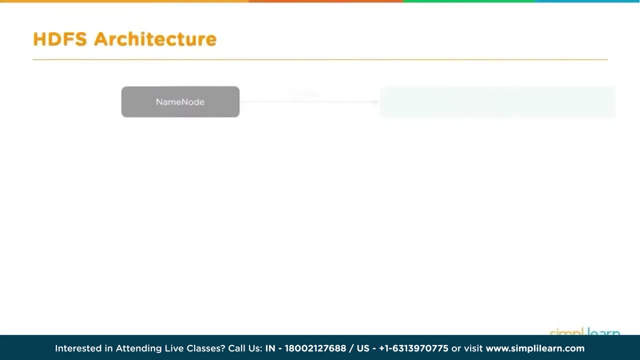 and block C, which will then replicate onto rack one and so on for all of your data, all the way up to block D or whatever, how much ever data you have on there. So let's look over the architecture as a bigger picture. 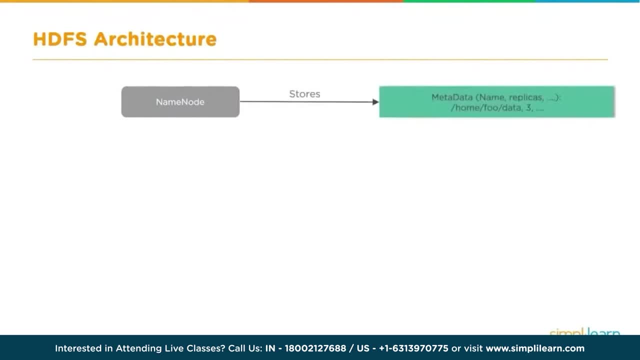 We looked at the name node and we stored some metadata names, replicas, home, food, data, three. so it has all your different metadata stored on there, And then we have our data nodes and you can see our data nodes are each on different racks. 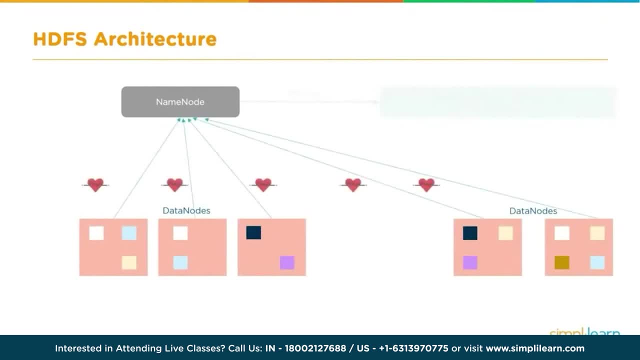 with our different machines And we have our name node and you can see we have a heartbeat or pulse here And a lot of times one of the things that confuses people sometimes in class is they talk about nodes versus machines. So you could have a data node that's a Hadoop data node. 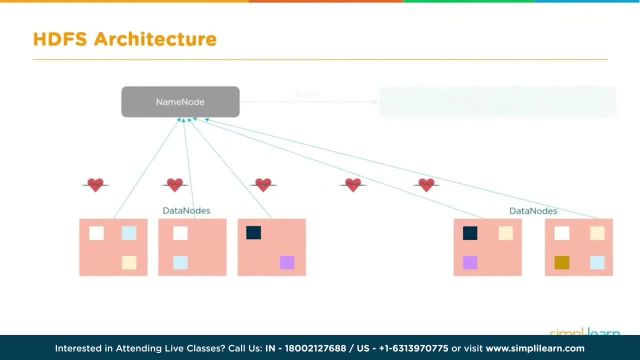 and you could also have a Spark node on there. Spark's a different architecture And these are each daemons that are running on these computers. That's why you refer to them as nodes and not just always as servers and machines. So even though I use them interchangeable- 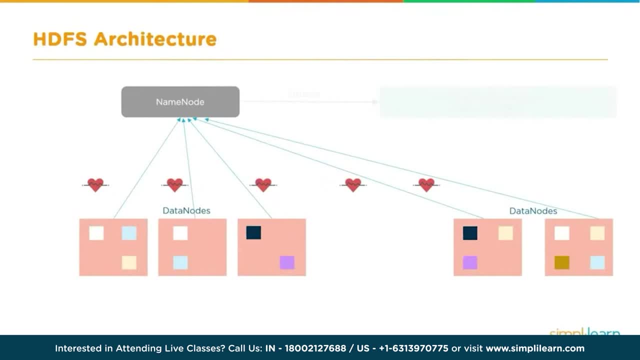 be aware that these nodes you can even have virtual machines. if you're testing something out, It doesn't make sense to have ten virtual nodes on one machine and deploy it, because you might as well just run your code on the machine, And so we have our heartbeat going on here. 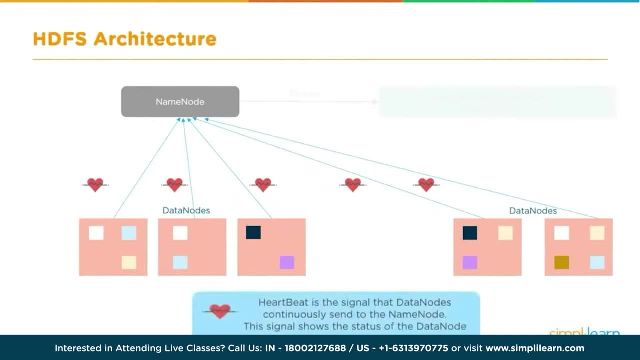 And the heartbeat is a signal that data nodes continuously send to the name nodes. This signal shows the status of the data node, So there's a continual pulse going up and saying: hey, I'm here, I'm ready for whatever instructions or data you want to send me. 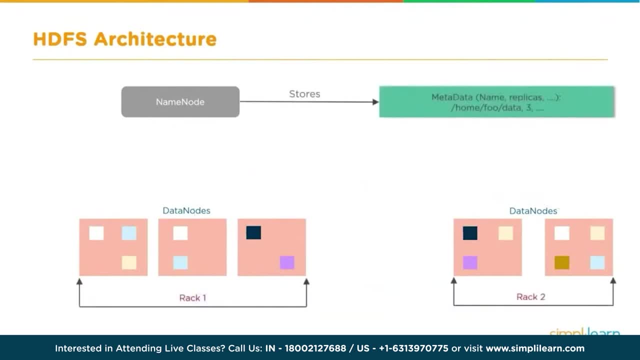 And you can see here we've divided up into rack one and rack two and our different data nodes, And it also has the replications. We talked about how to replicate data and it replicates it in three different locations And then we have a client machine. 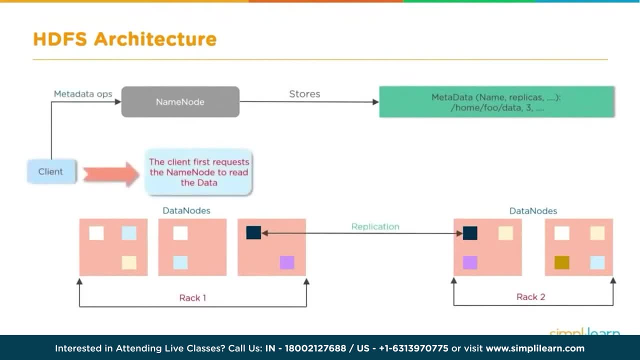 And the client first requests the name node to read the data. Now, if you're not familiar with the client machine, the client is you, the programmer, The client is. you've logged in external to this Hadoop file system and you're sending it instructions. 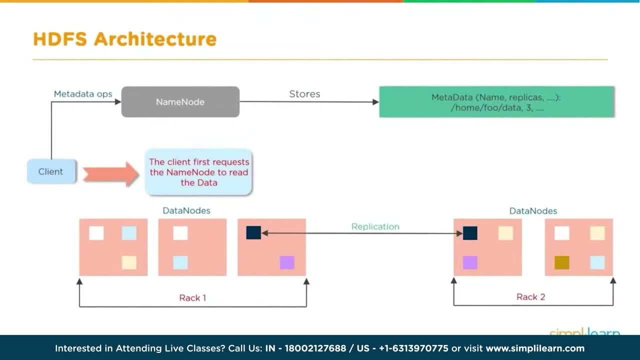 And so the client, whatever instructions or script you're sending- first requests the name node to read the data. The name node allows the client to read the requested data from the data nodes. The data is read from the data nodes and sent to the client. 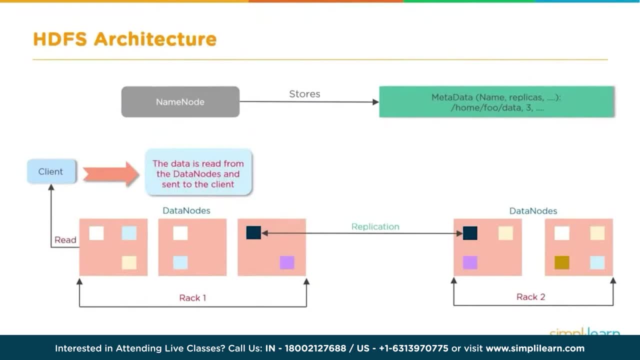 And so you can see here that basically the name node connects the client up and says: here, here's the data stream, And now you have the query that you sent out returning the data you asked for. And then of course it goes and finishes it and says: 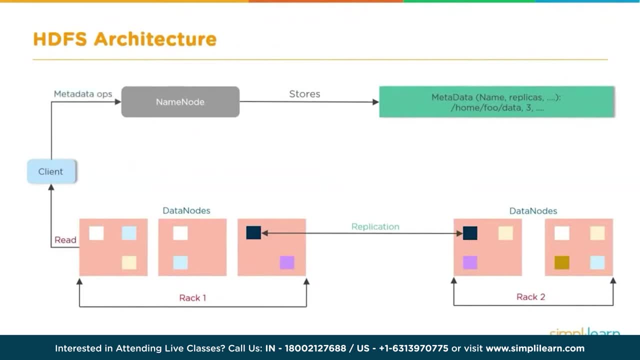 oh, metadata operations, And it goes in there and finalizes your request. The other thing the name node does as you're sending your information, because the client sends the information in there- is your block operations. So your block operations performs creation of data. 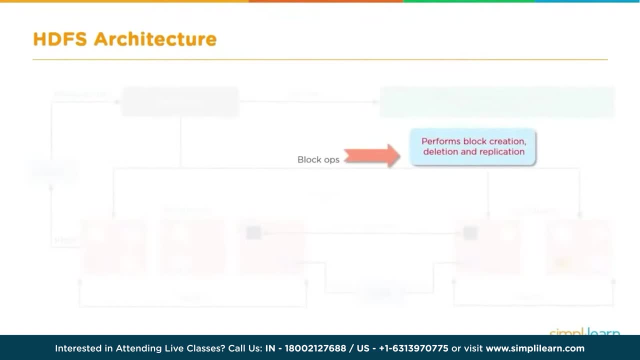 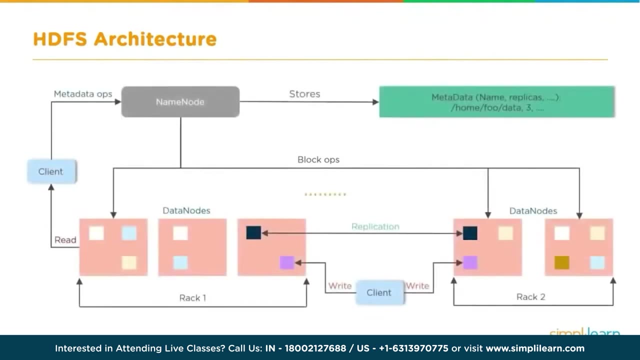 So you're going to create new files and folders, You're going to delete the folders, And also it covers the replication of the folders which goes on in the background, And so we can see here that we have a nice full picture. You can see where the client machine comes in. 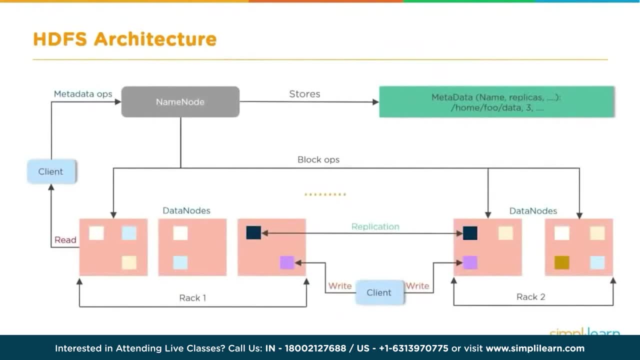 It queues the metadata, The metadata goes into, it stores the metadata And then it goes into block operations And maybe you're sending the data to the Hadoop file system. Maybe you're querying, Maybe you're asking it to delete. If you're sending data in there, it then does the replication on there. 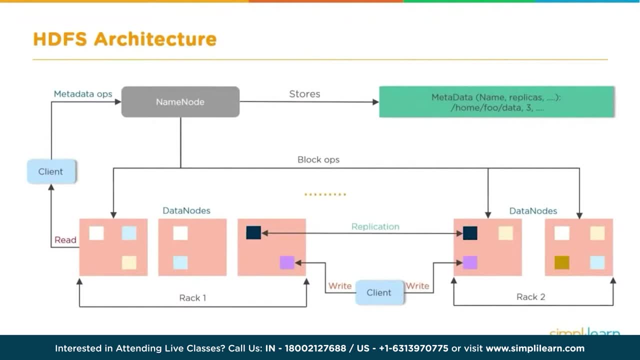 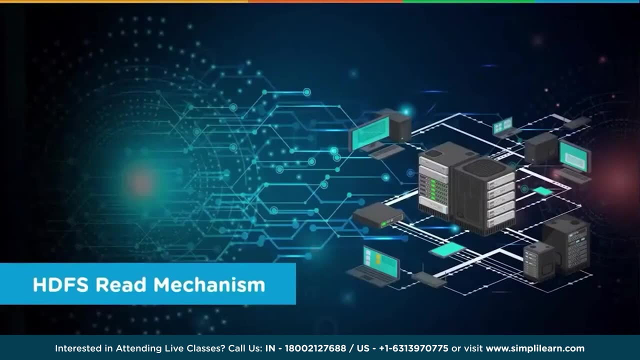 It goes back. so you have your data client, which is writing the data into the data node and, of course, replicating it, And that's all part of the block operations. And so let's talk a little bit about read mechanisms in the Hadoop file system. 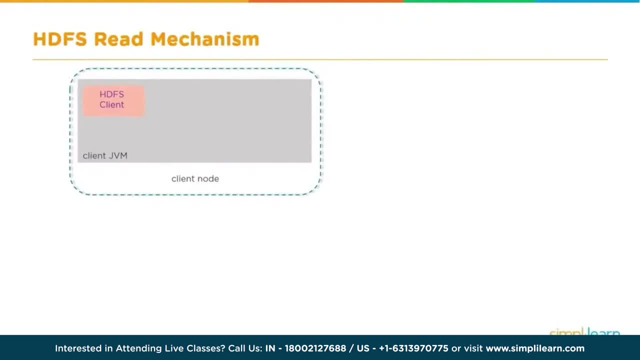 The Hadoop file system read mechanism. We have our Hadoop file system client- That's you- on your computer, And the client JVM on the client node, And so we have our client JVM or the Java virtual machine that it's going through. 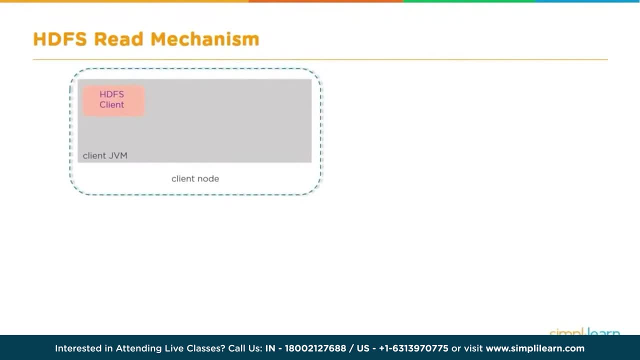 And then your client node And we're zooming in on the read mechanism. So we're looking at this picture here. As you can guess, your client is reading the data And I also have another client down here writing data. We're going to look a little closer at that. 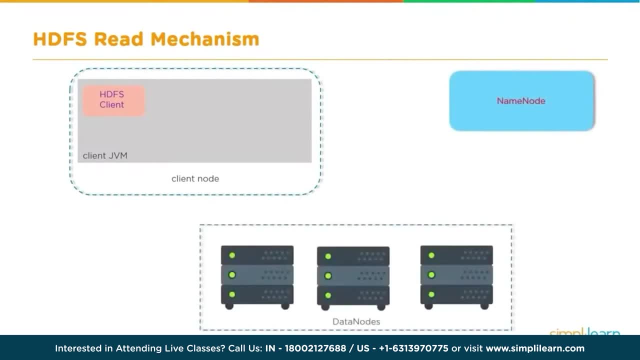 And so we have our name node up here, We have our racks of your data nodes and your racks of computers down here, And so our client. the first thing it does is it opens a connection up with the distributed file system to the HDFS. 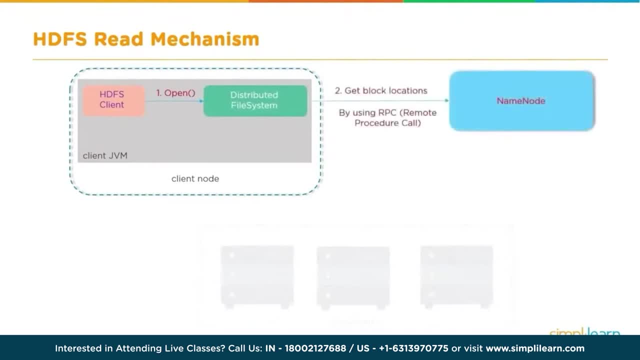 And it goes: hey, can I get the block locations? And so it goes by using the RPC remote procedure, call it, gets those locations And the name node first checks if the client is authorized to access the requested file And if yes, it then provides a block location and a token to the client. 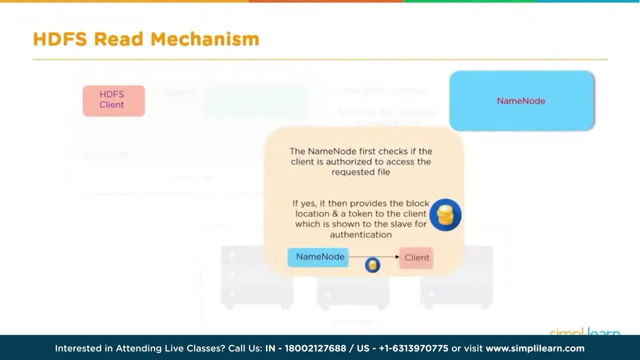 which is shown to the slave for authentication. So here's the name node. It tells the client: hey, here's the token, The client's going to come in and get this information from you. And it tells the client: oh hey, here's where the information is. 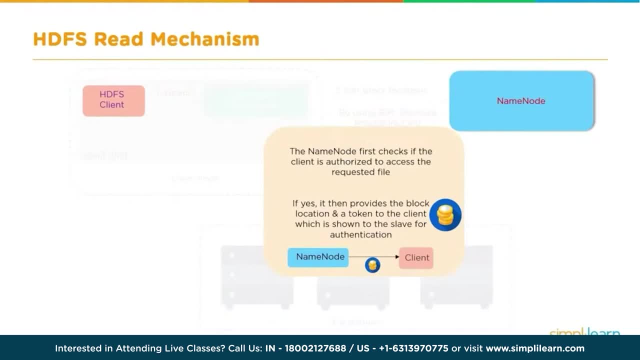 So this is what it's telling your script. you sent to query your data whether you're writing your script in one of the many setups that you have available through the Hadoop file system, or a connection through your code, And so you have your client machine at this point. then reads: 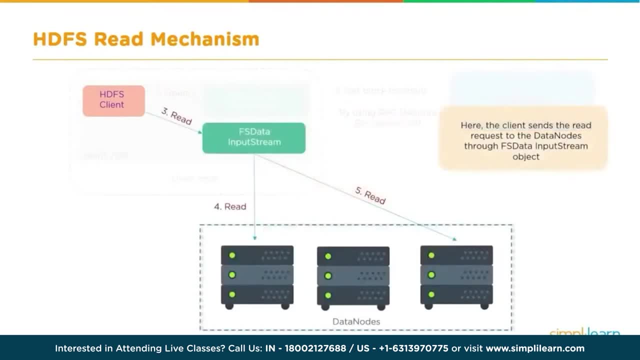 So your FS data input stream comes through and you have, and you can see right here, we did one and two, which is verify who you are and give you all the information you need. Then three, you're going to read it from the input stream. 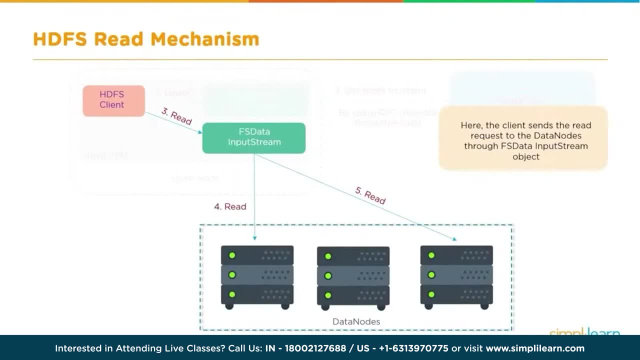 And then the input stream is going to grab it from the different nodes where it's at, And it'll supply the tokens to those machines saying, hey, this client needs this data. Here's a token for that. We're good to go. 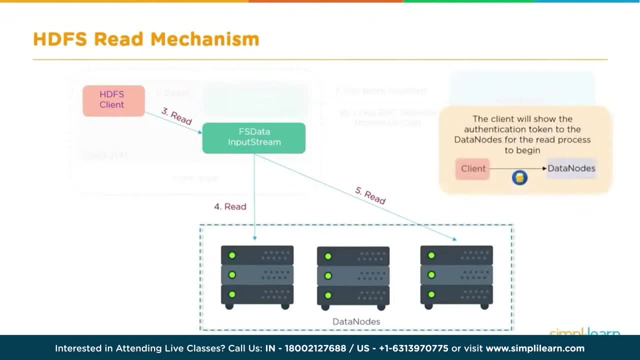 Let me have the data. The client will show the authentication token to the data nodes for the read process to begin. So after reaching the end of the data block, the connection is closed And we can see here where we've gone through the different steps. 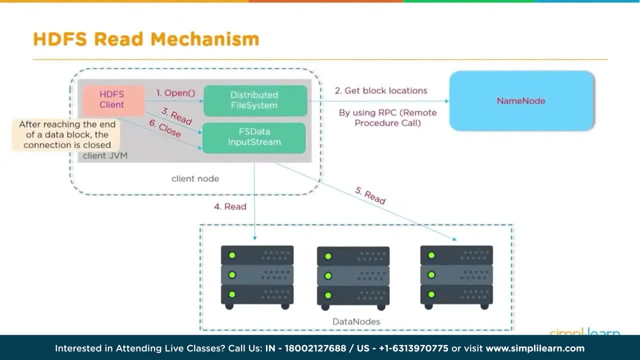 get block locations. We have step one. you open up your connection, You get the block locations by using the RPC, Then you actively go through the FS data input stream to grab all those different data, Brings it back into the client And then, once it's done, it closes down that connection. 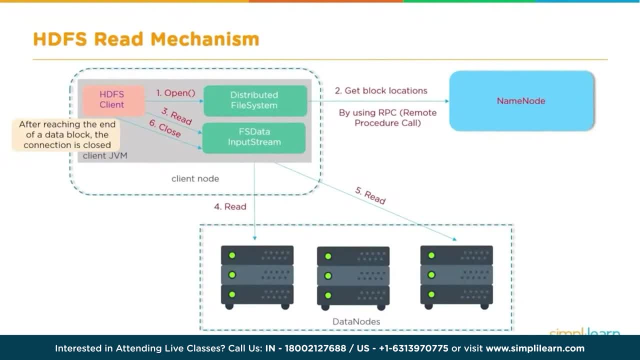 And then once the client- or in this case the programmer- you know managers- come in and PIG script, you can do that. There's an actual coding in Hadoop. We're pulling data called PIG or HIVE. Once you get that data back, we close the connection. 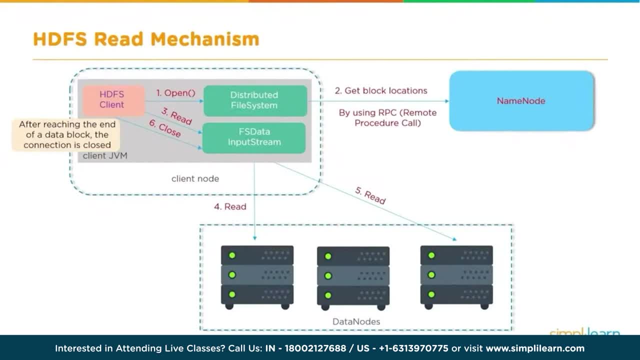 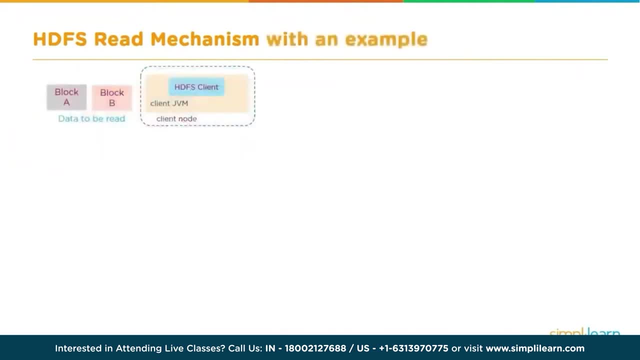 delete all those randomly huge series of tokens so they can't be used anymore, And then it's done with that query And we can go ahead and zoom in just a little bit more here And let's look at this even a little closer. 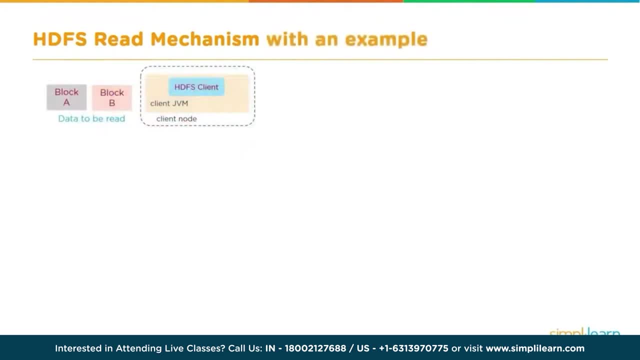 Here's our Hadoop file system client and our client JVM, our Java virtual machine, on the client node, And we have the data to be read- block A, block B- And so we request to read block A and B and it goes into the name node. 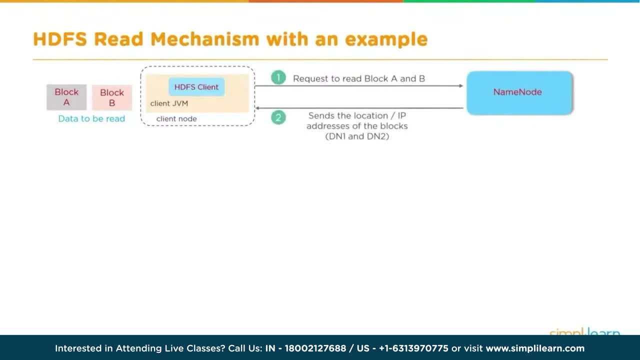 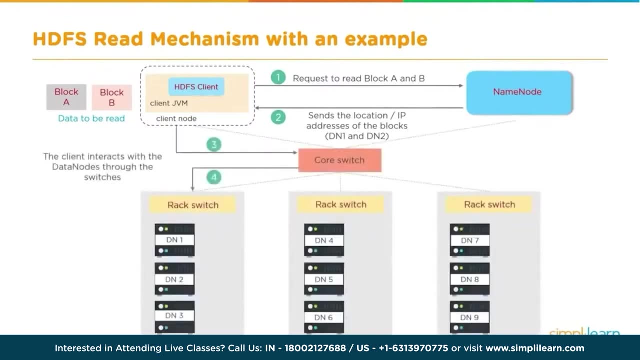 Two. then it sends the location- in this case of IP addresses of the blocks for the DN1 and DN2, where those blocks are stored. Then the client interacts with the data nodes through the switches, And so you have here the core switch. 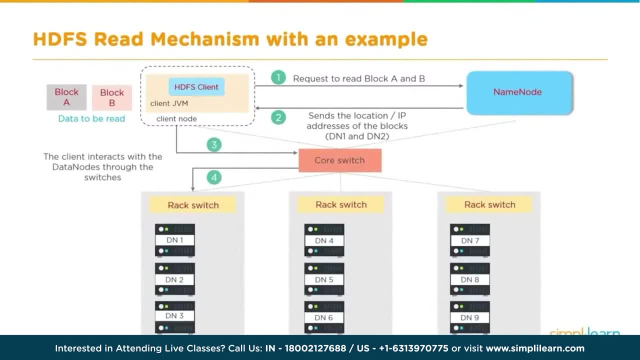 So your client node comes in Three and it goes to the core switch And that then goes to rack switch one, rack switch two and rack switch three. Now, if you're looking at this, you'll automatically see a point of failure. 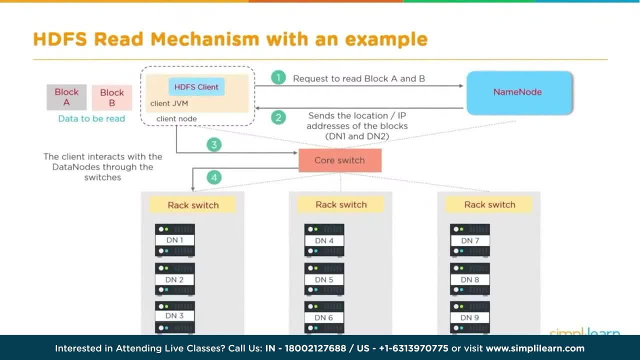 in the core switch And certainly you want a high-end switch mechanism for your core switch. You want to use enterprise hardware for that. And then when you get to the racks, that's all commodity, all your rack switches. So if one of those goes down you don't care as much. 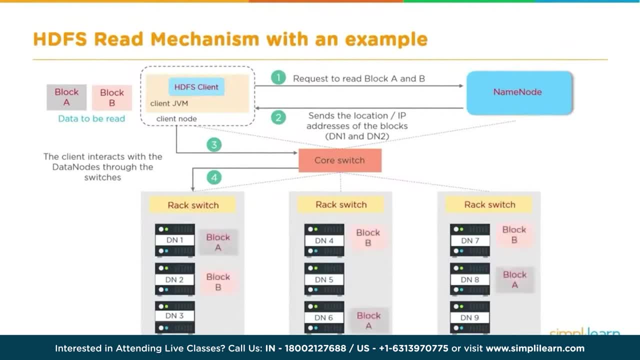 You just have to get in there and swap it in and out really quick And you can see here we have block A which is replicated three times, And so is block B, And it'll pull from there. So we come in here. 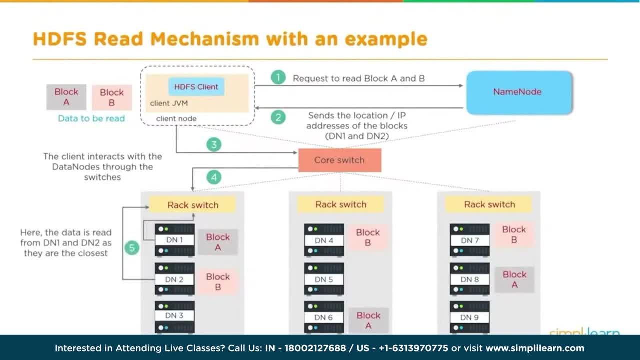 and here the data is read from the DN1 and DN2 as they are the closest to each other, And so you can see here that it's not going to read from two different racks, It's going to read from one rack, whatever the closest setup is for that query. 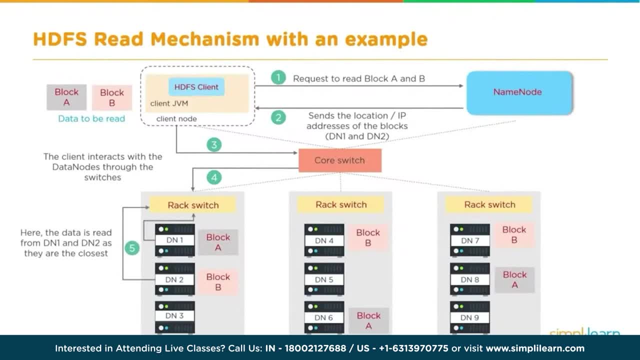 The reason for this is if you have 10 other queries going on, you want this one to pull all the data through one setup and it minimizes that traffic. So the reason for this is it responds from the data nodes to the client that read: the operation was successful. 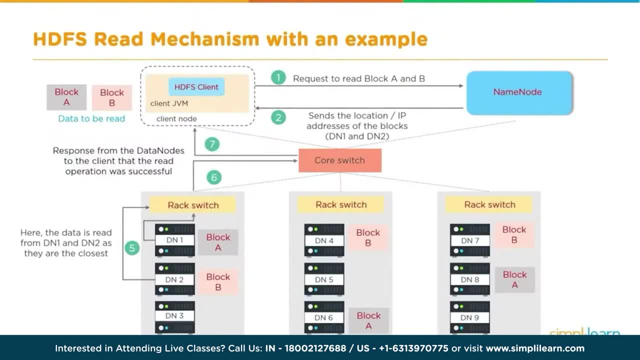 It says: ah, we've read the data, We're successful, which is always good. We like to be successful. I don't know about you, I like to be successful. So if we're looking at the read mechanism, let's go ahead and zoom in. 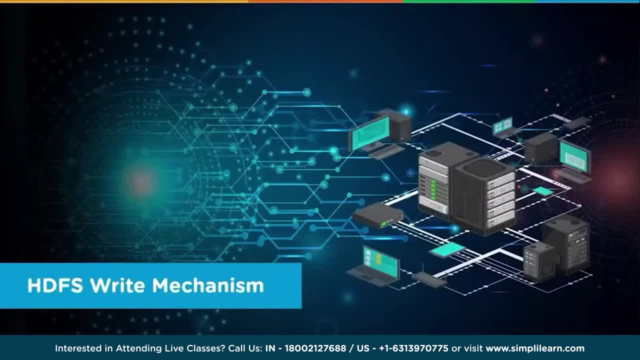 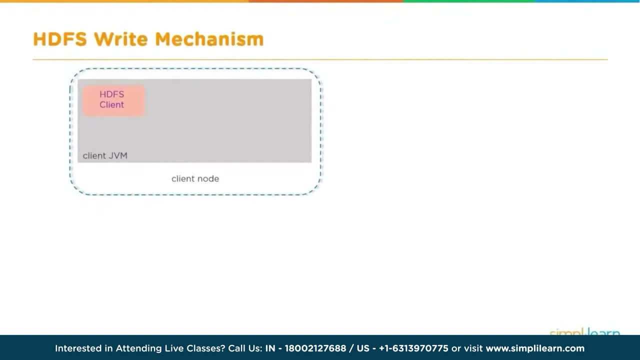 and look at the write mechanism for the Hadoop file system, So our HDFS write mechanism. And so when we have the HDFS write mechanism, here's our client machine. This is again the programmer on their end computer And it's going through the client Java machine. 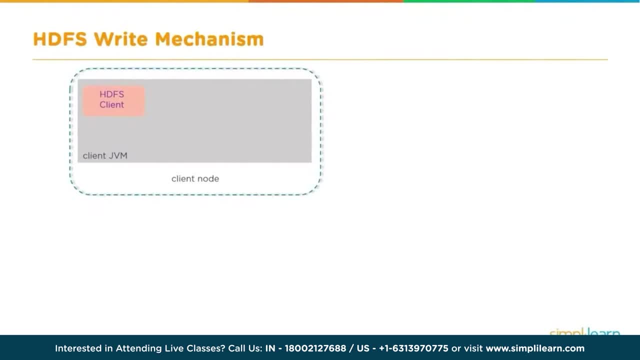 or Java virtual machine, the JVM, And this is all occurring on the client machine. So we have our client node, somebody's office, or maybe it's on the local server for the office, So we have our name node, We have data nodes. 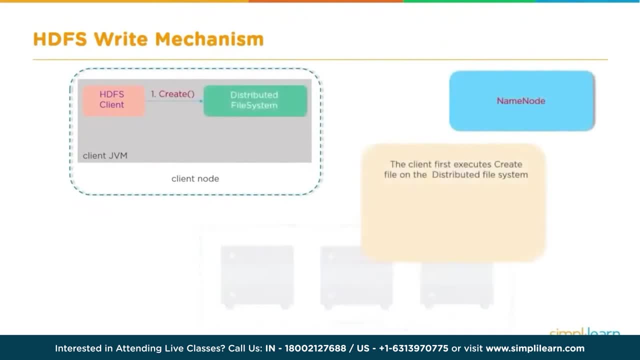 And we have the distributed file system. So the client first executes: create file on the distributed file system. It says: hey, I'm going to create this file over here, And then it goes through the RPC call, just like our read did. 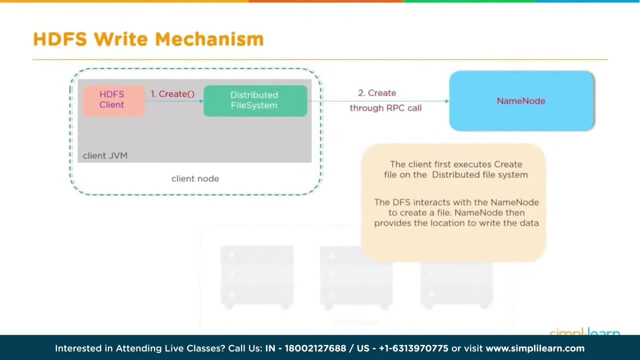 The client first executes create file on the distributed file system. Then the DFS interacts with the name node to create a file. Name node then provides a location to write the data, And so here we have our HDFS client and the FS data output stream. 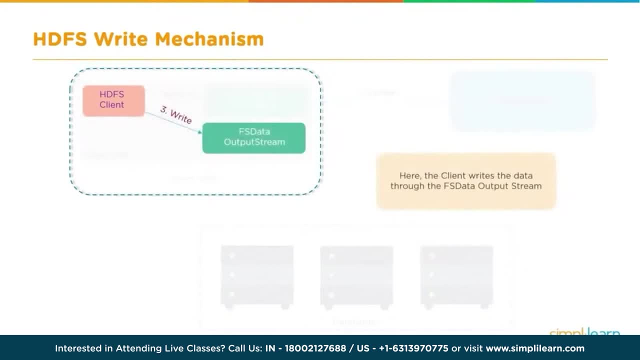 So this time, instead of the data going to the client, it's coming from the client, And so here the client writes the data through the FS data output stream. Keep in mind that this output stream, the client, could be a streaming code. 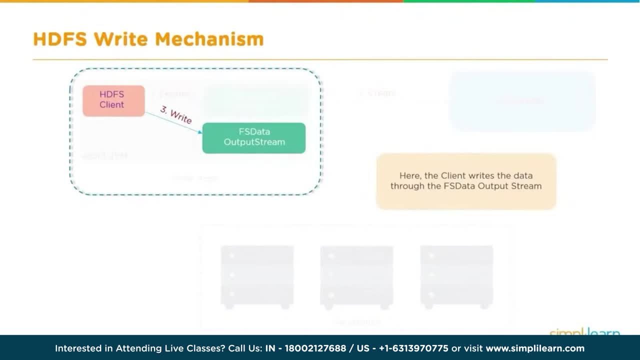 It could be. I mean, you know I always refer to the client as just being this computer that your programmer is writing on. It could be you have your SQL server there where your data is that's current with all your current cells, And it's archiving all that information. 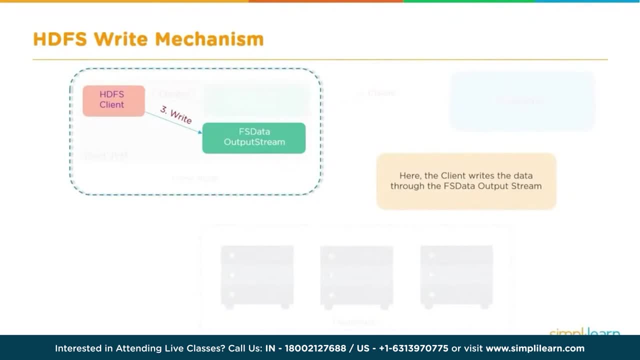 through a scoop, one of the tools in the Hadoop file system. It could be streaming data, It could be a connection to the stock servers And you're pulling stock data down from those servers at a regular time And that's all controlled. 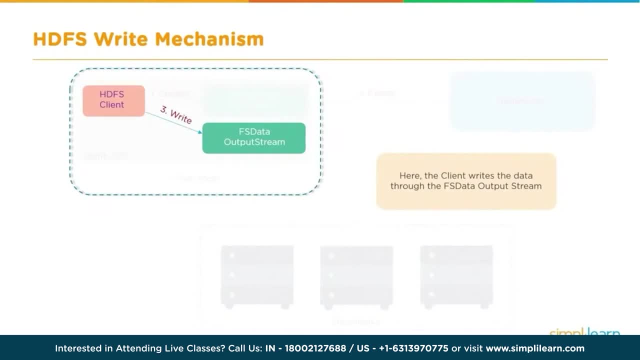 You can actually set that code up to be controlled in many of the different features in the Hadoop file system and some of the different resources you have that sit on top of it. So here the client writes the data through the FS data output stream. 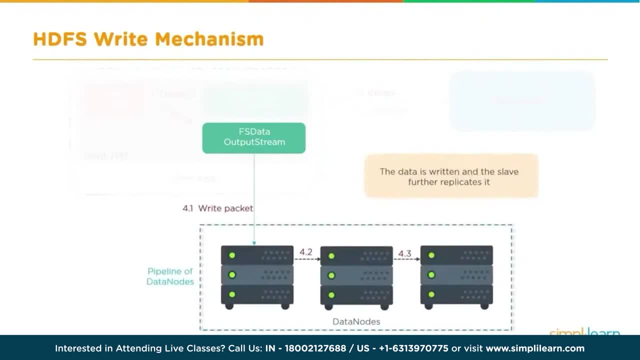 And the FS data output stream, as you can see, goes into write packet. So it takes, divides it up into packets- 128 megabytes- And the data is written and the slave further replicates it. So here's our data coming in. 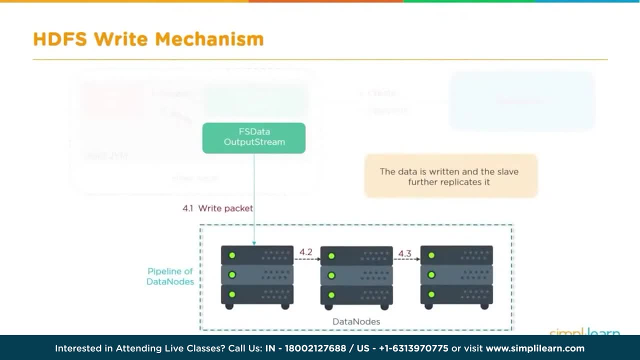 And then, if you remember correctly, that's part of the FS data setup is it tells it where to replicate it out. But the data node itself is like: oh, hey, okay, I've got the data coming in and it's also given the tokens. 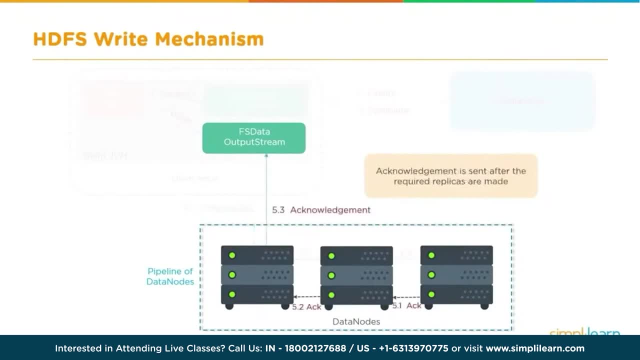 of where to send the replications to, And then acknowledgement is sent after the required replicas are made. So then that goes back up saying hey, successful, I've written data, made three replications on this, As far as I know. 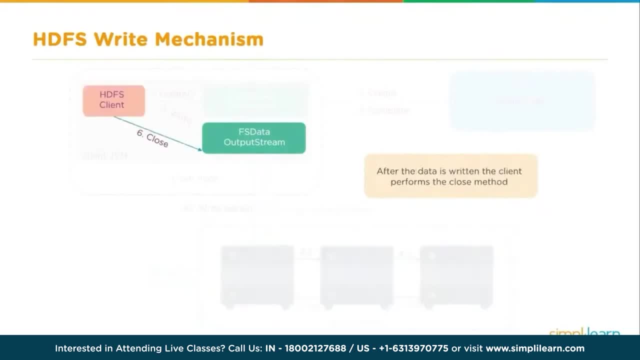 that's what we're doing, And then the client goes back and says, okay, I'm done, Here's the end of the data, We're finished. And after the data is written, the client performs a close method And we can see here: 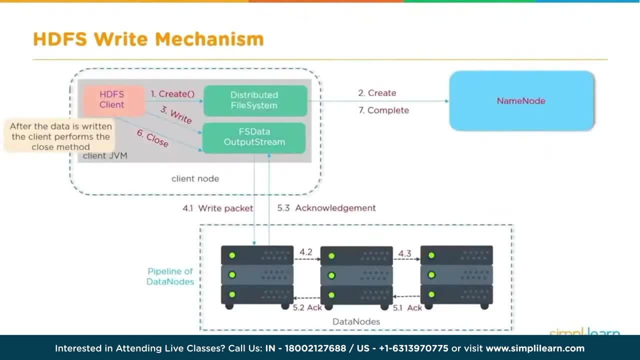 just a quick reshape. We go in there just like we did with the read. We create the connection. This creates a name node which lets it know what's going on. Step two, step three. that also includes the tokens and everything. 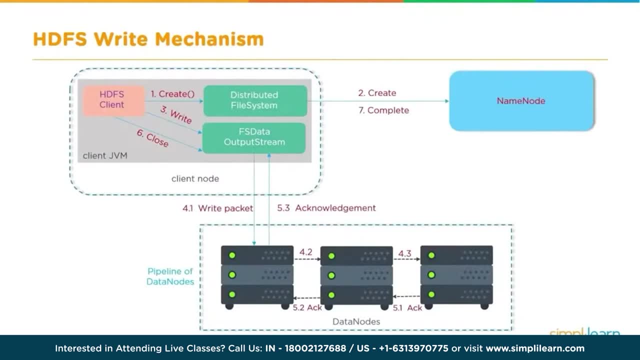 And then we go into step three, which lets it know what's going on: Step four, step five, step six, step seven, step eight, step nine and step 10.. And then we go into step three, where we're now writing through. 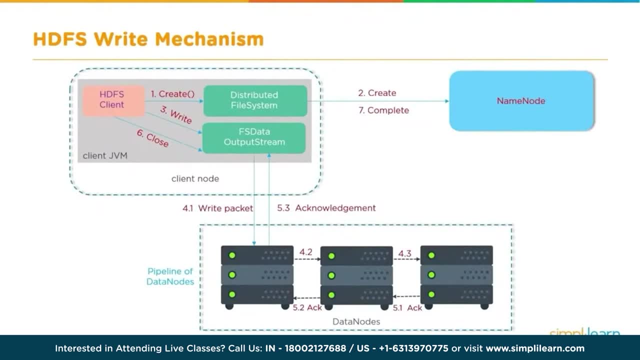 the FS data output stream And that sorts it out into whatever data node it's going to go to and which also tells it how to replicate it, So that data node then sends it to other data nodes. so we have a replication And, of course, 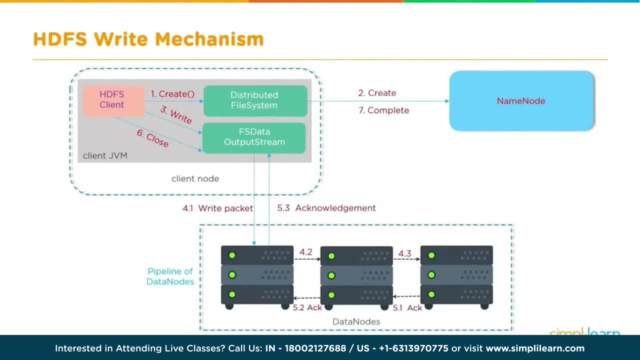 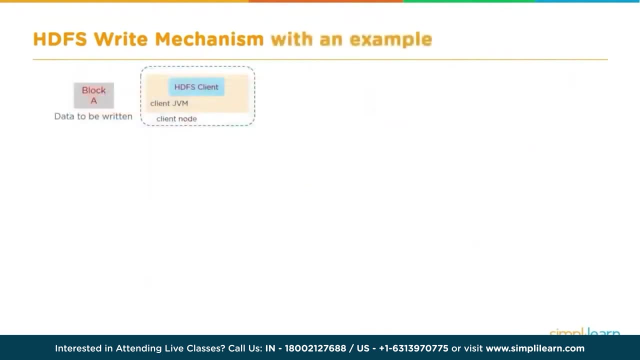 you finalize it and close everything up, marks it, complete to the name node and it deletes all those magical tokens in the background so that they can't be reused. And we can go ahead and just do this with an example, the same setup. 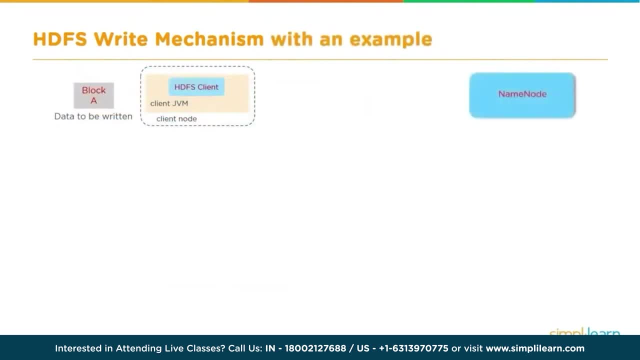 And whether you're doing a read or a write, they're very similar. As we come in here from our client node and you can see right here we're actually depicting these as the actual rack and the switches going on And so, as the data comes in, 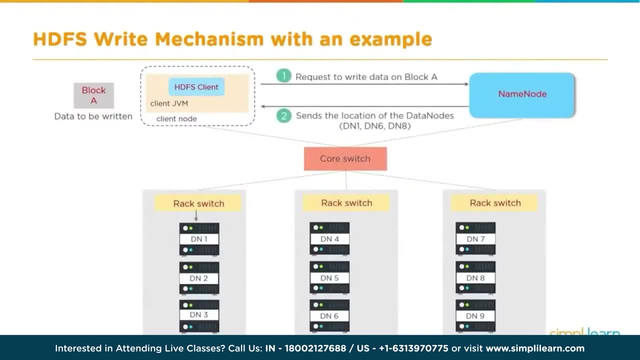 you have your request. like we saw earlier, It sends a location of the data nodes and this actually turns your IP addresses, your dynamic node connections. They come back to your client, your HDFS client, and at that point, with the tokens, 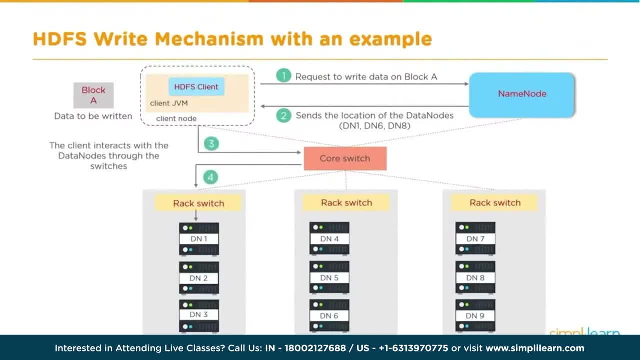 it then goes into the core switch and the core switch says, hey, here it goes. The client interacts with the data nodes through the switches And you can see here where you're writing in block A. replication of block A and a second replication. 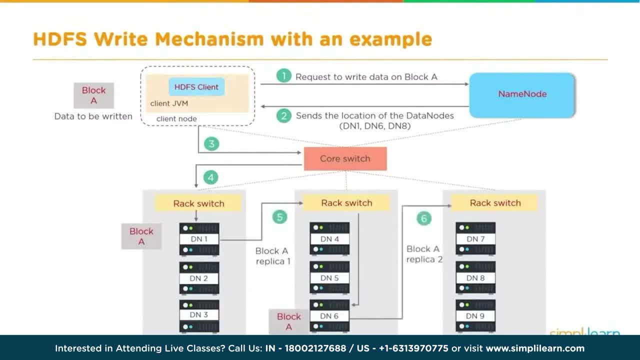 of block A on the second server. So block A gets replicated on the second server and the third server. At this point you now have three replications of block A and it comes back and says it acknowledges. it says hey, we're done. 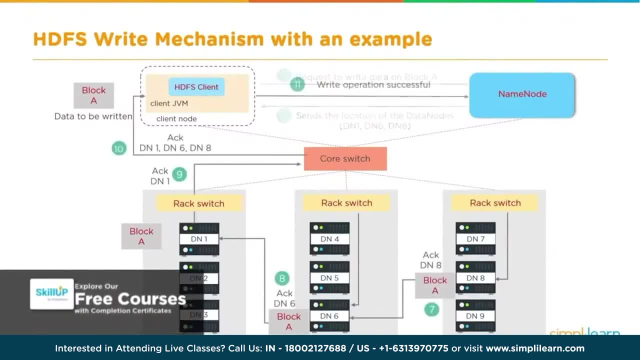 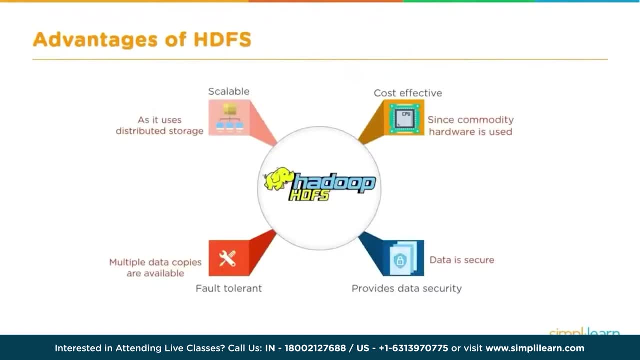 And that goes back into your Hadoop file system. to the client It says, okay, we're done And finally the success written to the name node and it just closes everything down. A quick recap of the Hadoop file system and the advantages. 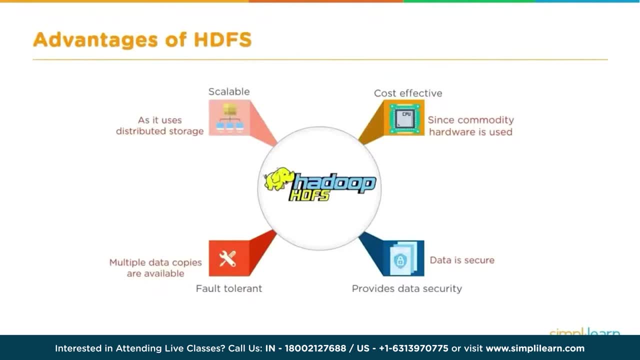 of Hadoop. So the first one is probably one of the all of these are huge One you have multiple data copies are available, So it's very fault tolerant. Whole racks can go down, Switches can go down, Even your main name, node. 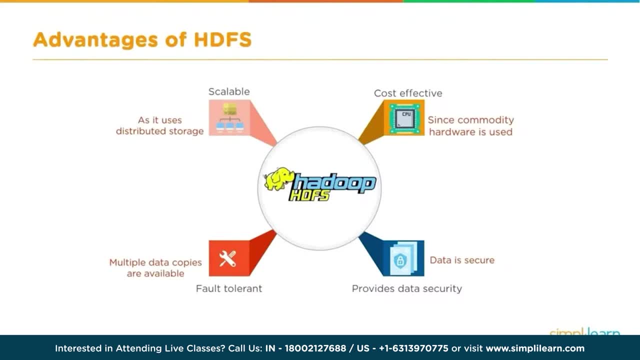 can go down if you have a secondary name node. Something we didn't talk too much about is how scalable it is, As it uses distributed storage. you run into there and you're: oh my gosh, I'm out of space or I need to do. 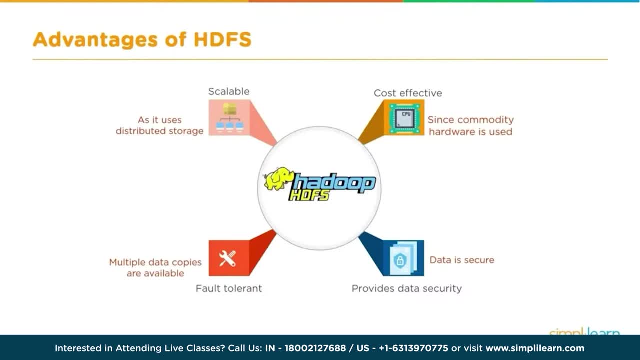 some heavier processing. Let me just add another rack of computers So you can scale it up very quickly. It could be if you bought a server you would have to pay a lot of money to get that. the Craig computer. Remember the big Craig? 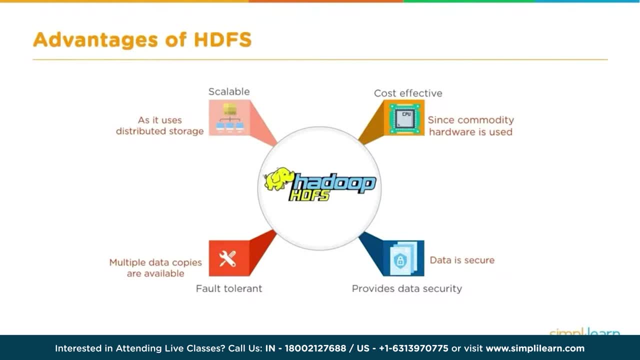 computers coming out. The Craig computer runs two million a year just the maintenance to liquid cool it. That's very expensive compared to just adding more racks of computer and extending your data center. So it's very cost effective Since commodity hardware is used. 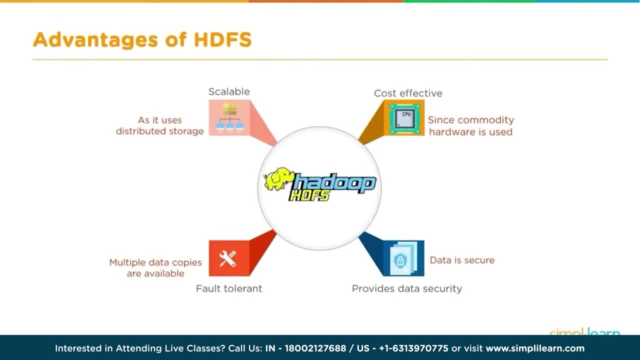 we're talking cheap knockoff computers. You still need your high end enterprise for the name node, But the rest of them, literally it is a tenth of the cost of storage and storing data on more traditional high end computers, And then the data is secure. 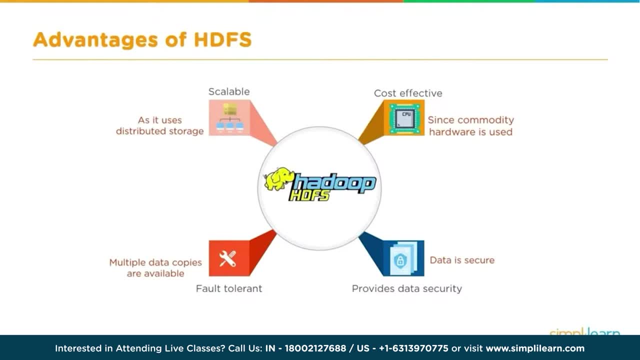 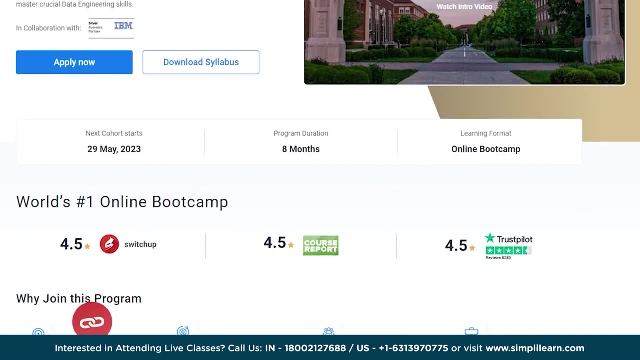 So it has a very high end data security and provides data security for your data. Hello learners, Simplion brings you a post graduate program in data engineering, developed in partnership with Purdue University and IBM. To learn more about this course, you can find the course. 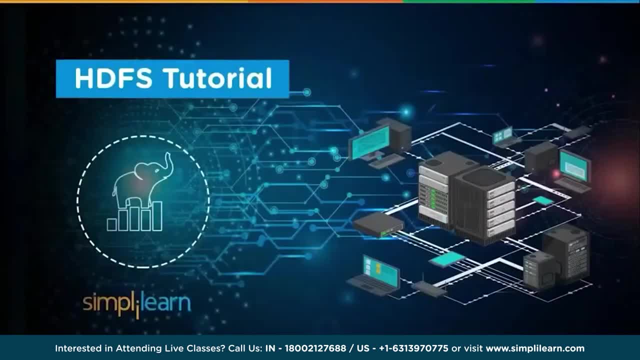 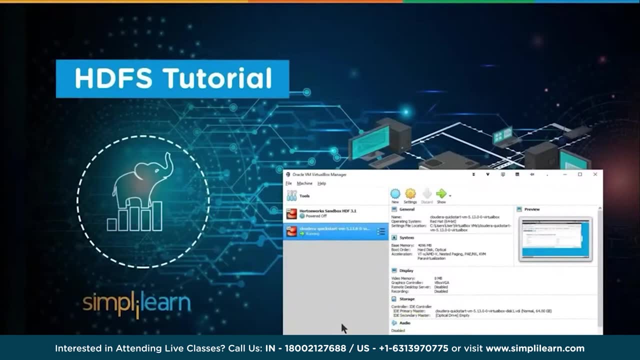 link in the description box below. So all theory and no play doesn't make for much fun. So let's go ahead and show you what it looks like, as far as some of the dimensions, when you're getting into pulling data or putting data into the Hadoop file system. 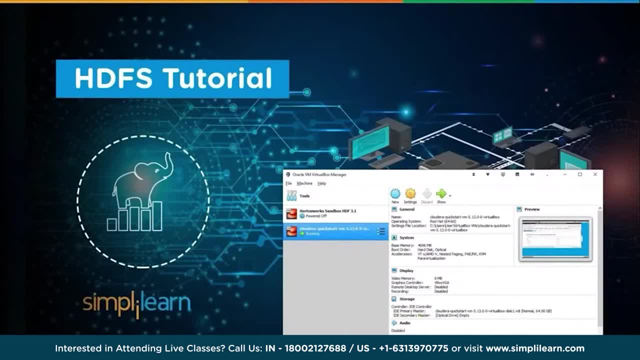 And you can see here I have Oracle Virtual Machine Virtual Box Manager. I have a couple of different things loaded on there. Cloudera is one of them, So we should probably explain some of these things if you're new to virtual machines. The Oracle Virtual Box. 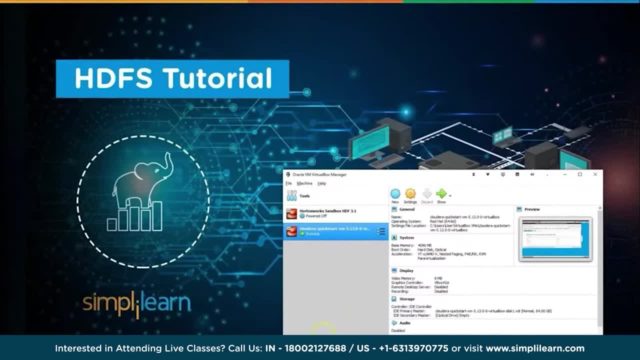 allows you to spin up a machine as if it is a separate computer. So in this case this is running, I believe, a CentOS, a Linux, and it creates like a box on my computer. So the CentOS is running on my machine. 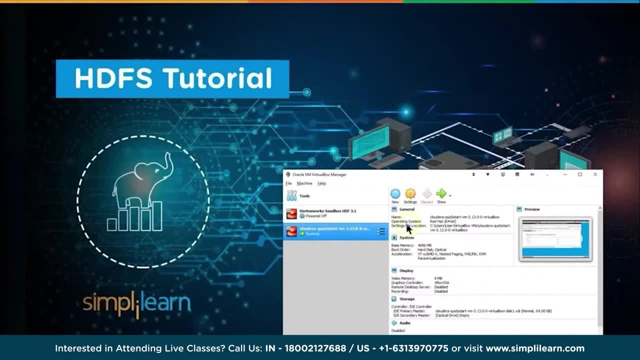 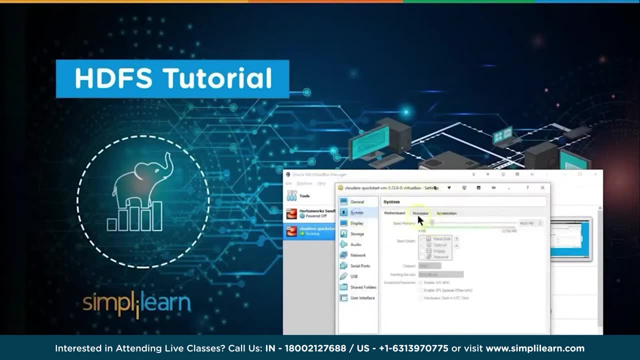 while I'm running my Windows 10.. This happens to be a Windows 10 computer, And then underneath here I can actually go under. let me just open up the general. It might be hard to see there And you can see I can. 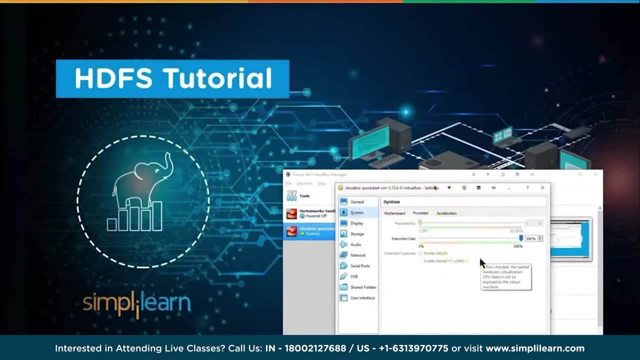 actually go down to System Processor. I happen to be on an 8-core. It has 16 dedicated threads, registers of 16 CPUs but 8 cores, And I've only designated this for one CPU, So it's only going. 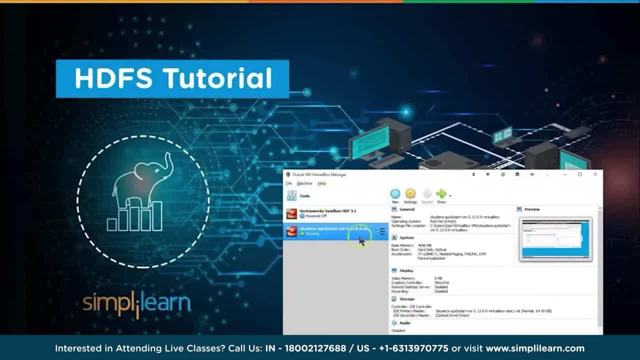 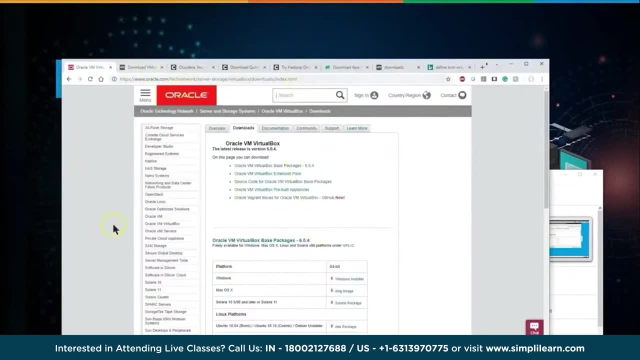 to use one of my dedicated threads on my computer And this, the Oracle Virtual Machine, is open source And you can see right here we're on the Oracle wwworaclecom. I usually just do a search for downloading VirtualBox, If you search for. 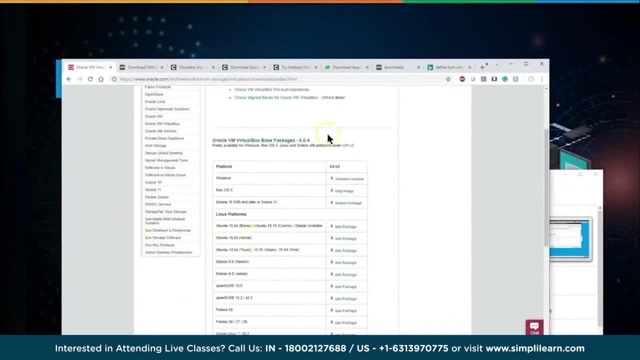 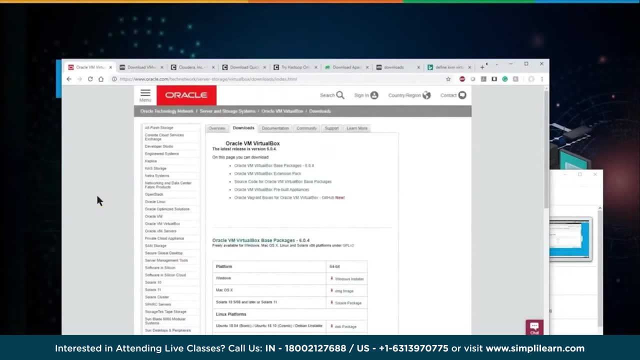 VirtualBox, all one word. it will come up with this page and then you can download it for whatever operating system you're working with. There certainly are a number of different options, And let me go ahead and point those out. if you're setting this up, 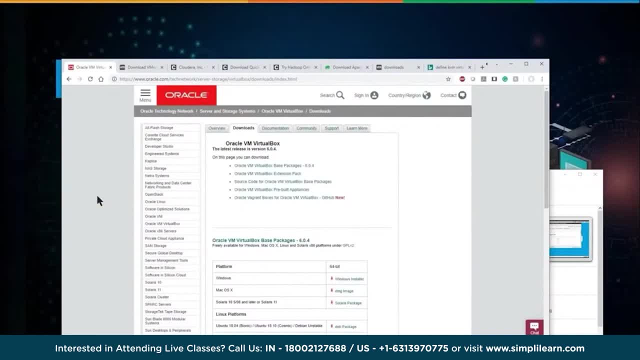 as a for demoing for yourself. The first thing to note: for doing a VirtualBox and doing it, for doing a Cloudera or Horton setup on that VirtualBox, for doing the Hadoop system, to try it out, you need a minimum of 12 gigabytes. 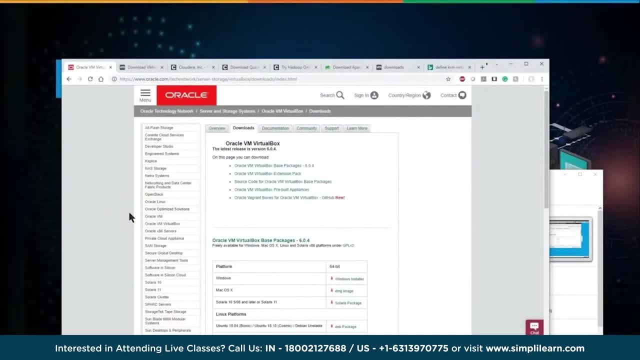 It cannot be a Windows 10 home edition, because you'll have problems with your virtual setup And sometimes you have to go turn on the virtual settings so it knows it's in there. So if you're on a home setup, there are other sources. 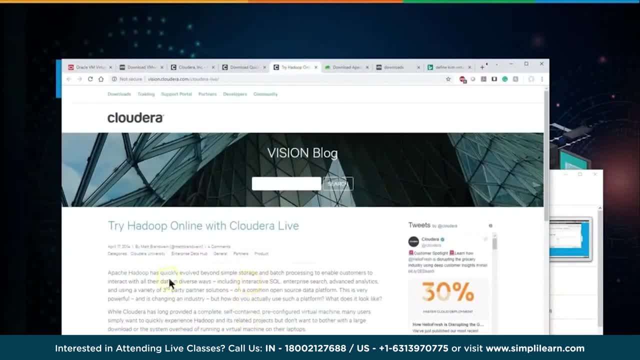 There's Cloudera and we'll talk a little bit about Cloudera here in just a second. But they have the Cloudera online live. We can go try the Cloudera setup. I've never used it, but Cloudera is. 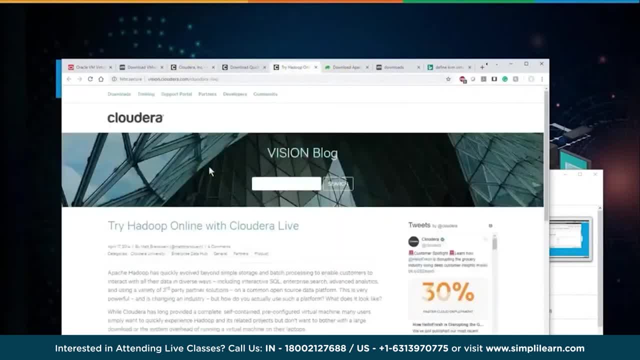 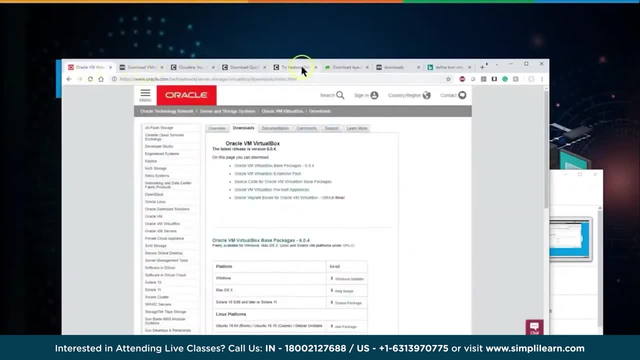 a pretty good company. Cloudera and Hortonworks are two of the common ones out there And we'll actually be running a Cloudera Hadoop cluster on our demo here. So you have Oracle Virtual Machine. You also have the option of doing it on. 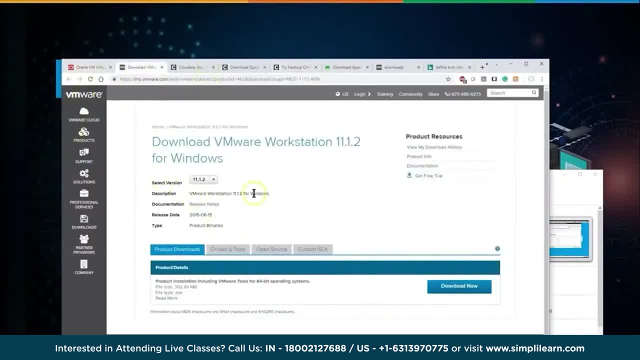 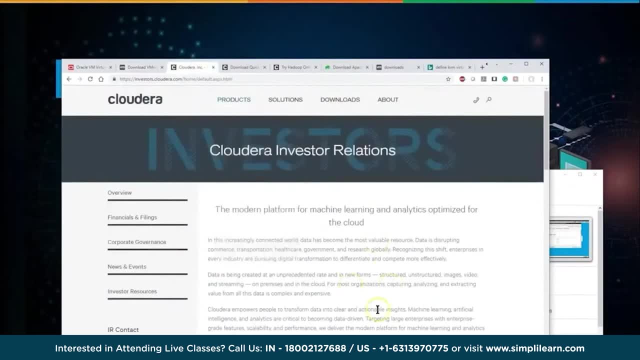 different VMware. That's another one like Virtual Machine. This is more of a paid service. There is a free setup for just doing it for yourself, which will work fine for this, And then in the Cloudera, like again, they have the new. 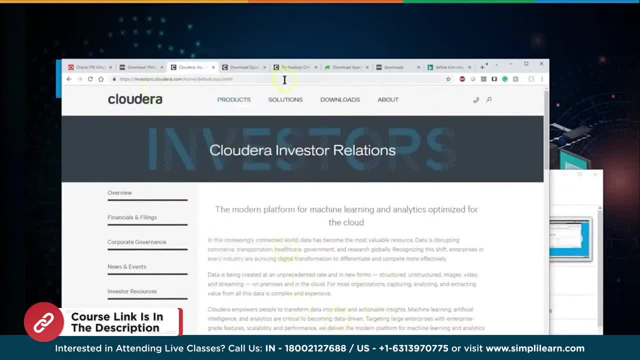 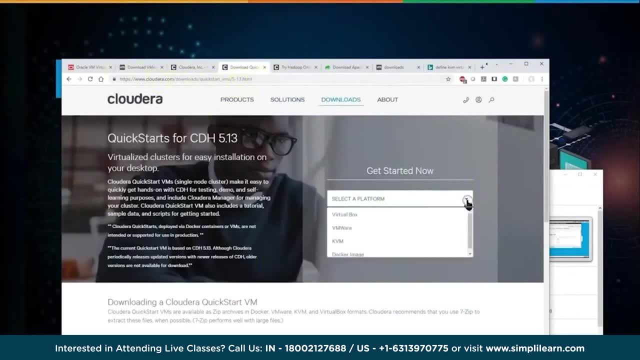 online setup where you can go in there to the online And for Cloudera you want to go underneath the Cloudera Quick Start. If you type in a search for Cloudera Quick Start, it'll bring you to this website and then you can select. 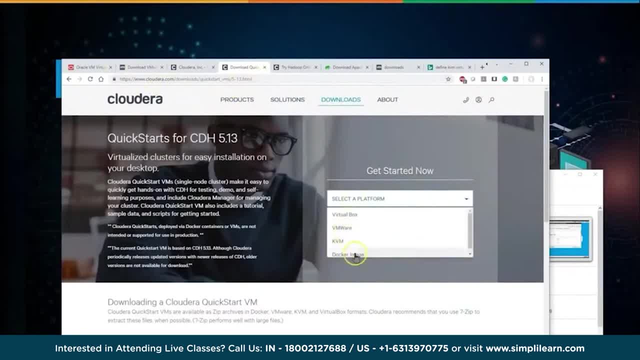 your platform. In this case, I did Virtual Box. There's VMware. we just talked about Docker. Docker is a very high-end virtual setup. Unless you already know it, you really don't want to mess with it. Then your KVM. 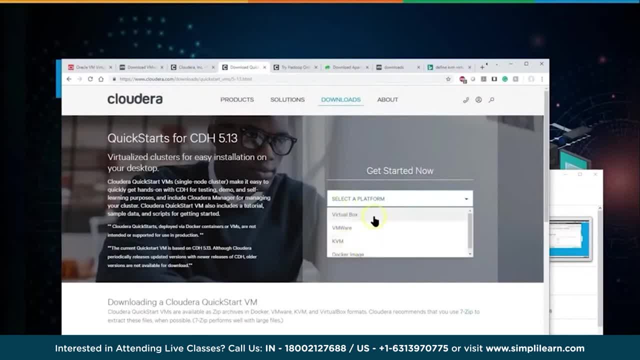 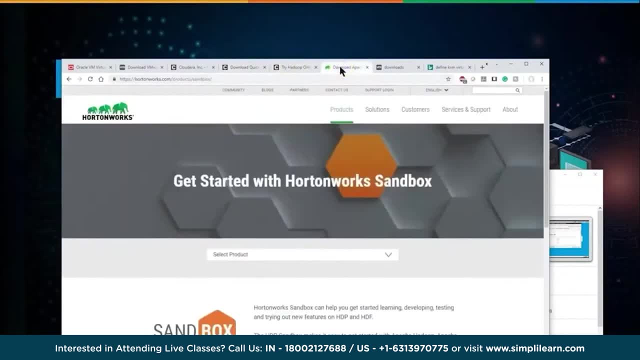 is if you're on a Linux computer, that sets up multiple systems on that computer. So the two you really want to use are usually the Virtual Box or do an online setup And you can see here with the download if you're going into the Horton version. 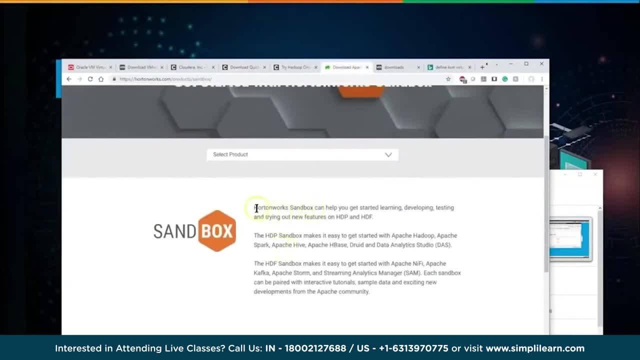 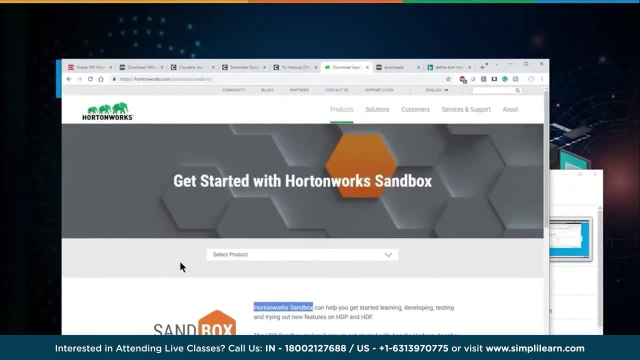 it's called Hortonworks and they call it Sandbox, So you'll see the term Hortonworks, Sandbox, And these are all test demos. You're not going to deploy a single node Hadoop systems. That would just be kind of ridiculous and defeat the whole purpose. 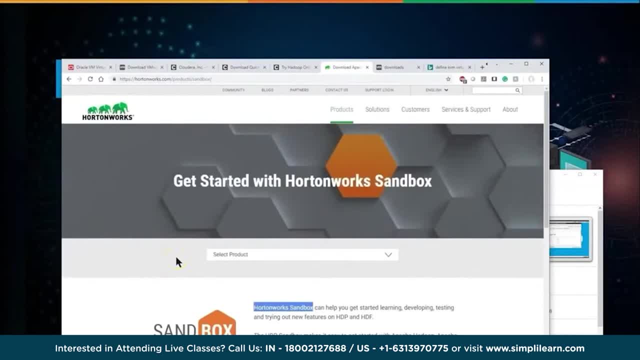 of having a Horton or having a Hadoop system if it's only installed on one computer in a virtual node. So a lot of different options If you're not on a professional Windows version or you don't have at least 12 gigabytes RAM. 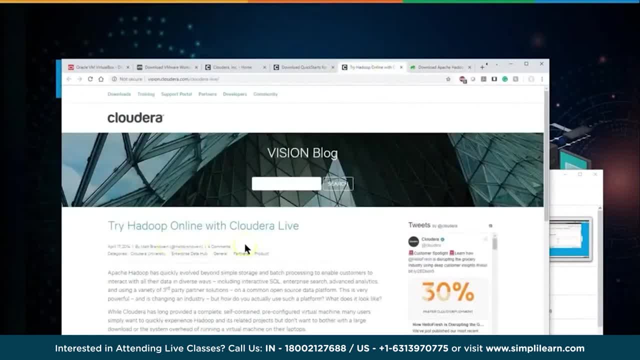 to run this. you'll want to try and see if you can find an online version And, of course, Simply Learn has our own labs. If you sign up for our classes, we set you up. I don't know what it is now. 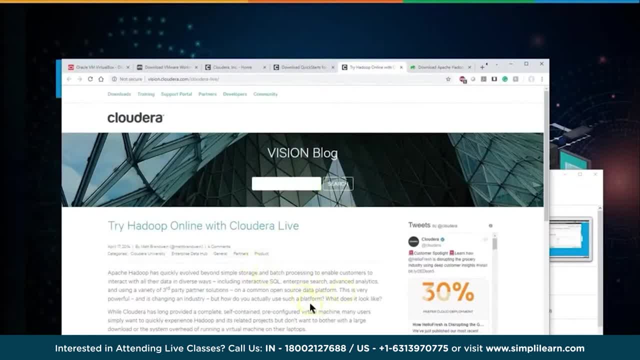 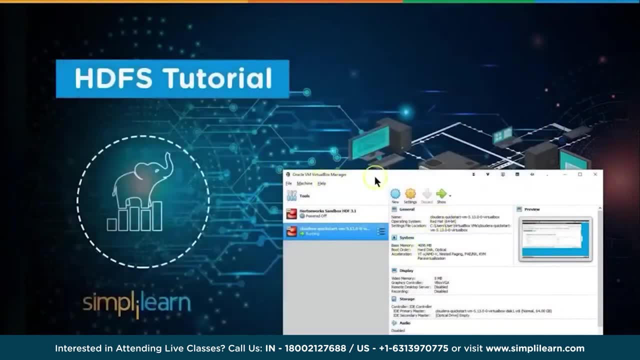 but last time I was in there was a five node setup so you could get around and see what's going on Whether you're studying for the admin side or for the programming side and script writing. And if I go into my Oracle Virtual Box and I go under my Cloudera. 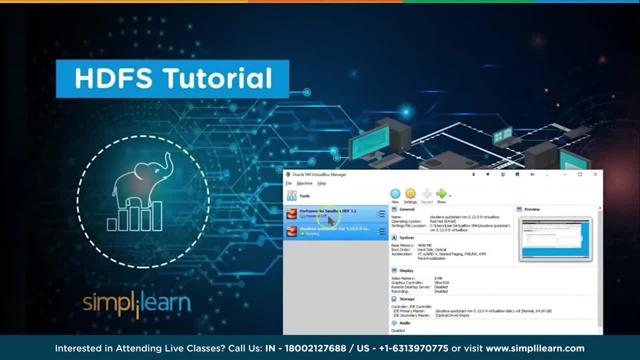 and I start this up, and each one has their own flavors. Horton uses just a login, So you log everything in through a local host, through your Internet Explorer or might use Chrome. Cloudera actually opens up a full interface, So you actually are. 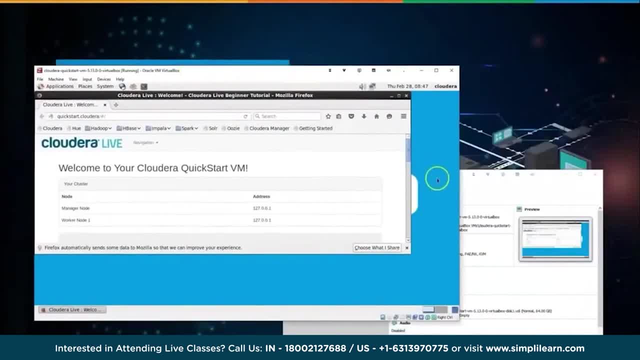 in that setup And you can see when I started it. let me go back here Once I downloaded this. this is a big download. by the way, I had to import the appliance in Virtual Box The first time I ran it. it takes a long time. 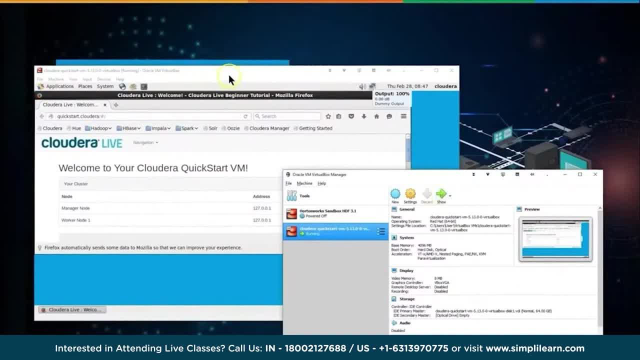 to configure the setup. And the second time it comes up pretty quick. And with the Cloudera Quick Start, again, this is a pretend single node. It opens up and you'll see that it actually has Firefox here. so here's my web browser. 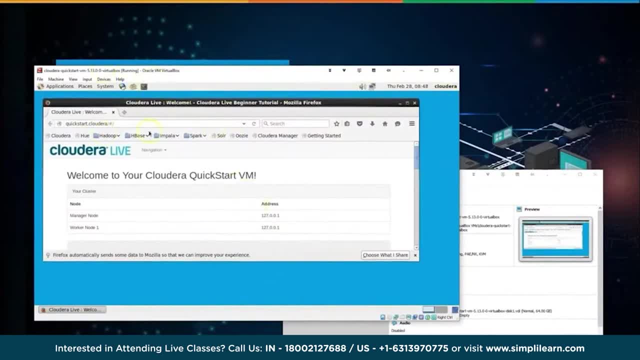 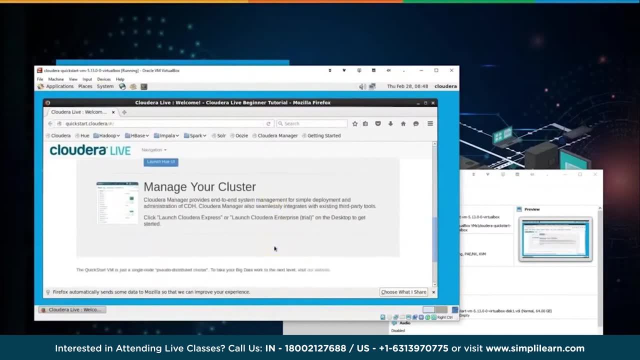 I don't have to go to local host. I'm actually already in the Quick Start for Cloudera And if we come down here, you can see getting started. I have some information: analyze your data, manage your cluster, your general information. 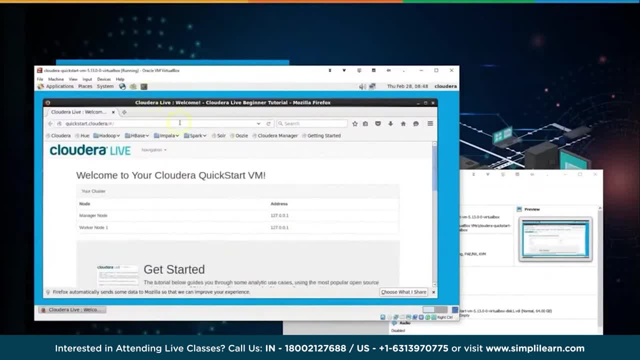 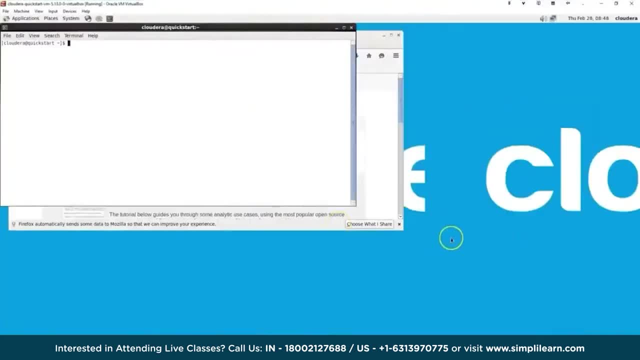 on there, And what I always want to start to do is to go ahead and open up a terminal window. So we'll open up a terminal, widen this a little bit. Let me just maximize this out here so you can see. So we are now. 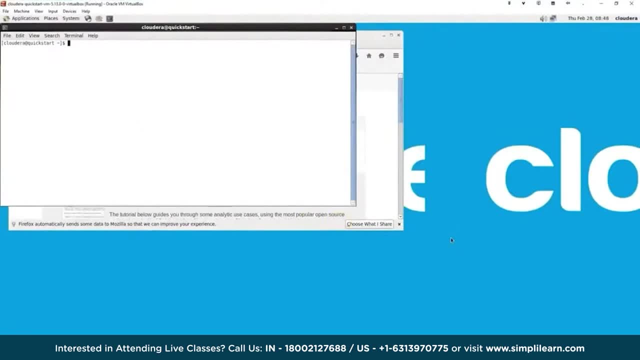 in a virtual machine. This virtual machine is CentOS Linux, So I'm on a Linux computer and so when I'm on this terminal window, this is your basic terminal. If I do list, you'll see documents Eclipse. These are the different. 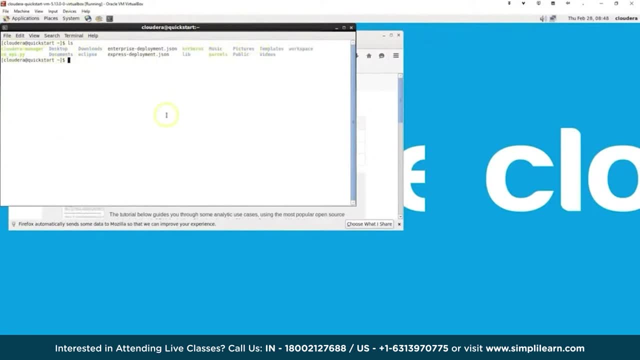 things that are installed with the Quick Start guide on the Linux system. So this is a Linux computer And then Hadoop is running on here. So now I have Hadoop single node, So it has both the name node and the data node. 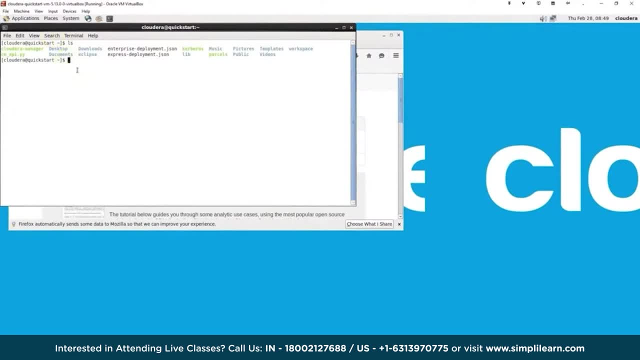 and everything squished together in one virtual machine. We can then do- let's do- HDFS, telling it that it's a Hadoop file system. DFS minus LS. Now notice, the LS is the same. I have LS for list. 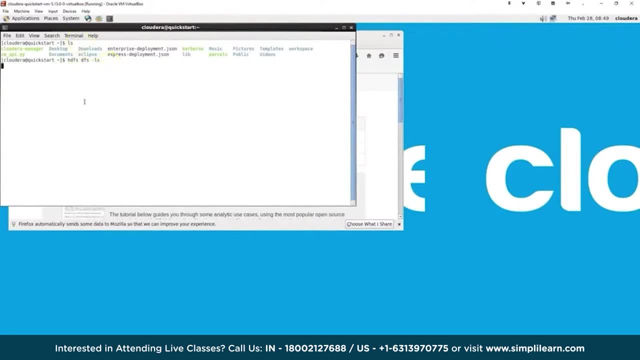 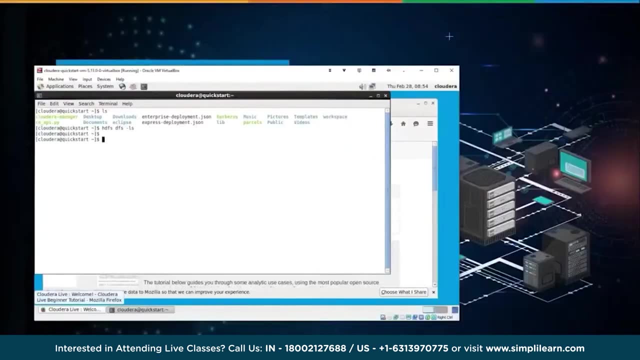 and LS for list And I click on here and it'll take you just a second reading- the Hadoop file system And it comes up with nothing. So a quick recap. Let's go back over this. Three different environments. I have this one out here. 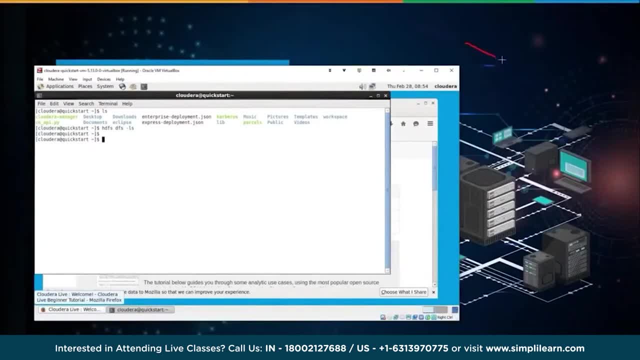 Let's just put this in a bright red so you can actually see it. I have this environment out here, which is my slides. I have this environment here where I did a list That's looking at the files on the Linux CentOS computer And then we have 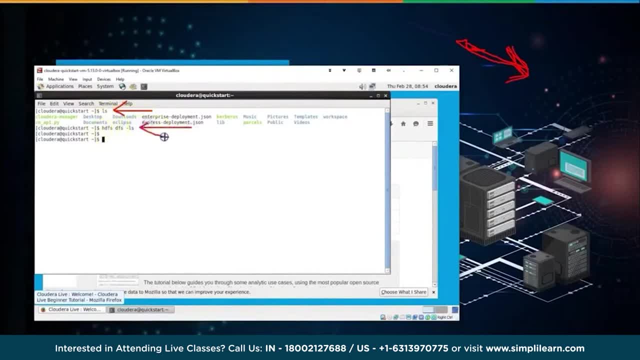 this system here, which is looking at the files on the Hadoop file system, So three completely separate environments, And then we connect them. And so right now we have- I have whatever files, I have my personal files and the. of course we're also. 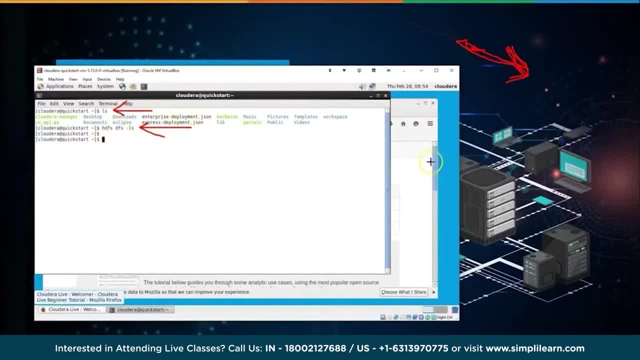 looking at the screen for my Windows 10.. And then we're looking at the screen here. Here's our list. there Let's look at the files. and this is the screen for CentOS Linux. And then this is looking at the files right here. 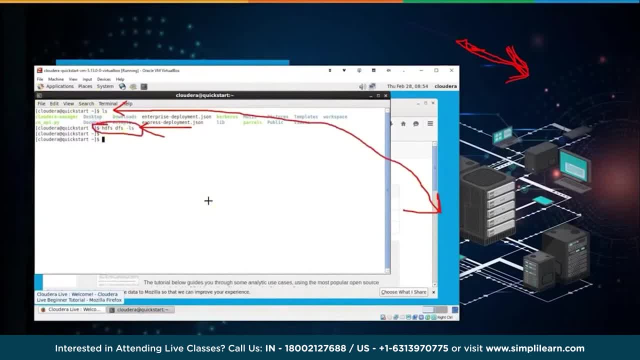 For the Hadoop file system, So three completely separate files. This one here, which is the Linux, is running in a virtual box. So this is a virtual box. I'm using one core to run it, or one CPU, And everything in there has its own file system. 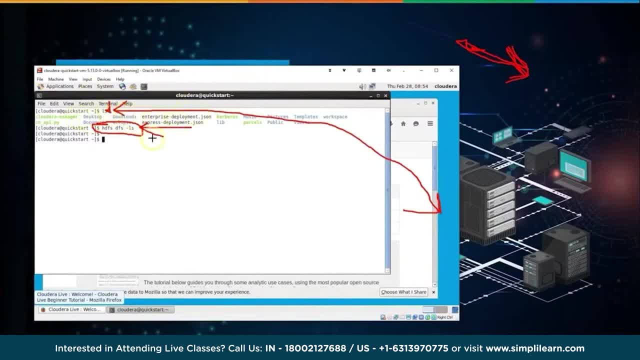 You can see we have our desktop and documents and whatever in there And then you can see here: we right now have no files in our Hadoop file system And this Hadoop file system currently is stored on the Linux machine. But it could be stored. 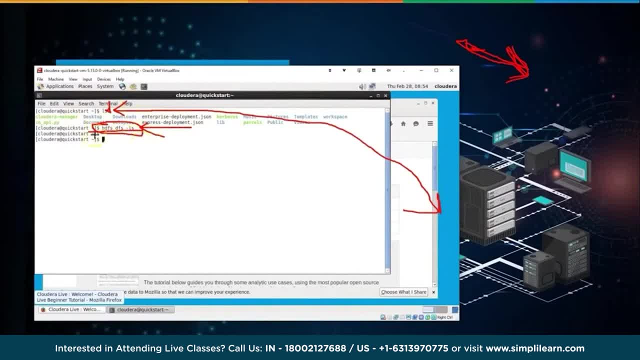 across 10 Linux machines, 20,, 100, this could be stored across in petabytes. I mean it could be really huge. or it could just be, in this case, just a demo, where we're putting it on just one computer And then, once we're in here, 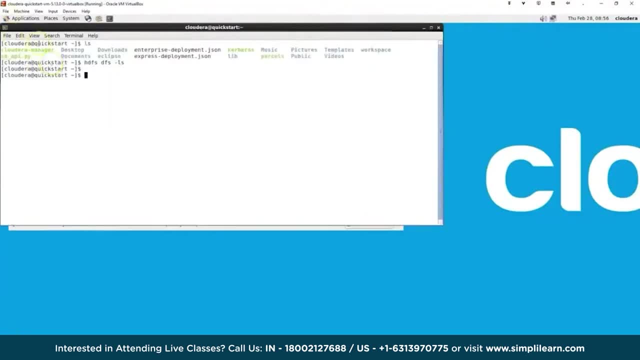 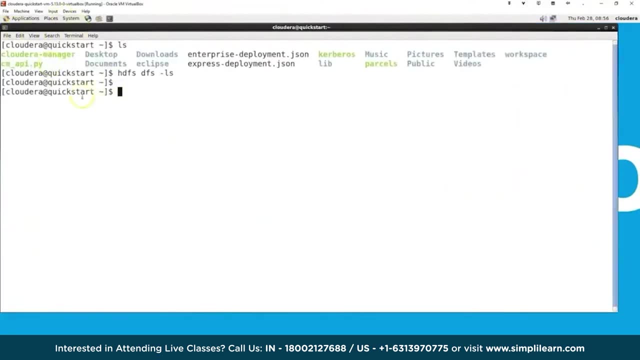 let me just see real quick if I can go under view zoom in. view zoom in And this is just a standard browser so I could use any like the control plus and stuff like that to zoom in, And this is very common to be in a browser window. 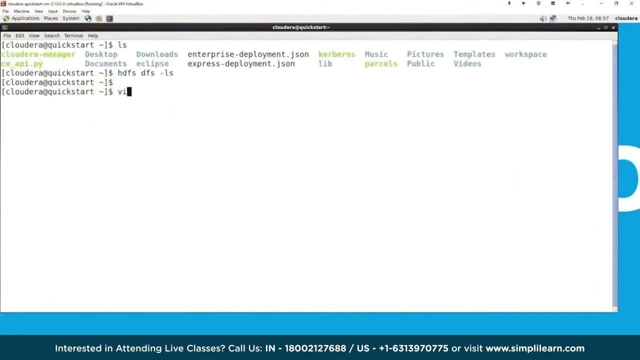 with the Hadoop file system. So right now I'm in a Linux and I'm going to do: oh, let's just create a file, We'll go file my new file And I'm going to use vi and this is a vi editor. 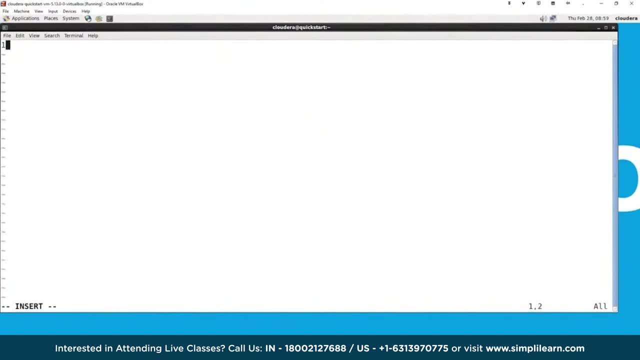 just a basic editor And we go ahead and type something in here: One, two, three, four, maybe it's columns 44,, 66, 77.. Of course I do file system, just like your regular computer can also. 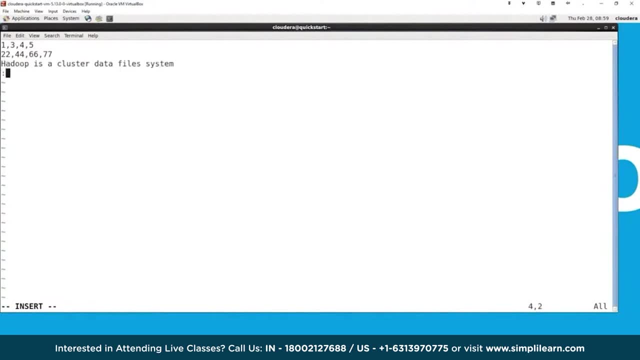 So in our vi editor you hit your colon. I actually work with a lot of different other editors And we'll write quit vi, So let's take a look and see what happened here. I'm in my Linux system. I type in ls for list. 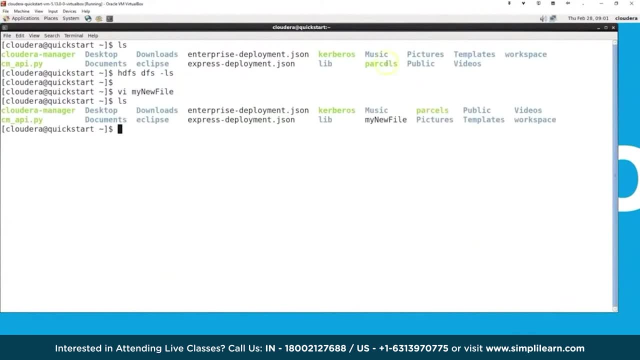 and we should see my new file. And sure enough, we do over here. There it is. Let me just highlight that my new file. And if I then go into the Hadoop system, hdfs, dfs minus ls for list, we still show nothing. 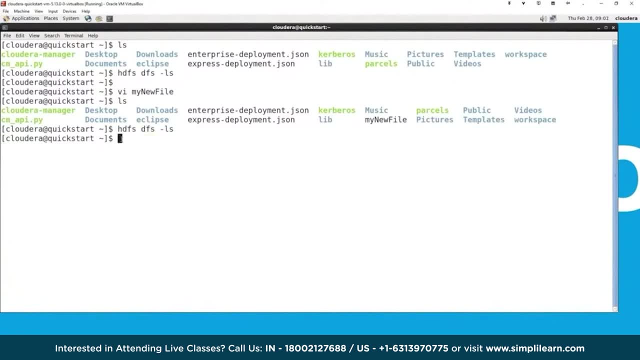 It's still empty. So what I can simply do is I can go hdfs, dfs, minus, put, And then we're going to put my new file, And this is just going to move it from the Linux system, because I'm in this file folder. 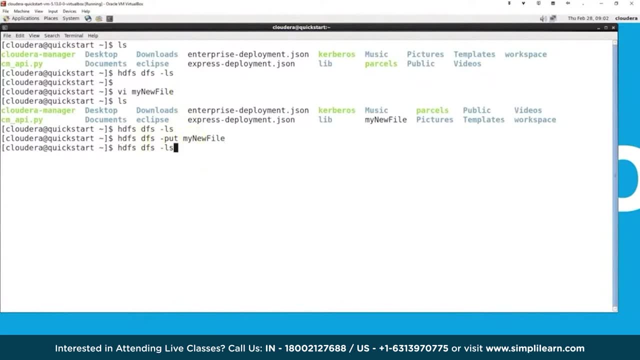 into the Hadoop file system And now if we go in and we type in our list for Hadoop file system, you will see in here that I now have just the one file on there, which is my new file And very similar to Linux. 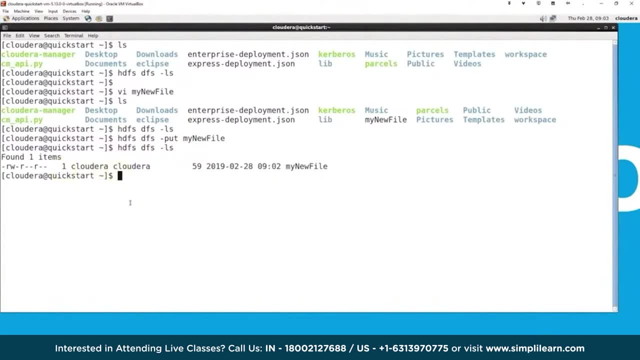 we can do cat, And the cat command simply evokes reading the file. So hdfs, dfs minus cat, And I had to look it up. Remember Cloudera, The format is going to be user, Then of course, the path location. 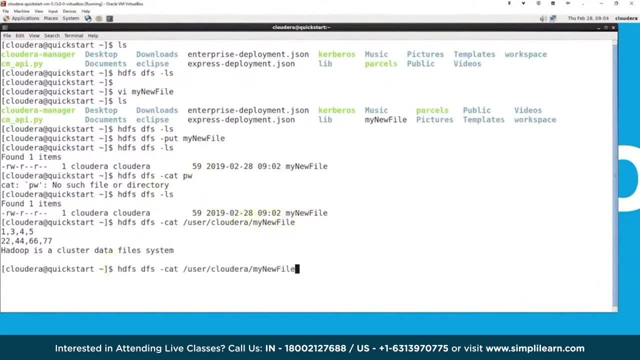 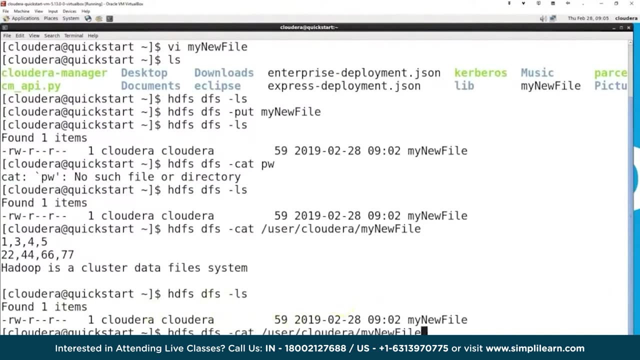 and the file name And in here when we did the list, here's our list, So you can see. it lists our file here And we realize that this is under user Cloudera And so I can now go user Cloudera, my new file. 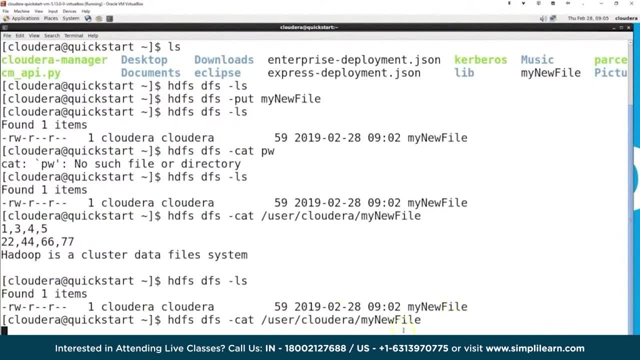 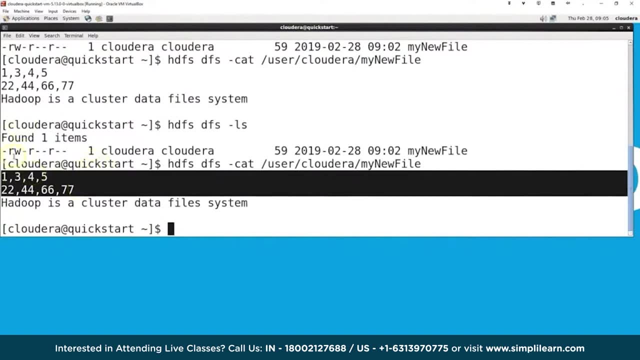 and the minus cat and we'll be able to read the file in here And you can see right here. this is the file that was in the Linux system. It is now copied into the Cloudera system and it's 1345 what I entered in there. 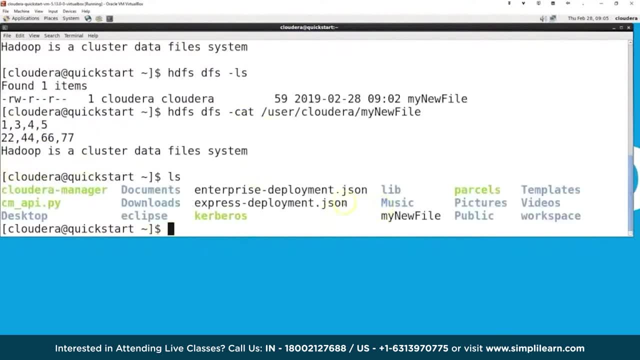 And if we go back to the Linux and do list, you'll still see it in here, my new file, And we can also do something like this in our hdfs minus mv. I will do my new file and we're going to change it to my new new file. 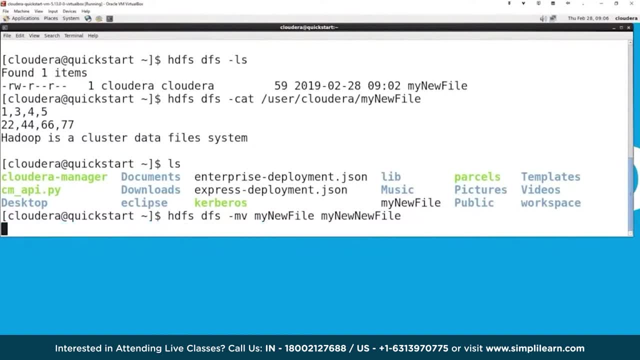 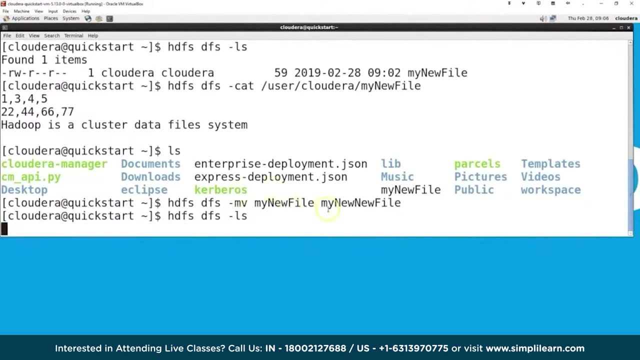 And if we do that underneath our Hadoop file system the minus mv will rename it. So if I go back here to our Hadoop file system ls, you'll now see instead of my new file it has my new new file coming up And there it is. 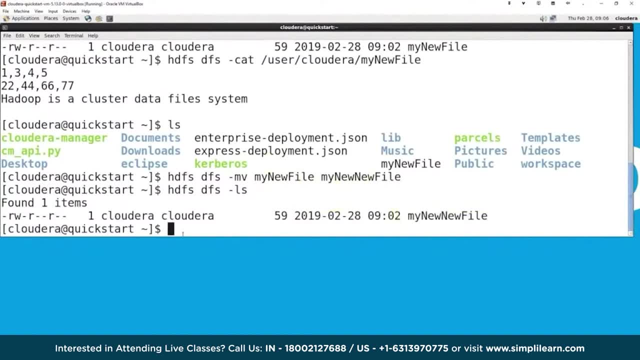 my new new file, So we've renamed it. We can also go in here and delete this, So I can now come in here. so in our hdfs dfs we can also do a remove and this will remove the file. And so if we come in here, 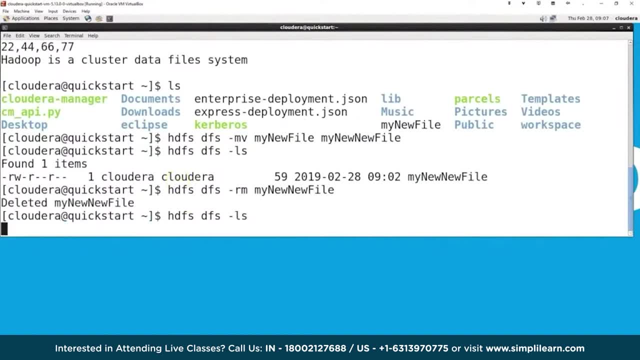 and we run this, we'll see that when I come back and do the list, the file is gone And now we just have another empty folder with our Hadoop file system And, just like any file system, we can take this and we can go ahead. 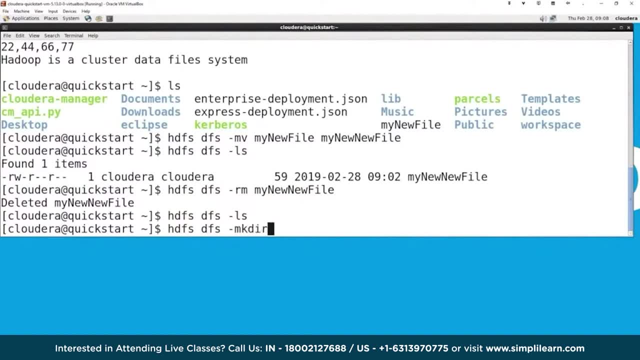 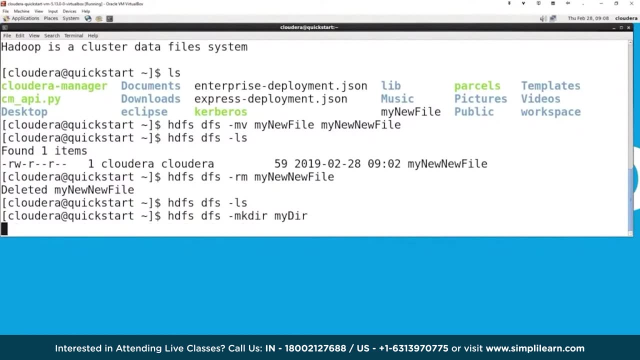 and make directory. create a new directory. so mk for make directory. we'll go ahead and we'll call this my dir. so we're going to make a directory my dir. it'll take it just a second and, of course, if we do the list command, you'll see that we now have 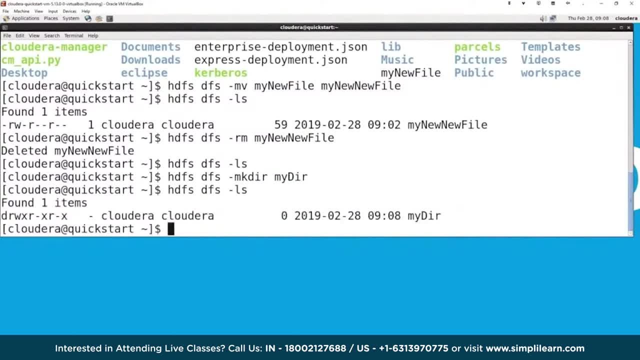 the directory in there. Give it just a second. there it comes my dir and, just like we did before, I can go in here and we're going to put the file- and if you remember correctly from our files in the setup I called it my new file. 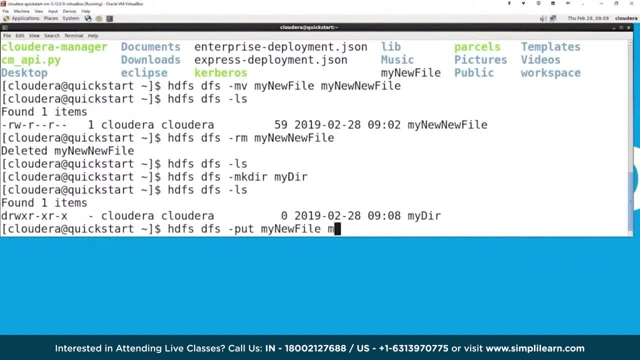 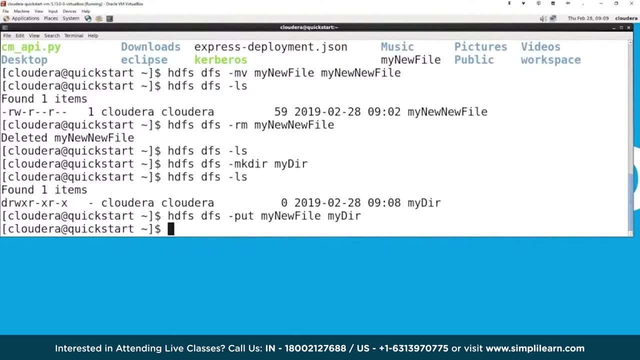 So this is coming from the Linux system and we're going to put that into my dir. That's the target in my Hadoop setup. So if I hit enter on there, I can now do the Hadoop list and that's not going to show. 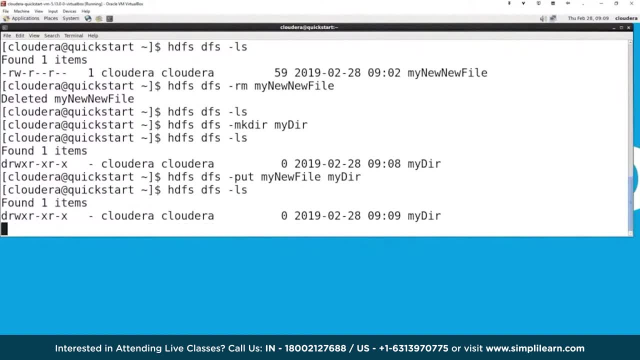 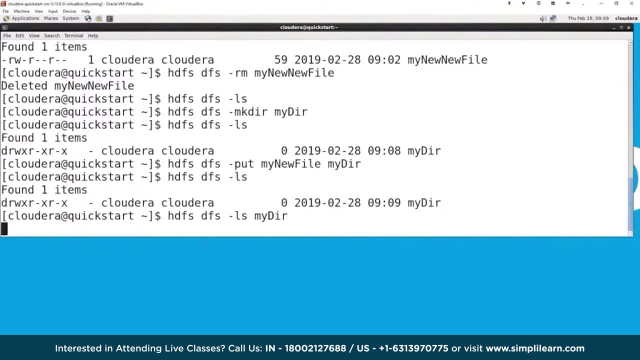 the file because, remember, I put it in a sub folder. So if I do the Hadoop list, this will show my directory and I can do list. and then I can do my dir for my directory and you'll see underneath the my directory in the Hadoop file system. 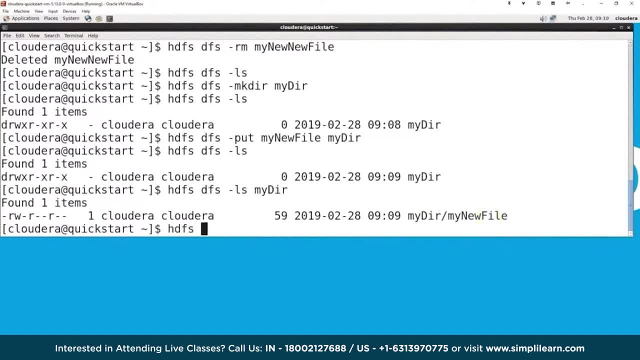 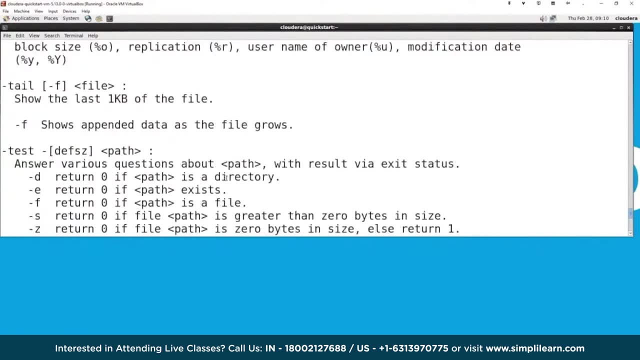 it now has my new file put in there, And with any good operating system we need a minus help. So just like you can type in help in your Linux, you can now come in here and type in hdfs help and it shows you a lot of the commands. 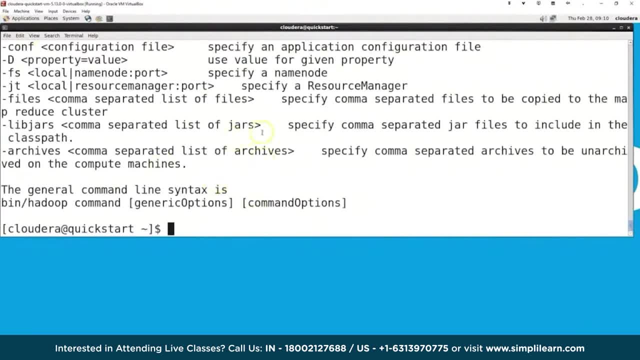 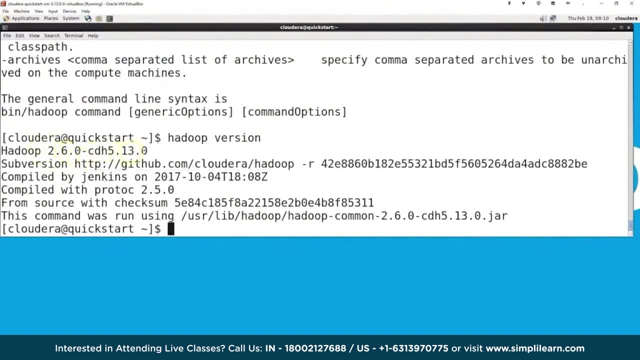 in there underneath the Hadoop file system. Most of them should be very similar to the Linux on here And we can also do something like this Hadoop version and the Hadoop version shows up that we're in Hadoop 2.60 CDH. is that we're? 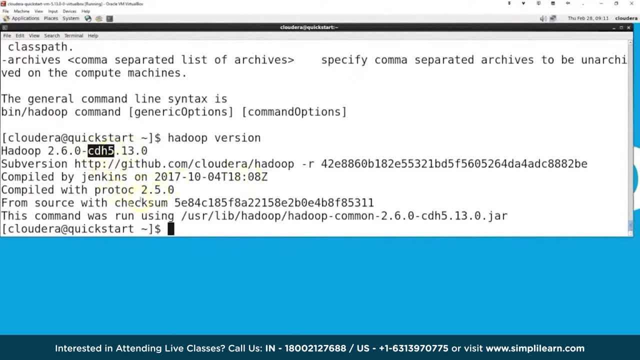 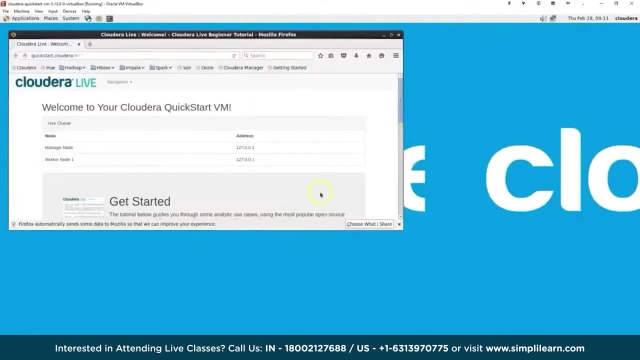 Cloudera 5 and compiled by Jenkins, and it has a date and all the different information on our Hadoop file system. So this is some basics in the terminal window. Let me go ahead and close this out because if you're going to play with this, 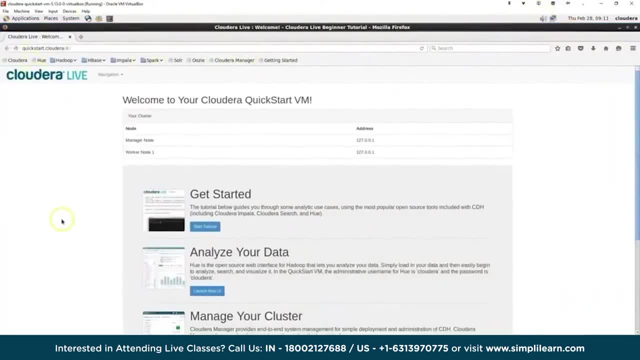 and say, come in here, let me just maximize the Cloudera, and it opens up in a browser window And so once we're in here again, this is a browser window which you could access. might look like any access for a Hadoop file system. 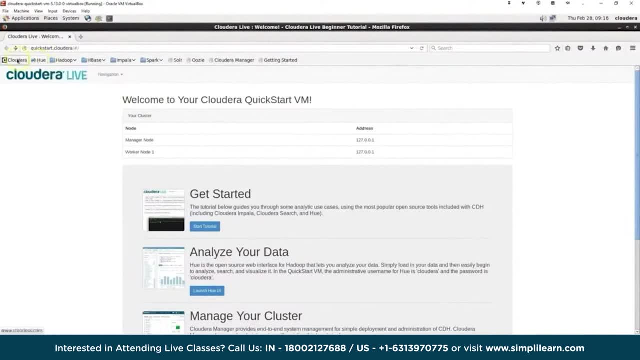 One of the fun things to do when you're first starting is to go under Hue. You'll see it up here at the top. has Cloudera Hue, Hadoop, your HBase, your Impala, your Spark. These are standard installs now. 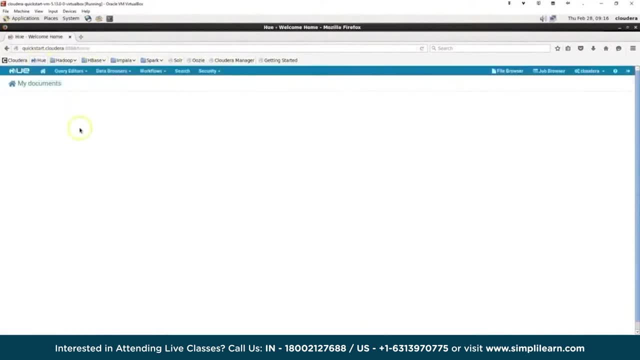 And Hue is basically an overview of the file system, And so come up here and you can see these. as far as if you have a HBase or a Hive- the Hive database- We can go over here to the top where it says file browser. 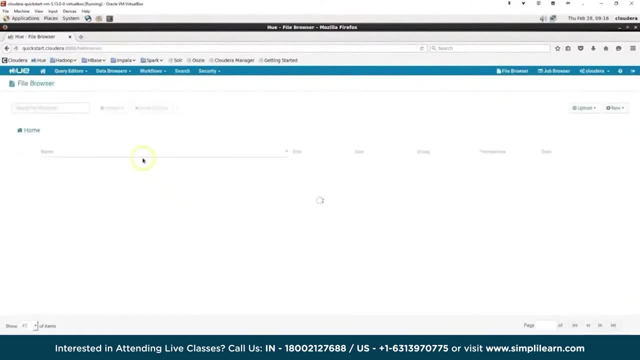 And if we go under file browser now, this is the Hadoop file system we're looking at. And once we open up the file browser, you can now see there's my directory, which we created, And if I click on my directory there's my new file. 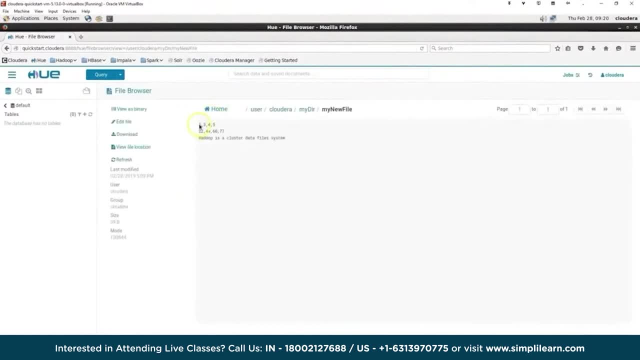 which is in here, And if I click on my new file it actually opens it up and you can see from our Hadoop file system. this is in the Hadoop file system, the file that we created. So we covered the terminal window And you can see. 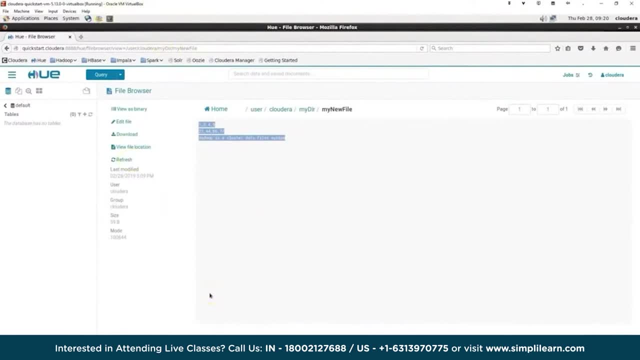 here's the terminal window up here. It might be if you were in a web browser it'll look a little different because it actually opens up as a web browser terminal window, And we've looked a little bit at Hue, which is one of the most. 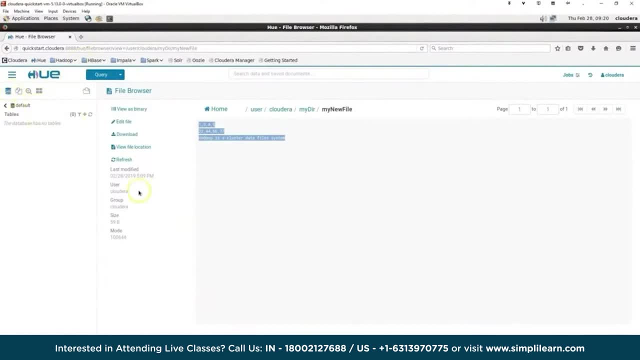 basic components of Hadoop, one of the original components for going through and looking at your data and your databases. Of course, now they're up to the Hue 4.. It's gone through a number of changes And you can see there's a lot of different. 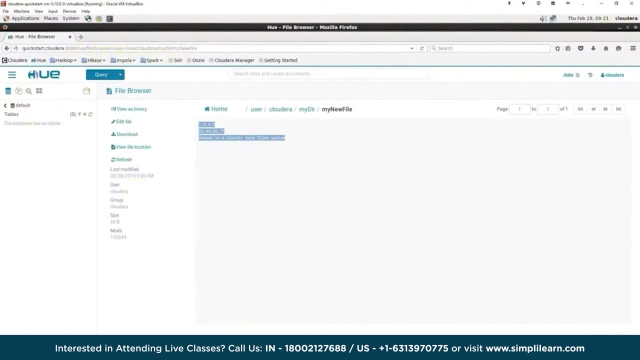 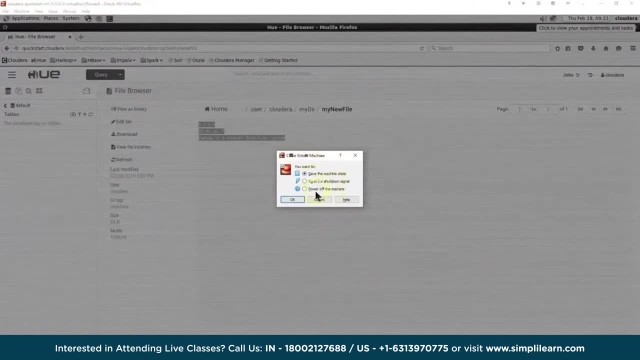 choices in here for other different tools in the Hadoop file system And I'll go ahead and just close out of this. And one of the cool things about this virtual box: I can either save the machine state, send the shutdown signal or power off the machine. 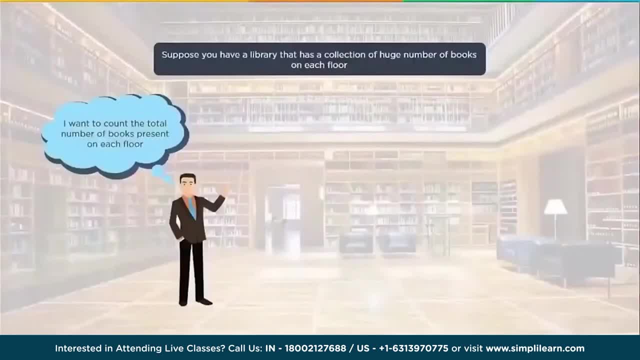 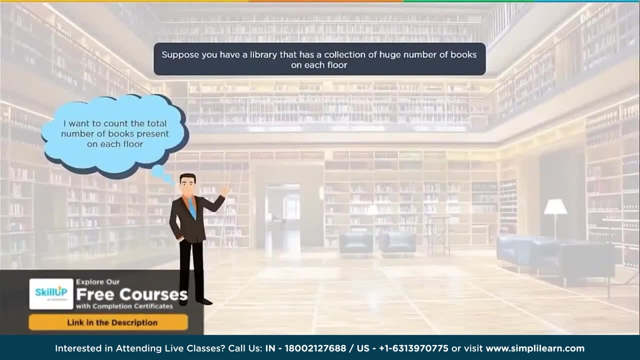 I'll go ahead and just power off the machine completely. Now suppose you have a library that has a collection of huge number of books on each floor And you want to count the total number of books present on each floor. What would be your approach? 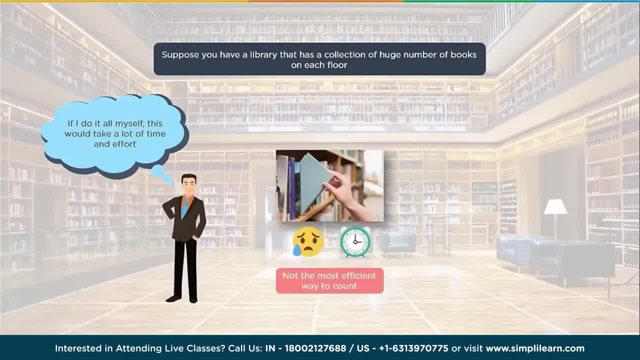 You could say I will do it myself, But then don't you think that will take a lot of time And that's obviously not an efficient way of counting the number of books in this huge collection of books. You want to count the number of books. 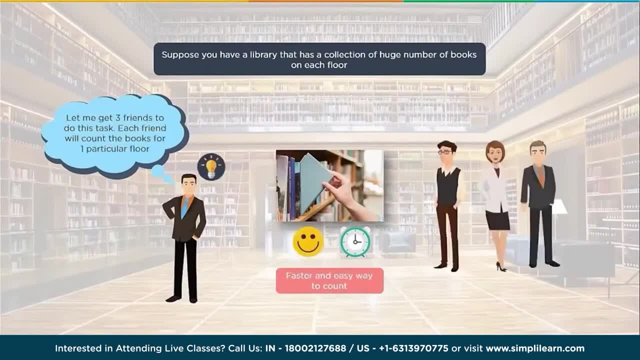 in this huge collection on every floor by yourself. Now there could be a different approach or an alternative to that. You could think of asking three of your friends or three of your colleagues, And you could then say if each friend could count the books on every floor. 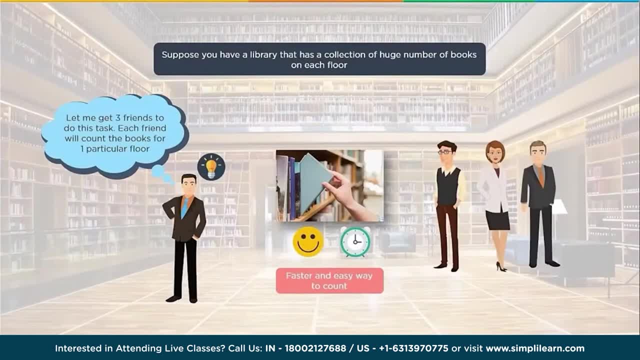 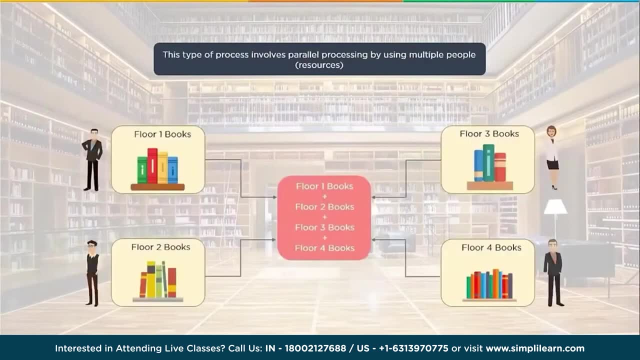 then obviously that would make your work faster and easier to count the books on every floor. Now this is what we mean by parallel processing. So when you say parallel processing, in technical terms, you're talking about using multiple machines to count the books on every floor. 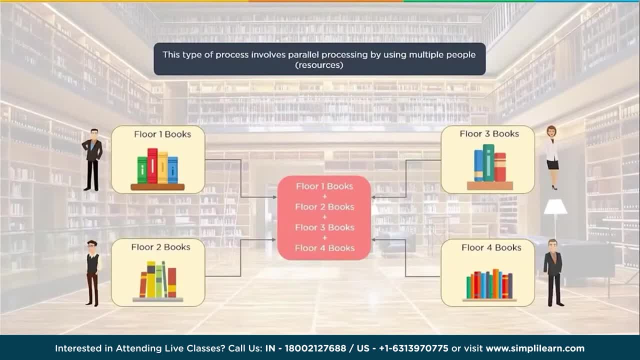 So you're using multiple machines, and each machine would be contributing its RAM and CPU cores for processing, and your data would be processed on multiple machines at the same time. Now, this type of process involves parallel processing, in our case, or in our library example, where you would have 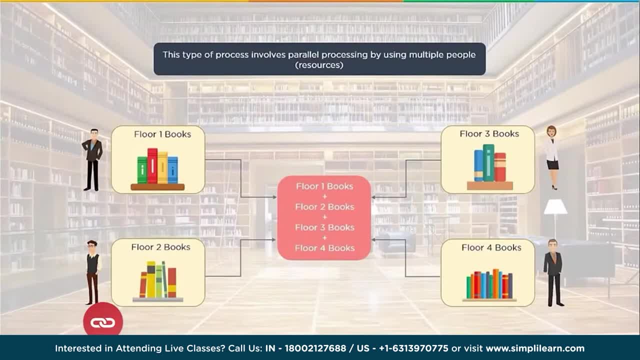 person one, who would be taking care of books on floor one and counting them. person two on floor two. Then you have someone on floor three and someone on floor four, So every individual would be counting the books on every floor in parallel, so that reduces the time consumed. 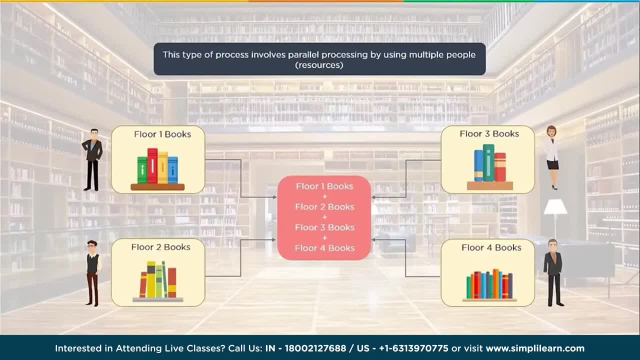 for this activity, and then there should be some mechanism where all these counts from every floor can be aggregated. So what is each person doing here? Each person is mapping the data of a particular floor, or you can say each person is doing a kind of activity. 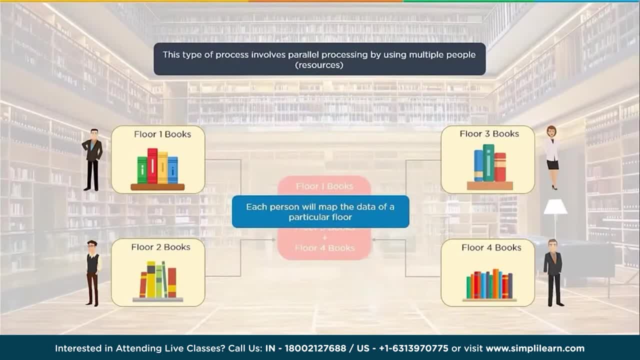 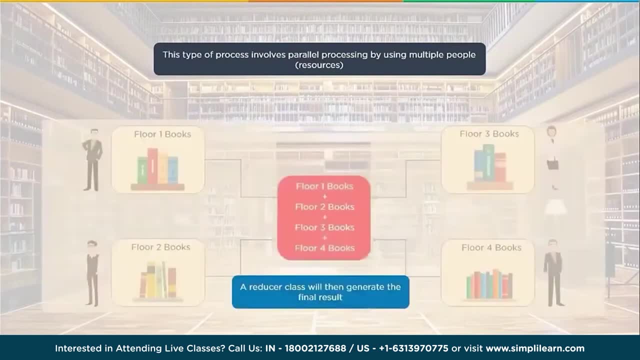 or basically a task on every floor, and the task is being done on every floor, and the task is being done on every floor and the task is counting the books on every floor. Now then you could have some aggregation mechanism that could basically reduce or summarize this total count. 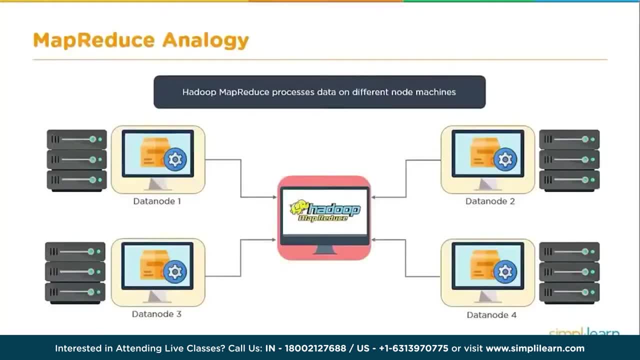 and in terms of map reduce, we would say that's the work of reducer. So when you talk about Hadoop, map reduce, it processes data on different node machines. Now, this is the whole concept of Hadoop framework right, that you not only have your data. 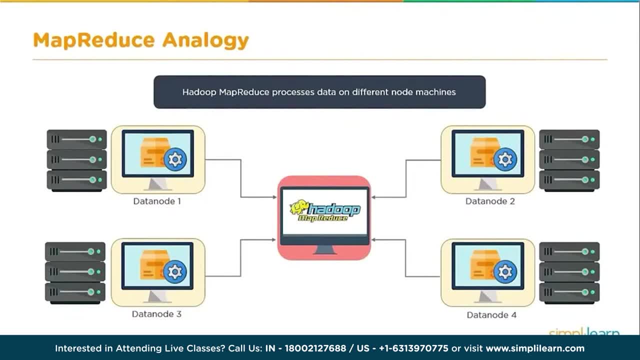 stored across machines manually. So instead of transferring the data from one machine to other machine or bringing all the data together into some central processing unit and then processing it, you would rather have the data processed on the machines, wherever that is stored. So we know in case of Hadoop. 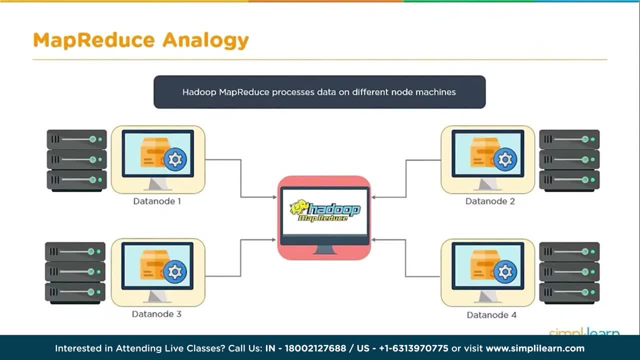 cluster, we would have our data stored on multiple data nodes, on their multiple disks, and that is the data which needs to be processed. but the requirement is that we want to be as fast as possible, and that could be achieved by using parallel processing. Now, in case of map, 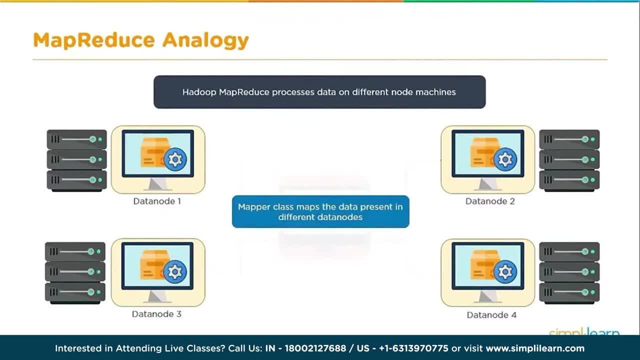 reduce. we basically have the first phase, which is your mapping phase. So in case of map reduce programming model, you basically have two phases: one is mapping and one is reducing. Now, who takes care of things in mapping phase? it is a mapper class, and this mapper class has 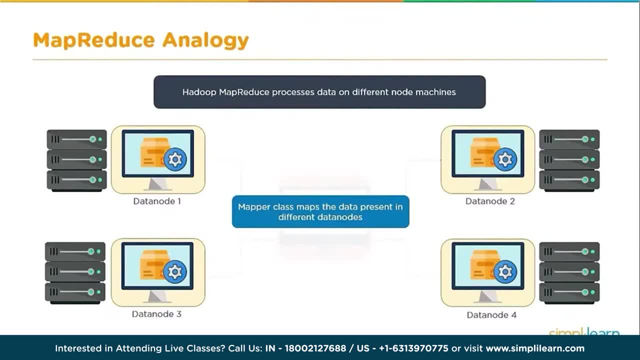 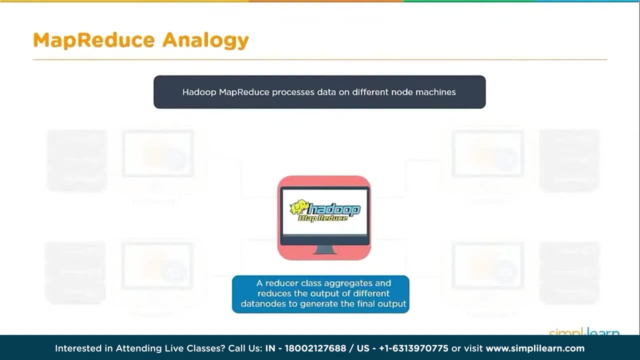 the function which is provided by the developer, which takes care of these individual map tasks, which is, the map tasks which will work on multiple nodes in parallel. Your reducer class belongs to the reducing phase, So a reducing phase basically uses a reducer class which provides a function that. 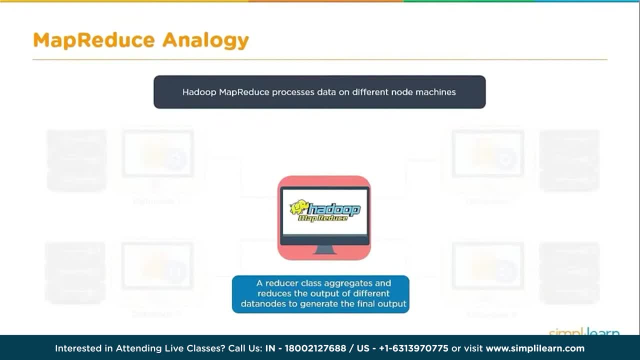 will aggregate and reduce the output of different data nodes to generate the final output. Now that's how your map reduce works: using mapping and then, obviously, reducing. Now you could have some other kind of jobs which are map reducing required, but we are not talking about those. 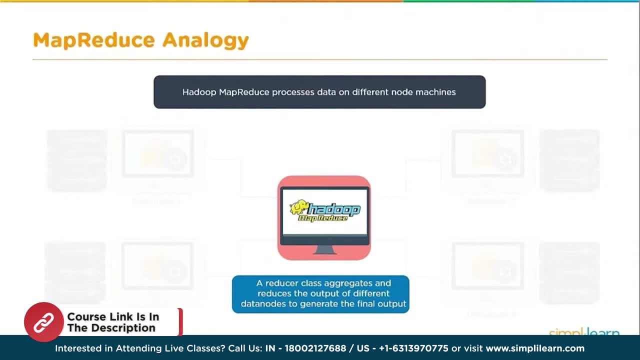 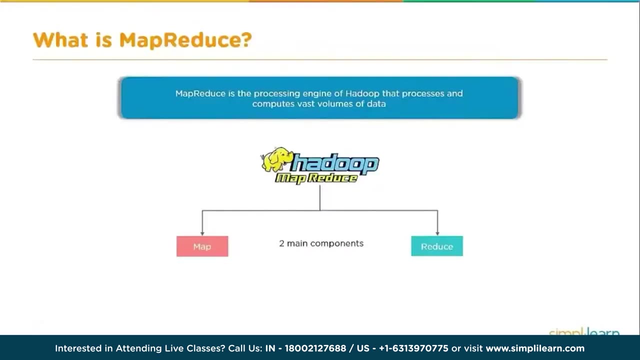 we are talking about our requirement where we would want to process the data using mapping and reducing, especially when data is huge, when data is stored across multiple machines and you would want to process the data in parallel. So when you talk about map, reduce, you could say: 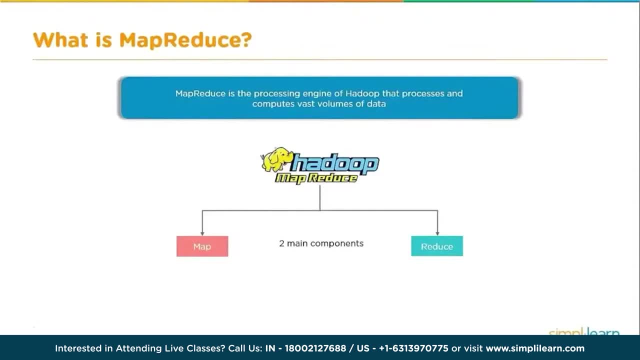 it's a programming model. you could say internally it's a processing engine of Hadoop that allows you to process huge volumes of data. We can talk about terabytes, we can talk about petabytes, exabytes and that amount of data which needs to be processed. 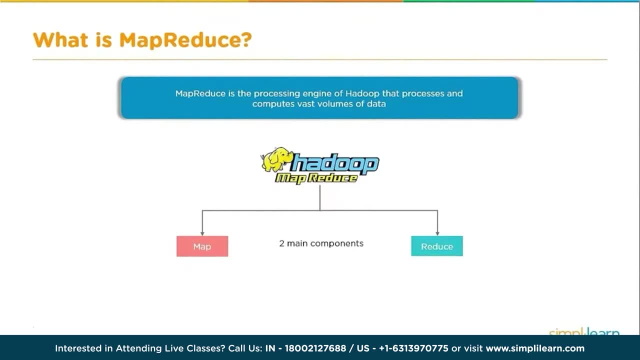 on a huge cluster. We could also use map reduce programming model and run a map reduce algorithm in a local mode. but what does that mean If you would go for a local mode? it basically means it would do all the mapping and reducing on the same. 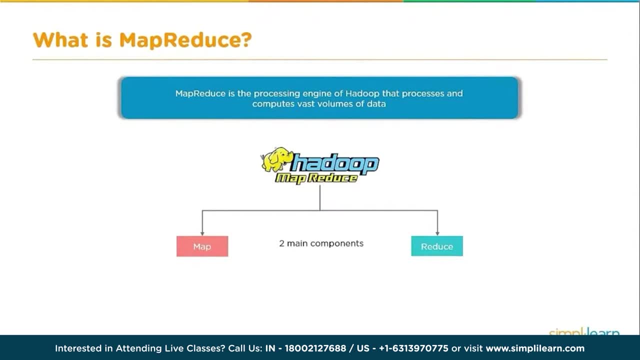 node using the processing, which is not really efficient. In fact, we would want to have our map reduce work on multiple nodes, which would obviously have mapping phase followed by a reducing phase and intermittently there would be data generated. there would be different other phases which help this whole. 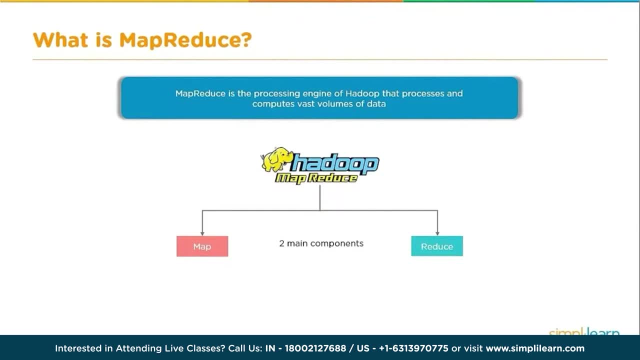 processing. So when you talk about Hadoop, map reduce, you are mainly talking about two main components or two main phases, that is. so you would have your data, which would be stored on multiple machines. now, when we talk about data, data could be in different formats. we 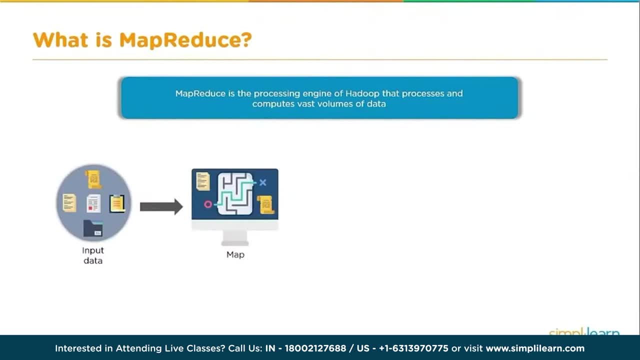 could, or the developer could, specify what is the format which needs to be used to understand the data which is coming in. that data then goes through the mapping. internally. there would be some shuffling, sorting and then reducing the data which is being stored on SDFS. we 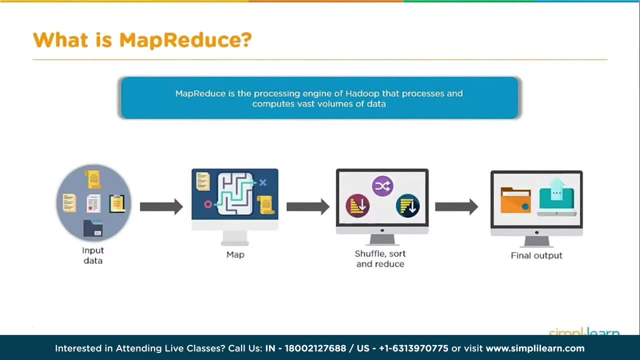 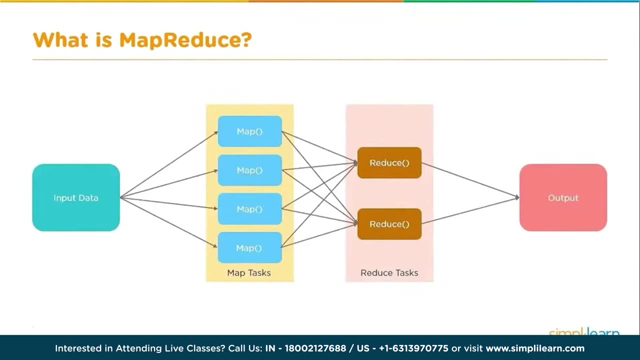 have our input data, which would have one or multiple files and one or multiple directories, and your final output is also stored on SDFS to be accessed, to be looked into and to see if the processing was done correctly. so this is how it looks. so you have the 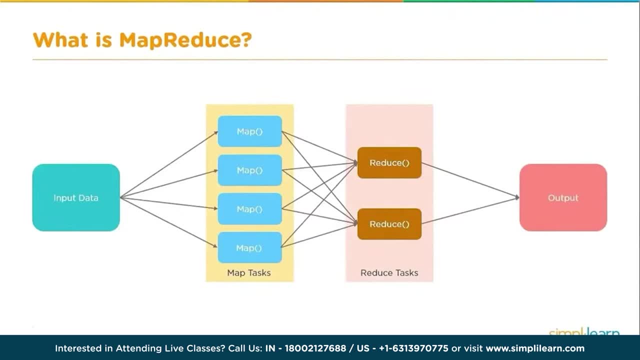 input data which would then be worked upon by multiple map tasks. now, how many map tasks? that basically depends on the cluster. you would have a file which is broken down into blocks depending on its size. so the default block size is 128 MB, which can then still be. 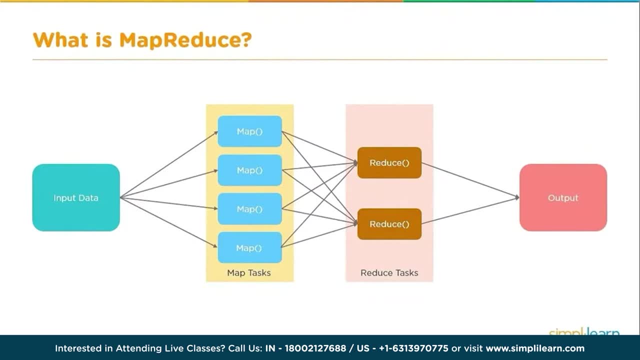 customized based on your average size of data which is getting stored on the cluster. so if I have really huge files which are getting stored on the cluster, I would certainly set a higher block size so that my every file does not have huge number of blocks creating a load on. 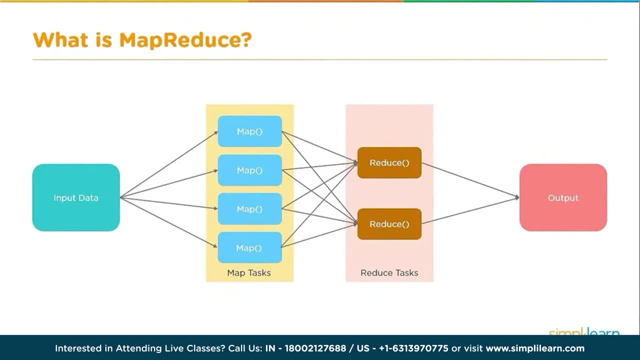 name nodes RAM, because that's tracking the number of elements in your cluster or number of objects in your cluster. so, depending on your file size, your file would be split into multiple chunks and for every chunk we would have a map task running. now, what is this map task? 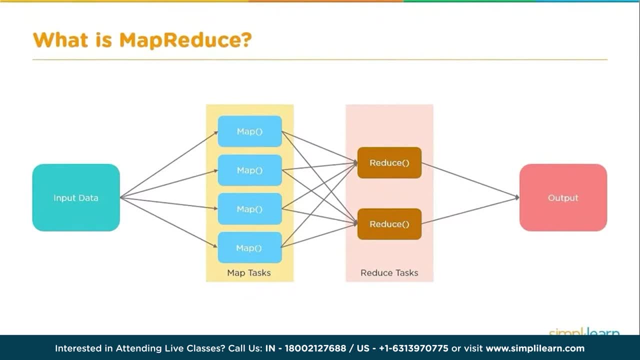 doing that is specified within the mapper class. so within the mapper class you have the mapper function, which basically says what each of these map tasks has to do on each of the chunks which has to be processed. this data is stored in the mapper, where it is sorted, and 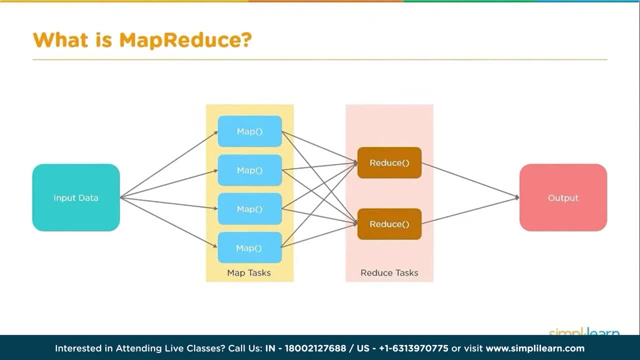 shuffled. and then you have internal phases, such as partitioner, which decides how many reduce tasks would be used or what data goes to which reducer. you could also have a combiner phase, which is like a mini reducer, doing the same reduce operation before it reaches reduce. then you have 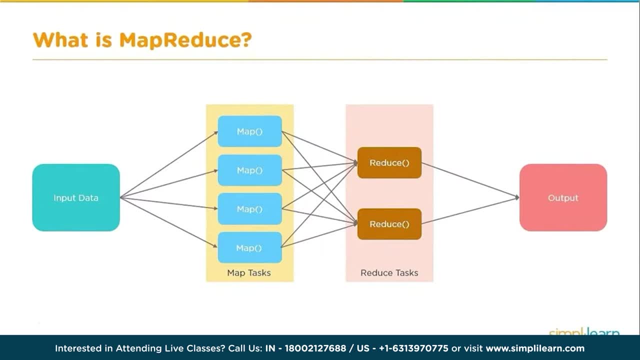 your reducing phase, which is taken care by a reducer class, and internally, the reducer will have reduced task running on the data which comes as an output from map tasks. finally, your output is then generated, which is stored on HDFS. now, in case of Hadoop, it accepts data in. 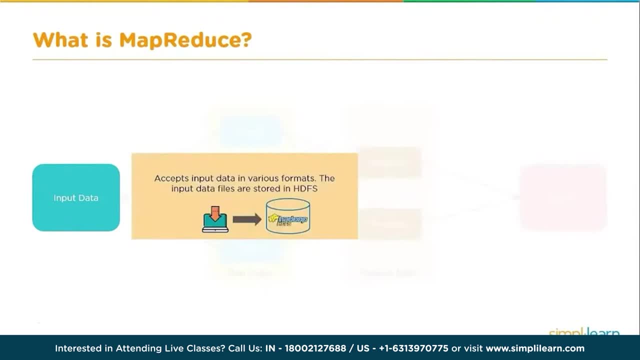 different formats. your data could be in compressed format. your data could be in parquet. your data could be in Avro text, CSV, TSV, binary format and all of these formats are supported. however, remember, if you are talking about data being compressed, then you have to also look into 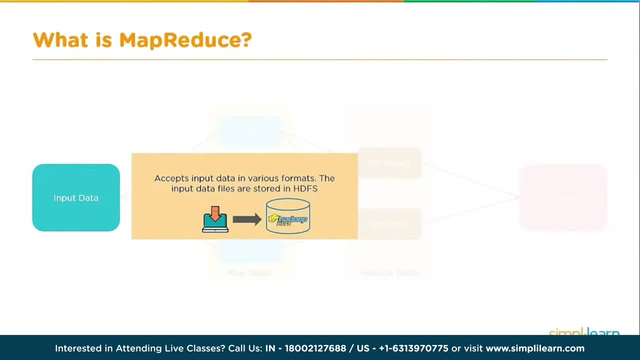 what kind of split ability the compression mechanism supports. otherwise, when map reduce processing happens, it would take the complete file as one chunk to be processed. so HDFS accepts input data in different formats. this data is stored in HDFS and that is basically our input, which is. 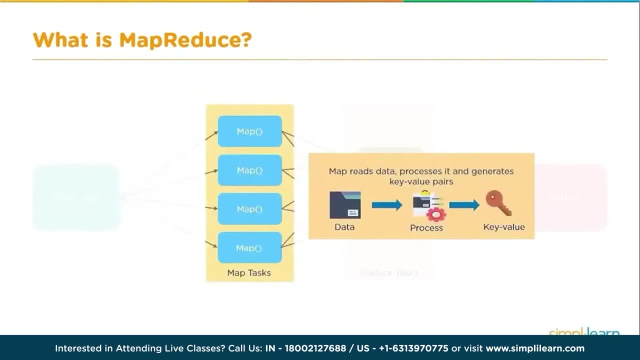 then passing through the mapping phase. now, what is mapping phase doing? as I said, it reads record by record. depending on the input format, it reads the data task running on multiple chunks. once this data is being read, this is broken down into individual elements, and when I say individual, 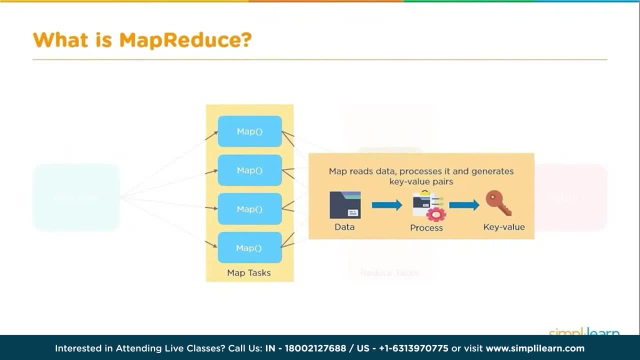 element. I could say: this is my list of key value pairs. so your records, based on some kind of delimiter or without delimiter, are broken down into individual elements and thus your map creates key value pairs. now, these key value pairs are not my final output. these key value pairs, 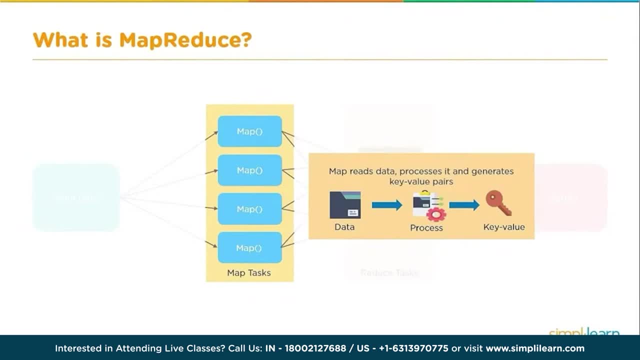 are basically a list of elements which will then be subjected to further processing. so you would have internally shuffling and sorting of data so that all the relevant key value pairs are brought together, which basically benefits the processing, and then you have your reducing, which aggregates the key value. 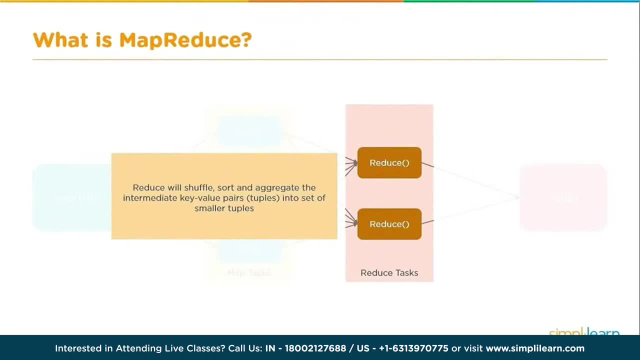 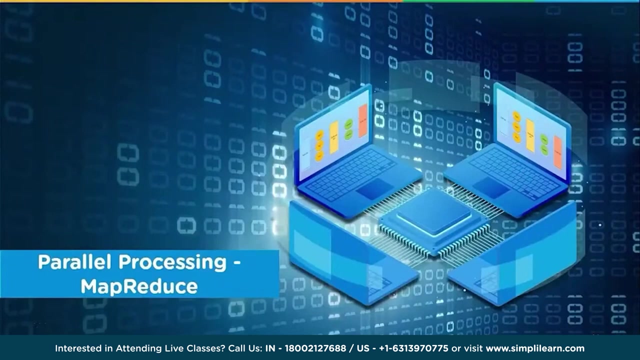 pairs into set of smaller tuples, or tuples as you would say. finally, your output is getting stored in the designated directory as a list of aggregated key value pairs which you can then store in your output. so when we talk about map reduce, one of the key factors here is 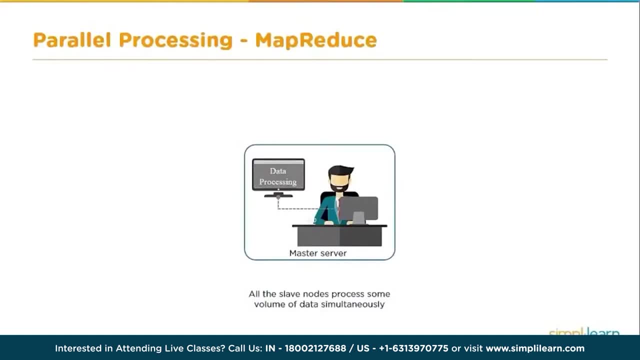 the parallel processing which it can offer. so we know that we, our data, is getting stored across multiple data nodes and you would have huge volume of data which is split and randomly distributed across data nodes, and this is the data which needs to be processed and the best way would be. 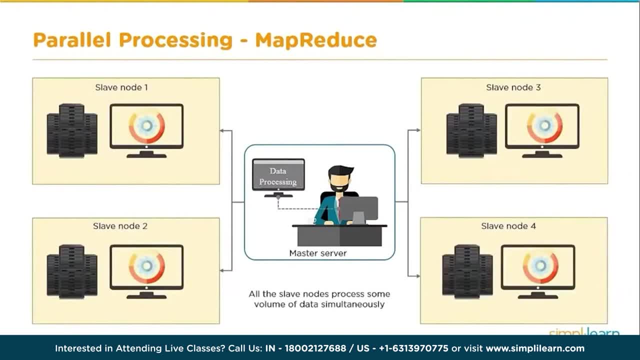 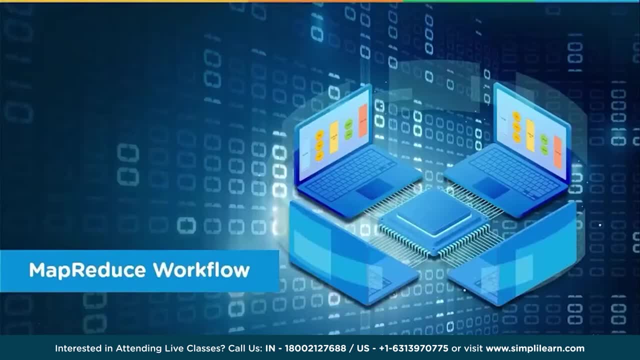 parallel processing, so you could have your data getting stored across multiple slave nodes and each slave node would have again one or multiple disks to process this data. basically, we have to go for parallel processing approach. we have to use the map reduce. now let's look at the map. 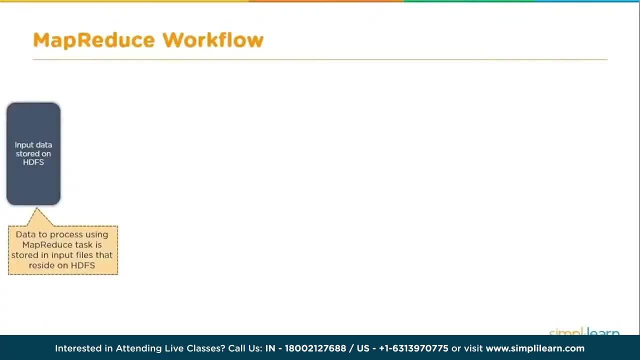 reduce workflow to understand how it works. so basically, you have your input data stored on sdfs. now this is the data which needs to be processed. it is stored in input files and the processing which you want can be done on one single file or it can be. 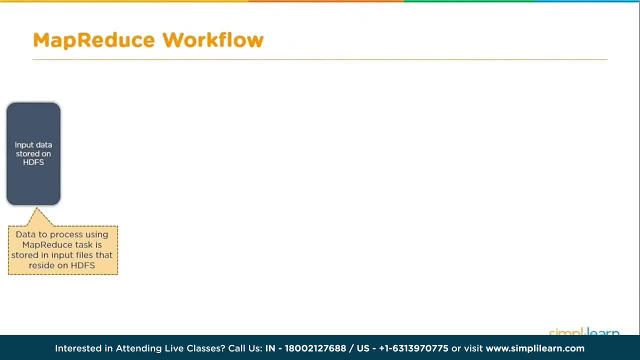 done on a directory which has multiple files. you could also later have multiple outputs merged, which we achieve by using something called as chaining of mappers. so here you have your data getting stored on sdfs now. input format is basically something to define the input specification and 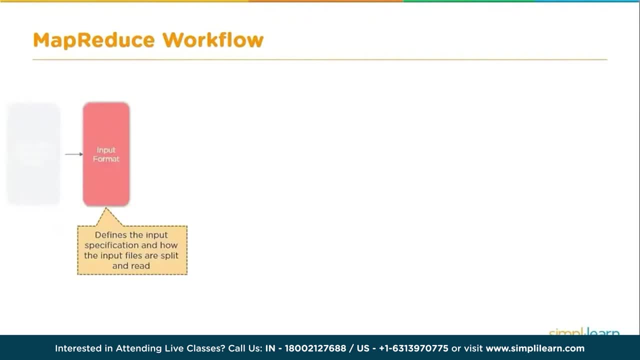 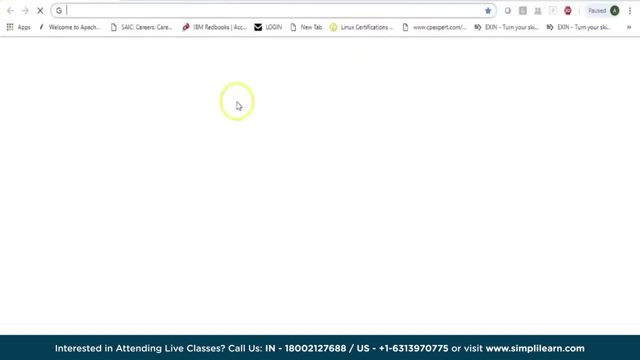 how the input files will be split. so there are various input formats. now we can search for that. so we can go to google and we can basically search for hadoop map reducer and we can basically search for map reduce yahoo tutorial. this is one of the good. 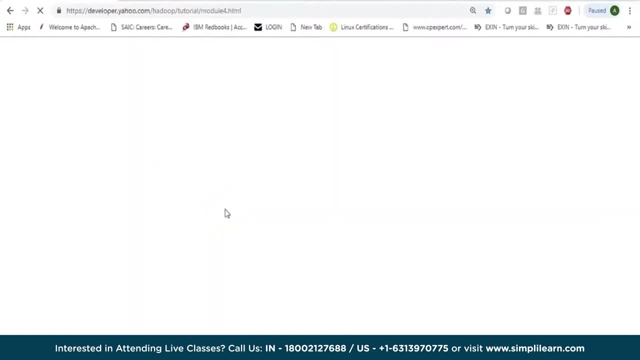 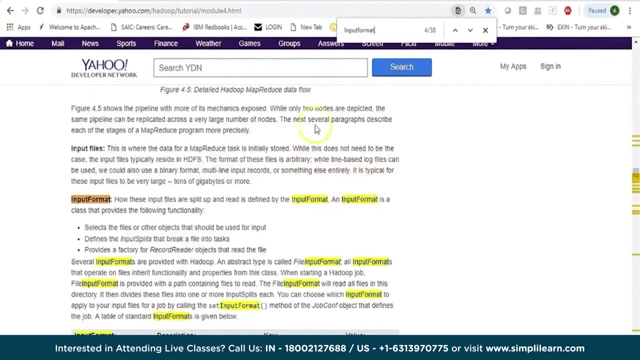 links and if i look into this link, i can search for different input formats and output format. so let's search for input format. so when we talk about input format, you basically have something to define how input files are split. so input files are split up and read based. 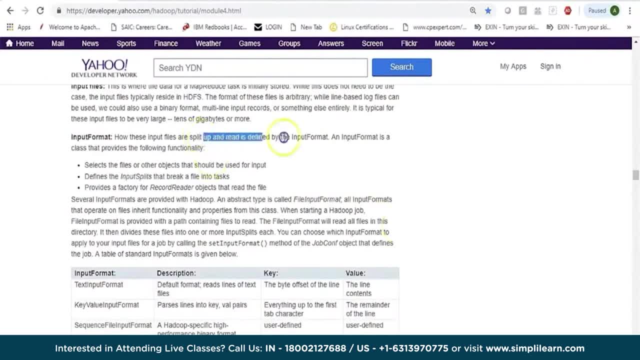 on what input format is specified. so this is a class that provides following functionality: it selects the files or other objects and then it selects the files or other objects and then selects the objects that should be used for input. it defines the input split that break a file into. 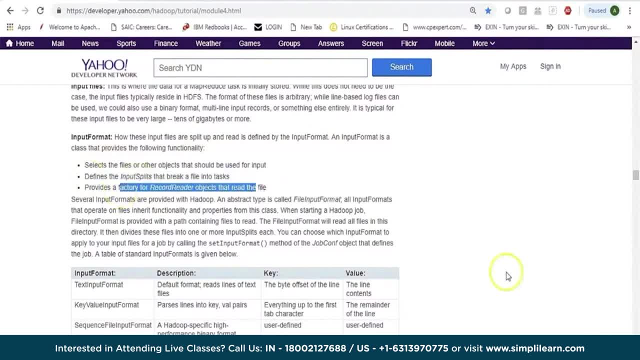 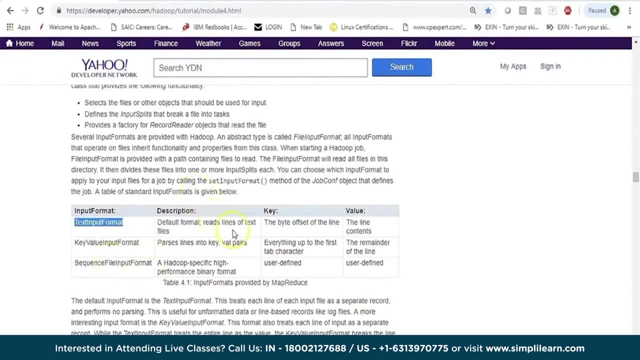 tasks provides a factory for record reader objects that read the file. so there are different formats. if you look in the table here and you can see that the text input format is the default format, which reads lines of a text file and each line is considered as a. 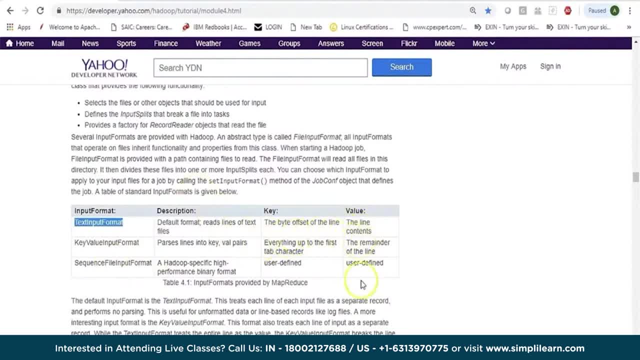 record. here the key is the byte offset of the line and the value is the line content itself. you can have key value input format which parses lines into key pairs. everything up to the first tab character is the key and the remainder is the line. you could also have sequence. 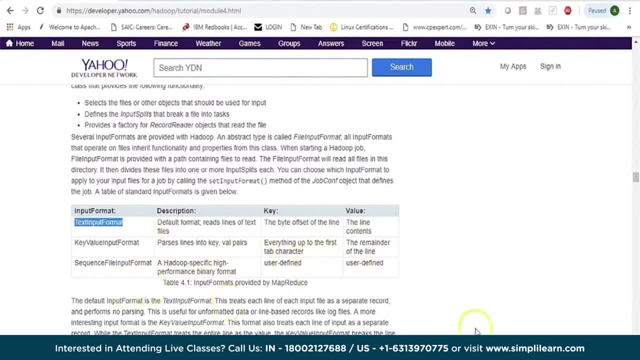 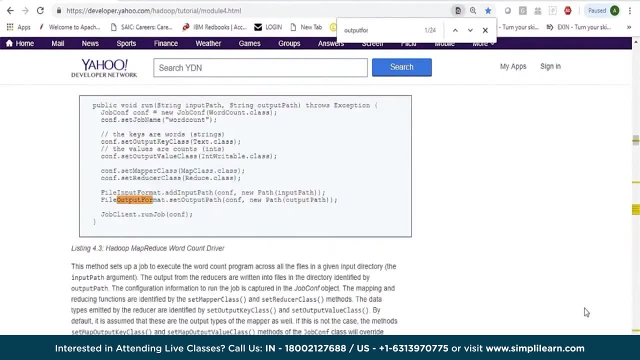 file input format which basically works on binary format. so you have input format and in the same way you can also search for output format, which takes care of how the data is handled after the processing is done. so the key value pairs provided to this output collector are: 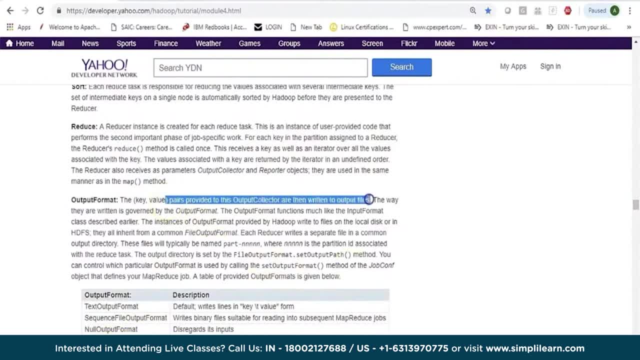 then written to output files. the way they are written is governed by output format, so the key value pairs provided to output files is the output format. so it functions pretty much like input format as described in earlier. right, so we could set what is the output format to be. 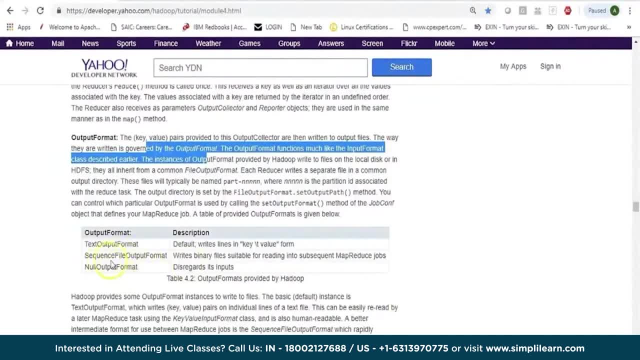 followed and again you have text output sequence, file output format, null output format, and so on. so these are different classes which take care of how your data is handled when it is being read for processing, or how is the data being written when the processing is done. so, based on the 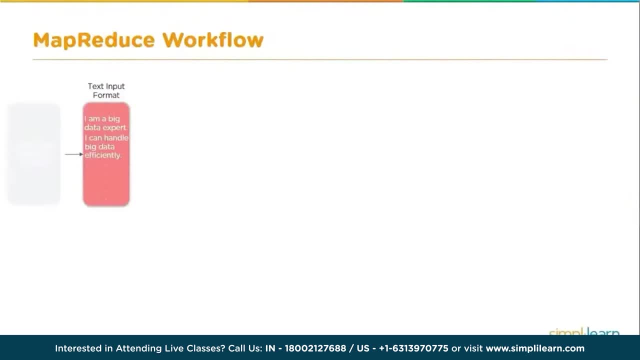 input format. the file is broken down to the output format. file is broken down into splits and this logically represents the data to be processed by individual map tasks or you could say individual mapper functions. so you could have one or multiple splits which need to be processed, depending on the 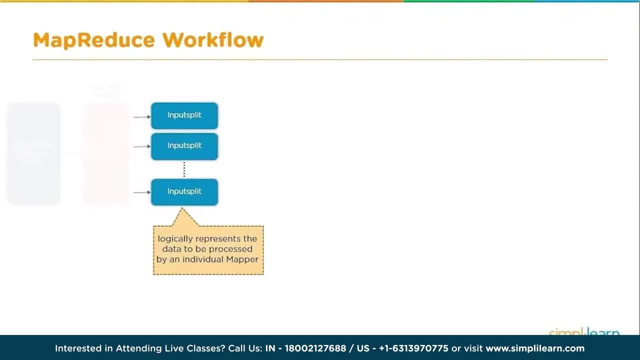 file size, depending on what properties have been set. now, once this is done, you have your input splits, which are subjected to mapping phase. internally, you have a record reader which communicates with the input split and converts the data into the key value pairs suitable to be read by mapper. 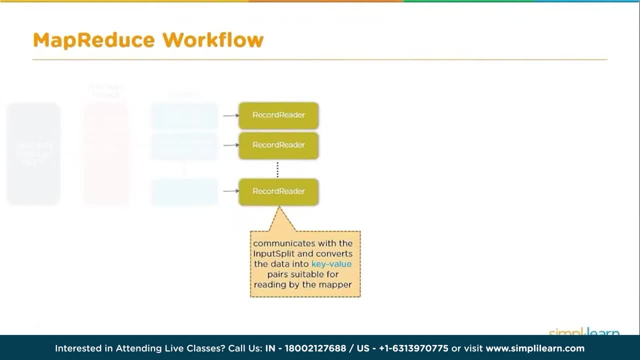 and what is mapper doing? it is basically working on these key value pairs, the map task, giving you an intermittent output which would then be forwarded for further processing. now, once that is done and we have these key value pairs, which is being worked upon? my map, your map. 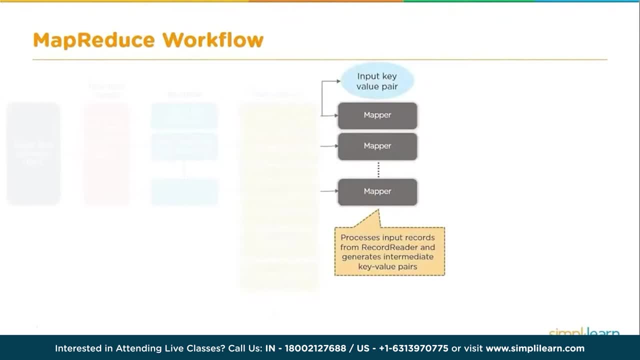 tasks as a part of your mapper function are generating your key value pairs, which are your intermediate outputs to be processed further. now you have, as I said, a combiner phase or, internally, a mini reducer phase. now combiner does not have its own class, so combiner 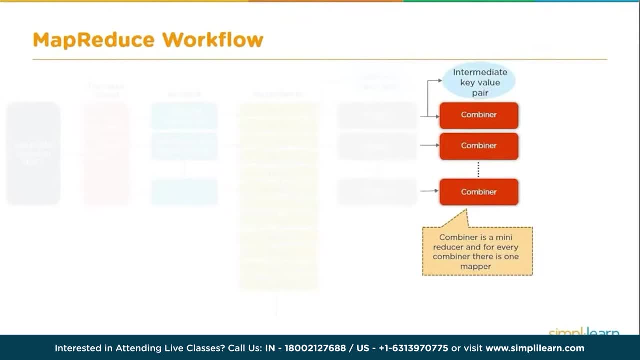 basically uses the same class as the reducer class provided by the developer and its main work is to do the reducing, or its main work is to do some kind of mini aggregation on the key value pairs which were generated by map. so once the data is coming in from 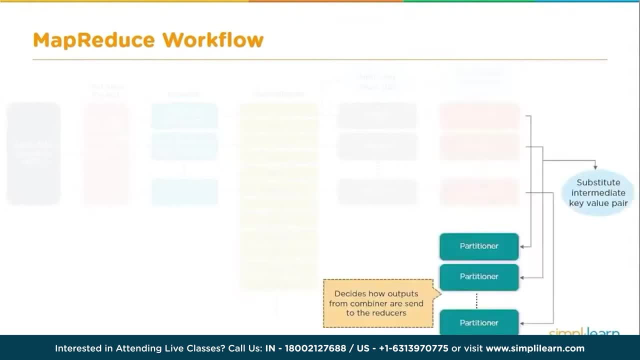 the combiner. then we have a partitioner phase which decides how outputs from combiners are sent to the reducers. or you could also say that, even if I did not have a combiner, partitioner would decide based on the keys and values, based on the type of keys. 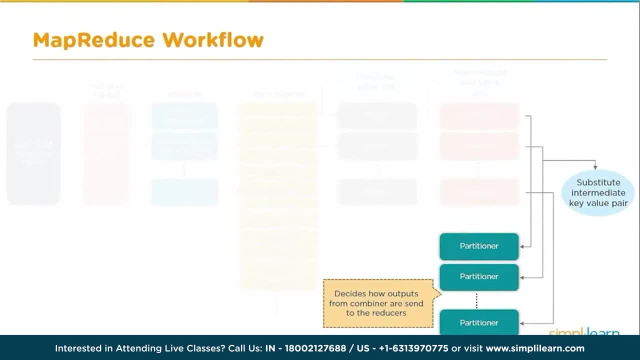 how many reducers would be required or how many reduced tasks would be required to work on your output, which was generated by map task. now, once partitioner has decided that, then your data would be then sorted and shuffled, which is then fed into the reducer. so when you talk, 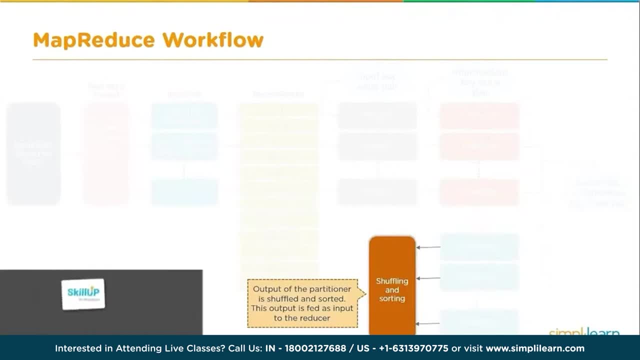 about your reducer. it would basically have one or multiple reduced tasks. now that depends on what or what partitioner decided or determined for your data to be processed. it can also depend on the configuration properties which have been set to decide how many reduced tasks should be used now internally. 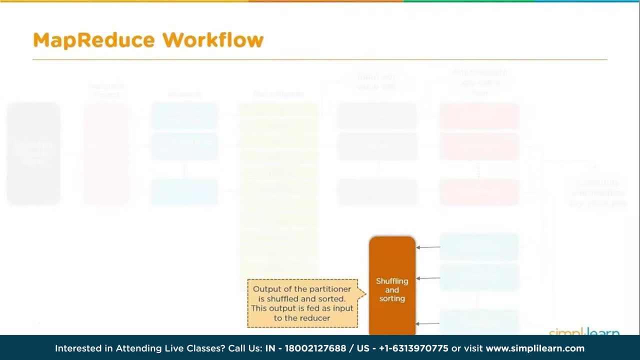 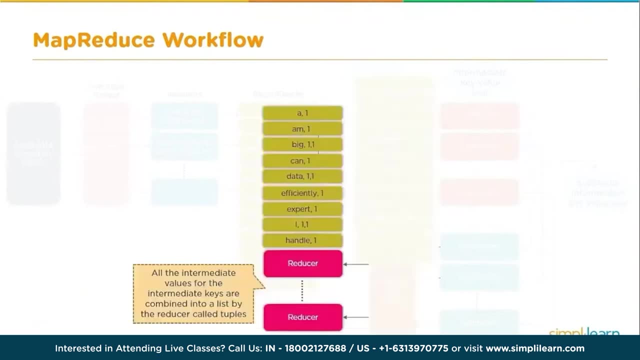 all this data is obviously going through sorting and shuffling so that you are able to use it in the right way, and then it becomes an easier task. once we have this done, we basically have the reducer, which is the code for the reducer is provided by the. 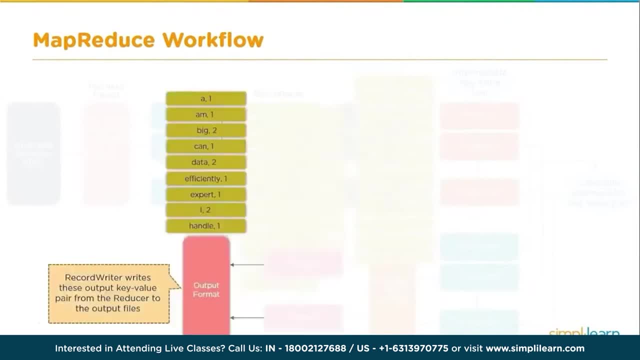 developer, and all the intermediate data has then to be aggregated to give you a final output which would then be stored on SDFS. and who does this? you have an internal record writer which writes these output key value pairs from reducer to the output files. now this final output data: 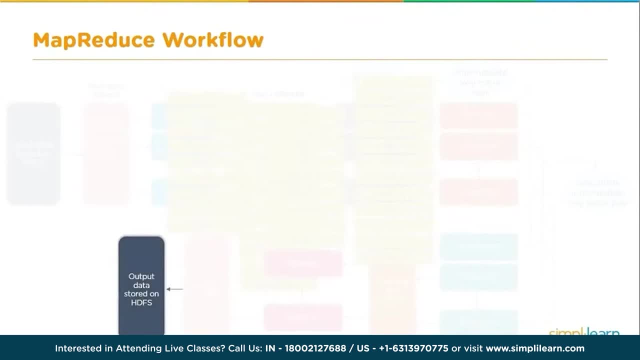 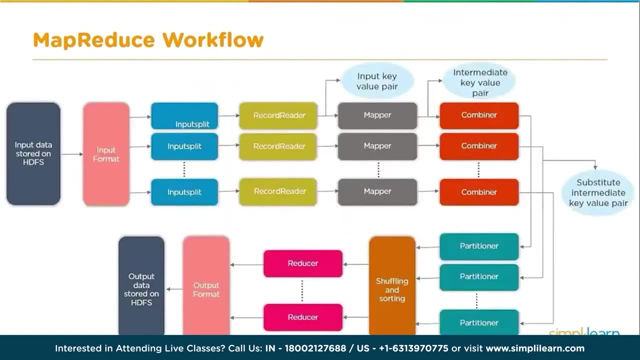 can be not only stored but then read or accessed from SDFS, or even used as an input for further map reduce kind of processing. so this is how it overall looks. so you basically have your data stored on SDFS. based on input format, you have the splits, then 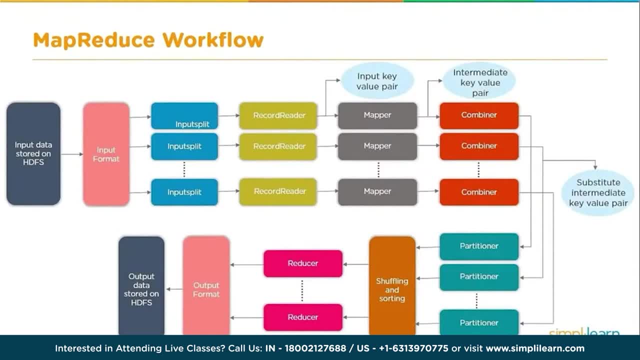 you have record reader, which gives your data to the mapping phase, which is then taken care by your mapper function, and mapper function basically means one or multiple map tasks working on your channel. you could have chunks of data. you could have a combiner phase, which is optional. 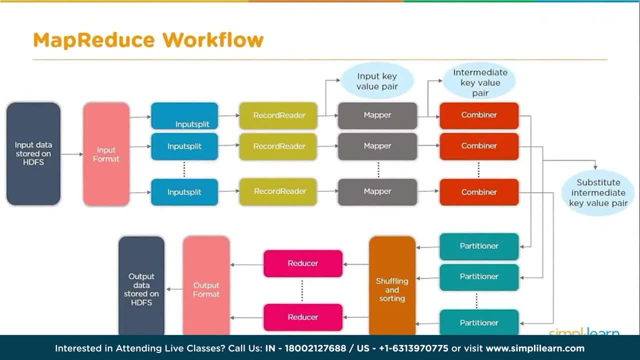 which is not mandatory. then you have a partitioner phase which decides on how many reduce tasks or how many reducers would be used to work on your data. internally, there is sorting and shuffling of data happening and then, basically, based on your output format, your record reader. 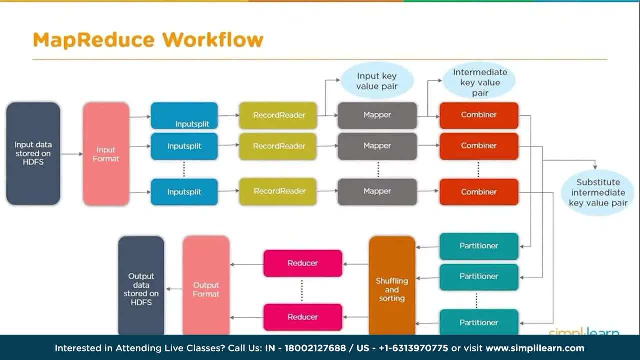 will write the output to SDFS directory now internally. you could also remember that data is being stored locally, so you would have the output of each task which is being worked upon stored locally. however, we do not access the data directly from data nodes. we access it from: 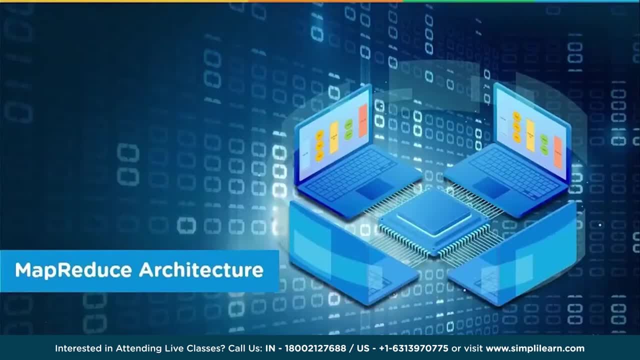 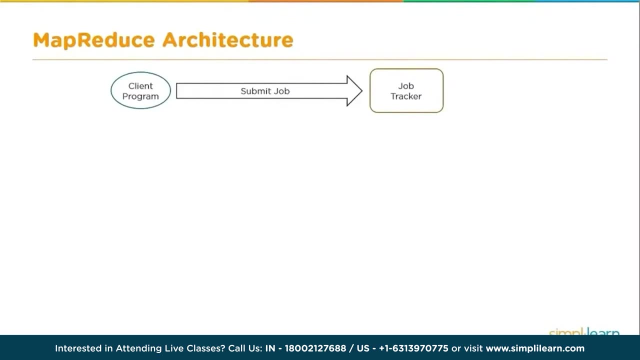 SDFS, so our output is stored on SDFS. so that is your MapReduce workflow. when you talk about MapReduce architecture, now, this is how it would look. so you would have basically edge node or a client program or an API which intends to process some data. so it 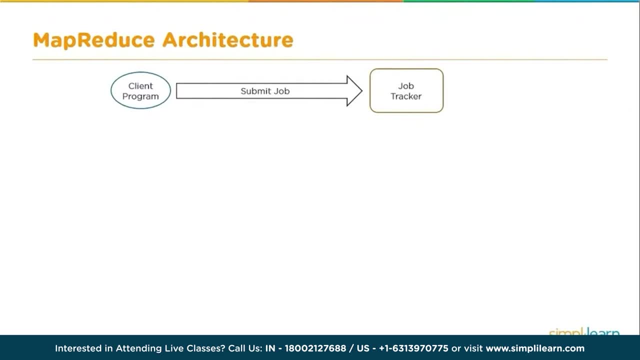 submits the job to the job tracker so you can say: resource manager in case of Hadoop yarn framework. right now, before this step, we can also say that an interaction with name node would have already happened, which would have given information of data nodes which have the relevant. 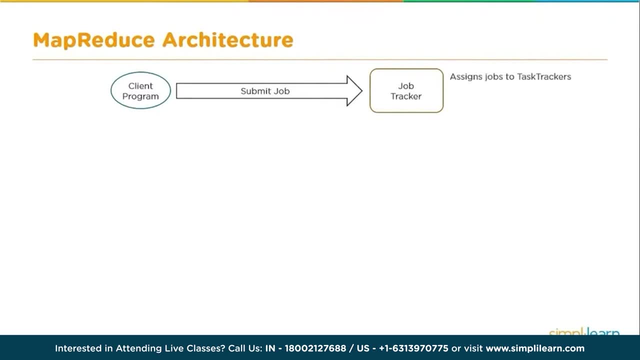 data stored, then your master processor. so in Hadoop version 1 we had job tracker and then the slaves were called task trackers. in Hadoop version 2, instead of job tracker, you have resource manager instead of task trackers. so basically, your resource manager has to assign the 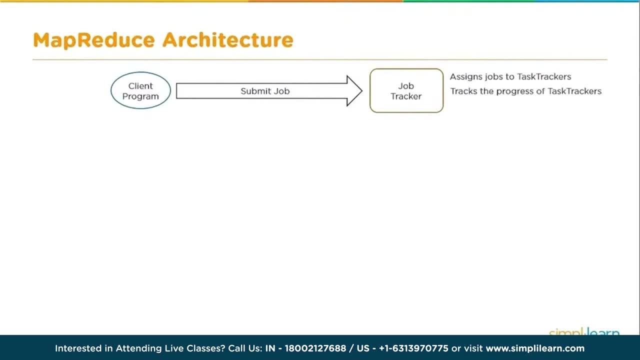 job to the task trackers or node managers. so your node managers, as we discussed in yarn, are basically taking care of processing, which happens on every node. so internally there is all of this work happening by resource manager, node managers and application master. then you can refer to the yarn based 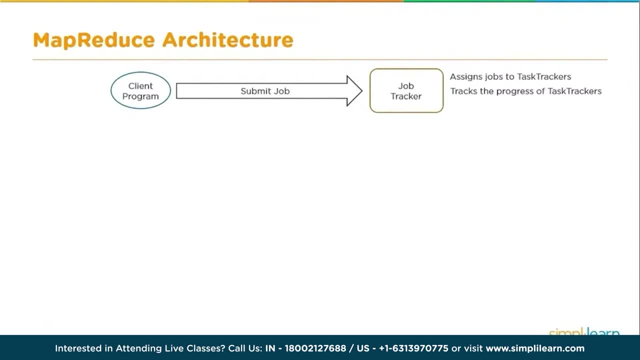 tutorial to understand more about that. so here your processing master is basically breaking down your task trackers and application, breaking down the application into tasks. what it does internally is, once your application is submitted, your application to be run on yarn processing framework is handled by resource manager. now forget about. 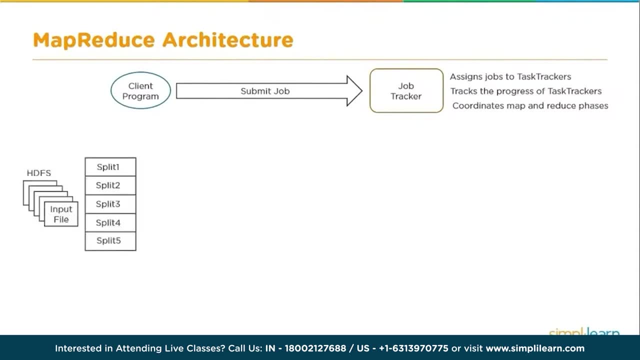 the yarn part as of now? I mean, who does the negotiating of resources? who allocates them? how does the processing happen on the nodes right? so that's all to do with how yarn handles the processing request. so you have your data, which is stored in its DFS, broken. 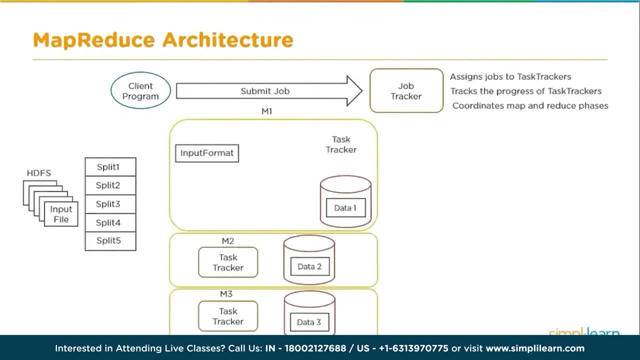 down into one or multiple splits, depending on the input format which has been specified by the developer. your input splits are to be worked upon by your one or multiple map tasks, which will be running within the container on the nodes. basically, you have the resources which are being utilized. 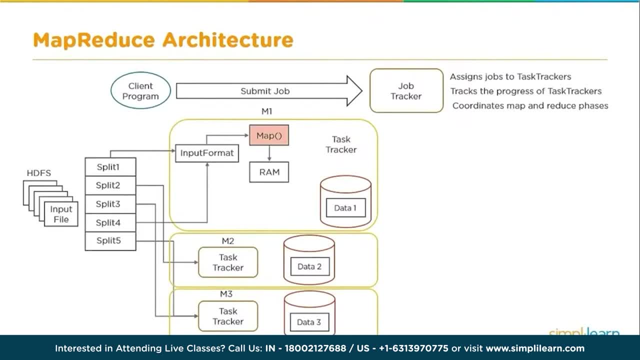 so for each map task you would have some amount of RAM which will be utilized, and then further the same data which has to go through reducing phase. that is, your reduce task will also be utilizing some RAM and CPU cores. now, internally you have these functions which take care of. 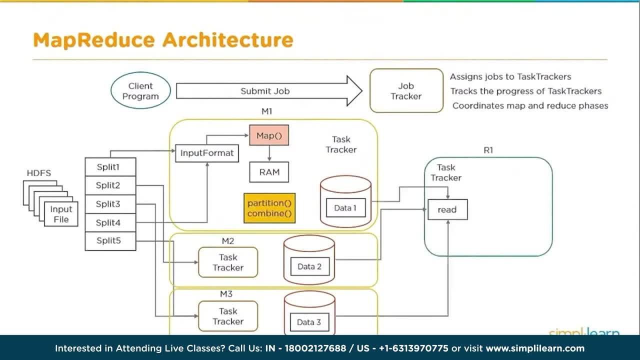 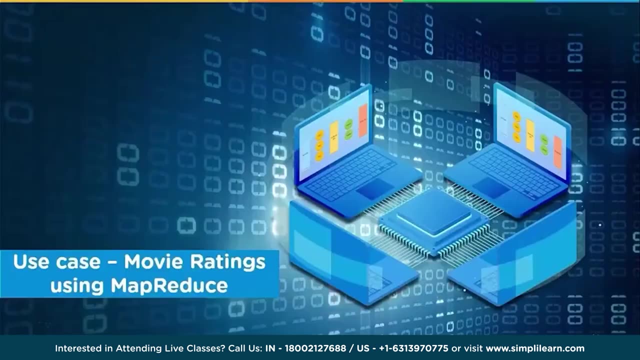 deciding on number of reducers, doing a mini reduce and basically reading and processing the data from multiple data nodes. now this is how your map reduce programming model makes parallel processing work or processes your data, which is stored across multiple machines. finally, you have your output, which is getting stored. 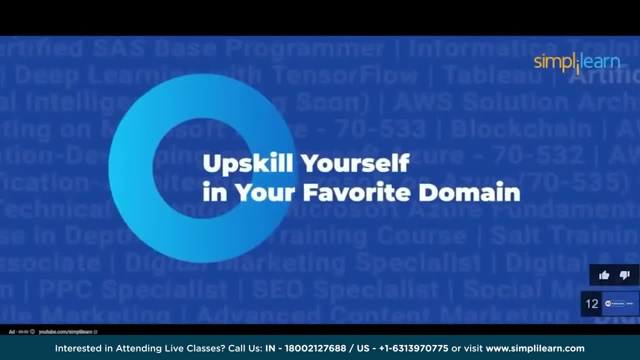 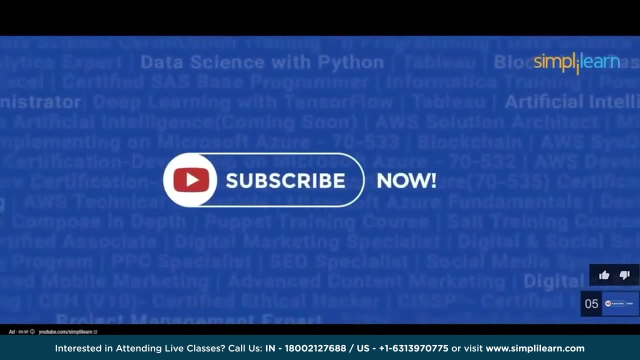 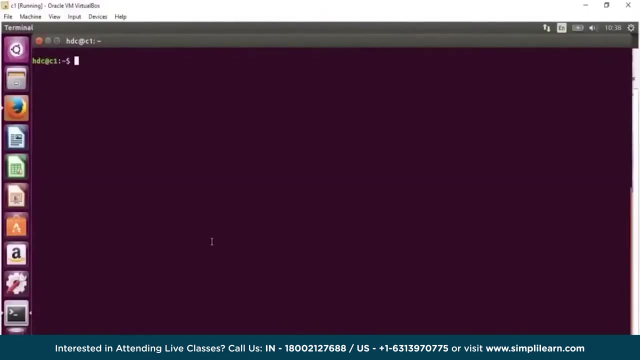 on its DFS. so let's have a quick demo on map reduce and see how it works on a Hadoop cluster. now we have discussed briefly about map reduce, which contains mainly two phases, that is, your mapping phase and your reducing phase, and mapping phase is taken care by 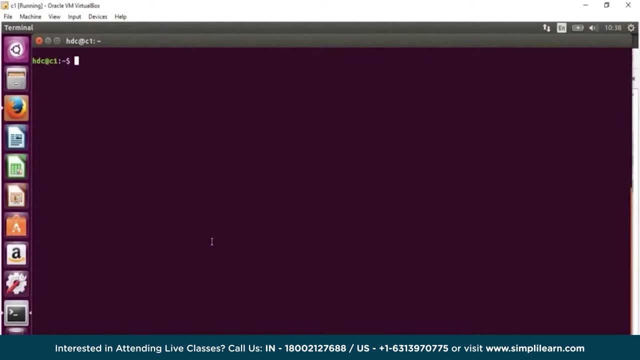 your mapper function and your reducing phase is taken care by your reducer function. now, in between, we also have sorting and shuffling, and then you have other phases, which is partitioner and combiner, and we will discuss about all those in detail in later sessions. but let's have a 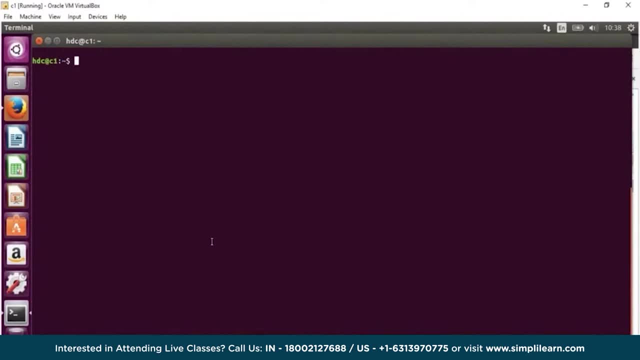 quick demo on how we can run a map reduce, which is already existing as a package jar file within your Apache Hadoop cluster or even in your cloud data cluster. so let's have a quick demo on how we can run a map reduce in our cloud data cluster. 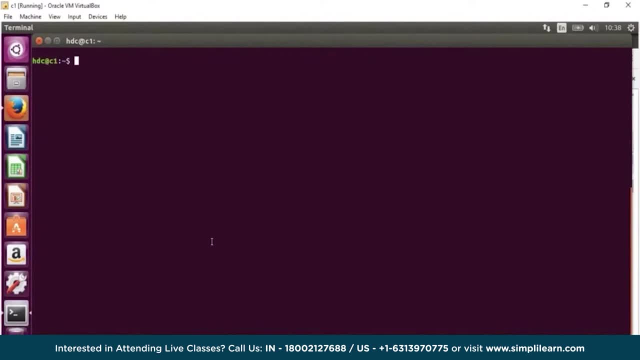 now we can build our own map reduce programs. we can package them as jar, transfer them to the cluster and then run it on a Hadoop cluster on yarn, or we could be using already provided default program. so let's see where they are now. these are my. 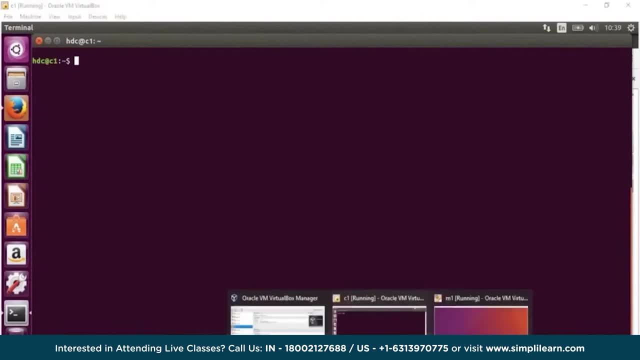 two machines which I have brought up and basically this would have my Apache Hadoop cluster running. now we can just do a simple start hyphen, all dot sh. now I know that this script is deprecated, so we can just run it and it says: instead use start. 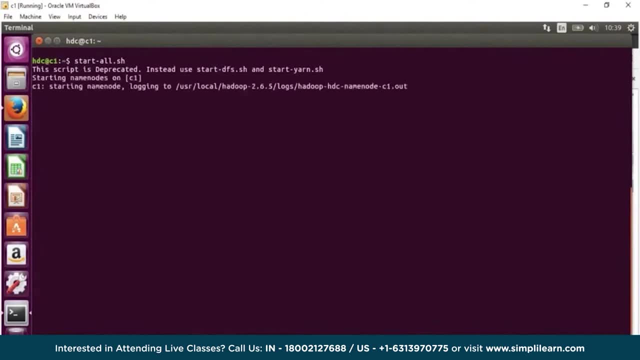 DFS and start yarn, but then it will still take care of starting off my cluster on these two nodes where I would have one single name node, two data nodes, one secondary name node, one resource manager and two node managers. now, if you have any doubt in how this 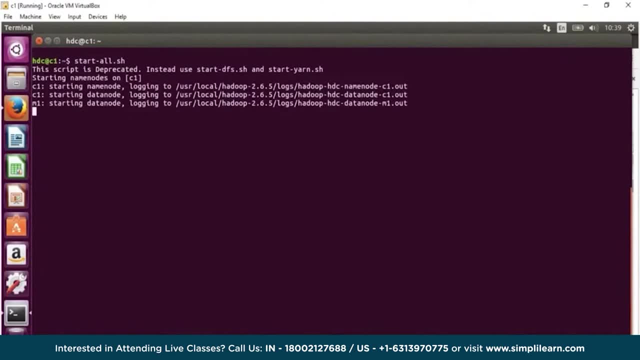 cluster came up. you can always look at the previous sessions where we had a walkthrough in setting up a cluster on Apache, and then you could also have your cluster running using the same structure that we had in the previous session. so you could have less than 3 GB of. 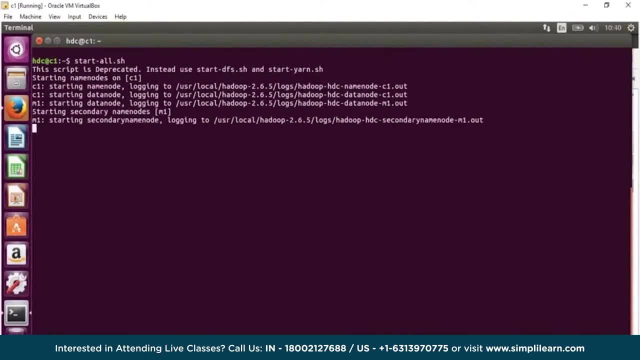 your total machine RAM and you could have a Apache cluster running on your machine. now, once this cluster comes up, we will also have a look at the web UI which is available for name node and resource manager. now, based on the settings, what we have given, our UIs will show. 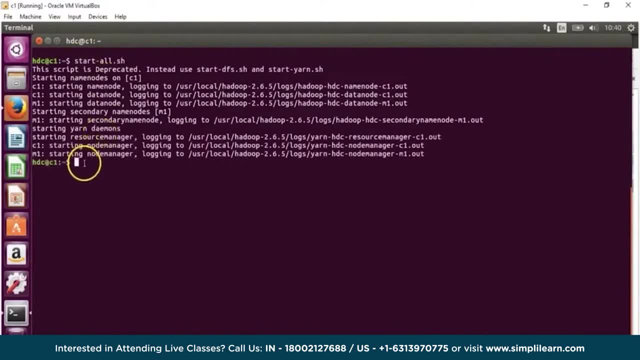 us details of our cluster. but remember, the UI is only to browse. now here my cluster has come up. I can just do a JPS to look at Java related processes and that will show me what are the processes which are running on C1, which is your data. 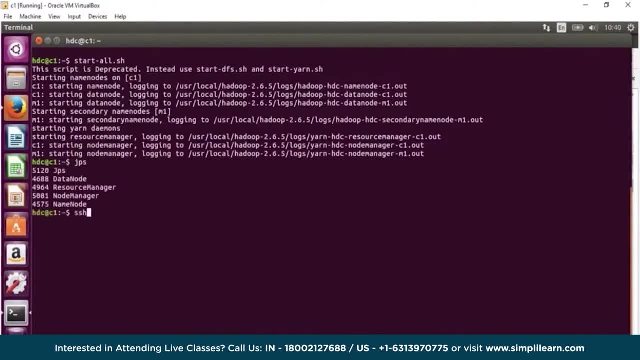 node, resource manager, node manager and name node. and on my M1 machine, which is my second machine which I have configured here, I can always do a JPS and that shows me the processes running. which also means that my cluster is up with two data nodes, with 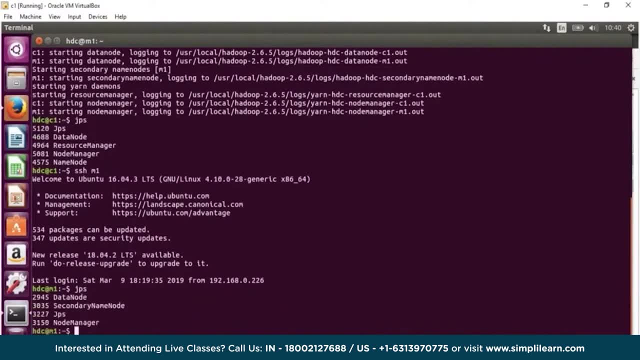 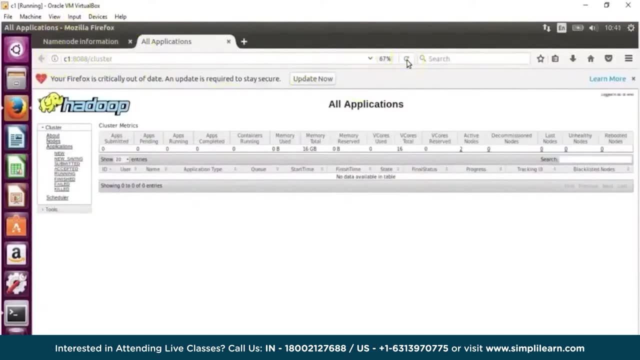 two node managers, and here I can have a look at my web UI, so I can just do a refresh. and the same thing with this one: just do a refresh, and then I can look at my web UI, so I can just do a refresh. and the same thing with: 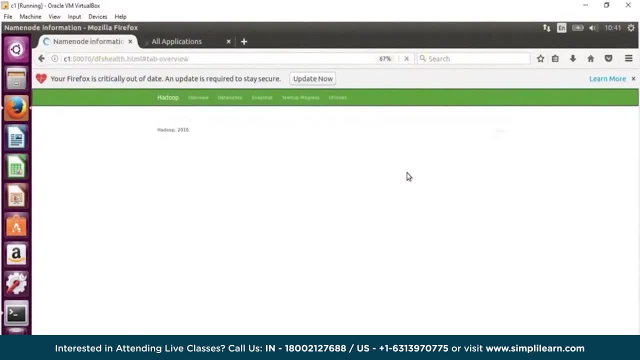 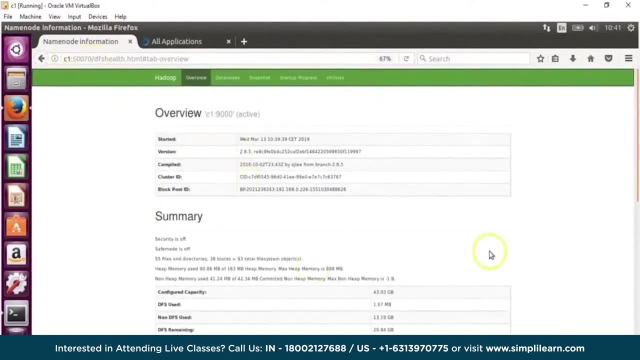 this one just refresh, so I had already opened the web pages. so you can always access the web UI using your name, nodes, host name and 570 port. it tells me what is my cluster ID, what is my block pool ID. it gives you information of what is the space. 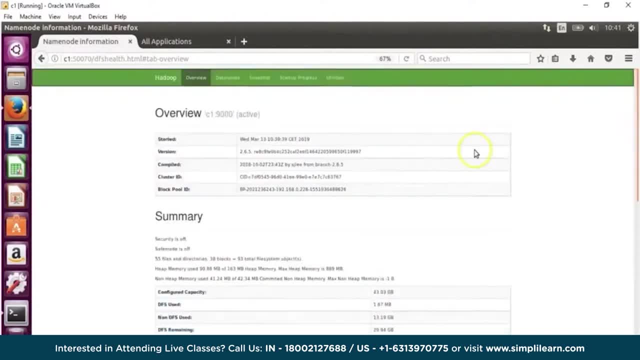 usage, how many live nodes you have, and you can even browse your file system. so I have put in a lot of data here. I can click on browse the file system and this basically shows me multiple directories, and these directories are one or multiple files which we will use for our 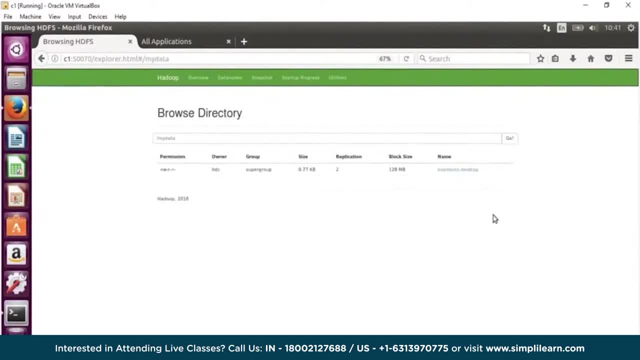 MapReduce example. now, if you see, here these are my directories which have some sample files, although these files are very small, like 8.7 kilobytes, if you look into this directory, if you look into this, I have just pulled in some of my Hadoop logs and 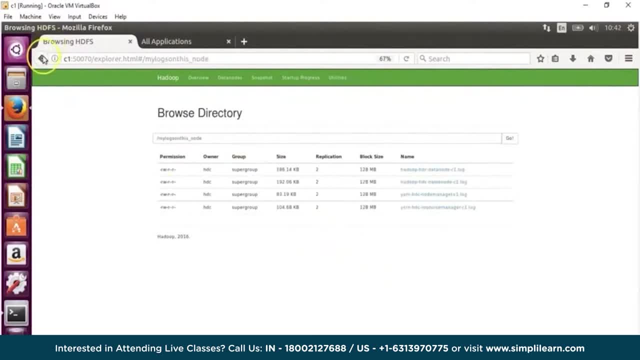 I have put it on my SDFS. these are a little bigger files, and then we also have some other data which we can see here, and this is data which I have downloaded from web. now we can either run it from the MapReduce on a single file or in a. 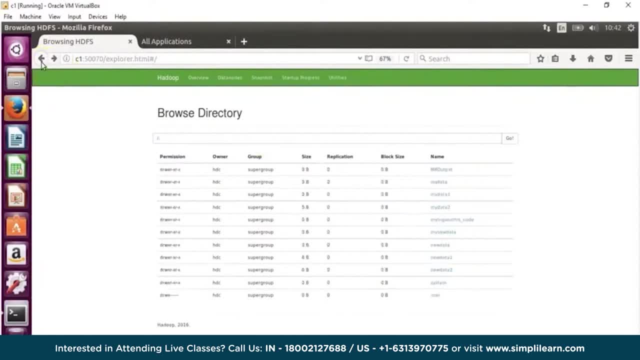 directory which contains multiple files. let's look at that before looking a demo on MapReduce. also remember, MapReduce will create a output directory and we need to have that directory created. plus, we need to have the permissions to run the MapReduce job. so by default, since I 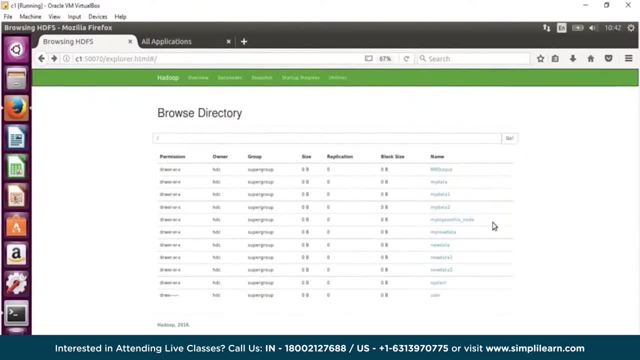 am running it using admin ID, I should not have any problem. but then if you intend to run MapReduce with a different user, then obviously you will have to ask the admin ID to run the MapReduce or you will have to give the user permission to read and write. 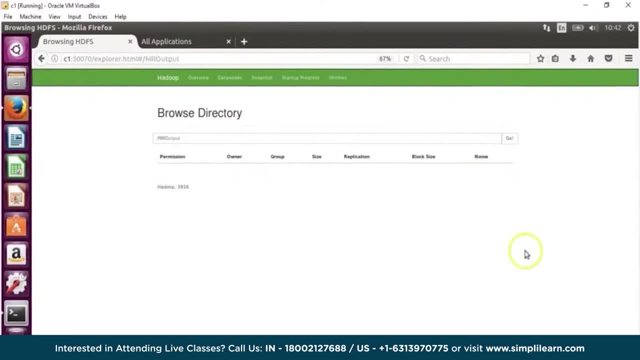 from SDFS. so this is the directory which I have created, which will contain my output once the MapReduce job finishes, and this is my cluster file system. if you look on this UI, this shows me about my yarn, which is available for taking care of any processing. 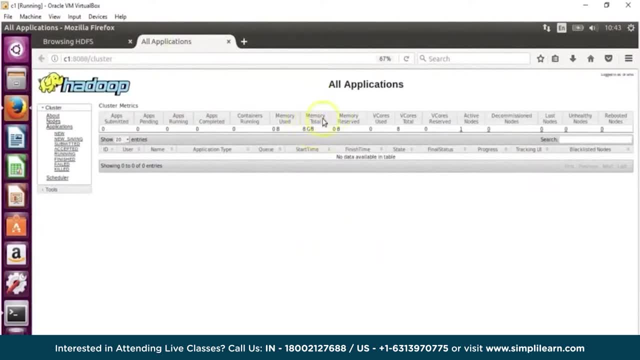 it as of now shows that I have total of 8 GB memory and I have 8 V cores. now that can be depending on what kind of configuration we have set or how many nodes are available. we can look at nodes which are available and that shows me I. 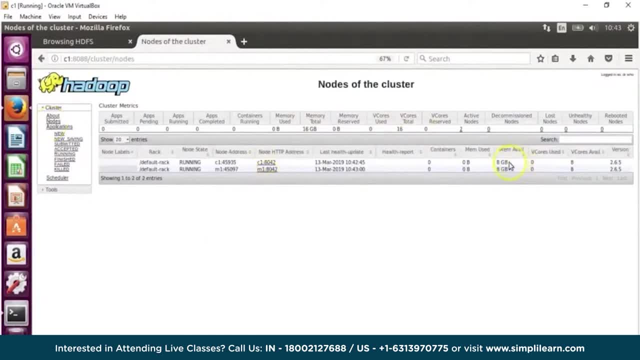 have 2 node managers running, each has 8 GB memory and 8 V cores. now, that's not true actually, but then we have not set the configurations for node managers and that's why it takes the default properties, that is, 8 GB RAM and 8 V cores. 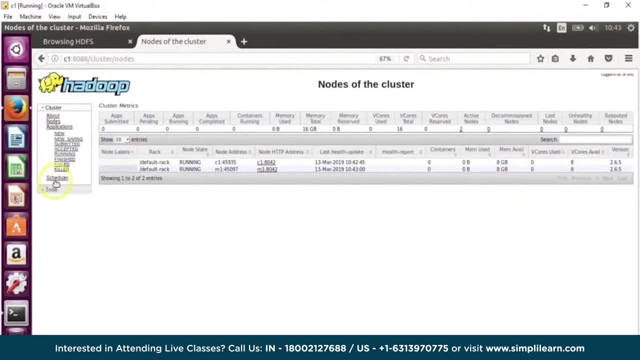 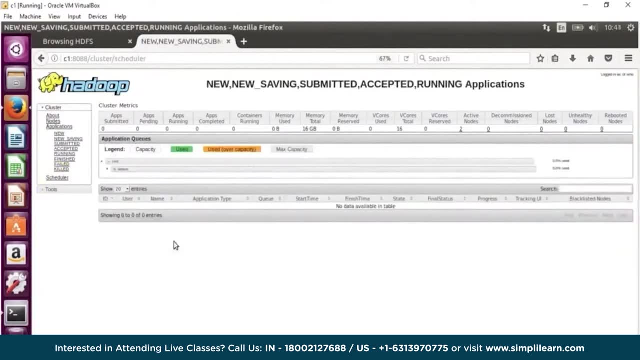 now, this is my yarn UI. we can also look at scheduler, which basically shows me the different queues, if they have been configured, and configured where you will have to run the jobs. we'll discuss about all these in later in detail. now let's go back to our 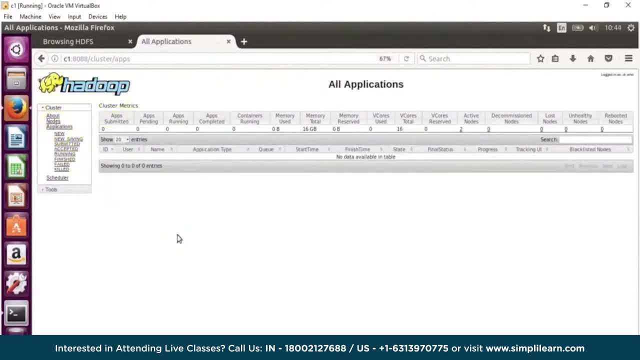 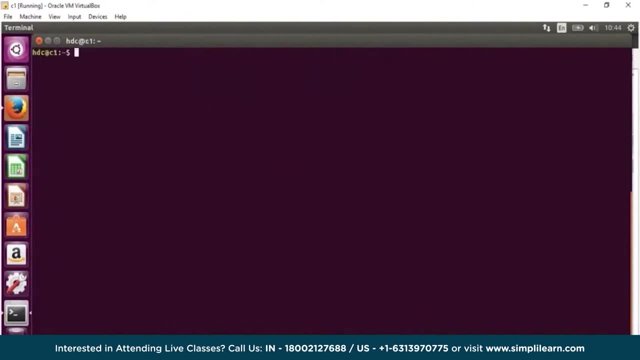 terminal and let's see where we can find some sample applications which we can run on the cluster. so once I go to the terminal I can well submit the MapReduce job from any terminal. now here I know that my Hadoop related directory is here and within. 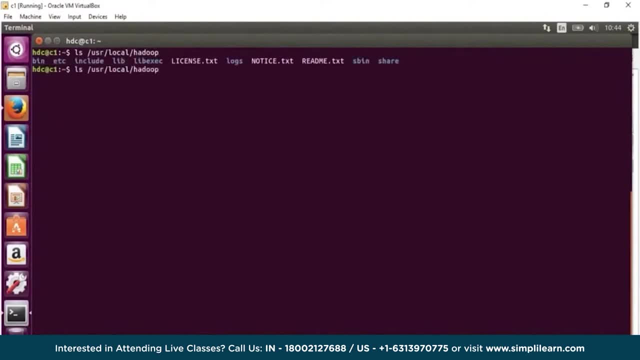 Hadoop. you have various directories. we have discussed that. in binaries you have the commands and then you can run the commands which you can run in sbin. you basically have the startup scripts and here you also notice there is a share directory in the end. if you look in the 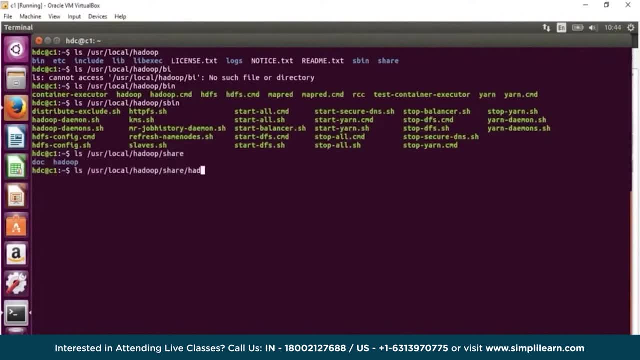 shared directory you would find Hadoop, and within Hadoop you have various sub directories in which we will look for MapReduce. now this MapReduce directory has some sample jar files which we can use to run a MapReduce on the cluster. similarly, if you are working on a 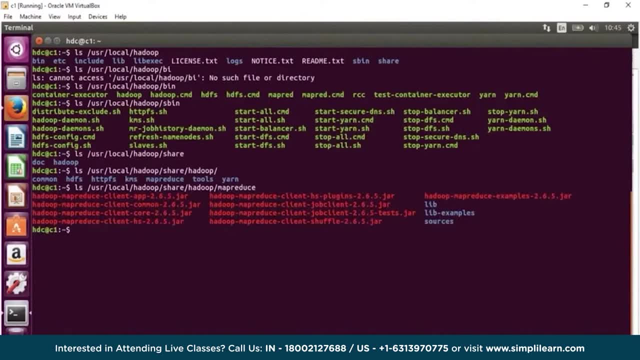 Cloudera cluster. you would have to go into the MapReduce directory and you can have to go into opt cloudera parcels, cdh slash lib and in that you would have directories for sdfs MapReduce or sdfs yarn, where you can still find the 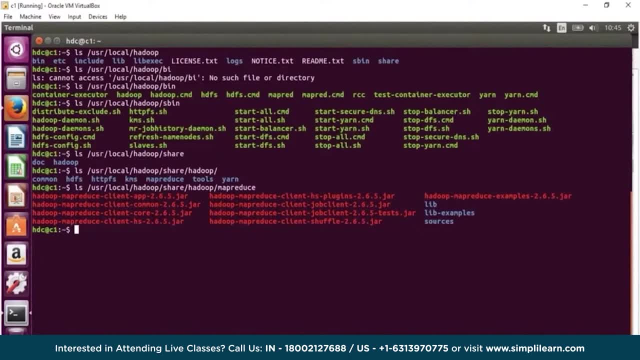 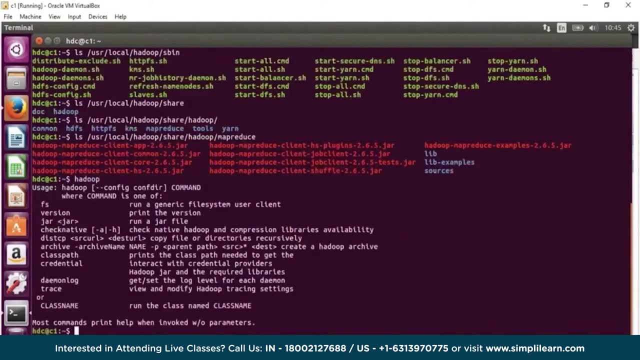 same jars. it is basically a package which contains your multiple applications. now how do we run a MapReduce? we can just type in Hadoop and hit enter, and that shows me that I have an option called jar which can be used to run a jar file. now 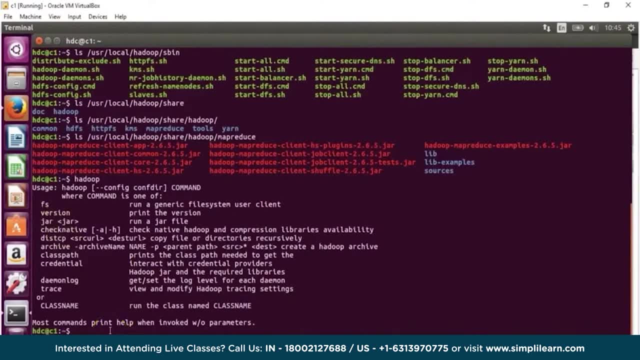 at any point of time. if you would want to see what are the different classes which are available in a particular jar, you could always do a jar minus xvf. for example, I could say jar xvf and I could say user local Hadoop, share Hadoop. 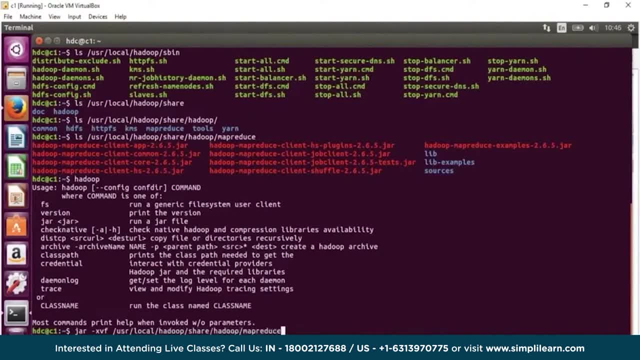 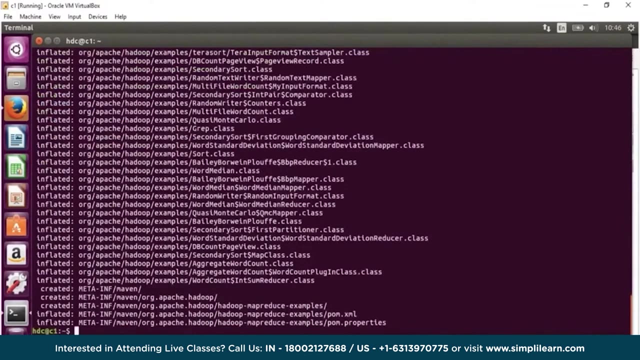 MapReduce and then list down your jar file. so I will say Hadoop, MapReduce examples, and if I do this, this should basically unpack it to show me what classes are available within this particular jar. and it has done this. it has created a meta file and it has. 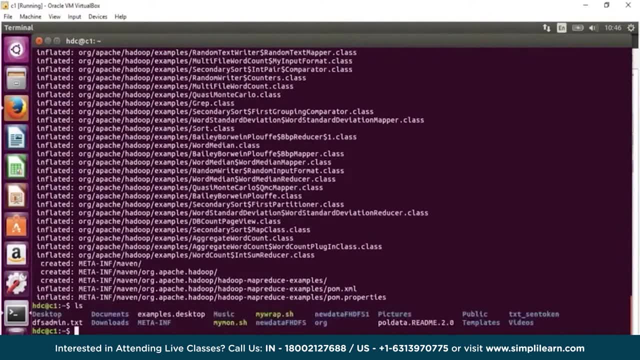 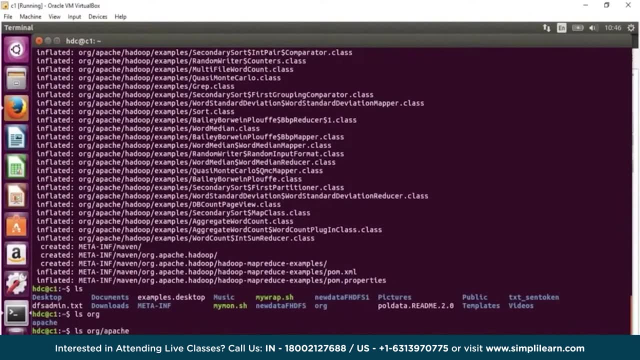 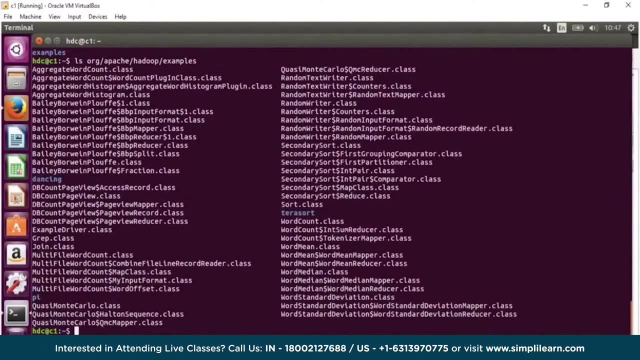 created a org directory. we can see that by doing a ls and here if you look in ls org- since I ran the command from a phone directory, I can look into org patchy Hadoop examples which shows me the classes which I have and those classes contain which. 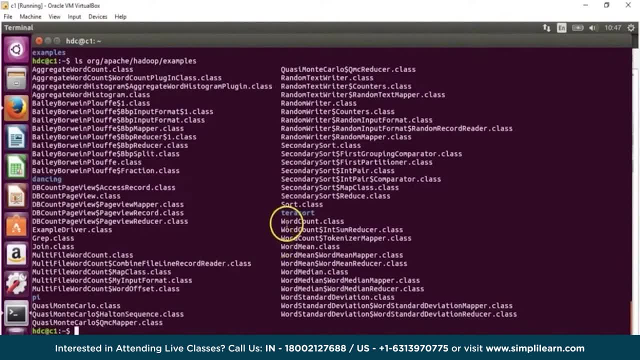 mapper or reducer classes. so it might not be just mapper and reducer but you run a word count program. so, for example, I am targeting to use word count program which does a word count on files and gives me a list of words and how many times they occur. 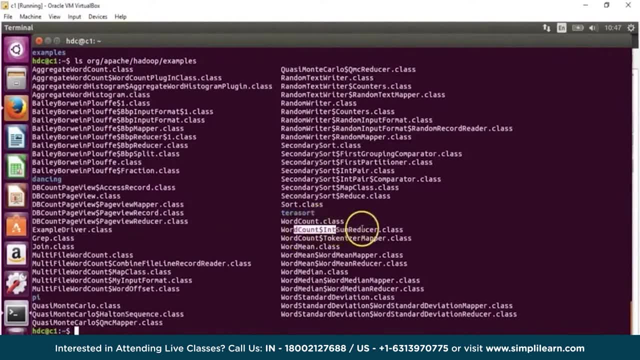 in a particular file or in set of files, and this shows me that what are the classes which belong to word count? so we have a int sum reducer. so this is my reducer class. I have tokenizer mapper, that is my mapper class, right, and basically this is what is used. 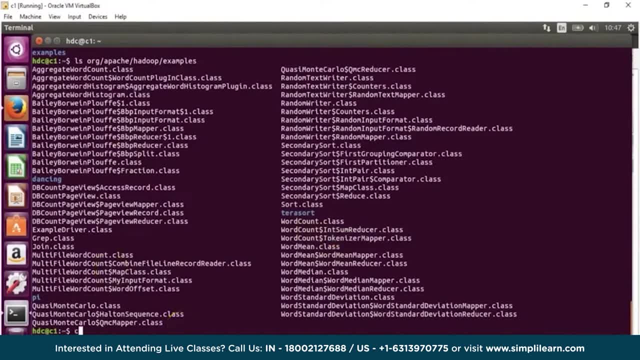 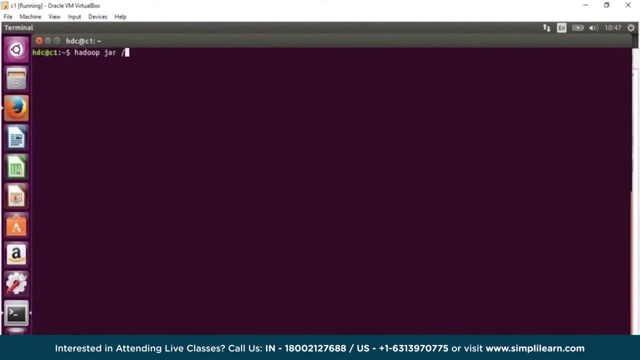 so there are many other programs which are part of this jar file and we can expand and see that. so I can say Hadoop jar and give your path. so I will say Hadoop jar. user: local Hadoop share. Hadoop map reduce. Hadoop map reduce. 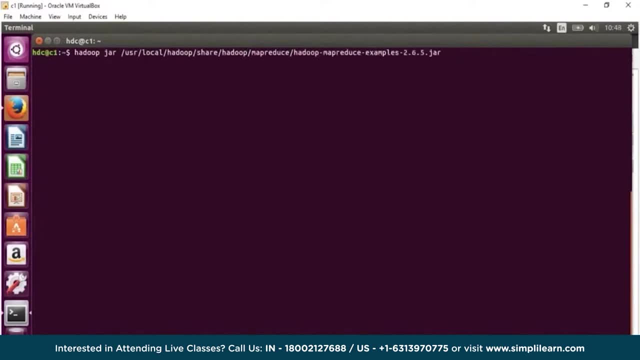 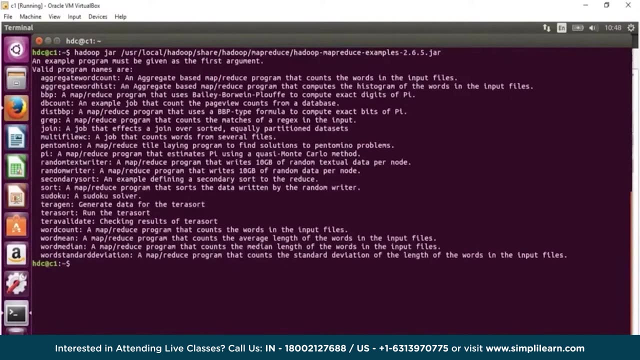 examples and if I hit on enter, that will show me what are the inbuilt classes which are already available now. these are certain things which we can use now. there are other jar files also. for example, I can look at the Hadoop and here we can look at the. 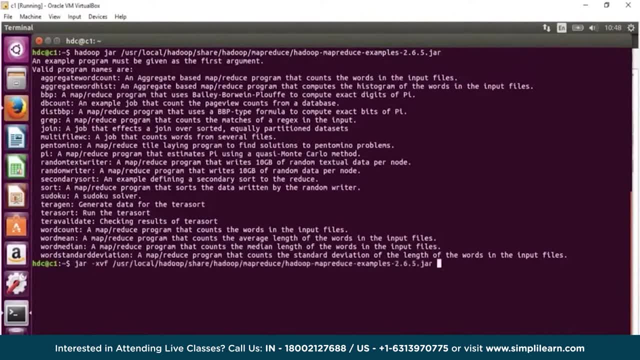 jar files which we have in this particular path. so this is one Hadoop map reduce examples which you can use. you can always look in other jar files, like you can look for Hadoop map reduce, client, job, client, and then you can look at the test one. so 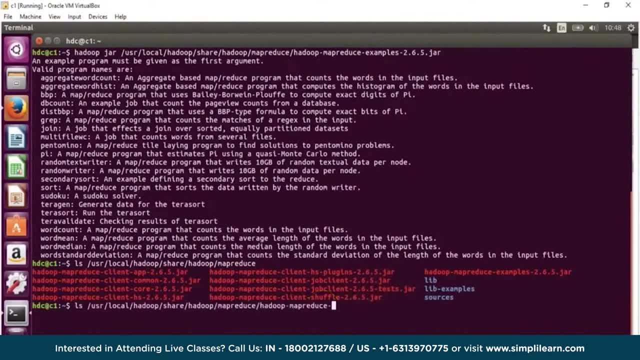 that is also an interesting one. so you can always look into Hadoop map: reduce client, job client, and then you have something ending with this. so if I would have tried this one using my Hadoop jar command- so in my previous example when we did this, it was- 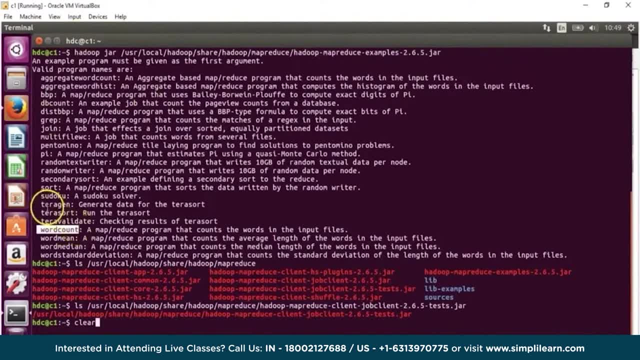 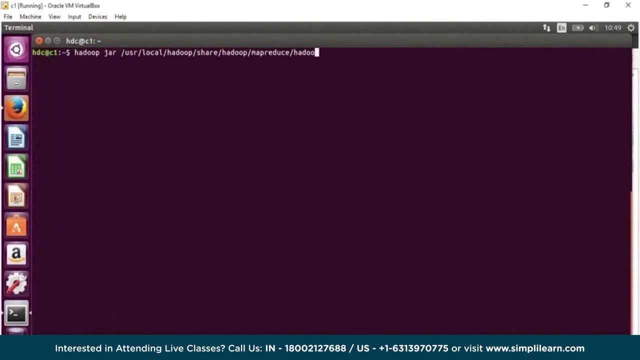 showing me all the classes which are available, and that already has a word count. now there are other good programs which you can try, like TerraGen to generate dummy data, TerraSort to check your sorting performance and so on, and TerraValidate to validate the results. similarly, we can also do a 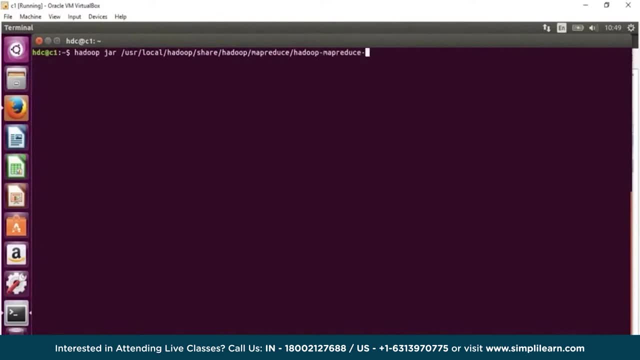 Hadoop jar, as I said on map reduce- I think that was client- and then we have job client and then test jar. now this has a lot of other classes which can be used or programs which can be used for doing a stress, testing or checking your cluster. 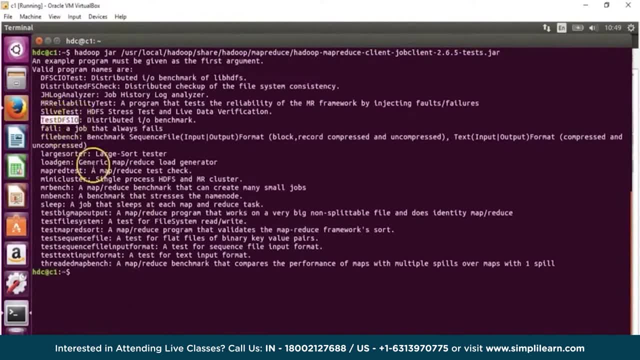 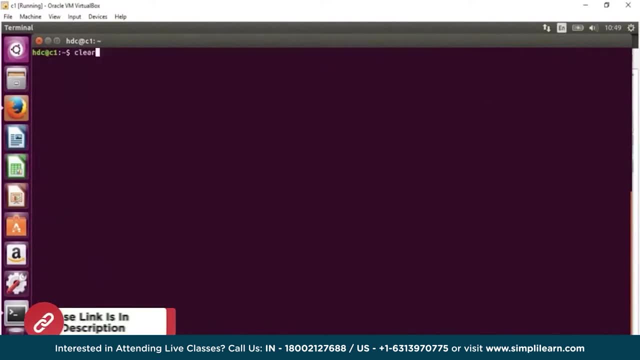 status and so on. one of them- interesting one- is test, the FSIO. but let's not get into all the details. in first instance, let's see how we can run a map reduce. now, if I would want to run a map reduce, I need to give Hadoop. 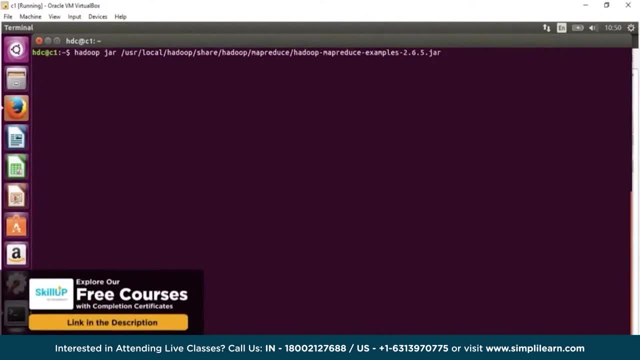 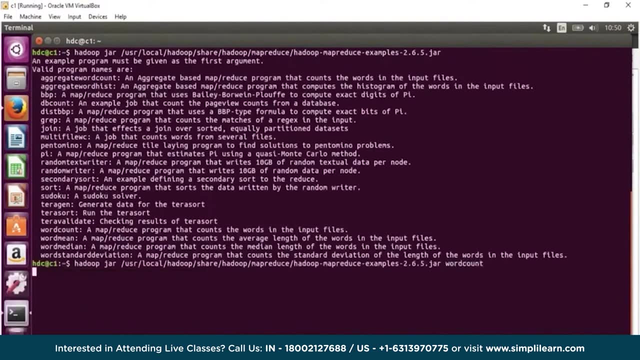 jar and then my jar file, and if I hit on enter it would say it needs the input and output. it needs which class you want to run. so, for example, I would say word count and again if I hit on enter, it tells me that you need to give me. 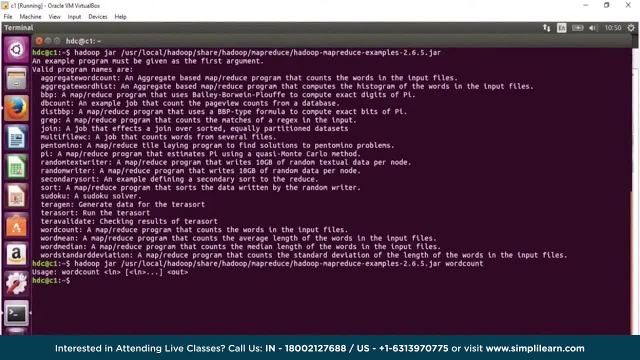 some input and output to process and obviously this processing will be happening on cluster- that is our yarn processing framework, unless and until you would want to run this job in a local mode. so there is a possibility that you can run the job in a local mode. but let's. 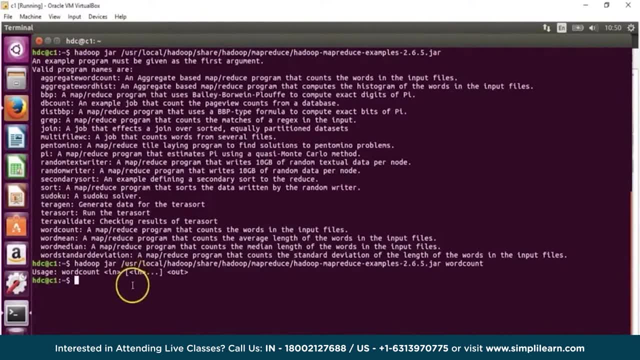 first try how it runs in the cluster. so how do we do that? now, here I can do a HDFS LS slash command to see what I have on my HDFS now through my UI. I was already showing you that we have set of files and directories which 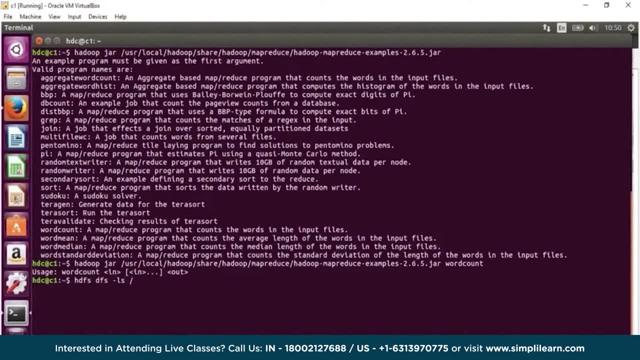 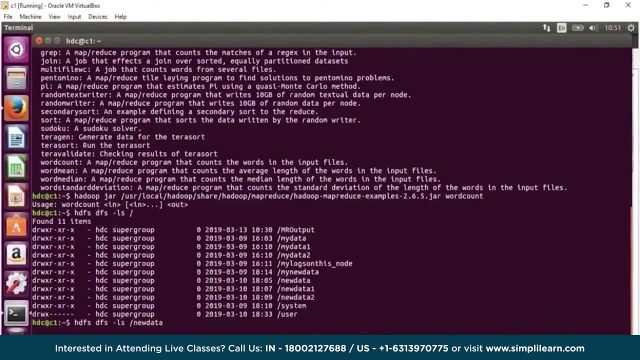 we can use to process. now we can take up one single file. so, for example, if I pick up new data and I can look into the files here, what we have, and we can basically run a map, reduce on a single file or multiple files and we can 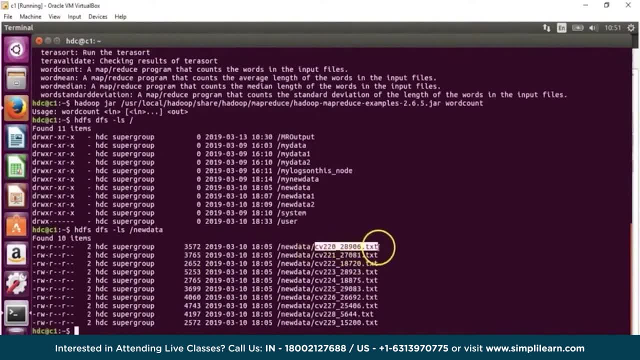 basically run a map, reduce on a single file. so let's take this file, whatever that contains, and I would like to do a word count so that I get a list of words and their occurrence in this file. so let me just copy this now I also need my output. 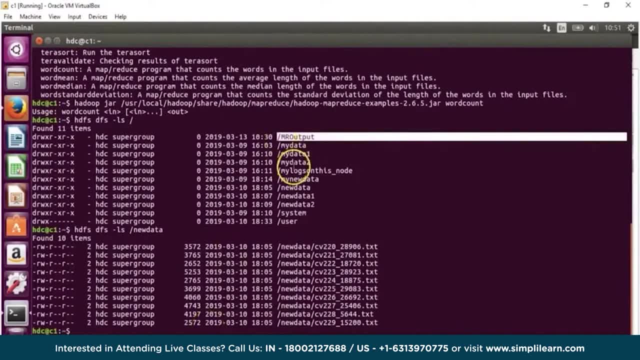 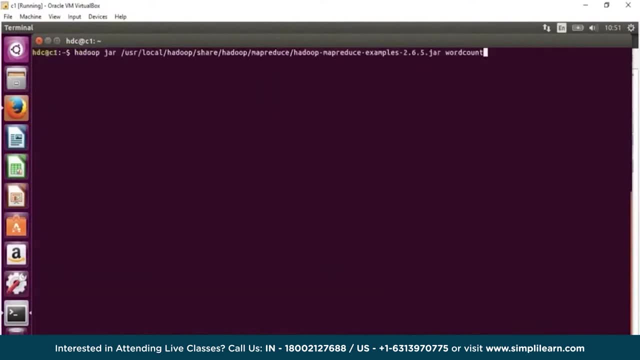 to be written and that will be written here. so here, if I want to run a map reduce, I can say Hadoop, which we can pull out from history, so Hadoop jar word count. now I need to give my input, so that will be new data and 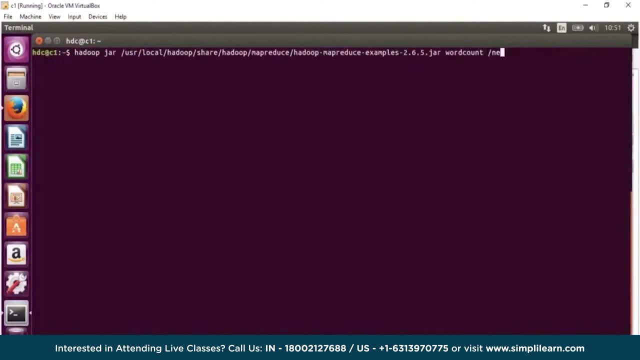 then I will run a map reduce, I can say Hadoop, which we can pull out from history, and then I will give this file which we just copied. now I am going to run the word count on you on a single file and I will basically have my 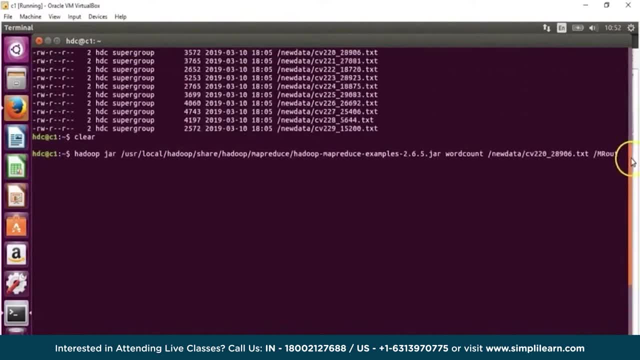 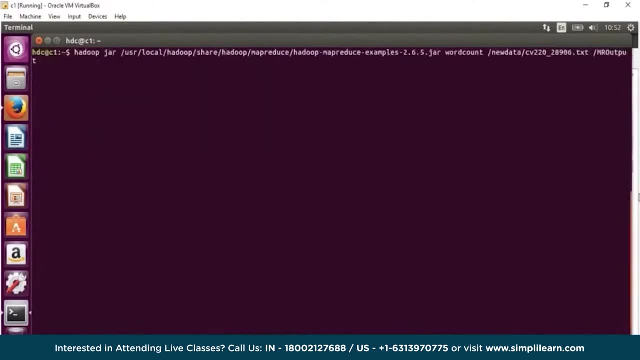 output which will be stored in this directory, the directory which I have created already, mr output. so let's do this output, and this is fair enough. now you can give many other properties. you can specify how many map jobs you want to run, how many reduce jobs you want to. 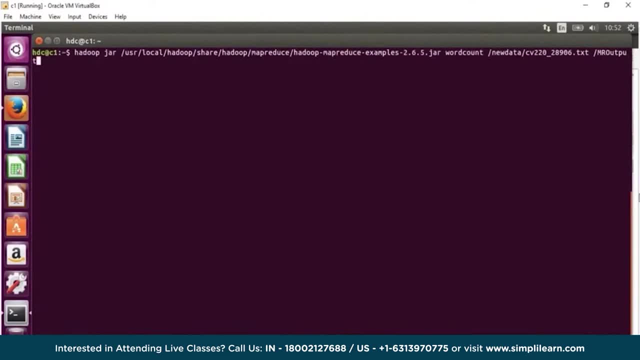 run. do you want your output to be compressed, or you want your output to be merged, or many other properties can be defined when you are specifying word count, and then you can pass in an argument to pass properties from the command line which will affect your output. now, once I go, 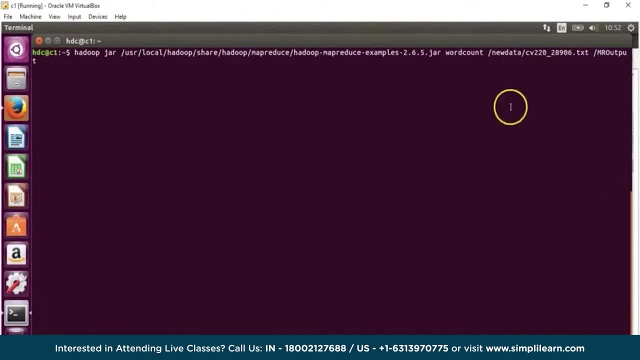 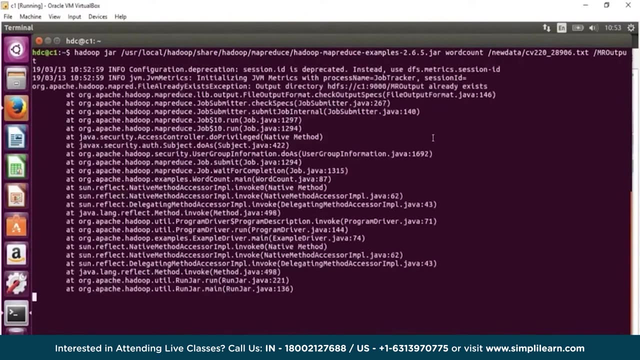 ahead and submit this. this is basically running a simple inbuilt map reduce job on our Hadoop cluster. now, obviously, internally it will be looking for name node. now we have some issue here and it says the output already exists. now what we have to do is to 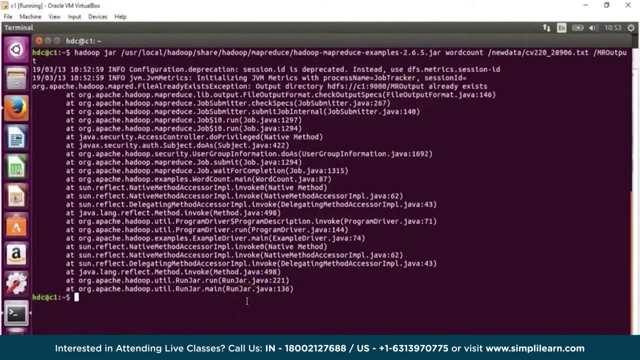 create an output for this. what does that mean? so it basically means that Hadoop will create an output for you. you just need to give a name, but then you don't need to create it. so let's give, let's append the output with number one, and then let's go. 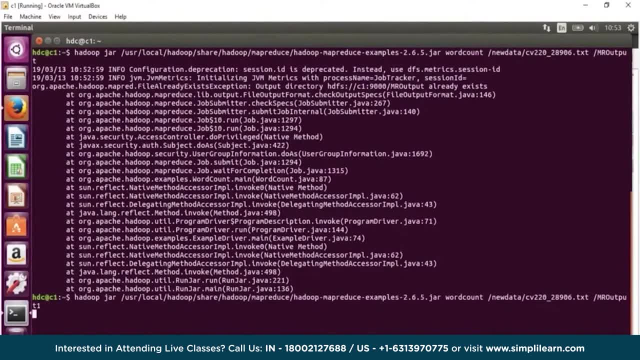 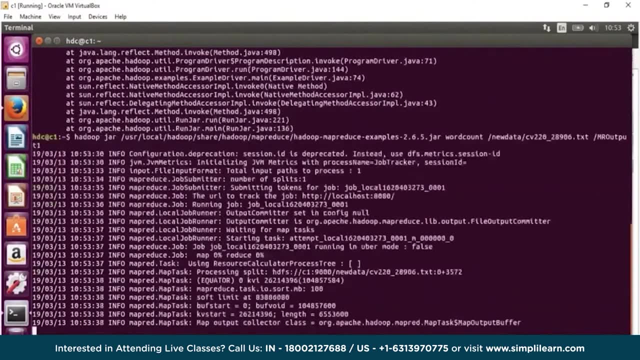 ahead and run this, so I've submitted this command now. this can also be run in background if you would want to run multiple jobs on your cluster at the same time, so it takes total input paths to processes one. so that is, there is only one job of this. 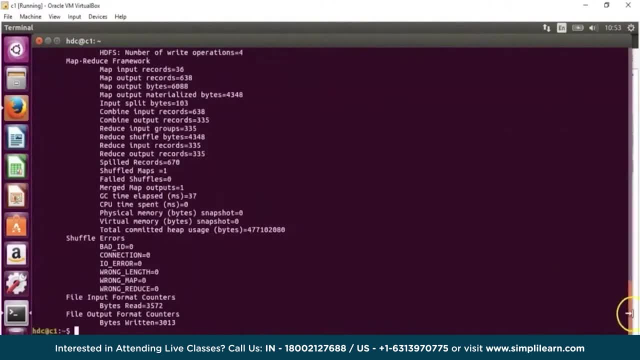 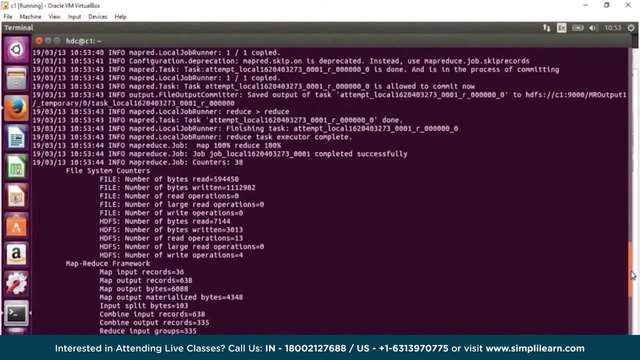 and you can actually try to contact your resource manager and basically this is done. so here we can have a look and we can see some counters here. now, what I also see is for some property which it is missing. it has run the job, but it has run in a 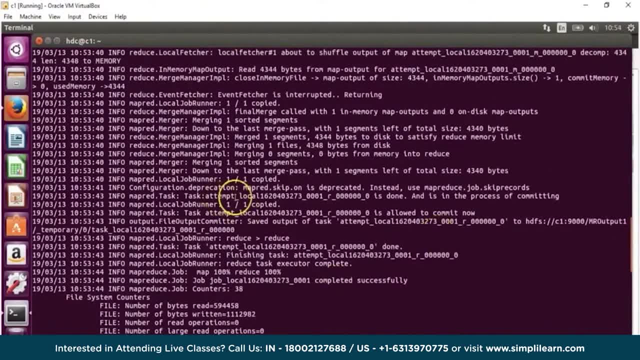 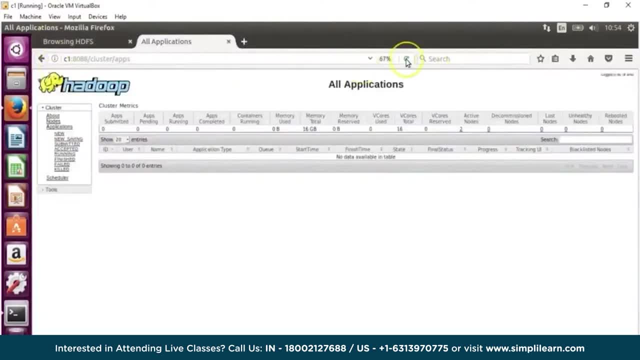 local mode. it has run in a local mode so, although we have submitted, so this might be related to my yarn settings and we can check that. so if I do a refresh when I have run my application, it will show that I have submitted something in my. It has completed. It would have created an output, But the only thing is it did not interact with. 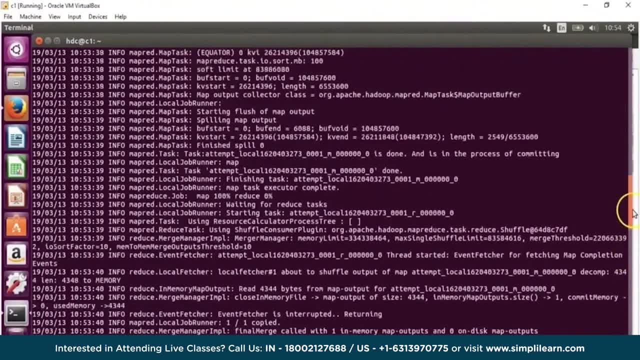 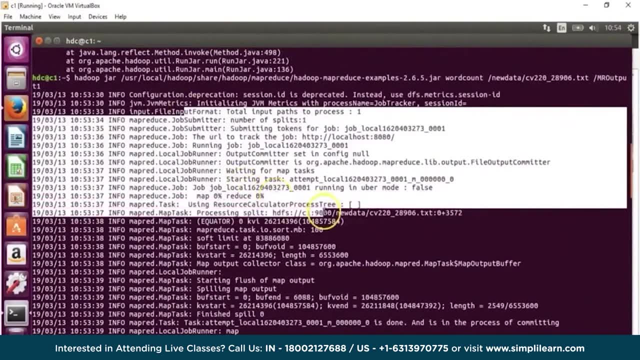 your yarn. It did not interact with your resource manager. We can check those properties And here, if we look into the job, it basically tells me that it went for mapping and reducing It would have created an output. It worked on my file, but then it ran in a local mode. It ran in. 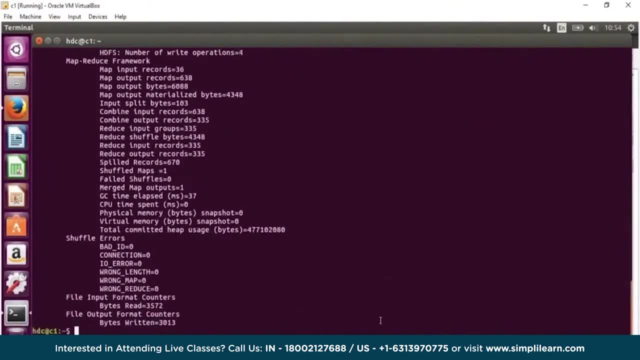 a local mode. So map reduce, remember, is a programming model right Now. if you run it on yarn, you get the facilities of running it on a cluster where yarn takes care of resource management. If you don't run it on yarn and run it on a local mode, it will use your machine's RAM. 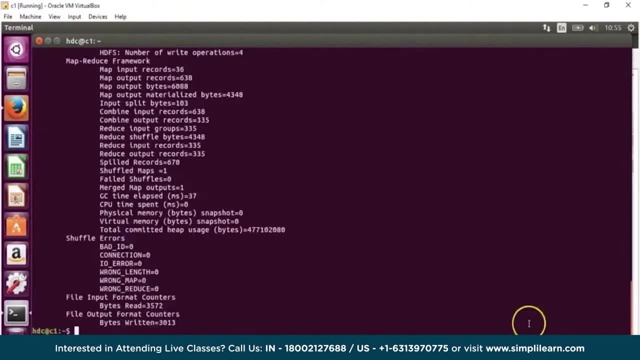 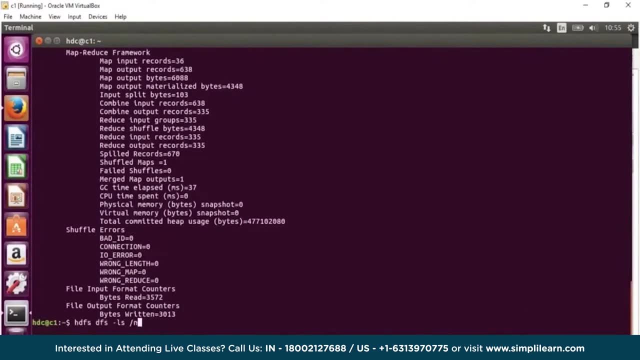 and CPU cores for processing, But then we can quickly look at the output and then we can also try running this on yarn. So if I look into my HDFS and if I look into my output- MR output- that's the directory which was not used. actually, Let's look into the other directory which is 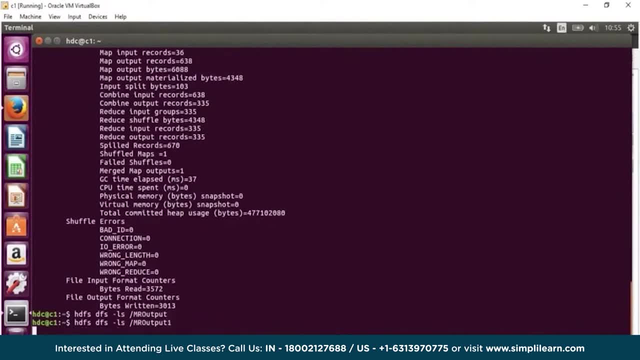 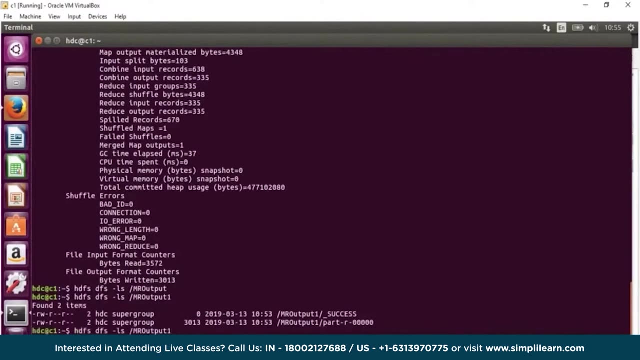 ending And that should show me the output created by this map reduce. Although it ran in a local mode, it fetched an input file from your HDFS and it would have created output in HDFS. Now that's my part file which is created And if you look at part minus R, minus these zeros, 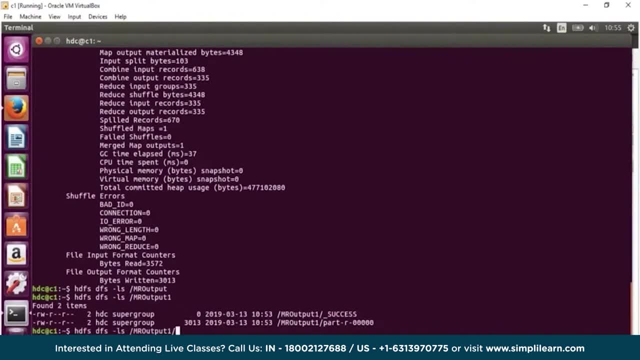 if you would have more than one reducer running, then you would have multiple such files created. We can look into this. What does this file contain which would have my word count, and here I can say cat, which basically shows me what is the output created by my MapReduce. 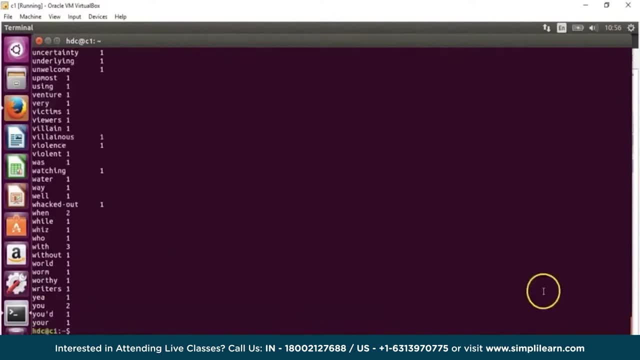 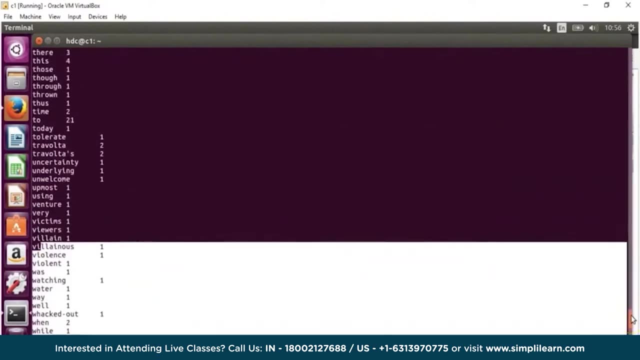 Let's have a look into this. So the file which we gave for processing has been broken down and now we have the list of words which occur in the file plus a count of those words. So if there is some word which is in is more, then it shows me the count. So this is a list. 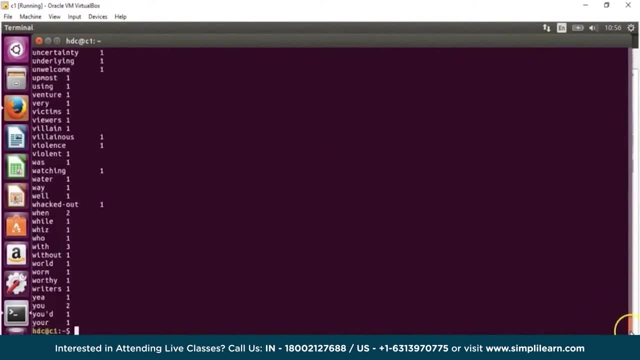 of my words and the count for that. So this is how we run a sample MapReduce job. I will also show you how we can run it on YARN. Now let's run MapReduce on YARN and initially when we tried running a MapReduce it did not hit YARN, but it ran in a local mode and that was. 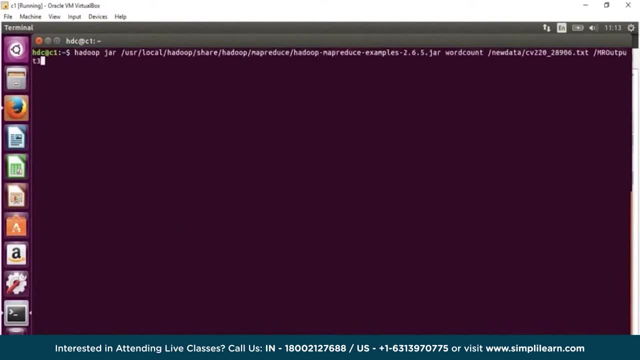 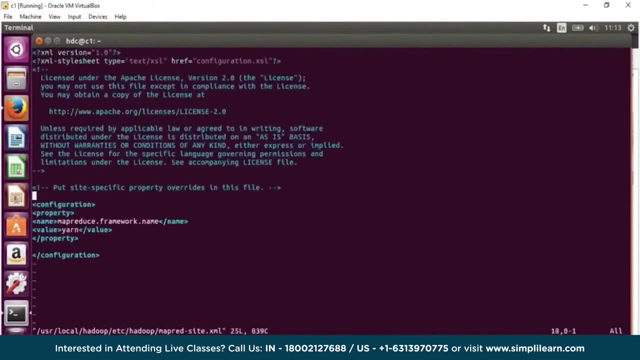 because there was a property which had to be changed in MapReduce-site file. So basically, if you look into this file, the error was that I had given a property which says MapRedframeworkname and that was not the right property name and it was ignored. 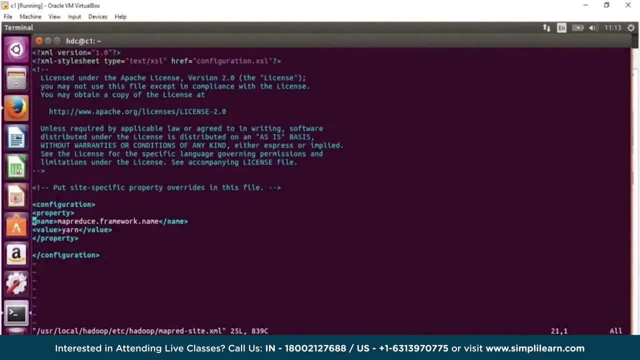 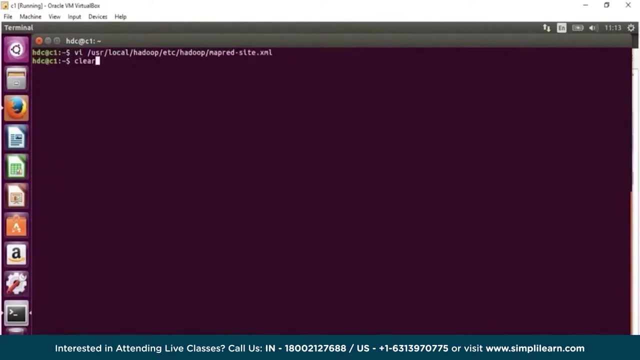 and that's why it ran in a local mode. So I changed the property to MapReduceframeworkname, restarted my cluster and everything should be fine now, and that MapRed-site file has also been copied across the nodes Now to run a MapReduce on a Hadoop cluster, so that 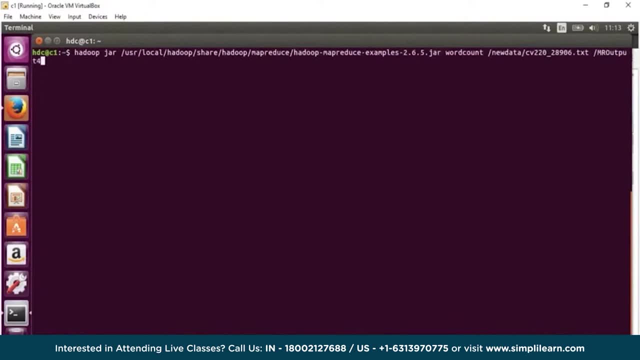 it uses YARN, and YARN takes care of resource allocation on one or multiple machines. So I'm just changing the output here and now I will submit this job, which should first connect to the resource map, And if it connects to the resource manager, that means our job will be run using YARN. 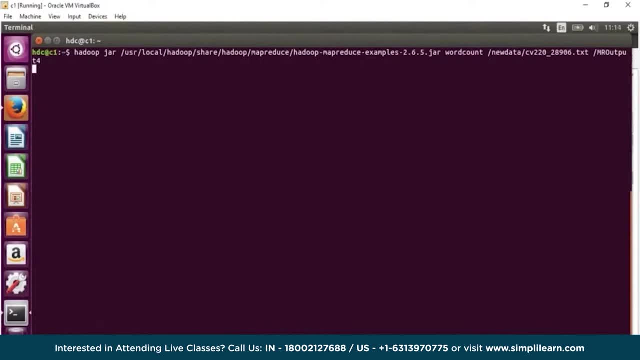 on the cluster rather than in a local mode. So now we have to wait for this application to internally connect to resource manager, and once it starts there, we can always go back to the web UI and check if our application has reached YARN. So it shows me that there. 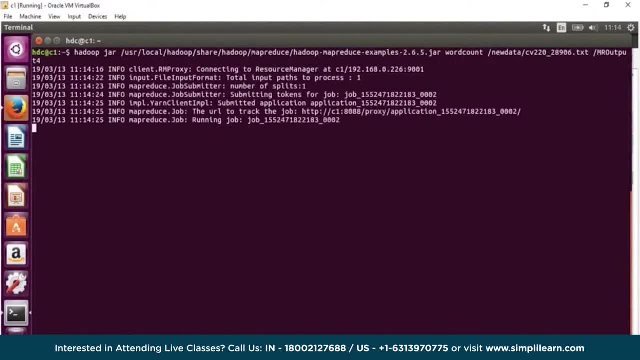 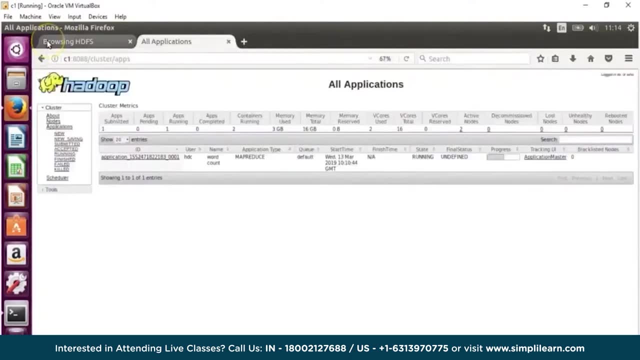 is one input part to be processed. that's my job ID. that's my application ID, which you can even monitor status Now here, the job has been submitted, so let's go back here and just do a refresh on my YARN. 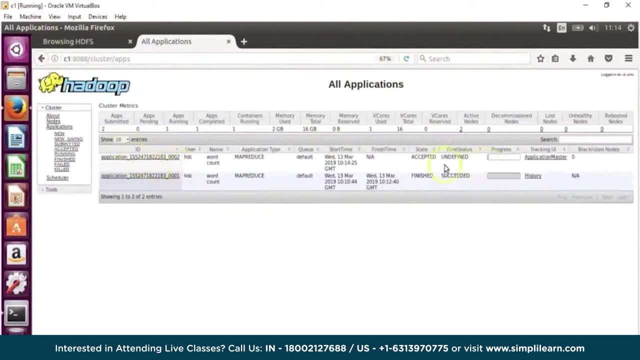 UI, which should show me the new application which is submitted. It tells me that it is in accepted state. application master has already started and if you click on this link, it will also give you more details of how many map and reduce tasks would run. So 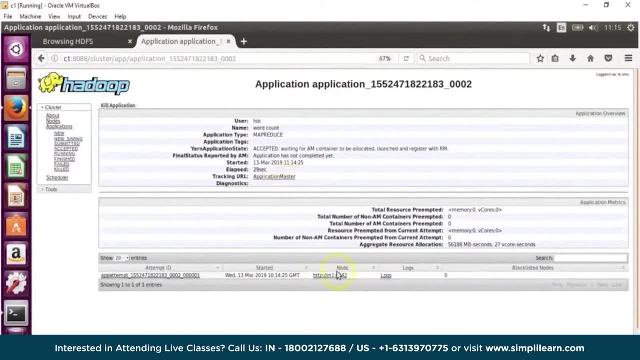 as of now, it says the application master is running. it would be using this node, which is M1.. We can always look into the log and we can see that it's running. and we can always look into the log and we can see that it's running. So, as of now, it says the application master. is running. it would be using this node, which is M1.. We can always look into the log and we can see that it's running. and we can always look into the log and we can see that it's running and we can see that it's running. So, as of now, it says the application master. 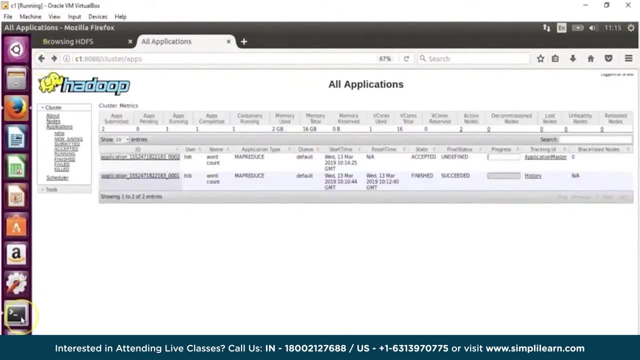 is running and we can always look into the log. and we can always look into the log. we can see that there is a one task attempt which is being made And now, if I go back to my terminal, I will see that it is waiting to get some resources from the cluster And 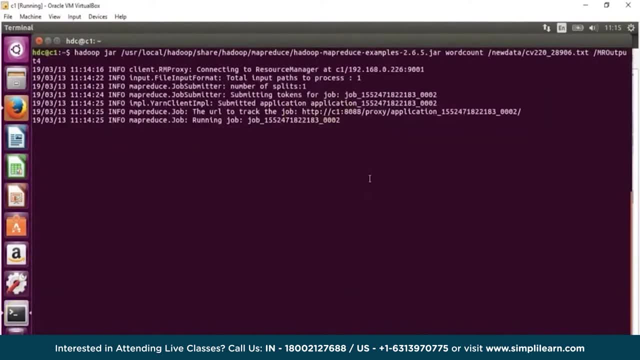 once it gets the resources, it will first start with the mapping phase. where the mapper function runs, it does the map tasks, one or multiple, depending on the splits. So right now we have one file and one split, so we will have just one map task running and once. 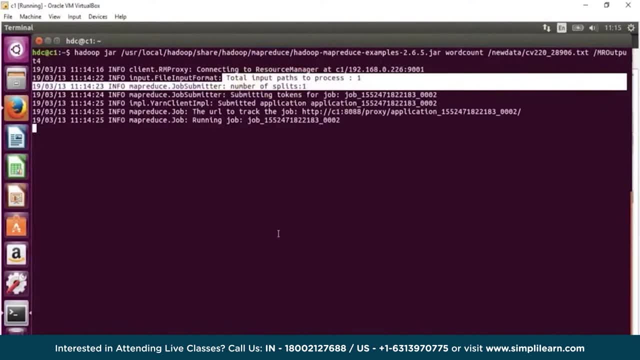 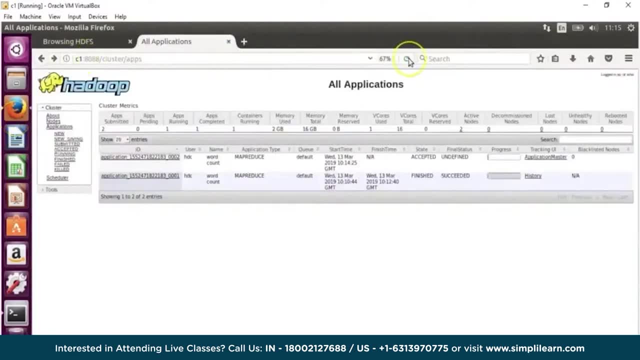 the mapping phase completes, then it will get into the M1. And once it gets the map task running, it will run the mapping phase. And once it gets the map task running, we can now go back into the command and it will say: yes, this is. 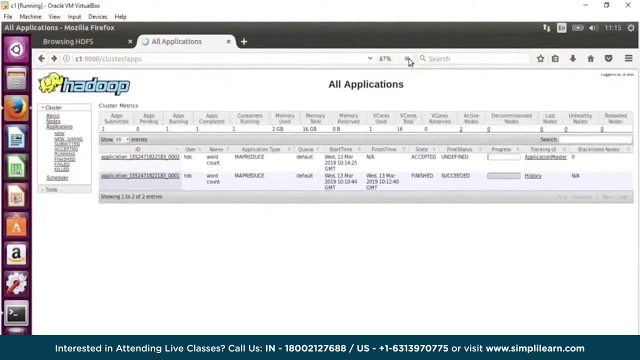 the mapping phase and it will return the map task in the mapper And we can also see that. we can see what the mapping phase has been running. So, for example, if we go to the map tab here, it's already running. Let's say, we want to change the map size to. 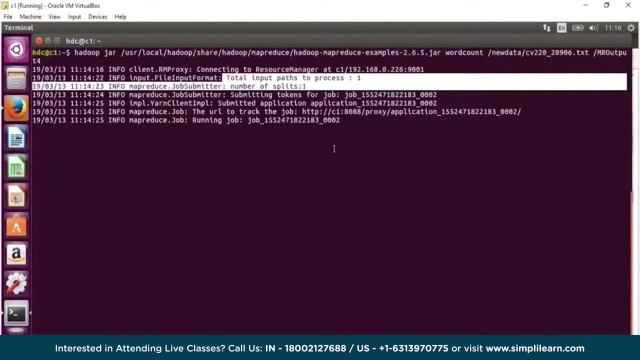 the size of the mapper and we can use that. We can also choose the length of the map, to be possible, and we can choose the length of the map as well. if the resources were used by some other application, they will have to be freed up Now internally. 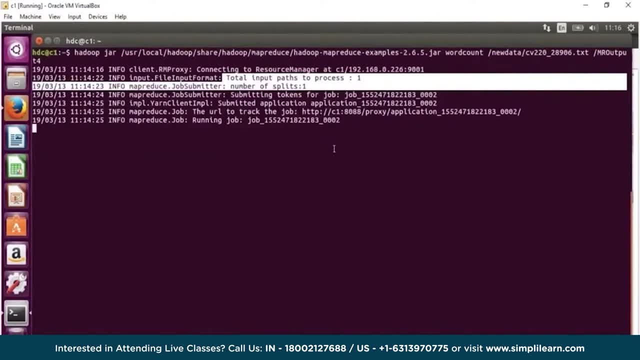 yarn takes care of all that which we will learn more detail in yarn or you might have already followed the yarn based session. Now here we will have to just give it some more time and let's see if my application proceeds. with the resources, what yarn can allocate. 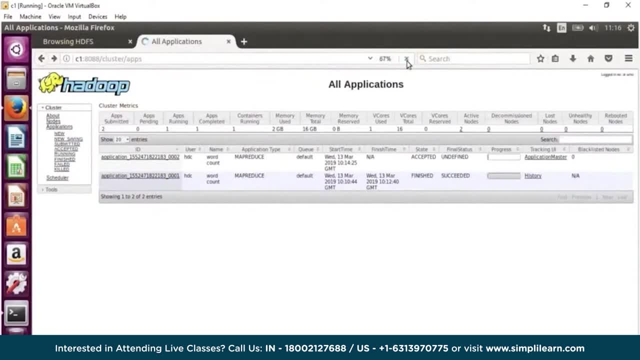 to it. Sometimes you can also see a slowness in what web UI shows up, and that can be related to the amount of memory you have allocated to your nodes. Now for Apache, we can have less amount of memory and we can still run the cluster and, as I said, the memory which 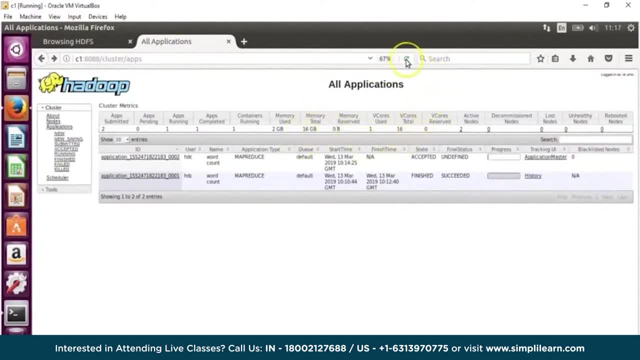 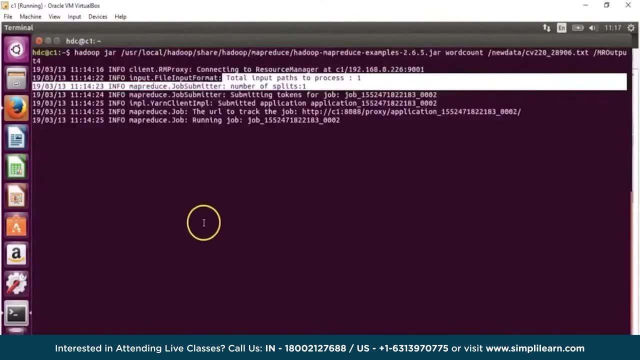 shows up here. 16 GB and 16 cores is not the true one. those are the default settings, right? but then my yarn should be able to facilitate running of this application. Let's just give it couple of seconds and then let's look into the output. here Again, I had to make some. 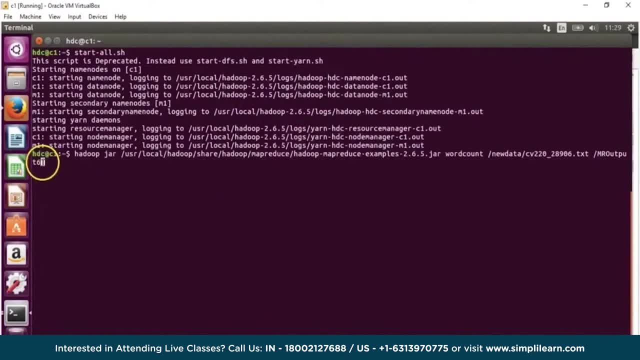 changes in the settings because our application was not running. So let's just give it a couple of seconds to see what happens. So here I have submitted my application, which is running on the first page, and my application has not taken up the storage space. So my application 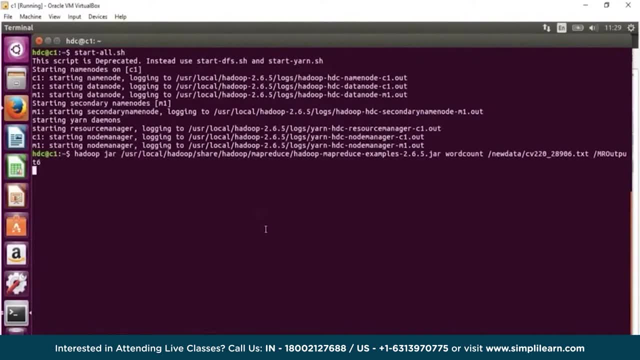 is not getting enough resources, and then basically restarted my cluster. Now let's submit the application again to the cluster, which first should contact the resource manager and then basically the map and reduce process should start. So here I have submitted an application, it is connecting to the resource manager and then basically it will start internally in. 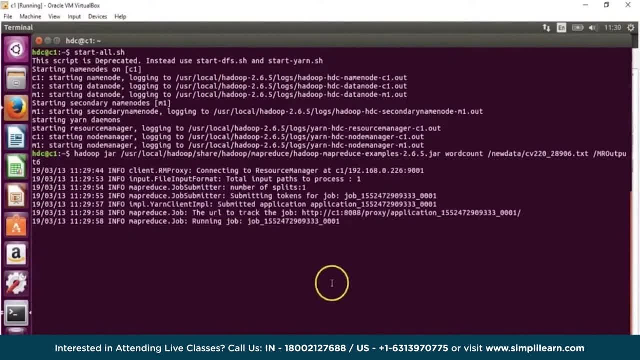 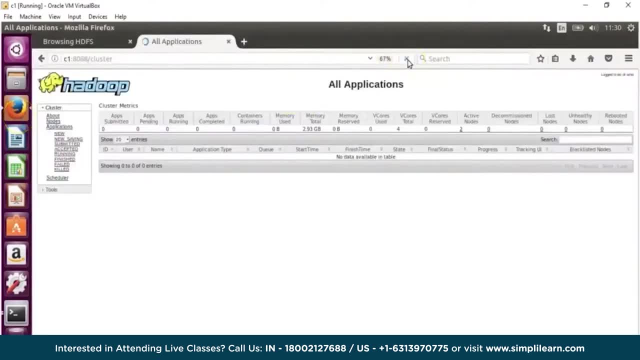 the app master. That is application master. it basically then starts running the job. it also gives you a tracking URL to look at the output. and now we should go back and look at our yarn UI, if our application shows up here and we will have to give it a couple of seconds when. 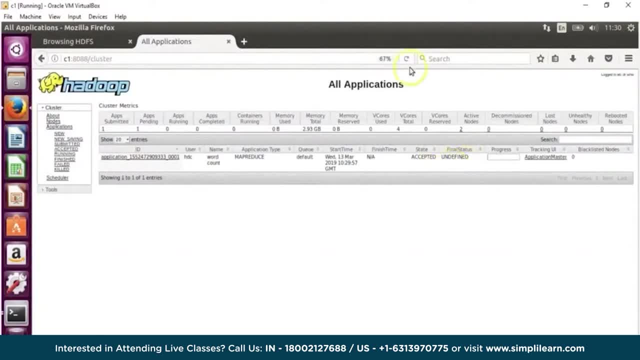 it can get the final status change to running and that's where my application will be getting resources. now, if you closely notice here, I have allocated specific amount of memory, that is, 1.5 GB for node manager on every node, and I have basically given two cores each, which my machines also have, and my yarn. 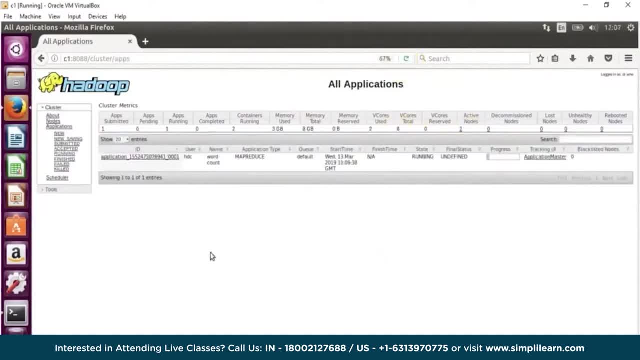 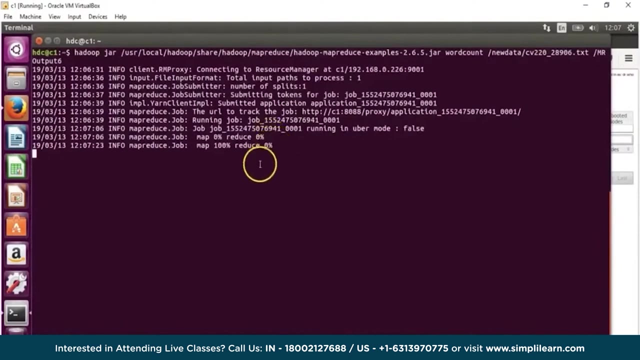 should be utilizing these resources rather than going for default. now the application has started moving and we can see the progress bar here, which basically will show what is happening, and if we go back to the terminal, it will show that first it went in deciding, map and reduce it. 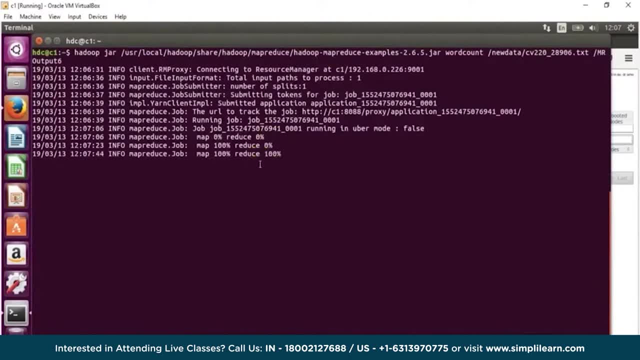 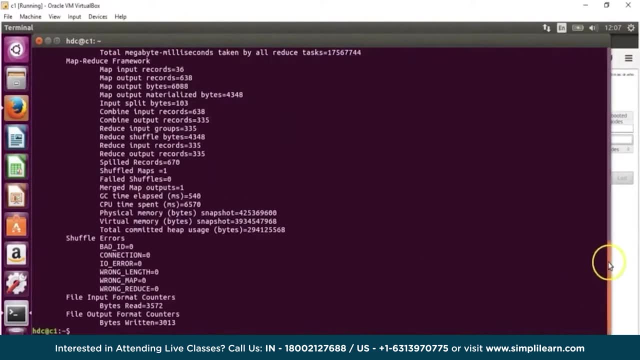 goes back to the terminal, and then it goes back to the terminal and then it goes for map. once the mapping phase completes, then the reducing phase will come into existence. and here my job has completed. so now it has basically used. we can always look at how many map and reduce tasks were run. it shows me that. 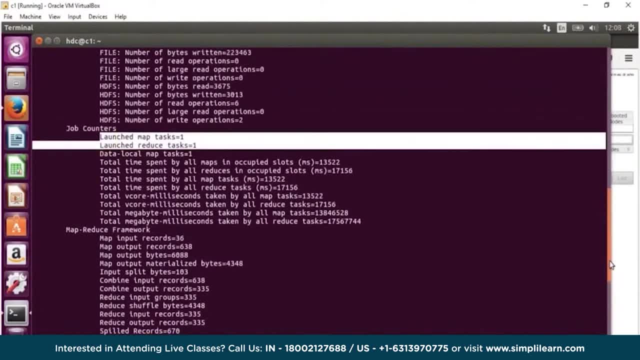 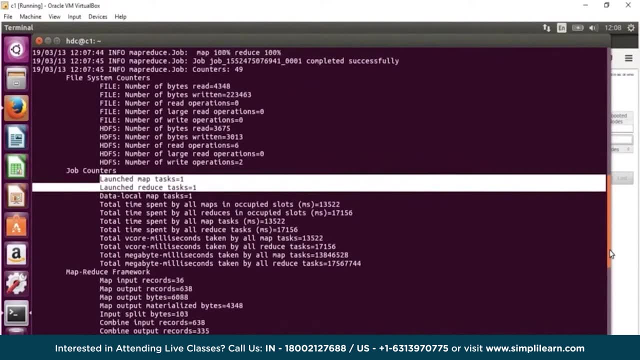 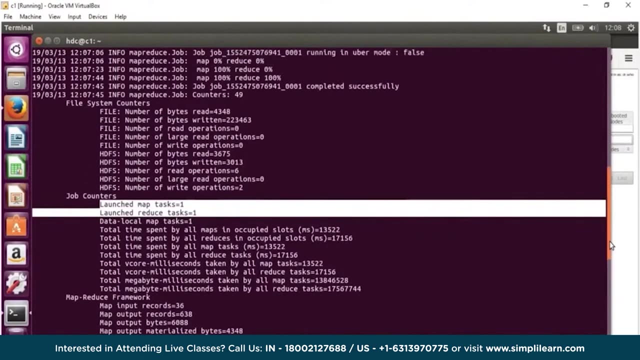 there was one map and one reduce task. now, with the number of map tasks depends on the number of splits, and we had just one file which is less than 128 MB. so that was one split to be processed. and reduce task is internally decided by the reducer or depending on what kind of property has been set in Hadoop config. 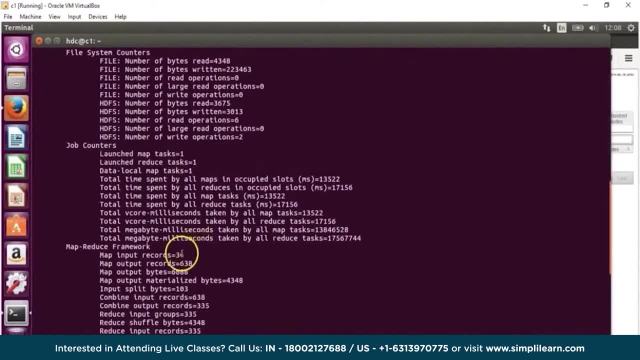 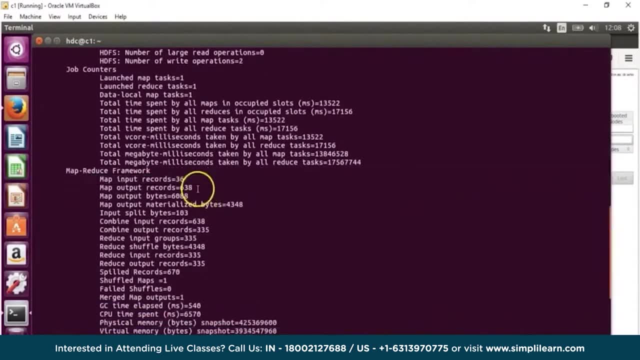 files now. it also tells me how many input records were read, which basically means these were the number of lines in the file. it tells me output records, which gives me the number of total words in the file- now there might be duplicates- and that which is processed by internal combiner: further processing or forwarding. 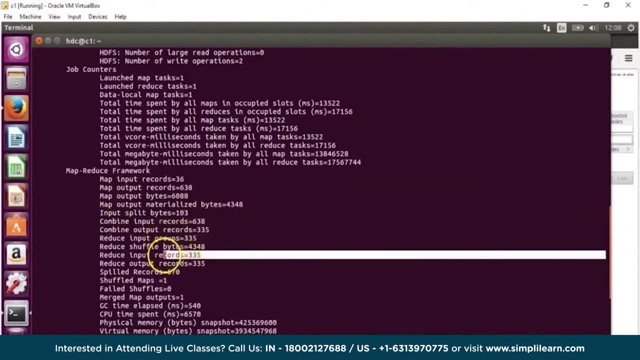 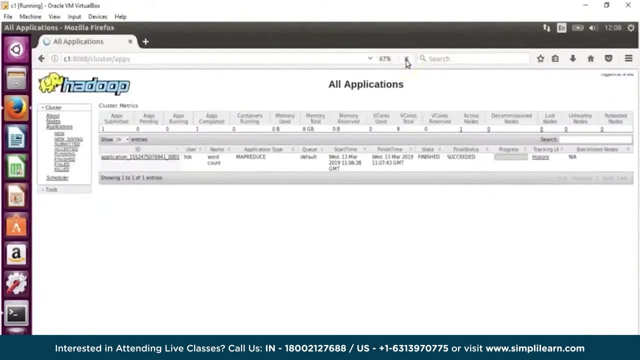 that information to reducer and basically reducer, works on three thirds of the time. so that is basically what we have done so far in this video. thirty five records gives us a list of words and their count. now, if I do a refresh here, this would obviously show my application is completed, says: 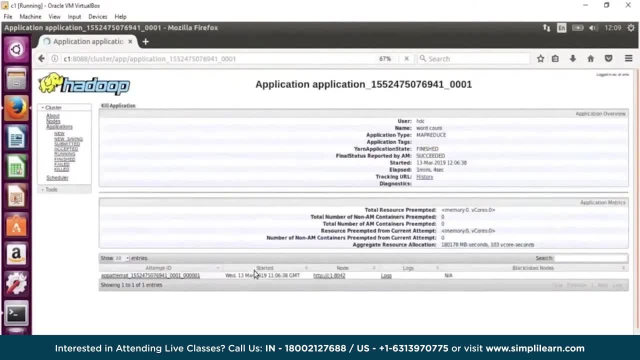 succeeded. you can always click on the application to look for more information. it tells me where it ran. now we do not have a history server running as of now, otherwise we can always access more information. so this leads to history server where all your applications are stored. but I can click on this attempt. 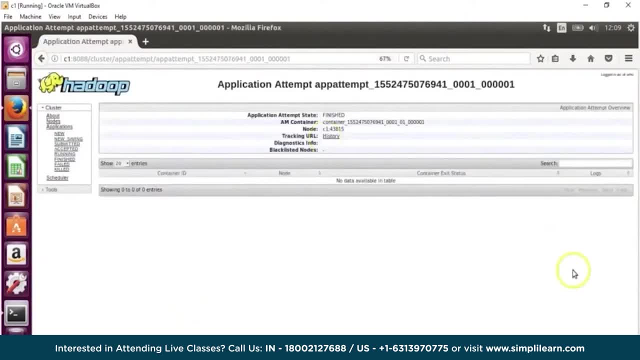 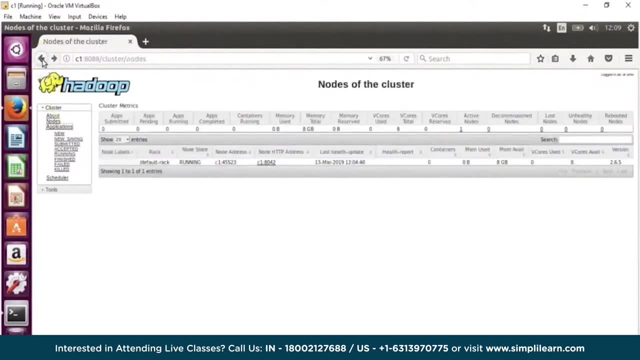 tasks, and this will be the history server that we are using now. so that is will basically show me the history URL or you can always look into the logs. so this is how you can submit a sample application which is inbuilt, which is available in the jar on your Hadoop cluster and that will utilize your 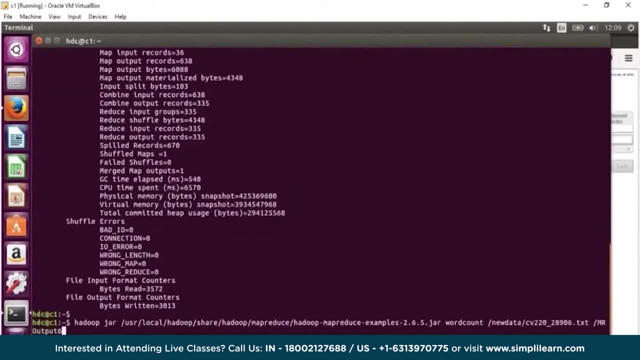 cluster to run now. you could always, as I said, when you are running a particular job, remember to change the output directory and if you would not want it to be processing is a single individual file, you could also point it to a directory. that basically means it will have multiple files and, depending on the 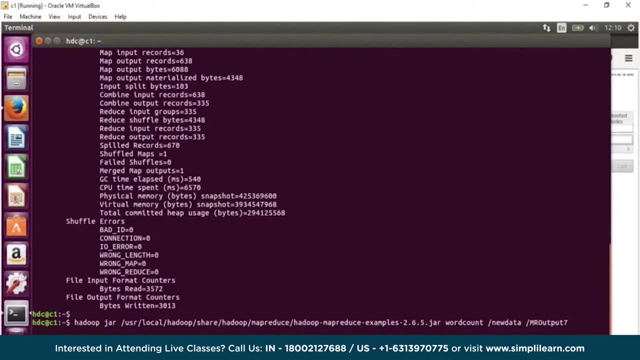 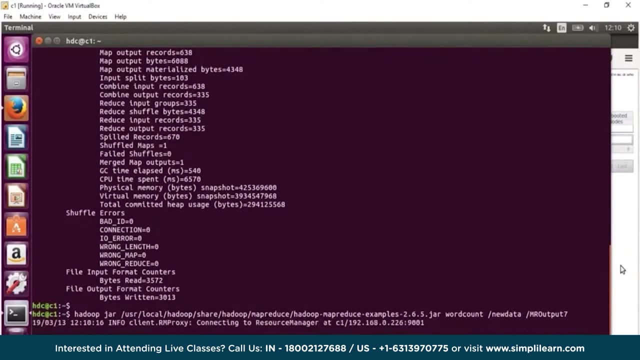 file sizes, there would be multiple splits and according to that, multiple map tasks will be selected. so if I click on this, this would submit my second application to the cluster, which should first connect to resource manager. then resource manager has to start an application master. now here we are. 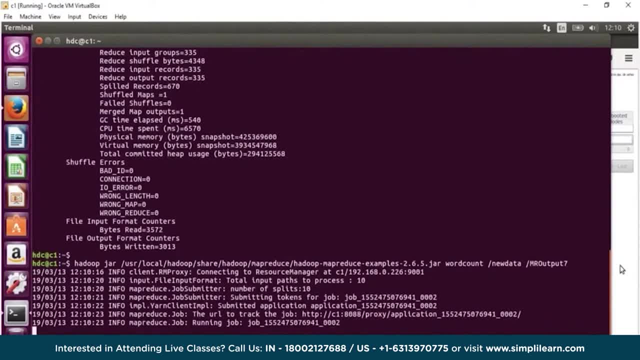 targeting 10 splits. now you have to sometimes give a couple of seconds in your machines so that the resources which were used are in your cluster, so that the resources which were used are in your internally already freed up, so that your cluster can pick it up, and then 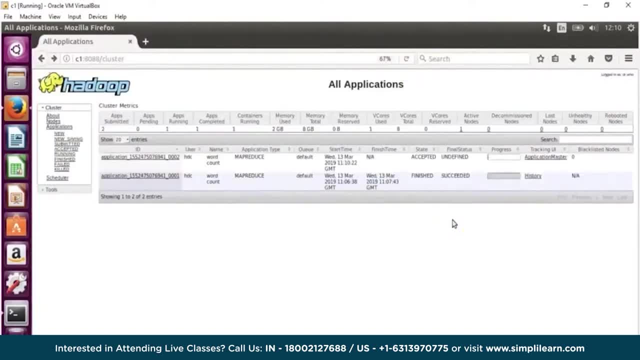 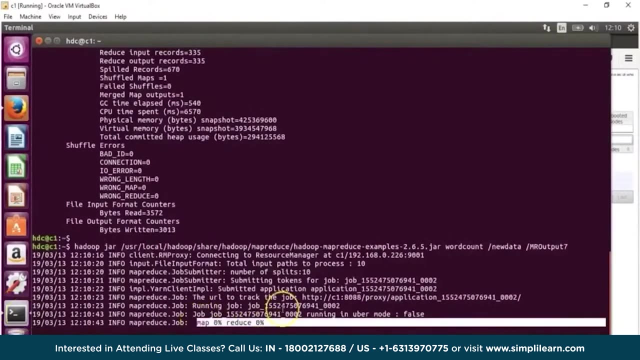 your yarn can take care of resources. so right now my application is an undefined status, but then, as soon as my yarn provides it the resources, we will have the application running on our yarn cluster. so it has already started. if you see it is going further, then it would launch 10 map tasks and it would the 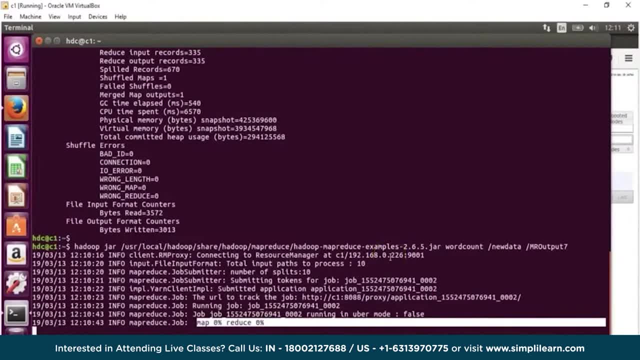 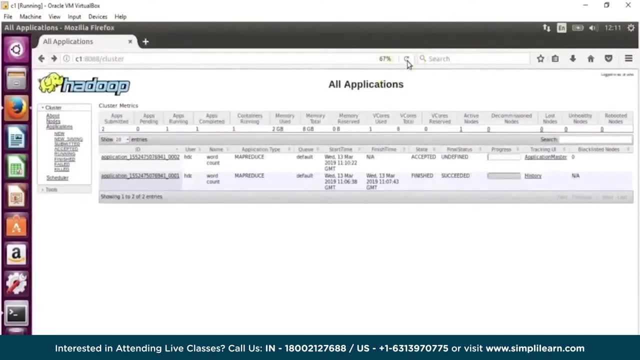 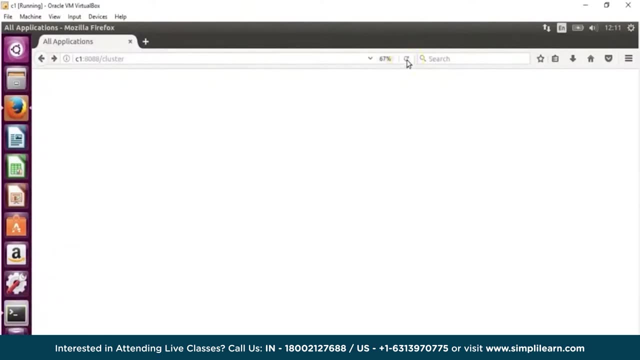 number of reduced tasks would be decided on either the way your data is or based on the properties which have been set at your cluster level. let's just do a quick refresh here on my yarn UI to show me the progress. also, take care that when you are submitting your application you need to have the output. 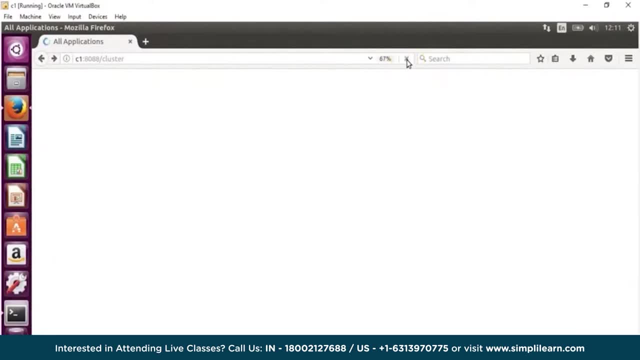 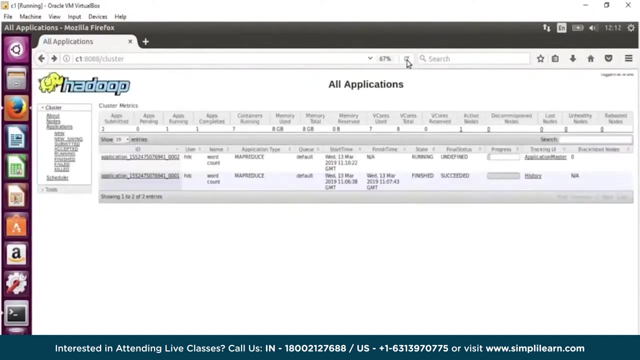 directory mentioned. however, do not create it. Hadoop will create that for you. now this is how you run a map reduce without specifying properties, but then you can specify more properties. you can look into what are the things which can be changed for your mapper and reducer, or basically having a combiner class. 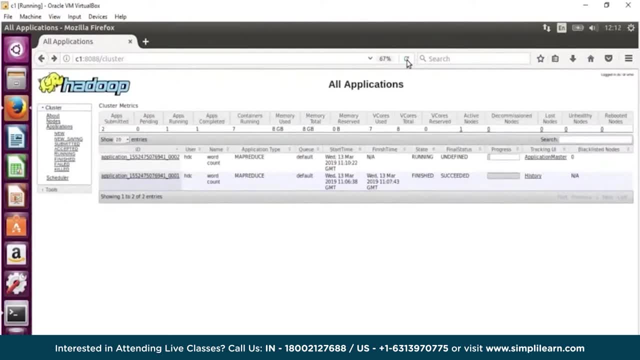 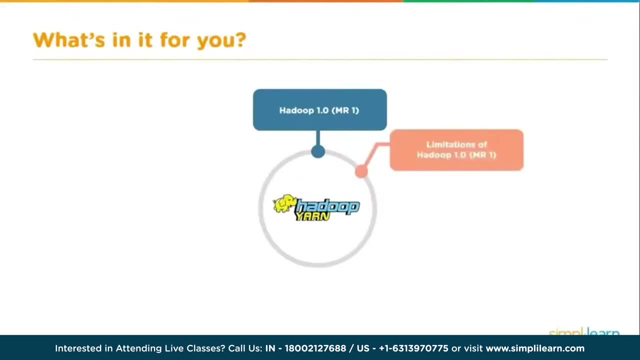 which can do a mini reducing and all those things can be done. so we will learn about that in the later sessions. now we will compare Hadoop version 1, that is, with MapReduce version 1. we will understand and learn about the limitations of Hadoop version 1. what is the need of yarn? what is yarn? what kind? 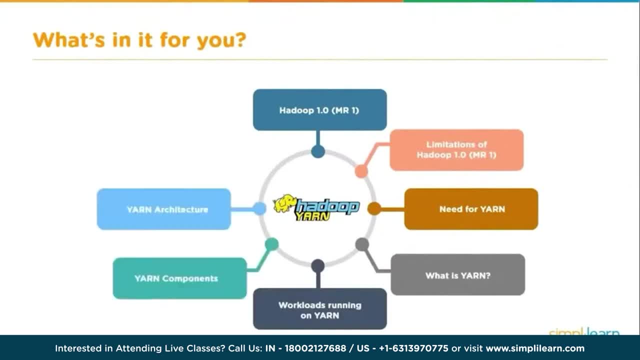 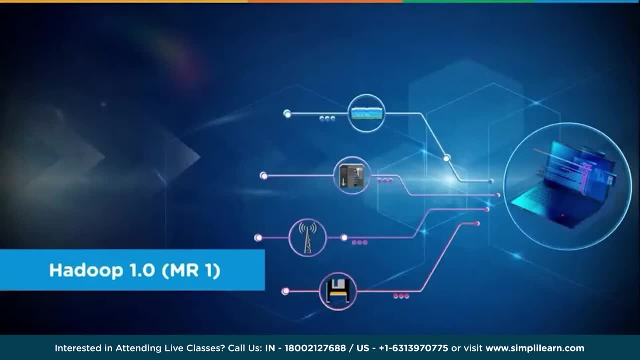 of workloads can be running on yarn. what are yarn components, what is yarn architecture? and for that, we will learn more about Hadoop version 1, so let's get started. finally, we will see a demo on yarn. so Hadoop version 1, or MapReduce version 1. 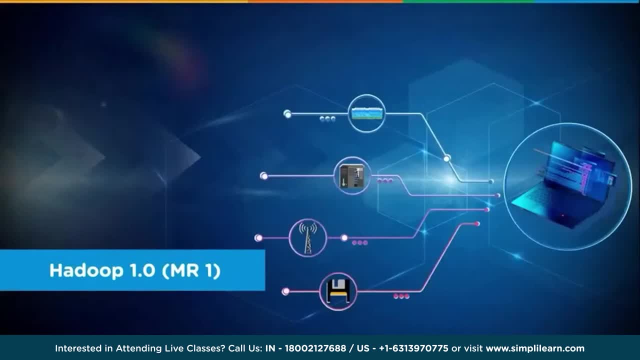 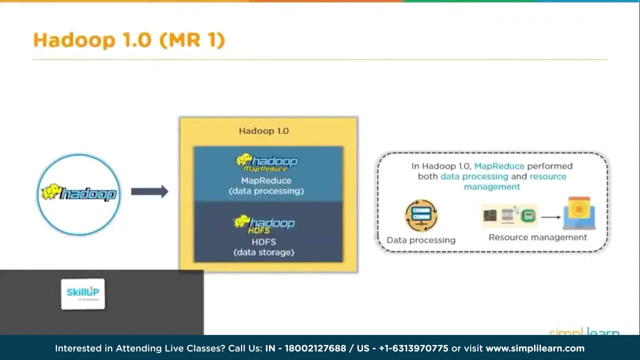 well, that's outdated now and nobody is using Hadoop version 1, but it would be good to understand what was in Hadoop version 1 and what were the limitations of Hadoop version 1, which brought in the thought for the future processing layer. that is yarn. now when we talk about Hadoop, we already know that Hadoop is a. 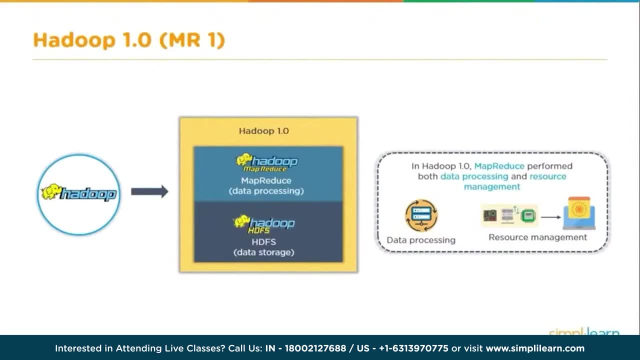 framework and Hadoop has two layers. Hadoop is a framework and Hadoop is a layer. one is your storage layer, that is, your HDFS Hadoop distributed file system, which allows for distributed storage and processing, which allows fault tolerance by inbuilt replication and which basically allows you to store huge. 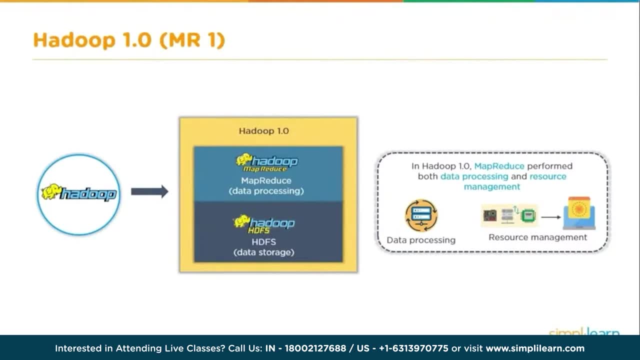 amount of data across multiple commodity machines. when we talk about processing, we know that MapReduce is the oldest and the most mature processing programming model which basically takes care of your data processing on your distributed file system. so in Hadoop version 1, MapReduce performed both data processing and resource management, and that's how it was. 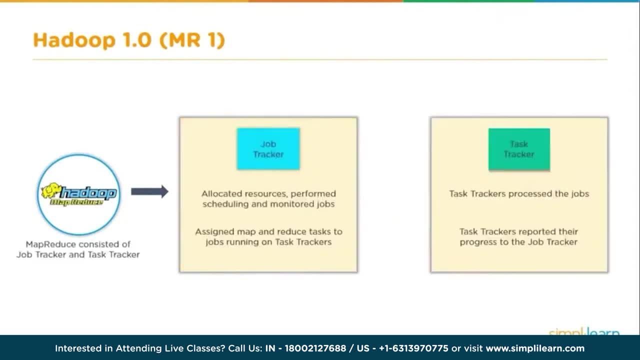 problematic in MapReduce. we had basically, when we talk about the processing layer, we had the master, which was called job tracker, and then you had the slaves, which were the task trackers. so your job tracker was taking care of allocating resources, it was performing scheduling and even monitoring the jobs. 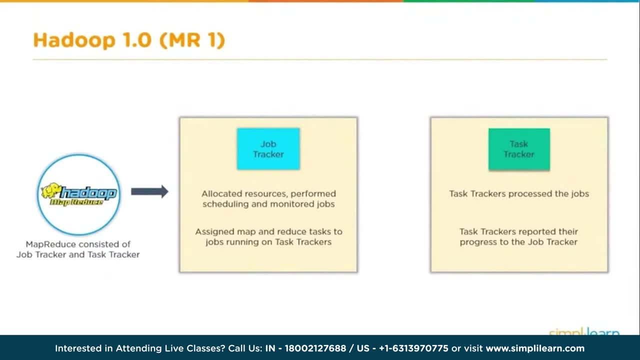 it basically was taking care of assigning, map and reduce tasks to the jobs running on task trackers. and task trackers, which were co-located with data nodes, were responsible for processing the jobs. so task trackers were the slaves for the processing layer which reported their progress to the job tracker. so 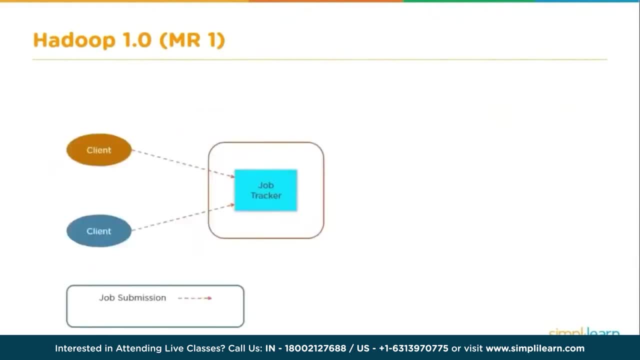 this is what was happening in Hadoop version 1. now, when we talk about Hadoop version 1, we would have say client machines, or an API or an application which basically submits the job to the master, that is, job tracker. now, obviously, we cannot forget that there would already be an involvement from name node, which 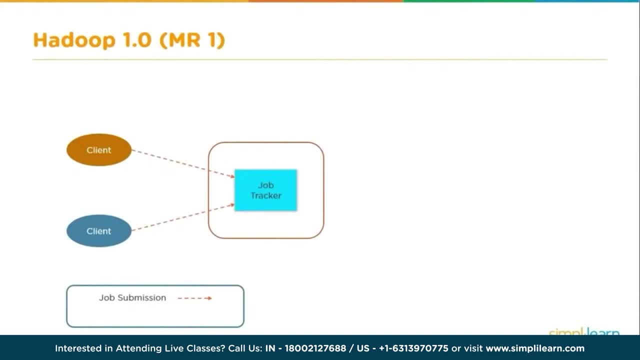 basically tells which are the machines or which are the data nodes where the data is already stored. now, once the job submission happens to the job tracker, job tracker being the master demon for taking care of your processing request and also resource management, job scheduling would then be interacting with your multiple task trackers, which would be 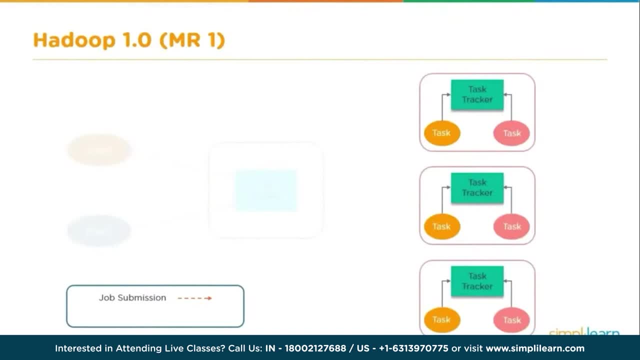 running on multiple machines. so each machine would have a task tracker running and that task tracker, which is a processing slave, would be co-located with the data nodes. now we know that in case of Hadoop, you have the concept of moving the processing to wherever the data is. 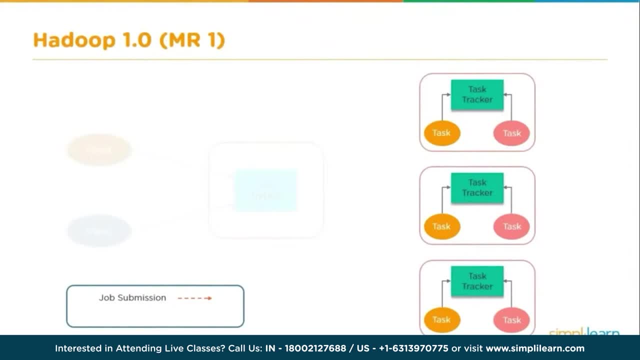 stored rather than moving the data to the processing layer. so we would have task trackers which would be running on multiple machines and these task trackers would be responsible for handling the task tasks. what are these tasks? these are the application, which is broken down into smaller tasks which would work on the data which is respectively stored on that particular node. 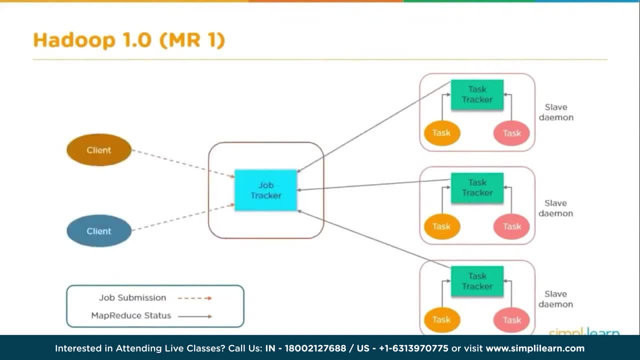 now, these were your slave demons, right? so your job tracker was not only tracking the resources, so your task trackers were sending heartbeats, they were sending in packets and information to the job tracker, which would then be knowing how many resources. and they talk about resources. we are talking about the CPU cores, we are talking about the RAM, which 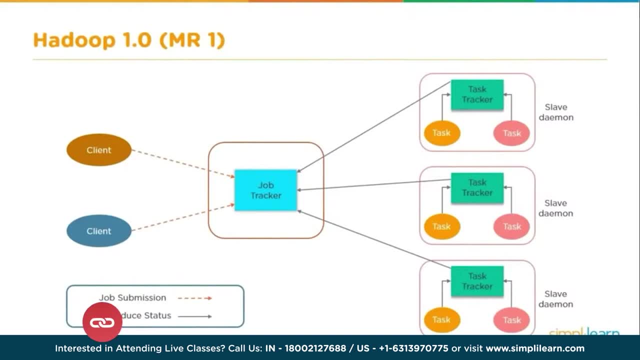 would be available on every node. so task trackers would be sending in their resource information to job tracker and your job tracker would be already aware of what amount of resources are available on a particular node, how loaded a particular node is, what kind of work could be given to the task. 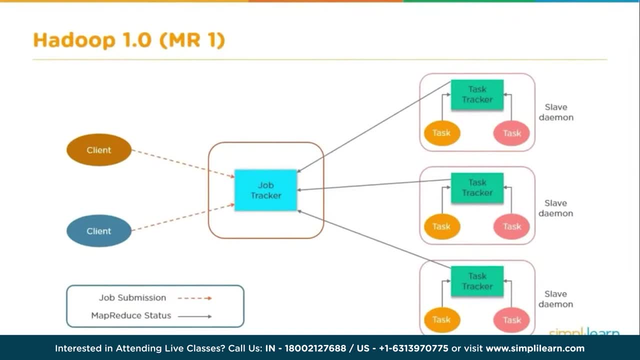 tracker. so job tracker was taking care of resource management and it was also breaking the application through tasks and doing the job scheduling part. assign different tasks to these slave demons. that is your task trackers. so job tracker was eventually overburdened, right, because it was managing jobs. it. 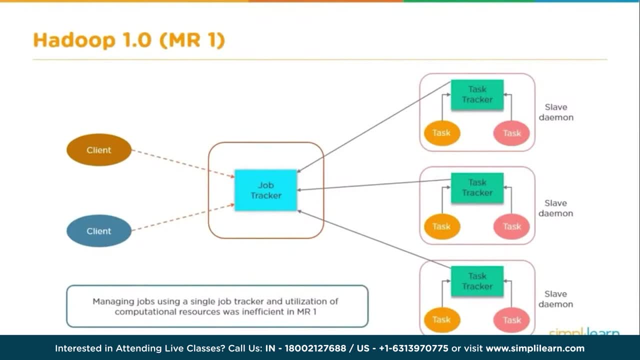 was tracking the resources from multiple task trackers and basically it was taking care of job scheduling. so job tracker would be overburdened and in a case if job tracker would fail then it would affect the overall processing. so if the master is killed, if the master demand dies, then the processing cannot proceed. now this was one of 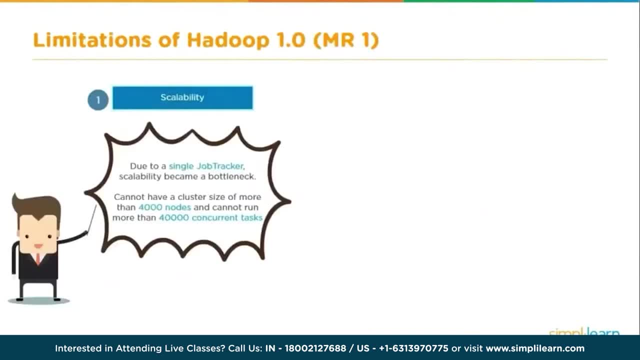 the limitations of Hadoop version one. so when you talk about scalability, that is, the capability to scale due to a single job tracker, scalability would be hitting a bottleneck. you cannot have a cluster size of more than four thousand nodes and cannot run more than forty thousand concurrent. 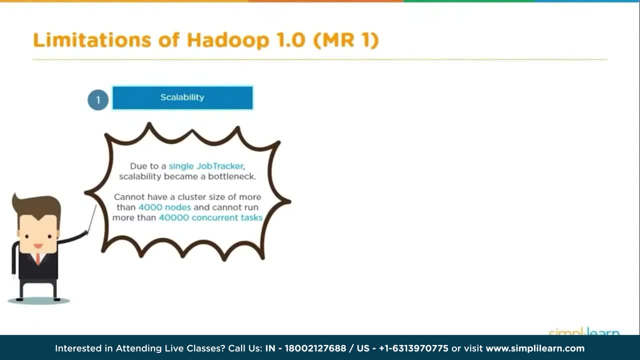 tasks. now, that's just a number. we could always look into the individual resources which each machine was having and then we can come up with an appropriate number. however, with a single job tracker, there was no horizontal scalability for the processing layer because we had single processing master. now, when we talk about availability, job tracker, as I mentioned, would be a single point. 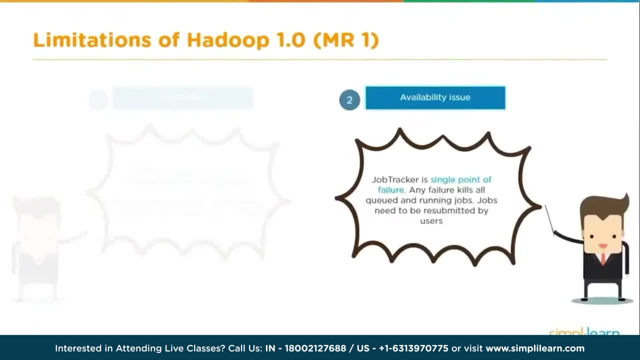 of failure. now, any failure kills all the queued and running jobs, and jobs would have to be resubmitted. now why would we want that? in a distributed platform, in a cluster which has hundreds and thousands of, in a cluster which has hundreds and thousands of machines, we would want a processing layer which can handle huge amount of processing, which could 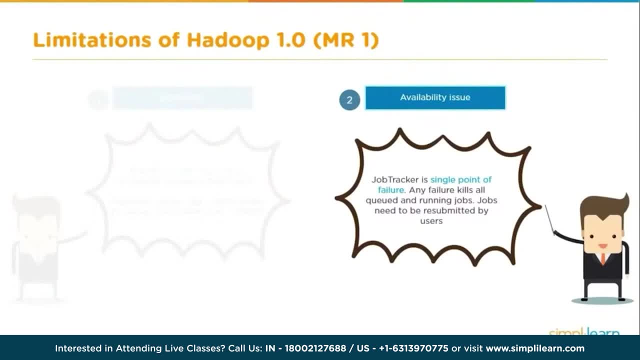 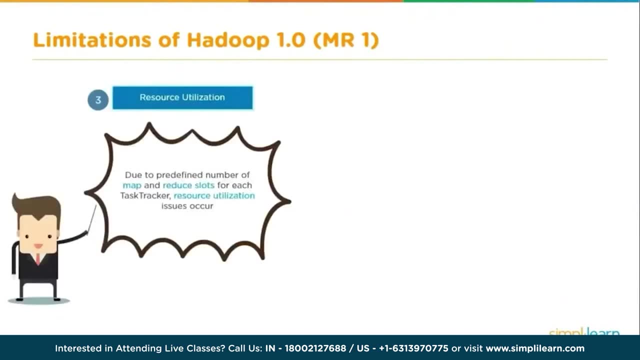 be more scalable, which could be more available and could handle different kind of workloads. when it comes to resource utilization, now, if you would have a predefined number of map and reduce slots for each task tracker, you would have issues which would relate to resource utilization and that. 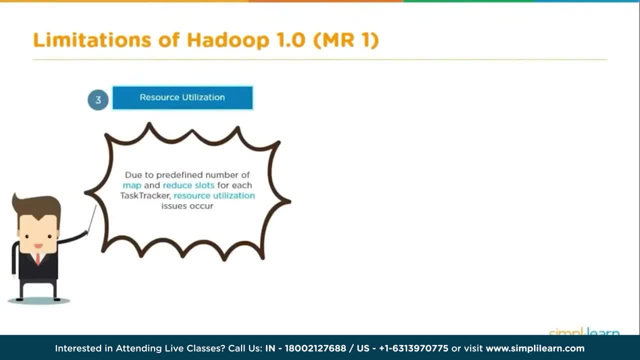 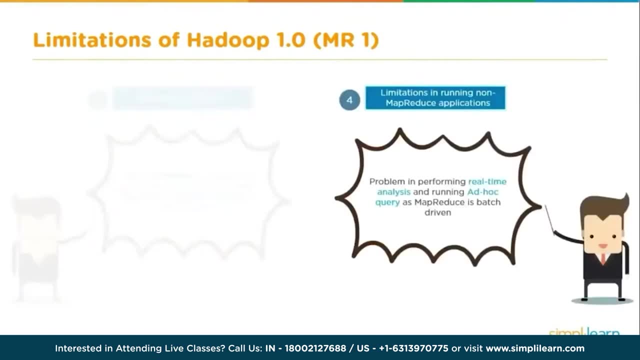 again is putting a burden on the master which is tracking these resources, which has to assign to jobs which can run on multiple machines in parallel. so limitations in running non MapReduce applications. now that was one more limitation of Hadoop version 1 and MapReduce: that the only kind of processing you could do is MapReduce. 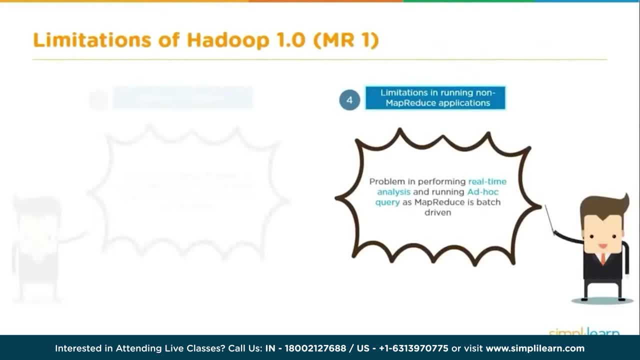 and MapReduce programming model. although it is good, it is oldest, it has matured over a period of time, but then it is very rigid. you will have to go for mapping and reducing approach, and that was the only kind of processing which could be done in Hadoop version 1. so when it comes to doing a real-time, 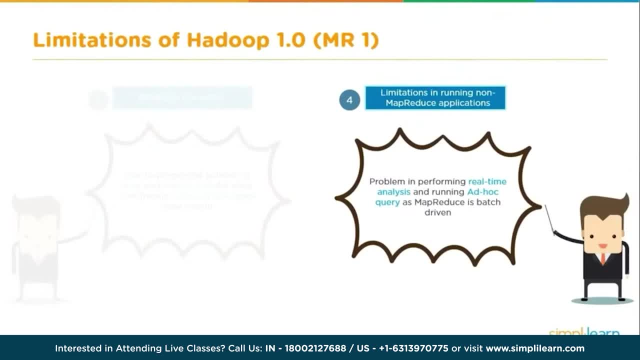 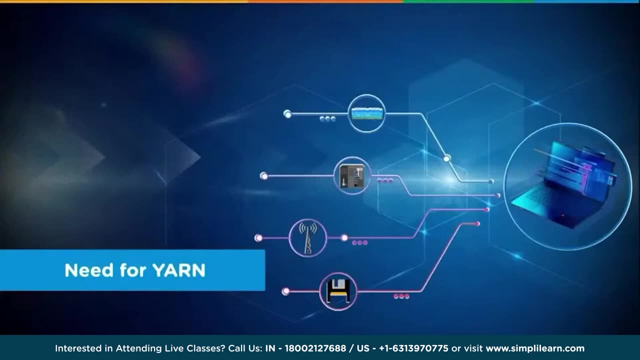 analysis, or doing ad hoc query, or doing a graph based processing or massive parallel processing. there were limitations because that could not be done in Hadoop version 1, which was having MapReduce version 1 as the processing component. now that brings us to the need for YAN. so YAN it stands. 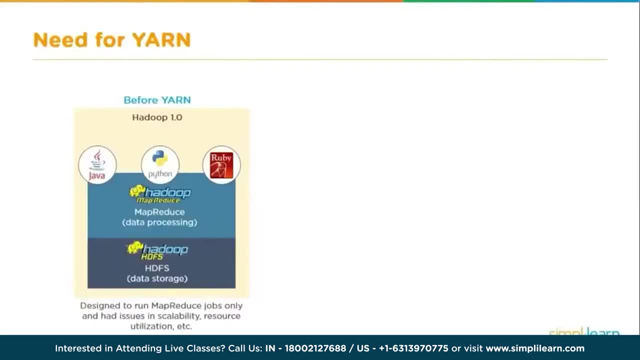 for yet another resource negotiator. so, as I mentioned before, YAN in Hadoop version 1. well, you could have applications which could be written in different programming languages, but then the only kind of processing which was possible was MapReduce. we had the storage layer, we had the processing, but then kind of 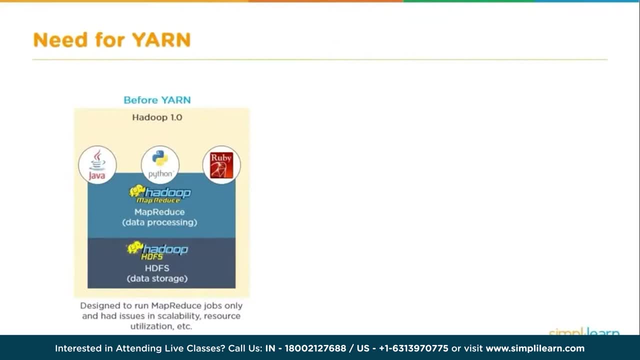 limited processing which could be done now. this was one thing which brought in a thought that why shouldn't we have a processing layer which can handle different kind of work layer, which can handle different kind of work layer which can handle different kind of work loads? as I mentioned, might be graph processing, might be real-time processing. 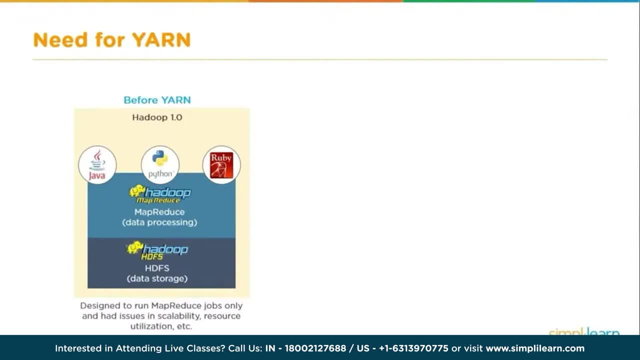 might be massive parallel processing or any other kind of processing which would be requirement of an organization now designed to run MapReduce jobs only and having issues in scalability, resource utilization, job tracking, etc. that led to the need of something what we call as YAN. now, from Hadoop version 2 onwards, we 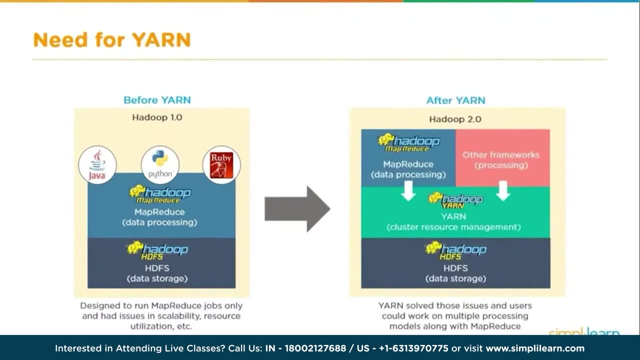 have. the two main layers have changed a little bit. you have the storage layer, which is intact, that is, your HDFS, and then you have the processing layer, which is called YAN- yet another resource negotiator. now we will understand how YAN works. but then YAN. 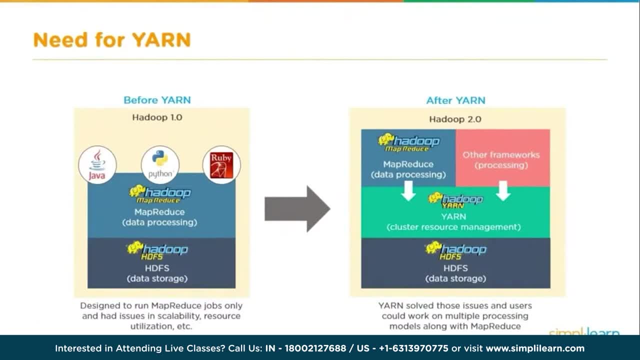 is taking care of your processing layer. it does support MapReduce, so MapReduce processing can still be done, but then now you can have a support to other processing frameworks. YAN can be used to solve the issues which Hadoop version 1 was posing: something like resource management, something like different. 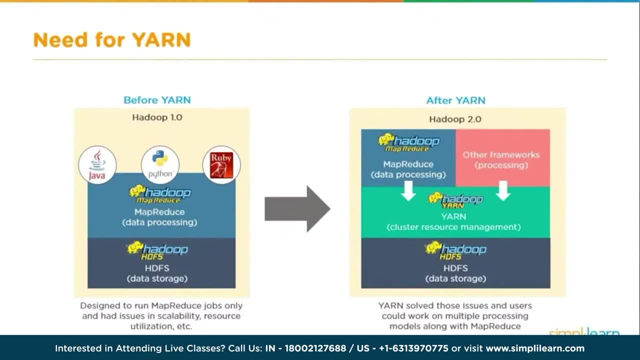 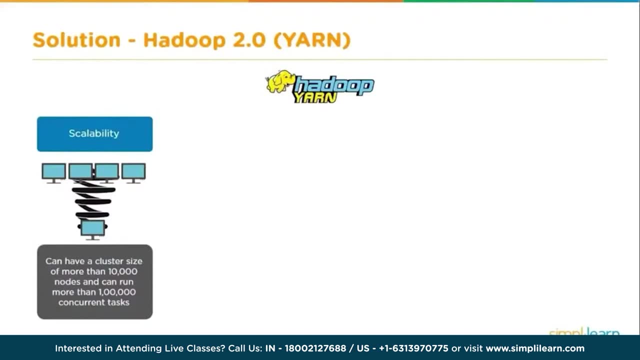 kind of workload processing, something like scalability, resource utilization. all that is now taken care by YAN. now, when we talk about YAN, we can have now a cluster size of more than 10,000 nodes and can run more than 100,000 concurrent tasks. that's just to take care of your scalability when you talk. 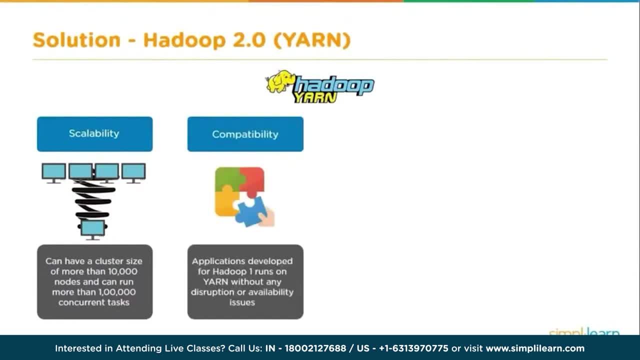 about compatibility: applications which were developed for Hadoop version 1, which were primarily MapReduce kind of processing, can run on YAN without any disruption or availability issues. when you talk about resource utilization, there is a mechanism which takes care of dynamic allocation of cluster resources and this basically improves the resource utilization. when we talk about 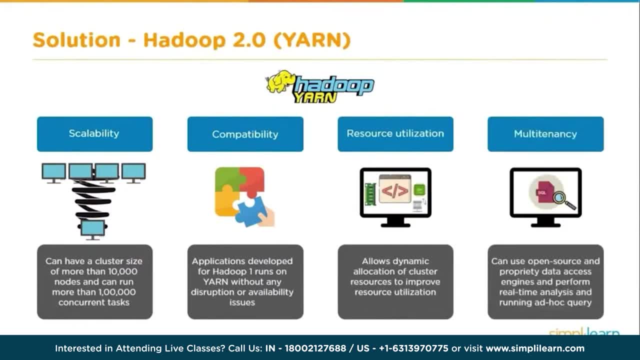 multi-tenancy. so basically now the cluster can handle different kind of workloads, so you can use open source and proprietary data access engines and you can perform real-time analysis. you can be doing graph processing, you can be doing ad hoc querying and this can be supported for multiple workloads, which 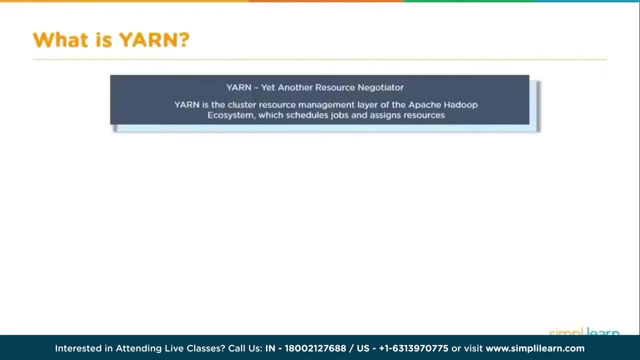 can run in parallel. so this is what YAN offers. so what is YAN? as I mentioned, YAN stands for yet another resource negotiator, so it is the cluster resource management layer for your Apache Hadoop ecosystem, which takes care of scheduling jobs and assigning resources. now just imagine when you 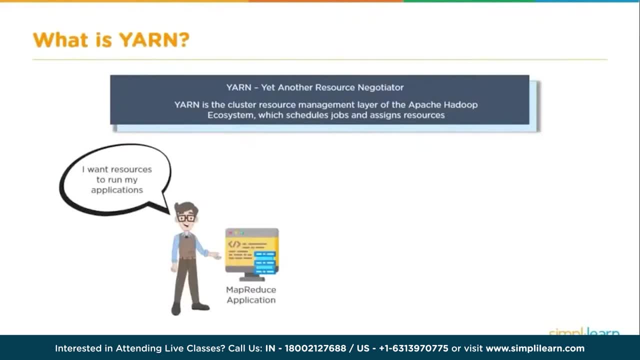 would want to run a particular application. you would basically be telling the cluster that I would want resources to run my applications. that application might be a MapReduce application. that might be a hive query which is triggering a MapReduce. that might be a pig script, which is 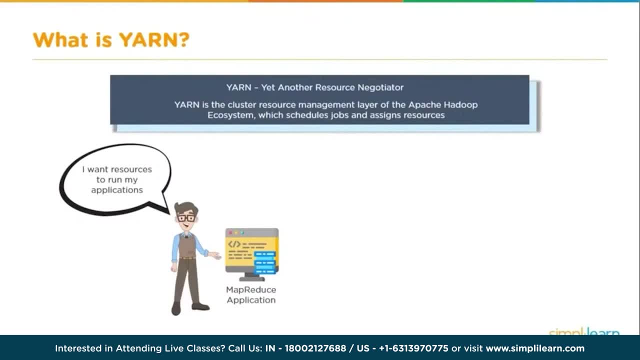 triggering a MapReduce. that could be hive with Taze as an execution engine, that could be a spark application, that could be a graph processing application. in any of these cases, you would still, you know, as, in in sense, client or basically an API, or the application would be. 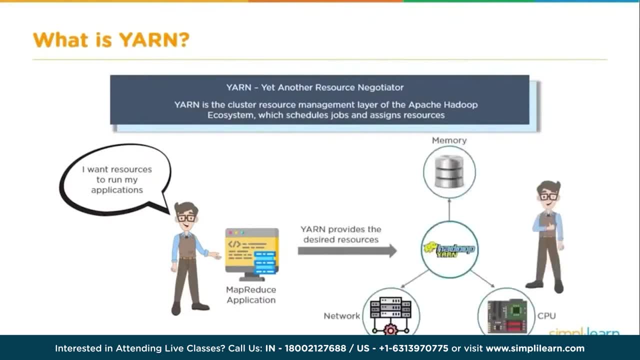 requesting for resources. YAN would take care of that, so YAN would provide the desired resources. now, when we talk about resources, we are mainly talking about the network related resources. we are talking about the CPU cores or, as in terms of YAN we say, virtual CPU cores. we would talk about RAM that is in GB. 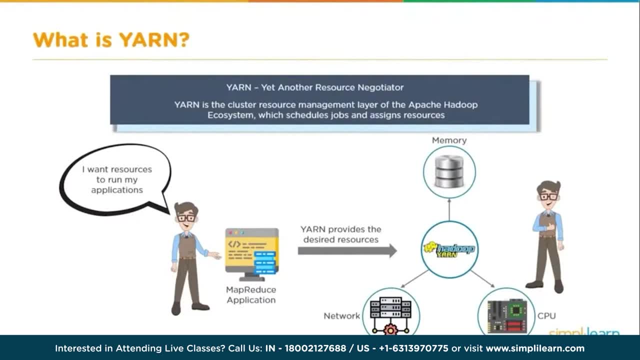 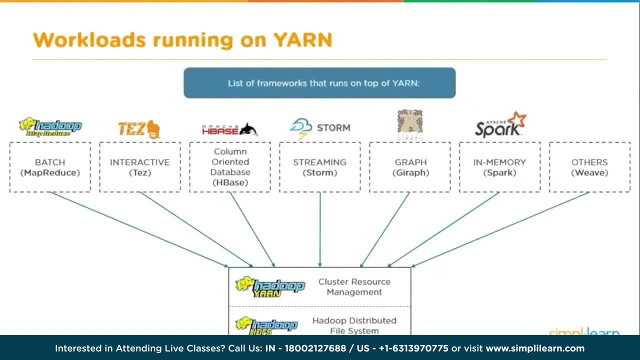 or mb or in terabytes offered from multiple machines, and yarn would take care of this. So with yarn you could basically handle different workloads. Now these are some of the workloads which are showing up here. You have the traditional MapReduce, which is mainly batch oriented. You could have an interactive 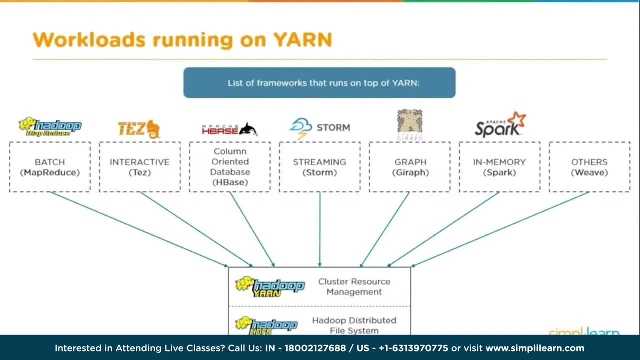 execution engine, something as TASE. You could have HBase, which is a column oriented or a four-dimensional database, And that would be not only storing data on SDFS but would also need some kind of processing. You could have streaming functionalities, which would be from Storm or 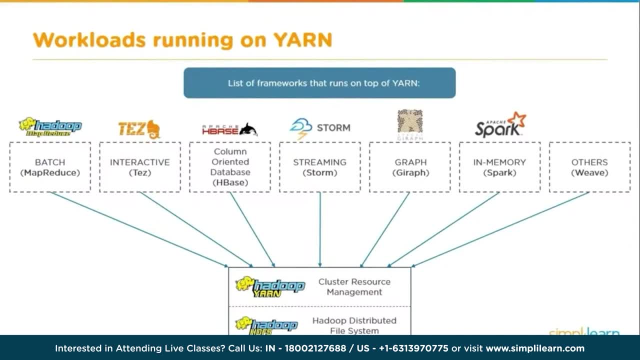 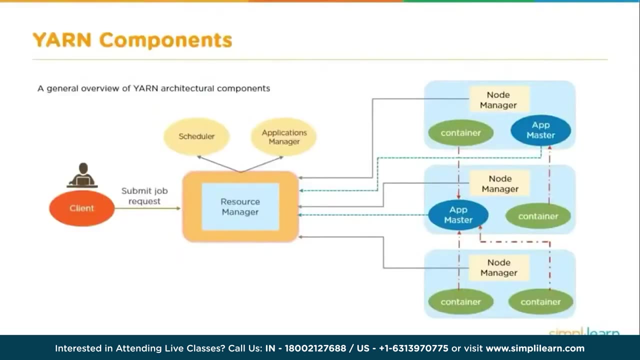 Kafka or Spark. You could have graph processing, You could have in-memory processing, such as Spark and its components, and you could have many others. So these are different frameworks which could now run and which can run on top of yarn. So how does yarn do that? Now, when we talk about 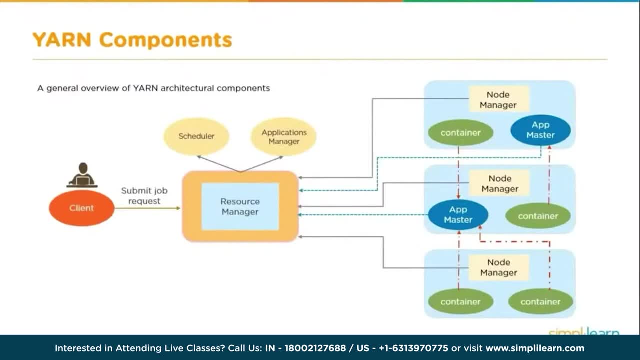 yarn. this is how a overall yarn architecture looks. So at one end you have a yarn architecture and at the other end you have a yarn architecture. So at one end you have a yarn architecture and at the other end you have a yarn architecture. 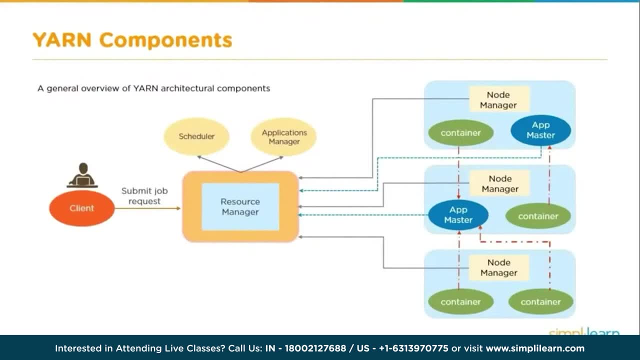 So at one end you have a yarn architecture and at the other end you have a yarn architecture. Now, client could be basically your edge node where you have some applications which are running. It could be an API which would want to interact with your cluster. It could be a user. 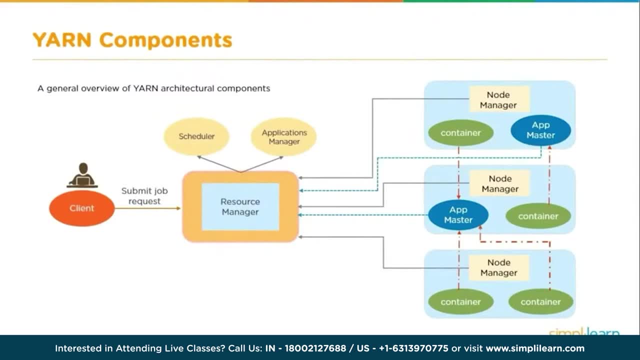 triggered application which wants to run some jobs which are doing some processing. So this client would submit a job request. Now what is resource manager doing? Resource manager is the master of your processing layer. In Hadoop version 1, we basically had job tracker and then we had 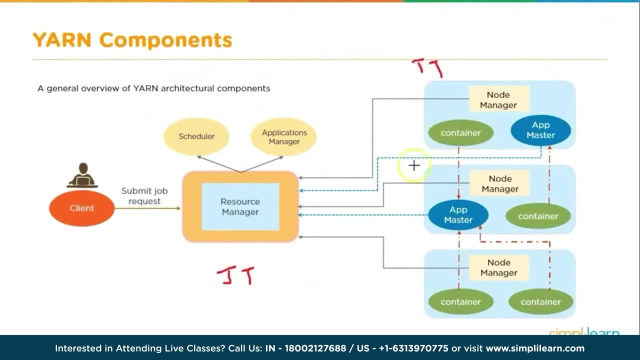 task trackers which were running on individual nodes. So your task trackers were sending your heartbeats to the job tracker. Your task trackers were sending it their resource information And job tracker was the one which was tracking the resources and it was doing the job scheduling. 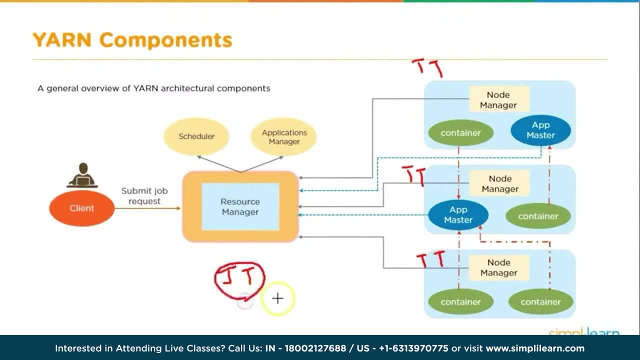 And that's how, as I mentioned earlier, job tracker was overburdened. So job tracker is now replaced by your resource manager, which is the master for your processing layer. Your task tracker are replaced by node managers, which would be then running on every node, And we have a temporary 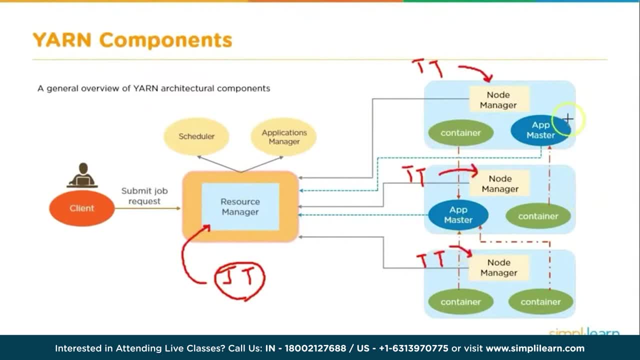 daemon, which you see here in blue, and that's your app master. So this is what we mentioned when we say yet another resource negotiator. So app master would be existing in a Hadoop version 2.. Now, when we talk about your resource manager, resource manager is the master for processing. 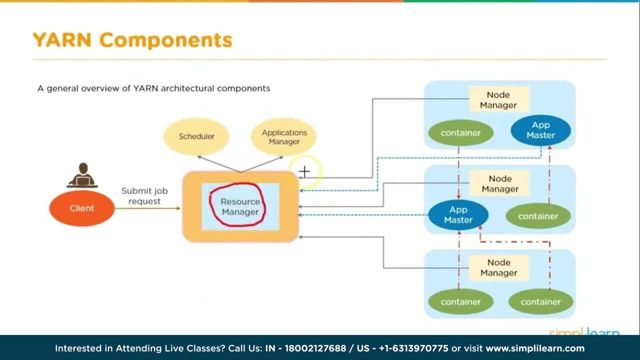 layer. So it would already be receiving Heartbeats and you can say, resource information from multiple node managers which would be running on one or multiple machines. And these node managers are not only updating their status, but they are also giving an information of the amount of resources they have. Now, when we talk, 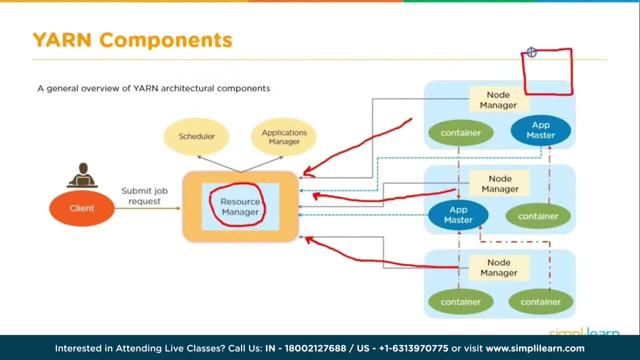 about resources. we should understand that if I'm talking about this node manager, then this has been allocated some amount of RAM for processing and some amount of CPU cores, And that is just a portion of what the complete node has. So if my node has say, imagine my node. 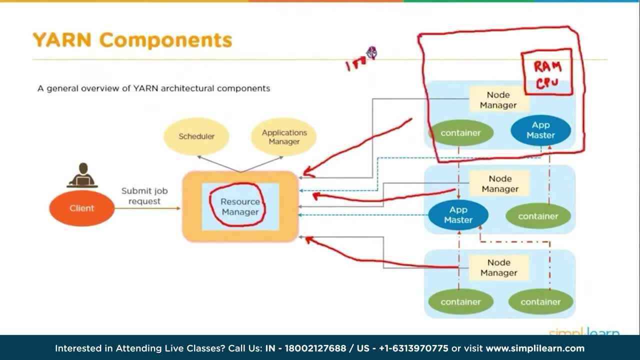 has around 100 GB RAM and I have, say, 60 cores. all of that cannot be allocated to node manager. So node manager is just one of the components of Hadoop ecosystem. It is the slave of the processing layer. So we could say keeping in all the aspects, such as different services. 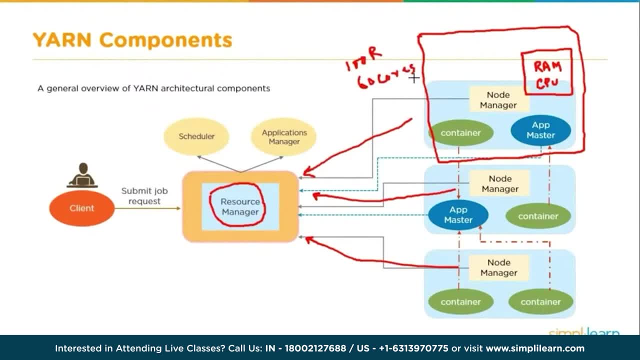 which are running on Hadoop ecosystem. it is the slave of the processing layer. So we could say might be Cloudera or Hortonworks related services running system processes running on a particular node. Some portion of this would be assigned to node manager for processing. So we could say: 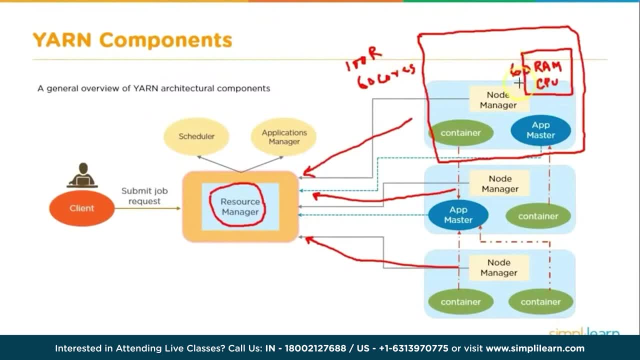 for example, say 60 GB RAM per node and say 40 CPU cores. So this is what is allocated for the node manager on every machine. Similarly we would have here. Similarly we would have here. So node manager is constantly giving an update. 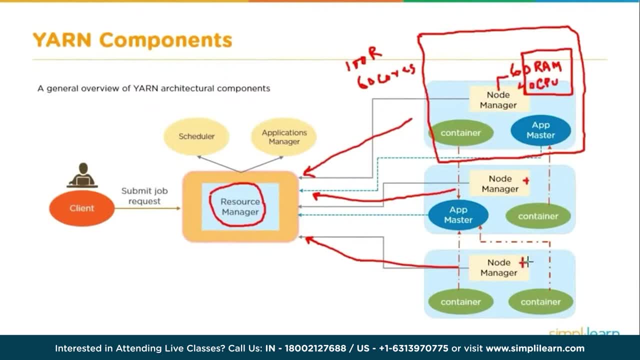 to resource manager about the resources, what it has. Probably there might be some other applications running and node manager is already occupied, So it gives an update. Now we also have a concept of containers, which is basically we will, we will talk about. 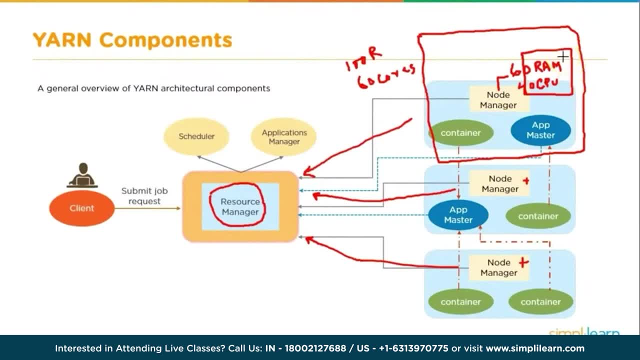 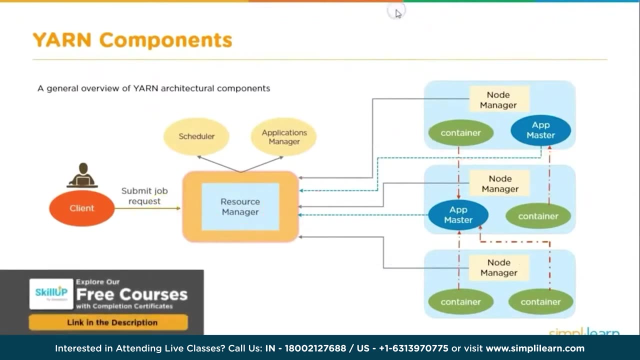 which is about these resources being broken down into smaller parts. So resource manager is keeping a track of the resources which every node manager has, And it is also responsible for taking care of the job request. How do these things happen Now, as we see here? resource manager at a higher level, you can always. 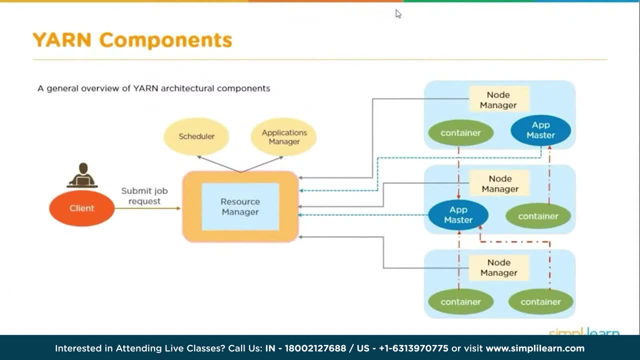 say: this is the processing master which does everything, but in reality, it is not the resource manager which is doing it, but it has internally different services or components which are helping it to do what it is supposed to do. Now let's look further. Now, as I mentioned your 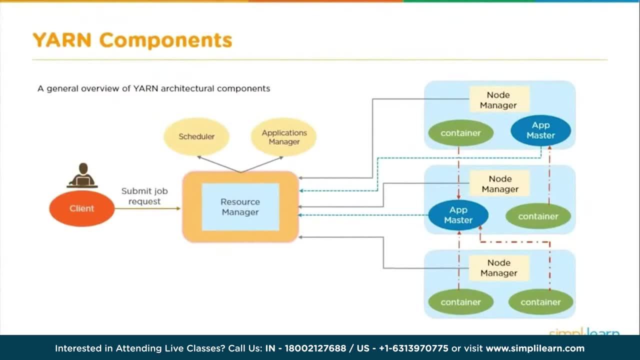 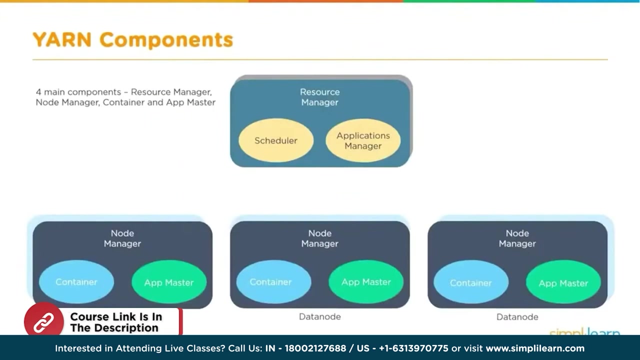 resource manager has these services or components, which basically helps it. It is basically a an architecture where multiple components are working together to achieve what yarn allows. So resource manager has mainly two components, That is, your scheduler and applications manager, And these are, at high level, four main components here. So we talk about 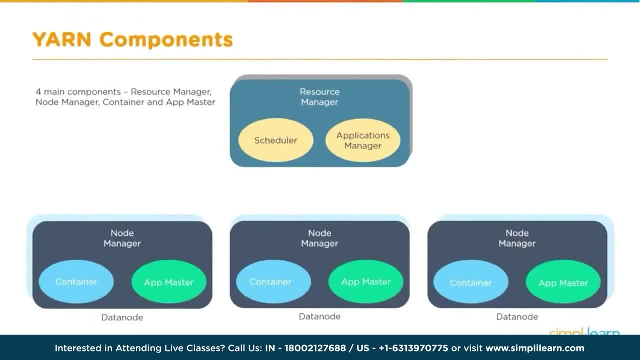 resource manager, which is the processing master. You have node managers, which are the processing slaves which are running on every nodes. You have the concept manager, which is the processing master. You have the concept of container and you have the concept of application master. 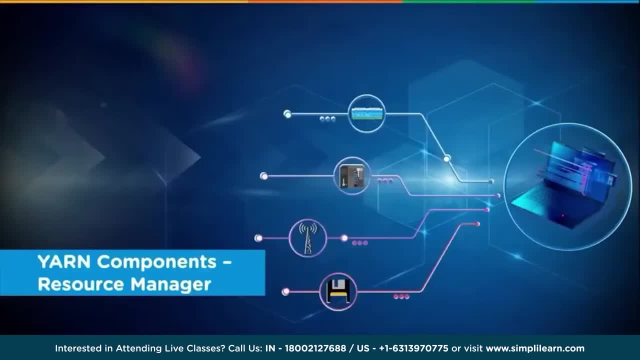 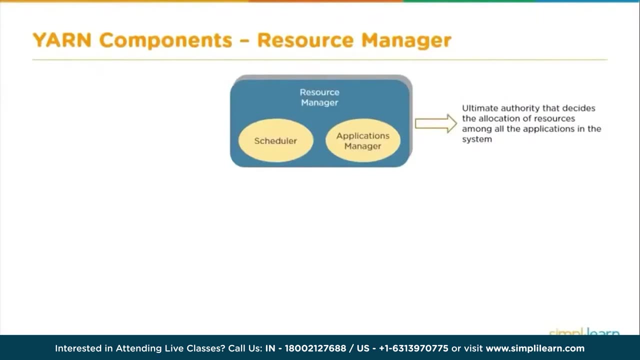 How do all these things work? Now let's look at yarn components. So resource manager basically has two main components, You can say, which assist resource manager in doing what it is capable of. So you have scheduler and applications manager. Now there is when you talk about resources. 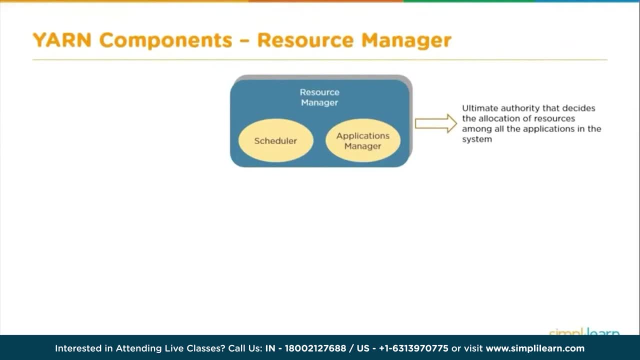 there is always a requirement for the applications which need to run on cluster of resources. So your application, which has to run, which was submitted by client, needs resources And these resources are coming in from multiple machines wherever the relevant data is stored and a node. 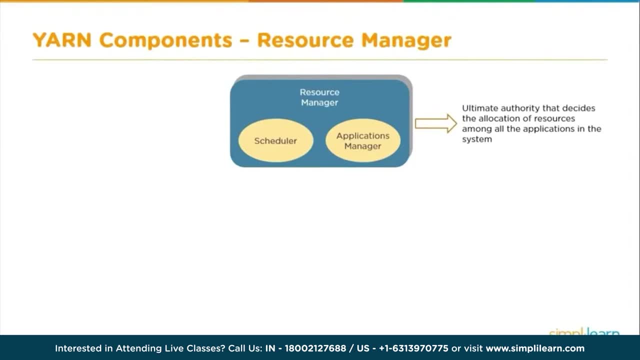 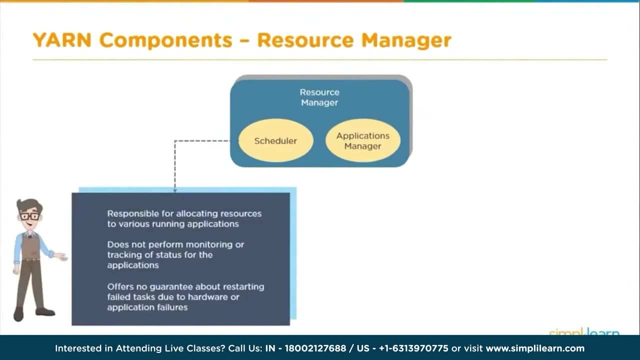 manager is running, So we always know that node manager is co-located with data nodes. Now what does the scheduler do? So we have different kinds of schedulers here. We have basically a capacity scheduler, We have a fair scheduler, or we have a low capacity scheduler. We have a low capacity scheduler, or we have a low capacity scheduler. 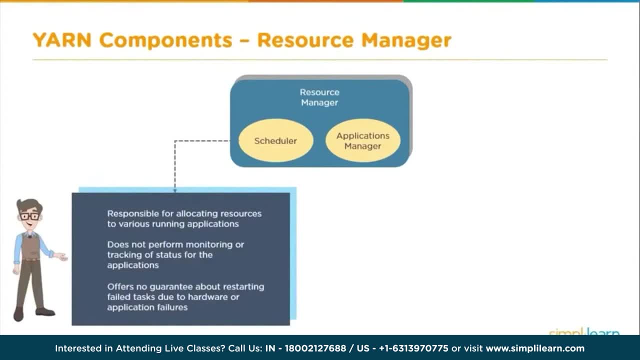 We could have a FIFO scheduler, So there are different schedulers which take care of resource allocation. So your scheduler is responsible for allocating resources to various running applications. Now imagine a particular environment where you have different teams or different departments which are working on the same cluster. So we would call the cluster as a 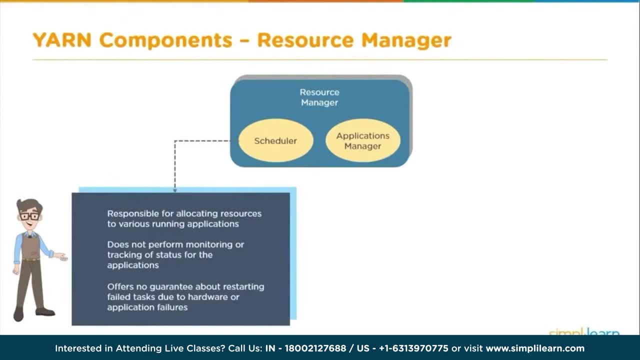 multi-tenant cluster and on the multi-tenant cluster you would have different applications which would want to run simultaneously accessing the resources. How is that managed? So there has to be some component which has a concept of pooling or queuing, so that different departments or different users can get dedicated resources or can share resources. 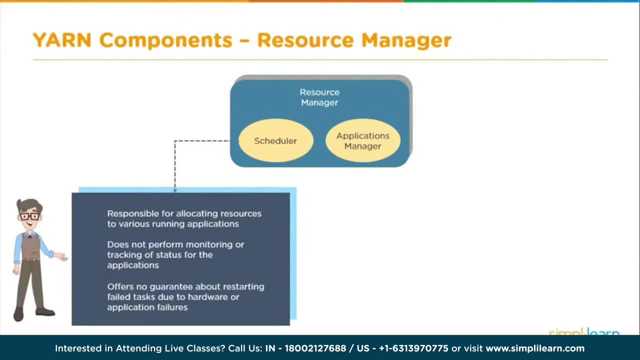 on the cluster. So scheduler is responsible for allocating resources to various running applications. Now it does not perform monitoring or tracking of the status of applications. That's not the part of scheduler. It does not offer any guarantee about restarting the failed tasks due to hardware or 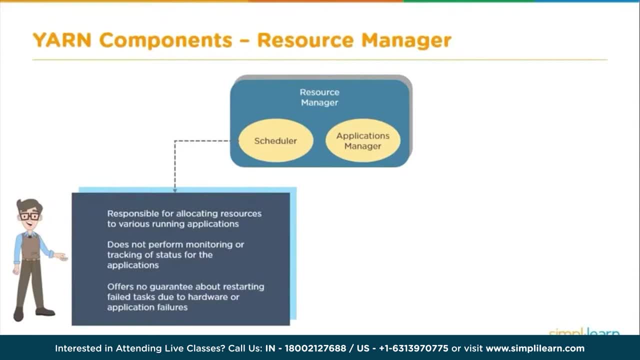 network or any other failures. Scheduler is mainly responsible for allocating resources. Now, as I mentioned, you could have different kinds of schedulers. You could have a FIFO scheduler, which was mainly in older version of Hadoop, which stands for first in first out. 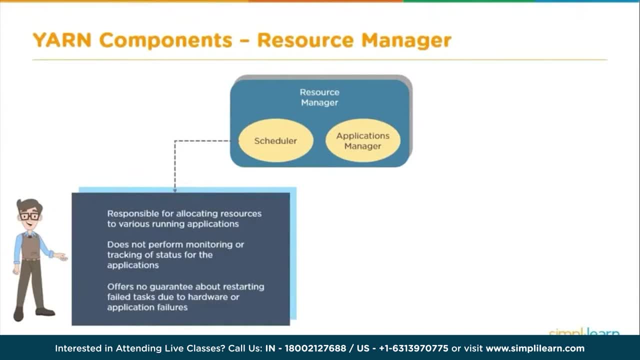 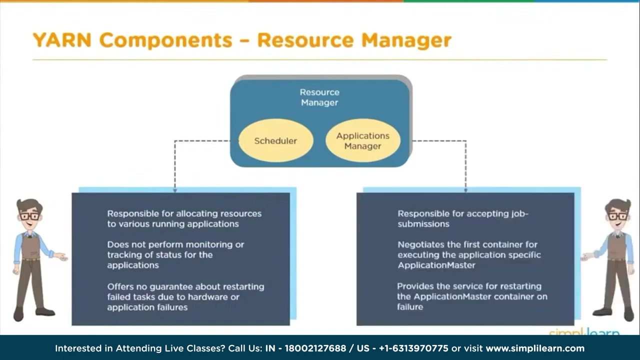 You could have a fair scheduler, which basically means multiple applications could be running in the cluster and they would have a fair share of the resources. You could have a capacity scheduler, which would basically have dedicated or fixed amount of resources across the cluster. Now, whichever scheduler is being used, scheduler is mainly responsible for allocating resources. 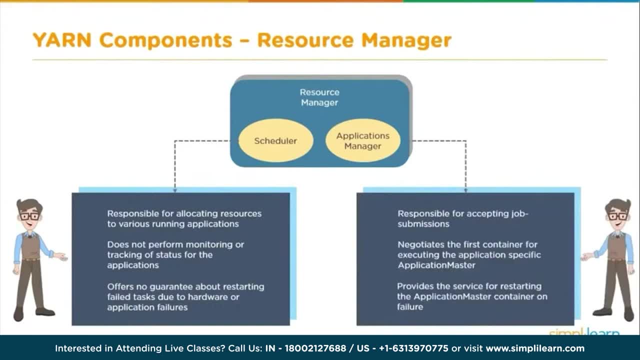 Then it's your applications manager. Now this is responsible for accepting job submissions. Now, as I said, at higher level, we could always say resource managers doing everything, It is negotiating the resources. It is negotiating the resources. It is also taking care of listening to. 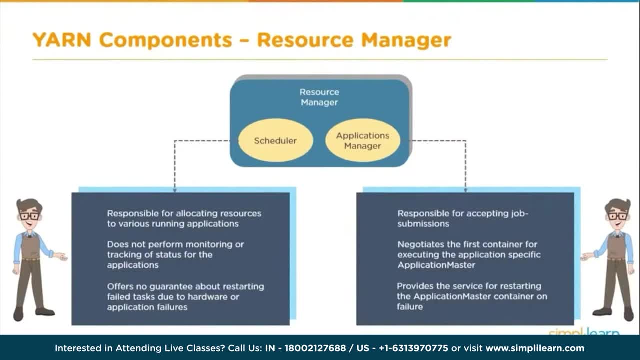 the clients and taking care of job submissions. But who is doing it in real? It is these components. So you have applications manager, which is responsible for accepting job submissions. It negotiates the first container for executing the application. specific application master. It provides the service for restarting the application master. Now how does this work? 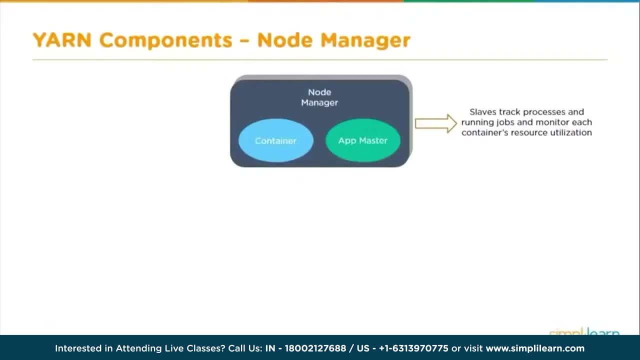 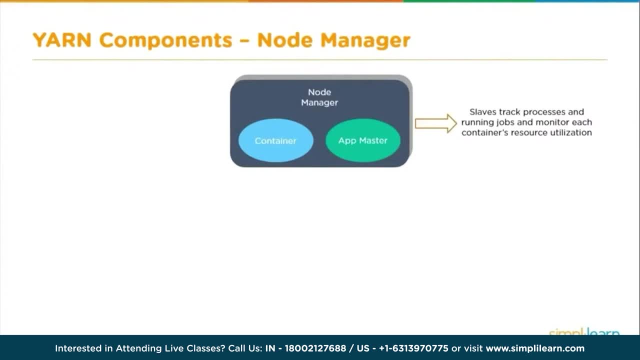 It is tracking the processes, It is taking care of running the jobs And, basically, it is tracking each container resource utilization. So let's understand what is this container? So normally when you talk about an application request which comes from a client, so let's say this: 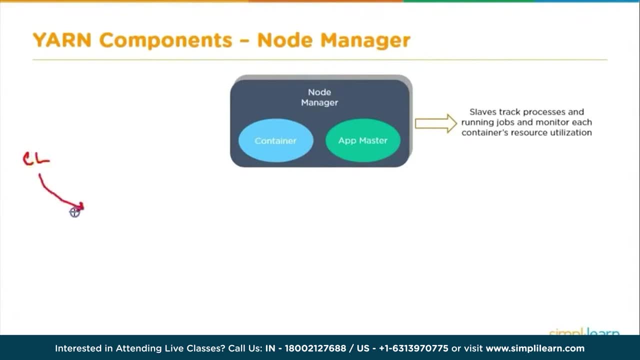 is my client which is requesting, or which is coming up with an application which needs to run on the cluster. Now, this application could be anything. It first contacts your master, That's, your resource manager, which is the master for your processing layer. Now, as I mentioned, and 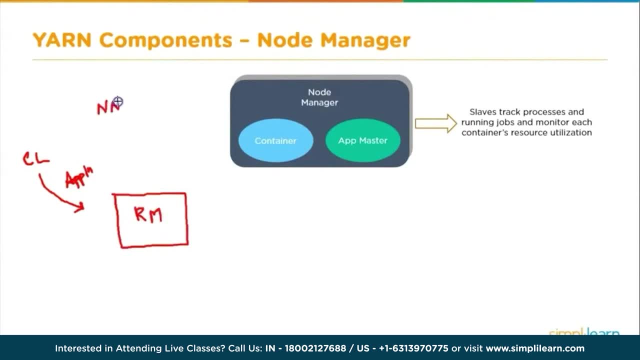 as we already know, that your name node, which is the master of your cluster, has the meta data in its RAM, which is aware of the data being split into blocks, the blocks when stored on multiple machines and other information. so obviously there was a interaction with the master, which has given this information of the relevant. 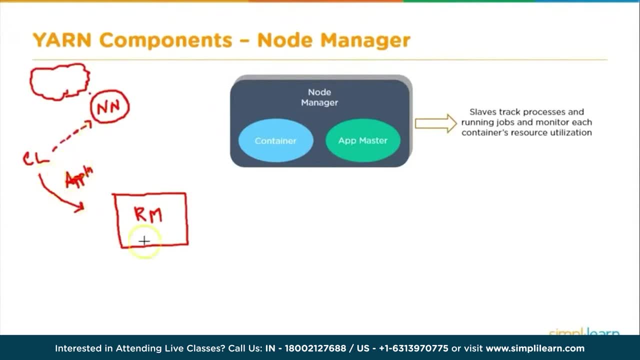 nodes where the data exists. now for the processing need, your client, basically the application which needs to run on the cluster. so your resource manager, which basically has the scheduler, which takes care of allocating resources, and a resource manager has mainly these two components which are helping it to do its work. now for a particular application which might be needing: 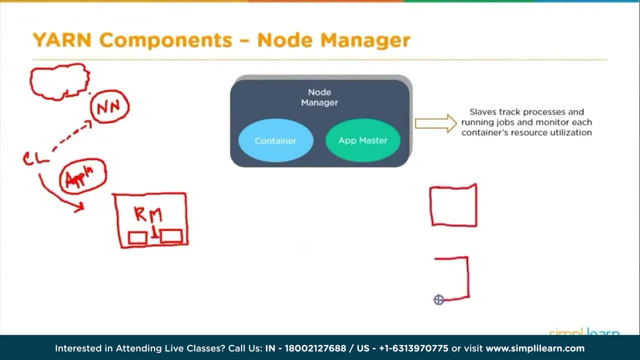 data from multiple machines. now we know that we would have multiple machines where we would have node manager running, we would have a data node running and data nodes are responsible for storing the data on disk. so your resource manager has to negotiate the resources now. when i say 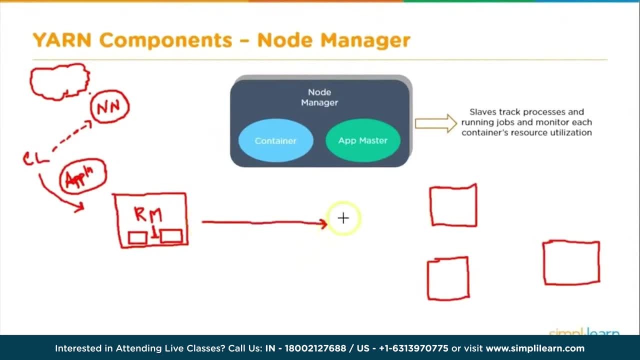 negotiating the resources. it could basically ask each of these node managers for some amount of resources. for example, it would be saying: can i have one gb of ram and one cpu core from you, because there is some data residing on your machine and that needs to be processed as part of my application. can i again have one gb and? 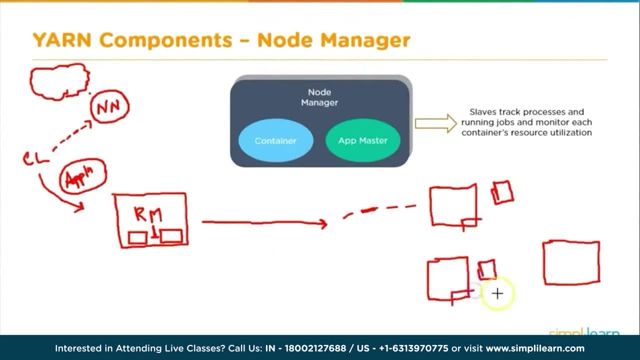 one cpu core from you, and this is again because some relevant data is stored and this request which resources manager makes of holding the resources, of total resources which the node manager has, your resource manager is negotiating or is asking for resources from the processing slave. so this request of 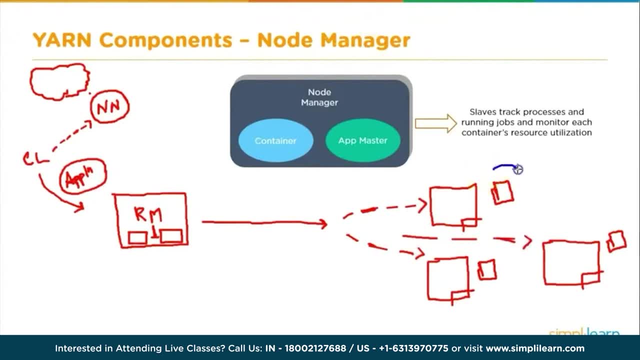 holding resources can be considered as a container. so resource manager- now we know it is not actually the resource manager, but it is the application manager which is negotiating the resources. so it negotiates the resources which are called container. so this request of holding resource can be considered as a container. so, basically, a container can be of different sizes. we will talk. 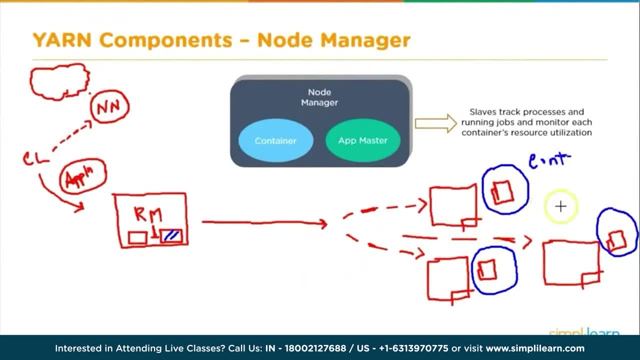 about that. so resource manager negotiates the resources with node manager. now node manager, which is already giving an update of the resources it has, what amount of resources it holds, how much busy it is, it can basically approve the status on the container so that inside the container it is. 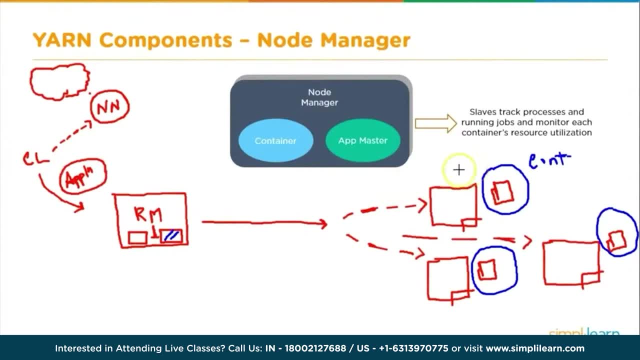 doing the same. so basically the result is, of course the container has to be ужас. who is doing the samevariations or deny this request. so node manager would basically approve in saying, yes, I could hold these resources, I could give you this container of this particular 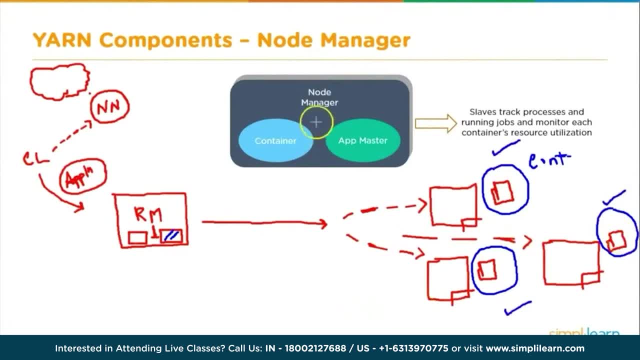 size. now, once the container has been approved or allocated- or you can say granted- by your node manager, resource manager now knows that resources to process the application are available and guaranteed by the node manager. so resource manager starts a temporary daemon called app master. so this is a 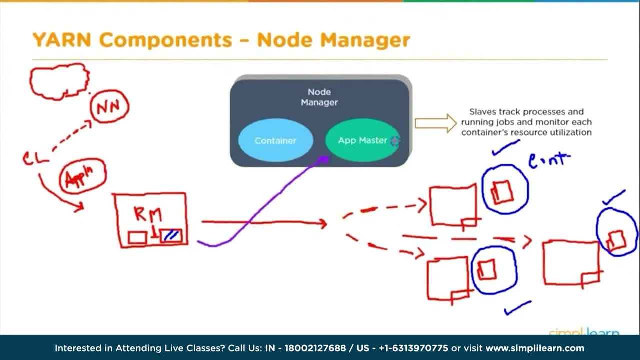 piece of code which would also be running in one of the containers. it would be running in one of the containers which would then take care of execution of tasks in other containers. so your application master is per application. so if I would have ten different applications coming in from, 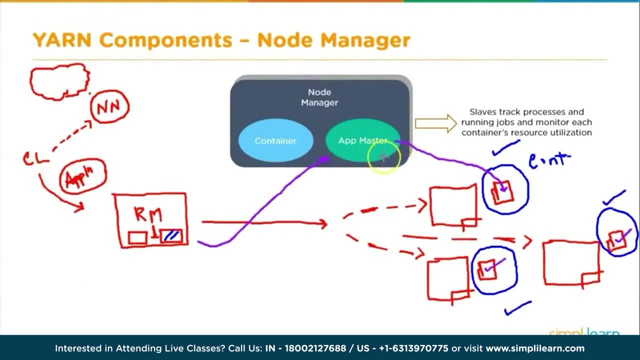 the client. then we would have ten app masters, one app master being responsible for per application. now what does this app master do? it basically is a piece of code which is responsible for execution of the application. so your app master would run in one of the containers and then it. 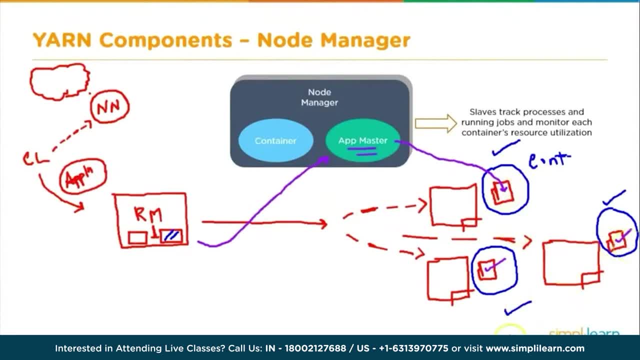 would use the other containers which node manager is guaranteed that it will give when the request, application request comes to it, and using these containers the app master will run the processing tasks within these designated resources. so it is mainly the responsibility of application master to get the execution done and then 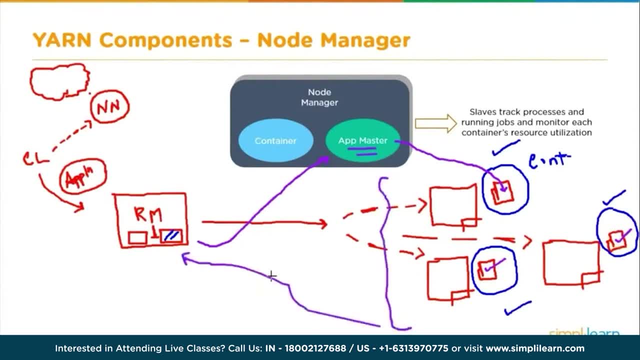 communicate it to the master. so resource manager is tracking the resources, it is negotiating the resources and once the resources have been negotiated, it basically gives the control to application master to application master is then running within one of the containers on one of the nodes and using the other containers to take care of. 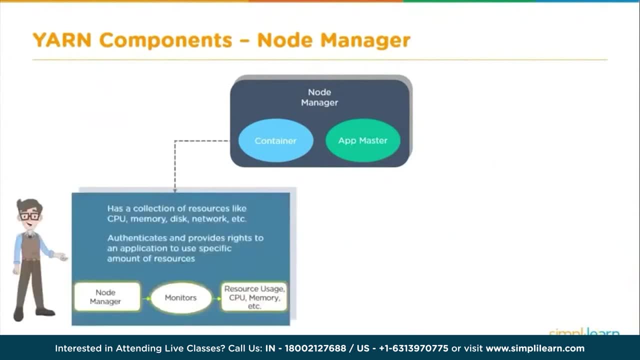 execution. this is how it looks. so basically, container, as i said, is a collection of resources like cpu memory, your disk which would be used or which already has the data and network. so your node manager is basically looking into the request from application master and it basically is granting this request or basically is allocating 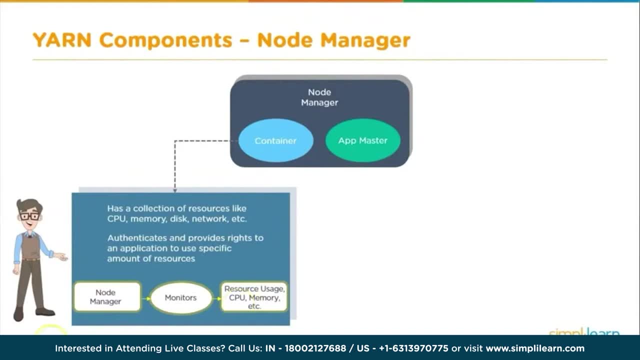 these containers. now again, we could have different sizing of the containers. let's take an example here. so, as i mentioned, from the total resources which are available for a particular node, some portion of resources are allocated to the node manager. so let's imagine this is my node, where 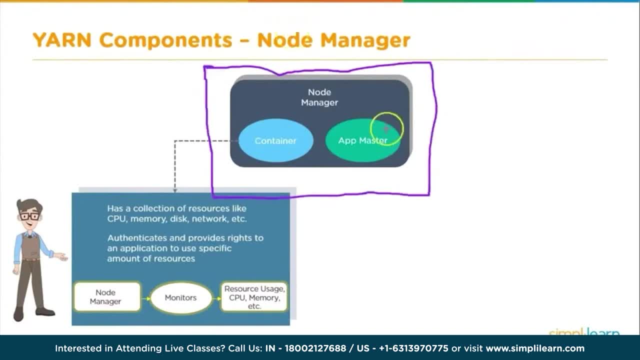 node manager, as a processing slave, is running. so from the total resources which the node has, some portion of ram and cpu cores is basically allocated to the node manager. so i could say out of total 100 GB RAM we can say around 60 cores which the particular node has. so this is my RAM. 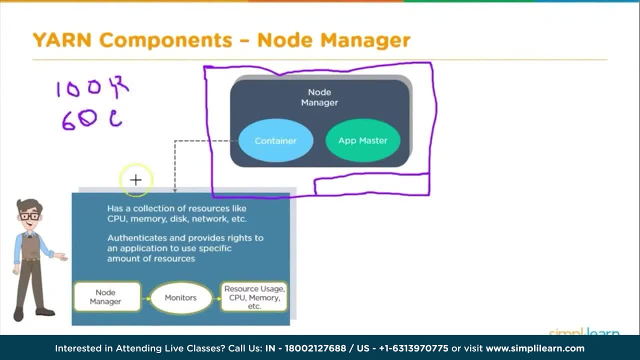 which the node has, and these are the CPU cores which the node has, some portion of it right, so we can say might be 70 percent or 60 percent of the total resources. so we could say around 60 GB RAM and then we could say around 40 V cores have been allocated to node manager. so there are these. 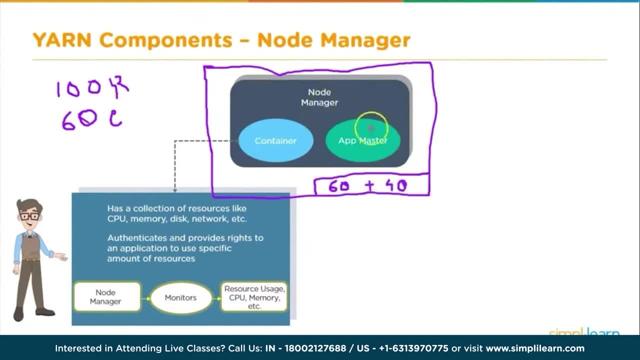 settings which are given in the yarn hyphen site file. now, apart from this allocation, that is, 60 GB RAM and 40 V cores, we also have some properties which say what will be the container sizes. so, for example, we could have a small container setting which could say my every container. 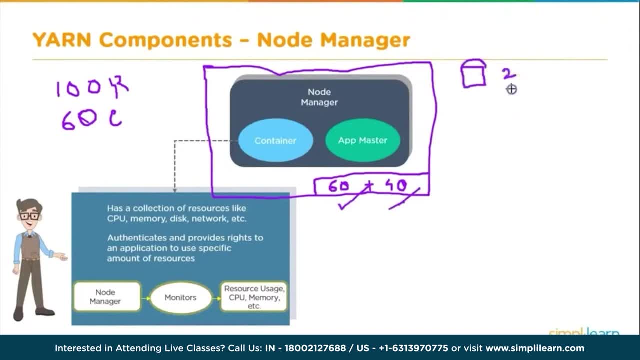 container is 60 GB RAM and then we could say around 40 V cores have been allocated to node manager, could have 2 GB RAM and say one virtual CPU core. so this is my smallest container. so based on the total resources, you could calculate how many such small containers could be running. so if I say 2 GB, 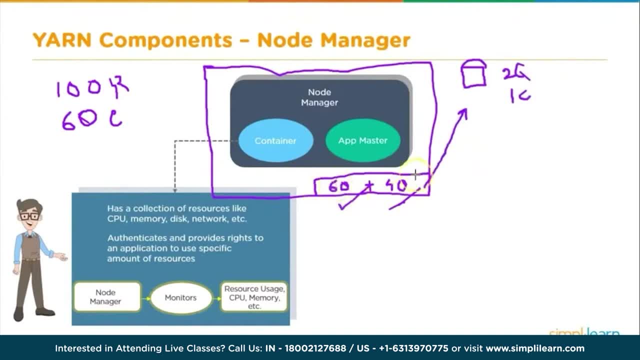 RAM, then I could have around 30 containers, but then I'm talking about one virtual CPU core. so totally, I could have around 30 small containers which could be running in parallel on a particular node and, as of that calculation, you would say 10 CPU cores are not being utilized. you could have a. 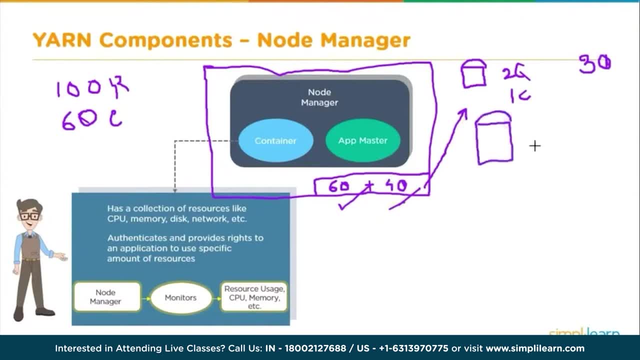 bigger container size which could say I would go for 2 CPU cores and 3gb RAM. so 3gb RAM and 2 CPU cores, so that would give me around 20 containers of bigger size. so this is the container sizing which is again defined in the yarn hyphen site file. so what we know is on a particular node which has 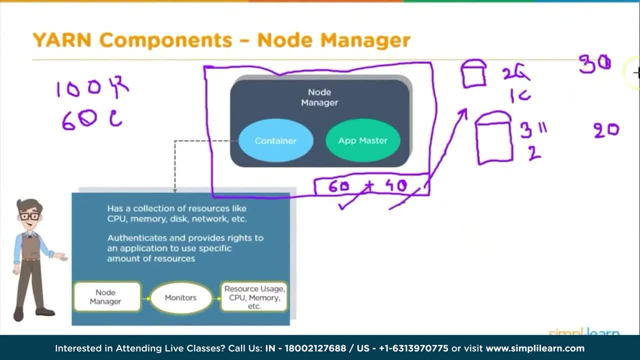 this kind of allocation. either we could have 30 small containers running or we could have 20 big containers running, and same would apply to multiple nodes. so node manager, based on the request from application master, can allocate these containers. now, remember, it is within this one of these containers you would. 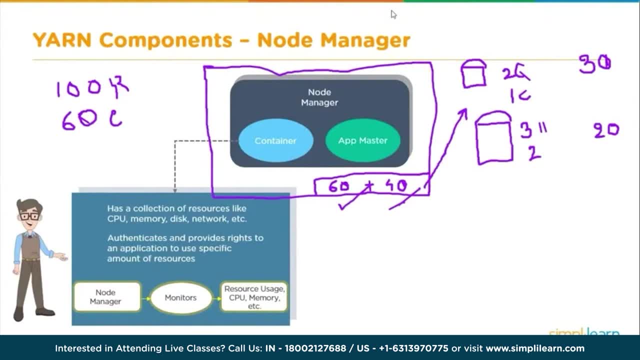 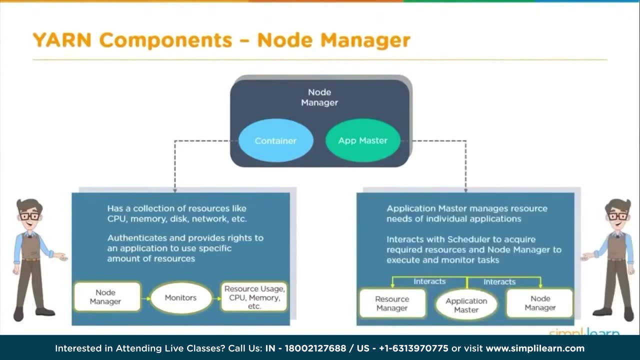 have an application master running and other containers could be used for your processing requirement. application master, which is per application, it is the one which uses these resources. it basically manages or uses these resources for individual application. so remember, if we have 10 applications running on yarn, then it would be 10 application masters, one responsible for 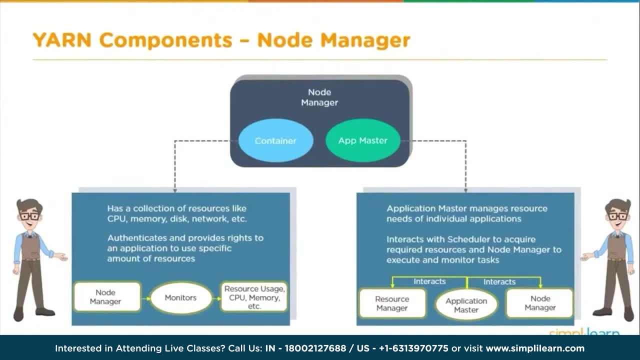 each application. your application master is the one which also interacts with the scheduler to basically know how much amount of resources could be allotted for one application, and your application master is the one which uses this- these resources- but it can never negotiate for more resources to node manager. application master. 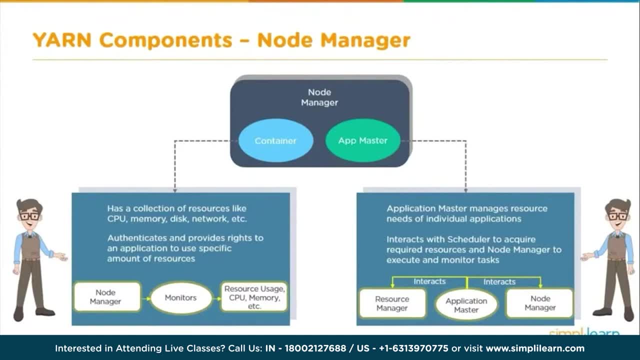 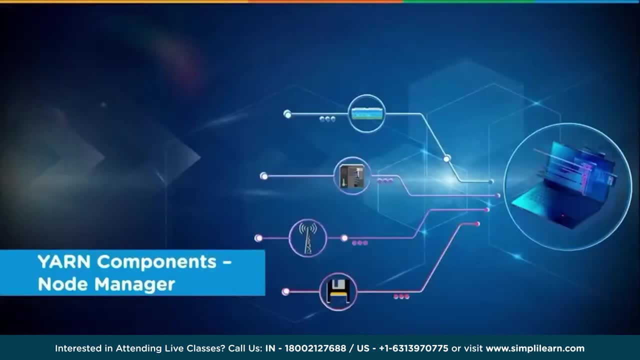 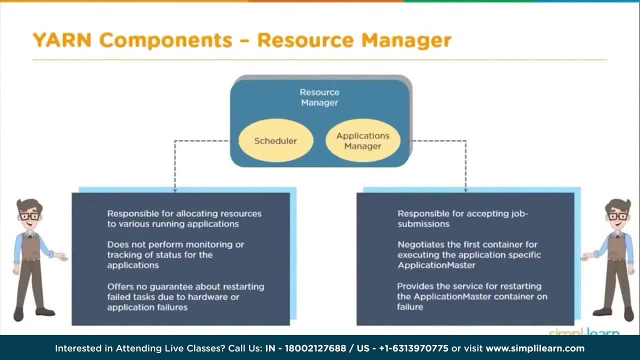 cannot do that. application master has to always go back to resource manager if it needs more resources. so it is always the resource manager- and internally resource manager's component, that is, application manager- which negotiates the resources at any point of time, due to some node failures or due to any other requirements, if application master needs more resources. 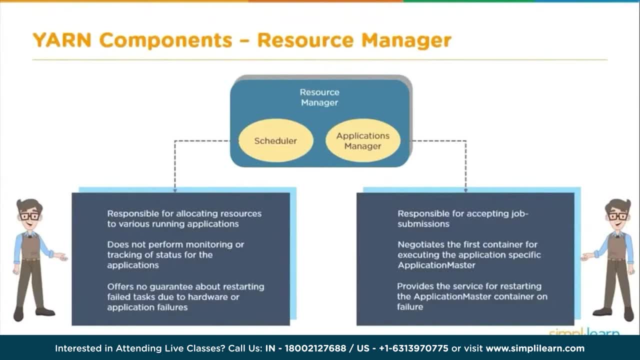 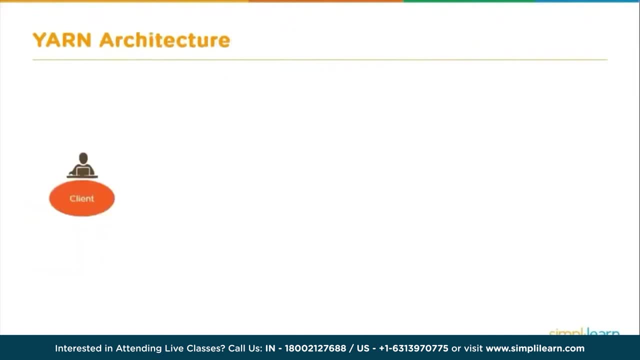 on one or multiple nodes, it will always be contacting the resource manager internally, the applications manager, for more containers. now this is how it looks. so your client submits the job request to resource manager. now we know that resource manager internally has scheduler and applications manager node managers which are running on multiple machines. 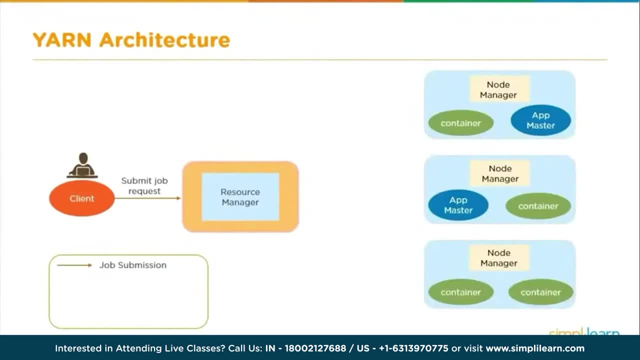 are the ones that are running on multiple machines. so if your client submits the job request to once, which are tracking their resources, giving this information to resource manager so that resource manager, or i would say its component applications manager, could request resources from multiple node managers. when i say request resources, it is these containers, so your resource. 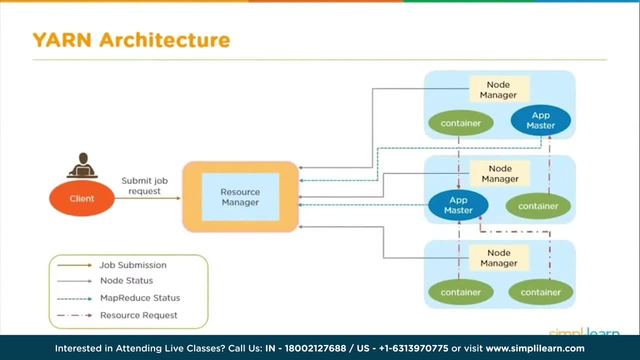 manager basically will request for the resources on one or multiple nodes. node manager is the one which approves these containers and once the container has been approved, your resource manager triggers a piece of code that is application master, which obviously needs some resources. so it would run in one of the containers. 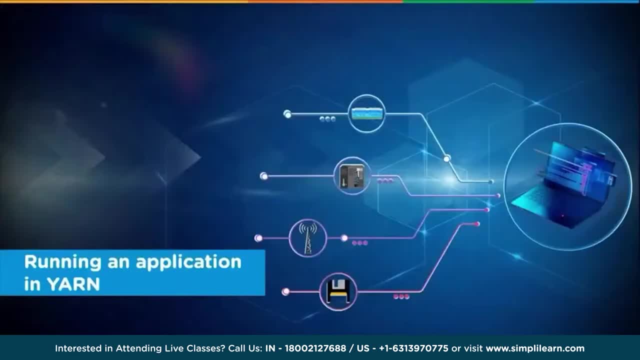 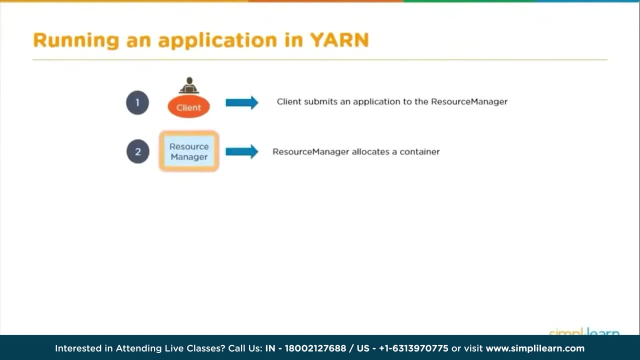 and will use other containers to do the execution. so your client submits an application to resource manager, resource manager allocates a container or i would say this is at a high level- right resource manager is negotiating the resources and internally, who is negotiating the resources? it is your applications manager who is granting this request, it is node manager and that's how we can. 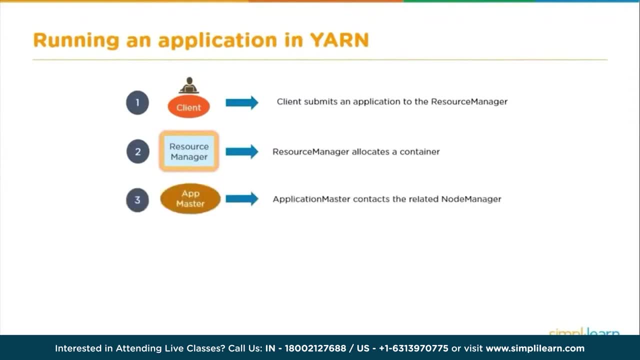 say, resource manager allocates a container, application master basically contacts the related node manager because it needs to use the containers. node manager is the one which launches the container or basically gives those resources within which an application can run. an application master itself will then accommodate itself in one of the containers and then use other containers for. 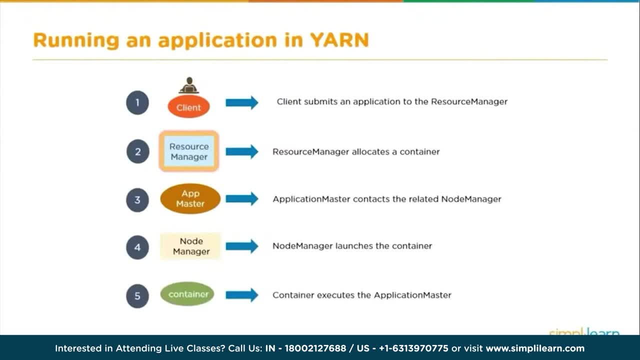 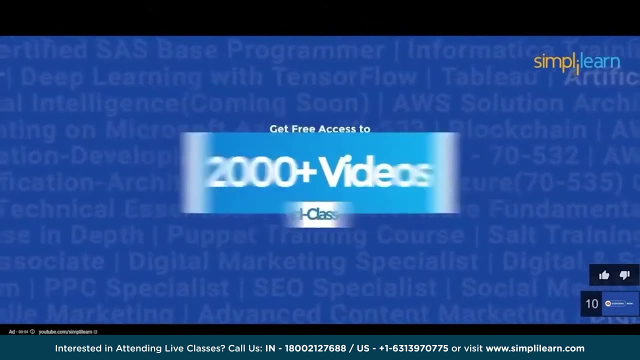 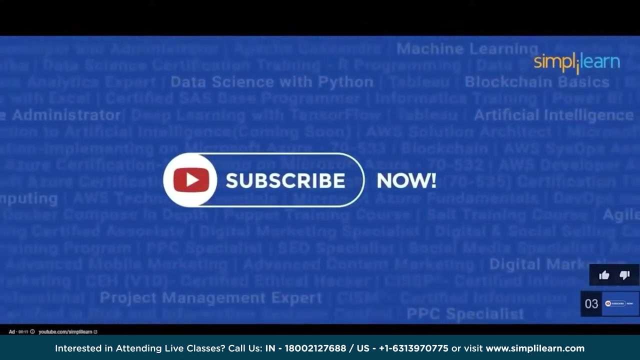 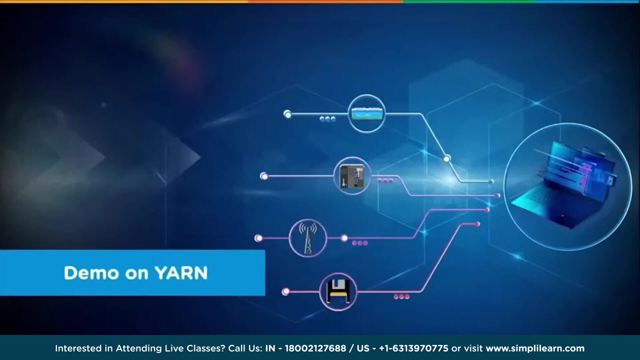 the process processing, And it is within these containers the actual execution happens. Now that could be a map task, that could be a reduce task, that could be a Spark executor taking care of Spark tasks and many other processing. So before we look into the demo on how YARN works, I would suggest looking into one of 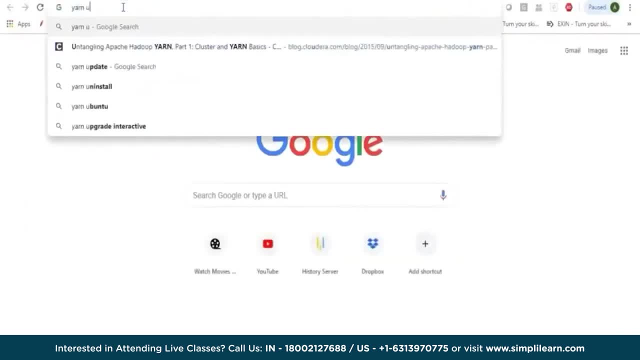 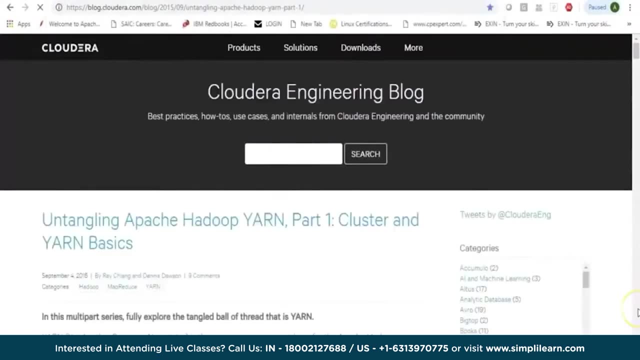 the blogs from Cloudera. So you can just look for YARN Untangling and this is really a good blog which basically talks about the overall functionality which I explained just now. So, as we mentioned here, so you basically have the master process, you have the worker. 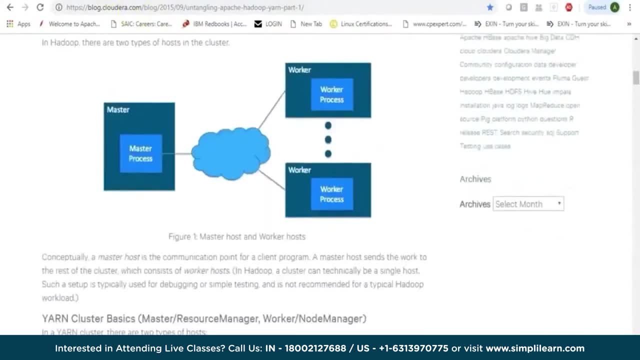 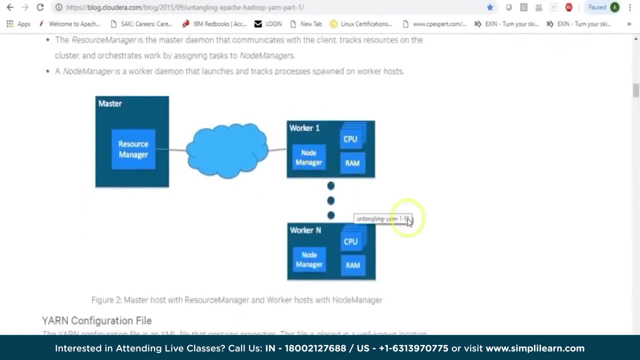 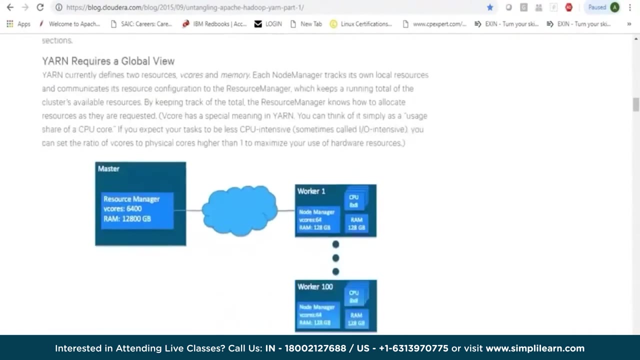 process which basically takes care of your processing, your resource manager being the master And node manager being the slave. This also talks about the resources which each node manager has. It talks about the YARN configuration file where you give all these properties. It basically shows you node manager which reports the amount of resources it has to 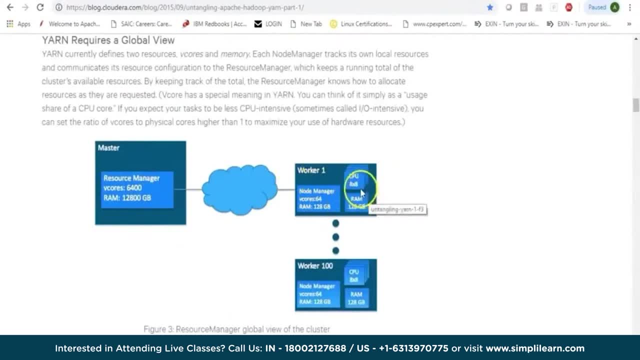 resource manager. Now remember: if worker node shows 8 into 8 CPU cores and 128 GB RAM and if your node manager says 64 V cores and RAM 128 GB, then that's not the total capacity, It is some portion of your node which is allocated to node manager. 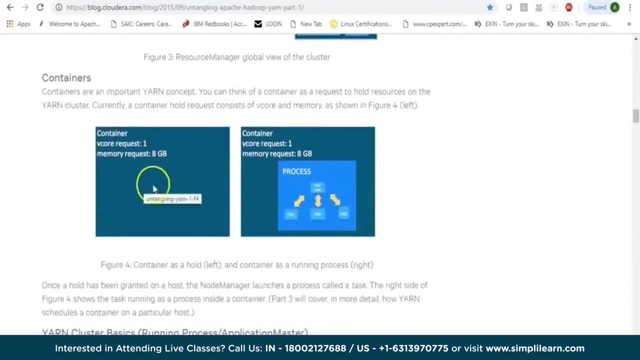 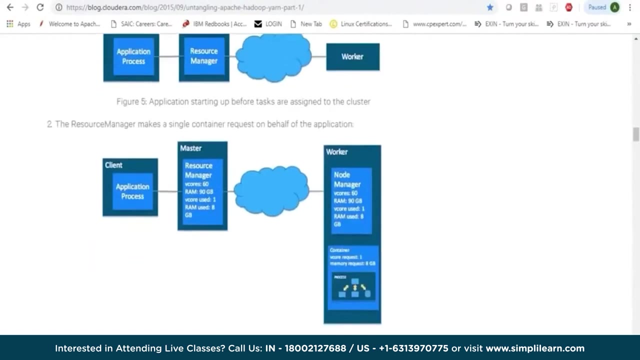 Now, once your node manager reports that your resource manager is requesting for containers based on the application, What is a container? It is basically a logical name given to a combination of V-Core and RAM. It is within this container where you would have basically the process running. 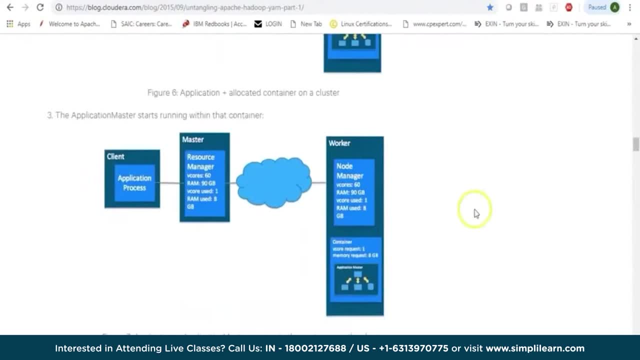 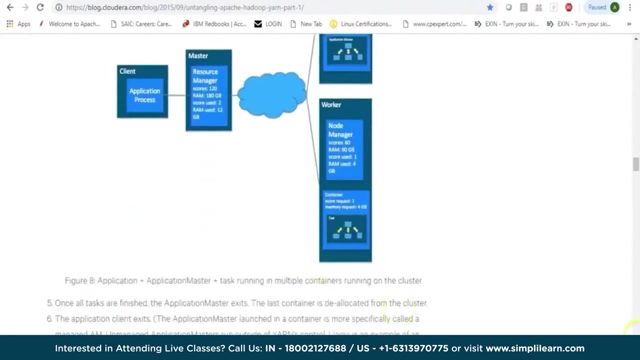 So once your application starts and once node manager is guaranteed these containers, your or your resource manager has basically already started an application master within the container. and what does that application master do? it uses the other containers where the tasks would run. so this is a very good blog which you can refer to, and this also talks about map reduce, if you have. 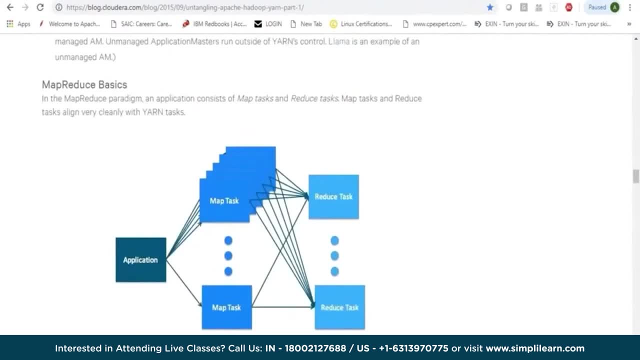 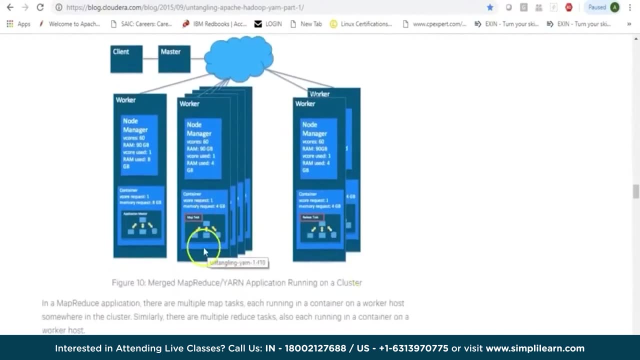 already followed the map reduce tutorials in past, then you would know about the different kind of tasks, that is, map and reduce, and these map and reduce tasks could be running within the container in one or multiple. as i said, it could be map task, it could be reduced task, it could be a spark based. 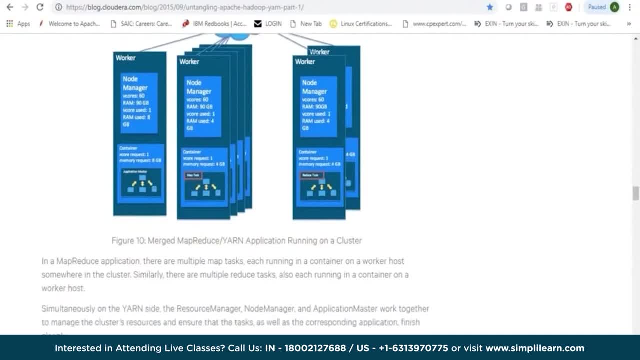 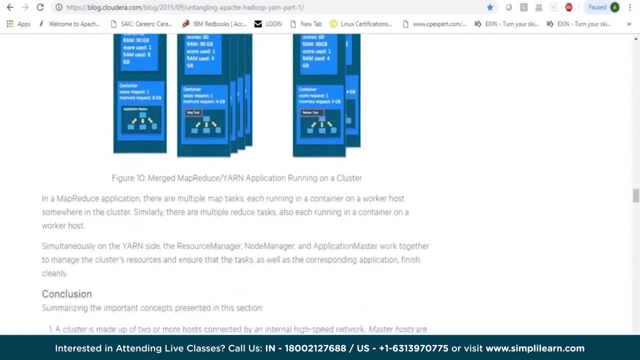 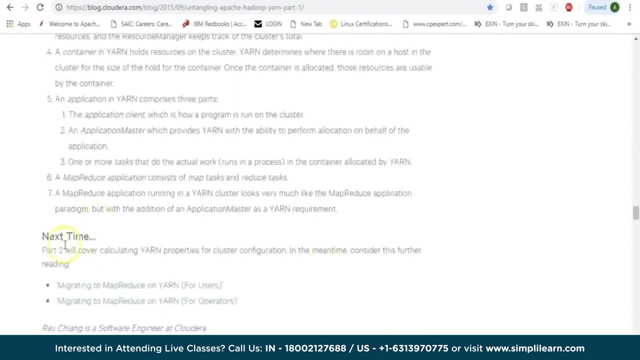 task which would be running within the container now, once the task finishes, basically that resources can be freed up, so the container is released and the resources are given back to yarn so that it can take care of further processing. if you'll further look in this blog, you can also look into 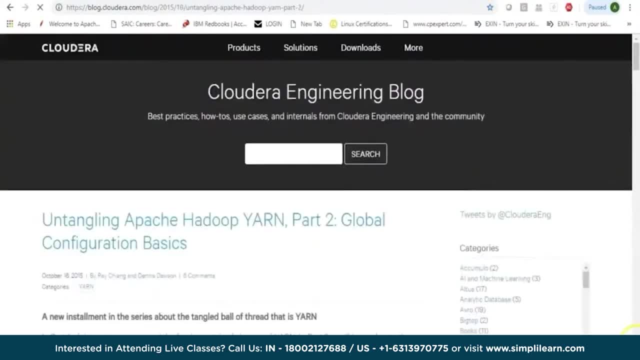 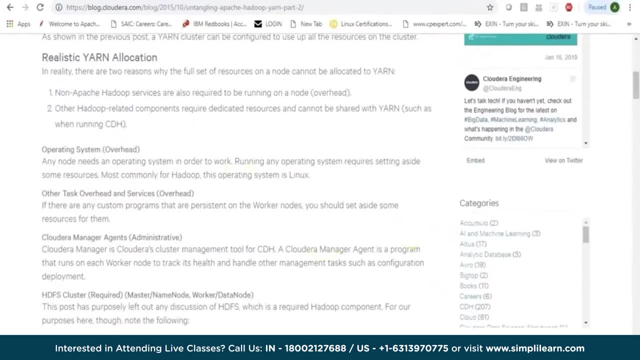 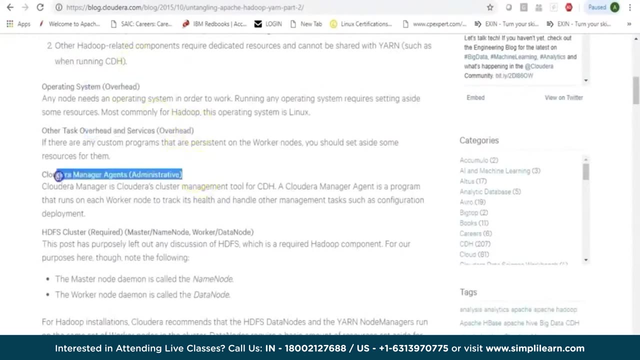 the part two of it, where you talk mainly about configuration settings- you can always look into this- which talks about why and how much resources are allocated to the node manager. it basically talks about your operating system overhead. it talks about other services. it talks about cloud at our hot and works related services running and other processes which might be running. 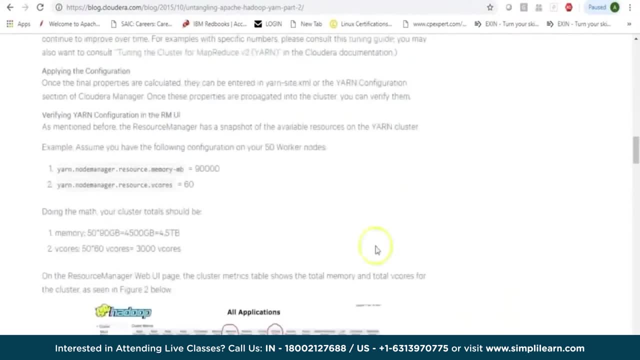 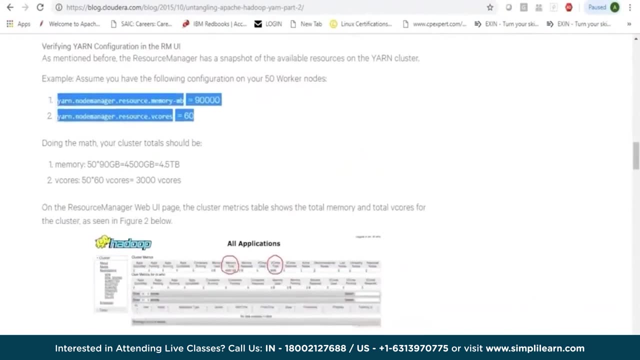 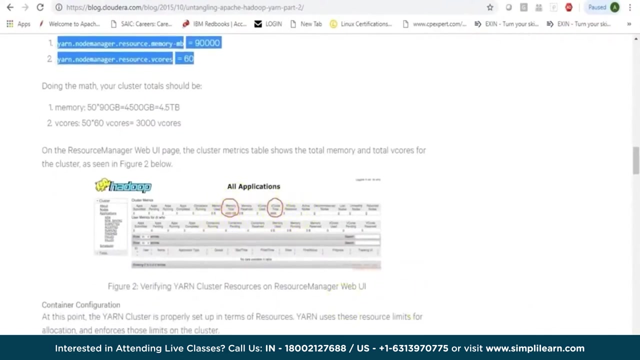 and based on that, some portion of ram and cpu cores would be allocated to node manager. so that's how it would be done in the yarn hyphen site file, and this basically shows you what is the total amount of memory and cpu cores which is allocated to node manager. then, within every machine where you have a node, 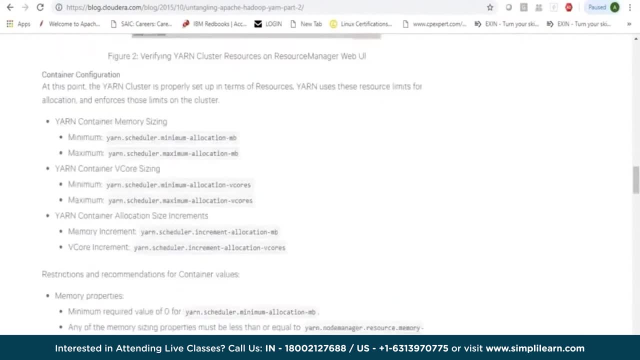 manager, running on every machine, in the yarn hyphen site file, you would have such properties which would say: what is the minimum container size, what is the maximum container size in terms of ram, what is the minimum for cpu cores, what is the maximum for cpu cores and what is the? 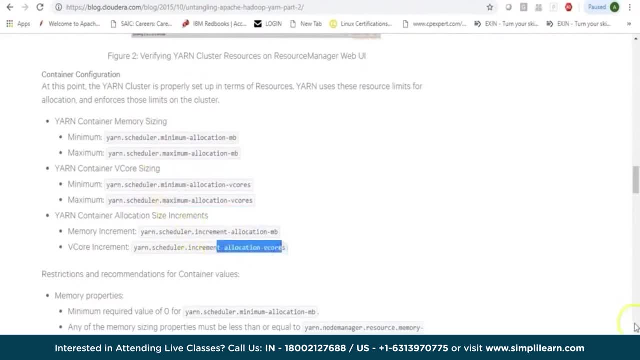 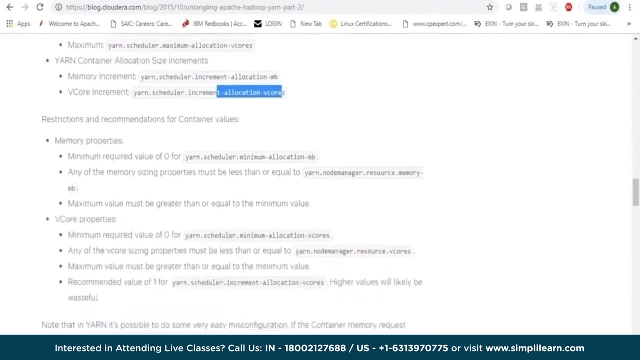 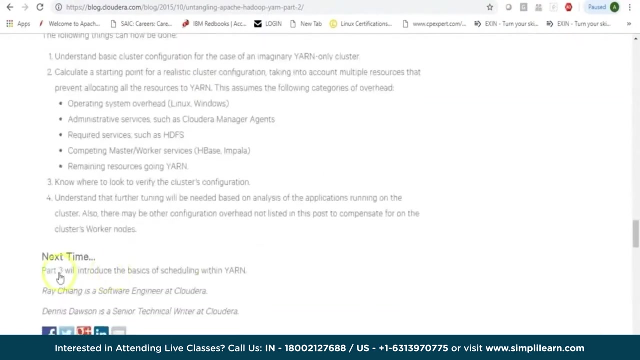 incremental size in where ram and cpu cores can increment. so these are some of the properties which define how containers are allocated for your application request. so have a look at this and this could be a good information which talks about different properties. now you can look further which talks about scheduling, if you look in this particular blog, which also talks. 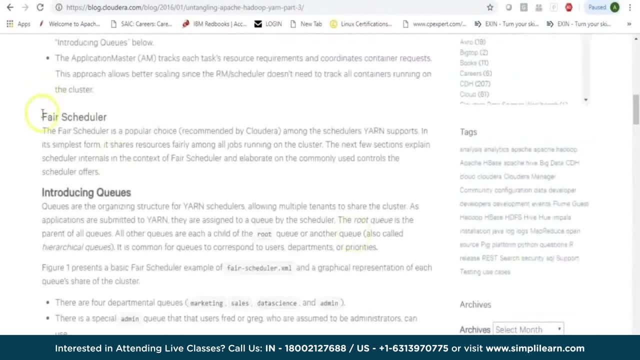 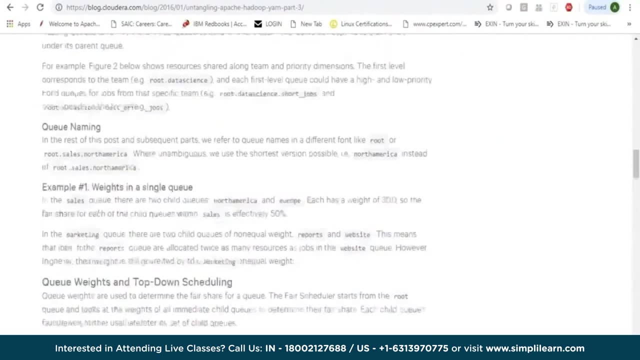 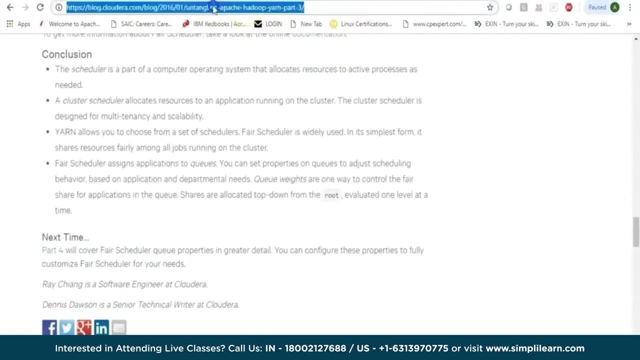 about scheduling, where it talks about scheduling in yarn, which talks about fair scheduler, or you basically having different queues in which allocations can be done. you also have different ways in which queues can be managed. you can also have different ways in which queues can be managed and different schedulers can be used. so you can always look at this series of blog. you can also be 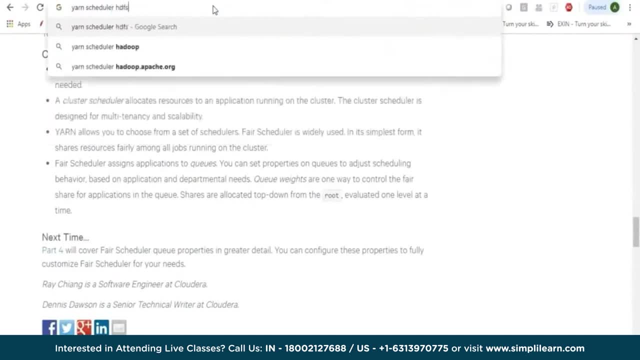 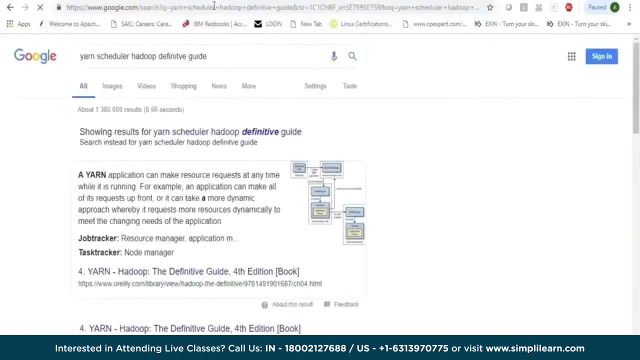 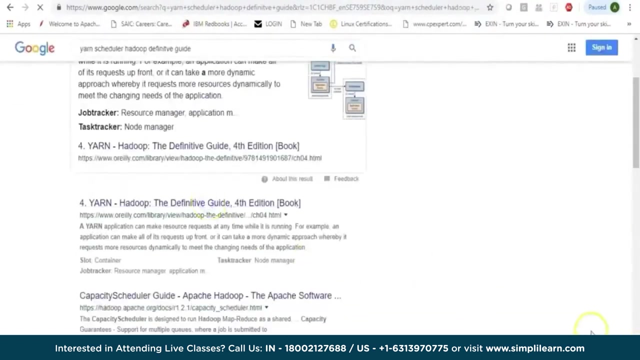 checking for yarn schedulers and then search for uh dupe definitive guide and that could give you some information on how it looks when you look for hadoop definitive guide. so if you look into this book which talks about the different resources as i mentioned, so you could have a fifo scheduler. 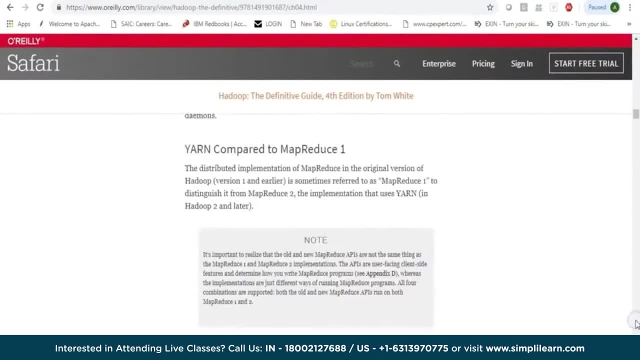 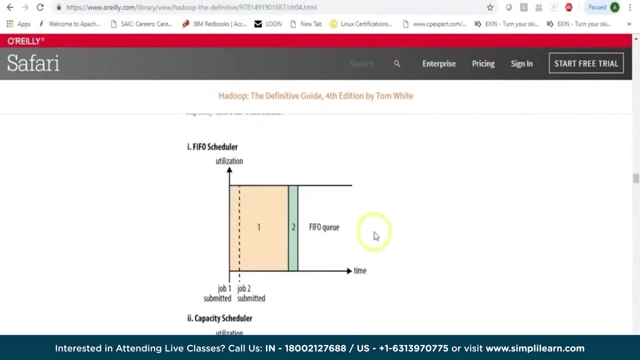 that is first in, first out, which basically means if a long running application is submitted to the cluster, all other small running applications will have to wait. there is no other way. but that would not be a preferred option. if you look in fifo scheduler, if you look for capacity scheduler, 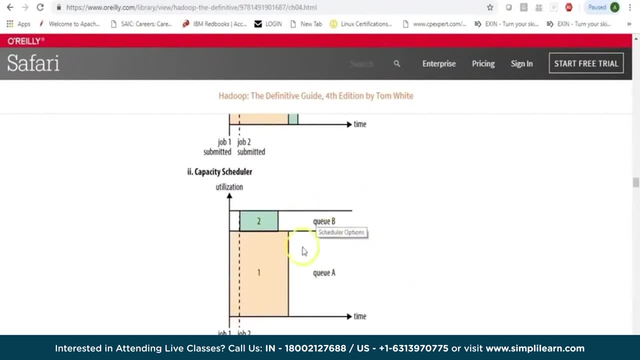 it basically means that you could have different queues created and those queues would have resources allocated. so then you could have a production queue where production jobs are running in a particular queue which has fixed amount of resources allocated. you could have a development queue where development jobs are running and both of them are running in parallel. you could then 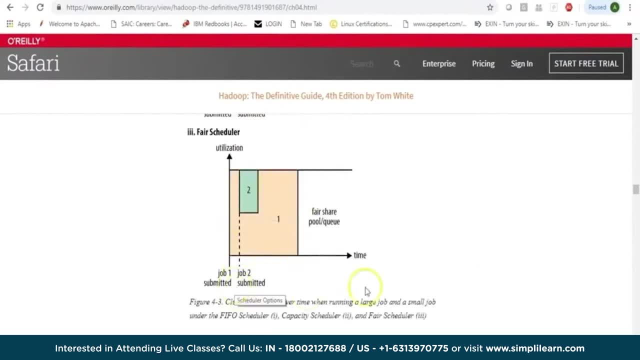 also look into fair scheduler, which basically means, again, multiple applications could be running on the cluster. however, they would have a fair share. so when i say fair share in brief, what it means is if i had given 50 percent of resources to a queue for production and 50 percent of resources. 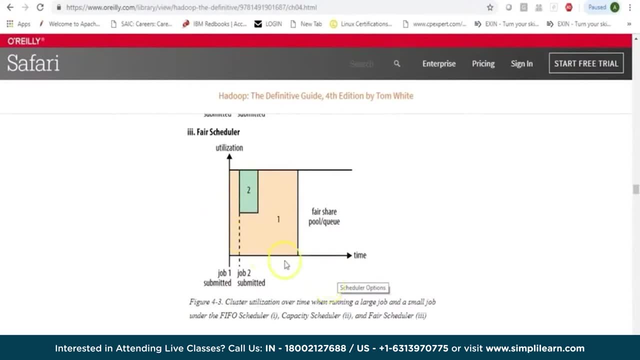 for a production were in the same queue, that will be active on the cluster and then we could have a fair share. so when i say fair share in brief, what it means is if i had given 50 percent of resources queue of development And if both of them are running in parallel, then they would have access. 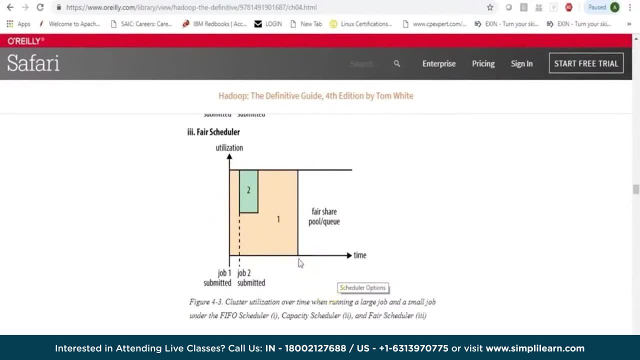 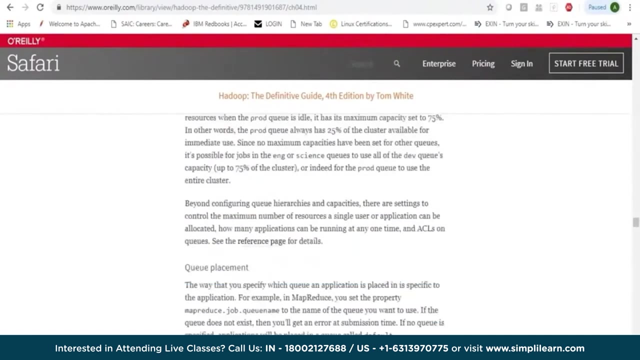 to 50% of cluster resources. However, if one of the queue is unutilized, then second queue can utilize all cluster resources. So look into the fair scheduling part. It also shows you about how allocations can be given and you can learn more about schedulers and how queues can be used. 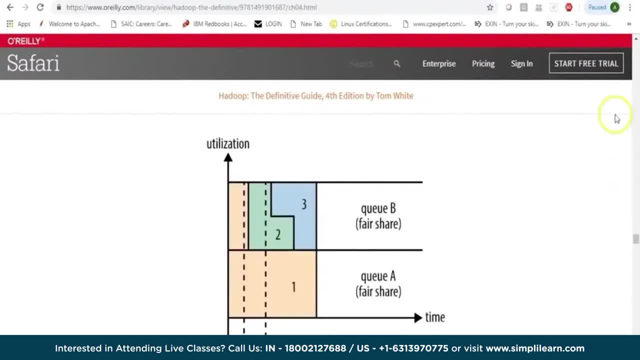 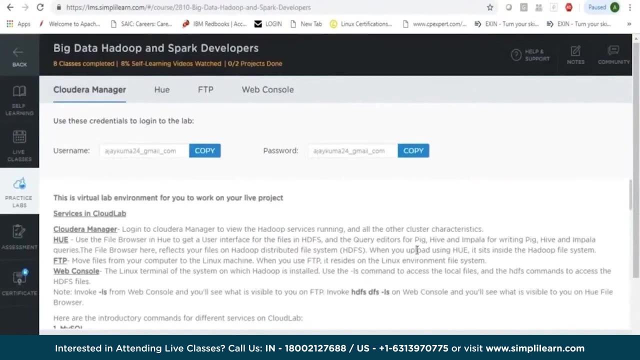 for managing multiple applications. Now we will spend some time in looking into few ways or few quick ways in interacting with YARN in the form of a demo To understand and learn on how YARN works. we can look into a particular cluster. Now here we have a designated cluster which can be used. 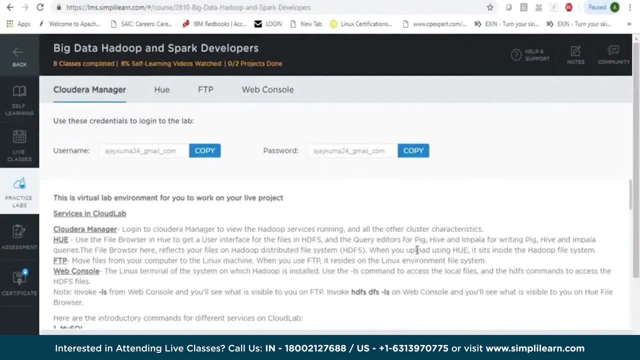 You could be using the similar kind of commands on your Apache-based cluster or a Cloudera Quickstart VM, if you already have it, Or if you have a Cloudera or a Hortonworks cluster running. There are different ways in which we can. 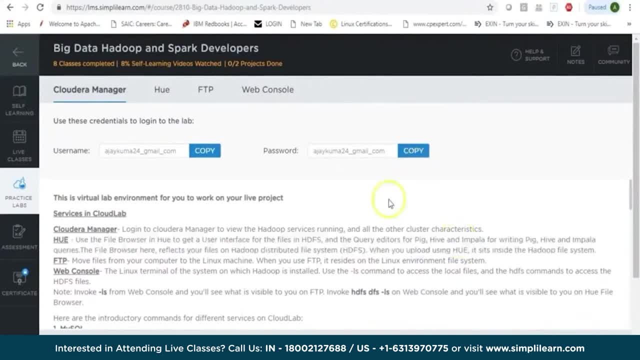 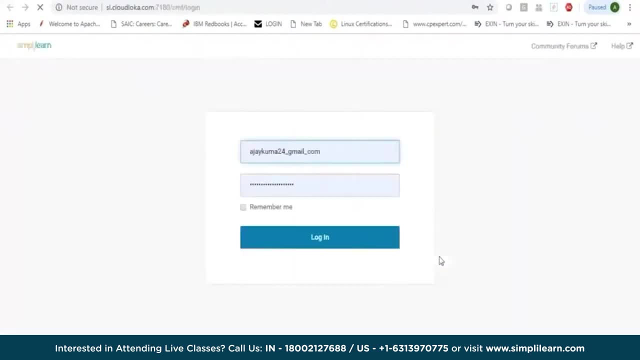 interact with YARN and we can look at the information. One is basically looking into the admin console. So if I would look into Cloudera Manager, which is basically an admin console for a Cloudera's distribution of Hadoop, Similarly you could have a Hortonworks cluster and access. 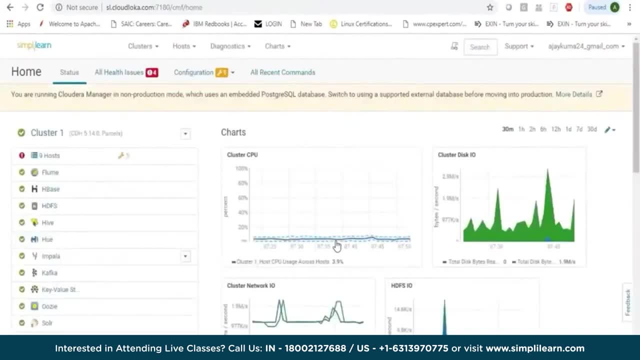 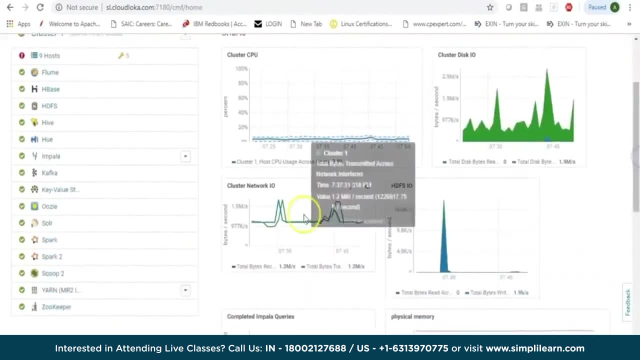 to the admin console. So if you have even read access for your cluster and if you have the admin console, you could have access to the admin console. So if you have even read access for your cluster and access to the admin console, then you can search for YARN as a service which is running. 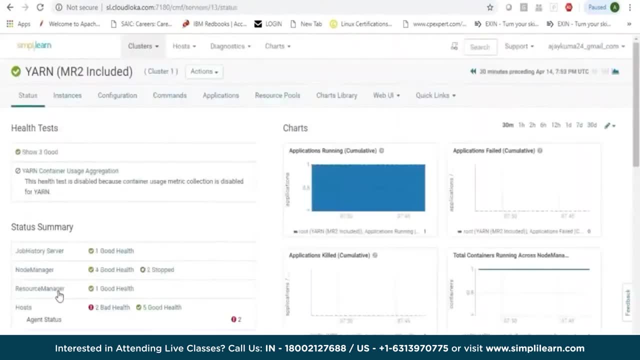 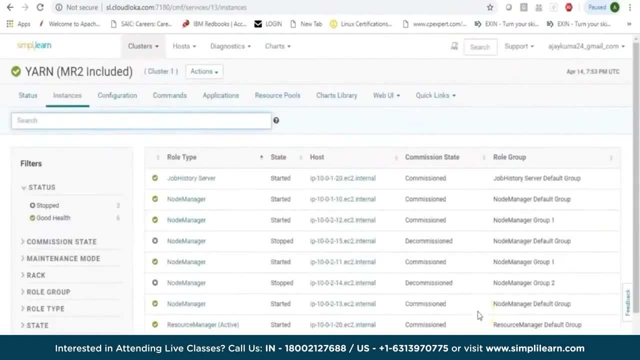 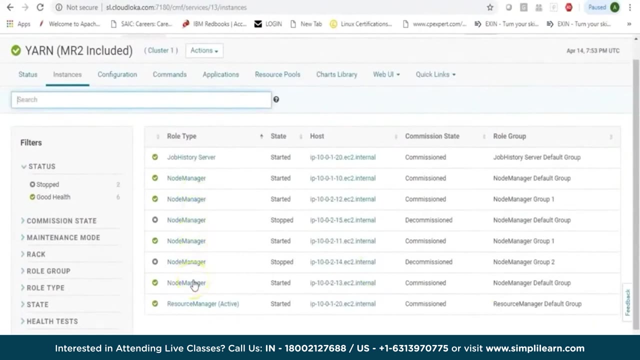 You can click on YARN as a service and that gives you different tabs. So you have the instances, which tells basically what are the different roles for your YARN service running. So we have here multiple node managers. Now, some of them show in stop status, but that's nothing to worry. 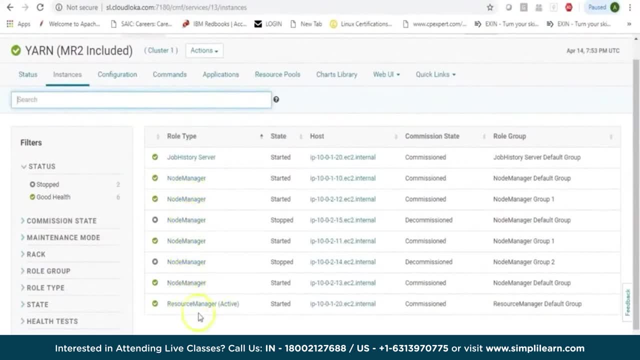 So we have three and six node managers. We have resource manager, which is one, but then that can also be in a high availability where you can have active and standby. You also have a job history server which would show you the applications once they have completed. Now you can look at. 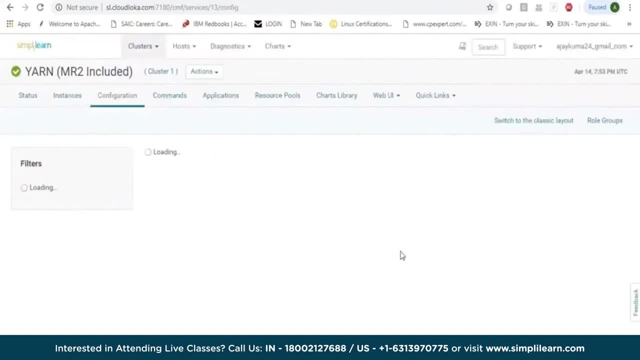 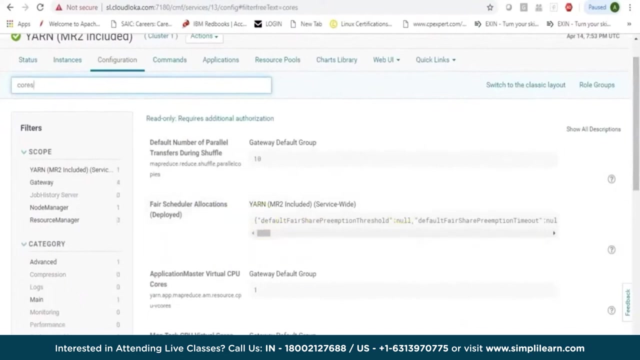 the YARN configurations And, as I was explaining, you can always look for the properties which are related to the allocation. So you can here search, for course, and that should show you the properties which talk about the allocations. So here, if we see, we can be looking for. 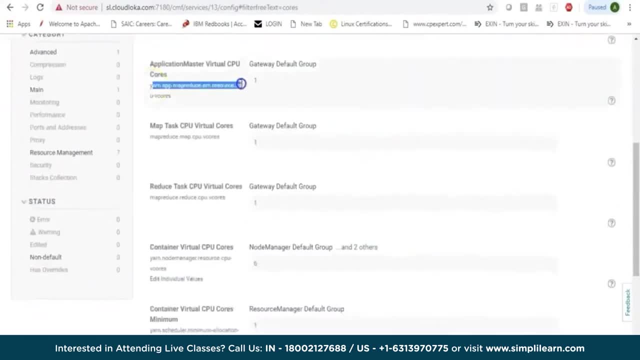 YARN app- MapReduce application master resource CPU course. What is the CPU course allocated for MapReduce, MapTask, ReduceTask? You can be looking at YARN node manager resource CPU course which basically says every node manager on every node would be allocated with six CPU course. 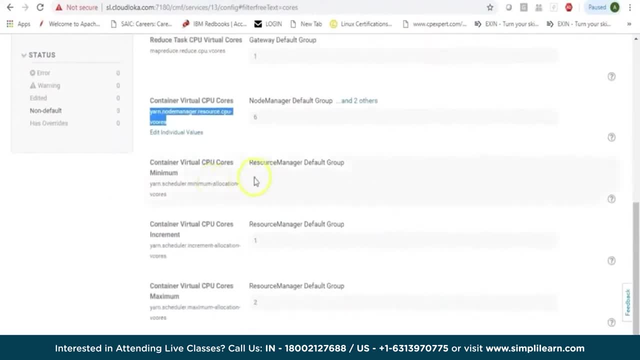 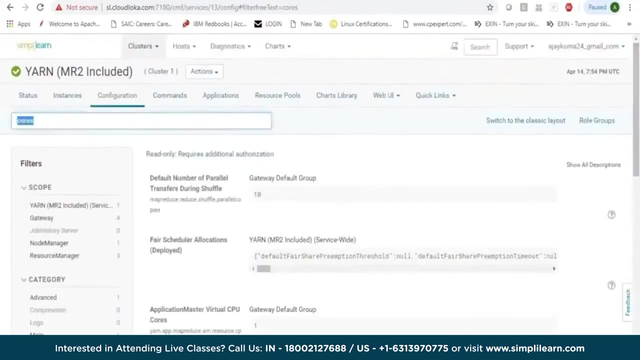 And the container sizing is with minimum allocation of one CPU core and the maximum could be two CPU cores. Similarly, you could also look for the container sizing So you can see here if you could also be searching for memory allocation, and here you could then scroll down to see what kind 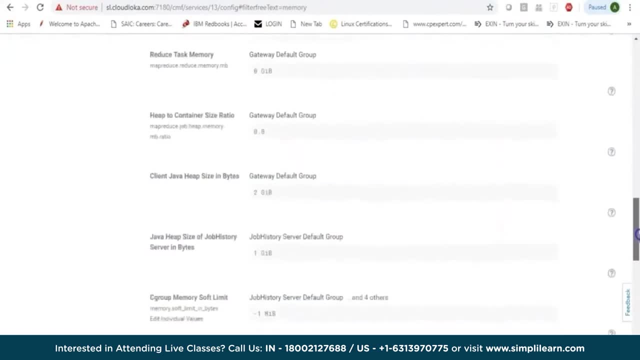 of memory allocation has been done for the node manager. So if we look further, it should give me information of node manager which basically says here that the container minimum allocation is two GB, the maximum is three GB and we can look at node manager which has been given. 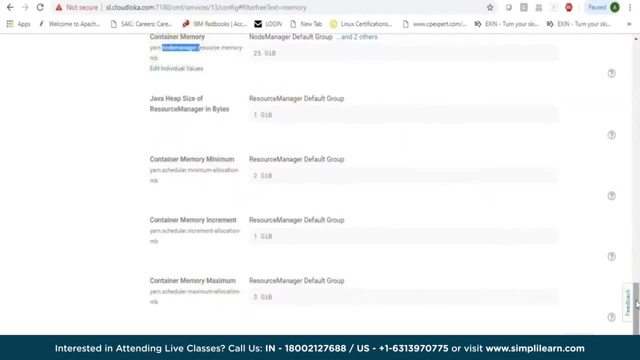 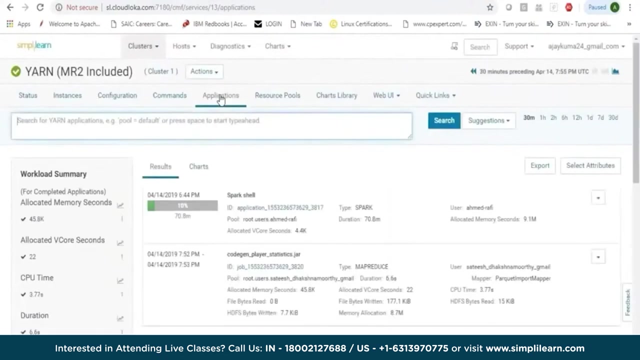 25 GB per node. So that's the total amount of memory allocation of this memory and CPU course, which is the total amount of resources which have been allocated to every node manager. Now we can always look into Applications tab. That would show us different applications which are submitted on YARN For. 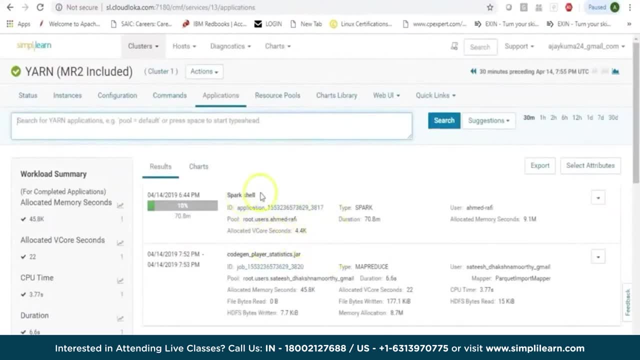 example, right now we see there is a Spark application running, which is basically a user who is using Spark Shell, which has triggered a application on Spark and that is running on YARN applications workload information. you can always do a search based on the. 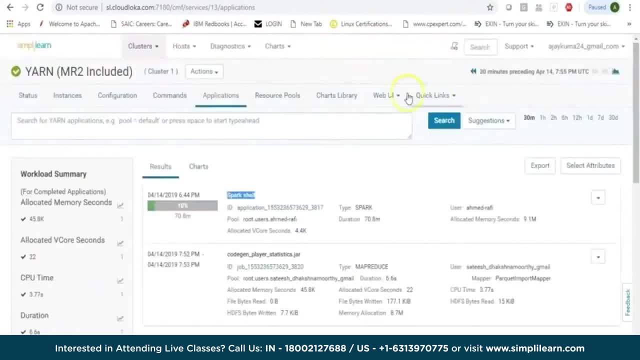 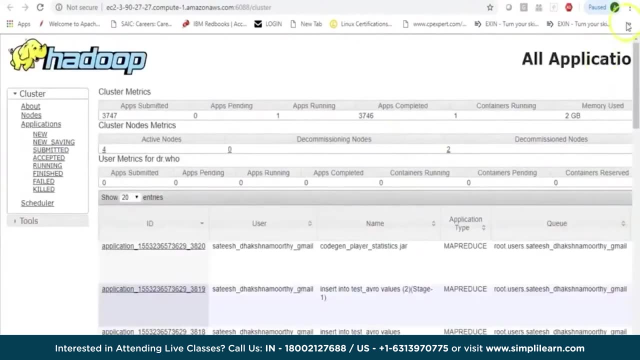 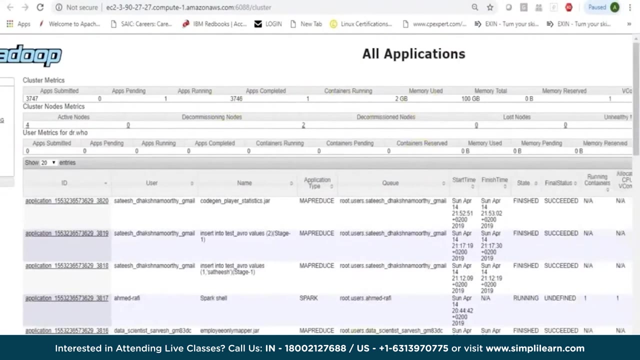 number of days, how many applications have run and so on. you can always go to the web UI and you can be searching for the resource manager web UI and if you have access to that, it will give you overall information of your cluster. so this basically says that here we have 100 GB memory allocated, so that could be. 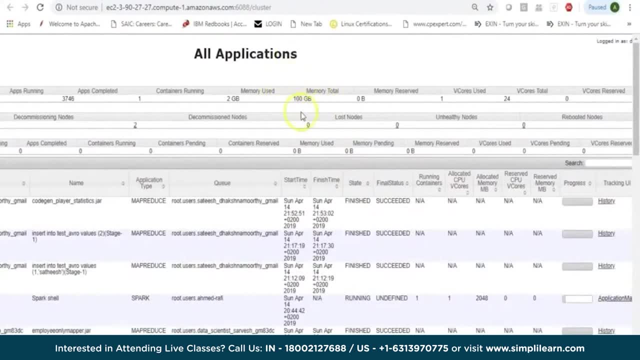 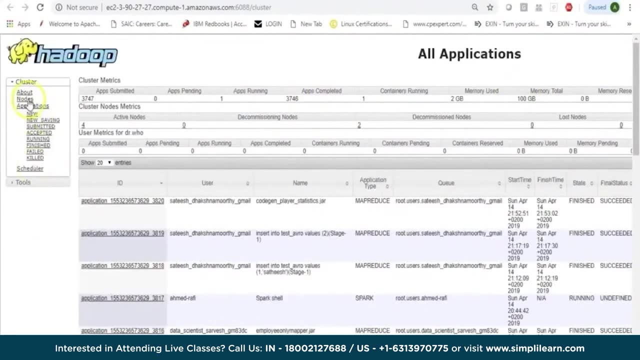 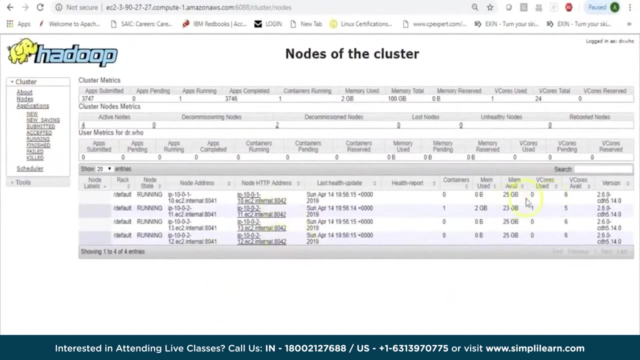 say 25 GB per node, and if we have four node managers running and we have 24 course, which is six course per node. if we look further here into nodes I could get more information. so this tells me that I have four node managers running and node managers basically have 25 GB memory allocated per node and six course. 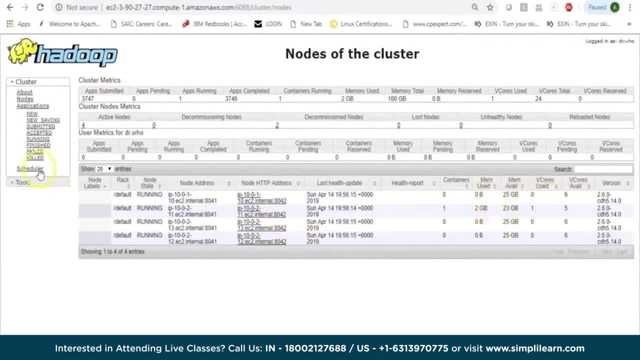 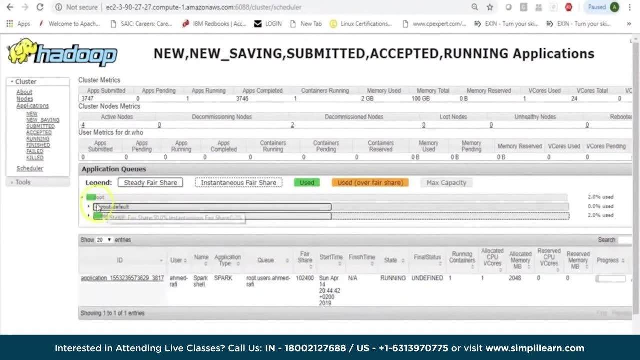 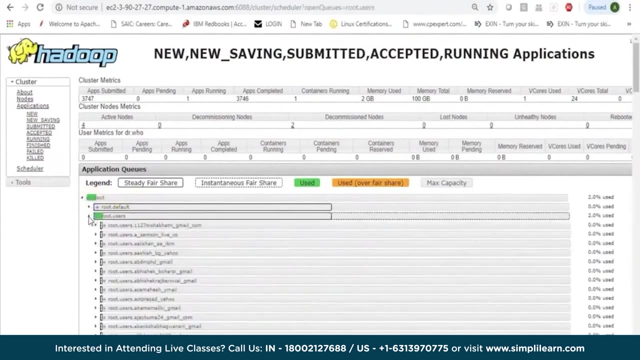 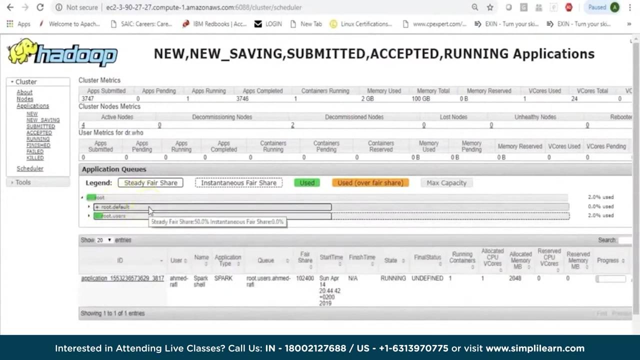 out of which some portion is being utilized. we can always look at the scheduler here, which can give us information what kind of scheduler has been a? So we basically see that there is just a root queue and within root you have default queue and you have basically users queue based on different users. We can always scroll here and that can give us information if it is a fair share. So here we see that my root dot default has 50% of resources and the other queue also has 50% of resources, which also gives me an idea that a fair scheduler is being used. 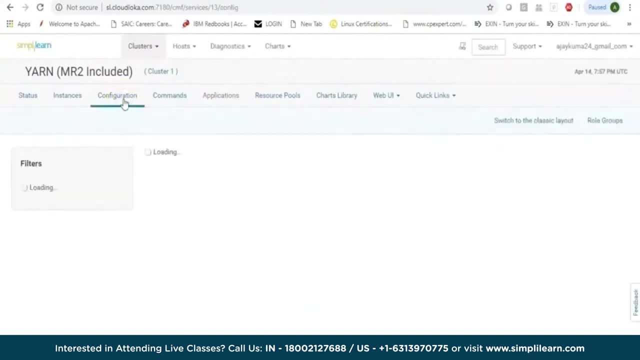 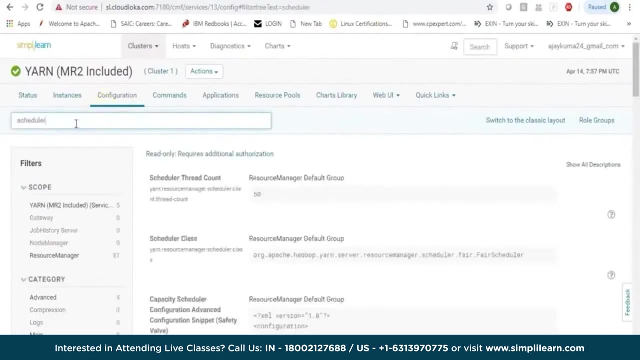 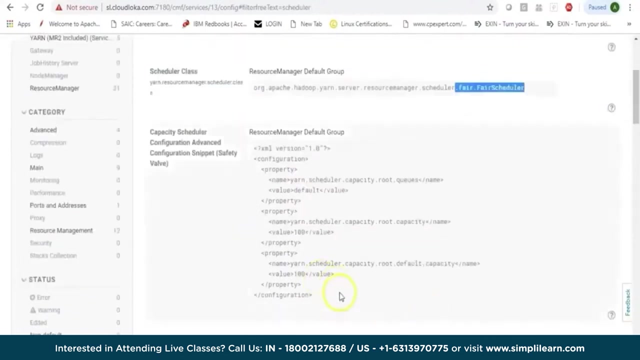 We can always confirm that if we are using a fair scheduler or a capacity scheduler which takes care of allocation. So search for scheduler and that should give you some understanding of what kind of scheduler is being used and what are the allocations given for that particular scheduler. 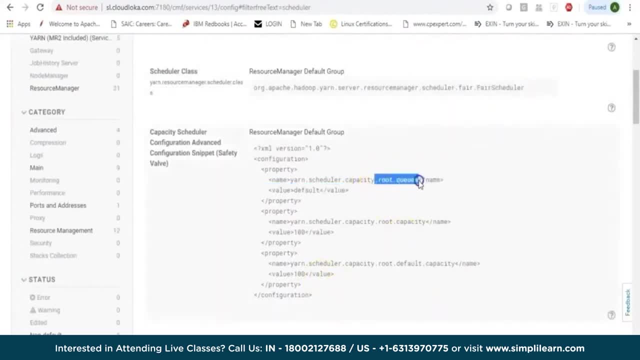 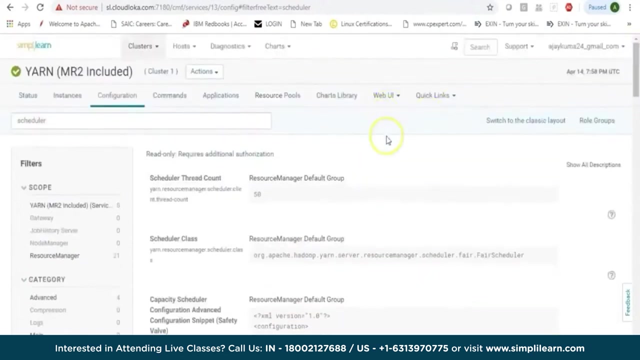 So here we have fair scheduler. It shows me. you have under root, you have the root queue which has been given 100% capacity, and then you have within that default, which also Takes 100%. So this is how you can understand about yarn. by looking into the yarn web UI, You can be looking into the configurations, you can look at applications, You can always look at different actions. Now, since we do not have admin access, the only information we have is to download the client configuration. We can always look at the history server, which can give us information of all the applications which have successfully completed. Now, this is from your yarn UI. What I can also do is I can also 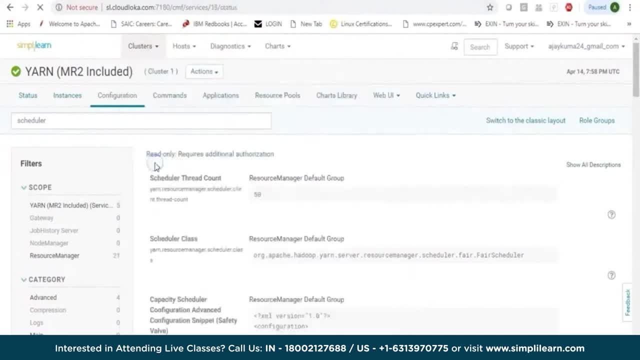 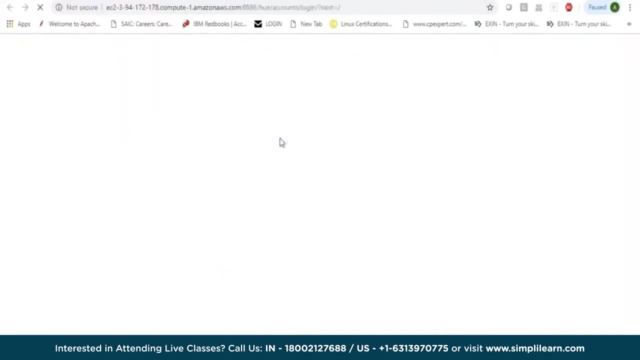 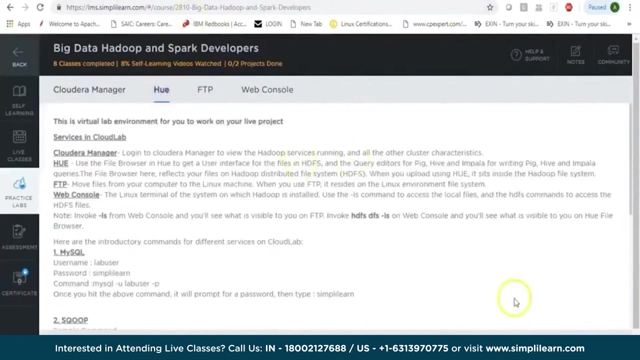 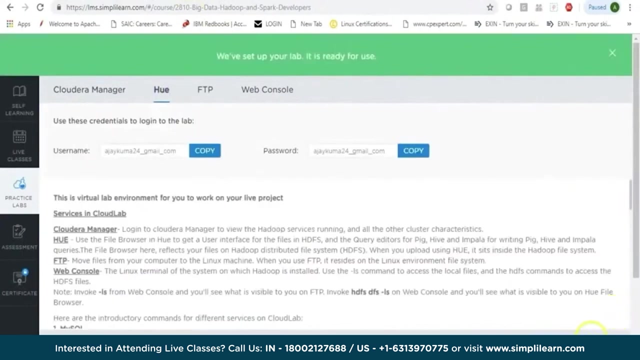 I can be going into hue, which is the web interface, and your web interface also basically allows you to look into the jobs. So you can click on hue web UI and if you have access to that, it should show up or you should have a way to get to your hue, which is a graphical user interface. mainly comes with your cloud error. You can also configure that with Apache. Hortonworks has a different way of giving you the web UI access. You can click and get into hue and that is also what you can do. 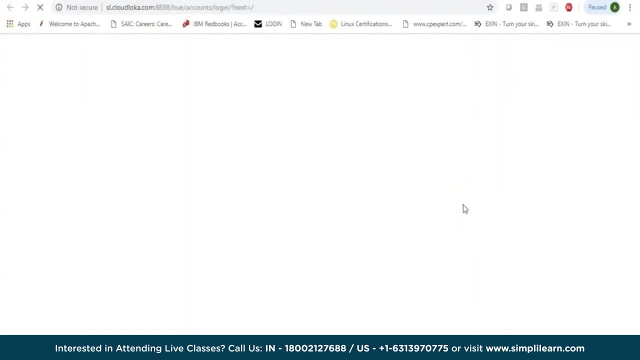 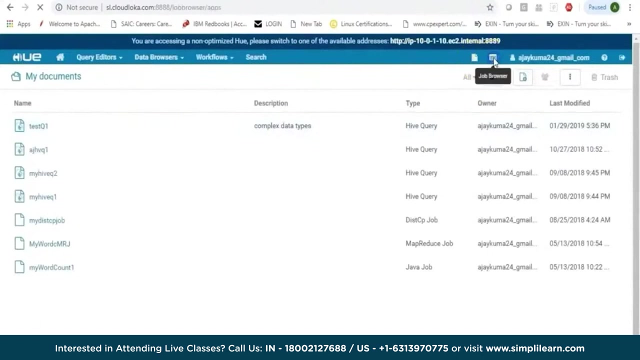 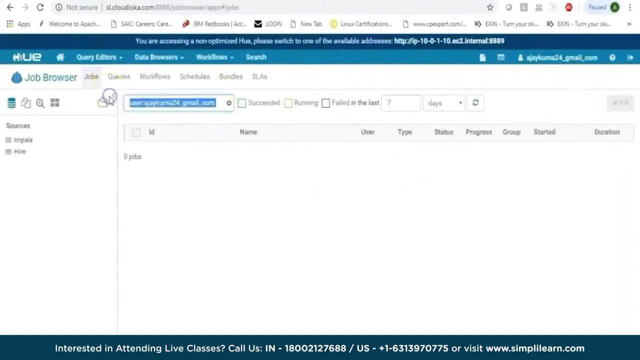 One way where you can look at yarn. you can look at the jobs which are running, if there are some issues with it, and these, these are your web interfaces. So either you look from yarn web UI or here in hue you have something called a job browser which can also give you information of your different applications which might have run. So here I can just remove this one, which would basically give me a list of all the different kind of jobs. 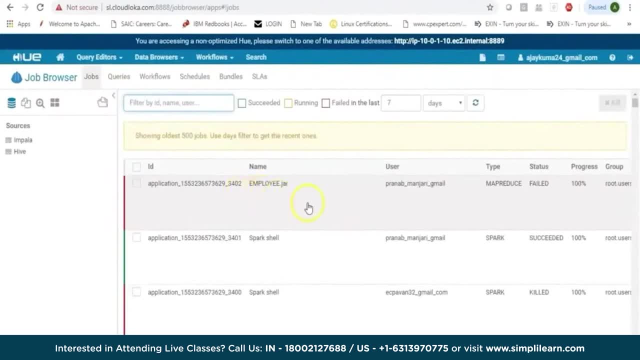 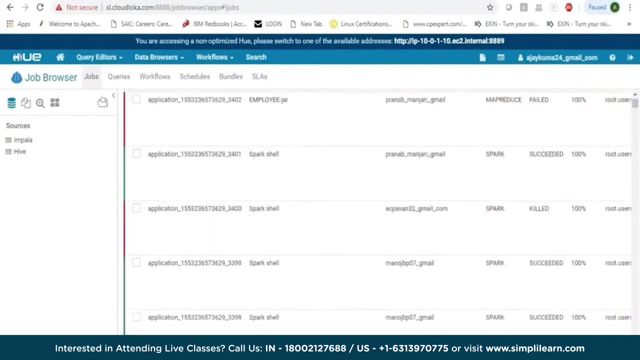 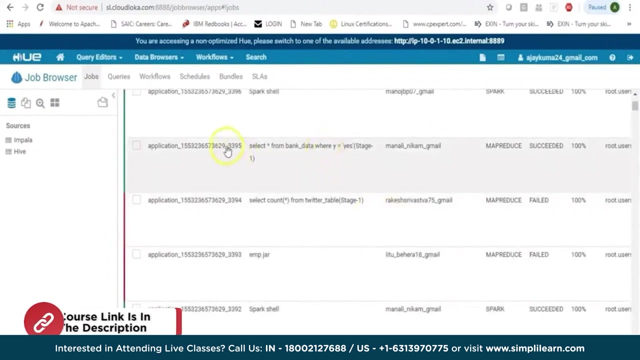 Or workloads which were run. So either it was a spark based application or it was a map reduce, or it was coming from hive. So here I have list of all the applications and it says this was a map reduce. This was a spark, Something was killed, Something was successful And this was basically a- probably a hive query which triggered a map reduce job. You can click on the application and that tells you how many tasks were run for it. So there was a 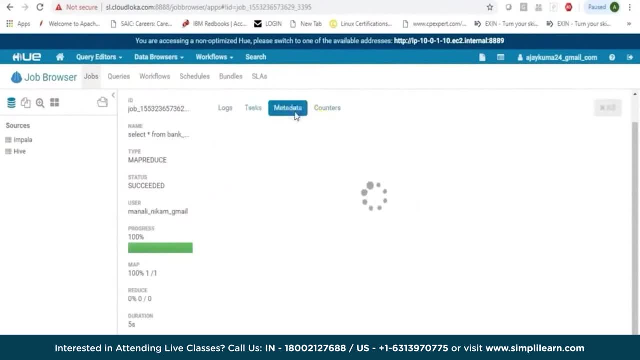 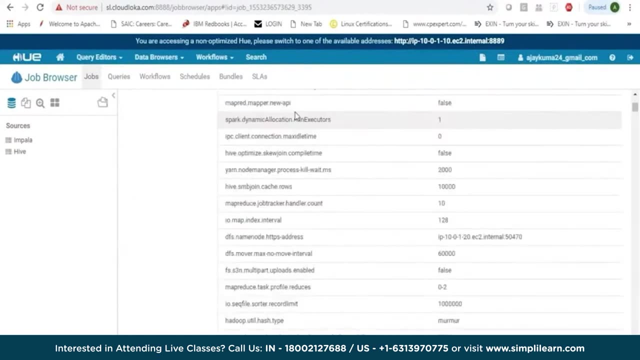 map task which ran for it. You can get into the metadata information which you can. obviously you can also look from the yarn UI to look into your applications which can give you a detailed information of if it was a map reduce, how many map and reduce tasks were run, What were the different counters. If it was a spark application, it can let you follow through spark history server or job history server So you can always use the web UI to look into the jobs. You can be finding in a lot of useful information. 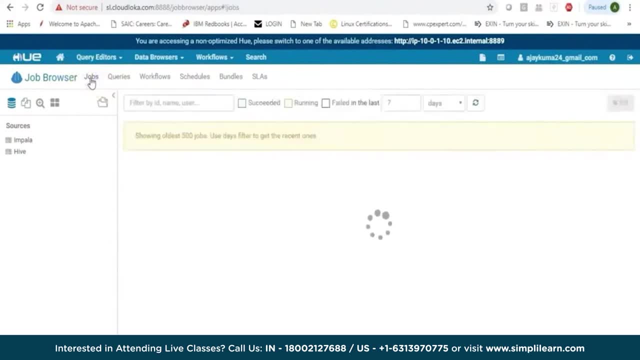 Here you can also be looking at how many resources were used and what happened to the job. Was it successful, Did it fail And what was the job status Now, apart from web UI, which always you might not have access to. So in a particular cluster, in a production cluster, there might be restrictions and the organization might not have access given to all the users to graphical user interface. like you, or might be you would not have access to the cloud data manager. 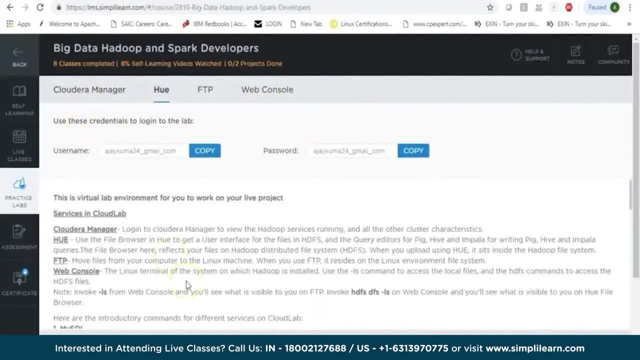 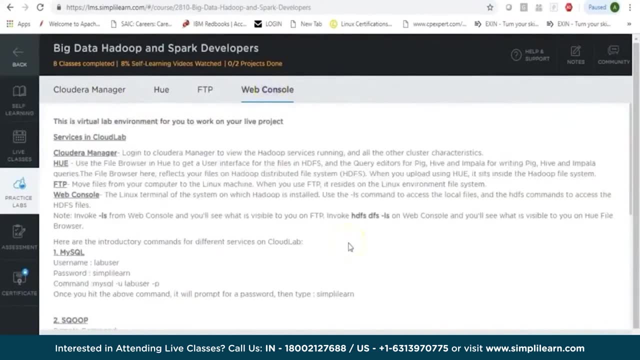 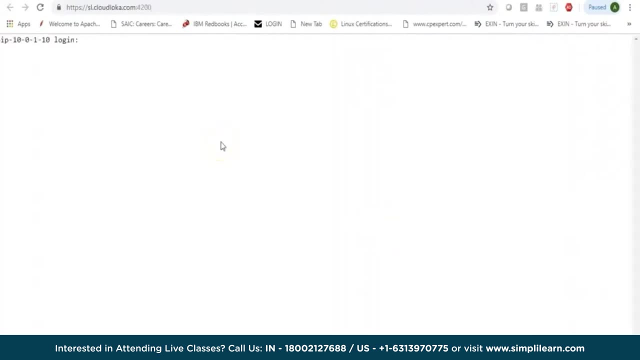 Or admin console, because probably organization is managing multiple clusters using this admin console. So the one way which you would have access is your web console, or basically your edge node or client machine, from where you can connect to the cluster and then you can be working. So let's log in here and now. here we can give different commands. So this is the command line from where you can have access to different details. You can always check by: 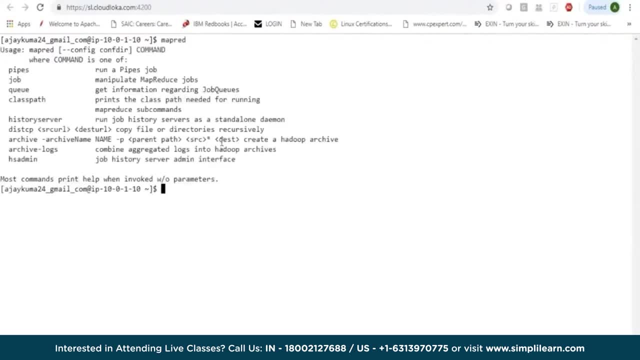 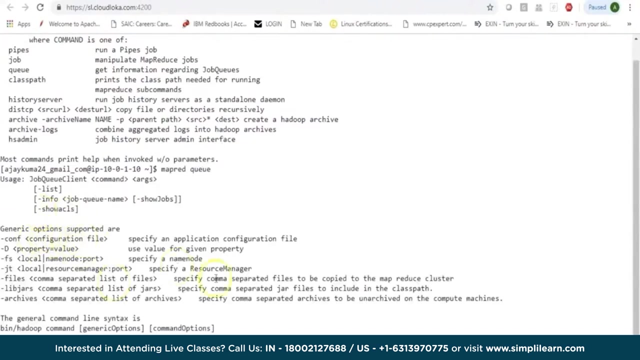 just typing in map red, which gives you different options where you can look at the map, reduce related jobs, You can look at different queues- If there are queues configured- you can look at the history server or you can also be doing some admin stuff, provided you have access. So, for example, if I just say map red and queue here, this basically gives me an option. says: what would you want to do? Would you want to list all the queues? Do you want information on a particular queue? So let's try a list. 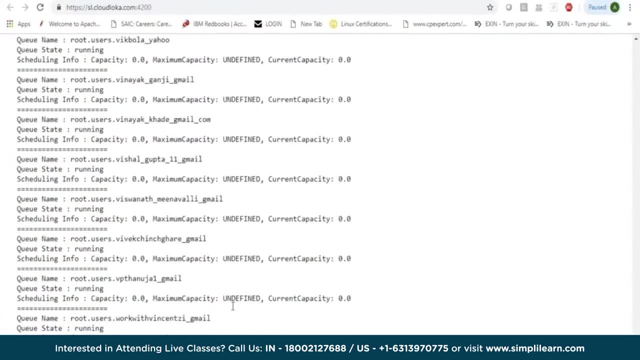 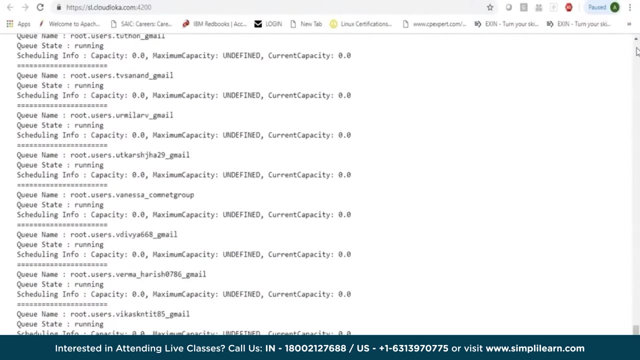 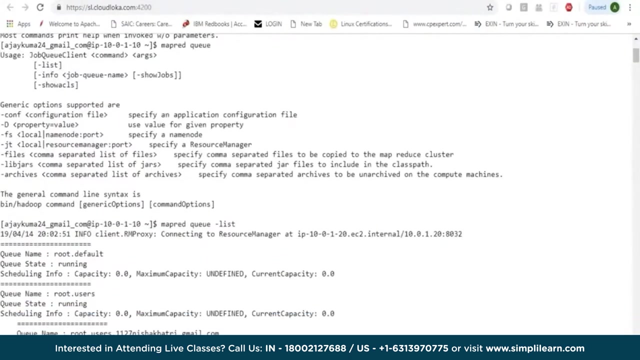 And that should give you different queues which were being used. Now here we know that per user a queue dynamically gets created which is under root dot users, and that gives me what is the status of the queue, What is the capacity? Has there been any kind of maximum capacity or capping done? So we get to see a huge list of queues which dynamically get configured in this environment, And then you also look at your root dot default. I could have also picked 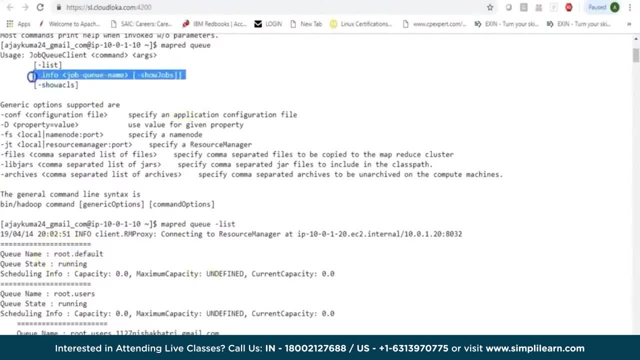 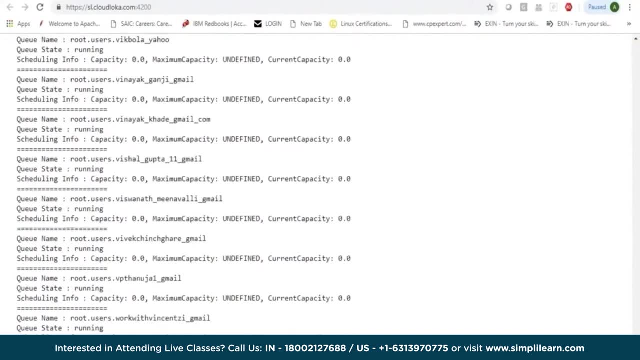 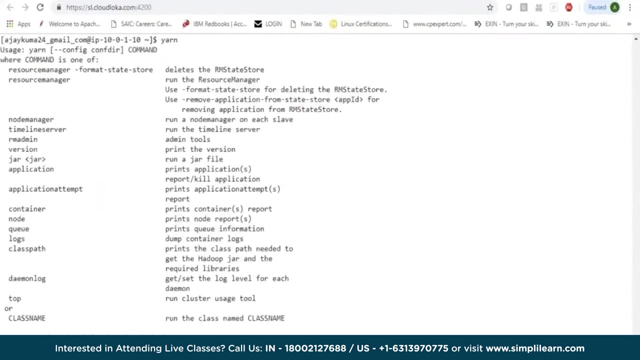 up one particular queue and I could have said: show me the jobs. So I could do that. Now here we can also give a yarn command. So let me just clear the screen and I will say yarn, and that shows me different options. So apart from your web interface, something like web UI, apart from your yarns web UI, you could also be looking for information using yarn commands here. So these are some list of commands which we can check. Now you can just 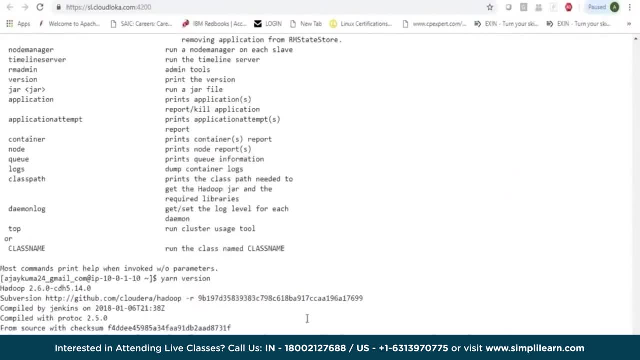 type in yarn and version, if you would want to see the version which basically gives you information of what is the Hadoop version being used and what is the vendor specific distribution version. So here we see. we are working on Cloudera's distribution 5.14, which is internally using Hadoop 2.6. Now, similarly, you can be doing a yarn application list. So if you give this, that could be an exhaustive list of all the applications which are running. 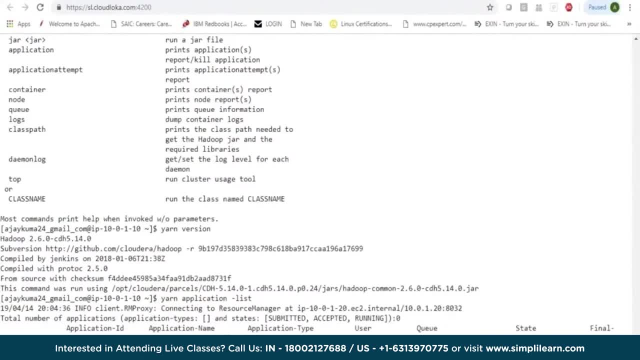 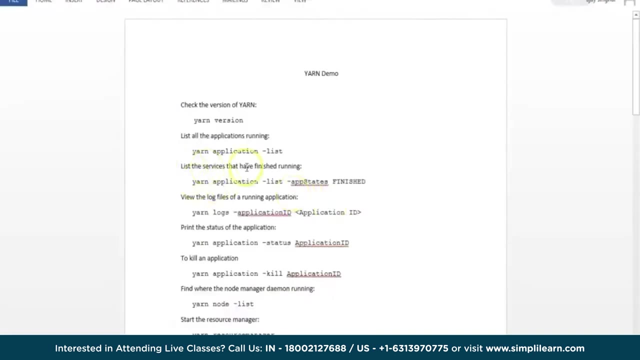 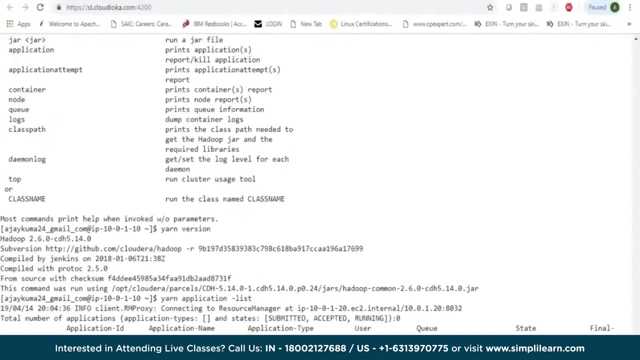 Or applications which have completed. So here we don't see any applications because right now probably there are no applications which are running. It also shows you you could be pulling out different status, such as submitted, accepted or running. Now you could also say: I would want to see the services that have finished running. So I could say yarn application list and app states as finished. So here we could be using our command So I could say yarn application. 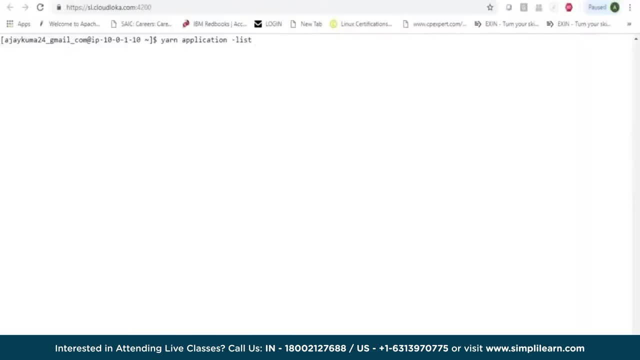 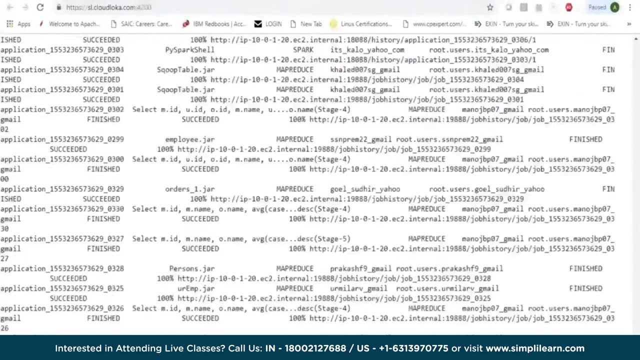 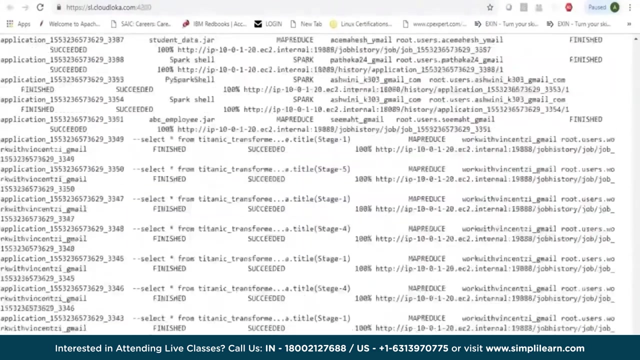 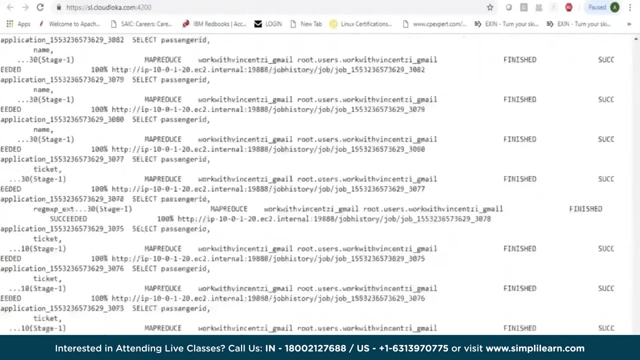 list, and then I would want to see the app states which gives me the applications which have finished, And we would want to list all the applications which finished. Now that might be applications which succeeded Right, And there is a huge list of application which is coming in from the history server which is basically showing you the huge list of applications which have completed. So this is one way, And then you could also be searching for one particular application If you would want. 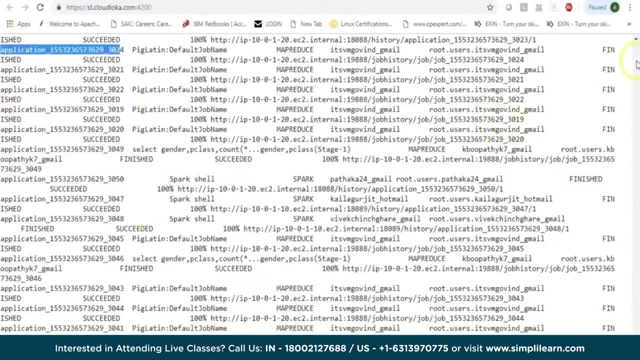 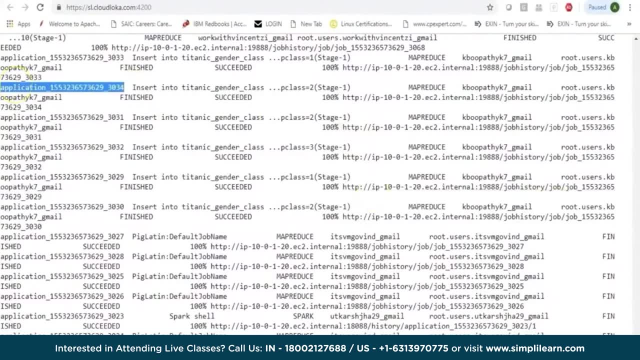 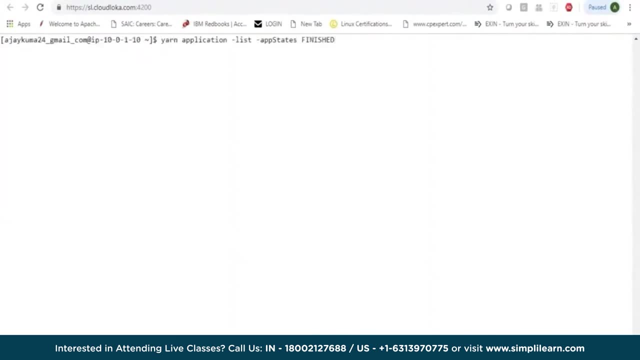 want to search a particular application, if you have the application id, you could always be doing a grip. that's a simple way i could say: basically, let's pick up this one, and if i would want to search for this, if i would want more details on this, i could obviously do that by calling in my 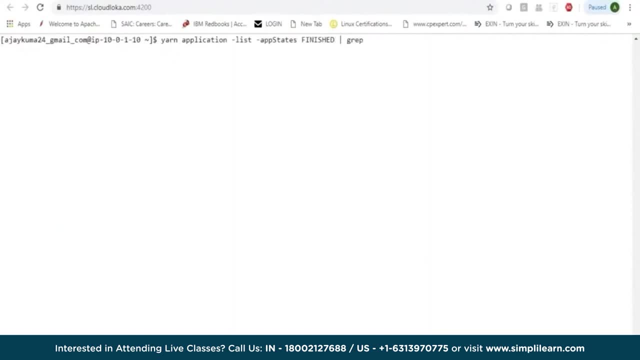 previous command and you could do a grip. if that's what you want to do and if you would want to search, is there any application which is in the list of my applications that shows my application? i could pull out more information about my application so i could look at the log files. 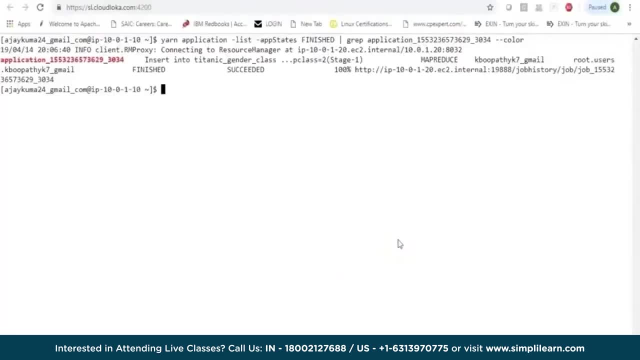 for a particular application by giving the application id. so i could say: yarn logs. now, that's an option and every time, anytime you have a doubt, just hit enter. it will always give you options, what you need to give with a particular command, so i can say: yarn logs, application. 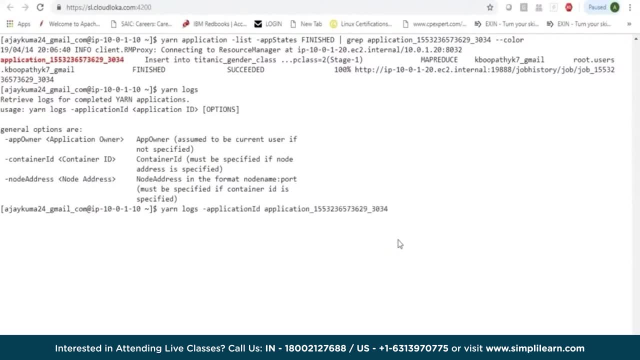 id. now we copied an application id and we could just give it here. we could give other options like and and owner, or if you would want to get into the container details or if you would want to check on a particular node. now, here I am giving yarn logs and then I am. 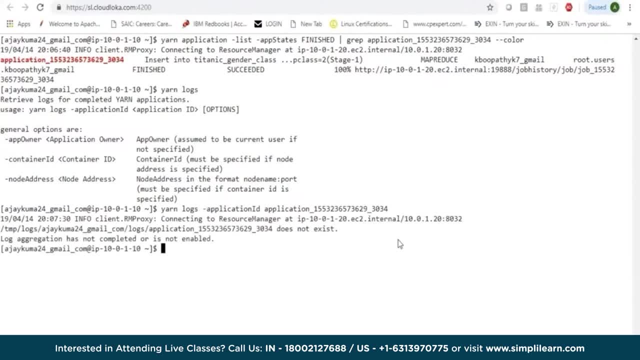 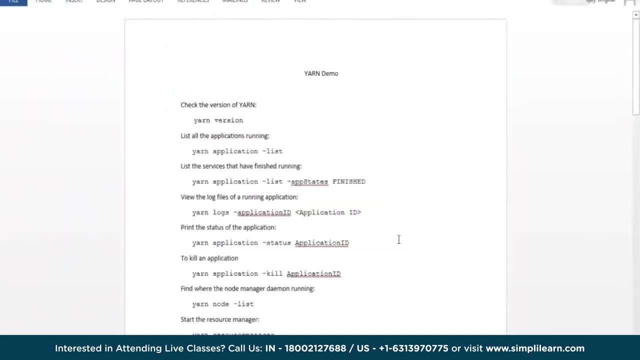 pointing it to an application ID and it says the log aggregation has not completed. might be. this was. might be. this was an application which was triggered based on a particular interactive shell or based on a particular query, so there is no log existing for this particular application. you can always look at the status of an application. you can kill an application. 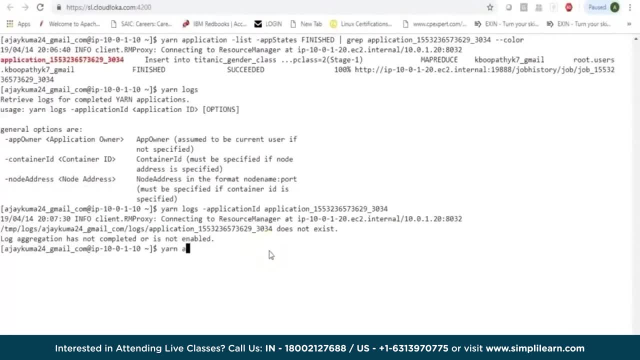 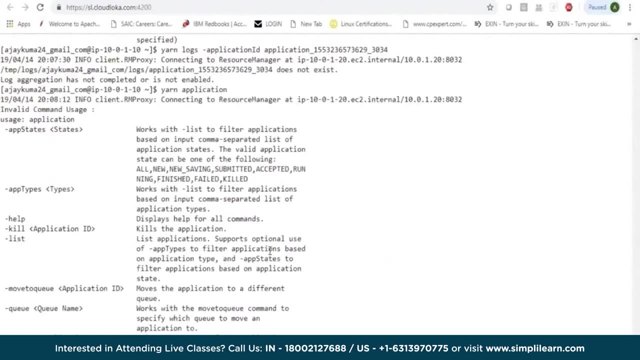 so here you can be saying yarn, yarn, application. and then what would you want to do with an application? hit an enter. it shows you the different options. so we just tried app states. you could always look at the last one which says status, and then, for my status, I could be giving my application ID. so that tells me what. 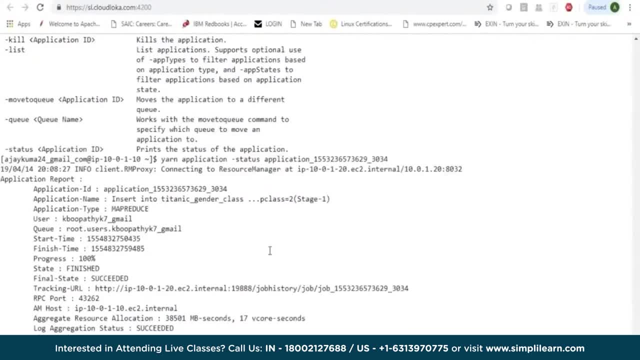 is the status of this application. it connects to the resource manager application and then it tells me what is the status of this application. it tells me what's the application ID, what kind of application it was, who ran it, which was the queue where the job was running, what was the start and end time. 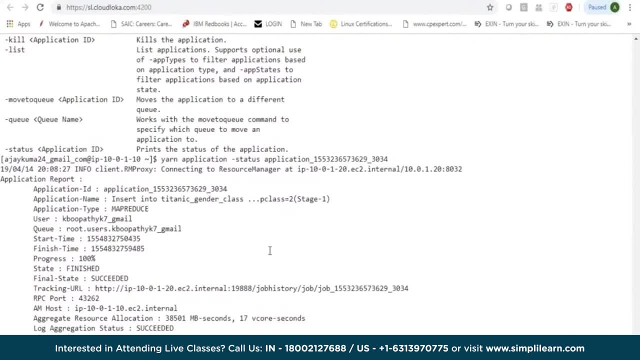 what is the progress, the status of it, if it is finished or if it has succeeded. and then it basically gives me also an information of where the application master was running. it gives me the information where you can find this job details in history server if you are interested in looking into it. also gives 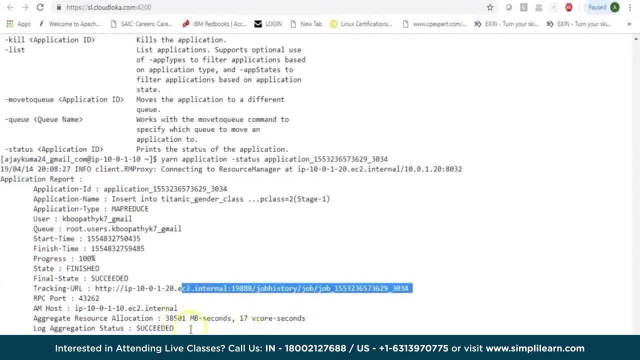 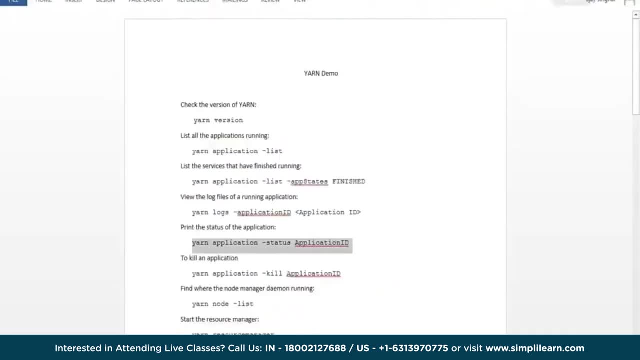 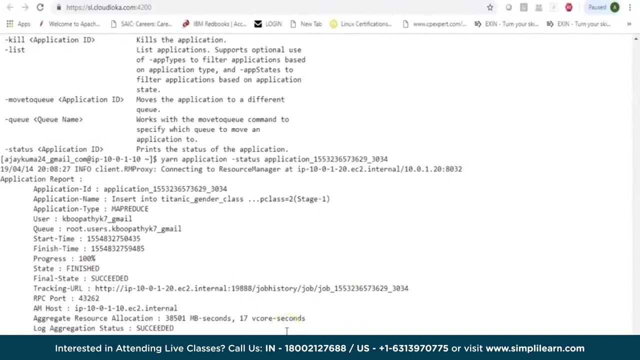 you a aggregate resource allocation which tells how much GB memory and how many c4 seconds it used. so this is basically looking out at the application details. now I could kill an application if the application was already running. I could always do a yarn- application minus kill, and then I could be giving my application. now I could try killing this. 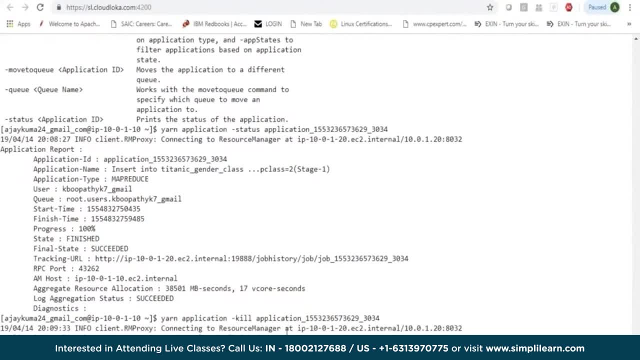 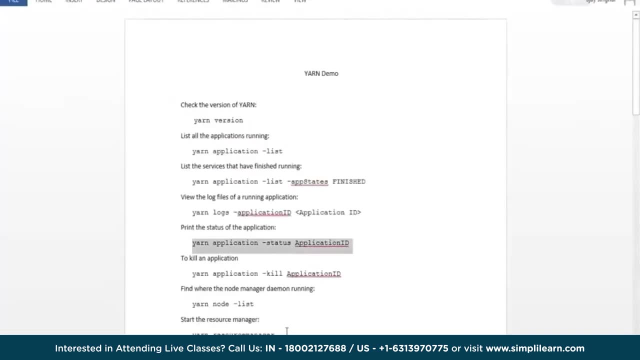 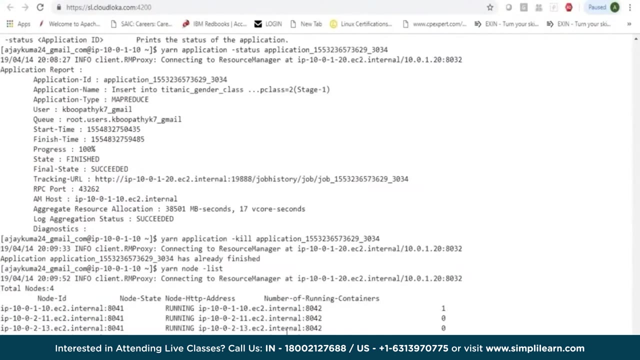 however, it would say the application is already finished. if I had an application running and if my application was already given an application ID by the source manager, I could just kill it. I can also say yarn node list, which would give me a list of the node managers. now, this is what we were looking from: the yarn web. 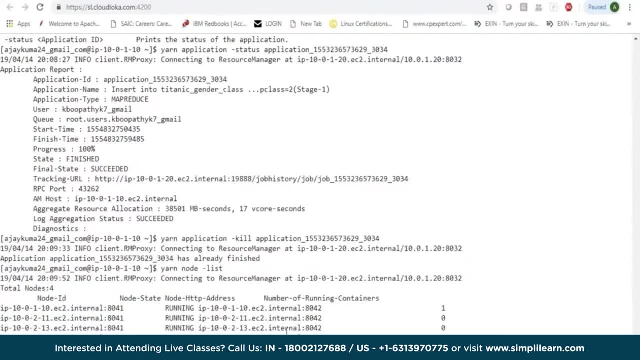 UI and we were pulling out the information so we can get this and kind of information from your command line. always remember and always try to be well accustomed with the command line so you can do various things from the command line. and then obviously you have the web UIs which can help you with a 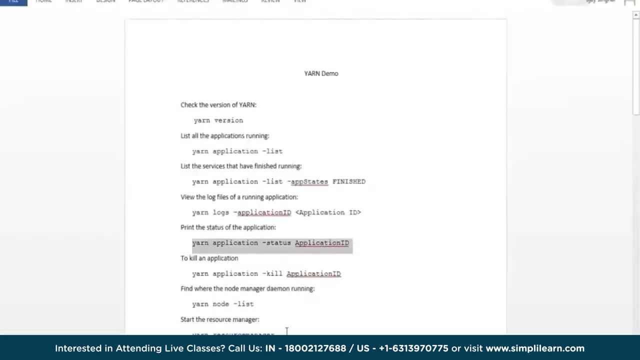 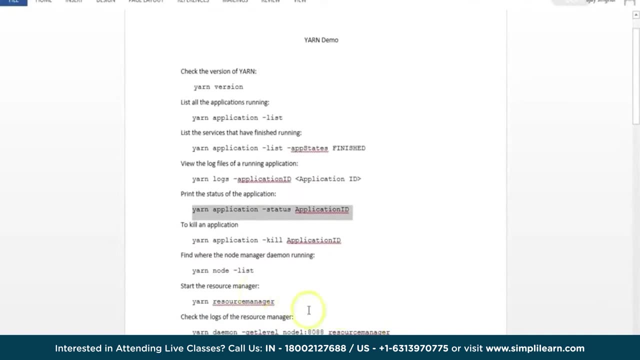 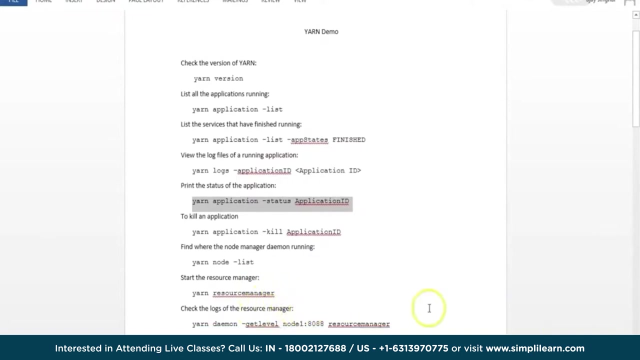 graphical interface easily able to access things. now you could be also starting the resource manager, which we would not be doing here because we are already running in a cluster. so you could give a yarn resource manager. you could get the logs of resource manager, if you would want, by giving yarn daemon. so we can try that, so you can say yarn and then daemon. 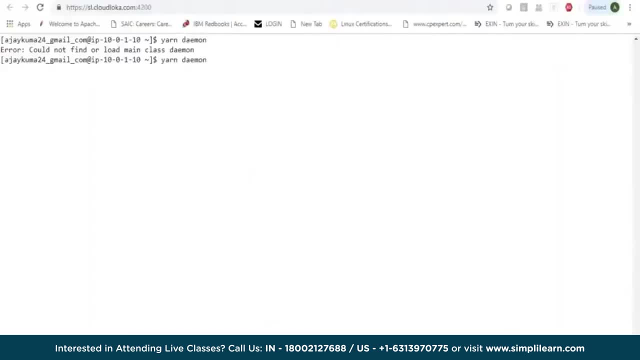 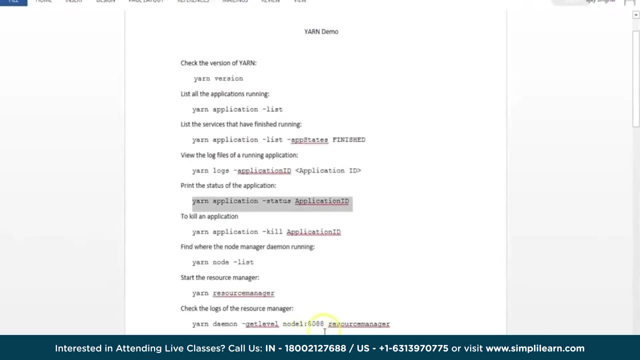 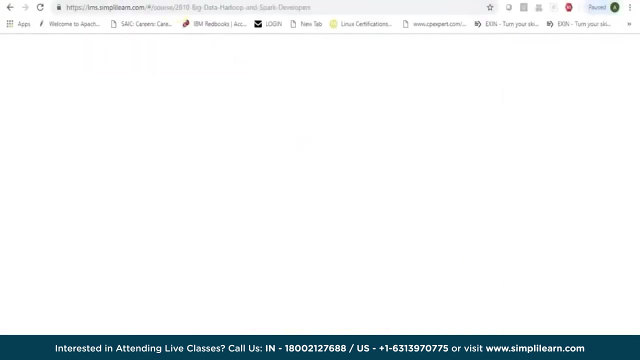 so it says it does not find the daemon. so you can give something like this: get level, and here I will have to give the node and the IP address where you want to check the logs of resource manager. so you could be giving this, for which we will have to then get into cloud data manager. 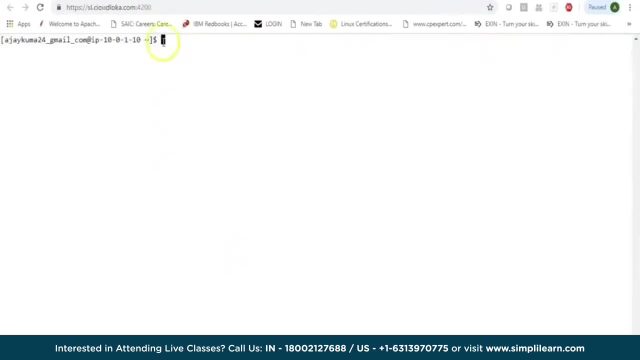 to look into the nodes and the IP address. you could be giving a command, something like this, which basically gives you the level of the log which you have, and I got this resource manager address from the web UI. now I can be giving in this command to look into the daemon log. 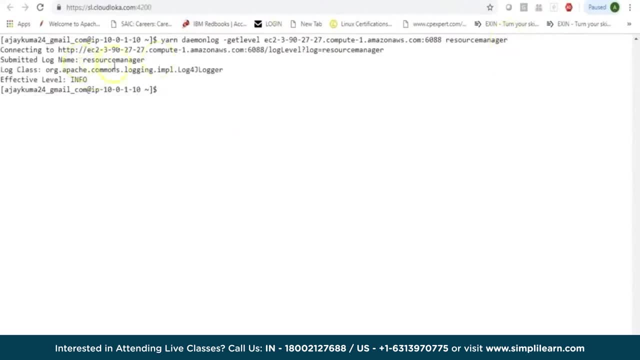 and it basically says: you would want to look at the resource manager related log and you have the log4j which is being used for logging the kind of level which has been set as info which can again be changed in the way you are logging the information. now you can try any other commands also, from yarn, for example. 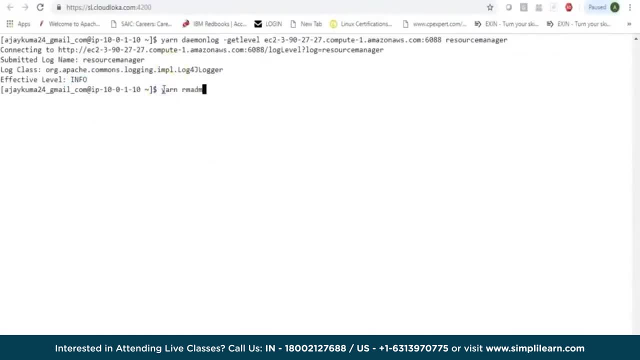 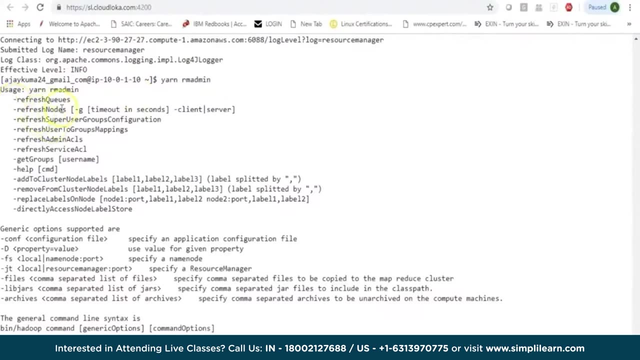 looking at the yarn RM admin, so you can always do a yarn RM admin and this basically gives you a lot of other informations, like refreshing the queues or refreshing the nodes or basically looking at the admin ACLs or getting groups, so you could always get group names for a particular user. now we could 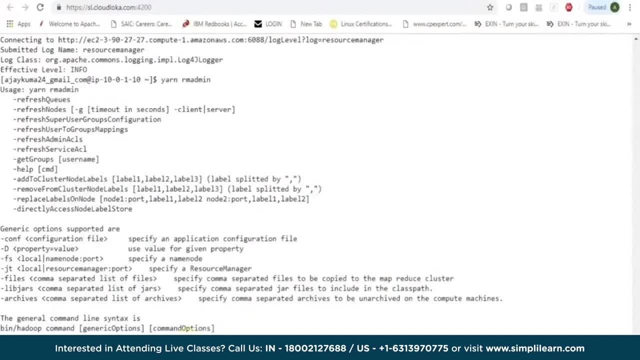 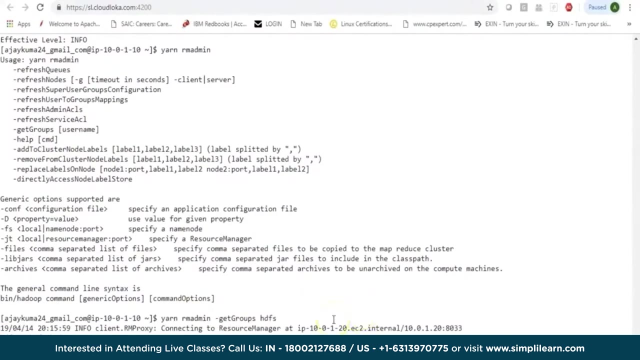 search for a particular user, such as yarn or HDFS itself. so I could just say here I would want get groups and then I could be searching for, say, user name HDFS. so that tells me HDFS belongs to a Hadoop group. similarly you could search for, say, mapred, or you could search for yarn. so 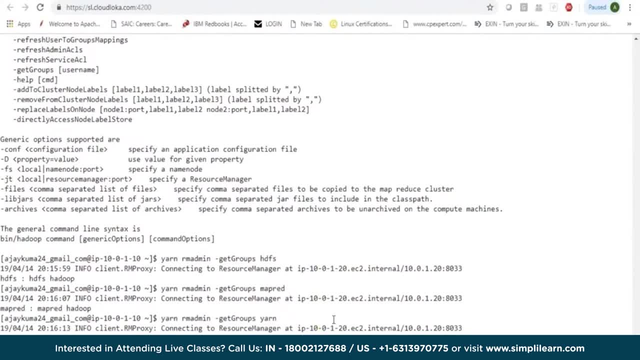 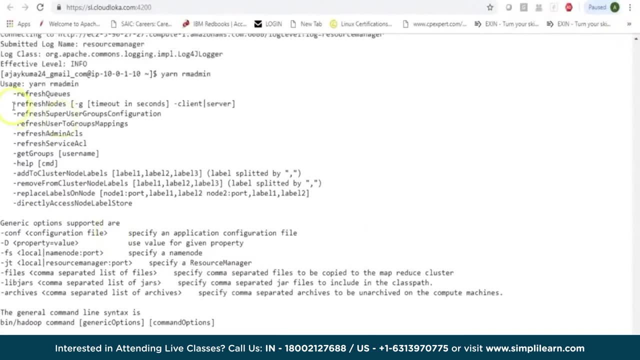 these are service related users which automatically get created and you can pull out information related to these. you can always do a refresh nodes kind of command, and that is mainly done internally. this can be useful when you are doing commissioning, decommissioning, but then in case of cloud era or hot, 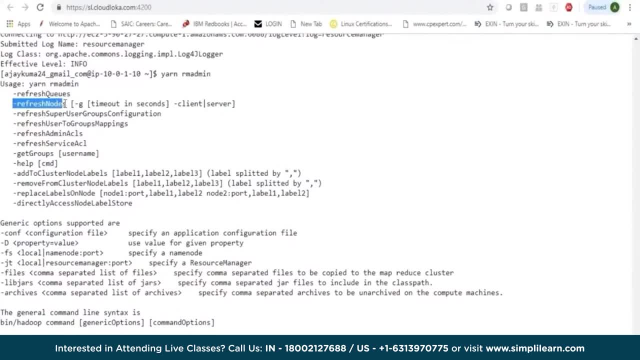 onworks kind of cluster, you would not be manually giving this command, because if commissioning decommissioning from an admin console and if you are an administrator, then you could just restart the services which are affected and that will take care of this. but if you were working in an Apache cluster, 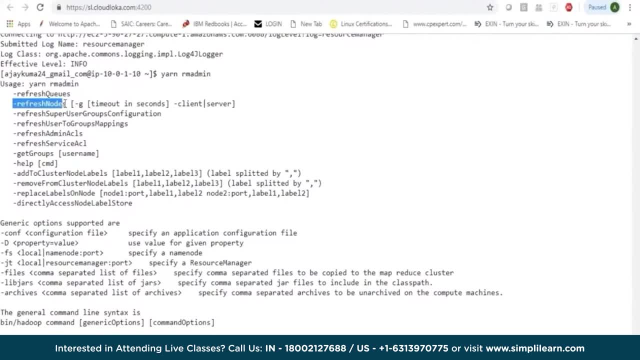 and if you are doing commissioning decommissioning, then you would be using in two commands refresh notes, and basically that's for refreshing the nodes which should not be used for processing, and similarly you could have a command refresh notes, which comes with HDFS. so these are different options. 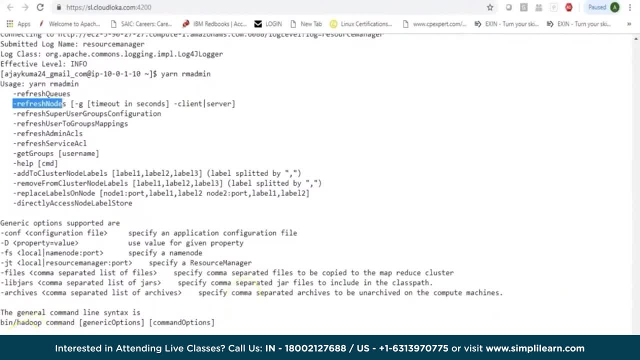 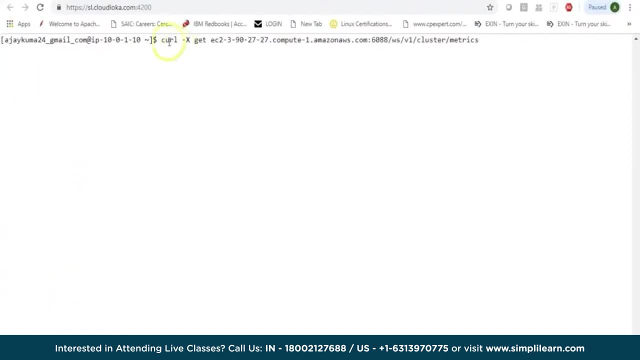 which you can use with your yarn on the command line. you could also be using curl commands to get more information about your clusters by giving curl minus X and then basically pointing out to your resource manager web UI address. now here I would like to print out the cluster related metrics and I could just 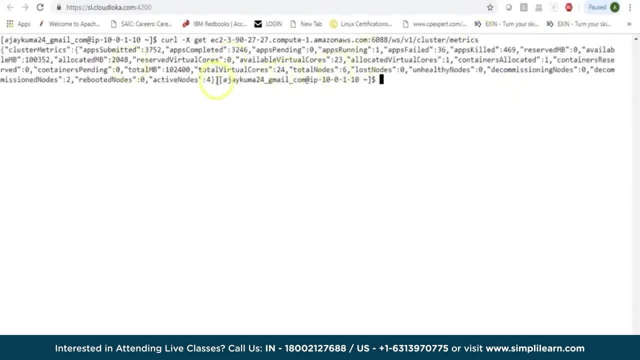 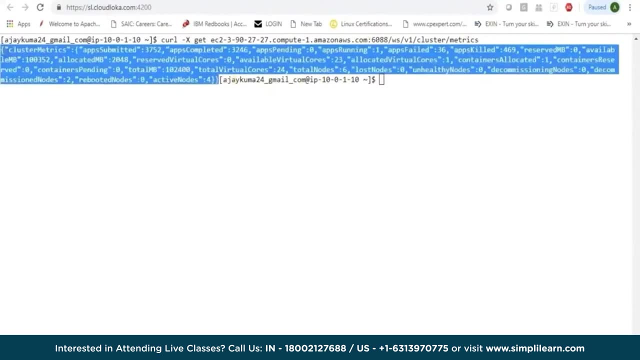 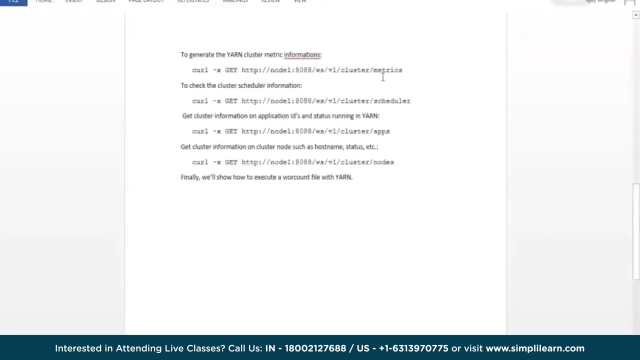 simply do this, which basically gives me a high-level information of how many applications were submitted, how many are pending, what is the reserved resources, what is the available amount of memory or CPU cores and all the information. similarly, you can be using the same curl commands to get more information, like scheduler information. 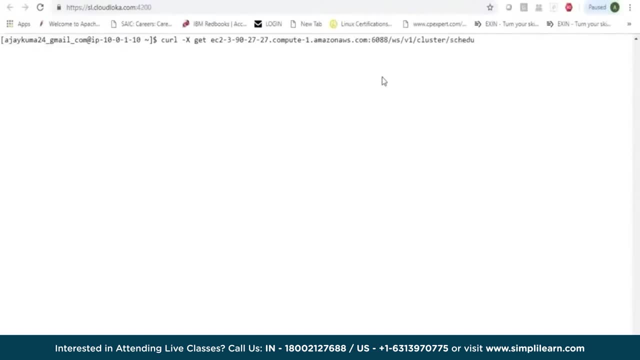 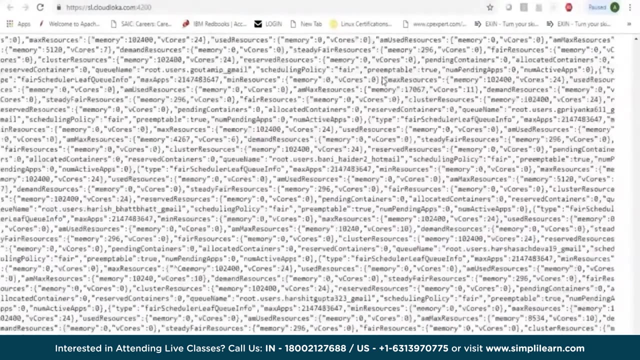 so you would just replace the metrics with scheduler and you could get the information of the different queues. now that's a huge list. we can cancel this and that would give me a lot of information about the cluster. and that's a huge list. we can cancel this and that would give me. 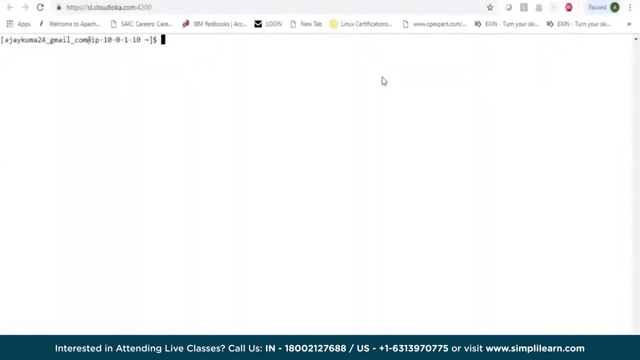 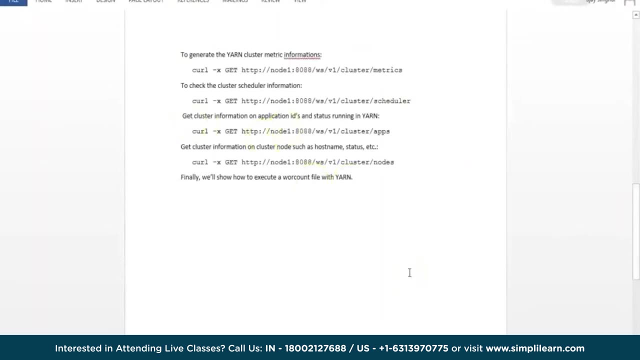 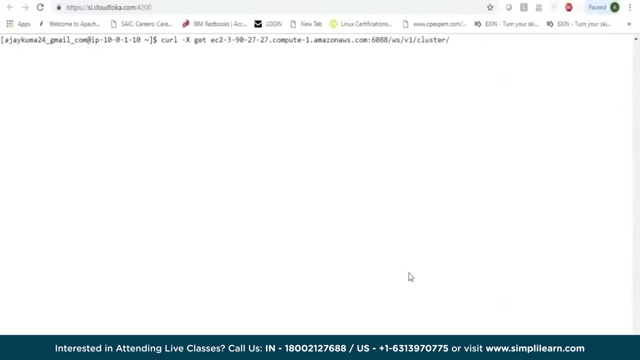 the list of all the queues which are allocated and what are the resources allocated for each queue. you could also get cluster information on application ids and status running of applications running in ya. so you would have to replace the last bit of it and you would say: I would want to look at the 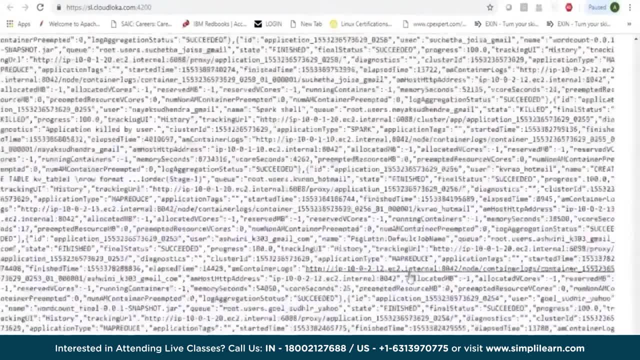 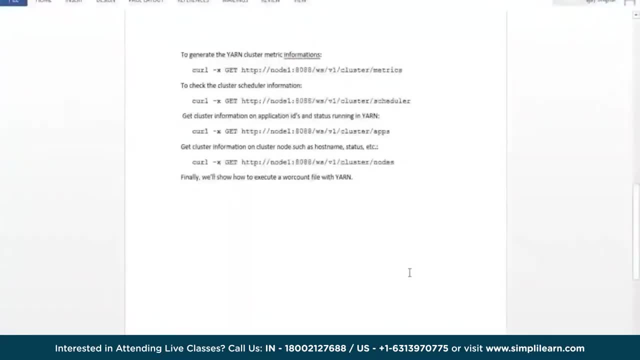 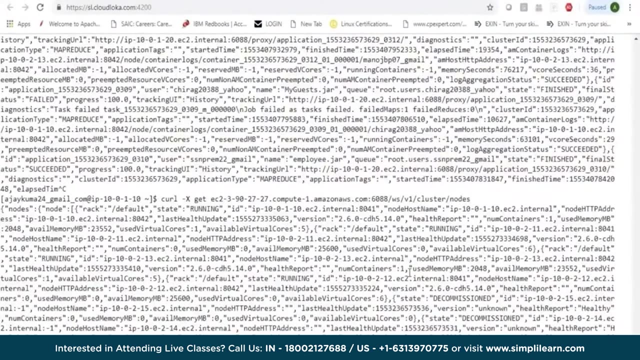 applications and that gives me a huge list of applications. then you can do a grep and you can be filtering out specific application related information. similarly, you looking at the nodes, So you can always be looking at node specific information which gives you how many nodes you have. But this could be mainly used when you have an application which wants to or a. 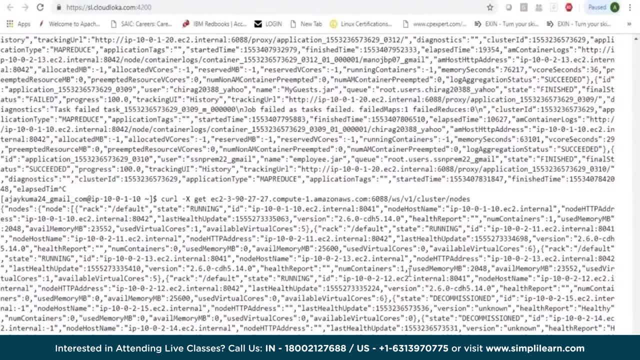 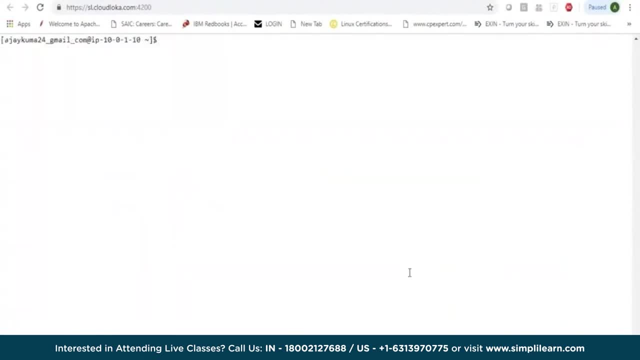 web application which wants to use a curl command and would want to get information about your cluster from an HTTP interface. Now, when it comes to application, we can basically try running a simple or a sample MapReduce job, which could then be triggered on YARN and it would use the 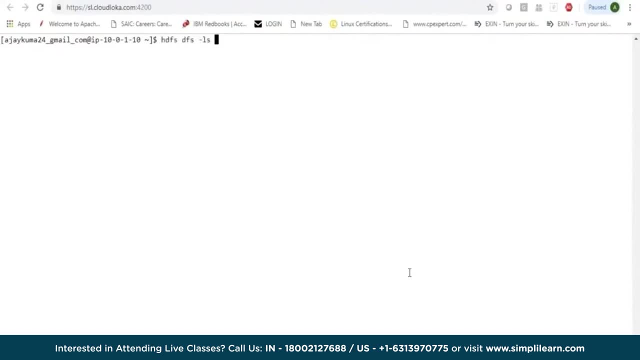 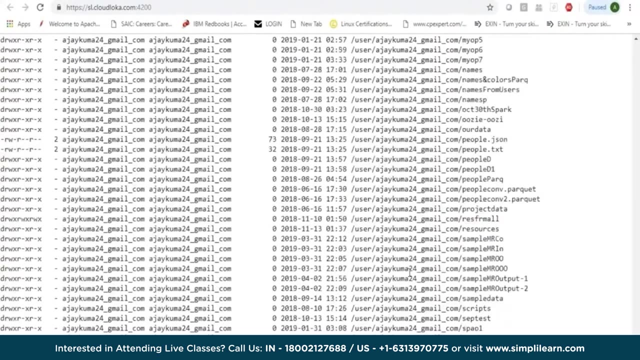 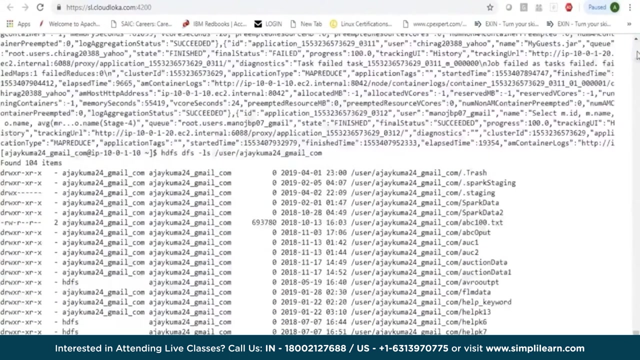 resources. Now I can look at my application here and I can be looking into my specific directory, which is this one, which should have a lot of files and directories which we have here. Now I could pick up one of these and I could be using a simple example to do some processing. Let's take up this. 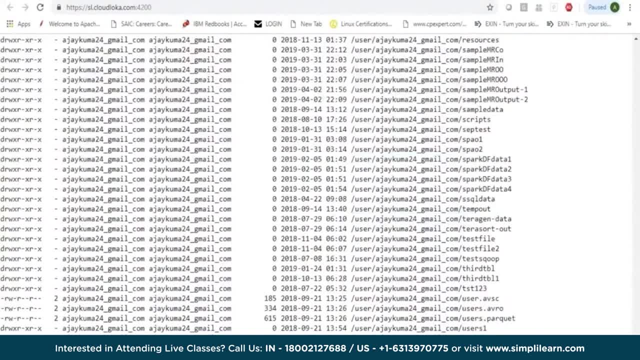 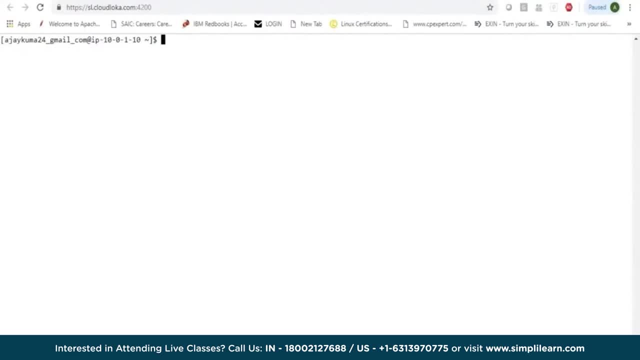 file. So there is a file and I could run a simple or a sample MapReduce job, which would then be a simple word count, or I could be running a hive query which triggers a MapReduce job. I could even run a Spark application, which would then show that the application is running on the cluster. So for 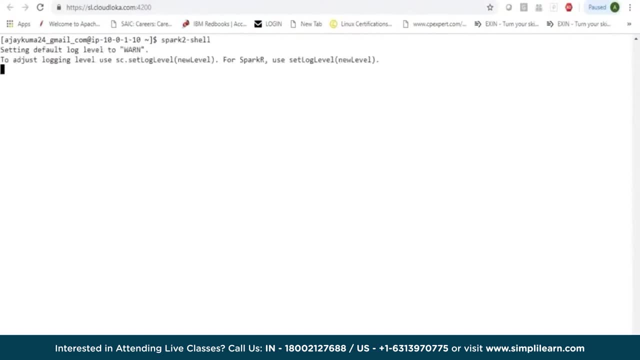 example, if I would say Spark to shell. Now, I know that this is an interactive way of working with Spark, but this internally triggers a Spark submit and this runs an application. So here when you do a Spark to shell, by default it will contact YARN, so it gets an application ID. 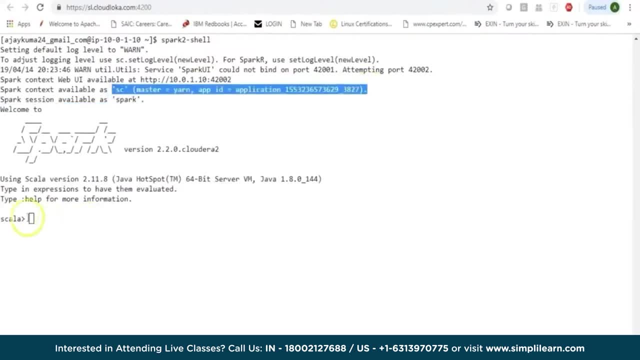 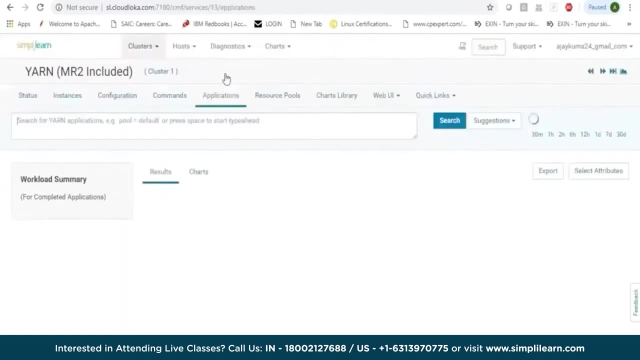 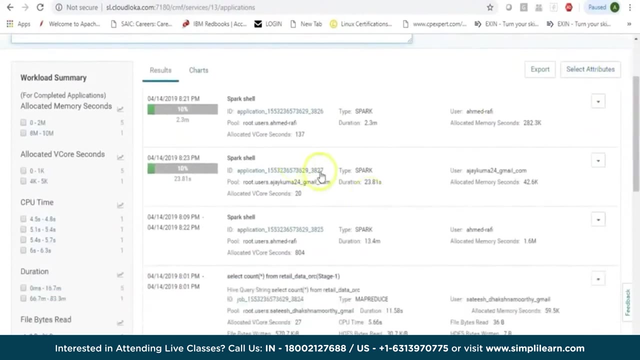 It is running on YARN, with the master being YARN, and now I have access to the interactive way of working with Spark. Now, if I go and look into applications, I should be able to see my application, which has been started here, and it shows up here. So this is my application 3827, which has been 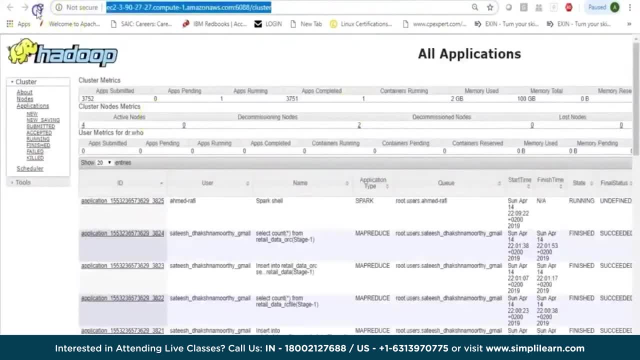 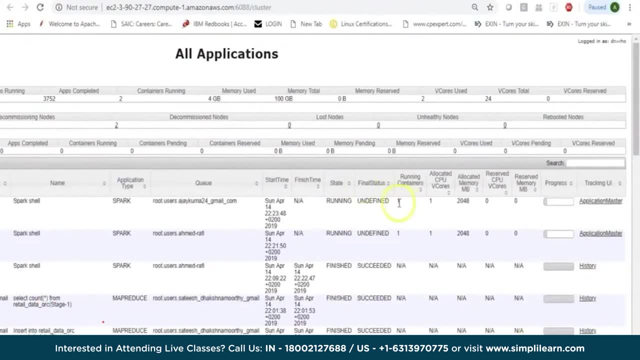 started on YARN and as of now we can also look into the YARN UI, and that shows me the application: one running container which has one CPU core allocated 2GB RAM, and it's in progress, although we are not doing anything there. So we can always look at our applications from the YARN UI or, as I 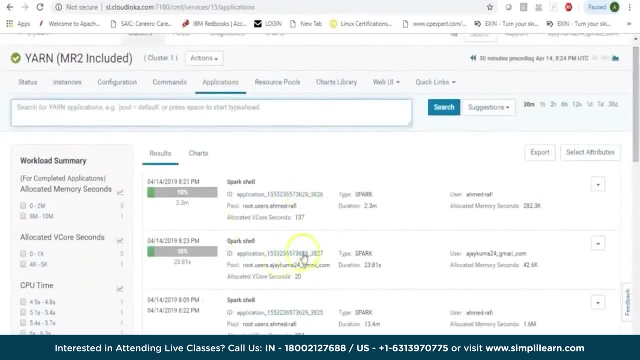 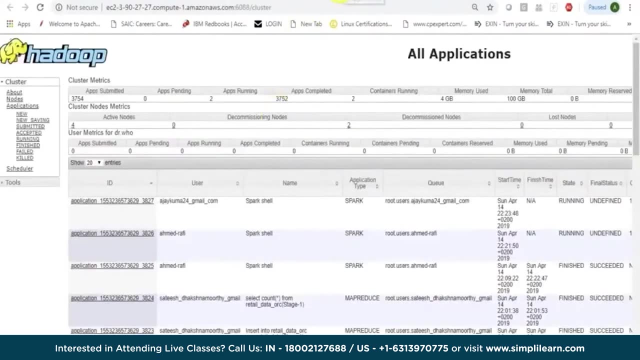 mentioned from your applications tab within YARN services, which gives us the information, and you can even click on this application to follow and see more information. but you should be given access to that Now. this is just a simple application which I triggered using Spark Shell. 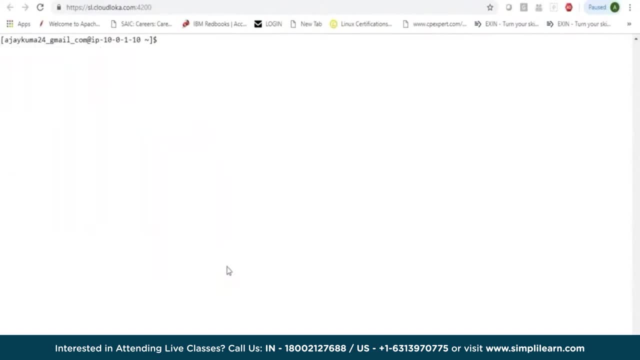 Similarly, I can basically be running a MapReduce. Now to run a MapReduce, I can say Hadoop, JAR, and that basically needs a class. so we can look for the default path, which is Opt, Cloud, Era, Parcels, CDH, Lib, Hadoop MapReduce, Hadoop MapReduce Examples, and then we can look at this particular. 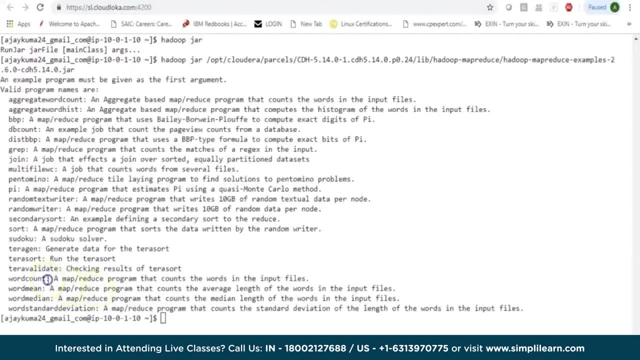 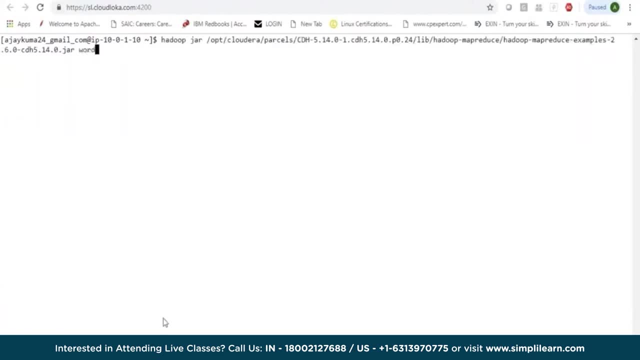 JAR file and if I hit on enter, it shows me the different classes which are part of this JAR. and here I would like to use word count, so I could just give this. I could say word count now, remember, I could run the job in a particular queue by giving in an argument here. so I could say: 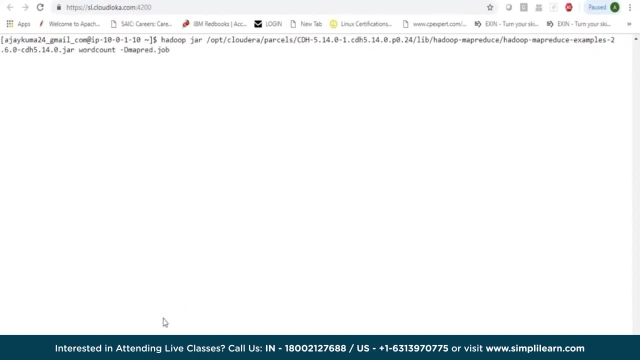 minus D MapRed dot job, dot queue, dot name, and then I can point my job to a particular queue. I can even give different arguments in saying I would want my MapReduce output to be compressed, or I want it to be stored in a particular directory, and so on. 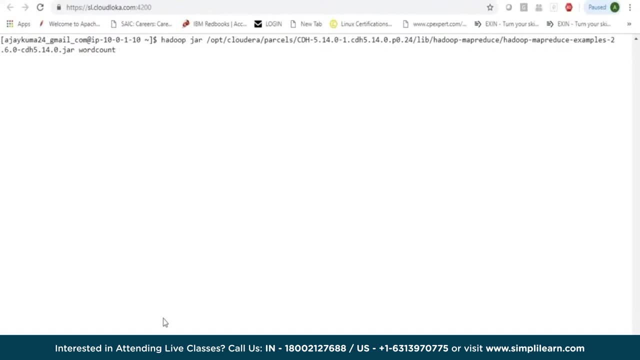 I have the word count and then basically, what I can be doing is I can be pointing it to a particular input path and then I can have my output which can be getting stored here again, a directory which we need to choose, and I will say output new and I can submit my job Now, once I have submitted my job, 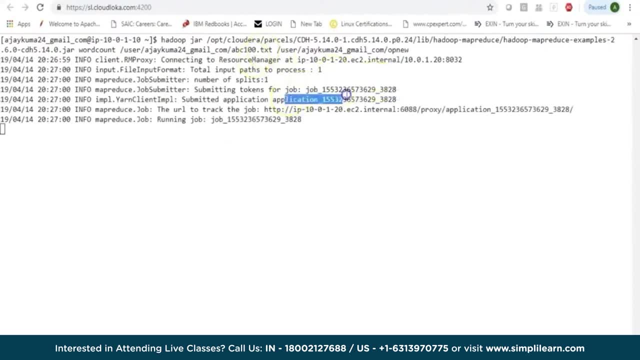 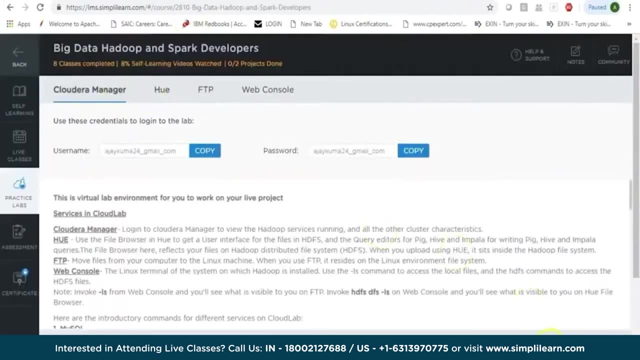 it connects to resource manager. it basically gets a job ID. it gets an application ID, it shows you from where you can track your job and then it will show you the job ID and then it will show you your application. you can always go to the yarn UI and you can be looking at your application and 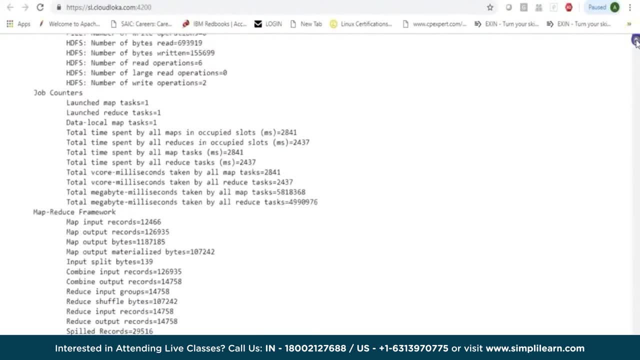 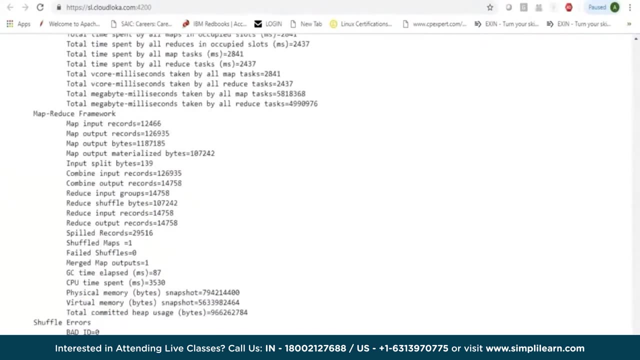 the resources it is using. so my application was not a big one and it has already completed. it triggered one map task, it launched one reduce task. it was working on around 12,466 records, where you have, then, the output of map, which is these many number of output records, which was 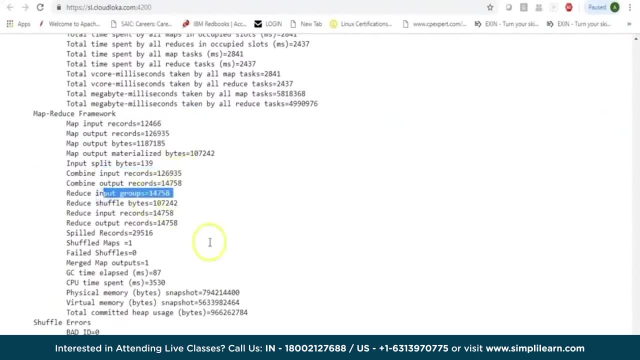 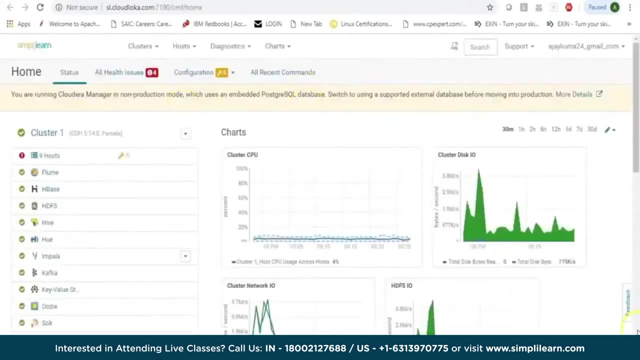 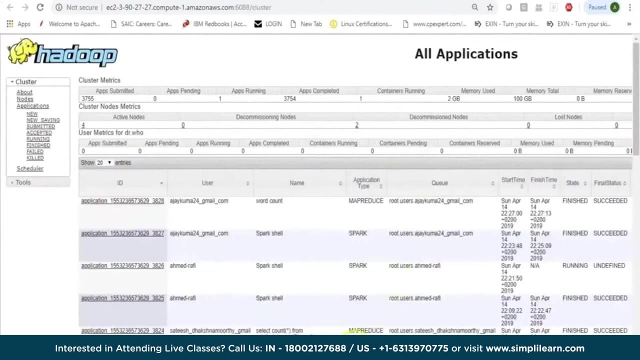 then taken by a combiner and finally by a reducer, Which basically gives you the output. so this is my yarn application, which has completed. now I could be looking into the yarn UI and if my job has completed you might not see your application here. so as of now it shows up here, the word count which I ran. it also shows me my previous Park shell job. 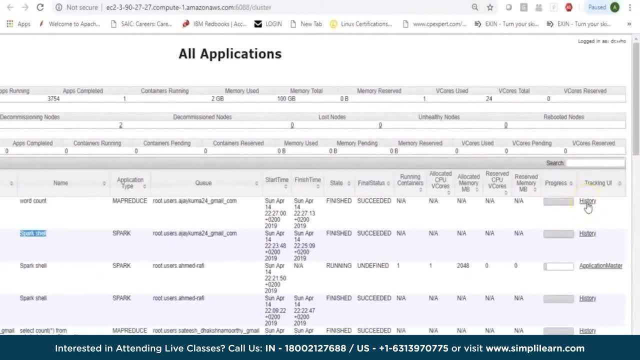 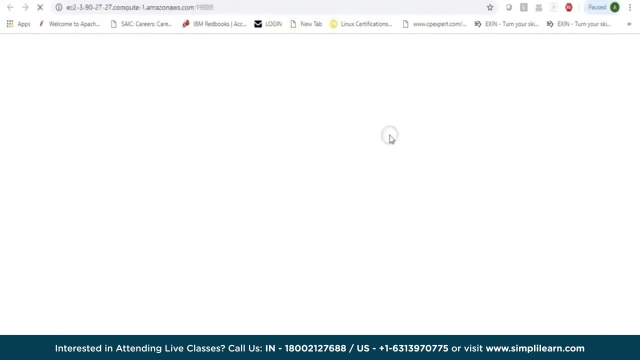 it shows me my application is completed and if you would want further information on this, you can click and go to the history server if you have been given access to it, Or directly go to the history server web UI where your application shows up. it shows how many map. 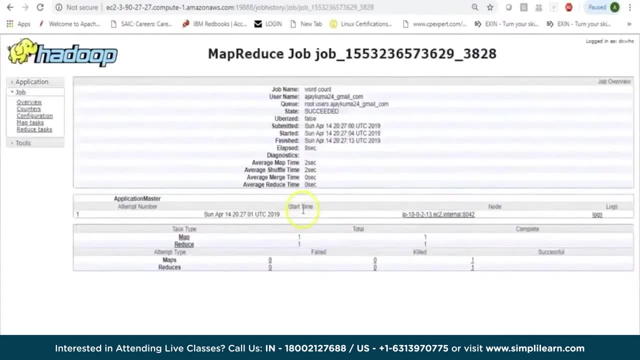 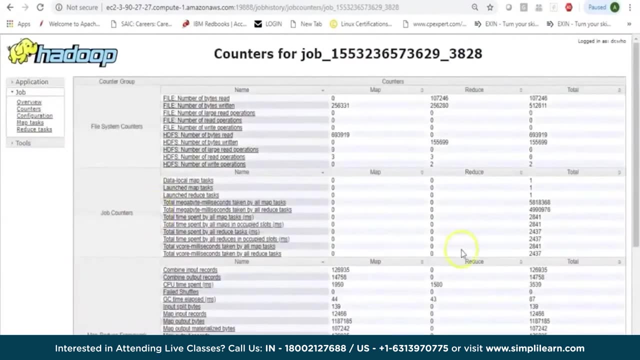 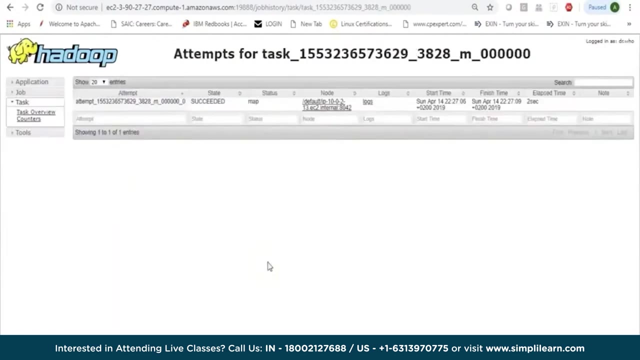 and reduce tasks it was running. you can click on this particular application which basically gives you information of your map and reduce tasks. you can look at different counters for your application. right, you can always look at map specific tasks. you can always look into one particular task. what? 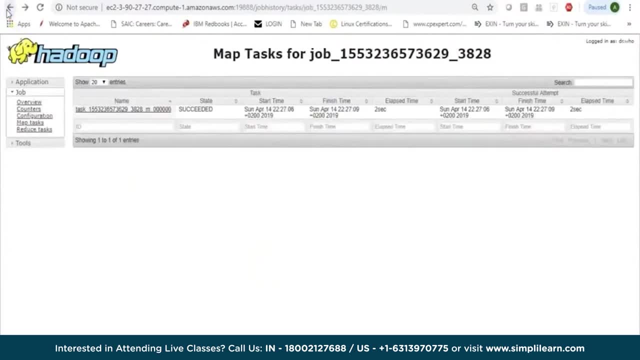 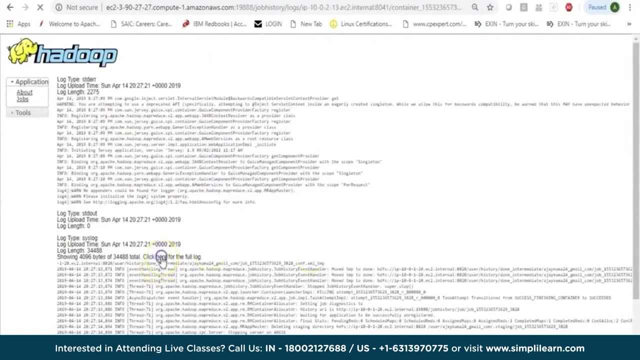 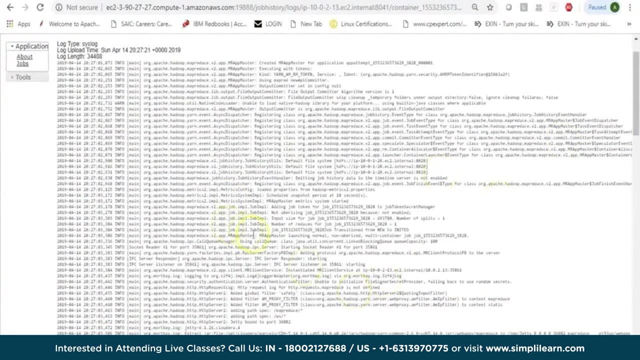 it did, on which node it was running, or you can be looking at the complete application log. so you can always click on the logs, and here you have. click here for full log which gives you the information, and you can always look for your application, which can give you information of. 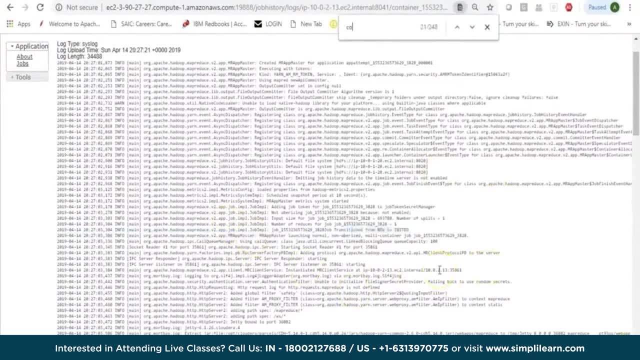 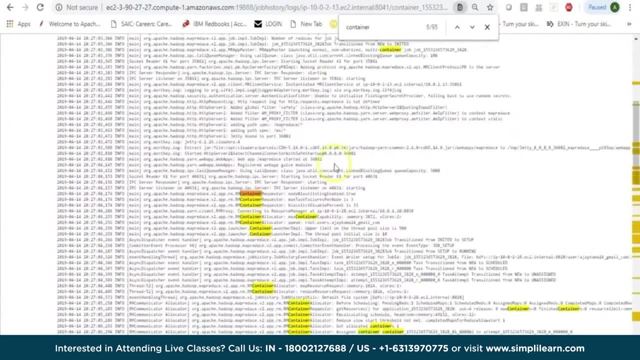 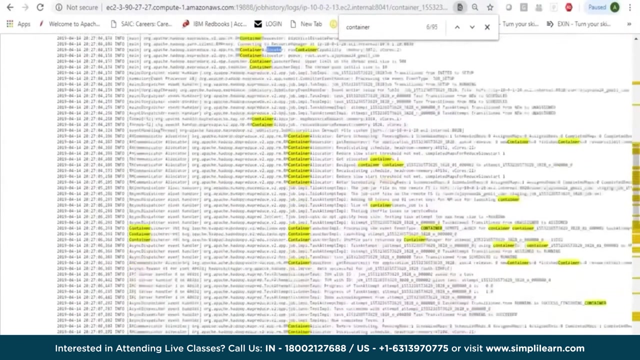 app master being launched, or you could have search for the word container so you could see a job which needs one or multiple containers and then you could say container is being requested, then you could see container is being allocated, then you can see what is the container size and then basically your task moves from initializing to running in the container and 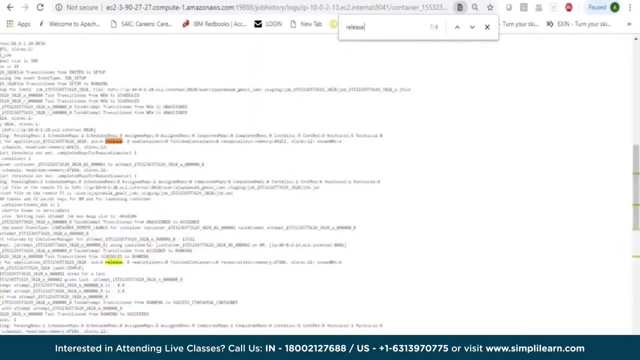 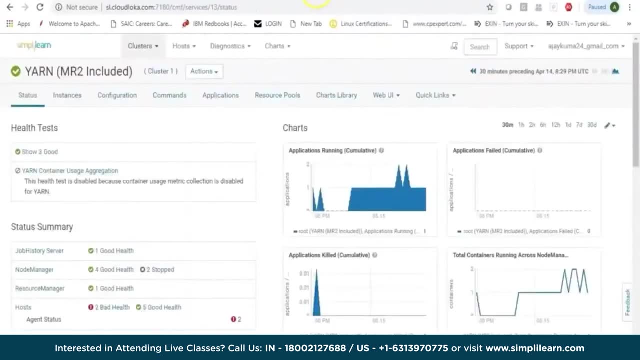 finally, you can even search for release, which will tell you that the container was released. so you can always look into the log for more information. so this is how you can interact with the yarn. this is how you can interact with your command line to look for more information. 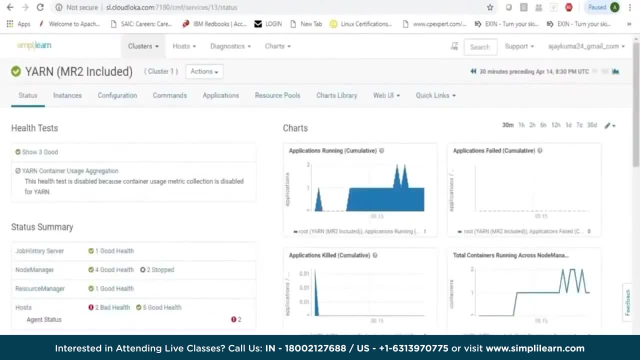 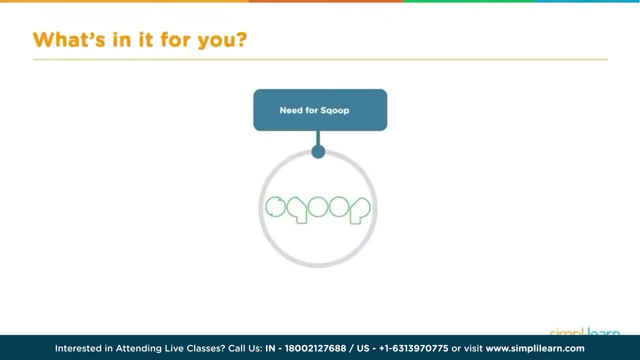 or using your yarn web UI, or you can also be looking into your hue for more information. welcome to scoop tutorial, one of the many features of the Hadoop ecosystem for the Hadoop file system. what's in it for you? today, we're going to cover the need for scoop. 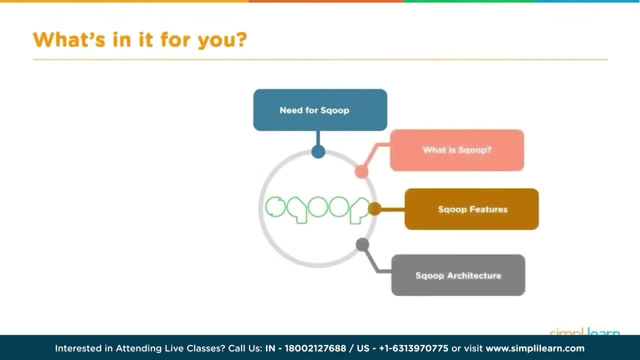 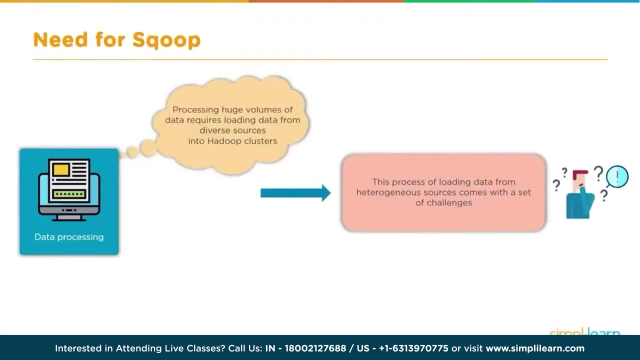 what is scoop? scoop features, scoop architecture, scoop import, scoop export, scoop processing. and then, finally, we'll have a little hands-on demo on scoops. you can see what it looks like. so where does the need for scoop come in in our big data Hadoop file system processing huge volumes of? 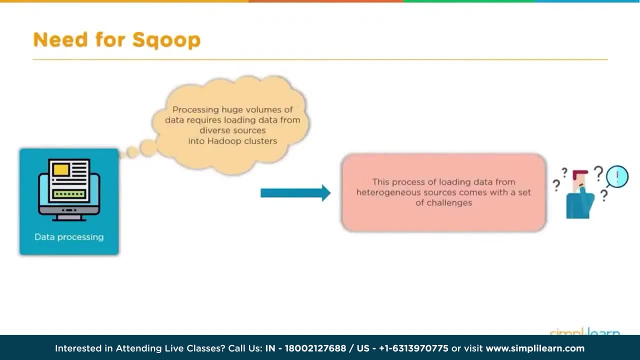 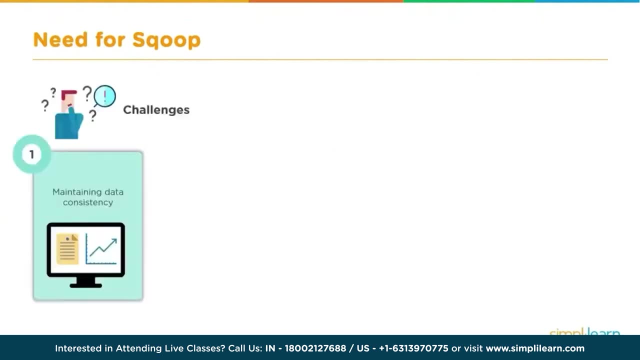 data requires loading data from diverse sources into Hadoop cluster, and you can see, here we have our data processing. and this process of loading data from the heterogeneous sources comes with a set of challenges. so what are the challenges? maintaining data consistency, ensuring efficient utilization of resources, especially when you're talking about big data. we can certainly use up the resources when importing. 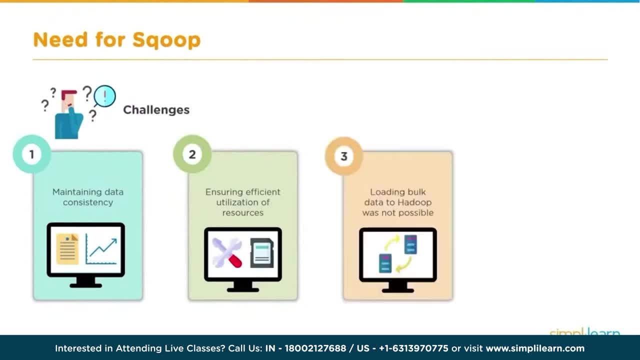 terabytes and petabytes of data over the course of time. loading bulk data to Hadoop was not possible. it's one of the big challenges that came up when they first had the Hadoop file system going, and loading data using script was very slow. in other words, you'd write a script in whatever language. 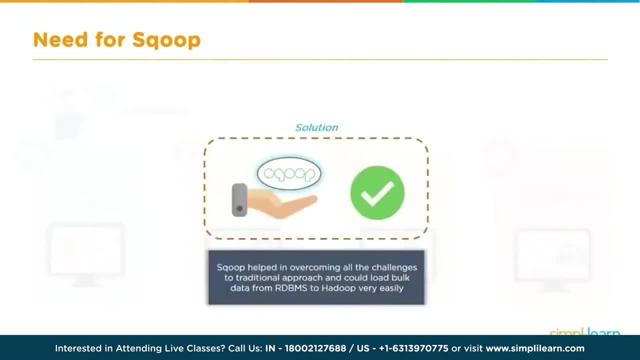 you're in and then it would very slowly load each piece and parse it in. so the solution scoop scoop helped in overcoming all the challenges to traditional approach and could lead bulk data from RDBMS to Hadoop very easily. so think your Enterprise server. you want to take the from my. 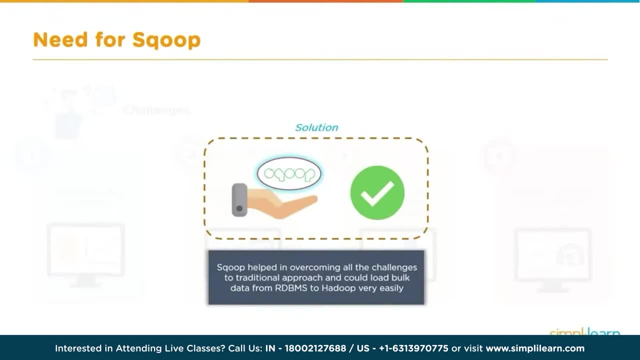 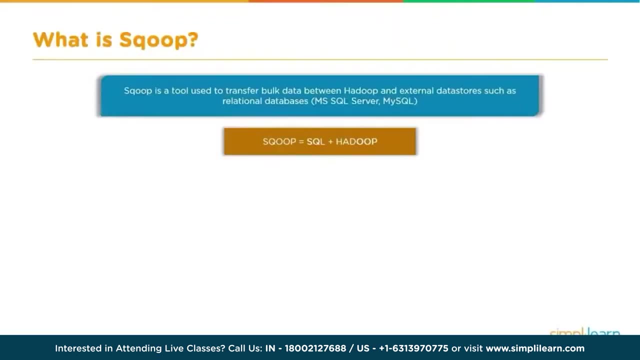 SQL or your SQL, and you want to bring that data into your Hadoop Warehouse, your data filing system, scoop. scoop is a tool used to transfer bulk of data between hadoop and external data storage such as relational databases and mysql server or the microsoft sql server or mysql server. so scoop. 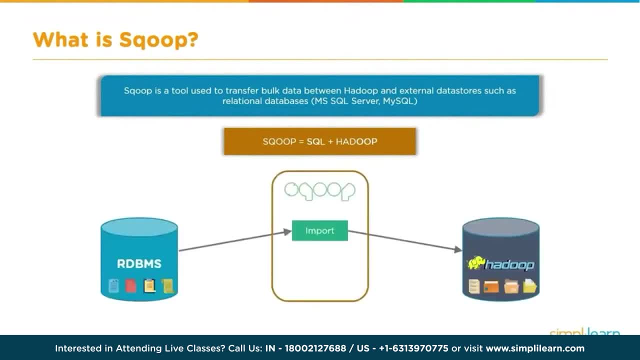 equals sql plus hadoop and you can see here we have our rdbms, all the data we have stored on there, and then your scoop is the middle ground and brings the import into the hadoop file system. it also is one of the features that goes out and grabs the data from hadoop and exports it back. 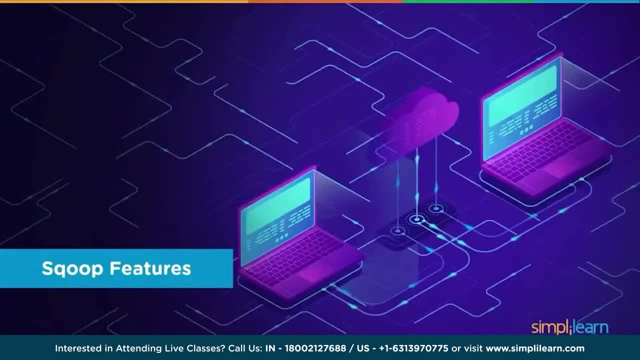 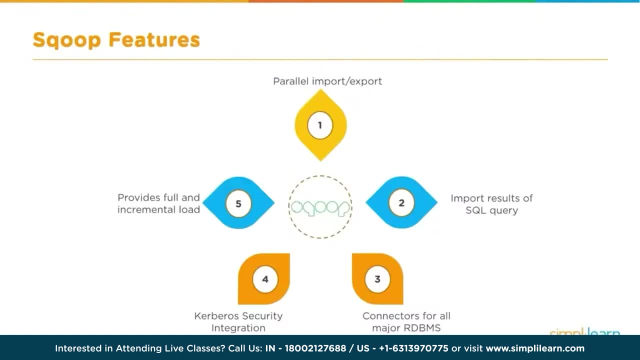 out into an rdbms. let's take a look at scoop features. scoop features has parallel import and export. it has import results of sql query connectors for all major rdbms databases. kerberos security integration provides full and incremental load. so we look at parallel import and export. scoop uses yarn- yet another resource negotiator framework- to import and. 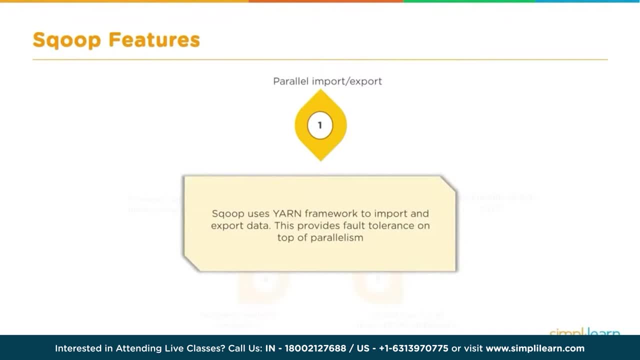 export data. this provides fault tolerance on a top of parallelism. scoop allows us to import the result return from an sql carry into the hadoop file system or the hdfs and you can see here where the import results of sql query come in. scoop provides connectors for: 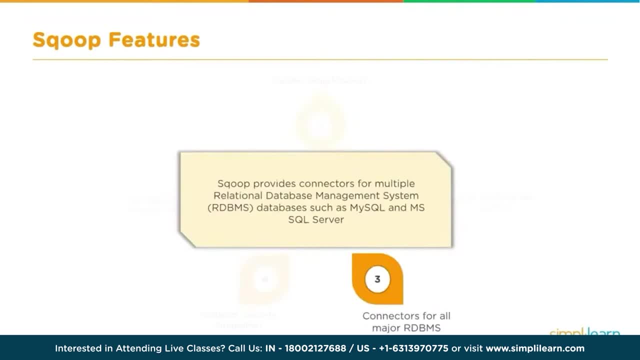 multiple relational database management system, rdbms databases such as mysql and microsoft sql server, and it has connectors for all major rdbms databases. scoop supports kerberos computer network authentication protocol that allows nodes communicating over a non-secure network to prove their identity to one another in a secure manner. scoop can load the whole table or parts of 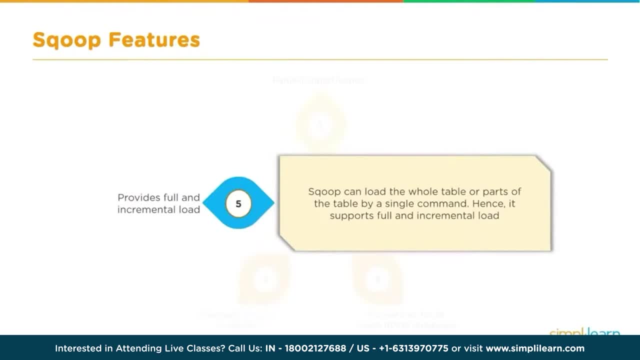 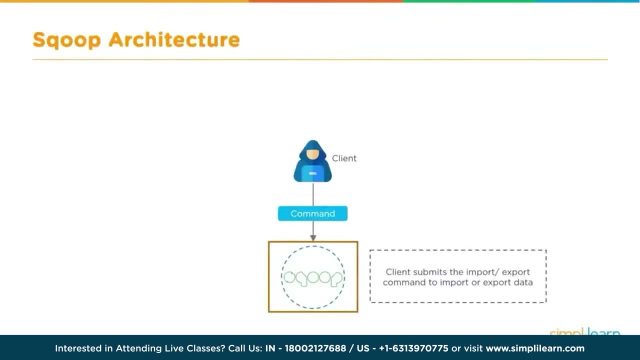 the table by a single command. hence it supports full and incremental load. let's dig a little deeper into the scoop. architecture: we have our client- in this case a hooded wizard- behind his laptop- you never know who's going to be accessing the hadoop cluster- and the client comes in and sends. 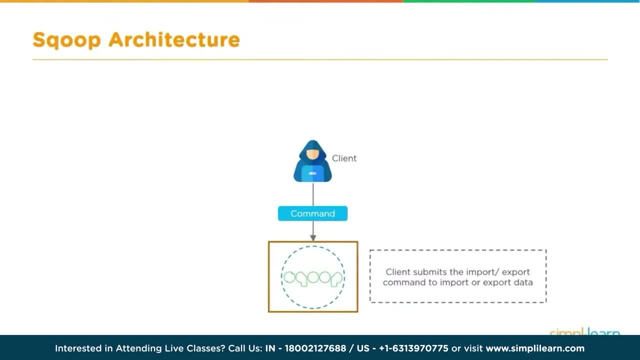 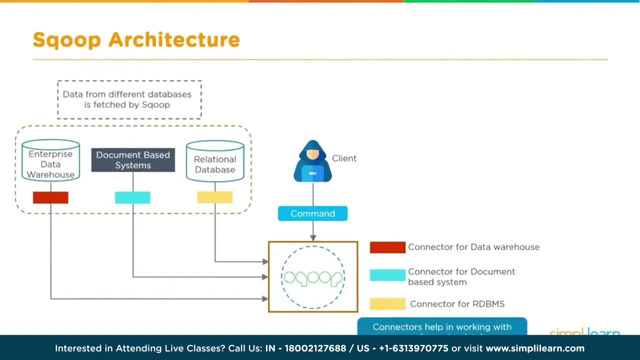 their command, which goes into scoop. the client submits the import export command to import or export data data from different databases, and so we have an enterprise data warehouse document based systems. you have connect connector for your data warehouse, a connector for document based systems which reaches out to those two. 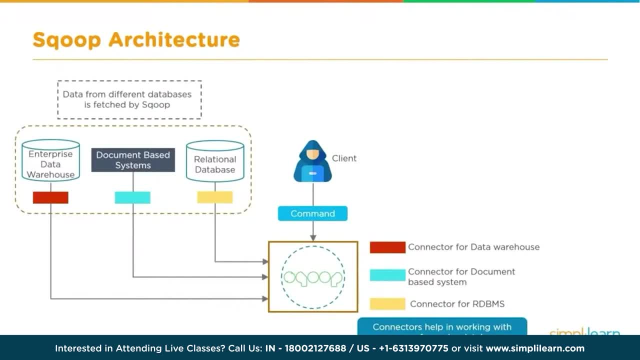 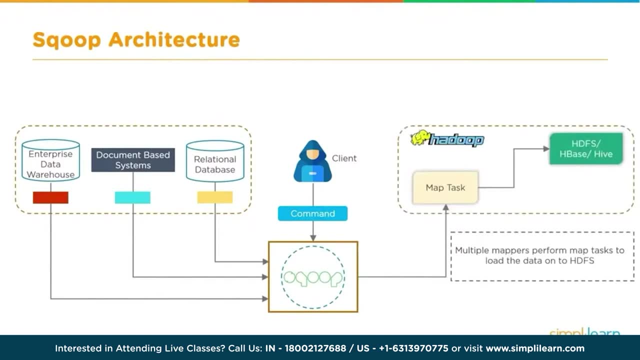 entities and we have our connector for the rdbms. so connectors help in working with a range of popular databases. multiple mappers perform map tasks to load the data onto hdfs, the hadoop file system, and you can see here we have the map task. if you remember from hadoop, hadoop is based on the. 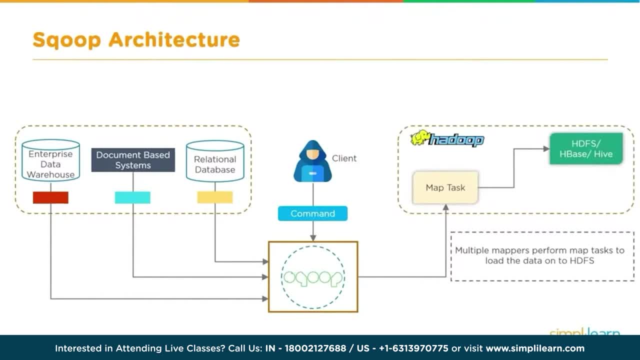 hdfs map reduce, because we're not reducing the data, we're just mapping it over. it only accesses the mappers and it opens up multiple mappers to do parallel processing and you can see here the hdfs hbase hive is where the target is for this particular one. similarly multiple map tests. 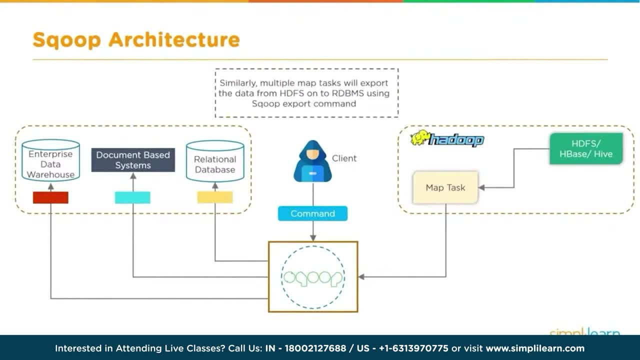 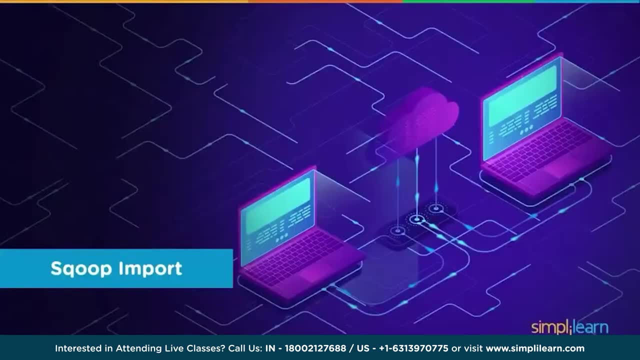 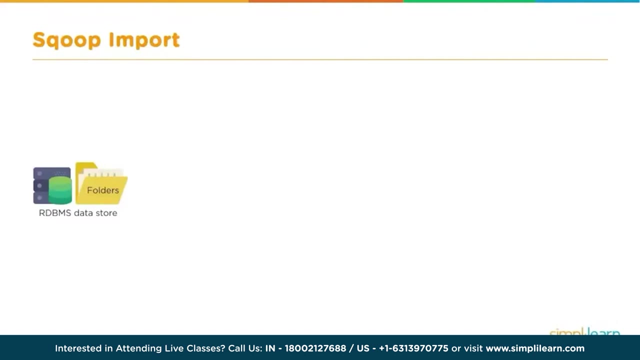 will export the data from hdfs onto rdbms using scoop export command. so just like you can import it, you can now export it using the multiple map routines, scoop import. so here we have rdbms datastore. we have the folders on there. so maybe it's your company's database, maybe it's an archive at google. 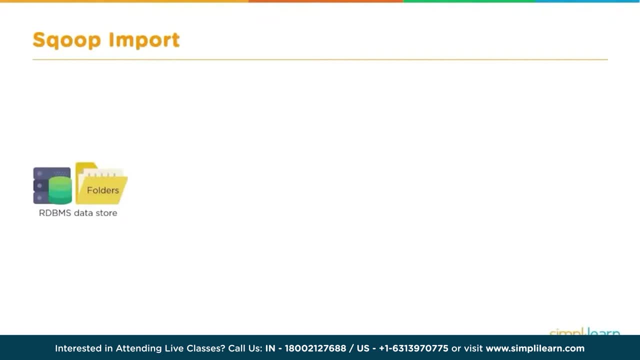 with all the searches going on, whatever it is usually you think with scoop, you think sql, you think my sql server or microsoft sql server, that kind of setup. so it gathers the metadata and you see the scoop. import so introspect database to gather metadata, primary key information, and then 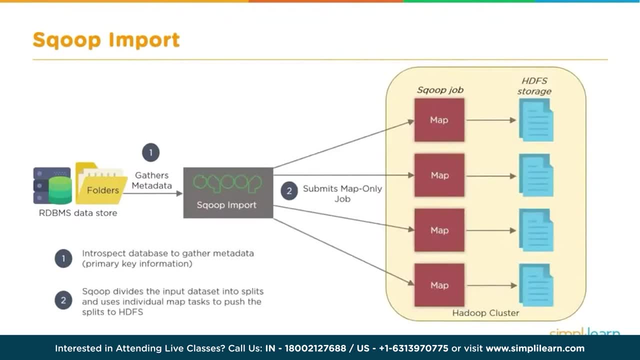 it submits. so you can see: submits map only job. remember we talked about map reduce. it only needs map side of it, because we're not reducing the data, we're just mapping it over. scoop divides the input data set into splits and uses individual map tests to push the splits into hdfs, so right into the. 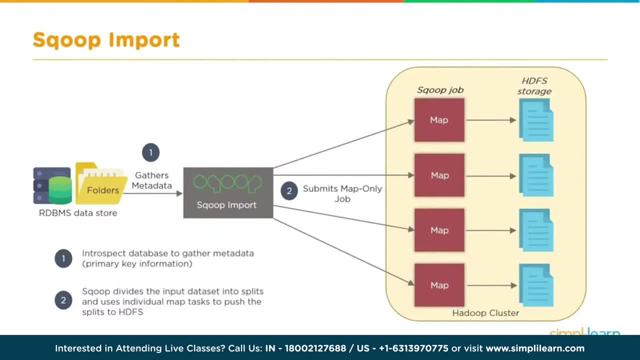 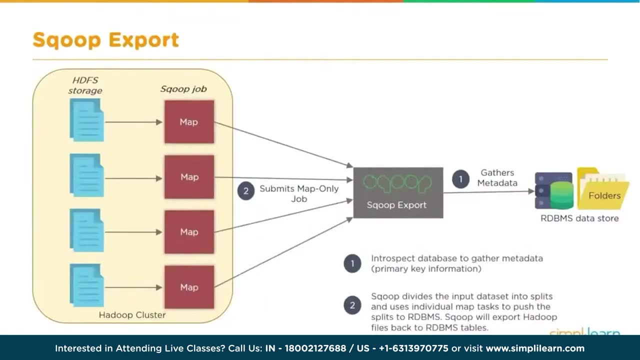 hadoop file system and you can see down on the right is kind of a small depiction of a hadoop cluster. and then you have scoop export. so we're going to go the other direction and with the other direction you have your hadoop file system storage, which is your hadoop cluster. you have your scoop. 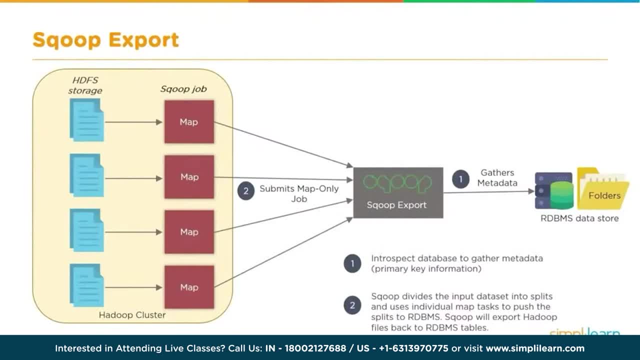 job and each one of those clusters then gets a map. mapper comes out to each one of the computers that has data on it. so the first step is: you've got to gather the metadata. so step one, you gather the metadata. step two submits map only job introspect database to 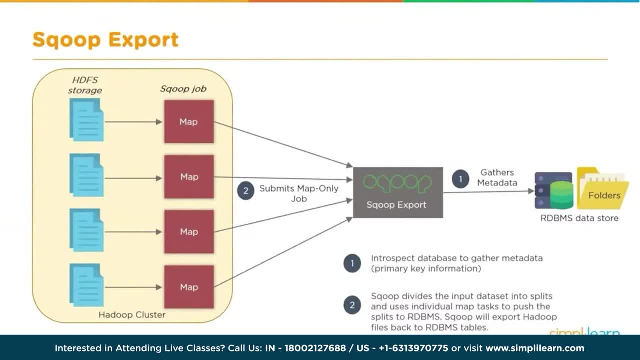 gather metadata: primary key information. scoop divides the input data set into splits and uses individual map tests to push the splits to rdbms. scoop will export hadoop files back to rdms tables and you can think of this in a number of different manners. one of them would be: if you're restoring a 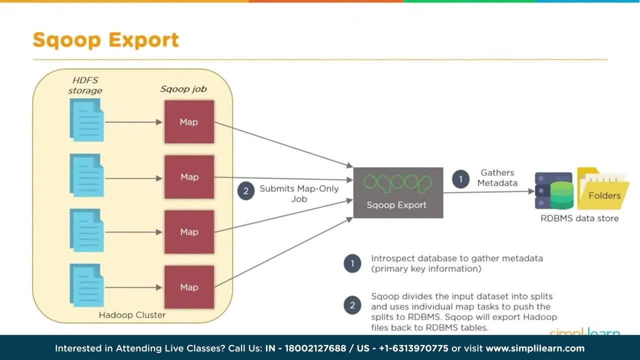 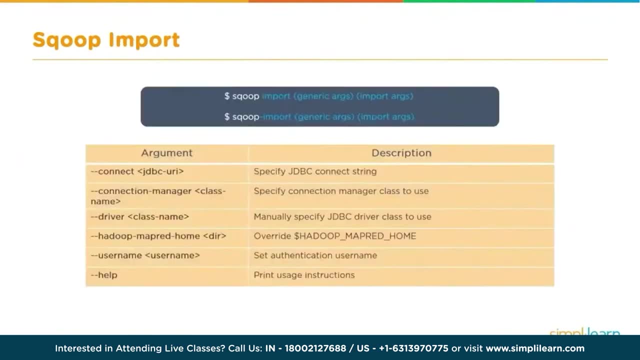 from the hadoop file system into your enterprise machines. there's certainly many others as far as exploring data and data science. so as we dig a little deeper into scoop input, we have our connect, our jdbc and our url, so specify the jdbc connect string. connecting manager. we specify the connection. 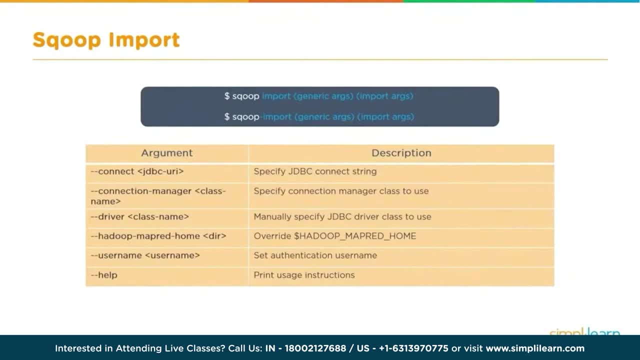 manager class to use. you can see here driver with the class name. manually specify the jdbc driver class to use: hadoop map. reduce home directory. override hadoop mapped home. use a username, set authentication username and, of course, help print uses instructions And with. 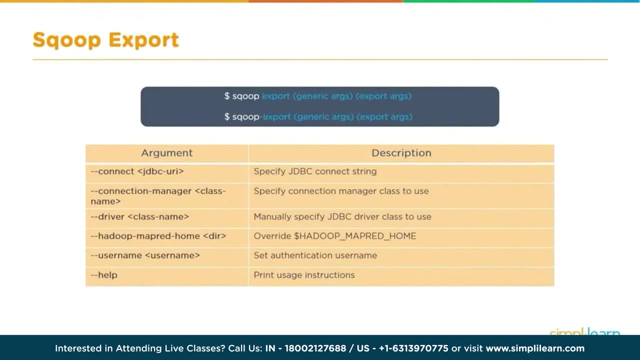 the export, you'll see that we can specify the JDBC connect string, specify the connection manager class to use manually, specify JDBC driver class to use- You do have to let it know- to override the Hadoop map, reduce home- and that's true on both of these- And set authentication username. and finally, 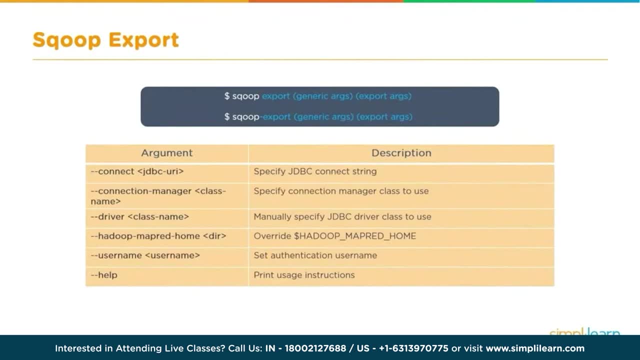 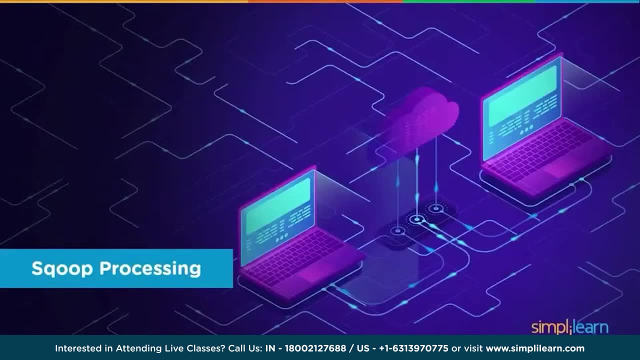 you can print out all your help setup So you can see. the format for scoop is pretty straightforward, both import and export. So let's continue on our path and look at scoop processing and what the computer goes through for that. And when we talk about scoop processing, first, scoop runs in the 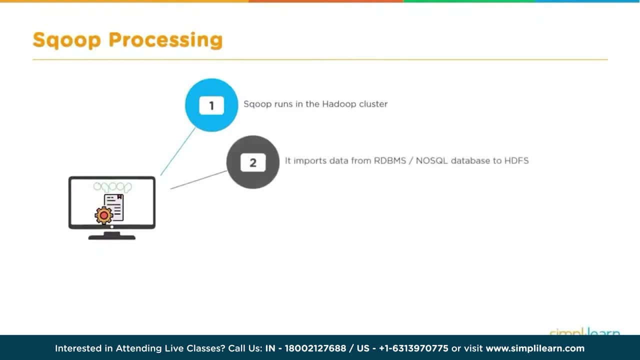 Hadoop cluster. It imports data from the RDBMS, the NoSQL database, to the Hadoop file system. So remember it might not be importing the data from a RDBMS, it might actually be coming from a NoSQL. 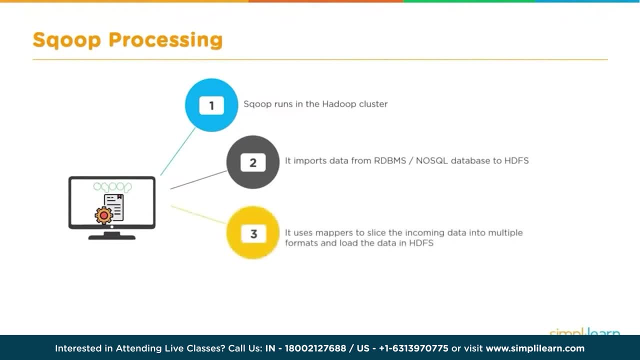 and there's many out there. It uses mappers to slice the incoming data into multiple formats and load the data into HDFS. It exports data back into an RDBMS, while making sure that the schema of the data in the database is maintained. So now that we've looked at the basic commands in our scoop, in the scoop. 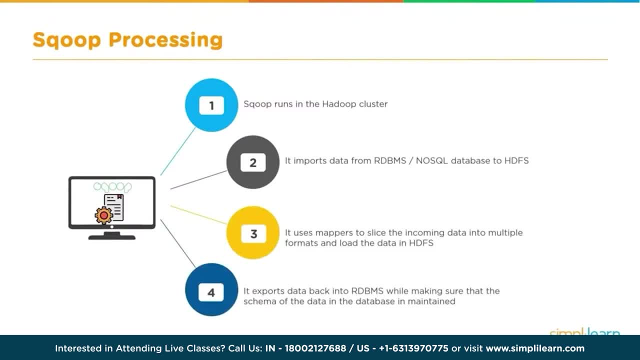 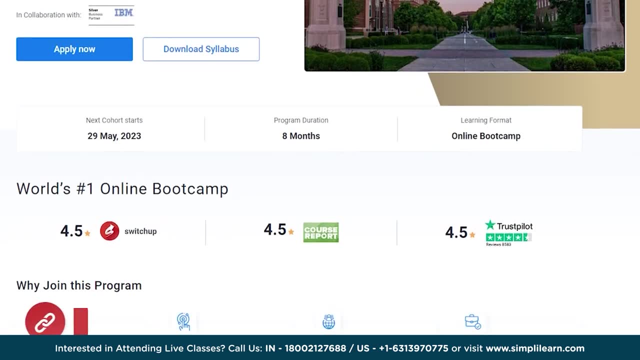 processing, or at least the basics as far as theory is concerned. Hello learners, SimplyN brings you a postgraduate program in data engineering, developed in partnership with Purdue University and IBM. To learn more about this course, you can find the course link in the description box below. Let's 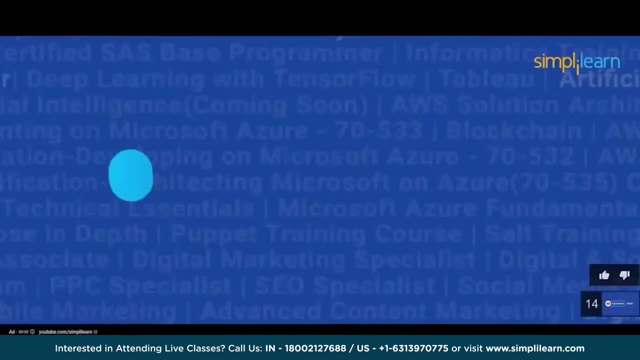 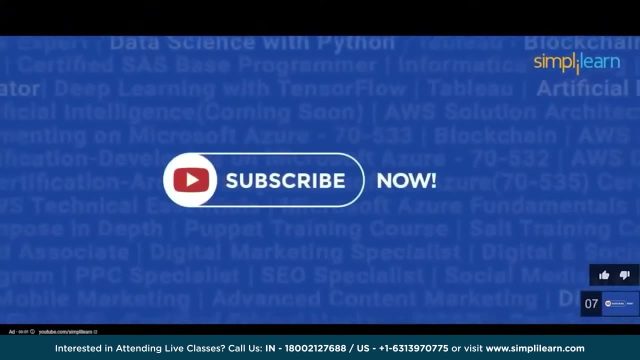 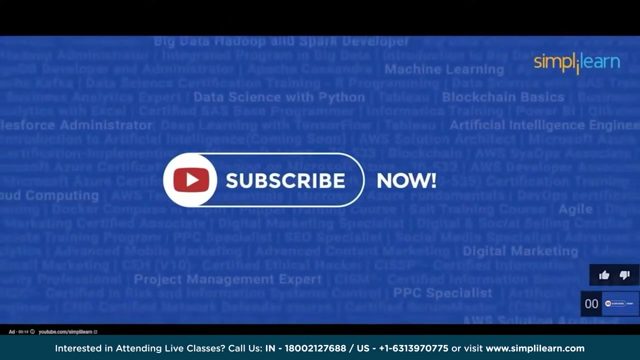 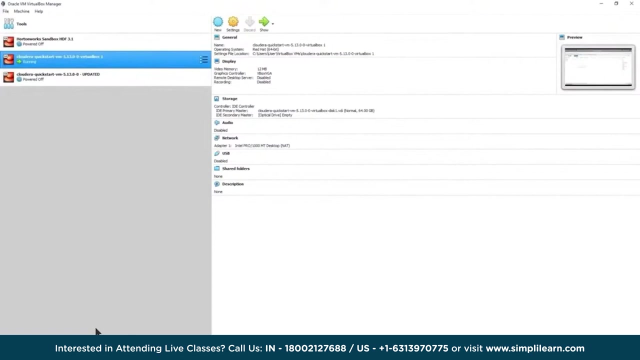 just jump in And take a look at a demo on Scoop. For this demo I'm going to use our Cloudera Quick Start. If you've been watching our other demos we've done, you'll see that we've been using that pretty consistently. Certainly this will work in any of your 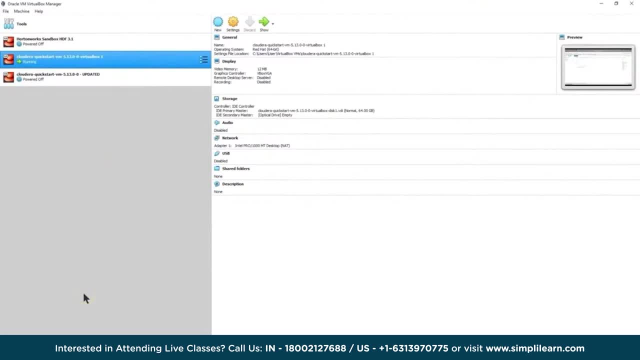 Horton sandbox, which is also a single node testing machine. Cloudera is one of them. There's a docker version instead of virtual box, And you can also set up your own Hadoop cluster Plan a little extra time If you're not an admin. it's actually a pretty significant endeavor For an admin if you've. 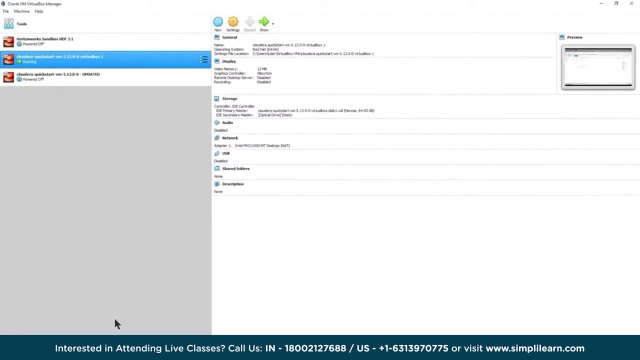 been adminning Linux machines for a very long time, and you know a lot of the commands. I find for most admins, it takes them about two to four hours the first time they go in and create a virtual machine and set up their own Hadoop. In this case, though, when you're just learning and getting 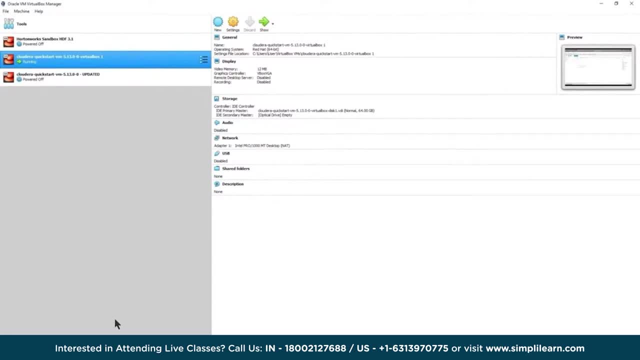 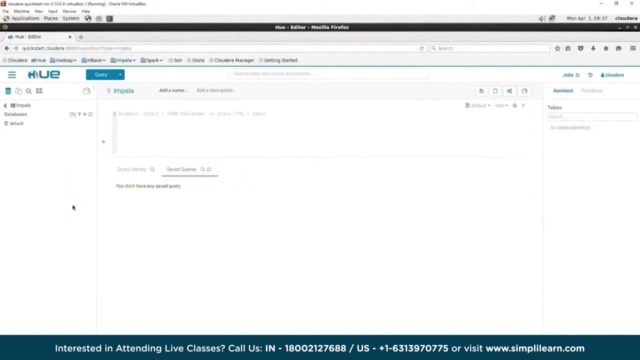 set up. best to start with Cloudera. Cloudera also includes an install version of MySQL. That way you don't have to reinstall the SQL version for importing data from and to. Once you're in the Cloudera Quick Start you'll see it opens a nice CentOS Linux interface And it has the desktop set up on there. 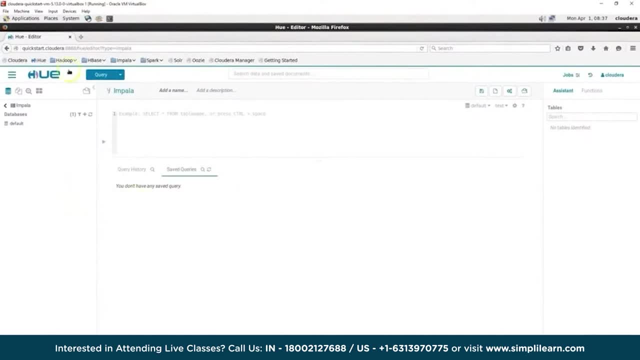 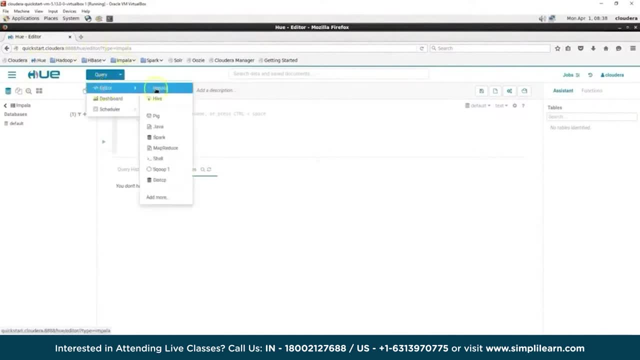 Under Hue, I can go under Query, I can pick an editor And we'll go right down to Scoop. So now I'm just going to load the Scoop Editor in our Hue. Now I'm going to switch over and do this all in command line. 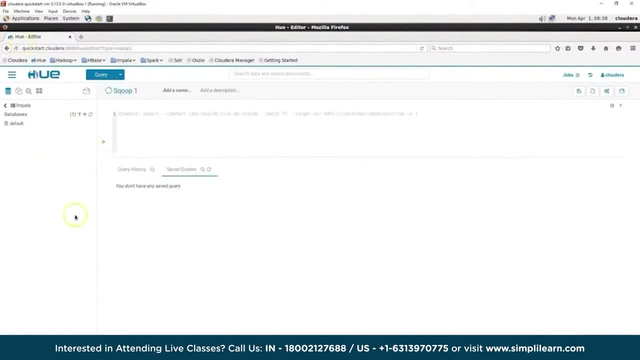 I just want to show that you can actually do this in Hue through the web-based interface. The reason I like to do the command line is specifically on my computer it runs much quicker. Or if I do the command line here and I run it, it tends to have an extra lag or an added layer in it. So for this we're going to go. 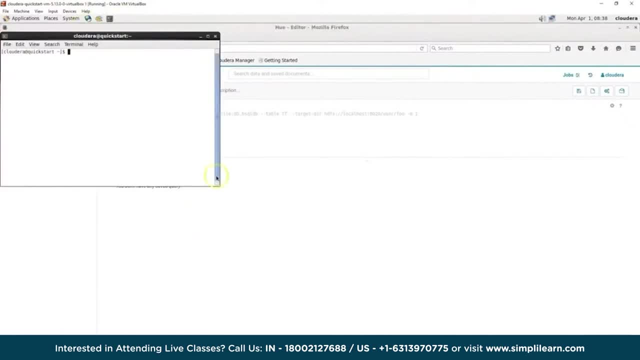 ahead and open our command line. The second reason I do this is we're going to need to go ahead and edit our MySQL so we have something to scoop in. Otherwise I don't have anything going in there And of course we zoom in. 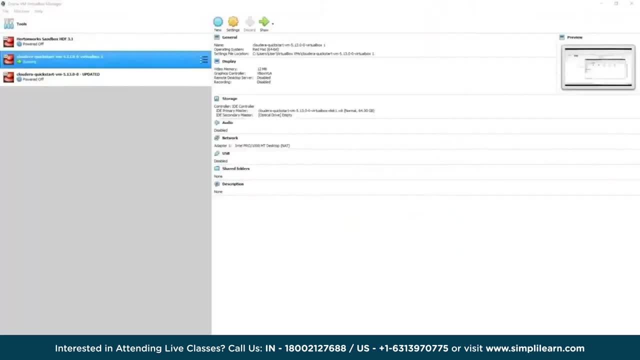 We'll zoom in this and increase the size of our screen. So for this demo our hands-on, I'm going to use Oracle VirtualBox Manager and the Cloudera QuickStart. If you're not familiar with this, we do have another tutorial we put out and you can send a note in the YouTube video below and let our team know and they'll send you a link. 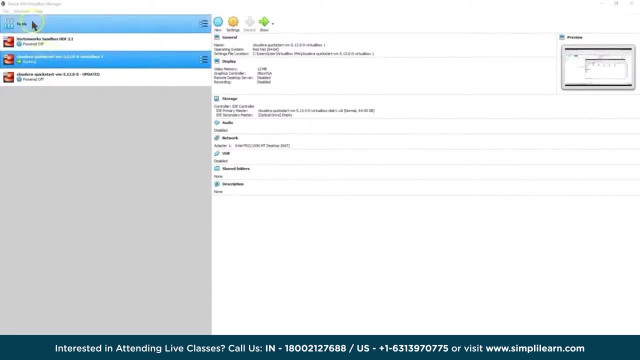 Or come visit wwwsimplylearncom. Now. this creates a Linux box on my Windows computer, so we're going to be in Linux and it'll be the Cloudera version with Scoop. It will also be using MySQL- MySQL Server. 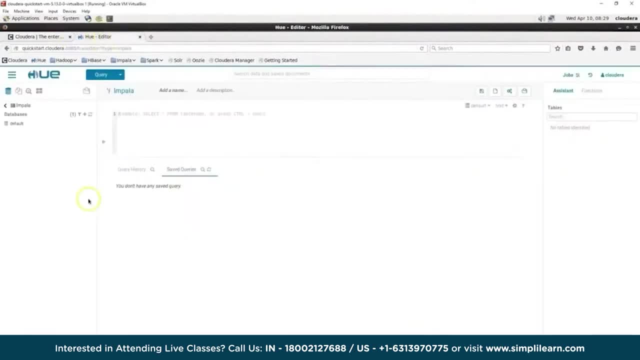 Once inside the Cloudera VirtualBox we'll go under the Hue Editor. Now we're going to do everything in Terminal Window, but I just want you to be aware that under the Hue Editor you can go under Query Editor and you'll see as we come down here. here's our scoop on this. 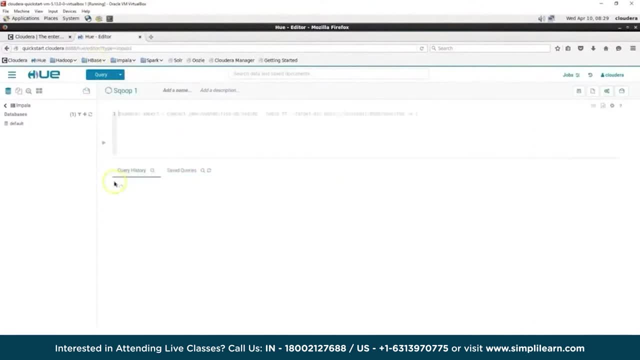 So you can run your scoop from in here. Now, before we do this, we have to do a little exploration in MySQL or MySQL Server. That way we know what data is coming in. So let me go ahead and open up a Terminal Window. 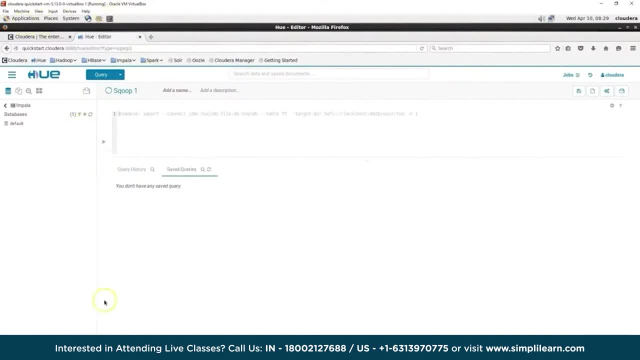 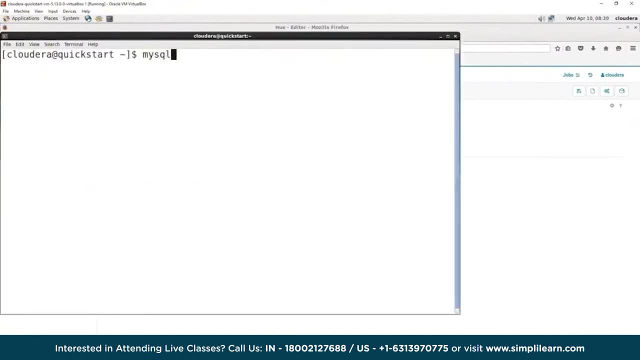 In Cloudera. you have a Terminal Window at the top here that you can just click on and open it up, And let me just go ahead and zoom in on here. Go View and Zoom In. Now to get into MySQL Server, you simply type in MySQL and this part will depend on your setup. 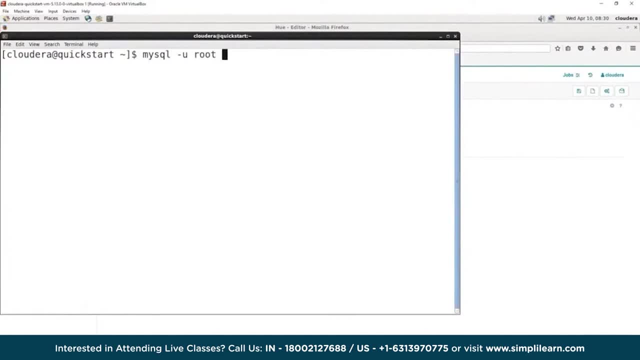 Now the Cloudera QuickStart comes up that the username is root and the password is Cloudera. Kind of a strange quirk is that you can put a space between the minus U and the root, but not between the minus P and the Cloudera. 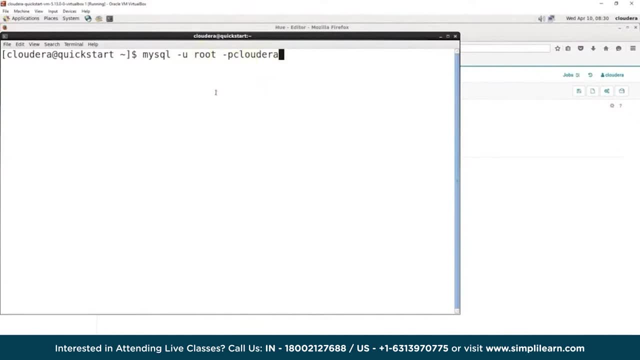 Usually you'd put in a minus capital P, and then it prompts you for your password on here For this demo. I don't worry too much about you knowing the password on that, so we'll just go right into MySQL Server, since this is the standard password for this QuickStart. 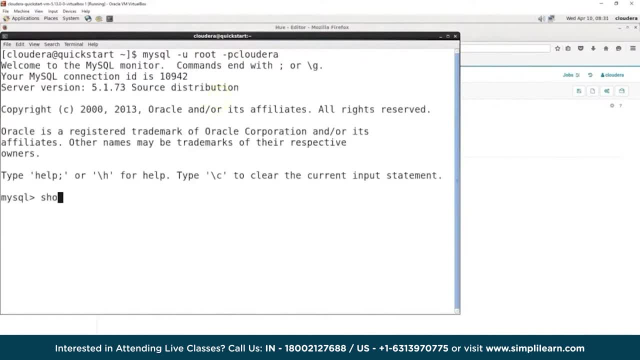 And you can see we're now into MySQL And we're going to do just a couple of quick commands in here. There's show database, There's show database, There's show database, And you follow by the semicolon. That's standard in most of these shell commands. so it knows it's the end of your shell command. 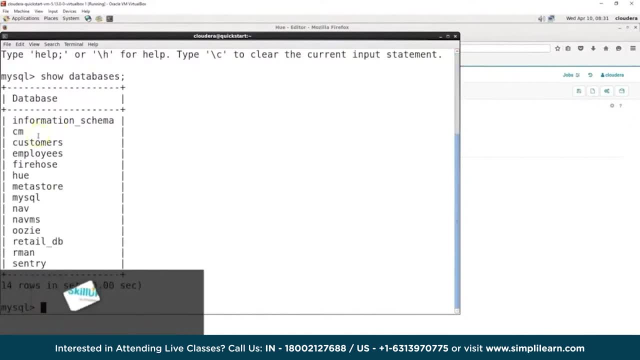 And you'll see in here, in the QuickStart, Cloudera, QuickStart, the MySQL comes with a standard set of databases. These are just some of these have to do with the Uzi, which is the Uzi part of Hadoop. 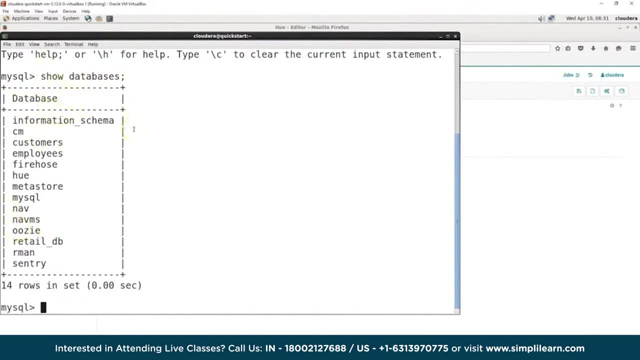 where others of these, like customers and employees and stuff like that, those are just for demo purposes. They come as a standard setup in there so that people going in for the first time have a database to play with, which is really good for us, so we don't have to recreate it. 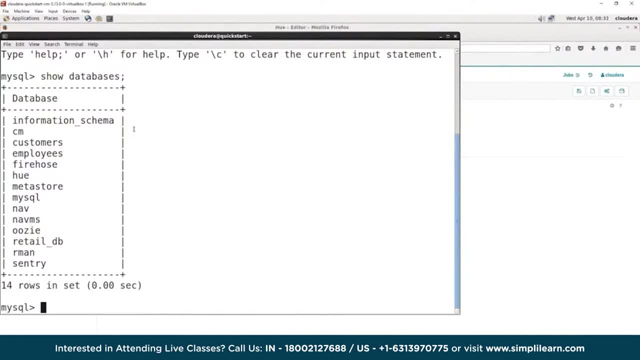 We don't have to recreate those databases And you will see on the list here we have a retail underscore DB And then we can simply do: use retail underscore DB. This will set that as a default in MySQL, And then we want to go ahead and show the tables. 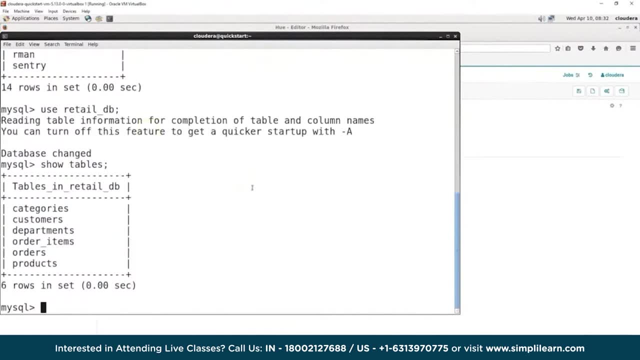 And if we show the tables, you can see under the database- the retail DB database- we have categories, customers, departments, order items, orders, products. So there's a number of tables in here And we're going to go ahead and just use a standard. 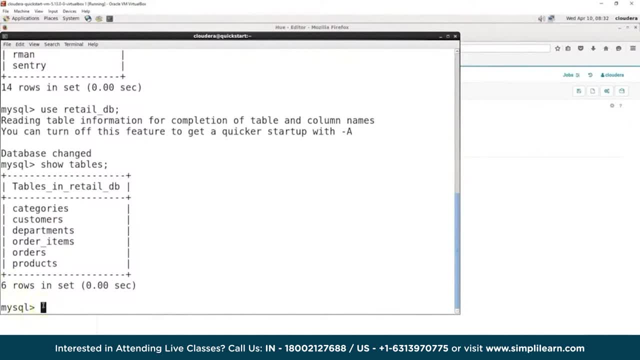 SQL command And if you did our hive language you'll note, remember it's the same for HQL. also on this, We're just going to select star everything from departments. So there's our departments table and we're going to list everything on the departments table. 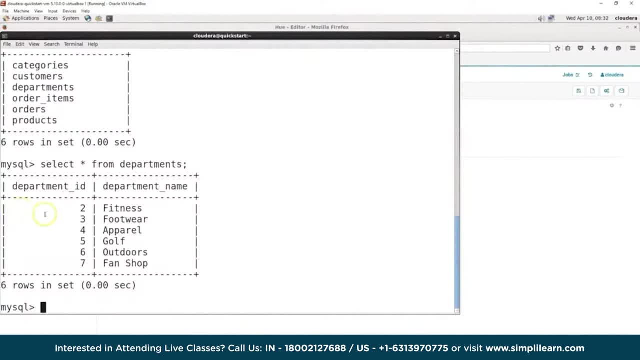 And you'll see we have six lines in here and it has a department ID and a department name: Two for fitness, three for footwear, so on and so forth. Now, at this point I can just go ahead and exit, But it's kind of nice to have this data up here so we can look at it. 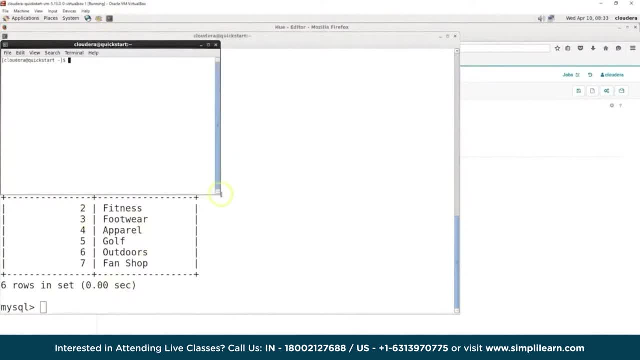 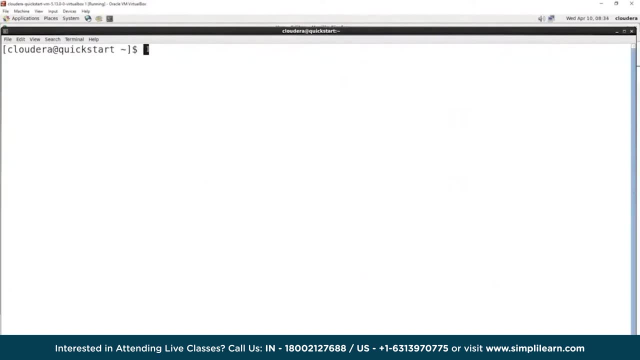 and flap back and forth between the tables because that's really cool forth between the screens. So I'm going to open up another terminal window and we'll go ahead and zoom in on this also, And it isn't too important for this particular setup, but it's always kind of 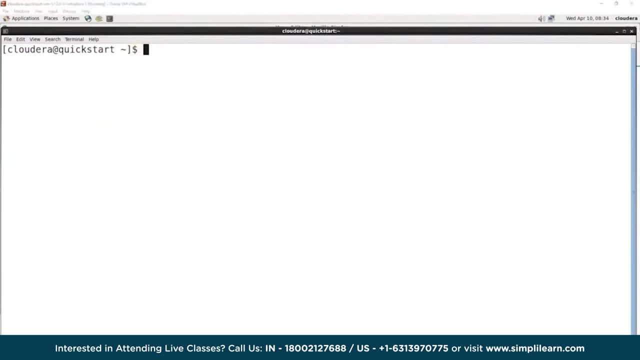 fun to know what your setup, you're working with, What is your host name? And so we'll go ahead and just type that in. This is a Linux command and it's a host name minus f, and you see we're on quick start Cloudera. No surprise there. Now this next command is going to be a little bit longer. 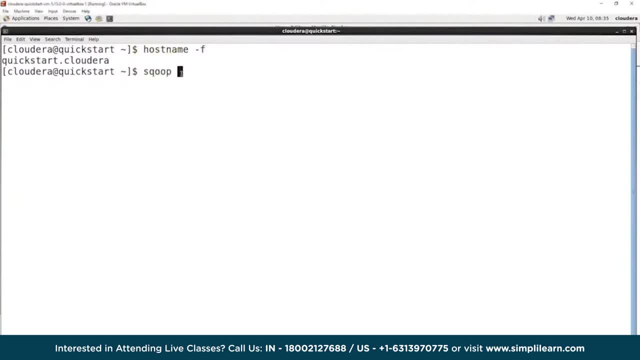 because we're going to be doing our first scoop command And I'm going to do two of them. We're going to list databases and list tables. It's going to take just a moment to get through this because there's a bunch of stuff going on here. So we have scoop, we have list databases, we have 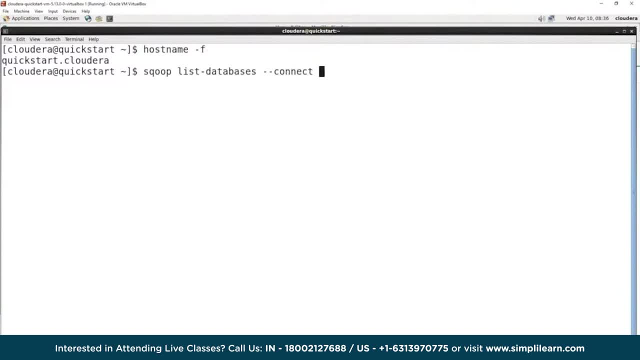 connect And under the connect command, we need to let it know how we're connecting. We're going to use the JDBC- This is a very standard one- JDBC, MySQL. So you'll see that if you're doing an SQL database, that's how you start it off with. 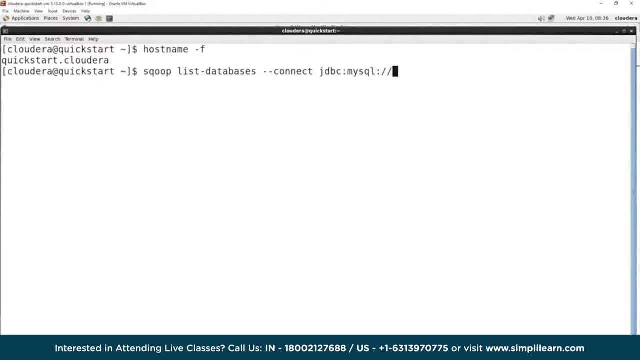 And then the next part. this is where you have to go look it up. It's how it was created. So if your admin created a MySQL server with a certain setup, that's what you have to go by And you'll see that. 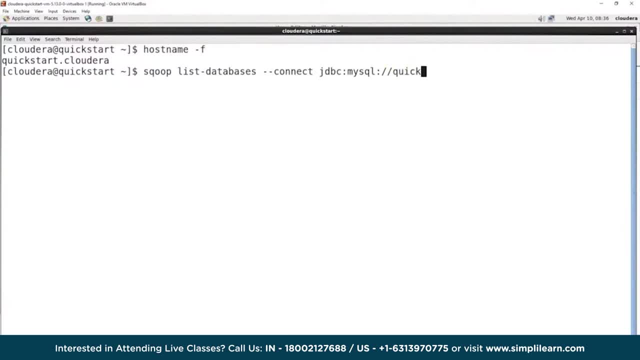 usually they list this as localhost, So you'll see something like localhost. sometimes There's a lot of different formats, But the most common is either localhost or the actual connection. So in this case we want to go ahead and do quick start 3306.. And so quick start is the name of the localhost. 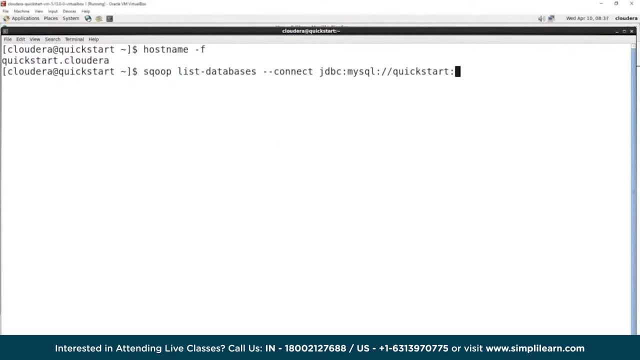 database and how it's hosted, And then we're going to go ahead and do quick start 3306.. And so quick start is the name of the localhost database and how it's hosted And when you set up the quick start for Hadoop. 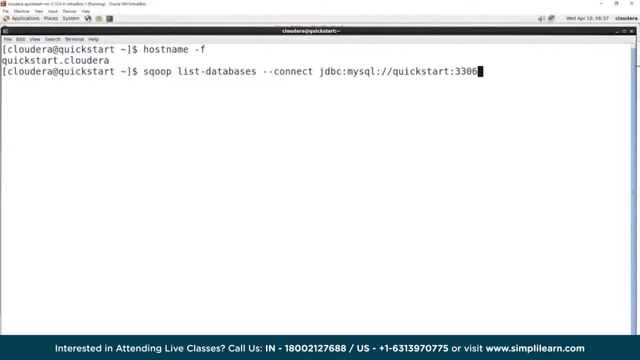 under Cloudera. it's port 3306 is where that's coming in, So that's where all that's coming from, And so there's our path for that. And then we have to put in our password. We type in the type password, If you. 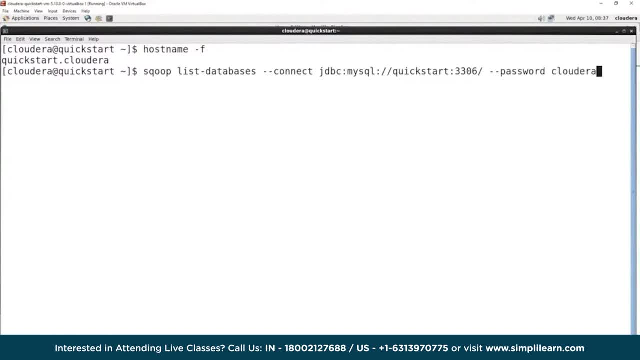 look it up. password on the Cloudera. quick start is Cloudera And we have to also let it know the username. And again, if you're doing this, you'd probably put in a minus capital. You can actually just do it for a prompt for the password. So if you leave that out, it'll prompt you And then you can. 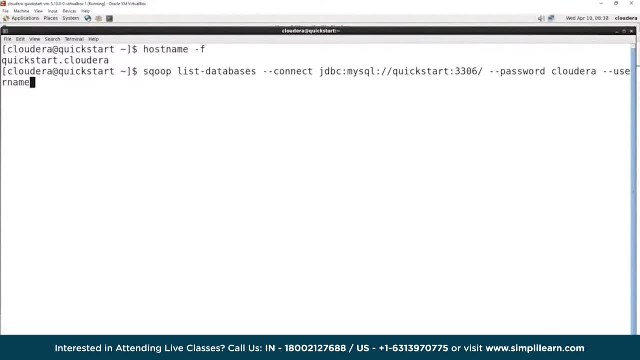 do, But for this it doesn't really matter. I don't care if you see my password, It's the default one for Cloudera: quick start, And then the username on here is simply root, And then we're going to put. 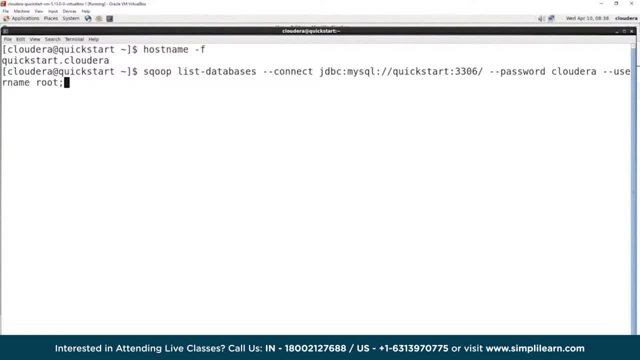 our semicolon at the end And so we have here our full setup. Then we go ahead and list the databases And you'll see you might get some warnings on here. I haven't run the updates on the quick start. I suggest you're not running the updates either if you're doing this for the first time, because 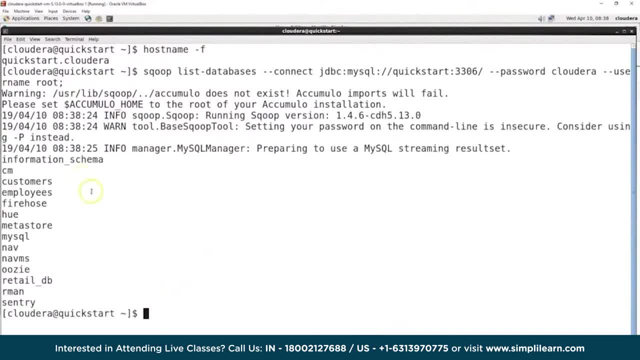 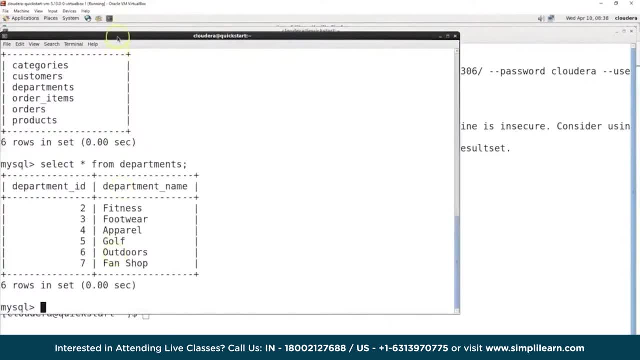 it'll do some reformatting on there And it quickly pops up and you can see. here's all of our the tables we went in the last week, And then we have our password, And then we have our password, And if we go back to on the previous window, we should see that these tables match. So here we. 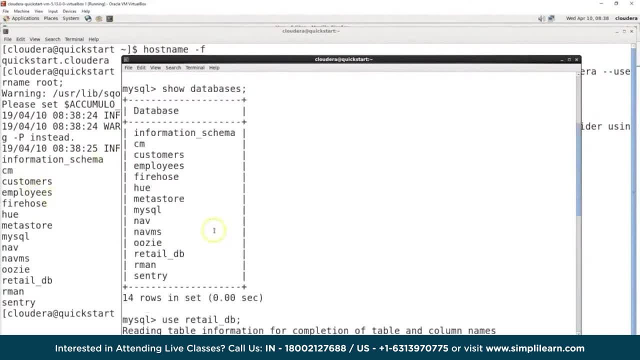 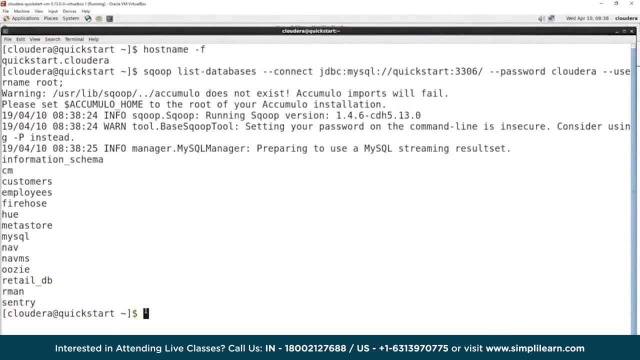 come in and here we have our databases And you can see back up here where we had the CM, customers, employees and so on, So the databases match. And then we want to go ahead and list the tables for a specific database. So let's go ahead and do that. I'm a very lazy typist So I'll put the up arrow. 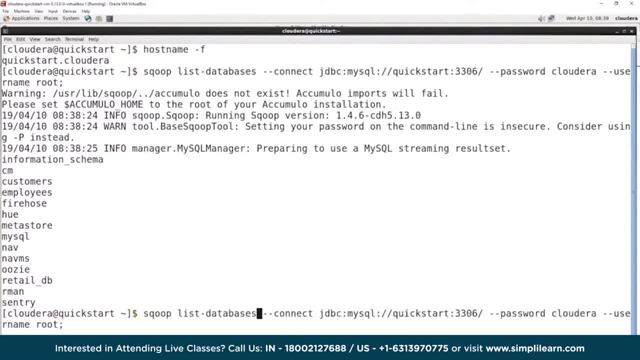 in And you can see here, scoop list databases. We're just going to go back and change this from databases to a specific database And then we're going to go ahead and list the tables for a specific database And then we're going to go ahead and do list tables. So we want to list the 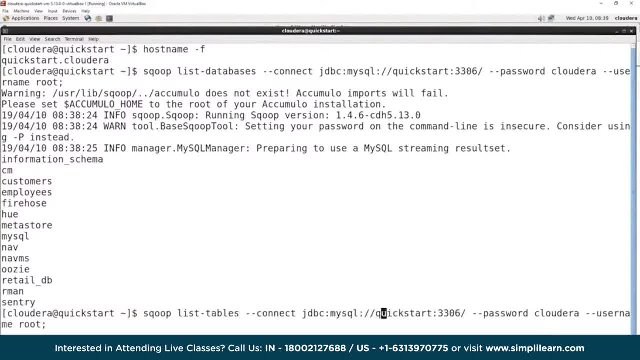 tables in here: Same connection, So most of the connection is the same, except we need to know which tables we're listing. An interesting fact is you can create a table without being under a database, So if you left this blank, it will show the open tables that aren't connected directly to. 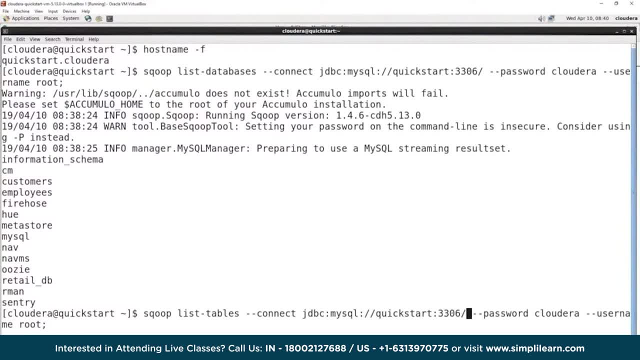 a database or under a database. But what we want to do is, right past this last slash on the 3306, we want to put that retail underscore DB, because that's the database we're going to be working with And this will go in there and show the tables And then we're going to go ahead and list the. 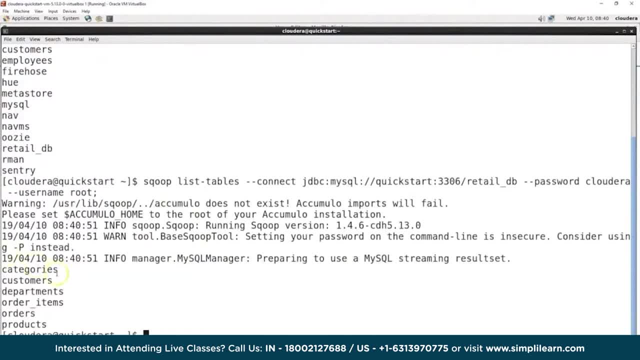 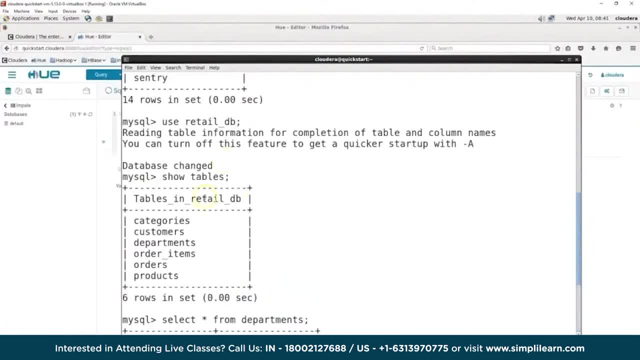 tables listed under that database. And here we go. We got categories, customers, departments, order items and products. If we flip back here real quick, there it is the same thing we had. We had categories, customers, departments, order items and so on. And so let's go ahead and run. 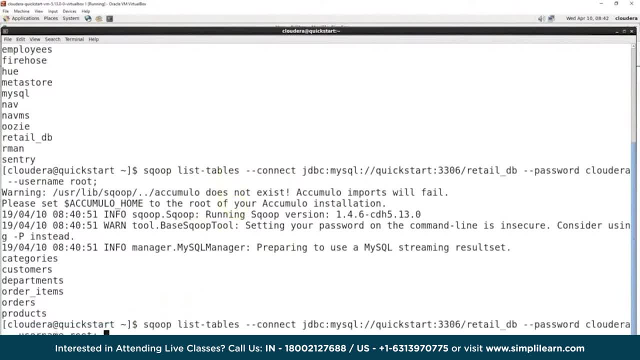 our first import command. And again I'm that lazy typer. So we're going to do scoop And instead of list tables we want to go ahead and import. So there's our import command. And so once we have our import command, we're going to tell it exactly what we're going to import. So everything else is. 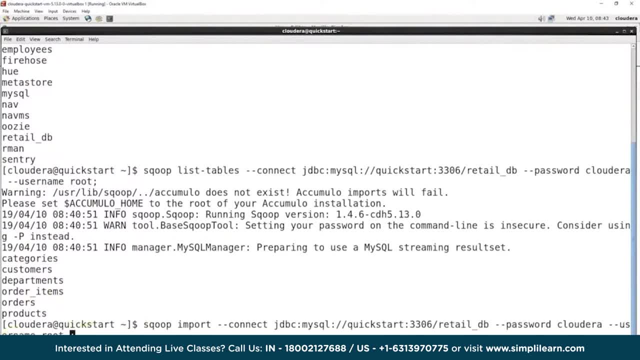 the same We're importing from the retail DB. So we keep that And then at the very end we're going to tag on dash, dash, table. That tells us we can tell it what table we're importing from And we're going to import departments. There we go. So this is pretty straightforward, because what's nice about? 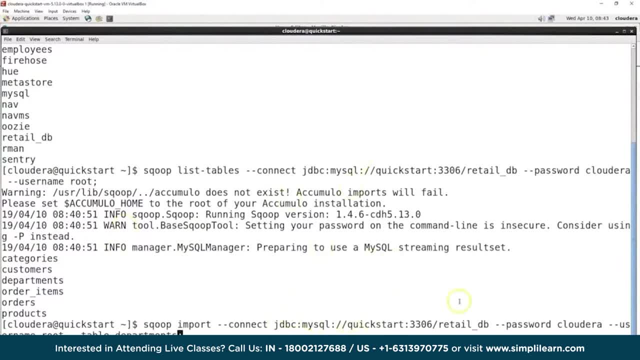 this is. you can see the commands are the same. I got the same connection. I change it for the whatever database I'm in. Then I come in here. Our password and the username are going to be the same. That's all under the MySQL server setup, And then we let it know that we're going to import. 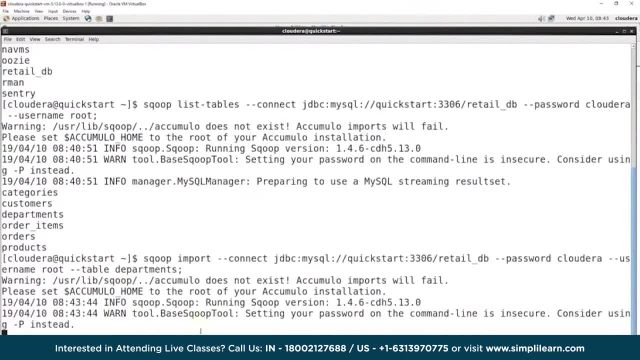 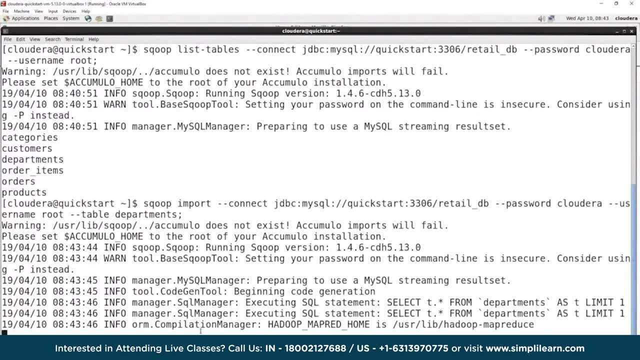 it And then we run this And this is going to actually go through the mapper process in Hadoop. So this is a mapping process. It takes the data and it maps it up to different parts in the setup in Hadoop on there and then saves that data into the Hadoop file system. And it does take it a. 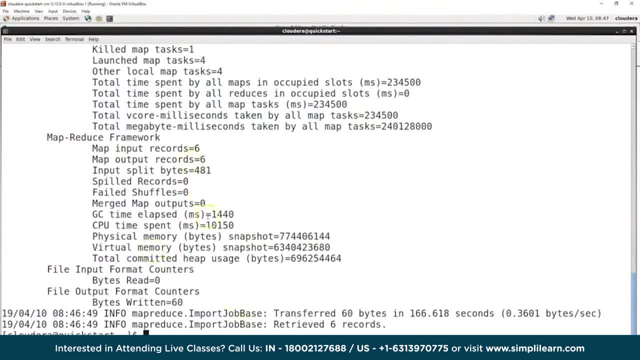 moment to zip through, which I kind of skipped over for you, Since it is running a. you know it's designed to run across the cluster, not on a single node. So when you're running on a single node it's going to run slow, even if you dedicate a couple cores to it. I think I put. 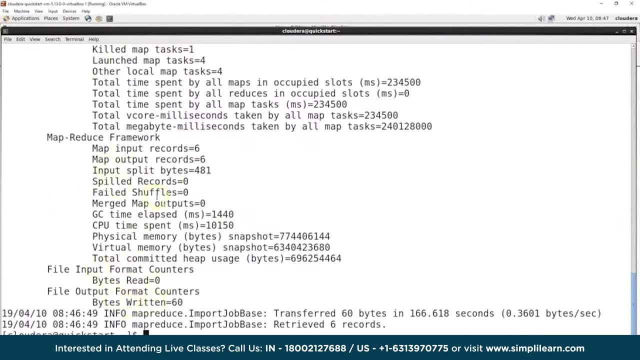 dedicated four cores to this one, And so you can see right down here we get to the end. It's now mapped in that information And then we can go in here, We can go under, can flip back to our Hue, And under Hue, on the top, I have there's databases, and the second icon over is your Hadoop. 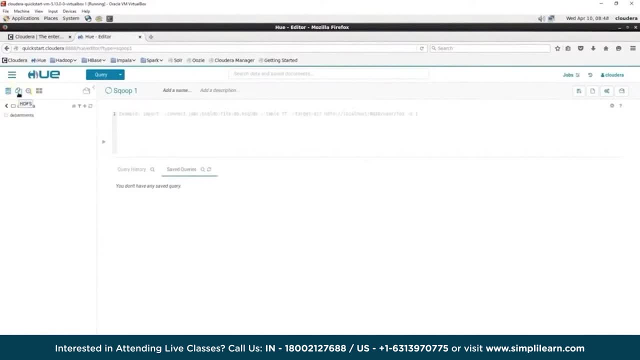 file system And we can go in here and look at the Hadoop file system And you'll see it show up underneath our documents. There it is departments, Cloudera, departments, And you can see there's always a delay when I'm working in Hue, which I don't like, And that's the quick start issue. 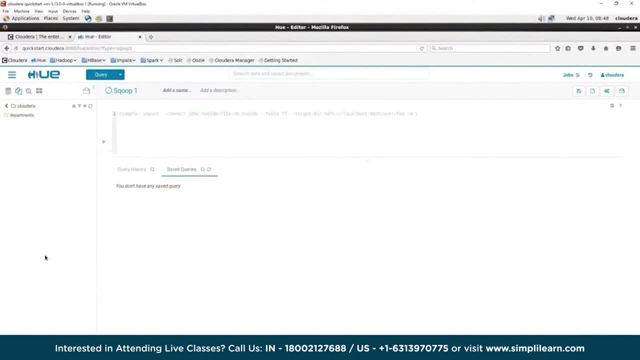 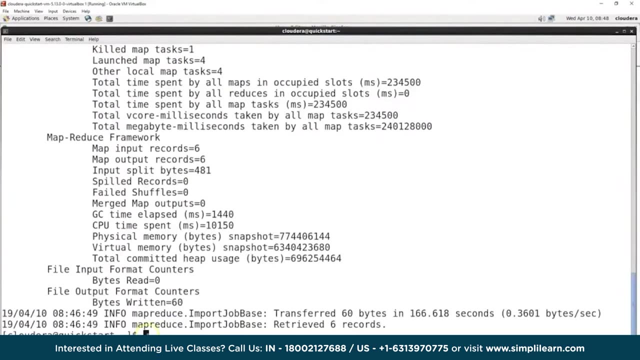 That's not necessarily running it on a server. When I'm running it on a server, you pretty much have to run through some kind of server interface. I still prefer the terminal window. It still runs a lot quicker. But we'll flip back on over here to the command line And we can do the Hadoop. 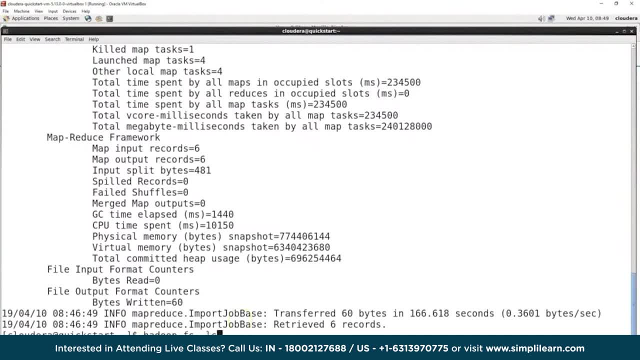 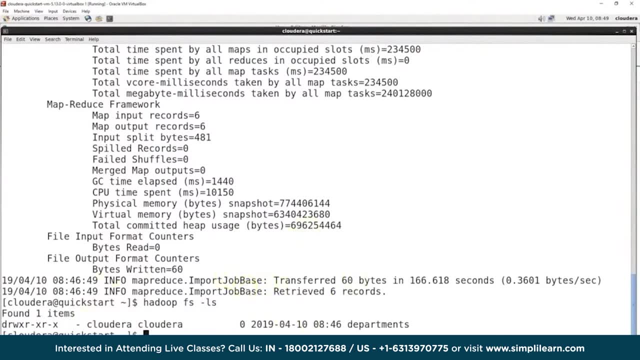 type in the Hadoop FS and then list minus LS, And if we run this you'll see underneath our Hadoop file system there is our departments which has been added in, And we can also do this kind of interesting For those who've gone through the Hadoop file system. everything you'll. 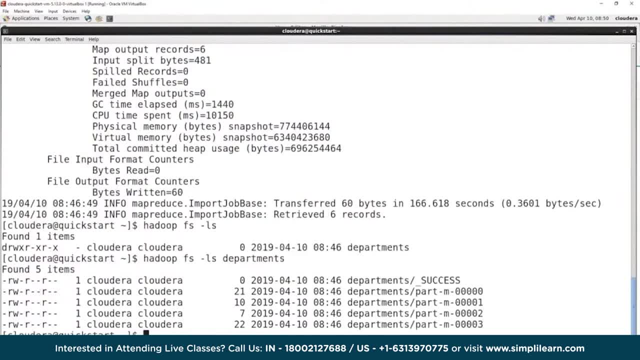 recognize this. on here I'm going to list the contents of departments And you'll see underneath departments we have part M000, 001, 002, 003.. So this is interesting because this is how Hadoop saves these files. This is in the file system. This is not in Hive, So we didn't directly import. 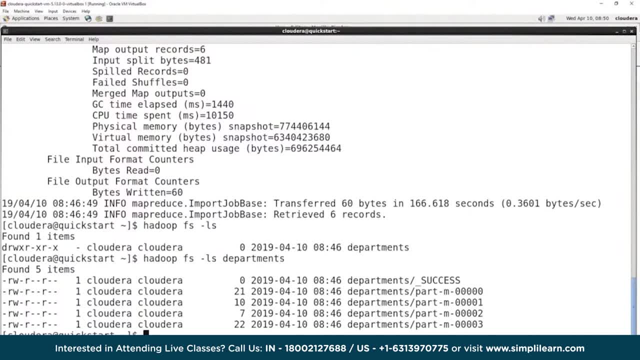 this into Hive. We put this in the Hadoop file system. Depending on what you're doing, you would have to look at the Hadoop file system. Certainly visit our Hive tutorial for more information on Hive specific So you can see in here are different files that it forms that are part of departments. 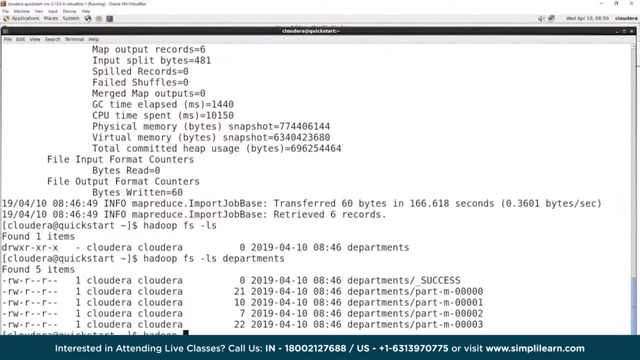 And we can do something like this: We can look at the contents of one of these files- FS minus LS, or a number of the files- And we'll simply do the full path, which is user Cloudera, And then we 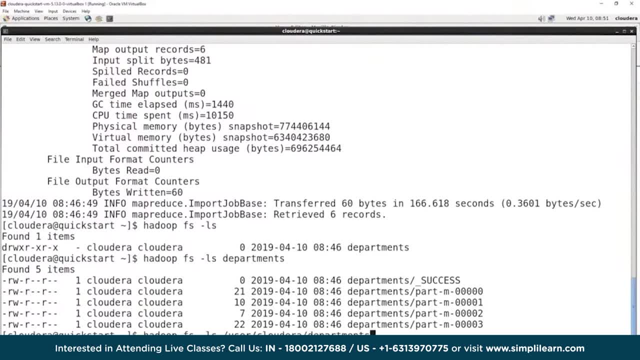 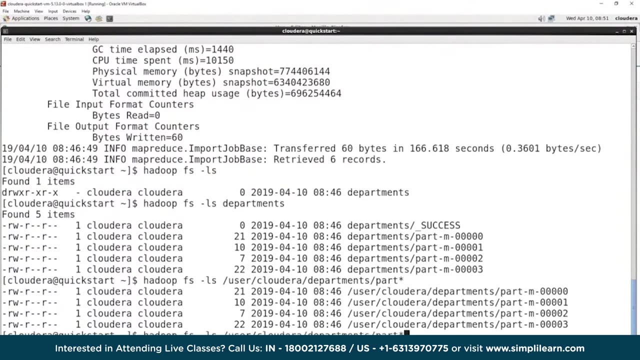 already know. the next one is departments. And then after departments we're going to put slash, part star And we're going to see anything that has part in it. So we have part dash, M000 and so on. We can go ahead and cat use that cat command or that list command to bring those up, And then we can use the. 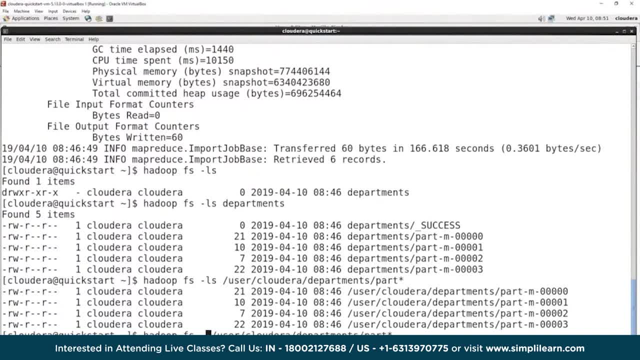 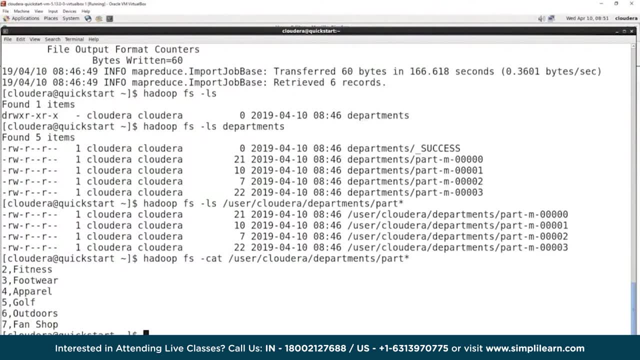 cat command to actually display the contents. And that's a Linux command, Hadoop Linux command to cat catinate, Not to be confused with catatonic catastrophic. There's a lot of cat got your tongue And we see here fitness footwear apparel That should look really familiar, because that's what 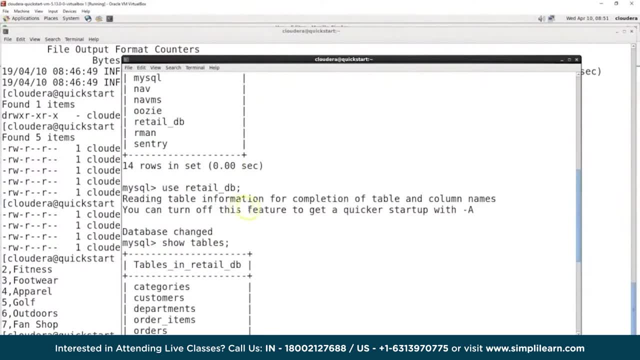 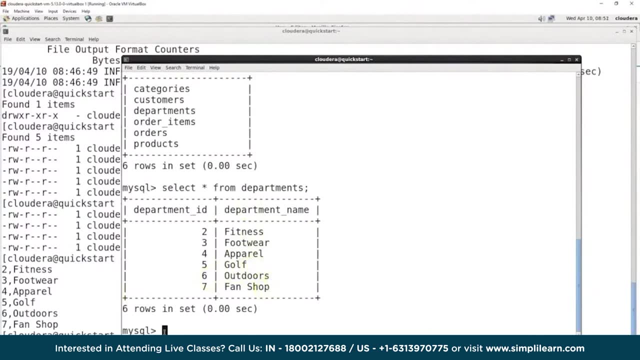 we had in our MySQL server. When we went in here, we did a lot of things like that, So we're going to get a select all on here. There it is Fitness, footwear, apparel, golf, outdoors and fan shop, And then of 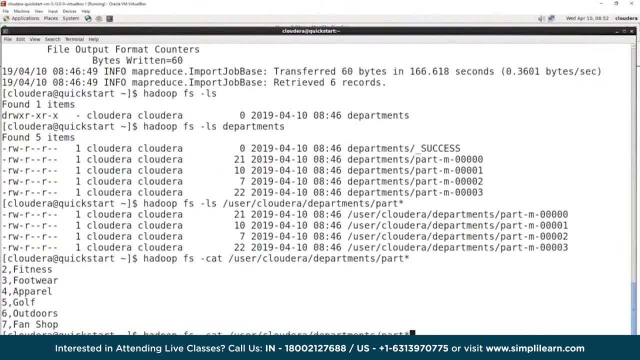 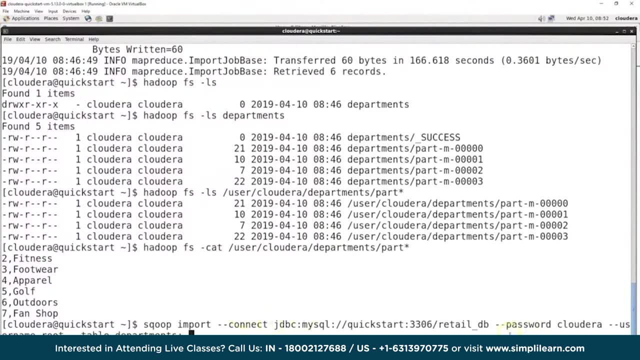 course it's really important- slip back on over here to be able to tell it where to put the data. So we go back to our import command. So here's our scoop: import, We have our connect, We have the DB underneath. 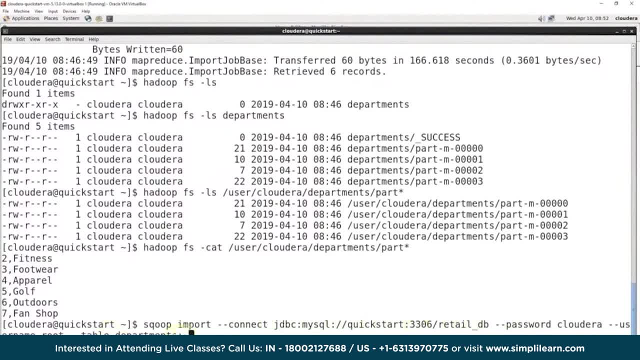 our connection, our MySQL server. We have our password, our username, the table going where it's going to, I mean the table where it's coming from, And then we can add a target on here. We can put in a target dash directory And you do have to put the full path. That's a Hadoop thing, It's a good. 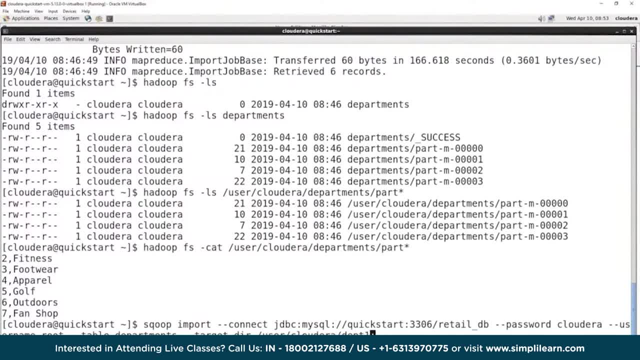 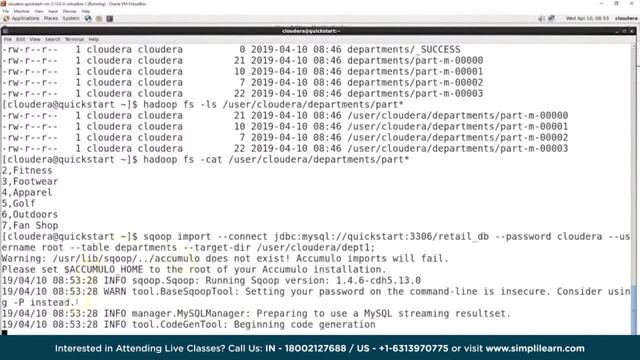 practice to be in And we're going to add it to department. We'll just do department one, And so here we now add a target directory in here and user cloud era department one, And this will take just a moment before, So I'll go ahead and skip over the process, since it's going to run very 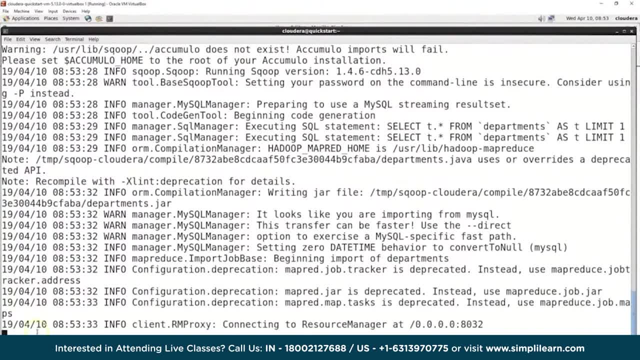 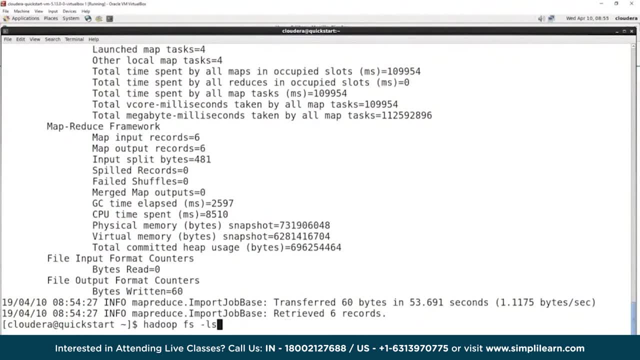 slowly. It's only running on, like I said, a couple cores And it's also on a single node. And now we can do the Hadoop. Let's just do the up arrow File system list. We want just straight list. And when we do the Hadoop file system minus LS or list, you'll see that we now have department. 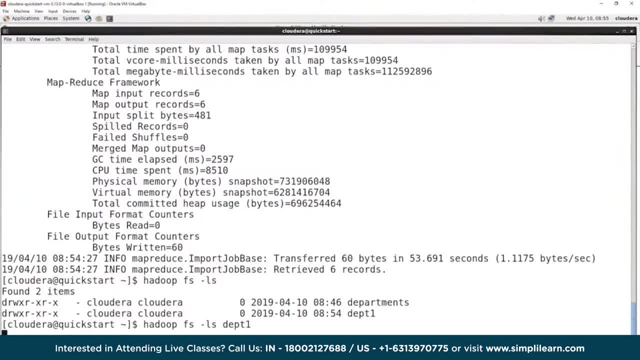 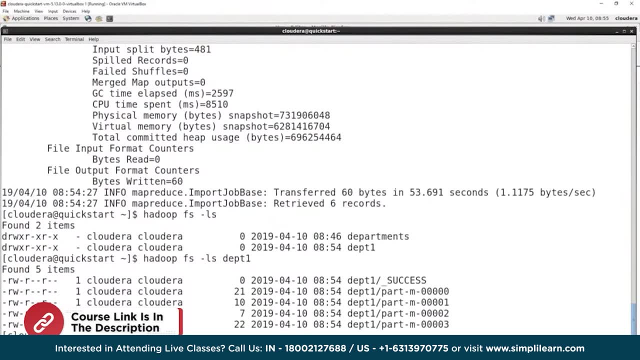 one, And we can of course do list department one And you can see we have the files inside department one And they mirrored what we saw before with the same files in there in the part MMO00 and so on. If we want to look at them, it would be the same thing we did before with the cat, Except instead of 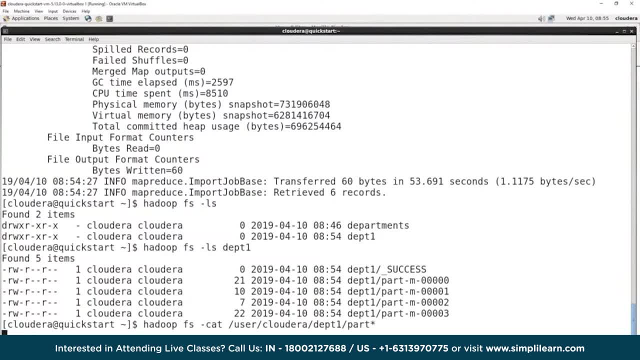 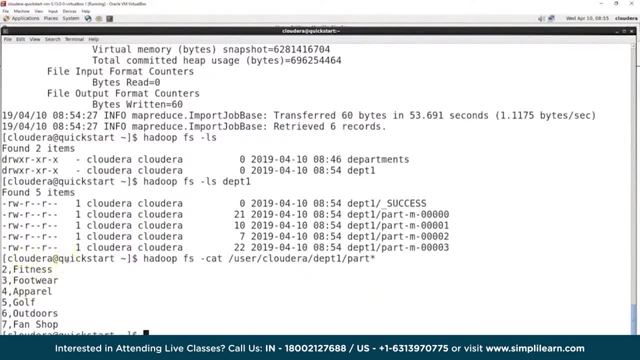 departments, we'd be department one. There we go, Something that's going to come up with the same data we had before. So these are the important things when you're importing data. And it's always a question to ask is: do you filter the data before it comes in? Do we want to filter this data as it comes in? so we're not storing. 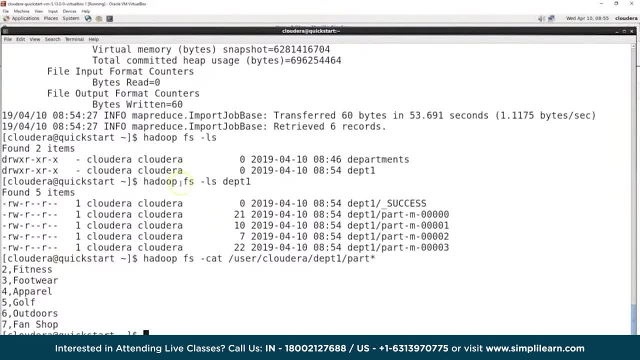 everything in our file system. You would think Hadoop big data, put it all in there. I know from experience that putting it all in there can turn a couple hundred terabytes into a petabyte very rapidly And suddenly you're having to really add on to that data store And you're storing duplicate data sometimes. 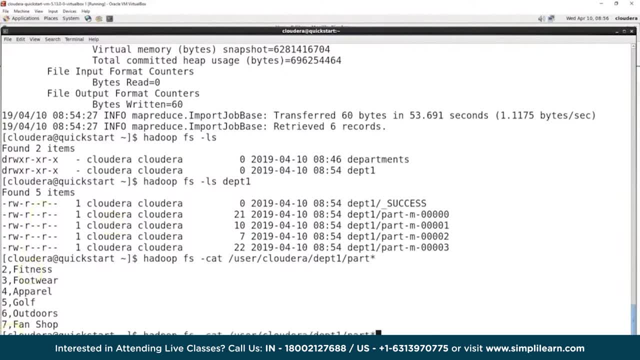 So you're going to have to really add on to that data store, And you're storing duplicate data sometimes, So you're really need to be able to filter your data out, And so let's go ahead and use our up arrow to go to our last import. 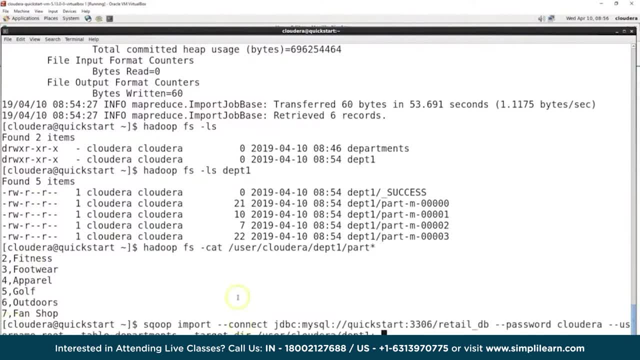 Since it's still a lot the same stuff. So we have all of our commands under import. We have the target. We're going to change this to department two, So we're going to create a new directory for this one. And then, after departments, there's another command that we didn't really slide in here. 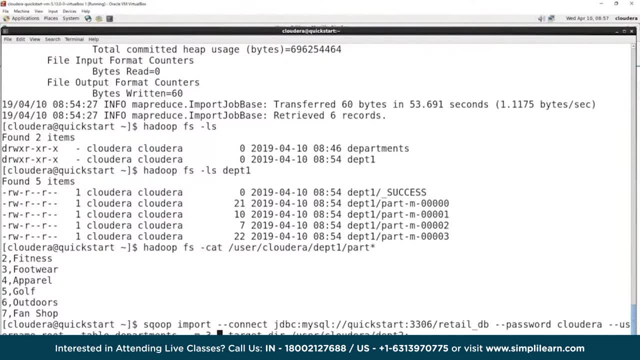 And that's our mapping, And I'll show you what this looks like in a minute. So we're going to put M3 in there. That doesn't have nothing to do with the filtering. I'll show you that in a second, though what that's for. 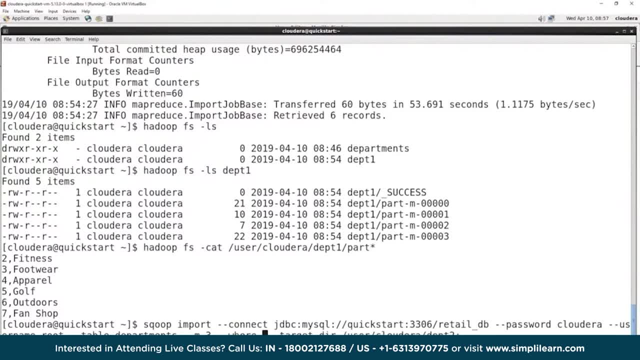 And we just want to put in where. So where and what is the where? In this case? we want to know where department ID And if you want to know where that came from, we can flip back on over here. We have department underscore ID. 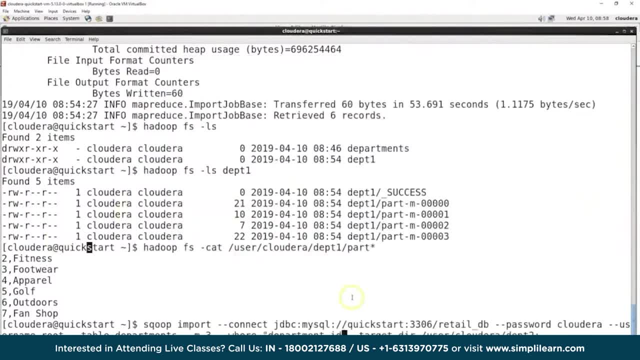 So this is where that's coming from. That's just the name of the column on here, And so we come in here to department. ID is greater than four, Simple logic. there You can see where you'd use that for maybe creating buckets for ages. You know, age from 10 to 15.. 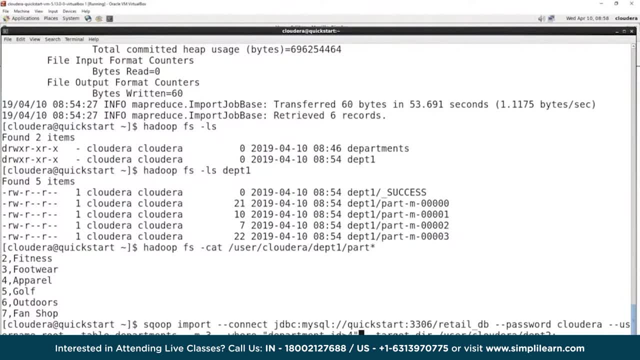 20 to 30. You might be looking for. I mean, there's all kinds of reasons why you could use the where command on here And filter information out. Maybe you're doing word counting and you want to know words that are used less than 100 times. 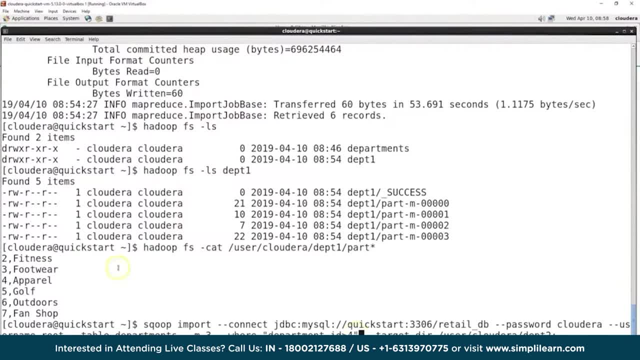 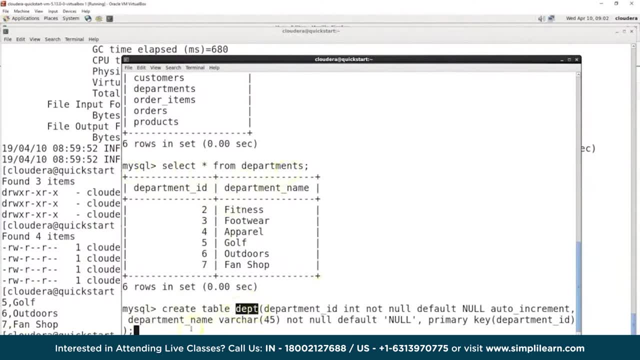 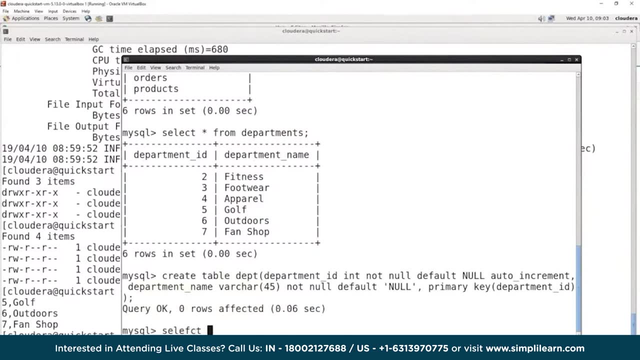 this case we're going to create a table called DEPT. so it's the same setup, but it's just gonna. we're just giving a different name, a different schema, and so we've done that and we'll go ahead and do a select star from DEPT. there we go. 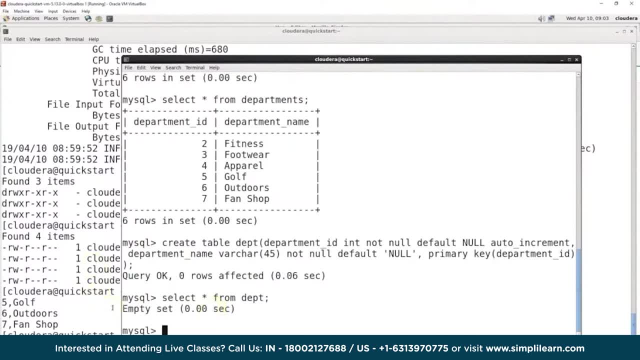 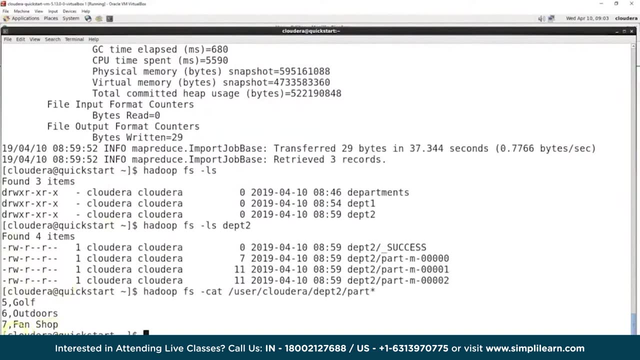 and it's empty. that's what we expect: a new database, a new data table- and it's empty in there. so now we need to go ahead and export our data that we just filtered out into there. so let's flip back on over here to our scoop setup. 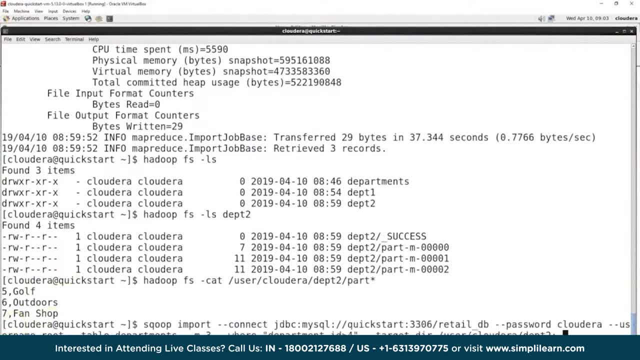 which is just our Linux terminal window. and let's go back up to one of our commands. here's scoop, import. in this case, instead of import, we're going to take the scoop and we're going to export. so we're going to just change that export and the connection is going to remain the same. so same connect, same. 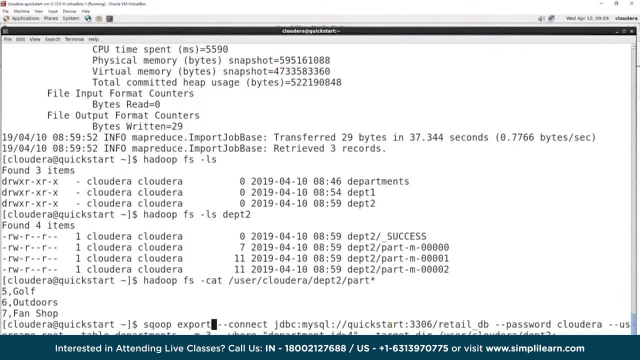 database. we're also. we're still doing the retail DB. we have the same password, so none of that changes. the big change here is going to be the table instead of departments. remember, we changed it and gave it a new name and we're going to go ahead and do that and we're going to go ahead and. 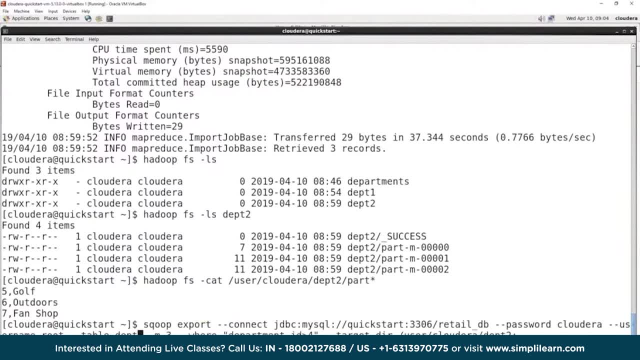 so we want to change it here. also DEPT so department. we're not going to worry about the mapper count and the where was part of our import. there we go and then finally it needs to know where to export from. so instead of target directory we have an export directory. that's where it's coming from. still, user Cloudera and 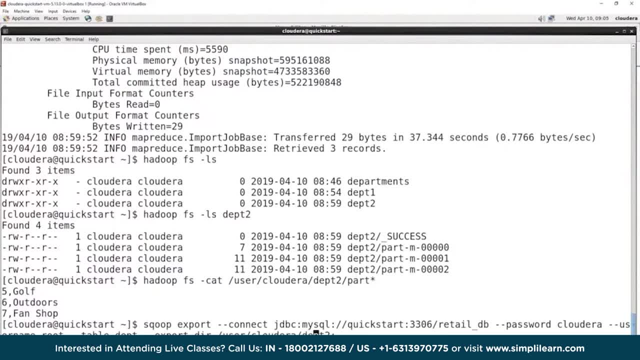 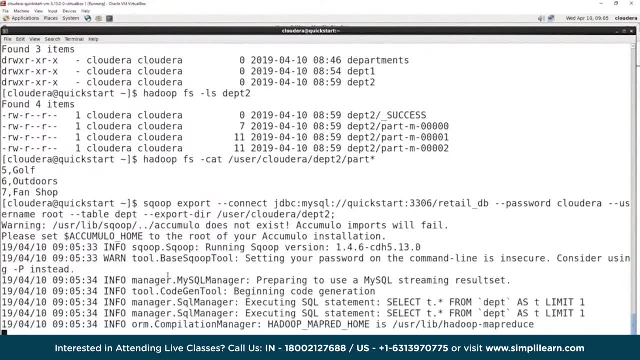 we'll keep it as department to, just so you can see how that data is coming back with the we filtered in and let's go ahead and run this. it'll take it just a moment to go through its steps and again, because it's slow, I'm just going to go ahead and skip this so you don't have to sit through it. 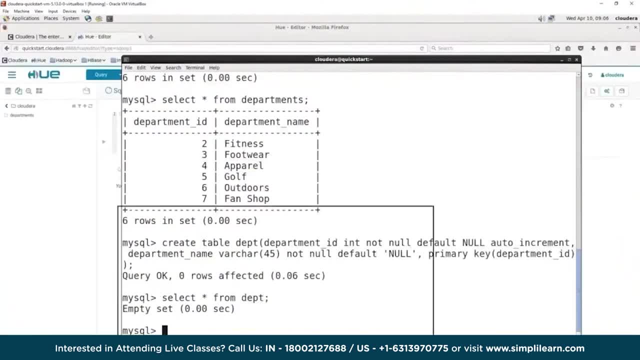 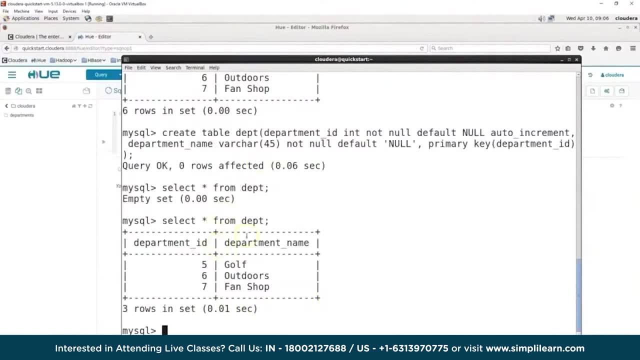 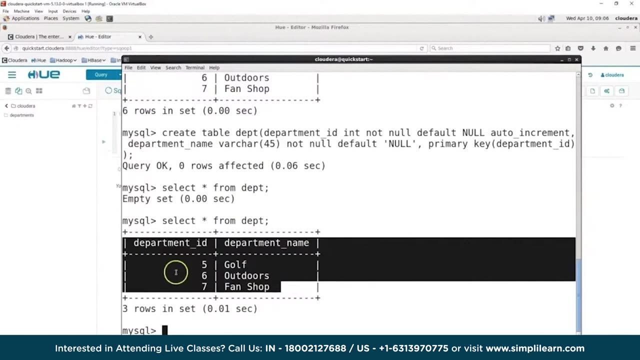 and once we've wrapped up our export, we'll flip back on over here to mysql, use the up arrow and this time we're going to select star from department and we can see that. there it is, it exported the golf outdoors and fan shop, and you can imagine also that you might have to use the where command in your export. 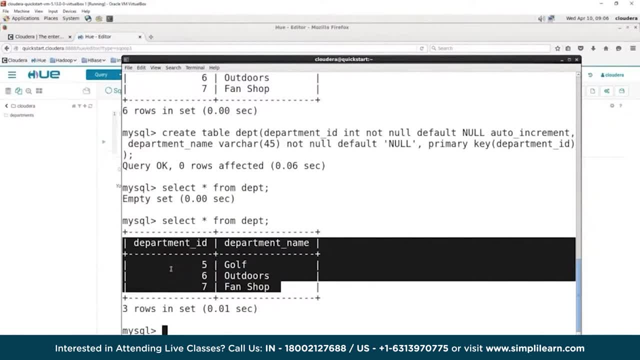 also. so there's a lot of mixing. the command line for scoop is pretty straightforward. you're going to want to make sure that you're going to use the up arrow, and this time we're going to use the up arrow, and this time we're going to. 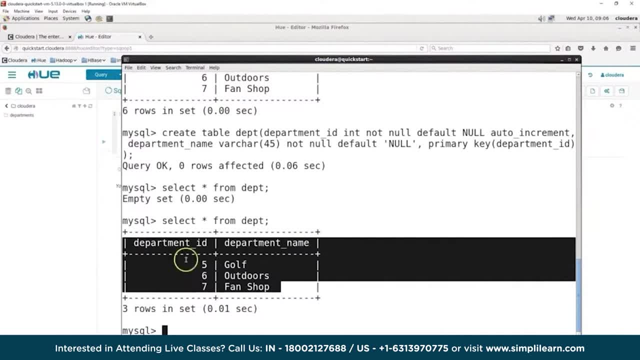 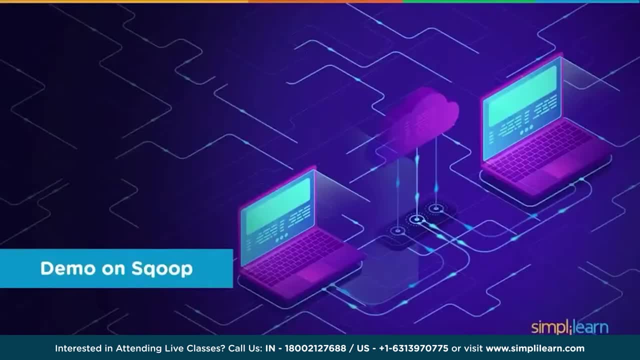 use the up arrow, and this time we're going to use the up arrow, and this time you're changing the different variables in there, whether you're creating a table listing a table listing databases- very powerful tool for bringing your data into the Hadoop file system and exporting it. so, now that we've wrapped up our demo on 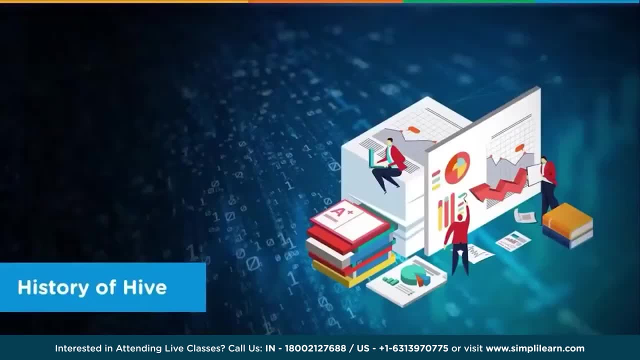 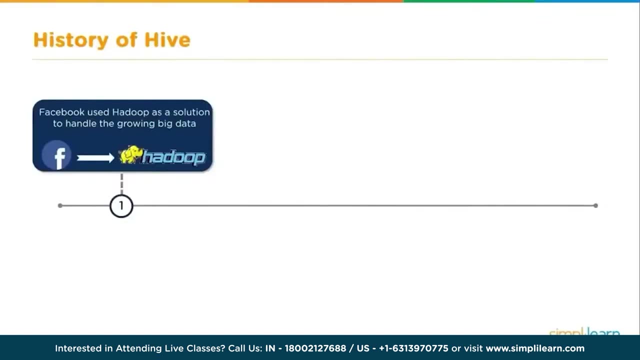 scoop and gone through a lot of basic commands. let's dive in with a brief history of hive. so the history of hive begins with Facebook. Facebook begin using Hadoop as a solution to handle the growing big data, and we're not talking about a data that fits on one or two or even five computers. 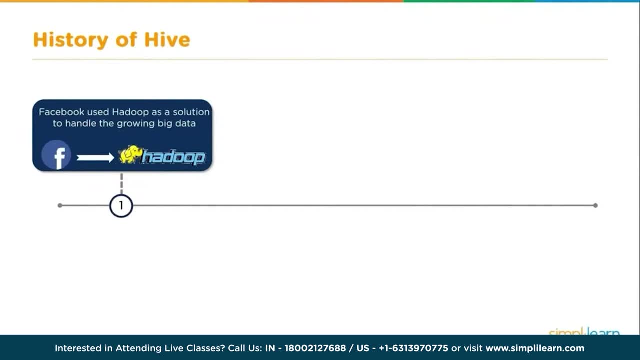 we're talking due to the fifth son. if you've looked at any of our other Hadoop tutorials, you'll know we're talking about very big data and data pools, and Facebook certainly has a lot of data it tracks. as we know, the Hadoop uses map. 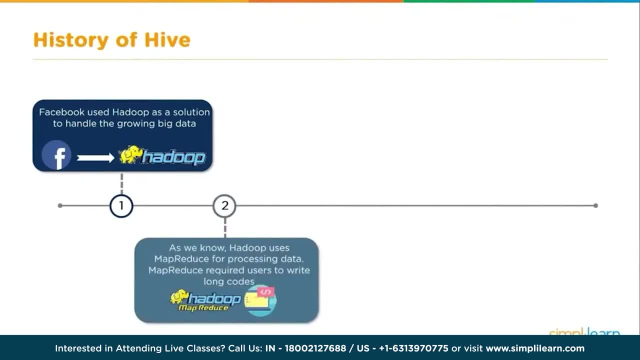 reduce for processing data map. reduce required users to write long codes. and so you have these really extensive Java codes, very complicated for the average person to use. not all users reversed in Java and other coding languages. this proved to be a disadvantage for them. users were comfortable with writing. 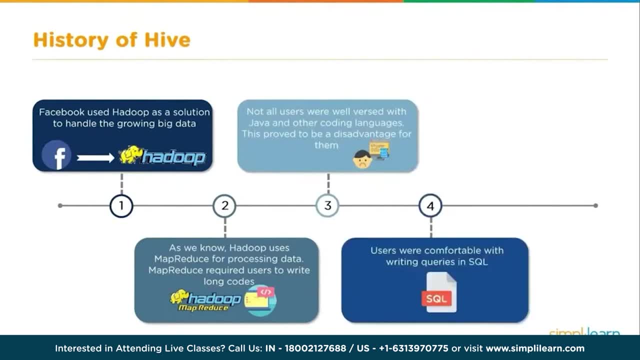 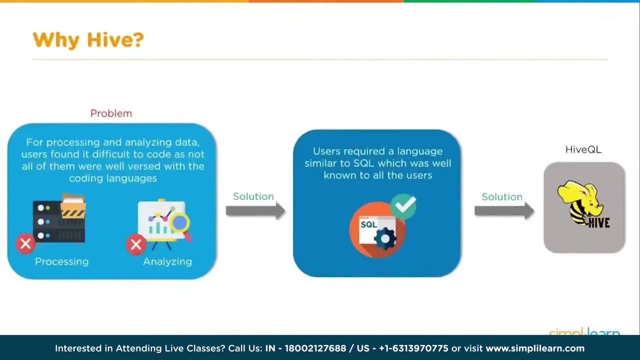 queries in SQL. SQL has been around for a long time. the standard sequel query language, hive, was developed with the vision to incorporate the concepts of tables, columns, just like SQL. so why hive? well, the problem was for processing and analyzing data. users found it difficult to code, is not all of them were well? 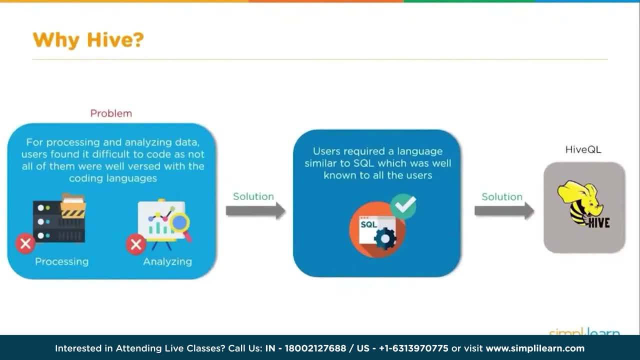 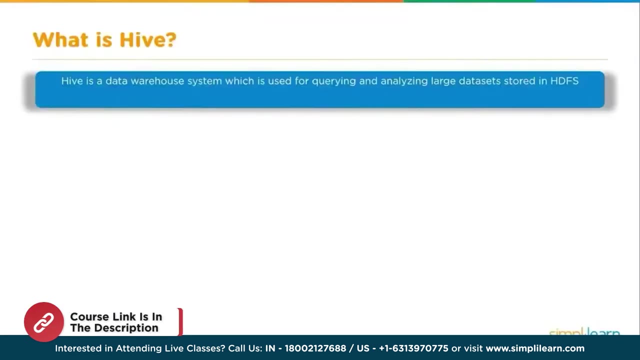 versed with the coding languages if you're processing, ever analyzing. so the solution was required- a language similar to SQL, which was well known to all the users, and thus the hive, or HQL, language evolved. what is hive? hive is a data warehouse system which is used for querying and analyzing large data set. 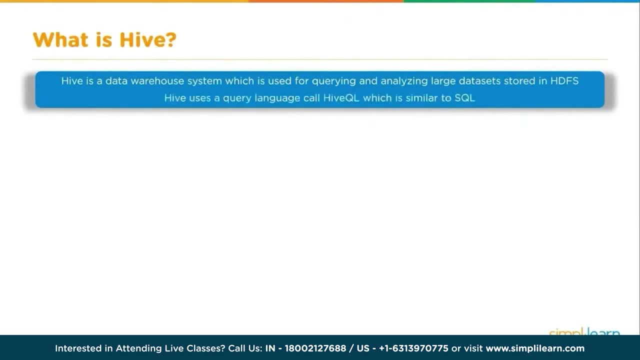 stored in the HDFS or the Hadoop file system. hive uses a query language that we call hive, QL or HQL, which is similar to SQL. so if we take our user, the user sends out their hive queries and then that is converted into a map reduce. 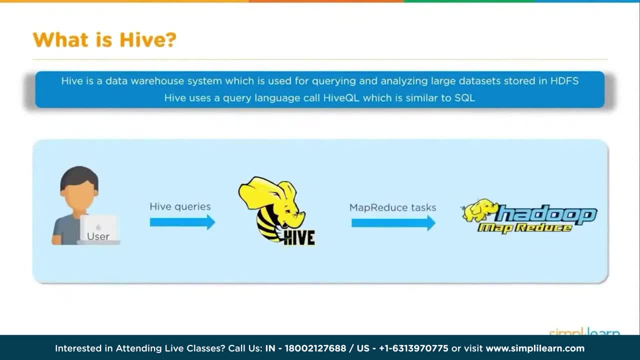 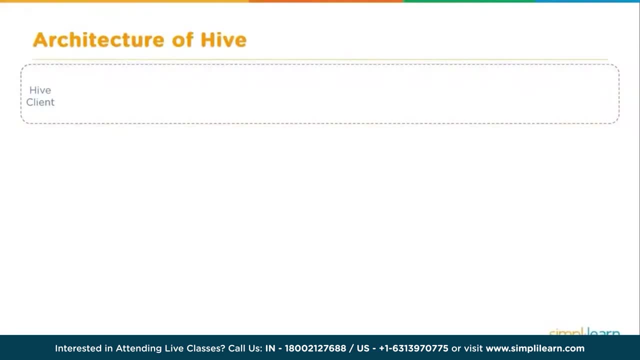 tasks and then accesses the Hadoop map reduce system. let's take a look at the architecture of hive. architecture of hive: we have the hive client, so that could be the programmer, or maybe it's a manager who knows enough SQL to do a basic query to look up the data they need. the hive. 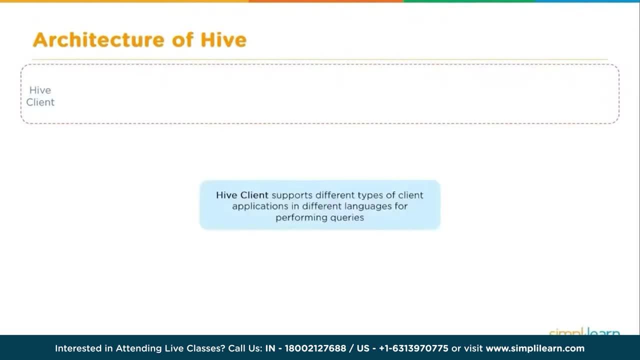 client supports different types of client applications in different languages prefer for performing queries, and so we have our thrift application in the hive thrift client. thrift is a software framework. hive server is based on thrift so it can serve the request from all programming language that support thrift. and then we have our JDBC application and the hive JDBC driver. 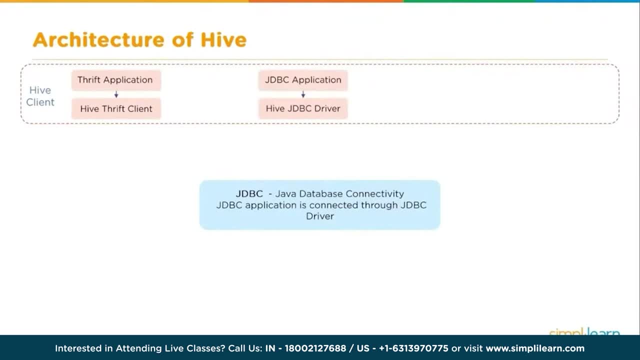 JDBC Java database connectivity. JDBC application is connected through the JDBC driver and then you have the ODBC application or the hive ODBC driver, the ODBC or open database connectivity. the odc application is connected through the ODBC driver. with the growing development of all of our different scripting, 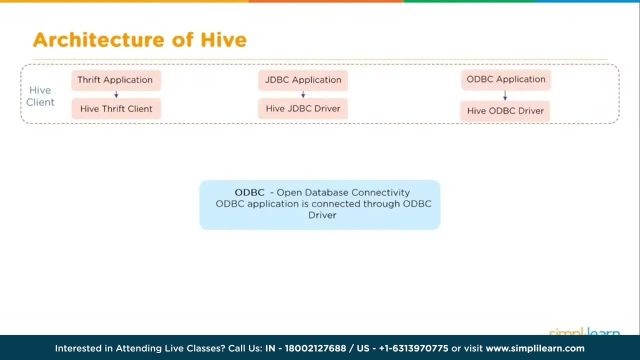 languages: C++, Spark, Java. You can find just about any connection in any of the main scripting languages, And so we have our Hive services. As we look at deeper into the architecture, Hive supports various services, So you have your Hive server. 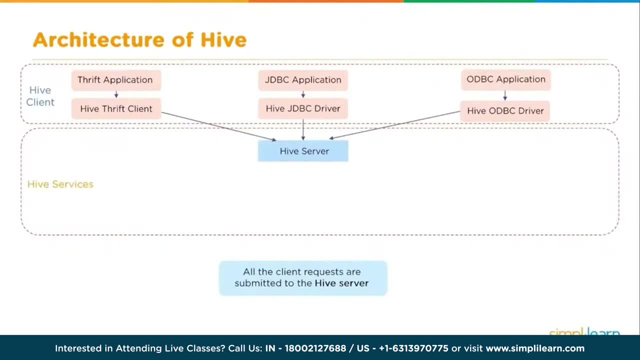 basically your Thrift application or your Hive Thrift client or your JDBC or your Hive JDBC driver, your ODBC application or your Hive ODBC driver. They all connect into the Hive server And you have your Hive web interface. You also have your CLI. Now the Hive web interface is a GUI is provided to. 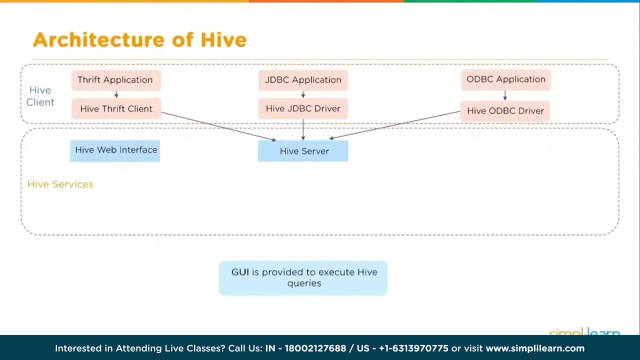 execute Hive queries And we'll actually be using that later on today So you can see kind of what that looks like and get a feel for what that means. Commands are executed directly in CLI And then the CLI is a direct terminal window And I'll 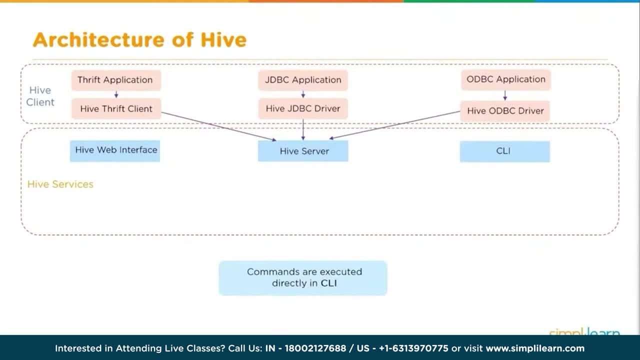 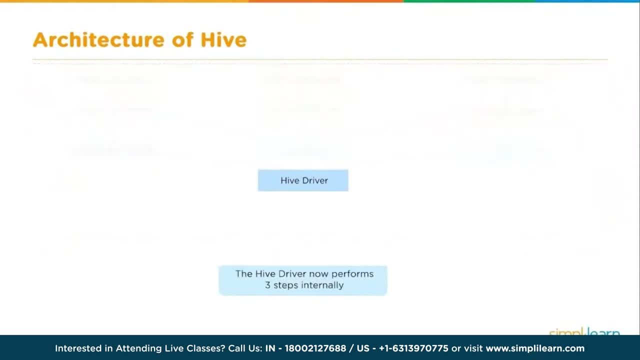 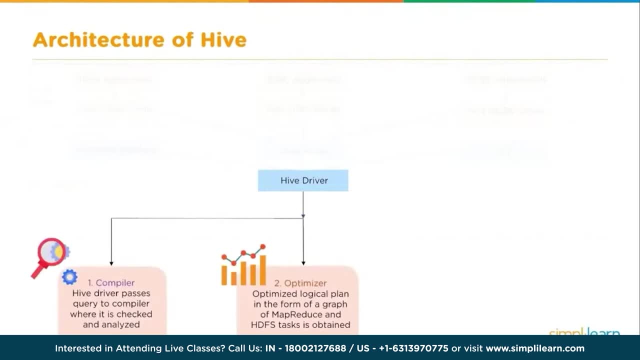 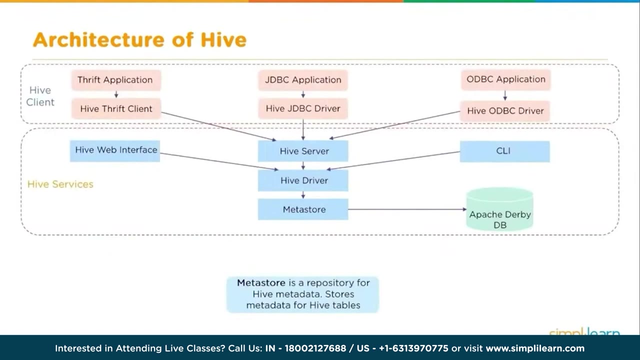 analyzed, Then the optimizer kicks in And the optimized logical plan in the form of a graph of MapReduce and HDFS tasks is obtained, And then finally, in the executor, in the final step, the tasks are executed. When we look at the architecture, we also have to note the Metastore. Metastore is a repository. 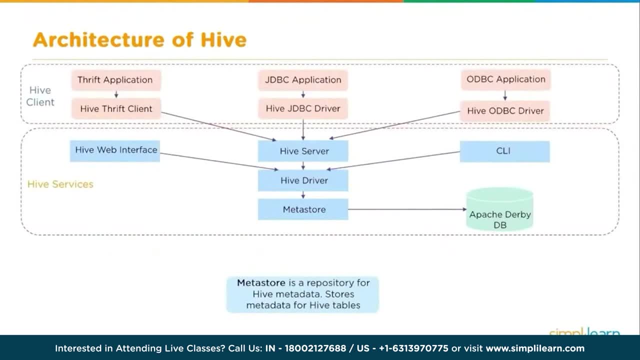 for Hive metadata Stores metadata for Hive tables And you can think of this as your schema. and where is it located? And it's stored on the Apache Derby DB. Processing and resource management is all handled by the MapReduce v1.. You'll 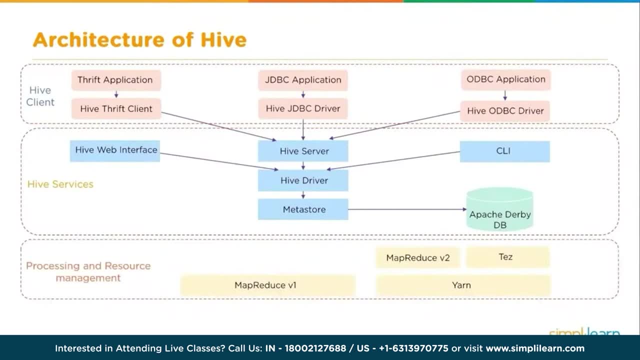 see MapReduce v2, the Yarn and the Tez. These are all different ways of managing these resources, depending on what version of Hadoop you're in. Hive uses MapReduce framework to process queries, And then we have our distributed storage, which is the HDFS, And if you looked at our Hadoop, 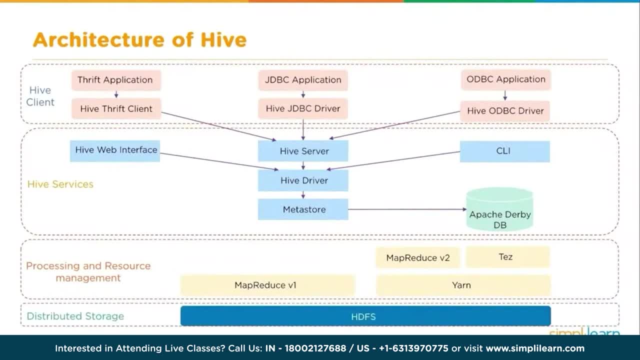 tutorials. you'll know that these are on commodity machines and are linearly scalable. That means they're very affordable. A lot of time, when you're talking about big data, you're talking about a tenth of the price of storing it on enterprise computers. And then we look at the data flow in Hive, So in our data, 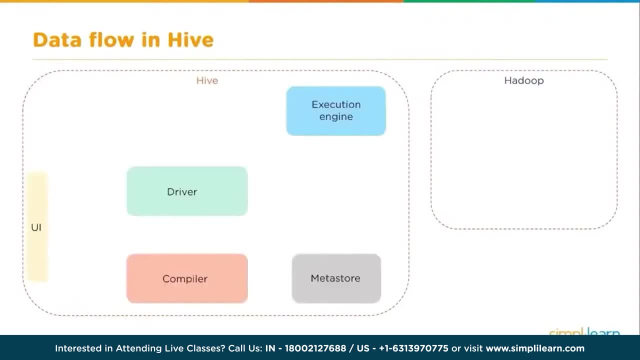 flow in Hive. we have our Hive and the Hadoop system And underneath the user interface or the UI, we have our driver, our compiler, our execution engine and our Metastore. That all goes into the MapReduce and the Hadoop file system. 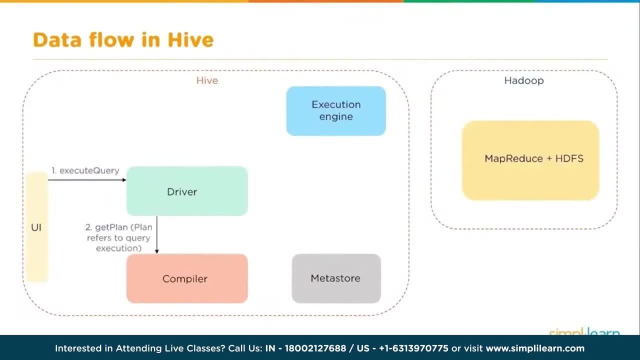 So when we execute a query, you see it coming in here. it goes into the driver. step one, Step two. we get a plan. What are we going to do? refers to the query execution. Then we go to the metadata. It's like, well, what kind of metadata are? 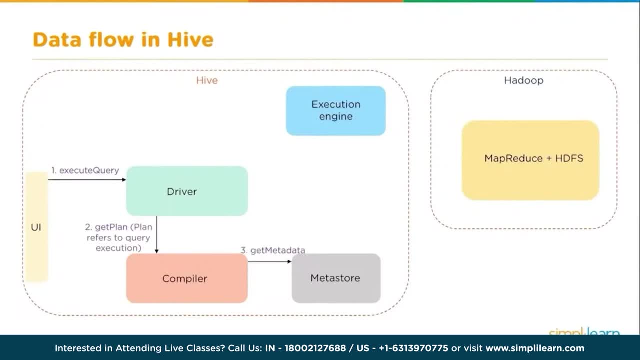 we actually looking at. Where is this data located? What is the schema on it? Then this comes back with the metadata into the compiler. Then the compiler takes all that information and the send plan returns it to the driver. The driver then sends the execute plan to the execution engine Once it's in the 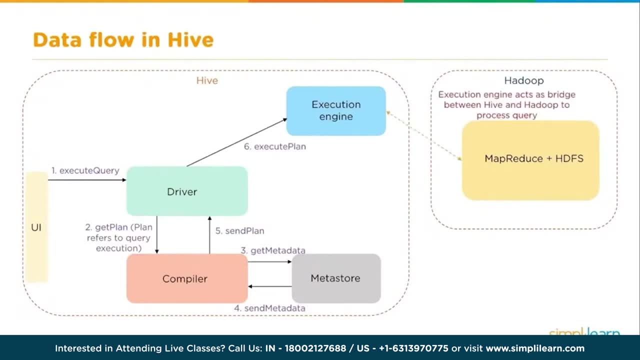 execution engine. the execution engine acts as a bridge between Hive and Hadoop to process the query And that's going into your MapReduce and your Hadoop file system or your HDFS And then we come back with the metadata operations. It goes back into the Metastore to update or let it know what's going on, Which. 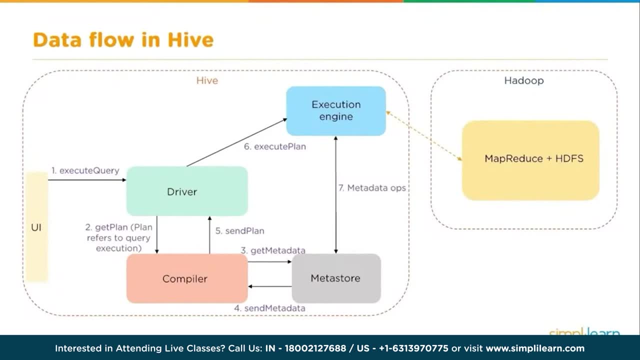 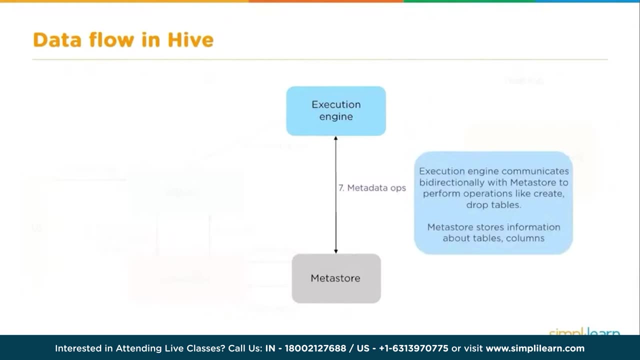 also goes to the between. it's a communication between the execution engine in the Metastore. Execution engine communications is bi-directionally with the Metastore to perform operations like create drop tables. Metastore stores information about tables and columns. So 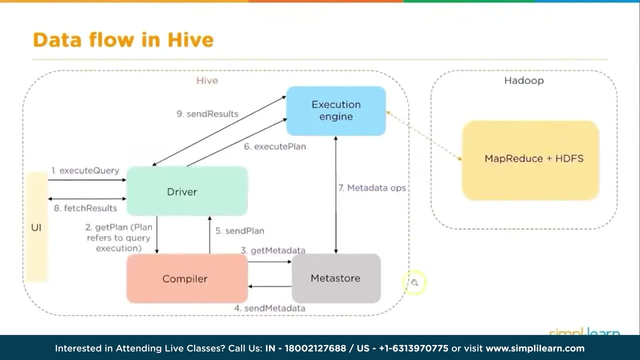 again, we're talking about the schema of your database And once we have that, we have a bi-directional send results communication back into the driver And then we have the fetch results which goes back to the client. So let's take a little bit. look at the Hive data modeling. Hive data modeling. So you have. 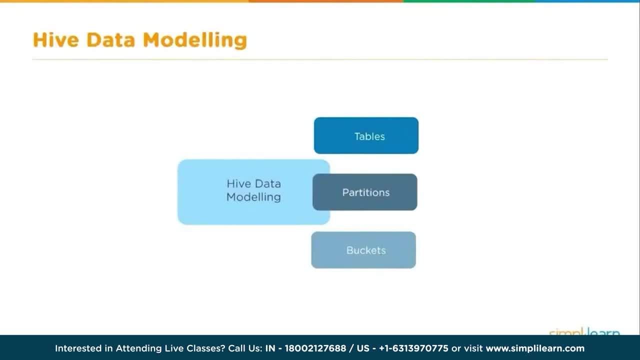 your Hive data modeling. You have your tables, you have your partitions and you have buckets. The tables in Hive are created the same way it is done in RDBMS. So when you're looking at your traditional SQL server or MySQL server, where you might have enterprise equipment and a lot of people pulling and 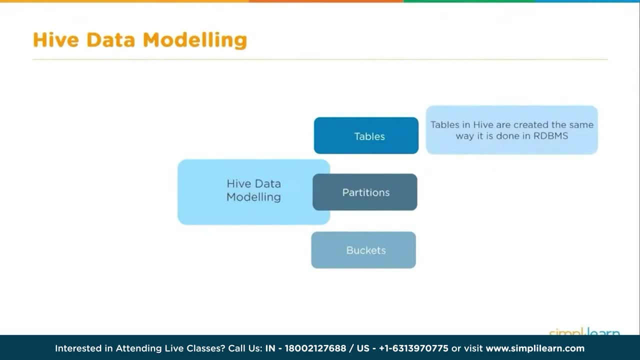 moving stuff off of there. The tables are gonna look very similar And this makes it very easy to take that information. and let's say you need to keep current information but you need to store all of your years of transactions back into the Hadoop Hive So you match those. Those all kind of look the same. The tables are the. 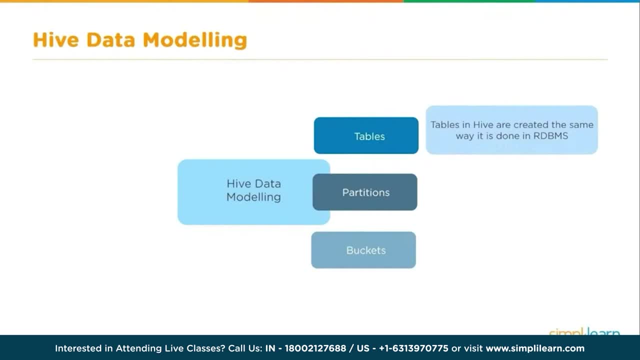 same. Your databases look very similar and you can easily import them back. You can easily store them into the Hive system Partitions: Here tables are organized into partitions for grouping same type of data based on partition key. This can become very important for speeding up. 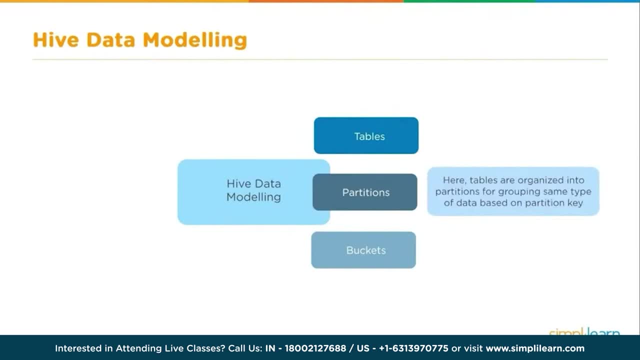 the process of doing queries. So, if you're looking at dates as far as, like, your employment dates of employees, if that's what you're tracking, you might add a partition there, because that might be one of the key things that you're always looking up as far as employees are concerned. And finally, we have 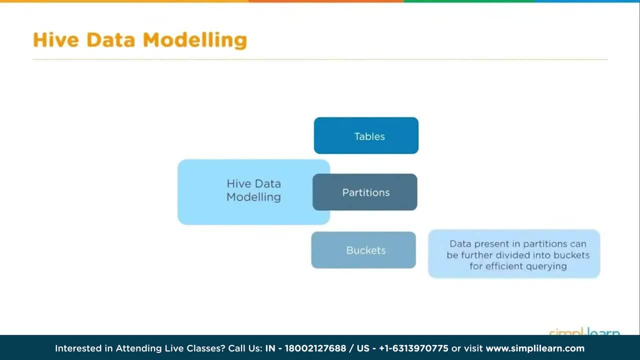 buckets, Data present in partitions. You can easily import and store data into the Hive system. Partitions can be further divided into buckets for efficient querying. Again, there's that efficiency At this level. a lot of times you're taught you're working with 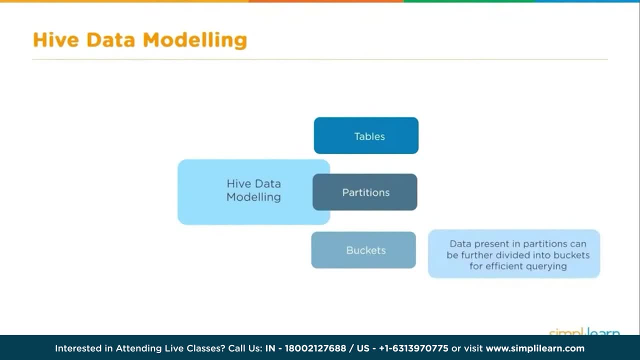 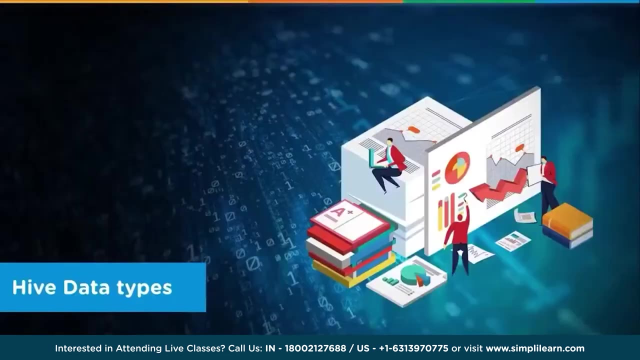 the programmer and the admin of your Hadoop file system to maximize the efficiency of that file system. So it's usually a two-person job. and we're talking about Hive data modeling. You want to make sure that they work together and you're maximizing your resources- Hive data types- So we're 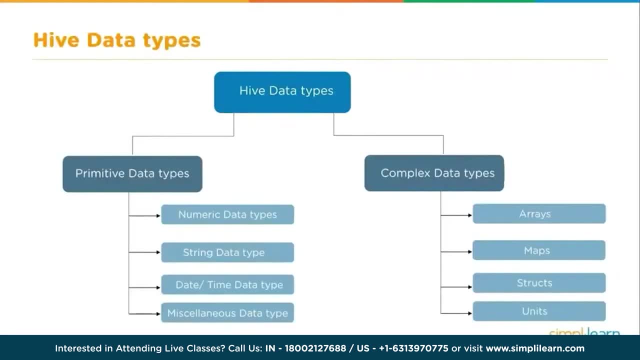 talking about Hive data types. We have our primitive data types and our complex data types. A lot of this will look familiar. It mirrors a lot of stuff in SQL. In our primitive data types we have the numerical data types, string data type, date, time data type and miscellaneous data type, And 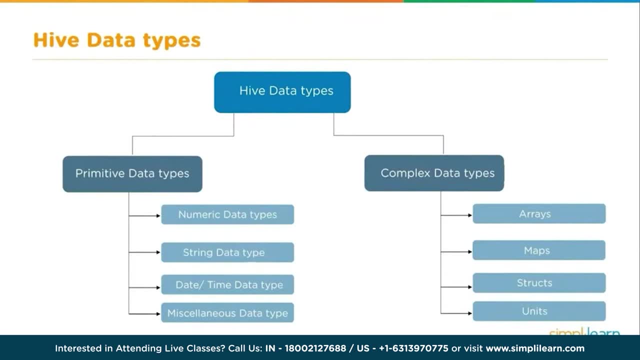 these should be very. they're kind of self-explanatory, but just in case, Numerical data is your floats, your integers, your short integers. all of that numerical data comes in as a number. A string, of course, is characters and numbers, and then you have your date, time stamp and 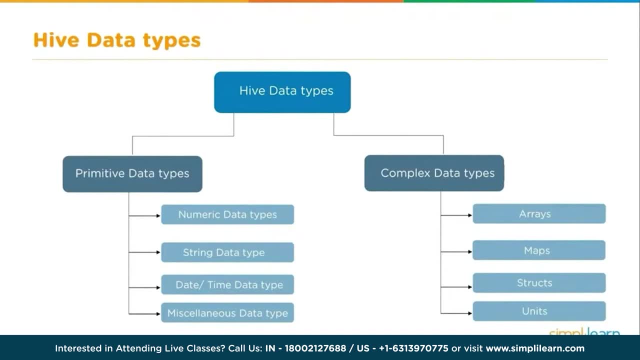 we have kind of a general way of pulling your own created data types in there. that's our miscellaneous data type and we have complex data types so you can store arrays, you can store maps, you can store structures and even units in there as we dig into hive data types and we have the primitive data. 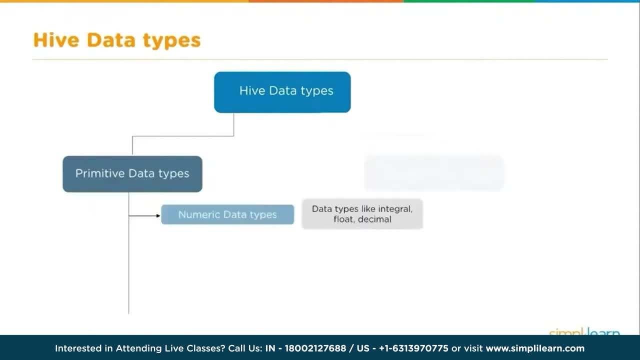 types and the complex data types. so we look at primitive data types and we're looking at numeric data types. data types like an integer, a float, a decimal- those are all stored as numbers in the hive data system. a string data type data types like characters and strings- you store the name. 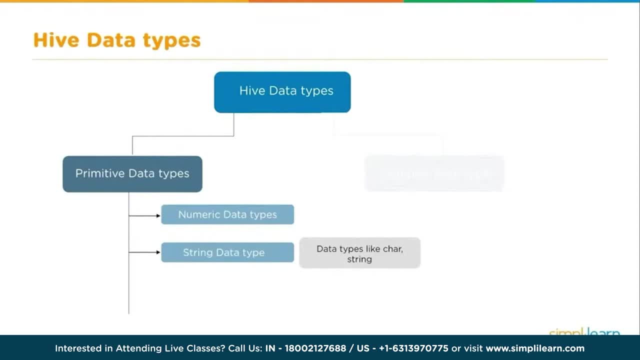 of the person you're working with. uh, you know, john doe, the city memphis, the state tennessee, maybe it's boulder, colorado, usa, or maybe it's hyperbad, india. that's all going to be string and stored as a string character and, of course, we have our date time. data type. data types like: 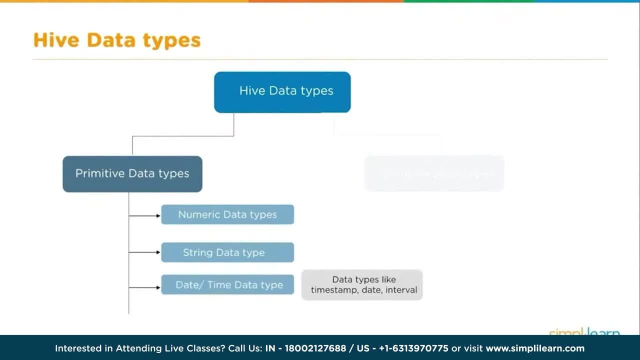 timestamp, date interval. those are very common as far as tracking sales, anything like that, you can just think if you can type a stamp of time on it. or maybe you're dealing with the race and you want to know the interval. how long did the person take to complete whatever task? it was all. 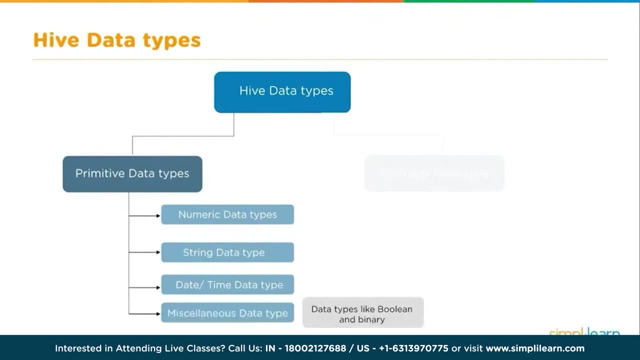 that is, date time data type. and then we talk miscellaneous data type. these are like boolean and binary, and when you get into boolean and binary you can actually almost create anything in there, but your yes knows zero one. now let's take a look at complex data types a little closer. 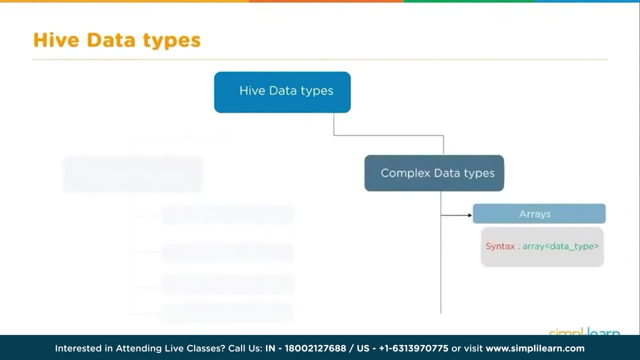 we have arrays, so your syntax is of data type and it's an array and you can just think of an array as a collection of same entities: one, two, three, four, if they're all numbers- and you have maps, this is a collection of key value pairs. so understanding maps is so central to hadoop. 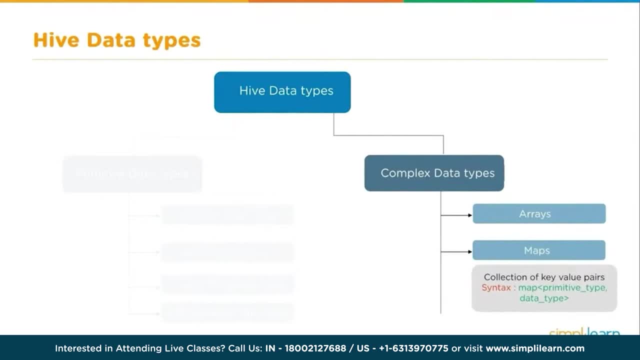 so when we store maps, you have a key which is a set. you can only have one key per mapped value, and so you in hadoop, of course, you collect the same keys and you can add them all up or do something with all the contents of the same key, but this is our map as a primitive type. data type. 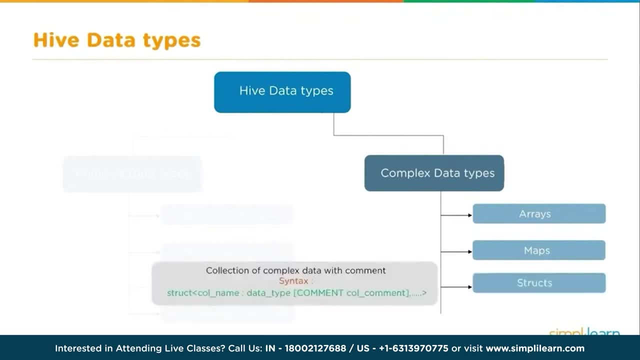 and our collection of key value pairs, pairs and then collection of complex data with comment, so we can have a structure where you have a column name, data type, comment, call a column comment, so you can get very complicated structures in here with your collection of data and your comment and setup. and then we have units and this. 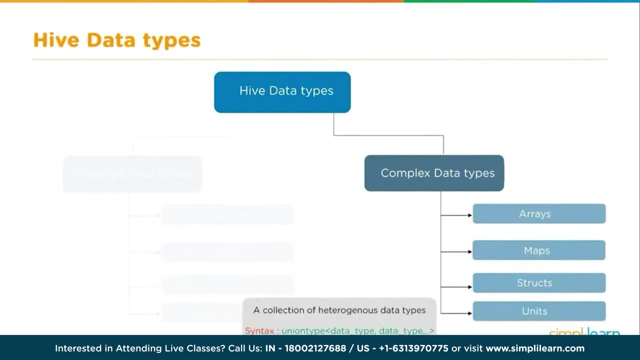 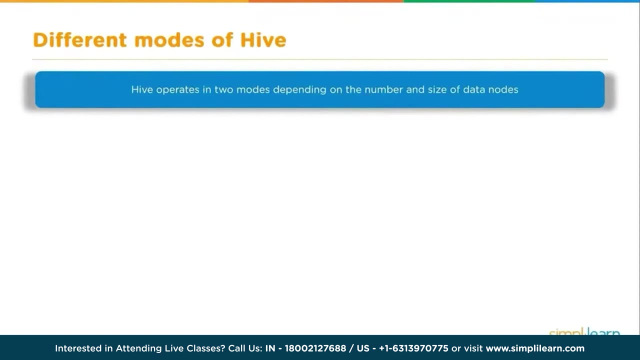 is a collection of heterogeneous data types, so the syntax for this is union type, data type, data type and so on. so it's all going to be the same, a little bit different than the arrays, where you can actually mix and match different modes of hive. hive operates in two modes, depending on the number and size of data nodes. 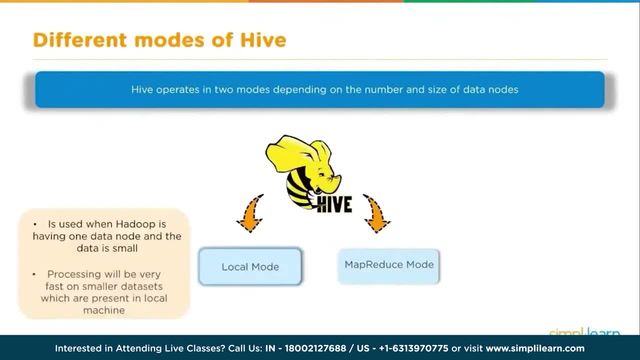 we have our local mode and our map reduce mode. when we talk about the local mode, it is used when hadoop is having one data node and the data is small. processing will be very fast on a smaller data sets which are present in local machine, and this might be that you have. 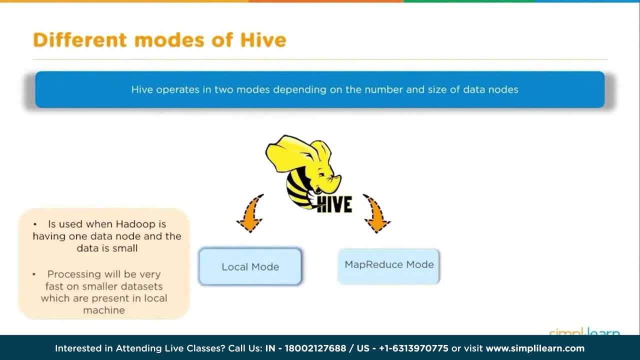 a local file of stuff you're uploading into the hive and you need to do some processes in there. you can go ahead and run those hive processes and queries on it. usually you don't see in the way of a single node hadoop system. if you're going to do that, you might as well just. 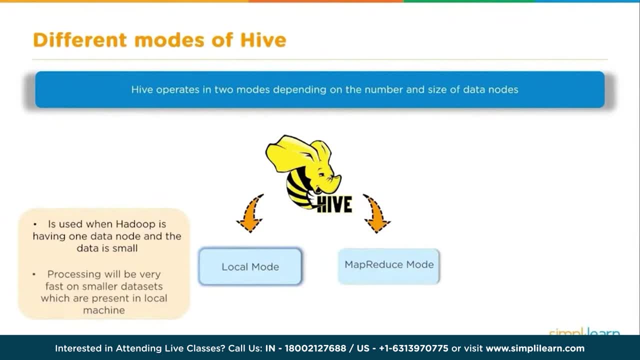 use like an sql database or even a java sqlite or something. python is sqlite, so you don't really see a lot of single node hadoop databases. but you do see the local mode in hive where you're working with a small amount of data that's going to be integrated into the larger database and then we 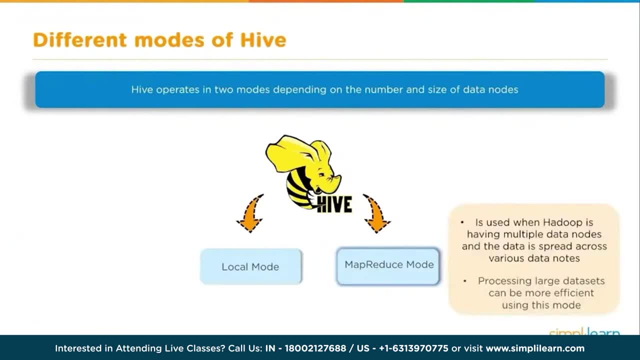 have the map reduce mode. this is used when hadoop is having multiple data nodes and the data is spread across various data nodes. processing large data sets can be more efficient using this mode, and this you can think of, instead of it being one, two, three or even five computers, we're usually 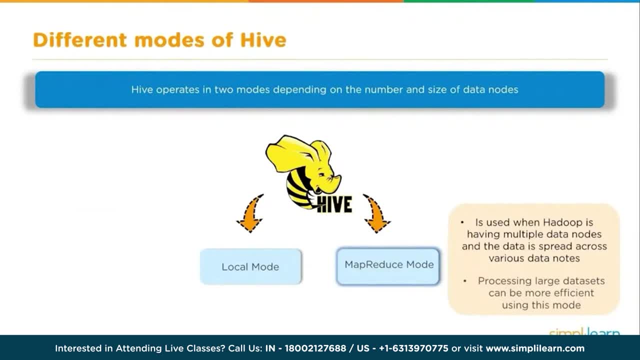 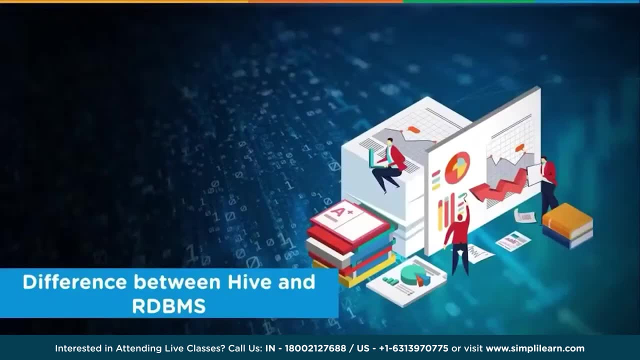 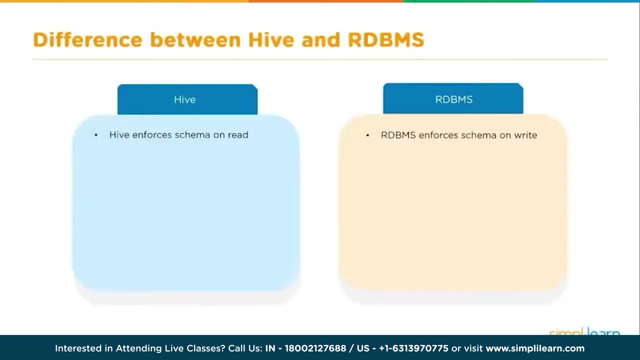 talking with the hadoop file system. we're looking at 10 computers, 15, 100, where this data is spread across, all those different hadoop nodes. difference between hive and rdbms: remember rdbms stands for the relational database management system. let's take a look at the difference between. 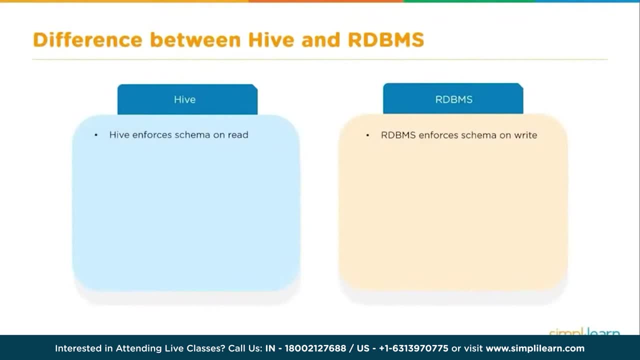 hive and rdbms. in the rdbms, with hive, hive enforces schema on read and it's very important that whatever's coming in, that's when hive's looking at it and making sure that it fits the model. the rdbms enforces a schema when it actually writes the data into the database, so it's read the data. 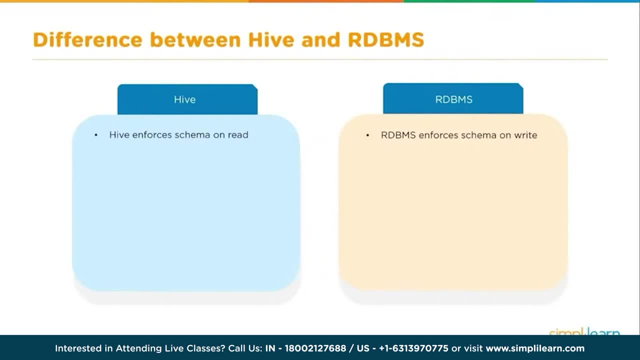 and then, once it starts to write it, that's where it's going to give you the error or tell you something's incorrect about your scheme. hive data size is in petabytes. that is hard to imagine. you know, when we're looking at your personal computer on your desk. 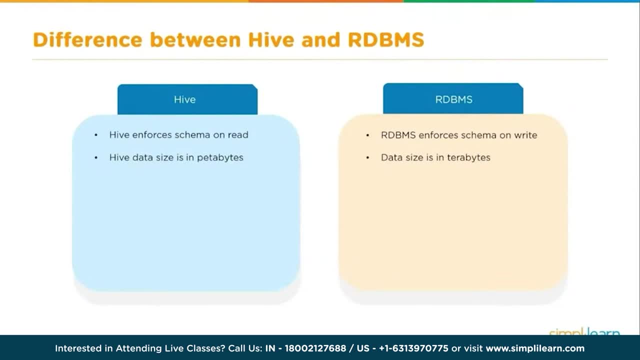 maybe you have 10 terabytes. if it's a high-end computer, we're talking petabytes, so that's hundreds of computers grouped together when rdbms data size is in terabytes. very rarely do you see an rdbms system that's spread over more than five computers and there's 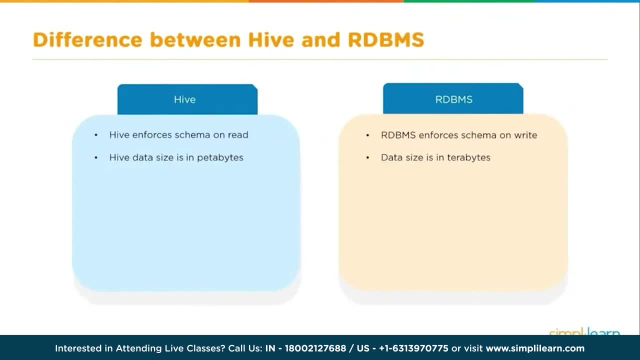 a lot of reasons for that. with the rdbms, it actually has a high-end amount of rights to the hard drive. there's a lot more going on there. you're writing and pulling stuff, so you really don't want to get too big with an rdb master. you're going to run into a lot of problems. 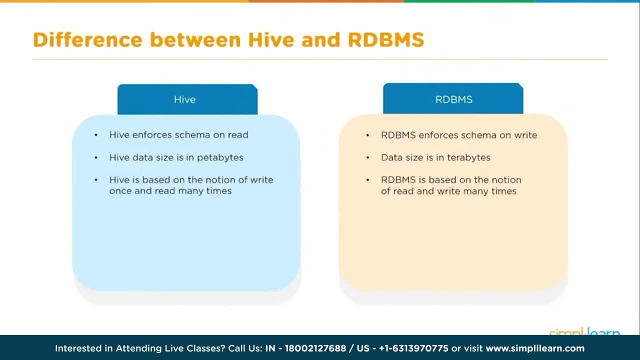 with hive. you can take it as big as you want. hive is based on the notion of write once and read many times. this is so important. they call it worm, which is right. w once o read r many times m they refer to it as worm, and that's true of any of you- a lot of your hadoop setup it's. it's altered a little. 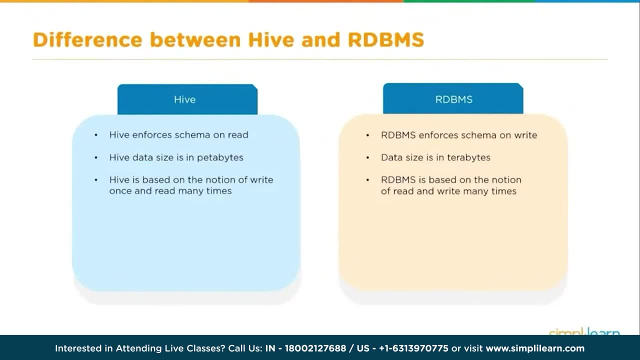 bit, but in general we're looking at archiving data that you want to do data analysis on. we're looking at pulling all that stuff off your rdbms from years and years and years of business or whatever your company does, or scientific research, and putting that into a huge data pool so that you can now do. 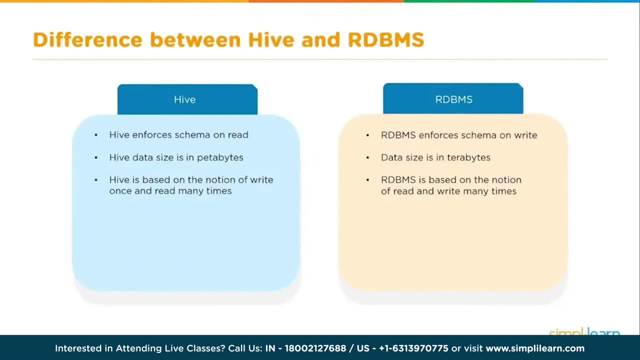 queries on it and get that information out of it with the rdbms. it's based on the notion of read and write many times. so you're continually updating this database. you're continually bringing up new stuff, new sales. the account changes because they have a different licensing. 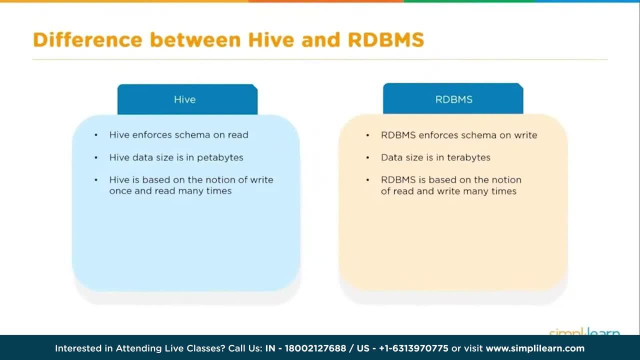 now, whatever software you're selling, all that kind of stuff where the data is continually fluctuating, and then hive resembles a traditional database by supporting sql, but it is not a database, it is a data warehouse. this is very important. it goes with all the other stuff we've talked about that we're not looking at a database, but a data warehouse to store the data. 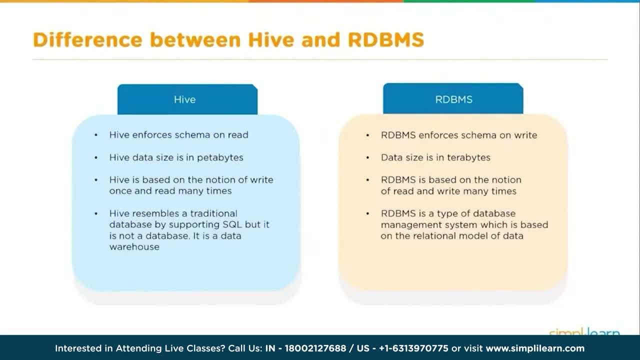 and still have fast and easy access to it for doing queries. you can think of twitter and facebook. they have so many posts that are archived back historically. those posts aren't going to change. they made the post, they're posted, they're there and they're in their database, but they have to. 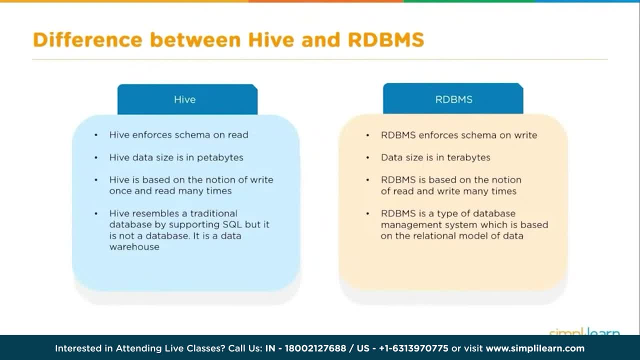 store it in a warehouse in case they want to pull it back up with the rdbms. it's a type of database management system which is based on the relational model of data and then, with hive, easily scalable at a low cost. again, we're talking maybe a thousand dollars. 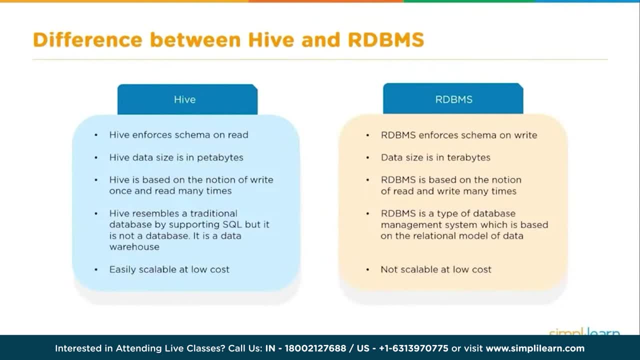 per terabyte. the rdbms is not scalable at a low cost. when you first start on the lower end, you're talking about 10 000 per terabyte of data, including all the backup on the models and all the added necessities to support it. as you scale it up, you have to scale those computers and hardware. 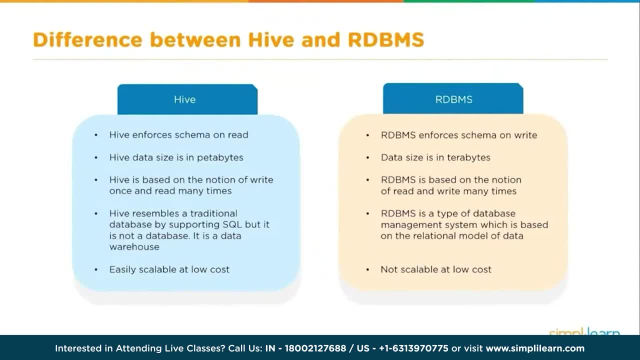 up so you might start off with a basic server and then you upgrade to a sun computer to run it and you spend, you know, tens of thousands of dollars for that hardware upgrade. with hive you just put another computer into your hadoop file system. so let's look at some of the features. 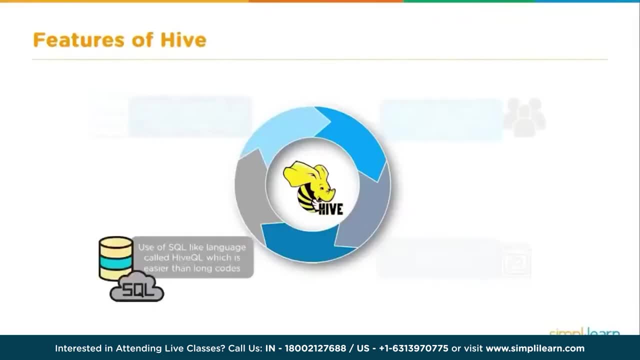 of hive. when we're looking at the features of hive, we're talking about the use of sql like language called hiveql. a lot of times you'll see that as hql, which is easier than long codes. this is nice if you're working with your shareholders. you come to them and you say: 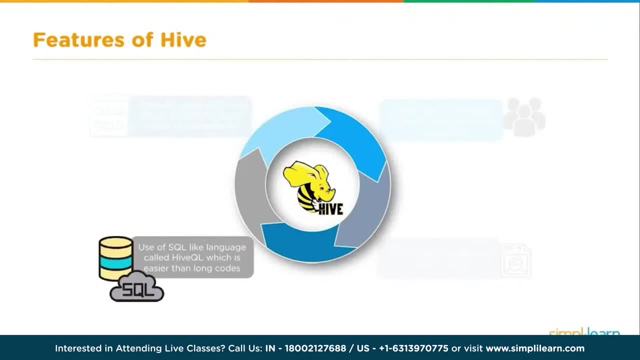 hey, you can do a basic sql query on here and pull up the information you need. this way you don't have to take off have your programmers jump in every time they want to look up something in the database. they actually now can easily do that if they're not skilled in programming and script. 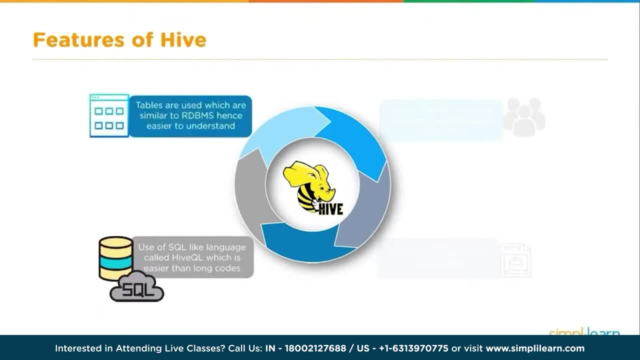 writing tables are used which are similar to the rdbms, hence easier to understand, and one of the things i like about this is when i'm bringing tables in from a mysql server- sql server. there's almost a direct reflection between the two. so when you're looking at one, which is the data which is? 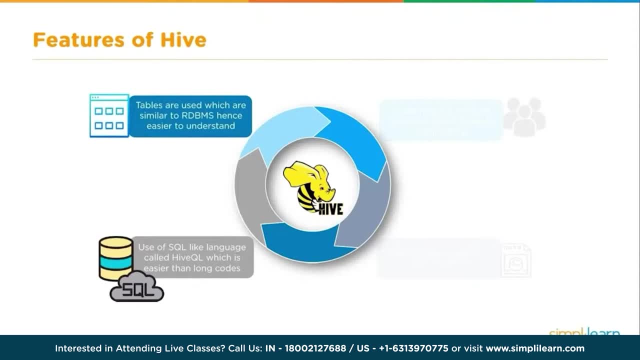 continually changing and then you're going into the archive database. it's not this huge jump where you have to learn a whole new language. you mirror that same schema into the hdfs, into the hive, making it very easy to go between the two, and then, using hiveql, multiple users can simultaneously. 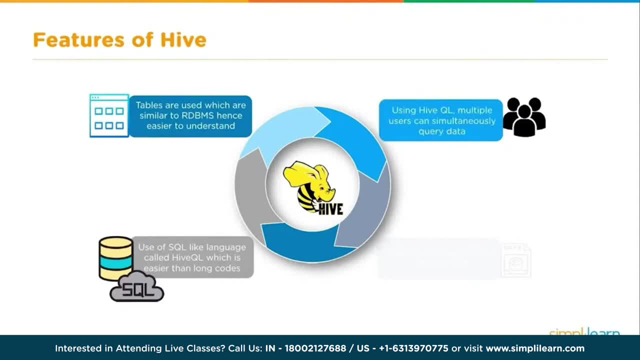 query data. so again you have multiple clients in there and they send in their query. that's also true with the rdbms, which kind of queues them up because it's running so fast you don't notice the lag time. well, you get that also with the hql. 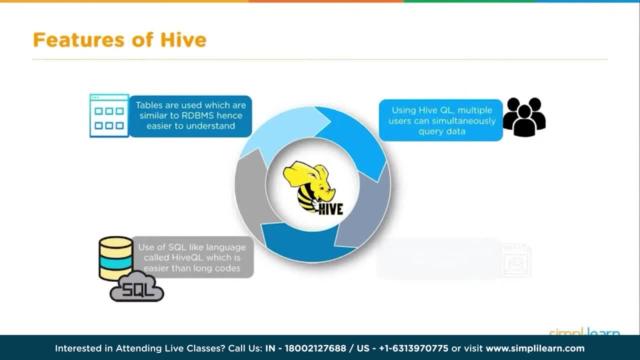 well, as you add more computers in the query can go very quickly depending on how many computers and how much resources each machine has to pull the information. and hive supports a variety of data types. so with hive it's designed to be on the hadoop system, which you can put almost 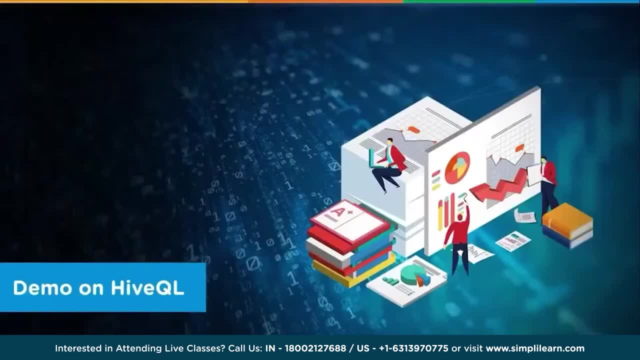 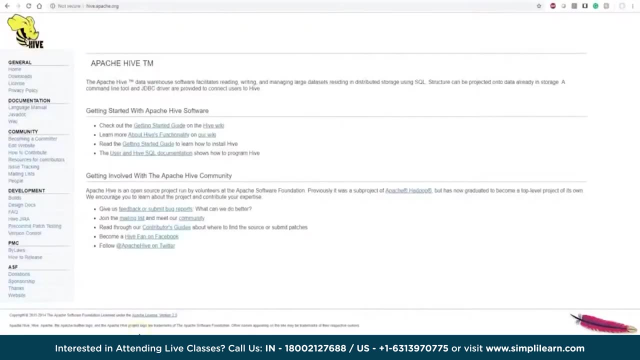 anything into the hadoop file system. so with all that, let's take a look at a demo on hive ql or hql. before i dive into the hands-on demo, let's take a look at the website hiveapacheorg. that's the main website since apache. it's an apache open source. 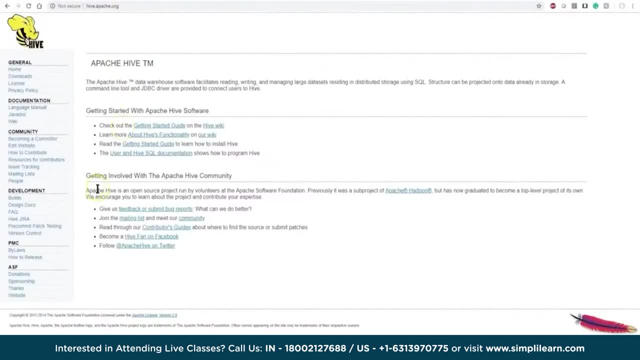 software. this is the main software or the main site for the build, and if you go in here you'll see that they're slowly migrating hive into beehive, and so if you see beehive versus hive, note the beehive is the new releases coming out. that's all it is. it reflects a lot of the same. 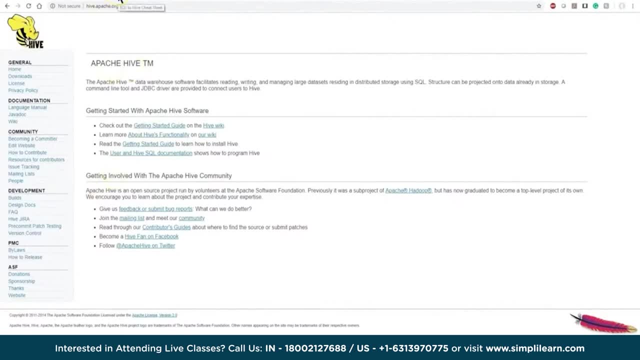 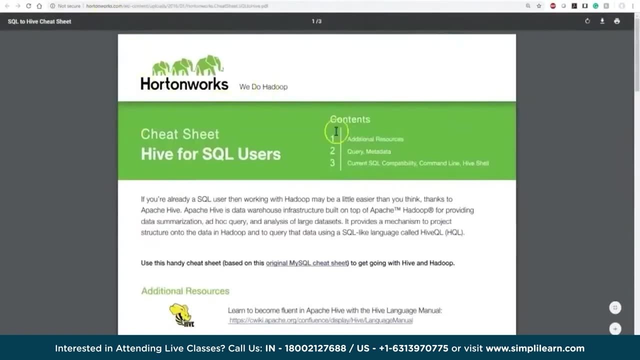 functionality of hive. it's the same thing. and then we like to pull up some kind of documentation on commands, and for this i'm actually going to go ahead and do a little bit of a look at the hortonworks hive cheat sheet, and that's because hortonworks and cloudera are two. 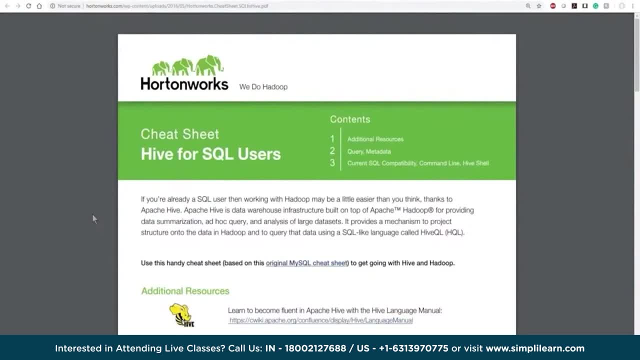 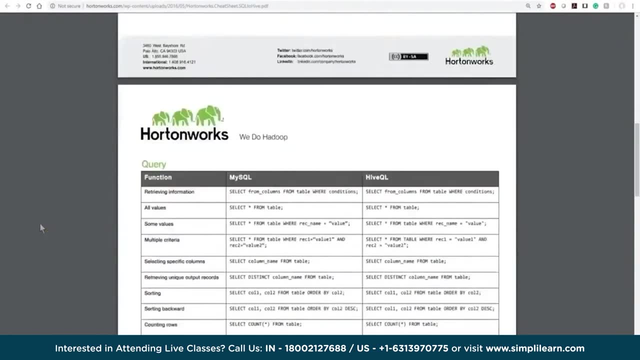 of the most common used builds for hadoop and for which include hive and all the different tools in there, and so hortonworks has a pretty good pdf. you can download cheat sheet on there. i believe cloudera does too, but we'll go ahead and just look at the horton one, because it's the one that comes. 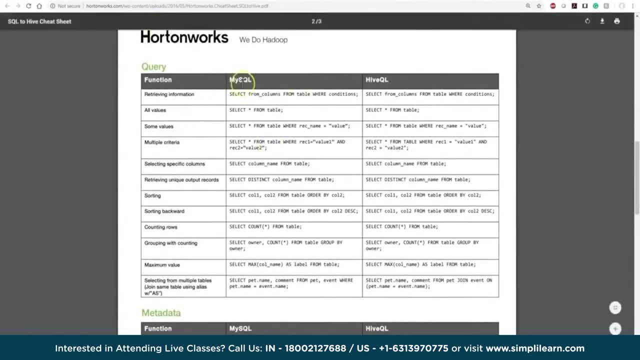 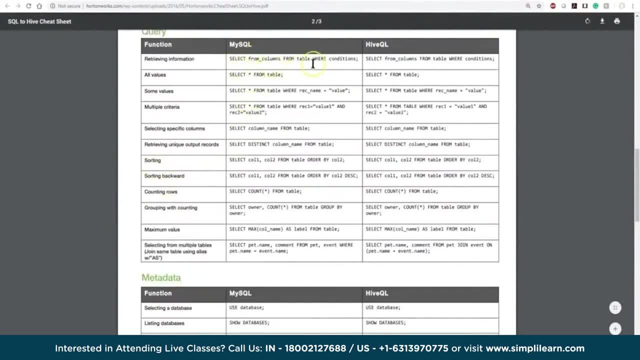 up really good and you can see when we look at the query language it compares mysql server to hive ql and we can see the basic select. we select from columns, from table where conditions exist. you know most basic command on there and they have different things. you can do with it just like you. 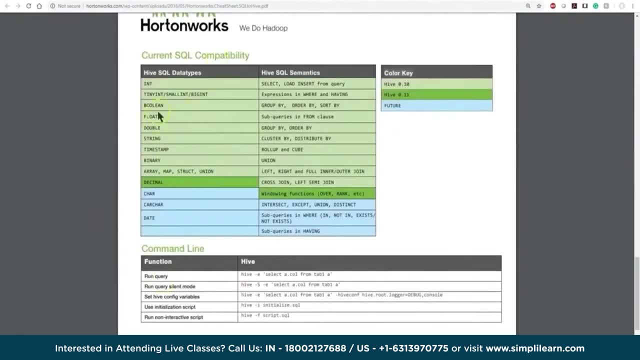 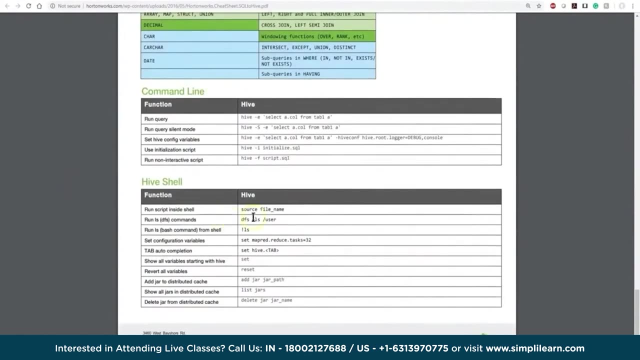 do with your sql and if you scroll down you'll see data types. so here's your integer, your flow, your binary double string timestamp and all the different data types. you can use some different semantics, different keys, features, functions for running a hive query, command line setup and of 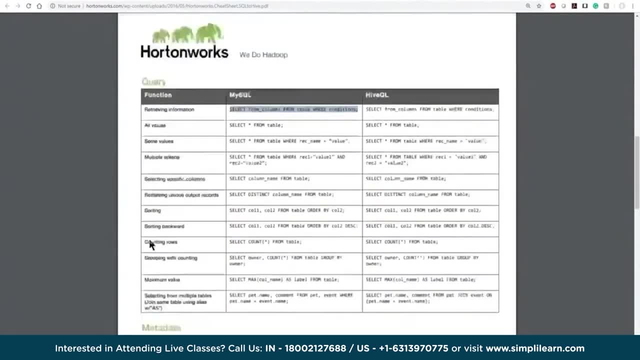 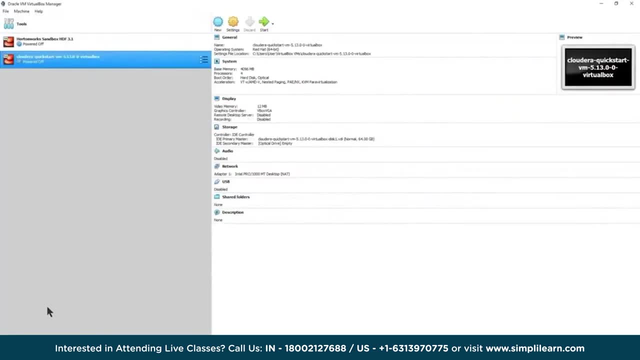 course the hive shell setup in here so you can see right here, if we loop through it, it has a lot of your basic stuff and it is. we're basically looking at sql across a horton database. we're going to go ahead and run our hadoop. 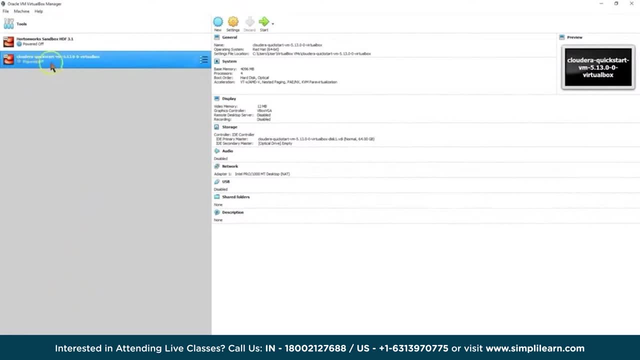 cluster hive demo and i'm going to go ahead and use the cloudera quick start. this is in the virtual box. so again, we have an oracle virtual box, which is open source, and then we have our cloudera quick start, which is the hadoop setup on a single node. now, obviously, hadoop and hive are designed 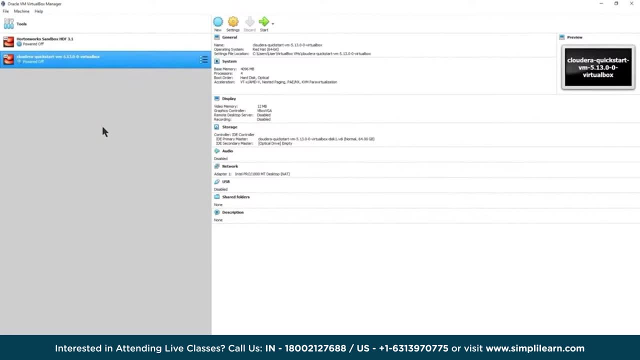 to run across a cluster of computers. So when we talk about a single node it's for education, testing, that kind of thing, And if you have a chance you can always go back and look at our demo we had on setting up a Hadoop system in a single cluster. 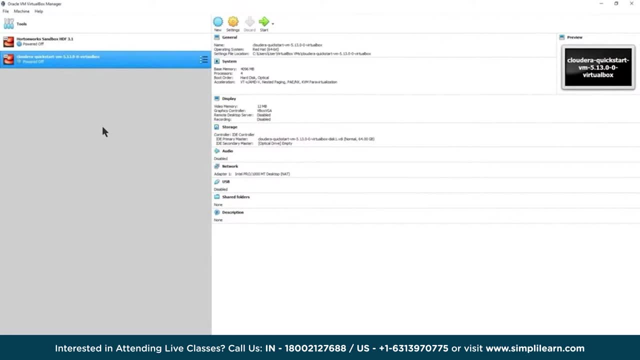 Just set a note down below in the YouTube video and our team will get in contact with you and send you that link if you don't already have it, Or you can contact us at the wwwsimplylearncom Now in here. it's always important to note. 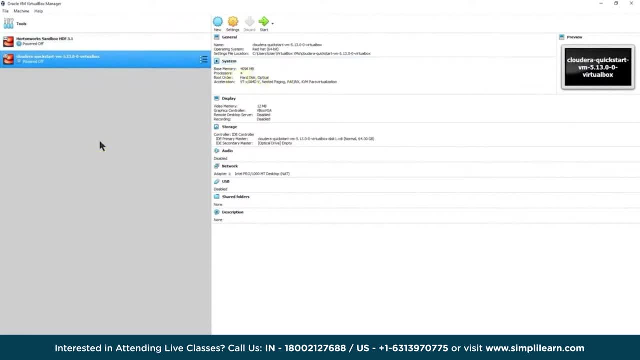 that you do need on your computer. if you're running on Windows- because I'm on a Windows machine- you're gonna need probably about 12 gigabytes to actually run this. It used to be. you could buy with a lot less, but as things have evolved, 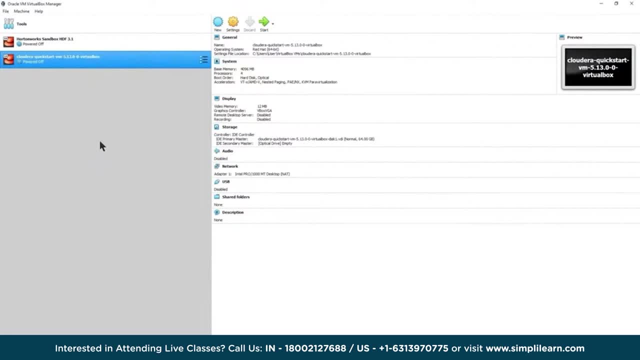 they take up more and more resources And you need the professional version If you have the home version. I was able to get that to run, but boy did it take a lot of extra work to get the home version to. let me use the virtual setup on there. 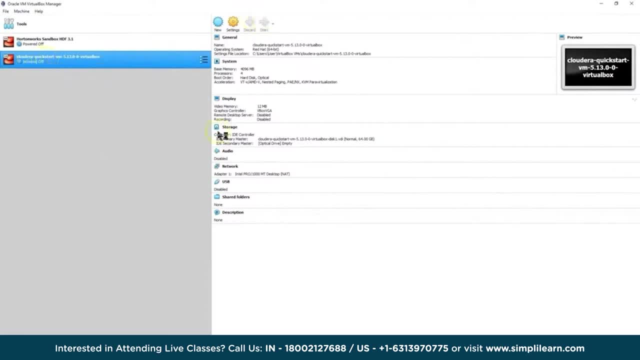 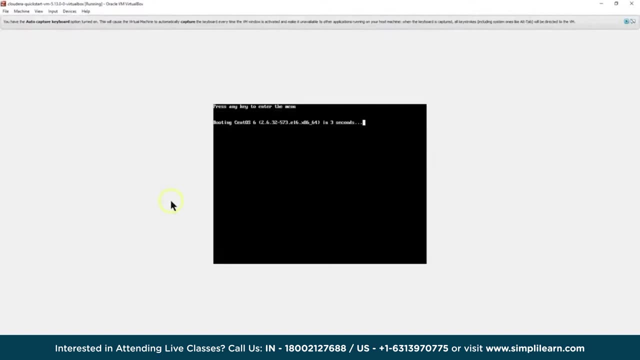 And we'll simply click on the Cloudera Quick Start and I'm gonna go ahead and just start that up. And this is starting up our Linux. so we have our Windows 10, which is the computer I'm on, and then I have the VirtualBox. 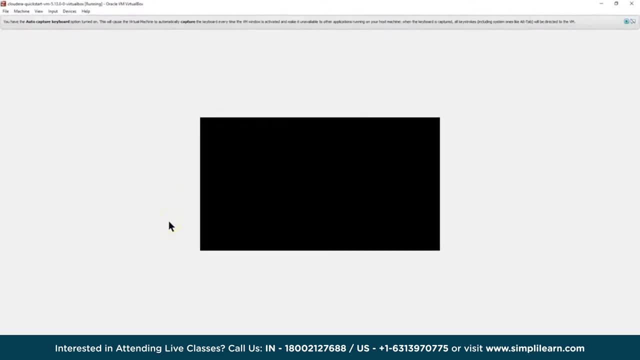 which is gonna have a Linux operating system in it, And we'll skip ahead so you don't have to watch the whole install. Something interesting to know about the Cloudera is that it's running on Linux CentOS and, for whatever reason, 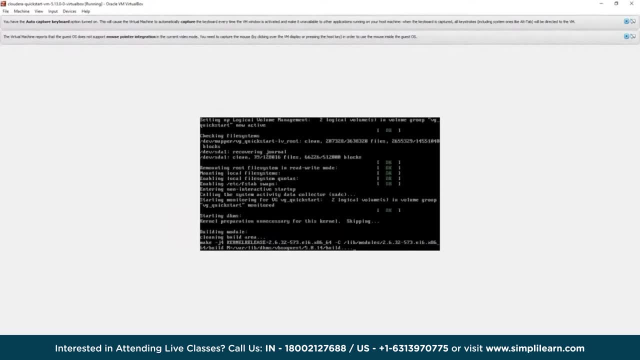 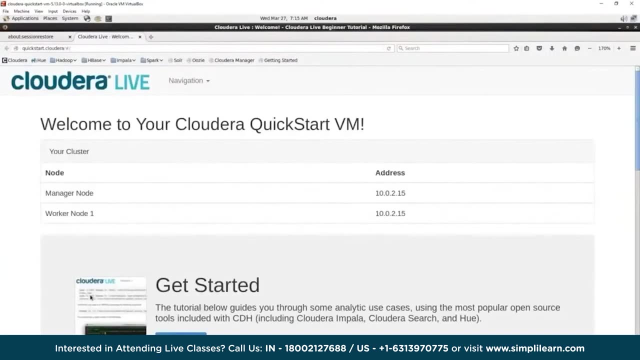 I've always had to click on it and hit the Escape button for it to spin up, And then you'll see the DOS come in here. Now that our Cloudera has spun up on our virtual machine with the Linux on, we can see: here we have our 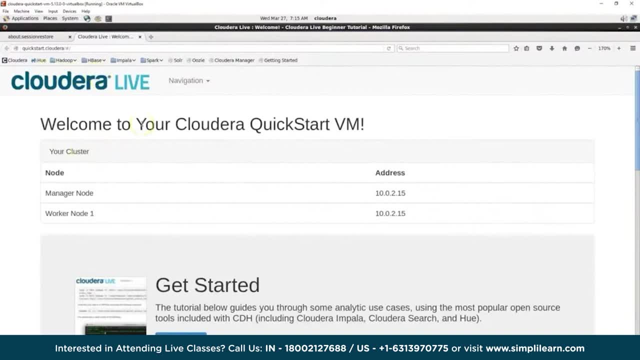 it uses the Thunderbird browser on here by default and automatically opens up a number of different tabs for us. And a quick note, because I mentioned the restrictions on getting set up on your own computer. if you have a home edition computer and you're worried about setting it up on there. 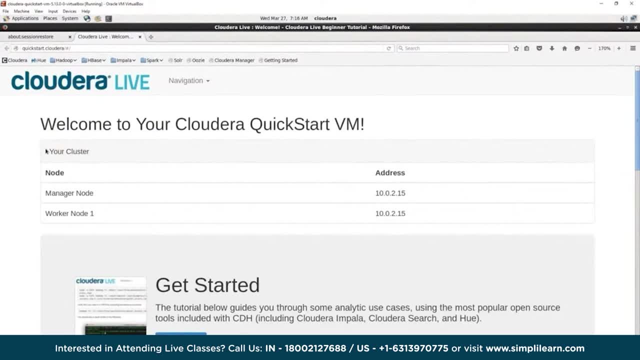 you can also go in there and spin up a one-month free service on Amazon Web Service to play with this. So there's other options. You're not stuck with just doing it on the Quick Start menu. You can spin this up in many other ways. 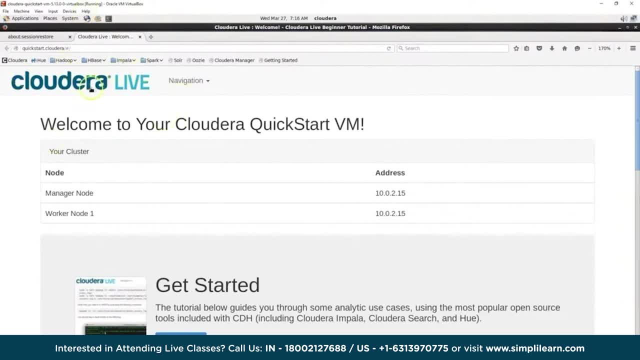 Now, the first thing we want to note is that we've come in here into Cloudera and I'm going to access this in two ways. The first one is we're going to use Hue And I'm going to open up Hue. 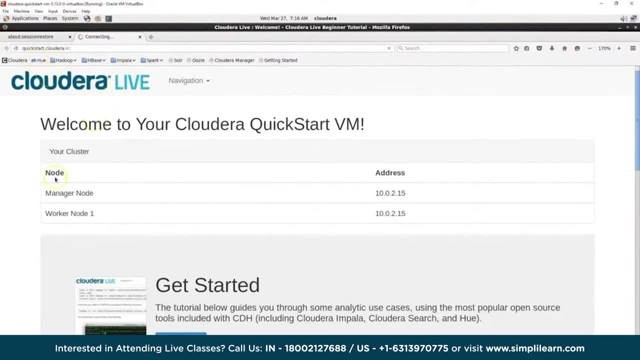 and I'll take it a moment to load from the setup on here. And Hue is nice. If I go in and use Hue as an editor into Hive or into the Hadoop setup, usually I'm doing it from an admin side because it has a lot more information. 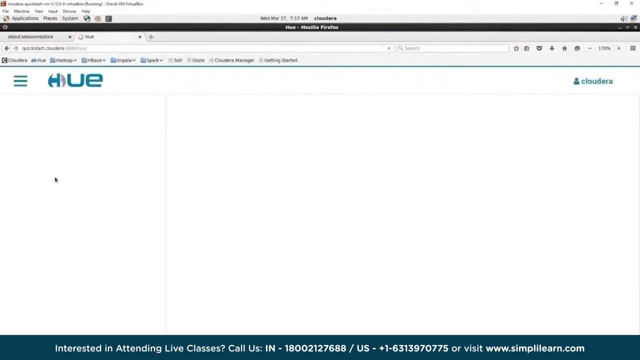 a lot of visuals, less to do with actually diving in there and just executing code, And you can also write this code into files and scripts and there's other ways you can upload it into Hive. But today we're going to look at the command lines. 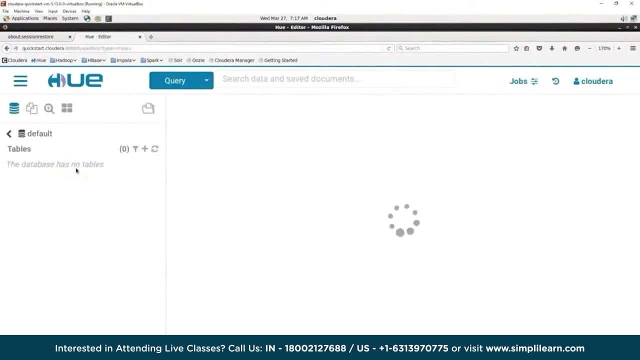 and we'll upload it into Hue And then we'll go into and actually do our work in a terminal window under the Hive shell Now in the Hue browser window, if you go under Query and click on the pull-down menu and then you go under Editor. 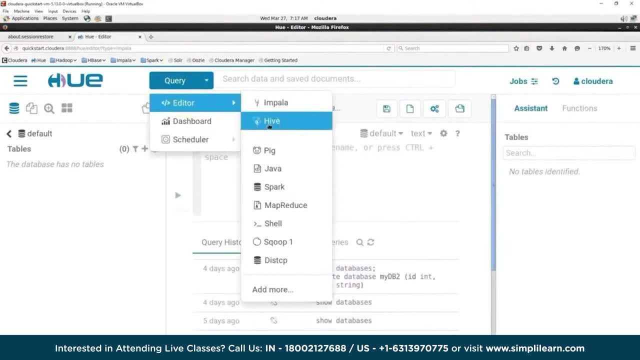 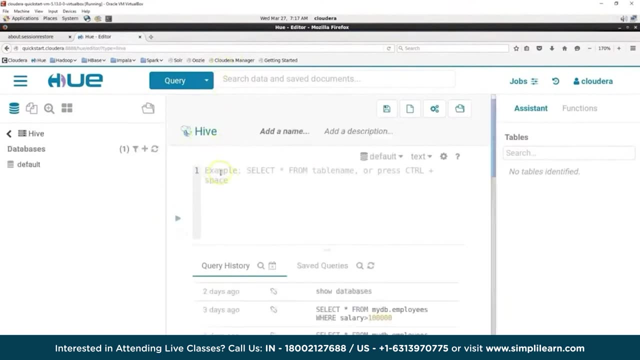 and you'll see Hive. There we go, There's our Hive setup. I go and click on Hive and this will open up our query down here. And now it has a nice little B that shows our Hive going And we can go something very simple down here. 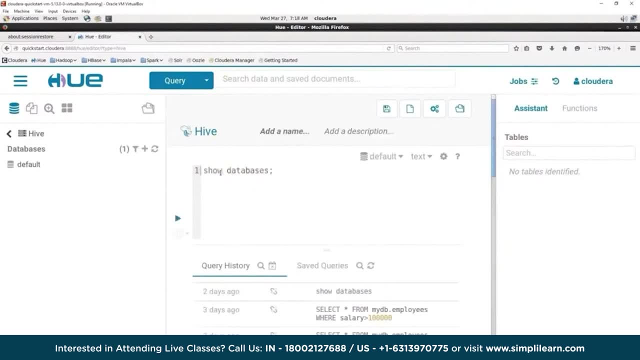 like Show Databases And we follow it with a semicolon. And that's the standard in Hive is? you always add our punctuation at the end there And I'll go ahead and run this and the query will show up underneath And you'll see down here. 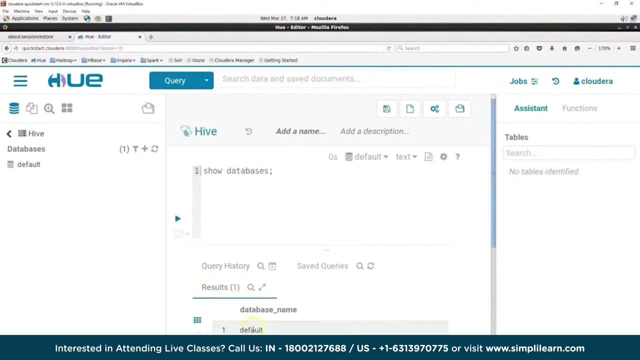 since this is a new quick start I just put on here. you'll see it has the default down here for the databases. That's the database name. I haven't actually created any databases on here. And then there's a lot of other. 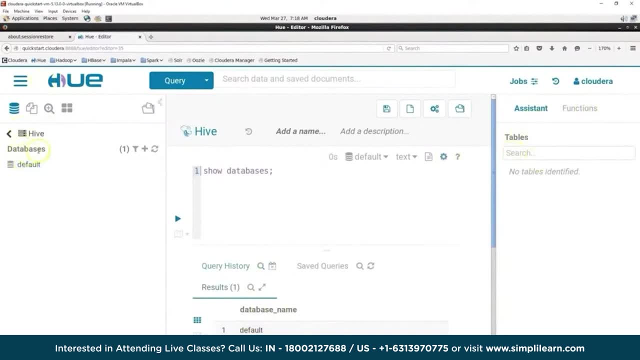 like assistant functions, tables, your databases up here. There's all kinds of things you can research, you can look at through Hue as far as a bigger picture. The downside of this is it always seems to lag For me whenever I'm doing this. 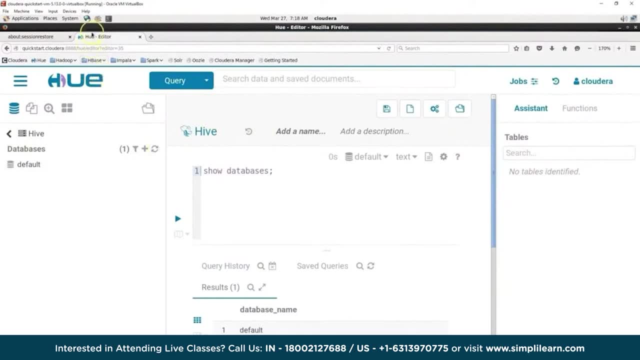 I always seem to run slow. So if you're in Cloudera, you can open up a terminal window. They actually have an icon at the top. You can also go under Applications, and under Applications, System Tools and Terminal. Either one will work. 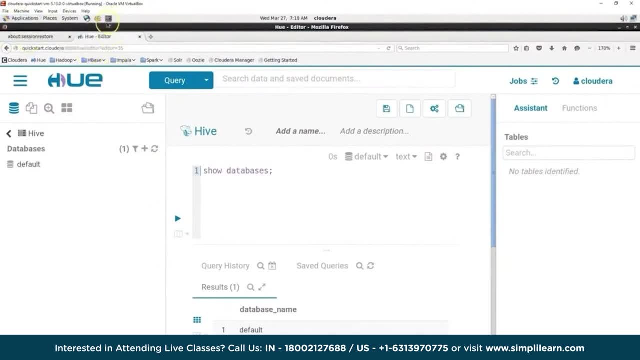 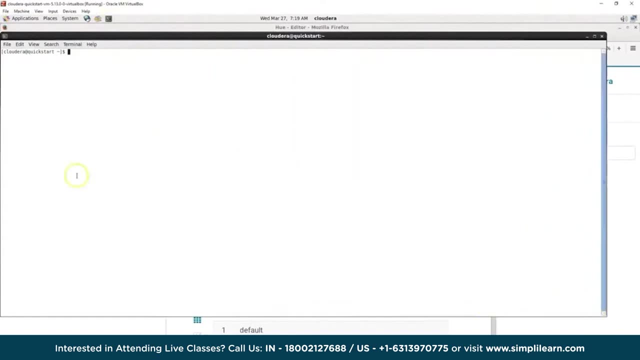 It's just a regular terminal window And this terminal window is now running underneath our Linux. So this is a Linux terminal window on our virtual machine which is resting on our regular Windows 10 machine, And we'll go ahead and zoom this in. 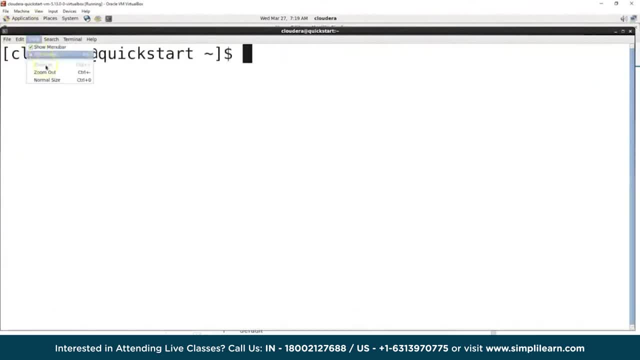 so you can see the text better on your own video, And I simply just clicked on View and Zoom In And then all we have to do is type in Hive And this will open up the shell on here And it takes it just a moment to load. 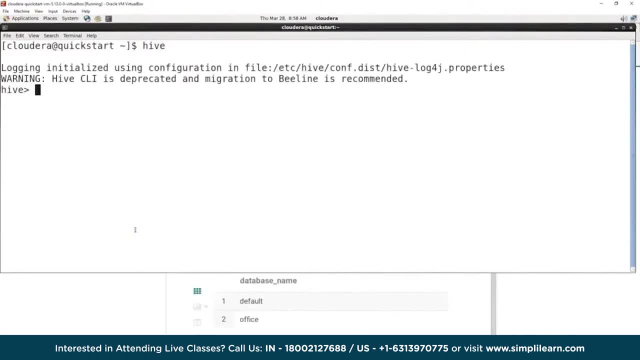 When starting up Hive. I also want to note that, depending on your rights on the computer you're on in your action, you might have to do sudo hive And put in your password and username. Most computers are usually set up with the Hive login. 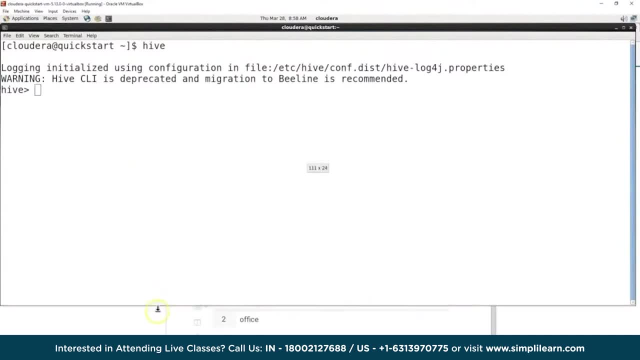 Again, it just depends on how you're accessing the Linux system in the Hive shell. Once we're in here, we can go ahead and do a simple HQL command- Show Databases, And if we do that we'll see here that we don't have any databases. 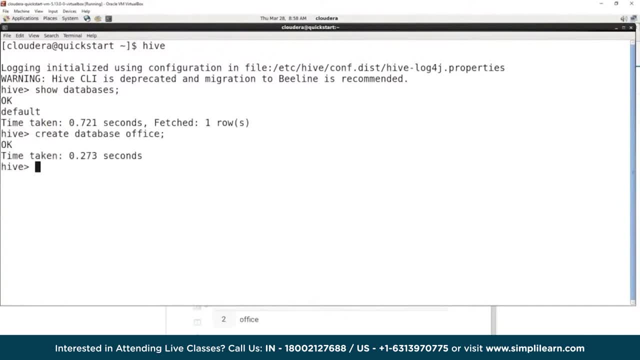 So we can go ahead and create a database And we'll just call it Office for this moment. Now, if I do Show, we'll just do the up arrow. Up arrow is a hot key that works in both Linux and in Hive, So I can go back and page through. 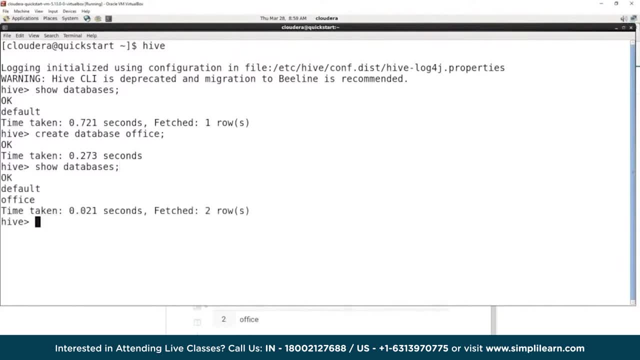 all the commands I've typed in And we can see. now that I have my, there's, of course, the default database and then there's the Office database. So now we've created a database. It's pretty quick and easy And we can go ahead and drop the database. 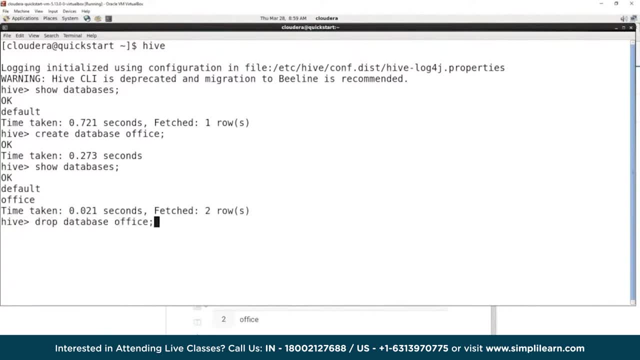 We can do Drop Database Office. Now this will work on this database because it's empty. If your database was not empty, you would have to do Cascade And that drops all the tables in the database and the database itself. Now, if we do Show Database, 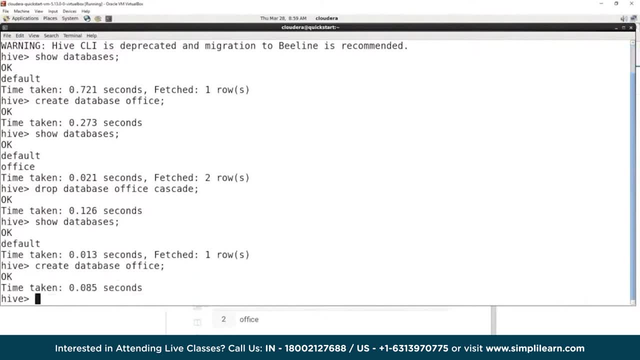 and we'll go ahead and recreate our database because we're going to use the Office database for the rest of this hands-on demo. A really handy command, now set with the SQL or HQL, is to use Office, And what that does is that sets Office. 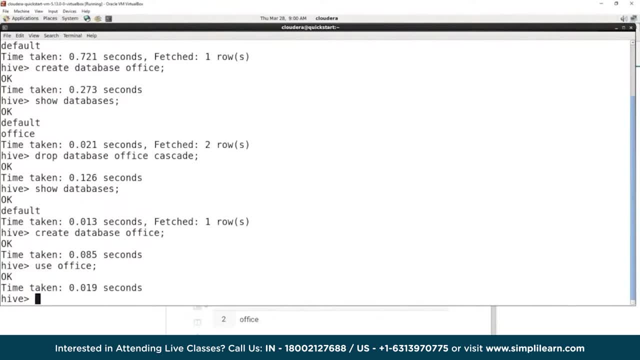 as the default database. So, instead of having to reference the database every time we work with a table, it now automatically assumes that's the database being used for whatever tables we're working on. The difference is: is you put the database name period table? 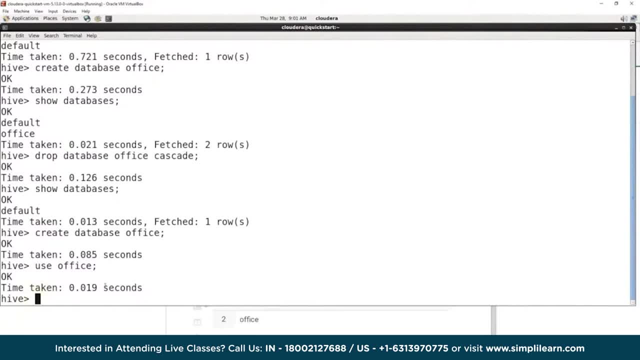 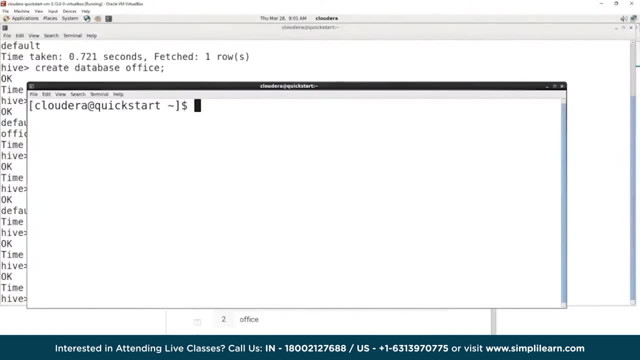 I'll show you in just a minute what that looks like and how that's different. If we're going to have a table and a database, we should probably load some data into it. So let me go ahead and switch gears here and open up a terminal window. 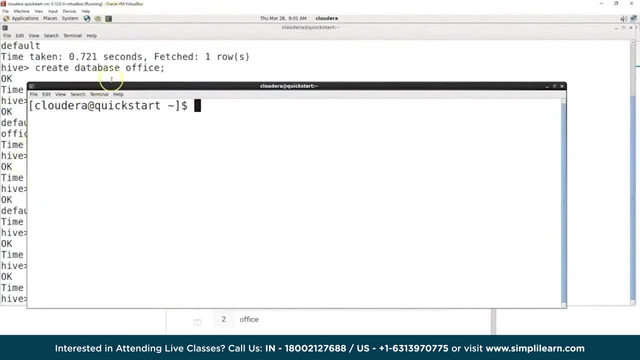 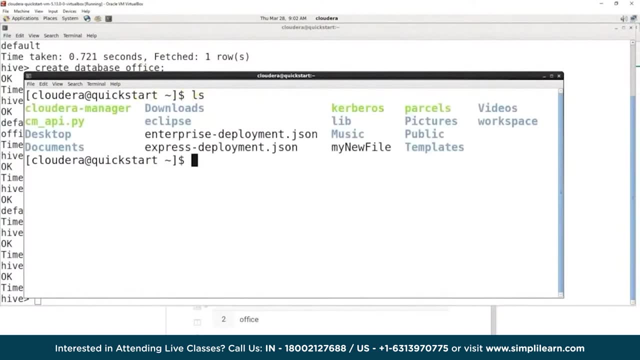 You can just open another terminal window and it'll open up right on top of the one that you have Hive Shell running in. And when we're in this terminal window first, we're going to go ahead and just do a list, which is, of course, a Linux command. 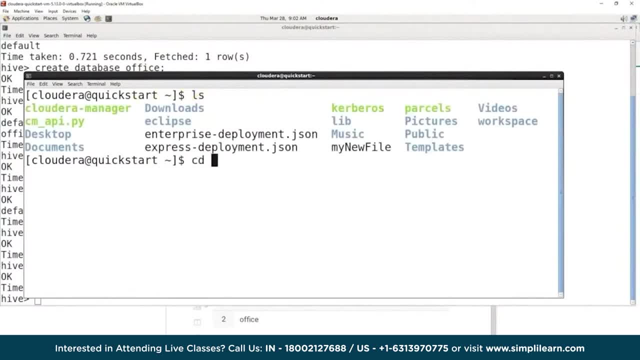 You can see all the files I have in here. This is the default load. We can change directory to Documents, We can list in Documents And we're actually going to be looking at employeecsv. A Linux command is the cat. You can use this actually to combine documents. 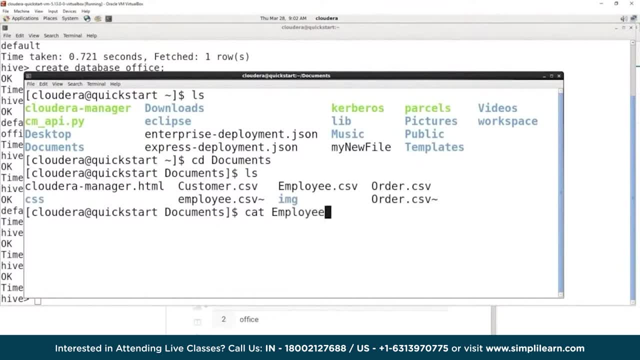 There's all kinds of things that cat does. But if we want to just display the contents of our employeecsv file, we can simply do cat employee csv. And when we're looking at this we want to know a couple things. One, there's a line at the top: 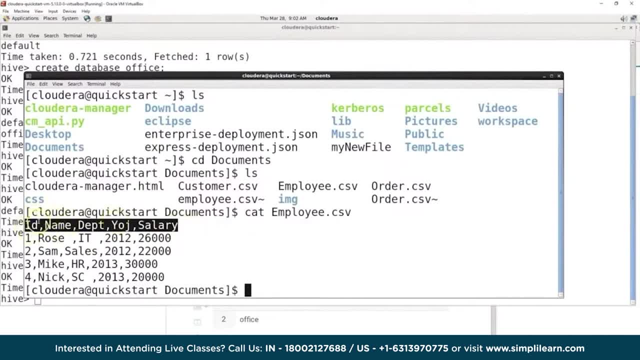 Okay, so the very first thing we notice is that we have a header line. The next thing we notice is that the data is comma separated And in this particular case you'll see a space here. Generally, with these you've got to be real careful. 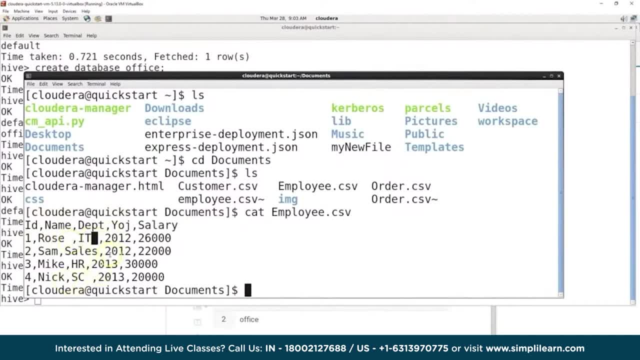 with spaces. There's all kinds of things you've got to watch out for because it can cause issues. These spaces won't, because these are all strings that the space is connected to. If this was a space next to the integer, you would get a null value that comes into the database. 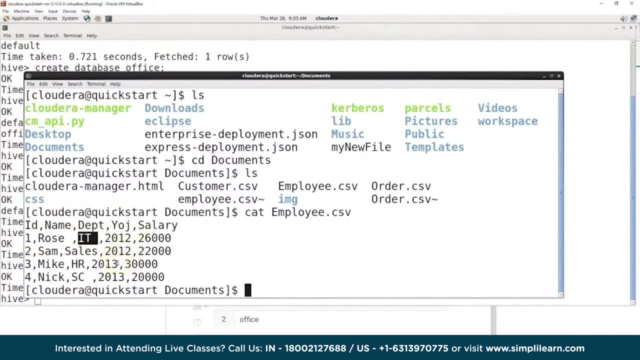 without doing something extra in there. Now, with most of Hadoop, that's important to know that you're writing the data once, reading it many times, And that's true of almost all your Hadoop things coming in. So you really want to process the data. 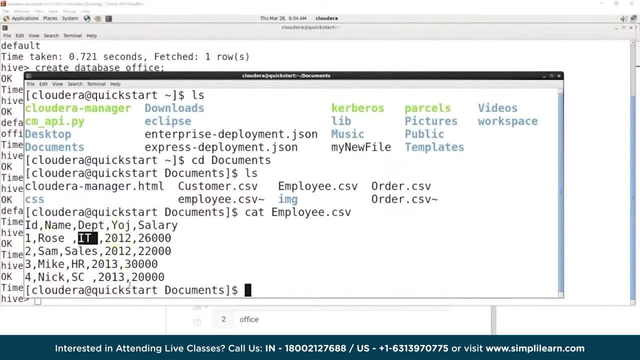 before it gets into the database. And for those of you who have studied data transformation, that's the etl, where you extract transfer form and then load the data. So you really want to extract and transform before putting it into the hive. 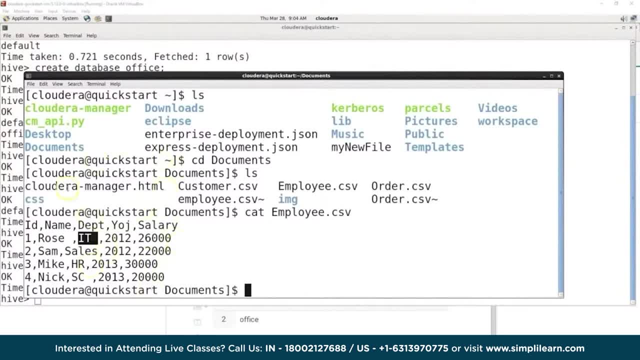 Then you load it into the hive with the transformed data. And of course we also want to note the schema. We have an integer, string, string, integer, integer. So we kept it pretty simple in here as far as the way the data is set up. 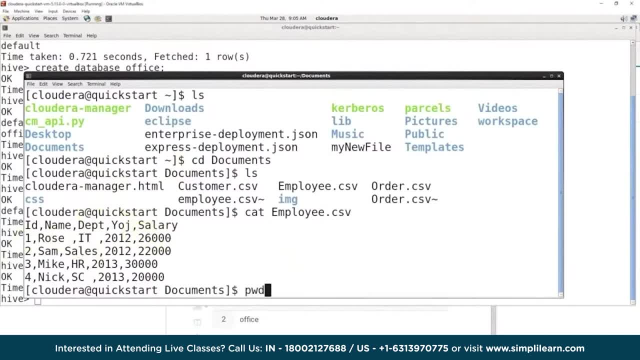 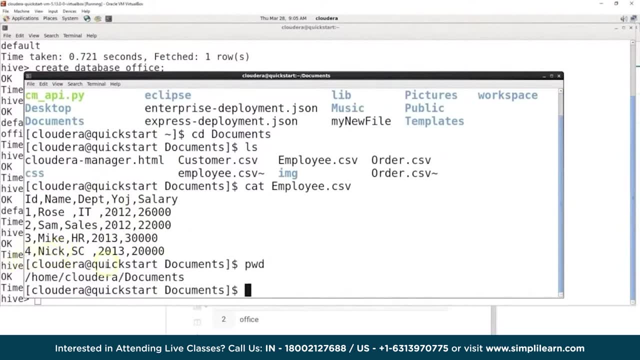 The last thing that you're going to want to look up is the source. Since we're doing local uploads, we want to know what the path is. We have the whole path. In this case it's home slash, Cloudera slash documents. 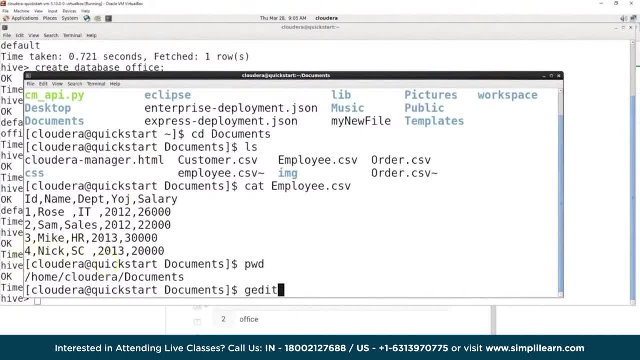 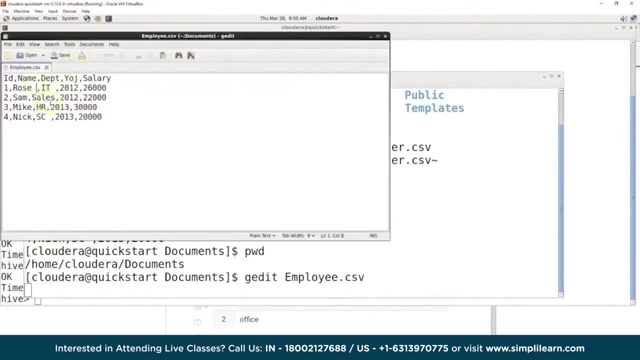 And these are just text documents we're working with right now. We're not doing anything fancy, So we can do a simple get edit employee dot csv And you'll see it comes up here. It's just a text document so I can easily remove these added spaces. 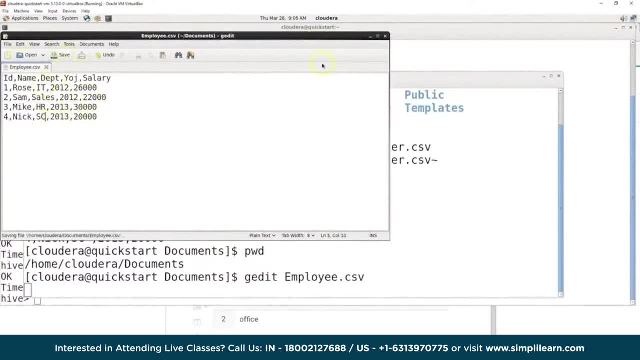 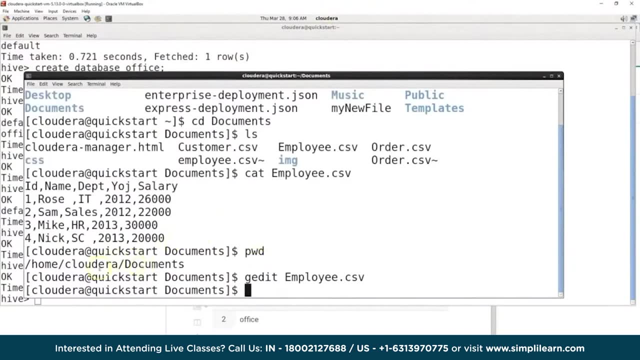 There we go, And then we go ahead and just save it, And so now it has a new setup in there. We've edited it. The gedit is usually one of the default that loads into Linux, So any text editor will do. 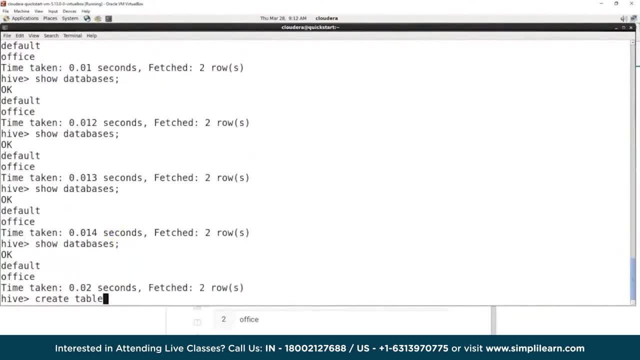 Back to the hive shell. So let's go ahead and create a table employee, And what I want you to note here is I did not put the semicolon on the end here. Semicolon tells it to execute that line. So this is kind of nice if you're. 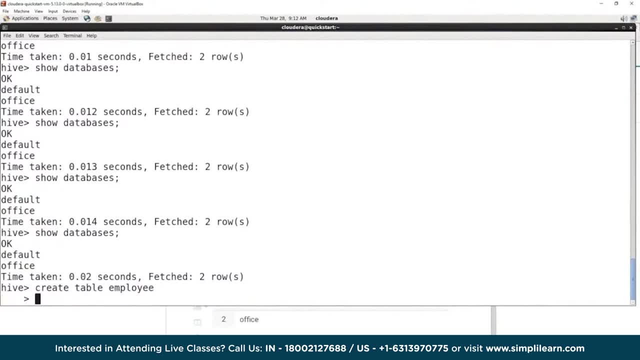 you can actually just paste it in if you have it written on another sheet And you can see right here where I have create table employee and it goes into the next line on there, so I can do all of my commands at once. Now, just so I don't have any typo errors. 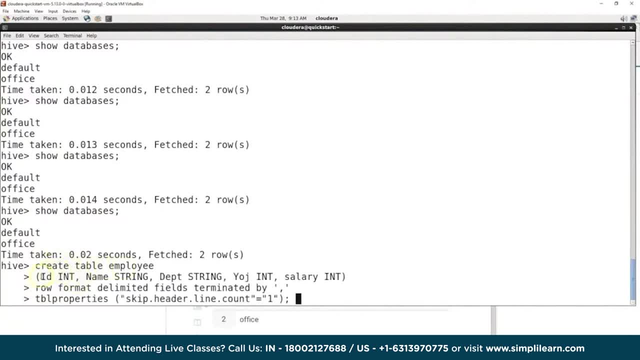 I went ahead and just pasted the next three lines in, And the next one is our schema. If you remember correctly, from the other side we had the different values in here, which was ID name, department, year of joining and salary. 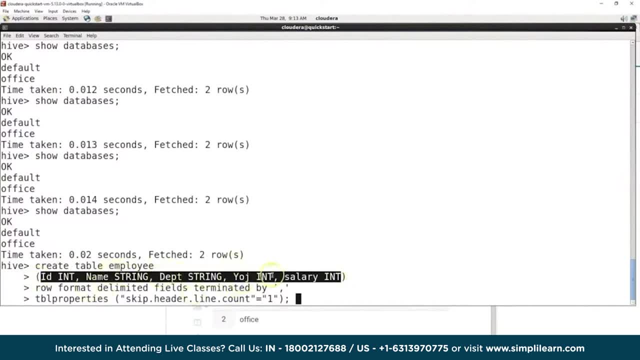 And the ID is an integer, name is a string department, string, year of joining energy salary and integer And they're in brackets. We put close black brackets around them And you could do this all as one line And then we have row format. 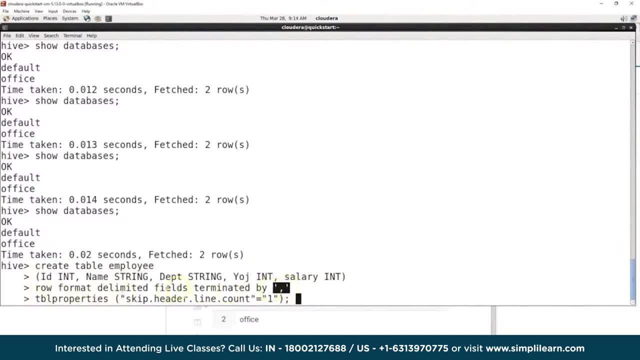 delimited fields terminated by comma. And this is important because the default is tabs. So if I do it now, it won't find any terminated fields, So you'll get a bunch of null values loaded into your table. And then, finally, our table properties. 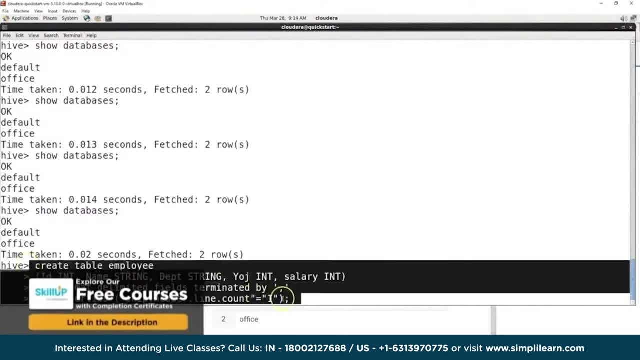 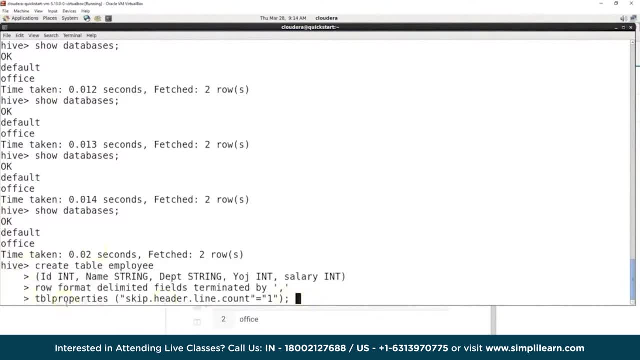 we wanna skip the header line. count equals one. Now this is a lot of work for uploading a single file. It's kinda goofy when you're uploading a single file that you have to put all this in here. But keep in mind Hive and Hadoop. 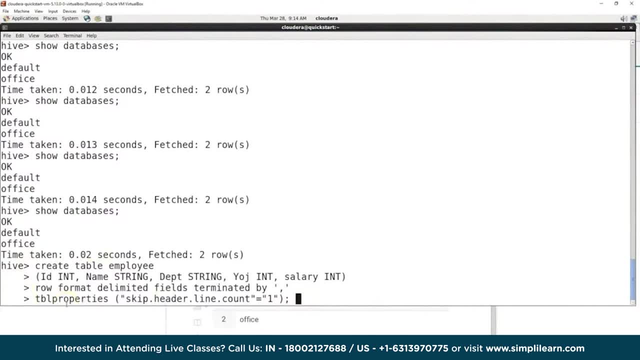 is designed for writing many files into the database. You write them all in there and then you can. they're saved. it's an archive, it's a data warehouse, And then you're able to do all your queries on them. So a lot of times we're not looking at. 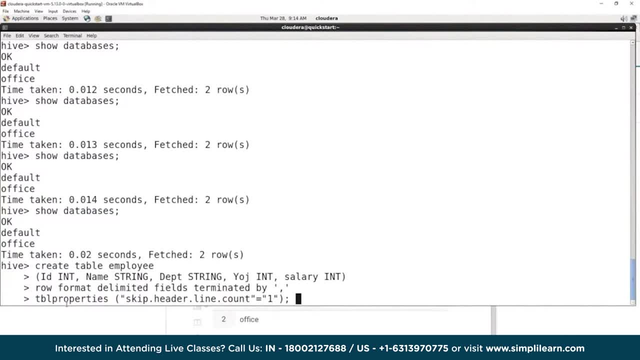 just the one file coming up. we're loading hundreds of files. You have your reports coming off of your main database. All those reports are being loaded. You have your log files. you have, I mean, all this different data is being dumped into Hadoop. 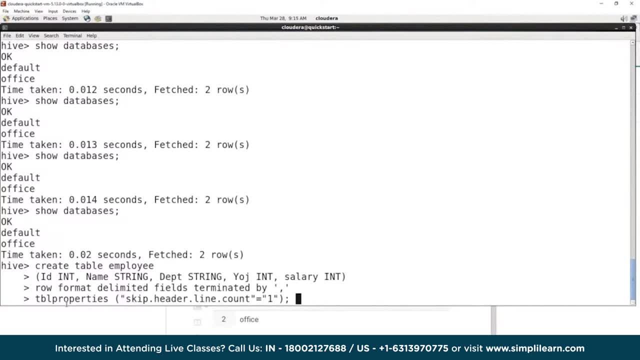 and in this case, Hive on top of Hadoop, And so we need to let it know. hey, how do I handle these files coming in? And then we have the semicolon at the end, which lets us know to go ahead. 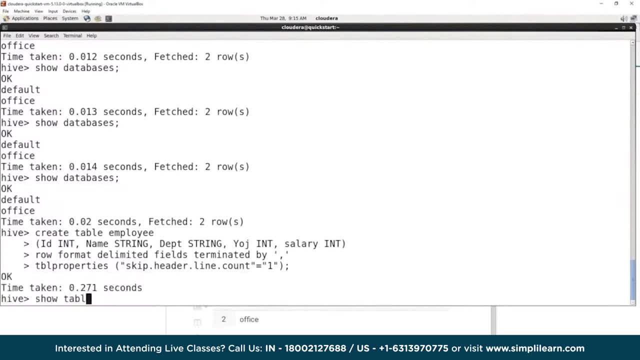 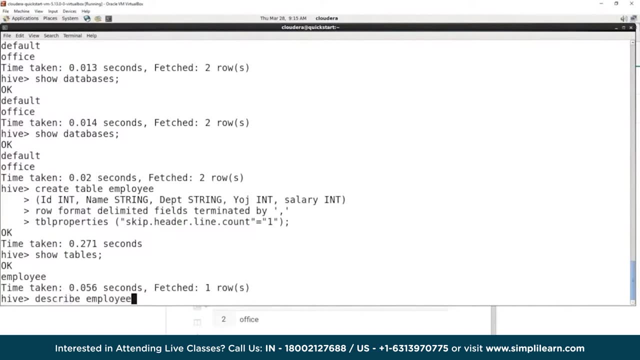 run this line and so we'll go ahead and run that. And now, if we do a show tables, you can see there's our employee on there. We can also describe. If we do describe employee, you can see that we have our ID. integer. 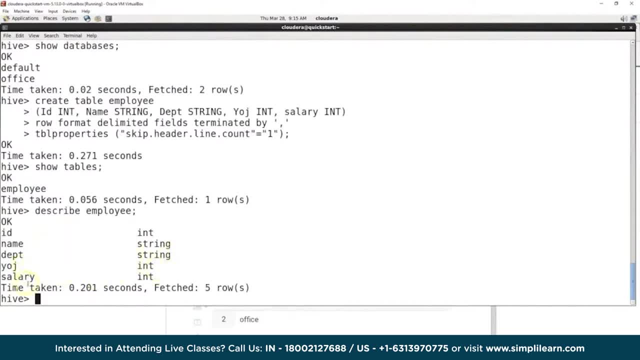 name string, department string, year of joining: integer and salary: integer. And then finally, let's just do a select star from employee. very basic SQL and HQL command selecting data. It's gonna come up and we haven't put anything in it. 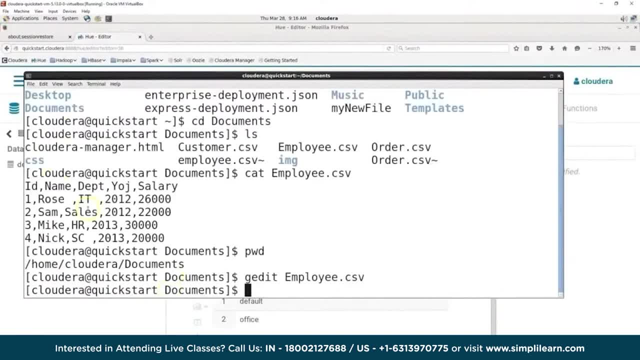 so, as we expect, there's no data in it. So if we flip back to our Linux terminal window, you can see where we did the cat employeecsv and you can see all the data we expect to come into it. And we also did our PWD. 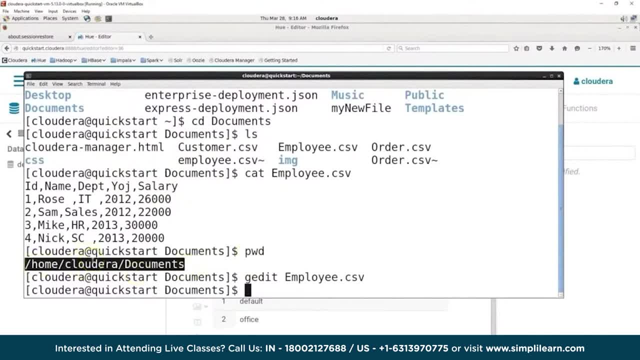 and right here you see the path. You need that full path when you are loading data. You know you can do a browse and if I did it right now with just the employeecsv as a name, it will work, But that is a really bad habit in general. 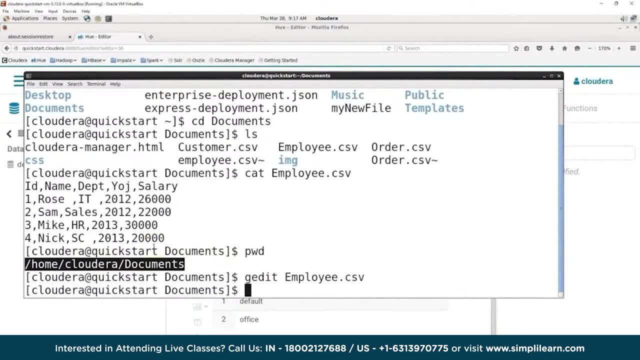 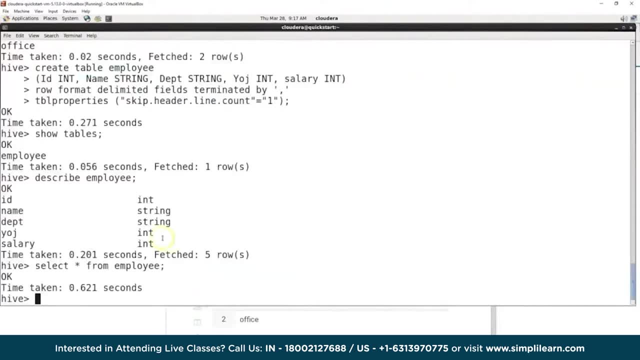 when you're loading data, because you don't know what else is going on in the computer. You wanna do the full path almost in all your data loads, So let's go ahead and flip back over here to our Hive shell. we're working in. 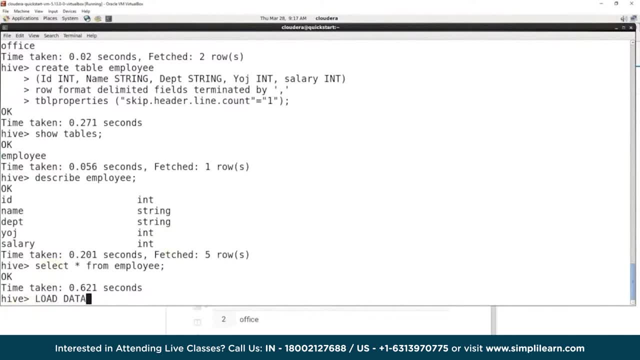 and the command for this is load data. So that says, hey, we're loading data, That's a Hive command, HQL, And we want local data. so you gotta put down local and path. so now it needs to know where the path is. 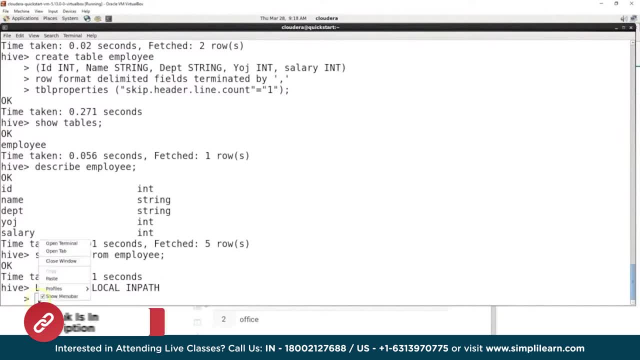 Now, to make this more legible, I'm just gonna go ahead and hit enter and then we'll just paste the full path in there, which I have stored over on the side Like a good prepared demo, And you'll see, here we have home. 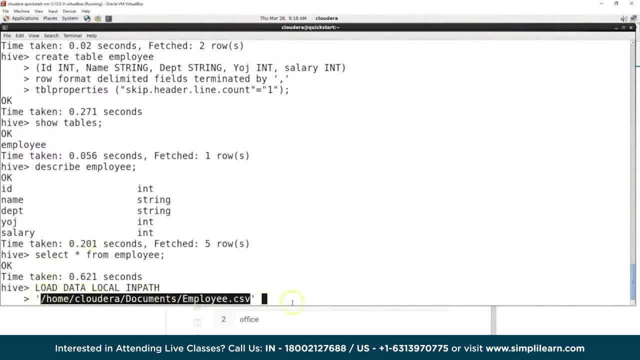 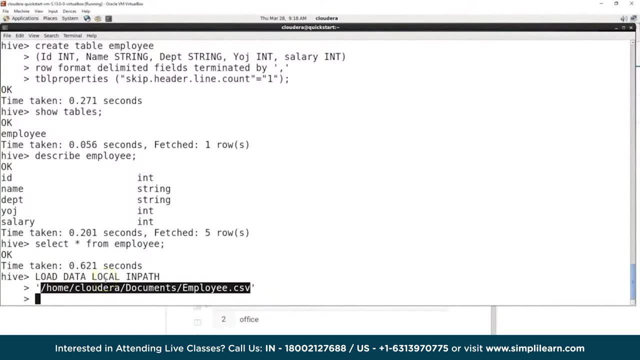 Cloudera documents- employeecsv. So it's a whole path for this text document in here And we go ahead and hit enter in there and then we have to let it know where the data's going. So now we have a source and we need a destination. 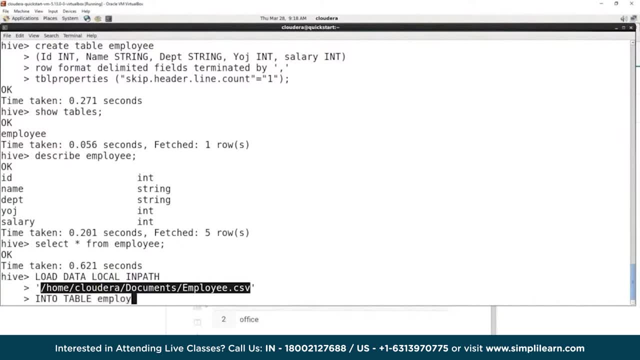 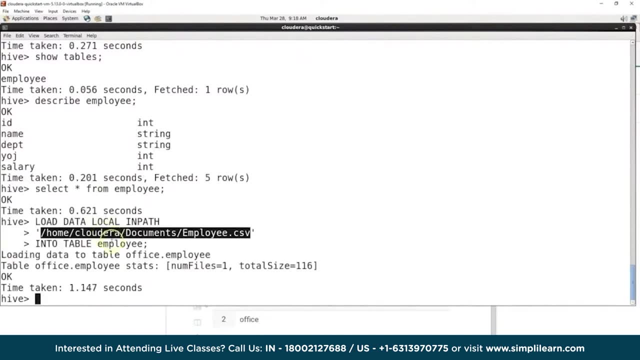 And it's gonna go into the table and we'll just call it employee. We'll just match the table in there And, because I want it to execute, we put the semicolon on the end. it goes ahead and executes all three lines. 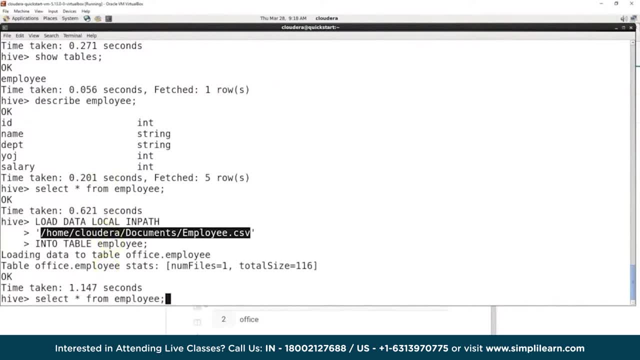 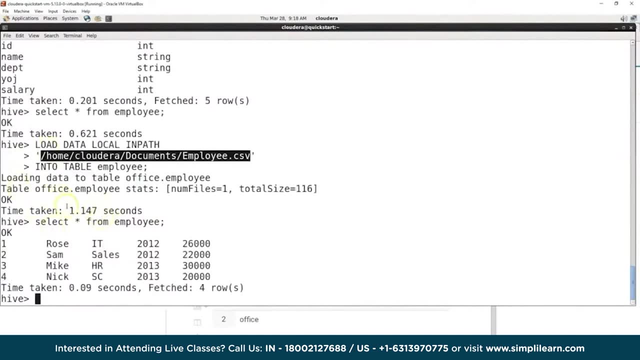 Now, if we go back, if you remember, select star from employee just using the up error to page through my different commands I've already typed in. You can see right here we have as we expect. we have Rose, Sam, Mike and Nick. 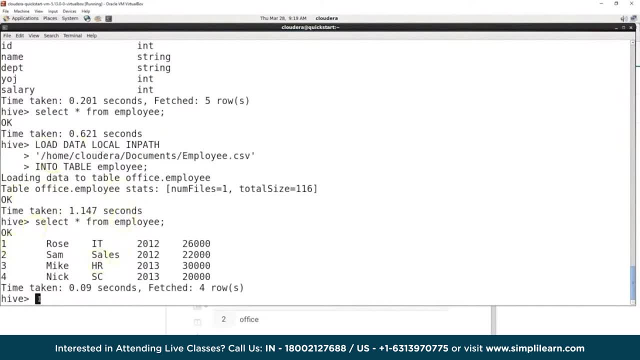 and we have all their information showing in our four rows. And then let's go ahead and do select and count. We'll just look at a couple of these different select options you can do. We're gonna count everything from employee. Now, this is kind of interesting. 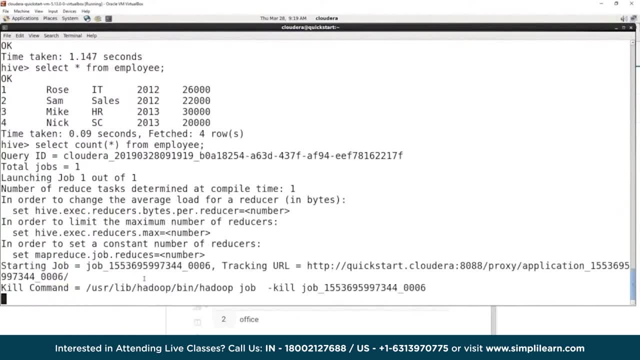 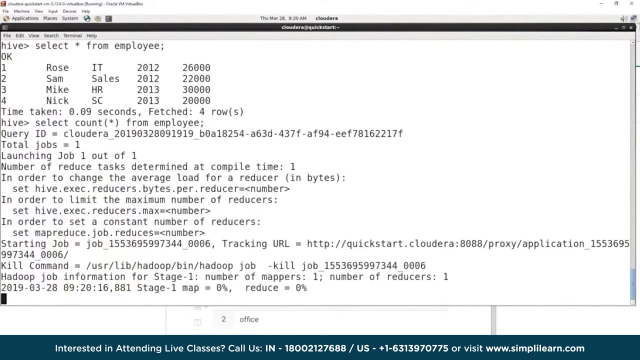 because the first one just pops up with a basic select, because it doesn't need to go through the full map reduce phase, But when you start doing a count it does go through the full map reduce setup in the Hive and Hadoop And because I'm doing this demo on a single node. 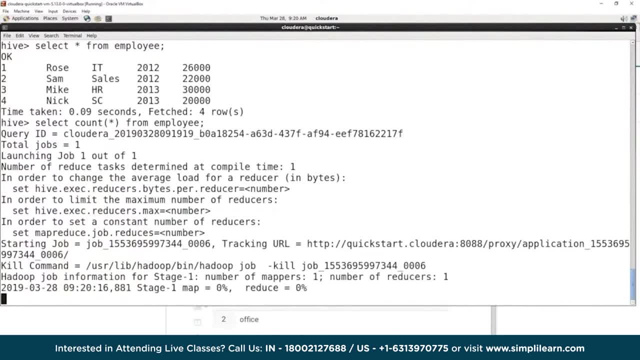 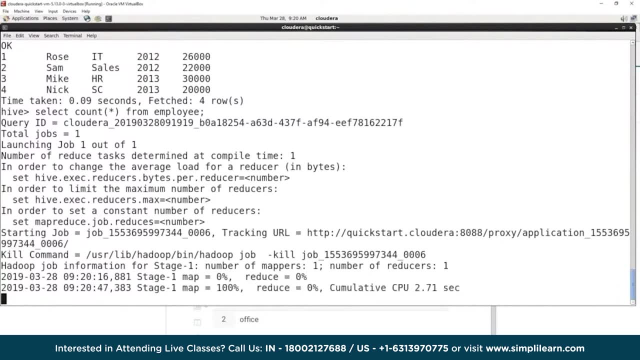 Cloudera virtual box on top of a Windows 10, all the benefits of running it on a cluster are gone and instead it's now going through all those added layers, so it takes longer to run. You know, like I said, when you do a single node, 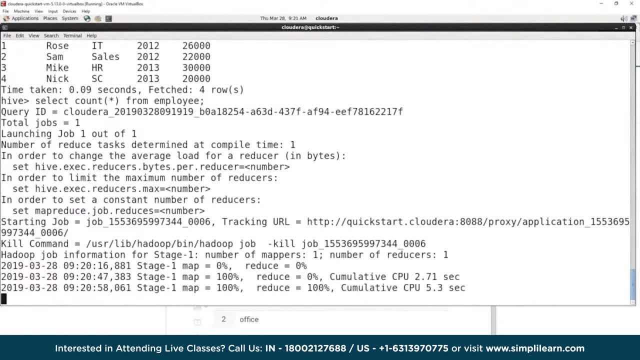 as I said earlier, it doesn't do any good as an actual distribution, because you're only running it on one computer and then you've added all these different layers to run it And we see it comes up with four. and that's what we expect. 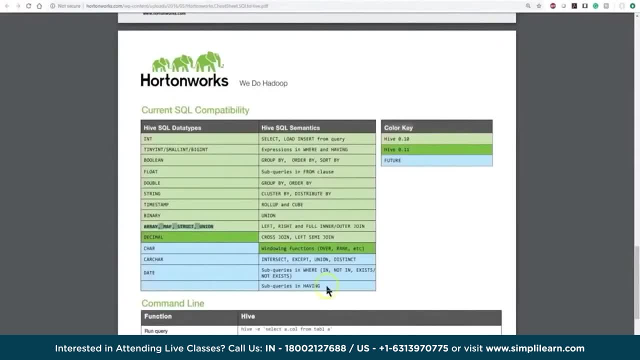 We have four rows. we expect four at the end And if you remember from our cheat sheet which we brought up here from Horton's, it's a pretty good one. there's all these different commands we can do. We'll look at one more command where we do the. 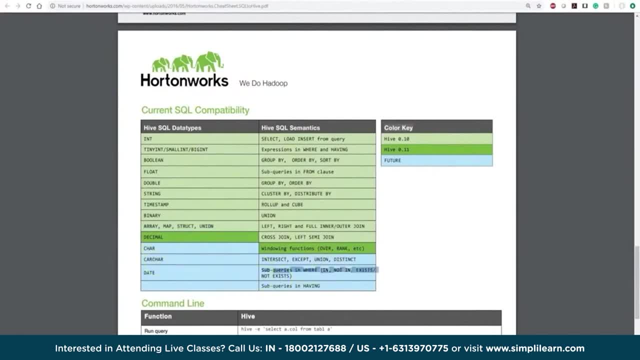 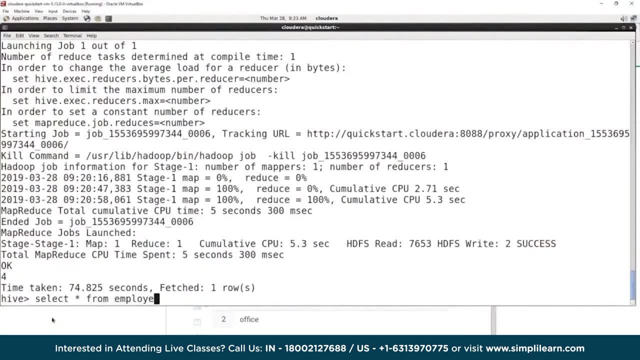 what they call sub queries right down here, because that's really common to do a lot of sub queries, And so we'll do select star or all different columns from employee. now, if we weren't using the office database, it would look like this: from office dot- employee. 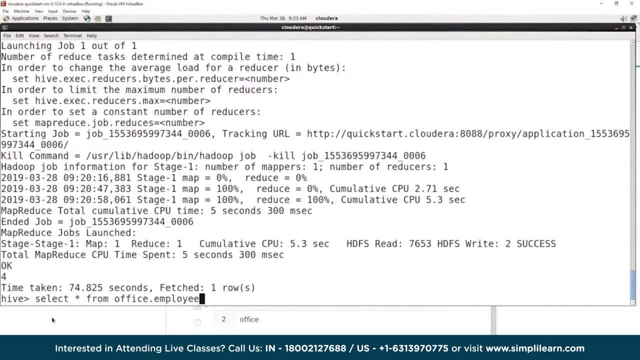 And either one will work on this particular one, because we have office set as a default on there. So from office employee and then the command where creates a subset and in this case we want to know where the salary is greater than 25,000.. 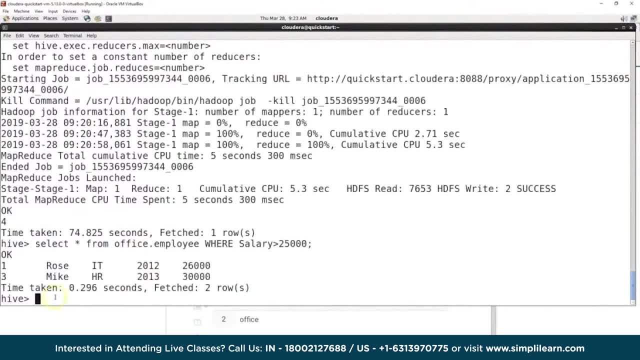 There we go and of course, we end with our semicolon And if we run this query, you can see it pops up and there's our salaries of people, top earners. We have Rose in IT and Mike in HR. 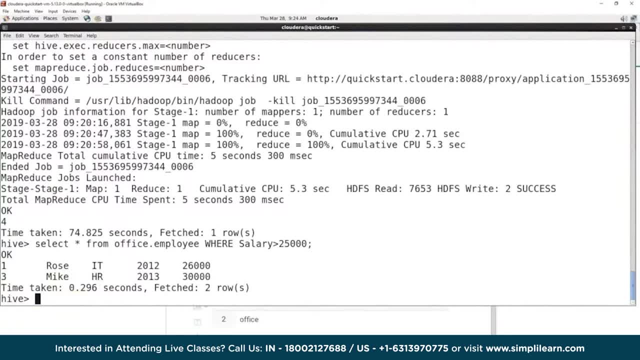 Kudos to them. of course, they're fictitional. I don't actually. we don't actually have a Rose and a Mike in those positions, or maybe we do. So, finally, what we want to go ahead and do is: we're done with this table. 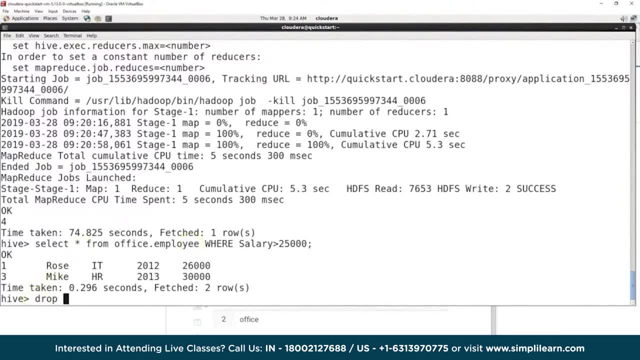 Now, remember you're dealing with a data warehouse, so you usually don't do a lot of dropping of tables and databases, but we're going to go ahead and drop this table here before we drop it. One more quick note is we can change it. 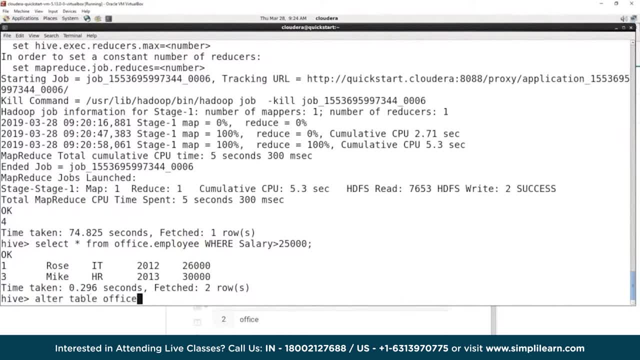 So what we're going to do is we're going to alter table office employee and we want to go ahead and rename it. There's some other commands you can do in here, but rename's pretty common And we're going to rename it to. 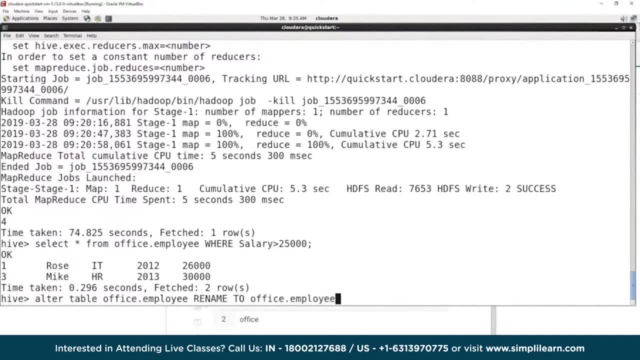 and it's going to stay in office. and it turns out one of our shareholders really doesn't like the word employee. he wants employees plural. it's a big deal to him, So let's go ahead and change that name for the table. 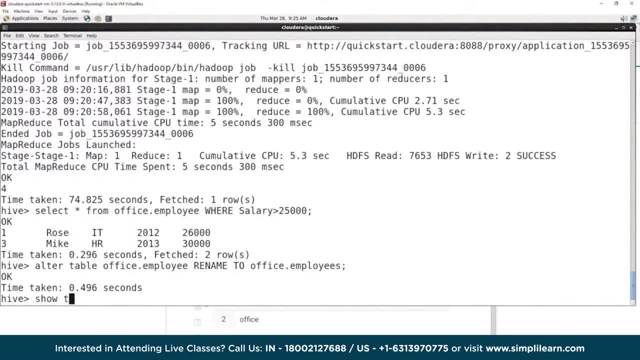 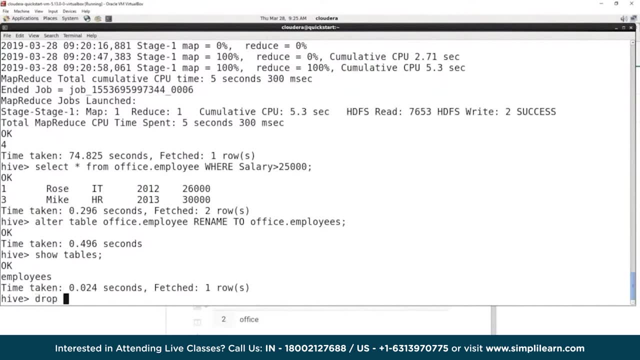 It's that easy because it's just changing the metadata on there. And now, if we do show tables, you'll see we now have employees, not employee, And then at this point maybe we're doing some house cleaning, because this is all practice. 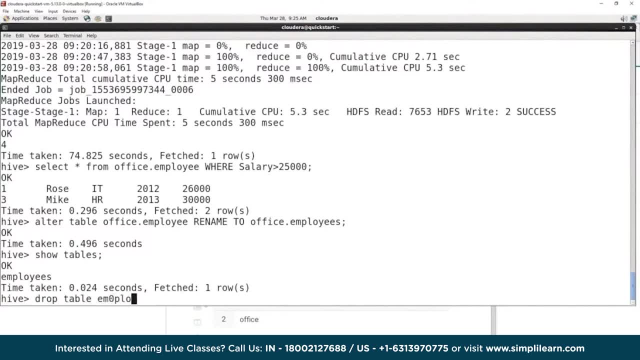 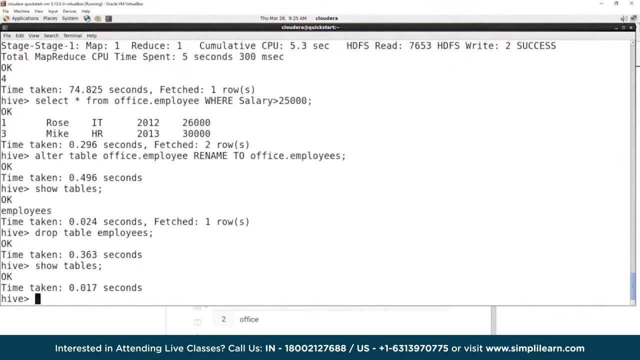 So we're going to go ahead and drop table and we'll drop table employees because we changed the name in there. So if we did employee it'd just give us an error. And now, if we do show tables, you'll see all the tables are gone. 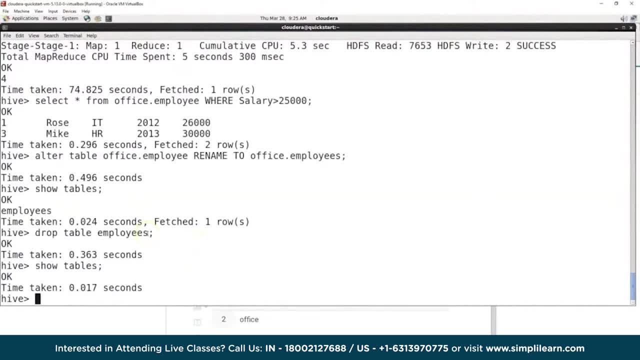 Now the next thing we want to go ahead and take a look at and we're going to walk back through the loading of data just real quick, because we're going to load two tables in here And let me just float back to our terminal window. 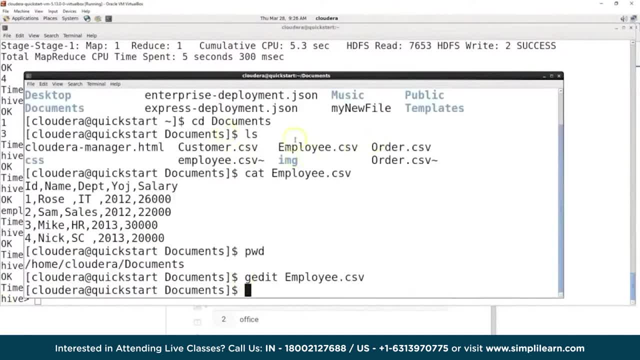 so we can see what those tables are that we're loading, And so up here we have a customer file and we have an order file. We want to go ahead and put the customers and the orders into here. So those are the two we're doing. 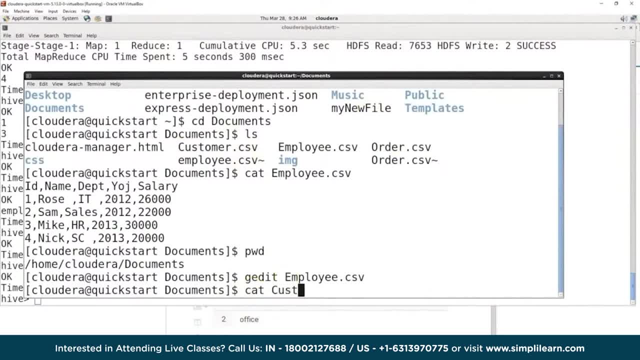 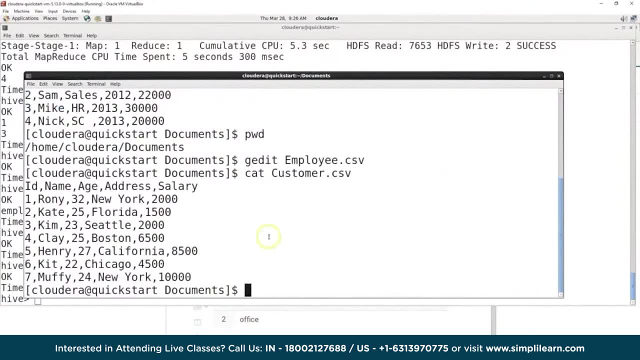 And, of course, it's always nice to see what you're working with. So let's do our cat customercsv. We could always do gedit, but we don't really need to edit these. We just want to take a look at the data in customer. 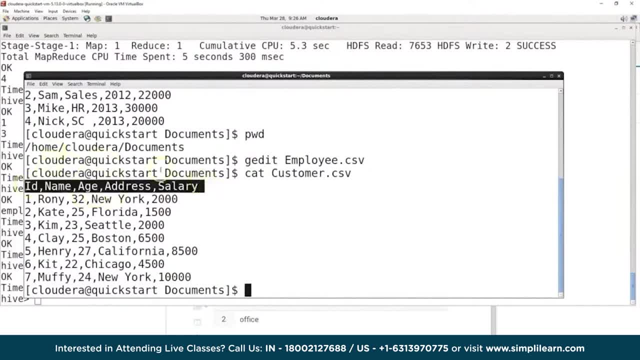 And important in here is again, we have a header, So we have to skip a line, comma separated. Nothing odd with the data. We have our schema, which is: oh, integer, string, integer, string, integer. So you'd want to take that, note, that down. 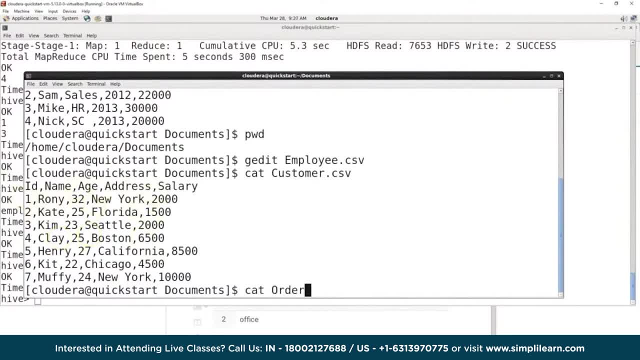 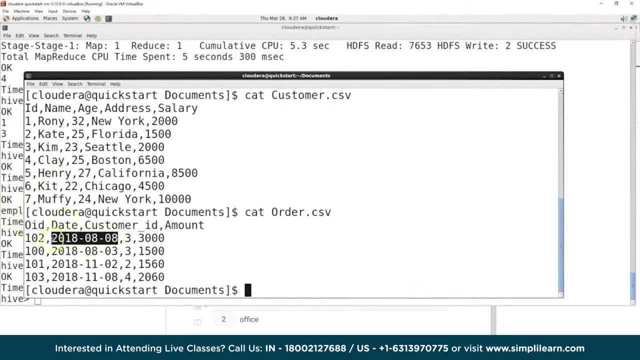 or flip back and forth when you're doing it. And then let's go ahead and do cat ordercsv And we can see we have OID, which I'm guessing is the order ID. We have a date- Something new. We've done integers and strings, but we haven't done date. 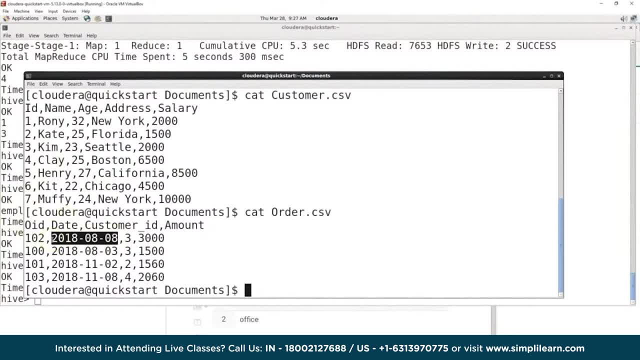 When you're importing new and you've never worked with the date. date's always one of the more trickier fields to port in, And that's true of just about any scripting language I've worked with. All of them have their own idea of how. 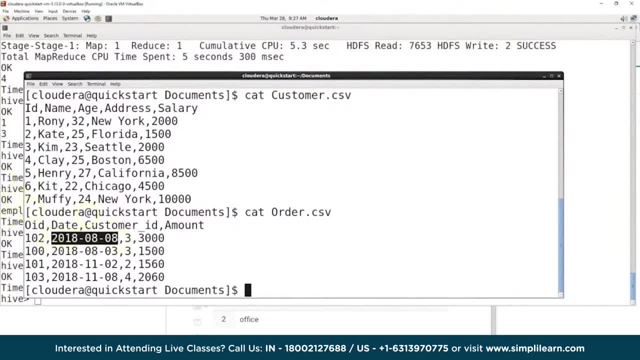 date's supposed to be formatted, what the default is. This particular format, where it's year and it has all four digits dash month, two digits dash day, is the standard import for the hive. So you'll have to look up and see. 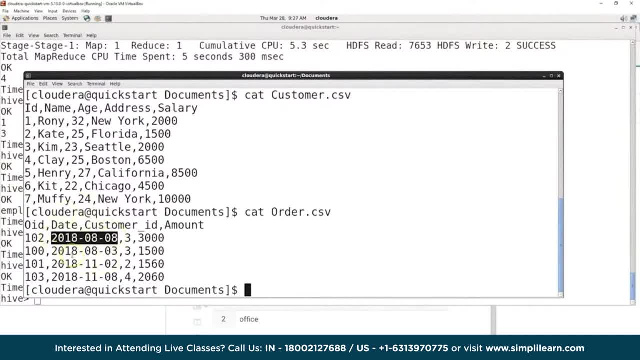 what the different formats are. if you're going to do a different format in there coming in or you're not able to pre-process the data, But this would be a pre-processing of the data thing coming in, If you remember correctly from our etl, which is e just. 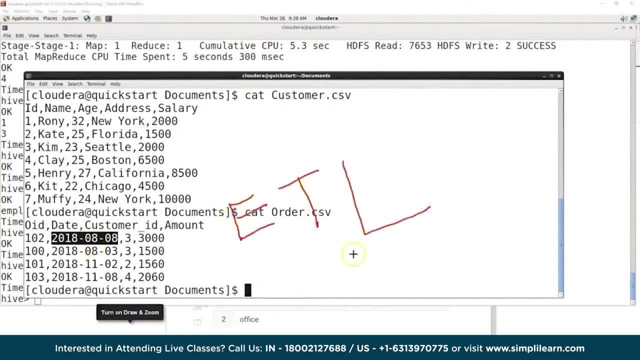 in case you weren't able to hear me last time- etl, which stands for extract, transform, then load. So you want to make sure you're transforming this data before it gets into here, And so we're going to go ahead and bring both this data in here. 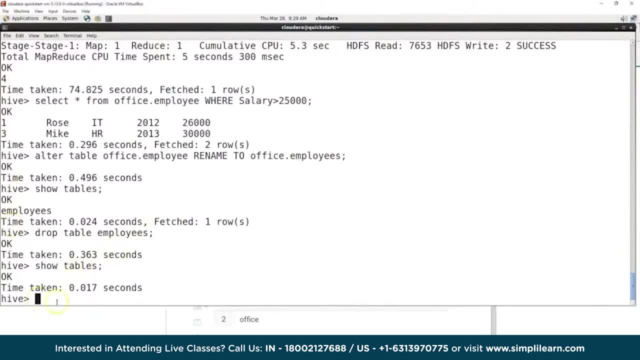 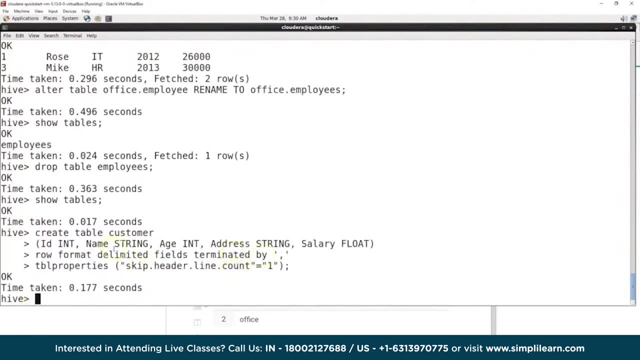 And really we're doing this so we can show you the basic join There is, if you remember from our setup: merge, join, all kinds of different things you can do, But joining different data sets is so common, So it's really important to know how to do this. 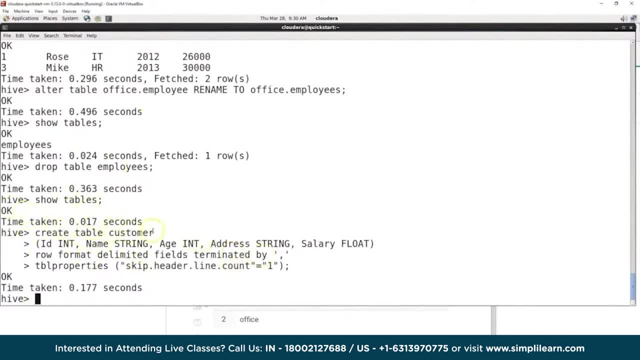 We need to go ahead and bring in these two data sets And you can see where I just created table customer. Here's our schema: the integer name, age, address, salary. Here's our delimited by commas, and our table properties. 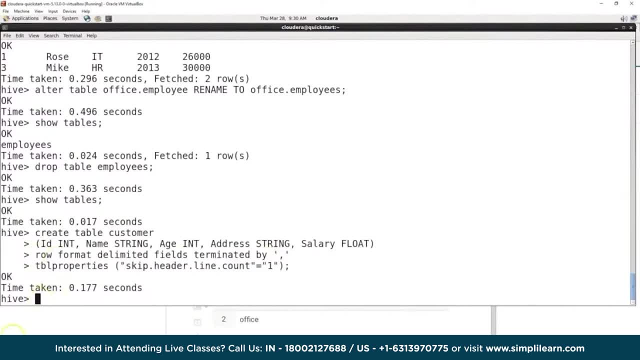 where we skip a line. Well, let's go ahead and load the data first, And then we'll do that with our order, And let's go ahead and put that in here, And I've got it split into three lines so you can see it easily. 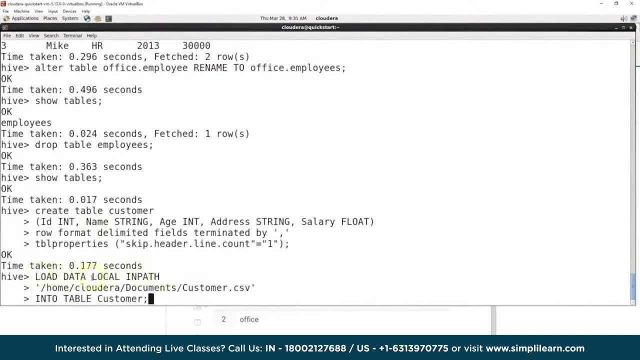 We've got load data local in path. So we know we're loading data, We know it's local And we have the path. Here's the complete path for oops. this is supposed to be order csv Grabbed the wrong one. 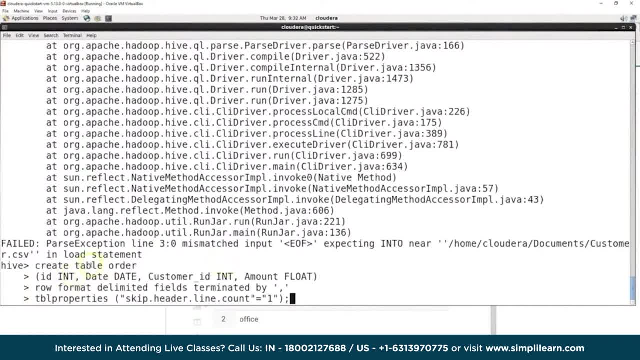 Of course it's going to give me errors because you can't recreate the same table on there. And here we go: Create table. Here's our integer date customer, the basic setup that we had coming in here for our schema. row format, commas. 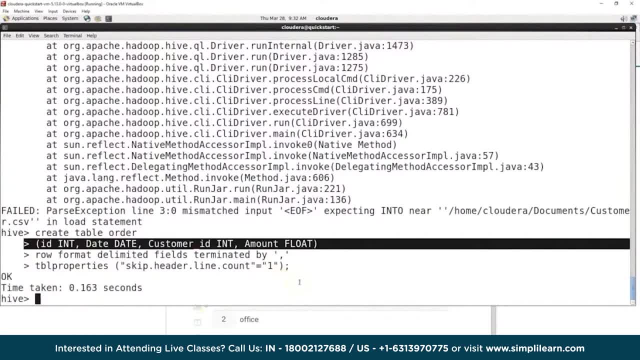 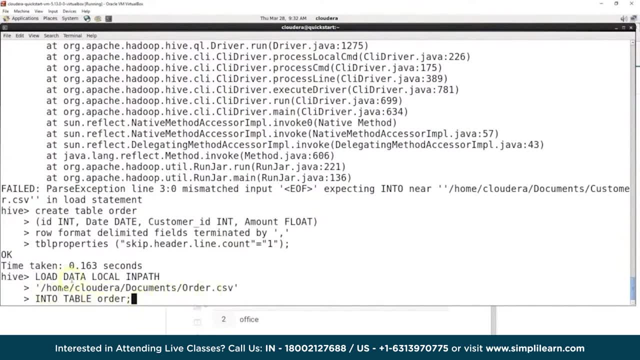 table properties. skip header line And then, finally, let's load the data into our order table. Load data local in path home, Cloudera documents, ordercsv- into table order. Now, if we did everything right, we should be able to do select star from customer. 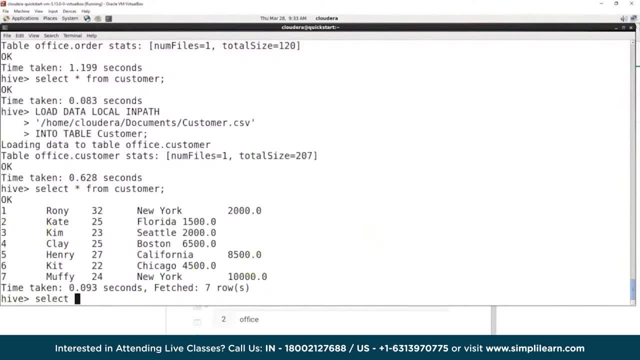 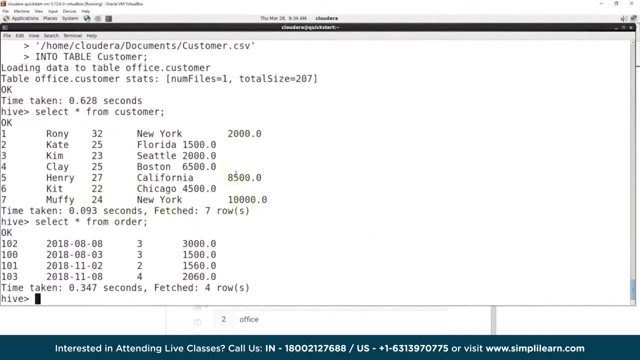 And you can see we have all seven customers. And then we can do select star from order And we have four orders. So this is just like a quick frame. We have a lot of times when you have your customer databases in business you have thousands of customers from years and years. 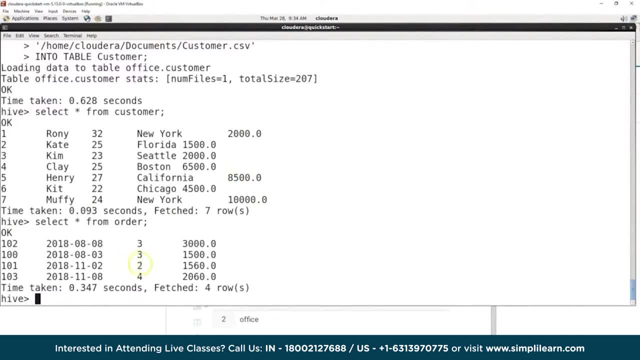 And some of them they close their business, They change names, All kinds of things happen. So what we want to do is we want to go ahead and find just the information connected to these orders and who's connected to them, And so let's go ahead. 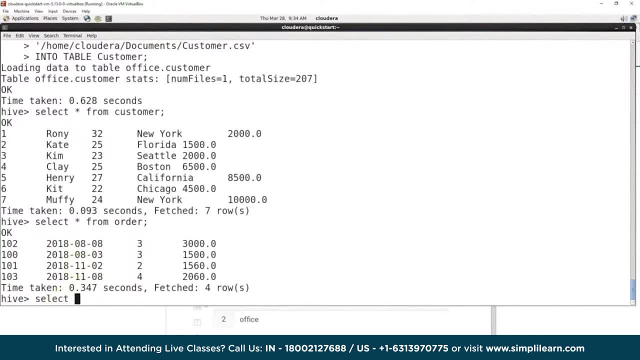 And do. it's a select because we're going to display information, So select, and this is kind of interesting. We're going to do cid And I'm going to define c as customer, as a customer table, in just a minute. 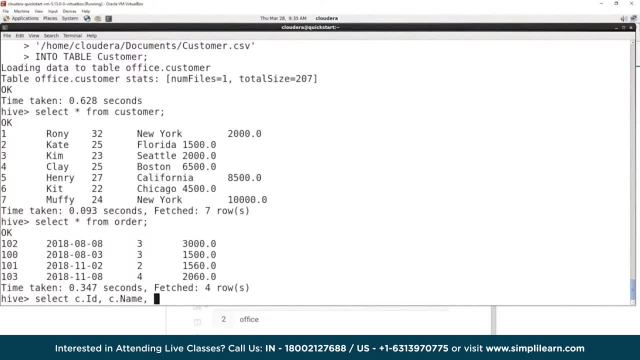 Then we're going to do cname And again we're going to define the c cage. So this means from the customer we want to know their ID, their name, their age, and then I'd also like to know the order amount. 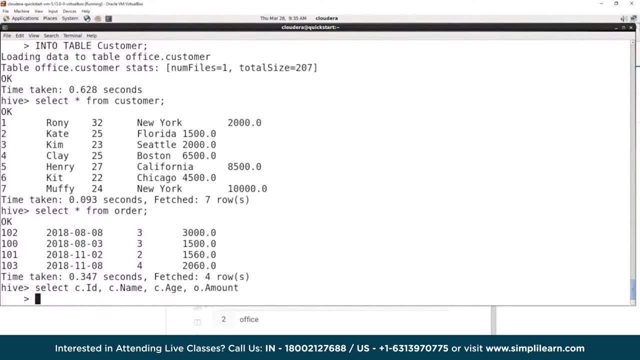 So let's do oamount, And then this is where we need to go ahead and define what we're doing, And I'll go ahead and capitalize from customer. So we're going to take the customer table in here And we're going to name it c. 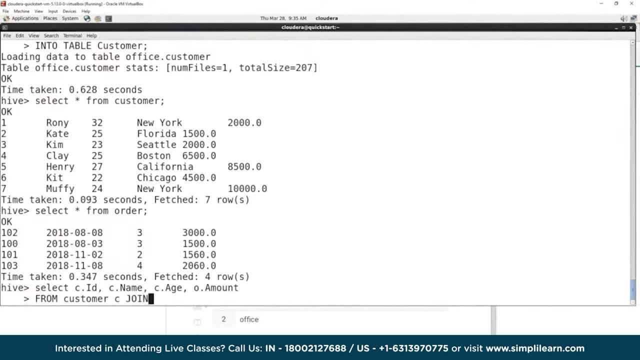 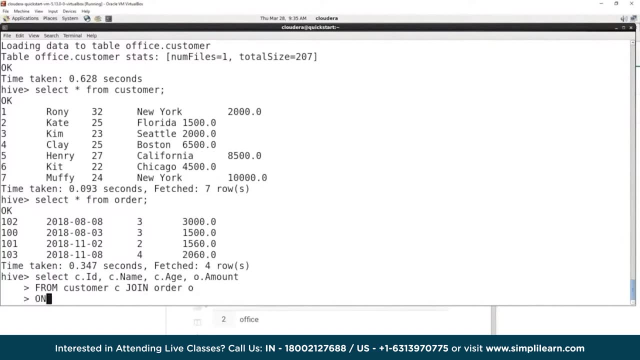 That's where the c comes from, So that's the customer table c And we want to join order as o. That's where our o comes from, So the oamount is what we're joining in there, And then we want to do this on. we've got to tell it. 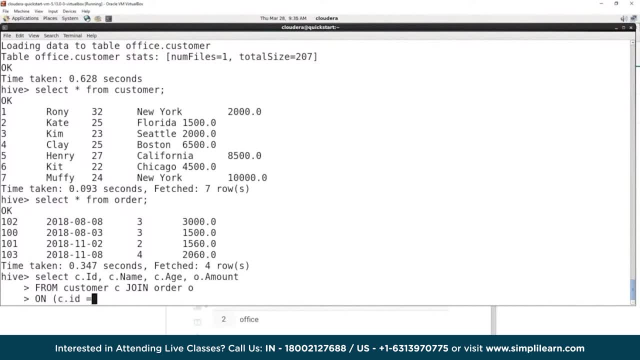 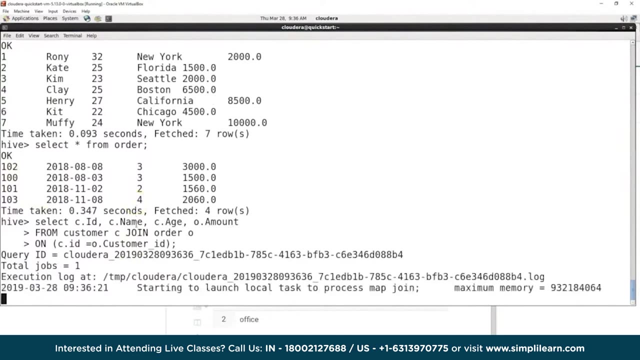 how to connect the two tables. cid equals ocustomer underscore id. So now we know how they're joined. And now remember, We have seven customers in here, We have four orders And, as it processes, we should get a return of four different names joined together. 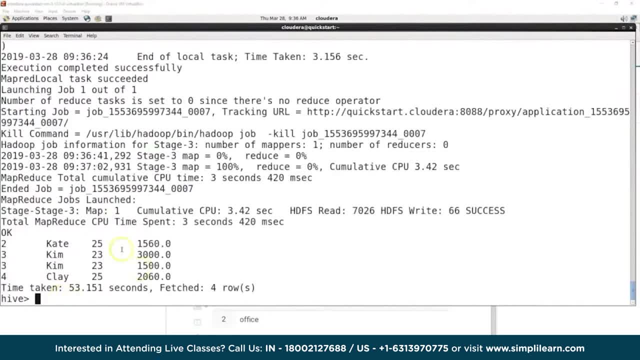 And they're joined based on, of course, the orders on there, And, once we're done, we now have the order number, the person who made the order, their age and the amount of the order which came from the order table. 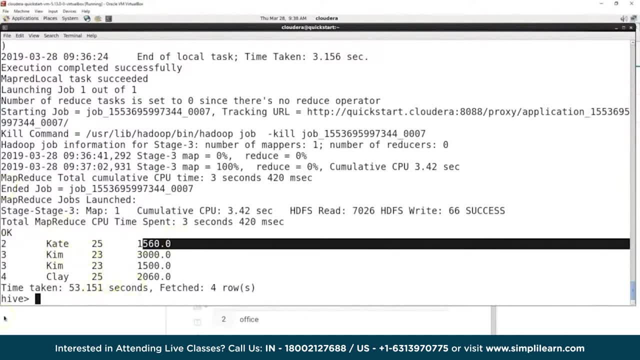 So you have your different information And you can see how the join works here. Very common use of tables in HQL and SQL. And let's do one more thing with our database, And then I'll show you a couple other Hive commands. 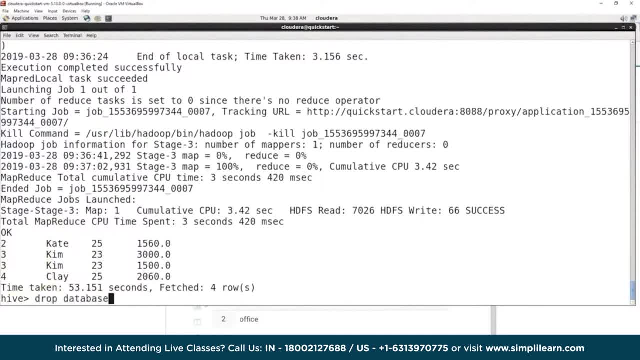 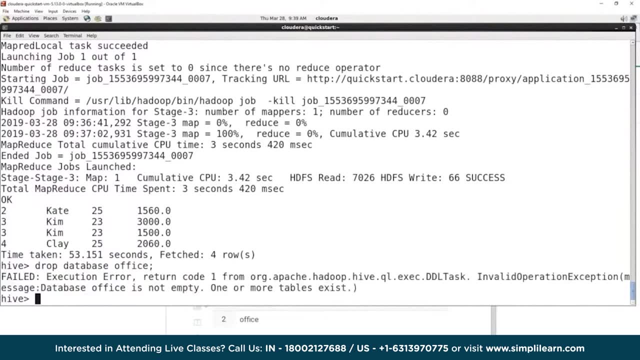 And let's go ahead and do a drop And we're going to drop database office And if you're looking at this and you remember from earlier, this will give me an error And let's just see what that looks like. It says: failed to execute. 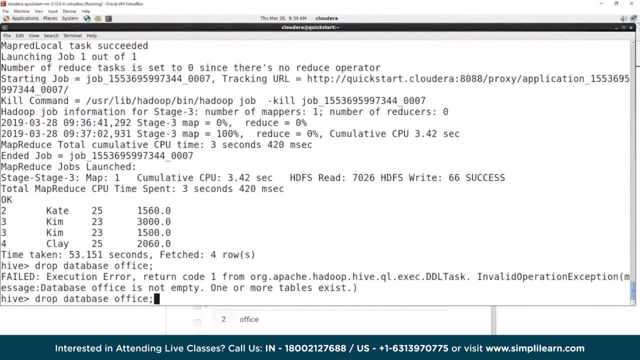 Exception, one or more tables exist. So if you remember from before, you can't just drop a database unless you tell it to cascade. That lets it know. I don't care how many tables are in it, let's get rid of it. 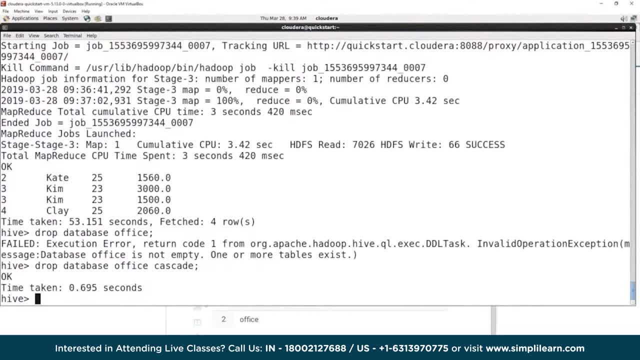 And in Hadoop, since it's a warehouse, a data warehouse- you usually don't do a lot of dropping. Maybe at the beginning, when you're developing the schemas and you realize you messed up, you might drop some stuff. But down the road you're really just. 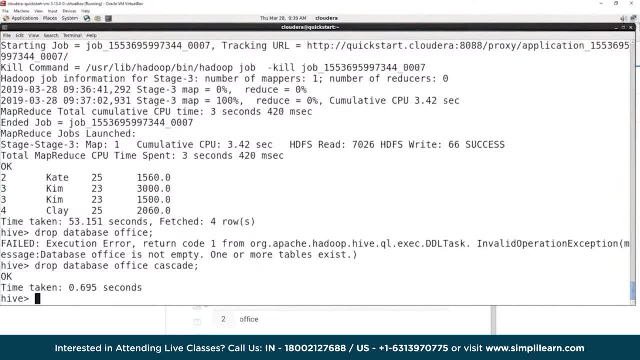 adding commodity machines to take up so you can store more stuff on it. So you usually don't do a lot of database dropping And some other fun commands to know is you can do select round 2.3 as round value. You can do a round off in Hive. 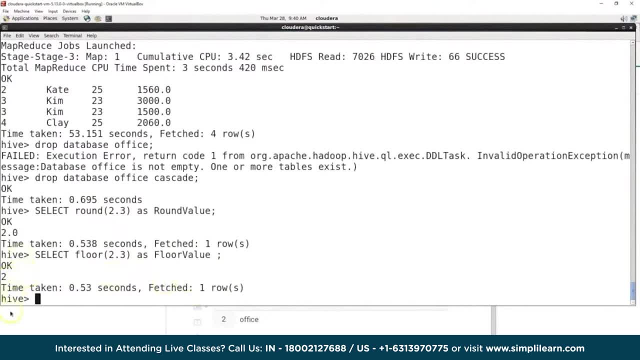 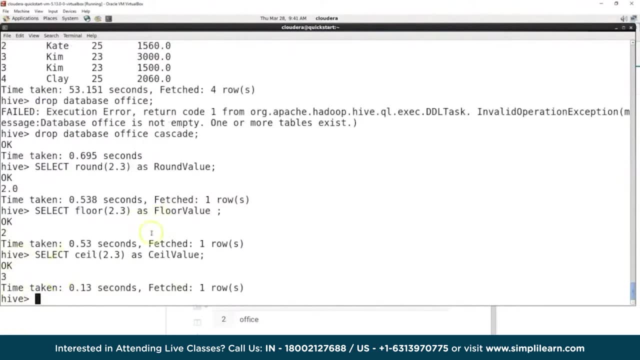 We can do as floor value, which is going to give us a 2. So it turns it into an integer versus a float. It goes down, basically truncates it, but it goes down, And we can also do ceiling, which is going to round it up. 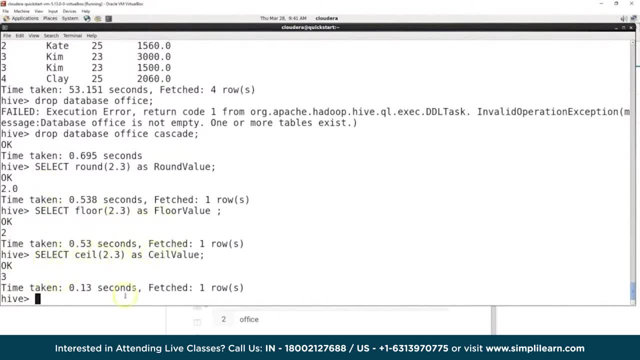 So we're looking for the next integer. above There's a few commands we didn't show in here because we're on a single node. As an admin, to help speedy the process, you usually add in partitions for the data and buckets. You can't do that on a single node because when you add 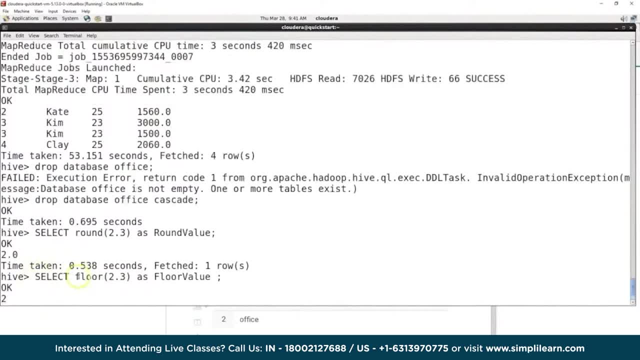 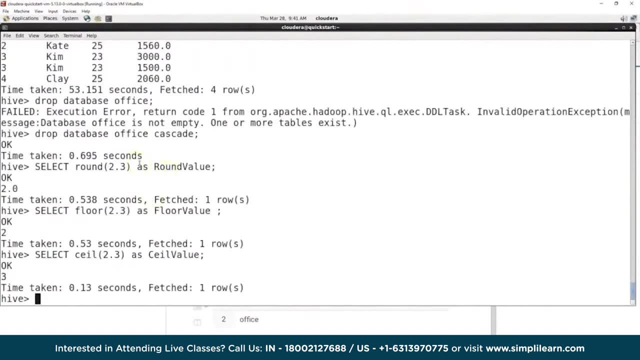 a partition. it partitions it across separate nodes, But beyond that you can see that it's very straightforward. We have SQL coming in And all your basic queries that are in SQL are very similar to HQL. Let's get started with PIG. 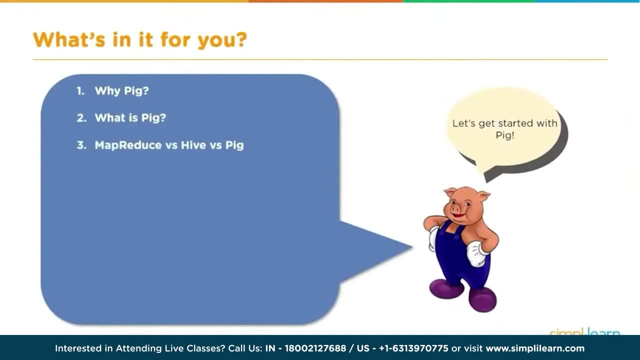 Why PIG? What is PIG? MapReduce versus Hive versus PIG. Hopefully you've had a chance to do our Hive tutorial and our MapReduce tutorial. If you haven't, send a note over to Simply Learn and we'll follow up with a link to you. 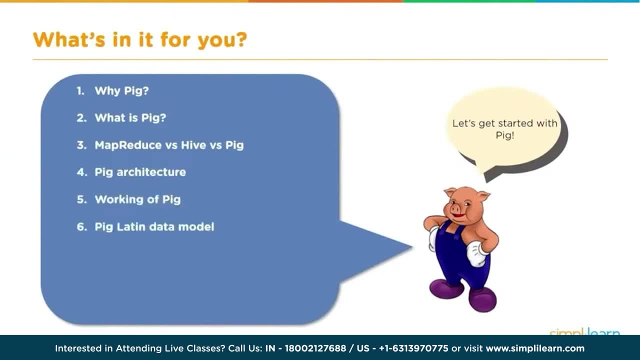 We'll look at PIG architecture, working, a PIG, PIG Latin data model, PIG execution modes, a use case, Twitter and features of PIG, And then we'll tag on a short demo so you can see PIG in action. 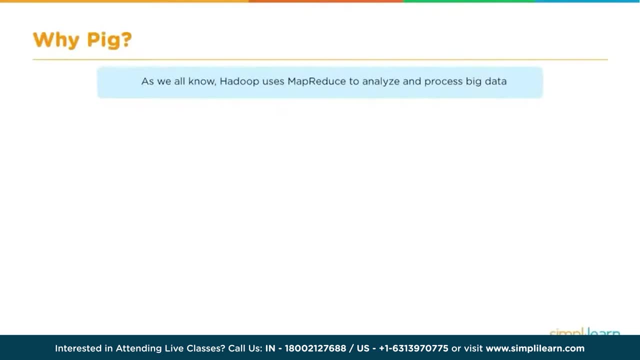 So why PIG? As we all know, Hadoop uses MapReduce to analyze and process big data. Processing big data consumed more time, So before we had the Hadoop system, they'd have to spend a lot of money on a huge set of computers and enterprise machines. 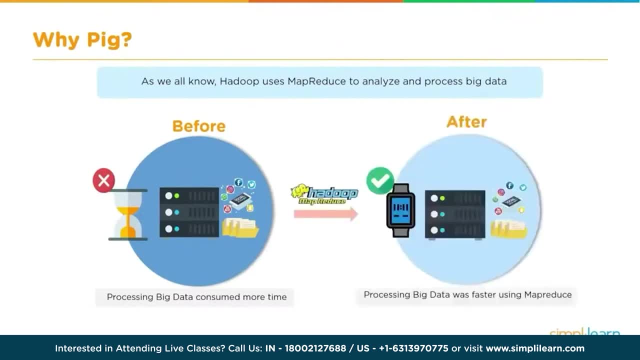 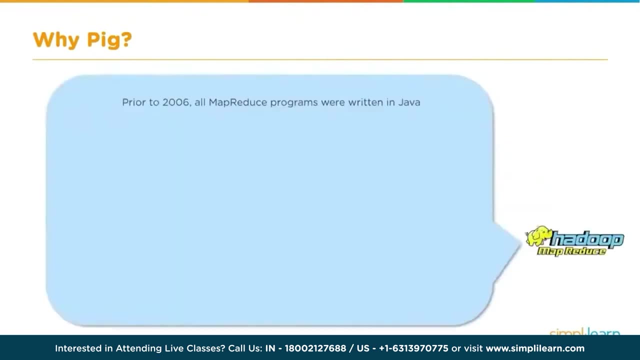 So we introduced the Hadoop MapReduce, And so afterwards processing big data was faster using MapReduce. Then what is the problem with MapReduce? Prior to 2006,, all MapReduce programs were written in Java. Non-programmers found it difficult. 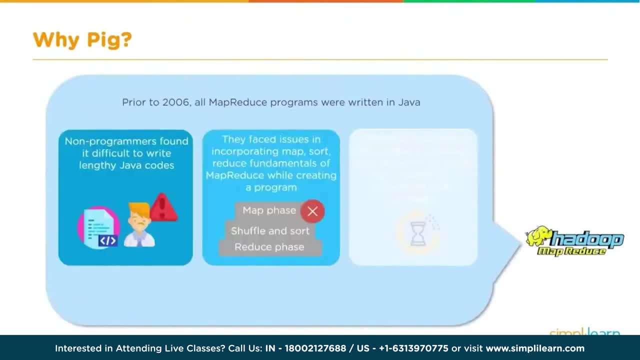 to write lengthy Java codes. They faced issues in incorporating MapSortReduce to fundamentals of MapReduce while creating a program. You can see here MapPhase, Shuffle and SortReduce phase. Eventually it became a difficult task to maintain and optimize a code. 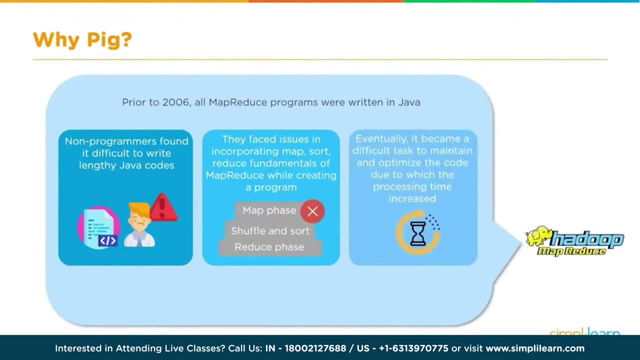 due to which the processing time increased. You can imagine a manager trying to go in there and needing a simple query to find out data, and he has to go talk to the programmers anytime he wants anything, So that was a big problem. Not everybody wants to have a on-call programmer. 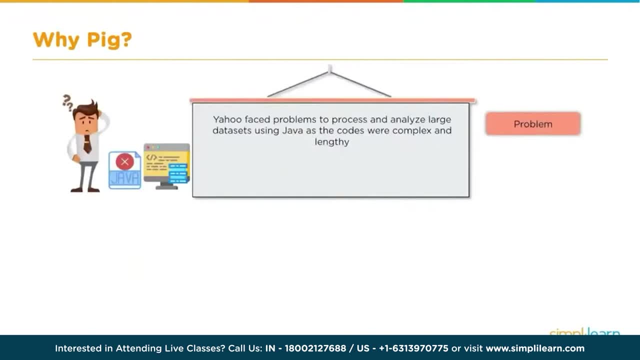 for every manager on their team. Yahoo faced problems to process and analyze large data sets using Java, as the codes were complex and lengthy. There was a necessity to develop an easier way to analyze large data sets without using time-consuming complex Java modes and codes and scripts. and all of that. 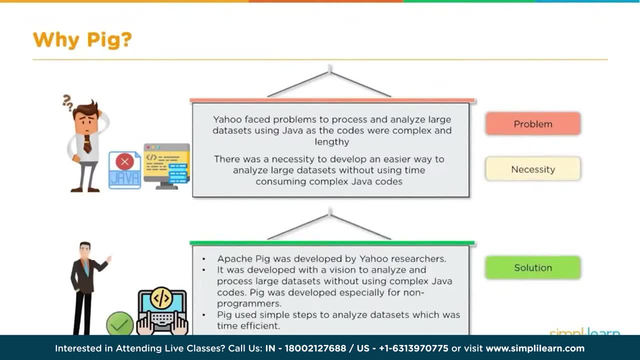 So the problem with MapReduce was that the code was too complex and lengthy. All that fun stuff. Apache Pig was developed by Yahoo. It was developed with the vision to analyze and process large data sets without using complex Java codes. Pig was developed especially for non-programmers. 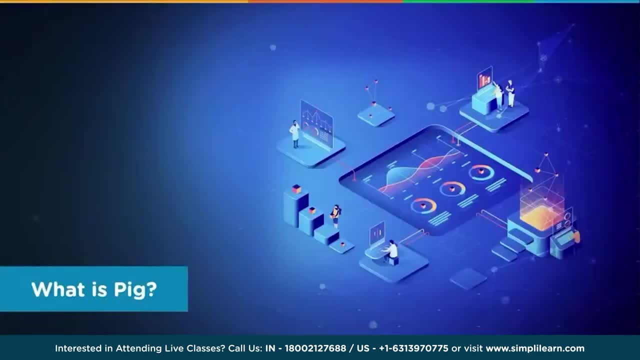 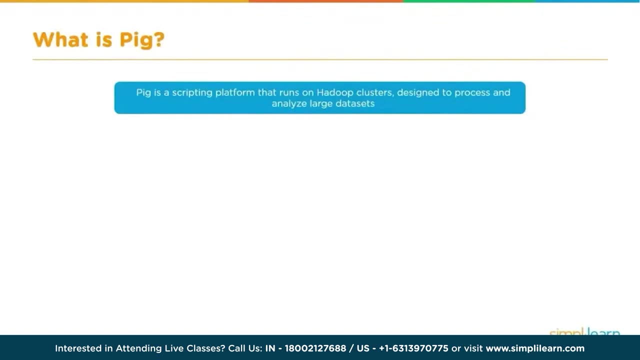 Pig used simple steps to analyze data sets, which was time-efficient. So what exactly is Pig? Pig is a scripting platform that runs on Hadoop clusters, designed to process and analyze large data sets. And so you have your Pig, which uses SQL-like queries. 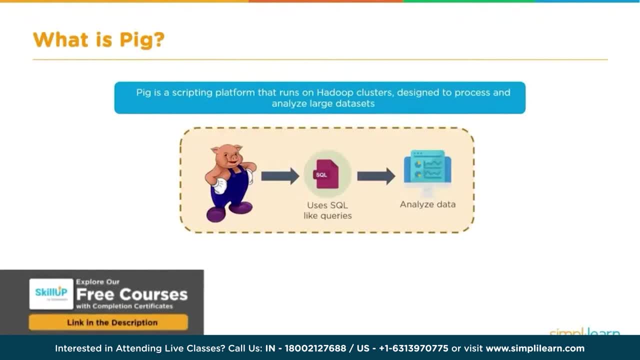 They're definitely not SQL, But some of them resemble SQL queries And then we use that to analyze our data. Pig operates on various types of data, like structured, semi-structured and unstructured data. Let's take a closer look at MapReduce versus Hive versus Pig. 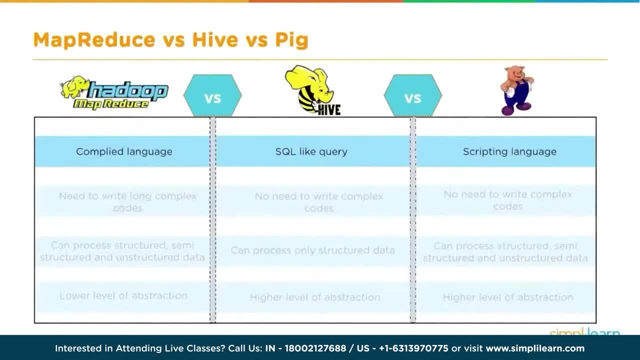 So we start with a compiled language, your MapReduce, And we have Hive, which is your SQL-like query, And then we have Pig, which is a scripting language. It has some similarities to SQL, but it has a lot of its own stuff. 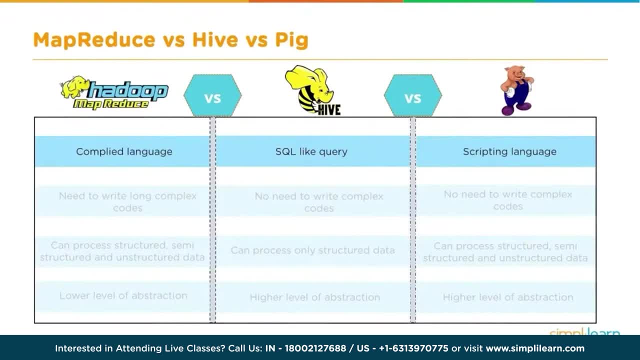 Remember, SQL-like query, which is what Hive is based off, looks for structured data, And so when you get into scripting languages like Pig now we're dealing more with semi-structured and even unstructured data With a Hadoop MapReduce, we have a need to write long, complex codes. 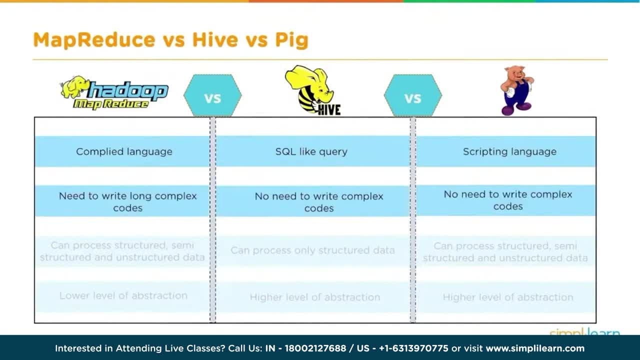 With Hive, no need to write complex codes. You could just put it in a simple SQL query or HQL, HiveQL. And in Pig- no need to write complex codes as we have Pig Latin Now, remember- in the MapReduce it can produce structured. 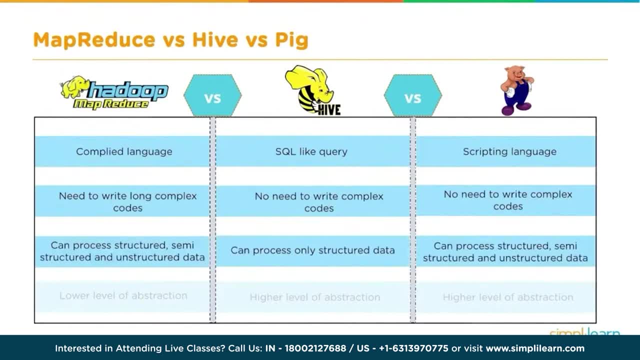 semi-structured and unstructured data And, as I mentioned before, Hive can process only structured data. Think rows and columns, Where Pig can process structured, semi-structured and unstructured data. You can think of structured data as rows and columns. 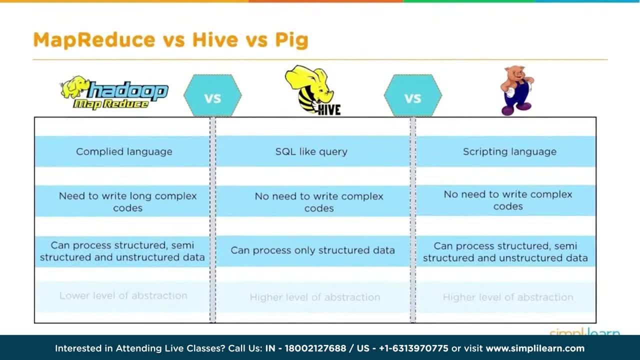 semi-structured as your HTML XML documents that you have on your web pages, And unstructured could be anything from groups of documents and written format Twitter tweets. any of those things come in as very unstructured data And with our Hadoop MapReduce we have a lower level. 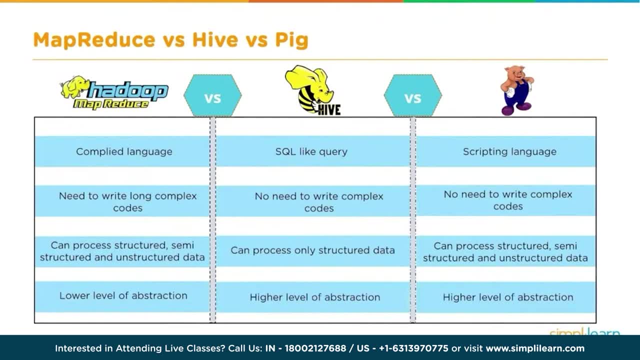 abstraction. With both Hive and Pig we have a higher level abstraction, So it's much more easy for someone to use without having to dive in deep and write a very lengthy MapReduce code, And those Map and Reduce codes can take 70, 80 lines of code. 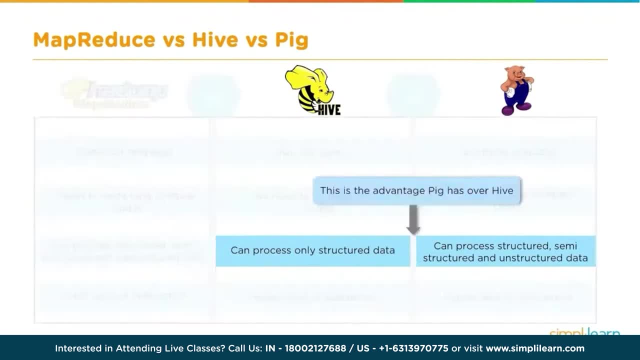 when you can do the same thing in one or two lines with Hive or Pig. This is the advantage Pig has over Hive: It can process only structured data in Hive, while in Pig it can process structured, semi-structured and unstructured data. 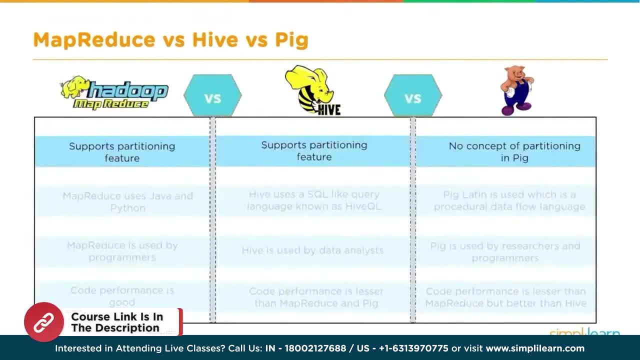 Some other features. to note that separates the different query languages is when we look at Map and Reduce. MapReduce supports partitioning features, as does Hive Pig- no concept of partitioning in Pig- so it doesn't support your partitioning feature. 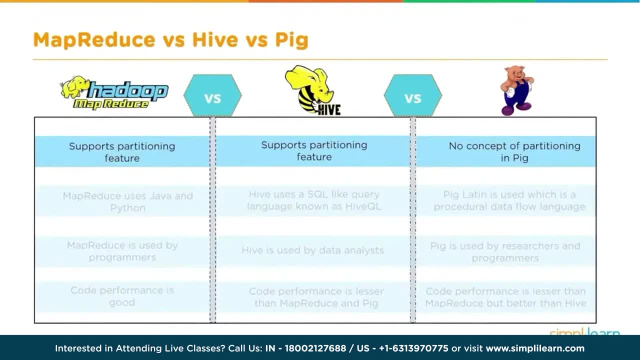 Your partitioning features allow you to partition the data in such a way that it can be queried quicker. You're not able to do that in Pig. MapReduce uses Java and Python, while Hive uses an SQL-like query language known as HiveQL or HQL. 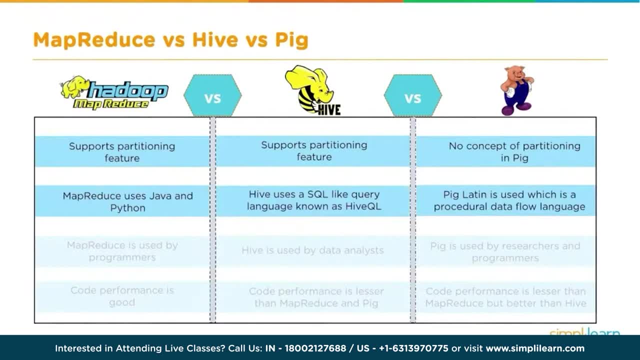 Pig, Latin is used, which is a procedural data flow language. MapReduce is used by programmers, pretty much as straightforward on Java. Hive is used by data analysts. Pig is used by researchers and programmers. Certainly there's a lot of mix between all three. 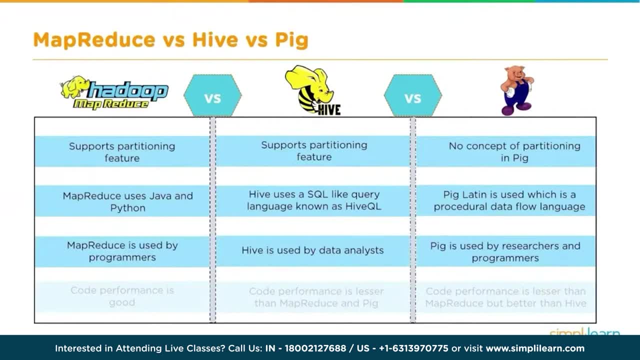 Programmers have been known to go in and use a Hive for a quick query and anybody's been able to use Pig for a quick query or research. Under Map and Reduce code performance is really good. Under Hive, code performance is lesser than Map and Reduce and Pig. 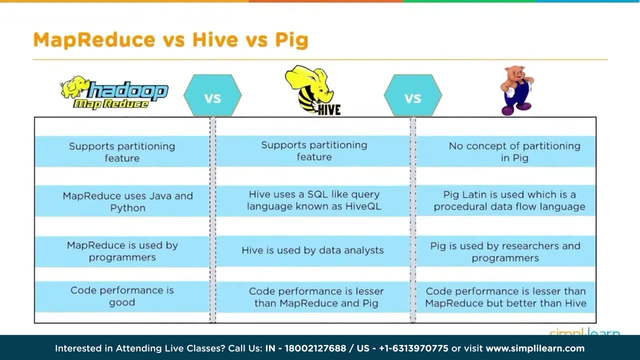 Under Pig code performance is lesser than MapReduce but better than Hive. So if we're going to look at speed and time, the MapReduce is going to be the fastest performance on all of those where Pig will have second and Hive follows in the back. 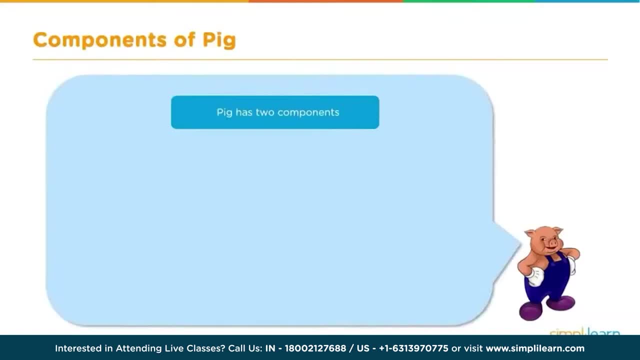 Let's look at components of Pig. Pig has two main components. We have Pig Latin. Pig Latin is a procedural data flow language used in Pig to analyze data. It is easy to program using Pig Latin. It is similar to SQL. And then we have the runtime engine. 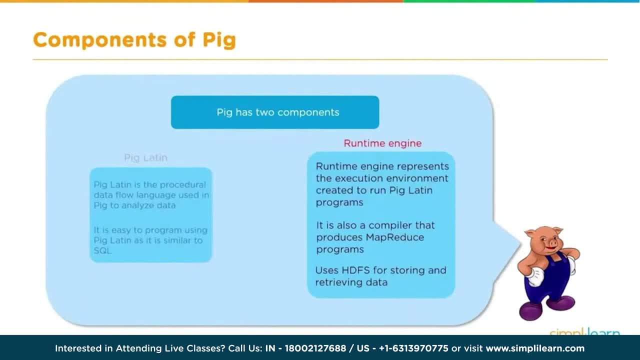 Runtime engine represents the execution environment created to run Pig Latin programs. It is also a compiler. It is a compiler that produces MapReduce programs. It uses HDFS or your Hadoop file system for storing and retrieving data. And as we dig deeper into the Pig architecture, 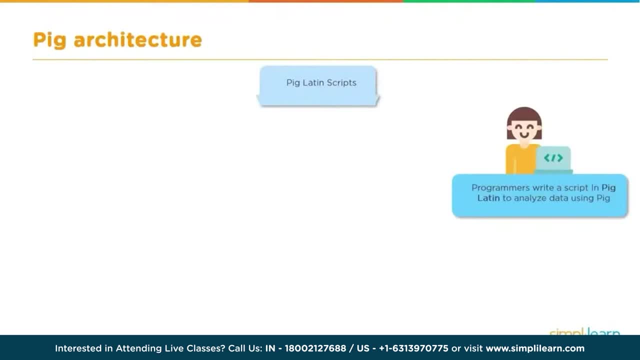 we'll see that we have Pig Latin scripts. Programmers write a script in Pig Latin to analyze data using Pig. Then you have the grunt shell And it actually says grunt when we start it up, and we'll show you that here in a little bit. 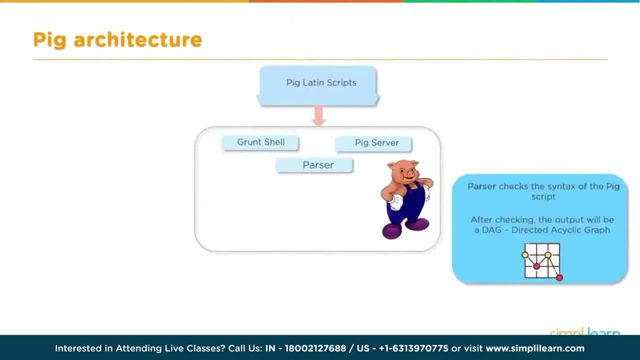 which goes into the Pig server, And this is where we have our parser. Parser checks the syntax of the Pig script. After checking, the output will be a DAG directed and a helix graph. And then we have an optimizer which optimizes after your DAG. 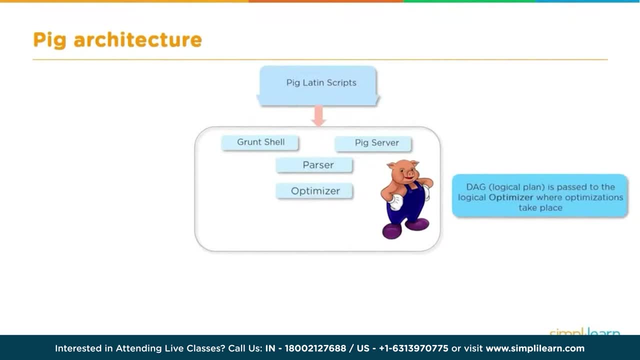 your logical plan is passed to the logical optimizer, where an optimization takes place. Finally, the compiler converts the DAG into MapReduce jobs And then that is executed on the MapReduce under the execution engine. The results are displayed using dump statement and stored in HDFS using store statement. 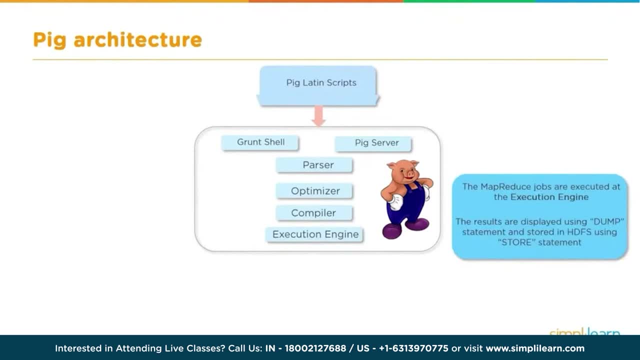 And again we'll show you that The kind of end you always want to execute everything once you've created it, And so dump is kind of our execution statement And you can see right here, as we were talking about earlier, once we get to the execution engine. 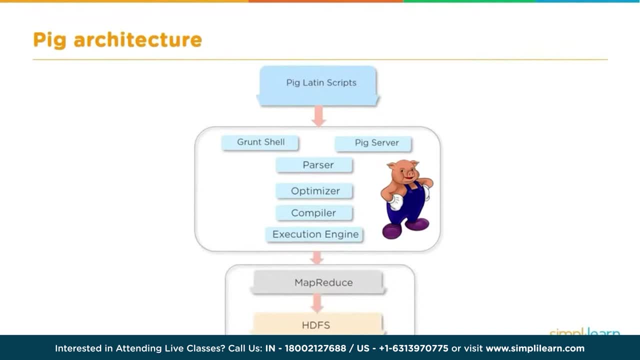 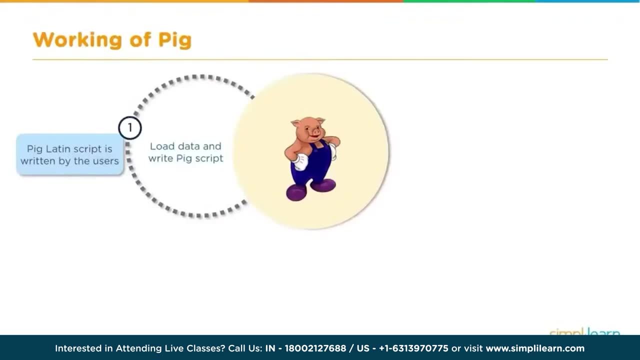 and it's coded into MapReduce. then the MapReduce processes it onto the HDFS Working of Pig. Pig Latin script is written by the users. So you have load data and write Pig script and Pig operations. So when we look at the working of Pig, 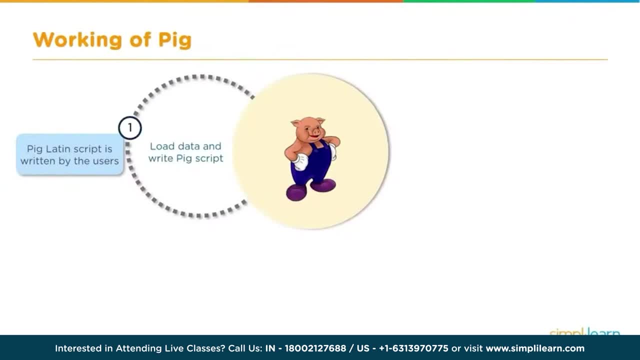 Pig Latin script is written by the users. There's step one- we load data and write Pig script, And step two. in this step all the Pig operations are performed by parser, optimizer and compiler. So we go into the Pig operations. 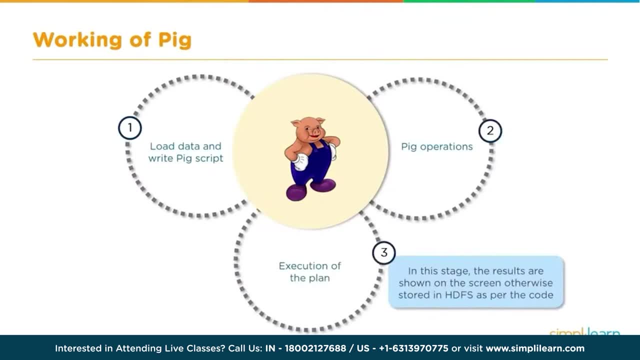 And then we get to step three: execution of the plan. In this stage the results are shown on the screen, otherwise stored in the HDFS as per the code. So it might be of a small amount of data. you're reducing it to. 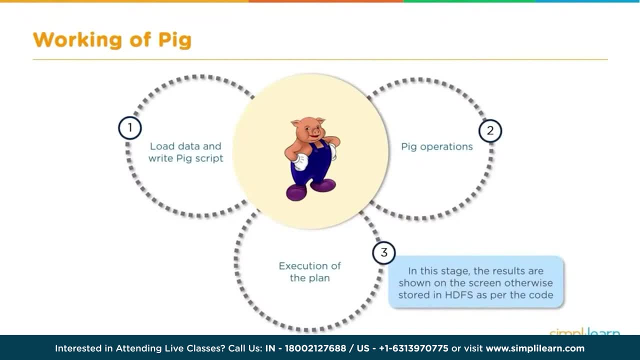 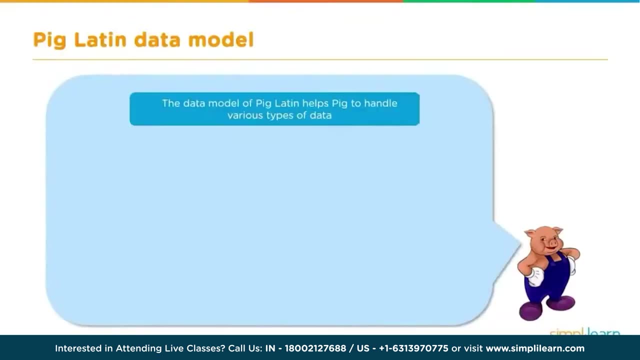 and you want to put that on the screen, or you might be converting a huge amount of data which you want to put back into the Hadoop file system for other use. Let's take a look at the Pig Latin data model. The data model of Pig Latin. 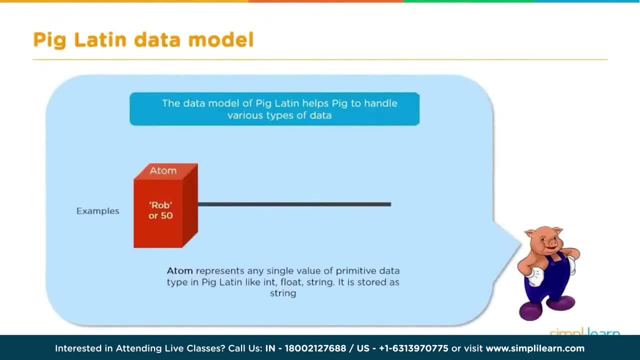 helps Pig to handle various types of data. For example, we have Adam, Rob or 50. Adam represents any single value of primitive data type in Pig Latin, like integer, float string, It is stored as a string Tuple. so we go from our Adam. 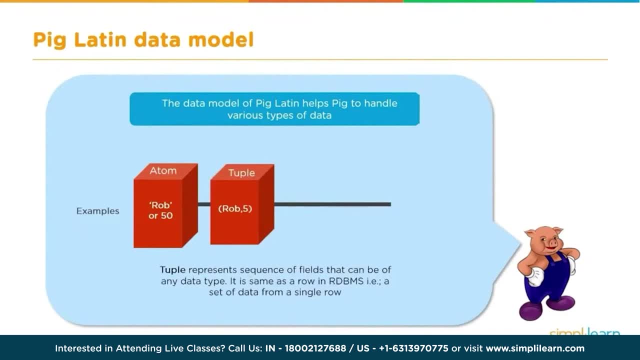 which our most basic thing. So if you look at just Rob or just 50, that's an Adam. That's our most basic object we have in Pig Latin. Then you have a tuple. Tuple represents sequence of fields that can be of any data type. 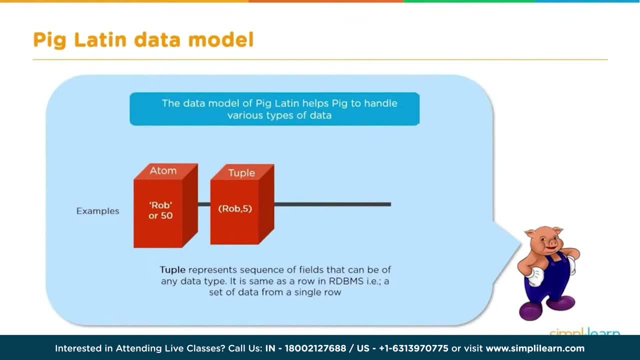 It is the same as a row in RDBMS, For example, a set of data from a single row. You can see here we have Rob, comma five, And you can imagine with many of our other examples we've used. you might have the ID number. 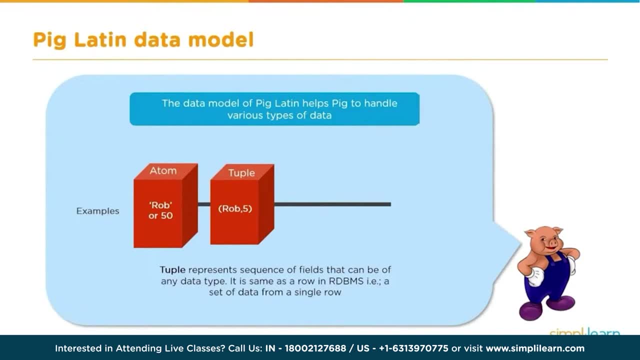 the name where they live, their age, their date of starting the job. That would all be one row and stored as a tuple. And then we create a bag. A bag is a collection of tuples. It is the same as a table in RDBMS. 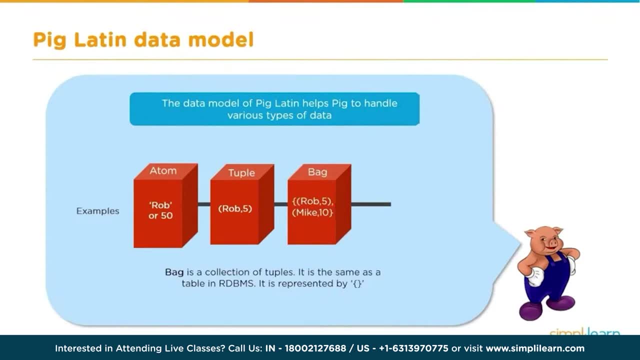 and is represented by brackets, And you can see, here we have our table with Rob five, Mike 10.. And we also have a map. A map is a set of key value pairs. Key is of character array, type and a value can be of any type. 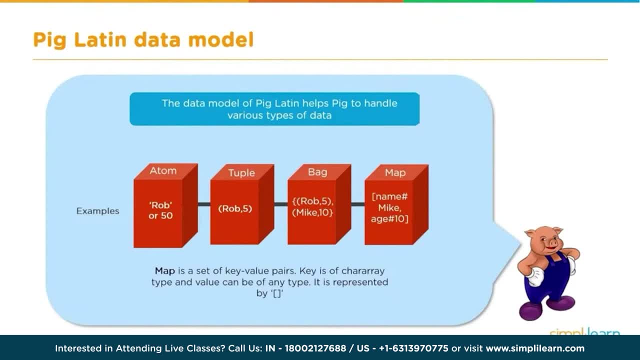 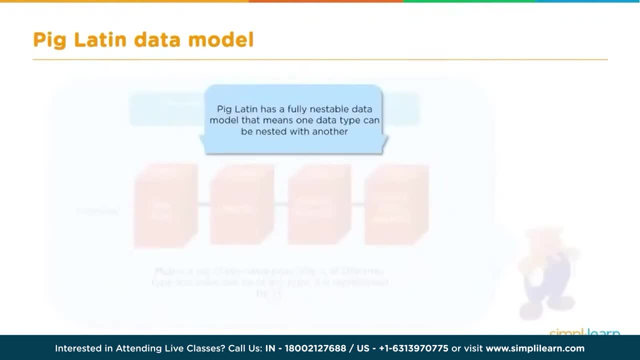 It is represented by the brackets, And so we have name and age, where the key value is Mike and 10.. Pig Latin has a fully nestable data model. That means one data type can be nested within another. Here's a diagram representation of Pig Latin data model. 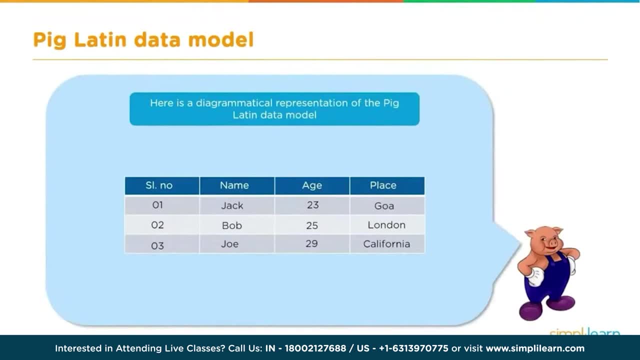 And in this particular example, we have basically an ID number, a name, an age and a place, And when we break this apart, we look at this model from a Pig Latin perspective. We start with our field And, if you can remember, 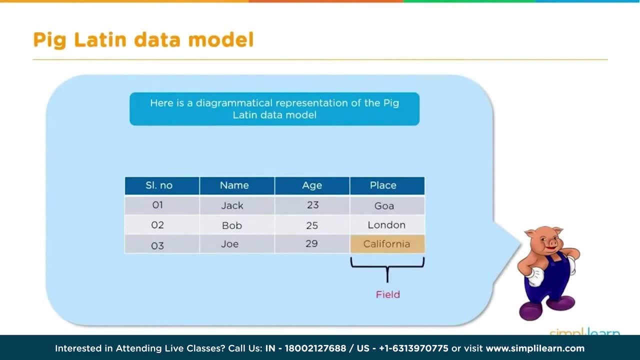 a field contains basically an atom. It is one particular data type, And the atom is stored as a string, which then converts it into either an integer number or character string. Next we have our tuple, And in this case you can see that it represents a row. 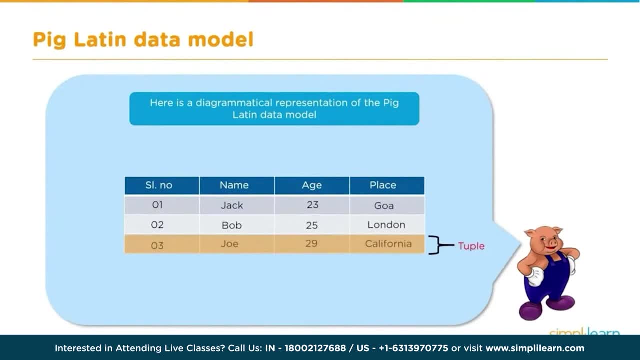 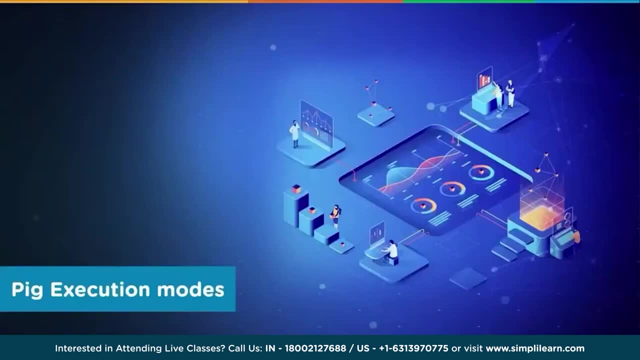 So our tuple would be: three comma Joe comma 29 comma California. And finally we have our bag, which contains three rows in it. in this particular example, Let's take a quick look at some of the execution modes. Pig works in two execution modes. 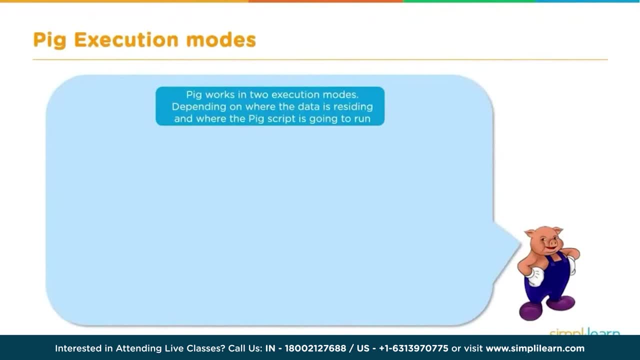 depending on where the data is reciting and where the Pig script is going to run. We have local mode Here. the Pig engine takes input from the Linux file system and the output is stored in the same file system- Local mode. Local mode is useful in analyzing small data sets using Pig. 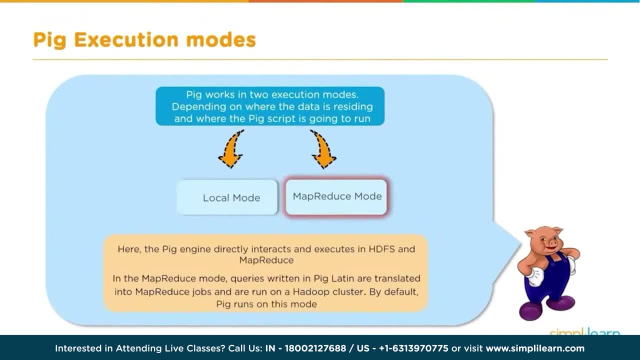 And we have the MapReduce mode. Here the Pig engine directly interacts and executes in HDFS and MapReduce. In the MapReduce mode, queries written in Pig Latin are translated into MapReduce jobs in a run on a Hadoop cluster. By default Pig runs in this mode. 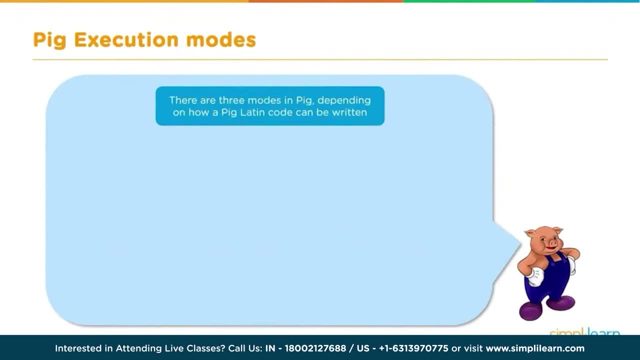 There are three modes in Pig, depending on how a Pig Latin code can be written. We have our interactive mode, batch mode and embedded mode. The interactive mode means coding and executing the script line by line. When we do our example, we'll be in the interactive mode. 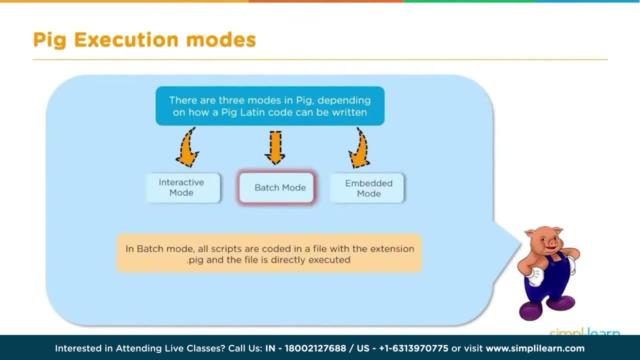 In batch mode, all scripts are coded in a file with the extension pig, and the file is directly executed. And then there's embedded mode. Pig lets its users define their own functions- UDFSs in a programming language such as Java. 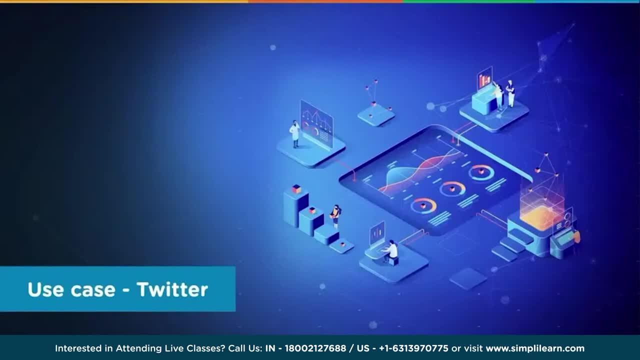 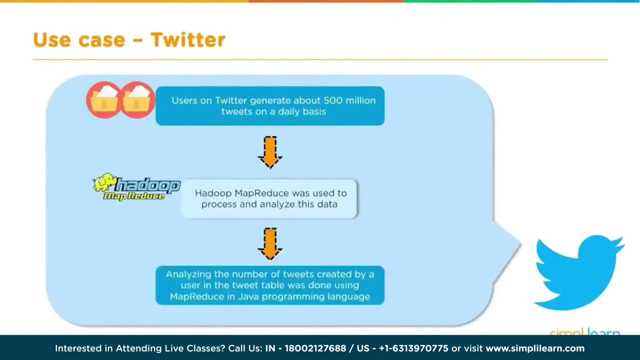 So let's take a look and see how this works in a use case. In this case, use case Twitter. Users on Twitter generate about 500 million tweets on a daily basis. The Hadoop MapReduce was used to process and analyze this data. 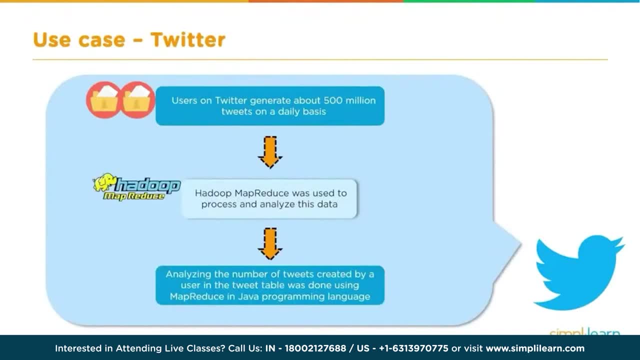 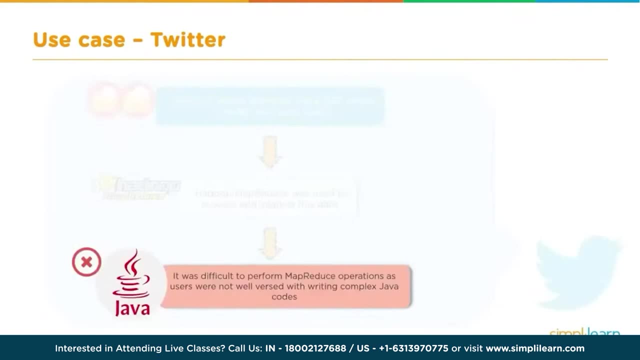 Analyzing the number of tweets created by a user in the tweet table was done using MapReduce and Java programming language, And you can see the problem. It was difficult to perform MapReduce operations because users were not well versed with written, complex Java codes. 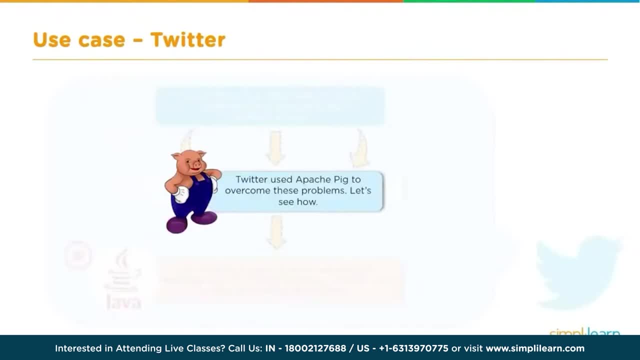 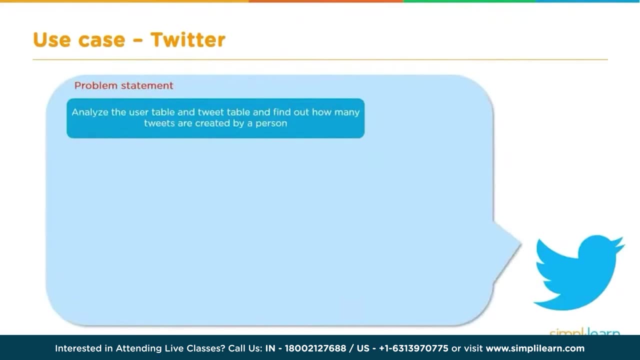 So Twitter used Apache Pig to overcome these problems, And let's see how. Let's start with the problem statement. Analyze the user table and tweet table and find out how many tweets are created by a person, And here you can see we have a user table. 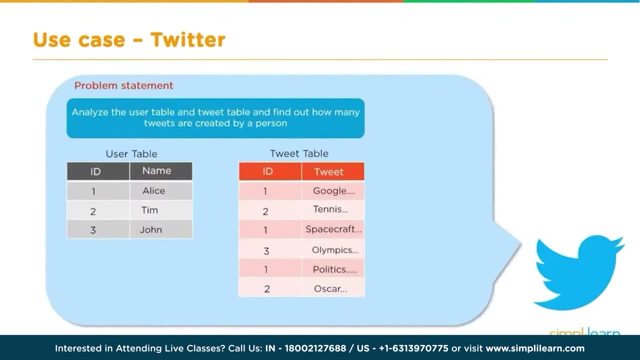 We have Alice, Tim and John with their ID, numbers One, two, three And we have a tweet table. In the tweet table you have the ID of the user and then what they tweeted. Google was a good, whatever it was. 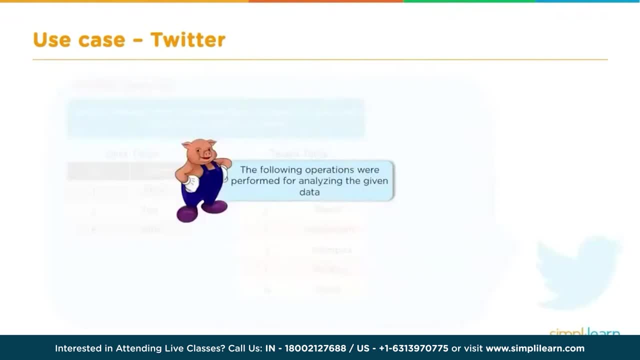 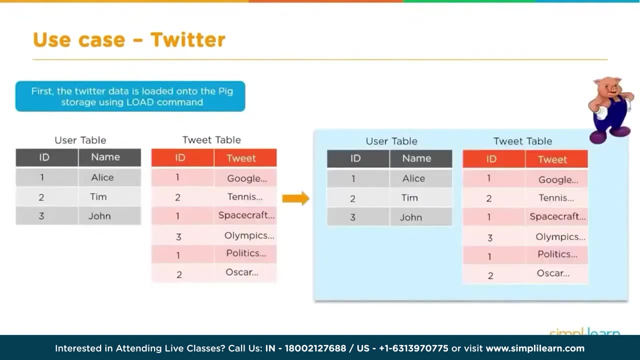 Olympics, politics, whatever they're tweeting about. The following operations were performed for analyzing given data: First, the Twitter data is loaded into the pig storage using load command And you can see here we have our data coming in and then that's going into pig storage. 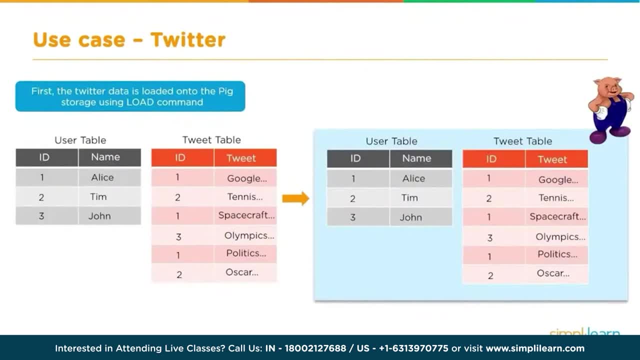 And this data is probably on an enterprise computer, So this is actually active Twitter's going on. and then it goes into Hadoop file system. Remember, the Hadoop file system is a data warehouse for storing data, And so the first step is: we want to go ahead. 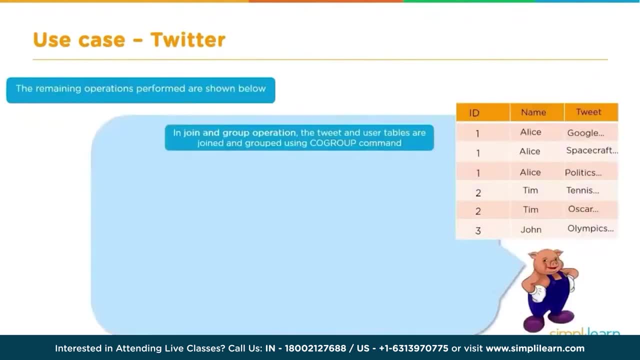 and load it into the pig storage, the pig storage system. The remaining operations performed are shown below. In join and group operation, the tweet and user tables are joined and grouped using co-group command And you can see here where we add a whole column. 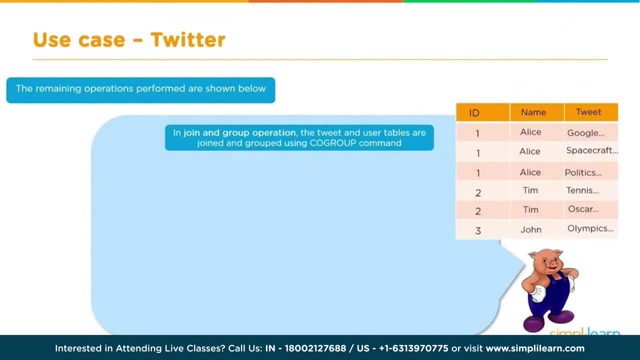 and we go from user names and tweet to the ID linked directly to the name. So Alice was user one, Tim was two and John three, And so now they're listed with their actual tweet. The next operation is the aggregation. 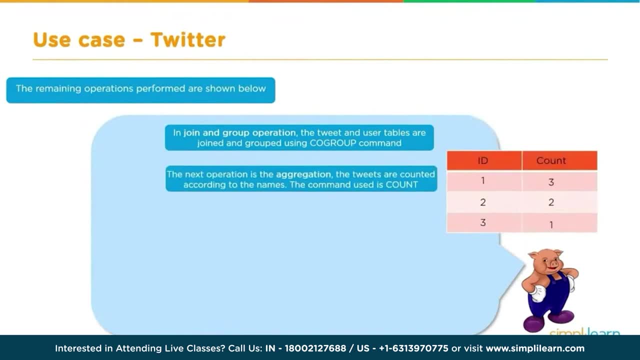 The tweets are counted according to the names. The command used is count, So it's very straightforward. We just want to count how many tweets each user is doing. And finally, the result after the count operation is joined with the user table to find out the user name. 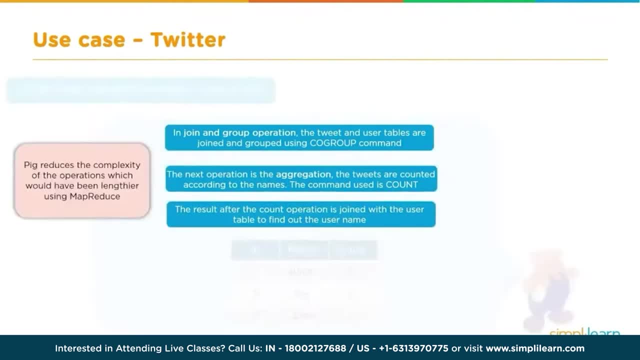 And you can see here where Alice had three, Tim two and John one Pig, reduces the complexity of the operations, which would have been lengthy, using MapReduce. In join and group operation, the tweet and user tables are joined and grouped using co-group command. 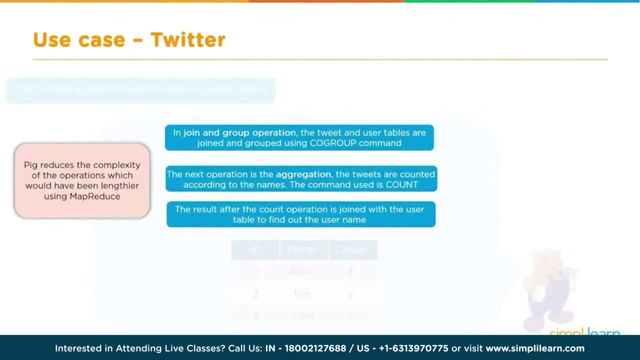 The next operation is the aggregation. The tweets are counted according to the names. The command used is count. The result after the count operation is joined with the user table to find out the user name And you can see we're talking about three lines of script. 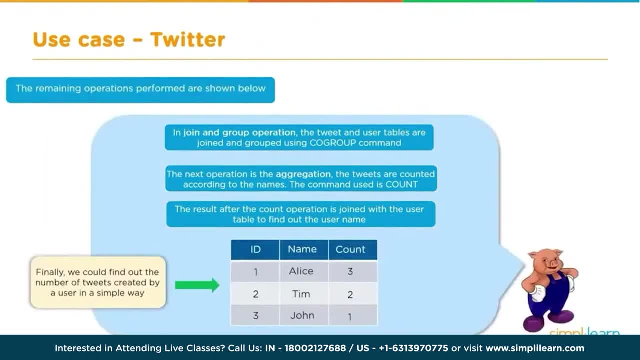 versus a MapReduce code of about 80 lines. Finally, we can find out the number of tweets created by a user in a simple way. So let's go quickly over some of the features of Pig that we already went through most of these. 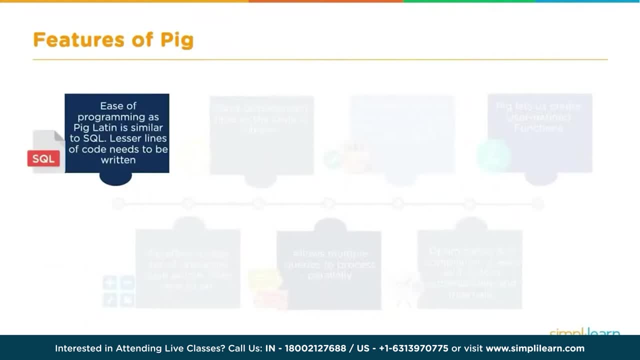 First, ease of programming. as Pig Latin is similar to SQL, Lesser lines of code need to be written. Short development time: as the code is simpler, It queries out rather quickly instead of having to have a programmer spend hours on it. It handles all kinds of data, like structured 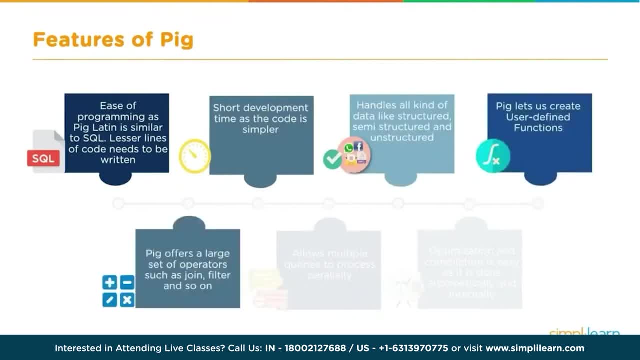 semi-structured and unstructured. Pig lets us create user-defined functions. Pig offers a large set of operators such as join, filter and so on. It allows for multiple queries to process unparallel, And optimization and compilation is easy, as it is done automatically and internally. 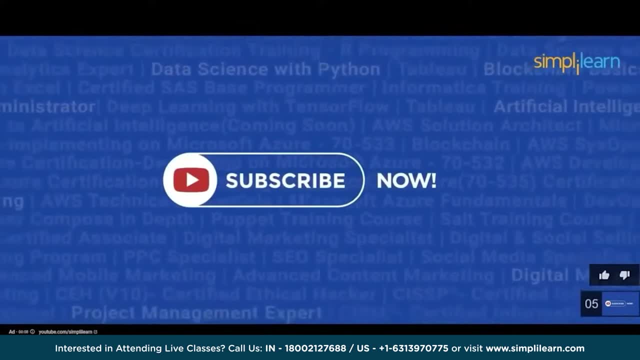 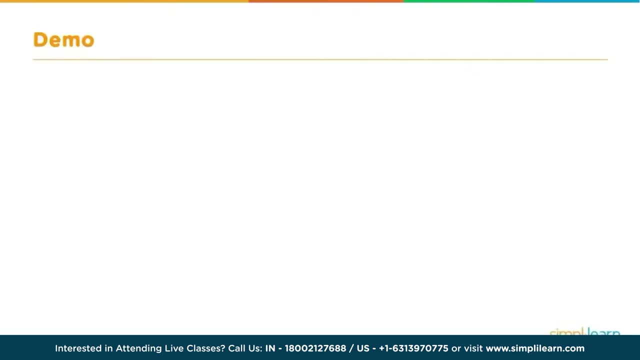 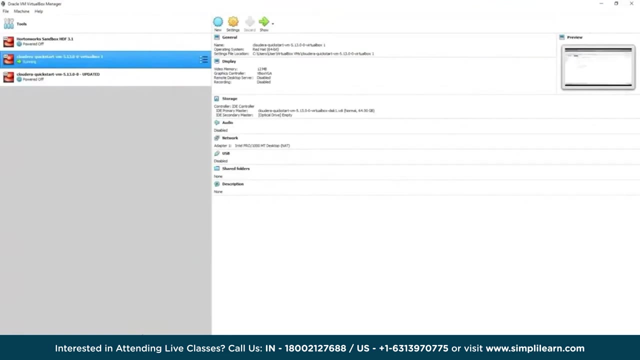 So enough theory, Let's dive in and show you a quick demo on some of the commands you can do in Pig. Today's setup will continue as we have in the last three demos- to go ahead and use Cloudera Quickstart, And we'll be doing this in VirtualBox. 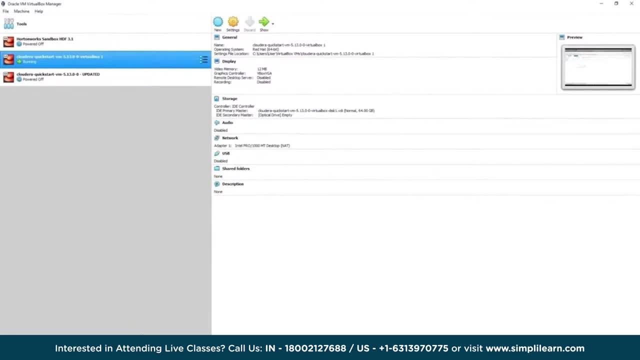 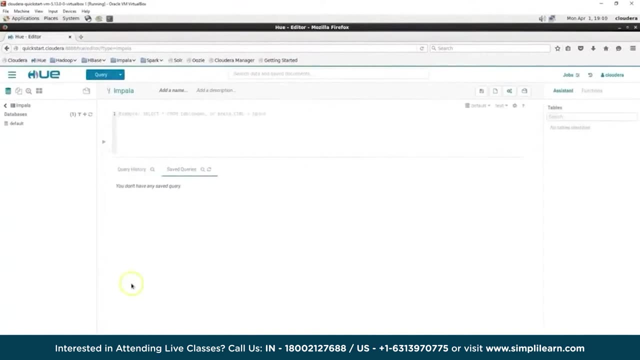 We do have a tutorial in setting that up. You can send a note to our Simply Learn team and they can get that linked to you. Cloudera Quickstart has spun up And remember this is VirtualBox. We've created a virtual machine. 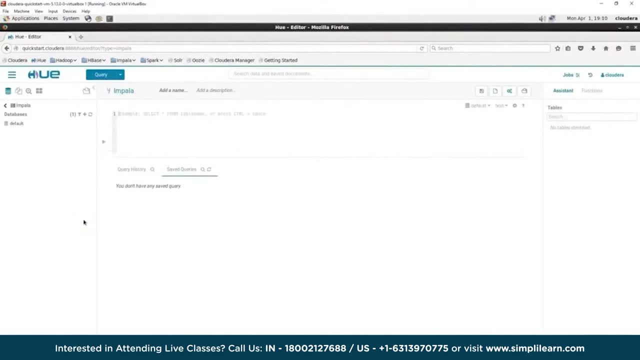 And this virtual machine is CentOS Linux. Once it's spun up, you'll be in a full Linux system here And, as you can see, we have Thunderbird Browser which opens up to the Hadoop Basic System Browser, And we can go underneath the hue. 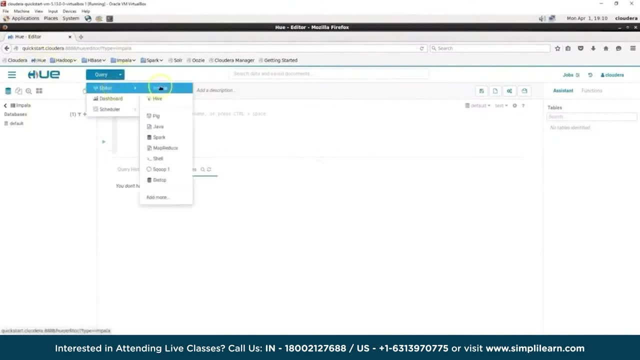 where it comes up by default. If you click on the pull-down menu and go under Editor, you can see there's our Impala, our query languages you can use And we're going under Pig. And then, once you're in Pig, 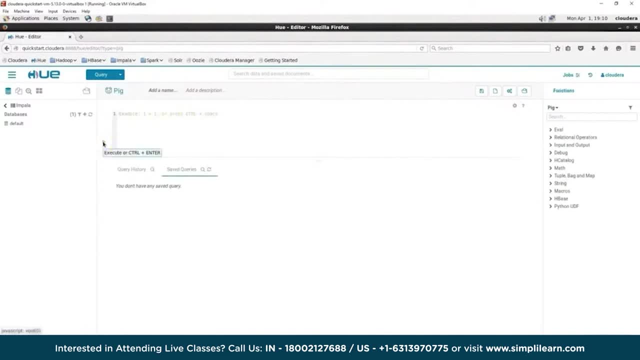 we can go ahead and use our command line here and just click that little blue button to start it up and running. We will actually be working in Terminal Window And so if you're in the Cloudera Quickstart, you can open up the Terminal Window up top. 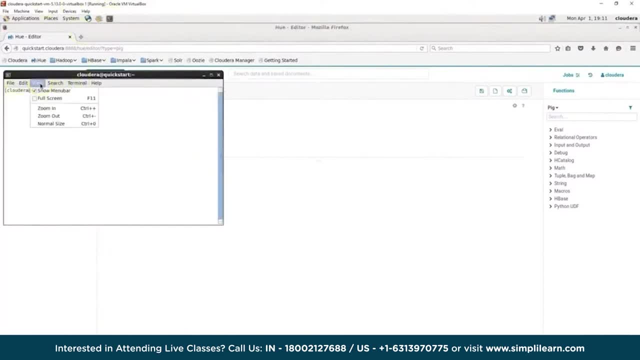 Or if you're in your own setup and you're logged in, you can easily use all of your commands here in Terminal Window And we'll zoom in. That way you get a nice view of what's going on. So let's go ahead and do a Hadoop command. 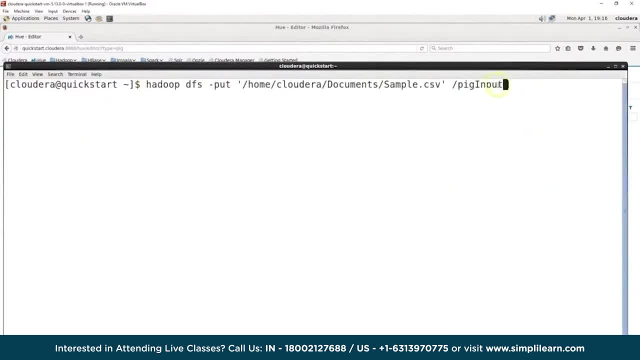 and import some data into the Hadoop system, in this case a Pig input. And let's take a look at this. We have Hadoop DFS. There's actually four variations of DFS, So if you have HDFS or whatever, that's fine. 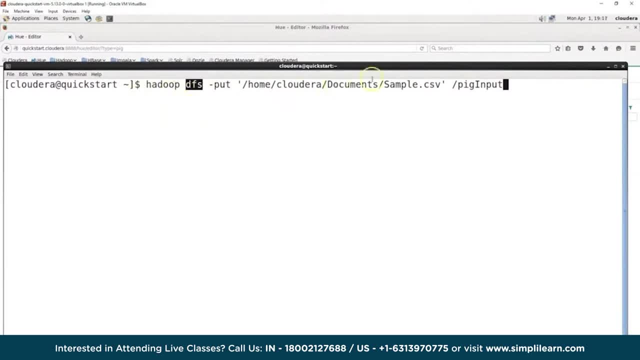 All four of them used to be different setups underneath different things, and now they all do the same thing. And we want to put this file, which in this case is under Hadoop, into the Pig input. And let's take a look at that file. 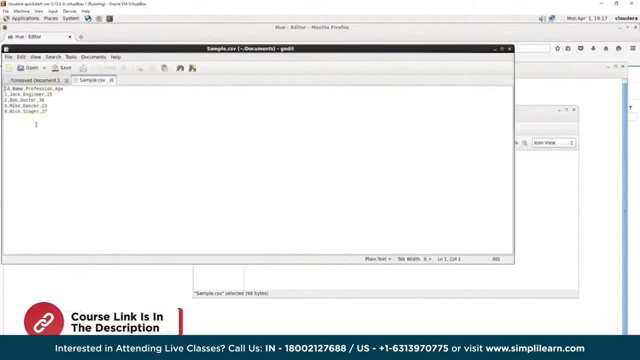 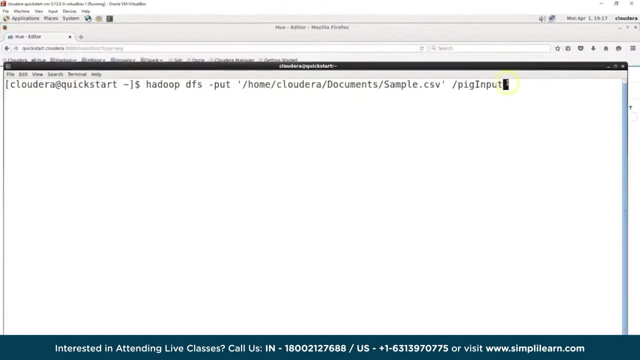 If I go into my document browsers and open this up, you'll see it's got a simple ID, name, profession and age. We have 1jackengineer25.. And that was in one of our earlier things we had in there. 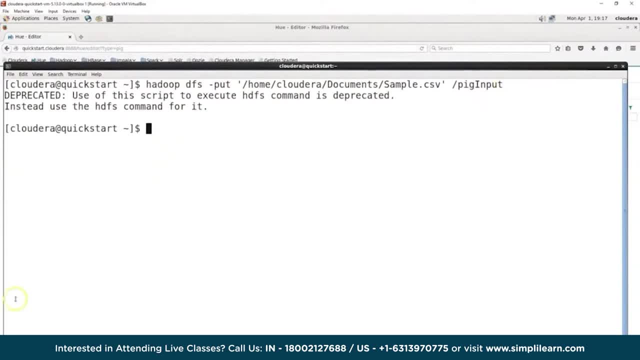 And so let's go ahead and hit enter and execute this, And now we've uploaded that data and it's gone into our Pig input. And then a lot of the Hadoop commands. we have cat as one of our commands Or it has a hyphen before it. 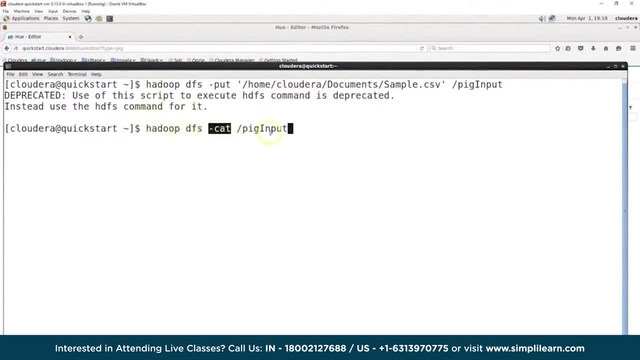 So we execute that with Hadoop DFS hyphen cat slash pig input, Because that's what we called it. That's where we put our sample CSV at And we execute this. You can see from our Hadoop system it's going to go in and pull that up. 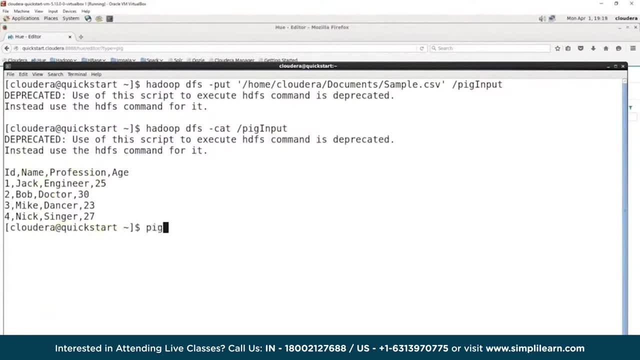 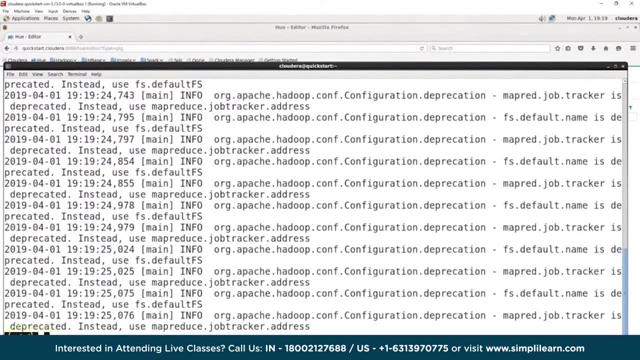 and, sure enough, it pulls out the data file we just put in there, And then we can simply enter the Pig Latin or Pig Editor mode by typing in pig, And we can see here, by our grunt, there's our grunt command line. So we are now in the pig shell. 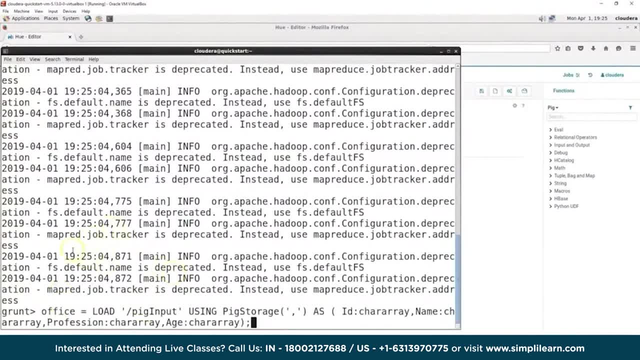 And then we'll go ahead and put our load command in here, And the way this works is I'm going to have office equals load, And here's my load. In this case it's going to be pig input. We have that in single brackets. 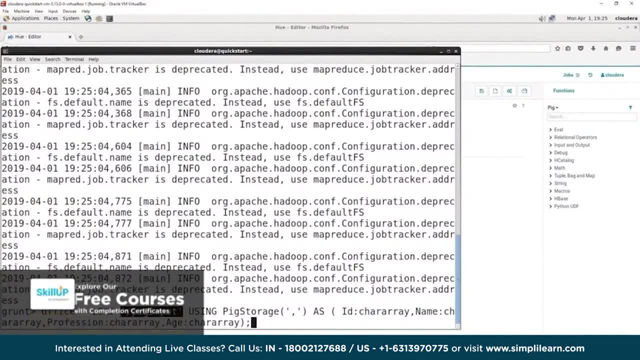 You remember? that's where the data is in the Hadoop file system, where we dumped it into there. We're going to be using pig storage. Our data was separated as with a comma, So there's our comma separator, And then we have as. 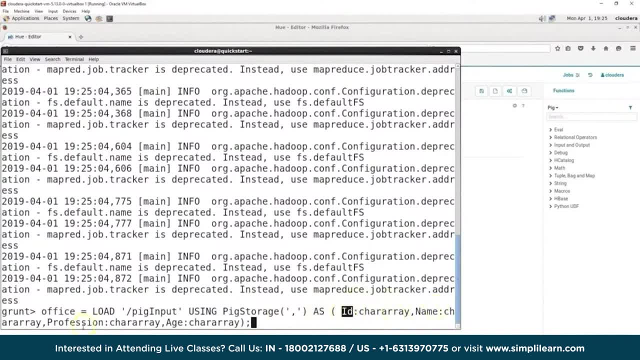 And in this case we have an id character array, name character array, profession character array and age character array, And we're just going to do them all as character arrays just to keep this simple for this one, And then, when I hit, put this all in here. 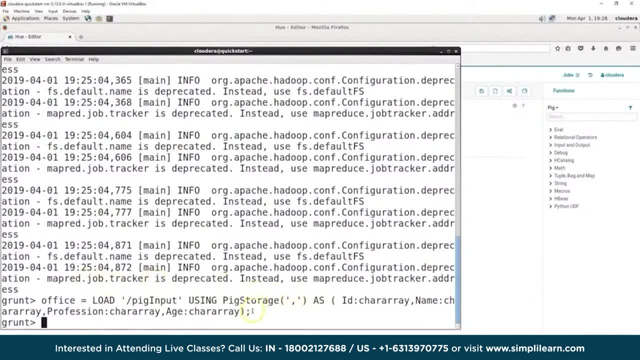 you can see that's our full command line going in and we have our semicolon at the end. So when I hit enter it's now set office up, But it hasn't actually done anything yet. It doesn't do anything until we do dump office. 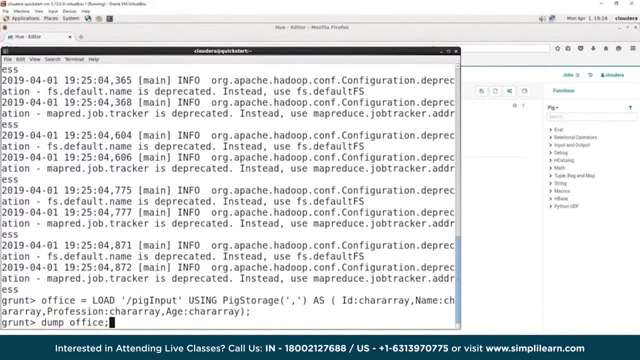 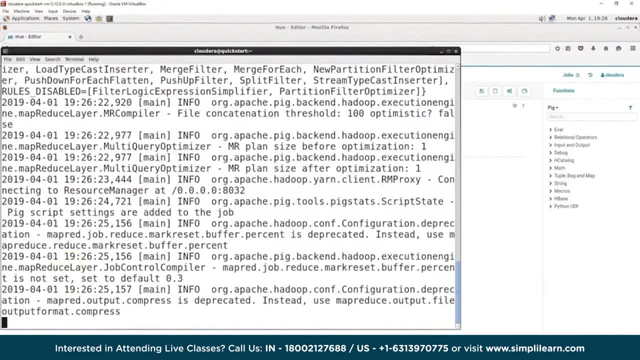 So there's our command to execute whatever we've loaded or whatever setup we have in here. You can see it go through the different languages and this is going through the MapReduce. Remember, we're not doing this locally, We're doing this on the Hadoop setup. 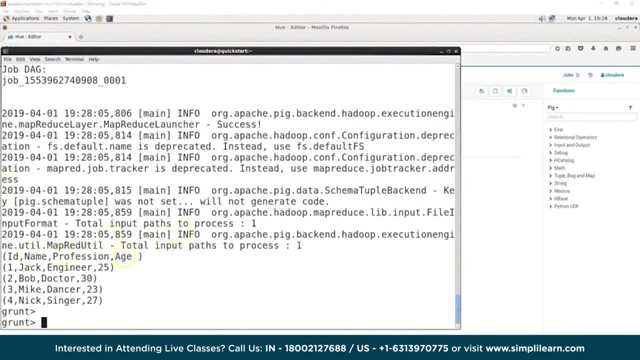 And once we've finished our dump, you can see we have id name, profession, age and all the information that we just dumped into our pig. We can now do. let's say we have a request just for- we'll keep it simple in here, but just for the name. 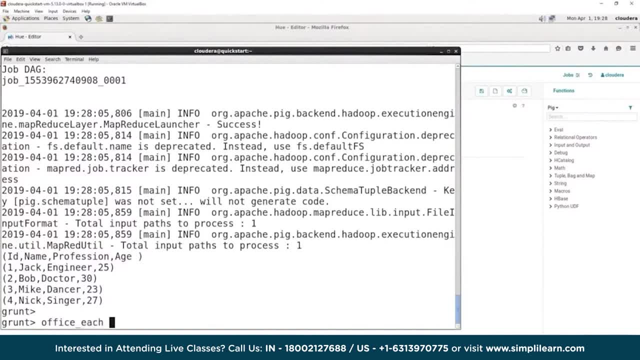 and age, And so we can go office. we'll call it each as our variable underscore. each For each office, generate name, comma, age And for each means that we're going to do this for each row And, if you're thinking, MapReduce. 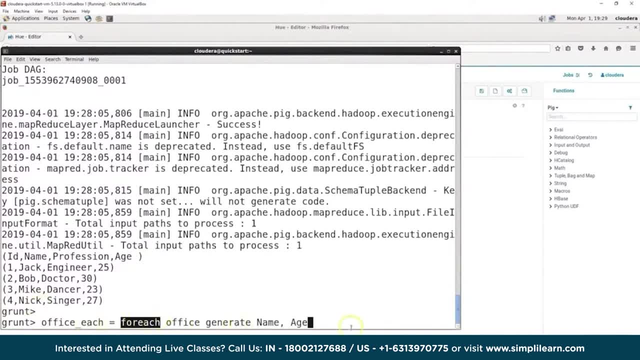 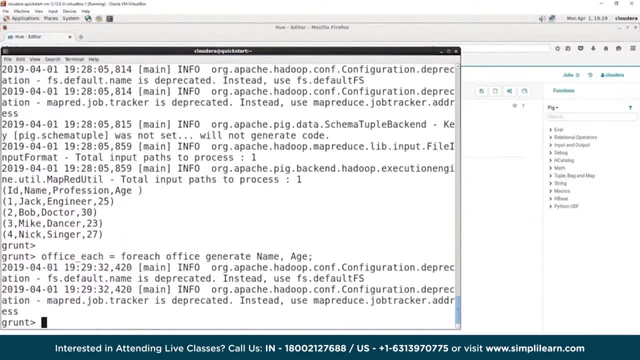 you know that this is a map function Because it's mapping each row and generating name and age on here, And of course we want to go ahead and close it with a semicolon And then, once we've created our query or the command line in here, let's go ahead and dump. 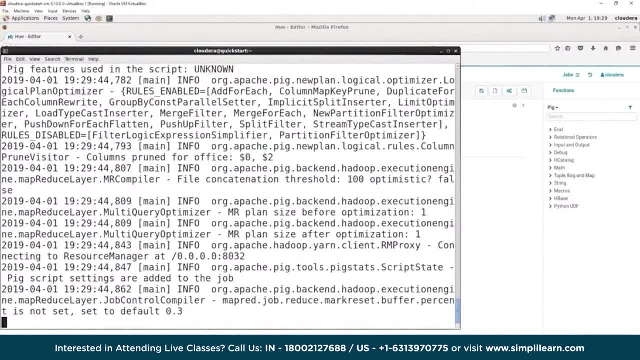 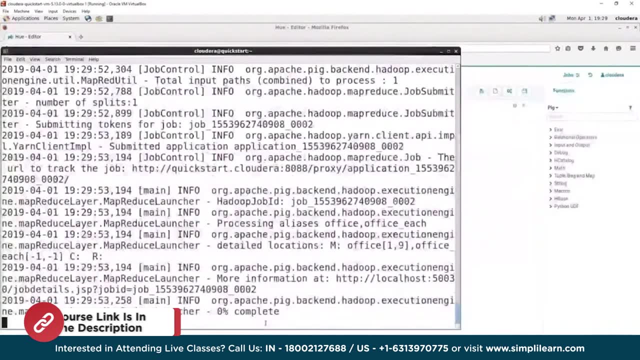 office underscore each in with our semicolon And this will go through our MapReduce setup on here And if we were on a large cluster, the same processing time would happen. In fact it's really slow because I have multiple things on this computer and this particular 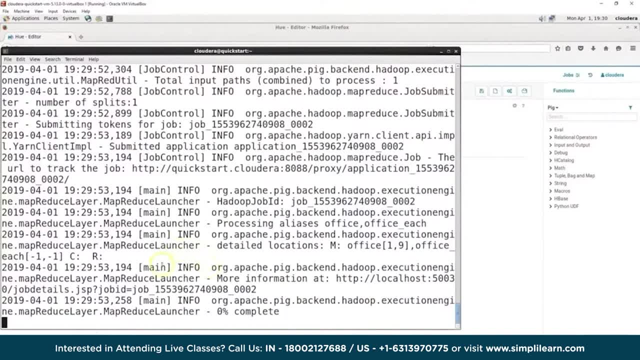 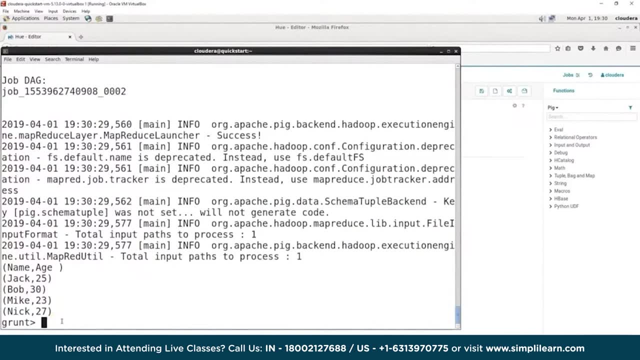 virtual box is only using a quarter of my processor. It's only dedicated to this And you can see here. there it is name and age, And it also included the top row, since we didn't delete that out of there or tell it not to, And that's fine for this. 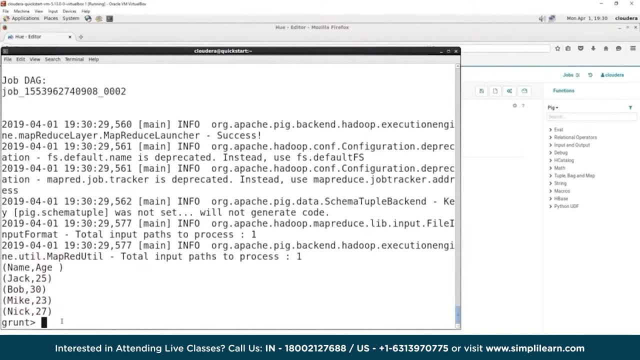 example. But you need to be aware of those things when you're processing a significantly large amount of data or any data. And we can also do office and we'll call this DSC for descending. So maybe the boss comes to you and says, hey, can we order? 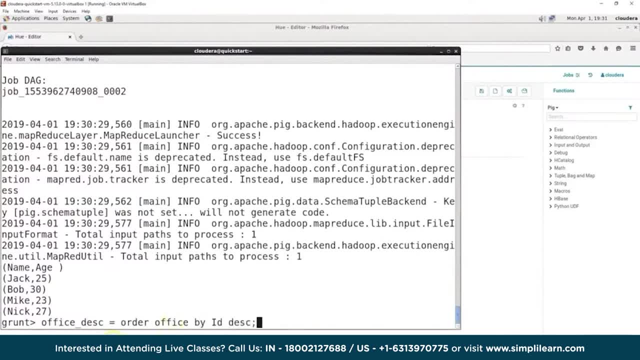 office by ID descending And, of course, your boss. you've taught them how to your shareholder sounds a little derogatory when you say boss, You've talked to the shareholder and you said: and you've taught them a little bit of pig Latin and they know. 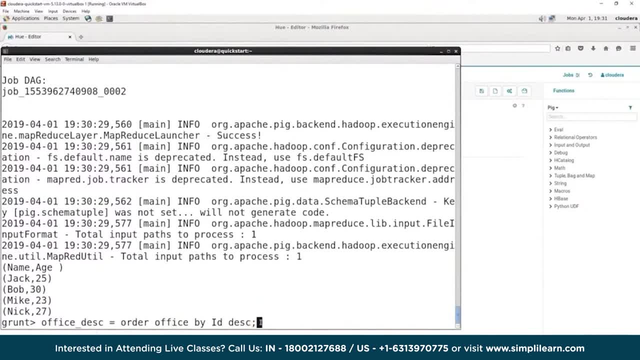 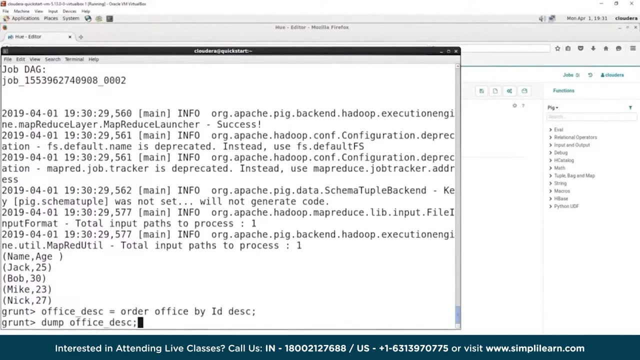 that they can now create office description And we can order office by ID description. And of course, once we do that, we have to dump office underscore description so that it'll actually execute. And there it goes into our MapReduce. It'll take just a moment for it to come up because 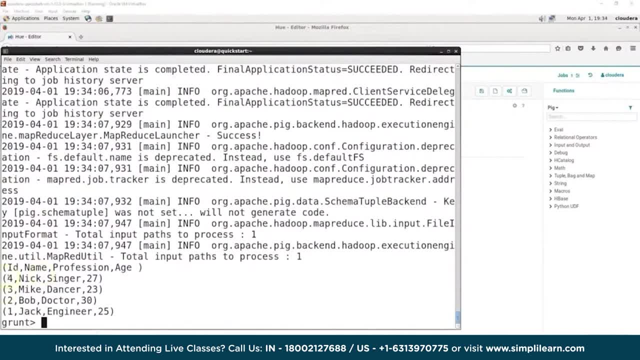 again. I'm running on only a quarter of my processor And you can see we now have our IDs in descending order, returned. Let's also look at- and this is so important with anytime you're dealing with big data. Let's create office with a limit And you can. 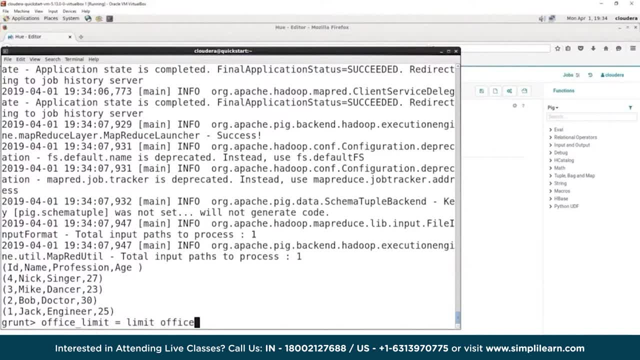 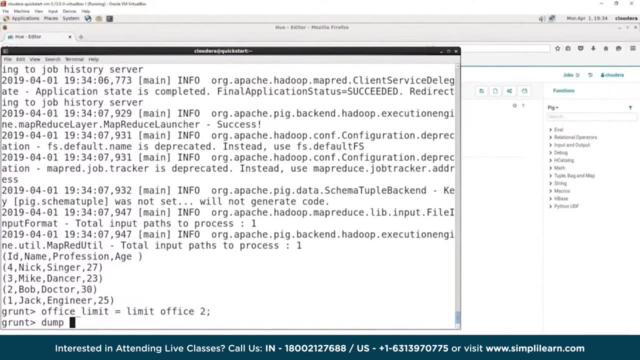 of course, do any of this instead of with office. we could do this with office descending, so you get just the top two IDs on there, But we're going to limit just to two And of course, to execute that we have to dump office underscore limit. 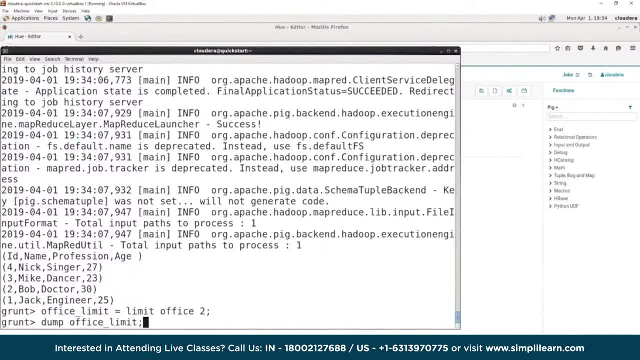 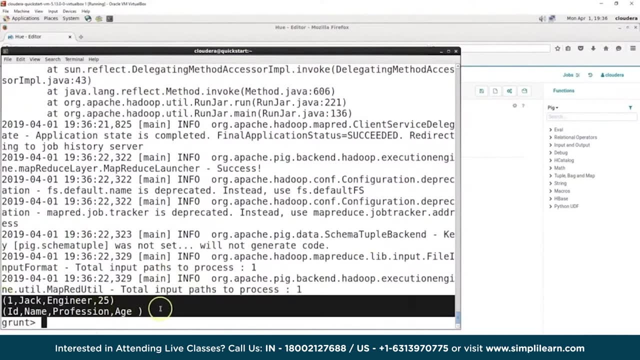 And you can just think of dumping your garbage into the pig pen for the pig to eat. There we go, Dump office limit two And that's going to just limit our office to the top two, And for our output we get our first row which had our ID name: profession. 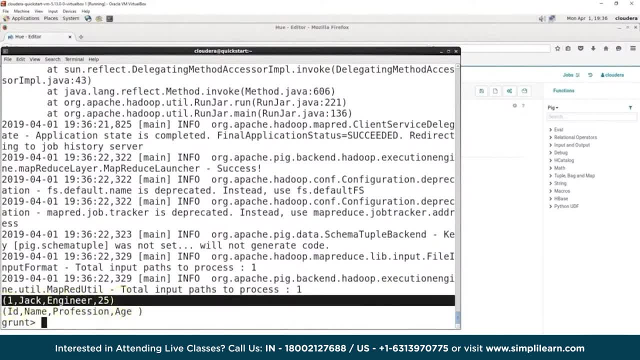 and age, And our second row, which is Jack, who's an engineer. Let's do a filter. We'll call it office underscore filter. You guessed it: Equals filter. office by profession: equals. And keep note, this is similar to how Python does it with the double equal signs. 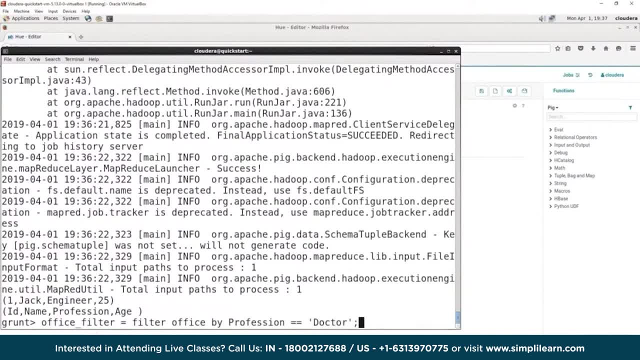 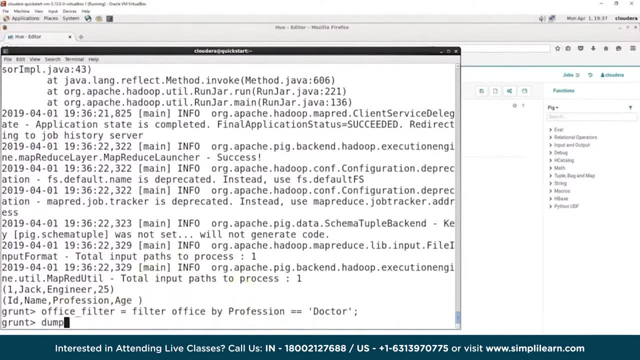 for equal, for doing a true false statement. So for your logic statement, remember to use two equal signs in pig And we're going to say it equals doctor. So we want to find out how many doctors do we have on our list And we'll go ahead and do our dump. 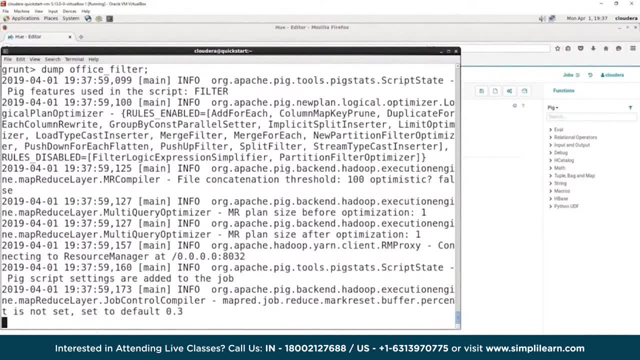 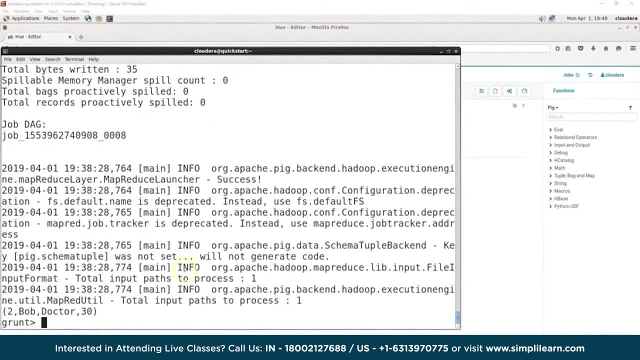 We're dumping all our garbage into the pig pen and we're letting pig take over and see what it can find out. and see who's a doctor on our list And we find employee ID number two. Bob is a doctor, years old. For this next section, 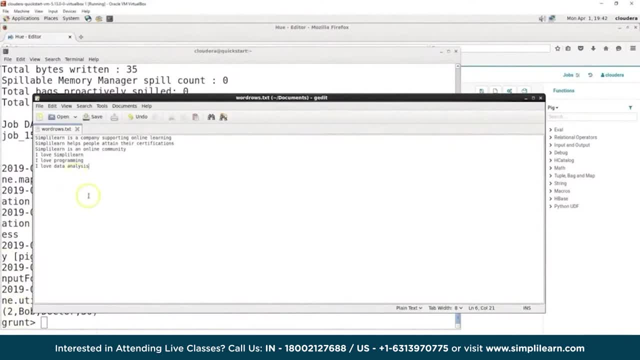 we're going to cover something we see a lot nowadays in data analysis And that's word counting: Tokenization. That is one of the next big steps as we move forward in our data analysis: where we go from, say, stock market analysis of highs and lows. 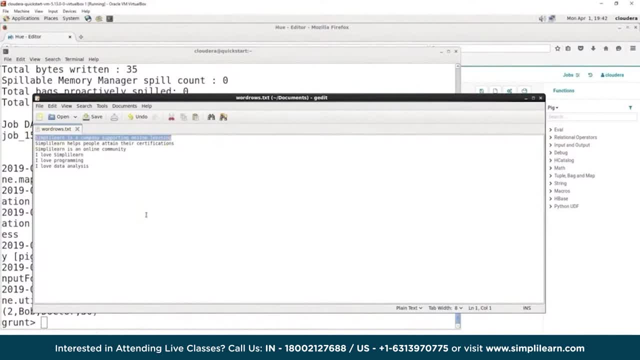 and all the numbers to what are people saying about companies on Twitter? What are they saying on the web pages and on Facebook? Suddenly, you need to start counting words and finding out how many words are total. how many are in the first part of the document. 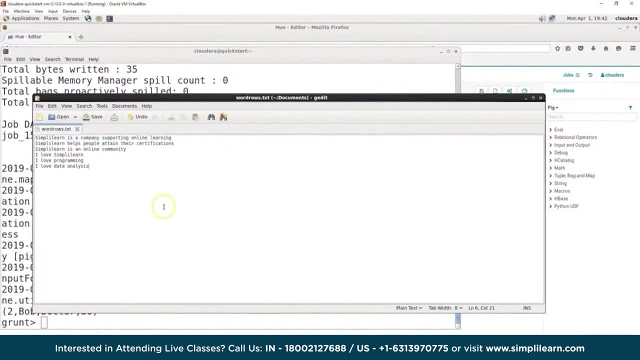 and so on. We're going to cover a very basic word count example And in this case I've created a document called word rows dot text. And you can see here we have SimpliLearn as a company supporting online learning. SimpliLearn helps people attain their 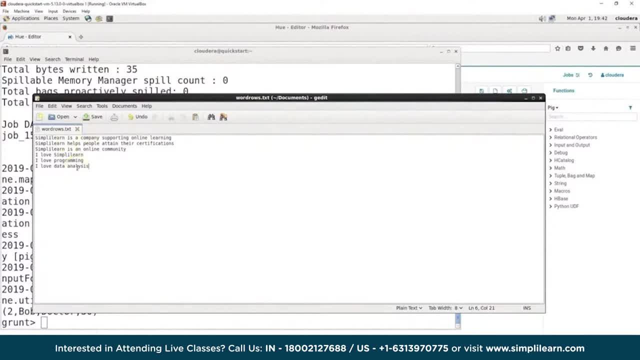 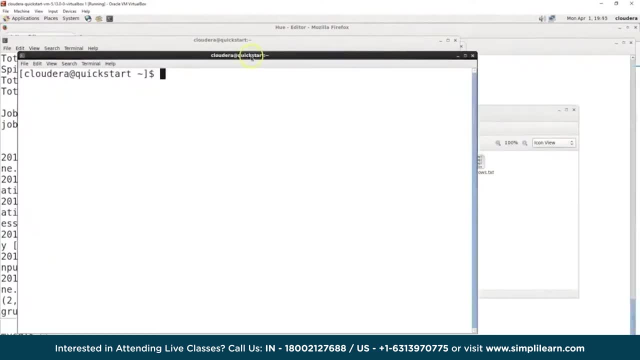 certifications. SimpliLearn is an online community. I love SimpliLearn, I love programming, I love data analysis, And I went and saved this into my documents folder so we could use it. And let me go ahead and open up a new terminal window for our word count. 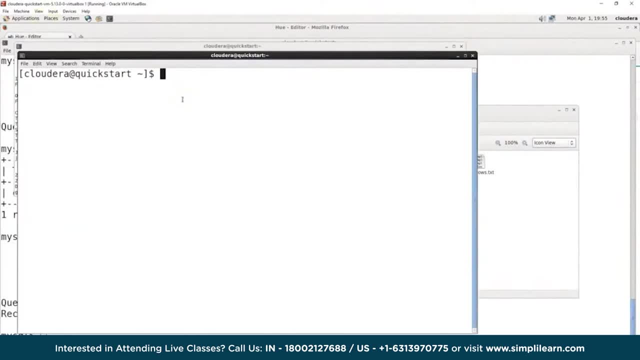 Let me go ahead and close the old one. So we're going to go in here and instead of doing this as pig, we're going to do pig minus x local, And what I'm doing is I'm telling the pig to start the pig shell. but we're going to be looking at files. 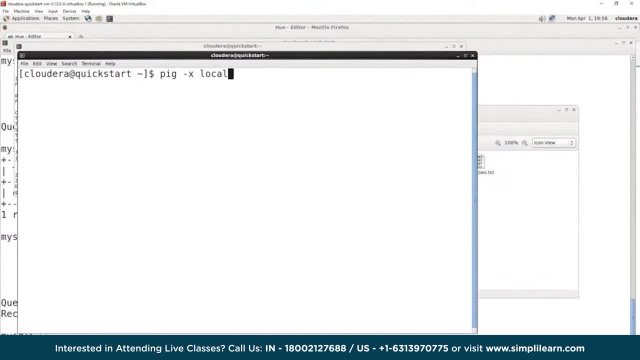 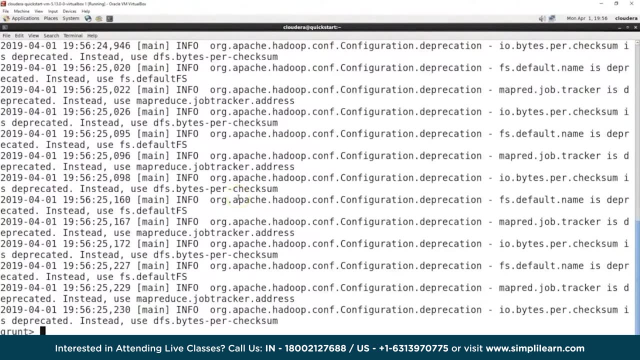 local to our virtual box or this CentOS machine, And let me go ahead and hit enter on there. Just maximize this up. There we go And it will load pig up and it's going to look just the same as the pig we were doing, which? 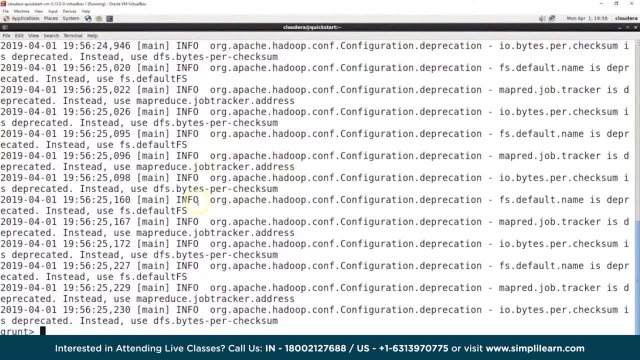 was defaulted to high to our Hadoop system, To our HDFS. This is now defaulted to the local system. Now we're going to create lines and we're going to load it straight from the file. Remember last time we took the HDFS and loaded it into. 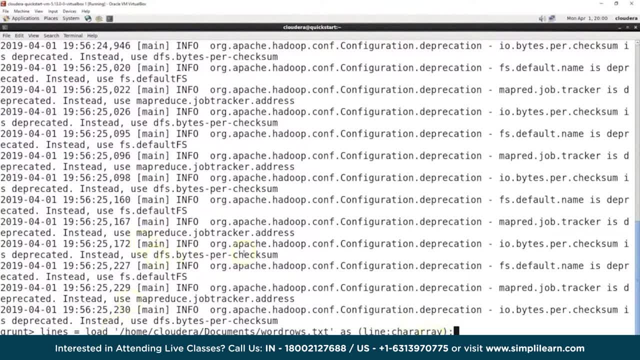 there and then loaded it into pig. Since we've gone the local, we're just going to run a local script. We have lines equals: load home, The actual full path Home. Cloudera documents, and I called it word rows dot text. 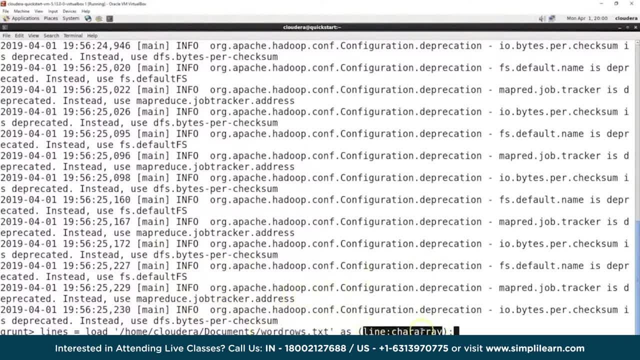 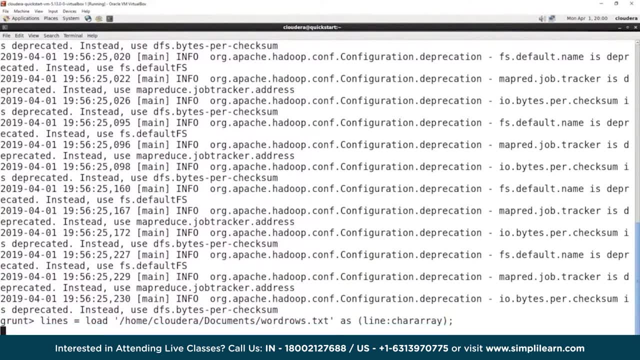 And as line, as a character array, So each line, and I've actually you can change this to read each document, I certainly have done a lot of document analysis And then you go through and do word counts and different kind of counts in there. 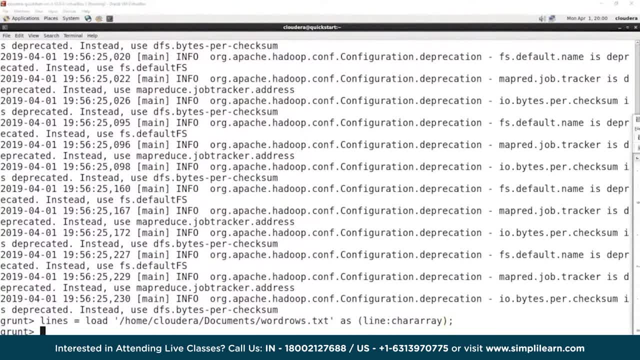 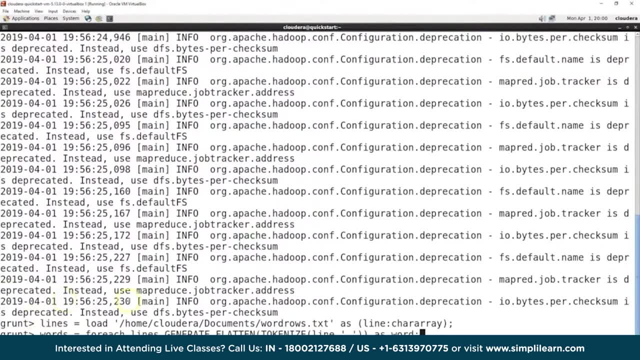 So, once we go ahead and create our line, instead of doing the dump, we're going to go ahead and start entering all of our different setups, or each of our steps we want to go through. And let's just take a look at this next one. 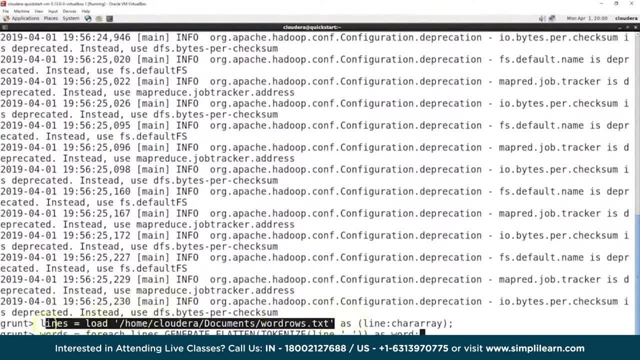 Because the load is straight forward. We're loading from this particular file. Since we're local, it's loading it directly from here instead of going into the Hadoop file system. And it says as: and then each line is read as a character array. Now we're going to. 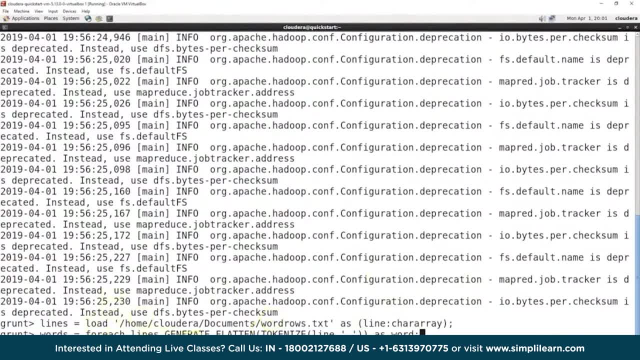 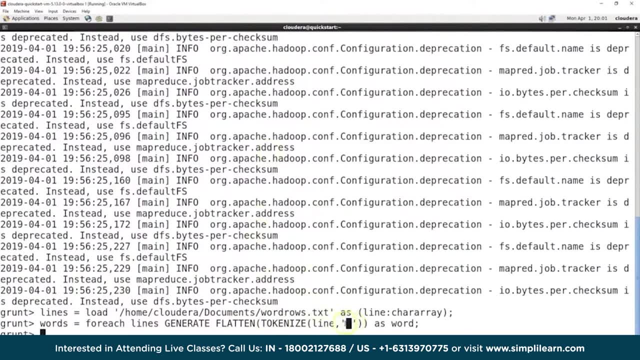 do words equal for each of the lines. generate flat, tokenize line space as word. Now, there's a lot of ways to do this. This is, if you're a programmer, you're just splitting the line up by spaces. There's actual ways to tokenize it. You've got to look for periods. 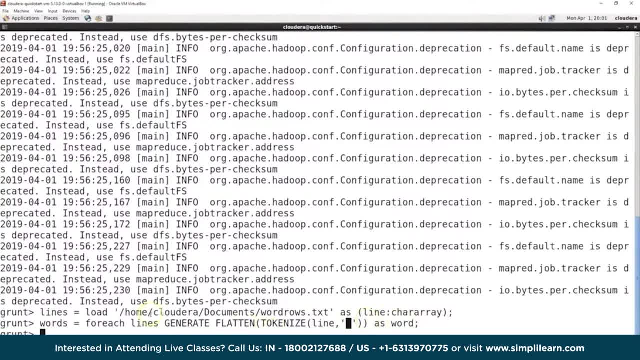 capitalization. There's all kinds of other things you play with with this, But for the most basic word count we're just going to separate it by spaces. The flatten takes the line and just creates a. it flattens each of the words out. 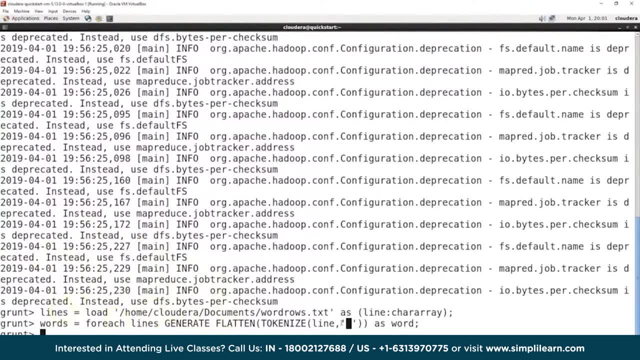 So this is: we're just going to generate a bunch of words for each line, And then each of those words is, as a word, A little confusing in there. but if you really think about it, we're just going down each line, separating it out, and we're generating. 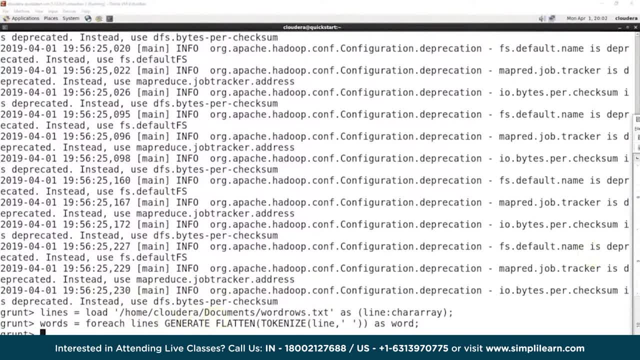 a list of words. One thing to note is the default for tokenize. You can just do tokenize line without the space in there. If you do that, it'll automatically tokenize it by space. You can do either one And then we're going to. 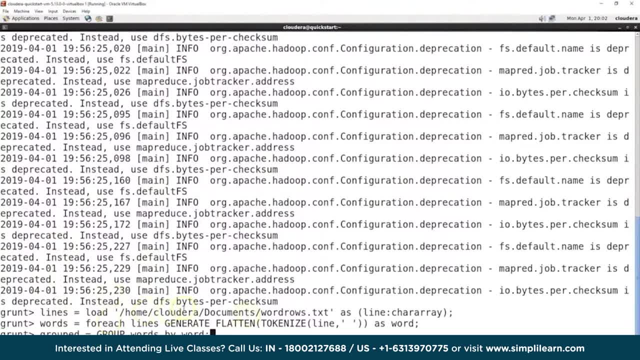 do group, We're going to group it by words. So we're going to group words by word. So when we split it up, each token is a word and it's a list of words, And so we're going to grouped equals, group words by words. 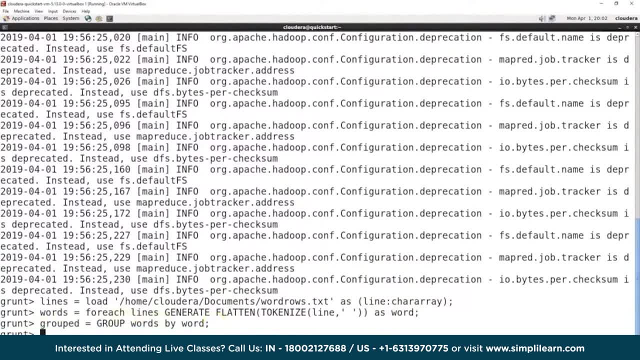 So we're going to group all the same words together, And if we're going to group them, then we want to go ahead and count them. And so, for count, we'll go ahead and create a word count variable, And here's our for each. So for each grouped, 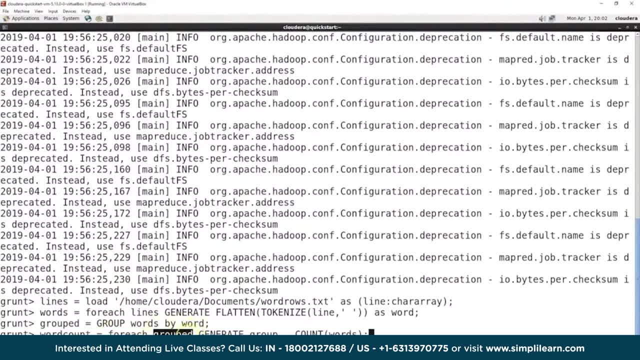 grouped is our line where we group all the words in the line that are similar. We're going to generate a group And then we're going to count the words For each grouped. so for each line where we group the words together, we're going to generate a group. 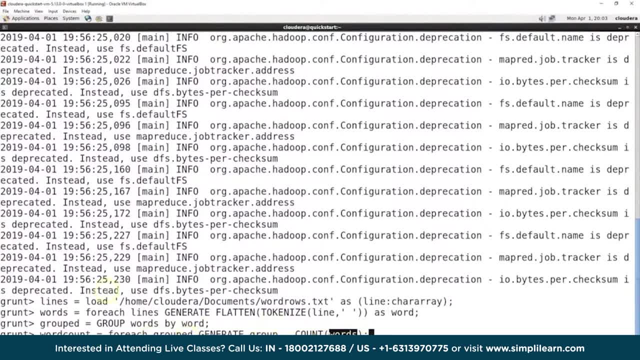 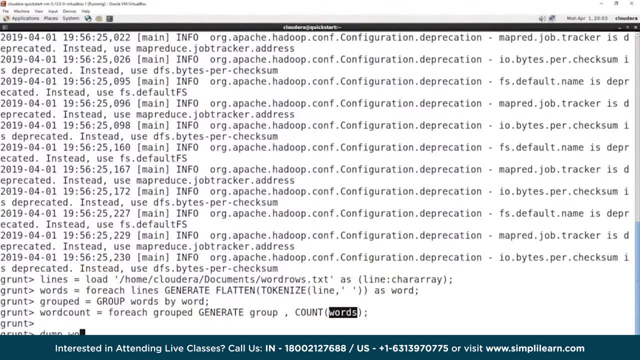 and that's going to count the words. We want to know the word count in each of those And that comes back in our word count. And finally, we want to take this and we want to go ahead and dump word count And this is a little. 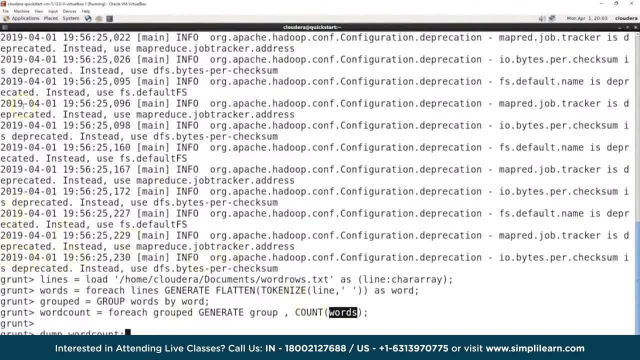 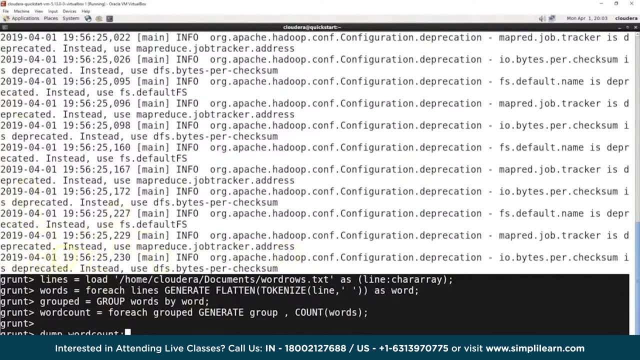 bit more what you see when you start looking at grunt scripts. You'll see right here these lines. right here we have each of the steps you take to get there. So we load our file for each of our lines We're going to generate and tokenize. 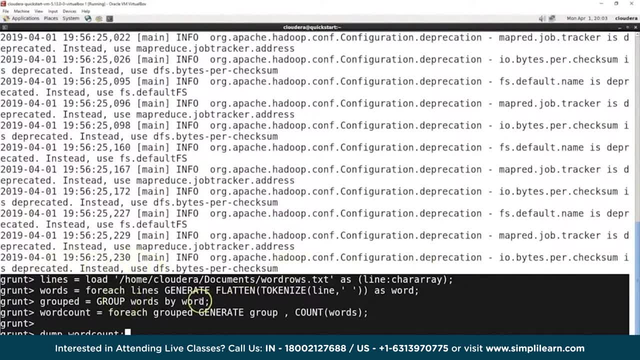 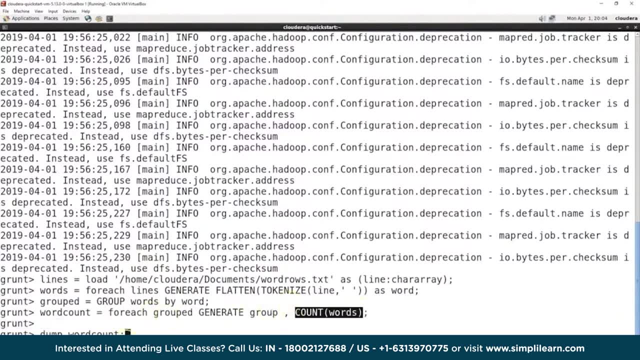 it into words. Then we're going to take the words and we're going to group them by same words For each grouped. we're going to generate a group and we're just going to count the words. So we're going to summarize all the words in here. 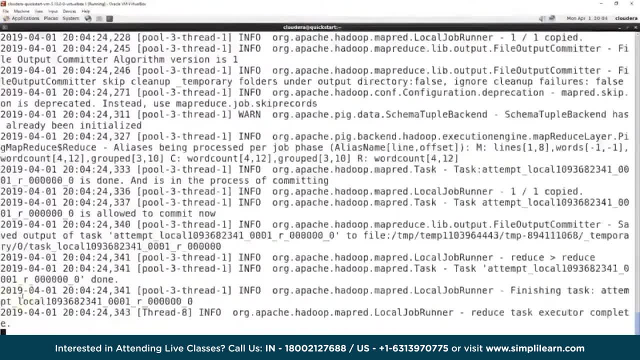 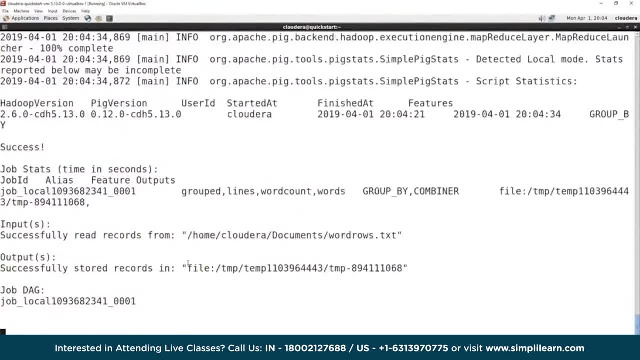 And let's go ahead and do our dump word count, which executes all this And it goes through our MapReduce. It's actually a local runner. You'll see down here. you start seeing where they still have MapReduce, but it's a special runner. We're mapping it. 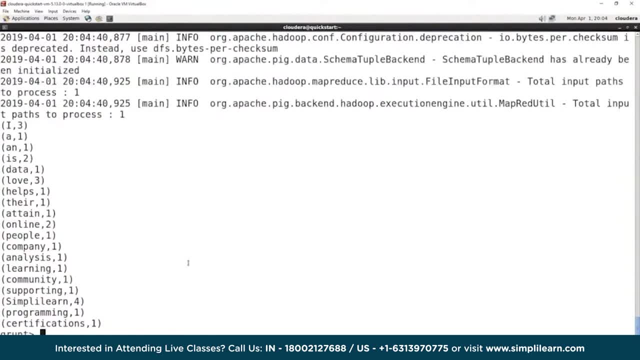 That's a part of each row being counted and grouped, And then when we do the word count, that's the reducer. The reducer creates these keys. The I is used three times. A came up once, N came up, once Is two. 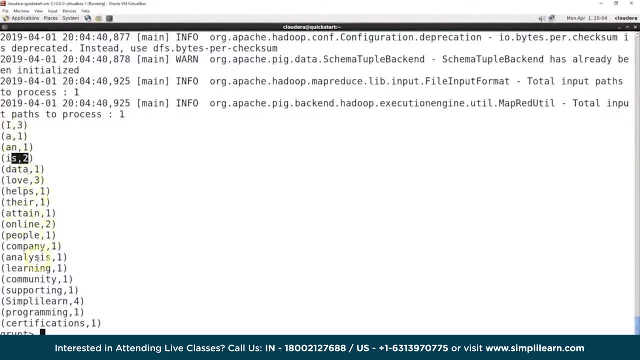 Continue on down here to attain online people company analysis. simply learn: They took the top rating with four Certification. So all these things are then counted in the how many words are used, And in data analysis, this is probably the very 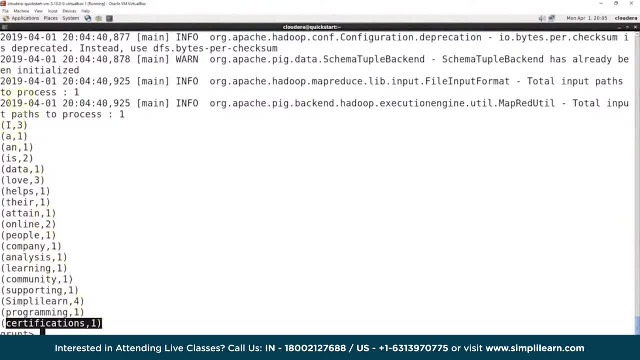 beginnings of data analysis where you might look at it and say, oh, they mentioned love three times. So whatever's going on in this post, it's about love And what do they love? And then you might attach that to the different objects in here. 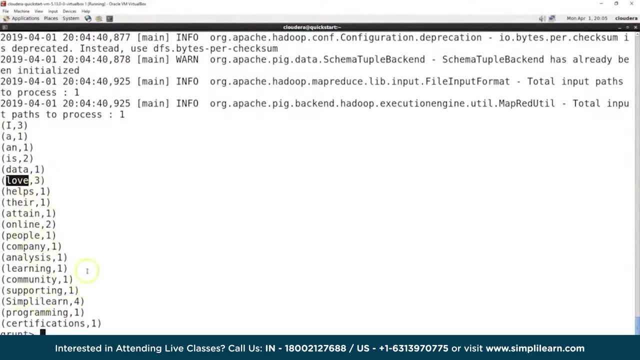 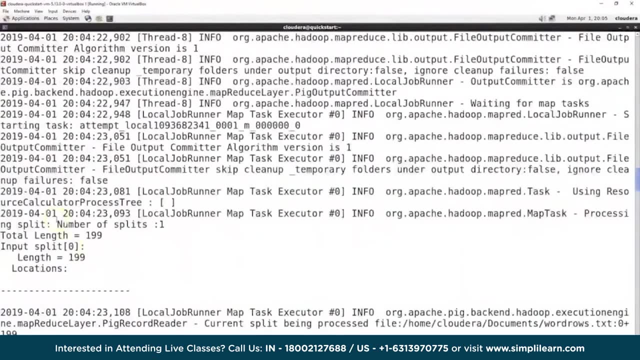 So you can see that PigLatin is fairly easy to use. There's nothing really. you know, it takes a little bit to learn the script, depending on how good your memory is. As I get older, my memory leaks a little bit more, so I don't memorize it as much. 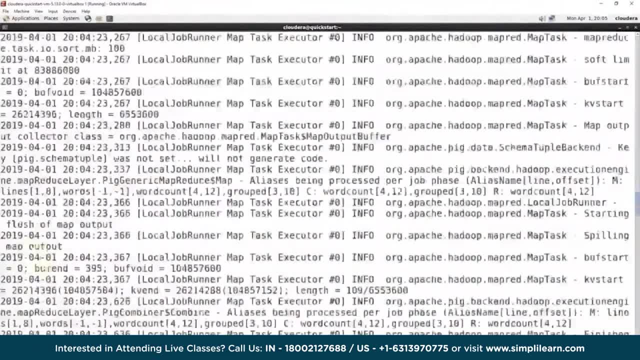 But that was pretty straightforward: the script we put in there And then it goes through. the full map- reduce, localize, run- comes out and, like I said, it's very easy to use. That's why people like PigLatin is. 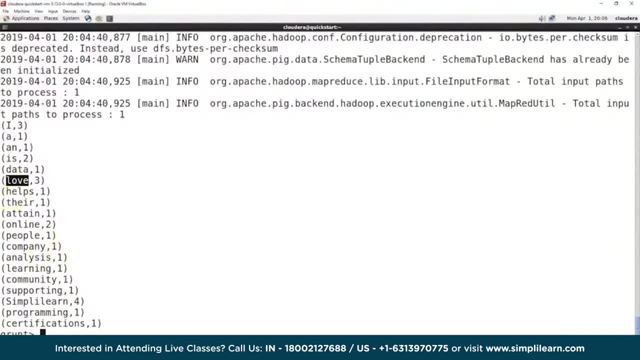 because it's intuitive. One of the things I like about PigLatin is when I'm troubleshooting, When we're troubleshooting, a lot of times you're working with a small amount of data and you start doing one line at a time, And so I can go. 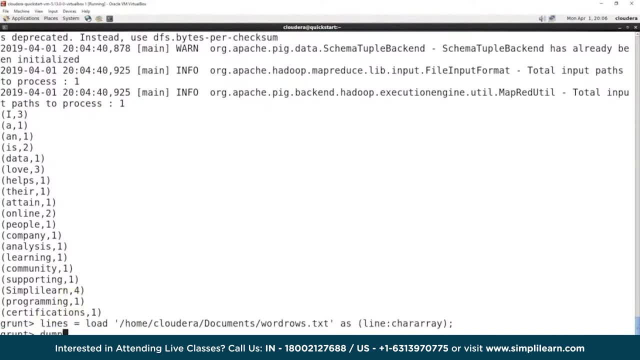 lines equal load and there's my loaded text and maybe I'll just dump lines And then it's going to run, it's going to show me all the lines that I'm working on in this small amount of data And that way. 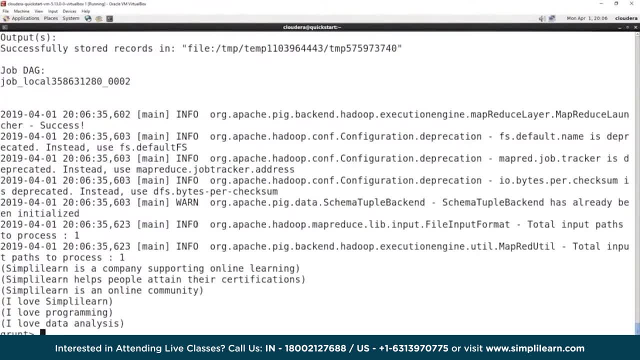 I can test that. If I got an error on there that said, oh, this isn't working, maybe I'll be like, oh my gosh, I'm in map reduce, or I'm in the basic grunt shell instead of the local path grunt, So maybe. 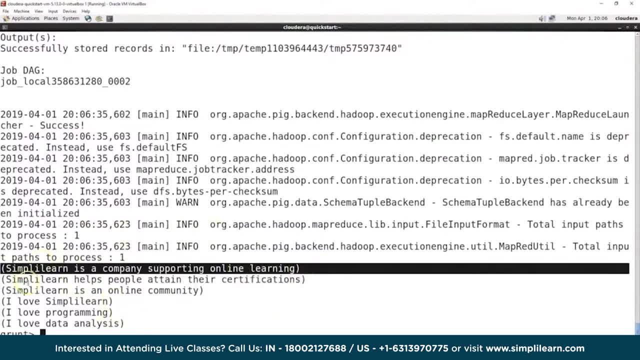 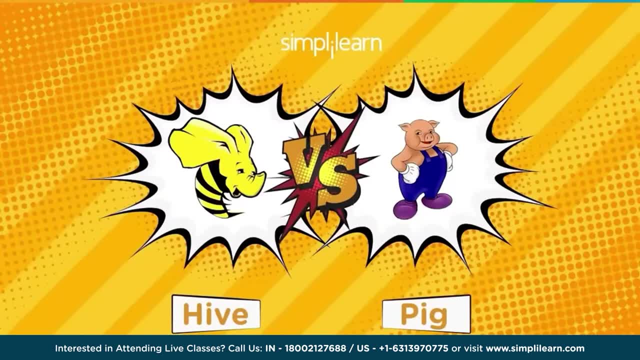 it'll generate an error on there And you can see here it just shows each of the lines going down: Hive versus pig: On one side we'll have our sharp stinger on our black and yellow friend and on the other side our thick hide. 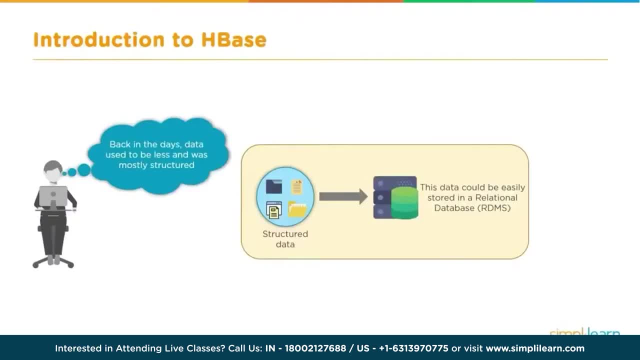 on our pig. Let's start with an introduction to HBase. Back in the days, data used to be less and was mostly structured. You can see we have structured data here. We usually had it like in a database where you had every field. 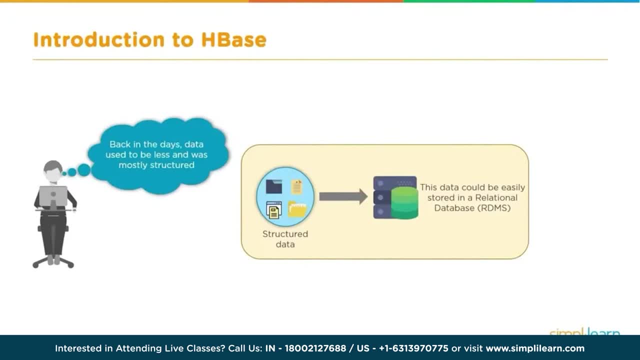 was exactly the correct length. So if you had a name field, it was exactly 32 characters. Remember the old access database in Microsoft? The files were small. If we had hundreds of people in one database, that was considered big data. This data. 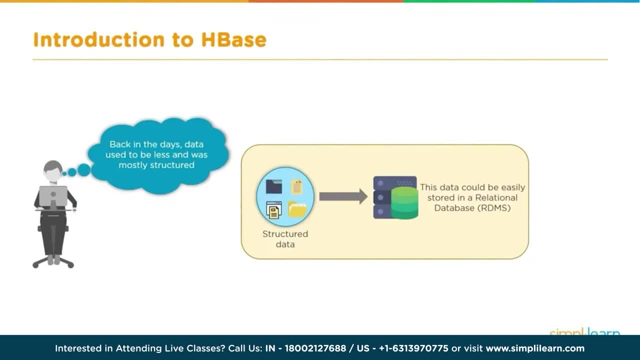 could be easily stored in relational database or RDBMS. When we talk about relational database, you might think of Oracle, you might think of SQL, Microsoft, SQL, MySQL. All of these have evolved even from back then to do a lot more today than they did. 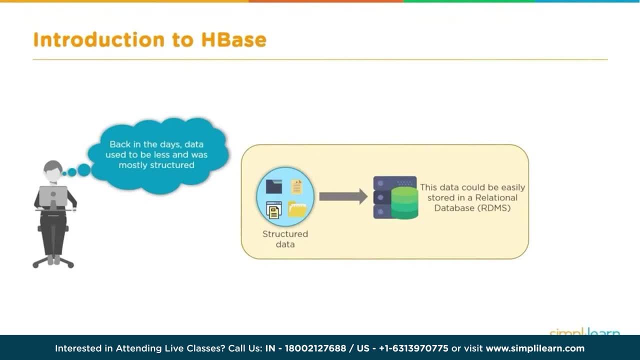 But they still fall short in a lot of ways And they're all examples of an RDMS or relationship database. Then internet evolved And huge volumes of structured and semi-structured data got generated, And you can see here with the semi-structured 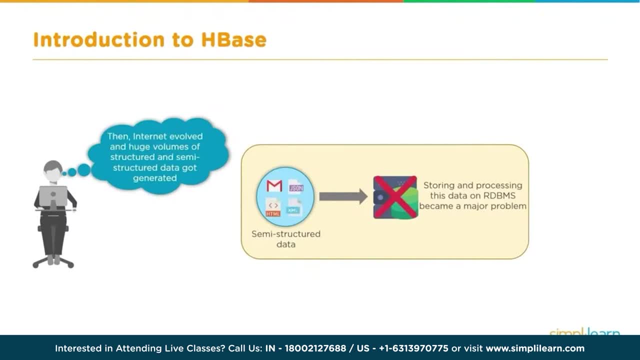 data. we have email. If you look at my spam folder, you know what we're talking about: All the HTML pages, XML, which a lot of times is displayed on our HTML and help desk pages, JSON- All of this really has 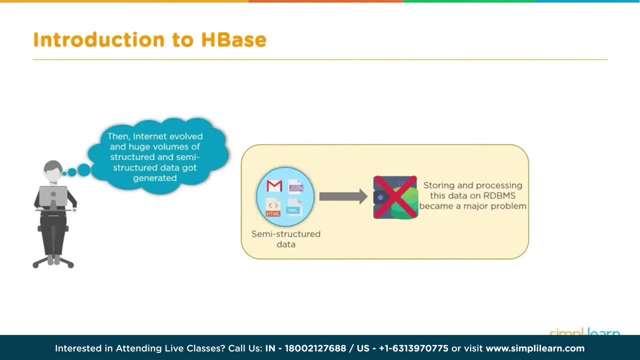 just even in the last, each year it almost doubles from the year before. how much of this is generated, So storing and processing this data on an RDBMS has become a major problem, And so the solution is we use Apache HBase. 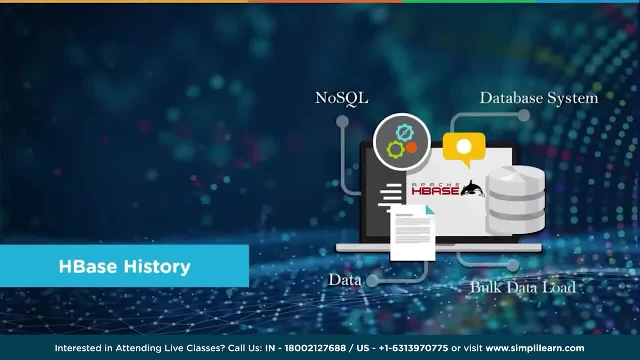 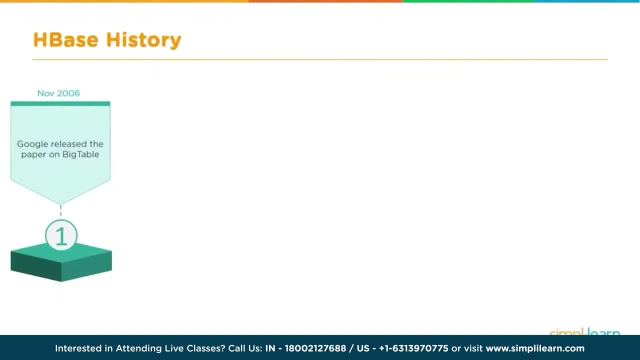 Apache HBase was the solution for this. Let's take a look at the history, the HBase history, And we look at the HBase history. we're going to start back in 2006,. November, Google released the paper on Bigtable, And then in 2017,. 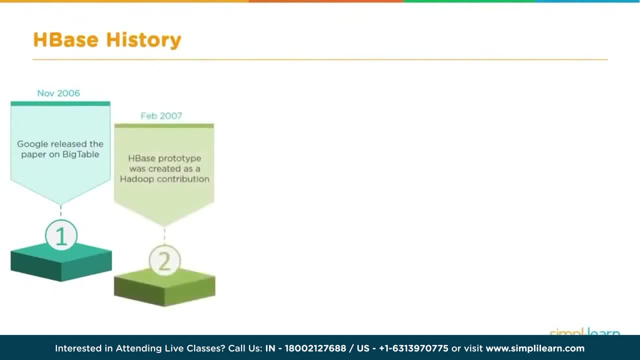 just a few months later, HBase prototype was created as a Hadoop contribution. Later on in the year 2007,. in October, first usable HBase along with the Hadoop 0.15 was released, And then in January of 2008,. 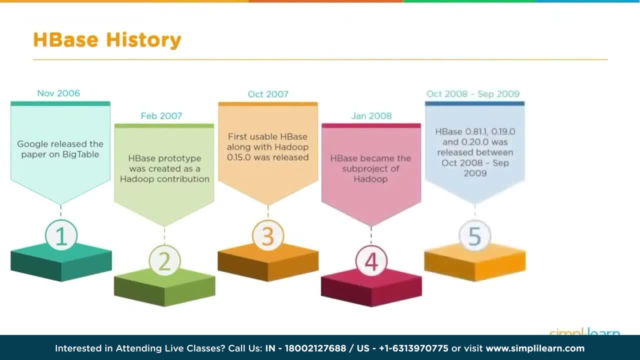 HBase became the subproject of Hadoop And later on that year, in October, all the way into September the next year, HBase was released, the 0.81 version, the 0.19 version and 0.20.. And finally, in May of. 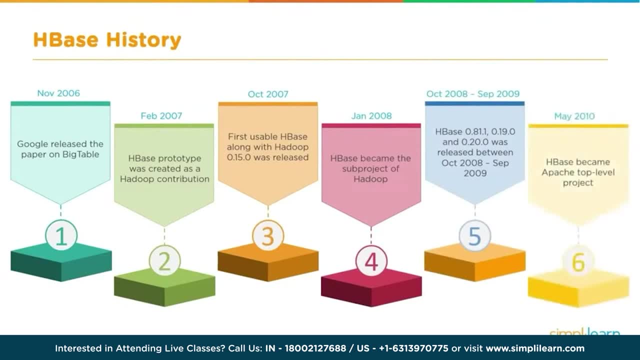 2010, HBase became Apache top level project And so you can see, in the course of about four years, HBase started off as just an idea on paper and has evolved all the way until 2010 as a solid project under the Apache And since. 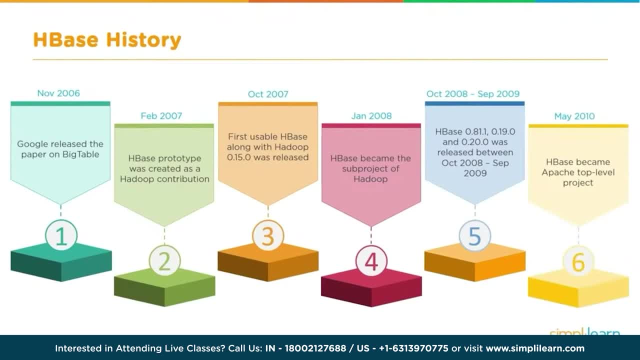 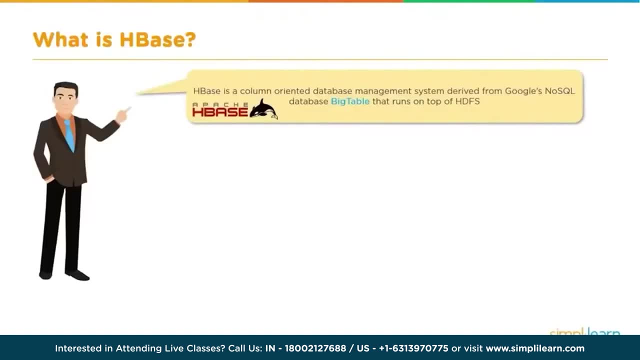 2010,. it's continued to evolve and grow as a major source for storing data in semi-structured data. So what is HBase? HBase is a column-oriented database management system derived from Google's NoSQL database Bigtable that runs on top of the. 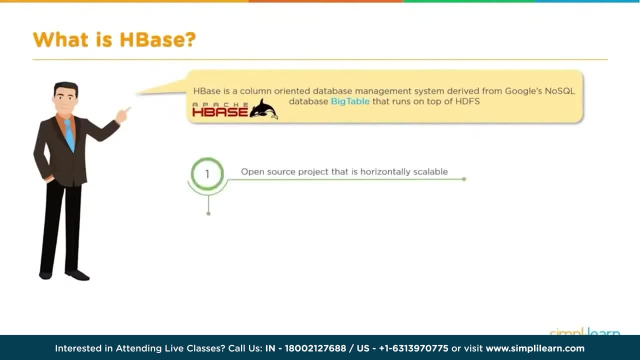 Hadoop file system or the HDFS. It's an open source project that is horizontally scalable And that's very important to understand, that you don't have to buy a bunch of huge, expensive computers. You're expanding it by continually adding commodity machines, And so it's. 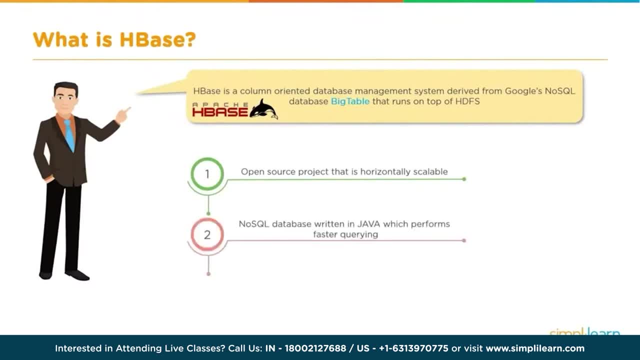 a linear cost expansion as opposed to being exponential NoSQL database written in Java, which permits faster querying. So Java is the back end for the HBase setup And it's well suited for sparse data sets, So it can contain missing or NA values and 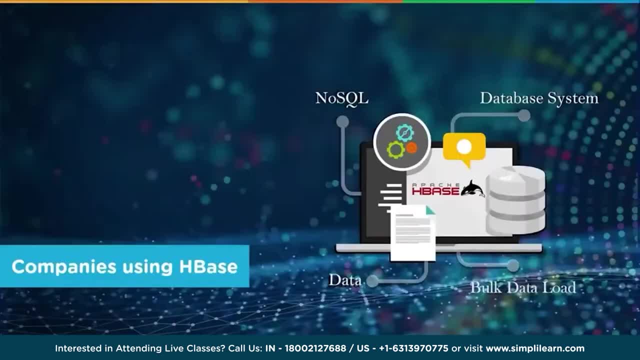 this doesn't boggle it down like it would another database Companies using HBase. So let's take a look and see who is using this NoSQL database for their servers and for storing their data. And we have Hortonworks, which isn't a surprise. 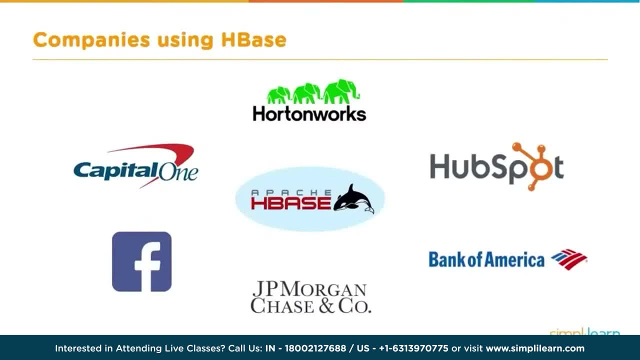 because they're one of the like Cloudera Hortonworks, They are behind Hadoop and one of the big developments and backing of it And, of course, Apache HBase is the open source behind it And we have Capital One as banks. 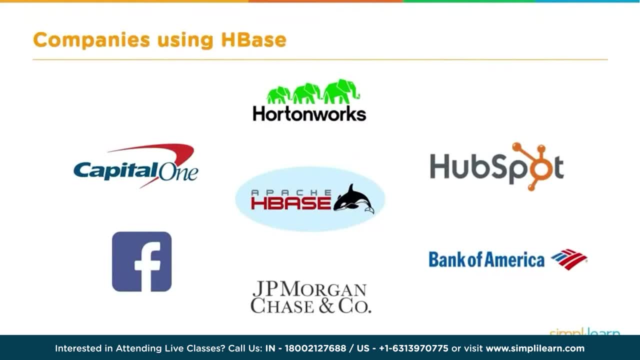 You also see Bank of America where they're collecting information on people and tracking it, So their information might be very sparse. They might have one bank way back when they collected information as far as the person's family and what their income for the whole family is. 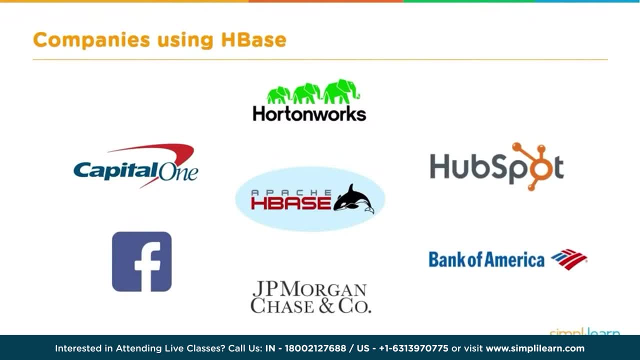 and their personal income, And maybe another one doesn't collect the family income, As he started saying, where you have data that is very difficult to store, where it's missing a bunch of data, HubSpot is using it. Facebook, certainly all of your Facebook, Twitter. 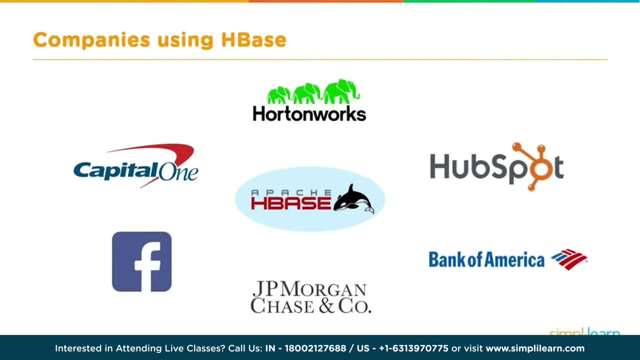 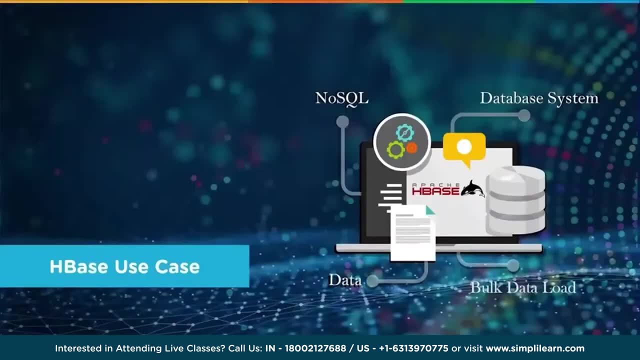 most of your social medias are using it. And then, of course, there's JP Morgan Chase and company, Another bank that uses the HBase as their data warehouse for NoSQL. Let's take a look at an HBase use case So we can dig. 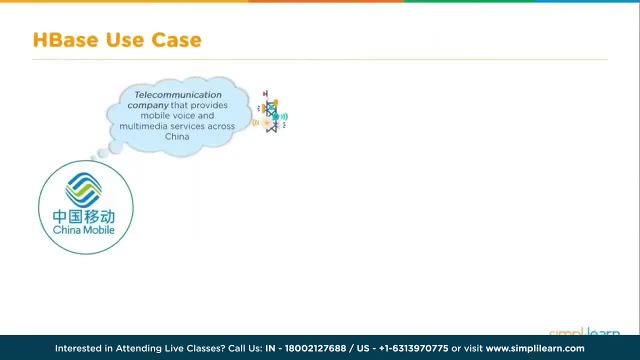 a little bit more into it to see how it functions. Telecommunication company that provides mobile voice and multimedia services across China, The China Mobile And China Mobile. they generate billions of call detailed records, or CDR, And so these CDRs and all. 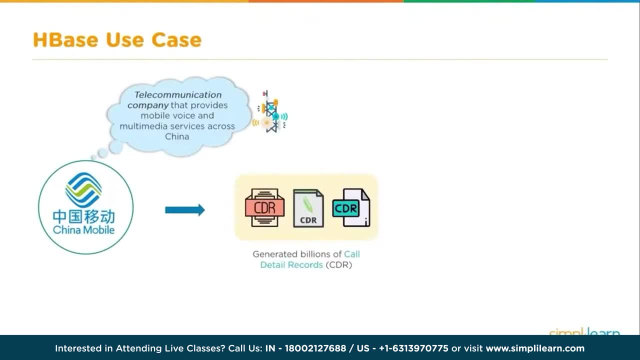 these records of these calls and how long they are, and different aspects of the call, Maybe the tower they're broadcasted from. All of that is being recorded so they can track it. A traditional database systems were unable to scale up to the vast volumes of data and provide a cost. 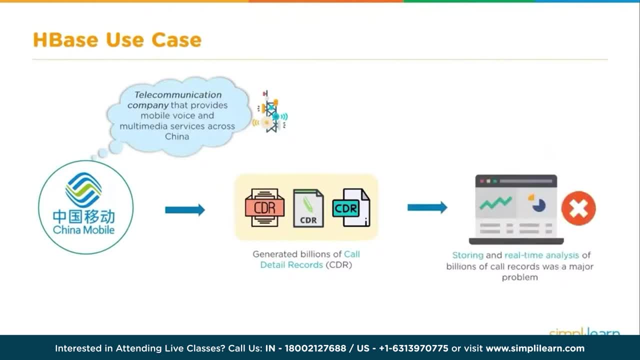 effective solution? No good. So storing in real time analysis of billions of call records was a major problem for this company Solution: Apache HBase. HBase stores billions of rows of detailed call records. HBase performs fast processing of records using SQL queries, So you can mix. 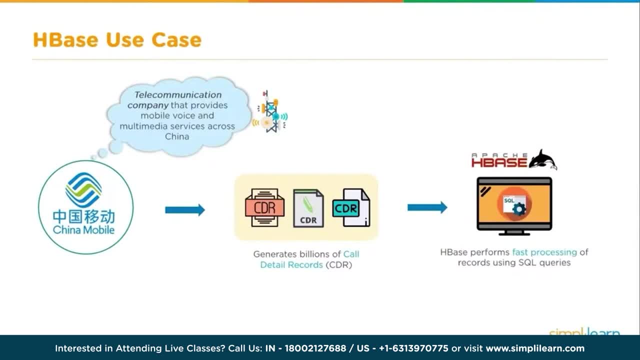 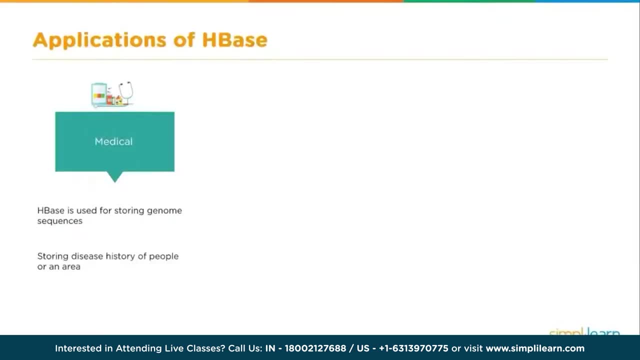 your SQL and NoSQL queries And easy to say NoSQL queries because of the way the query works- Applications of HBase. One of them would be in the medical industry. HBase is used for storing genome sequences, Storing disease history of people of an area. 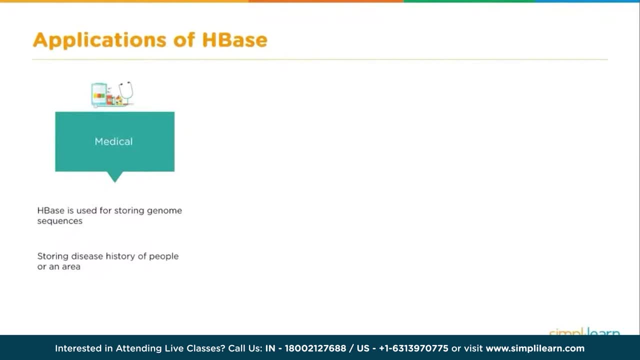 And you can imagine how sparse that is. as far as both of those A genome sequence might be only have pieces to it that each person is unique or is unique to different people, And the same thing with disease. You really don't need a column for every possible disease. 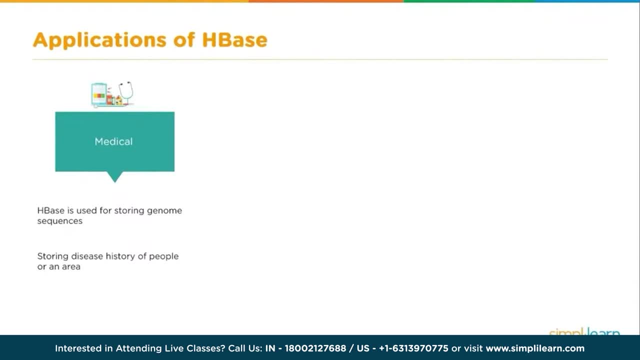 a person could get. You just want to know what those diseases, those people have had to deal with In that area. E-commerce HBase is used for storing logs about customer search history, Performs analytics and target advertisement for better business insights. Sports. 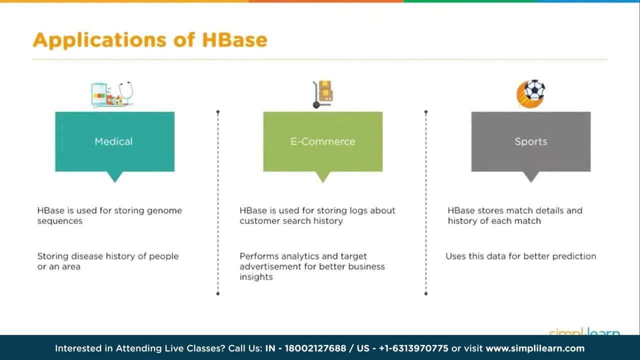 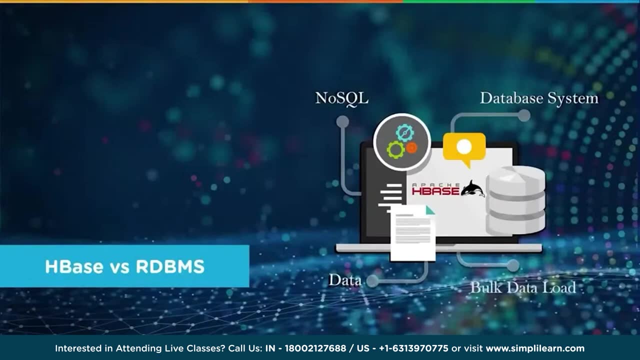 HBase stores match details and the history of each match, Uses this data for better prediction. So when we look at HBase, we all want to know what's the difference between HBase versus RDBMS, That is, a relational database management system. HBase versus 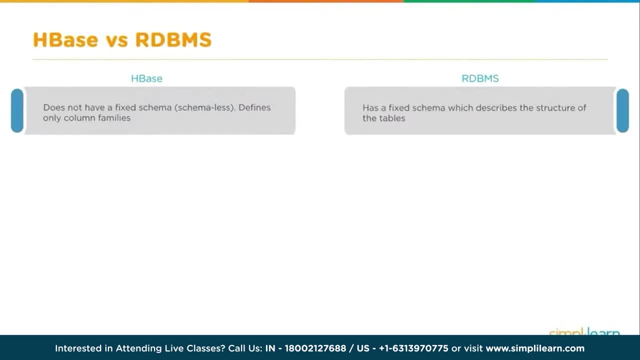 RDBMS. So the HBase does not have a fixed schema. It's schemaless, Defines only column families, And we'll show you what that means later on. RDBMS has a fixed schema which describes the structure of the tables. 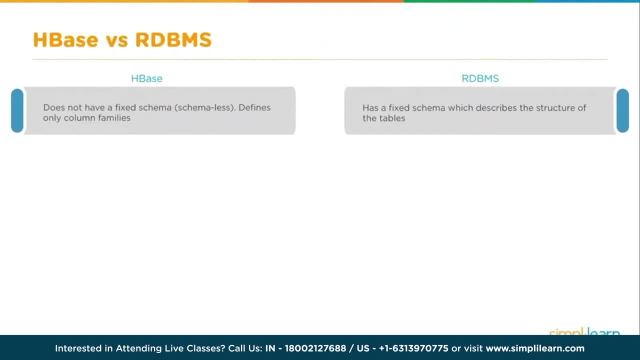 And you can think of this as you have a row and you have columns And each column is a very specific structure: How much data can go in there and what it does With the HBase. it works well with structured and semi-structured data. 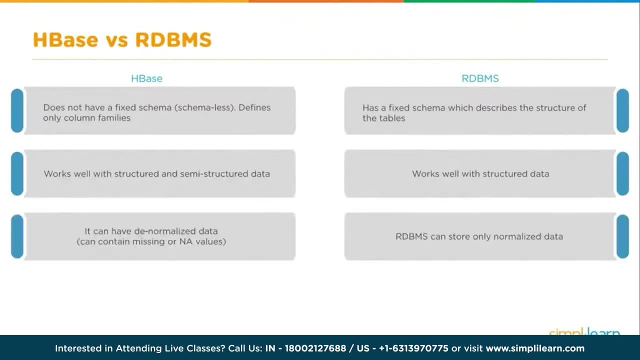 With the RDBMS it works only well with structured data. With the HBase it can have denormalized data. It can contain missing or null values. With the RDBMS it can store only normalized data. Now you can still store a null value. 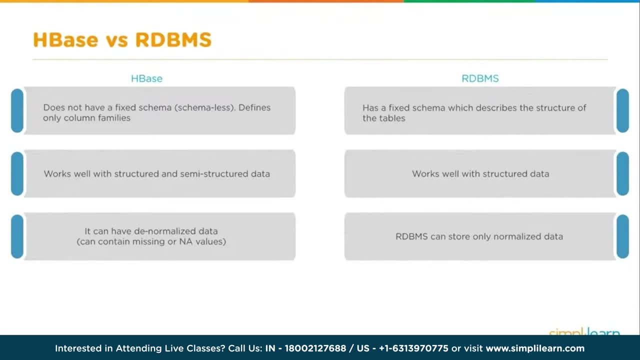 in the RDBMS, but it still takes up the same space as if you're storing a regular value in many cases, And it also for the HBase- is built for wide tables. It can be scaled horizontally, For instance, if you were doing a. 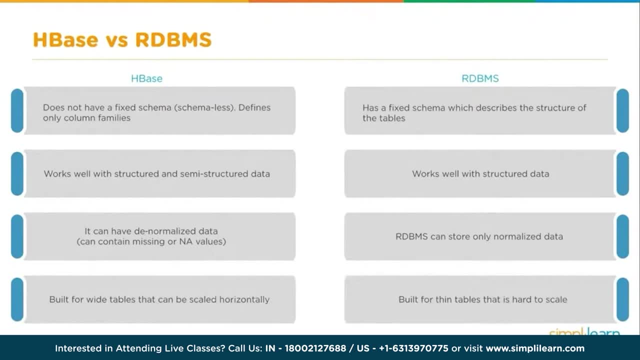 tokenizer of words and word clusters. you might have 1.4 million different words that you're pulling up and combinations of words. So with an RDBMS it's built for thin tables that are hard to scale. You don't want to store 1.4 million columns. 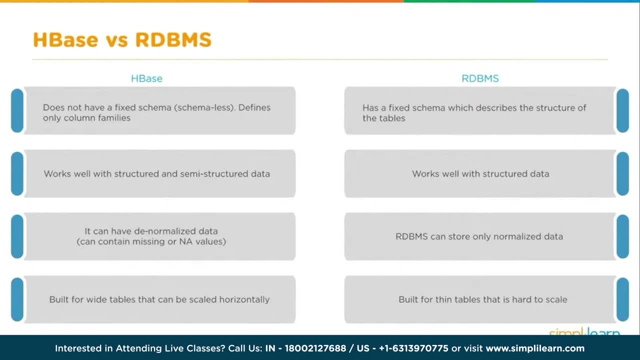 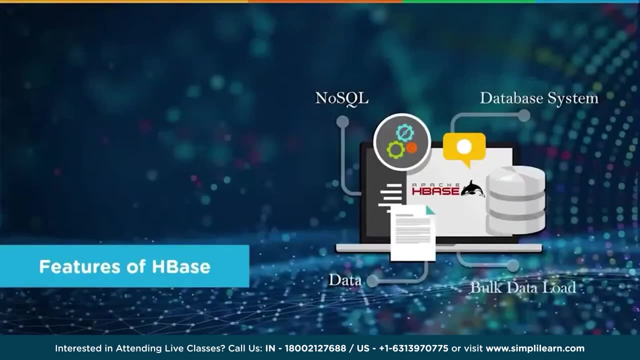 in your SQL. It's going to crash and it's going to be very hard to do searches With the HBase. it only stores that data, which is part of whatever row you're working on. Let's look at some of the features of the HBase. It's scalable. 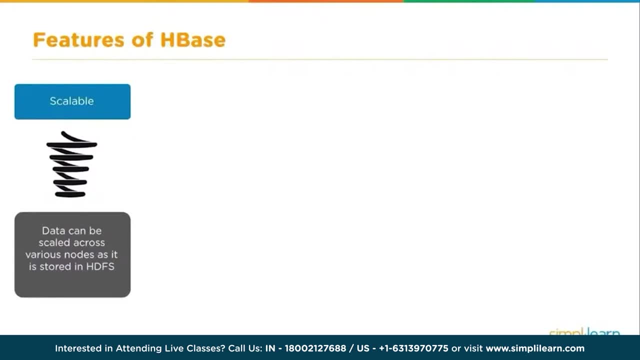 Data can be scaled across various nodes as it is stored in the HDFS, And I always think about this. it's a linear add-on. For each terabyte of data, I'm adding on roughly a thousand dollars in commodity computing With an enterprise machine. 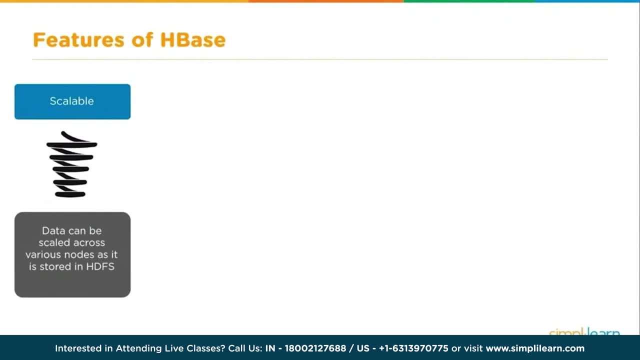 we're looking at about ten thousand at the lower end for each terabyte of data, And that includes all your backup and redundancy. So it's a big difference. It's like a tenth of the cost to store it across the HBase It has automatic. 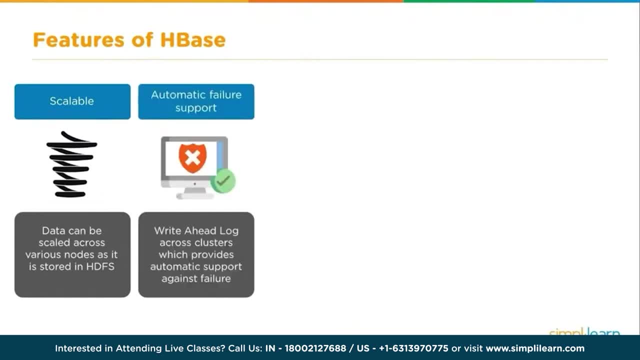 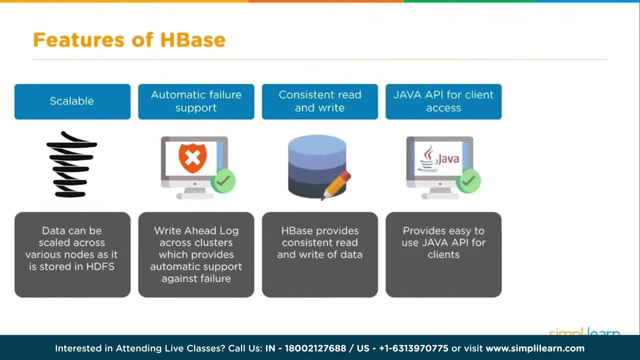 failure support Right ahead. log across clusters, which provides automatic support against failure. Consistent read and write HBase provides consistent read and write of the data. It's a Java API for client access. Provides easy to use Java API for clients. Block cache and bloom filters. 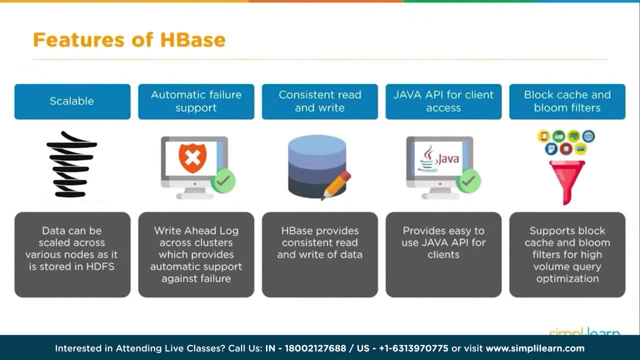 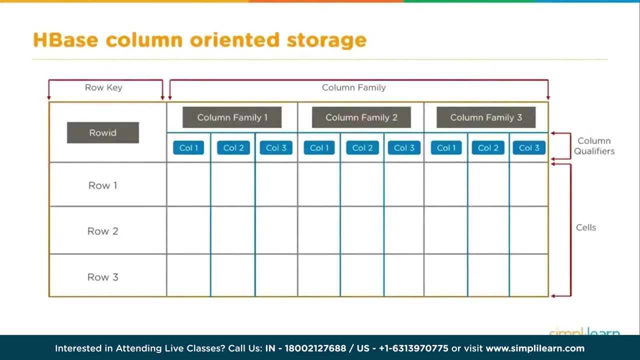 So the HBase supports block caching and bloom filters for high volume query optimization. Let's dig a little deeper into the HBase storage, HBase column oriented storage- And I told you we're going to look into this to see how it stores the data. And here you can see. 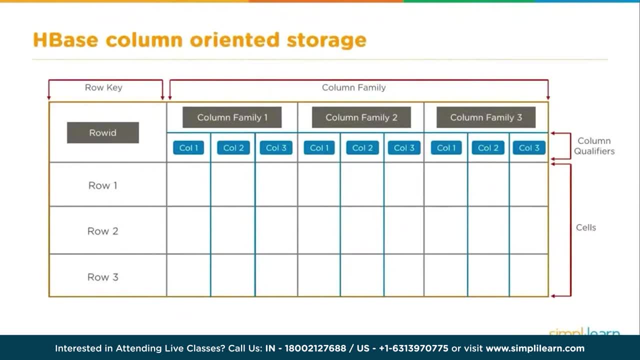 you have a row key, And this is really one of the important references is each row has to have its own key or your row ID. And then you have your column family And in here you can see we have column family 1, column family 2, column. 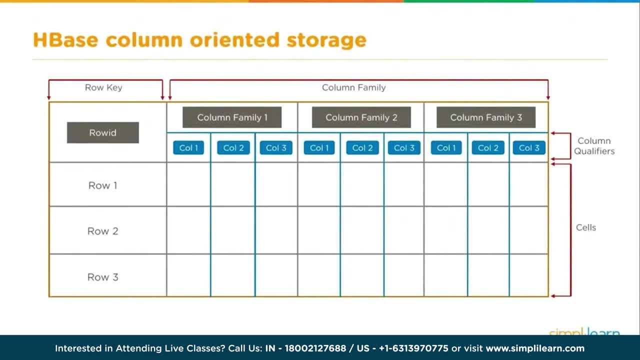 family 3. And you have your column qualifiers So you can have in column family 1, you can have three columns in there And there might not be any data in that. So when you go into column family 1 and do a query for every column that contains 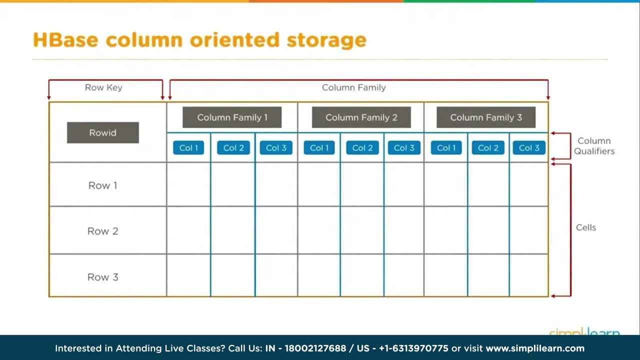 a certain thing, that row might not have anything in there and not be queried Where. in column family 2, maybe you have column 1 filled out and column 3 filled out, And so on and so forth, And then each cell is connected to the row. 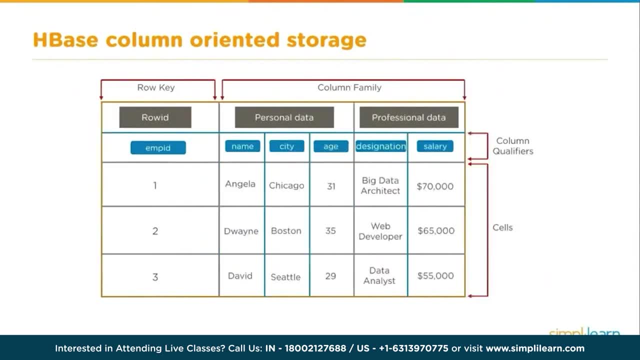 where the data is actually stored. Let's take a look at this and what it looks like when you fill the data in. So in here we have a row key with a row ID And we have our employee ID 123.. Let's 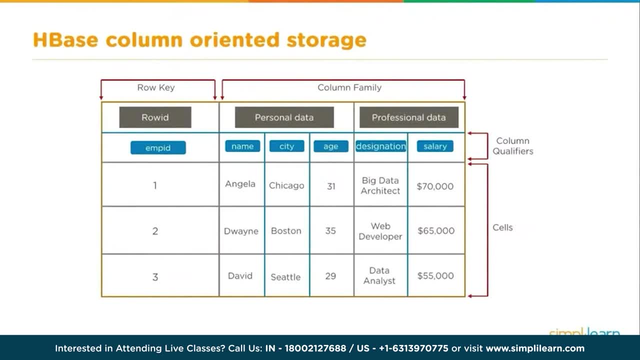 take a look at that. It's pretty straightforward. You probably would even have that on an SQL server And then you have your column family. This is where it starts really separating out. Your column family might have personal data And under personal data you would have name city. 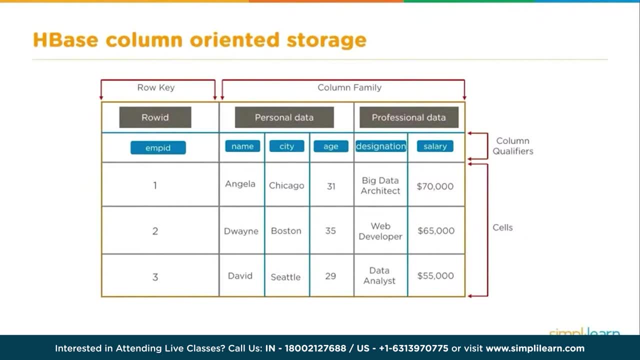 age. You might have a lot more than just that. You might have number of children, You might have degree, All those kinds of different things that go under personal data, And some of them might be missing. You might only have the name and the age. 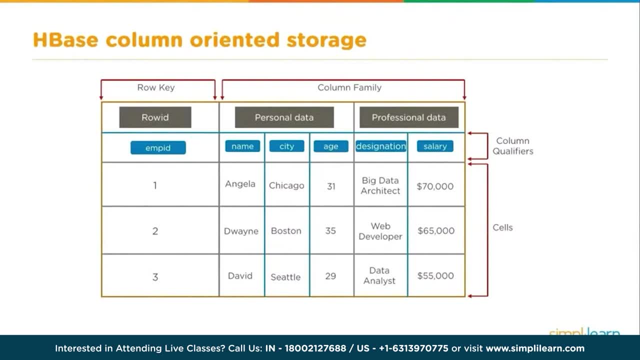 of an employee. You might only have the name, the city and how many children, And not the age, And so you can see with the personal data. you can now collect a large variety of data and store it in the HBase very easily, And then maybe you have a family. 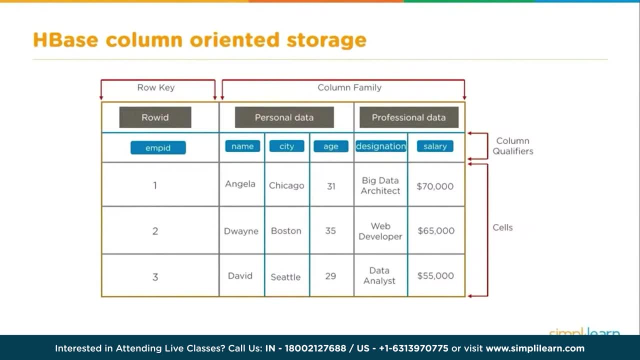 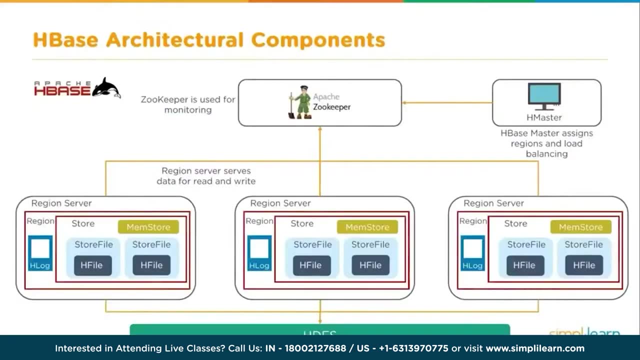 of professional data, Your designation, your salary, all the stuff that the employee is doing for you in that company. Let's dig a little deeper into the HBase architecture And so you can see here what looks to be a complicated chart. It's not as complicated as you. 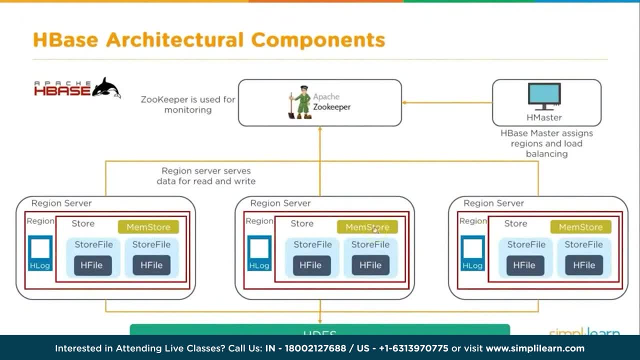 think From the Apache HBase. we have the Zookeeper, which is used for monitoring what's going on, And you have your HMaster. This is the HBase master assigns regions and load balancing And then, underneath the region or the HBase, 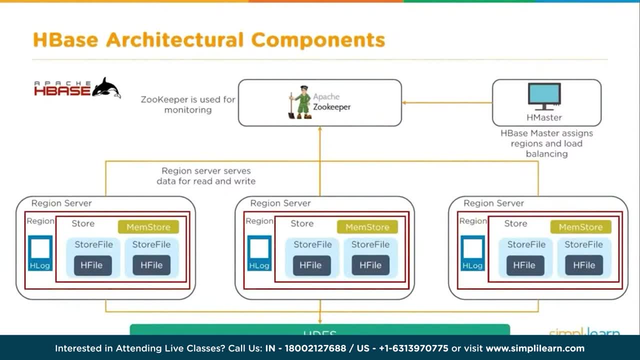 master. then under the HMaster or HBase master, you have your Read. Your Server Serves data for read and write, And the region server, which is all your different computers you have in your Hadoop cluster. you'll have a region. 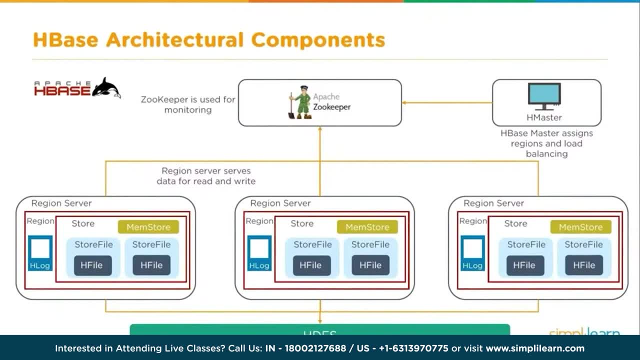 an HLog. you'll have a store memory store and then you have your different files for HFile that are stored on there And those are separated across the different computers And that's all part of the HDFS storage system. So when we look at the architectural components, 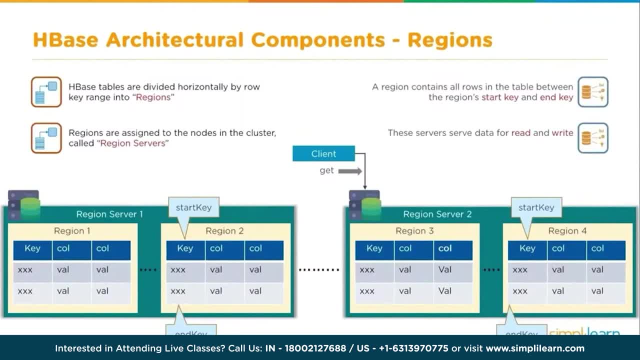 or regions, and we're drilling down a little bit. HBase tables are divided horizontally by a row, So you have a key range into regions. So each of those IDs you might have IDs 1 to 20,, 21 to 50,. 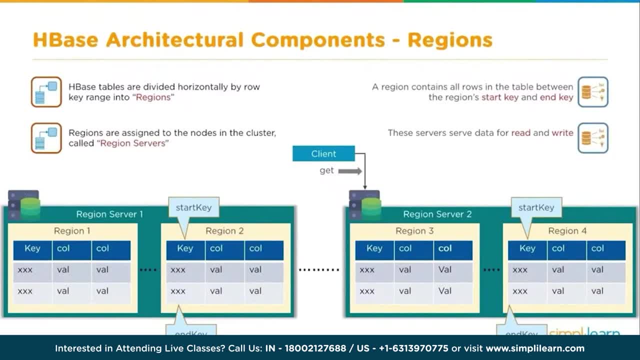 or whatever they are. Regions are assigned to the nodes in the cluster called region servers. A region contains all rows in the table between the region start key and the end key, Again 1 to 10,, 11 to 20, and so forth. These servers serve. 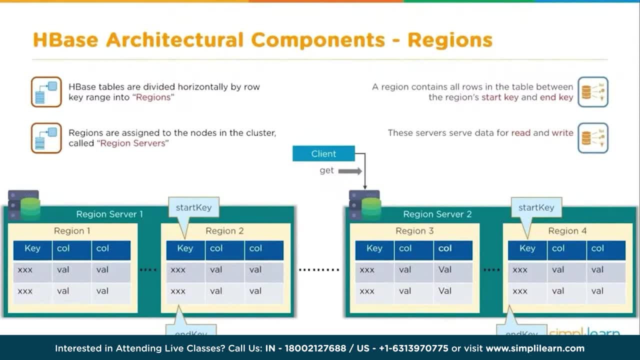 data for read and write. And you can see, here we have the client and the get and the get sends it out and it finds out where that start, if it's between which start keys and end keys, and then it pulls the data. 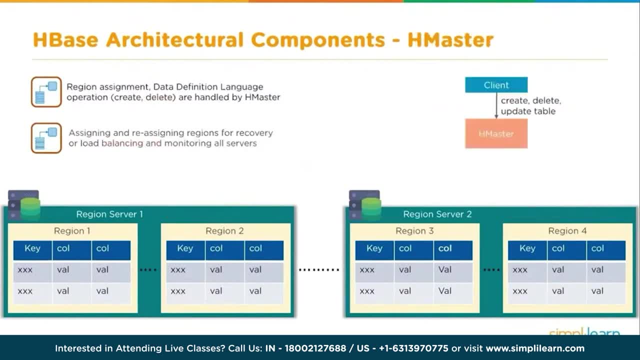 from that different region server And so the region sign data, definition, language operation, create, delete are handled by the HMaster. So the HMaster is telling it: what are we doing with this data? what's going out there Assigning and reassigning regions? 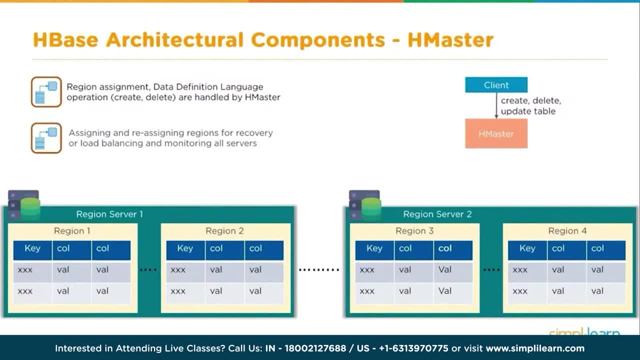 for recovery or load balancing and monitoring all servers. So that's also part of it. So you know your IDs. if you have 500 IDs across 3 servers, you're not going to put 400 IDs on server 1 and 100 on server 2. 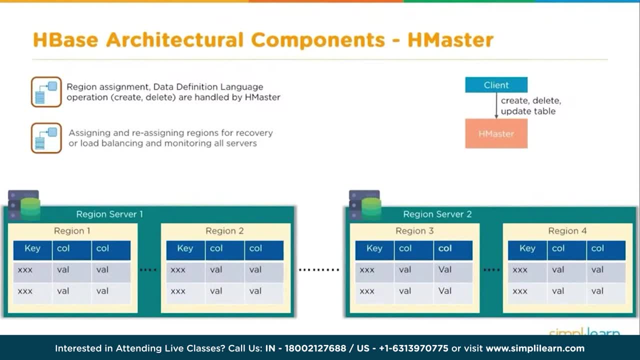 and leave region 3 and region 4 empty. You're going to split that up And that's all handled by the HMaster And you can see here: it monitors region servers, assigns regions to region servers. assigns regions to region servers. 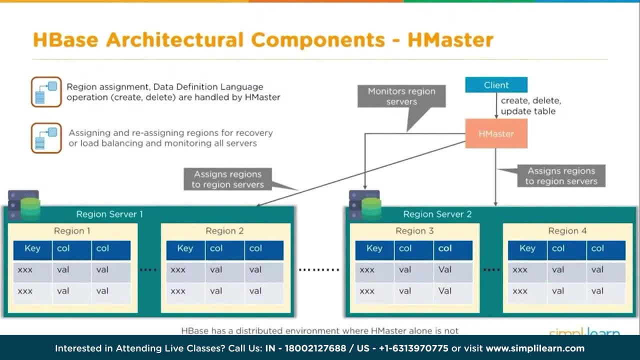 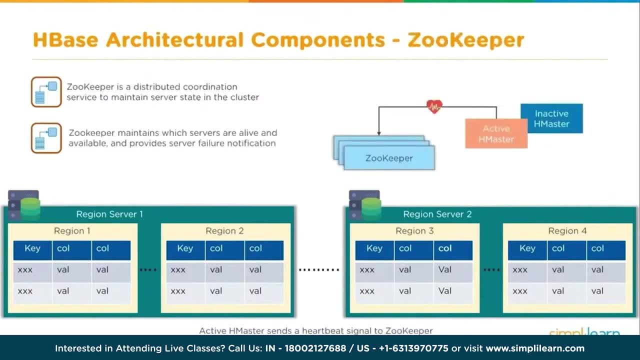 and so forth and so forth. HBase has a distributed environment where HMaster alone is not sufficient to manage everything. Hence ZooKeeper was introduced. It works with HMaster, So you have an active HMaster which sends a heartbeat signal to ZooKeeper, indicating 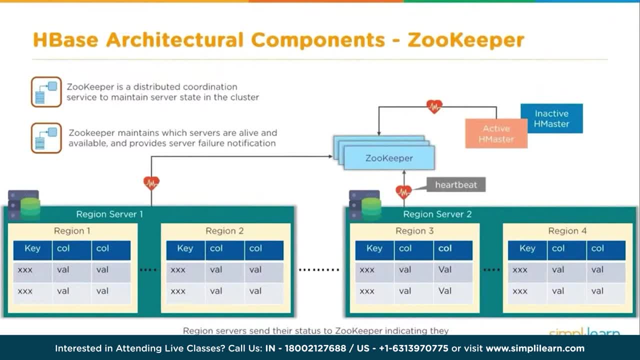 that it's active. And the ZooKeeper also has a heartbeat to the region servers. So the region servers send their status to ZooKeeper, indicating they are ready for read and write operation. Inactive server acts as a backup If the active HMaster fails. 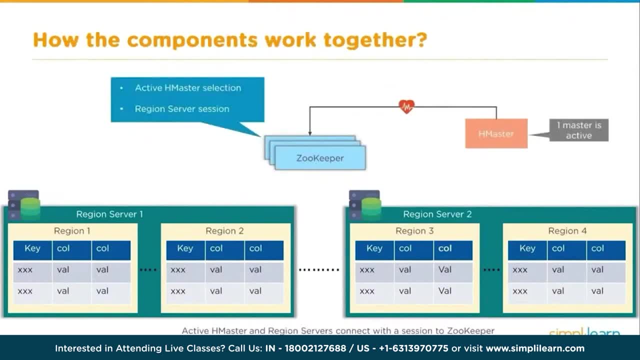 it will come to the rescue. Active HMaster and region servers connect with a session to ZooKeeper. So you see your active HMaster selection region server session. They're all looking at the ZooKeeper keeping that pulse. An active HMaster and region server connects with a session. 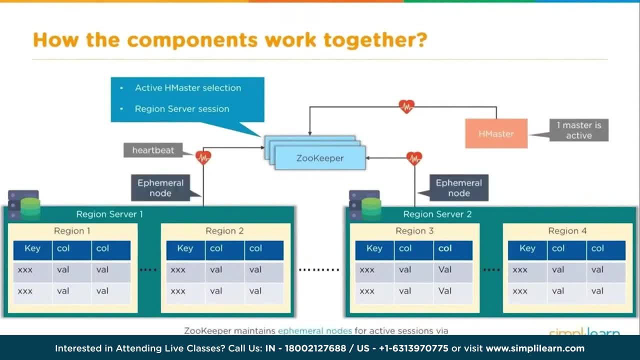 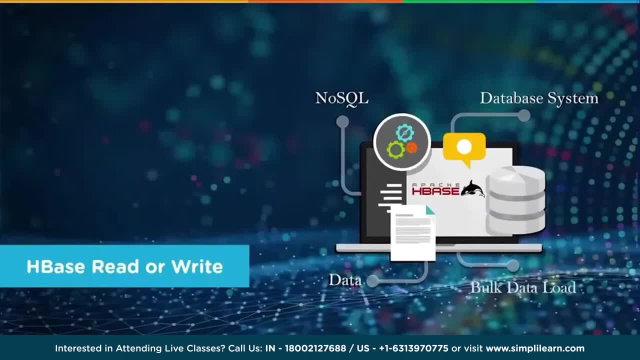 to the ZooKeeper And you can see here where we have ephemeral nodes for active sessions via heartbeats to indicate that the region servers are up and running. So let's take a look at HBase. read or write going on. There's a special HBase catalog. 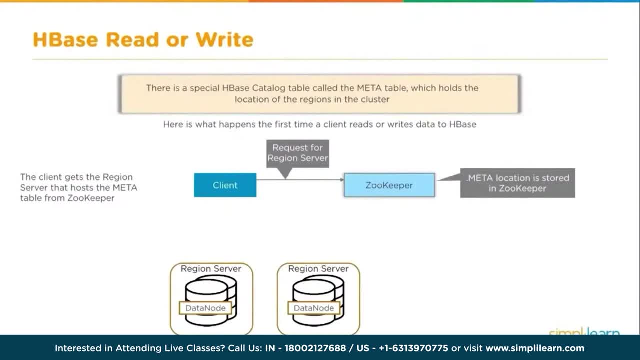 table called the meta table, which holds the location of the regions in the cluster. Here's what happens: the first time a client reads or writes data to HBase, The client gets the region server, the host, the meta table from ZooKeeper and you can see right here the client. 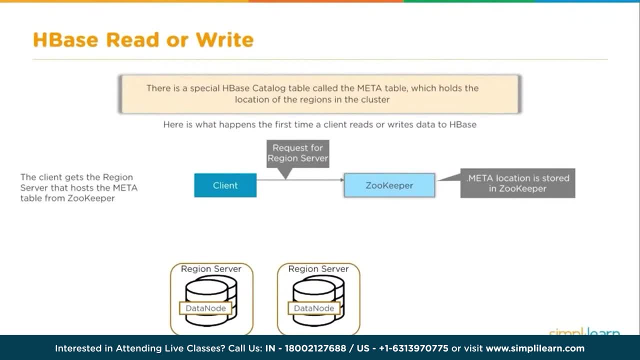 has a request for your region server and goes, hey, ZooKeeper, can you handle this? The ZooKeeper takes a look at it and goes, ah, meta location is stored in ZooKeeper, So it looks at its meta data on there. And then the meta data table. 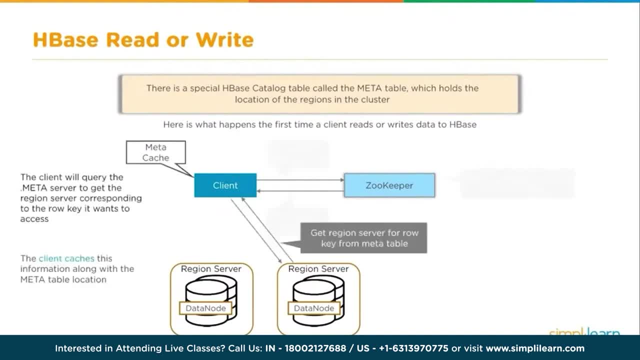 location is sent back to the client. The client will query the meta server to get the region server corresponding to the row key if it wants to access. The client caches this information along with the meta table location And you can see here the client going back and forth to the region. 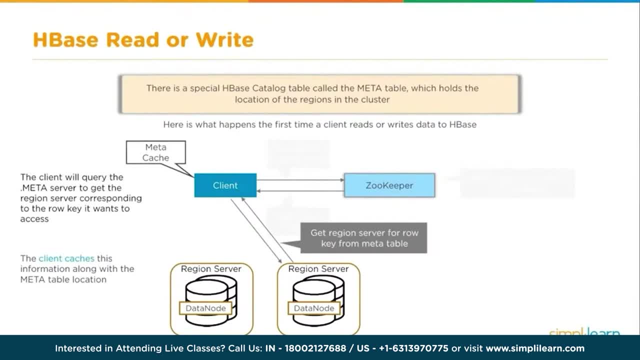 server with the information And it might be going across multiple region servers, depending on what you're querying. So we get the region server for row key from the meta table. That's where that row key comes in and says, hey, this is where we're going with this. 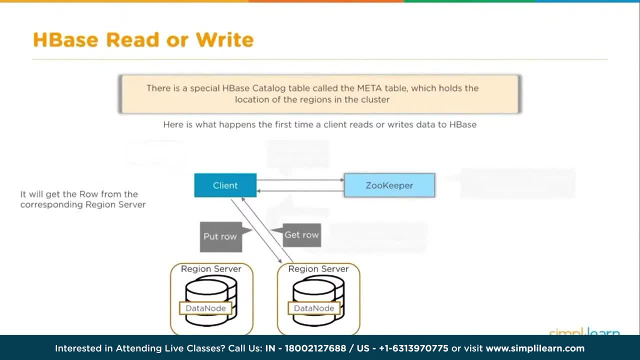 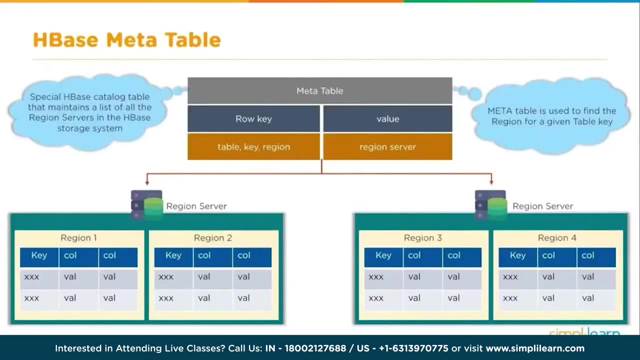 And so once it gets the row key from the corresponding region server, we can now put row or get row from that region server. Let's take a look at the HBase meta table, Special HBase catalog table that maintains a list of all the region servers. 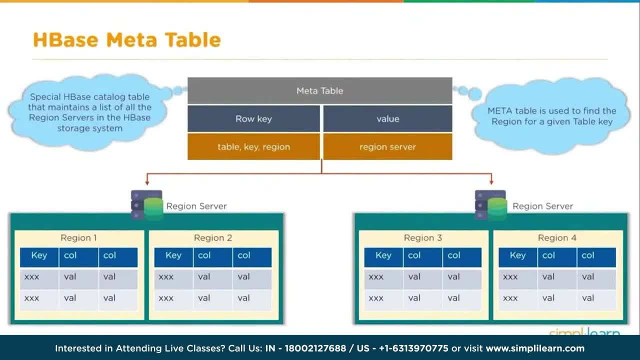 in the HBase storage system. So you see, here we have the meta table, We have our row key and a value table key: region, region server. So the meta table is used to find the region for the given table key And you can see down here. 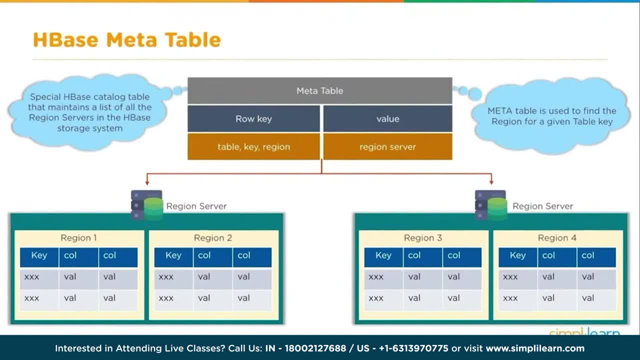 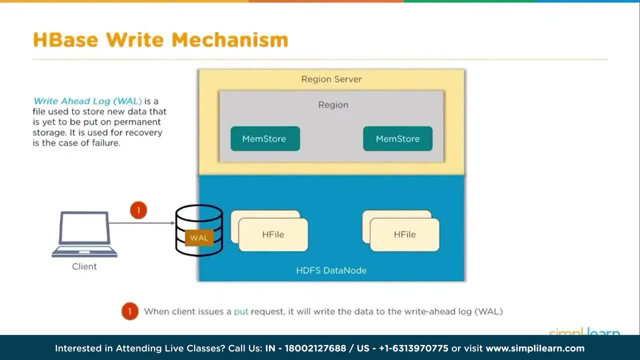 our meta table comes in and it's going to figure out where it's going with the region server And we look a little closer at the write mechanism. in HBase We have write ahead log, or wall as you abbreviate it, Kind of a way to remember. 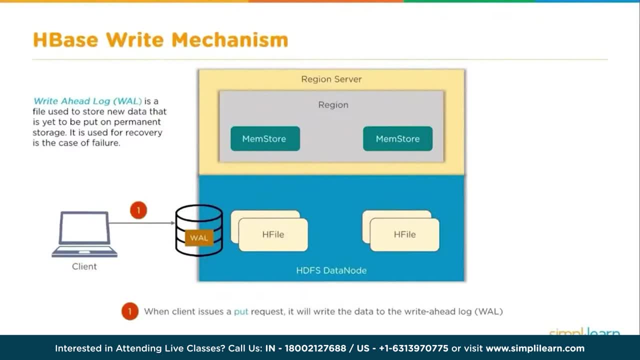 wall is write ahead log. It's a file used to store new data that is yet to be put on permanent storage. It is used for recovery in the case of failure, So you can see here where the client comes in and it literally puts the. 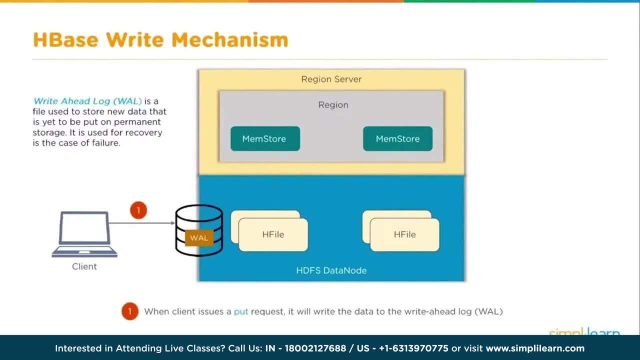 new data coming in into this kind of temporary storage or the wall on there. Once it's gone into the wall, then the memory store memstore is a write cache that stores the new data that has not yet been written to disk. There is one. 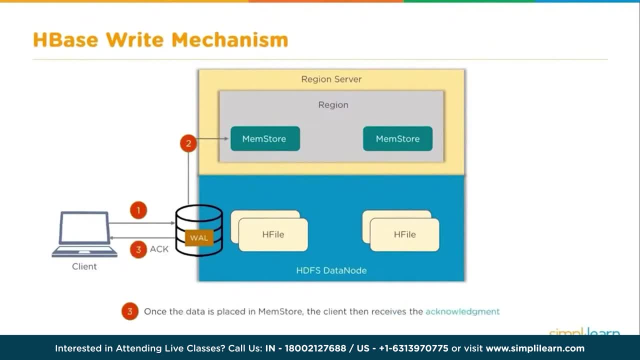 memstore per column family per region, And once we've done that, we have three ACK. Once the data is placed in memstore, the client then receives the acknowledgement. When the memstore reaches the threshold, it dumps or commits the data into HFile. 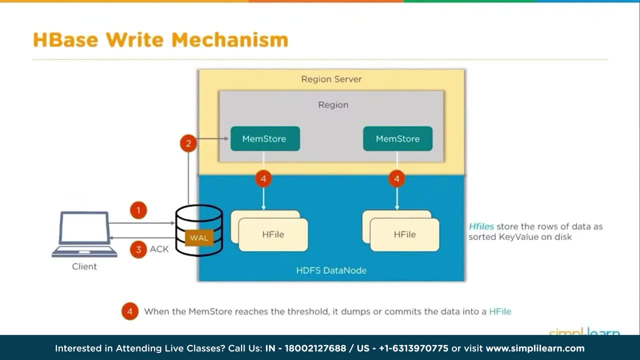 So you can see right here: we've taken our. it's gone into the wall. The wall then sorts it into the different memory stores And then the memory stores it says, hey, we're ready to dump that into our HFiles. 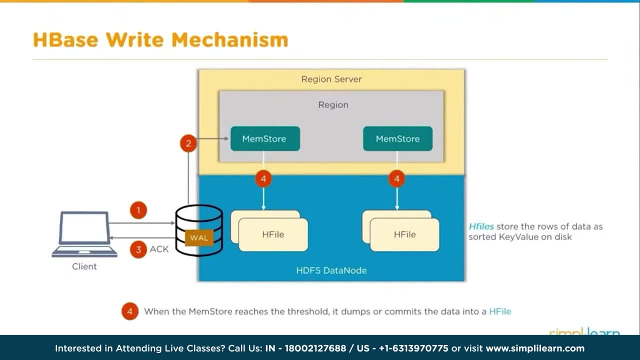 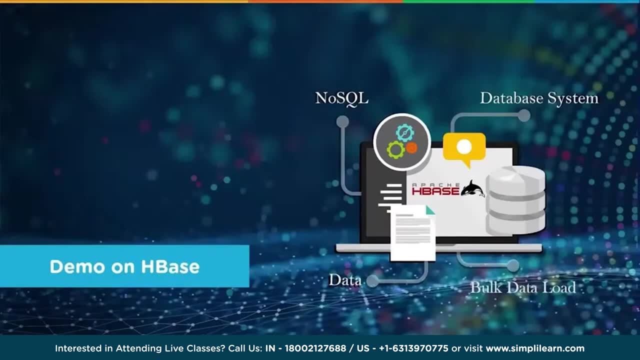 And then it moves it into the HFiles. HFiles store the rows of data as stored key value on disk. So here we've done a lot of theory. Let's dive in and just take a look and see what some of these commands look like. 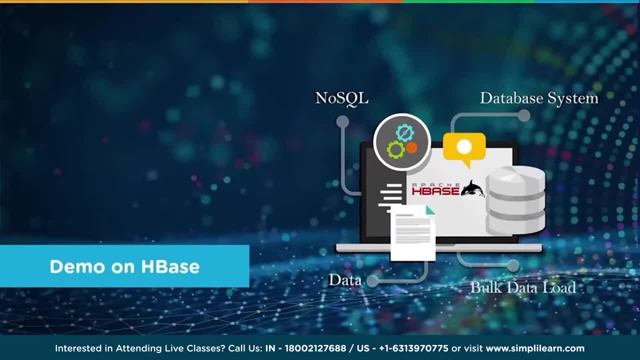 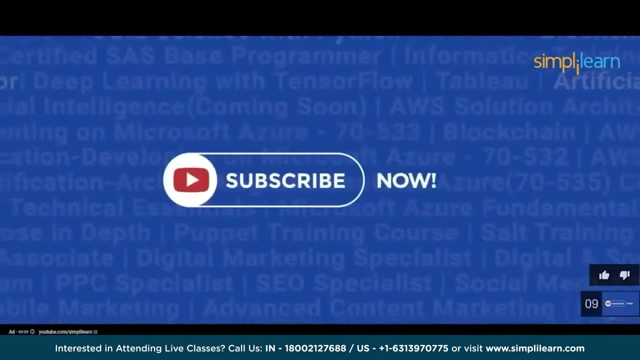 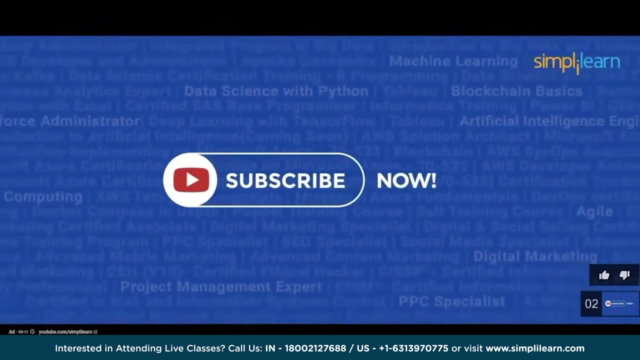 and what happens in our HBase when we're manipulating a NoSQL setup. So if you're learning a new setup, it's always good to start with. where is this coming from? It's open source by Apache And you can go to hbaseapacheorg. 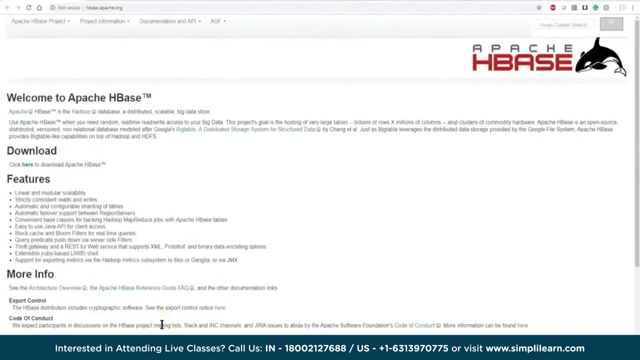 And you'll see that it has a lot of information. You can actually download the HBase separate from the Hadoop, although most people just install the Hadoop because it's bundled with it, And if you go in here you'll see that it has a lot of information. 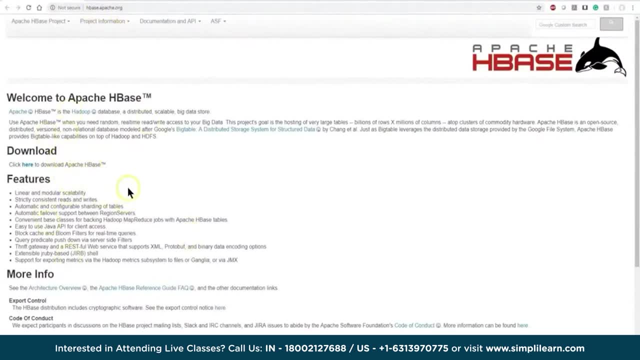 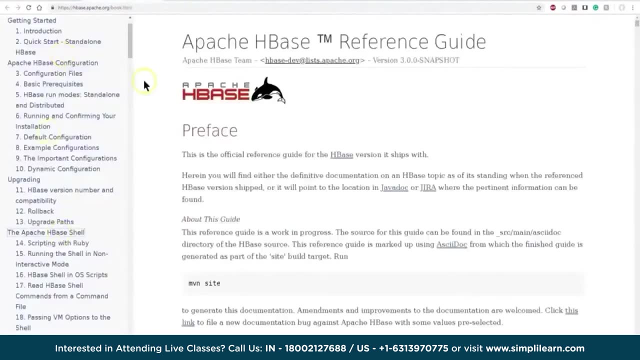 You can actually download the HBase separate from the Hadoop, although most people just install the Hadoop separate from the Hadoop. So you'll find a reference guide. You can go through the Apache reference guide. There's a number of things to look at. 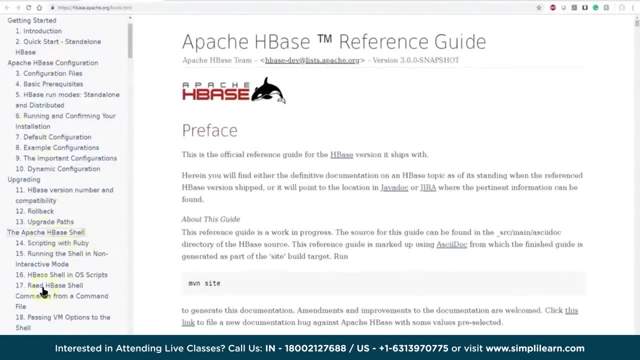 but we're going to be going through Apache HBase shell. That's what we're going to be working with. There's a lot of other interfaces on the setup. You can look up a lot of the different commands on here. So we go into the Apache HBase reference guide. 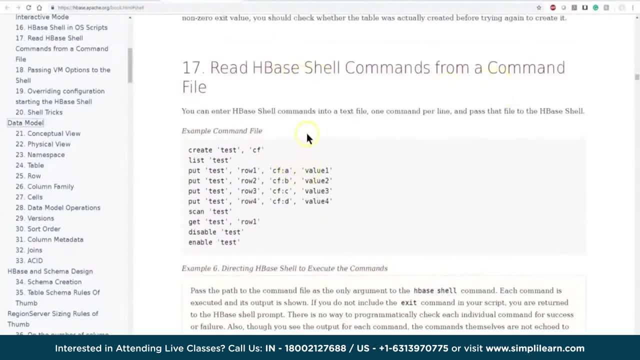 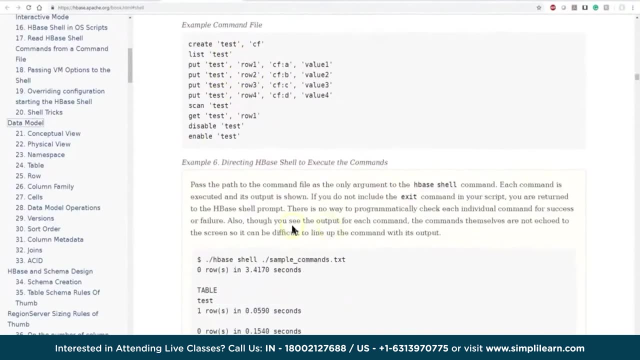 We can go down to read HBase shell commands from a command file. You can see here where it gives you different options of formats for putting the data in and listing the data. Certainly, you can also create files and scripts to do this too. 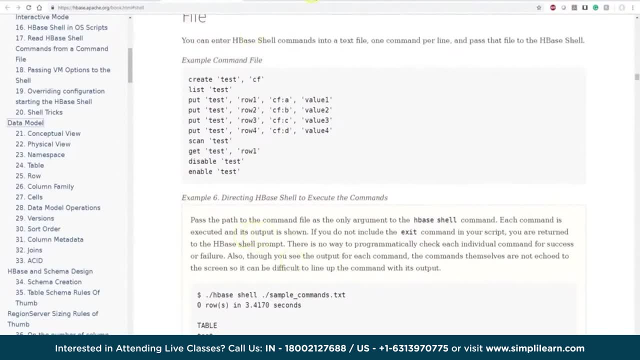 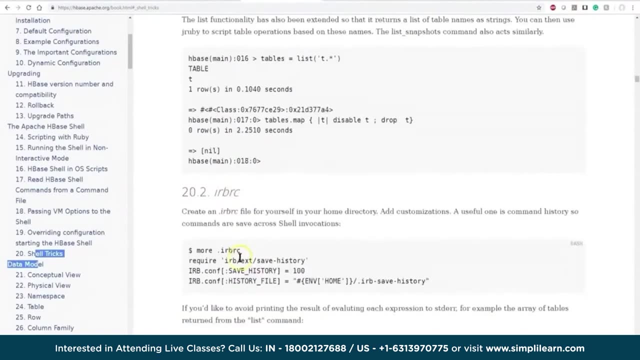 We're going to look at the basics. We're going to go through this on a basic HBase shell. One last thing to look at is, of course, if you continue down the setup, you can see here where they have more detail as far as how to create. 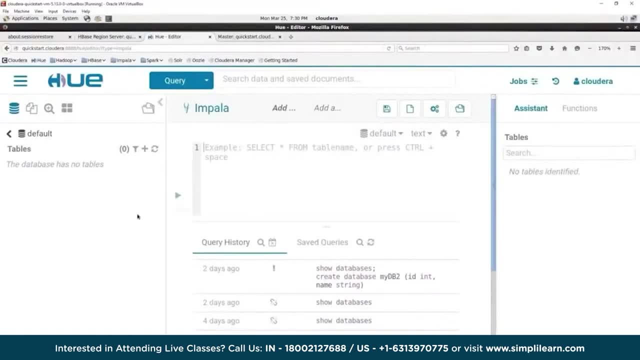 and how to get to your data on your HBase. Now I will be working in a virtual box. This is by Oracle. You can download the Oracle virtual box. You can put a note in below for the YouTube, as we did have a previous. 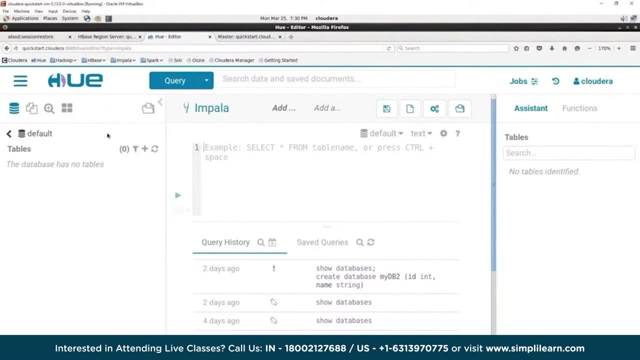 session on setting up virtual setup to run your Hadoop system. in there I'm using the Cloudera Quick Start installed in here. There's Horton's. You can also use the Amazon Web Service. There's a number of options for trying this out. In this case, we have 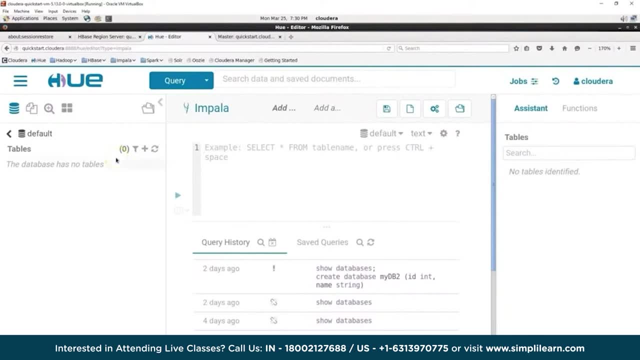 Cloudera on the Oracle virtual box. The virtual box has Linux CentOS installed on it and then the Hadoop has all the different Hadoop flavors, including HBase, And I bring this up because my computer is a Windows 10.. The operating system: 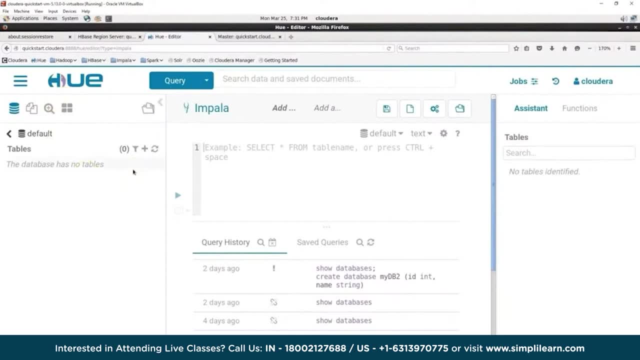 of the virtual box is Linux and we're looking at the HBase data warehouse. We have three very different entities all running on my computer. That can be confusing. if it's the first time in and working with this kind of setup, You'll notice in our 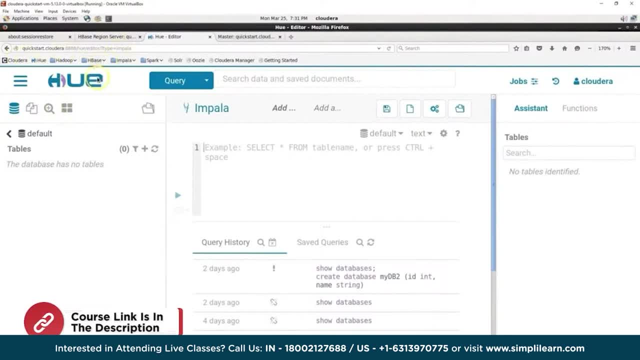 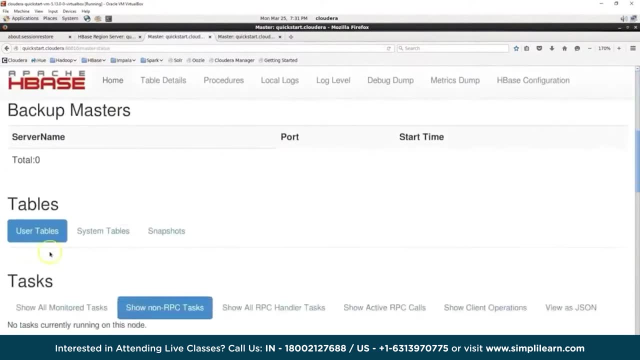 Cloudera setup. they actually have some HBase monitoring. I can go underneath here and click on HBase and master. It will tell me what's going on with my region servers. It will tell me what's going on with our backup tables. Right now I don't have 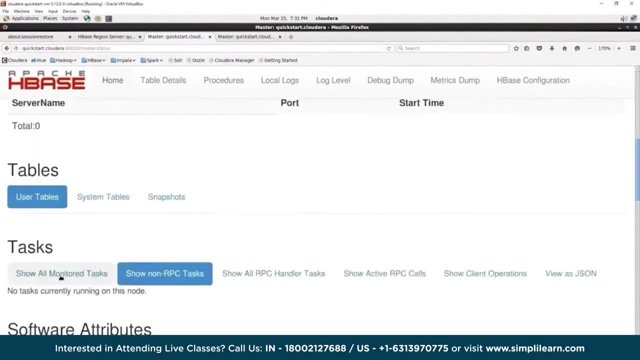 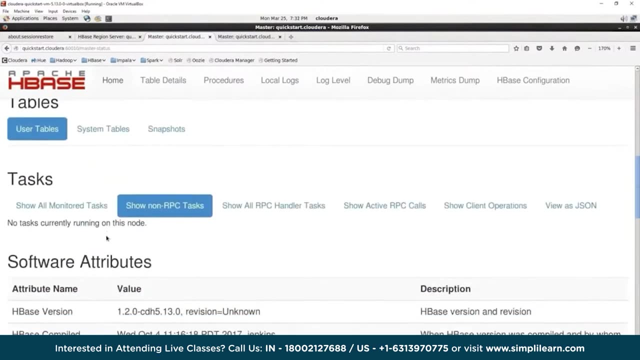 any user tables, because we haven't created any. This is only a single node and a single HBase. Tor, You're not going to expect anything too extensive in here, since this is for practice and education and perhaps testing out the package you're working on. 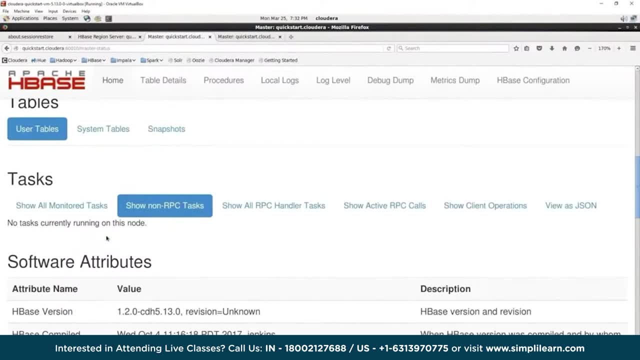 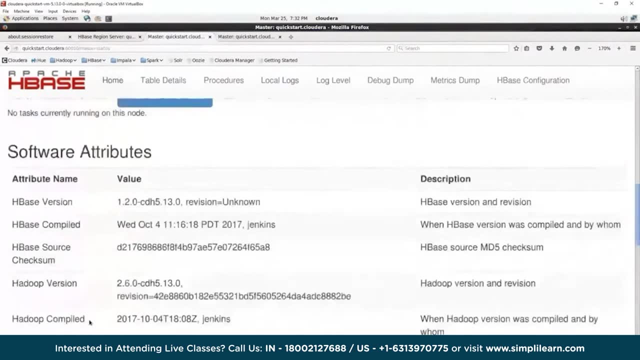 You can deploy Cloudera, of course, but when you talk about a quick start or a single node setup, that's what it's really for. So we can go through all the different HBases and you'll see all kinds of different information with Zookeeper, if you saw. 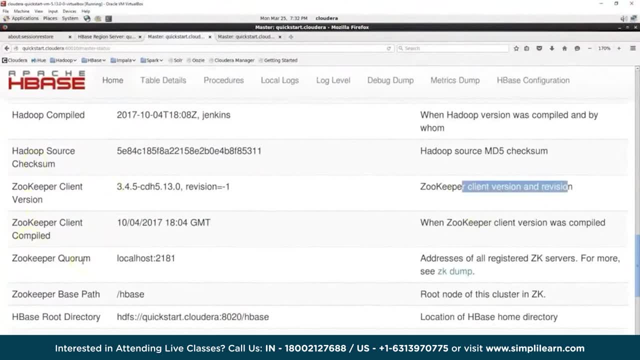 it flash by down here what version we're working in, since Zookeeper is part of the HBase setup. Where we want to go is we want to open up a terminal window, And in Cloudera it happens to be up at the. 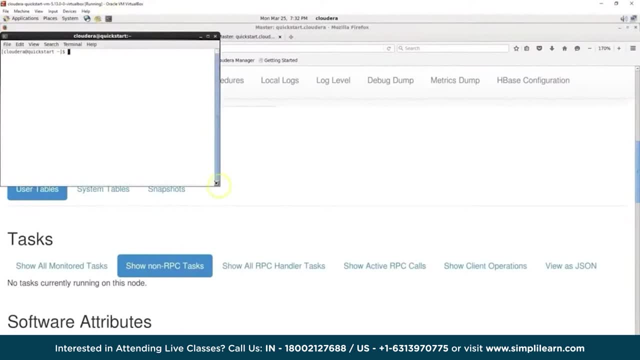 top, And when you click on here you'll see your Cloudera terminal window open. And let me just expand this so we have a nice full screen, And then I'm also going to zoom in. That way I have a nice big. 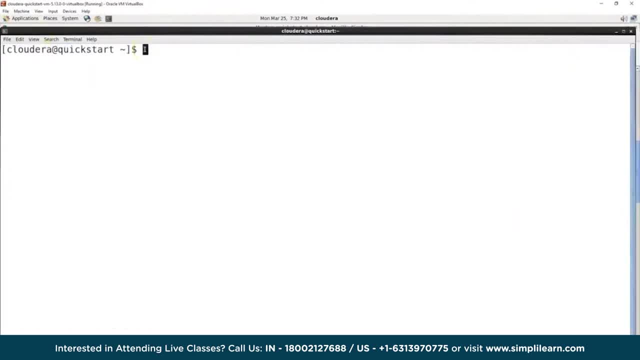 picture and you can see what I'm typing and what's going on. And to open up your HBase shell, simply type HBase shell to get in and hit enter And you'll see. it takes just a moment to load And we'll be in our HBase. 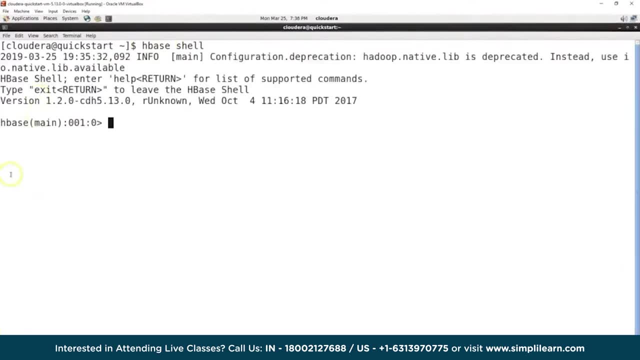 shell for doing HBase commands. Once we've gotten into our HBase shell, you'll see you'll have the HBase prompt information ahead of it. We can do something simple like list, And this is going to list whatever tables we have. 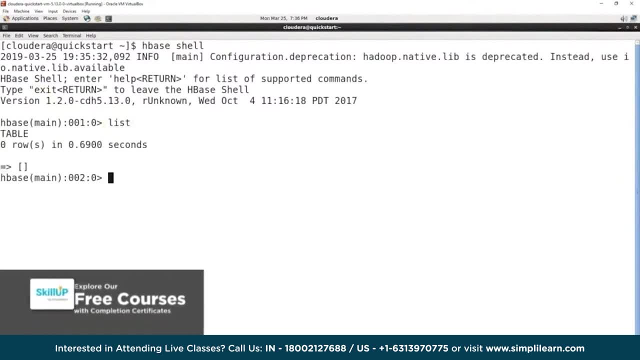 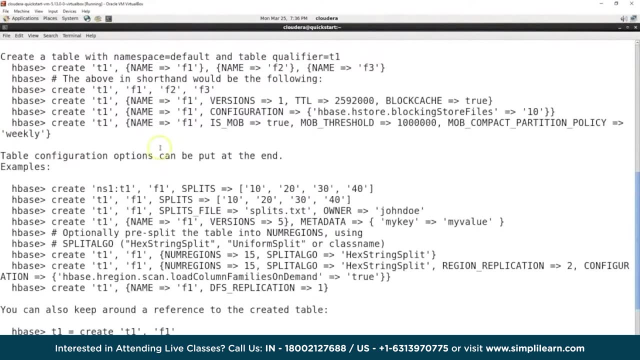 And it so happens that there's a base table that comes with HBase. Now we can go ahead and create, And I'm going to type in: just create. What's nice about this is it's going to throw me kind of a. it's going to say, hey, there's no, just straight. 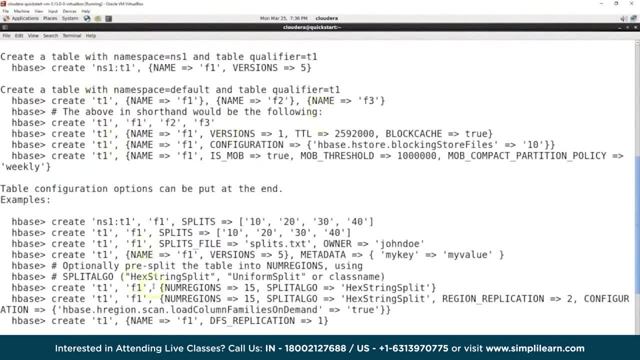 create, But it does come up and tell me all these different formats we can use for create, So we can create our table and one of our families. You can add splits, names, versions, all kinds of things you can do with this. But let's just start with a very basic. 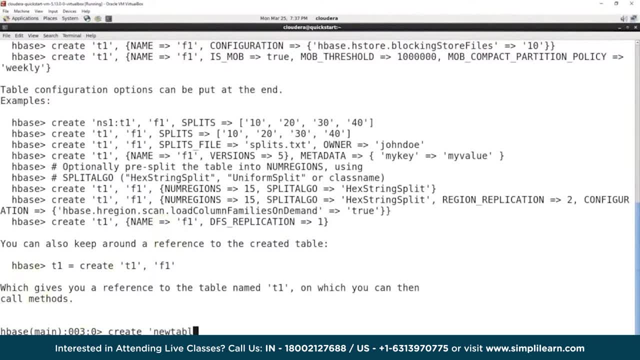 one on here And let's go ahead and create And we'll call it new table, Let's just call it new TBL for table, New table. And then we also want to do, let's do- knowledge. So let's take a look at this. I'm creating a new table. 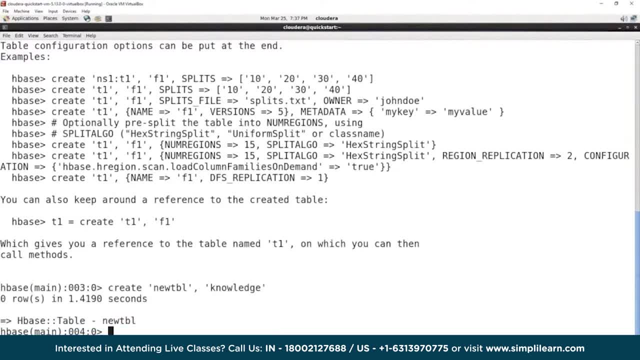 and it's going to have a family of knowledge in it. And let me hit enter, It's going to come up. It's going to take it a second to go ahead and create it Now. we have our new table in here, So if I go list, you'll now. 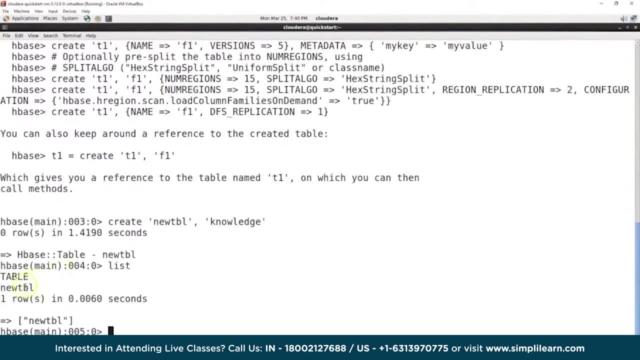 see table and new table. So you can now see that we have the new table and, of course, the default table that's set up in here And we can do something like describe. We can just describe and then we're going to do new TBL And when we describe it it's going to. 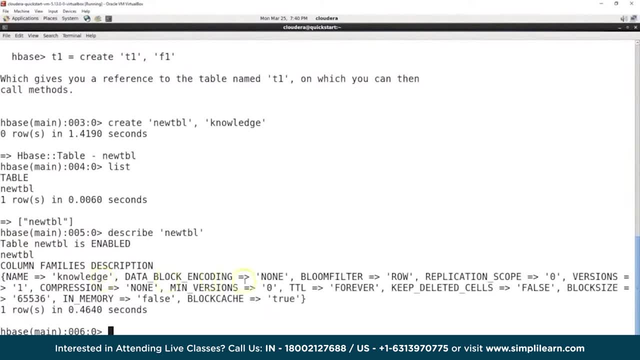 come up, It's going to say: hey name, I have knowledge. data block encoding none. bloom filter, row replication, scope, version, all the different information you need. New minimum version, zero, forever deleted cells, false block. 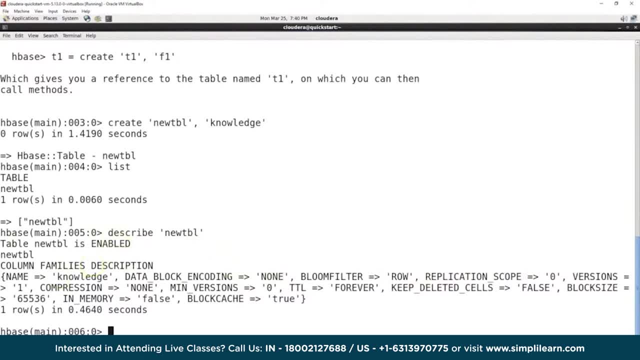 size in memory, And you can look this stuff up on Apacheorg to really track it down. One of the things that's important to note is versions, So you have your different versions of the data that's stored, And that's always important to understand. 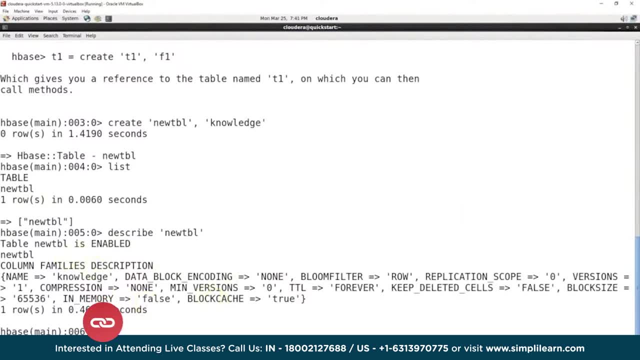 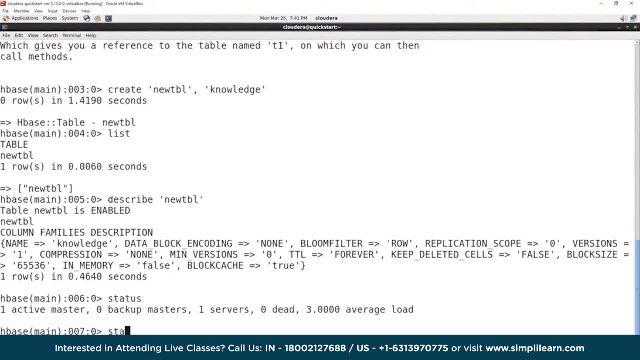 that We might talk about that a little bit later on. And then, after we describe it, we can also do a status. The status says I have one active master going on. That's our HBase as a whole. We can do status. 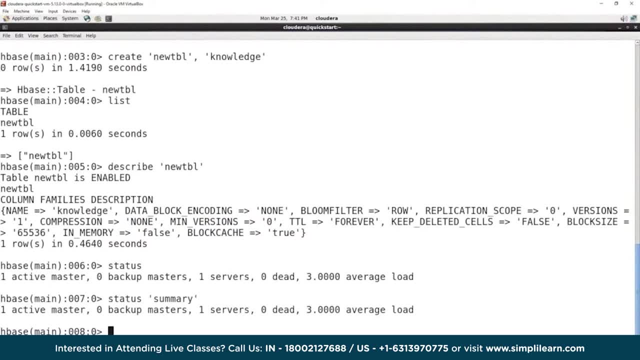 summary, And it should do the same thing as status. So we got the same thing coming up And now that we've created it, let's go ahead and put something in it. So we're going to put new TBL And then we want. 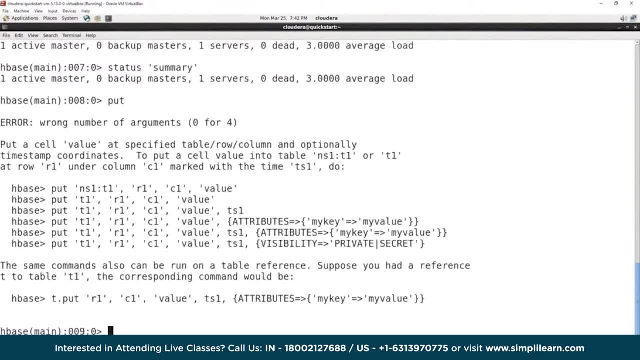 row one. You know what, before I even do this, let's just type in put And you can see. when I type in put, it gives us like a lot of different options of how it works and different ways of formatting our data as it goes in, And all of them usually. 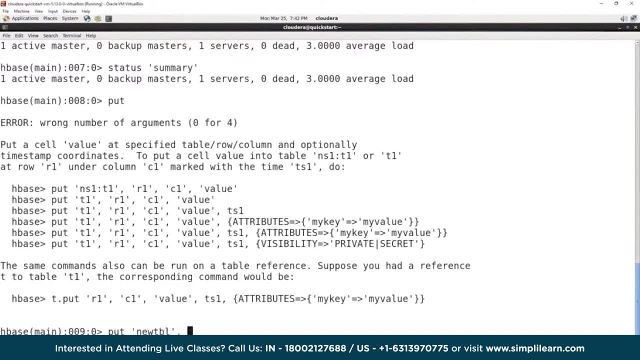 begin with the new table, new TBL, Then we have, in this case we'll call it row one, And then we'll have knowledge. Remember, we created knowledge already And we'll do knowledge sports, And then in knowledge and sports. 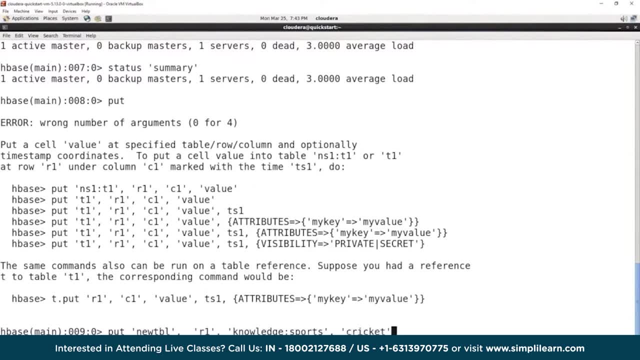 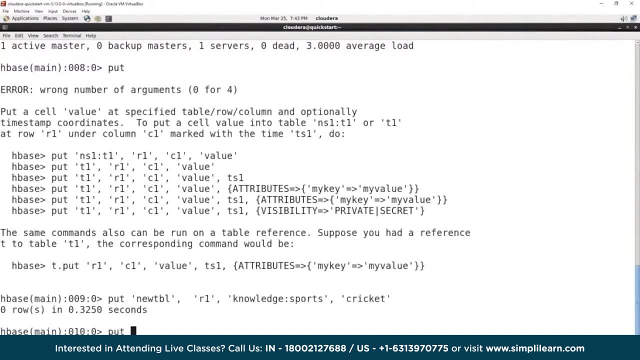 we're going to set that equal to cricket. So we're going to put underneath this our knowledge setup. We have a thing called sports in there And we'll see what this looks like in just a second. Let's go ahead and put in. we'll do a couple of these. 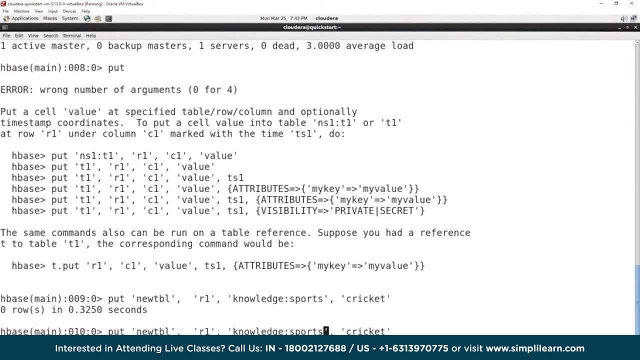 Let's see, let's do another row one, And this time, instead of sports, let's do science. You know this person. not only you know. we have row one which is both knowledgeable in cricket and also in chemistry, So it's a chemist who plays cricket. 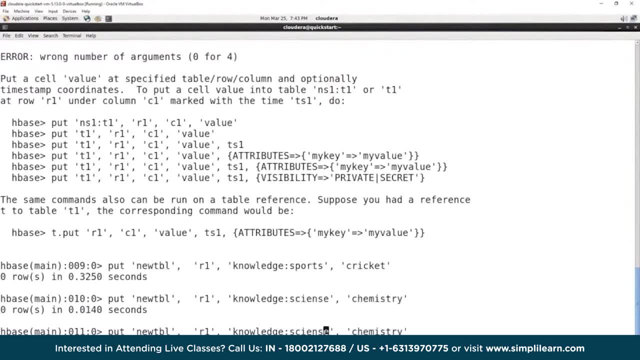 in row one And let's see if we have. let's do another row one, just to keep it going, And we'll do science. In this case, let's do physics, Not only in chemistry, but also a physicist, I have quite a joy in physics myself. 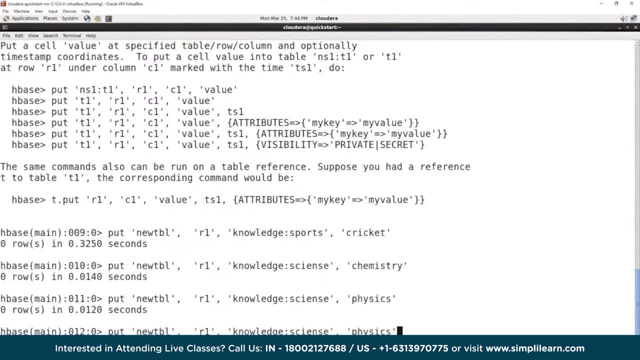 So here we go, We have row one, There we go, And then let's do row two. Let's see what that looks like when we start putting in row two. And in row two this person is: has knowledge in economics. 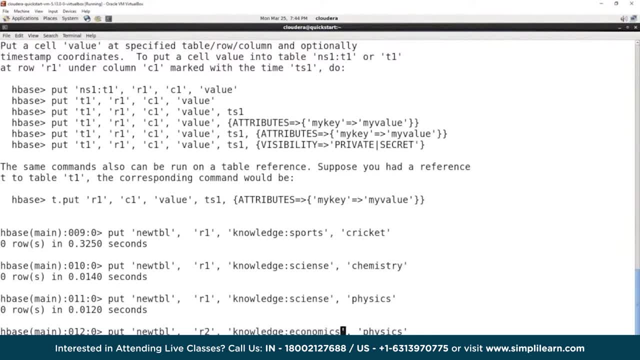 This is a master of business, and how- or maybe it's global economics, Maybe it's just for the business- and how it fits in with the country's economics And we'll call it macroeconomics. So I guess it is for the whole. 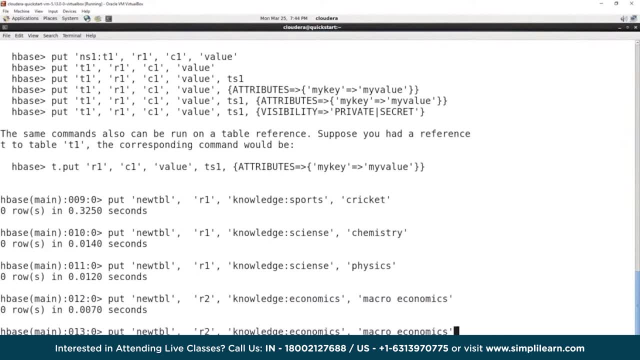 country there. So we have knowledge, economics, macroeconomics. And then let's just do one more: We'll keep it as row two, And this time our economist is also a musician, So we'll put music. And they happen to have knowledge. 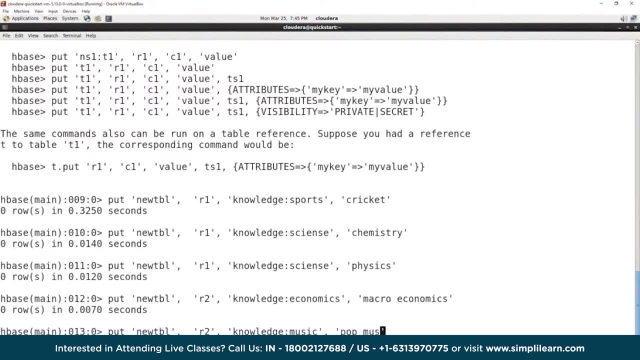 and they enjoy. oh, let's do pop music. They're into the current pop music going on. So we've loaded our database And you'll see we have two rows, Row one and row two, in here, And what we can do is we can. 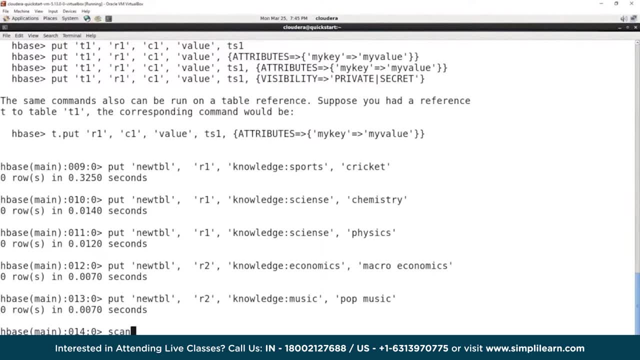 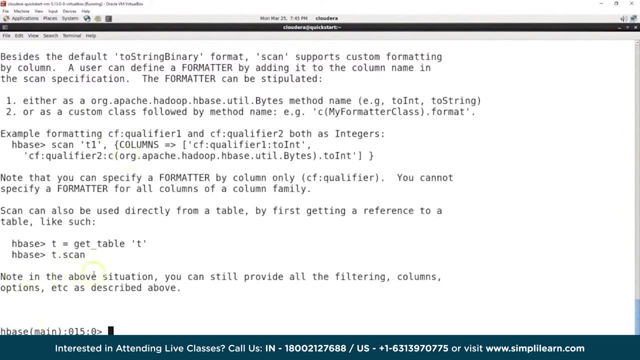 list the contents of our database by simply doing scan, Scan and then let's just do scan by itself. so you can see how that looks. You can always just type in there and it tells you all the different setups you can do with scan and how it. 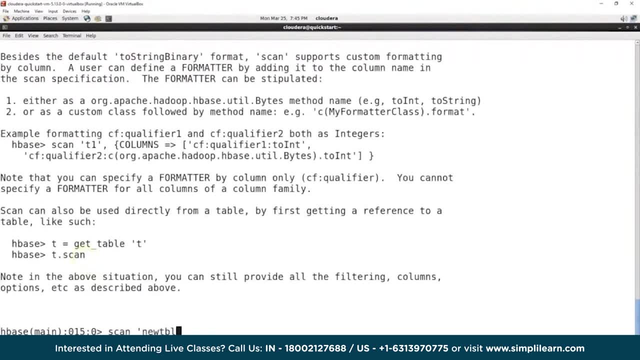 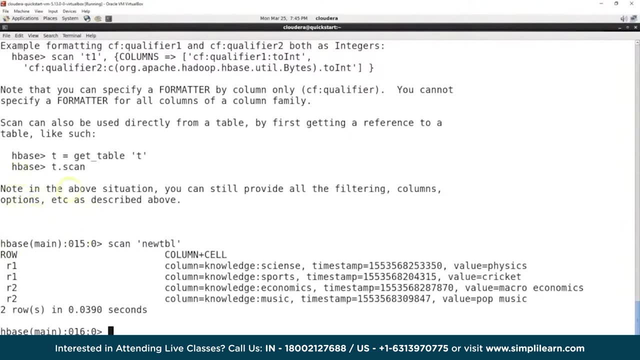 works. In this case we want to do scan new TBL And in our scan new TBL we have row one, row one, row two, row two And you'll see. row one has a column called knowledge, science, time step value. 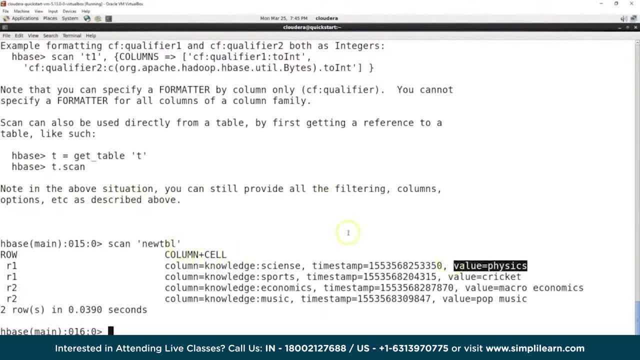 crickets value physics, So it has information as to when it was created, when the time stamp is Row one also has knowledge, sports and a value of cricket. So we have sports and science. And this is interesting because, if you remember, up here we 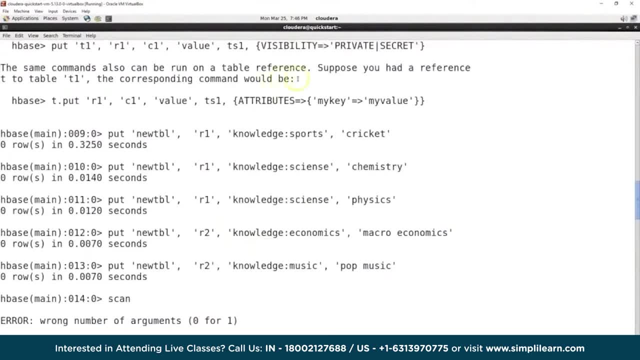 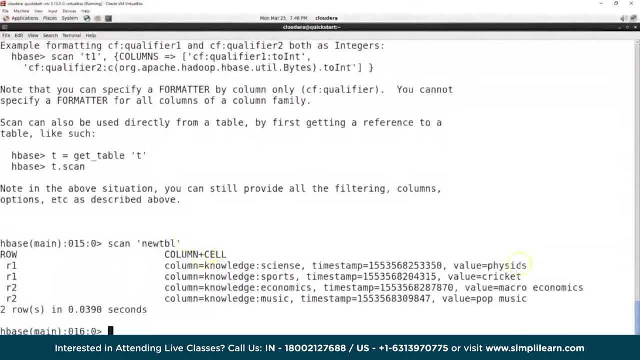 also gave it originally. we told it to come in here and have chemistry. We had science, chemistry and science, physics, And we come down here. I don't see the chemistry. Why? Because we've now replaced chemistry with physics. So the new value 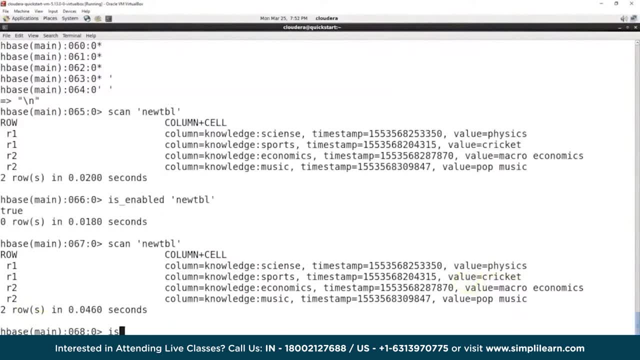 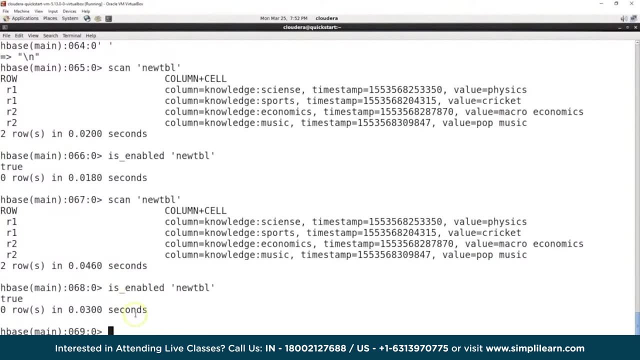 is physics on here. Let me go ahead and clear it down a little bit. And in this we're going to ask the question: is enabled, new table- When I hit enter in here, you're going to see it comes out true, And then we'll go ahead and disable. 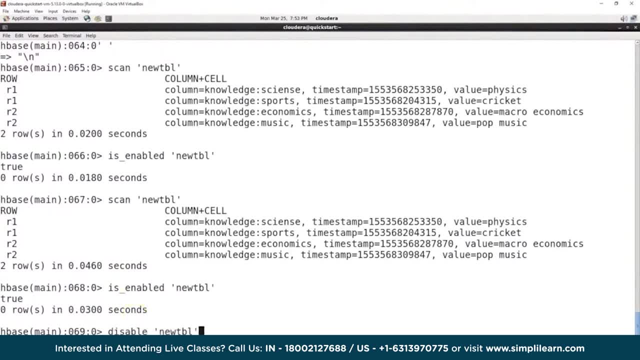 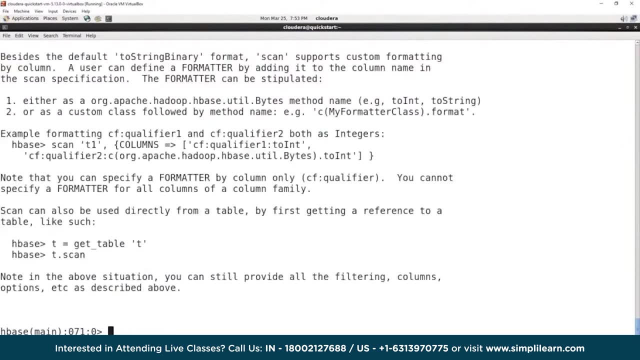 it. Let's go ahead and disable new table. Make sure I have our quotes around it. And now that we've disabled it, what happens when we do the scan? When we do the scan new table, I hit enter. you're going to see that we get. 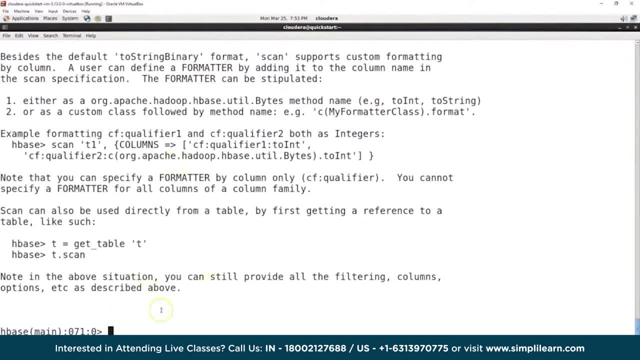 an error coming up. So once it's disabled, you can't do anything with it until we re-enable it. Now, before we enable the table, let's do an alteration on it, And here's our new table, And this should look a little familiar. 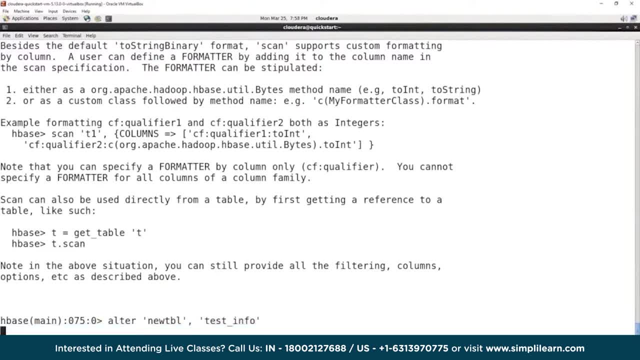 because it's very similar to create. We'll call this test info And we'll hit enter in there. It'll take just a moment for updating And then we want to go ahead and enable it. So let's go ahead and enable our new. 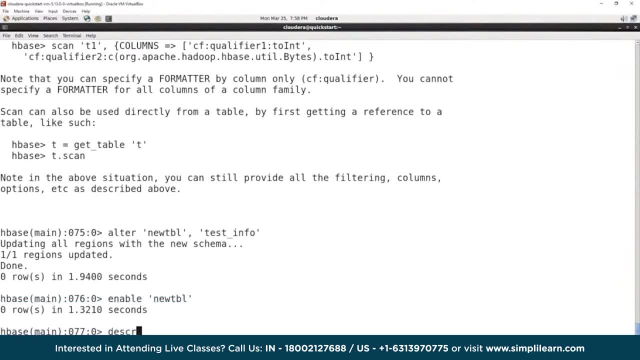 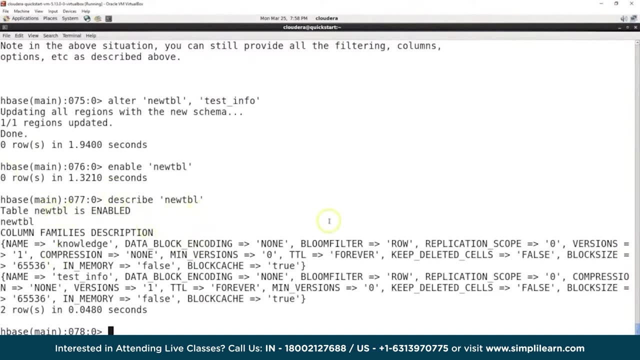 table. So it's back up and running And then we want to describe, Describe new table And we come in here. you'll now see we have name knowledge And under there we have our data encoding and all the information under knowledge. And then we also 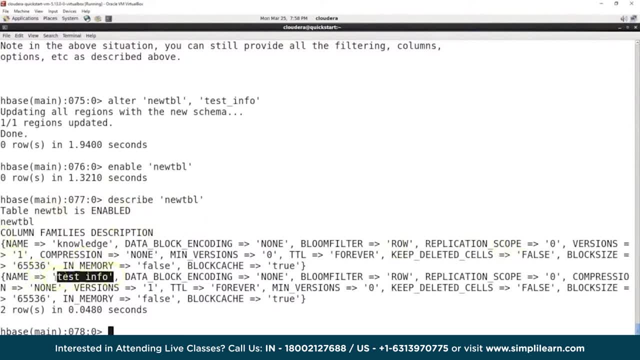 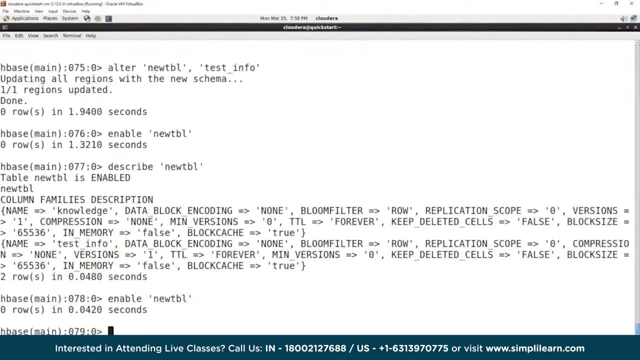 have down below test info. So now we have the name test info And all the information concerning the test info on here And we'll simply enable it. New table. So now it's enabled. Oops, I already did that. I guess we'll. 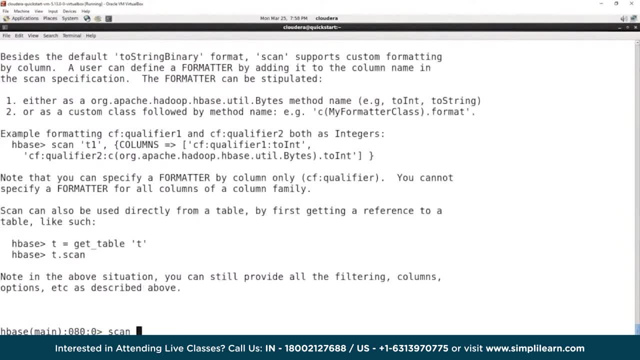 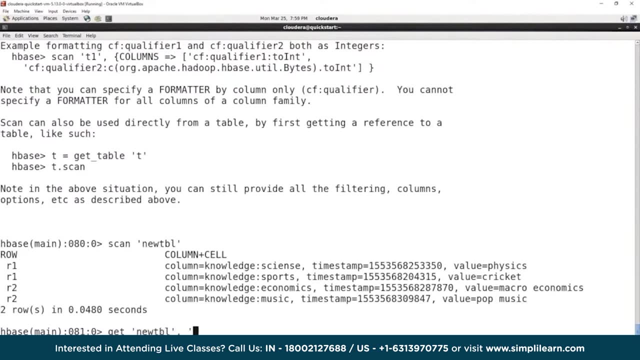 enable it twice, And so let's start looking at: well, we had scan new table And you can see, here we're going to get the data And this is going to bring up the information like this: But what if we want to go ahead and get a row? 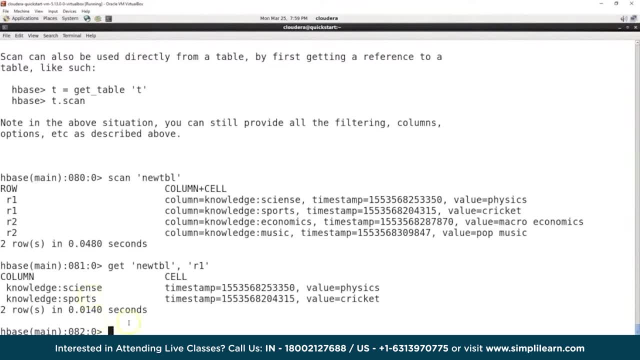 So we'll do R1.. And when we do HBase R1, you can see we have knowledge science, and it has a time stamp, Value physics. And we have knowledge sports, and it has a time stamp on it And value cricket. And then let's see what happens. 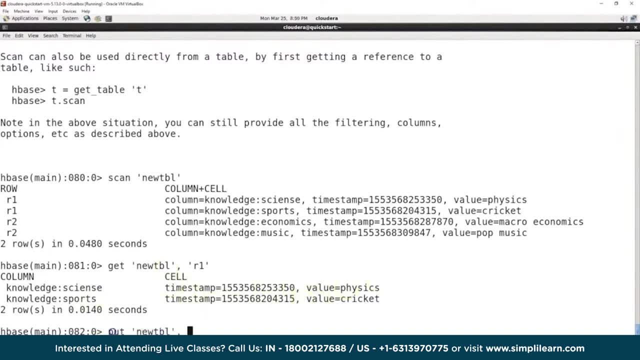 when we put into our new table, And in here we want row one And, if you can guess from earlier, because we did something similar- We're going to do knowledge economics and then it's going to be a sort of- I think it was what- macroeconomics. 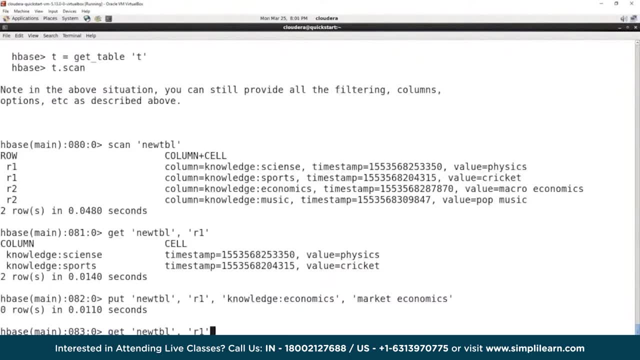 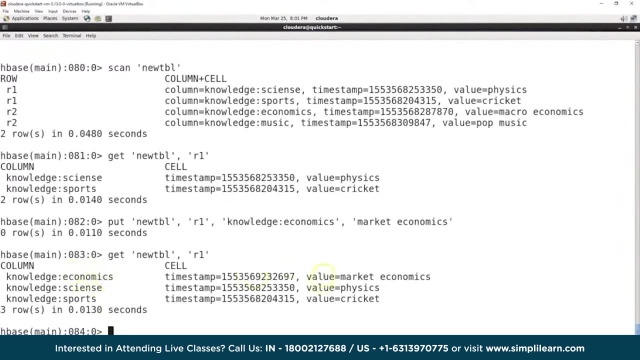 It's now market economics And we'll go back and do our get command And now see what it looks like And we can see here where we have knowledge economics- It has a time stamp, Value, market economics, Physics and cricket, And this is because we have 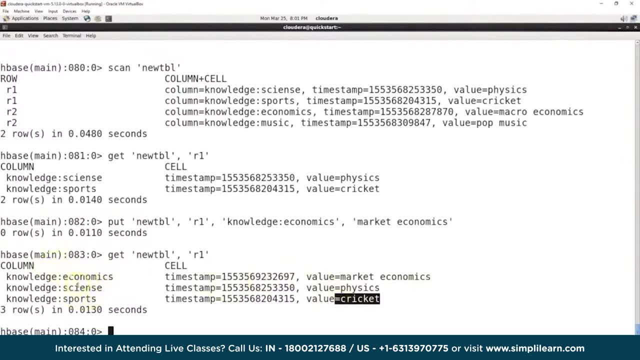 economics, science and sports. Those are the three different columns that we have, And then each one has different information in it, And so if you managed to go through all these commands and look at basics on here, you'll now have the ability to create a. 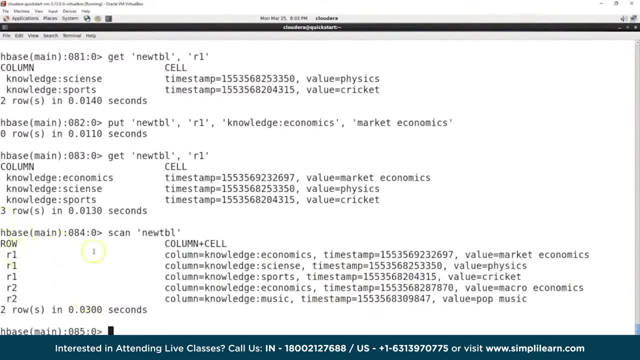 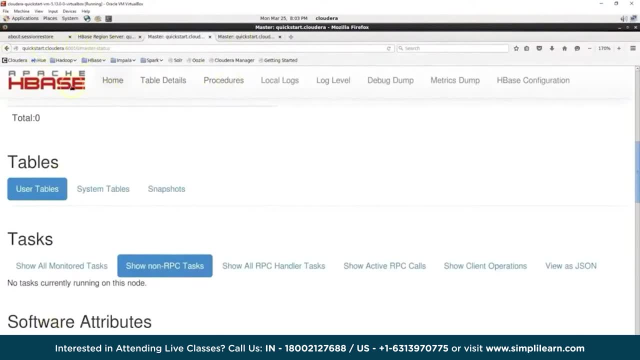 very basic HBase setup, No SQL setup Based on your columns and your rows. And just for fun, we'll go back to the Cloudera where they have the website up for the HBase master status And I'll go ahead and refresh. 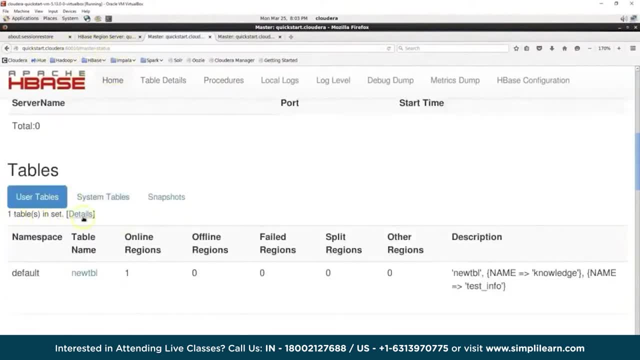 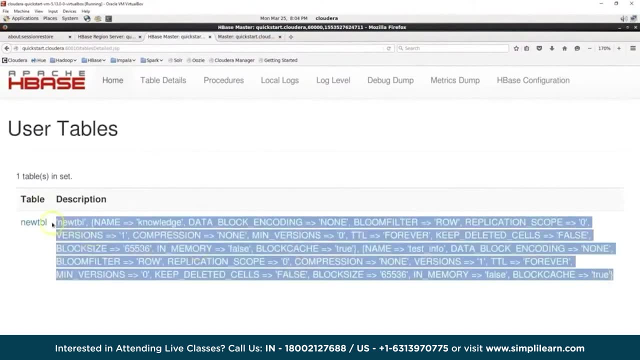 it. And then we can go down here and you'll see user tables, table set one, And we can click on details. and here's what we just did. It goes through. So if you're the admin looking at this, you can go: oh, someone just created. 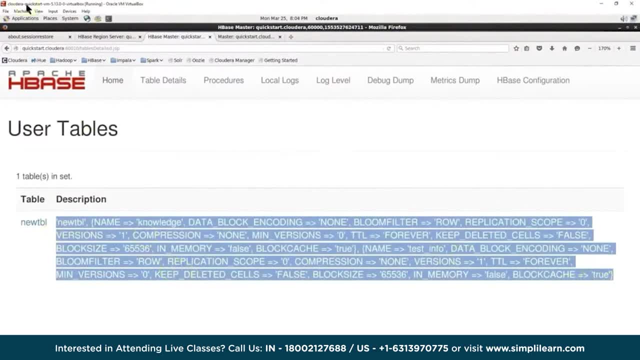 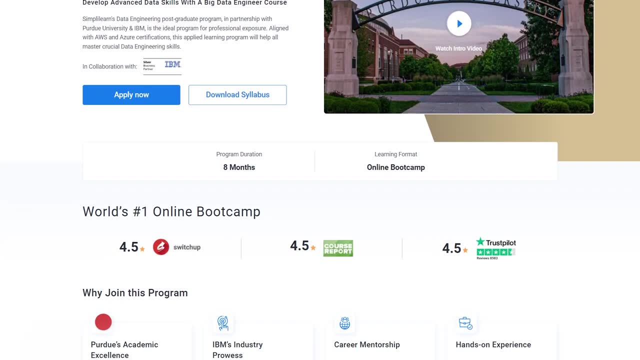 a new TBL and this is what they have underneath of it in their new table. Now, whether you are an aspiring data analyst, a seasoned IT professional or a business leader looking to leverage the power of big data, the data engineering post graduate program by SimplyLearn. 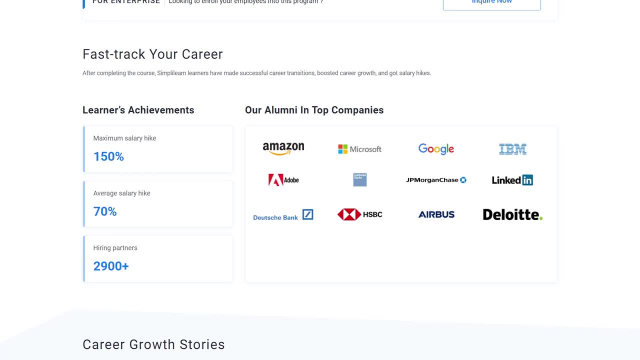 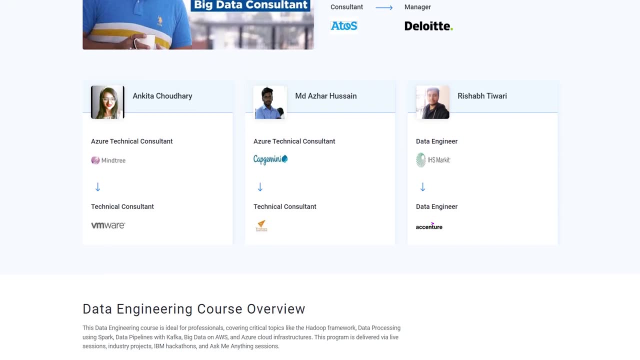 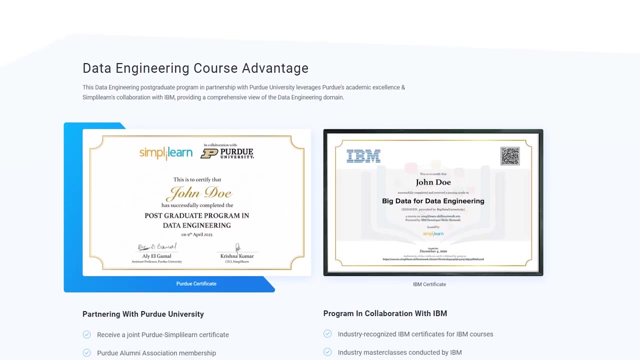 in collaboration with Purdue University and IBM, is tailored to meet your needs. This program offers an exceptional opportunity for professional growth and exposure, With a focus on practical learning and in alignment with industry leading certifications from AWS and Azure. Now this program equips participants with essential skills. 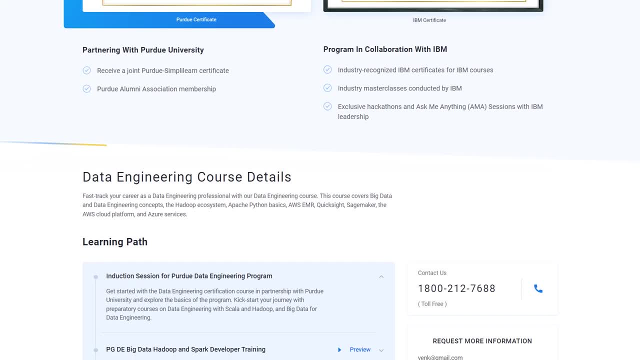 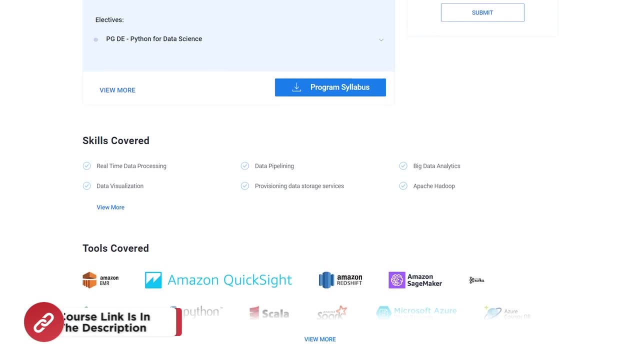 required to excel in this field of data engineering. By enrolling in this applied learning program, individuals can gain mastery over crucial data engineering techniques and technologies. Enroll today and take the next step towards becoming a proficient big data professional. Check out the course link in the description. 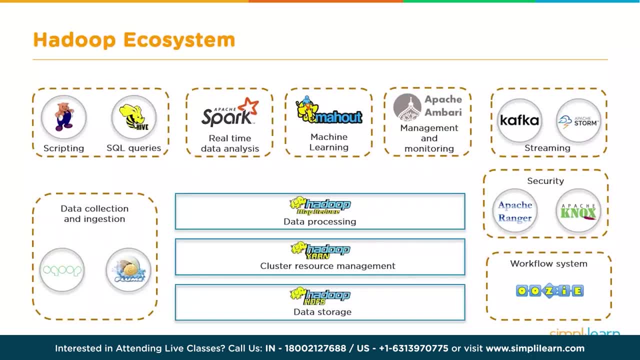 box below for more details. Today we're covering the Hadoop ecosystem- at least the very fundamentals of all the different parts that are in the Hadoop ecosystem- And it's very robust. It's grown over the years with different things added in. There's a lot of overlapping and a 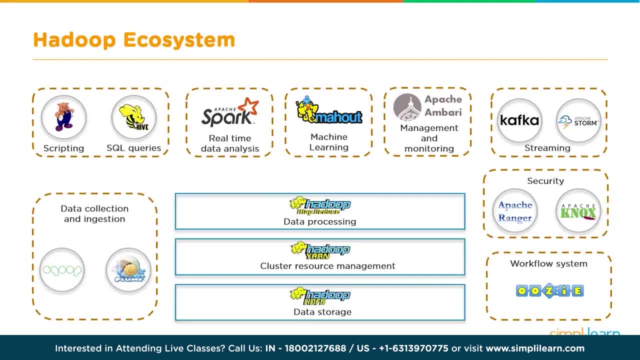 lot of these tools, But we're just going to cover these basic tools so you can see what's available in the Hadoop ecosystem. So let's go back to our Hadoop ecosystem. As you can see, we have all our different set up and let's focus on the Hadoop part. 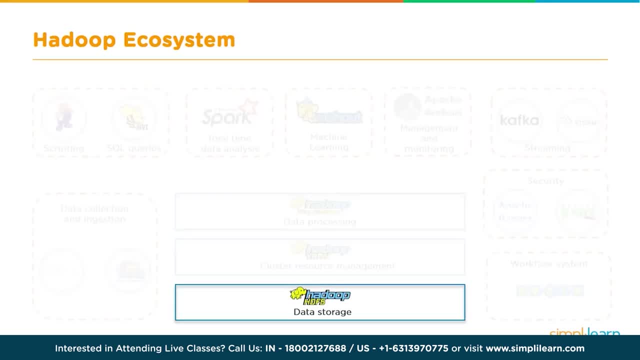 of it first, before we look at the different tools. We start with the Hadoop, or HDFS is for data storage. Write once, read many times. You can store a lot of data on it, affordably Distributed file system. And so we talk about. 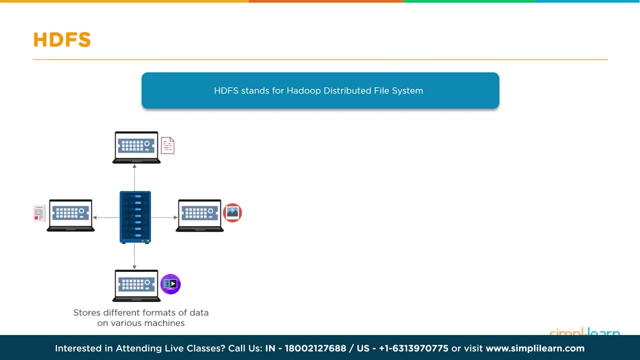 the Hadoop file system. It stores different formats of data on very various machines And so you have like a huge cluster of computers and you're able to store word documents, spreadsheets, structured data, non-structured data, semi structured, And in the Hadoop, 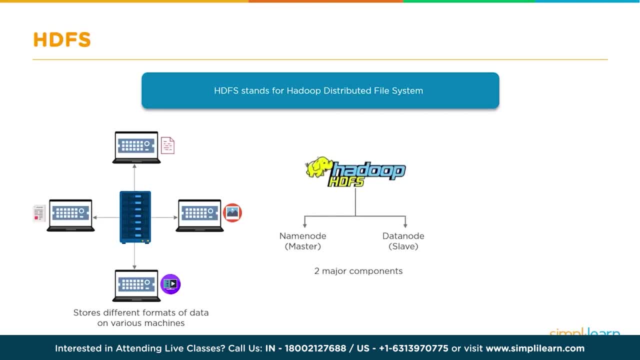 file system. there's the two different sets of servers in there. There's the name node, which is the master We talked about, that, That's your enterprise computer, And the other component is your data nodes, And so you'll usually have, like I said, 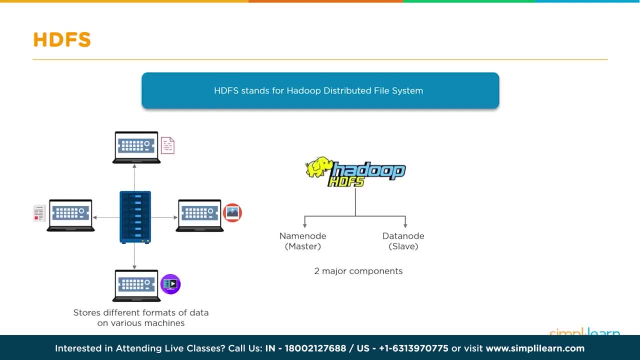 one to two. You'll have a name node and maybe a backup name node, And then you'll have as many data nodes as you want And you can just keep adding them. That's what makes it so affordable. You know, you have a rack of computers. 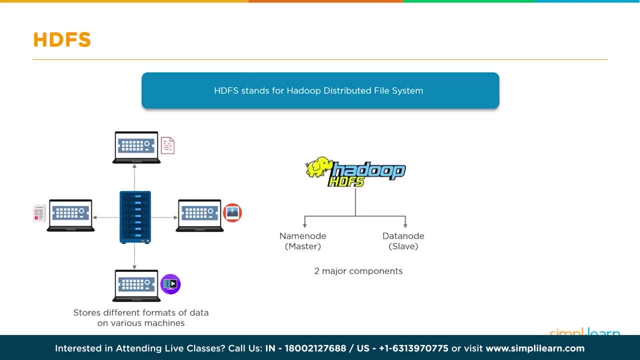 and you go: oh, I need more space, You just add another rack in, So it's very affordable and very easy to expand. And the way the Hadoop file system itself works behind the hood is it splits the data into multiple blocks. By default it's 128. 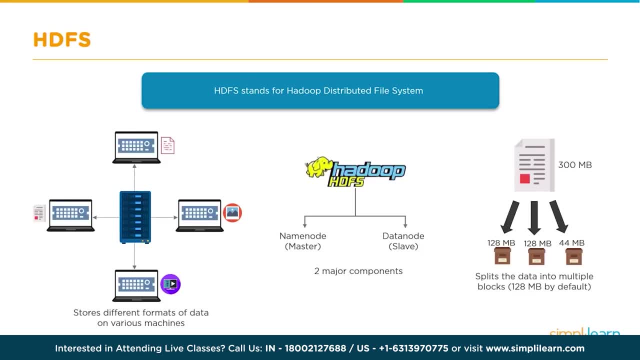 megabytes And the 120 megabytes. it is a default setting. You can change that. That works for most data. There's reasons for either processing speed Or for better distribution of the data. So if you have little tiny blocks of data that are less than 128, 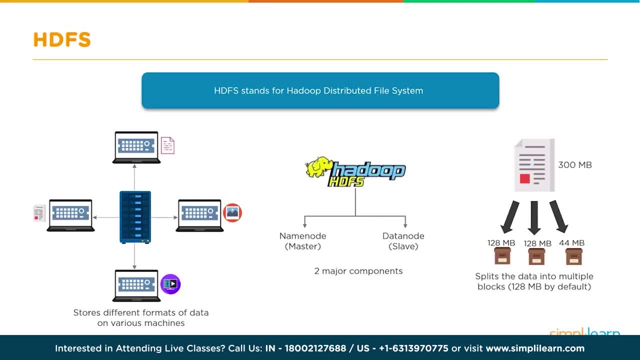 megabytes. If you have a lot of those, you might want to go down in size, and vice versa for larger blocks. And you can see, right here we have 300 megabytes And it takes that piece of data and it just divides it into blocks of data. 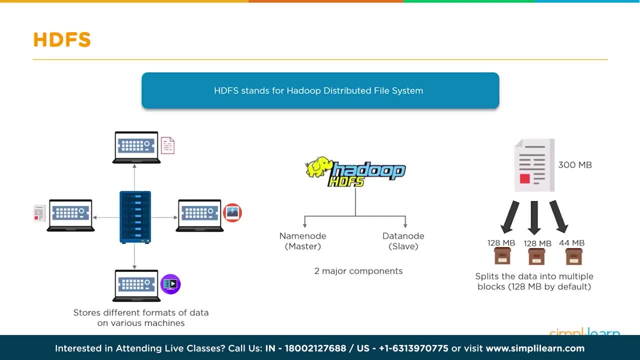 and each one is 128,, 128, and 44. Which, if you add together, equals 300 megabytes. Now that you understand the Hadoop file system, Or at least the basic overview of it, It's important to note what it sits on. What's actually making all this? 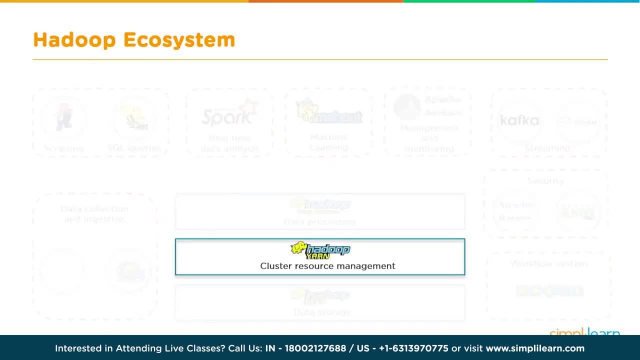 work on the backend, And this is YARN Hadoop. YARN is a cluster resource management, So it's how it manages this whole cluster right here that we just looked at, And YARN stands for Yet Another Resource Negotiator. Love the title It. 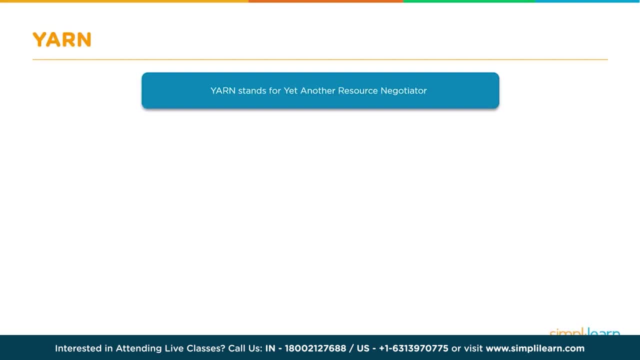 reminds me of an Iron Man movie with Tony Starks and Jarvis- Just a rather intelligent system, or whatever it stood for. But YARN has become very widely used And it's actually used as a backend for a lot of other packages, So it's not. 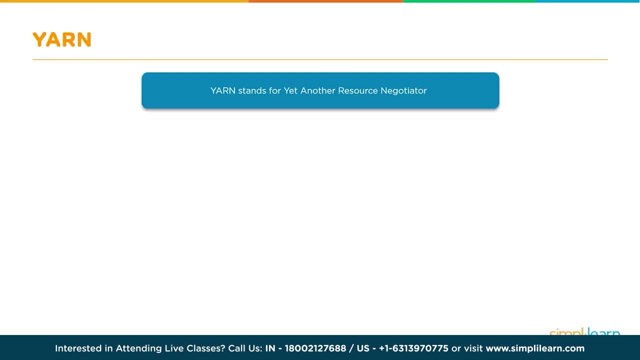 just in Hadoop, But Hadoop is where it came from And where it's set up, And there's some other ones. Another popular one is Mesos, Which I'll mention again briefly, And so the YARN. it handles the cluster of notes. 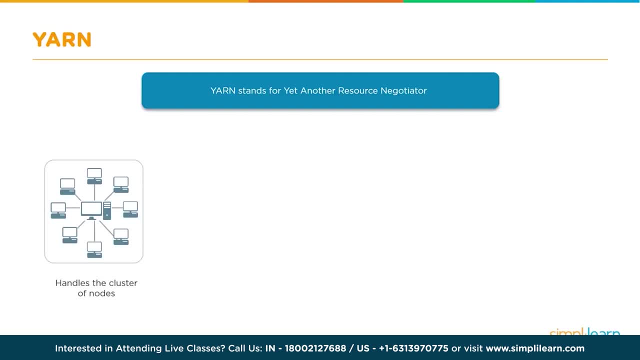 It's the one When you hear YARN, it's the one that's going: hey, where's our RAM at? Where's our hard drives at? Or if you have a solid state disk drive, Your SD, Where's that at? How much memory do I have? 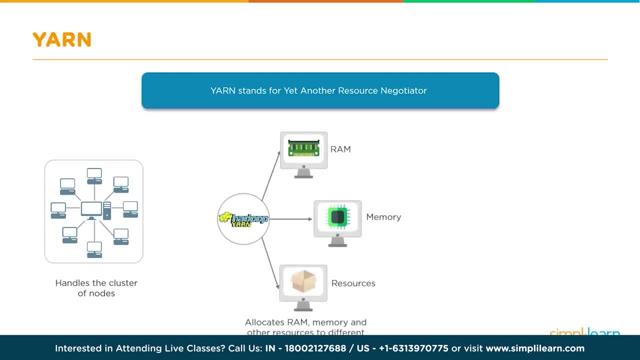 What can I put where? And so here we go. Nice image of it: RAM memory resources. So it's allocating all these different resources for different applications is what it's doing. When we talk about the Hadoop data processing We're going to 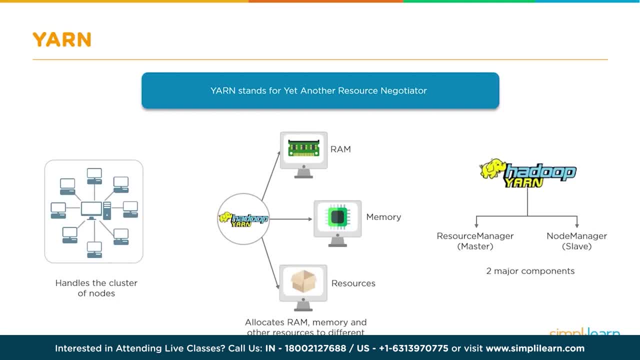 go back to the two major components. The two major components is your resource manager, That's on the master server Or your enterprise computer, And then that one is in control and managing what's going on with all of your nodes. Data processing in Hadoop MapReduce. 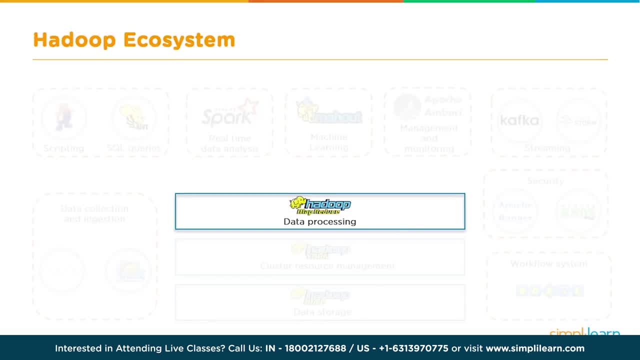 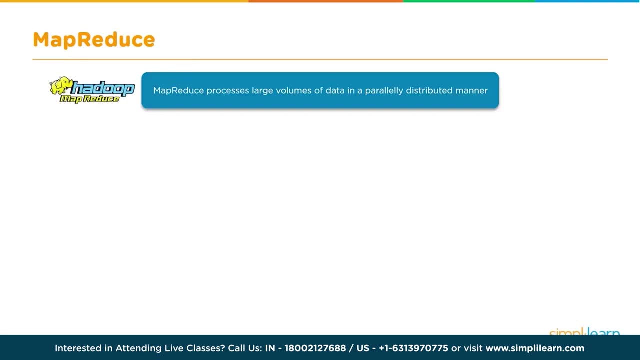 And we're going to talk about the MapReduce here in just a second. The Hadoop data processing is all built upon MapReduce. MapReduce processes a large volumes of data in a distributed manner. This is very core to Hadoop. But before we go on Because there's other tools, 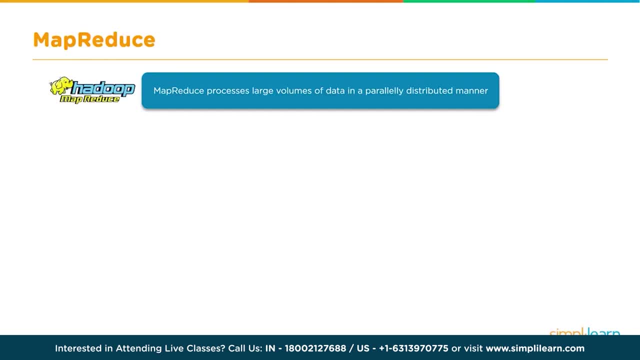 out there And things are slowly shifting And there's all kinds of new things. One of the things you want to look at is not just how the MapReduce works, But start thinking. MapReduce One of the best pieces of advice I had from. 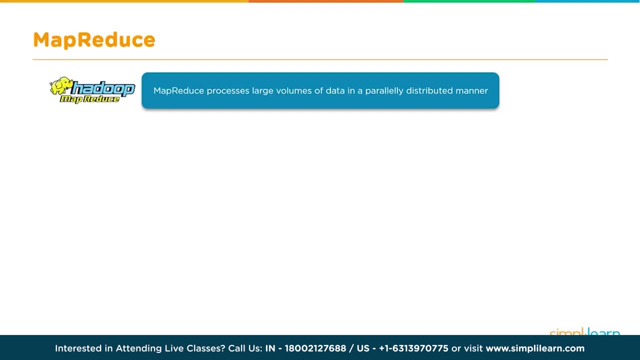 one of my mentors in data science was think MapReduce. This is really what you should be learning, But it is an actual process in the Hadoop system. So we have our big data And the big data comes out, And so this is the first step. 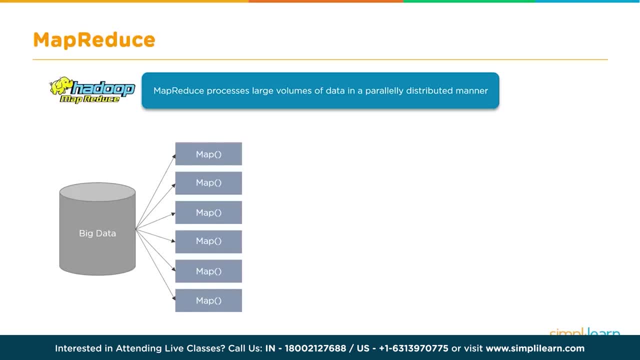 If I'm looking at my data, How do I map that data out? What am I looking at? And it could be something as simple as I just loaded into. I'm just looking at one line at a time, But it could be that I'm looking at the data one line. 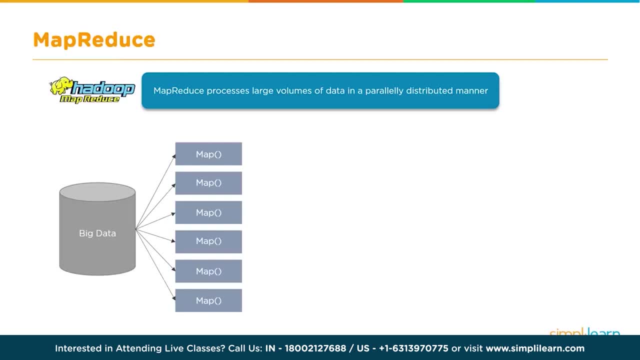 at a time, But I only need columns one and four. Maybe I'm looking at it one column at a time, But I need the total of column one added together And column one over column two, So you can start to get some very complicated mapping here. 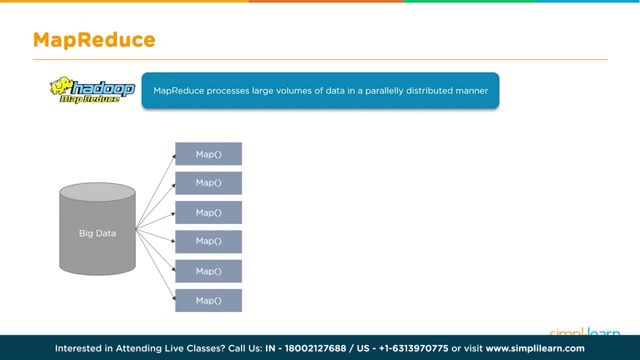 But the mapping is: what do you do with each line of data, Each piece of data? If you're in a spreadsheet, it's easy to see. you have a row. Whatever you do to that row, that's what you're mapping, Because it doesn't look at anything else. It doesn't know anything. 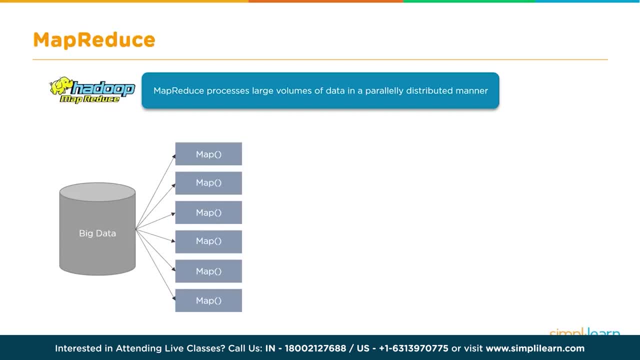 else, All it knows is what's on that row. If you're looking at documents, maybe it's pulling one document at a time And so your map is then a document, And then it takes those and we shuffle and sort them How. 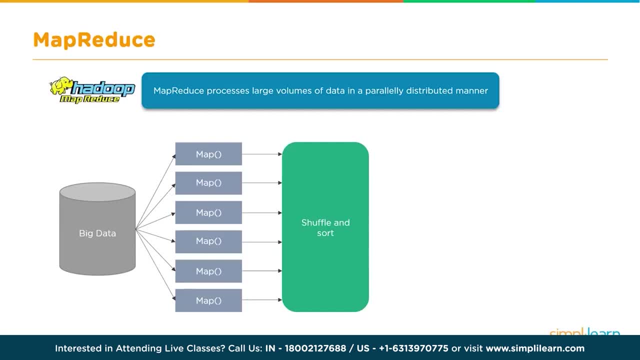 do we sort them around? Whether you're grouping them together, Whether you're taking the whatever information you mapped out of it, Word counts. You're counting the word A, So letter A comes out with how many for each mapping, If you have. 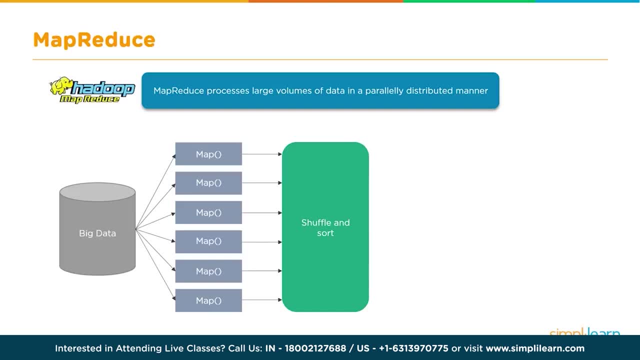 54 A's per the one document, 53 in the other ones. That's what's coming out of that mapping and going into the shuffle and sort. And so if it's counting A's and B's and C's, it'll shuffle. 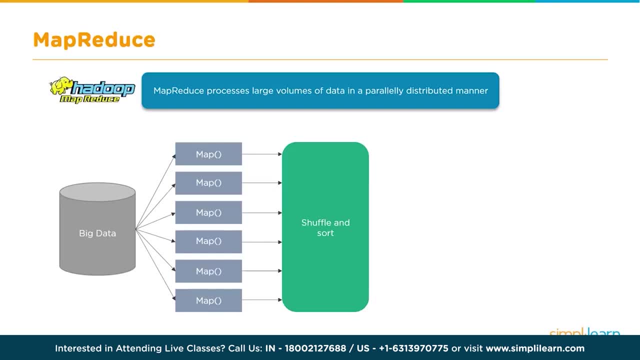 and sort all the A's together, All the B's together. If you're running big data for running agriculture- Apples and oranges- So it puts all the apples in one, All the stuff you mapped out that you said, hey, these are all apples. 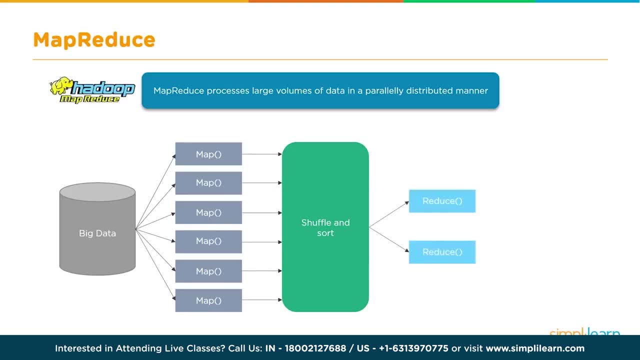 These are all oranges. Let's shuffle them and sort them together And then we reduce and reduce, So each of these groups reduce into the data you want out. So you have map, shuffle, sort, reduce And some important things to know about. 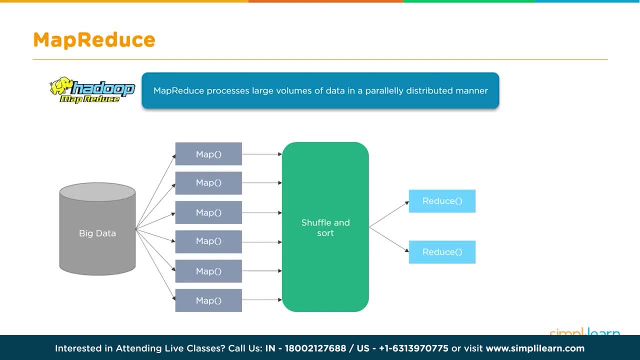 the Hadoop file system- Because I'm going to mention Spark in a little bit- Is. the Hadoop file system manages to do a lot of this by writing it to the hard drive. So if you're running a really low budget, Which nobody does anymore, 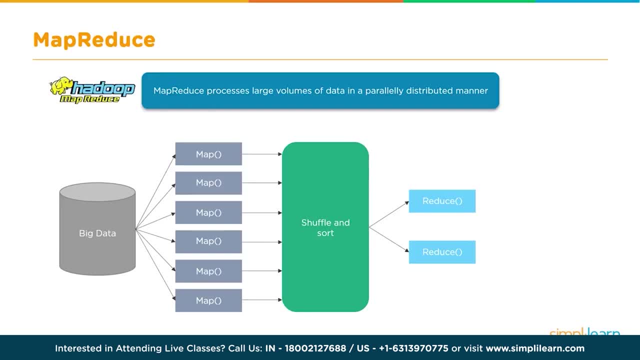 with the Hadoop file system And you have all your commodity. machines are all low. They only have a 8 gigabytes memory instead of 128 gigabytes. This process uses the hard drive And so it pulls it in to the RAM for your mapping. It maps. 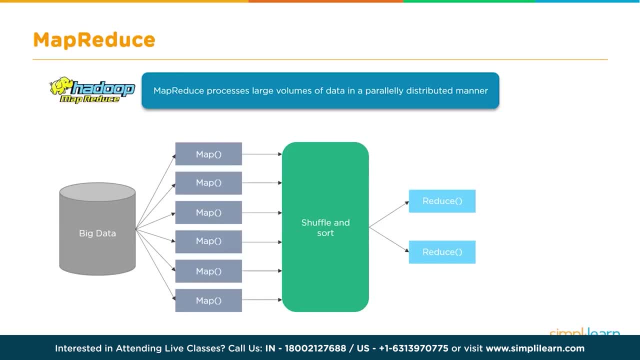 the one piece of data. Then it writes that map to the hard drive. Then it takes that mapping from the hard drive, Loads it up and shuffles it and writes it back to the hard drive To a different spot And then takes that information and 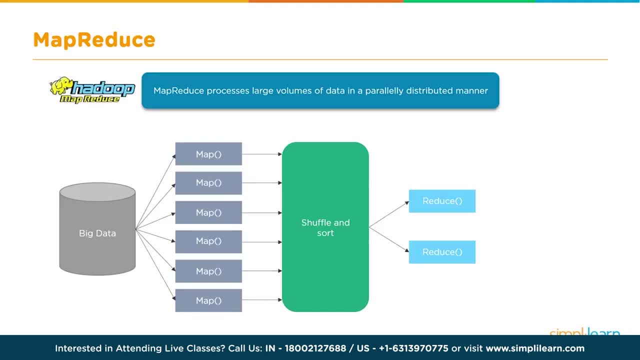 starts processing it in the reduce And then it writes the reduce answer to the hard drive. It runs slower Because you're accessing to and from your hard drive Or solid state drive if you have an SD card in there, But you can also utilize. 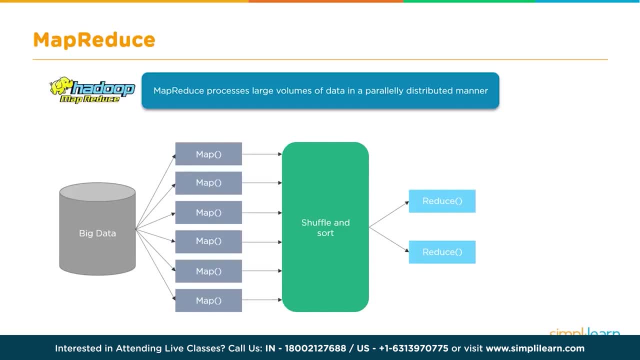 it's a lot more affordable, Like I said, having that higher end of RAM cost even on a commodity machine. So you can save a lot of money. Nowadays it's so affordable. people run the Spark setup on there Which does the same thing, but in 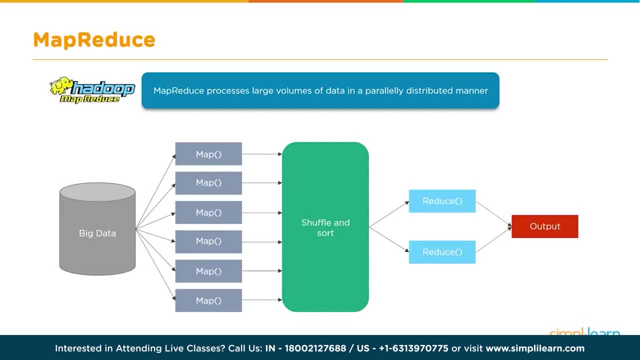 RAM, And again we'll talk about Spark in just a little bit- And of course the final thing is an output. So again your reduce are written to the hard drive And then your reduce is brought together to form one output. What is the maximum? 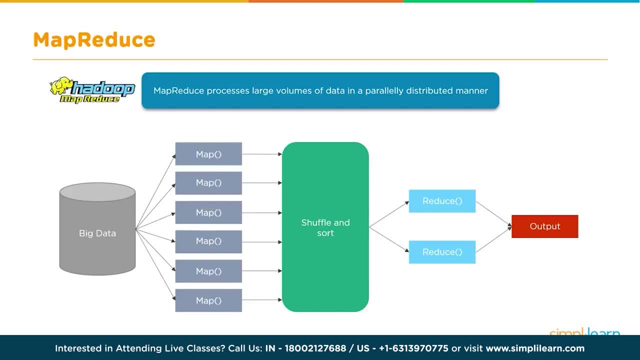 number of oranges sold per an area. I don't know, I'm making that up. One of the things about Hadoop is it covers so many different things that anything you can think of you can put in Hadoop. The question is, do you need to? 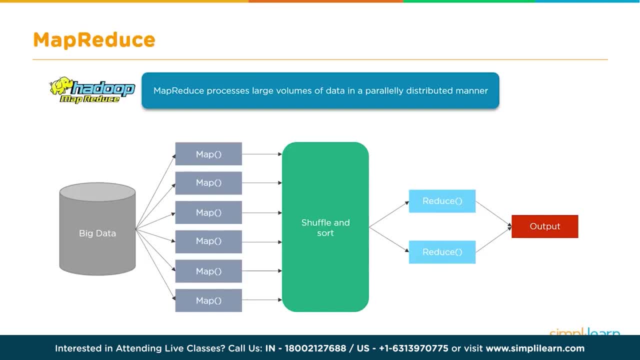 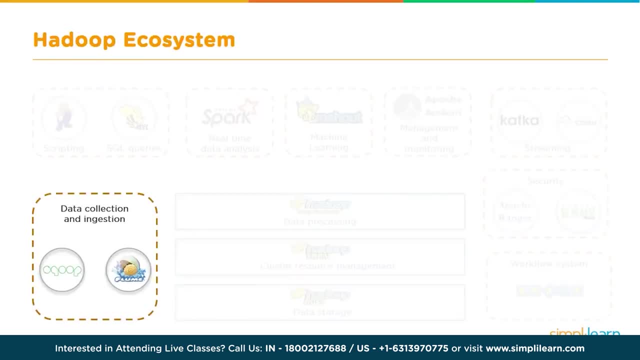 Do you have enough data or enough need for the high end processing? So again, look at map or reduce, But think of this not just as map or reduce. Start thinking, map and reduce. when you think big data, We're going to start getting into the tools Because you had all. 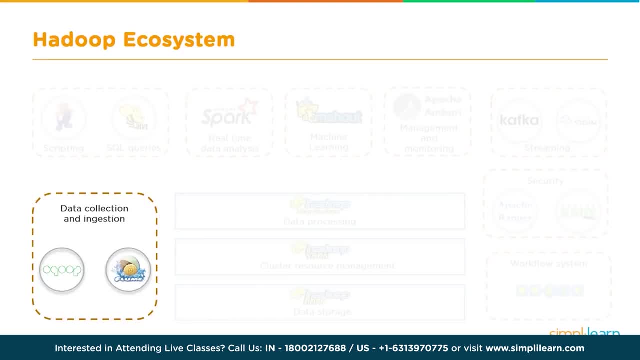 those pictures of all those cool tools we have. So we're going to look at the first two of those tools And in the tools we have scoop and flume, And this is for your data collection and ingestion. We're going to bring Spark up in just a second. 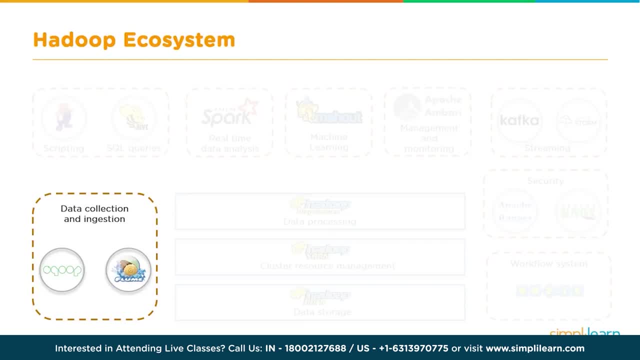 Can also play a major role in this Because Spark is it's own animal that, sprung from Hadoop, connects into Hadoop but it can run completely independent. But scoop and flume are specific to Hadoop and they're ways to bring in information into. 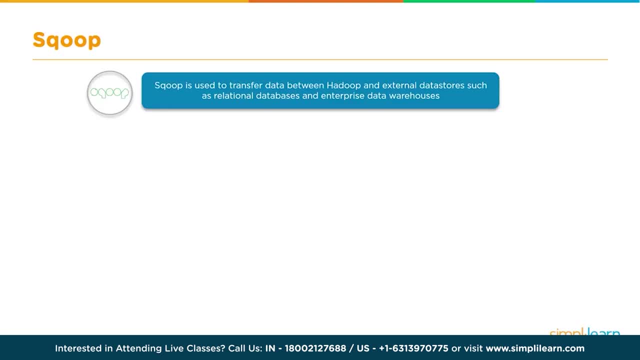 the Hadoop file system. So we talk about these. We'll start with scoop. Scoop is used to transfer data between Hadoop and external data stores, such as relational databases and enterprise data warehouses, And so you can see right here, Here's our Hadoop data and it's 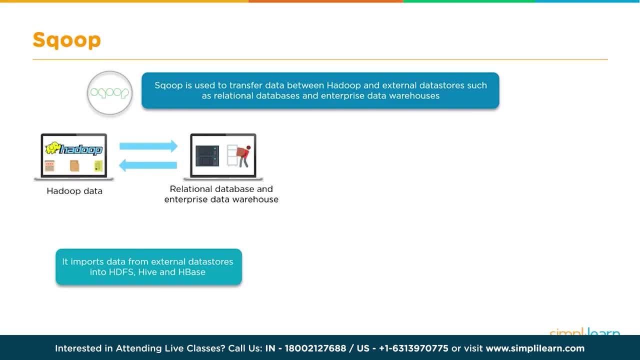 connecting up there and it's either pushing the data or pulling the data And we have our relational data database and enterprise data warehouse And there's that magic word enterprise. That means these are the servers that are very high end, So maybe you have a high end. 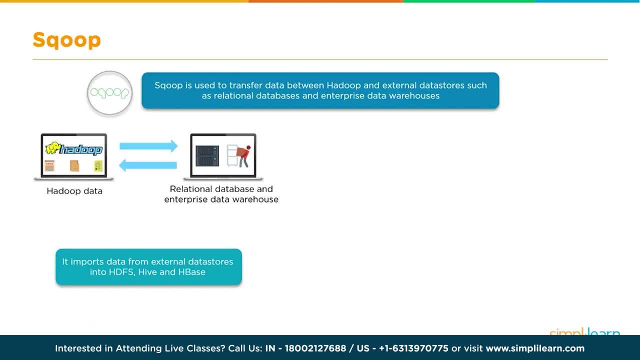 SQL server or MySQL server or whatever over there, And this is what's coming and going from the scoop. It imports data from external data stores into the HDFS Hive and Hbase. Those are two specific. The Hive setup is your SQL, basically, And you can see a nice little image here. 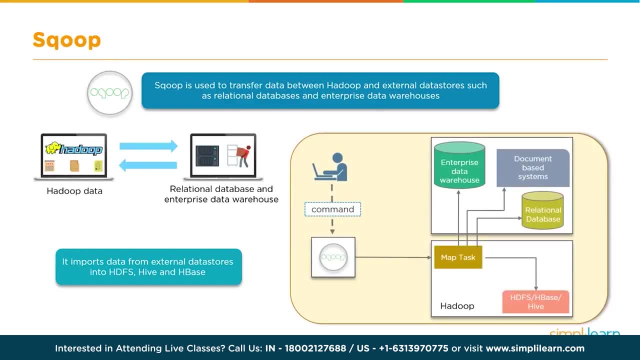 Here's somebody on their laptop- which would be considered the client machine- putting together their code. They push the scoop, The scoop goes into the task manager. The task manager then goes: hey, what have I got for the Hbase and Hive system in our? 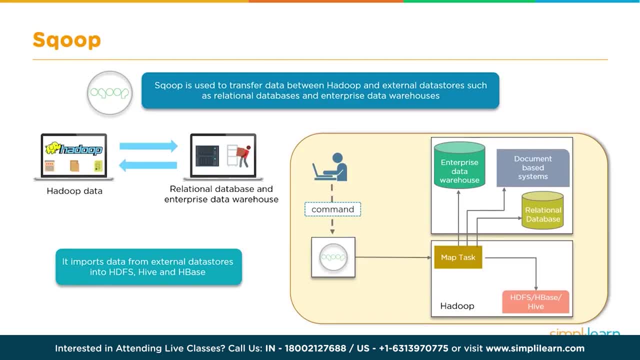 Hadoop system And then it reaches out to the enterprise data warehouse or into the document based system or relationship based database. Relationship is your non SQL Document, is just what it sounds like. You have HTML documents or Word documents or text documents, And it's able to map those tasks and then 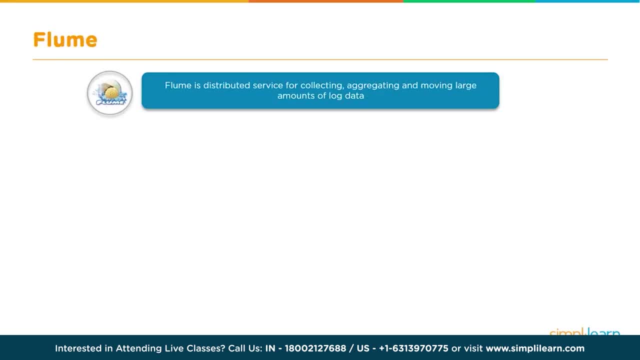 bring those into the Hadoop file system. Now, Flume is a distributed service for collecting, aggregating and moving large amounts of log data, So kind of focused a little bit on a slightly different set of data. although you'll find these overlap a lot, You can certainly 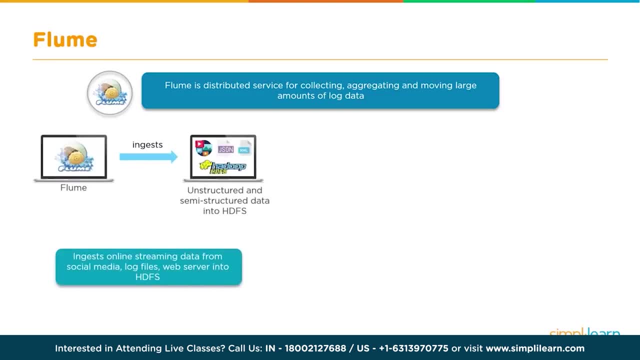 use Flume to do a lot of things that you can do in Scoop, and vice versa. Flume ingests the data, so we're looking at, say, a JSON call to a website, XML documents. Unstructured and semi-structured data is most commonly digested by. 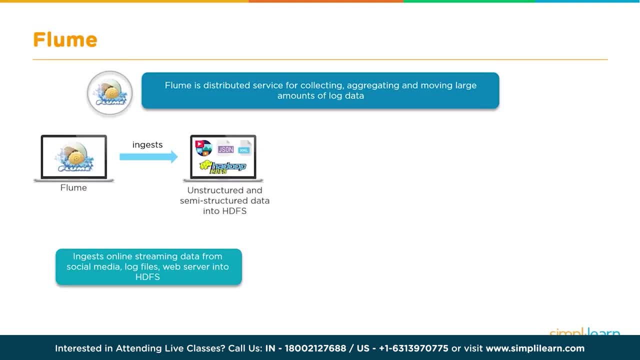 Flume. Best example I saw was a Twitter account pulling Twitter feeds into a Hadoop system So it ingests online streaming data from social media Twitter log files. So we want to know what's going on with error codes on your servers. 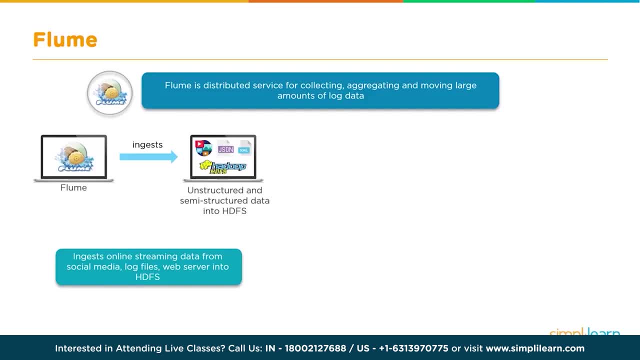 and all those log files, Web server: what's going on in your web server? We can bring all this stuff in and just dump it into the Hadoop data file system to be looked at and processed later, And it's a web server cloud. social media data Again. 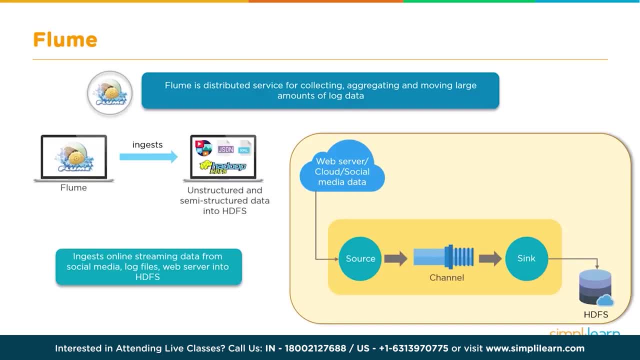 all those different sources it can be. It's kind of endless. It just depends on what your company needs. Versatility of Hadoop is what makes it such a powerful source to add into a company, And so it comes in. there You have your. 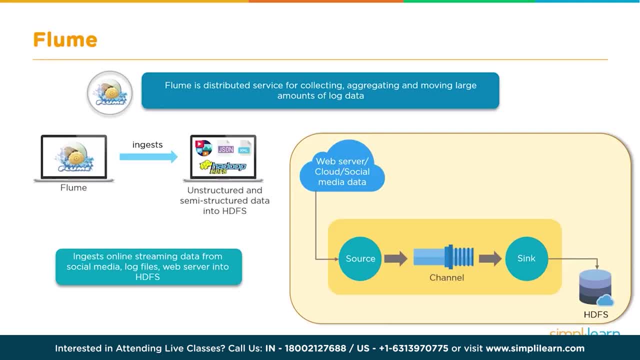 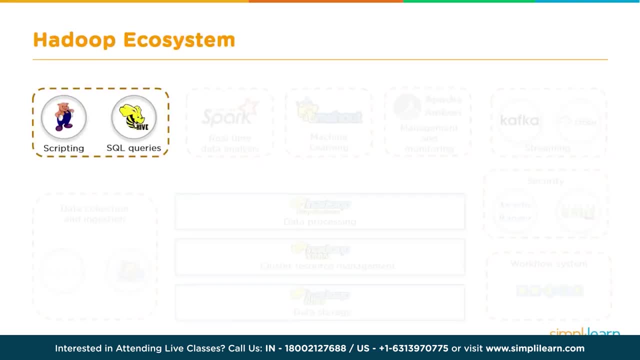 source, It goes through the channels, It then goes through kind of a sync feature to make sure everything is in sync And then it dumps it into the Hadoop file system. So we've covered in the Hadoop file system the first two things. Let's. 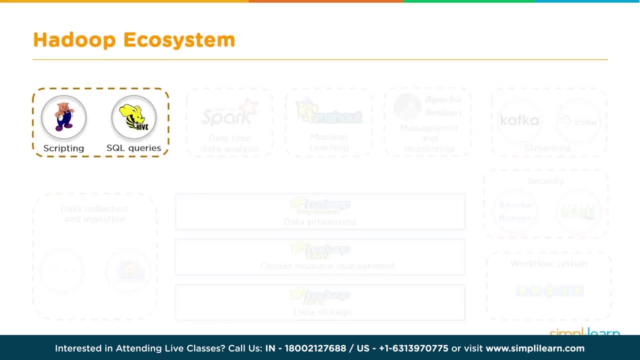 look at some of the scripting languages they have, And so we have the two here And you can also think of these. It actually says scripting and SQL queries. A lot of times they're both referred to as queries, So you have both the PIG. 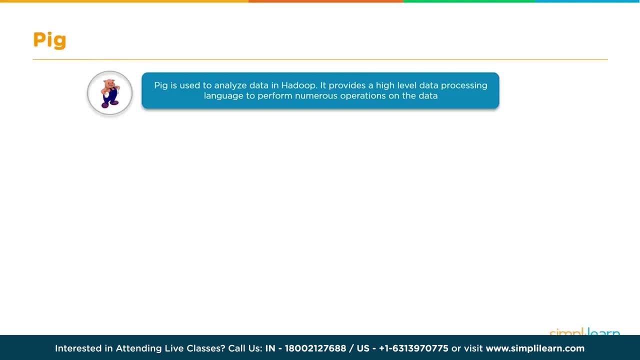 and the HIVE, And PIG is used to analyze data in Hadoop. It provides a high level data processing language to perform numerous operations on the data And it's made out of PIG Latin language for scripting. PIG Latin compiler. 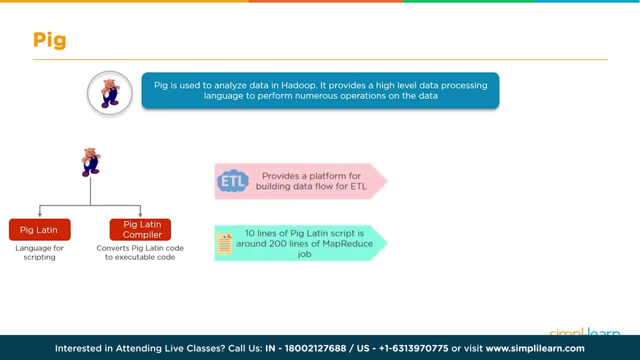 converts PIG Latin code to execute code. And then you have your ETL. The ETL provides a platform for building data flow for ETL And ETL is like the catch three letters now on any job interview. I look at It says ETL. It just means 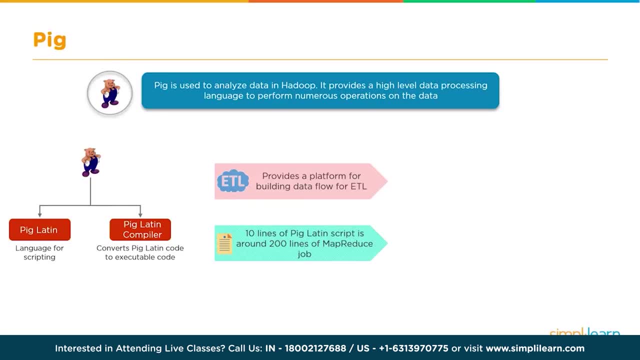 extract, transfer and load. So all we're doing is extracting the data, transferring it to where we need it and then loading it into, in this case, a Hadoop file system, And there's other pieces to that. It's actually a big thing. 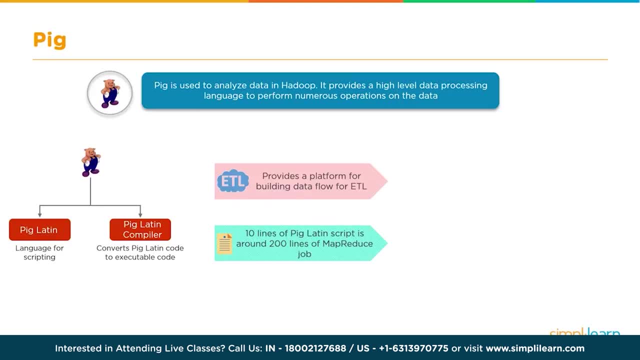 because whenever you're extracting data, do you want to dump all the data or do you want to do some kind of pre-processing? so you're only bringing in what you want. And then one of the cool things about PIG Latin is 10 lines of PIG Latin script is around. 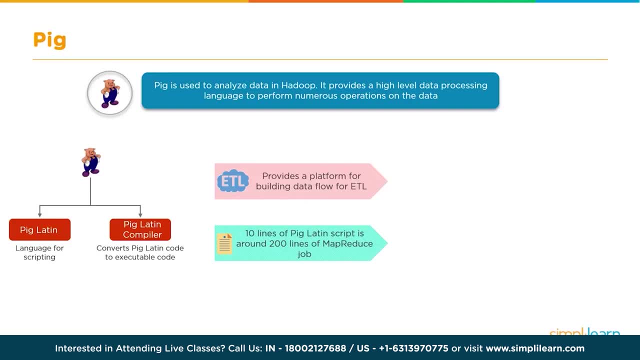 200 lines of MapReduce job. Again, the MapReduce is the backend processes that go on. So if we have PIG- and I'll be honest with you- PIG is very easy to use but as a scripter programmer I find 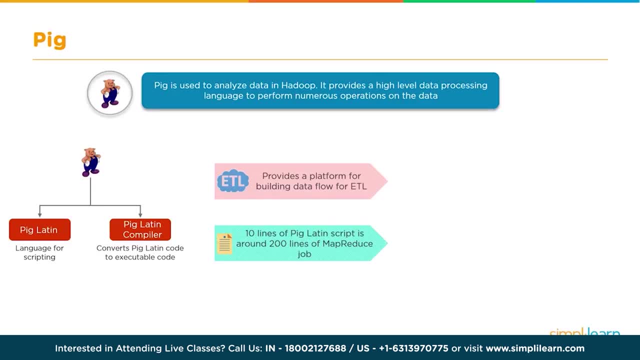 it's more for people who just need a quick pull of the data and able to do some very basic things very easily. So if you're doing some very high-end processing and model building, you usually end up in something else. So PIG's. 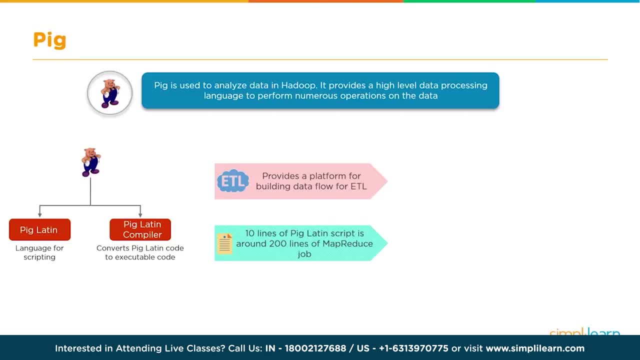 great for that, Like if you're in the management and you need to build a quick query report. PIG is really good for that, And so it definitely has its place. It's definitely a very useful script to know, And the PIG Latin. 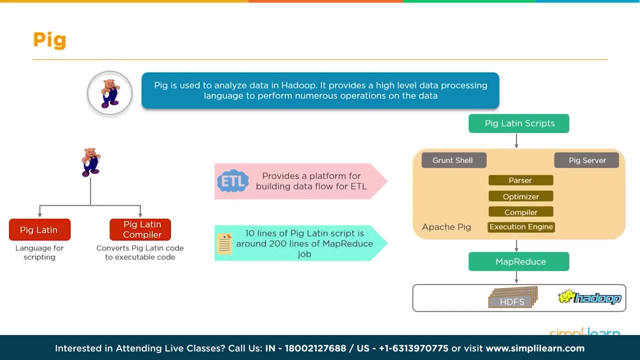 scripts. they call it the grunt shell. I guess it goes with pig because they grunt. You have your PIG server, you have a parser, an optimizer, a compiler, an execution engine, And that's all part of the Apache, PIG And this. 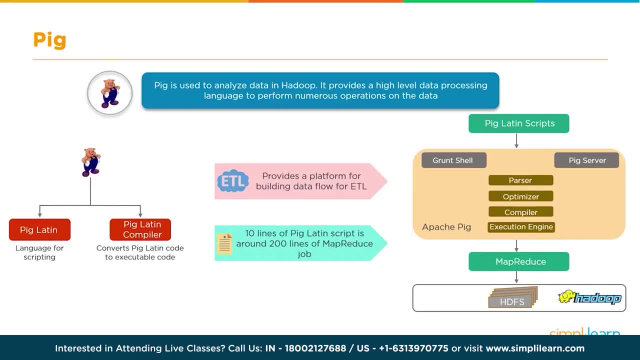 thing goes into the MapReduce, which then goes into the Hadoop file system. in the Hadoop And you'll see Apache with a lot of these, because it's under the open source, Hadoop's under the Apache open source. So all this. 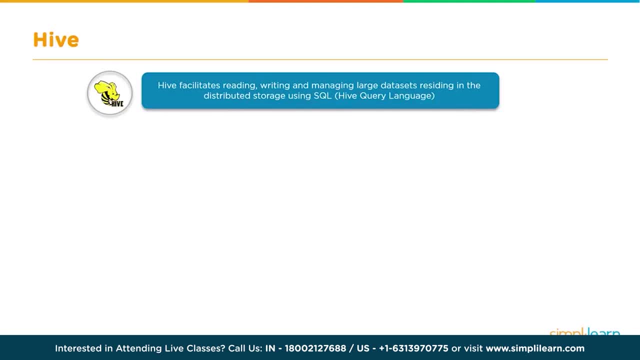 stuff. you'll see under Apache with the name tag on there And, if you're going to know, PIG Hive is the other one that's really popular for easy query. Hive facilitates reading, writing and managing large data sets residing in the distributed storage using 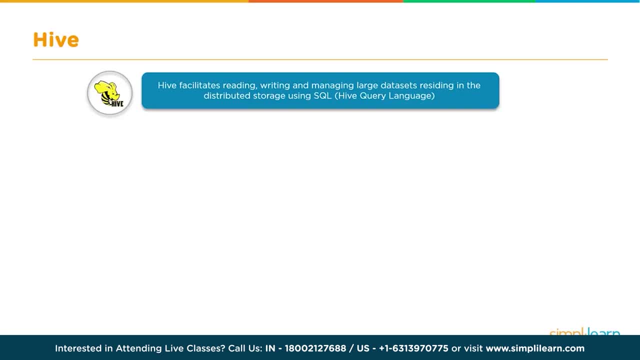 SQL Hive Query Language. And this is important because a lot of times you're coming from an SQL server. there's your enterprise set up and now you're archiving a history of what's going on on that server, So you're continually pulling data using Scoop. 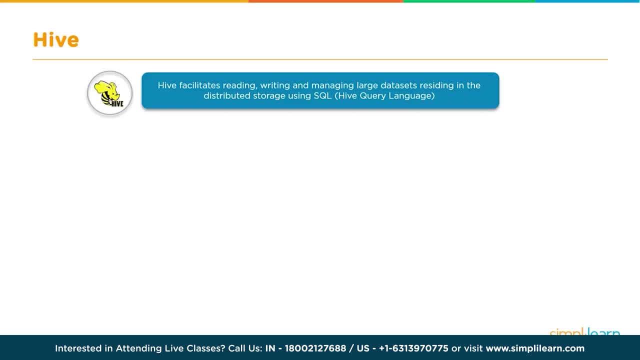 onto your into your H base Hive database And as it comes in there, it'd be nice to just use that same query to pull the data out of the Hadoop file system. And that's exactly what it does. So you have Hive command line. you can. 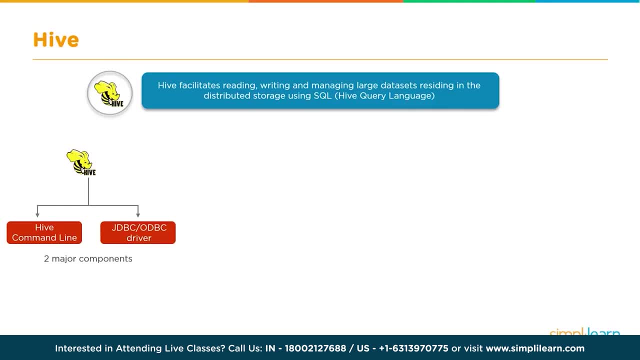 also use a JBC or ODBC driver And those drivers- like if you're working in Java or you're working in Python- you can use those drivers to access Hive So you don't have to go through the Hive command line. But it makes it real quick. I can take a. 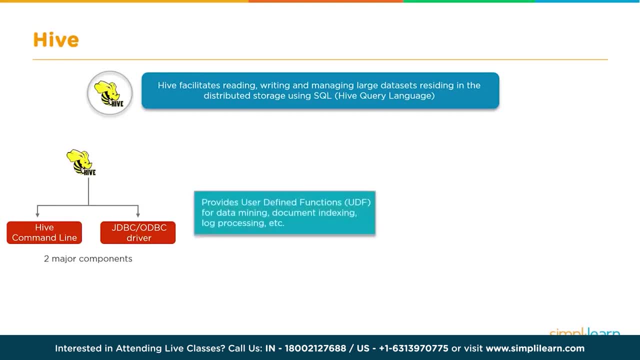 Hive command line and just punch in a couple words and pull up my data, And so it provides user defined functions, UDL, PDF for data mining, document indexing, log processing and anything that is in some kind of SQL format If it's stored. that. 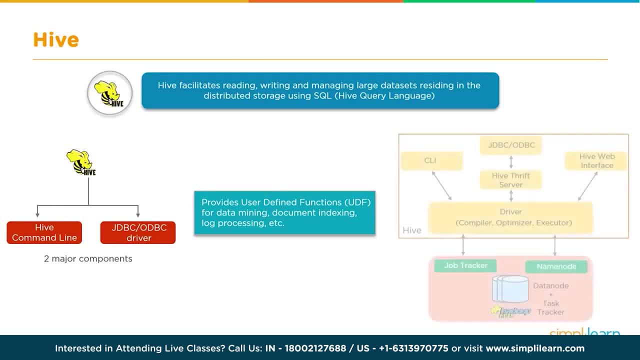 properly on the Hadoop file system. you can use your Hive to pull it out And you see even a more robust image of what's in the Hive. There's your client machine. that's you on your laptop or you're logged in. 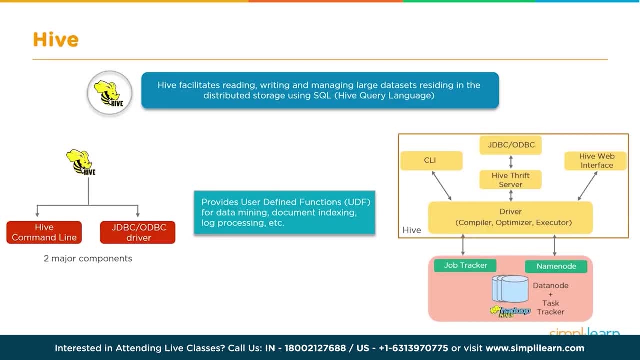 wherever you're at writing your script, That goes into the driver, where you have your compiler, your optimizer executor. You also have your JDBC ODBC connections, which goes into the Hive server, which then goes into the driver, Your Hive web interface. so you 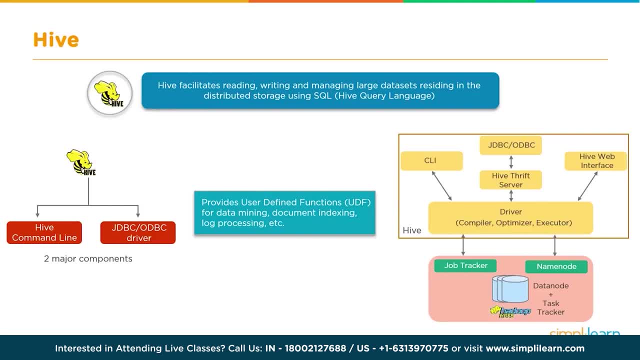 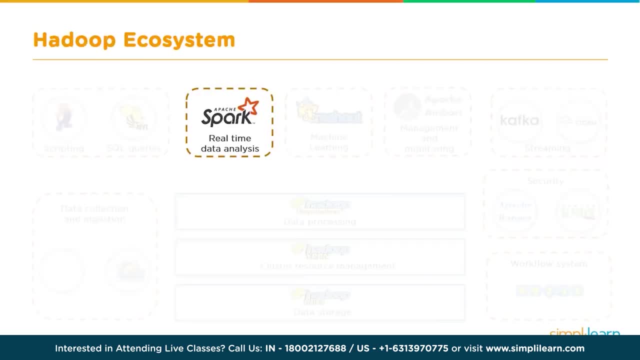 can just log in on the web and start typing away your SQL commands, and that again goes to the driver and all those pieces. And those pieces go to your job tracker, your name node and your actual Hadoop file system. So Spark. 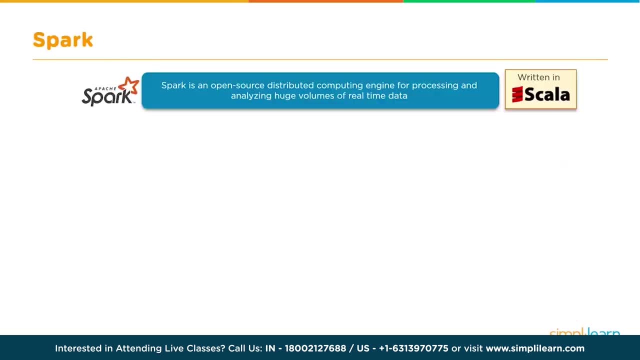 Real time data analysis. Spark is an open source distributed computing engine for processing and analyzing huge volumes of real time data, So it runs a hundred times faster than MapReduce. MapReduce is the basics of the Hadoop system, which is usually set up in a Java. 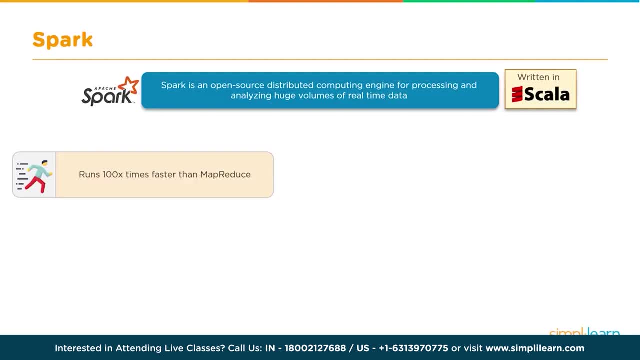 code In Spark, the MapReduce. instead of running, what happens in MapReduce is it goes, pulls it into the RAM, writes it to the hard drive, reads it off the hard drive, shuffles it around, writes it back to the hard drive, pulls it off the. 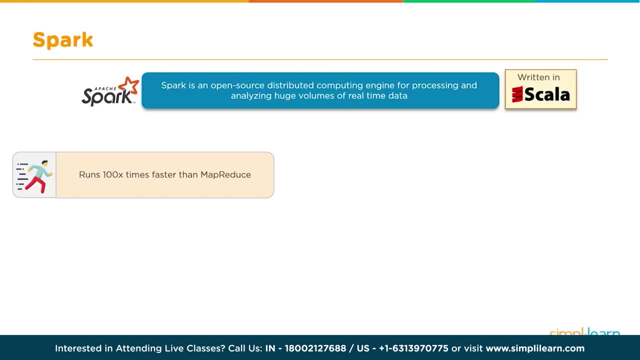 hard drive does its processing and you get the impression it's going in and out of RAM to the hard drive and back up again. So if you don't have a lot of RAM and you have older computers and you don't, 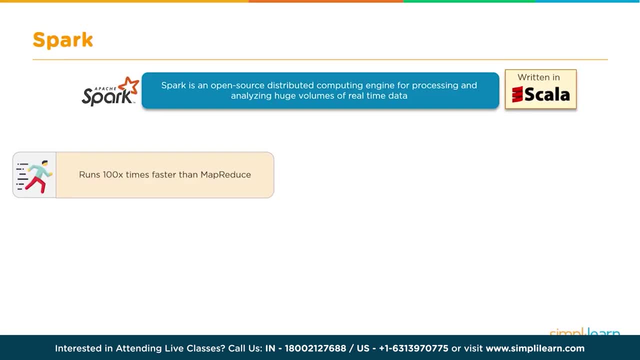 have the RAM to process something, then Spark and Hadoop are going to run the same speed. Otherwise Spark goes. hey, let's keep this all in the RAM and run faster. And that's what we're talking about. This provides in-memory computation of data, So it's 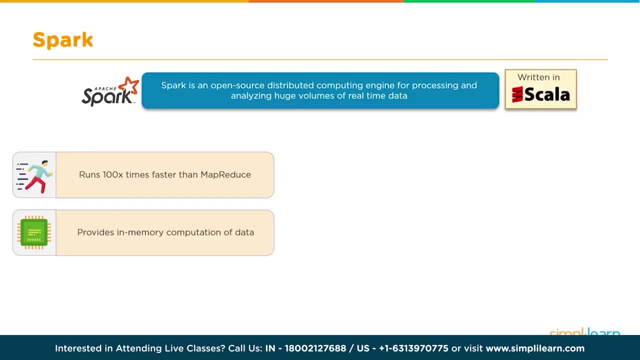 fast. You can see the guy running through the door there speedy versus a very slow Hadoop wandering around- And it's used to process and analyze real time streaming data such as stock market and baking data, So the Spark can have its own stuff going on. 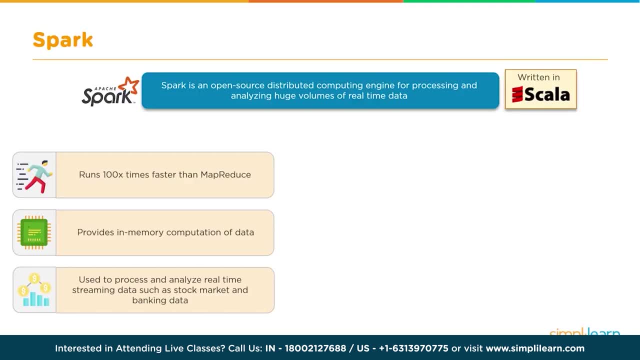 and then it can access the Hadoop database. it can pull data just like Scoop and Flume do, So it has all those features in it, And you can even run Spark with its own YARN. outside of Hadoop There's also Spark on Mesos, which is 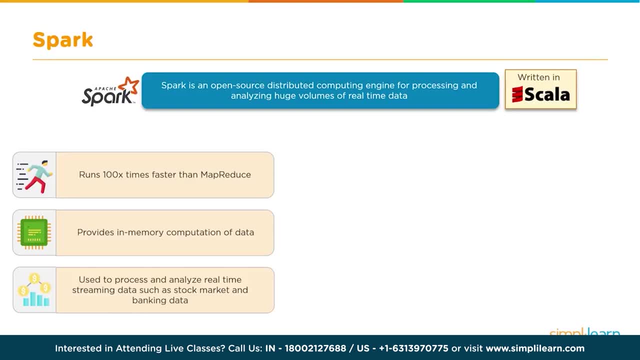 another resource manager. although YARN is most commonly used And currently Spark pretty much comes installed with Hadoop, And so your Spark running on top of Hadoop will use the same nodes. it has its own manager and it utilizes the RAM. 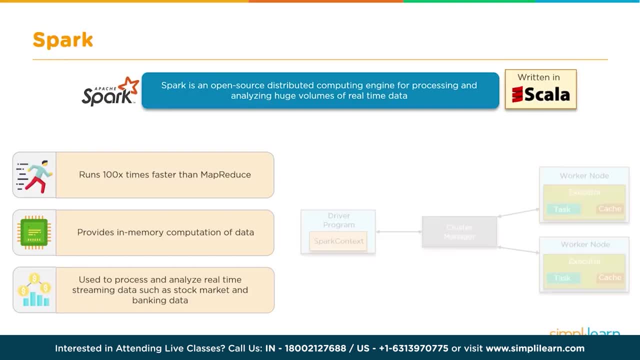 So you can have the Spark on top of there. And here we go. you have your driver program, your Spark context. it goes into your cluster manager, your YARN. then you have your worker nodes which are going to be executing tasks and cache. 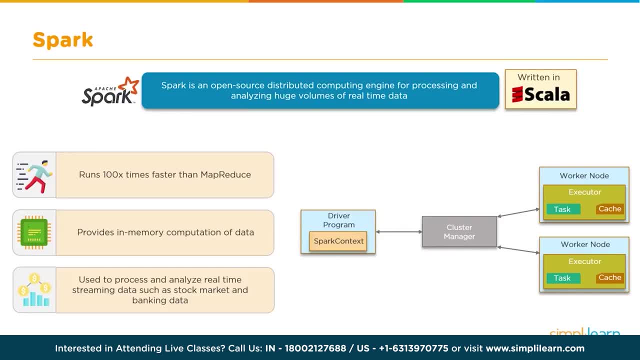 And it's important to remember when you're running the Spark setup. even though these are commodity machines, we're still usually a lot of them are like 128 gigabytes of RAM, So that Spark can run these high-end processes Certainly if it's. 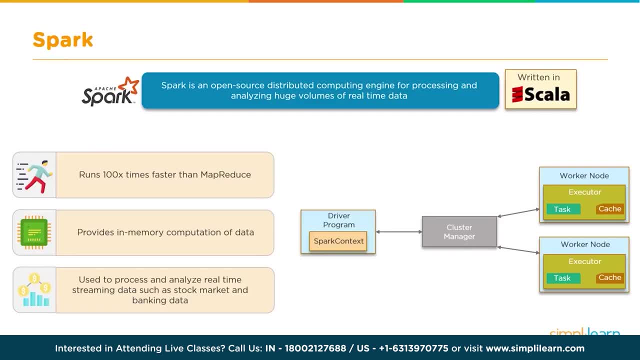 not accessed very much and you're building a Hadoop cluster. you could drop that RAM way down if you're doing just queries without any kind of processing on there And you're not doing a lot of queries. But you know, generally Spark you're looking at higher. 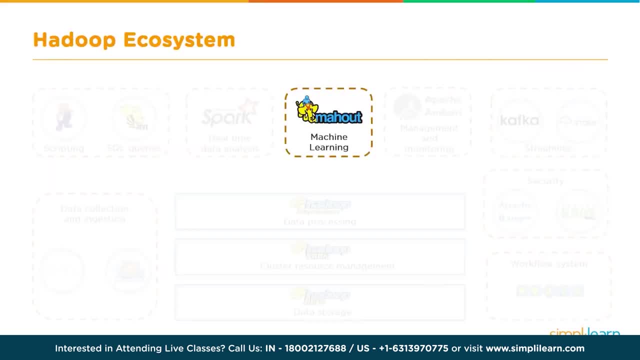 end, there's still commodity machines to do your work, And now we get into the Hadoop- machine learning, And so machine learning is its own animal. I keep saying that these are all kind of unique things. Mahout is being phased out. 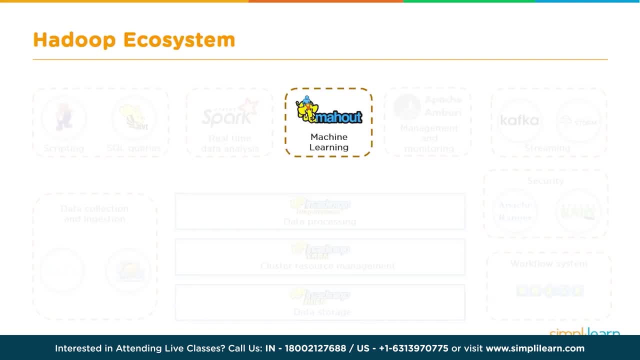 I mean people still use it. it's still important if you can write your basic machine learning that has most of the tools in there. You certainly can do it in Mahout. Mahout again. writes to the hard drive. reads from the hard drive. 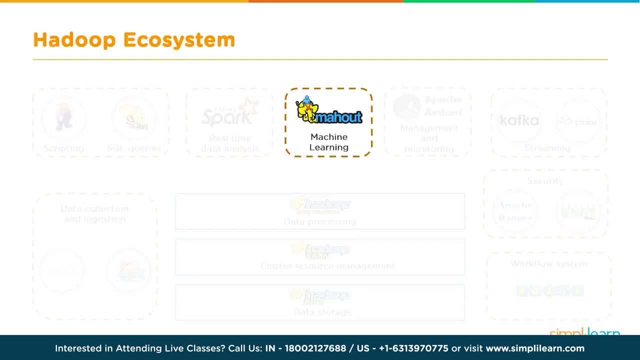 You can do all that in Spark, and it's faster because it's just in RAM, And so Spark has its own machine learning tools in it, And you can also use PySpark, which then accesses all the different Python tools, and there's just so many tools you can dump into Spark. 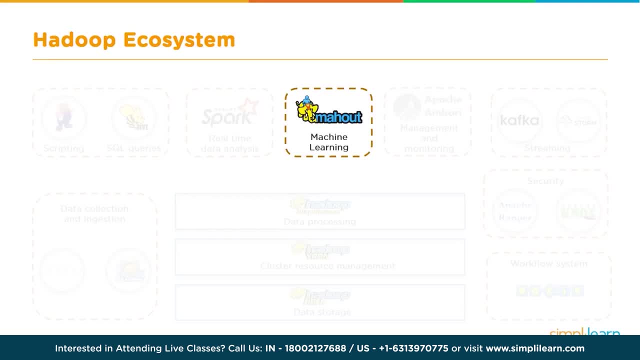 Mahout is very limited, but it's also very basic, which in itself can be really good. Sometimes simple is better. So Mahout is used to create scalable and distributed machine learning algorithms. So here we have our Mahout environment. It builds a machine learning application. 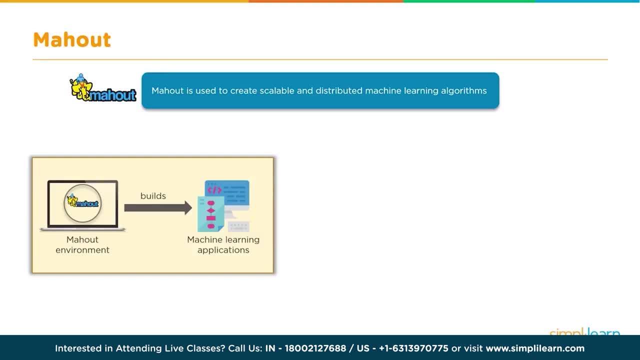 So you're doing linear regression, you're doing clustering, you're doing classification models. It has a library that contains inbuilt algorithms for all of these, and then it has collaborative filtering, And again there's our classification and there's our clustering. 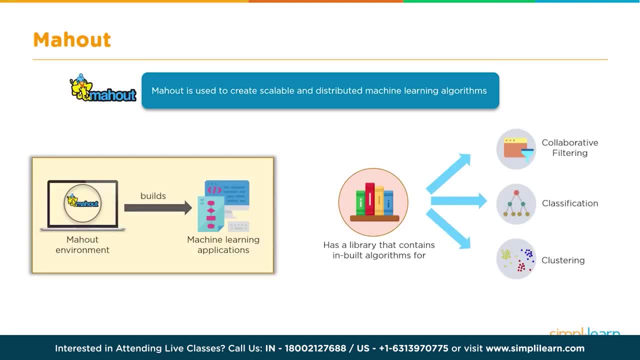 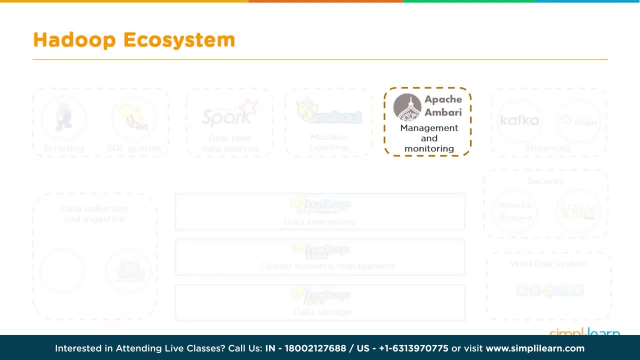 Regression, so you have your different machine learning tools. we can easily classify a large amount of data using Mahout. So this brings us to the next set of tools we have, or the next tool, which is the Apache Ambari. Ambari is an open source tool responsible. 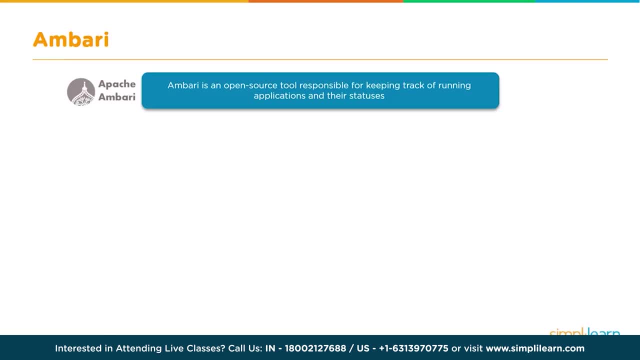 for keeping track of running applications and their statuses. Think of this as like a traffic cop, more like a security guard. You can open it up and see what's going on, And so the Apache Ambari manages monitors and provisions. Hadoop clusters. 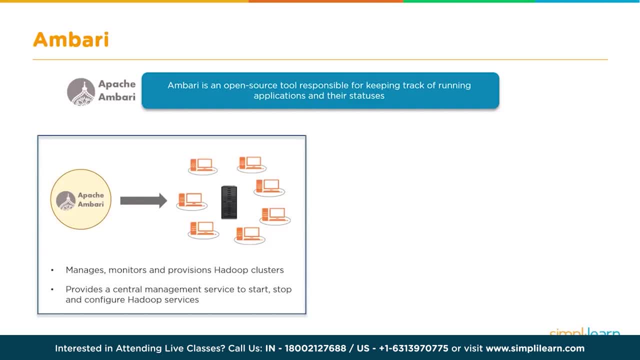 provides a central management service to start, stop and configure Hadoop services. So again it's like a traffic cop. Hey, stop over there, start, keep going. Hey, what's going on over that area in the through lane on the high speed? 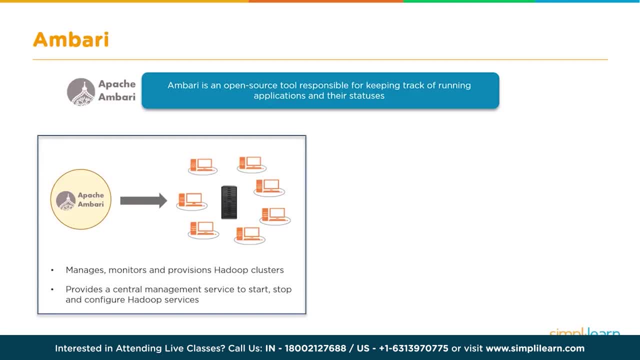 freeway And you can open this up and you have a really easy view of what's going on, And so you can see. right here you have the Ambari web. The Ambari web is what you're looking at, That's your interface that you've. 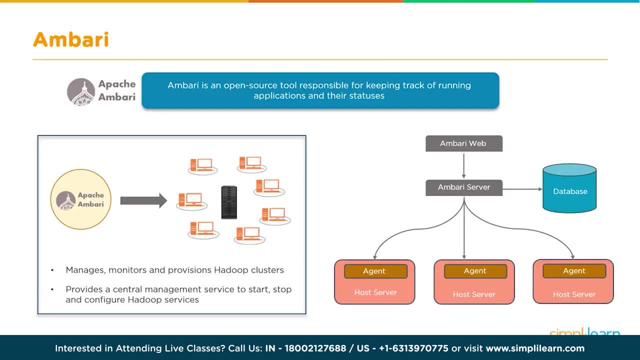 logged into the Ambari server. This will be usually on the master node. It's usually: if you're going to install Ambari, you might as well just install it on the same node And it connects up to the database and then it has. 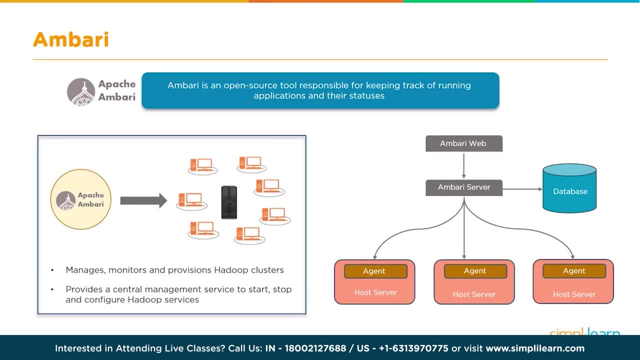 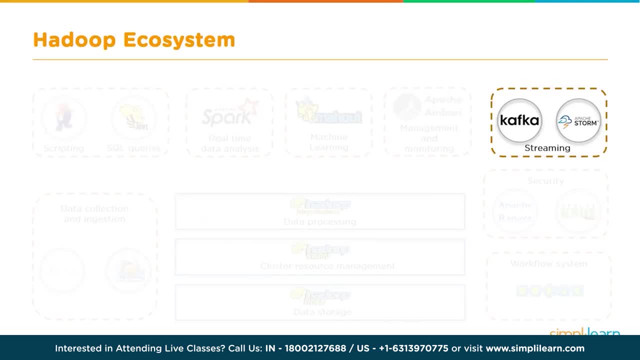 agents And each agent takes a look and see what's going on with its host server. And if you're going to have two more systems- and we talked about Spark streaming- there's also Kafka and Apache for streaming data coming in And Kafka is distributed. 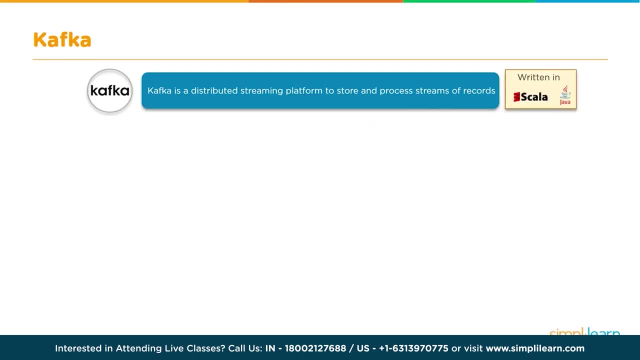 streaming platform to store and process streams of records, And it's written in Scala. Builds real time streaming data pipelines that reliably get data between applications. Builds real time streaming applications that transforms data into streams, So it kind of goes both ways on there. So Kafka uses: 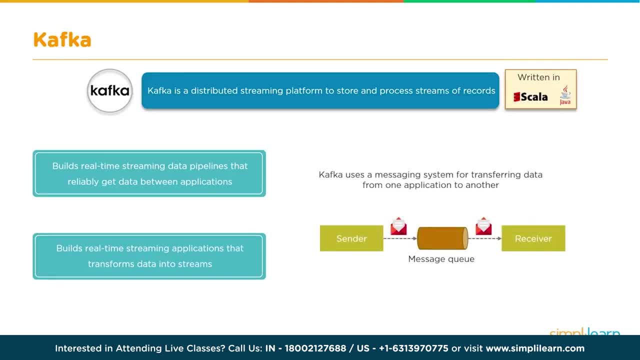 a messaging system for transferring data from one application to another. So we have our sender, we have our message queue and then we have our receiver. Pretty straightforward, very solid setup on there with the Kafka Apache Storm. Storm is a processing engine that. 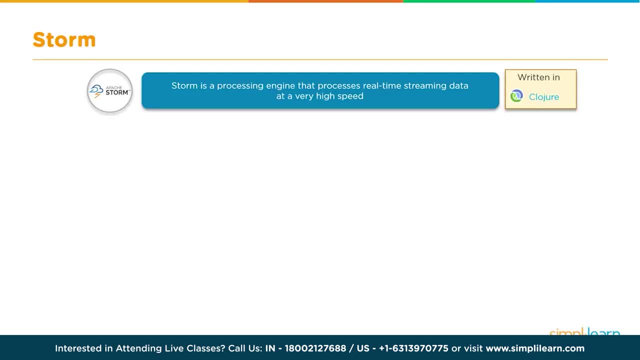 processes real time streaming at a very high speed And it's written in Clojure. They utilize the function based programming style of Clojure and it's based on Lisp to give it the speed. That's why Apache Storm is built on there, So you can think. 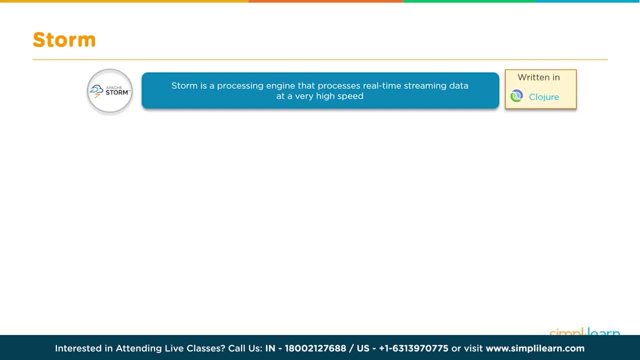 of Kafka as a slow moving, very solid communication network where Storm is looking at the real time data and grabbing that streaming data that's coming in fast, So it has the ability to process over a million jobs in a fraction of seconds on a node. So it's. 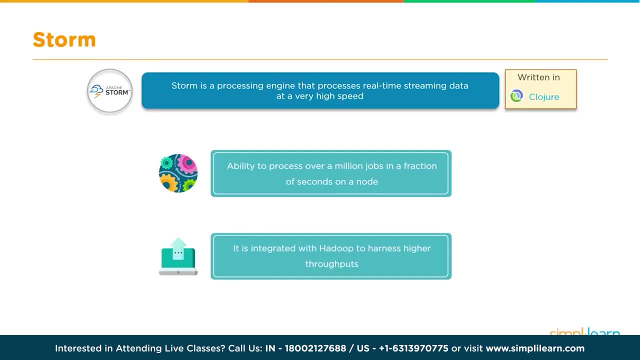 massive. It can really reach out there and grab the data, And it's integrated with Hadoop to harness higher throughputs. So this is the two big things about Storm, If you are polling. I think they mentioned stock coming in or something like that. 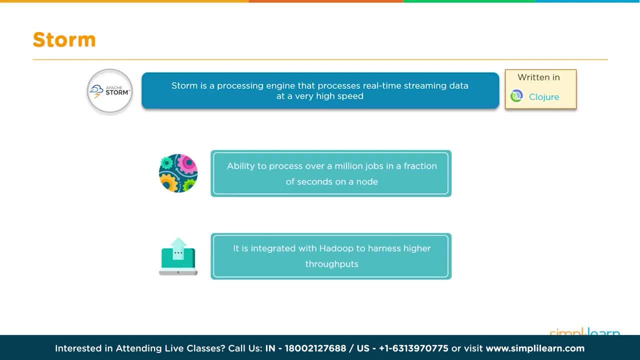 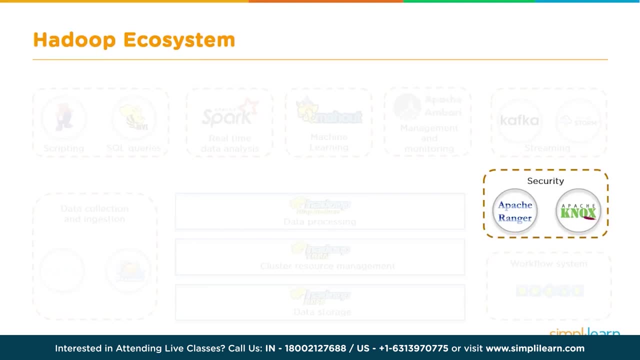 where you're looking for the latest data popping up. Storm is a really powerful tool to use for that, So we've looked at a couple more tools for bringing data in. We probably should talk a little bit about security. Security in Hadoop has the 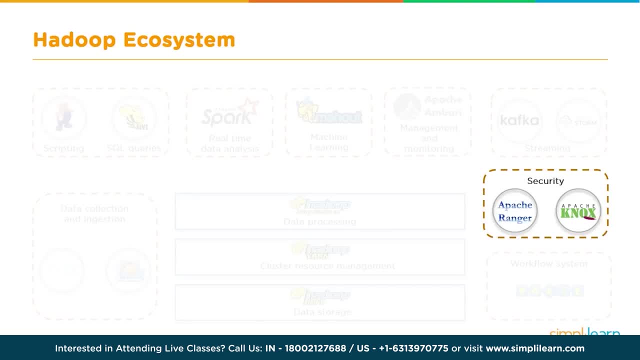 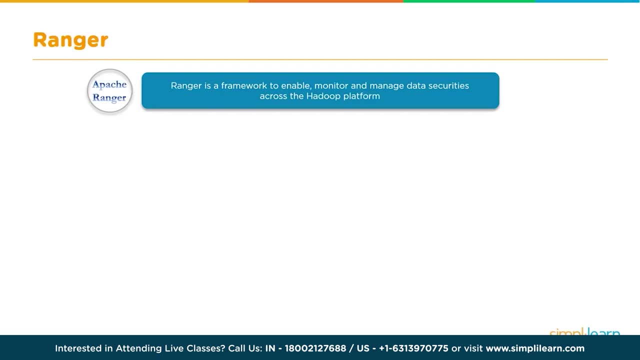 Apache Ranger and Apache Knox are the two most popular ones, And the Ranger- the Apache Ranger Ranger- is a framework to enable, monitor and manage data securities across the Hadoop platform. So the first thing it does is it provides centralized security administration to manage all. 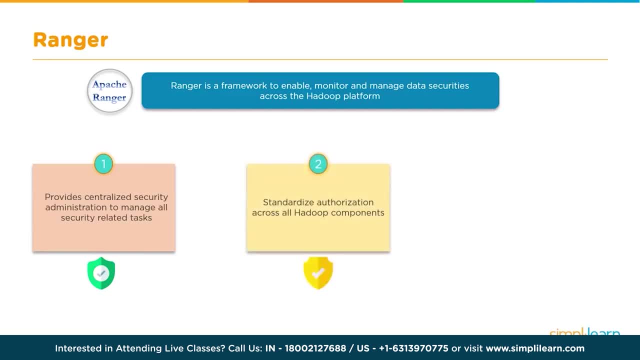 security related tasks. The second thing it does is it has a standardized authorization across all Hadoop components. And third, it uses enhanced support for different authorization methods: Role based access control, attribute based access control, etc. So your Apache Ranger can go. 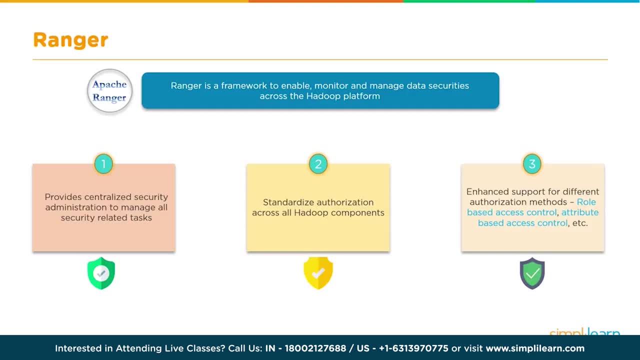 in there and your administrator coming in there can now very easily monitor who has what rights and what they can do and what they can access. So there's also Apache Knox. Knox is an application gateway for interacting with the REST APIs and the UIs of Hadoop. 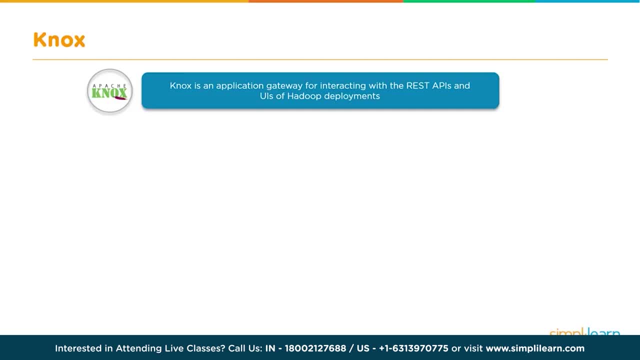 developers, And so we have our application programmer interfaces, our user interfaces and we talk about REST APIs. this means we're pulling. this is looking at the actual data coming in, what applications are going on. So if you have an application where people are pulling, 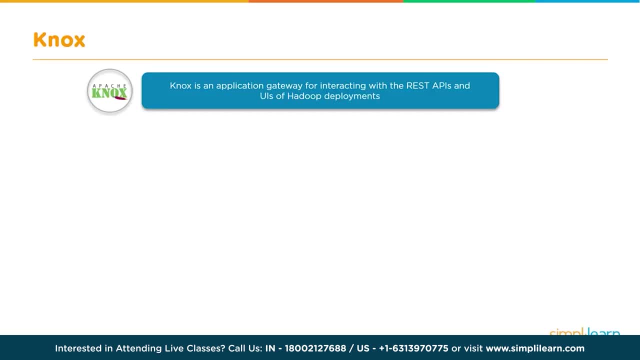 data off of the Hadoop system or pushing data into the Hadoop system. the Knox is going to be on that setup And it delivers three groups of user facing services. One, proxy services, provides access to Hadoop via proxying the HTTP. 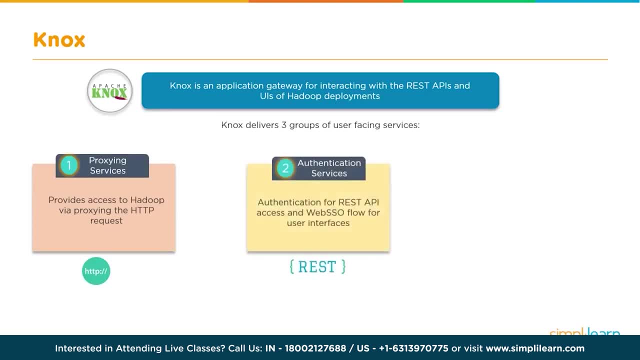 request Two authentication services: authentication for REST API access and web SSO flow for user interfaces. So there's our REST And finally client services. Client development can be done with the scripting through DSL or using the Knox shell classes. So the first one is if you have a website. 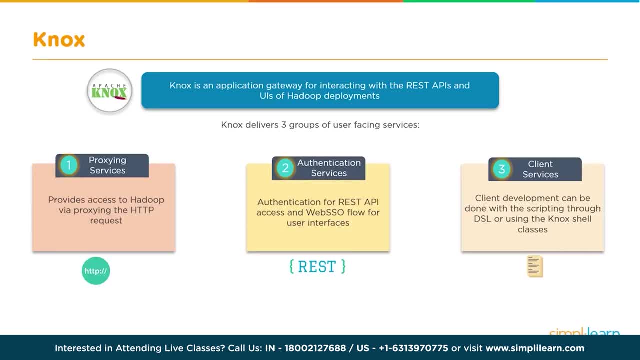 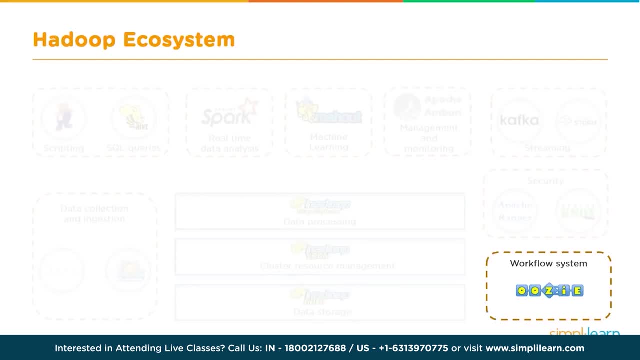 coming in and out of your HTTP request. Again, your three different services are what's coming in and out of the Hadoop file system. So there's a couple of the security setups. Let's go ahead and take a look at workflow system, the Uzi. 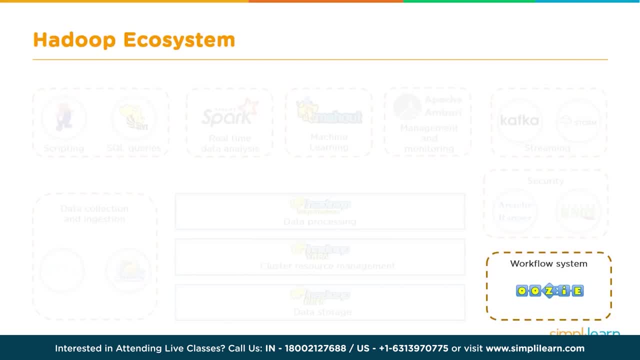 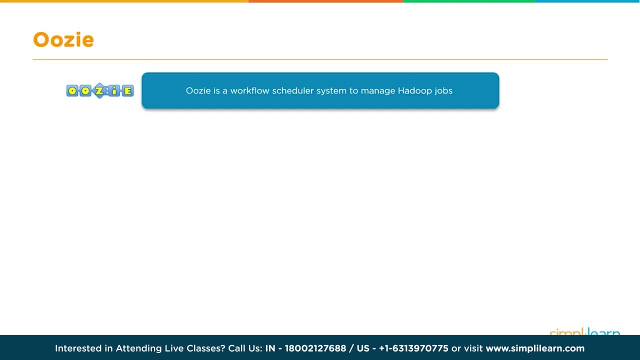 And there's some other ones out there. Uzi is the one that's specific to Hadoop. There's also like a Zookeeper out there and some other ones. Uzi's pretty good. Uzi is a workflow scheduler system to manage Hadoop jobs. 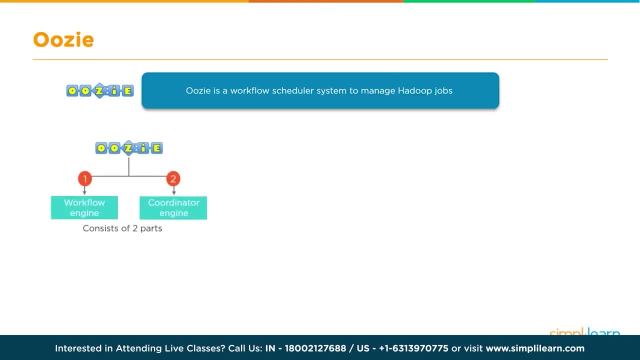 And so you have a workflow engine and a coordinator engine. So it consists of two parts: What's going on and coordinating. what's going on And directed acyclic graph, DAGs, which specifies a sequence of actions to be executed. These consist of workflow jobs. 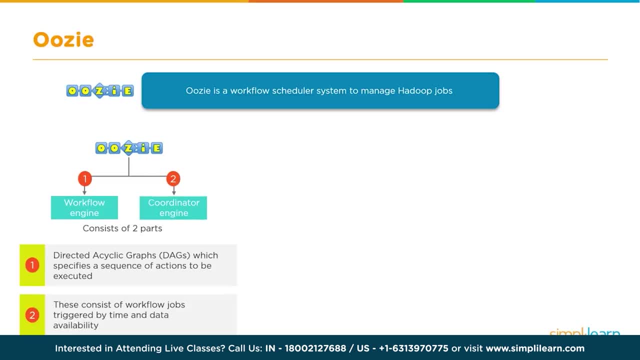 triggered by time and data available. And if you're not familiar with directed acyclic graphs or DAGs or whatever terminology you want to throw at this, this is basically a flow chart. You start with process A, then the next process would be process B when process A is done. 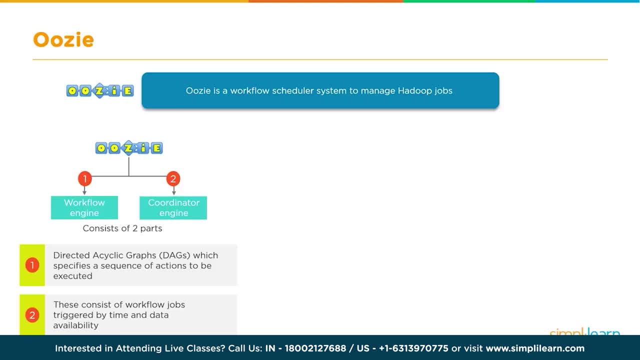 And it might be that process C can only be done when process D, E and F are done. So you want to be able to control this. You don't want it to process the machine learning script and then pull the data, in that you want to process it on. 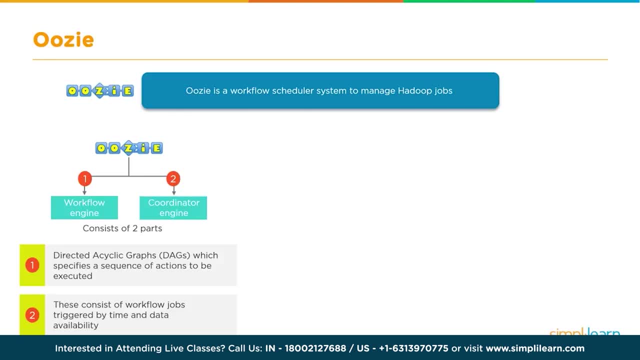 You want to make sure it's going in the right order. So these consist of workflow jobs and they're triggered by time and data availability. So maybe you're pulling stocks in the middle of the night and once the stock is all pulled, so there's our time sequence that says hey. 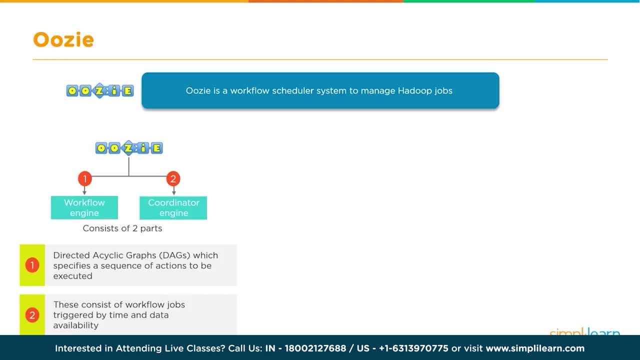 they've been posted on the other websites. They post them usually after the stock market closes, the highs and lows and everything Then once that data has been brought in, you know on a time specifics, bringing the data in at a certain time, once the data is available. 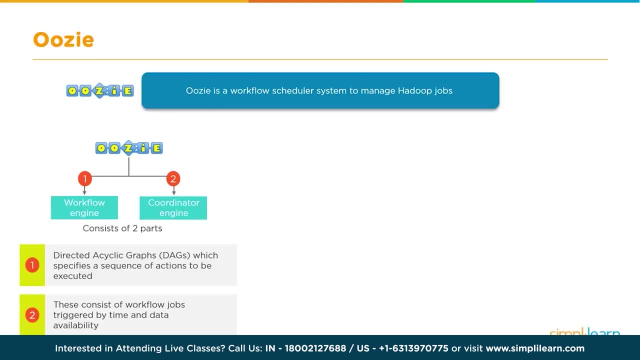 then we want to trigger our machine learning script for what's going to happen next. And so we can see, here we have start our MapReduce program, our action node, and it begins, and either we have a success, then we notify the client of. 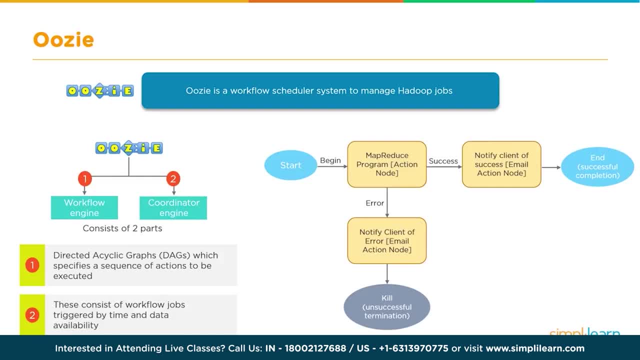 success, usually an email sent out in successful completion, Or we don't have a success. we have an error, Notify client of error. email action node skill, unsuccessful termination, And usually at this point they say email action notification, but I'm mostly 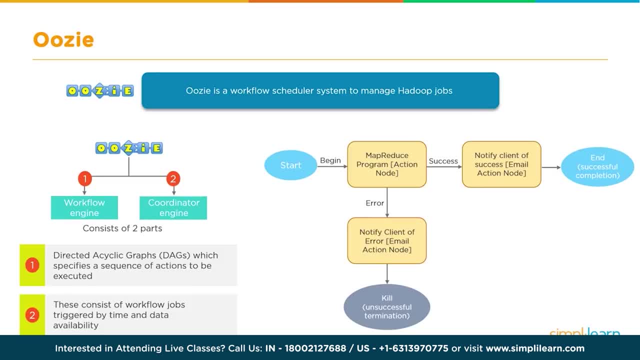 that's usually a pager system, and so you see all the tech guys running to the server room or wherever. you know our pager just went off. we gotta figure out what went down, You know. the other one is: you just look at them the next morning and you go. 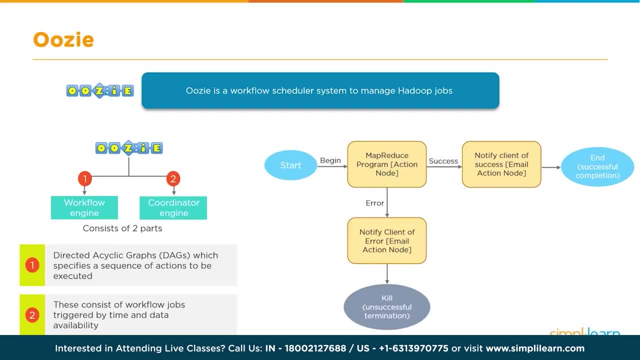 oh, let's make sure everything went through this morning and check all your successes With the error. usually it's sent to your pager and your emergency call to open up in the middle of the night and log in. So that concludes our basic setup with the. 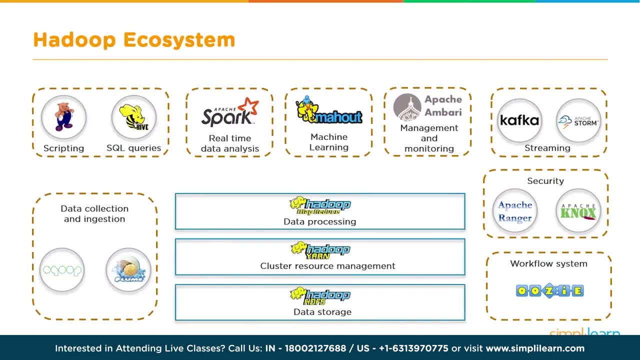 Hadoop ecosystem. So a quick recap on the Hadoop ecosystem. We covered going. looking at the middle part, we had the Hadoop as a file system and how it stores data across multiple servers. saves money because it's about a tenth of the cost of using. 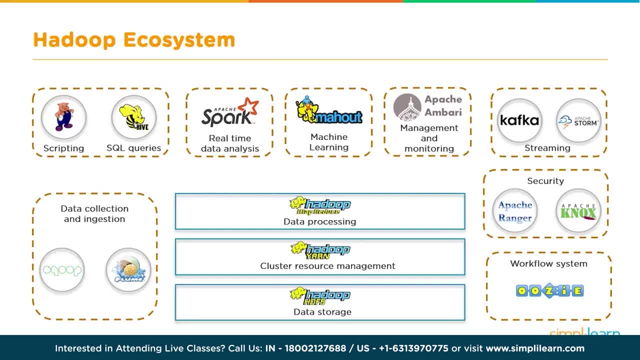 enterprise computers. We looked at yarn cluster resource management and how that works to hold everything together. And then we looked at a lot of data processing. How does it process in and out of the Hadoop system, including the map and reduce setup, which is the Hadoop? 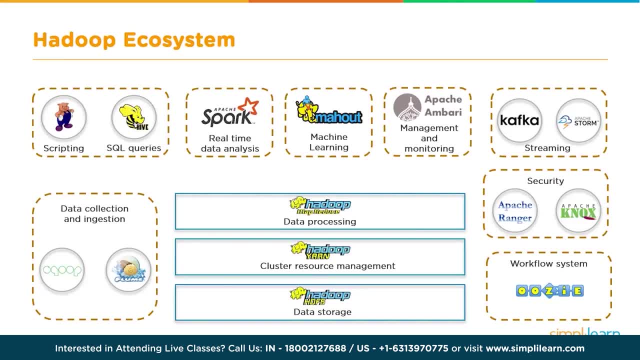 basic in Java And for that we looked at data collection and ingestion with Scoop and Flume. We looked at queries using the scripting language Pig and the SQL queries through Hive. We glanced at Spark. Remember, Spark usually comes installed now with the Hadoop system. 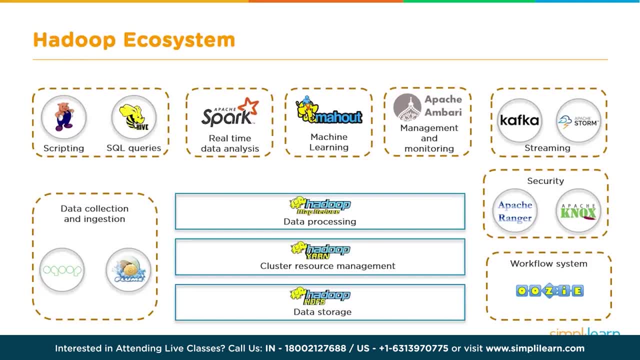 because it does so much of its own processing. It covers a lot of the data in real time data analysis setup on there. We looked at Mahout machine learning. We looked at Apache Ambari for management and monitoring kind of your security guard and traffic control. 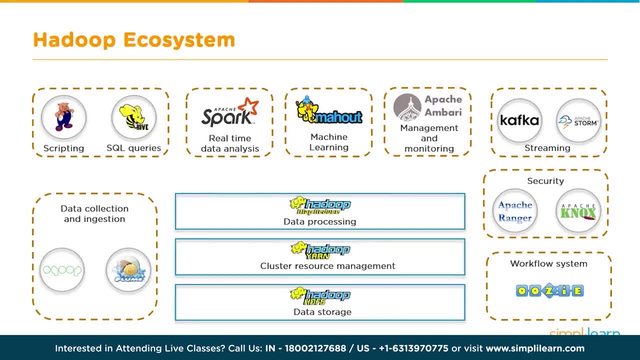 Just like we have Scoop and Flume, which brings data in there, We looked at Kafka and Apache Storm, which is for streaming data, And then we looked at Apache Ranger and Apache Knox for security And finally we went in through the. we took a glance at Uzi for your. 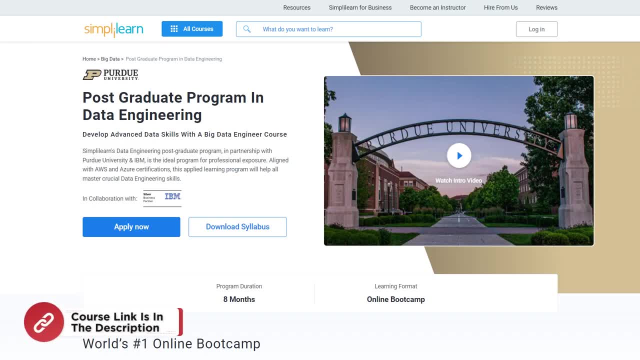 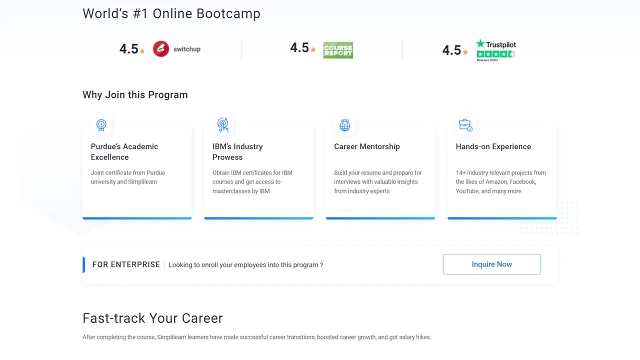 workflow system Now. whether you are an Aspirin data analyst, a seasoned IT professional or a business leader looking to leverage the power of big data, the data engineering post graduate program by Simply Learn, in collaboration with Purdue University and IBM, is tailored to meet your needs. This program 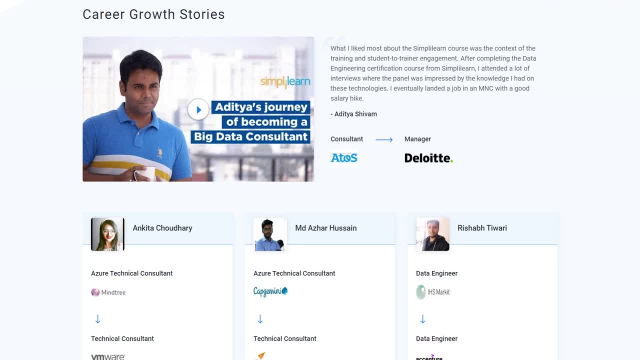 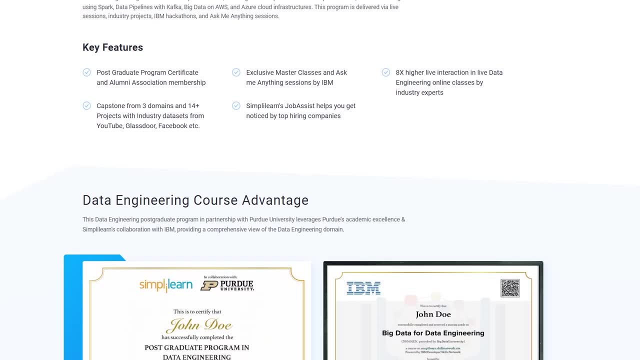 offers an exceptional opportunity for professional growth and exposure, with a focus on practical learning and in alignment with industry-leading certifications from AWS and Azure. Now this program equips participants with essential skills required to excel in this field of data engineering By enrolling in this. 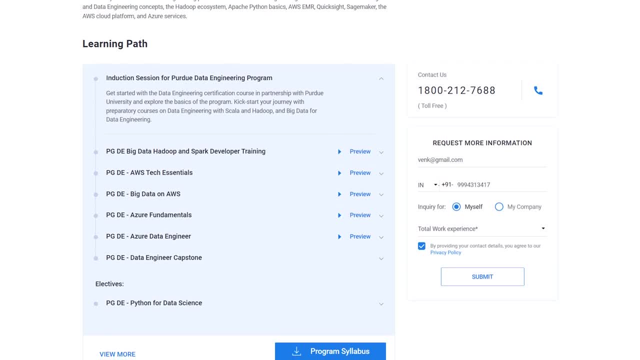 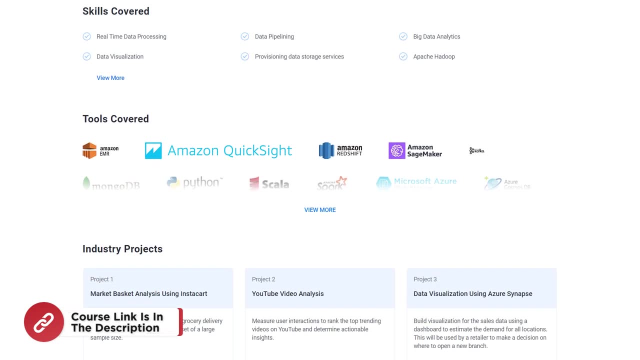 applied learning program. individuals can gain, master crucial data engineering techniques and technologies. Enroll today and take the next step towards becoming a proficient big data professional. Check out the course link in the description box below for more details. What is data science? Let's start with. 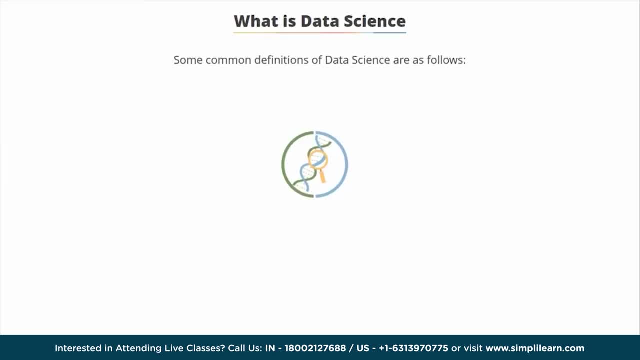 some of the common definitions that's doing the rounds. Some say that data science is a powerful new approach for making discoveries from data. Others term it as an automated way to analyze enormous amounts of data and extract information from it. Still others refer to it as a new discipline. 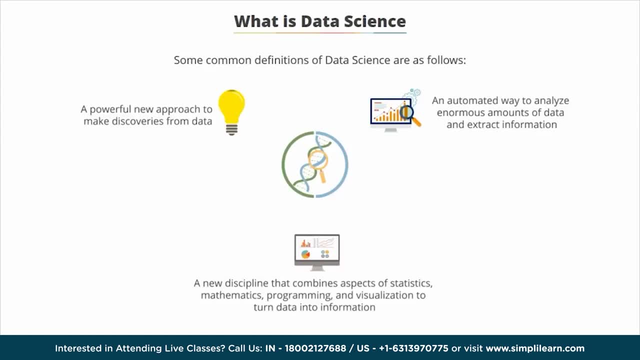 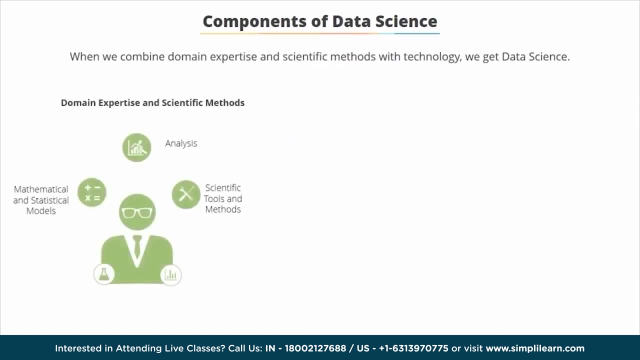 which combines aspects of statistics, mathematics, programming and visualization to gain insights. Now that you have looked at some of its definitions, let's learn more about data science. When domain expertise and scientific methods are combined with technology, we get data science, which enables one to find solutions. 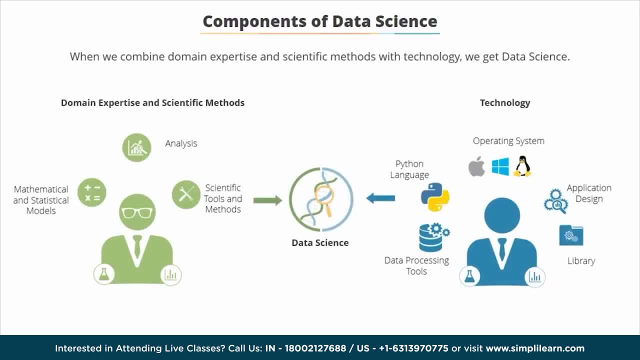 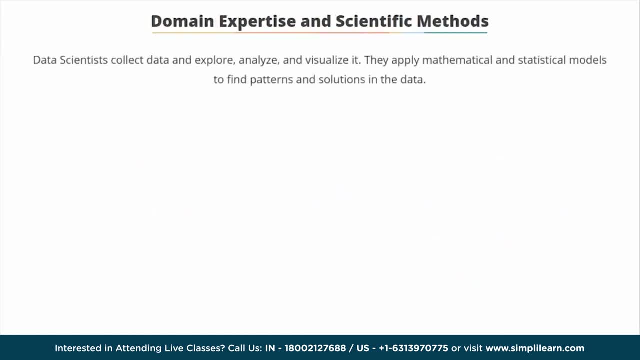 for existing problems. Let's look at each of the components of data science separately. The first component is domain expertise and scientific methods. Data scientists should also be domain experts, as they need to have a passion for data and a passion for technology. Data scientists should also be. 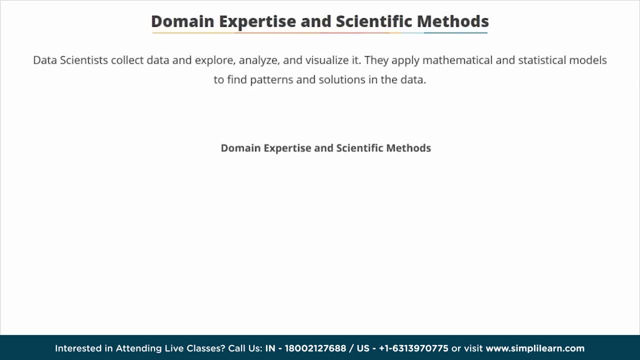 domain experts, as they need to have a passion for data and discover the right patterns in them. Traditionally, domain experts, like scientists and statisticians, collected and analyzed data in a laboratory setup or a controlled environment. The data was then subject to relevant laws or mathematical and statistical models. 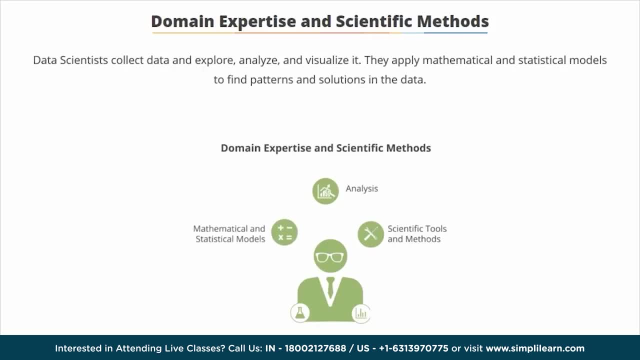 to analyze the data set and derive relevant information from it. For instance, they used the models to calculate the mean, median mode, standard deviation and so on of a data set. It helped them test their hypothesis or create a new one In the next slide. 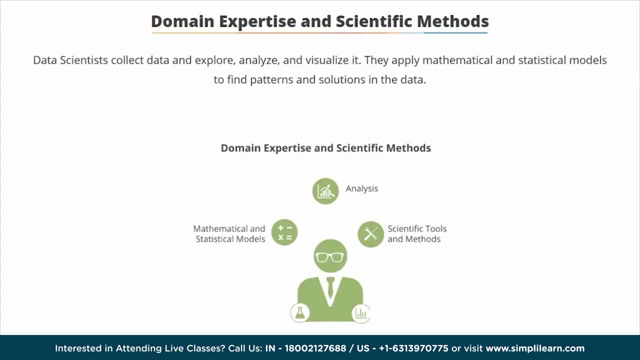 we will see how data science technology has now made this process faster and more efficient. But before we do that, let's understand the different types of data analysis, an important aspect of data science. Data analysis can either be descriptive, where one studies a data set. 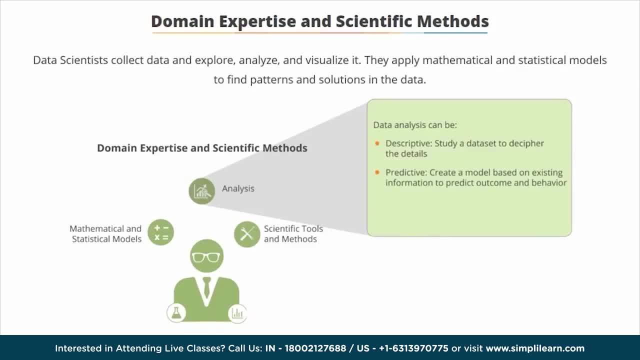 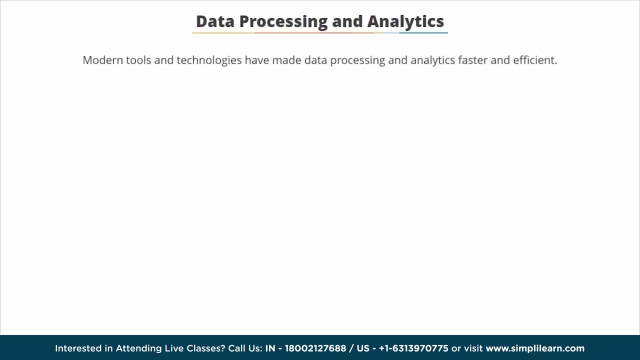 to explain what happened, or be predictive, where one creates information to predict the outcome and behavior. It can also be prescriptive, where one suggests the action to be taken in a given situation using the collected information. We now have access to tools and techniques that process data. 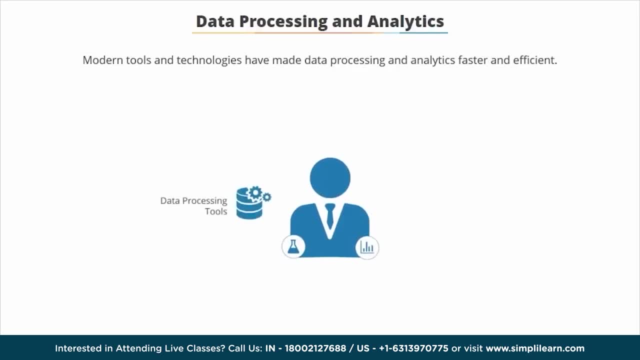 and extract the information we need. For instance, there are data processing tools for data wrangling. We have new and flexible programming languages that are more efficient and easier to use. For example, we can now integrate systems and process big data on multiple OS platforms. 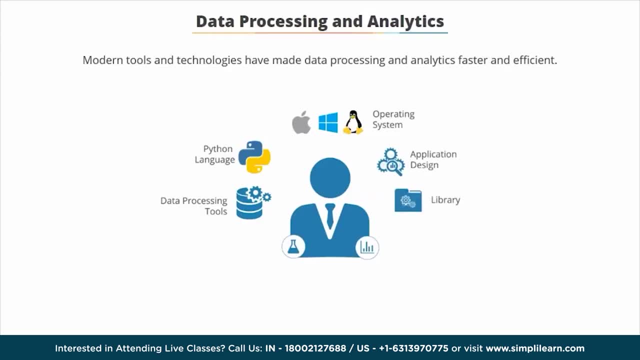 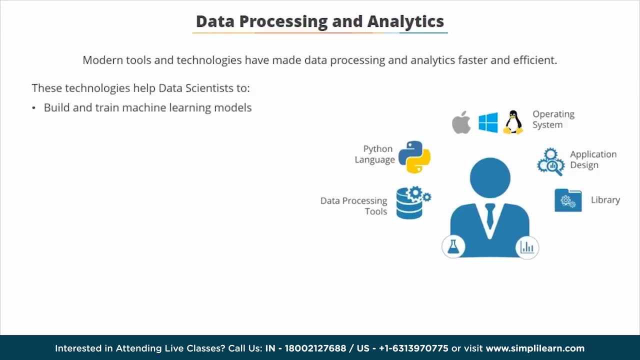 Application designs and extensive software libraries help develop more robust, scalable and data-driven applications. Data scientists use these technologies to build data models and run them in an automated fashion to predict the outcome efficiently. This is called machine learning, which helps provide insights into the underlying data. 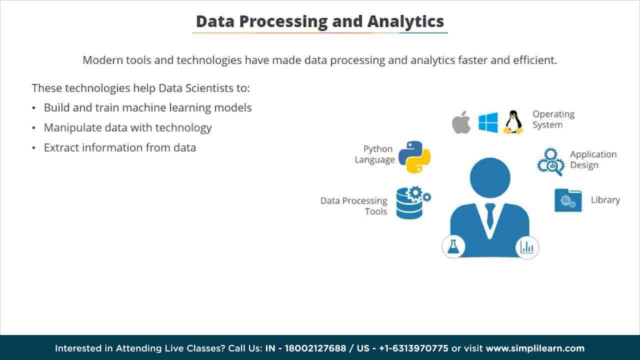 Data scientists use technology to manipulate data, extract information from it and use it to build tools, applications and services. But technological skills and domain expertise alone, without the right mathematical and statistical knowledge, might lead data scientists to find incorrect patterns and convey the wrong information. 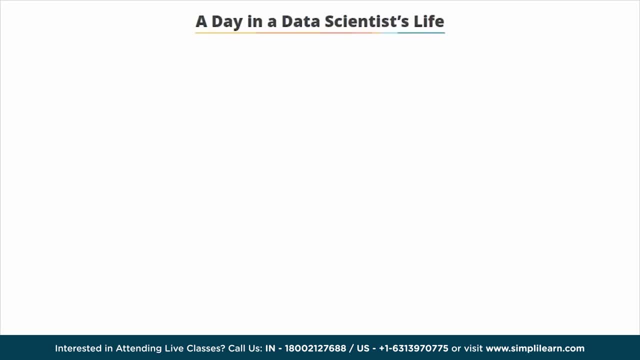 Now that you have learned what data science is, let's start with a question or a business problem. Then they use data acquisition to collect datasets from the real world. The process of data wrangling is implemented with data tools and modern technologies that include data cleansing. 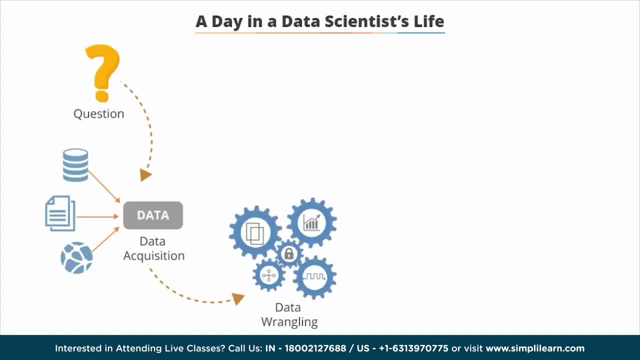 data manipulation, data discovery and data pattern identification. The next step is to create and train models for machine learning. They then design mathematical or statistical models. These models are created using data visualization techniques. The next task is to prepare a data report. After the report is prepared, 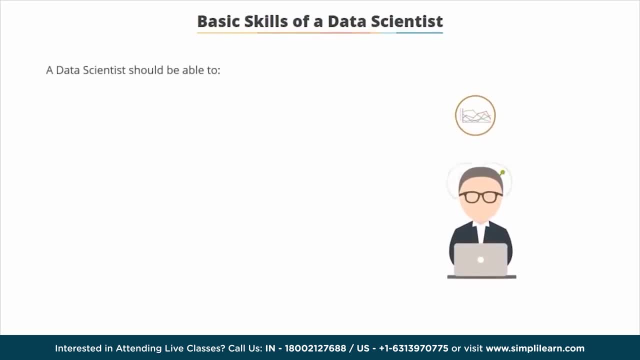 they finally create data products and services. Let us now look at the various skills a data scientist should have. Data scientists should ask the right questions, for which they need domain expertise, the curiosity to learn and create concepts and the ability to communicate questions effectively to domain experts. 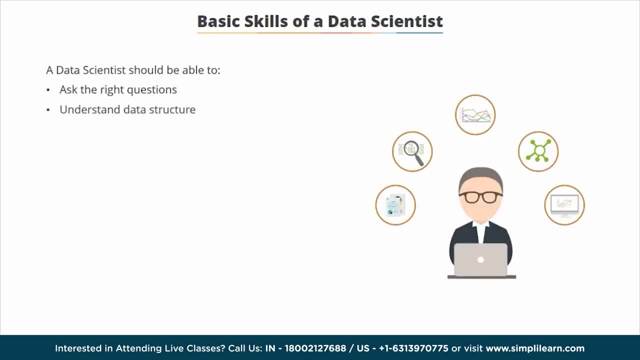 Data scientists should think analytically to understand the hidden patterns in a data structure. They should wrangle the data by removing redundant and irrelevant data collected from various sources. Statistical thinking and the ability to apply mathematical methods are important traits for a data scientist. 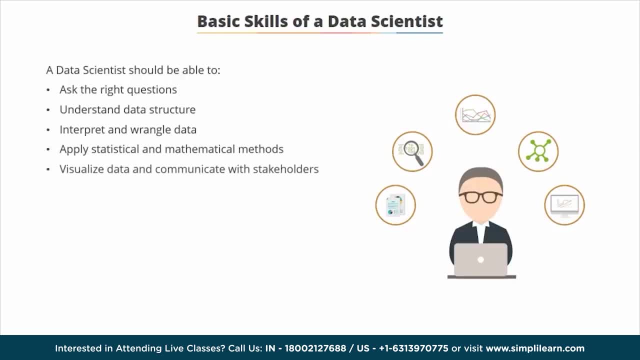 Data should be visualized with graphics and proper storytelling to summarize and communicate the analytical results to the audience. To get these skills, they should follow a distinct roadmap. They should use the required tools and techniques, like Python and its libraries. They should build projects using 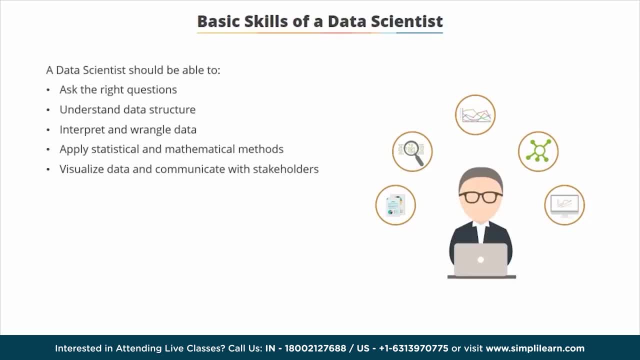 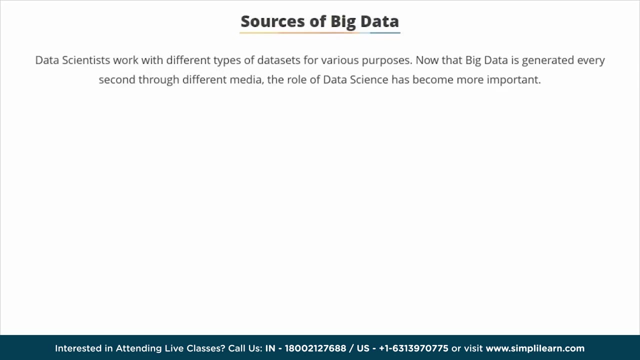 real-world data sets that include datagov, NYC Open Data, Gapminder and so on. They should also build data-driven applications for digital services and data products. Scientists work with different types of data sets for various purposes. Now that big data is generated, 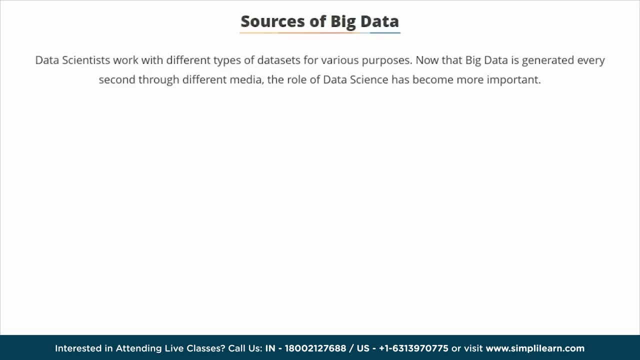 every second through different media. it has become more important, So you need to know what big data is and how you are connected to it to figure out a way to make it work for you. Every time you record your heartbeat through your phone's biometric sensors. 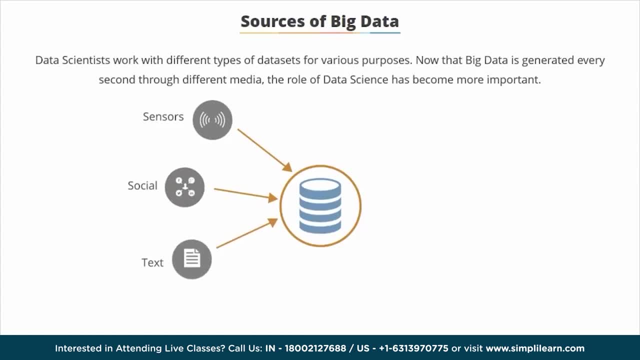 post or tweet on the social network, create any blog or website, switch on your phone's GPS network, upload or view an image, video or audio. In fact, every time you log into the internet, you are generating data about yourself, your preferences. 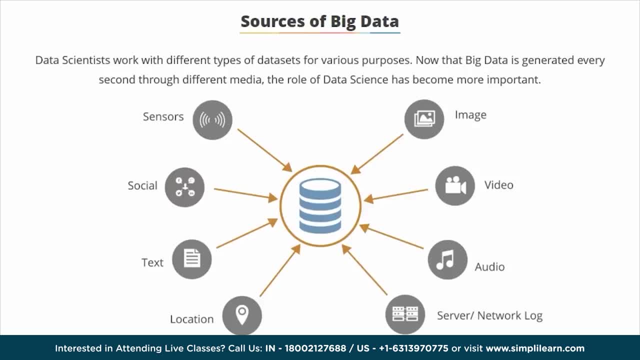 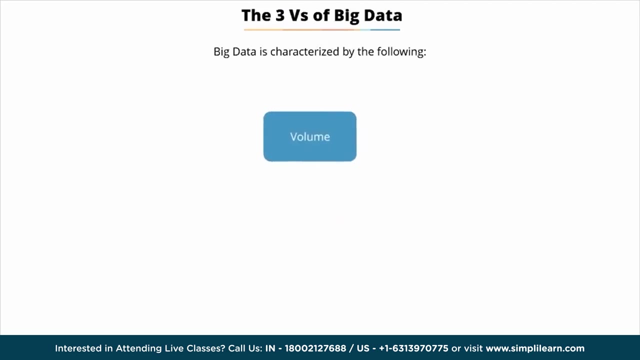 and your lifestyle. Big data is a collection of these and a lot more data that the world is constantly creating. In this age of the Internet of Things, or IoT, big data is a reality and a need. Big data is usually referenced by three Vs. 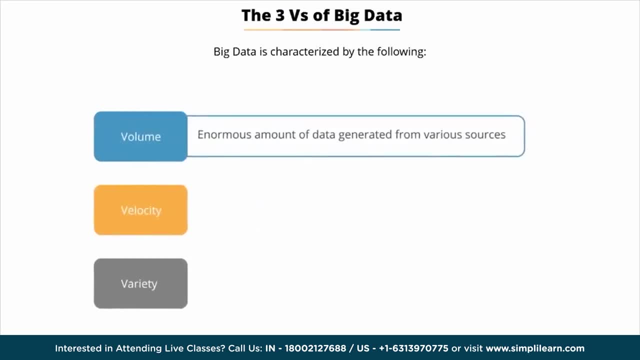 Volume, Velocity and Variety. Volume refers to the enormous amount of data generated from various sources. Big data is also characterized by velocity. Velocity is a tremendous speed from different devices, sensors and applications. To deal with it, an efficient and timely data processing is required. 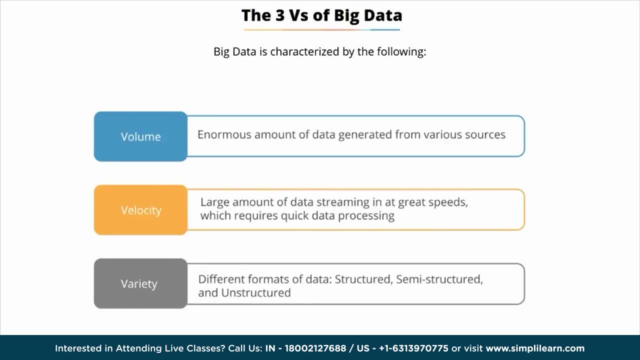 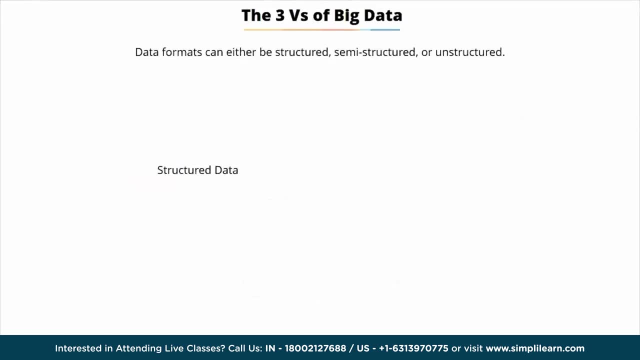 Variety is the third V of big data, because big data can be categorized into different formats like structured, semi-structured and unstructured. Structured data is usually referenced to as RDBMS data, which can be stored and retrieved easily through SQLs. 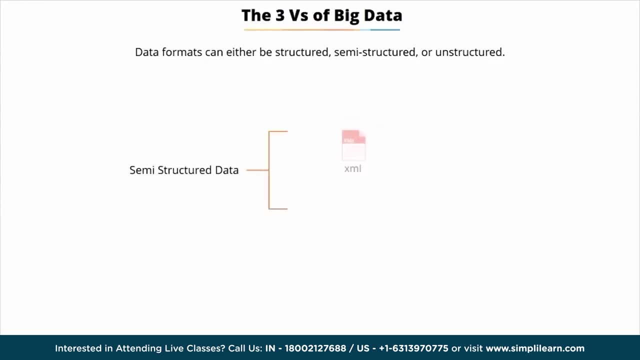 Semi-structured data are usually in the form of files like XML, JSON documents and NoSQL database. Text files, images, videos or multimedia content are examples of unstructured data. In short, big data is a very large information database usually stored on. 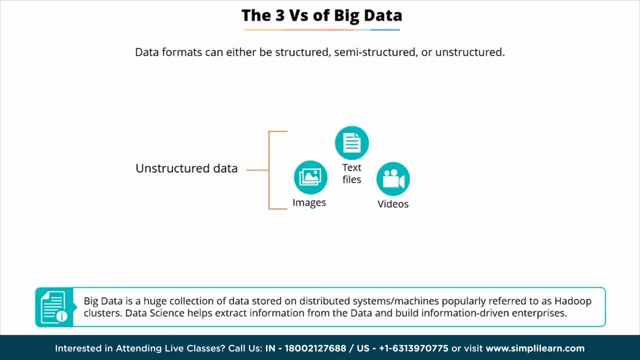 distributed systems or machines, popularly referred to as Hadoop clusters. But to be able to use this database, we have to find a way to extract the right information and data patterns from it. That's where data science comes in. Data science helps to build. 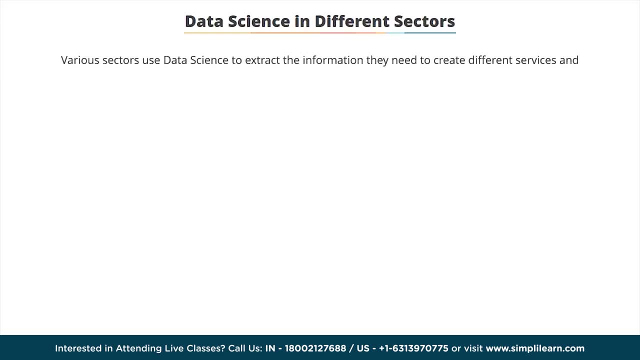 information-driven enterprises. Let's go on to see the applications of data science in different sectors. Social network platforms such as Google, Yahoo, Facebook and so on collect a lot of data every day, which is why they have some of the most advanced data centers. 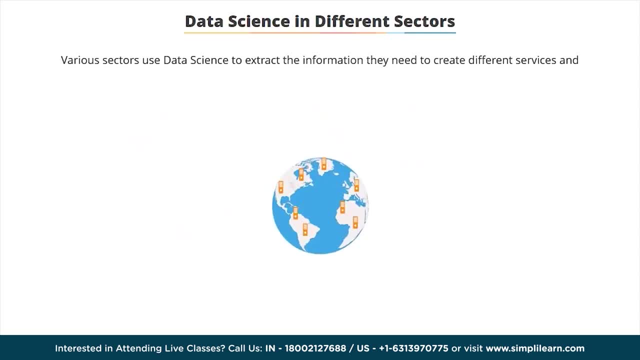 spread across the world. Having data centers all over the world, and not just in the US, help these companies serve their international needs better and faster, without any network latency. They also help them deal effectively with the enormous amount of data. So what do all these different sectors 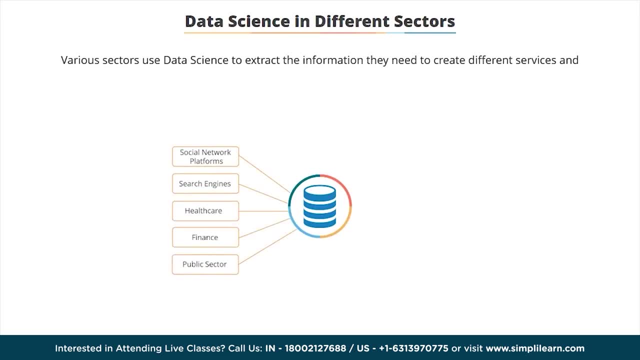 do with all this big data? Their team of data scientists analyze all the raw data with the help of modern algorithms and data models to turn it into information. They then use this information to build digital services, data products and information-driven apps. Now let's see. 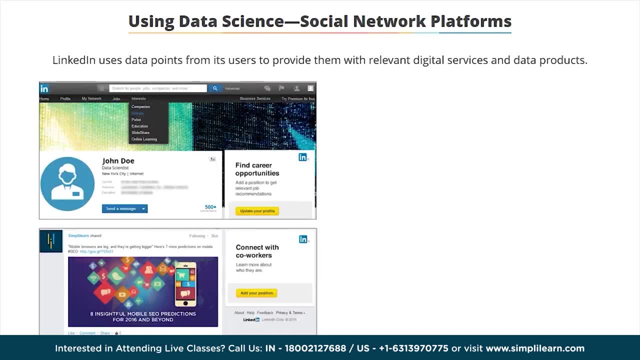 how these products and services work. We'll first look at LinkedIn. Let's suppose that you are a data scientist based in New York City, So it's quite likely that you would want to join a group or build connections with people related to data science. 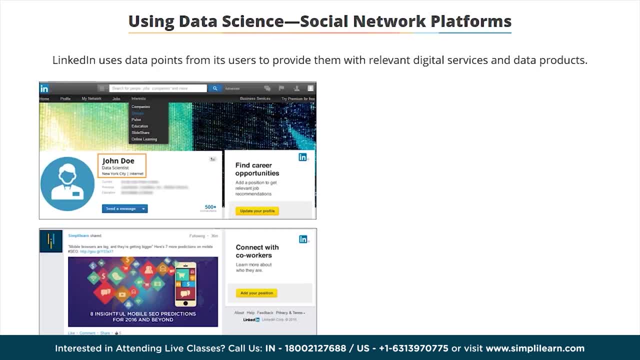 in New York City. Now what LinkedIn does, with the help of data science, is that it looks at your profile, your posts and likes the city you are from, the people you are connected to and the groups you belong to. Then it looks at the information. 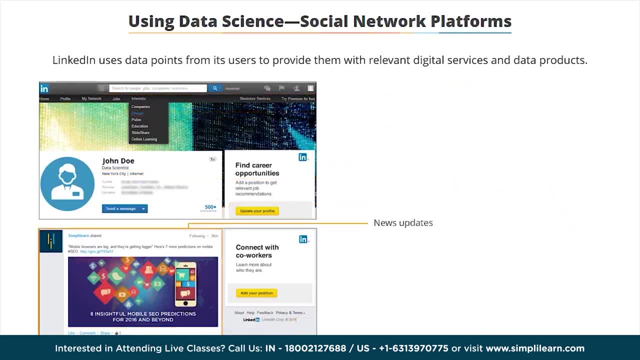 that is most relevant to you. This information could be in the form of news updates that you might be interested in, industry connections or professional groups that you might want to get in touch with, or even job postings related to your field and designation. These are all examples of data services. 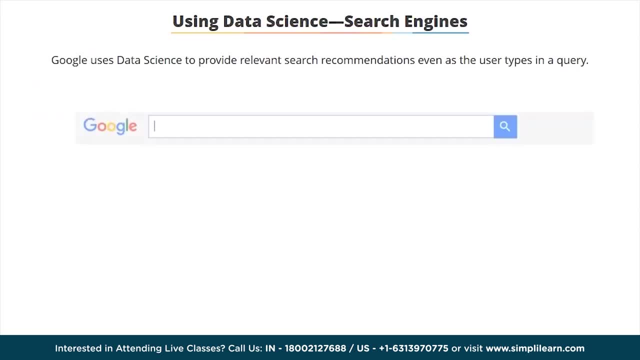 Let's now look at something that we use every day: Google's search engine. Google's search engine has the most unique search algorithm, which allows machine learning models to do a lot of calculations, even as a user types in his or her query. This feature is called AutoComplete. 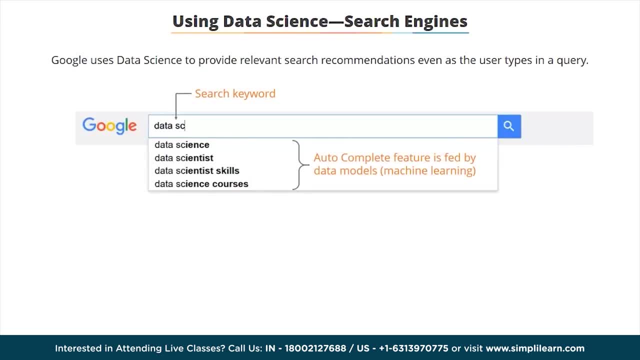 It is an excellent example of how powerful machine learning can be. There are several factors that influence this feature. The first one is query volume. Google's algorithms identify unique and verifiable users that search for any particular keyword on the web. Based on that, it builds a query volume. 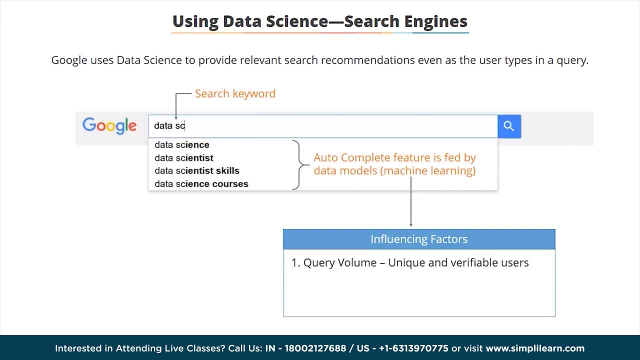 For instance, Republican Debate 2016, Ebola Threat, CDC or the Center of Disease Control, and so on are some of the most common user queries. Another important factor is a geographical location. The algorithms tag a query with the locations from where it is generated. 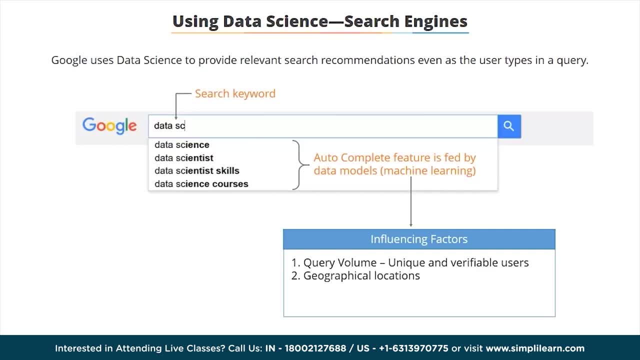 This makes a query volume location specific. It's a very important feature, because this allows Google to provide relevant search recommendations to its user based on his or her location. And then, of course, the algorithms consider the actual keywords and phrases that the user types in. 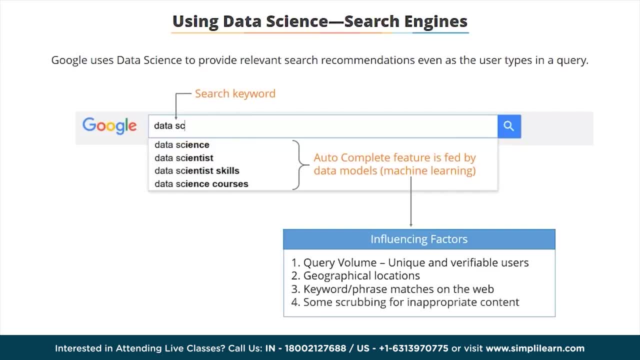 It takes up those words and crawls the web looking for similar instances. The algorithms also try to filter or scrub out inappropriate content, For instance sexual, violent or terrorism-related content. hate speeches and legal cases are scrubbed out from the search recommendations. 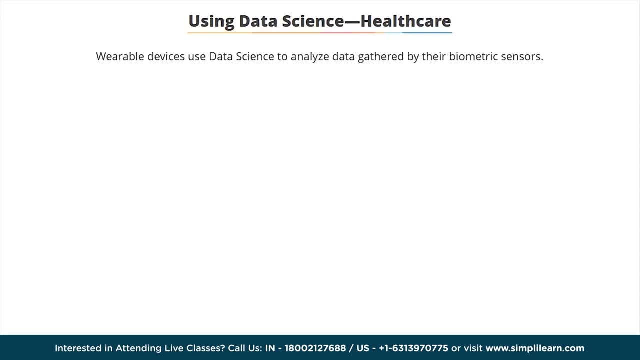 But how does data science help you? Today, even the healthcare industry is beginning to tap into the various applications of data science. To understand this, let's look at wearable devices. These devices have biometric sensors and a built-in processor to gather data from your body. 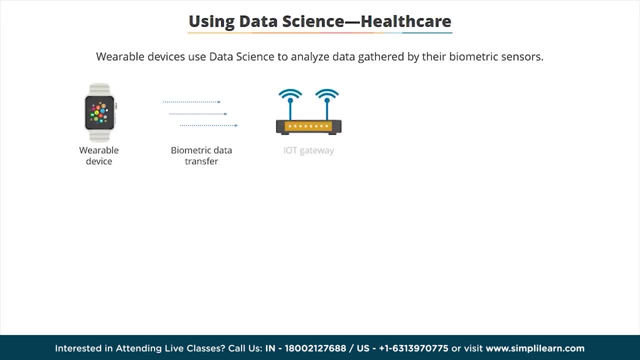 when you are wearing them. They transmit this data to the big data analytics platform via the IoT gateway. Ideally, the platform collects hundreds of thousands of data points and the system for further processing. The big data analytics platform applies data models created by data scientists. 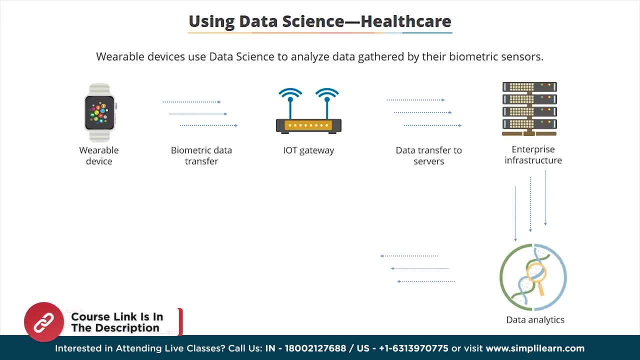 and extracts the information that is relevant to you. It sends the information to the engagement dashboard, where you can see how many steps you walked, what your heart rate is over a period of time, how good your sleep was, how much calories you burned. 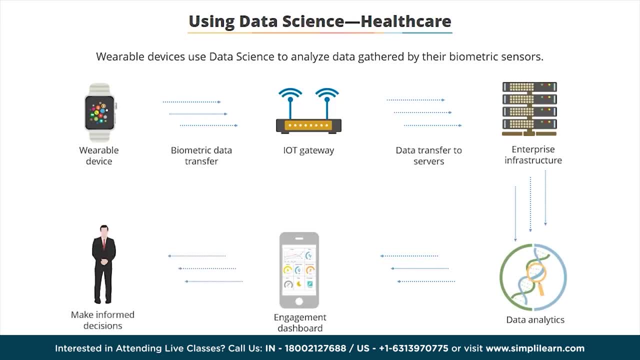 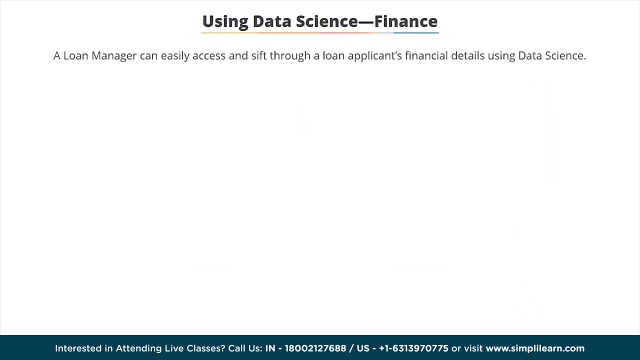 and so on. Knowing such details would help you to set personal goals to cover all healthcare and insurance costs. It would also help your doctor record your vitals and diagnose any issue. The finance sector can easily use data science to help it function more efficiently. 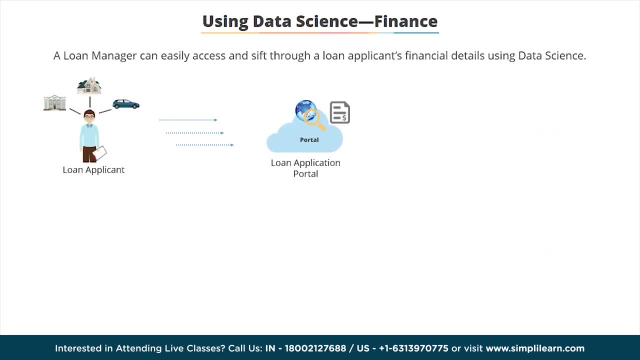 Suppose a person applies for a loan, The loan manager submits the application to the enterprise infrastructure for processing. The analytics platform applies data models and algorithms and creates an engagement dashboard with the loan manager. The dashboard would show the applicant's credit report credit history. 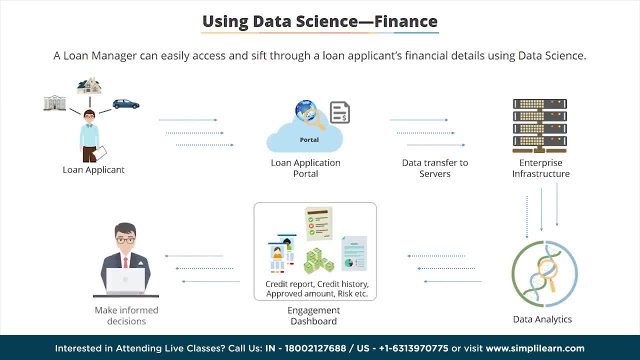 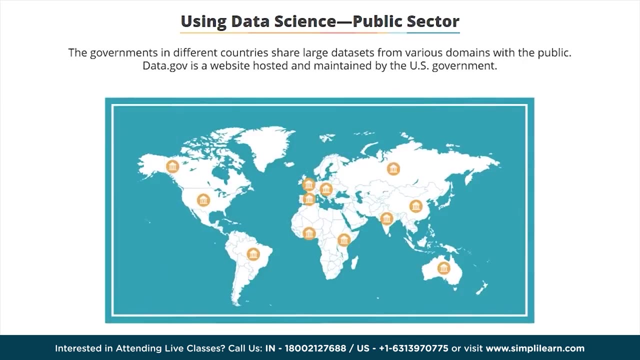 amount, if approved, and risks associated with him or her. The loan manager can now easily take a look at all the relevant information and decide whether the loan can be approved or not. Governments across different countries are gradually sharing large datasets from various domains with the public. 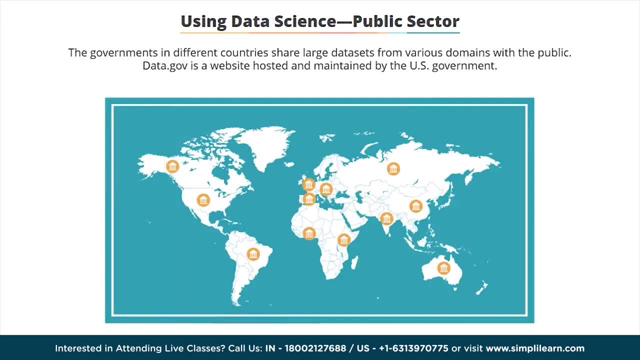 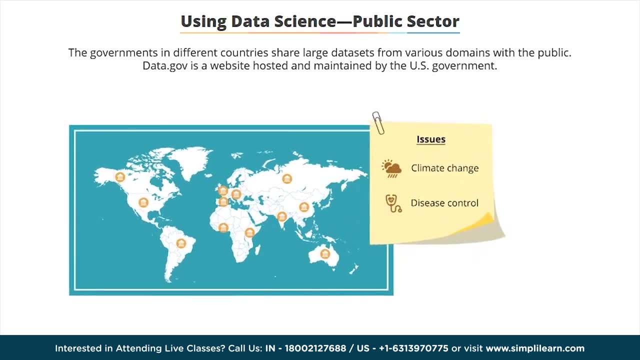 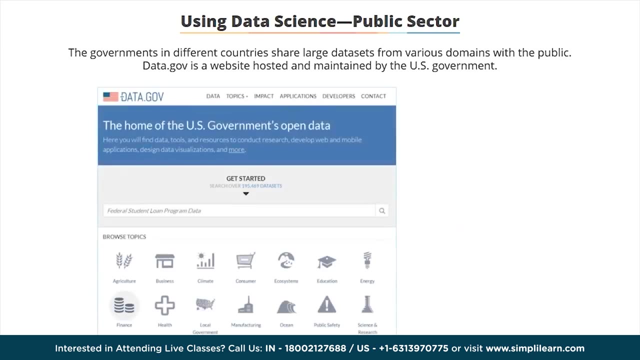 This kind of transparency makes governments seem more trustworthy. It provides the country data that can be used to prepare itself for different types of issues like climate change and disease control. It also helps encourage people to create their own digital products and services. The US government. 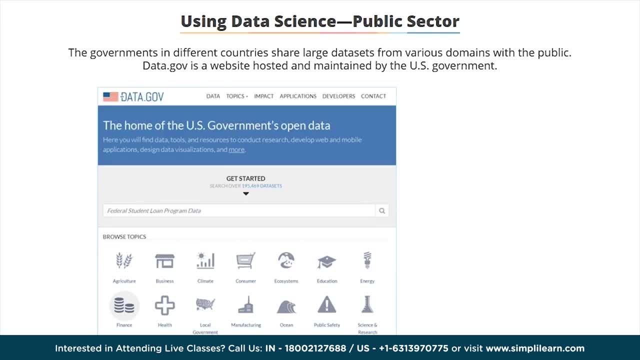 hosts and maintains Datagov, a website that offers information about the federal government. It provides access to over 195,000 datasets across different sectors. The US government has kicked off several strategic initiatives in the field of data science. that includes US Digital Service. 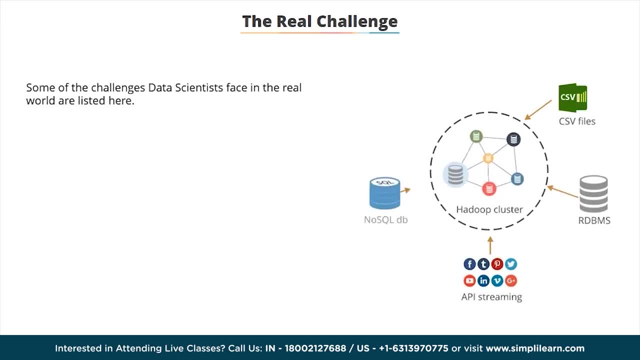 and Open Data, We have seen how data science can be applied across different sectors. Let's now take a look at the various challenges that a data scientist faces in the real world while dealing with datasets. Data quality- The quality of data is mostly not up to the set standards. 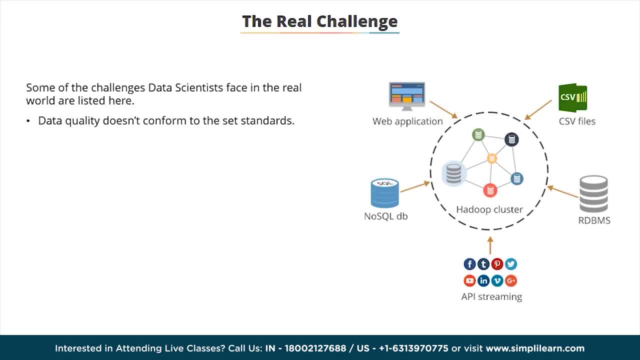 You will usually come across data that is inconsistent, inaccurate and with anomalies. Integration- Data integration with several enterprise applications and systems is a complex and painstaking task. Unified platform Data is distributed to Hadoop, Distributed File System or HDFS, from various sources to ingest. 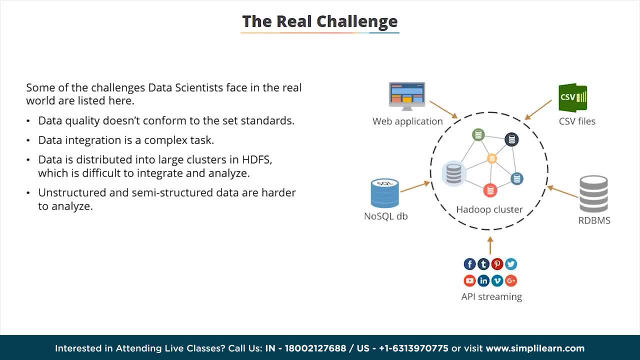 process, analyze and visualize huge datasets. The size of these Hadoop clusters can vary from few nodes to thousand nodes. The challenge is to perform analytics on these large datasets efficiently and effectively. This is where Python comes into play with its powerful set of libraries. 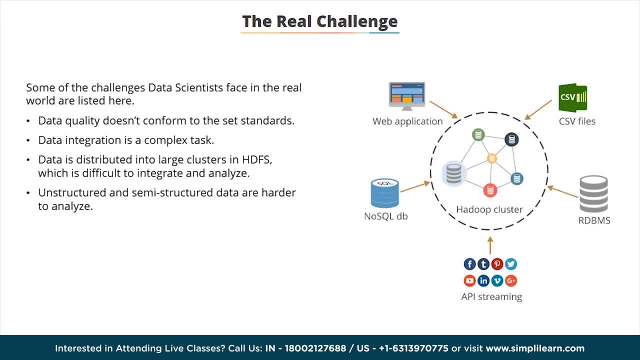 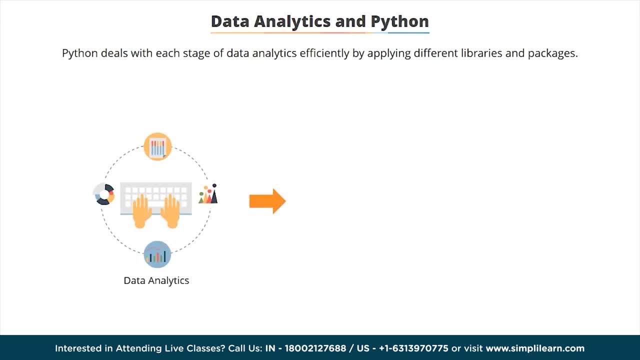 functions, modules, packages and extensions. Python can efficiently tackle each stage of data analytics. that includes data acquisition. Python libraries such as Scrappy comes handy here. Data wrangling- Python data frames are very efficient in handling large datasets and makes data wrangling easier. 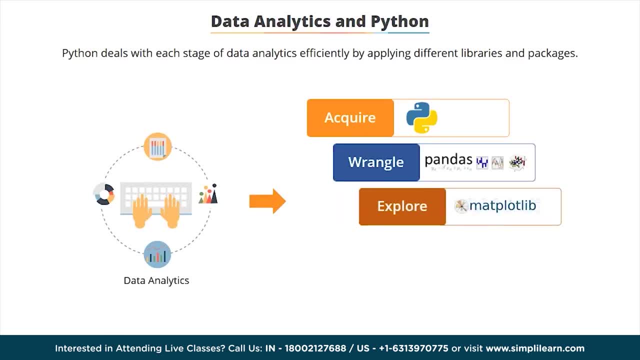 with its powerful functions Explore. Matplotlib libraries are very rich when it comes to data exploration. Model Scikit learns statistical and mathematical functions to help to build models for machine learning Visualization. Modern libraries such as Voka creates very intuitive and interactive. 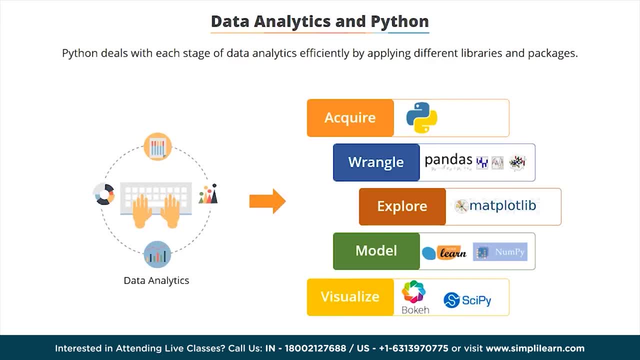 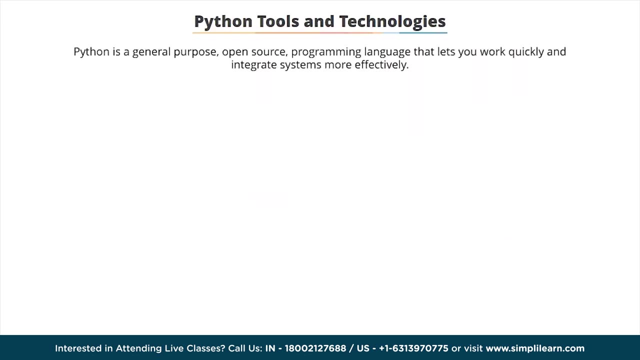 visualization. Its huge set of libraries and functions make big data analytics seem easy to use. Python applications and programs are portable and helps them scale out on any big data platform. Python is an open source programming language that lets you work quickly and integrate systems more effectively. 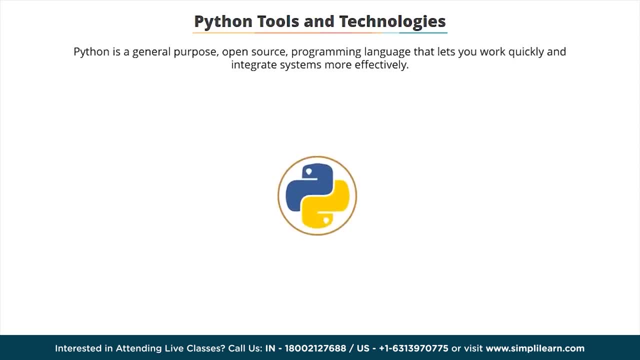 Now that we have talked about how the Python libraries help the different stages of data analytics, let's take a closer look at these libraries and how they support different aspects of data science. Numerical Python is the fundamental package for scientific computing. SciPy is the core of scientific 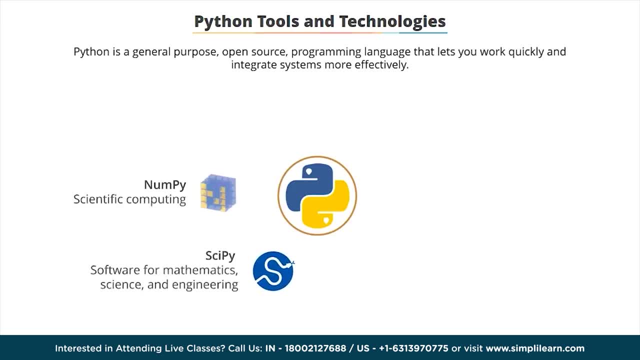 computing libraries and provides many user friendly and efficiently designed numerical routines. Matplotlib is a Python 2D plotting library which produces publication quality figures in a variety of hard copy formats and interactive environments across platforms. Scikit Learn is built on NumPy, SciPy and Matplotlib. 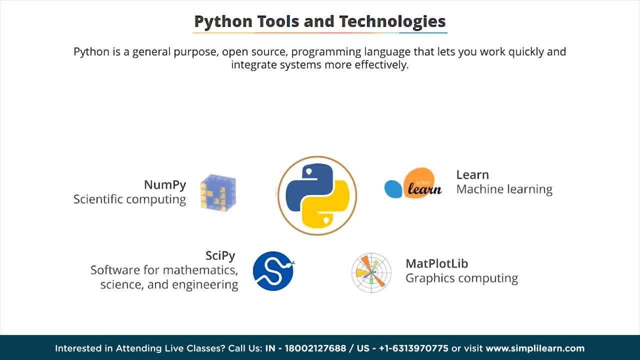 for data mining and data analysis. Pandas is a library providing high performance, easy to use data structures and data analysis tools for Python. All these libraries, modules and packages are open source and hence using them is convenient and easy. There are numerous factors which positions Python well. 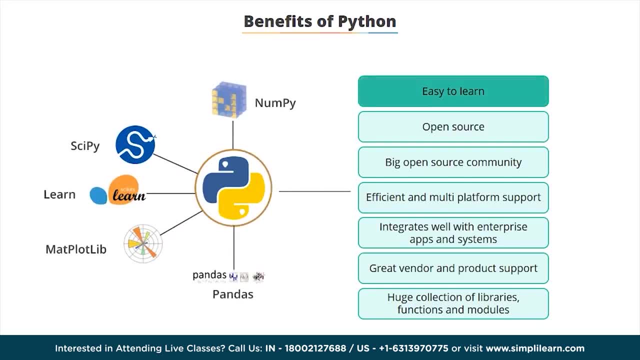 and makes it the tool for data science. Python is easy to learn. It's a general purpose function and object oriented programming language. As Python is an open source programming language, it is readily available, easy to install and get started. It also has a large presence of 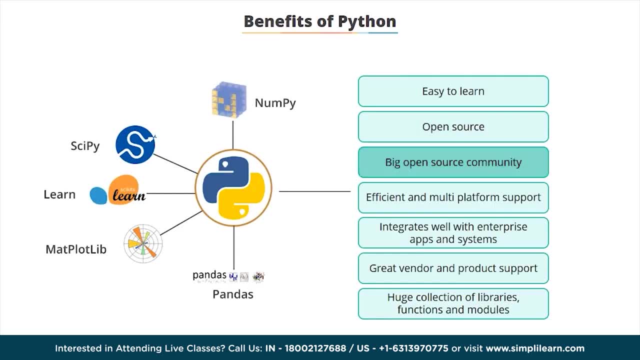 open source community for software development and support. Python and its tools enjoy multi-platform support. Applications developed with PyCon integrate easily with other enterprise systems and applications. There are a lot of tools, platforms and products in the market from different vendors, as they often 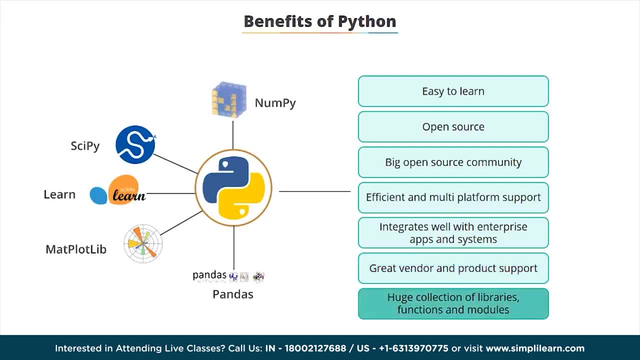 offer great support and services. Python and its libraries create unique combinations for data science. Because of all these benefits, it's usually popular among academicians, mathematicians, statisticians and technologists. Python is supported by well established data platforms and processing frameworks. 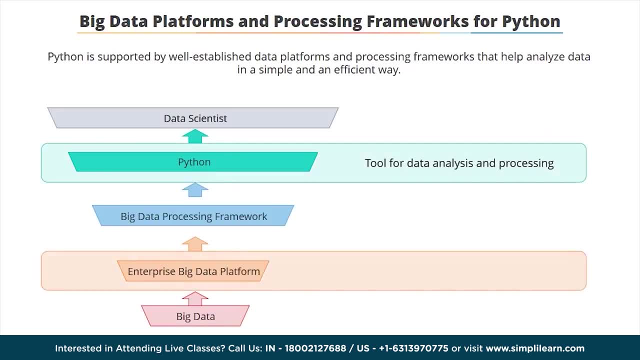 that help it analyze data in a simple and efficient way. Enterprise Big Data Platform. Cloudera is the pioneer in providing enterprise ready Hadoop Big Data Platform and supports Python. Hortonworks is another Hadoop Big Data Platform provider and supports Python. MapReduce. MapR is 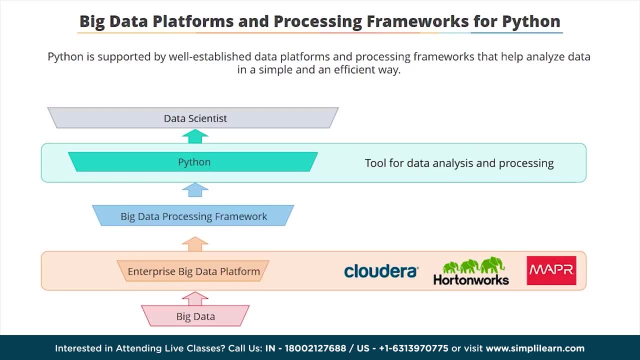 also committed to Python and provides the Hadoop Big Data Platform, Big Data Processing Framework, MapReduce, Spark and Flink. provides very robust and unique data processing framework and support Python Scala. Scala and Python languages are used for Big Data Processing Framework But to access Big Data. 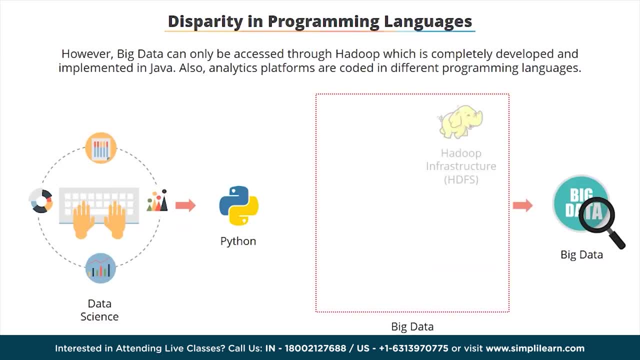 you have to use a Big Data Platform, which is a combination of the Hadoop infrastructure, also known as Hadoop, Distributed File System or HDFS, and an analytics platform. Hadoop is a framework that allows data to be distributed across clusters of computers for faster, cheaper and 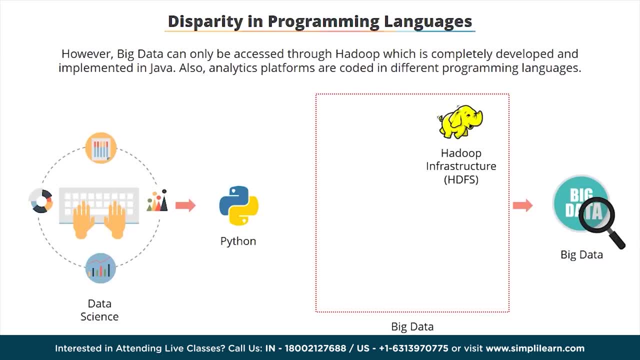 efficient computing. It's completely developed and coded in Scala. One of the most popular analytics platforms is Spark. It easily integrates with HDFS. It can also be implemented as a standalone analytics platform and integrated with multiple data sources. It helps data scientists perform their work. 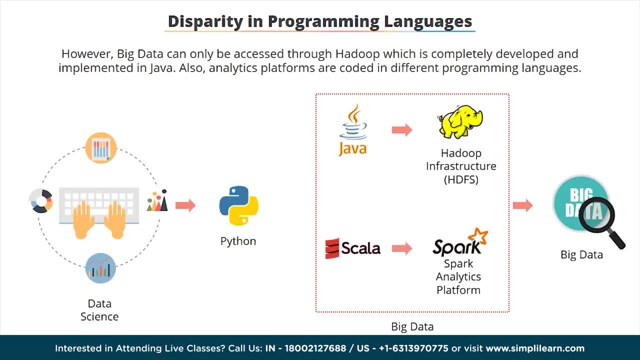 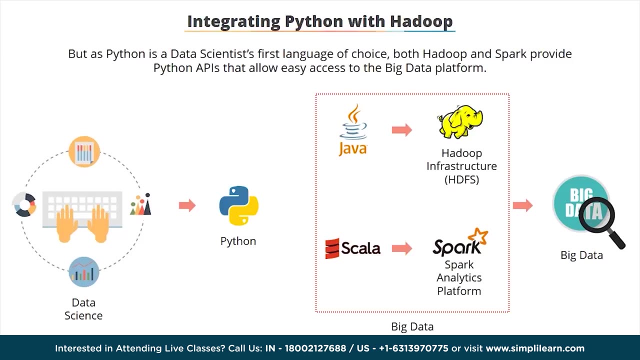 more efficiently. Spark is built using Scala, Since there is a disparity in the programming language that data scientists use and that of the Big Data Platform. it impedes data access and flow, As Python is a data scientist's first language of choice. both Hadoop and Spark provide 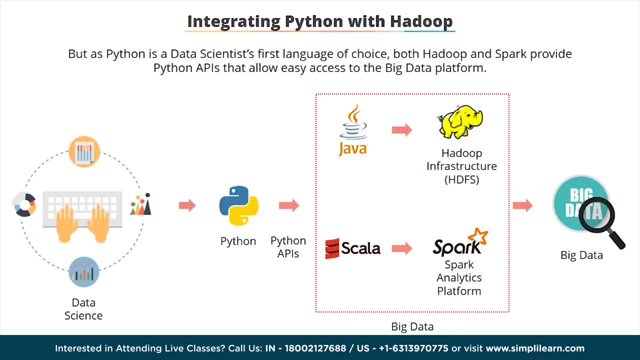 Python APIs that allow easy access to the Big Data Platform. Consequently, a data scientist need not learn Java or Scala or any other platform-specific data languages, and can instead focus on performing data analytics. There are several motivations for Python Big Data Solutions. Big Data is a 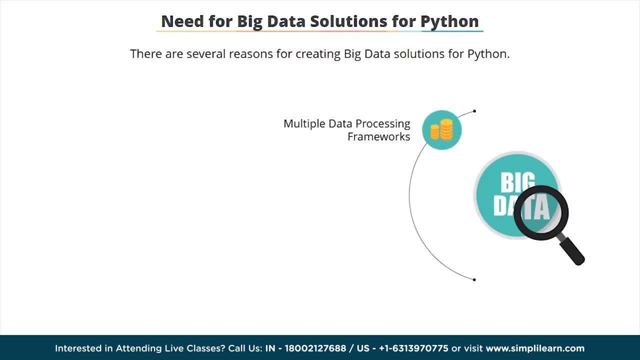 continuously evolving field, which involves adding new data processing frameworks that can be developed using any programming language. Moreover, new innovation and research is driving the growth of Big Data Solutions and platform providers. It would be difficult for data scientists to focus on analytics if they have to constantly. 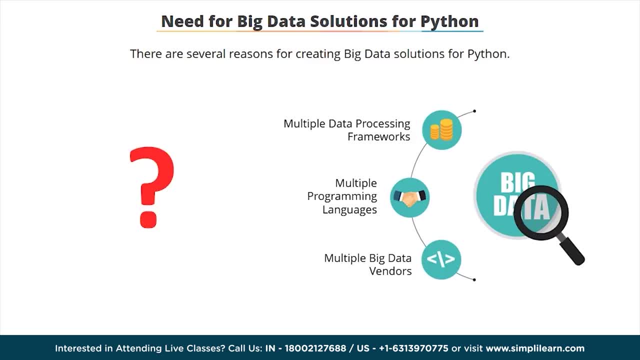 upgrade themselves on information or, under the hood, architecture or implementation of the platform. Therefore, it's important to keep the entire data science platform and any language agnostic, to simplify a data scientist's job. Consequently, almost all major vendors, solution providers and data processing 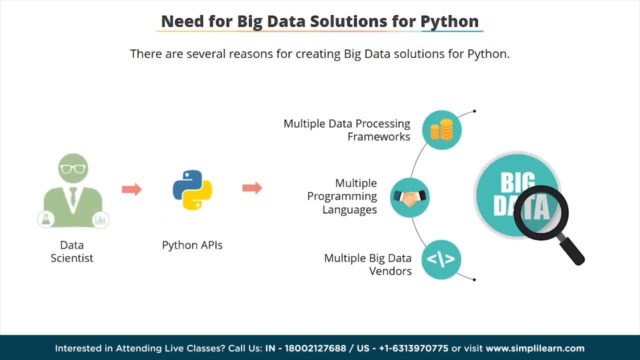 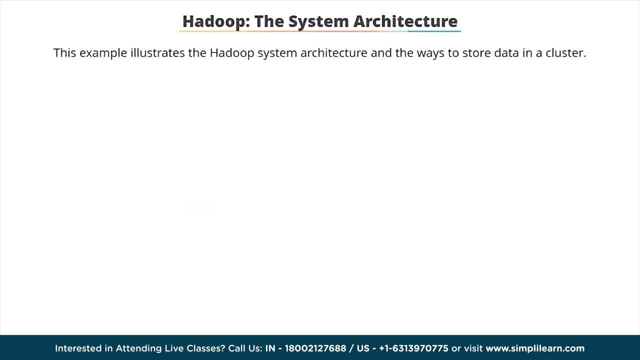 framework developers are providing Python APIs. This allows a data scientist to perform Big Data analytics using only Python, rather than learning other languages like Java or Scala to help them work on the Big Data Platform, Let's look at an example and understand how data is stored across Hadoop's distributed clusters. 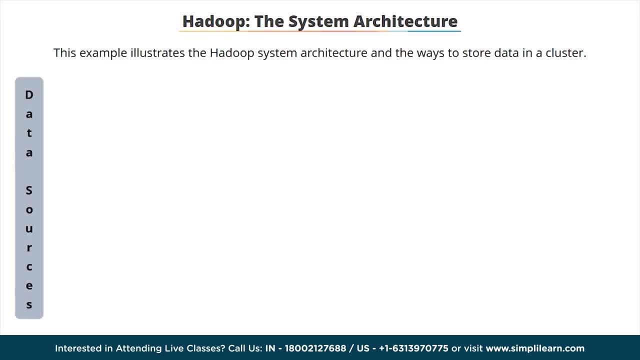 Big Data is generated from different data sources. A large file, usually greater than 100 megabytes, gets routed from a name node to data nodes. Name nodes hold the metadata information about the files stored on data nodes. It stores the address and information of a block of file. 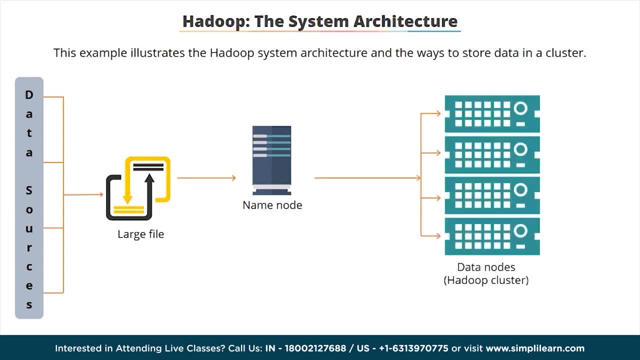 and the data node associated with it. Data nodes hold the actual data blocks. The file is split into multiple smaller files, usually of 24 megabytes or 128 megabyte size. It's then copied to multiple physical servers. The smaller files are also called. 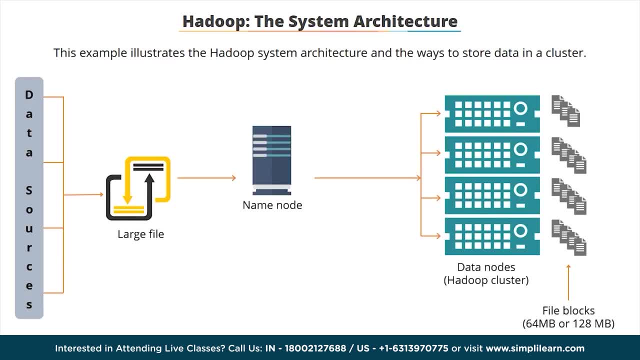 file blocks. One file block gets replicated to different servers. The default replication factor is 3,, which means a single file block gets copied at least three times on different servers or data nodes. There is also a secondary name node which keeps a backup of all the 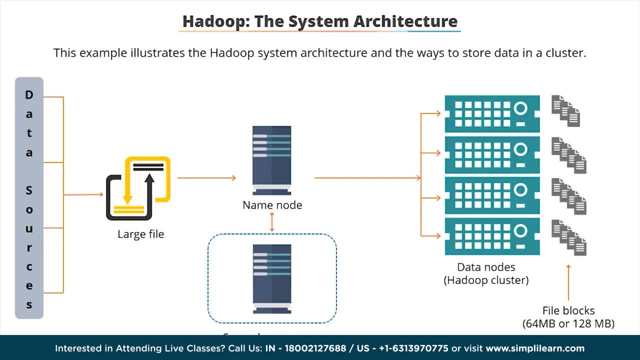 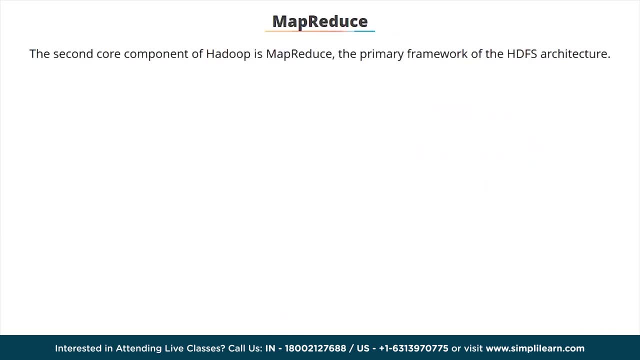 metadata information stored on the main or primary node If and when the main name node fails. Now that you have understood a little about HDFS, let's look at the second core component of Hadoop MapReduce, the primary framework of the HDFS architecture. 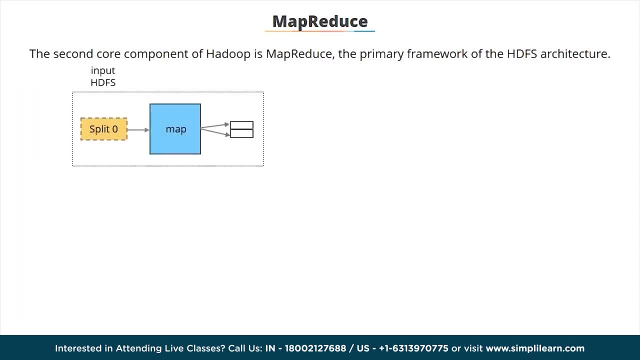 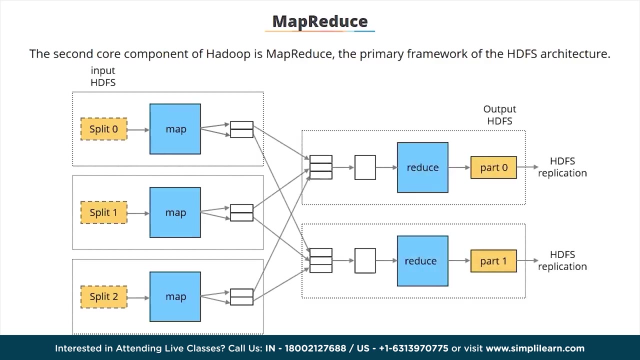 A file is split into three blocks as split0,, split1, and split2.. When a request comes in to retrieve the information, the map or task is executed on each data node that contains the file blocks. The mapper generates an output, essentially in the form of key value. 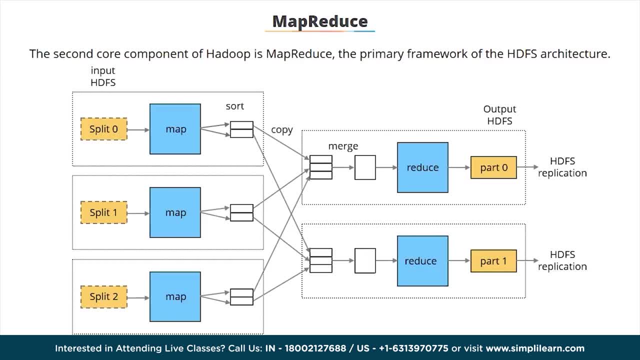 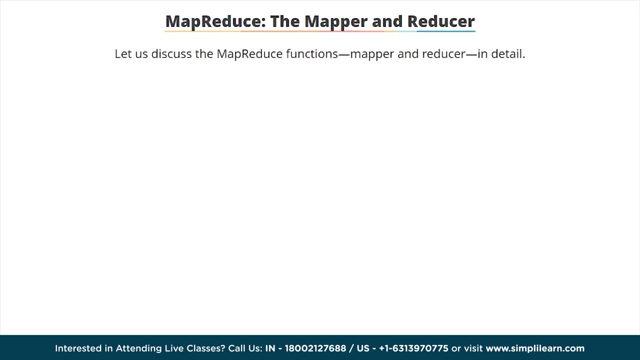 pairs that are sorted, copied and merged. Once the mapper task is complete, the reducer works on the data and stores the output on HDFS. This completes the MapReduce process. Let's discuss the MapReduce functions- mapper and reducer- in detail. 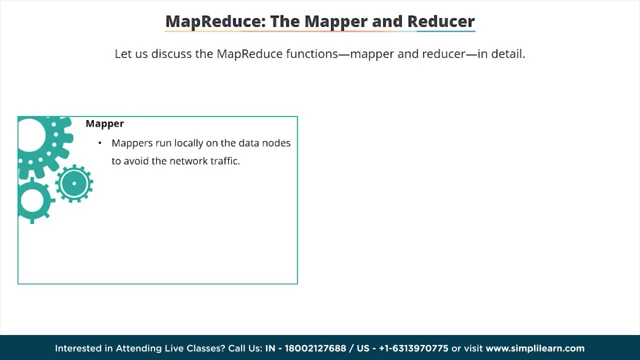 The Mapper Hadoop ensures that mappers run locally on the nodes which hold a particular portion of the data, to avoid the network traffic. Multiple mappers run in parallel and each mapper processes a portion of the input data: The input and output of the mapper. 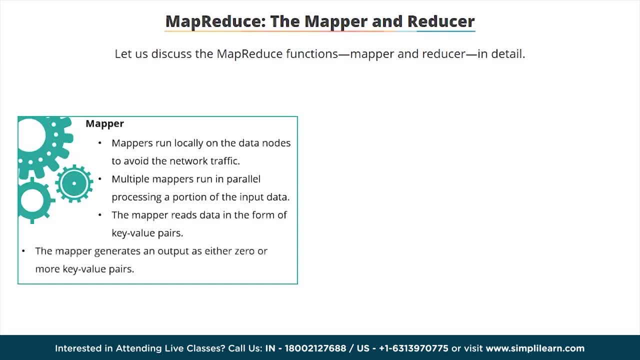 are in the form of key value pairs. Note that it can either provide zero or more key value pairs as output. The Reducer. After the map phase, all intermediate values for an intermediate key are combined into a list which is given to a reducer. 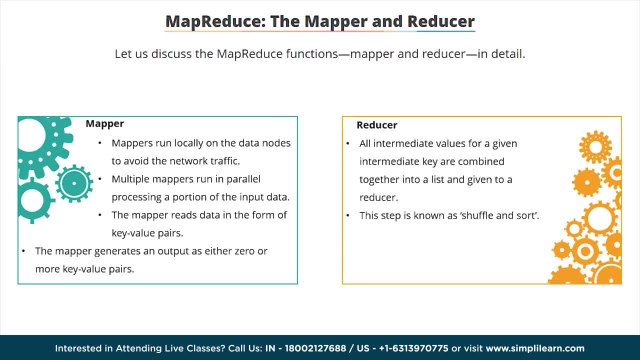 All values associated with a particular intermediate key are directed to the same reducer. This step is known as shuffle and sort. There may be a single reducer or multiple reducers. Note that the reducer also provides outputs in the form of zero or more than one final key value pairs. 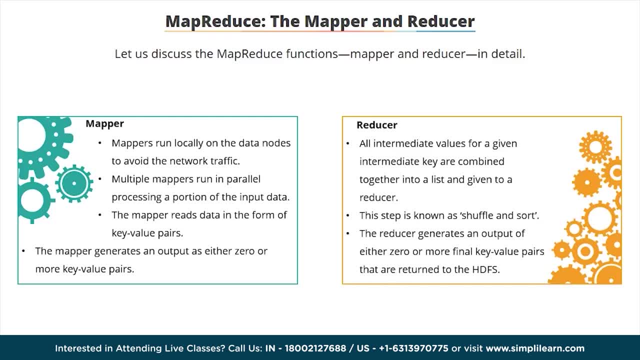 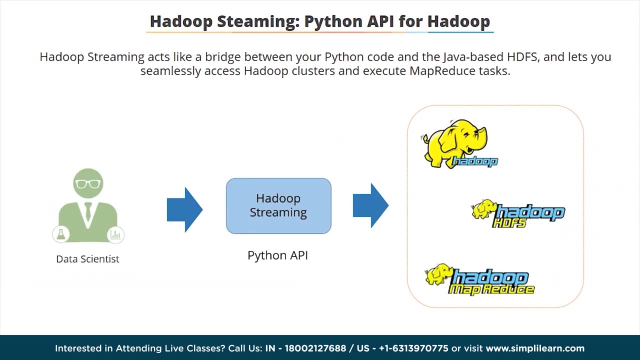 These values are then returned to HDFS. The reducer usually emits a single key value pair for each input key. You have seen how mapper reduces critical for HDFS to function. A good thing is you don't have to learn Java or other Hadoop-centric 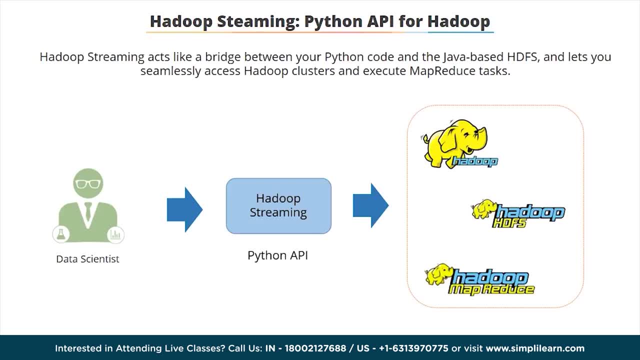 languages to write a mapper reduce program. You can easily run such Hadoop jobs with a code completely written in Python with the help of Hadoop Streaming API. Hadoop Streaming acts like a bridge between your Python code and the Java-based HDFS, and lets you seamlessly access. 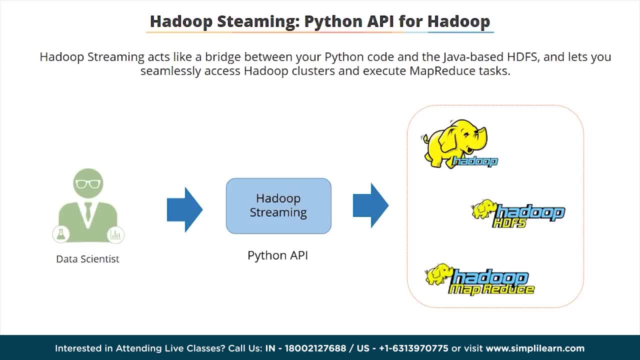 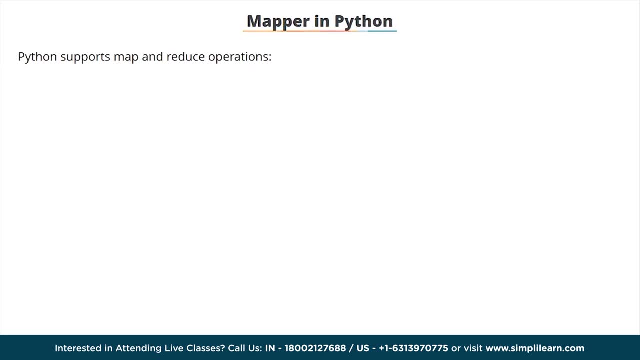 Hadoop clusters and execute mapper reduce tasks. You have seen how mapper reduce is critical for HDFS to function. Thankfully, you don't have to learn Java or other Hadoop-centric languages to write a mapper reduce program. You can easily run such Hadoop. 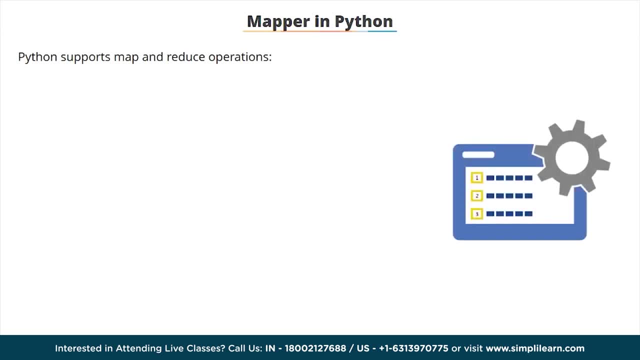 jobs with a code completely written in Python Shown. here are some user-friendly Python functions that are written for the mapper class. Suppose we have the list of numbers we want to square, We have the square function defined as shown on the screen. We can call the map function. 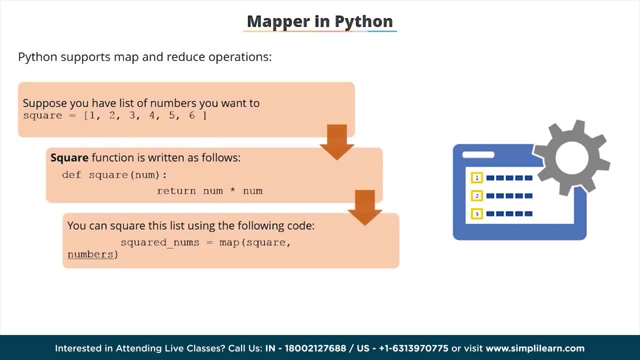 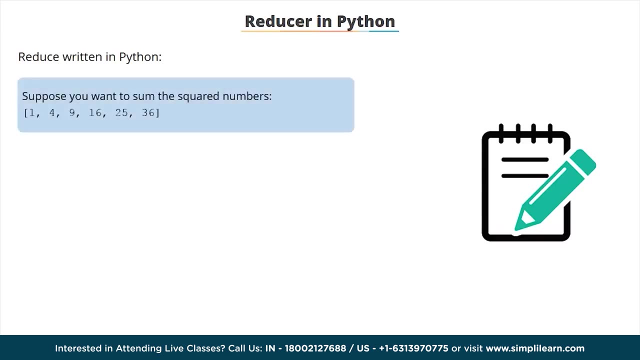 with the list and the function which is to be executed on each item in that list. The output of this process is as shown on the screen. Reducer can also be written in Python. Here we would like to sum the squared numbers of the previous. 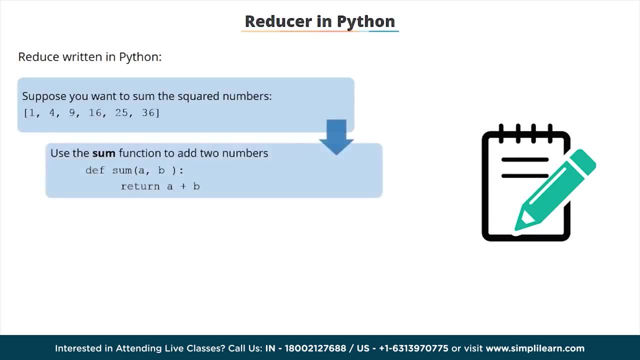 map operation. This can be done using the sum operation, as shown on the screen. We can now call the reduce function with the list of data which is to be aggregated, and aggregator function. in our case, sum, is used for this purpose. Big data analysis requires. 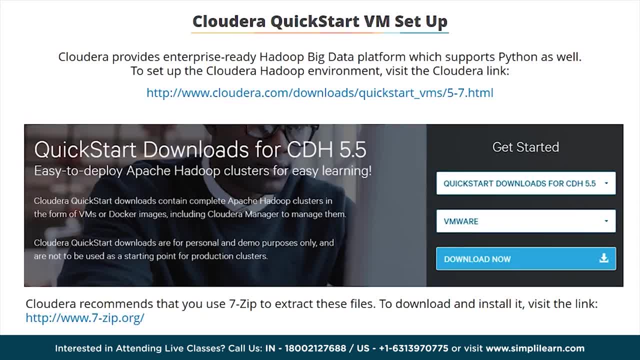 a large infrastructure. Cloudera provides enterprise-ready Hadoop big data platform which supports Python as well. To execute Hadoop jobs, you have to first install Cloudera. It's preferable to install Cloudera's virtual machine on a Unix system, as it functions. 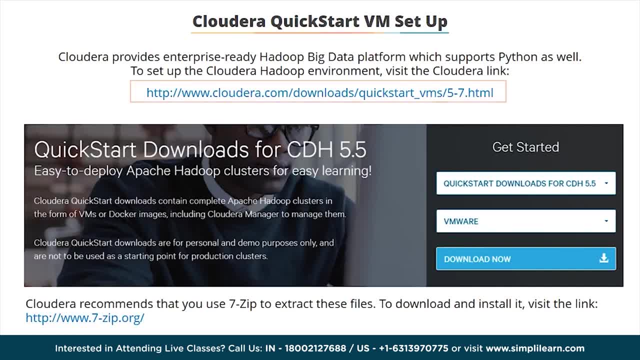 better than any other system To set up the Cloudera Hadoop environment. visit the Cloudera link shown here. Select Quick Start Download for CDH 5.5 and VMware from the drop-down lists. Click the Download Now button. 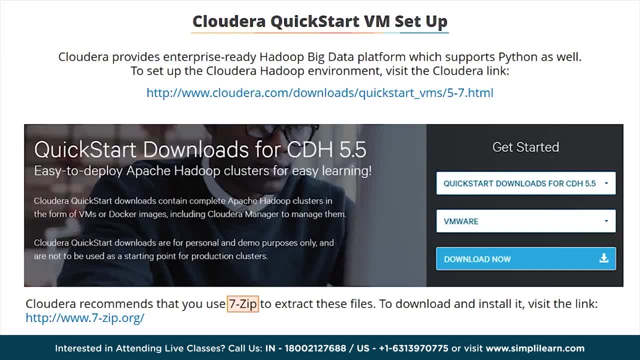 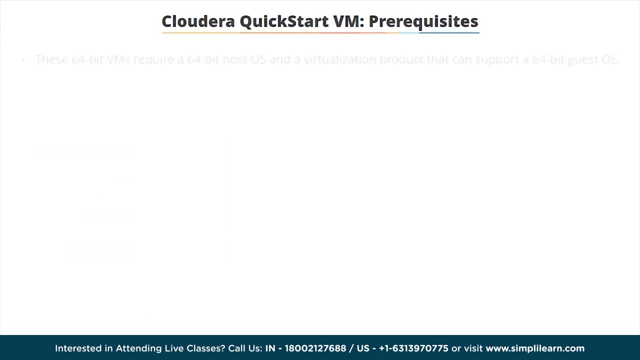 Once the VM image is downloaded, please use 7-Zip to extract the files To download and install it. visit the link shown on screen. Cloudera VMware has some system prerequisites. The 64-bit virtual machine requires a 64-bit host operating system. 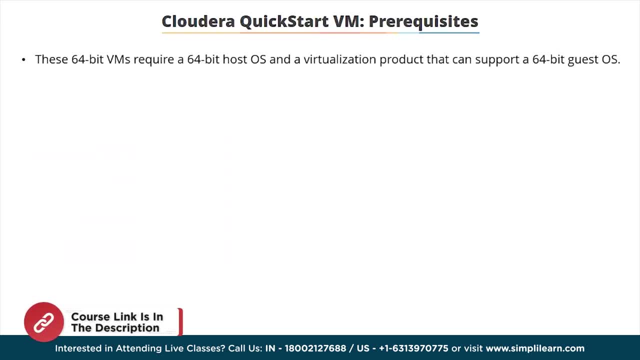 or OS and a virtualization product that can support a 64-bit guest OS. To use a VMware VM, you must use a player compatible with Workstation 8.x or higher, such as Player 4.x or higher or Fusion 4.x. 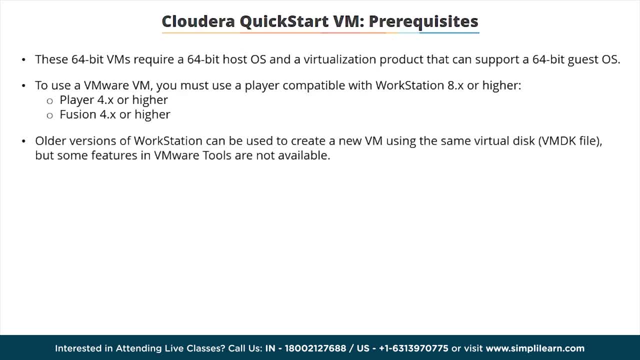 or higher. You can use older versions of Workstation to create a new VM using the same virtual disk or VMDK file, but some features in VMware tools will be unavailable. The amount of RAM required will vary depending on the runtime option you choose. 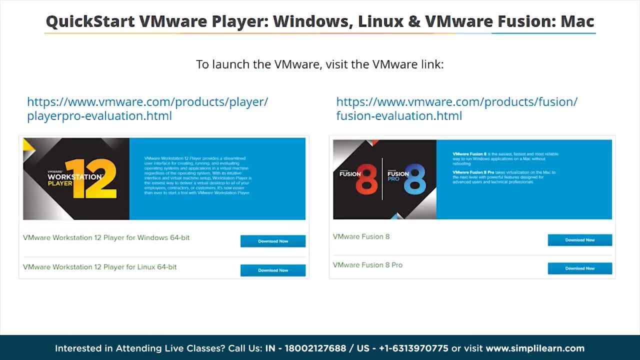 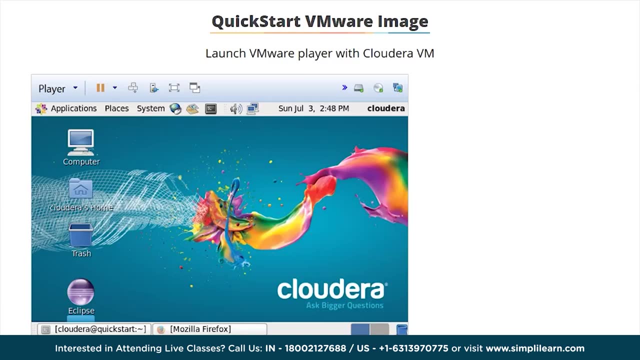 To launch the VMware Player, you will either need VMware Player for Windows and Linux or VMware Fusion for Mac, So please visit the VMware link shown on screen to download the relevant VMware Player. Now launch the VMware Player with the Cloudera VM. 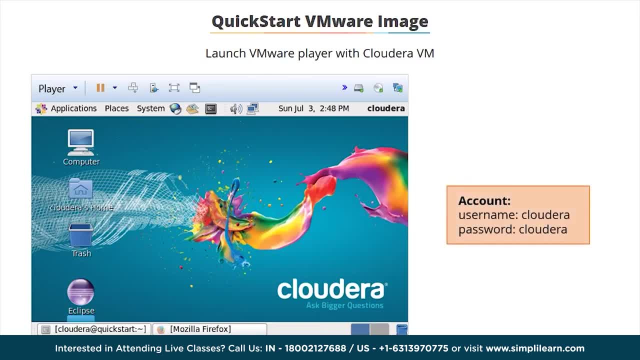 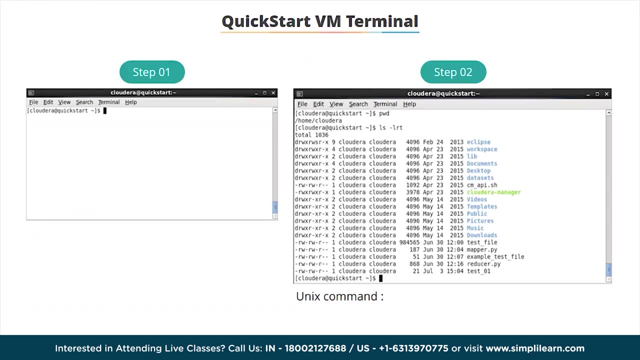 The default username and password is Cloudera. Click the terminal icon as shown here. It will launch the UNIX terminal for Hadoop HDFS interaction. To verify that the UNIX terminal is functioning correctly, type in pwd, which will show you the present working directory. You can also 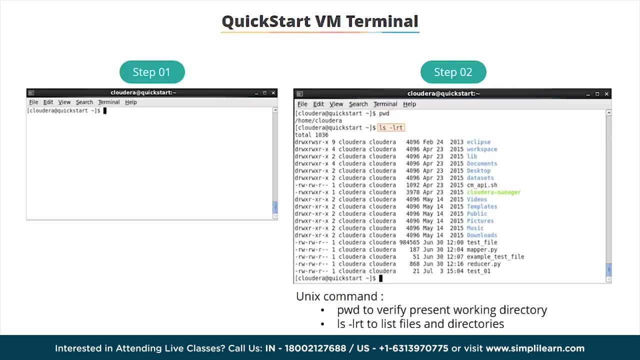 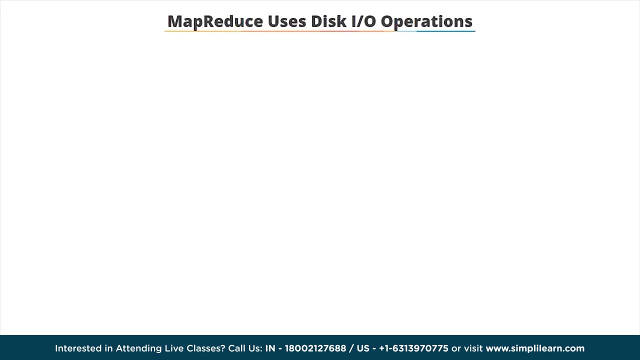 type in ls-lrt to list all the current files, folders and directories. These are some simple UNIX commands which will come in handy later while you are implementing MapReduce tasks. You have seen how the Hadoop distributed file system works along with MapReduce. 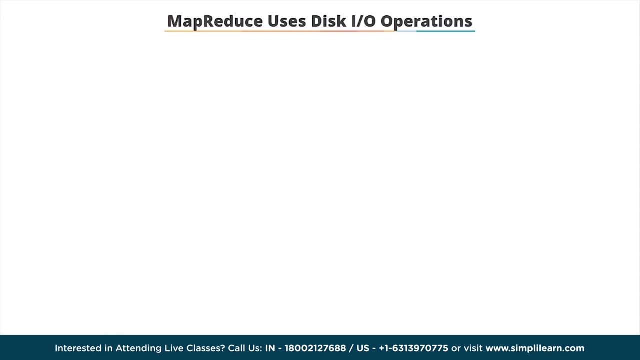 The data is written on and read by disks. MapReduce jobs require a lot of disk read and write operations, which is also known as DiskIO or Input and Output. Reading and writing to a disk is not just expensive, it can also be. 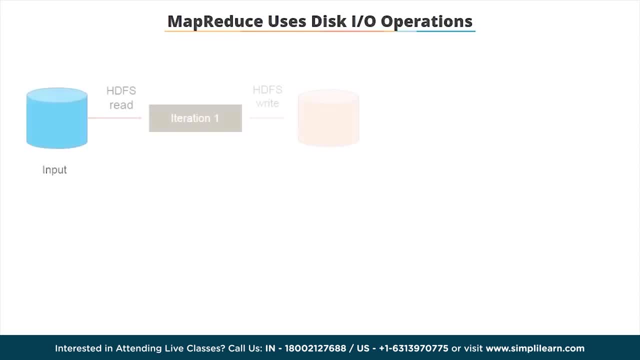 slow and impact the entire process and operation. This is specifically true for iterative processes. Hadoop is built for write-once-read-many type of jobs, which means it's best suited for jobs that don't have to be updated or accessed frequently, But in several cases, 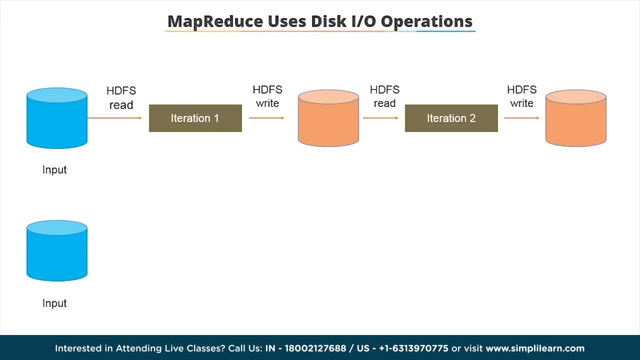 particularly in analytics and machine learning. users need to write and rewrite commands to access and compute on the same data more than once. Every time such a request is sent out, MapReduce requires that data is read and or written onto disks directly. Note that, though the time to access 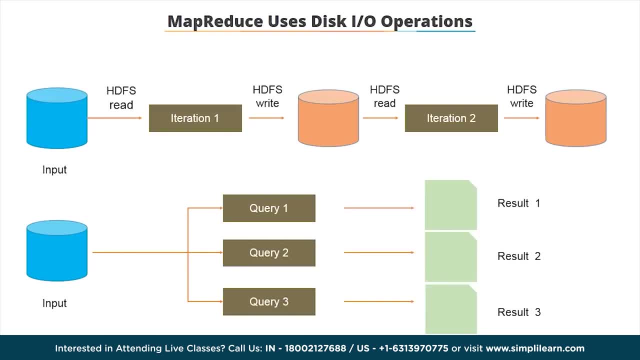 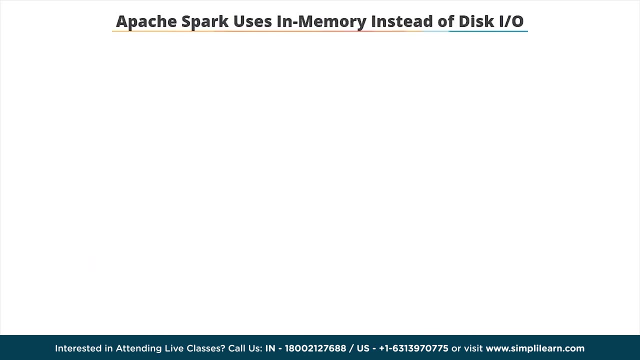 or write on disks is measured in milliseconds. when you are dealing with large file sizes, the time factor gets compounded significantly. This makes the process highly time-consuming. In contrast, Apache Spark uses resilient distributed data sets, or RDDs, to carry out such computations. 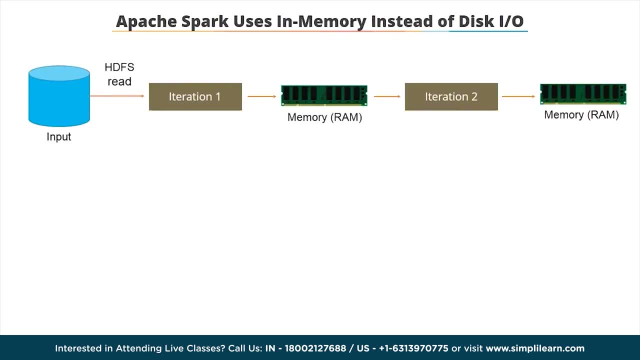 RDDs allow data to be stored in memory, which means that every time users want to access the same data, a disk IO operation is not required. They can easily access data stored in the cache. Accessing the cache or RAM is much faster. 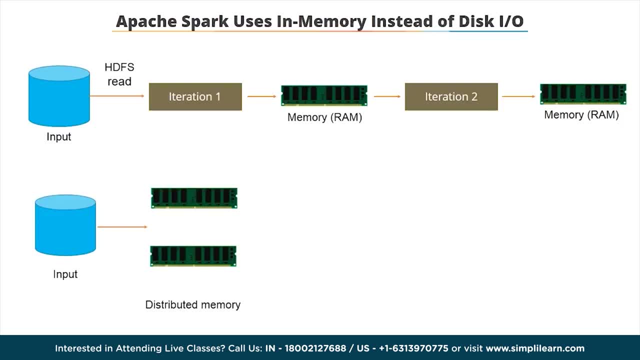 than accessing disks. For instance, if disk access is measured in milliseconds, in-memory data access is measured in sub-milliseconds. This radically reduces the overall time taken for iterative operations on large data sets. In fact, programs on Spark run at least 10 to 100 times faster. 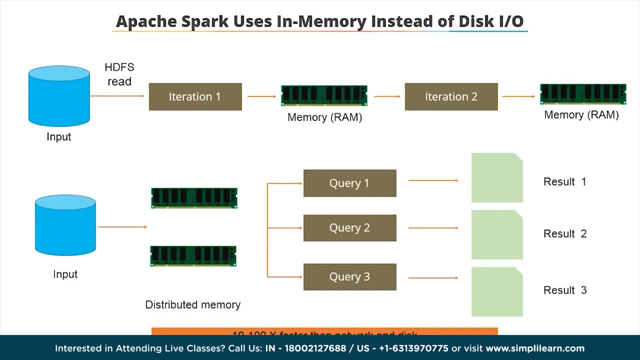 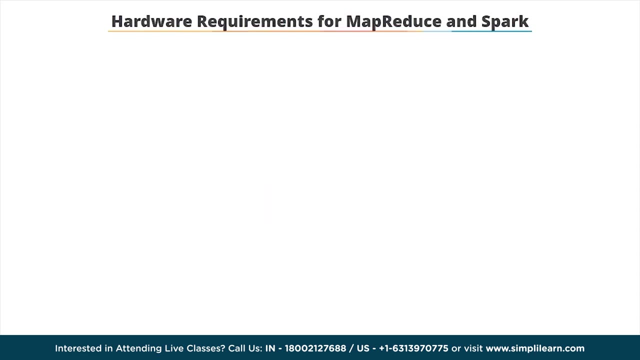 than on MapReduce. That's why Spark is gaining popularity among most data scientists, as it is more time efficient when it comes to running analytics and machine learning computations. One of the main differences in terms of hardware requirements for MapReduce and Spark is that, while 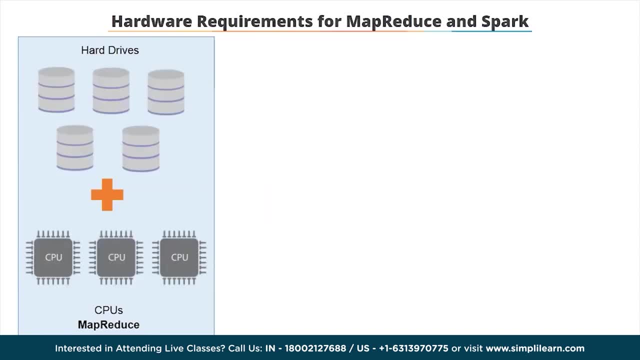 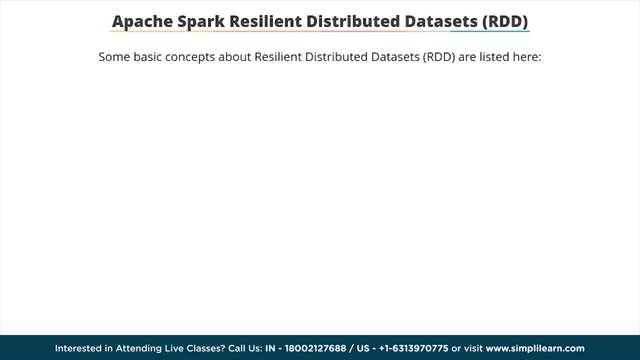 MapReduce requires a lot of servers and CPUs. Spark additionally requires a large and efficient RAM. Let's understand resilient distributed data sets in detail. As you have already seen, the main programming approach of Spark is RDD. RDDs are fault-tolerant collections. 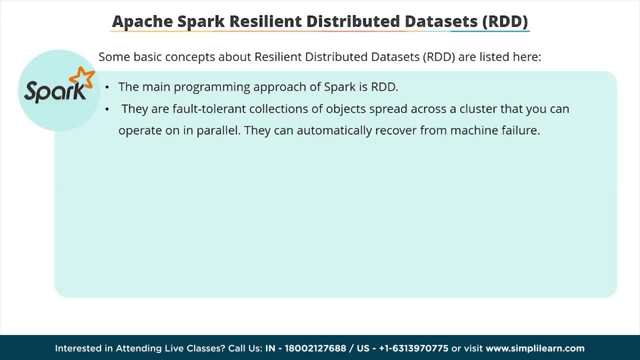 of objects spread across a cluster that you can operate on in parallel. They are called fault-tolerant because they can automatically recover from machine failure. You can create an RDD either by copying the elements from an existing collection or by referencing a data set stored externally. 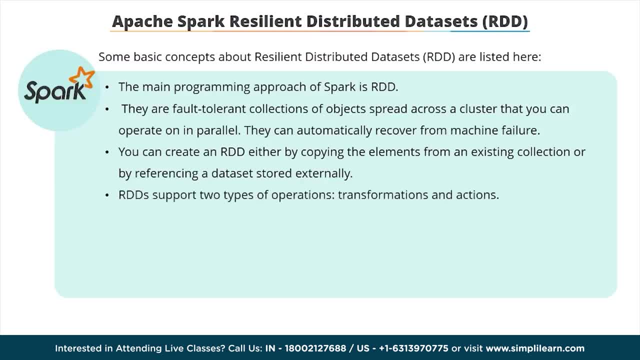 say on an HDFS. RDDs support two types of operations: transformations and actions. Transformations use an existing data set to create a new one. For example, Map creates a new RDD containing the results after passing the elements of the original data set through a function. 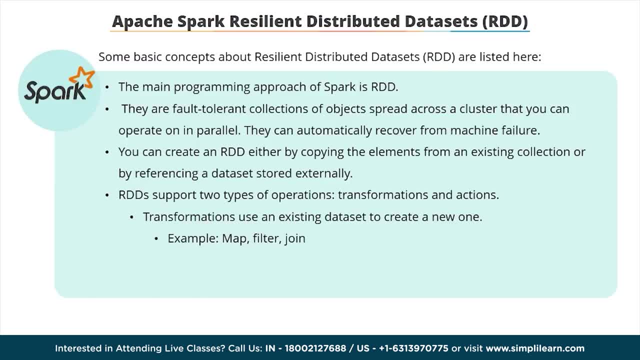 Some other examples of transformations are: Filter and Join Actions, compute on the data set and return the value to the driver program. For example, Reduce aggregates all the RDD elements using a specified function and returns this value to the driver program. Some other examples of actions: 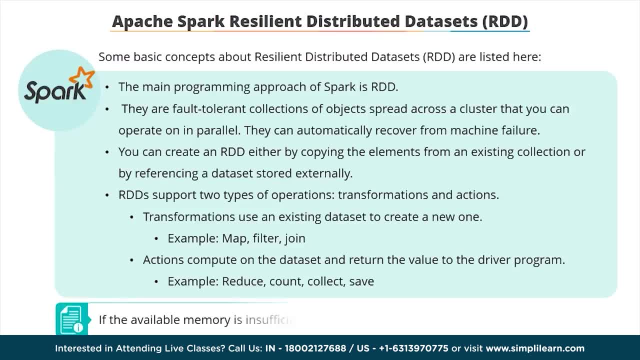 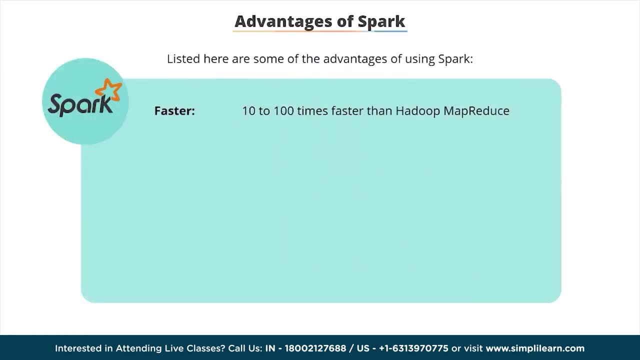 are Count, Collect and Save. It's important to note that if the available memory is insufficient, then Spark writes the data to disk. Here are some of the advantages of using Spark: It's almost 10 to 100 times faster than Hadoop MapReduce. 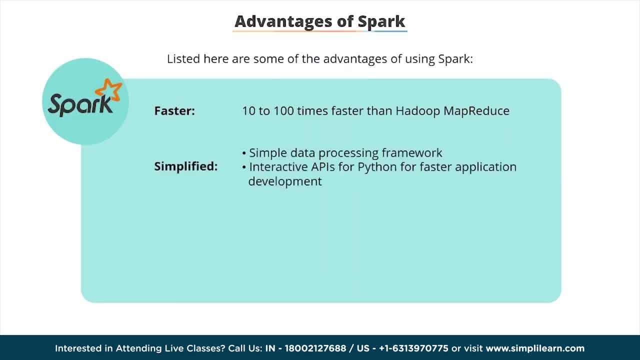 It has a simple data processing framework. It provides interactive APIs for Python that allow faster application development. It has multiple tools for complex analytics operations. These tools help data scientists perform machine learning and other analytics much more efficiently and easily than most existing tools. It can easily be integrated with. 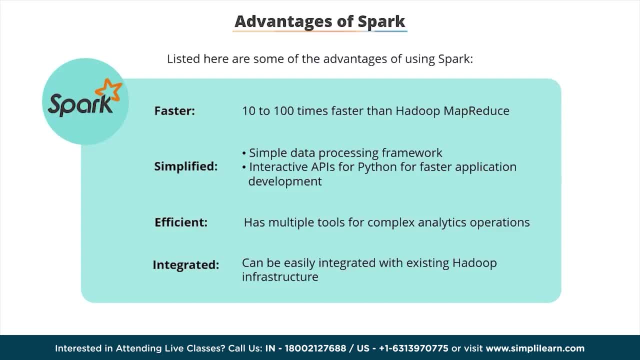 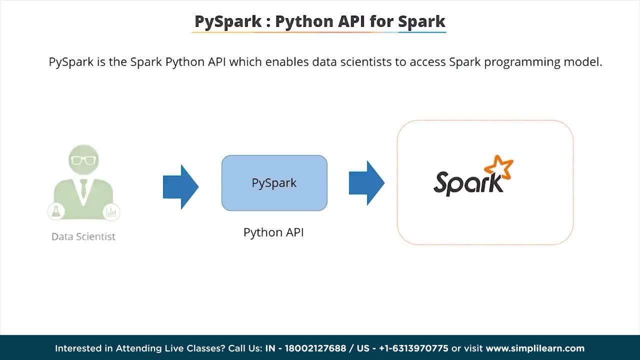 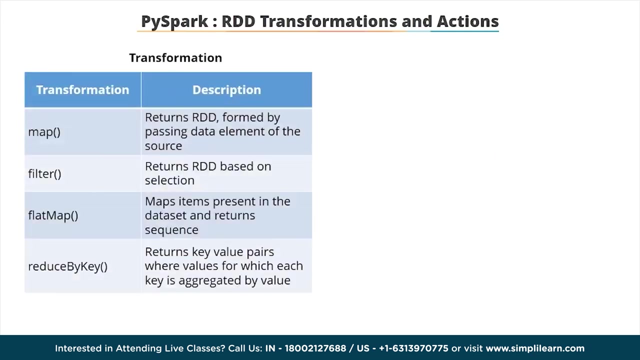 the existing Hadoop infrastructure. PySpark is the Python API used to access the Spark programming model and perform data analysis. Let's take a look at some transformation functions and action methods which are supported by PySpark for data analysis. These are some common transformation. 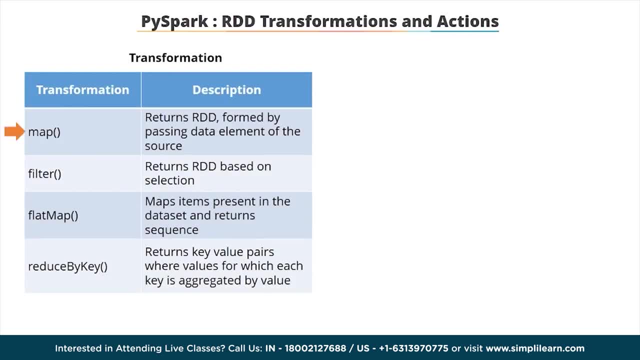 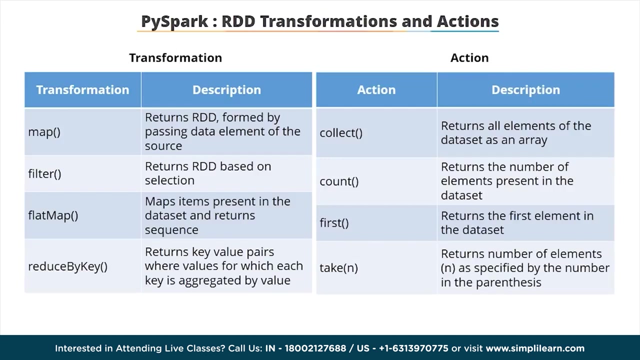 functions. Let's now look at some common action functions. Collect returns all elements of the dataset as an array. Count returns the number of elements present in the dataset First returns the first element in the dataset. Take returns the number of elements as specified by the number. 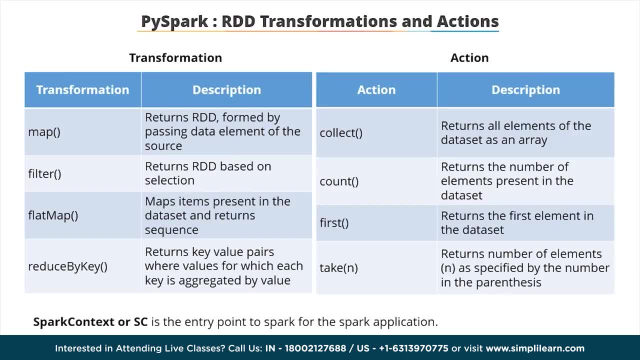 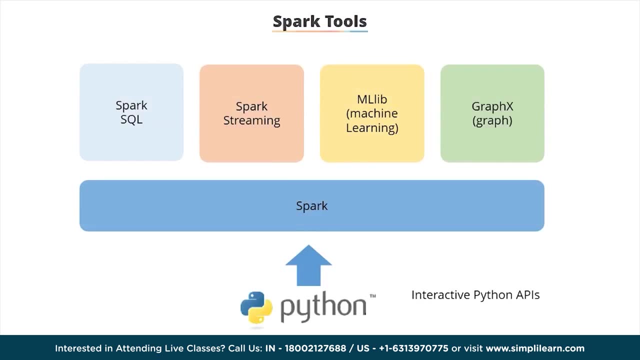 in the parentheses. Spark Context or SC, is the entry point to Spark for the Spark application And must be available at all times for data processing. There are mainly four components in Spark tools: Spark SQL: It's mainly used for querying the data stored on HDFS. 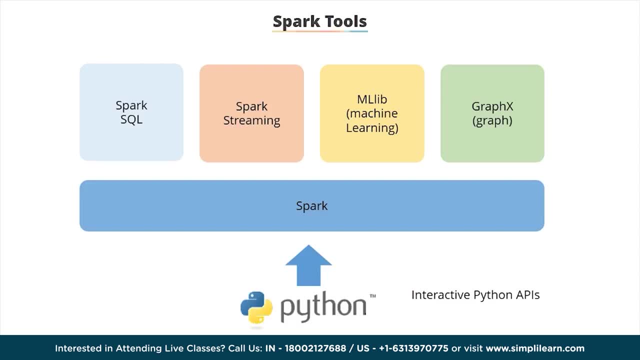 as a resilient distributed dataset, or RDD, in Spark, through integrated APIs in Python, Java and Scala. Spark Streaming: It's very useful for data streaming process and where data can be read from various data sources. MLlib- It's mainly used for machine learning processes, such as supervised 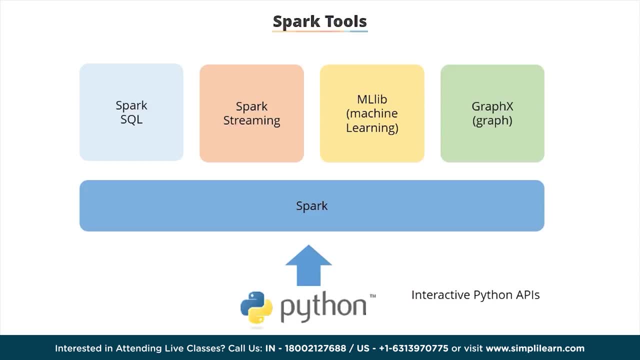 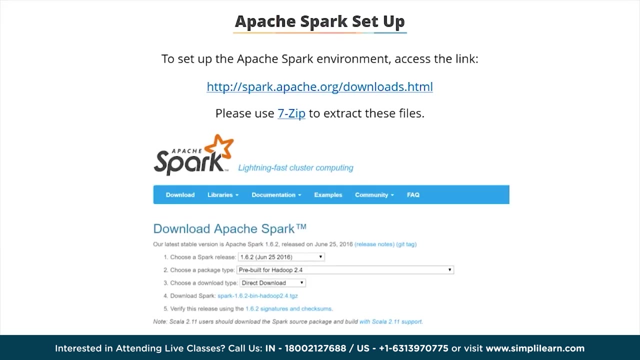 and unsupervised learning GraphX. It can be used to process or generate graphs with RDDs. Let's set up the Apache Spark environment and also learn how to integrate Spark with Jupyter Notebook. First visit the Apache link and download Apache Spark to your system. 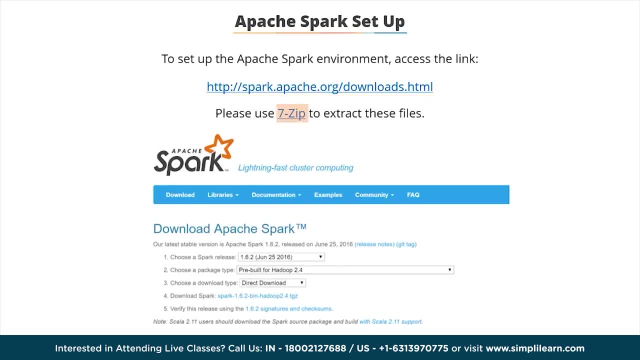 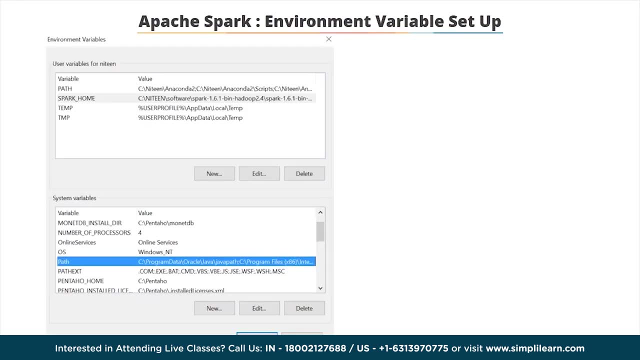 Now use 7-zip software and extract the files to your system's local directory. To set up the environment variables for Spark: first set up the user variables, Click New and then enter Spark Home in the variable name and enter the Spark installation path. 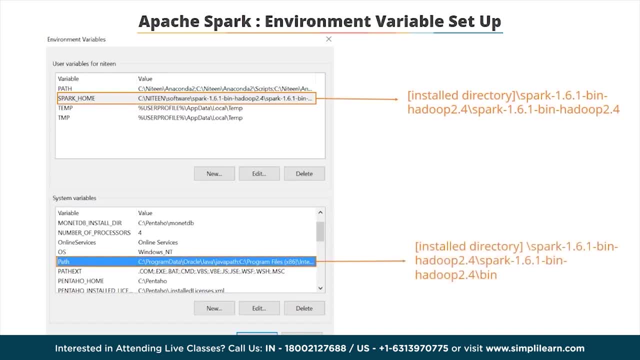 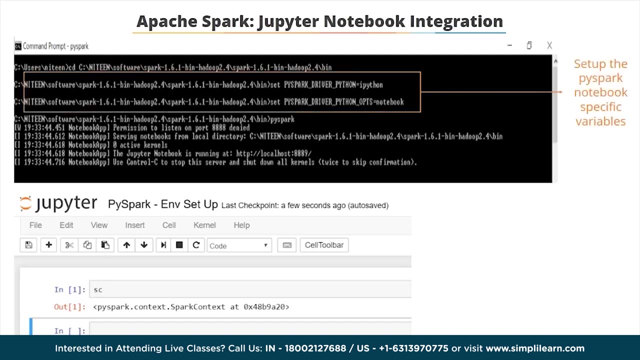 as variable value. Now click on the path and enter the Spark bin path from the installed directory location. Now let's set up the PySpark Notebook's specific variables. This will integrate the Spark engine with Jupyter Notebook Type in PySpark. 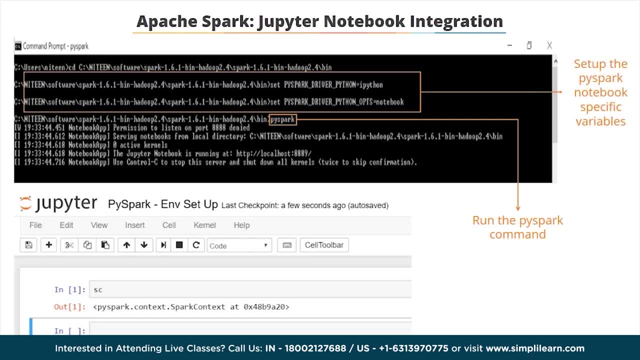 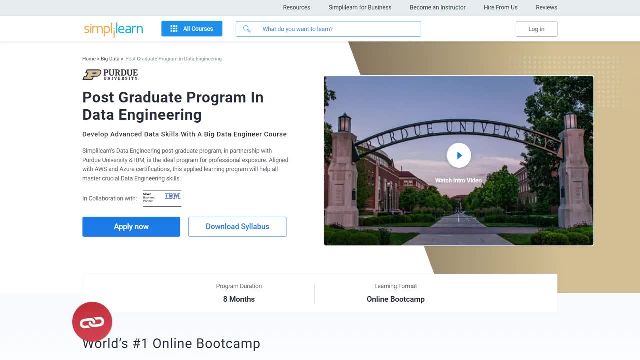 It will launch a Jupyter Notebook after a while. Create a Python Notebook and type in sc command to check the Spark context. Now, whether you are an aspirin data analyst, a seasoned IT professional or a business leader looking to leverage the power of big data, 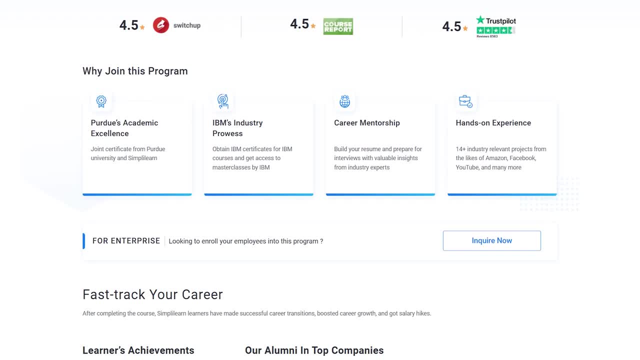 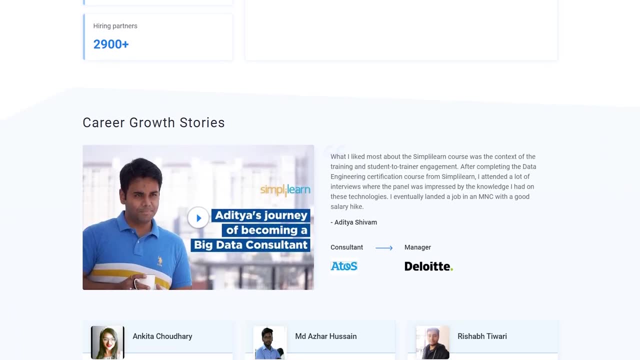 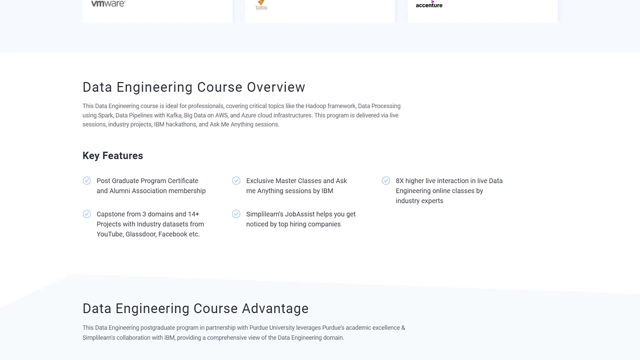 the Data Engineering Postgraduate program by SimplyLearn, in collaboration with Purdue University and IBM, is tailored to meet your needs. This program offers an exceptional opportunity for professional growth and exposure, with a focus on practical learning and in alignment with industry-leading certifications from AWS and Azure. 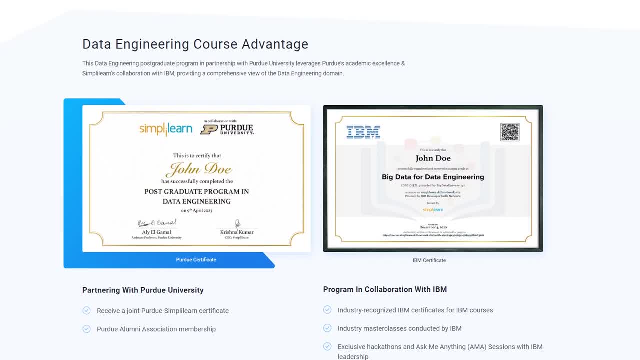 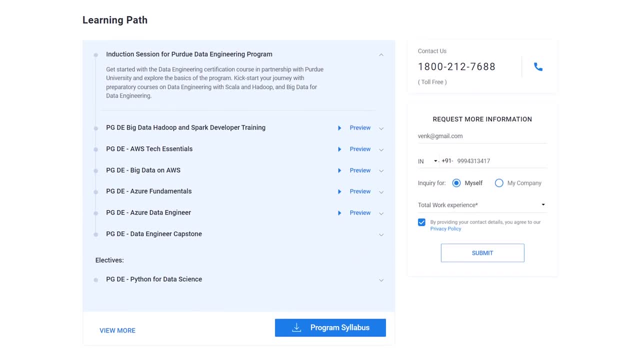 Now. this program equips participants with essential skills required to excel in this field of data engineering. By enrolling in this applied learning program, individuals can gain master of crucial data engineering techniques and technologies. Enroll today and take the next step towards becoming a proficient big data professional. 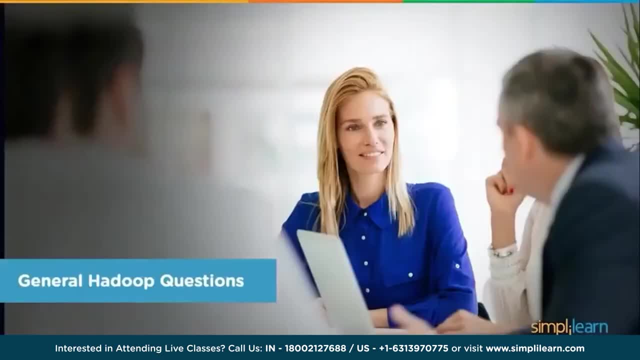 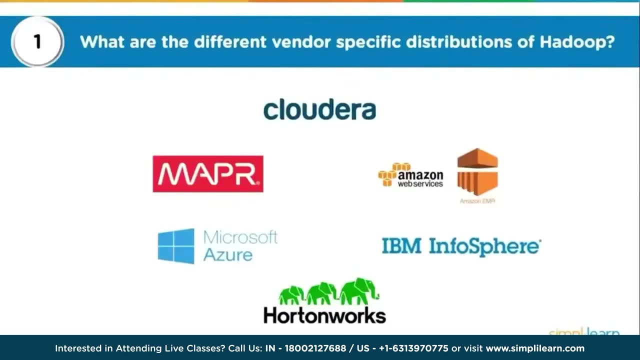 Check out the course link in the description box below for more details. Now let's look at some general Hadoop questions. So what are the different vendor specific distributions of Hadoop? Now, all of you might be aware that Hadoop, or Apache, 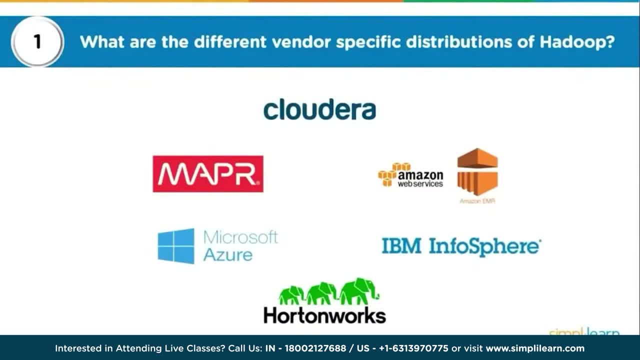 Hadoop is the core distribution of Hadoop, And then you have different vendors in the market which have packaged the Apache Hadoop in a cluster management solution which allows everyone to easily deploy, manage, monitor, upgrade your clusters. So here are some. 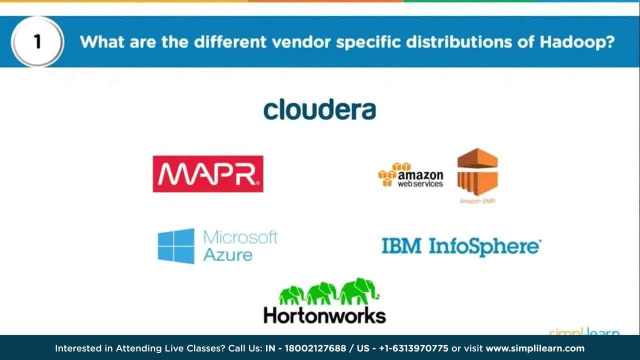 vendor specific distributions. We have Cloudera, which is the dominant one in the market. We have Hortonworks, and now you might be aware that Cloudera and Hortonworks have merged, So it has become a bigger entity. You have MapR. 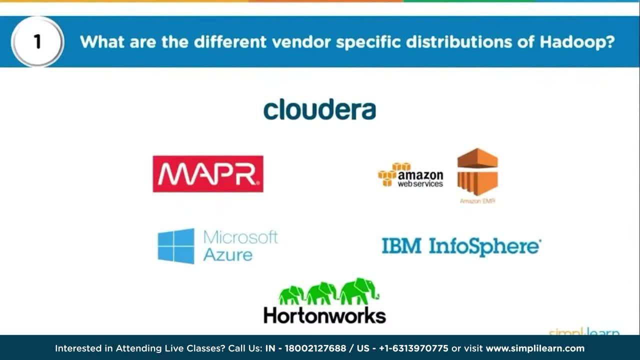 you have Microsoft Azure, IBM's InfoSphere and Amazon Web Services, So these are some popularly known vendor specific distributions. If you would want to know more about the Hadoop distributions, you should basically look into Google and you should check for Hadoop- different distributions- wiki. 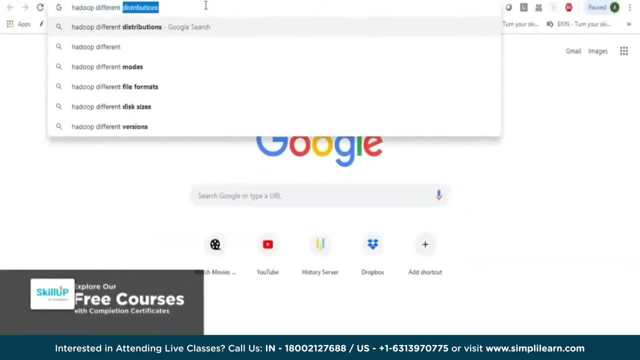 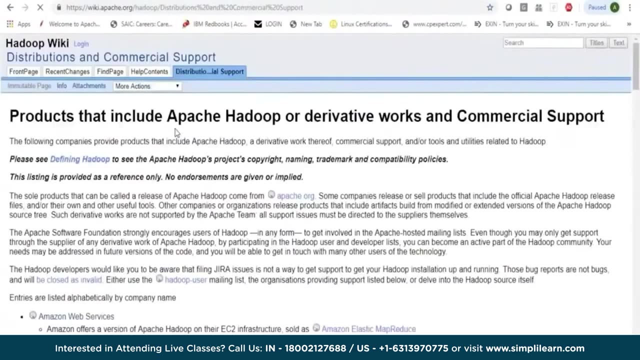 page. So if I type Hadoop- different distributions and then I check for the wiki page, that will take me to the distributions and commercial support page And this basically says that the sole products that can be called a release of Apache Hadoop come from Apacheorg. 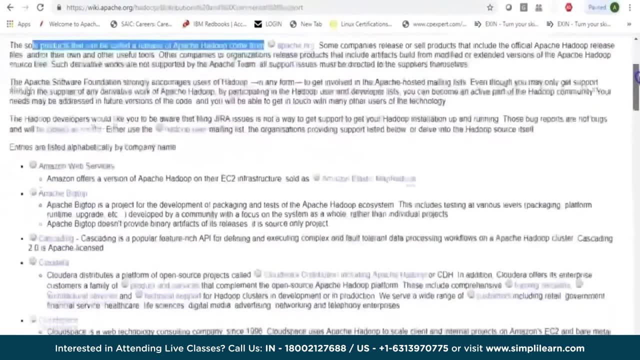 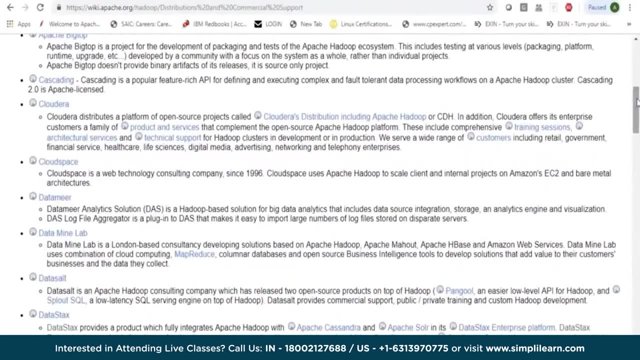 So that's your open source community, and then you have various vendor specific distributions which basically are running in one or the other way: Apache, Hadoop- but they have packaged it as a solution like an installer so that you can easily set up clusters on set of machines. So have a look at this page. 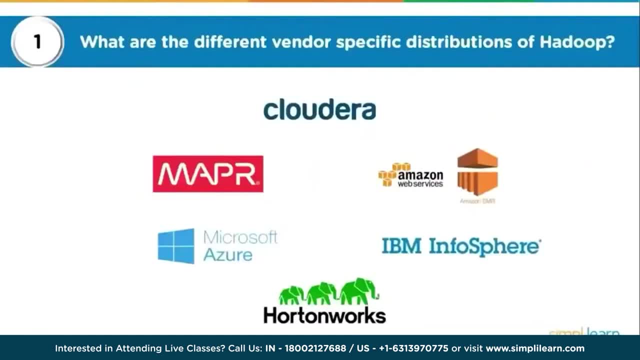 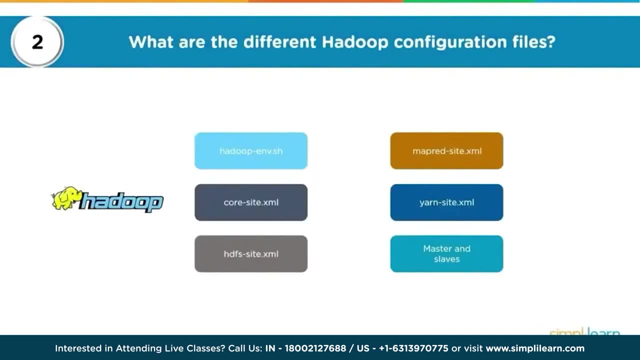 and read through about different distributions of Hadoop. Coming back, let's look at our next question. So what are the different Hadoop configuration files Now? whether you are talking about Apache, Hadoop, Cloudera, Hortonworks, MapR or no matter. 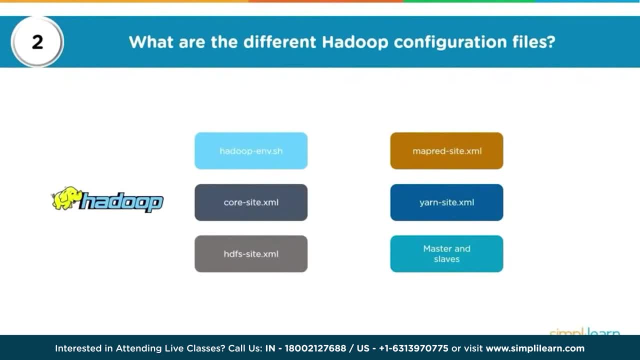 which other distribution. these config files are the most important and existing in every distribution of Hadoop. So you have Hadoop environmentsh, wherein you will have environment variables such as your Java path, what would be your process ID path? where will your logs get stored? 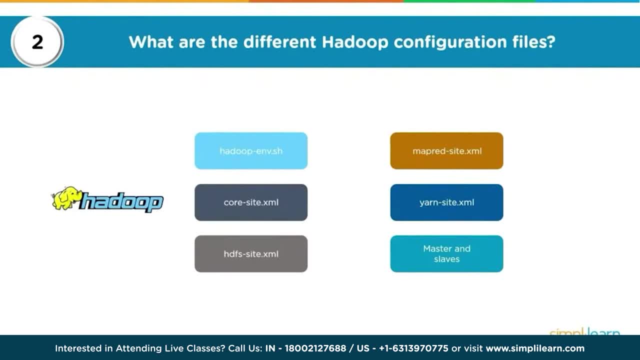 what kind of metrics will be collected, and so on. Your core-site file has the HDFS path. Now, this has many other properties, like enabling thrash, or enabling high availability, or discussing or mentioning about your zookeeper, but this is one of the most. 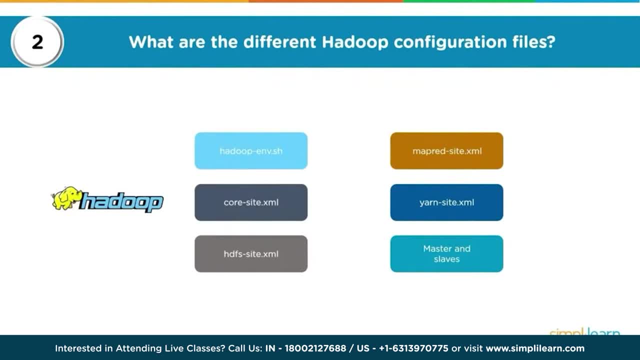 important file. You have HDFS hyphen site file Now. this file will have other information related to your Hadoop cluster, such as your replication factor. where will name node store its metadata? on disk. if a data node is running, where would data node 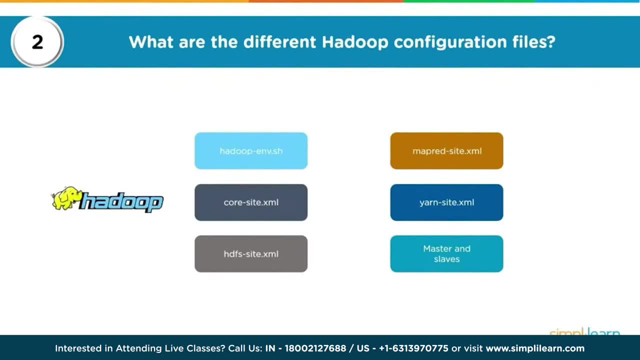 store its data? if a secondary name node is running, where would that store a copy of name node's metadata and so on? Your MapRed hyphen site file is a file which will have properties related to your MapReduce processing. You also have masters and slaves. 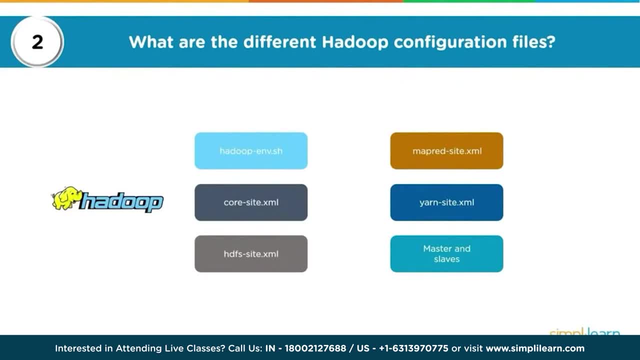 Now these might be deprecated in a vendor specific distribution and, in fact, you would have a yarn hyphen site file which is based on the yarn processing framework which was introduced in Hadoop version 2, and this would have all your resources allocation and resource manager. 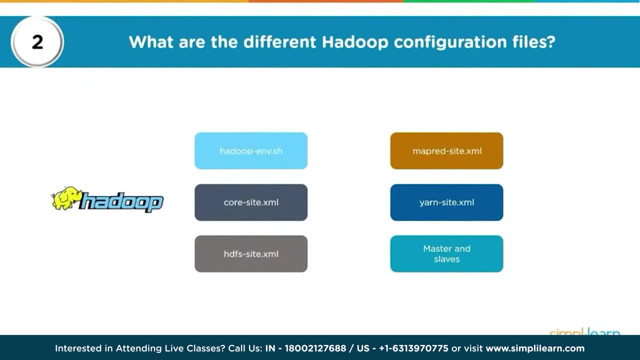 and node manager related properties. Again, if you would want to look at default properties for any one of these, for example, let's say, HDFS hyphen site file, I could just go to Google and type in one of the properties, For example. I would. 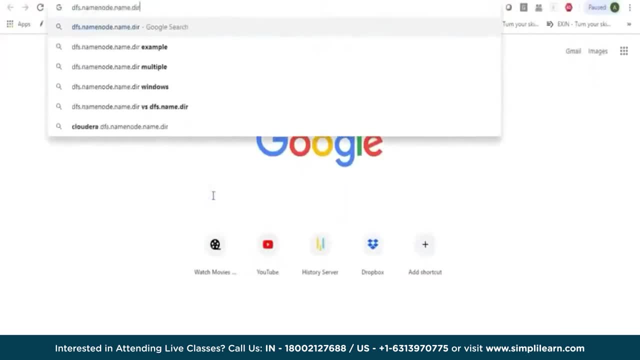 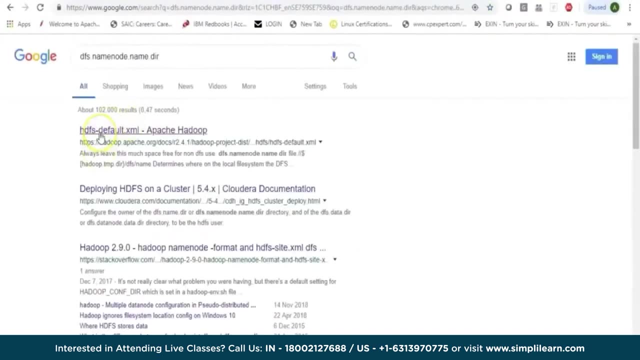 say dfs, dot name, node, dot name, dot directory and, as I know, this property belongs to HDFS hyphen site file and if you search for this, it will take you to the first link that says HDFS default XML. You can click on this and this. 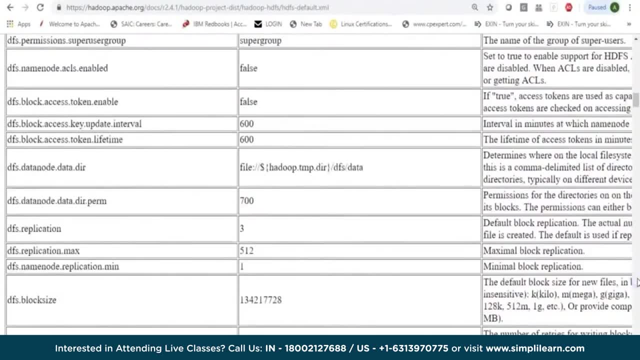 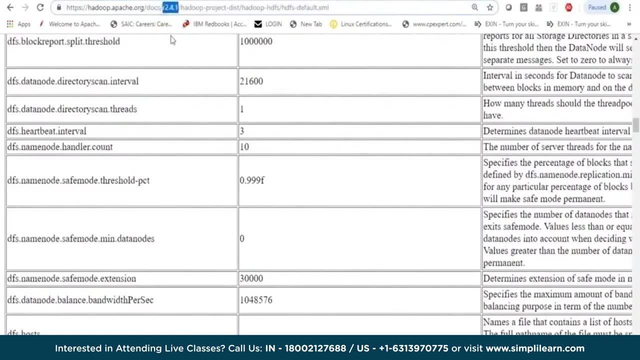 will show you all the properties which can be given in your HDFS hyphen site file. It also shows you which version you are looking at, and you can always change the version here. So, for example, if I would want to look at 2.6.5. 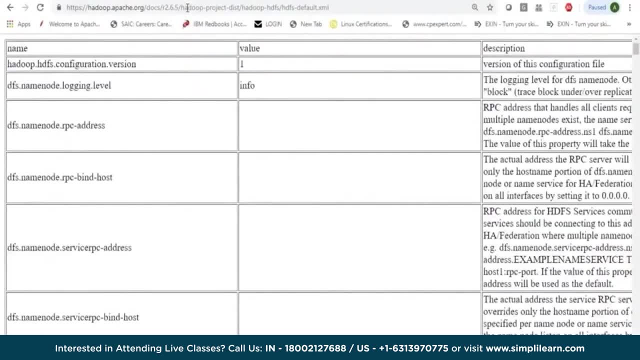 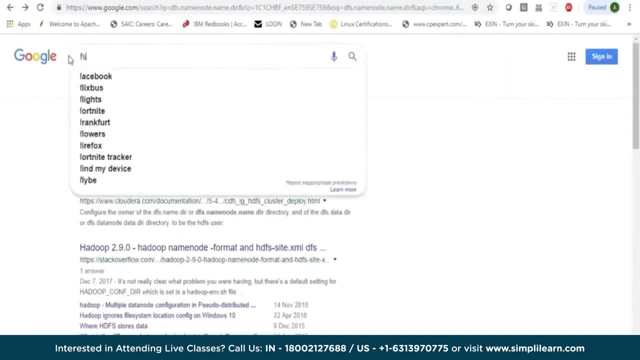 I just need to change the version and that should show me the properties. Similarly, you can just give a property which belongs to, say, core hyphen, site file. For example, I would say fs, dot, default, fs, and that's a property which is in core hyphen. 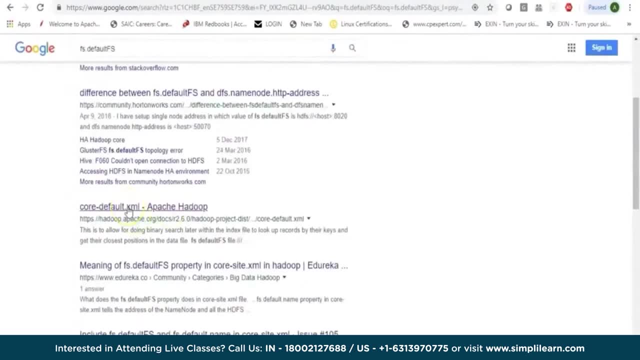 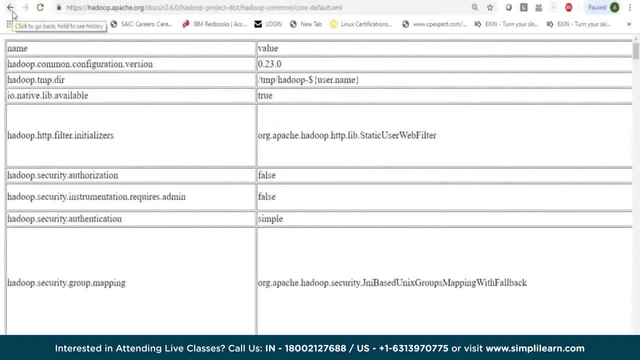 site file and somewhere here you would see core minus default dot xml and this will show you all the properties. So similarly, you could search for properties which are related to yarn hyphen site file or map red hyphen site file. So I could say: 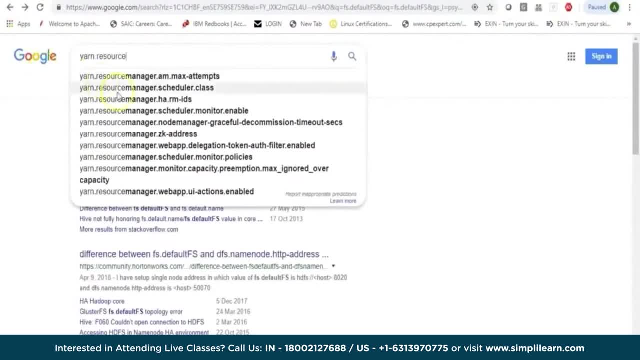 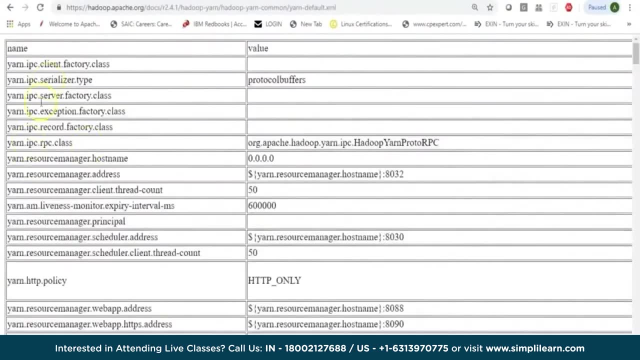 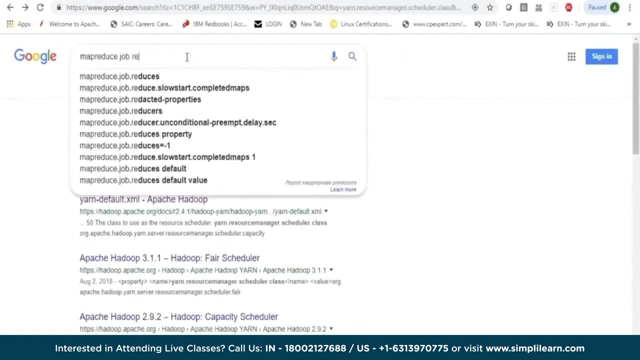 yarn dot resource manager and I could look at one of these properties which will directly take me to yarn default xml and I can see all the properties which can be given in yarn. and similarly you could say map reduce dot job dot reduces and I know this property belongs. 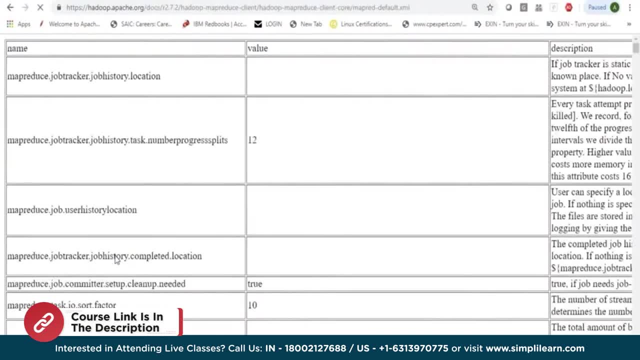 to map reduce hyphen site file and this takes you to the default xml. So these are important config files and, no matter which distribution of Hadoop you are working on, you should be knowing about these config files, Whether you work as a Hadoop. 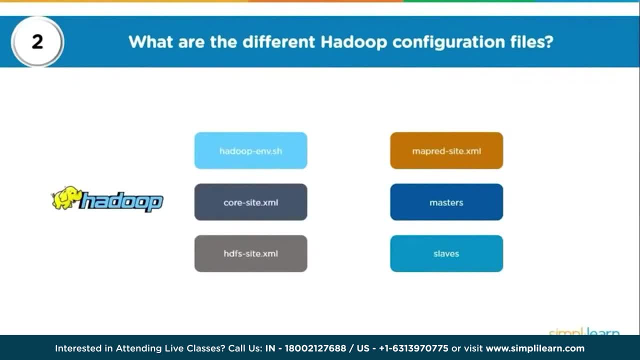 admin or you work as a Hadoop developer. knowing these config properties would be very important, and that would also showcase your internal knowledge about the configs which drive your Hadoop cluster. Let's look at the next question. So what are the three modes in which? 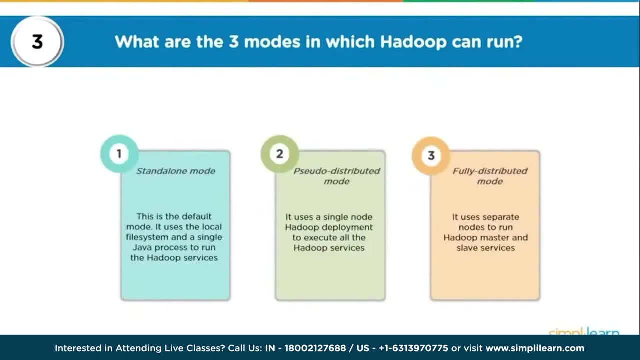 Hadoop can run. So you can have Hadoop running in a standalone mode. Now, that's your default mode. It would basically use a local file system and a single java process. So when you say standalone mode, it is as: 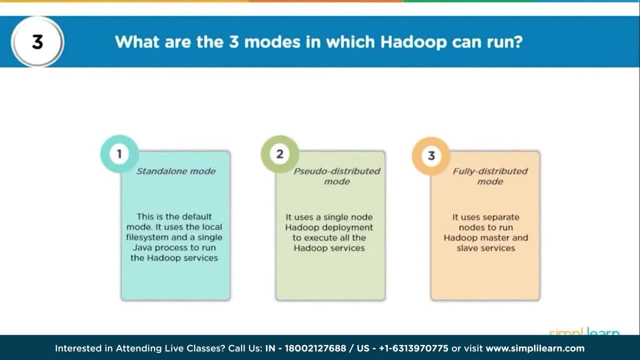 you downloading Hadoop related package on one single machine, but you would not have any process running. that would just be to test Hadoop functionalities. You could have a pseudo distributed mode which basically means it's a single node. Hadoop deployment, Now Hadoop as. 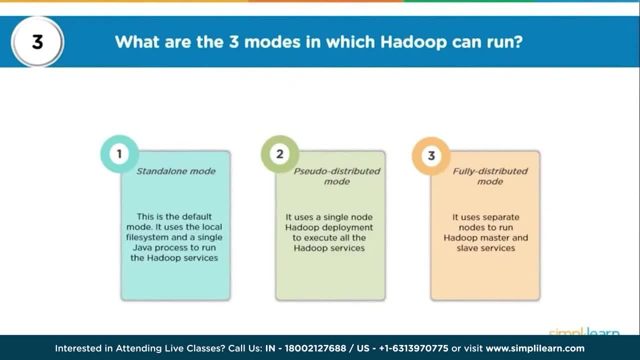 a framework has many, many services, So it has lot of services, and those services would be running irrespective of your distribution. Each service would then have multiple processes. So your pseudo distributed mode is a mode of cluster where you would have all the important processes belonging to 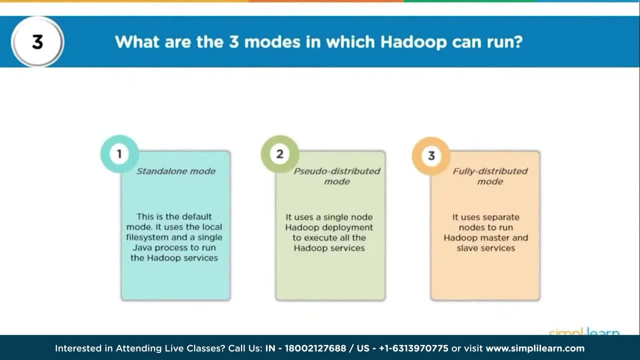 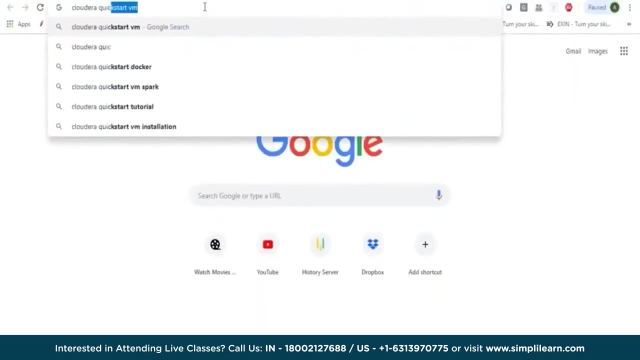 one or multiple services running on a single node. If you would want to work on a pseudo distributed mode and using a Cloudera, you can always go to Google and search for Cloudera's Quick Start VM. You can download it by just saying Cloudera Quick. 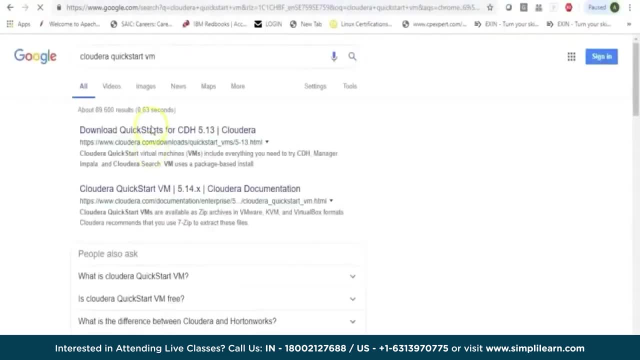 Start VM and you can search for this and that will allow you to download a Quick Start VM. follow the instructions and you can have a single node Cloudera cluster running on your virtual machines. For more information, you can refer to the YouTube tutorial, where I have 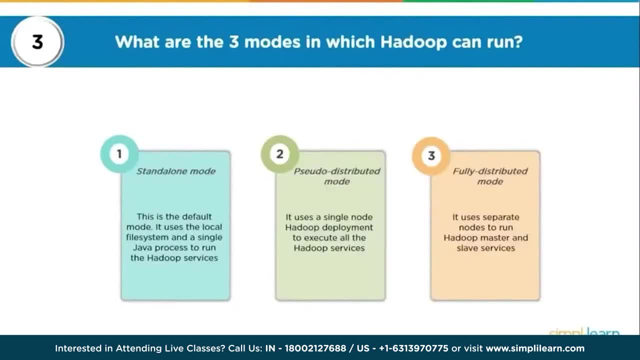 explained about how to set up a Quick Start VM. Coming back, you could have, finally, a production setup or a fully distributed mode, which basically means that your Hadoop framework and its components would be spread across multiple machines, So you would have multiple services, such as: 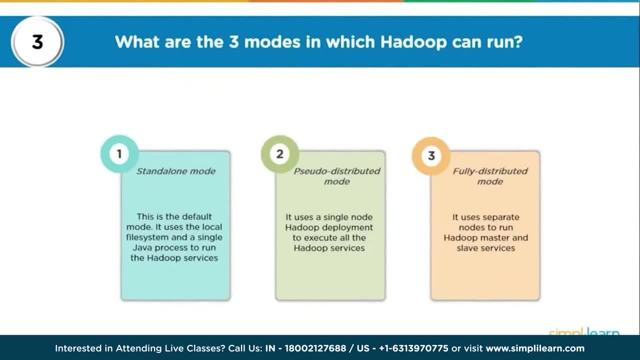 HDFS, YARN, Flume Scoop, Kafka, HBase, Hive Impala- and for these services there would be one or multiple processes distributed across multiple nodes. So this is normally what is used in production environment. So you could say standalone would be good. 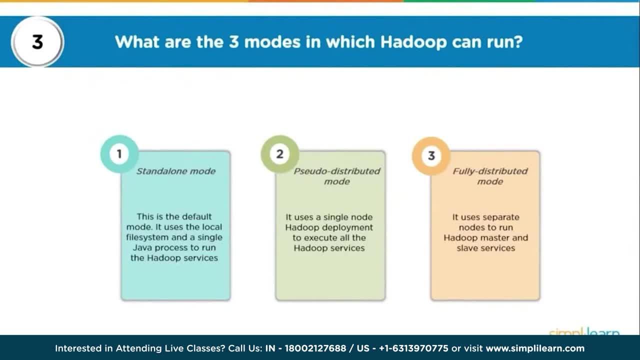 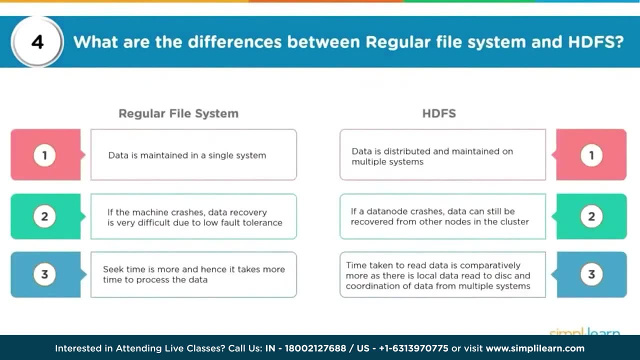 for testing. pseudo distributed could be good for testing and development, and fully distributed would be mainly for your production setup. Now, what are the differences between regular file system and HDFS? So when you say regular file system, you could be talking about a Linux file. 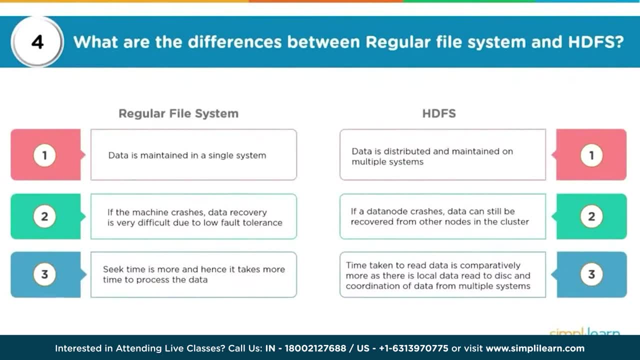 system, or you could be talking about a Windows based operating system. So in regular file system we would have data maintained in a single system. So the single system is where you have all your files and directories. So it is having low fault tolerance. 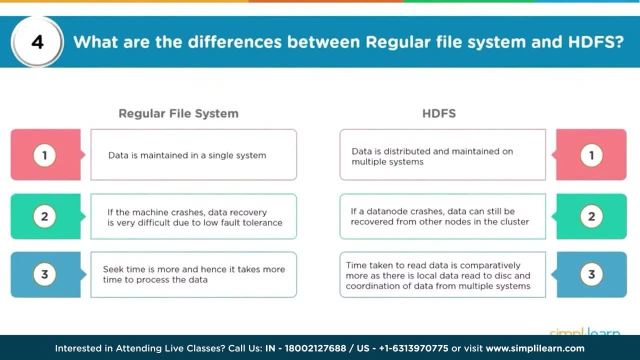 right. So if the machine crashes, your data recovery would be very difficult unless and until you have a backup of that data That also affects your processing. So if the machine crashes or if the machine fails, then your processing would be blocked. 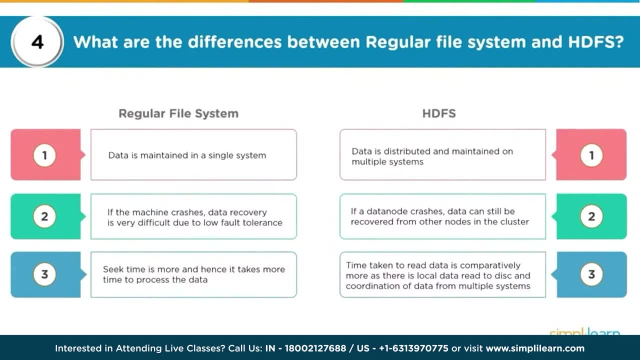 Now the biggest challenge with regular file system is the seek time, the time taken to read the data. So you might have one single machine with huge amount of disks and huge amount of RAM, but then the time taken to read that data when all the 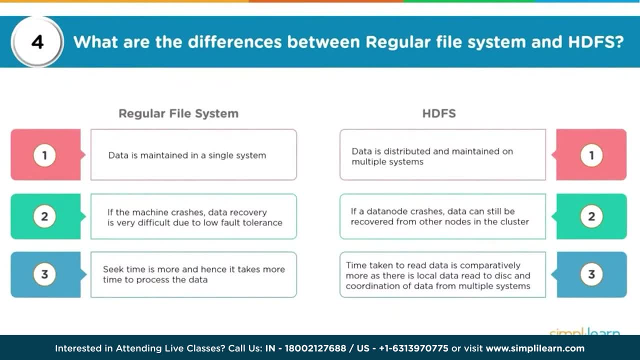 data is stored in one machine would be very high and that would be with least fault tolerance. If you talk about HDFS, your data is distributed, so SDFS stands for Hadoop, Distributed File System. So here your data is distributed and maintained on multiple. 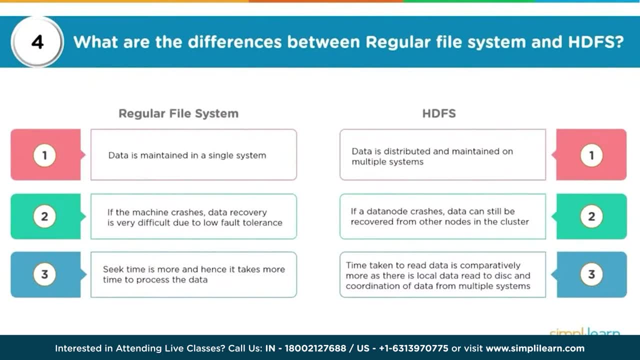 systems, So it is never one single machine. It is also supporting reliability. So whatever is stored in HDFS, say, a file being stored depending on its size is split into blocks, and those blocks will be spread across multiple nodes. Not only that, every block, 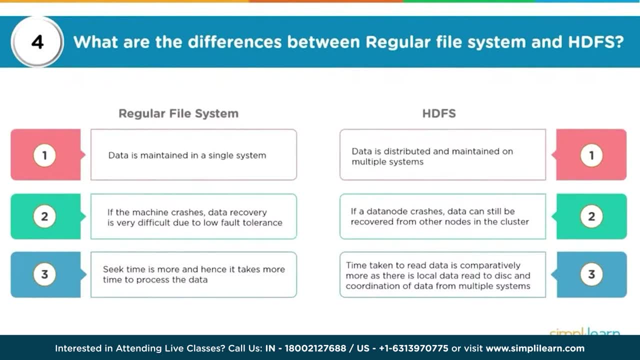 which is stored on a node will have its replicas stored on other nodes. Replication factor depends, but this makes HDFS more reliable In cases of your slave nodes or data nodes crashing. you will rarely have data loss because of auto replication feature. Now time taken to read. 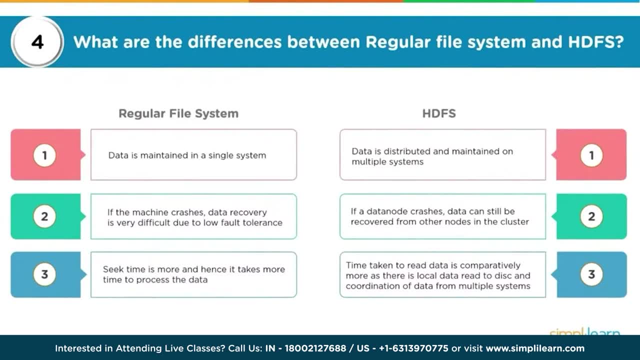 the data is comparatively more, as you might have situations where your data is distributed across the nodes and even if you are doing a parallel read, your data read might take more time because it needs coordination from multiple machines. However, if you are working with huge data which is getting stored, it will. 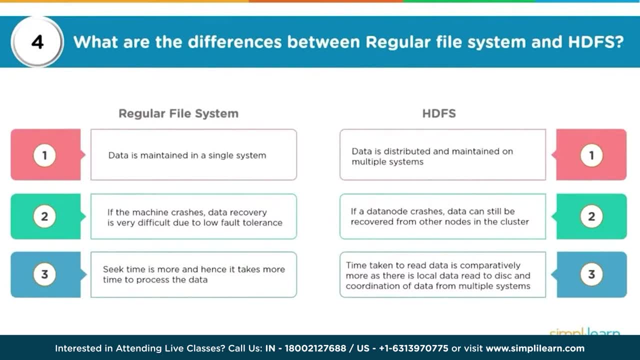 still be beneficial in comparison to reading from a single machine. So you should always think about its reliability through auto replication feature, its fault tolerance because of your data getting stored across multiple machines, and its capability to scale. So when you talk about HDFS, 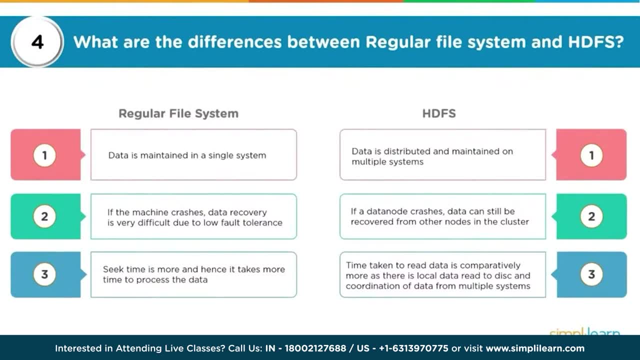 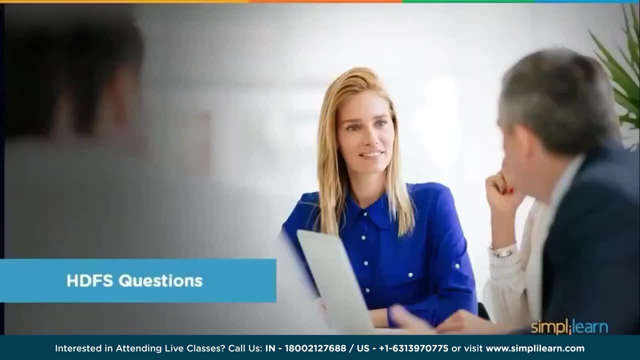 we are talking about horizontal scalability, or scaling out. When you talk about regular file system, you are talking about vertical scalability, which is scaling up. Now let's look at some specific HDFS questions. What is this? Why is HDFS fault tolerant? 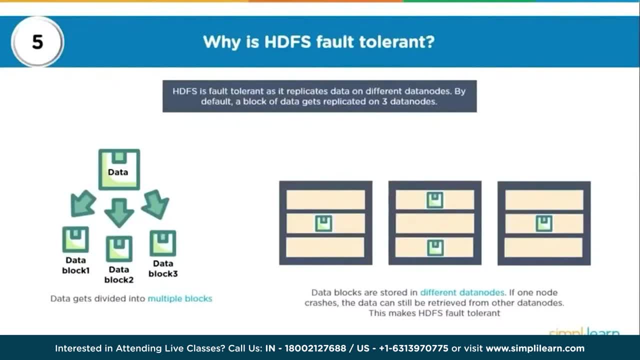 Now, as I just explained in previous slides, your HDFS is fault tolerant as it replicates data on different data nodes. So you have a master node and you have multiple slave nodes or data nodes where actually the data is getting stored. Now we also have a default. 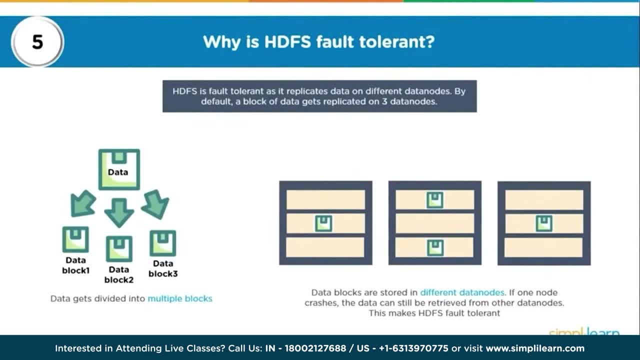 block size of 128 MB. That's the minimum since Hadoop version 2.. So any file which is up to 128 MB would be using one logical block, and if the file size is bigger than 128 MB then it will be split. 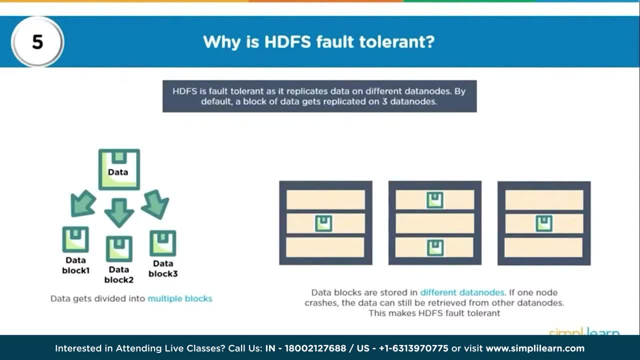 into blocks, and those blocks will be stored across multiple machines. Now, since these blocks are stored across multiple machines, it makes it more fault tolerant, because even if your machines fail, you would still have a copy of your block existing on some other machine. Now there are two aspects here. 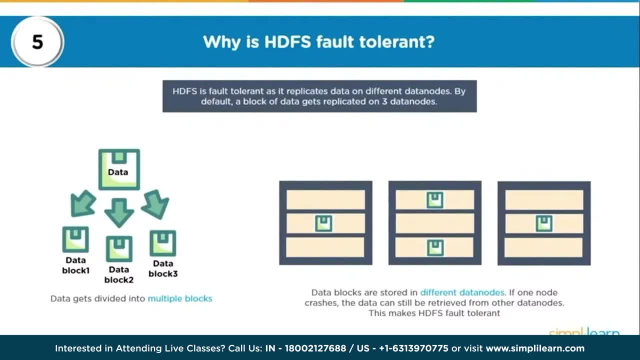 One. we talk about the first rule of replication, which basically means you will never have two identical blocks sitting on the same machine. and the second rule of replication is in terms of rack awareness. So if your machines are placed in racks, as we see in the right image, you will 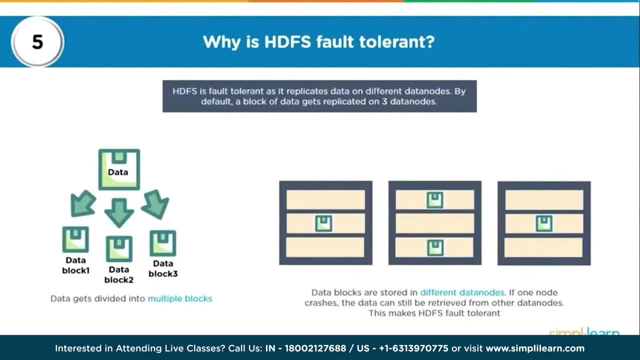 never have all the replicas placed on the same rack, even if they are on different machines. So it has to be fault tolerant and it has to maintain redundancy, So at least one replica will be placed on some other node, on some other rack. That's how. 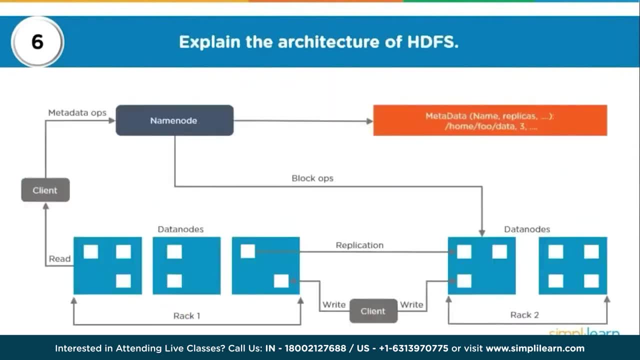 HDFS is fault tolerant. Now here let's understand the architecture of HDFS. Now, as I mentioned earlier, you would in a Hadoop cluster. the main service is your HDFS. So for your HDFS, you would have a name. 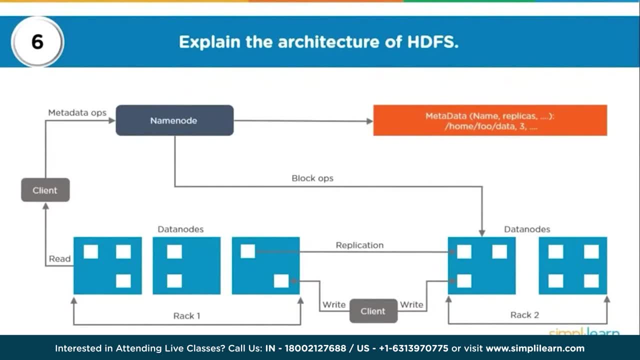 node, which is your master process running on one of the machines, and you would have data nodes, which are your slave machines getting stored across or getting, or the processes running across multiple machines. Each one of these processes has an important role to play When you talk about HDFS. 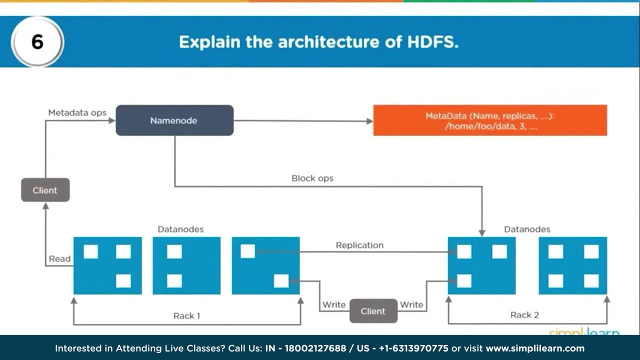 whatever data is written to HDFS, that data is split into blocks depending on its size, and the blocks are randomly distributed across nodes With auto-replication feature. these blocks are also auto-replicated across multiple machines, with the first condition that no. 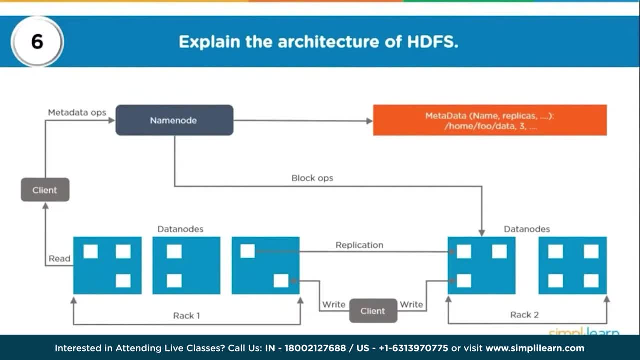 two identical blocks will sit on the same machine. Now, as soon as the cluster comes up, your data nodes, which are part of the cluster and based on config files, would start sending their heartbeat to the name node, and this would be every three seconds. What does name? 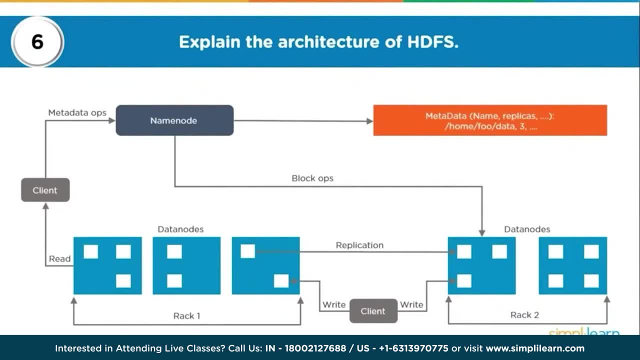 node do with. that Name node will store this information in its RAM. So name node starts building a metadata in its RAM and that metadata has information of what are the data nodes which are available in the beginning. Now, when a data writing activity starts and the blocks are, 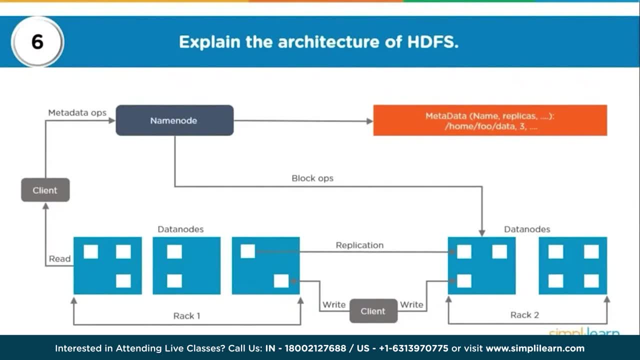 distributed across data nodes. data nodes every 10 seconds will also send a block report to name node. So name node is again adding up this information in its RAM or the metadata in RAM, which earlier had only data node information. Now name node will also have. 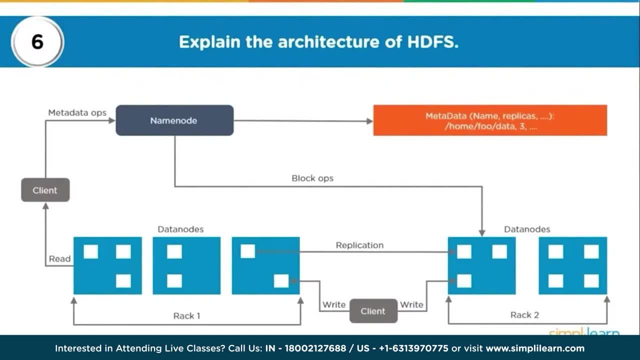 information about what are the files. the files are split in which blocks, the blocks are stored, on which machines and what are the file permissions. Now, while name node is maintaining this metadata in RAM, name node is also maintaining metadata in disk. Now, that is what we see. 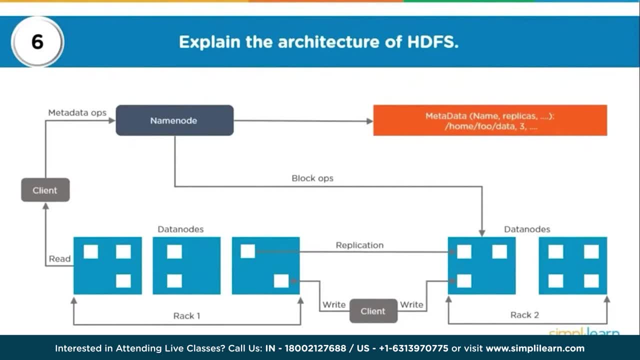 in the red box, which basically has information of whatever information was written to HDFS. So to summarize, your name node has metadata in RAM and metadata in disk. Your data nodes are the machines where your blocks or data is actually getting stored, and then there is a auto replication. 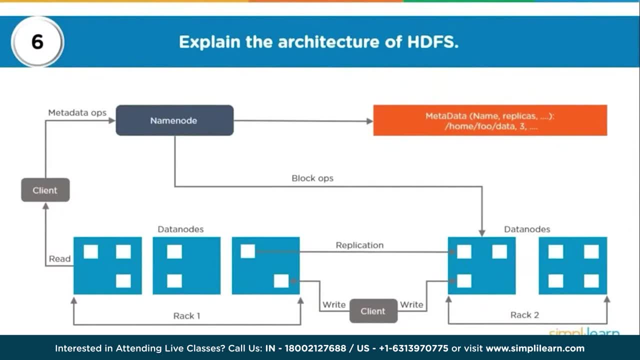 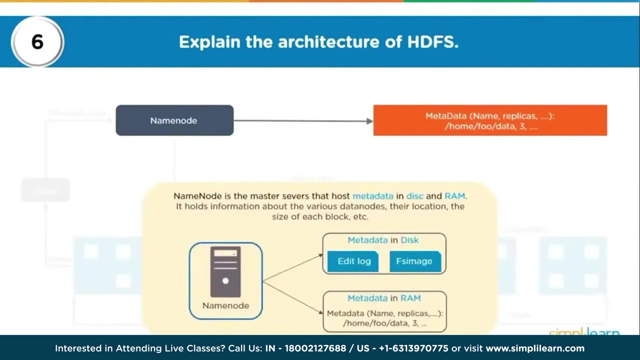 feature which is always existing unless and until you have disabled it, and your read and write activity is a parallel activity. However, replication is a sequential activity. Now, this is what I mentioned about when you talk about name node, which is the master process hosting metadata. 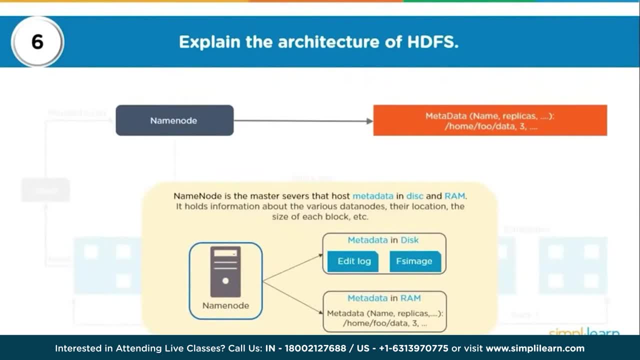 in disk and RAM. So when we talk about disk, it basically has a edit log, which is your transaction log, and your FS image, which is your file system image. Right from the time the cluster was started, this metadata in disk was existing and 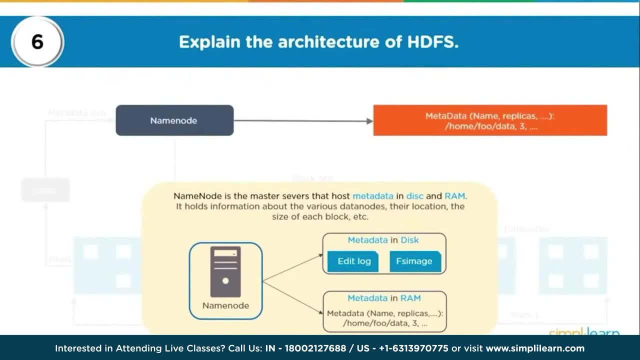 this gets appended every time read, write or any other operations happen on HDFS. Metadata in RAM is dynamically built every time the cluster comes up, which basically means that if your cluster is coming up, name node in the initial few seconds or few minutes would be in. 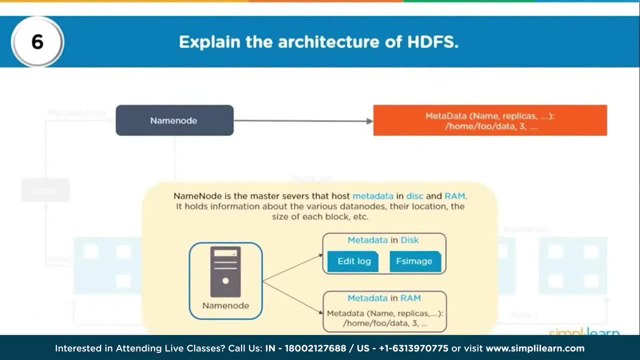 a safe mode, which basically means it is busy registering the information from data nodes. So name node is one of the most critical processes. if name node is down and if all other processes are running, you will not be able to access the cluster Name node's. 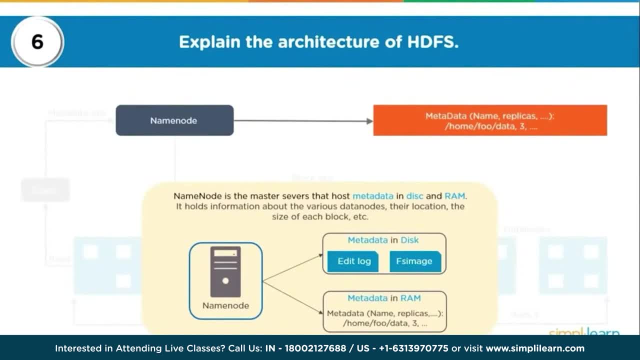 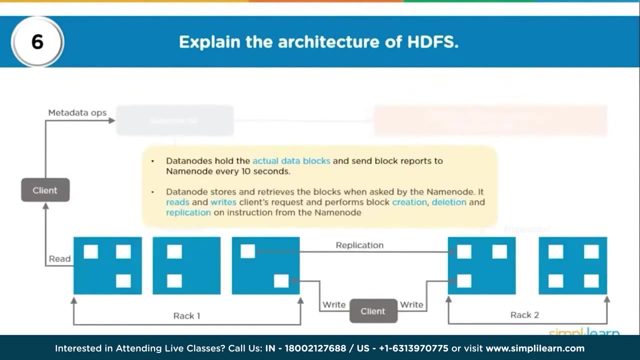 metadata in disk is very important for name node to come up and maintain the cluster. Name node's metadata in RAM is basically for all or satisfying all your client requests. Now, when we look at data nodes, as I mentioned, data nodes hold the actual data blocks and they are 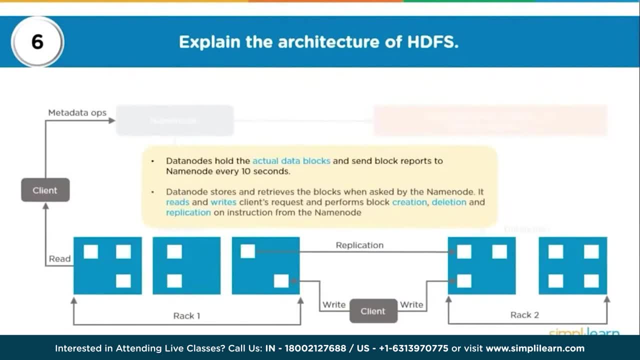 sending these block reports every 10 seconds. So the metadata in name node's RAM is constantly getting updated and metadata in disk is also constantly getting updated based on any kind of write activity happening on the cluster. Now data node which is storing the block will also. 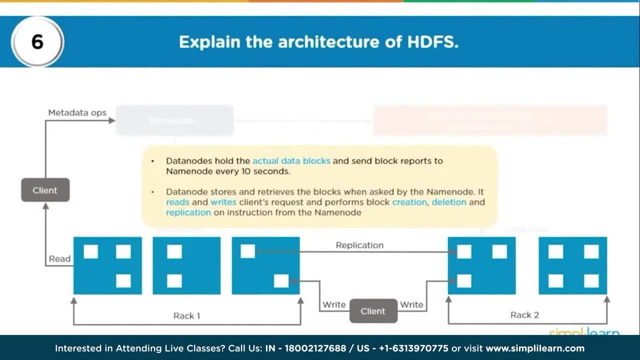 help in any kind of read activity whenever a client requests. So whenever a client or an application or an API would want to read the data, it would first talk to name node. Name node would look into its metadata on RAM and confirm to the client. 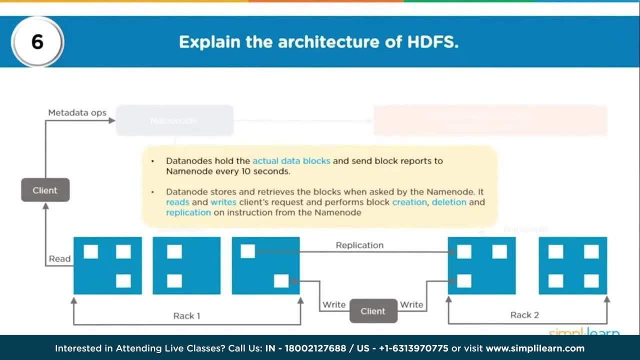 which machines could be reached to get to that data. That's where your client would try to read the data from SDFS, which is actually getting the data from data nodes, And that's how your read write requests are satisfied. Now, what are the two types of? 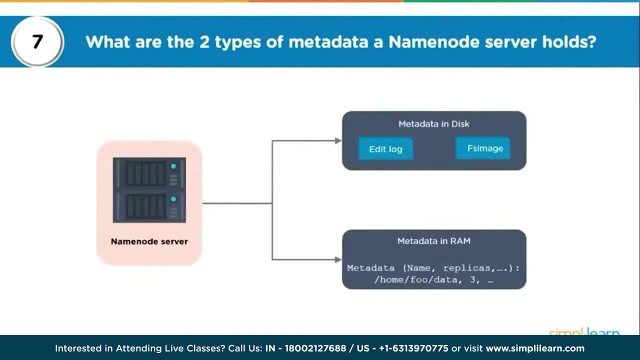 metadata in name. node server holds, As I mentioned earlier, metadata in disk, very important to remember: edit log, NFS image. metadata in RAM, which is information about your data nodes, files, files being split into blocks, blocks residing on data nodes. 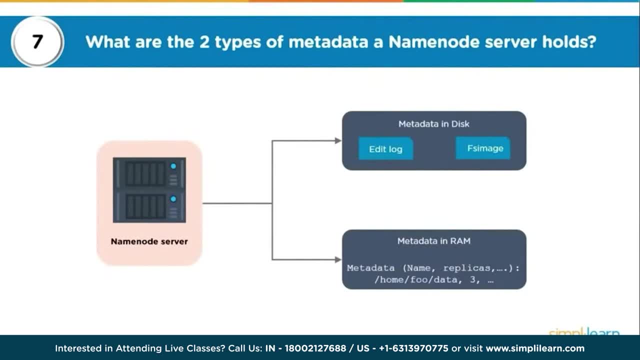 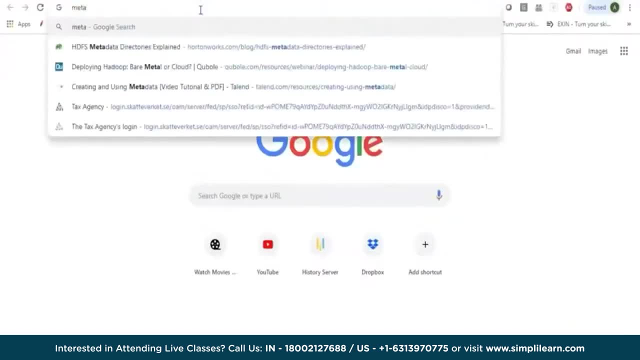 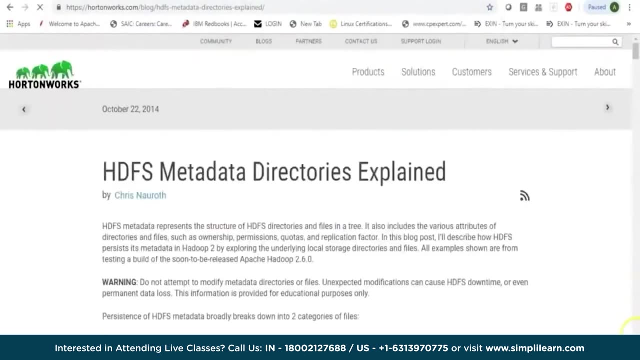 and file permissions. So I will share a very good link on this, and you can always look for more detailed information about your metadata So you can search for SDFS metadata directories explained Now. this is from Hortonworks, However, it talks about the metadata. 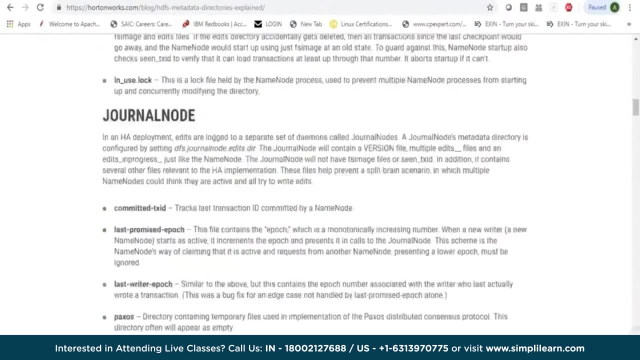 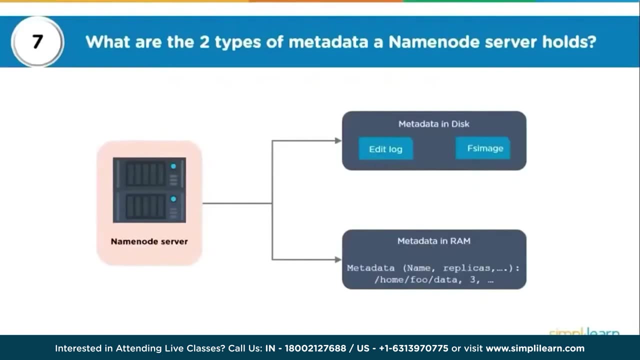 in disk which name node manages and details about this. So have a look at this link if you are more interested in learning about metadata on disk. Coming back, let's look at the next question. What is the difference between federation and high availability? 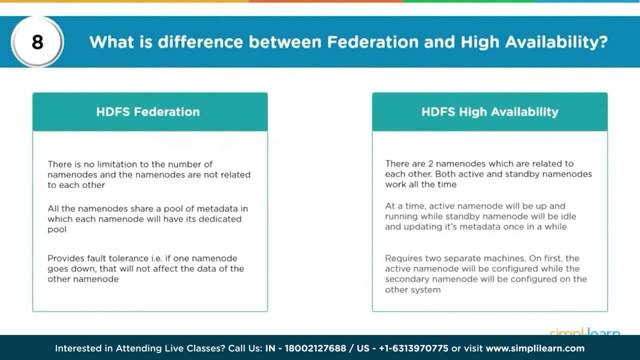 Now, these are the features which were introduced in Hadoop version 2.. Both of these features are about horizontal scalability of name node. So prior to version 2, the only possibility was that you could have one single master, which basically means that your cluster 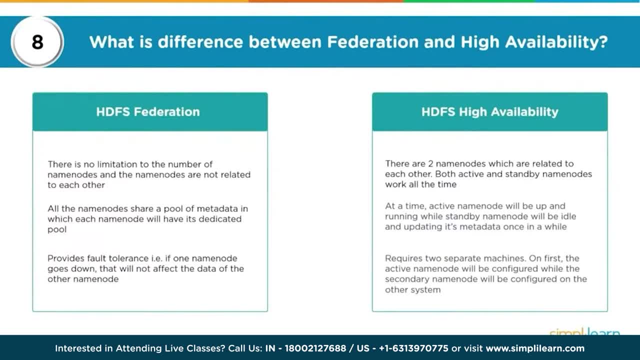 could become unavailable if name node would crash. So Hadoop version 2 introduced two new features: federation and high availability. However, high availability is a popular one, So when you talk about federation, it basically means any number of name nodes. So there is. 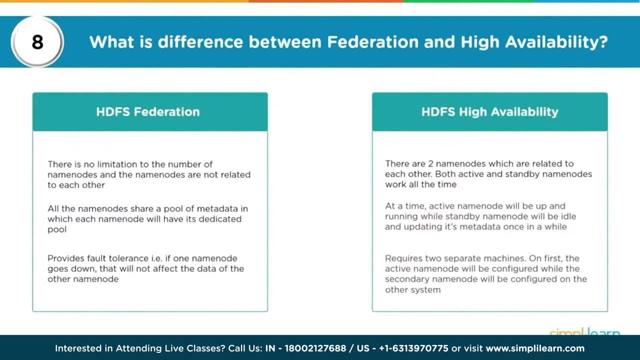 no limitation to the number of name nodes. Your name nodes are in a federated cluster, which basically means name nodes still belong to the same cluster but they are not coordinating with each other. So whenever a write request comes in one of the name node, 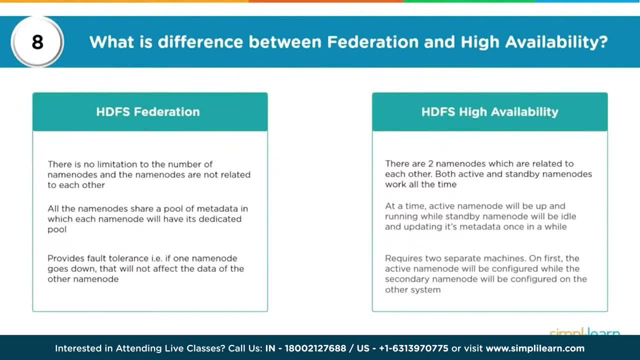 picks up that request and it guides that request for the blocks to be written on data nodes. But for this your name node does not have to coordinate with other name node to find out if the block ID which was being assigned was the same one as assigned by other name node. 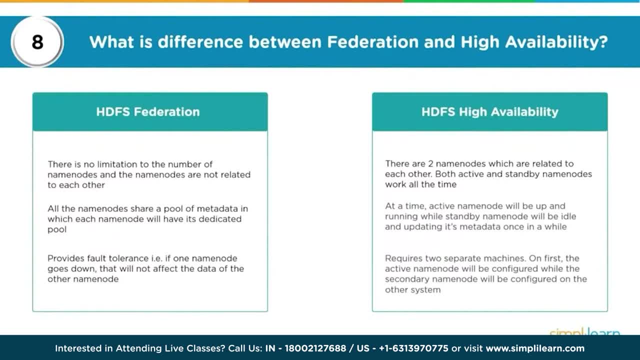 So all of them belong to a federated cluster. They are linked via a cluster ID. So whenever an application or an API is trying to talk to cluster, it is always going via an cluster ID and one of the name node would pick up the read. 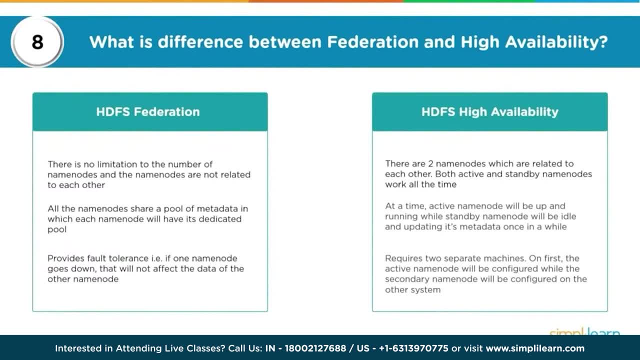 activity or write activity or processing activity. So all the name nodes are sharing a pool of metadata in which each name node will have its own dedicated pool, And we can remember that by a term called namespace or name service. So this also provides high fault tolerance. 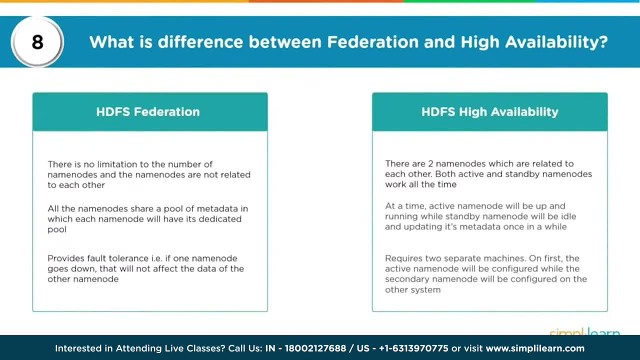 Suppose your one name node goes down, it will not affect or make your cluster unavailable. You will still have your cluster reachable because there are other name nodes running and they are available. Now, when it comes to heartbeats, all your data nodes- 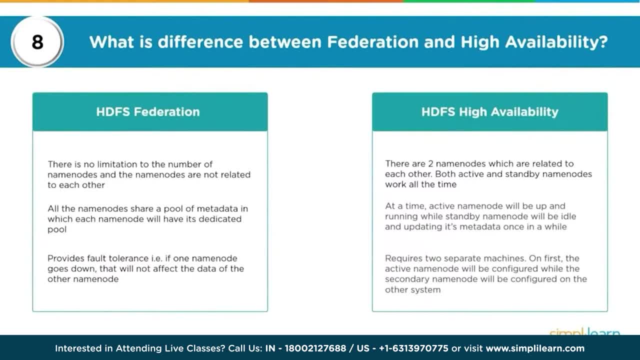 are sending their heartbeats to all the name nodes, And all the name nodes are aware of all the data nodes. When you talk about high availability, this is where you would only have two name nodes, So you would have an active and you would have a standby. Now, normally, 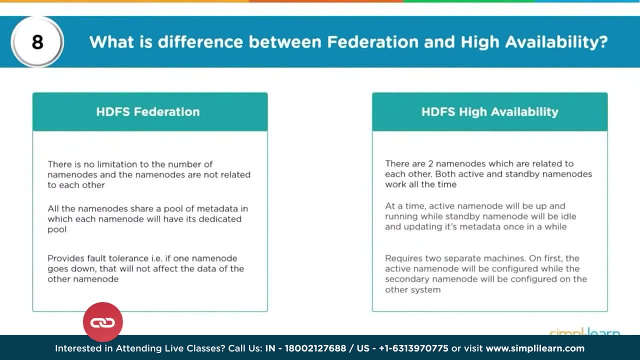 in any environment. you would see a high availability setup with Zookeeper. So Zookeeper is a centralized coordination service. So when you talk about your active and standby name nodes- election of a name node to be made as active and taking care of an automatic 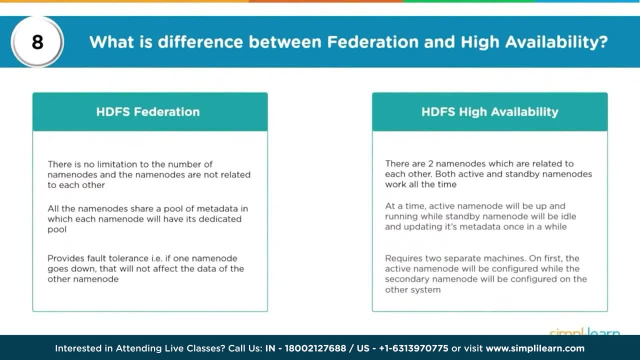 failover is done by your Zookeeper. High availability can be set up without Zookeeper, but that would mean that an admin's intervention would be required to make a name node as active from standby or also to take care of failover Now. 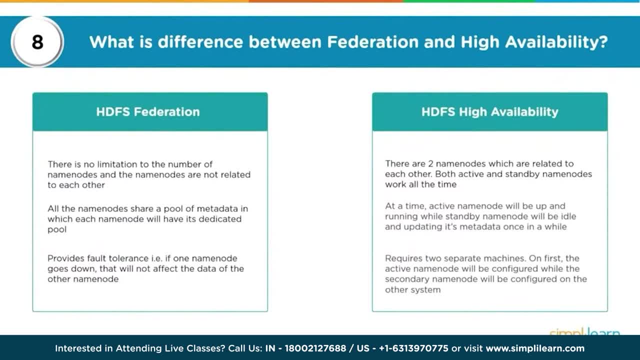 at any point of time in high availability. an active name node would be taking care of storing the edits about whatever updates are happening on SDFS and it is also writing these edits to a shared location. Standby name node is the one which is constantly. 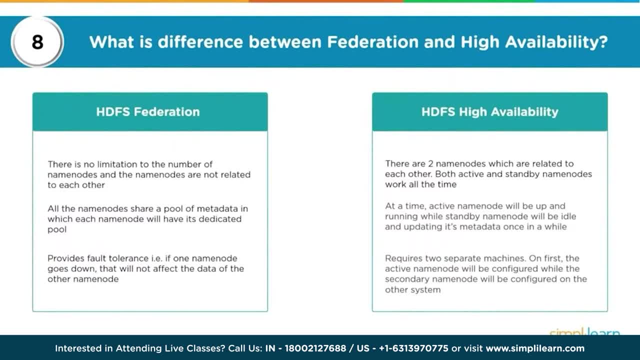 looking for these latest updates and applying to its metadata, which is actually a copy of whatever your active name node has. So in this way, your standby name node is always in sync with the active name node and if, for any reason, active name node fails, your 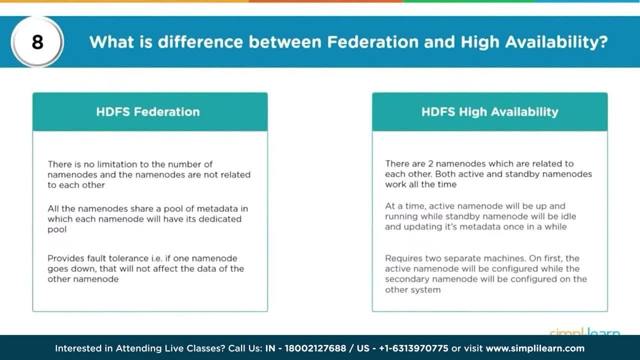 standby name node will take over and become the active. Remember, Zookeeper plays a very important role here. It's a centralized coordination service. One more thing to remember here is that in your high availability, secondary name node will not be allowed, So you would have an active name node. 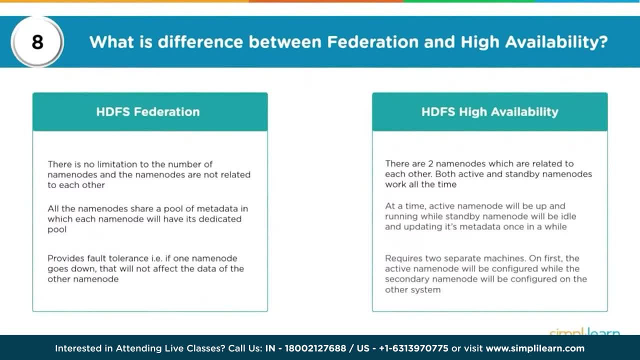 and then you will have a standby name node, which will be configured on a separate machine, and both of these will be having access to a shared location. Now, that shared location could be NFS, or it could be a quorum of general nodes. So for more, 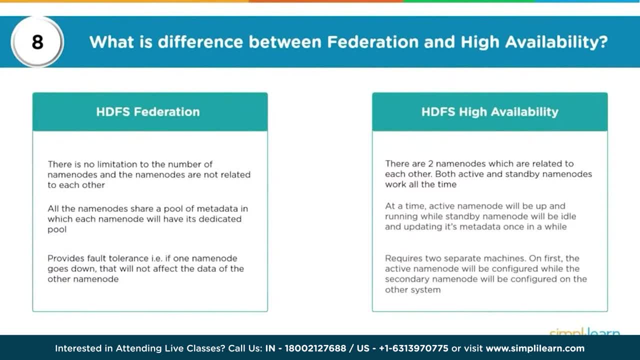 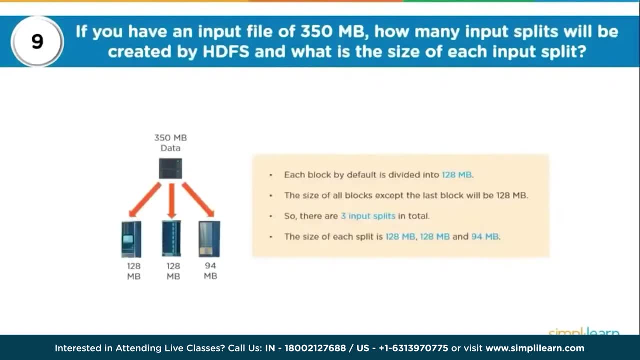 information. refer to the tutorial where I have explained about SDFS, high availability and federation. Now let's look at some logical question here. So if you have an input file of 350 MB, which is obviously bigger than 128 MB, how many input? 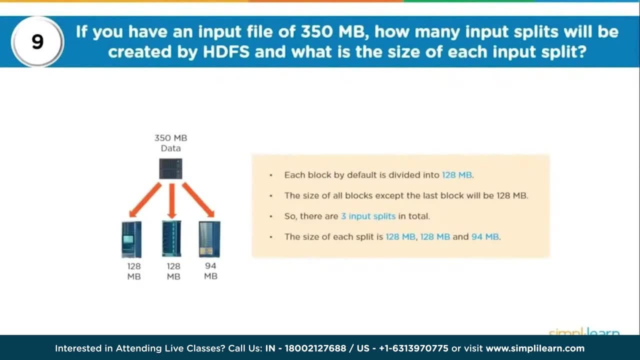 splits would be created by SDFS and what would be the size of each input split? So for this, you need to remember that by default, the minimum block size is 128 MB. Now that's customizable If your environment has more number. 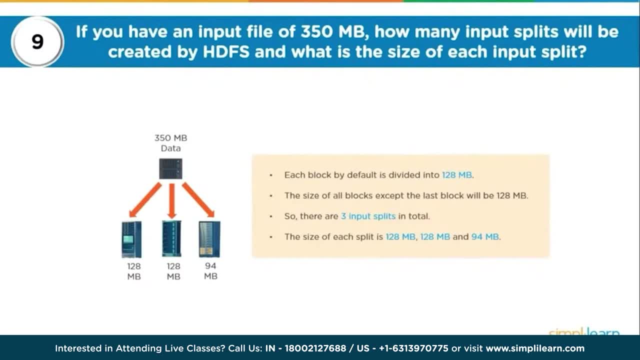 of larger files written on an average, then obviously you have to go for a bigger block size. If your environment has lot of files being written but these files are of smaller size, you could be okay with 128 MB. Remember, in Hadoop every. 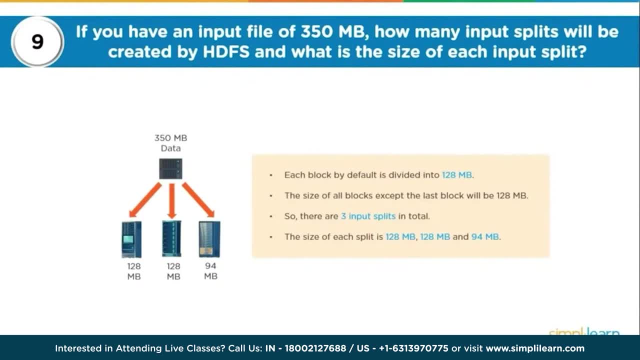 entity, that is, your directory on SDFS, file on SDFS and a file having multiple blocks. each of these are considered as objects and for each object Hadoop's name, node's RAM, 150 bytes, is utilized. So if your block, 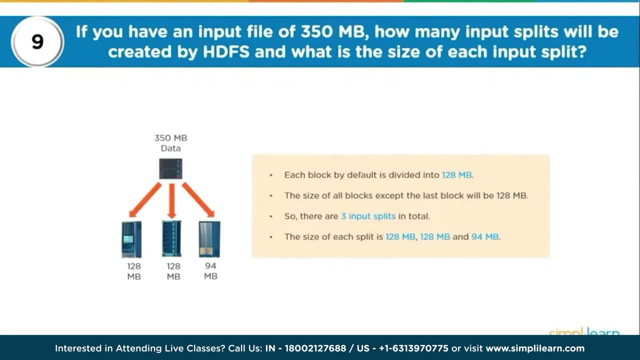 size is very small, then you would have more number of blocks which would directly affect the name node's RAM. If you keep a block size very high, that will reduce the number of blocks, but remember that might affect in processing because processing also depends on splits. 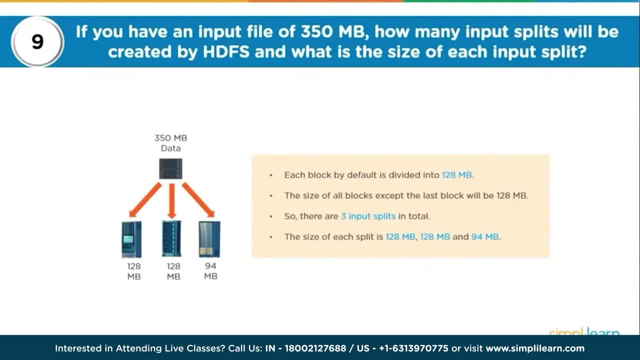 More number of splits, more the parallel processing. So setting of block size has to be done with consideration about your parallelism requirement and your name node's RAM, which is available. Now coming to the question, if you have a file of 350 MB, that would be split. 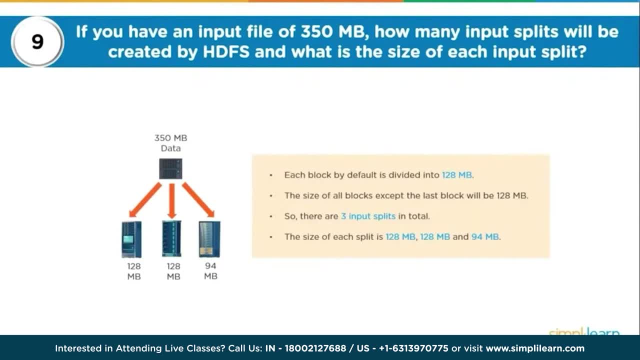 into three blocks, and here two blocks would have 128 MB data and the third block- although the block size would still be 128, it would have only 94 MB of data. So this would be the split of this particular file. Now let's. 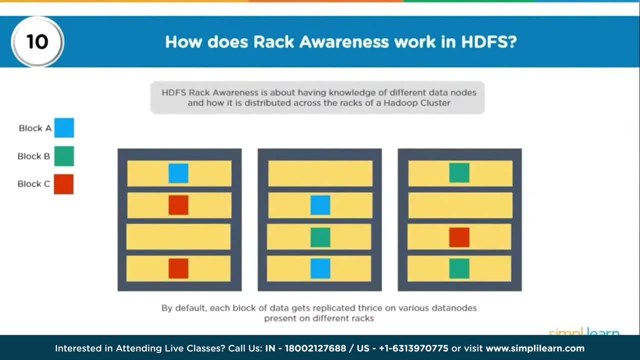 understand about rack awareness. How does rack awareness work? or why do we even have racks? So organizations always would want to place their nodes or machines in a systematic way. There can be different approaches. You could have a rack which would have machines running on the 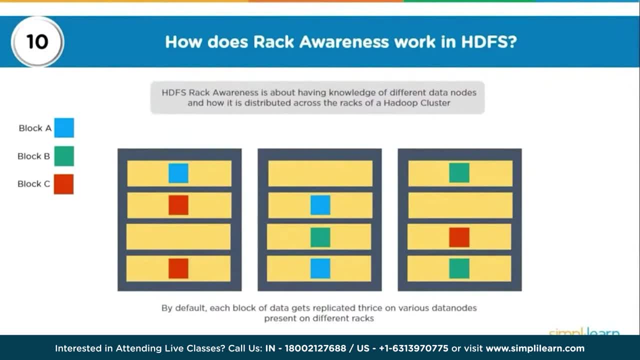 master processes and the intention would be that this particular rack could have higher bandwidth, more cooling, dedicated power supply, top of rack switch and so on. The second approach could be that you could have one master process running on one machine of every rack and 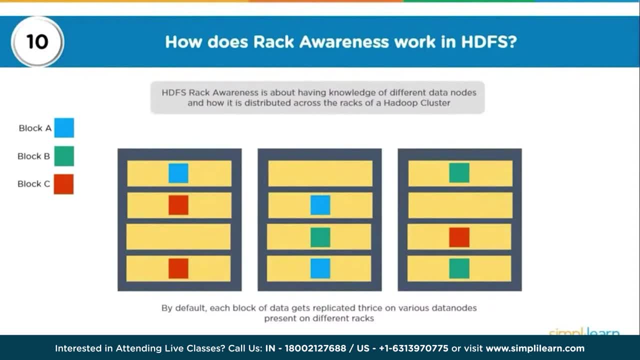 then you could have other slave processes running. Now, when you talk about your rack awareness, one thing to understand is that if your machines are placed within racks- and we are aware that Hadoop follows auto-replication, the rule of replication in a 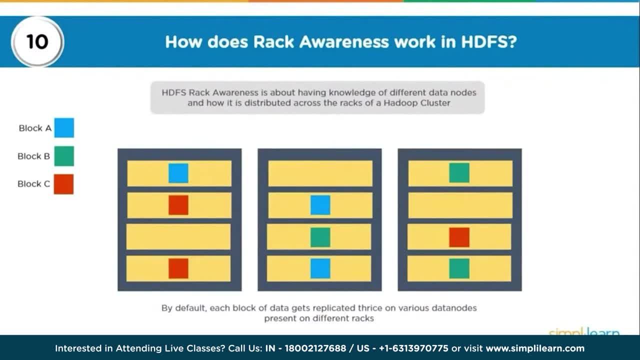 rack-aware cluster would be that you would never have all the replicas placed on the same rack. So if we look at this, if we have block A in blue color, you will never have all the three blue boxes in the same rack, even if they. 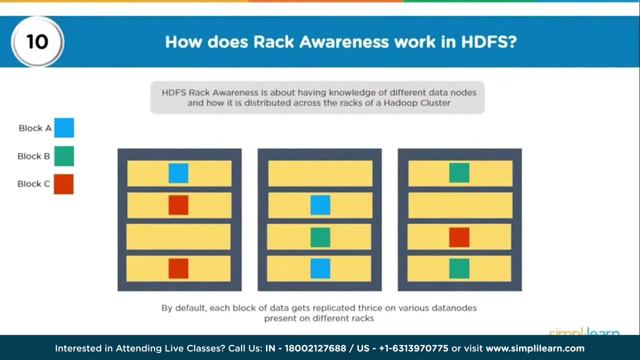 are on different nodes, because that makes us- that makes it- less fault tolerant. So you would have at least one copy of block which would be stored on a different rack on a different node. Now let's look at this. So, basically, here we are talking about 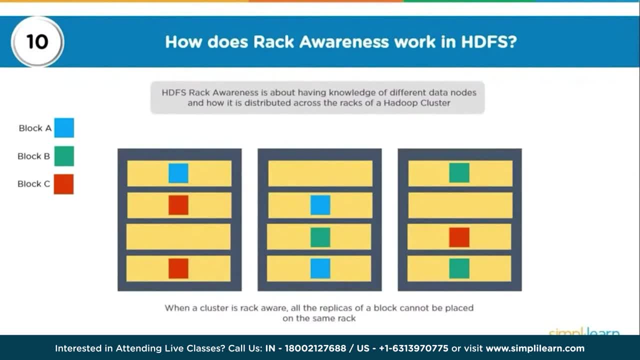 replicas being placed in such a way. Now somebody could ask a question: can I have my block and its replicas spread across three racks? And yes, you can do that, but then, in order to make it more redundant, you are increasing your bandwidth requirement. 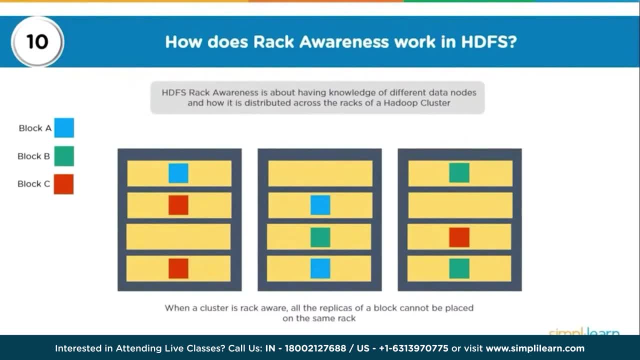 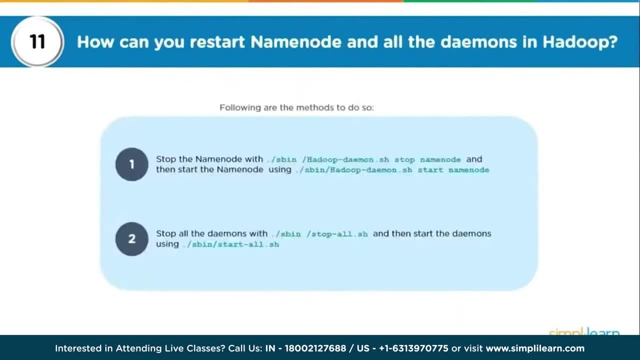 So the better approach would be two blocks on the same rack on different machines and one copy on a different rack. Now let's proceed. How can you restart name node and all daemons in Hadoop? So if you were working on an Apache Hadoop? 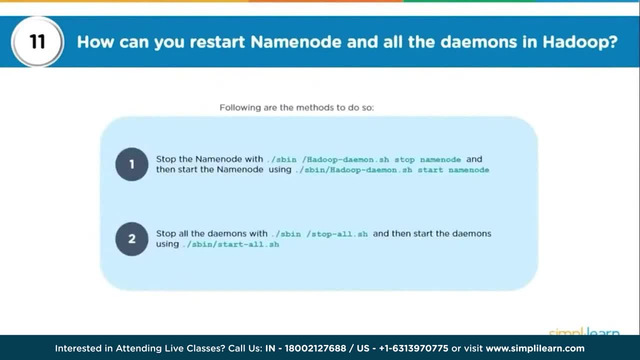 cluster, then you could be doing a start and stop using Hadoop daemon scripts. So there are these Hadoop daemon scripts which would be used to start and stop your Hadoop, And this is when you talk about your Apache Hadoop. So let's look at one. 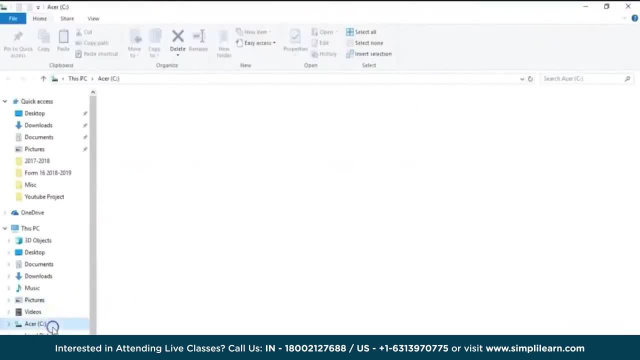 particular file which I would like to show you more information here, And this talks about your different clusters. So let's look into this. And so let's look at the start and stop, And here I have a file Let's look at. 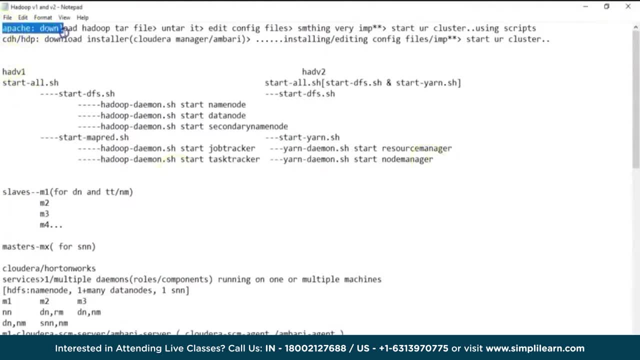 this one, And this gives you highlights. So if you talk about Apache Hadoop, this is how the setup would be done. So you would have it. download the Hadoop tarp file. You would have to untar it. edit. 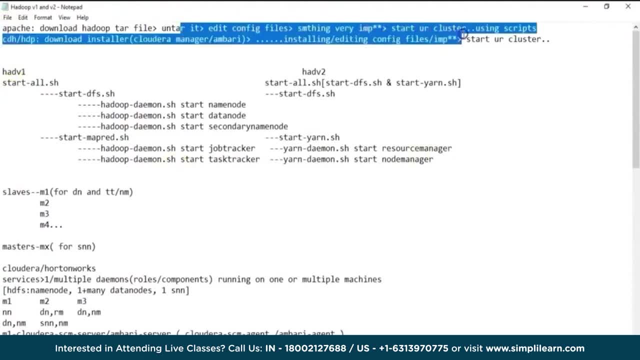 the config files, You would have to do formatting and then start your cluster. And here I have said using scripts, So this is in case of Apache Hadoop. you could be using a start all script that internally triggers start DFS and start yarn. 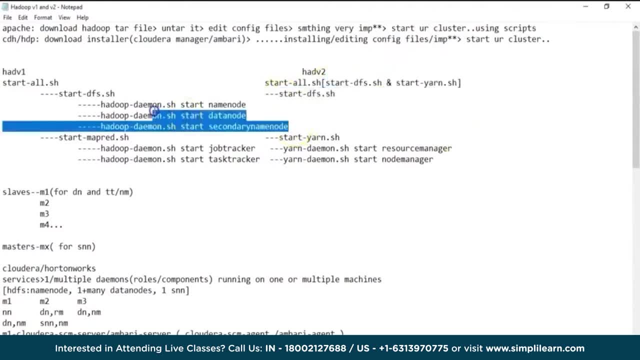 And these scripts start DFS internally would run Hadoop daemon multiple times based on your configs, to start your different processes. Then your start yarn would run yarn daemon script to start your processing related processes. So this is how it happens in Apache Hadoop. 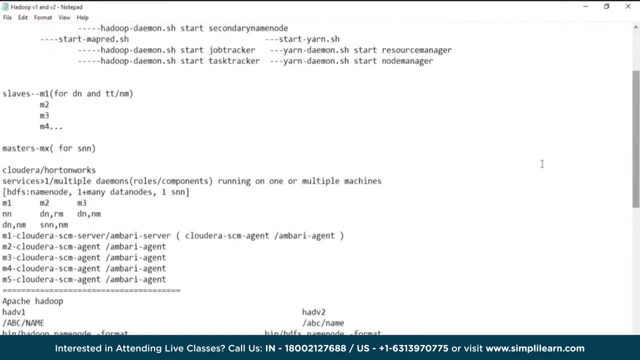 Now, in case of Cloudera or Hortonworks, which is basically a vendor, specific distribution, you would have, say, multiple services which would have one or multiple daemons running across the machines. Let's take an example here that you would have machine 1, machine 2. 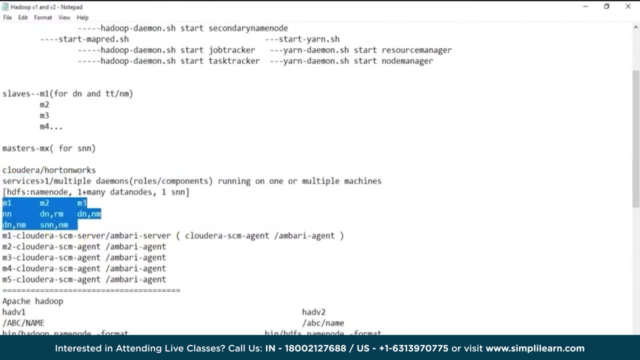 and machine 3, with your processes spread across. However, in case of Cloudera and Hortonworks, these are cluster management solutions, So you would never be involved in running a script individually to start and stop your processes. In fact, in case of Cloudera, 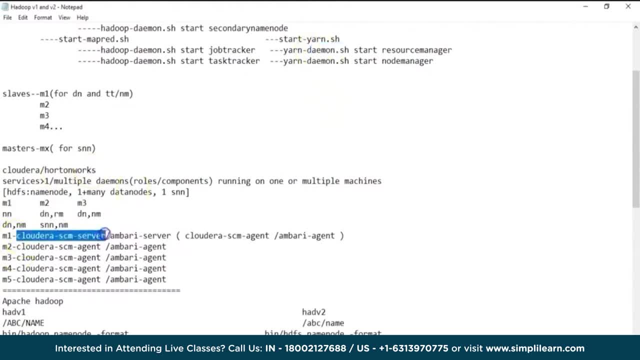 you would have a Cloudera SCM server running on one of the machines and then Cloudera SCM agents running on every machine. If you talk about Hortonworks, you would have Ambari server and Ambari agent running. So your agents. 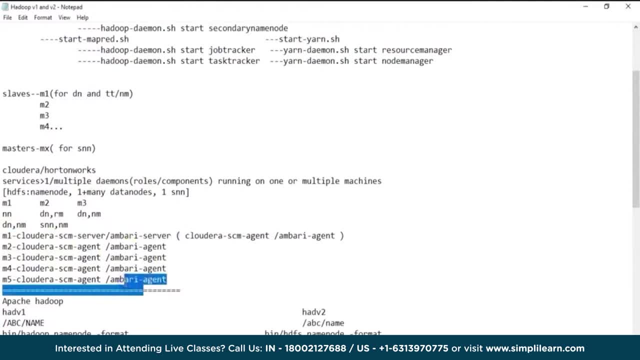 which are running on every machine, are responsible to monitor the processes, send also their heartbeat to the master. that is your server. And your server is the one, or a service, which basically will give instructions to the agents. So in case of vendor specific distribution, your start and stop. 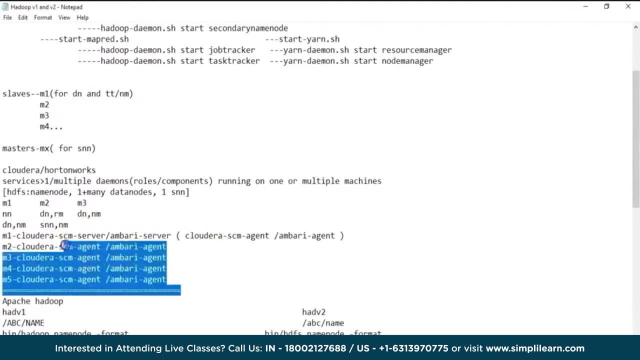 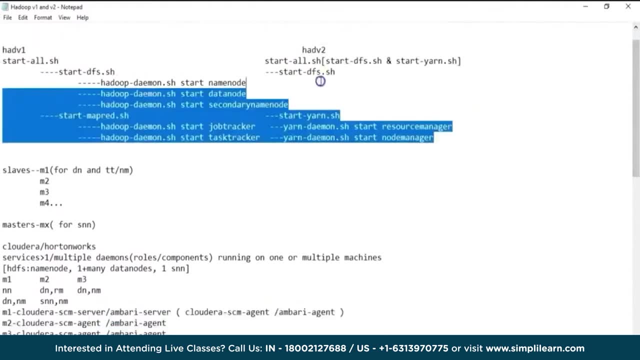 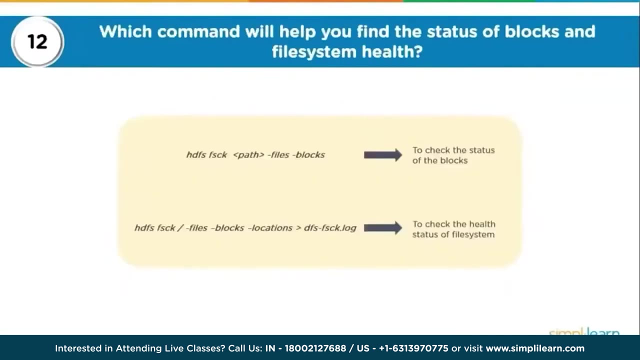 of processes is automatically taken care by these underlying services, And these services internally are still running these commands, However only in Apache Hadoop. you have to manually follow these to start and stop Coming back. we can look into some command related questions. So which command? 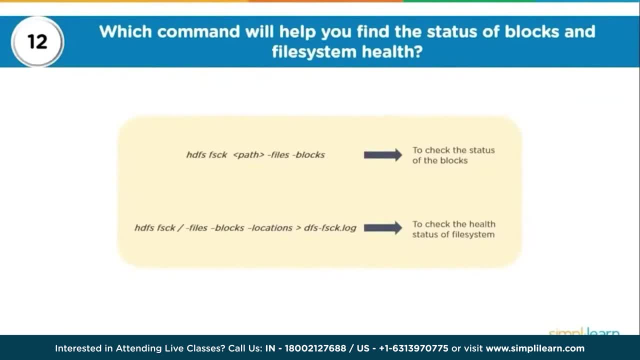 will help you find the status of blocks and file system health. So you can always go for a file system check command Now that can show you the files for a particular HDFS path. It can show you the blocks and it can also. 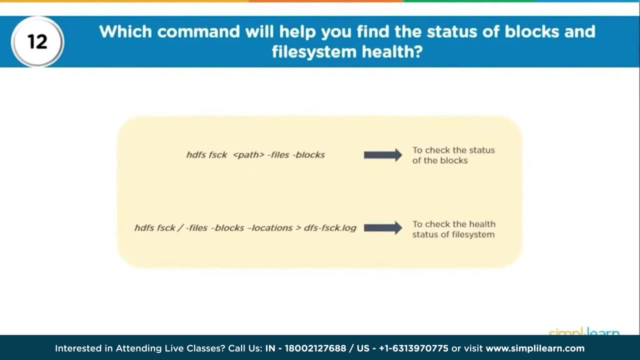 give you information on status, such as under-replicated blocks, over-replicated blocks, mis-replicated blocks, default replication and so on. So your FSCK file system check utility does not repair if there is any problem with the blocks, But it can give you information. 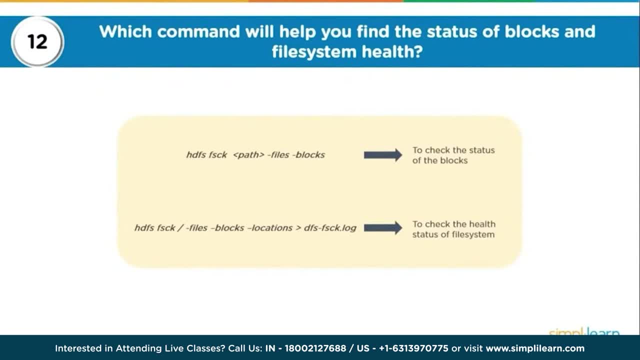 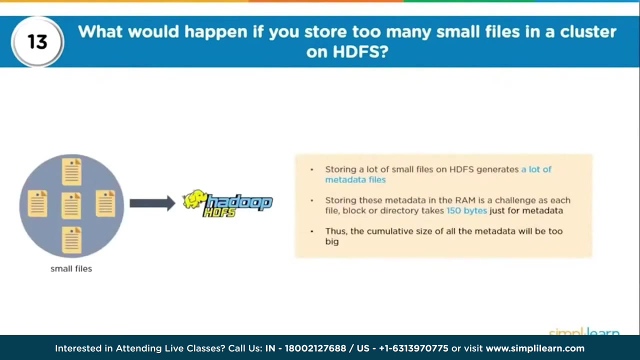 of blocks related to the files on which machines they are stored, if they are replicated as per the replication factor or if there is any problem with any particular replica. Now, what would happen if you store too many small files in a cluster, And this relates to the 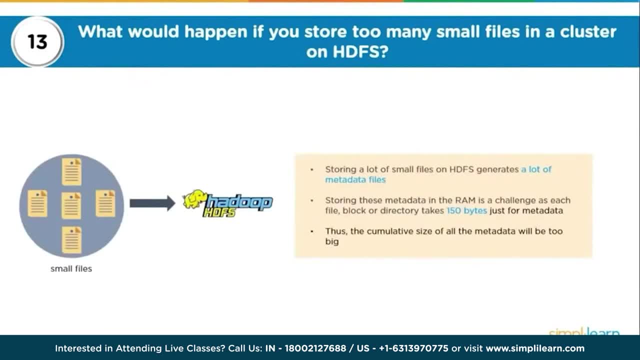 block information which I gave some time back. So remember, Hadoop is coded in Java, So here every directory, every file and file related block is considered as an object, And for every object within your Hadoop cluster NameNodes, RAM gets utilized. 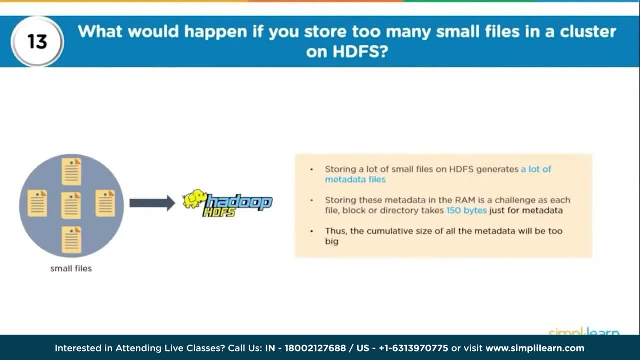 So more number of blocks you have, more would be usage of NameNodes RAM And if you are storing too many small files, it would not affect your disk, It would directly affect your NameNodes RAM. That's why in production clusters, admin guys or 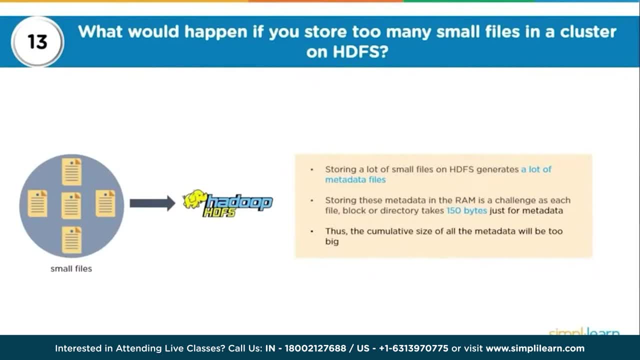 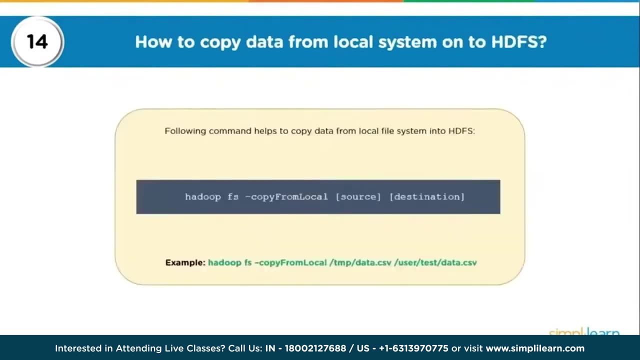 infrastructure specialist will take care that everyone who is writing data to HDFS follows a quota system, so that you could be controlled in the amount of data you write plus the count of data and individual writes on HDFS. Now how do you copy data from local system onto? 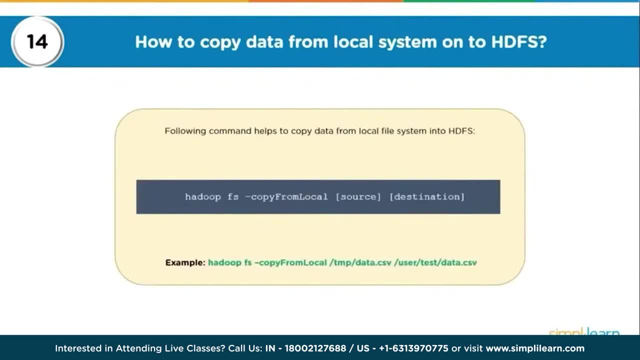 HDFS So you can use a put command or a copy from local and then given your local path, which is your source, and then your destination, which is your HDFS path. Remember, you can always do a copy from local using a minus F option. 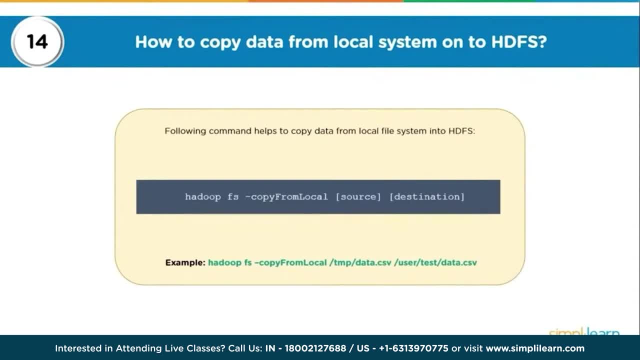 that's a flag option and that also helps you in writing the same file or a new file to HDFS. So with your minus F you have a chance of overwriting or rewriting the data which is existing on HDFS. So copy from local or minus put. 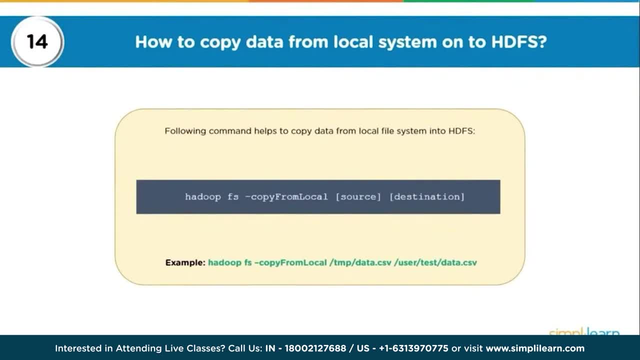 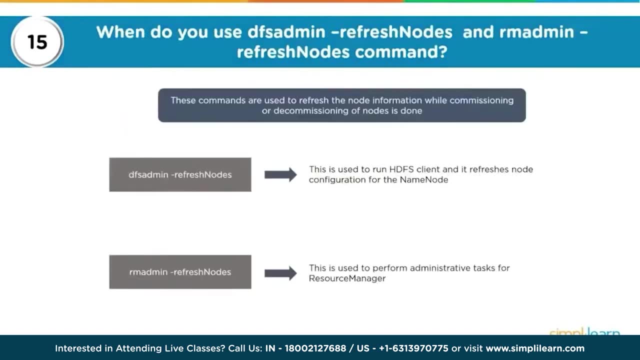 Both of them do the same thing and you can also pass an argument when you are copying to control your replication or other aspects of your file. Now, when do you use DFS admin Refresh nodes or the RMAdmin to refresh nodes, So as the 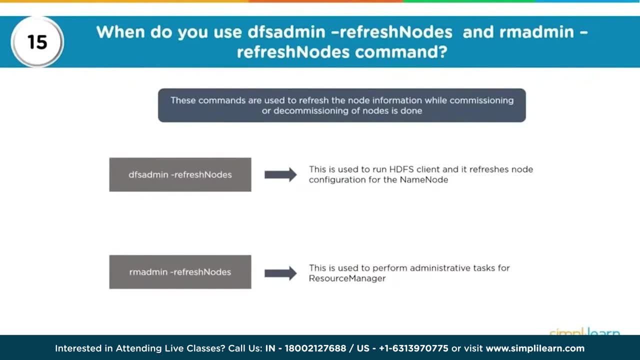 command says this is basically to do with refreshing the node information. So your refresh nodes is mainly used when, say, a commissioning or decommissioning of nodes is done, So when a node is added into the cluster or when a node is removed from. 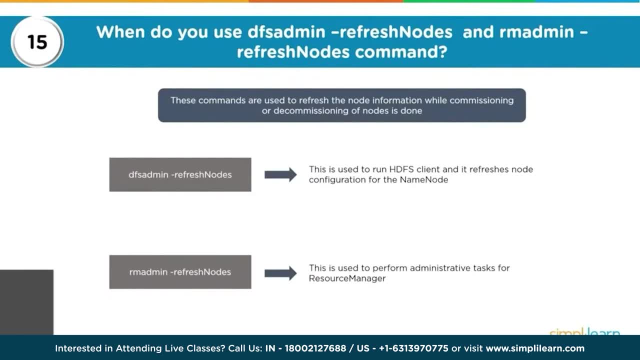 the cluster. you are actually informing Hadoop master that this particular node would not be used for storage and would not be used for processing. Now, in that case, you would be. once you are done with the process of commissioning or decommissioning, you would be. 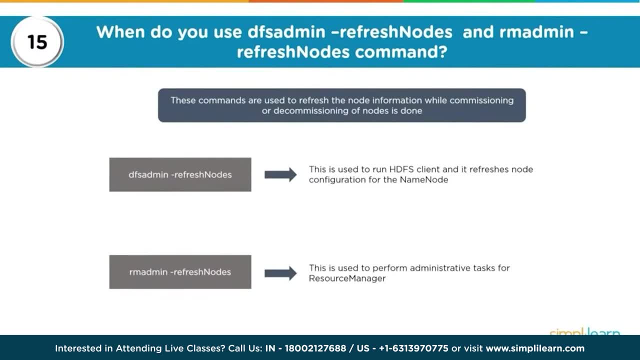 giving these commands, that is, refresh nodes and RMAdmin refresh nodes. So internally, when you talk about commissioning decommissioning, there are include and exclude files which are updated and these include and exclude files will have entry of machines which are being added to the cluster. 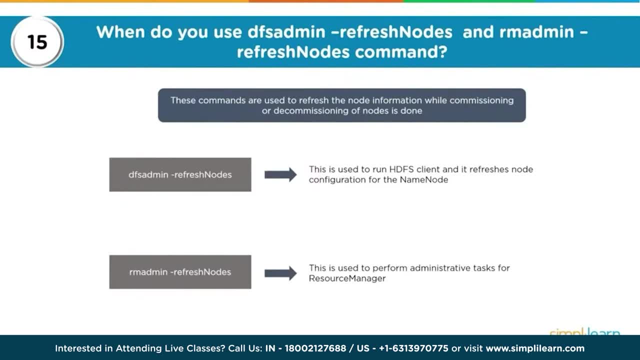 or machines which are being removed from the cluster, and while this is being done, the cluster is still running, So you do not have to restart your master process. However, you can just use these refresh commands to take care of your commissioning decommissioning. 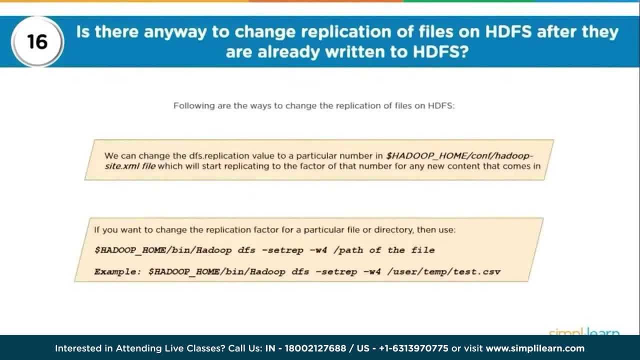 activities. Now, is there any way to change replication of files on HDFS after they are already written? And the answer is, of course, yes. So if you would want to set a replication factor at a cluster level and if you have admin access, then 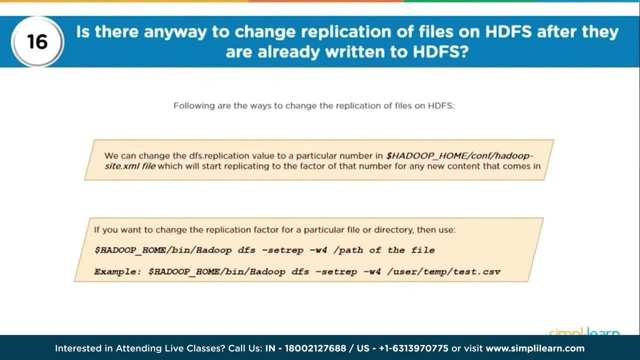 you could edit your HDFS-site file or you could say Hadoop-site file, and that would take care of replication factor being set at a cluster level. However, if you would want to change the replication after the data has been written, you could always use a. 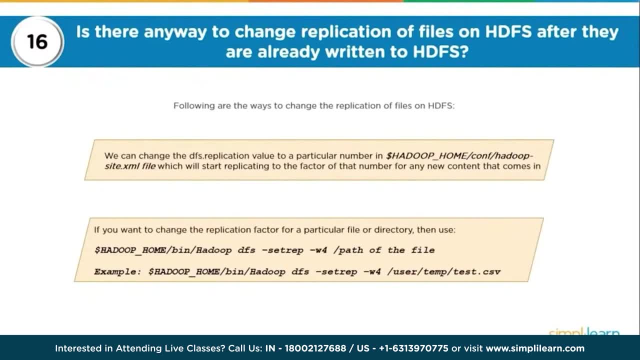 setrep command. So setrep command is basically to change the replication after the data is written. You could also write the data with a different replication and for that you could use a "-d dfsreplication and give your replication factor when you are writing data to the. 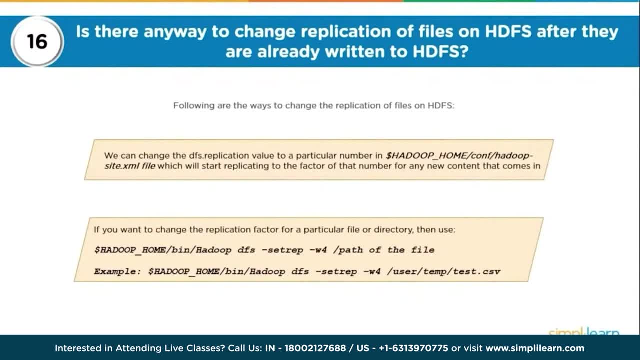 cluster. So in Hadoop you can let your data be replicated as per the property set in the config file. You could write the data with a different replication. You could change the replication after the data is written. So all these options are available. 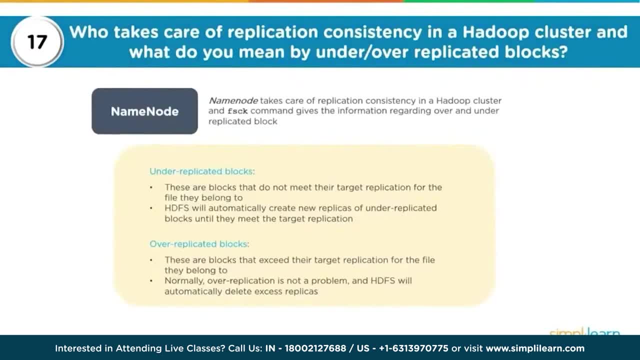 Now, who takes care of replication consistency in a Hadoop cluster, and what do you mean by under replicated blocks? Now, as I mentioned, your fsck command can give you information of over or under replicated blocks. Now, in a cluster, it is always and always. 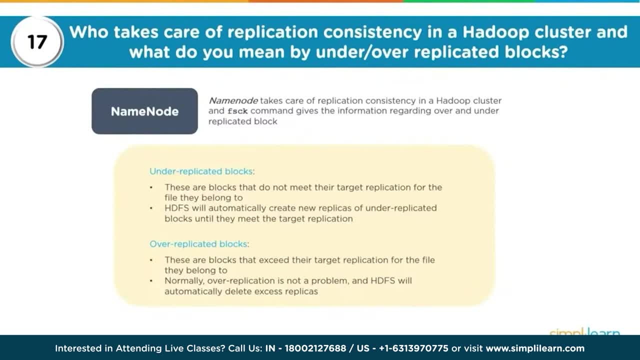 named node which takes care of replication consistency. So, for example, if you have set up a replication of three and since we know the first rule of replication, which basically means that you can not have two replicas residing on the same node, it would mean that if your replication 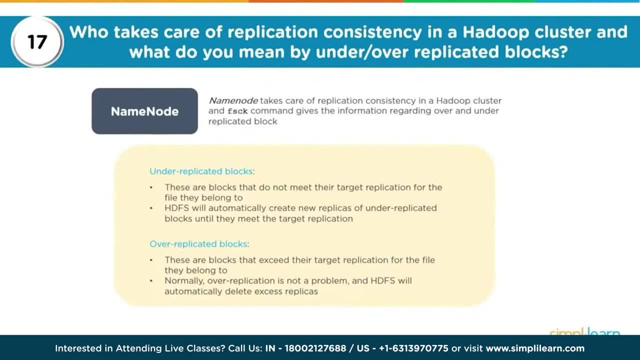 is three, you would need at least three data nodes available. Now say, for example, you had a cluster with three nodes and replication was set to three. At one point of time one of your name node crashed and if that happens, your blocks. 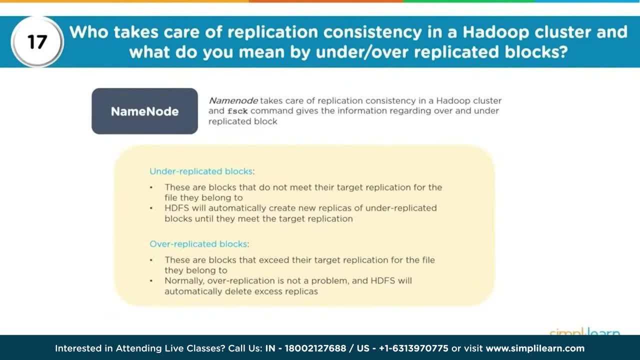 would be under replicated. That means there was a replication factor set, but now your blocks are not replicated or there are not enough replicas as per the replication factor set. This is not a problem. Your master process or name node will wait for some time before it will start. 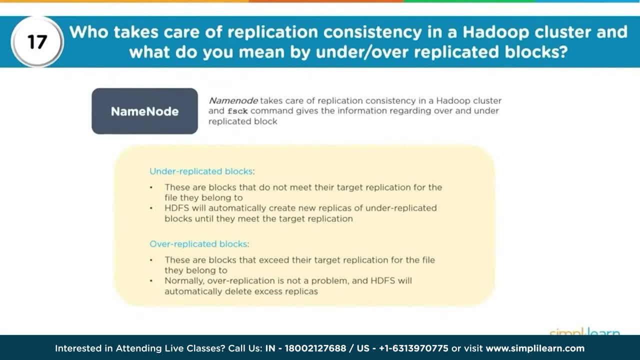 the replication of data again. So if a data node is not responding or if a disk has crashed and if name node does not get information of a replica, name node will wait for some time and then it will start re-replication of those missing blocks. 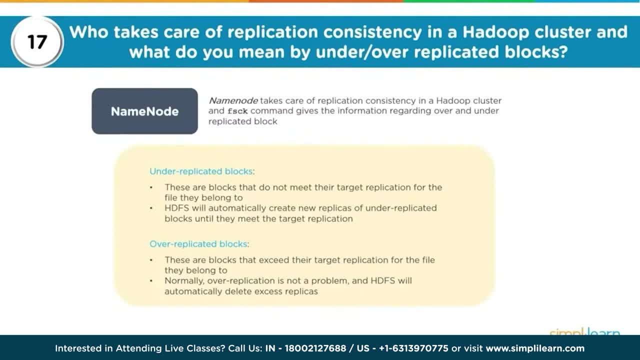 from the available nodes. However, while name node is doing it, the blocks are in under replicated situation. Now, when you talk about over replicated, this is a situation where name node realizes that there are extra copies of block. Now, this might be the case. 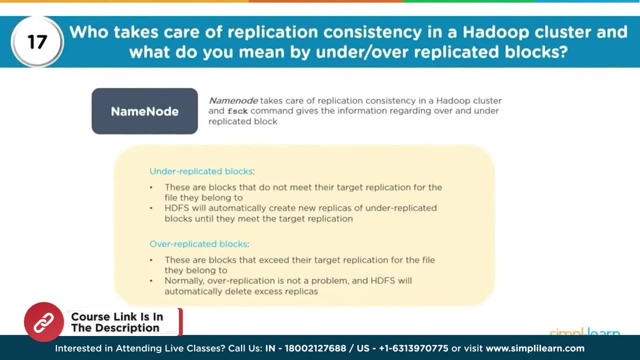 that you had three nodes running with a replication of three. One of the node went down due to a network failure or some other issue. Within few minutes, name node re-replicated the data and then the failed node is back with its set of blocks. 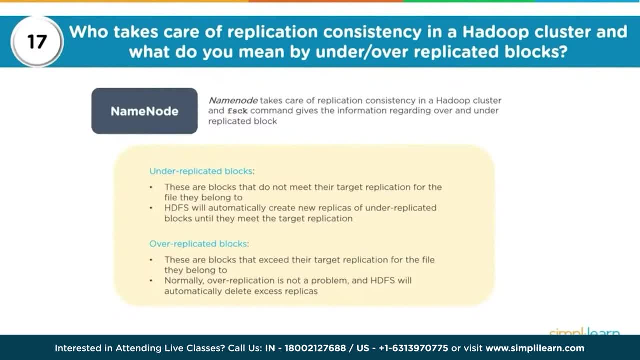 Again, name node is smart enough to understand that this is an over replication situation and it will delete set of blocks from one of the nodes. It might be the node which has been recently added, It might be your old node which has joined your cluster again, or 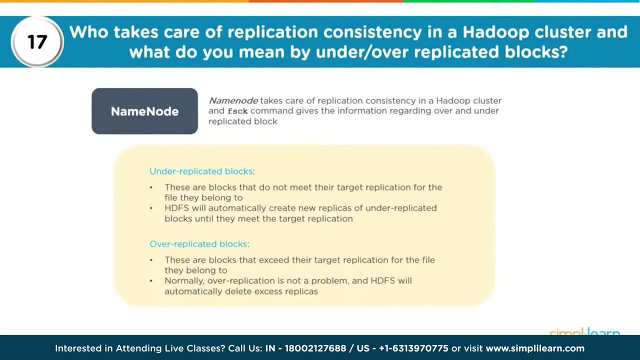 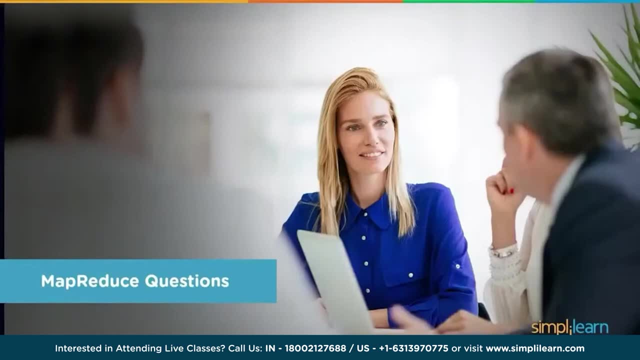 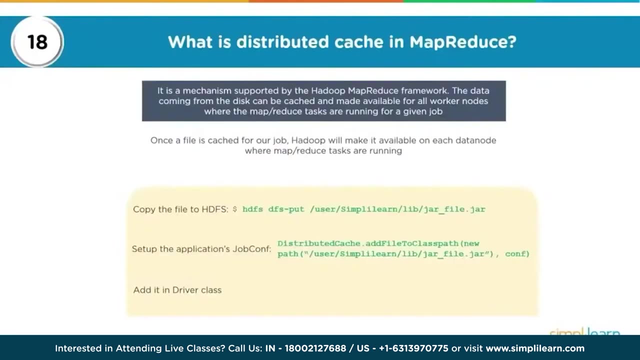 any node. That depends on the load on a particular node. Now we discussed about Hadoop. We discussed about SDFS. Now we will discuss about MapReduce, which is the programming model and, you can say, processing framework. What is distributed cache in MapReduce? Now we know. 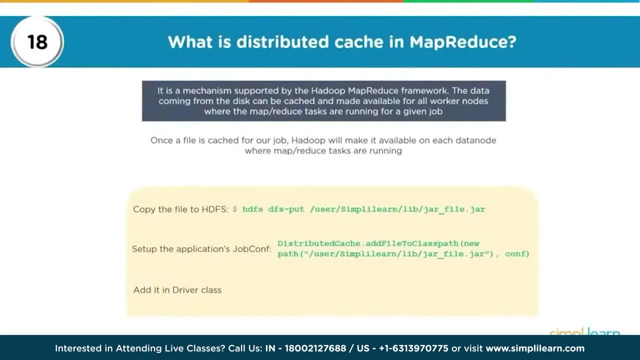 that when we talk about MapReduce, the data which has to be processed might be existing on multiple nodes. So when you would have your MapReduce program running, it would basically read the data from the underlying disks. Now this could be a costly 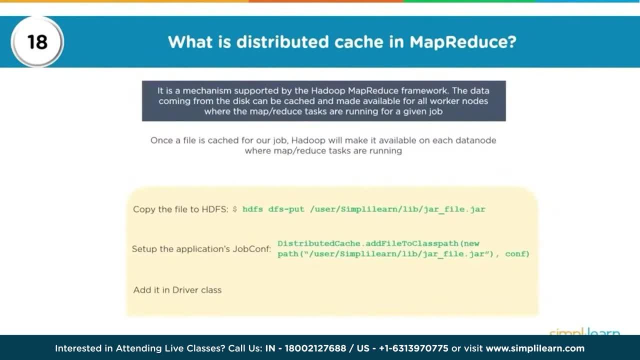 operation if every time the data has to be read from disk. So distributed cache is a mechanism wherein data set or data which is coming from the disk can be cached and available for all worker nodes. Now how will this benefit? So when a MapReduce 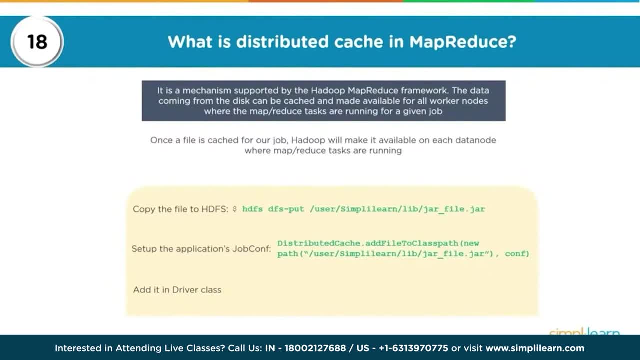 is running. instead of every time reading the data from disk, it would pick up the data from distributed cache and this will benefit your MapReduce processing. So distributed cache can be set in your job conf, where you can specify that a file should be picked. 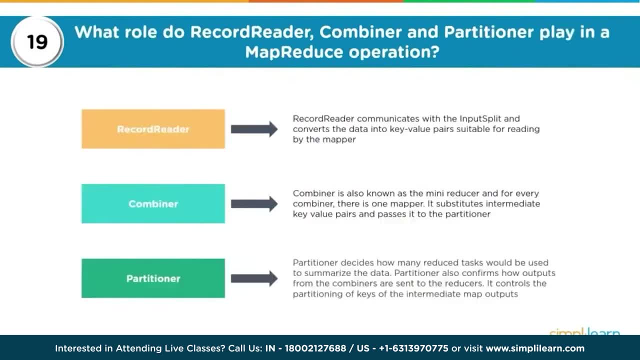 up from distributed cache. Now let's understand about these roles. So what is a record reader, What is a combiner, What is a partitioner, And what kind of roles do they play in a MapReduce processing paradigm or MapReduce operation? 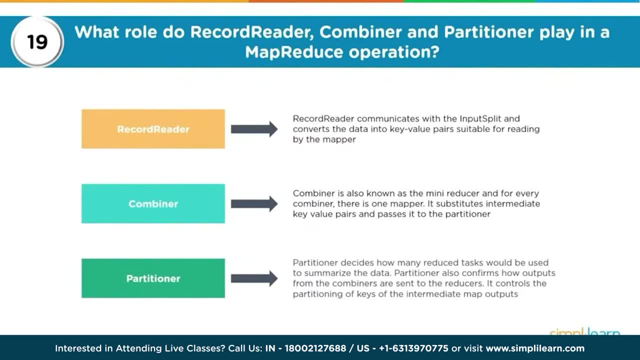 So record reader communicates with the input split and it basically converts the data into key value pairs, And these key value pairs are the ones which will be worked upon by the mapper. Your combiner is an optional phase. It's like a mini class, So combiner does not. 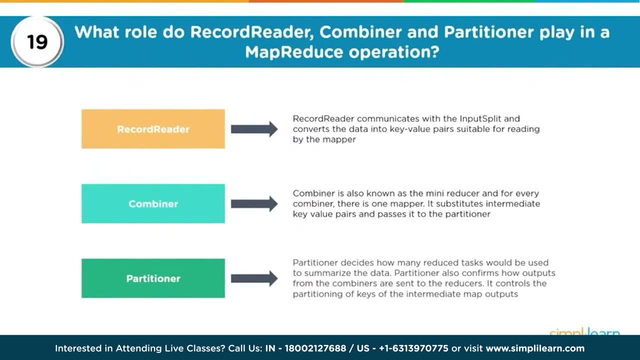 have its own class. It relies on the reducer class. Basically, your combiner would receive the data from your map tasks, which would have completed works on it, based on whatever reducer class mentions, and then passes its output to the reducer phase Partitioner. 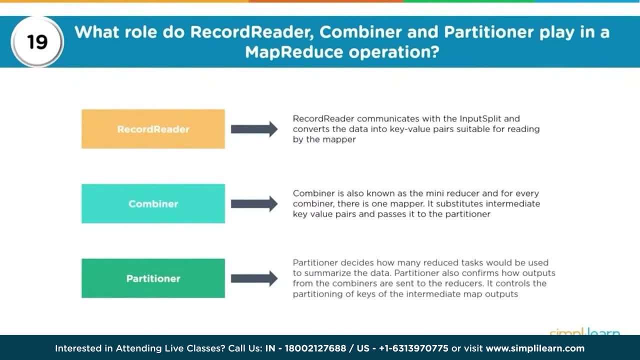 is basically a phase which decides how many reduced tasks would be used, aggregate or summarize your data. So partitioner is a phase which would decide based on the number of keys, based on the number of map tasks, Your partitioner would decide if. 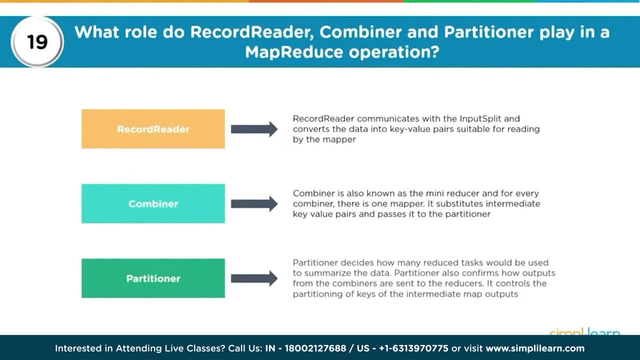 one or multiple reduced tasks would be used to take care of processing. So either it could be partitioner which decides on how many reduced tasks would run, or it could be based on the properties which we have set within the cluster which will take care of the. 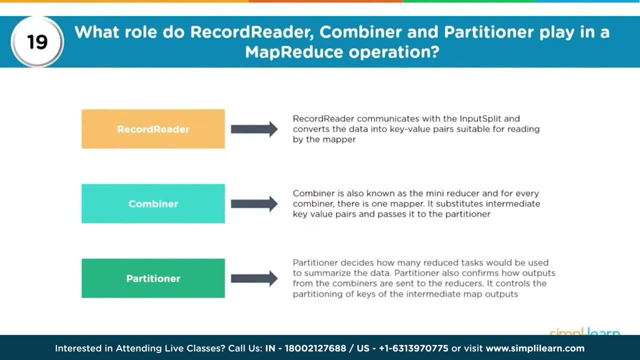 number of reduced tasks which would be used. Always remember, your partitioner decides how outputs from combiner are sent to reducer and to how many reducers. It controls the partitioning of keys of your intermediate map outputs. So map phase, whatever output it generates, is an. 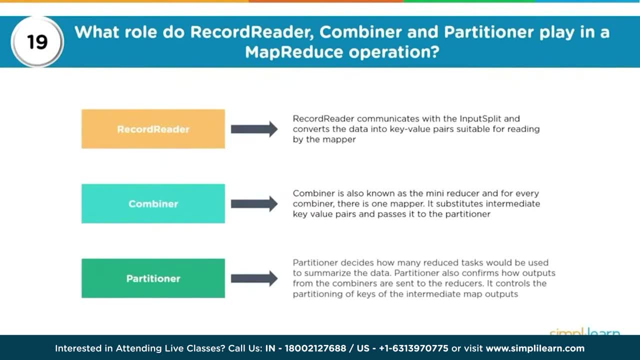 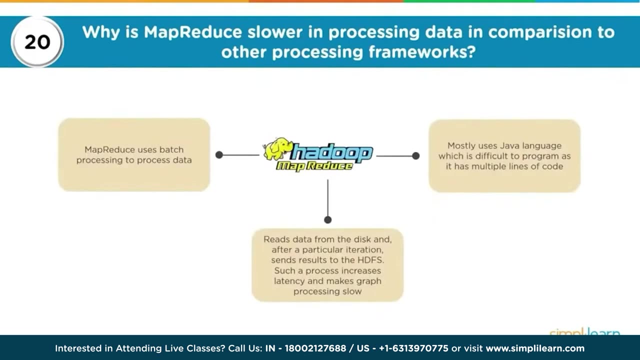 intermediate output and that has to be taken by your partitioner or by a combiner and then partitioner to be sent to one or multiple reduced tasks. This is one of the common questions which you might face. Why is map reduce slower In processing? so we know map. 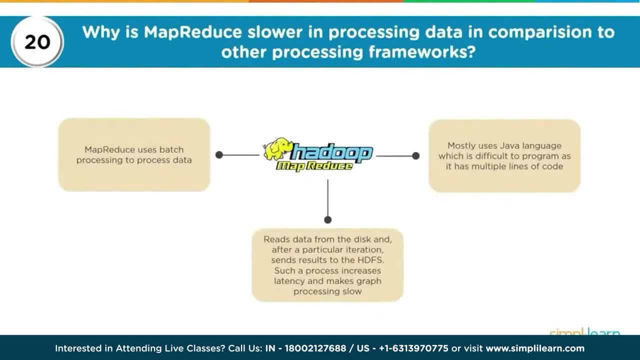 reduce goes for parallel processing. We know we can have multiple map tasks running on multiple nodes at the same time. We also know that multiple reduced tasks could be running Now why does then map reduce become a slower approach? First of all, your map reduce is: 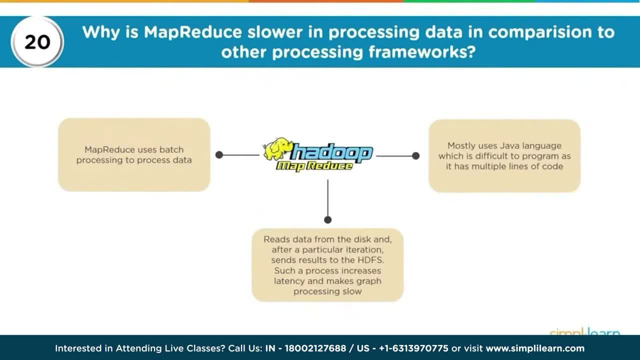 a batch oriented operation. Now, map reduce is very rigid and it strictly uses mapping and reducing phases. So no matter what kind of processing you would want to do, you would have to still provide the mapper function and the reducer function to work on data. 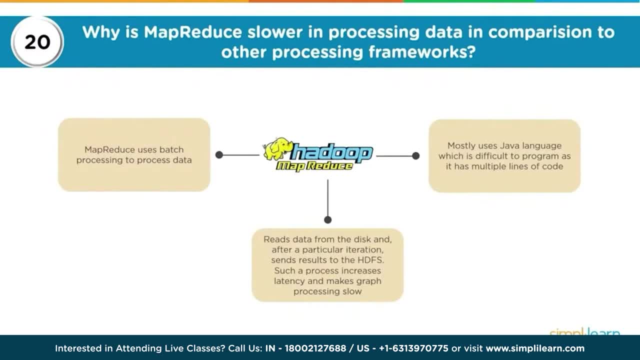 Not only this: whenever your map phase completes, the output of your map phase, which is an intermittent output, would be written to HDFS and thereafter underlying disks, And this data would then be shuffled and sorted and picked up for reducing phase. So, every time, your data 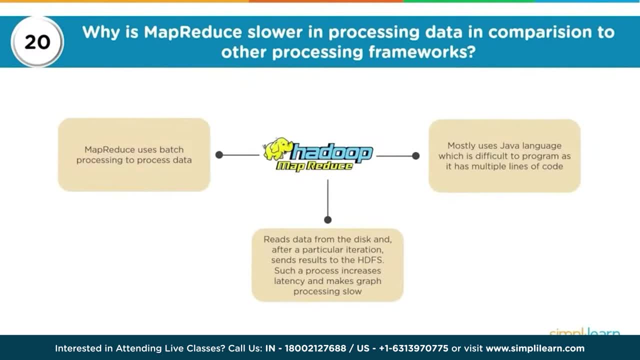 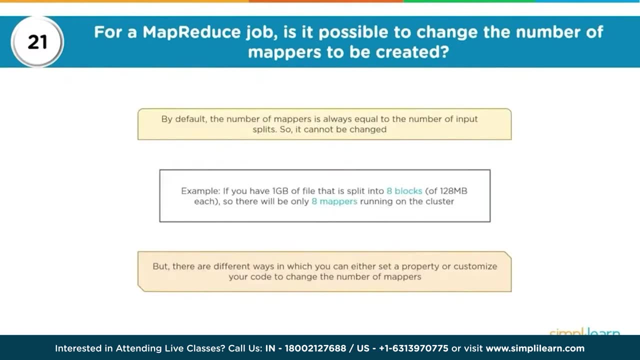 being written to HDFS and retrieved from HDFS makes map reduce a slower approach. The question is: for a map reduce job, is it possible to change the number of mappers to be created Now? by default, you cannot change the number of map tasks. 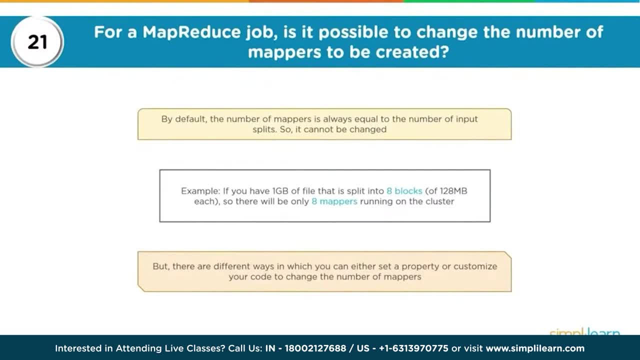 because number of map tasks depends on the input splits. However, there are different ways in which you can either set a property to have more number of map tasks which can be used, or you can customize your code or make it use a different format which can then control the number of 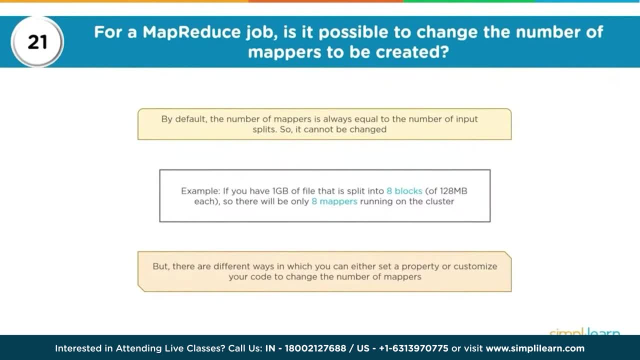 map tasks. By default, number of map tasks are equal to the number of splits of file you are processing. So if you have a 1 GB of file that is split into 8 blocks of 128 MB, there would be 8. 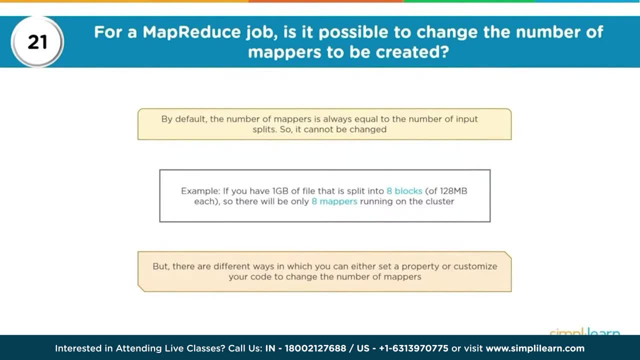 map tasks running on the cluster. These map tasks are basically running your mapper function. If you have hard coded properties in your mapper-site file to specify more number of map tasks, then you could control the number of map tasks. Let's also talk about some. 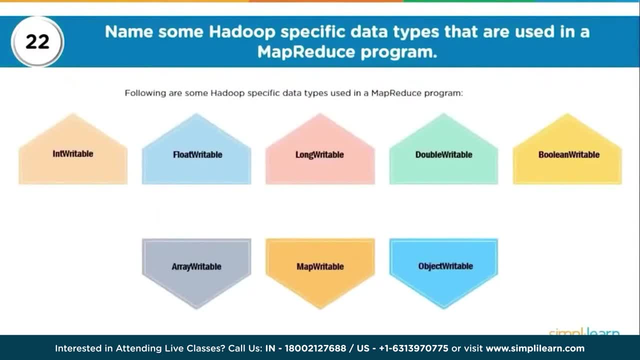 data types. So when you prepare for Hadoop, when you want to get into big data field, you should start learning about different data formats. Now there are different data formats, such as Avro Parquet. you have SQL sequence file or binary format. 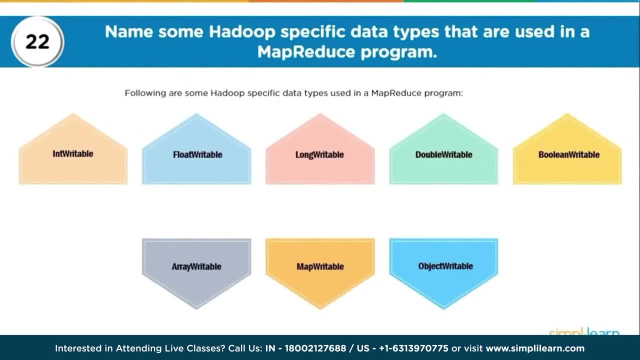 and these are different formats which are used. Now, when you talk about your data types in Hadoop, these are implementation of your writable and writable-comparable interfaces. So for every data type in Java, you have an equivalent in Hadoop, So int. 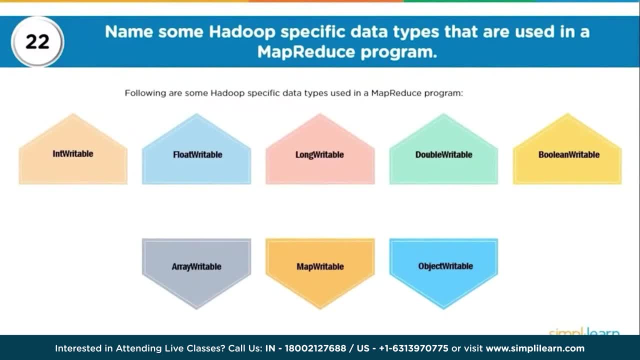 in Java would be int writable. in Hadoop, float would be float writable. long would be long writable, double writable, Boolean writable, array writable, map writable and object writable. So these are your different data types that could be used within your MapReduce program. 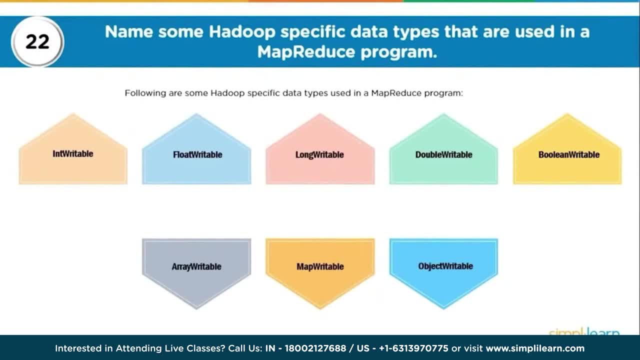 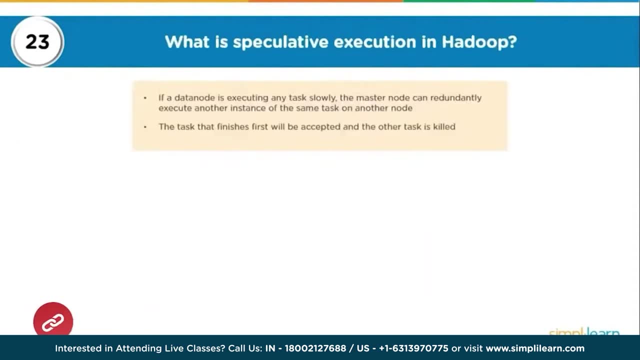 And these are implementation of writable and writable, comparable interfaces. What is speculative execution? Now imagine you have a cluster which has huge number of nodes and your data is spread across multiple slave machines or multiple nodes. Now, at a point of time, due to a disk degrade, 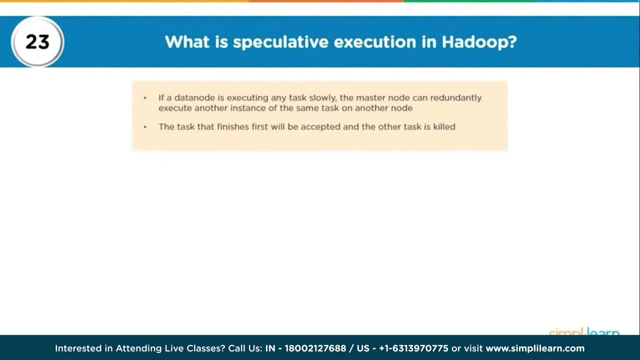 or network issues or machine heating up or more load being on a particular node, there can be a situation where your data node will execute task in a slower manner. Now, in this case, if speculative execution is turned on, there would be a shadow task or 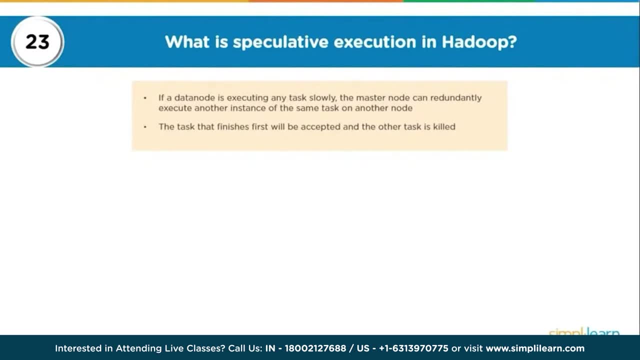 another similar task running on some other node for the same processing. So whichever task finishes first will be accepted and the other task would be killed. So speculative execution could be good if you are working in an intensive workload kind of environment where if a particular 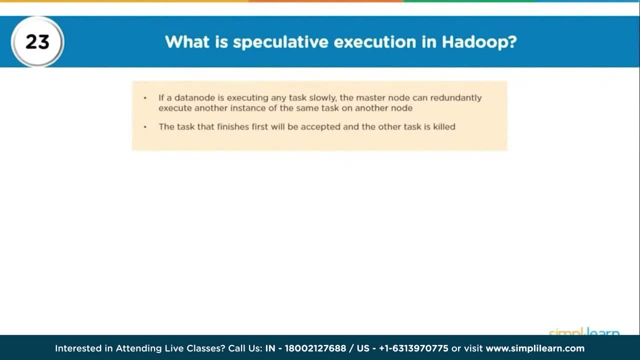 node is slower, you could benefit from an unoccupied or a node which has less load to take care of your processing Going further. this is how we can understand. So node A, which might be having a slower task, you would have a scheduler which is maintaining. 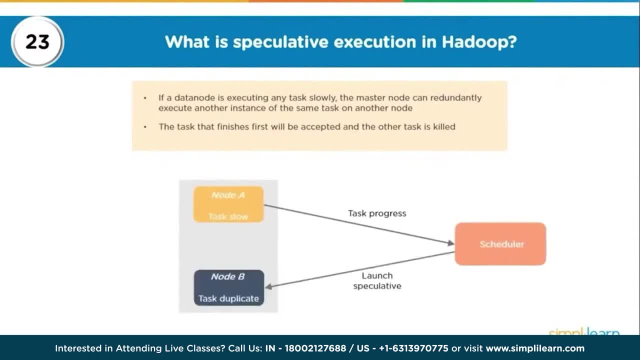 or having knowledge of what are the resources available. So if speculative execution as a property is turned on, then the task which was running slow, a copy of that task or you can say shadow task, would run on some other node and whichever task completes first. 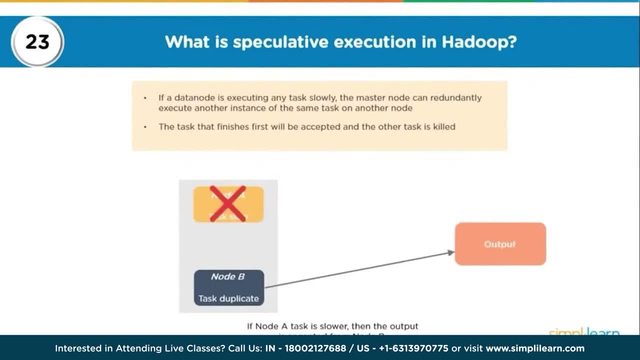 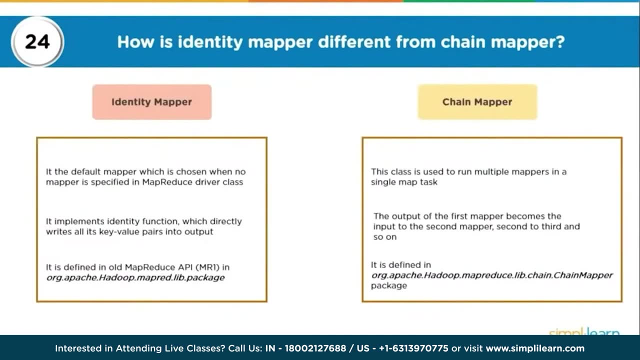 will be considered. This is what happens in your speculative execution. Now, how is identity mapper different from chain mapper? Now, this is where we are getting deeper into MapReduce concepts. So when you talk about mapper, identity mapper is the default. 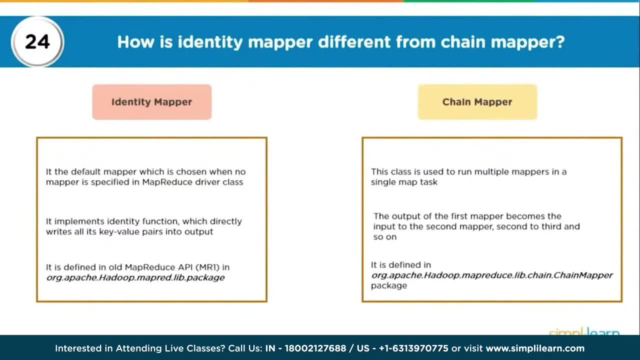 mapper which is chosen when no mapper is specified in MapReduce driver class. So for every MapReduce program you would have a map class which is taking care of your mapping phase, which basically has a mapper function and which would run one or multiple map tasks. 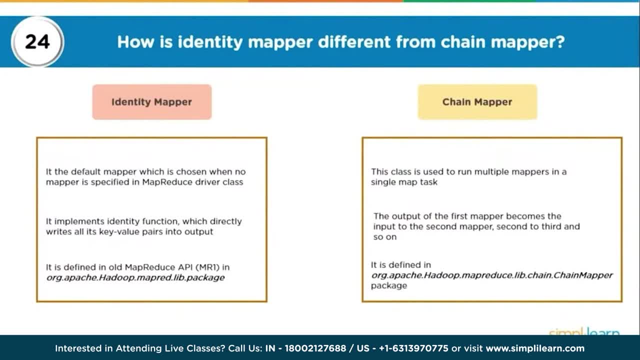 Your programming. your program would also have a reduce class, which would be running a reducer function which takes care of reduce tasks running on multiple nodes. Now, if a mapper is not specified within your driver class, so driver class is something which has all information about your 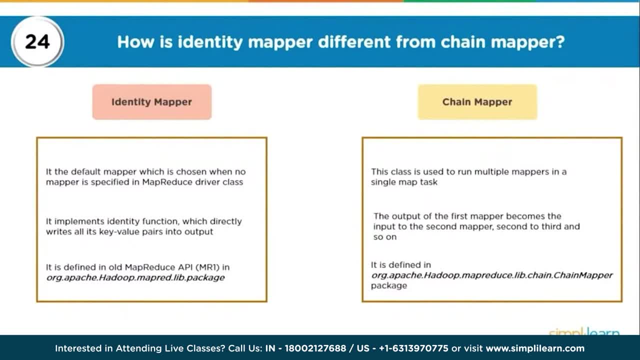 flow. What's your map class? What is your reduce class? What's your input format? What's your output format? What are the job configurations and so on? So identity mapper is the default mapper which is chosen when no mapper class is mentioned. 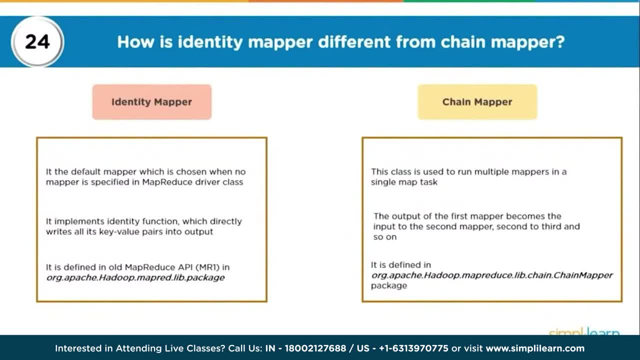 in your driver class. It basically implements an identity function which directly writes all its key pairs into output, and it was defined in old MapReduce API in this particular package. But when you talk about chaining mappers or chain mapper, this is basically a class. 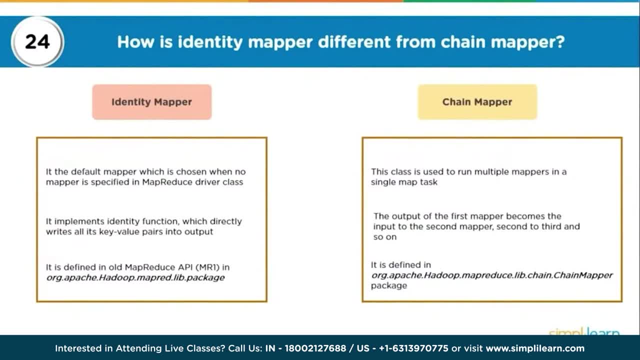 to run multiple mappers in a single map task, or basically you could say multiple map tasks would run as a part of your processing. The output of first mapper would become as an input to second mapper and so on, and this can be defined in the under mentioned. 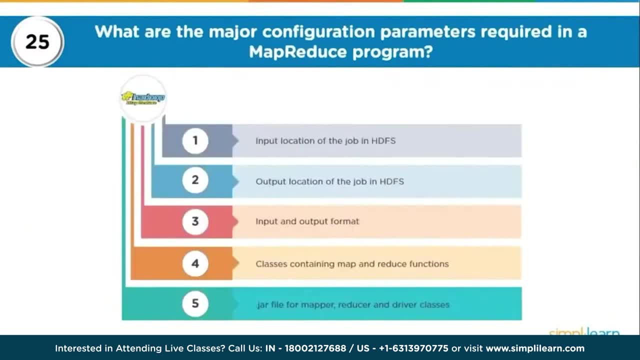 class or package. What are the major configuration parameters required in a MapReduce program? Obviously, we need to have the input location. We need to have the output location. So input location is where the files will be picked up from, and this would preferably on SDFS. 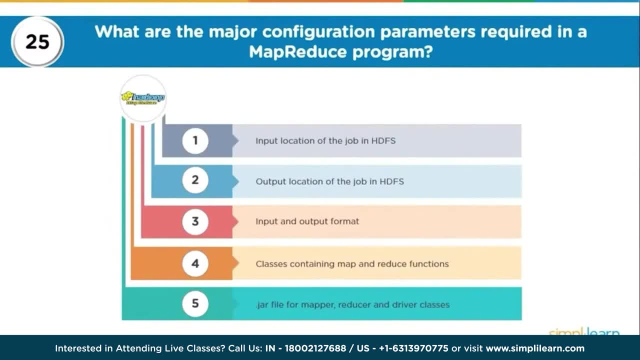 directory Output location is the path where your job output would be written by your MapReduce program. You also need to specify input and output formats. If you don't specify, the defaults are considered, Then we need to also have the classes which have your map and reduce. 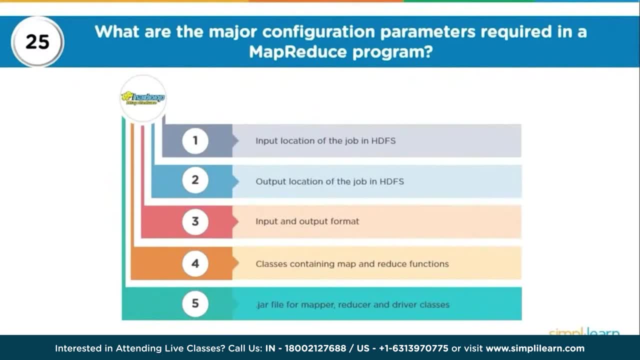 functions, and if you intend to run the code on a cluster, you need to package your class in a jar file, export it to your cluster and then this jar file would have your mapper reducer and driver classes. So these are important configuration parameters. 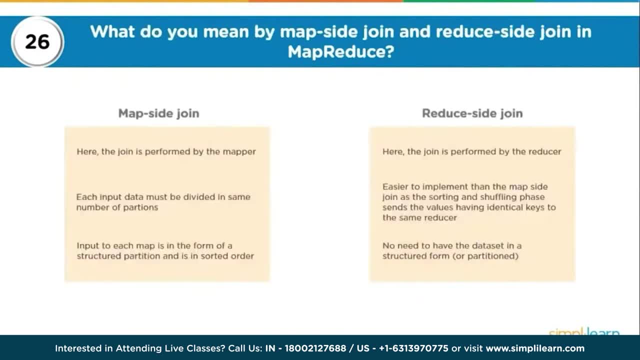 which you need to consider for a MapReduce program. Now, what is the difference or what do you mean by MapSideJoin and ReduceSideJoin? MapSideJoin is basically when the join is performed at the mapping level or at the mapping phase, or is performed by the mapper. 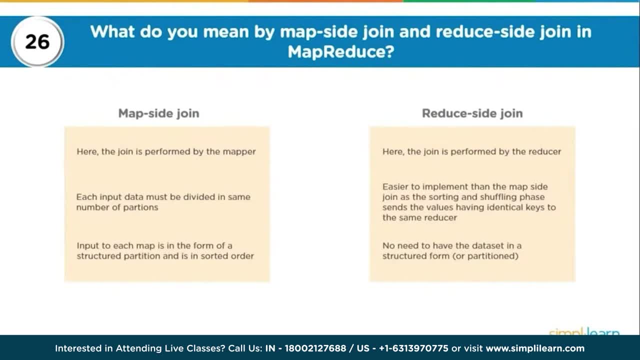 So each input data which is being worked upon has to be divided into same number of partitions. Input to each map is in the form of a structured partition and is in sorted order. So, MapSideJoin, you can understand it in a simpler way that, if you compare it with 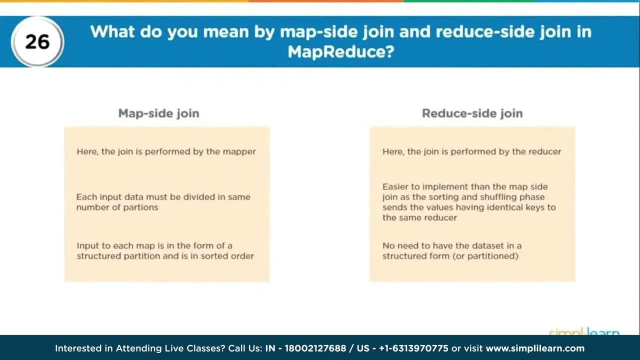 RDBMS concepts where you had two tables which were being joined. It will always be advisable to give your bigger table as the left side table or the first table for your join condition and it would be your smaller table on the left side and your bigger table. 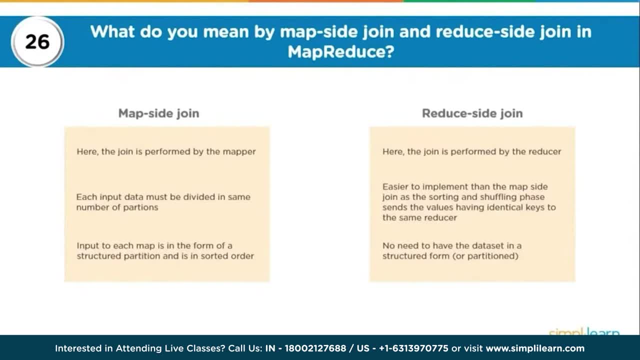 on the right side, which basically means the smaller table could be loaded in memory and could be used for joining. So MapSideJoin is a similar kind of mechanism where input data is divided into same number of partitions. When you talk about ReduceSideJoin, 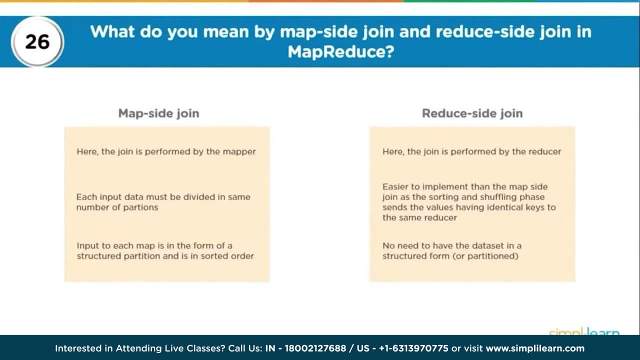 here the join is performed by the reducer, So it is easier to implement than MapSideJoin, as all the sorting and shuffling will send the values, or send all the values having identical keys to the same reducer, So you don't need to have your data set. 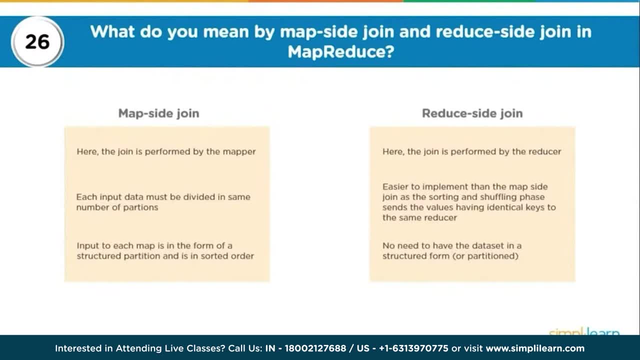 in a structured form. So look into your MapSideJoin or ReduceSideJoin and other joins just to understand how MapReduce works. However, I would suggest not to focus more on this, because MapReduce is still being used for processing, but the amount of MapReduce 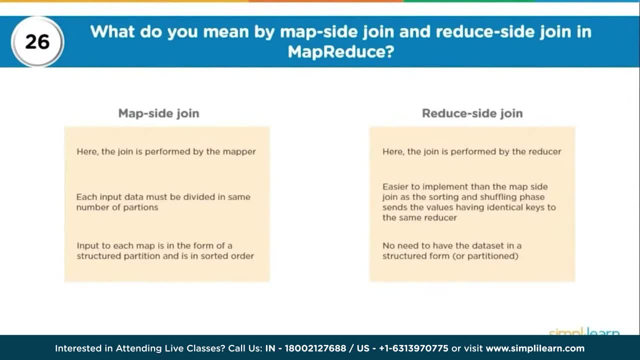 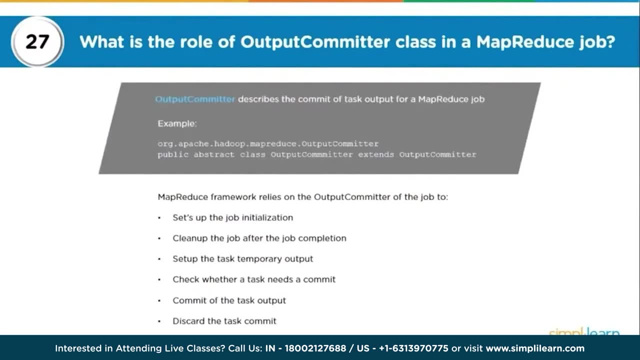 based processing has decreased overall or across the industry. Now what is the role of OutputCommitter class in a MapReduce job? So OutputCommitter, as the name says, describes the commit of task output for a MapReduce job. So we could. 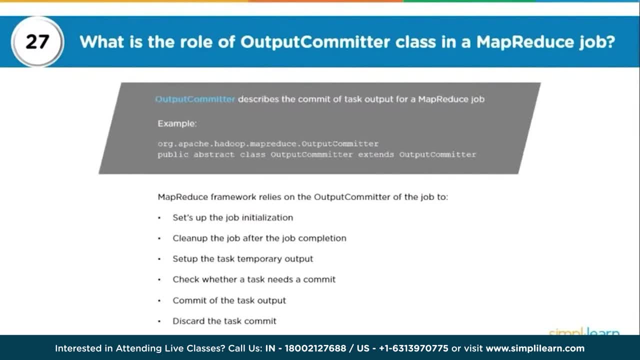 have this as mentioned, or Apache, Hadoop, MapReduce, OutputCommitter. You could have a class which extends your OutputCommitter class. So MapReduce relies on this. MapReduce relies on the OutputCommitter of the job to set up the job. 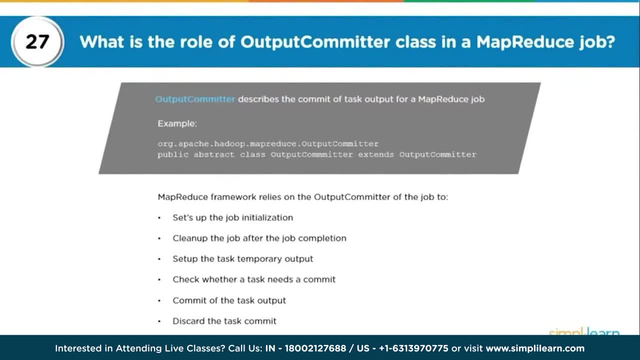 initialization, cleaning up the job after the job completion. that means all the resources which were being used by a particular job: setting up the task, temporary output, checking whether a task needs a commit, committing the task output and discarding the task output. So this is a very important class. 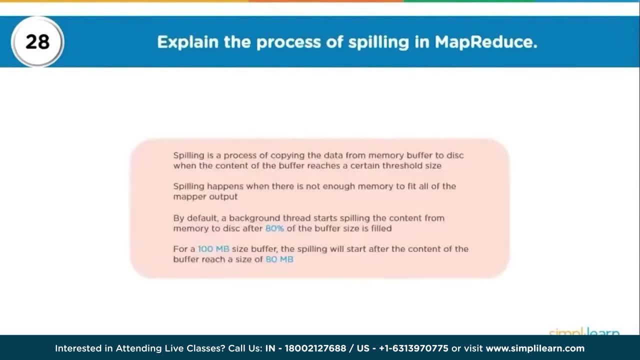 and can be used within your MapReduce job. What is the process of spilling in MapReduce? What does that mean? So spilling is basically a process of copying the data from memory buffer to disk when, obviously, the buffer usage reaches a certain threshold. So if there, 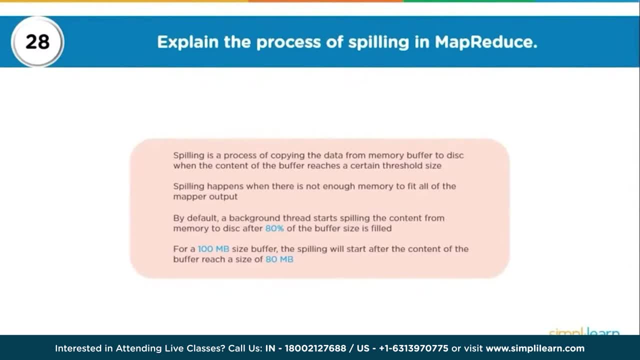 is not enough memory in your buffer, in your memory, then the content which is stored in buffer or memory has to be flushed out. So by default, a background thread starts spilling the content from memory to disk after 80% of buffer size is filled. Now, when is the buffer being used? 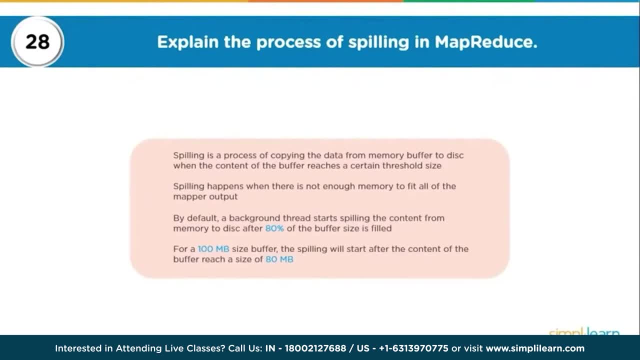 So when your MapReduce processing is happening, the data from data is being read from the disk, loaded into the buffer and then some processing happens. Same thing also happens when you are writing data to the cluster. So you can imagine for a 100 MB size. 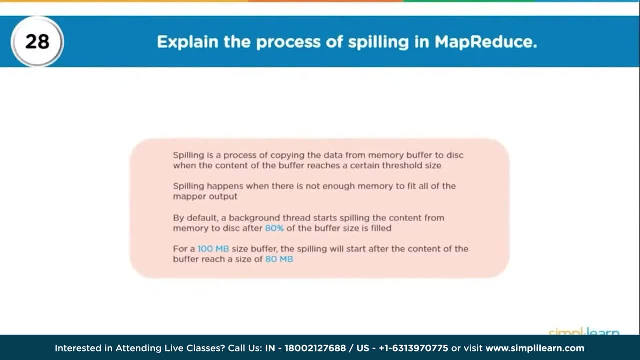 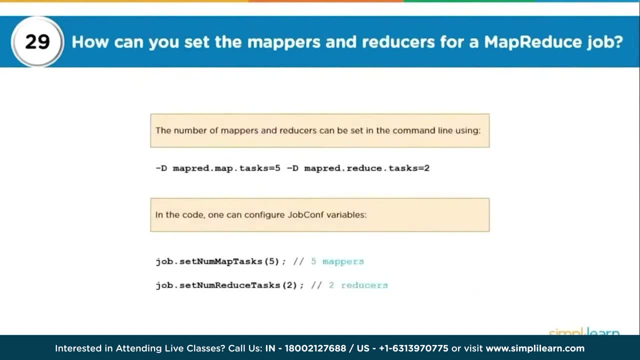 buffer. the spilling will start after the content of buffer reaches 80 MB. This is customizable. How can you set the mappers and reducers for a MapReduce job? So these are the properties. So number of mappers and reducers, as I mentioned earlier. 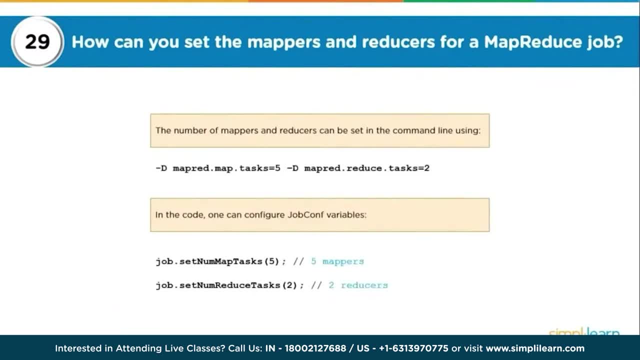 can be customized. So, by default, your number of map tasks depends on the split and number of reduced tasks depends on the partitioning phase, which decides number of reduced tasks which would be used, depending on the keys. However, we can set these properties either. 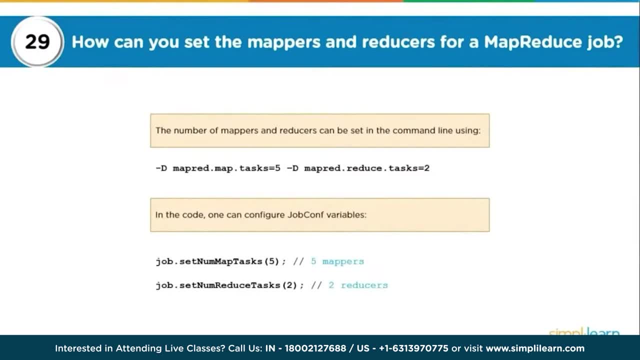 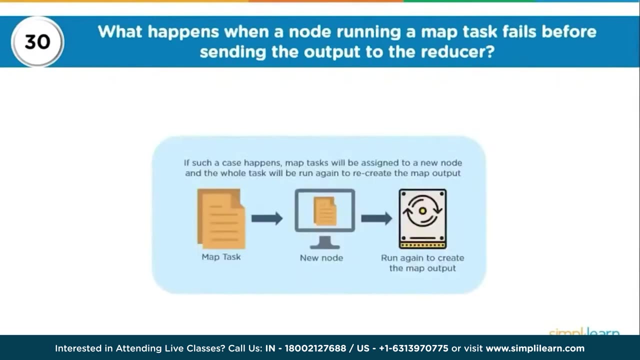 in the config files or provide them on the command line or also make them part of our code, and this can control the number of map tasks or reduced tasks which would be run for a particular job. Let's look at one more interesting question: What happens when a 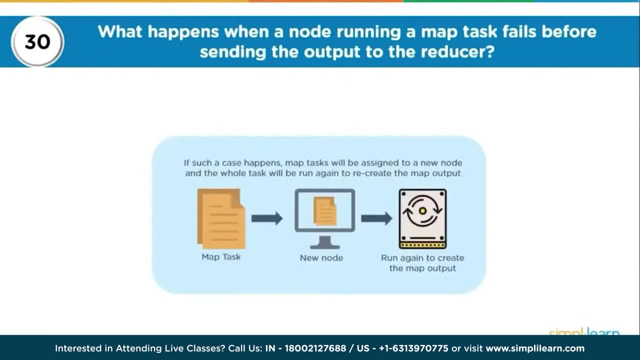 node running a map task fails before sending the output to the reducer. So there was a node which was running a map task and we know that there could be one or multiple map tasks running on one or multiple nodes and all the map tasks have to be completed. 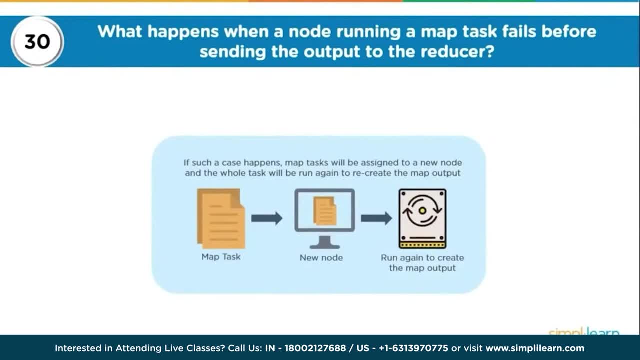 before the further stages, such as combiner or reducer, come into existence. So in a case if a node crashes where a map task was assigned to it, the whole task will have to be run again on some other node. So in Hadoop version. 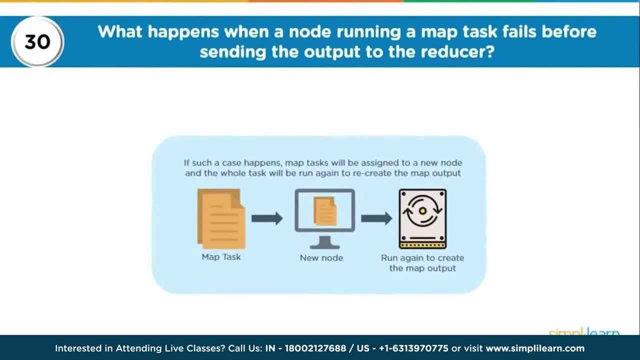 2, YARN framework has a temporary element called application master. So your application master is taking care of execution of your application and if a particular task on a particular node failed due to unavailability of node, it is the role of application master to have. 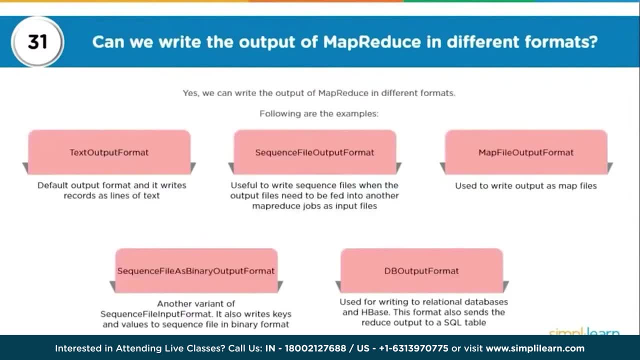 this task scheduled on some other node. Now, can we write the output of map reduce in different formats? Of course we can. So Hadoop supports various input and output formats, So you can write the output of map reduce in different formats, So you. 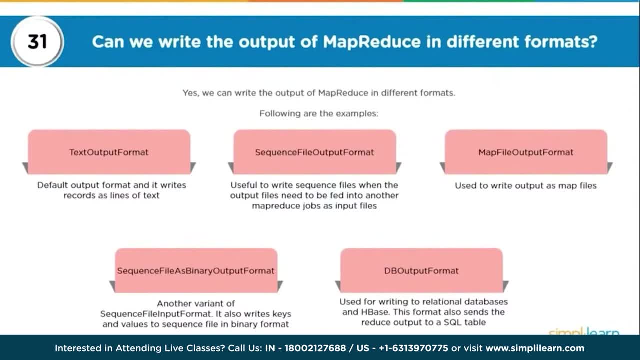 could have the default format, that is, text output format, wherein records are written as line of text. You could have sequence file, which is basically to write sequence files, or your binary format files, where your output files need to be fed into another map reduce jobs. You could go for a map. 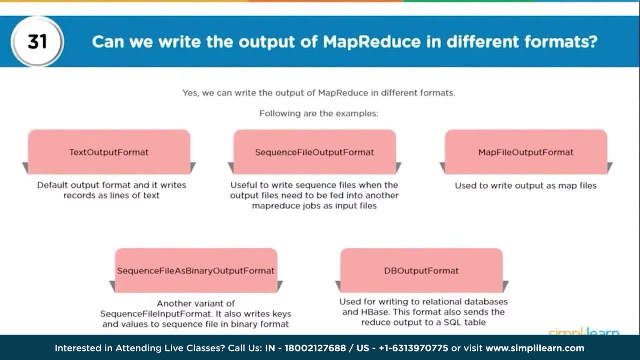 file output format to write output as map files. You could go for a sequence file as a binary output format. So that's again a variant of your sequence file input format. It basically writes keys and values to a sequence file. So when we 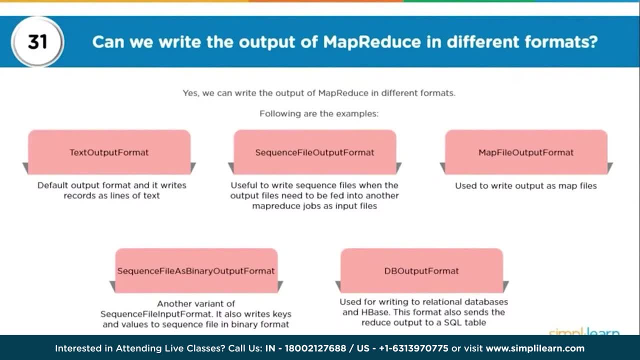 talk about binary format. we are talking about a non-human readable format, DB output format. now, this is basically used when you want to write data, to say relational databases or say no SQL databases such as HBase. So this format also sends the reduce output. 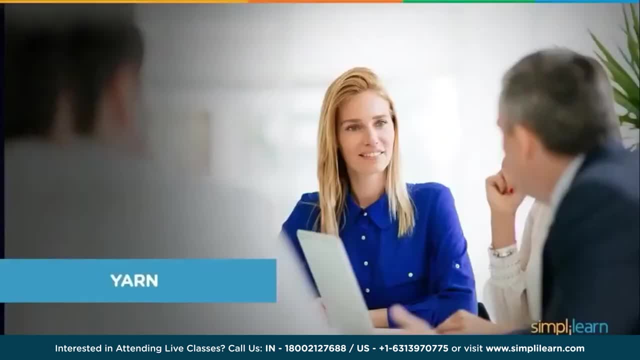 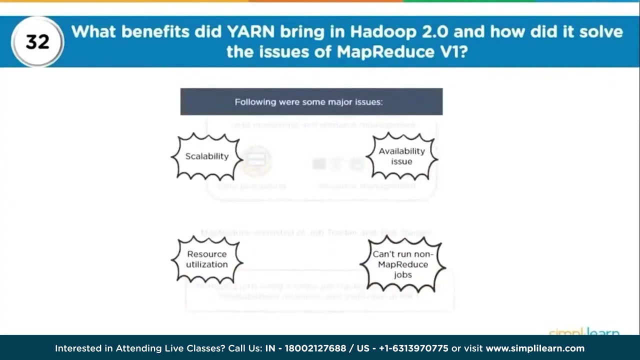 to a SQL table. Now let's learn a little bit about yarn, which stands for yet another resource negotiator. It's the processing framework. So what benefits did yarn bring in Hadoop version 2, and how did it solve the issues of MapReduce version 1?? 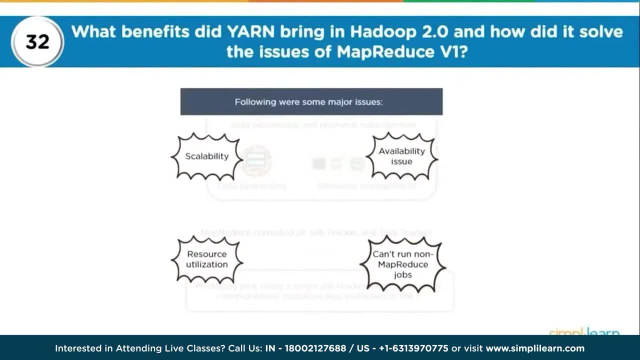 So MapReduce version 1 had major issues when it comes to scalability or availability because, sorry, in Hadoop version 1 you had only one master process for processing layer and that is your job tracker. So your job tracker was listening to all the task trackers which were 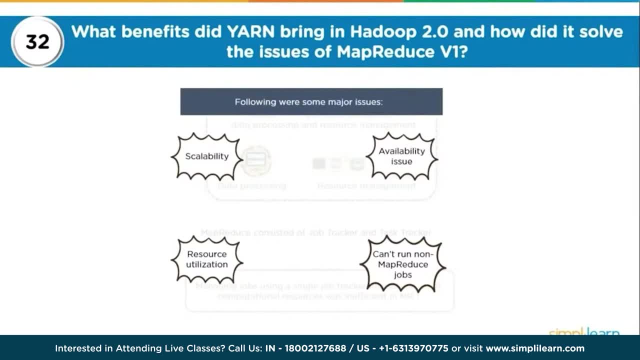 running on multiple machines, So your job tracker was responsible for resource tracking and job scheduling. In yarn you still have a processing master, but that's called resource manager instead of job tracker, and now, with Hadoop version 2, you could even have 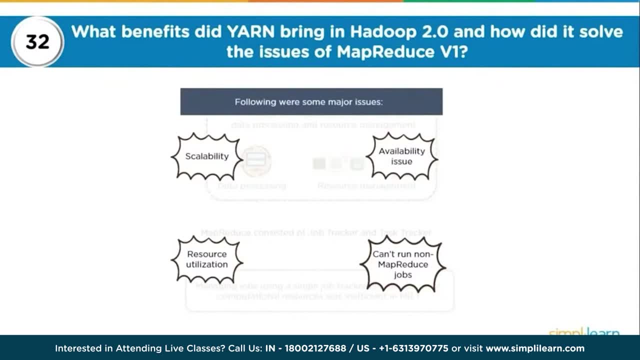 resource manager running in high availability mode. You have node managers which would be running on multiple machines, and then you have a temporary daemon called application master. So in case of Hadoop version 2, your resource manager or master is only handling the client connections. 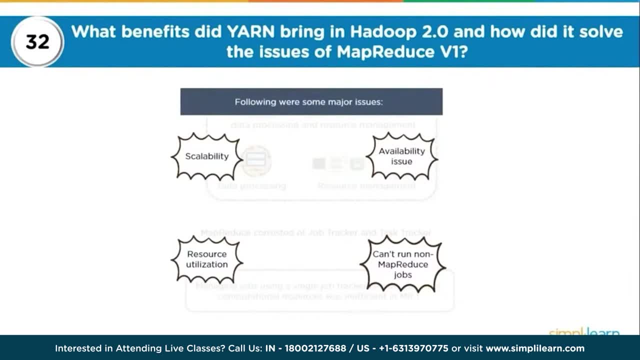 and taking care of tracking the resources, The job scheduling or basically taking care of execution across multiple nodes is controlled by application master till the application completes. So in yarn you can have different kind of resource allocations. that could be done and there is a concept. 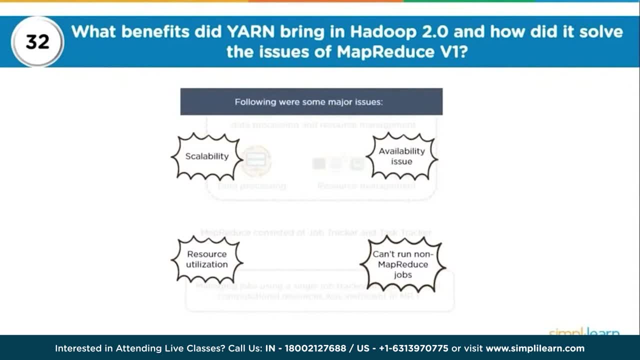 of container. So container is basically a combination of RAM and CPU cores. Yarn can run different kind of workloads, So it is not just MapReduce kind of workload which can be run on Hadoop version 2, but you could have graph processing. 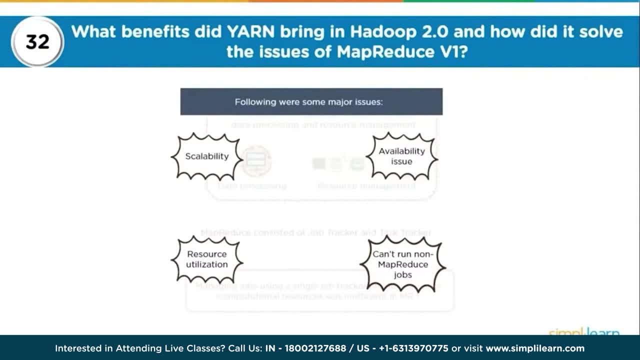 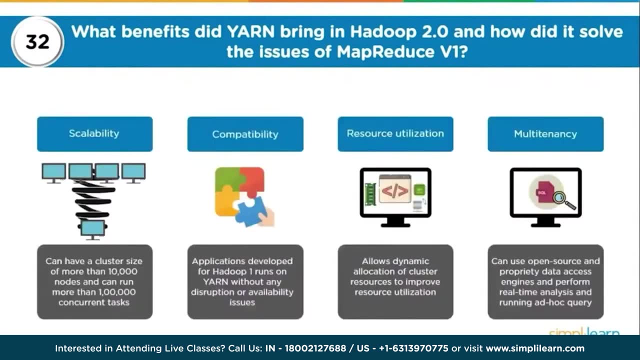 massive parallel processing. you could have real time processing and huge processing applications could run on a cluster based on yarn. So when we talk about scalability, in case of your Hadoop version 2, you can have a cluster size of more than 10,000 nodes and can. 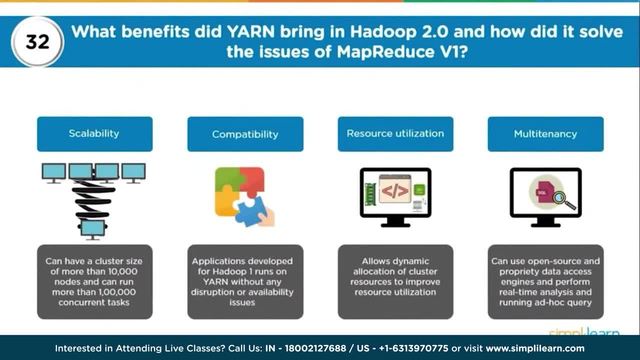 run more than 100,000 concurrent tasks and this is because, for every application which is launched, you have this temporary daemon called application master. So if I would have 10 applications running, I would have 10 app masters running taking care of. 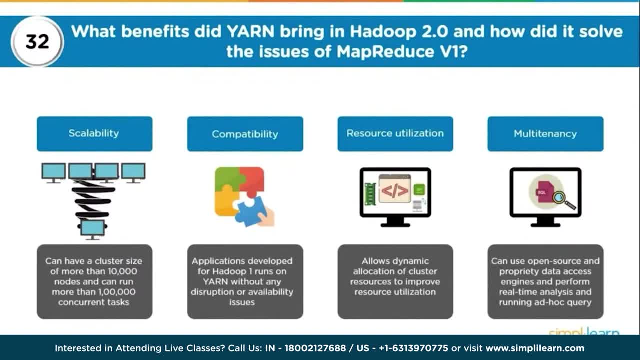 execution of these applications across multiple nodes Compatibility. So Hadoop version 2 is fully compatible with whatever was developed as per Hadoop version 1 and all your processing needs would be taken care by yarn. So dynamic allocation of cluster resources taking. 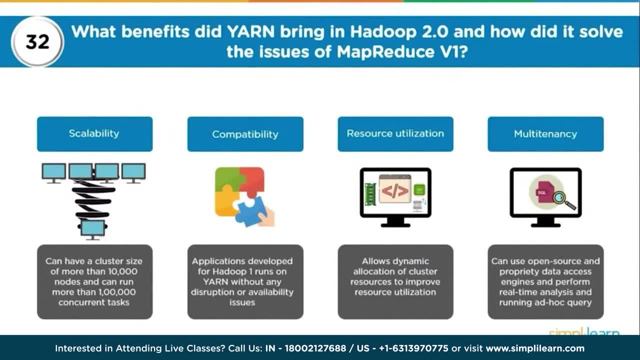 care of different workloads, allocating resources across multiple machines and using them for execution. all that is taken care by yarn Multi-tenancy, which basically means you could have multiple users or multiple teams. you could have open source and proprietary data service engines, and all of these. 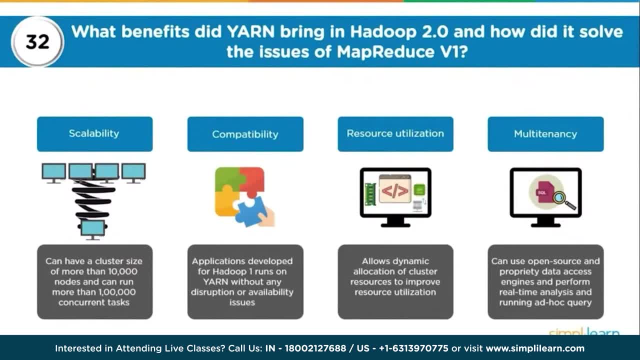 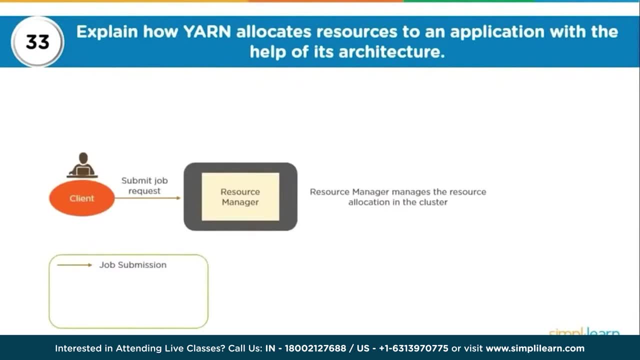 could be basically hosted using the same cluster. Now, how does yarn allocate resources to an application with the help of its architecture? So, basically, you have a client or an application or an API which talks to resource manager. Resource manager is, as I mentioned. 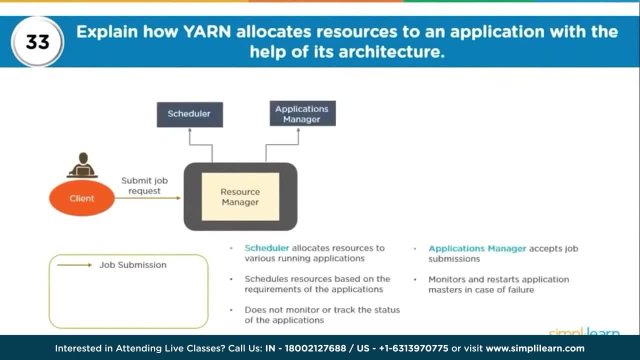 managing the resource allocation in the cluster. When you talk about resource manager, you have its internal two components: One is your scheduler and one is your applications manager. So when we say resource manager, being the master is tracking the resources, Resource manager is the one which is negotiating. 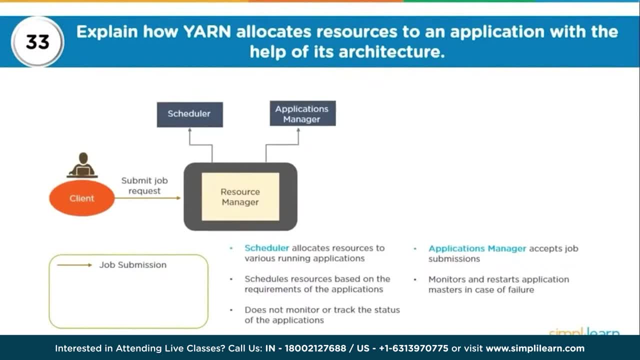 the resources. with slave It is not actually resource manager who is doing it, but these internal components. So you have a scheduler which allocates resources to various running applications. So scheduler is not bothered about tracking your resources or basically tracking your applications. So we can have different. 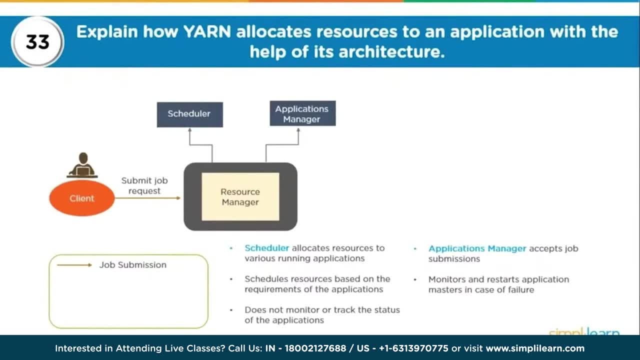 kind of schedulers such as FIFO, which is first in, first out. You could have a fair scheduler or you could have a capacity scheduler, and these schedulers basically control how resources are allocated to multiple applications when they are running in parallel. So there is 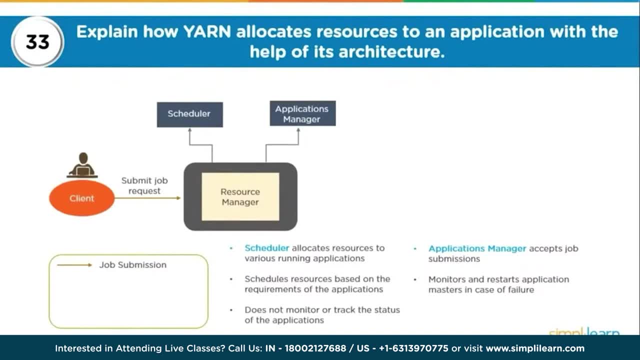 a queue mechanism. So scheduler will schedule resources based on requirements of application, but it is not monitoring or tracking the status of applications. Your application manager is the one which is accepting the job submissions. It is monitoring and restarting the application masters, So it's application manager which. 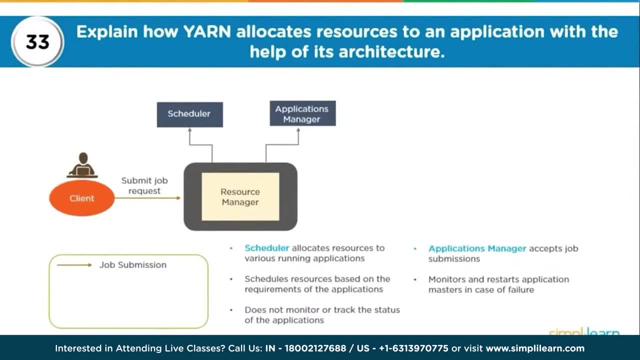 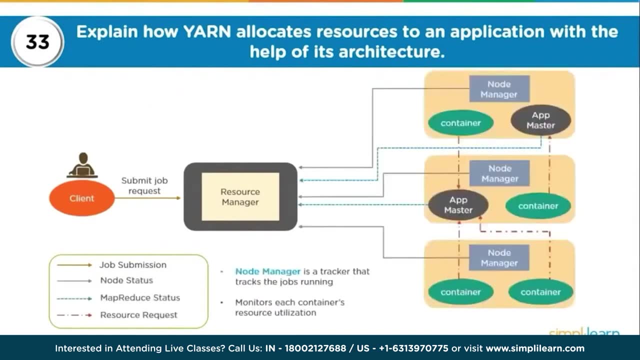 is basically then launching a application master which is responsible for an application. So this is how it looks. So whenever a job submission happens, we already know that resource manager is aware of the resources which are available with every node manager. So on every node which 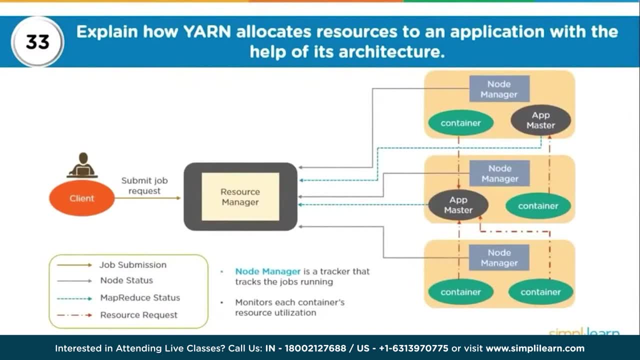 has fixed amount of RAM and CPU cores. some portion of resources, that is, your RAM and CPU cores, are allocated to node manager. Now resource manager is already aware of how much resources are available across nodes. So whenever a client request comes in, 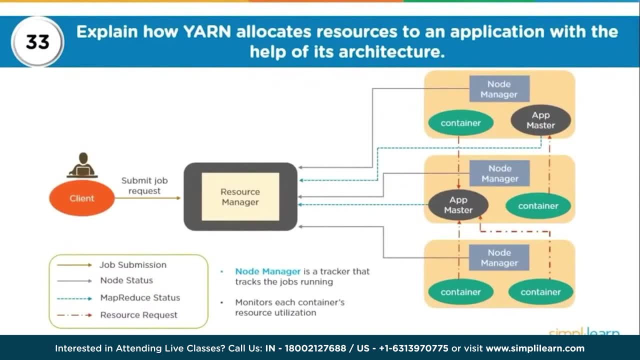 resource manager will make a request to node manager. It will basically request node manager to hold some resources for processing. Node manager would basically approve or disapprove this request of holding resources. And these resources- that is, a combination of RAM and CPU cores- are nothing but containers. 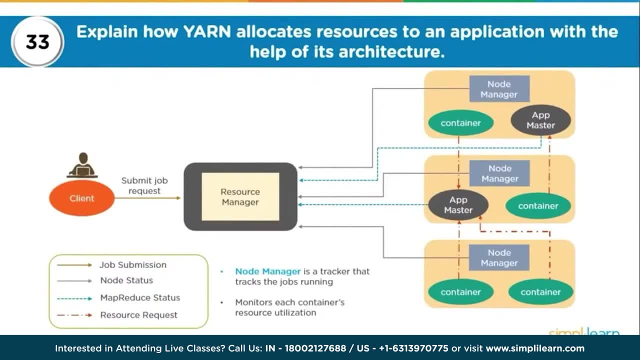 We can allocate containers of different sizes within yarn hyphen site file. So your node manager, based on a request from resource manager, guarantees the container which would be available for processing. That's when your resource manager starts a temporary domain called application master. 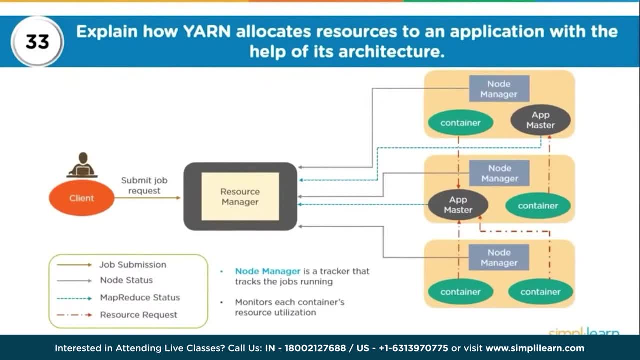 to take care of your execution. So your app master, which was launched by resource manager, or we can say internally by applications manager, will run in one of the containers, because application master is also a piece of code. So it will run in one of the containers. 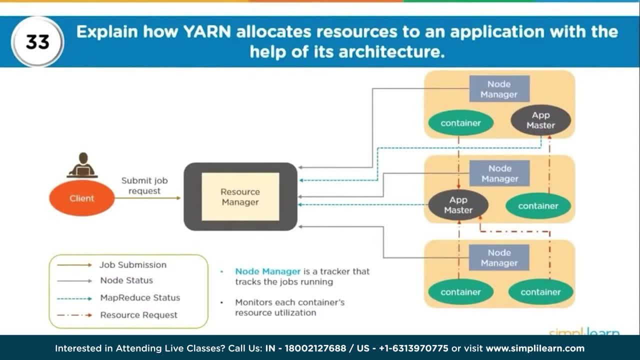 and then other containers will be utilized for execution. This is how yarn is basically taking care of your allocation. Your application master is managing resource needs. It is the one which is interacting with scheduler, and if a particular node crashes, it is the responsibility of app master to go. 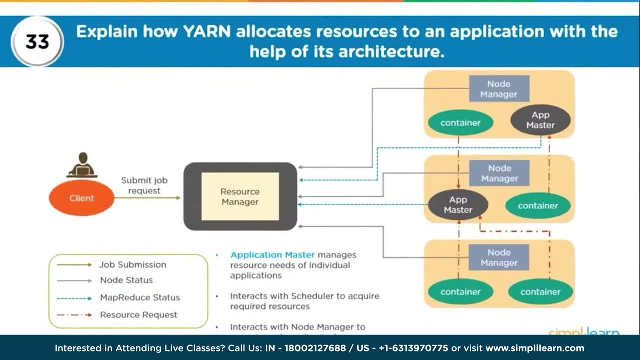 back to the master, which is resource manager, and negotiate for more resources. So your app master will never ever negotiate resources with node manager directly. It will always talk to resource manager and resource manager is the one which negotiates. the resources Container, as I said, is. 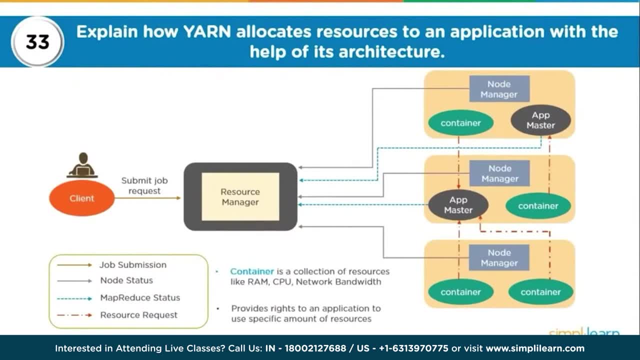 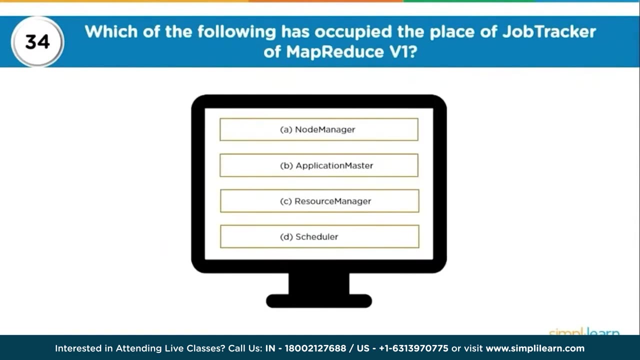 a collection of resources, like your RAM, CPU, network bandwidth and your container, is allocated based on the availability of resources on a particular node. Which of the following has occupied the place of a job tracker of MapReduce? It is your resource manager. So resource manager. 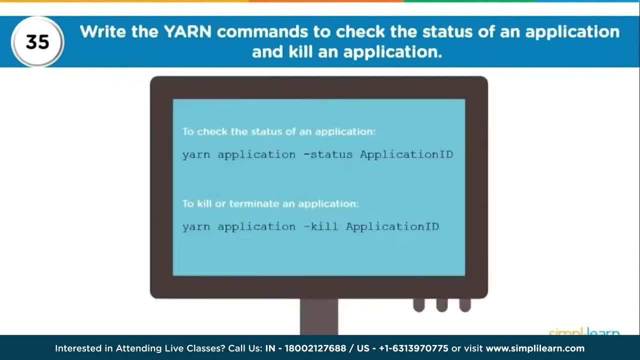 is the name of the master process in Hadoop version 2.. If you would have to write yarn commands to check the status of an application, we could just say yarn, application minus status and then the application id, and you could kill it also from the command. 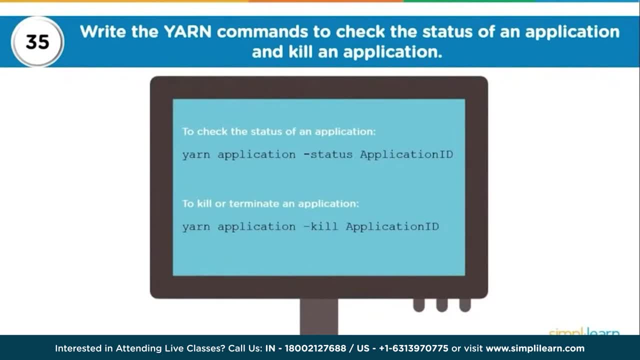 line. Remember, your yarn has a UI and you can even look at your applications from the UI. You can even kill your applications from the UI. However, knowing the command line commands would be very useful. Can we have more than one resource manager in a yarn based? 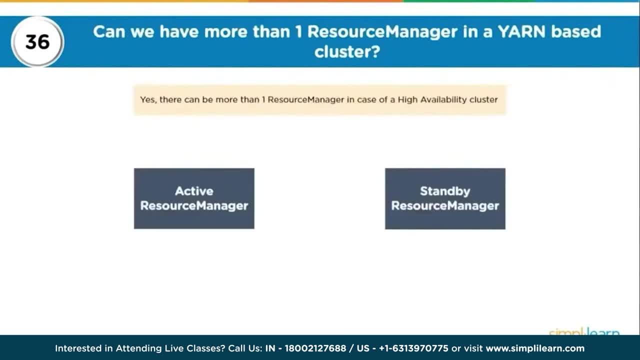 cluster. Yes, we can. That is what Hadoop version 2 allows us to have. So you can have a high availability yarn cluster where you have an active and standby and the coordination is taken care by your zookeeper At a particular 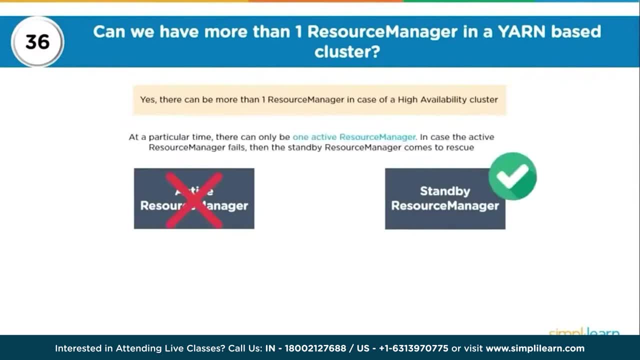 time, there can only be one active resource manager and if active resource manager fails, your standby resource manager comes and becomes active. However, zookeeper is playing a very important role. Remember, zookeeper is the one which is coordinating the server state and it is doing the election of. 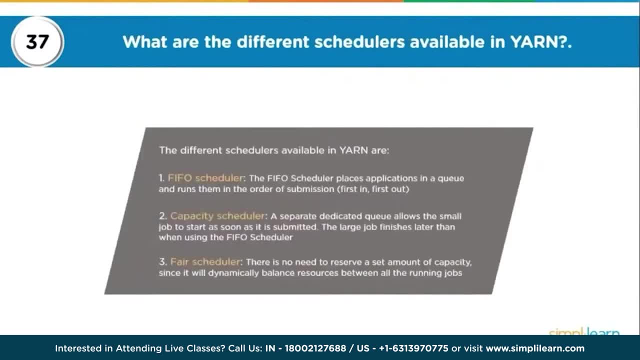 active to standby failover. What are the different schedulers available in yarn? So you have a FIFO scheduler that is first in, first out, and this is not a desirable option because in this case a longer running application might block all other small running applications. Your 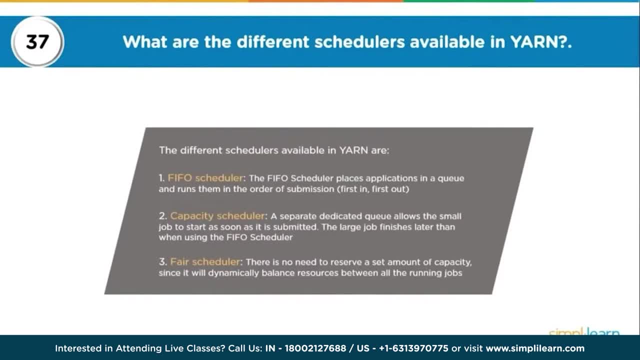 capacity scheduler is basically a scheduler where dedicated queues are created and they have fixed amount of resources, So you can have multiple applications accessing the cluster at the same time and they would be using their own queues and the resources allocated to them, If you talk. 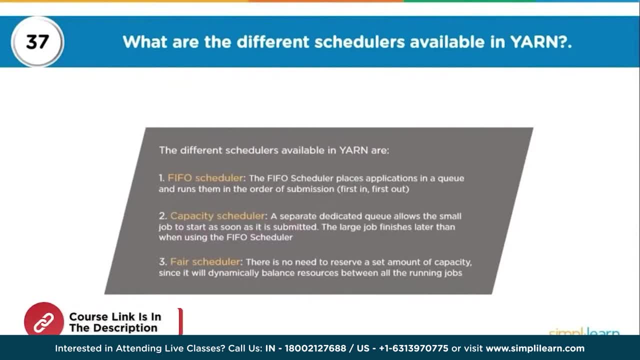 about fair scheduler. you don't need to have a fixed amount of resources. You can just have a percentage and you could decide what kind of fairness is to be followed, which basically means that if you were allocated 20 gigabytes of memory, however, the cluster has 100 gigabytes. 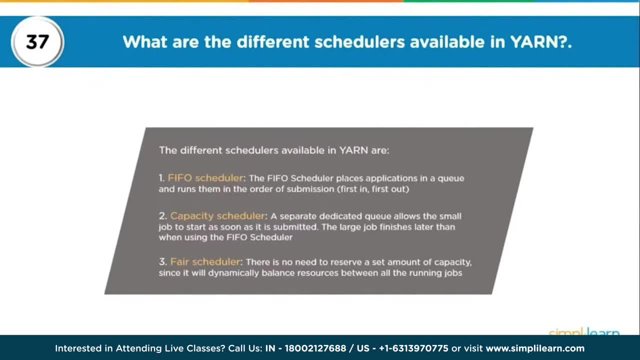 and the other team was assigned 80 gigabytes of memory, then you have 20% access to the cluster and other team has 80%. However, if the other team does not come up or does not use the cluster in a fair scheduler, 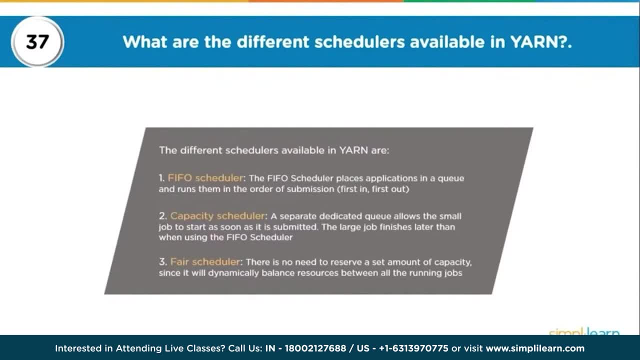 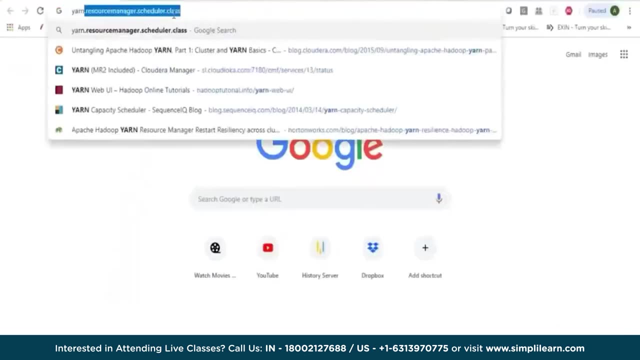 you can go up to maximum 100% of your cluster. To find out more information about your schedulers, you could either look in Hadoop definitive guide, or what you could do is you could just go to Google and you could type, for example, yarn. 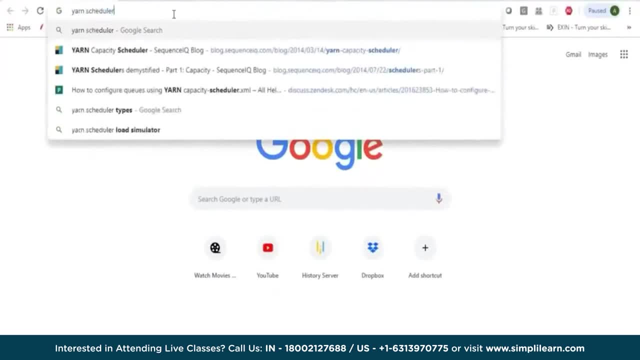 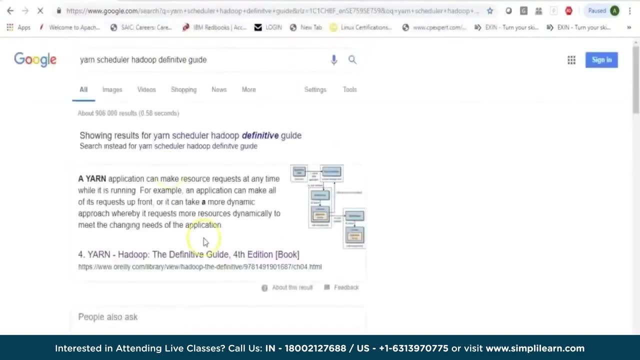 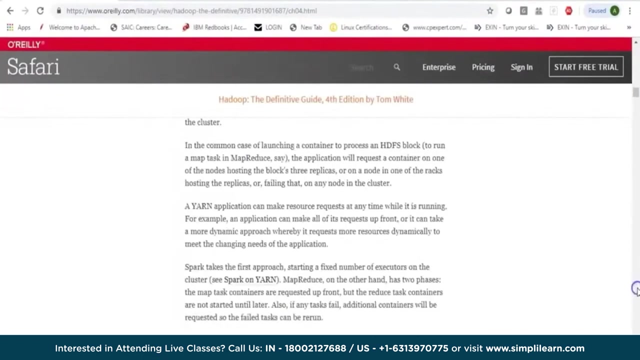 scheduler. Let's search for yarn scheduler and then you can look in Hadoop definitive guide. and so this is your Hadoop definitive guide and it beautifully explains about your different schedulers. how do multiple applications run, and that could be in your FIFO kind of. 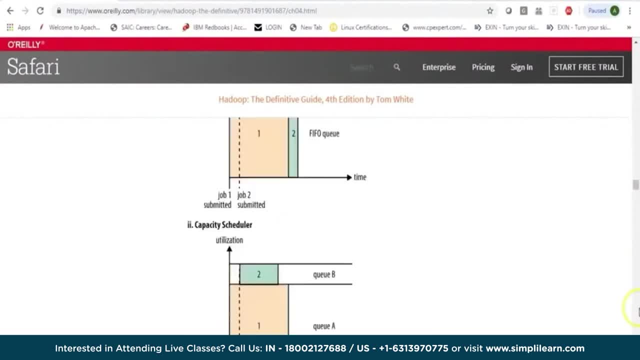 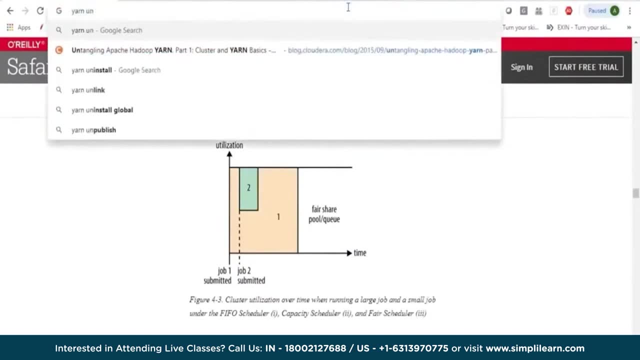 scheduling. It could be in capacity scheduler or it could be in a fair scheduling. So have a look at this link. It's a very good link. You can also search for yarn untangling and this is a blog of four, or this is a series of four blogs, where 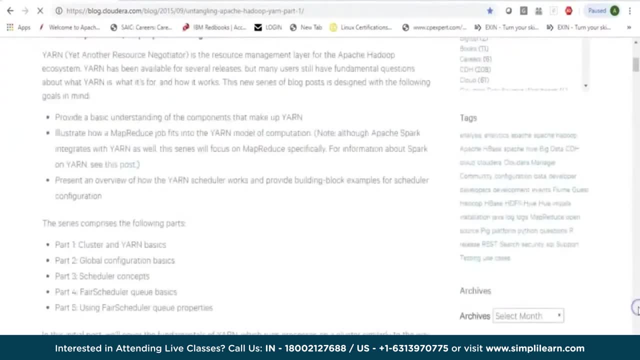 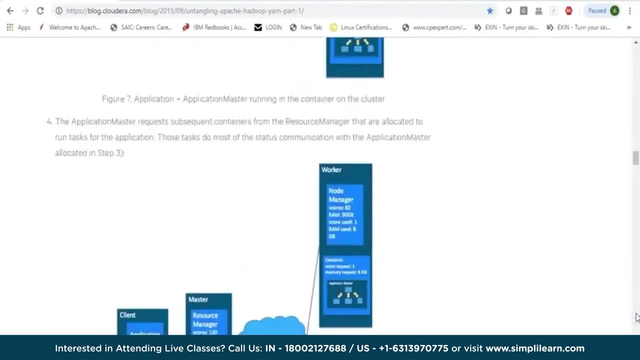 it's beautifully explained about your yarn, how it works, how the resource allocation happens, what is a container and what runs within the container. So you can scroll down, you can be reading through this and you can then also search for part two of it, which talks about allocation. 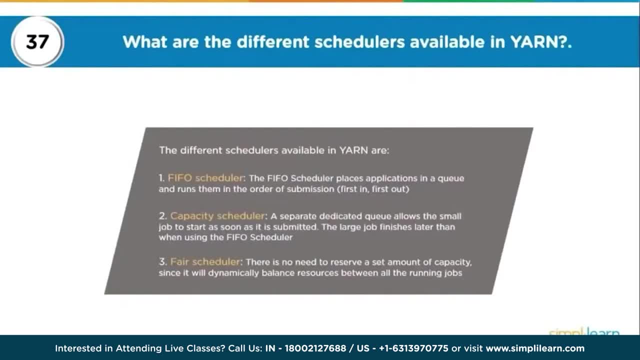 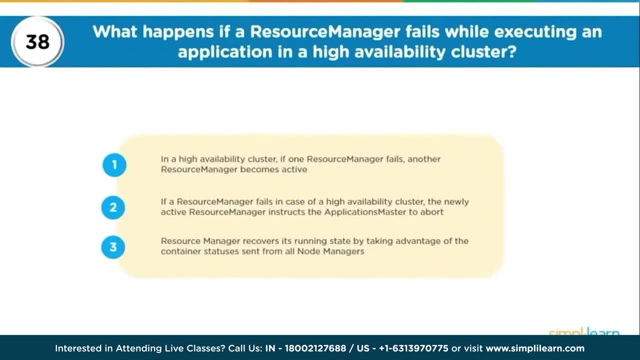 and so on. So, coming back, we basically have these schedulers. What happens if a resource manager fails while executing an application in a high availability cluster? So, in a high availability cluster, we know that we would have two resource managers, one being active. 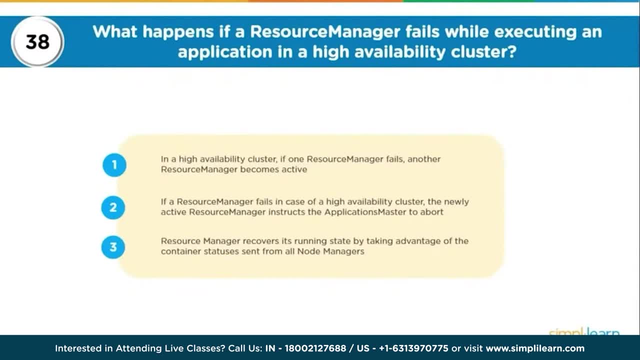 one being standby and zookeeper, which is keeping a track of the server states. So if a RM fails in case of high availability, the standby will be elected as active and then basically your resource manager or the standby would become the active one And this one would instruct. 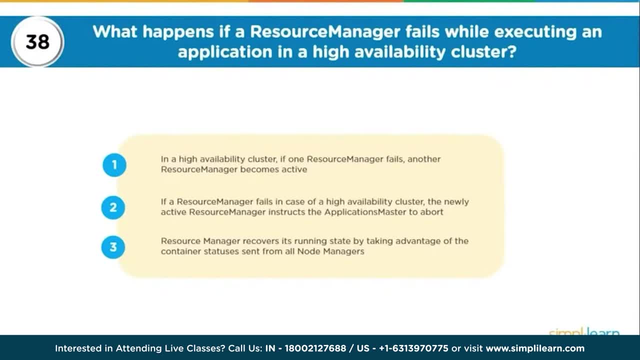 the application master to abort in the beginning. Then your resource manager recovers its running state. So there is something called as RM state store where all the applications which are running their status is stored. So resource manager recovers its running state by looking. 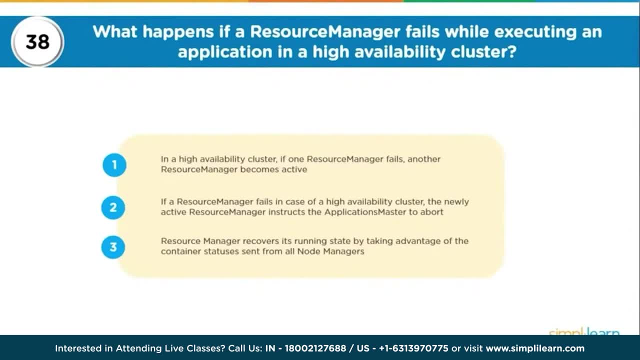 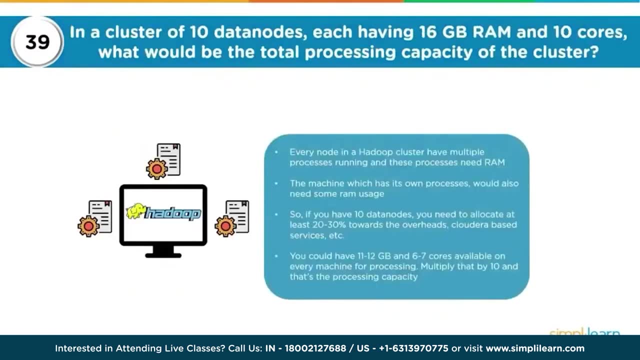 at your state store by taking advantage of container statuses and then continues to take care of your processing. Now, in a cluster of 10 data nodes, each having 16 GB and 10 cores, what would be total processing capacity of the cluster? Take a minute. 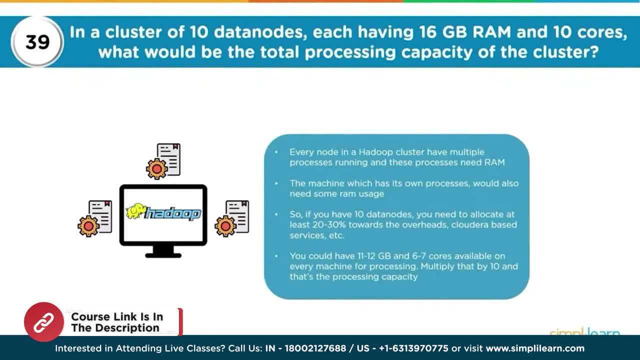 to think: 10 data nodes, 16 GB RAM per node, 10 cores. So if you mention the answer as 160 GB RAM and 100 cores, then you went wrong. Now think of a cluster which has 10 data nodes, each having 16. GB RAM and 10 cores. Remember, on every node in a Hadoop cluster you would have one or multiple processes running. Those processes would need RAM. The machine itself, which has a Linux file system, would have its own processes, So that would also be having some RAM usage. 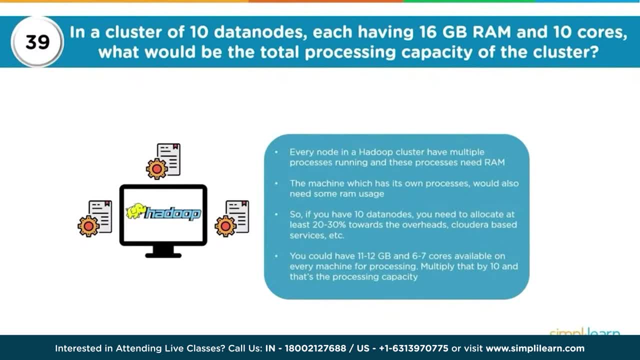 Which basically means that if you talk about 10 data nodes, you should deduct at least 20 to 30% towards the overheads, towards the cloud database services, towards the other processes which are running, And in that case I could say that you could have. 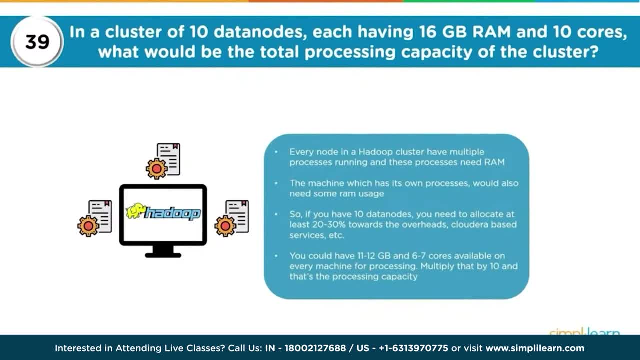 11 or 12 GB available on every machine for processing and say 6 or 7 cores. Multiply that by 10 and that's your processing capacity. Remember the same thing applies to the disk usage also. So if somebody asks you in a 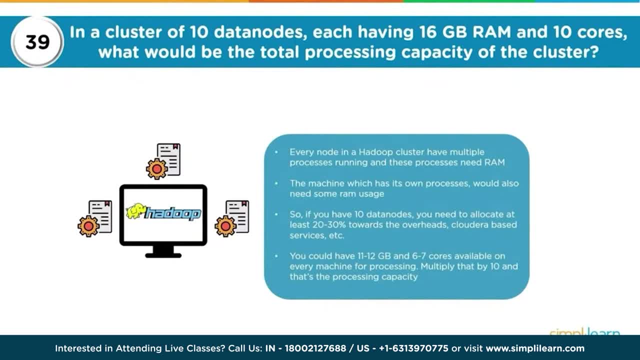 10 data node cluster where each machine has 20 terabytes of disks. what is my total storage capacity available for its DFS? So the answer would not be 200.. You have to consider the overheads And this is basically which gives you your processing capacity. 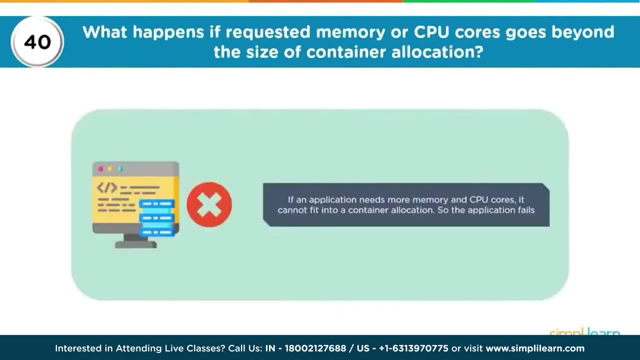 Now let's look at one more question. So what happens if requested memory or CPU cores beyond, or goes beyond the size of container? Now, as I said, you can have your configurations which can say that in a particular data node which has 100 GB RAM, I could. 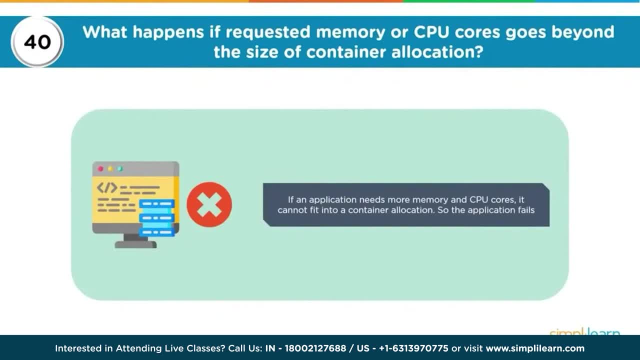 allocate, say, 50 GB for the processing Out of 100 cores. I could say 50 cores for processing. So if you have 100 GB RAM and 100 cores, you could ideally allocate 100 for processing. but that's not ideally possible. So if you have 100, 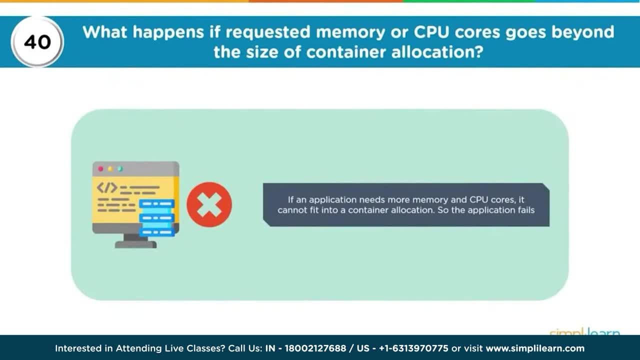 GB RAM, you would go for 50 GB, and if you have 100 cores, you would go for 50 cores. Now, within this RAM and CPU cores, you have the concept of containers. So container is a combination of RAM and CPU cores, So you could have a minimum. 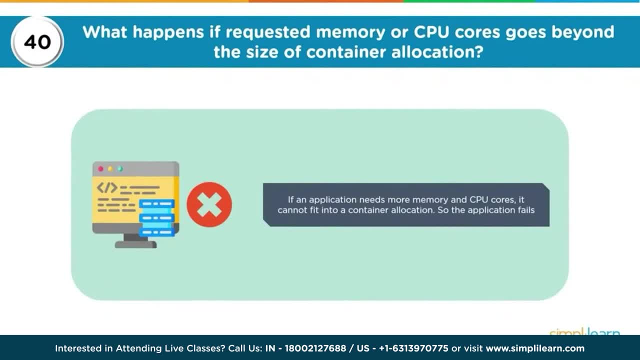 size container and maximum size container. Now, at any point of time, if your application starts demanding more memory or more CPU cores and this cannot fit into a container allocation, your application will fail. Your application will fail because you requested for a memory or a combination of memory and CPU cores. 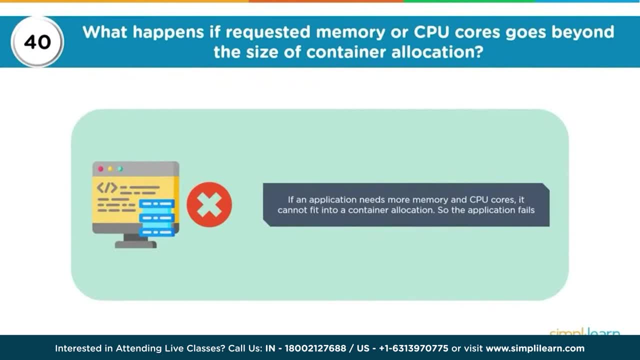 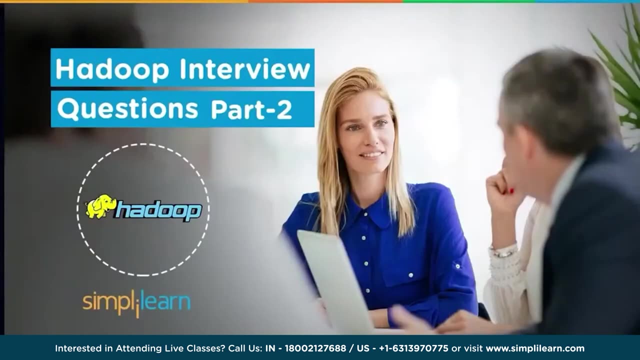 which is more than the maximum container size. So look into this yarn tangling website which I mentioned, and look for the second blog in those series which explains about these allocations. Now here we will discuss on Hive, PEG, HBase and these components of Hadoop. 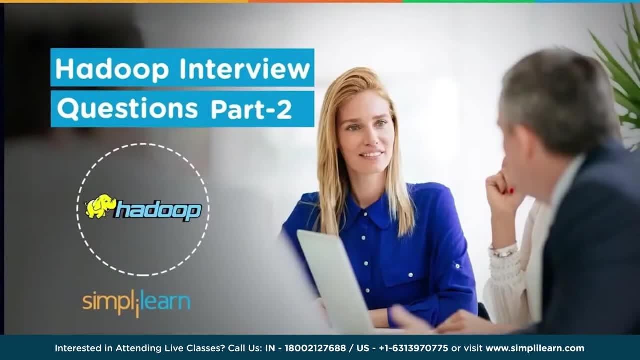 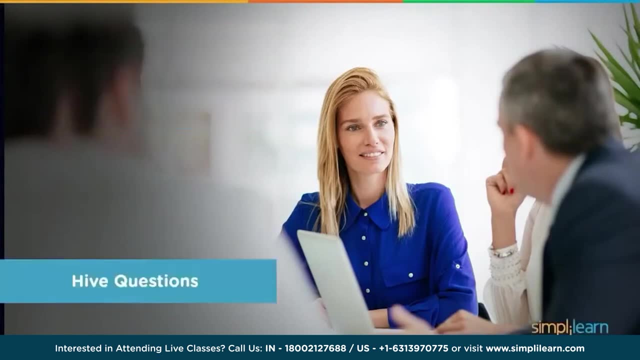 which are being used in the industry for various use cases. Let's look at some questions here and let's look how you should prepare for them. So first of all, we will learn on Hive, which is a data warehousing package. So the question is: 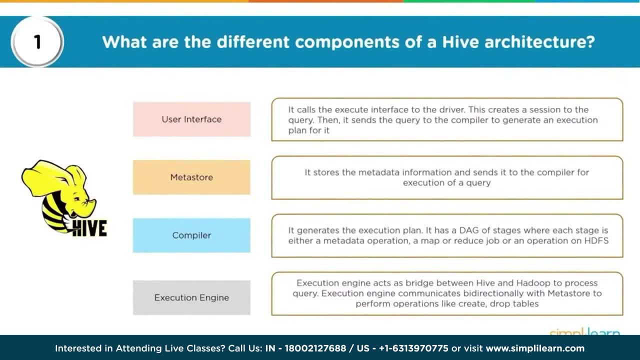 what are the different components of a Hive architecture? Now, when we talk about Hive, we already know that Hive is a data warehousing package which basically allows you to work on structured data or data which can be structurized. So normally people are well versed. 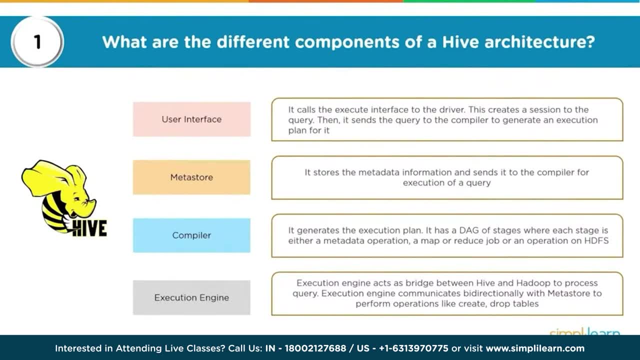 with querying or basically processing the data using SQL queries. Lot of people come from database backgrounds and they would find it comfortable if they know structured query language. Hive is one of the data warehousing package which resides within a Hadoop ecosystem. It uses Hadoop's 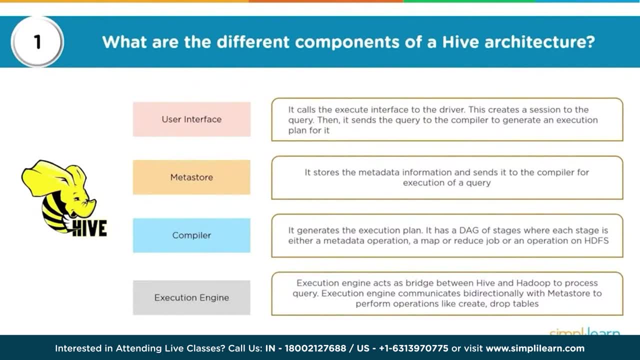 distributed file system to store the data, and it uses RDBMS usually to store the metadata, Although metadata can be stored locally also. So what are the different components of an Hive architecture? So it has a user interface. So user interface calls the execute interface. 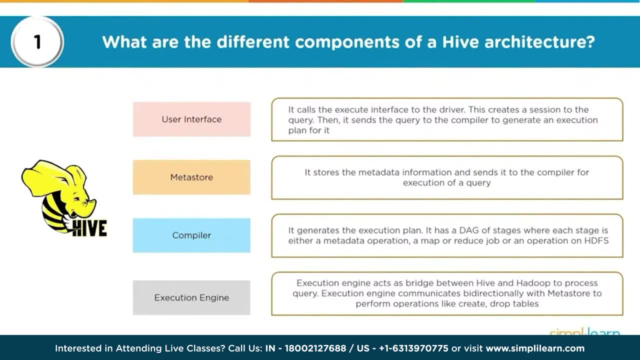 to the driver. This creates a session to the query and then it sends the query to the compiler to generate an execution plan for it. Usually, whenever Hive is set up, it would have its metadata stored in an RDBMS. Now to establish the connection between RDBMS. 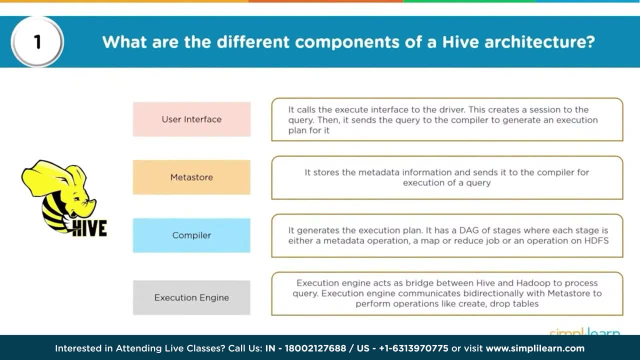 and Hadoop. we need ODBC or JDBC connector jar file and that connector jar file has a driver class. Now this driver class is mandatory to create a connection between Hive and Hadoop. So user interface creates this interface using the driver. Now we 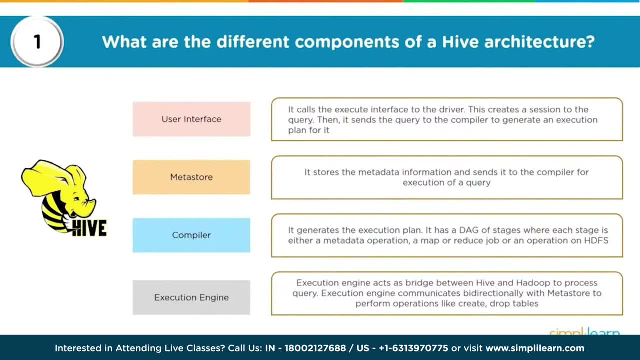 have metastore. Metastore stores the metadata information. So any object which you create, such as database table, indexes. their metadata is stored in metastore, and usually this metastore is stored in an RDBMS so that multiple users can connect to Hive. So your 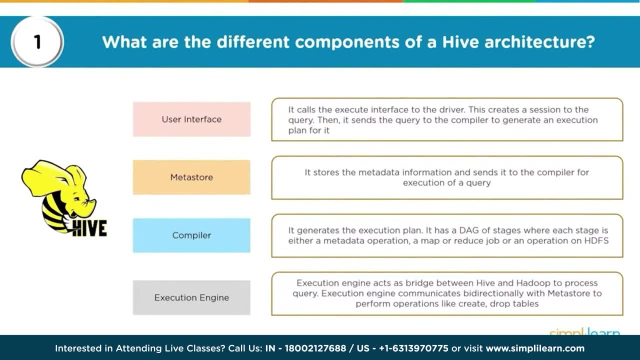 metastore stores the metadata information and sends that to the compiler for execution of a query. What does the compiler do? It generates the execution plan. It has a DAG. Now DAG stands for direct graph, So it has a DAG of stages where each stage 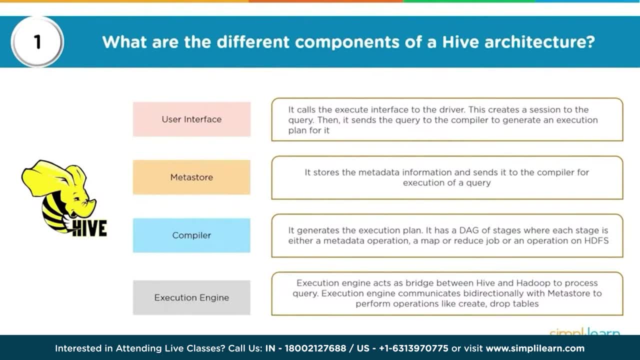 is either a metadata operation, a map or reduce job, or an operation on HDFS. And finally we have execution engine that acts as a bridge between Hive and Hadoop to process the query. So execution engine communicates bidirectionally with metastore to perform. 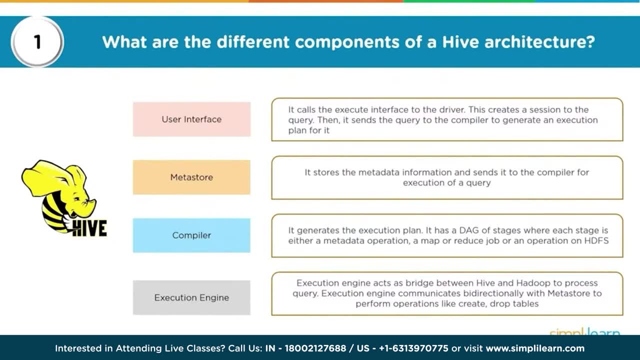 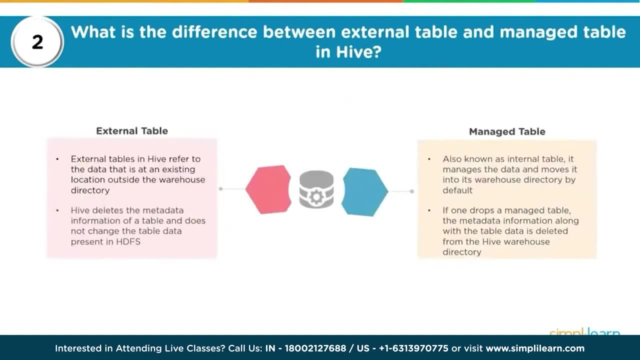 operations like create or drop tables. So these are four important components of Hive architecture. Now, what is the difference between external table and managed table in Hive? So we have various kinds of table in Hive, such as external table, managed table, partition table. The major difference, 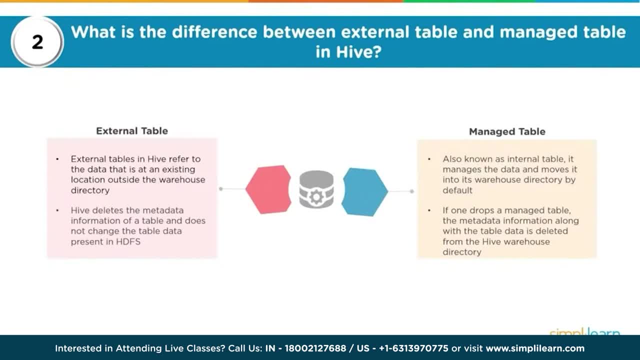 between your managed and external table is in respect to what happens to the data if the table is dropped. Usually, whenever we create a table in Hive, it creates a managed table, or we could also call that as an internal table. Now this manages the data and moves it into. 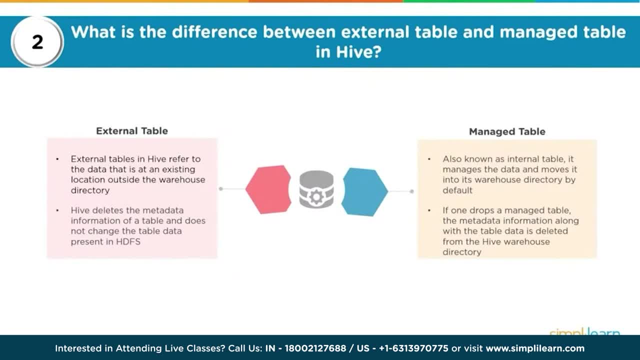 warehouse directory by default. Whether you create a managed table or external table, usually the data can reside in Hive's default warehouse directory or it could be residing in a location chosen. However, when we talk about managed table, if one drops, a managed table not 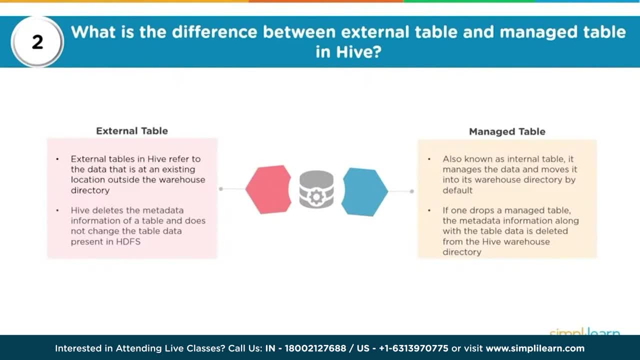 only the metadata information is deleted, but the table's data is also deleted from HDFS. If we talk about external table, it is created with an external keyword explicitly, and if an external table is dropped, nothing happens to the data which resides in HDFS. So that's the 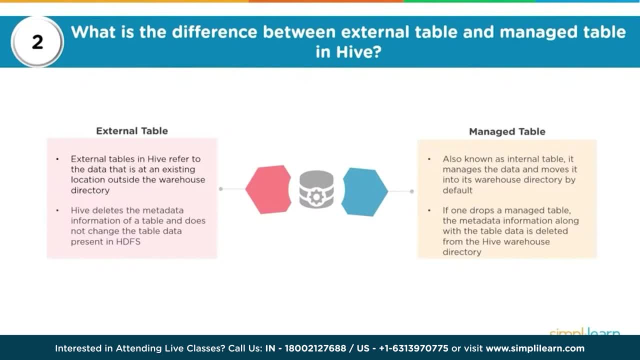 main difference between your managed and external table. What might be the use case if somebody asks you There might be a migration kind of activity or you are interested in creating lot of tables using your queries, So in that case you could dump all the data. 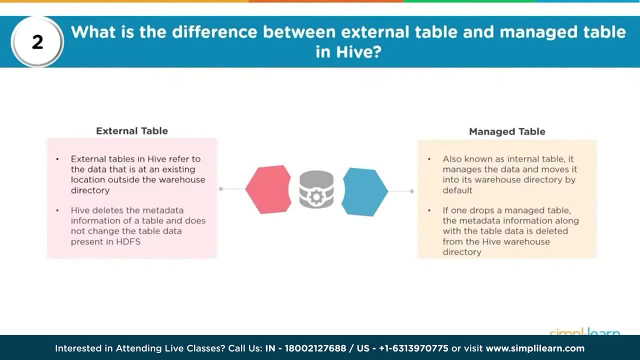 on HDFS, and then you could create a table by pointing to a particular directory or multiple directories. Now you could then do some testing of your tables and would decide that you might not need all the tables, So in that case it would be advisable to create external tables. 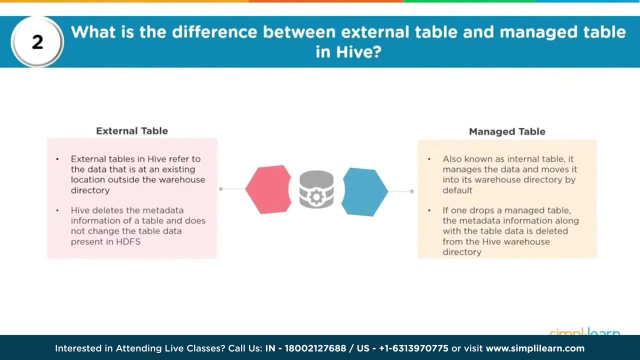 so that even if the table is later dropped, the data on HDFS will be intact, unlike your managed table, where dropping of table will delete the data from HDFS. also, Let's learn a little bit on partition. So what is partition in HIFE? 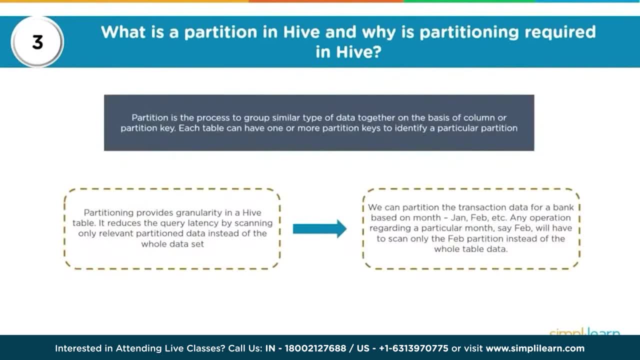 and why is partitioning required in HIFE? if somebody asks you that, Now, normally in world of RDBMS, partition is the process to group similar type of data together, and that is usually done on basis of a column, or what we call as partitioning key. Now, each 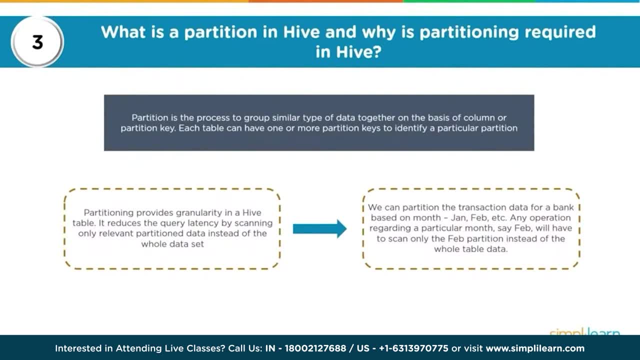 table usually has one column in context of RDBMS, which could be used to partition the data. And why do we do that? So that we can avoid scanning the complete table for a query and restrict the scan to set of data or to a particular partition In. 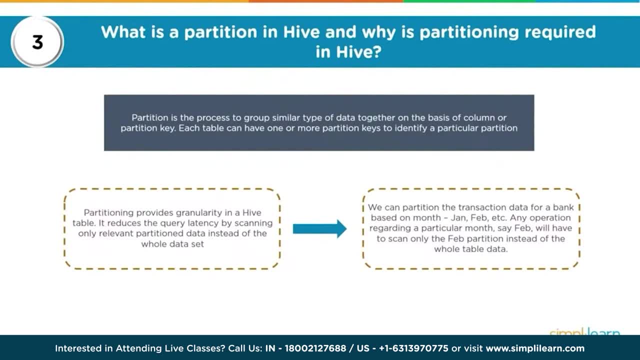 HIFE we can have any number of partition keys. So partitioning provides granularity in HIFE table. It reduces the query latency by scanning only relevant partition data instead of whole data set. We can partition at various levels. Now, if I compare RDBMS with HIFE, in case 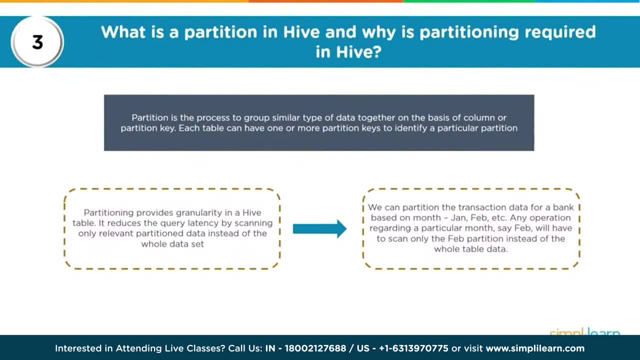 of RDBMS, you could have one column which could be used for partitioning, and then you could be querying the specific partition. So in case of RDBMS, your partition column is usually a part of the table definition. So, for example, if I have 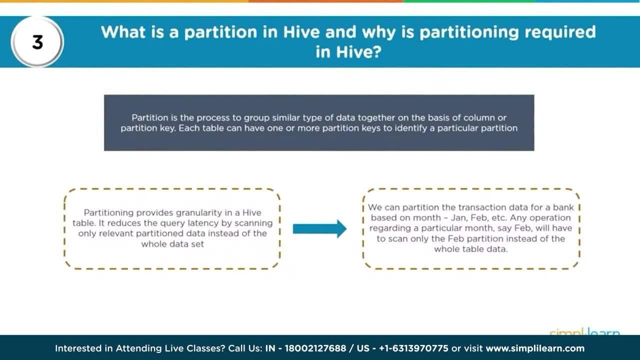 an employee table. I might have employee ID, employee name, employee age and employee salary as four columns and I would decide to partition the table based on salary column. Now, why would I partition it? Because I feel that employee table is growing very fast. 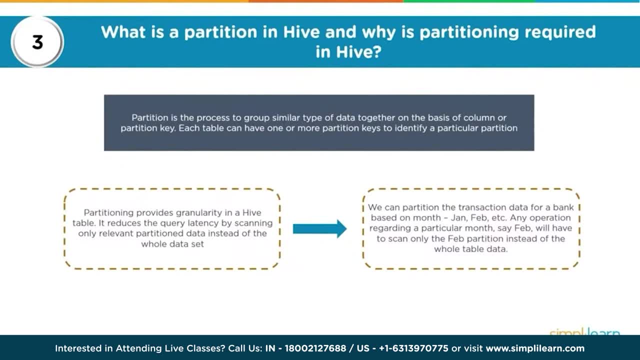 It is or it will have huge amount of data and later when we query the table, we don't want to scan the complete table, So I could split my data into multiple partition based on a salary column giving some ranges In HIFE it is. 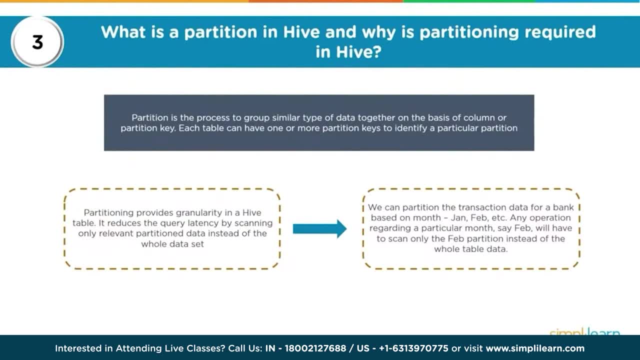 a little different. In HIFE you can do partitioning and there is a concept of static and dynamic partitioning. But in HIFE the partition column is not part of table definition. So you might have an employee table with employee ID name. 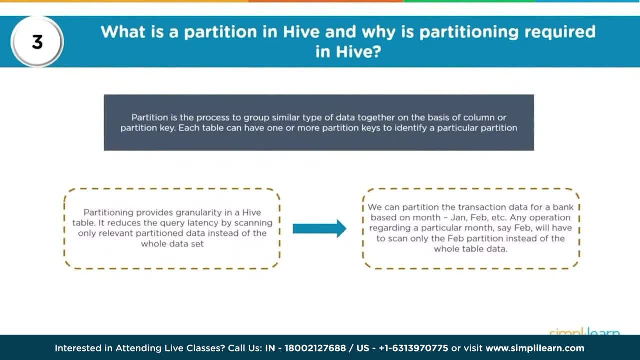 age, and that's it. That would be the table definition, But you could then have partitioning done based on salary column, which will then create a specific folder on SDFS. In that case, when we query the data, we can see the partition. 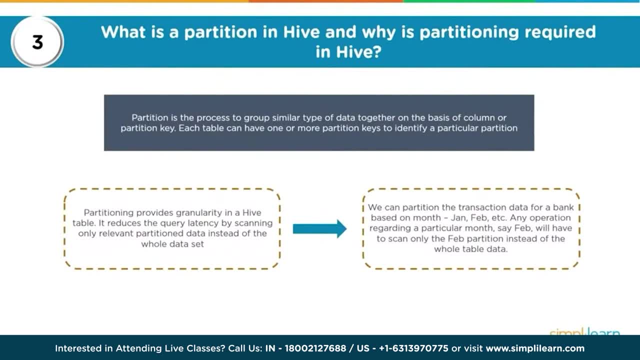 column also showing up. So we can partition the transaction data for a bank, for example, based on month, like Jan, Feb, etc. And any operation regarding a particular month will then allow us to query that particular folder. That is where partitioning is useful. Now why does HIFE? 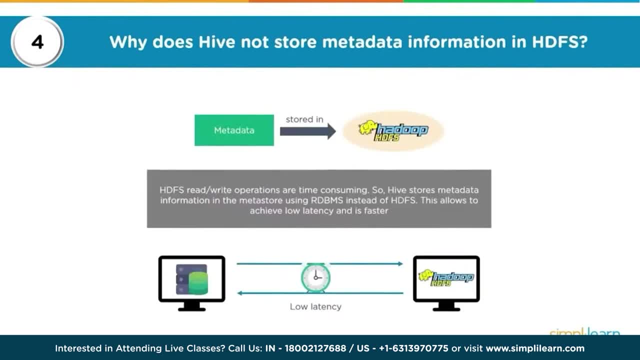 not store metadata information in SDFS if somebody asks you So. we know that HIFE's data is stored in SDFS, which is Hadoop Distributed File System. However, the metadata is either stored locally and that mode of HIFE would be called as embedded. 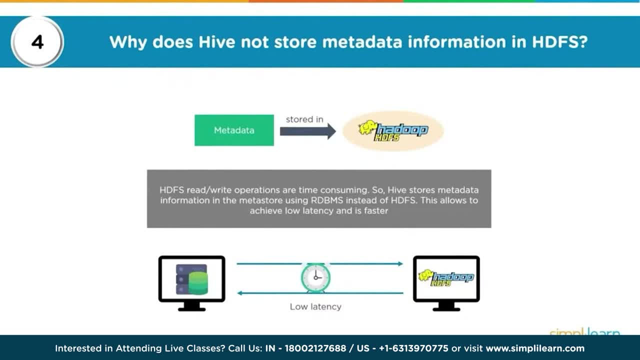 mode, or you could have HIFE's metadata stored in RDBMS so that multiple clients can initiate a connection. Now this metadata, which is very important for HIFE, would not be stored in SDFS, So we already know that SDFS read and write operations. 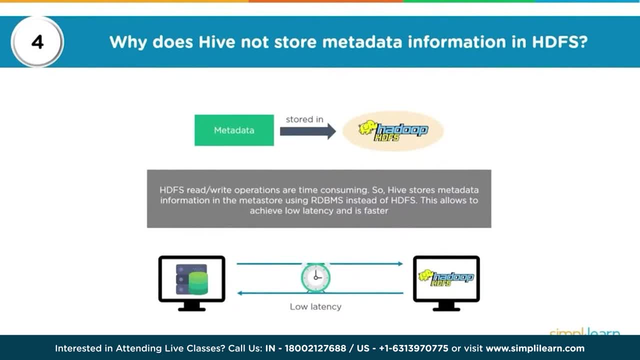 are time consuming. It is a distributed file system and it can accommodate huge amount of data. So HIFE stores metadata information in Metastore using RDBMS instead of SDFS. So this allows to achieve low latency and faster data access. Now, if somebody asks, 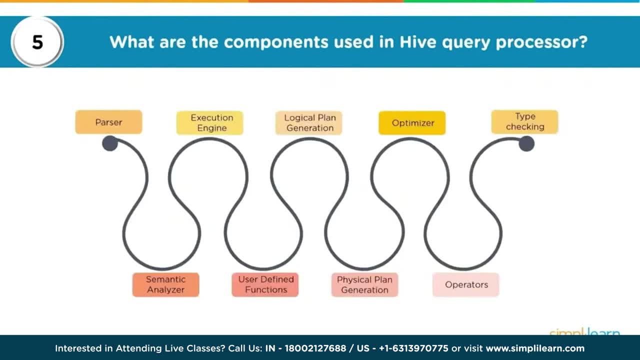 what are the components used in HIFE Query Processor? So usually we have the main components are your parser, your execution engine, logical plan generation optimizer and type checking. So whenever a query is submitted it will go through a parser and parser would check the syntax. 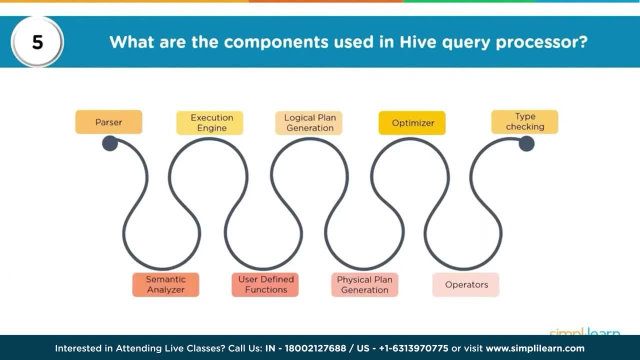 it would check for objects which are being queried and other things to see if the query is fine. Now, internally you have a semantic analyzer which will also look at the query. You have an execution engine which basically will work on the execution part, That is. 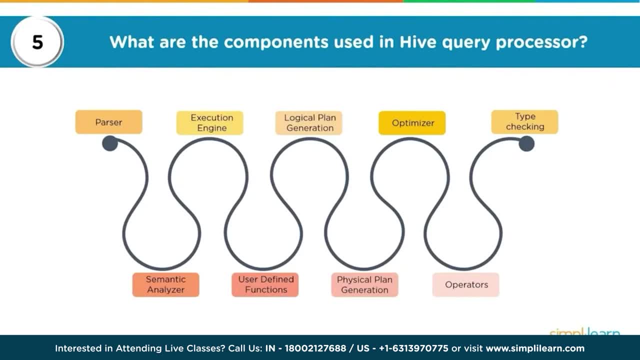 the best generated execution plan which could be used to get the results for the query. You could also have user defined functions which a user would want to use, and these are normally created in Java or Java programming language, and then, basically, these user defined functions are added to the classpath. 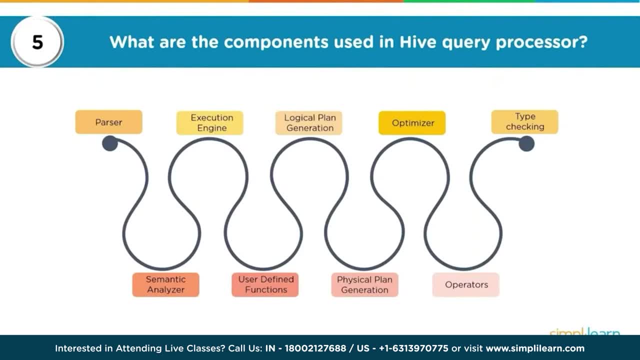 Now you would have a logical plan generation which basically looks at your query and then generates a logical plan or the best execution path which would be required to get to the results. Internally, there is a physical plan generated which is then looked in by optimizer to get the 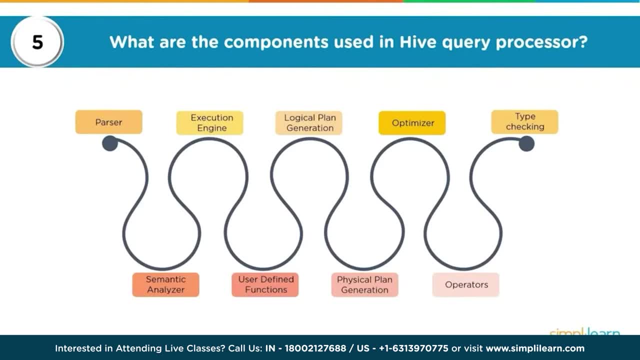 best path to get to the data, and that might also be checking your different operators which you are using within your query. Finally, we would also have type checking. So these are important components in Hive, So somebody might ask you if you are querying your data using Hive. 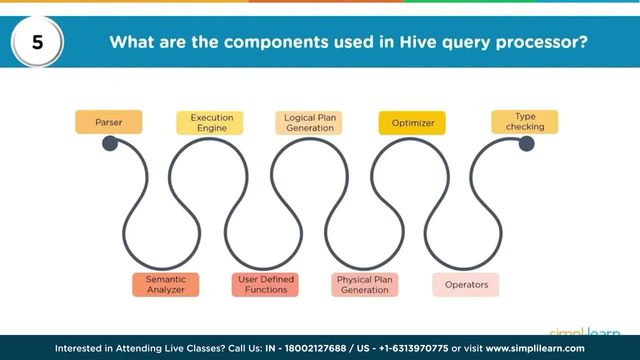 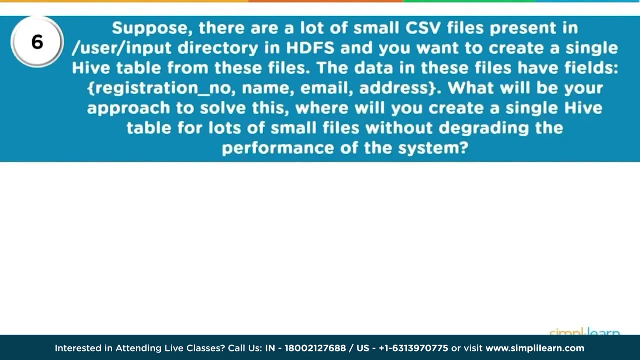 what are the different components involved, or if you could explain what are the different components which work when a query is submitted. So these are the components. Now let's look a scenario based question. Suppose there are lot of small CSV files which are present in a 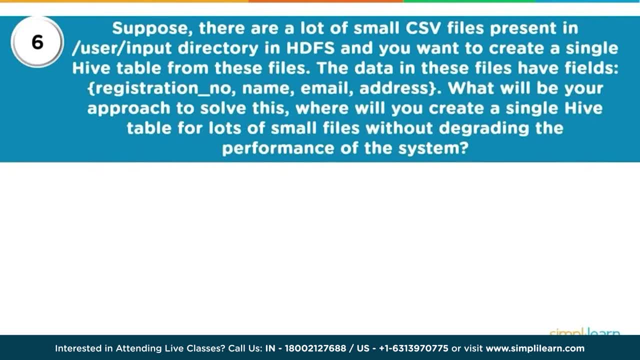 SDFS directory and you want to create a single Hive table from these files. So data in these files have fields like registration number, name, email address. So if this is what needs to be done, what will be your approach to solve it? Where will you create? 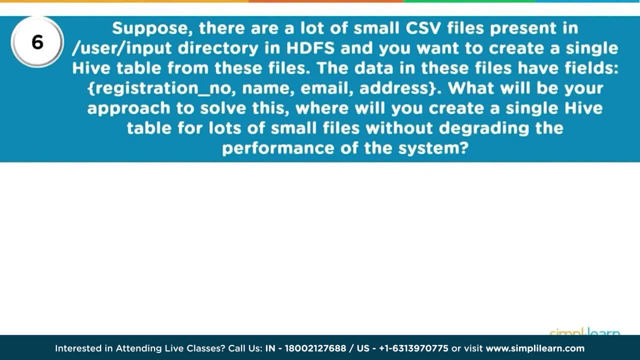 a single Hive table for lots of small files without degrading the performance of the system. So there can be different approaches. Now we know that there are lot of small CSV files which are present in a directory, So we know that when we create a 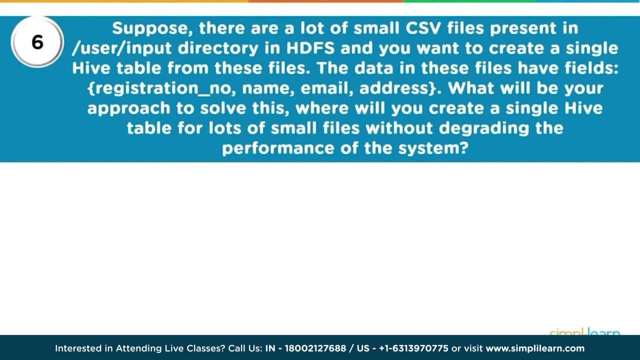 table. in Hive we can use a location parameter. So I go and say: create table, give a table name, give the column and their data types, I could specify the delimiters and finally I could say location and then point it to a directory on SDFS and this directory. 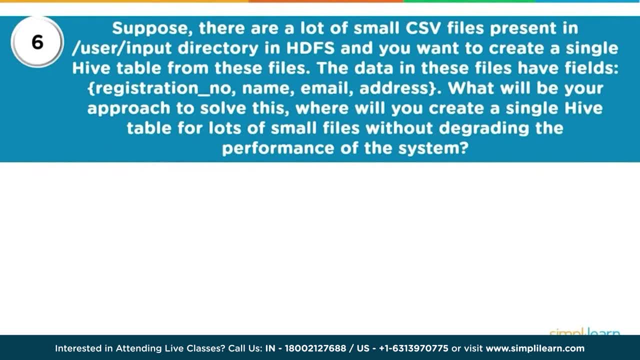 might be the directory which has lot of CSV files. So in this case I will avoid loading the data in the table, because table pointing to the directory will directly pick up the data from one or multiple files, and we also know that Hive does schema check on read. 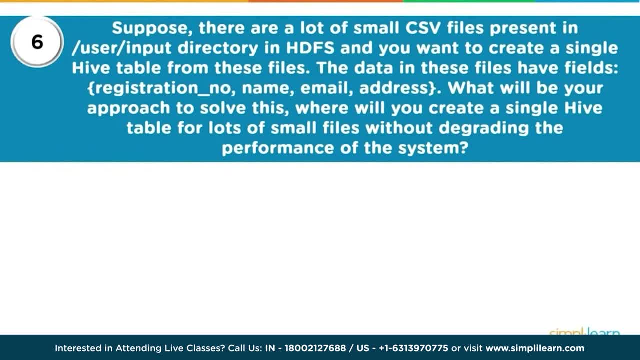 So it does not do a schema check on write. So in case there were one or two files which did not follow the schema of the table, it would not prevent data loading. Data would anyways be loaded. Only when you query the data. it might show you null values. 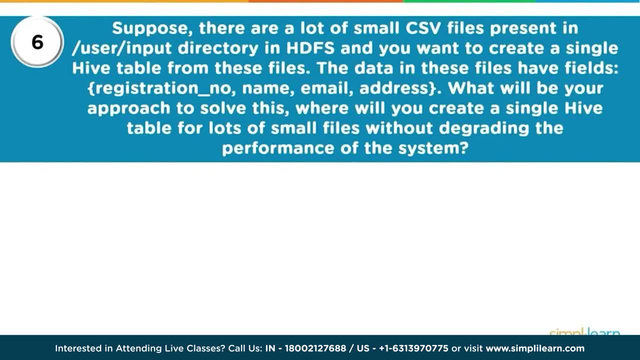 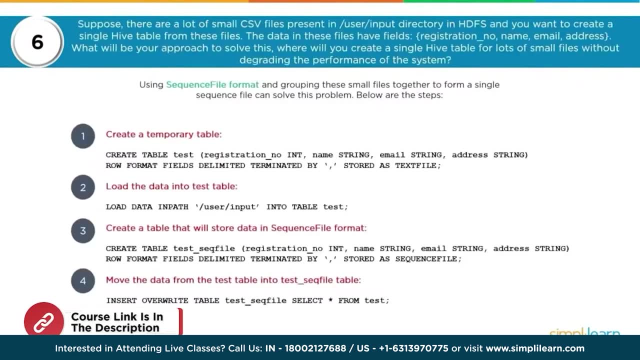 if data which was loaded does not follow the schema of the table. This is one approach. What is the other approach? So let's look at that. You can think about sequence file format, which is basically a smart format, or a binary format, and you can 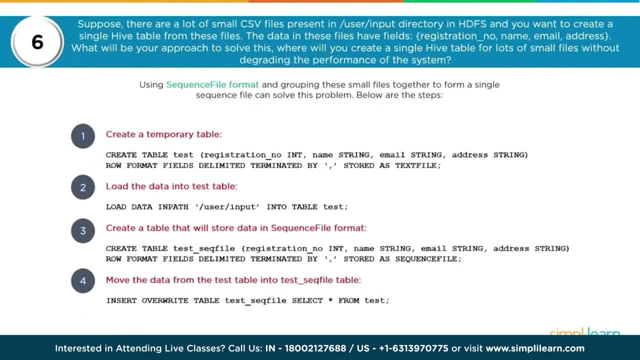 group these small files together to form a sequence file. Now this could be one other smarter approach. So we could create a temporary table. so we could say: create table, give a table name, give the column names and their data types. We could specify the delimiters as it shows here. 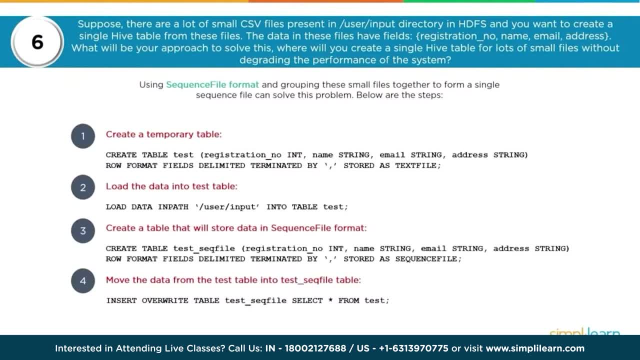 that is, row format and fields terminated by and. finally, we can store that as text file, Then we can load data into this table by giving a local file system path and then we can create a table that will store data in sequence file format. So my point one is storing the 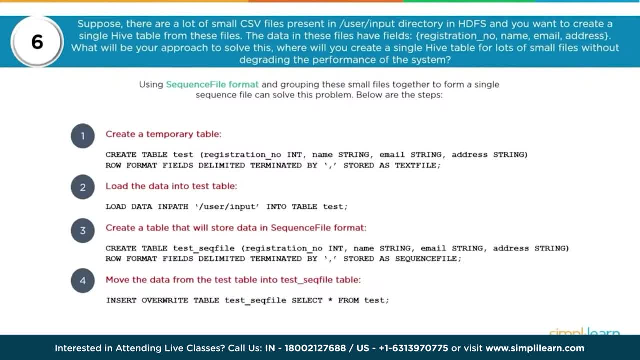 data in text file. Point three would be storing the data in sequence file format. So we say create table, give the specifications, we say row format: delimited fields are terminated by comma. stored as sequence file. Then we can move the data from test table into test sequence. 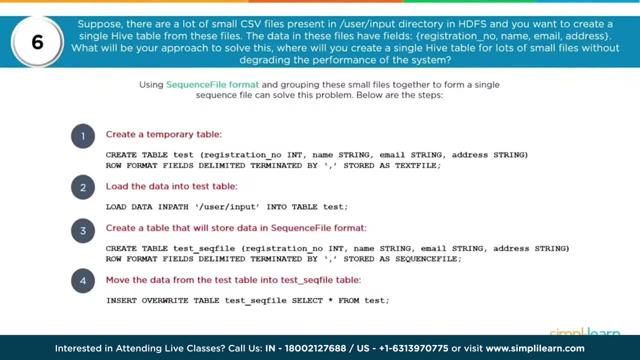 file table. So I could just say: insert, overwrite my new table as select star from other table. Remember, in hive you cannot do insert, update, delete. However, if the table is existing, you can do a insert overwrite from an existing table into a new table. So this could be one. 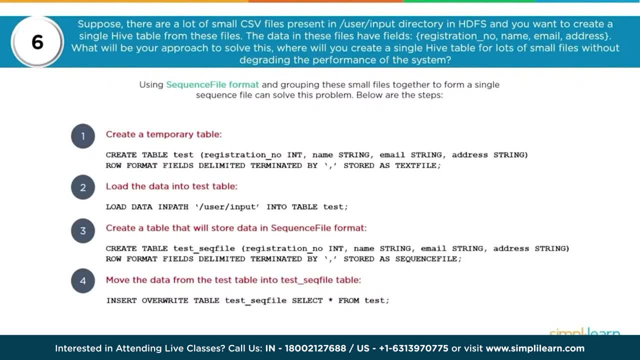 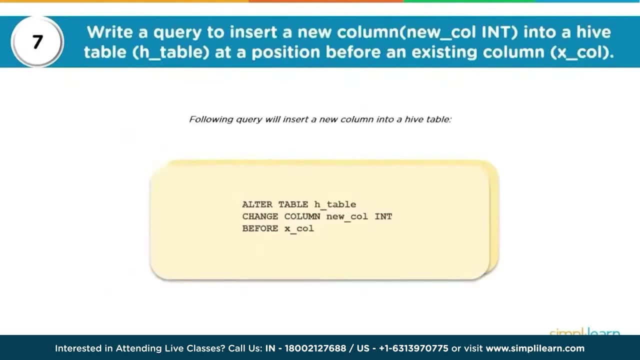 approach where we could have lot of CSV files or smaller files club together as one big sequence file and then store it in the table. Now if somebody asks you write a query to insert a new column that is integer data type into a hive table and the requirement might be that 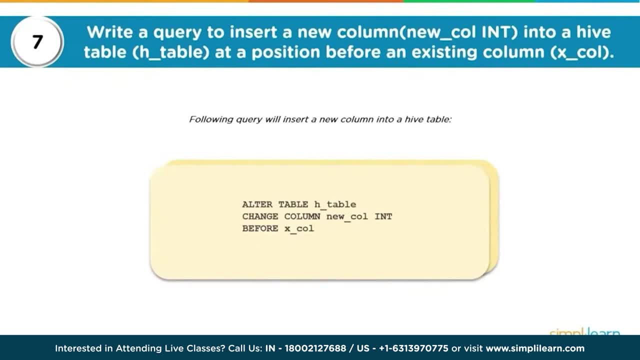 you would want to insert this table at a position before an existing column. Now that's possible by doing an alter table, giving you a table name and then specifying change column, giving you a new column with the data type before an existing column. This is a simple 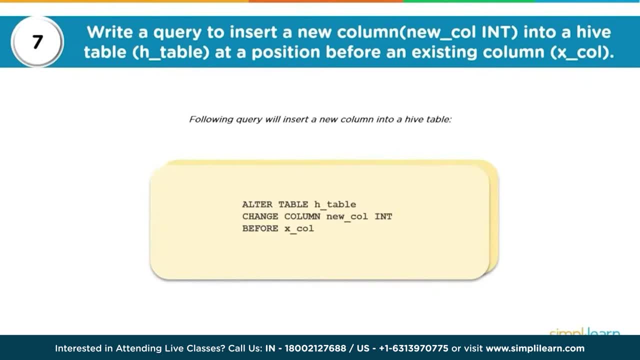 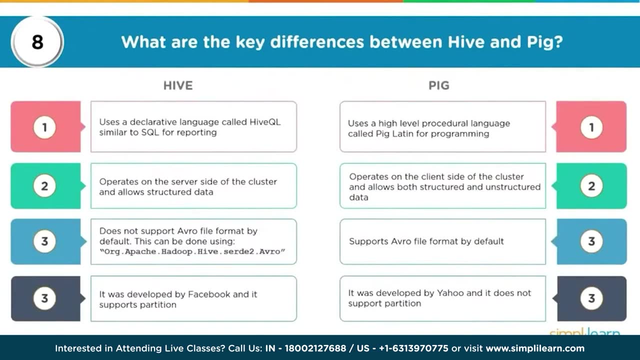 way wherein you can insert a new column into a hive table. What are the key differences between hive and pig? Now, some of you might have heard: hive is a data warehousing package and pig is more of a scripting language. Both of them are used for data analysis. 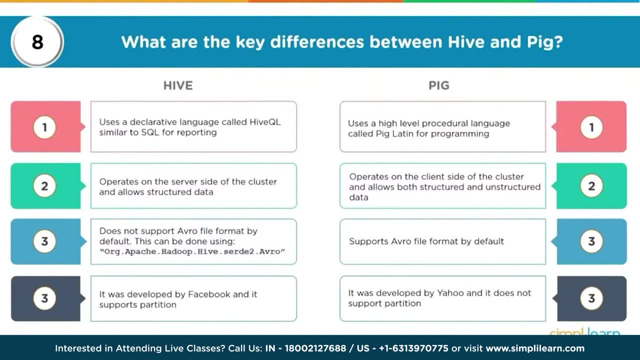 trend detection, hypothesis testing, data transformation and many other use cases. So if we compare hive and pig, hive uses a declarative language called hiveql, that is hive querying language, similar to SQL, and it is for reporting or for data analysis, even for data transformation or for. 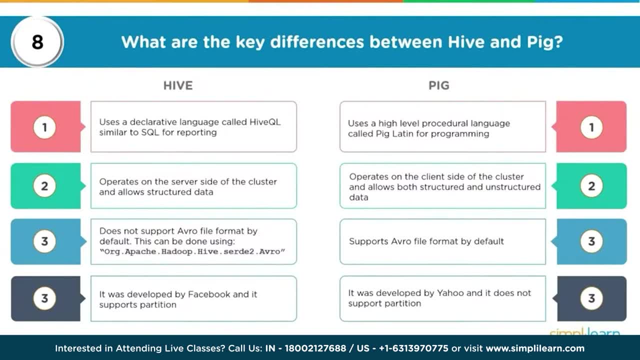 your data extraction. Pig uses a high level procedural language called pig latin for programming. Both of them- remember, use map reduce processing framework. So when we run a query in hive to process the data or when we create and submit a pig script, both of them trigger a map reduce job. 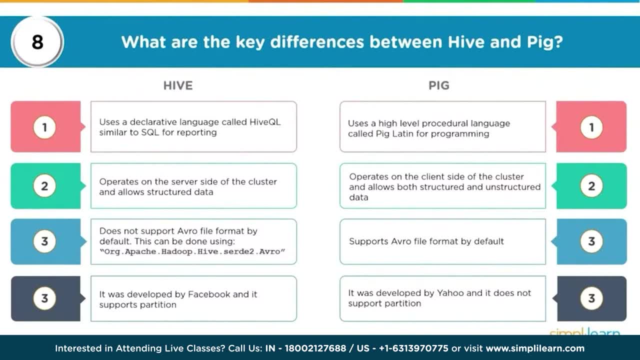 unless and until we have set them to local mode. Hive operates on the server side of the cluster and basically works on structured data or data which can be structurized. Pig usually works or operates on the client side of the cluster and allows both structured 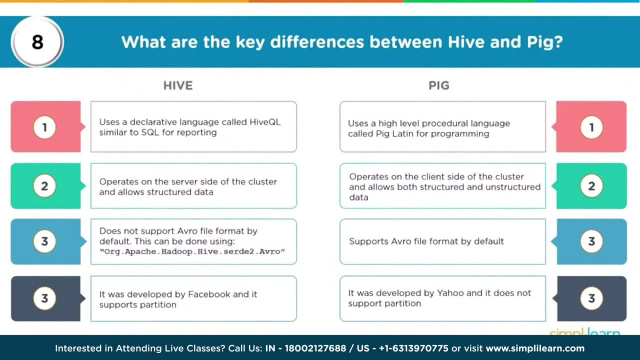 unstructured, or even I could say semi structured data. Hive does not support Avro file format by default. However, that can be done by using the right serializer deserializer, So we can have hive table related data stored in Avro format in sequence file. 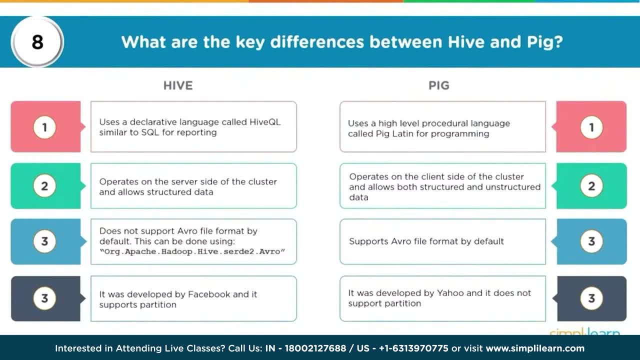 format, in parquet format or even as a text file format. However, when we are working on smarter formats like Avro or sequence file or parquet, we might have to use specific serializers- deserializers For Avro. this is the package which allows us to use Avro. 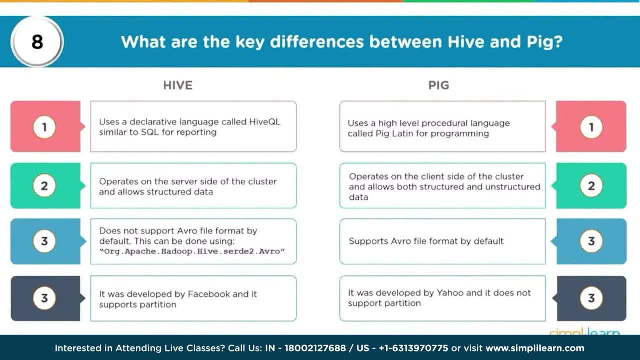 format. Pig supports Avro format by default. Hive was developed by Facebook and it supports partitioning, and pig was developed by yahoo and it does not support partitioning. So these are high level differences. There are lots and lots of differences. Remember, hive is more of a. 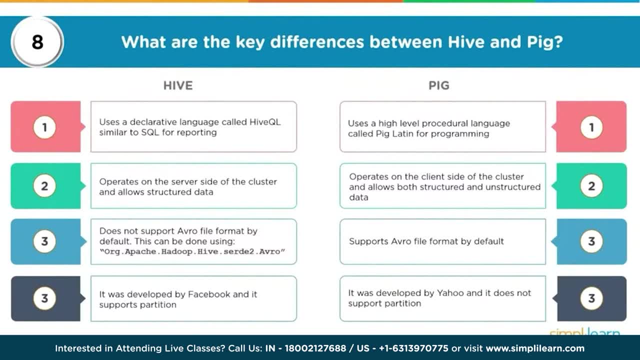 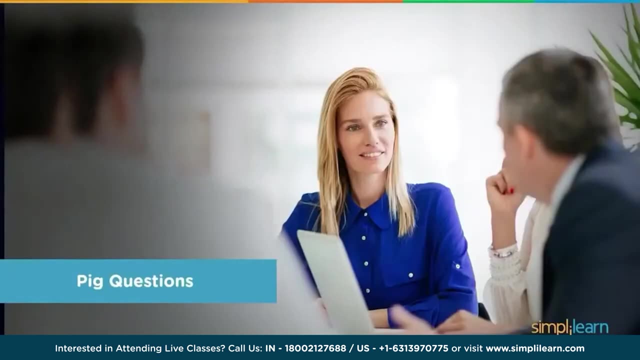 data warehousing package, and pig is more of a scripting language or a strictly procedural flow following scripting language, which allows us to process the data. Now let's get more, and let's get more deeper and learn about pig, which is, as I mentioned, a scripting language. 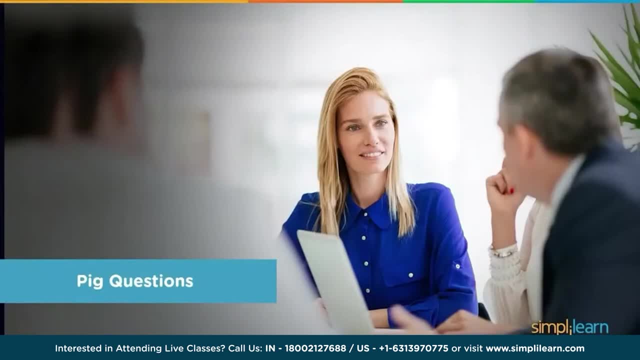 which can be used for your data processing. It also uses MapReduce, although we can even have pig run in a local mode. Let's learn about pig in the next section. Now let's learn on some questions about pig, which is a scripting language, and it is extensively. 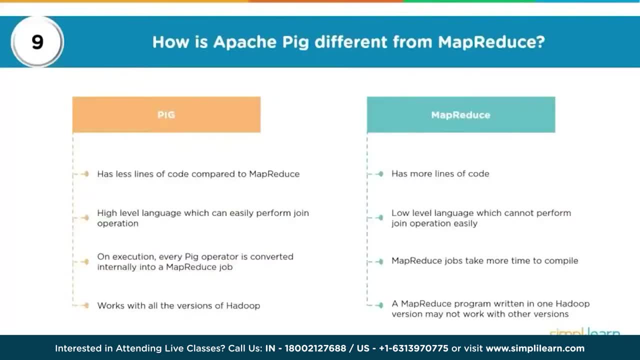 used for data processing and data analysis. So the question is: how is Apache pig different from MapReduce? Now, we all know that MapReduce is a programming model. It is. it's quite rigid when it comes to processing the data, because you have to do the mapping and reducing. 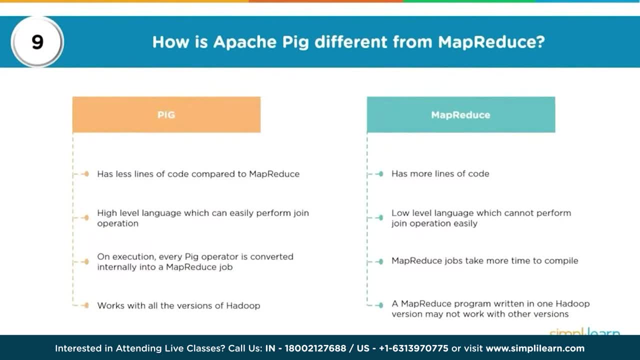 You have to write huge code. Usually MapReduce is written in Java, but now it can also be written in Python. it can be written in Scala and other programming languages. So if we compare pig with MapReduce, pig obviously is very concise. it has less lines of. 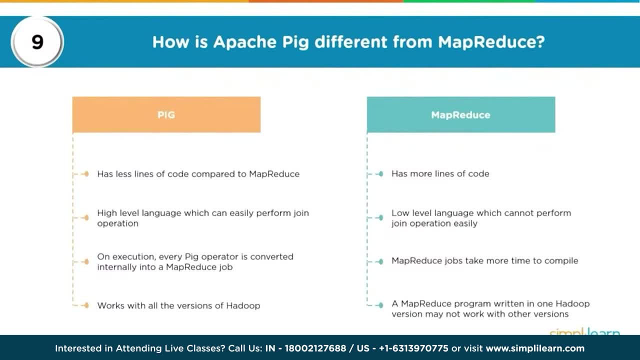 code when compared to MapReduce. Now we also know that pig script internally will trigger a MapReduce job. However, user need not know about MapReduce programming model. They can simply write simple scripts in pig and that will automatically be converted into MapReduce. However, MapReduce has 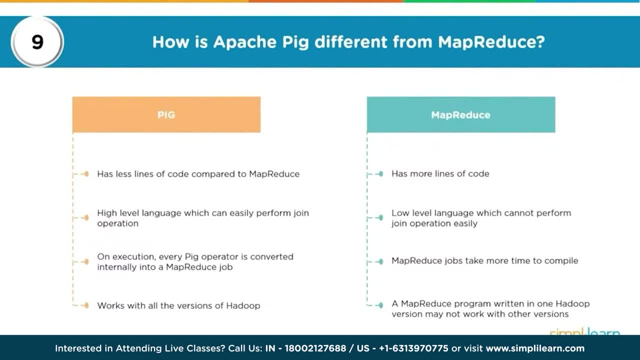 more lines of code. Pig is high level language which can easily perform join operations or other data processing operations. MapReduce is a low level language which cannot perform job join operations easily. So we can do join using MapReduce. however, it's not really easy. 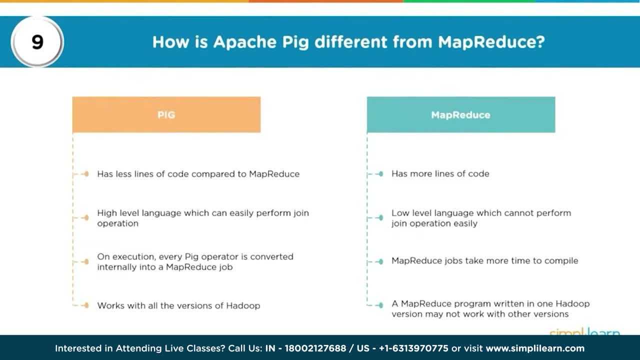 in comparison to pig. Now, as I said, on execution every pig operator is converted internally into a MapReduce job. So every pig script which is run which would be converted into MapReduce job. Now, MapReduce overall is a batch oriented processing, so it takes 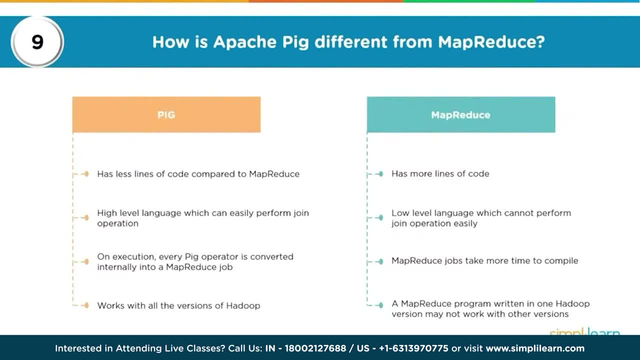 more time to compile. it takes more time to execute either when you run a MapReduce job or when it is triggered by pig script. Pig works with all versions of Hadoop and when we talk about MapReduce program, which is written in one Hadoop version. 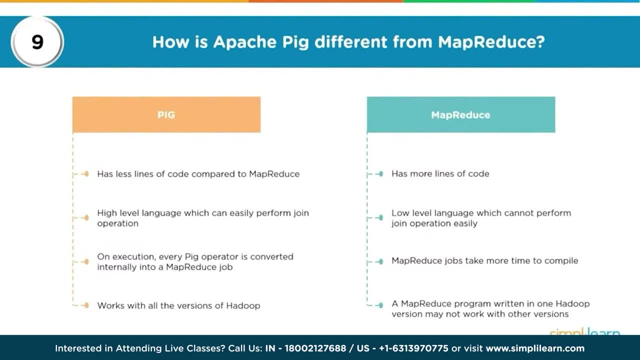 may not work with other versions. It might work or it might not. It depends on what are the dependencies, what is the compiler you are using, what programming language you have used and what version of Hadoop you are working on. So these are the main. 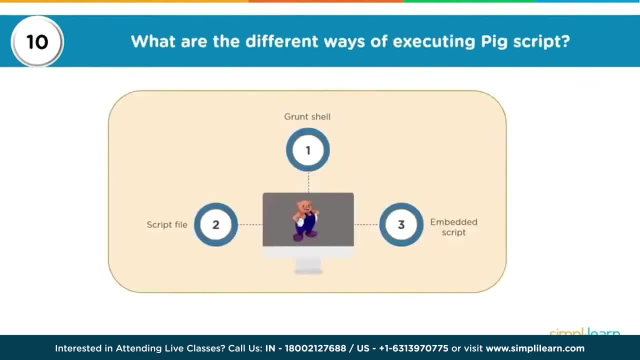 differences between Apache, pig and MapReduce. What are the different ways of executing pig script? So you could create a script file, store it in dot pig or dot text and then you could execute it using the pig command. You could be bringing up the grunt. 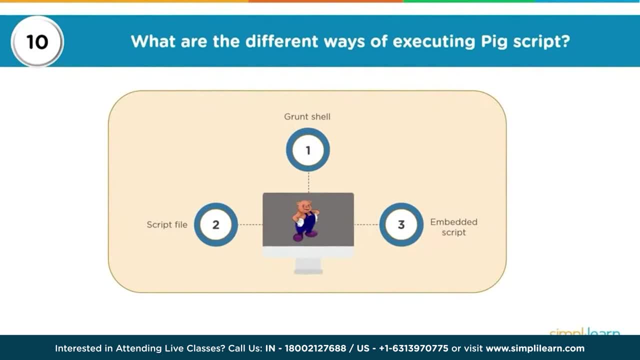 shell, that is pig's shell. Now that usually starts with MapReduce mode, but then we can also bring it up in a local mode and we can also run pig embedded as an embedded script in other programming language. So these are the different ways of executing your. 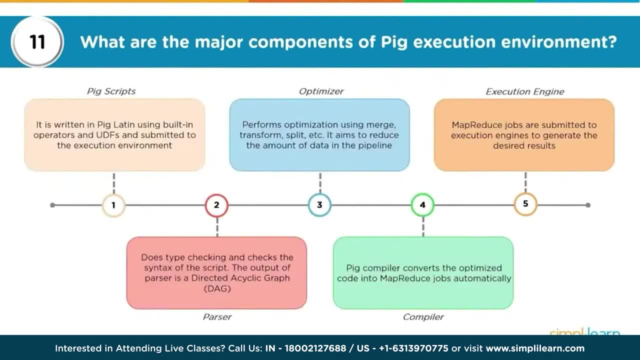 pig script. Now, what are the major components of pig execution environment? This is a very common question. Interviewers would always want to know different components of Hive, different components of pig, even different components which are involved in Hadoop ecosystem. So when we want to 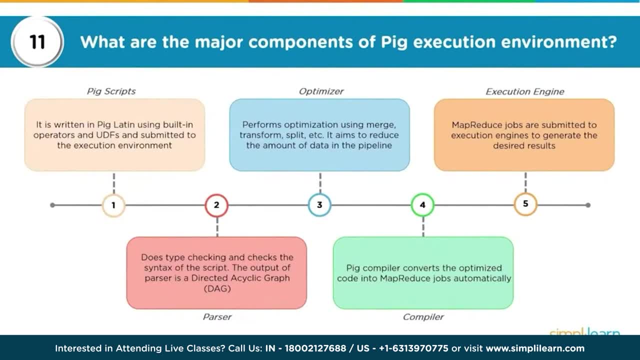 learn about major components of pig execution environment. here are some. So you have pig scripts Now that is written in pig Latin using built-in operators and user defined functions and submitted to the execution environment. That's what happens when you would want to process the data. 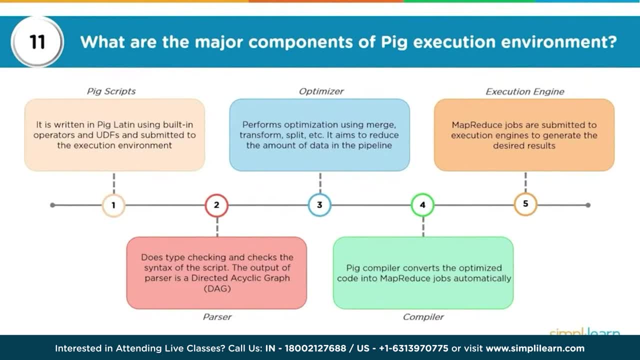 using pig. Now there is a parser which does type checking and checks the syntax of the script. The output of parser is a DAG direct acyclic graph. So look in Wikipedia for DAG. So DAG is basically a sequence of steps which run in one direction. Then you have 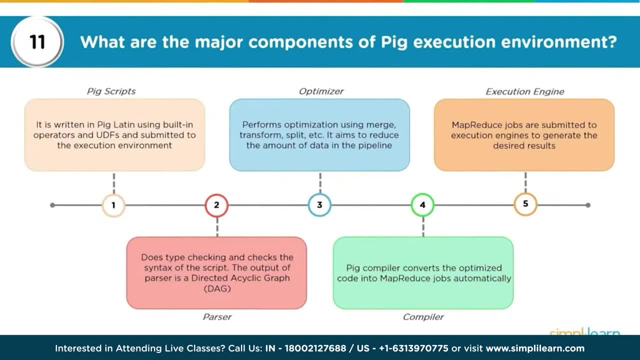 an optimizer. Now this optimizer performs optimization using merge, transform, split, etc. It aims to reduce the amount of data in the pipeline. That's the whole purpose of optimizer. You have a internal compiler, So pig compiler converts the optimizer optimized code into a 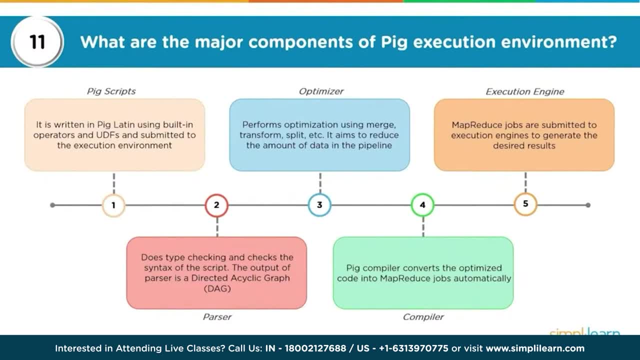 MapReduce job. And here user need not know the MapReduce programming model or how it works or how it is written. They all need to know about running the pig script which would be internally converted into a MapReduce job. And finally we have an execution. 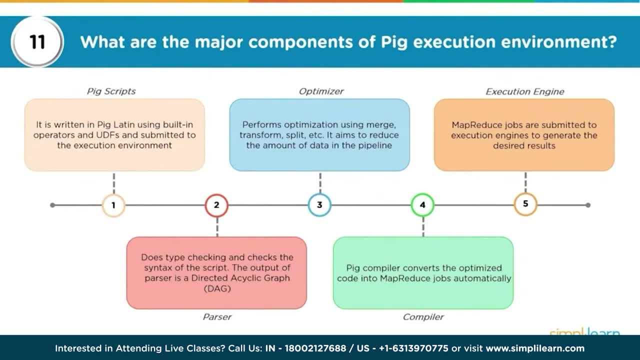 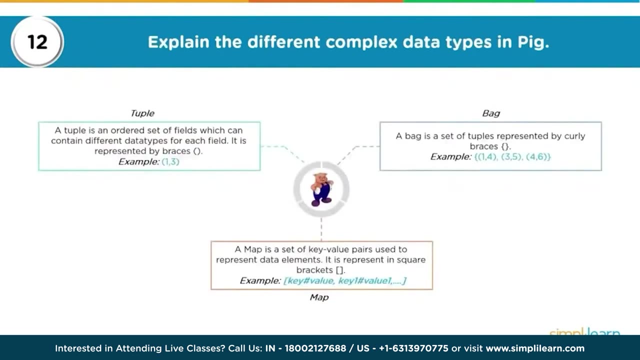 engine. So MapReduce jobs are submitted to the execution engine to generate the desired results. So these are major components of pig execution environment. Now let's learn about different complex data types in pig. Pig supports various data types. The main ones are tuple bag. 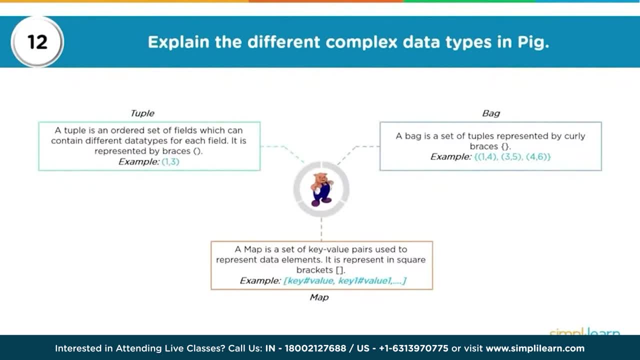 and map. What is tuple or tuple? As you might have heard, tuple is an ordered set of fields which can contain different data types for each field. So in array you would have multiple elements but that would be of same types. List can also have different types. 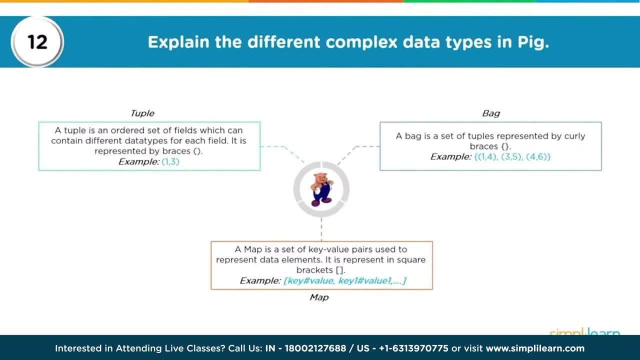 Your tuple is a collection which has different fields and each field can be of different type. Now we could have an example as 1 comma 3 or 1 comma 3 comma, a string or a float element and all of that form. a tuple Bag is a set of. 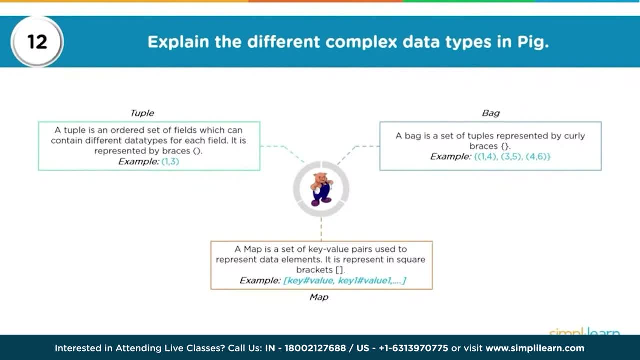 tuples, So that's represented by curly braces. So you could also imagine this like a dictionary which has various different collection elements. What is a map? Map is a set of key value pairs used to represent data. So when you work in big data field, you need 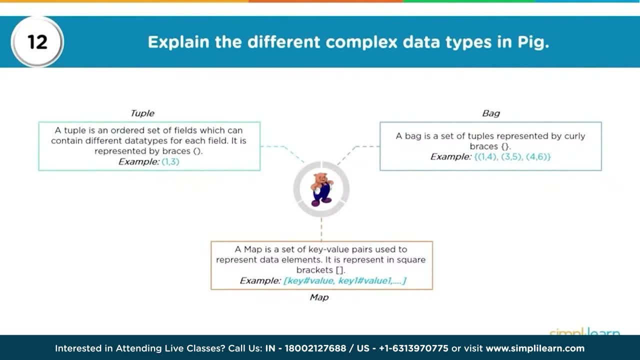 to know about different data types which are supported by pig, which are supported by hive, which are supported in other components of Hadoop. So, tuple bag, map, array, array, buffer. you can think about list, you can think about dictionaries, you can think about 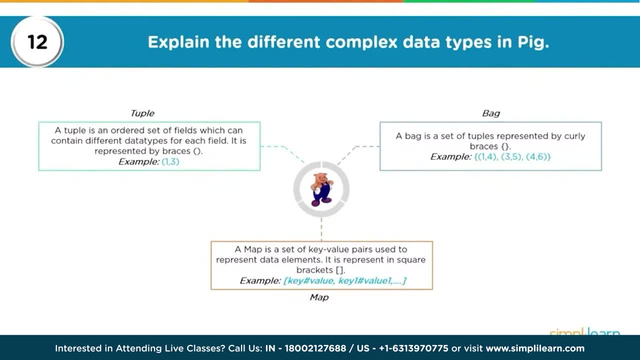 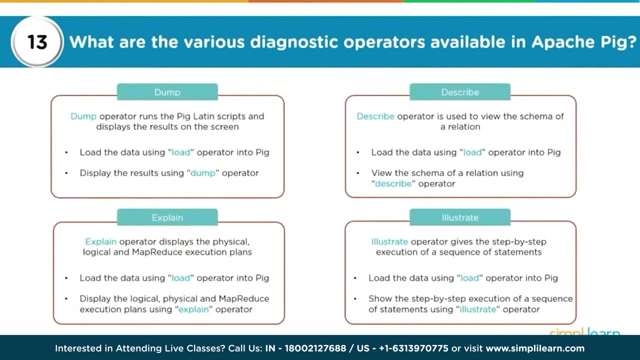 map, which is key value pair. so these are your different complex data types, other than the primitive data types, such as integer, character string, boolean, float and so on. Now, what are the various diagnostic operators available in Apache pig? So these are some of the operators, or 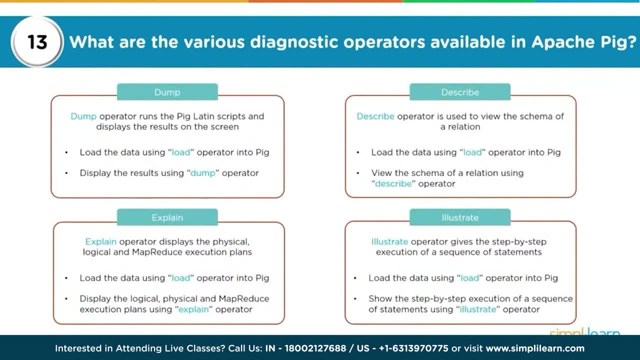 options which you can give in a pig script. You can do a dump. Now. dump operator runs the pig latin scripts and displays the result on the screen. So either I could do a dump and see the output on the screen or I can even do a dump into. 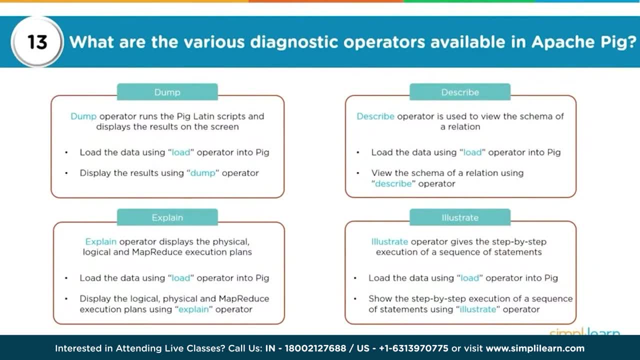 and I could store my output in a particular file So we can load the data using load operator in pig. and then pig also has different internal storage, like JSON loader or pig storage, which can be used if you are working on specific kind of data and then 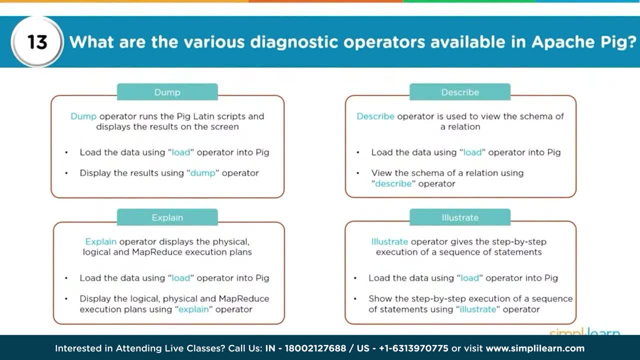 you could do a dump, either before processing or after processing, and dump would produce the result. The result could be stored in a file or seen on the screen. You also have a describe operator now that is used to view the schema of a relation, So you can load the. 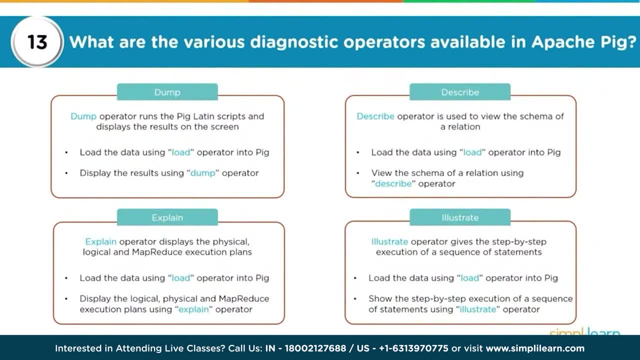 data and then you can view the schema of relation using: describe, operator, Explain. as we might already know, displays the physical, logical and map reduce execution plans. Normally in RDBMS when we use explain. we would like to see what happens behind the scenes when a particular 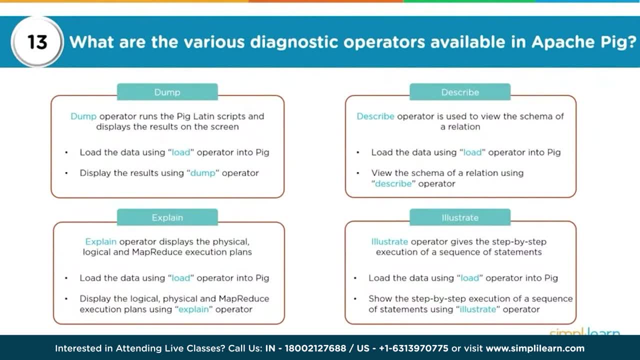 script or a query runs. So we could load the data using load operator as in any other case, and if we would want to display the logical, physical and map reduce execution plans, we could use explain operator. There is also an illustrate operator Now that gives the step by step. 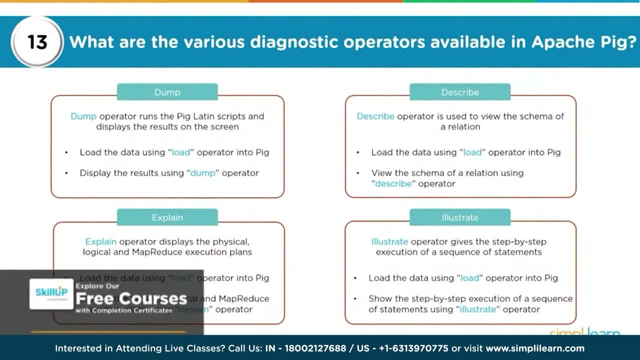 execution of sequence of statement. So sometimes when we would want to analyze our script to see how good or bad they are, or would that really serve our purpose, we could use illustrate. and again, you can test that by loading the data using load operator and you could. 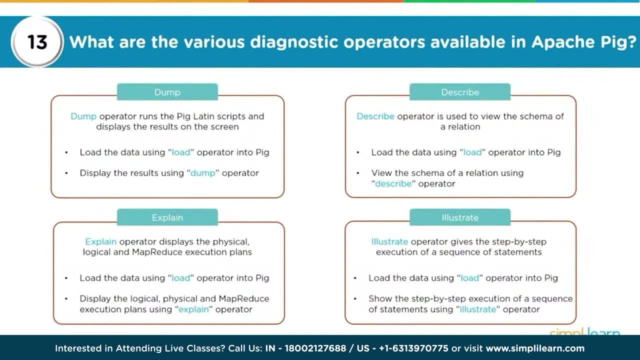 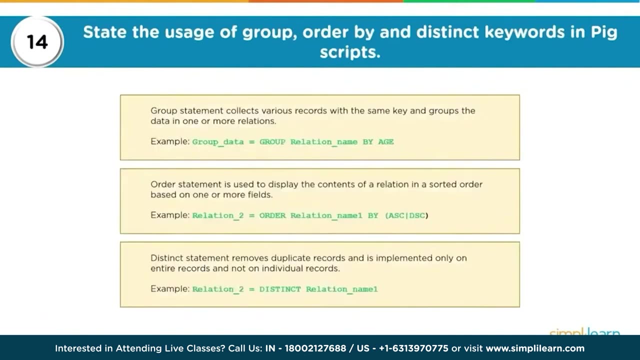 just use illustrate operator to have a look at the step by step execution of the sequence of statements which you would want to execute. So these are different diagnostic operators available in Apache PIC. Now, if somebody asks state the usage of group order by and string keywords in PIC script. 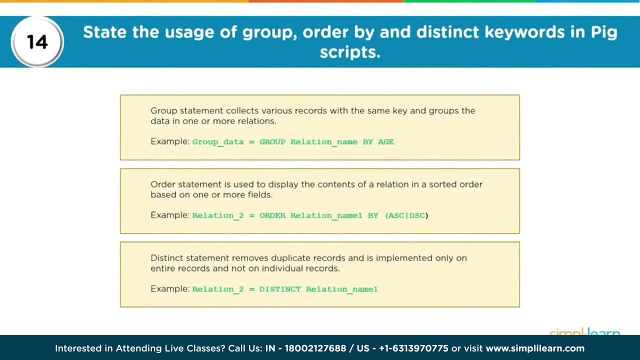 So, as I said, PIC is a scripting language so you could use various operators. so group basically collects various records with the same key and groups the data in one or more relations. Here is an example: You could do a group data. so that is basically a variable, or you can give some other name. 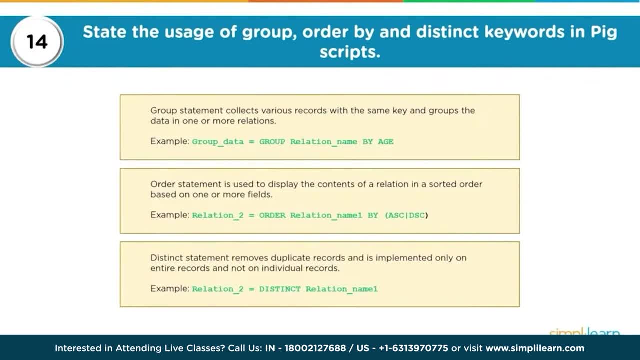 and you can say group relation name by age. Now, say, I have a file where I have field, various fields, and one of the field is relation name. so I could group that by a different field. Order by is used to display the contents of relation in a sorted order, whether 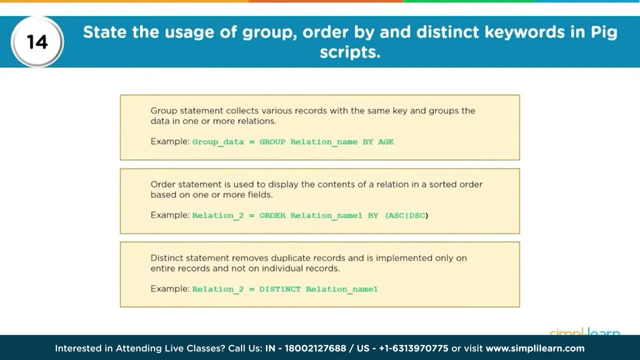 ascending or descending. So I could create a variable called relation two and then I could say order relation name one by ascending or descending order Distinct basically removes the duplicate records and it is implemented only on entire records, not on individual records. So if you would want to find out the 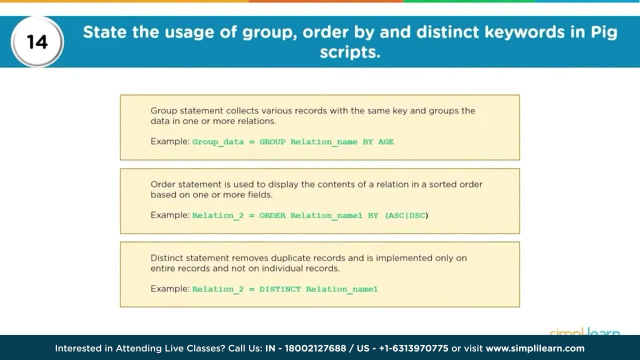 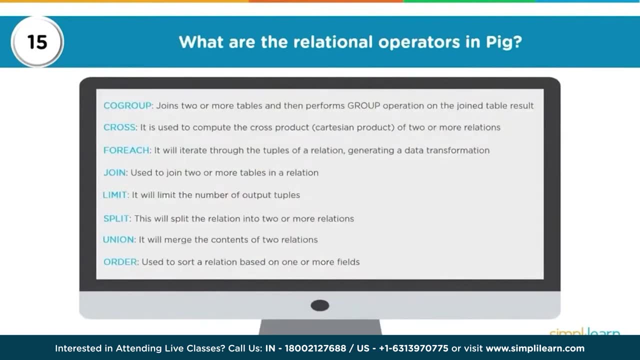 distinct values and relation names of a field, I could use distinct. What are the relational operators in PIG? So you have various relational operators which help data scientists or data analysts or developers who are analyzing the data, such as co-group which joins two or more. 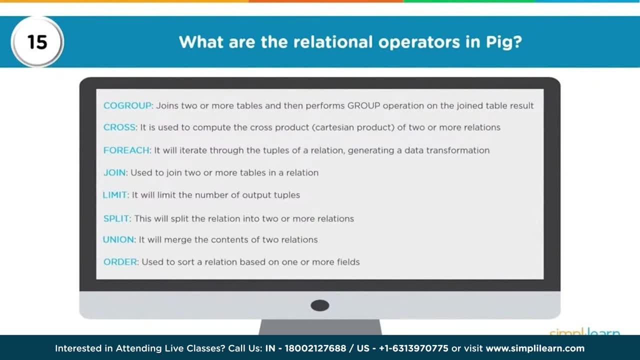 tables and then performs group operation on the join table. result: You have cross. It is used to compute the cross product, that is a Cartesian product of two or more relations, For each is basically to do some iteration. So if it will iterate through tuples of a relation, 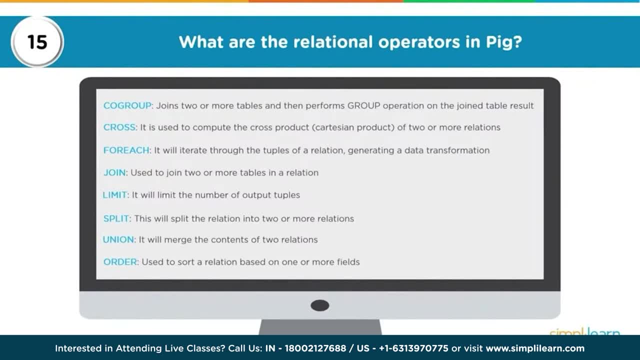 generating a data transformation. So, for example, if I say variable A equals, and then I load a file in A and then I could create a variable called B where I could say, for each A I would want to do something. say, group Join is to join two or more. 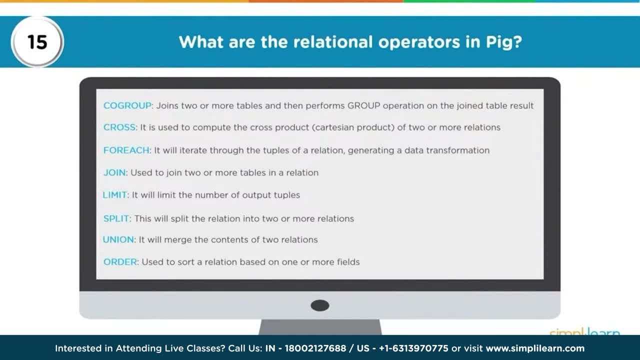 tables in a relation. Limit is to limit the number of output tuples or output results. Split is to split the relation into two or more relations. Union is to get a combination that it will merge the contents of two or more relations, and order is to get a sorted result. So these 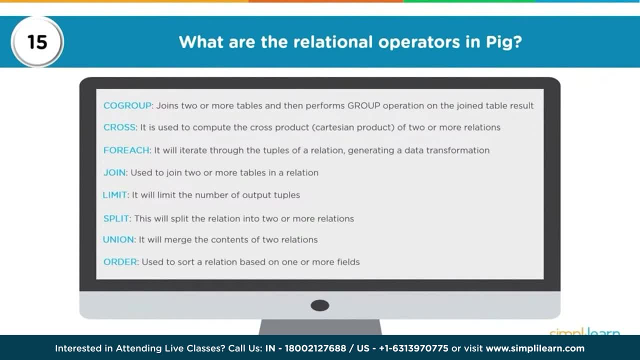 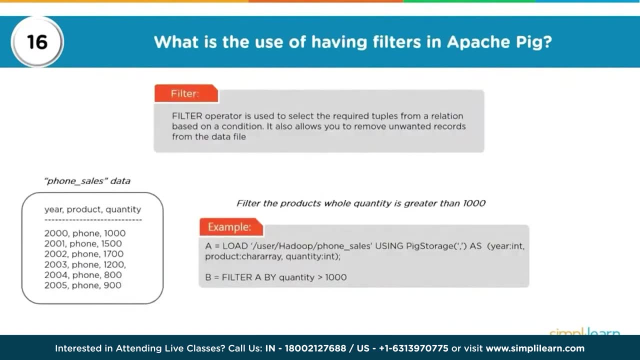 are some relational operators which are extensively used in PIG for analysis. What is the use of having filters in Apache PIG? Now say, for example, I have some data which has three fields: year, product quantity and this is my phone sales data. So filter. 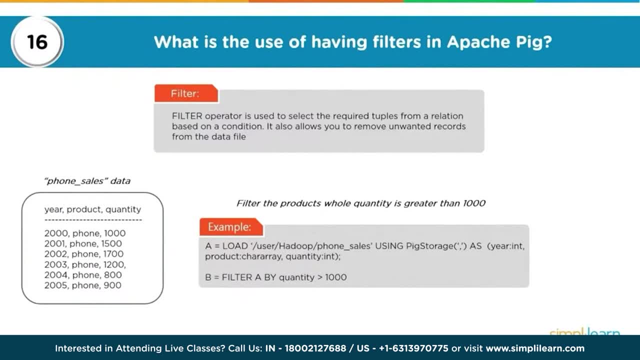 operator could be used to select the required values from a relation based on a condition. It also allows you to remove unwanted records from data file, So, for example, filter the products where quantity is greater than 1000.. So I see that I have one. 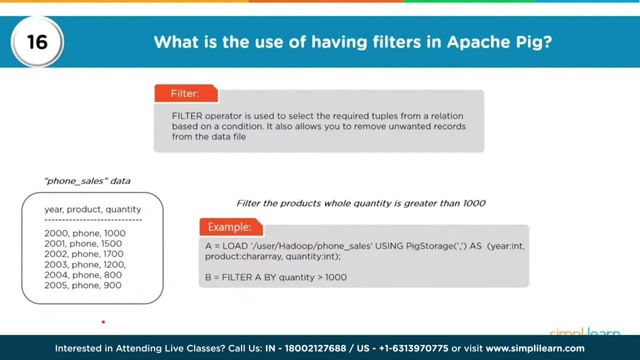 row wherein, or multiple rows where the quantity is greater than 1000, such as 1500, 1700, 1200.. So I could create a variable called A. I would load my file using PIG storage, as I explained earlier. PIG. 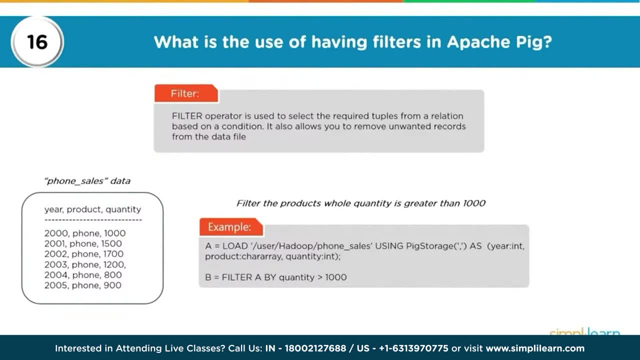 storage is an internal parameter which can be used to specify the delimiters. Now, here my delimiter is comma, So I could say, using PIG, storage as, and then I could specify the data type for each field, So year being integer, product being character. 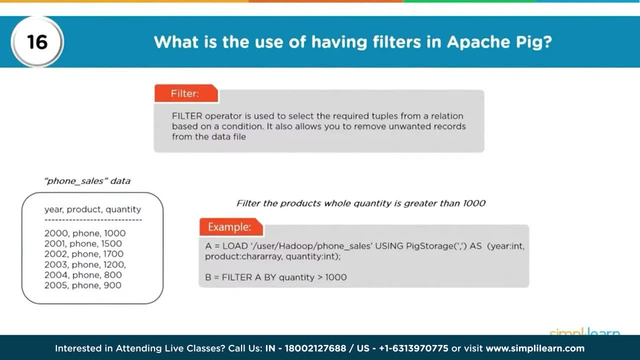 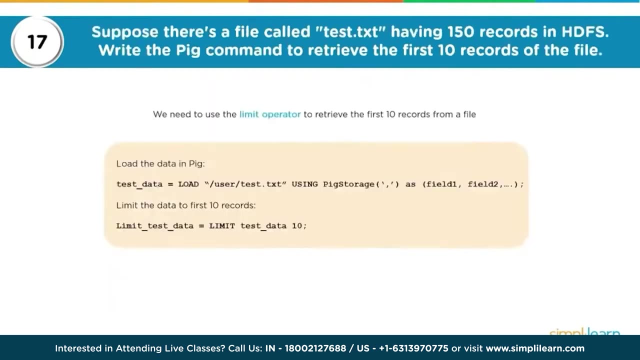 array and quantity being integer, Then B, I could say filter A, whatever we have in A, by quantity greater than 1000.. So it's very concise, it's very simple and it allows us to extract and process data in a simpler way. Now suppose there is a file called testtxt. 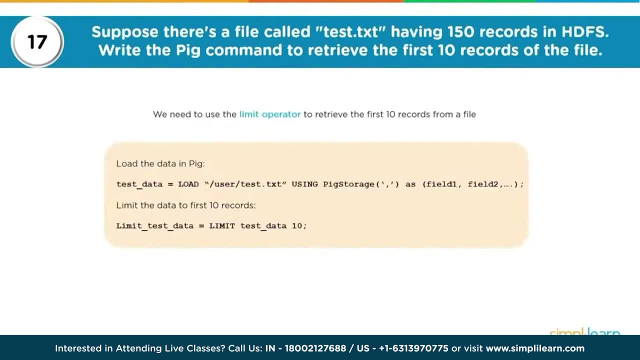 having 150 records in its DFS. So this is a file which is stored on its DFS and it has 150 records where we can consider every record being one line And if somebody asks you to write a PIG command to retrieve the first 10 records of 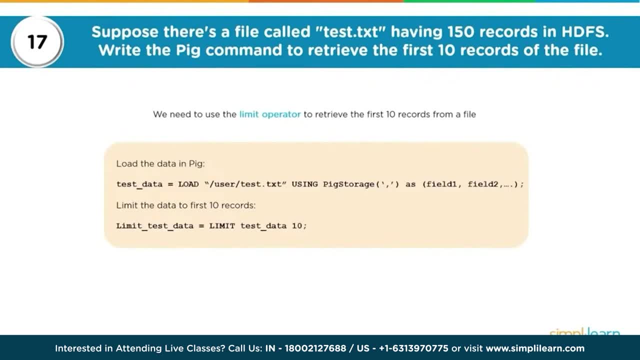 the file. First we will have to load the data. So I could create a variable called test underscore data and I would say: load my file using PIG storage, specifying the delimiter as, comma as, and then I could specify my fields, whatever fields our file have, and then 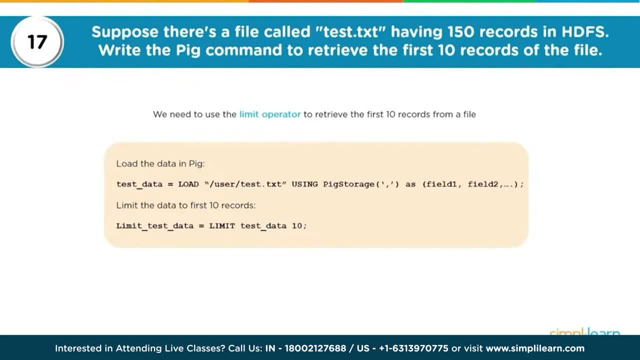 I would want to get only 10 records for which I could use the limit operator, So I could say limit on test data and give me 10 records. This is very simple and we can extract 10 records from 150 records which are stored in the file on its DFS. 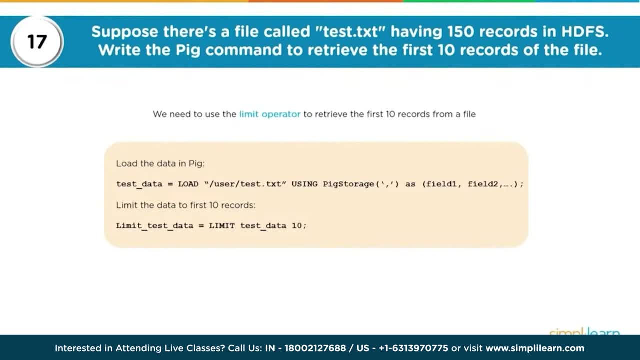 Now we have learnt on PIG. We have learnt some questions on HIF. You could always look more in books like programming in HIF or programming in PIG and look for some more examples and try out these examples on a existing Hadoop setup. Now let's learn. 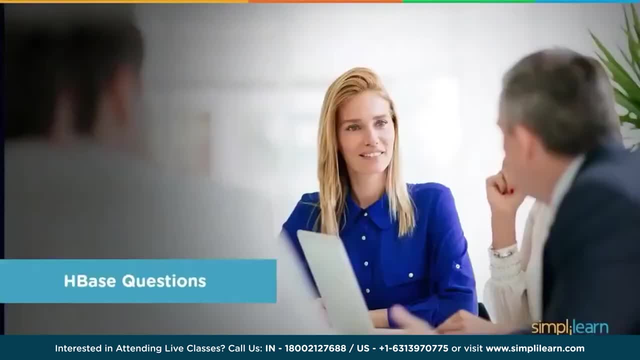 on HBase, which is a NoSQL database. Now HBase is a 4 dimensional database in comparison to your RDBMS, which usually are 2 dimensional. So RDBMS have rows and columns, but HBase has 4 coordinates, It has row. key, which is always unique, column family, which can be any number. column qualifiers, which can again be any number per column family, and then you have a version. So these 4 coordinates make HBase a 4 dimensional key value store or a column family store. 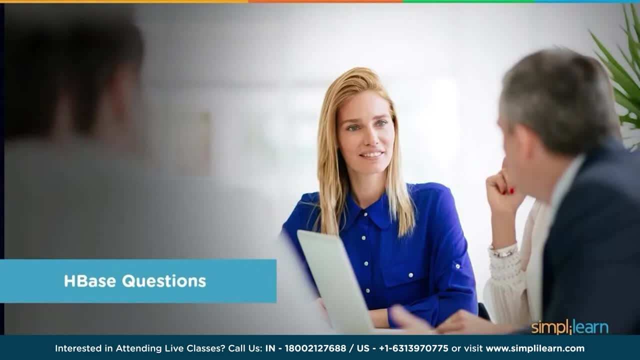 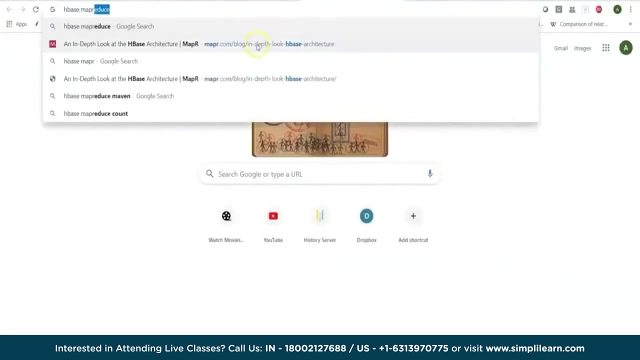 which is unique for storing huge amount of data and extracting data from HBase. There is a very good link which I would suggest everyone can look at if you would want to learn more on HBase, and you could just say HBase mapper and this basically brings up. 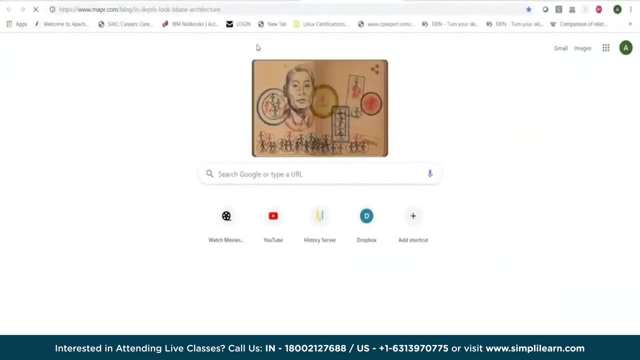 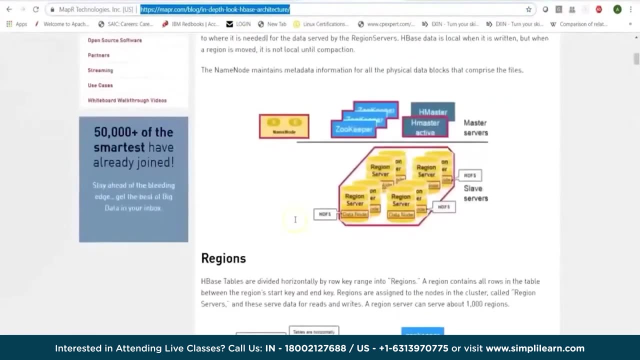 a documentation which is from mapper, but then that's not specific to mapper and you can look at this link which will give you a detailed explanation of HBase: how it works, what are the architectural components and how data is stored and how it makes HBase. 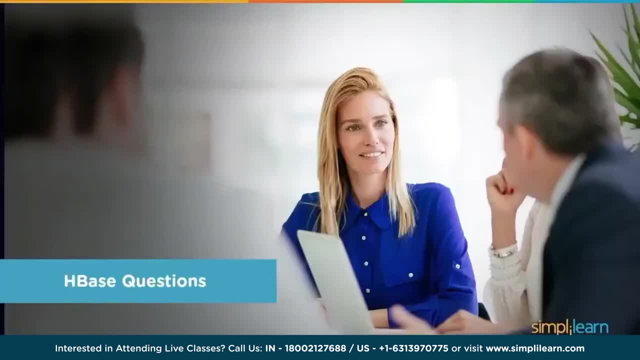 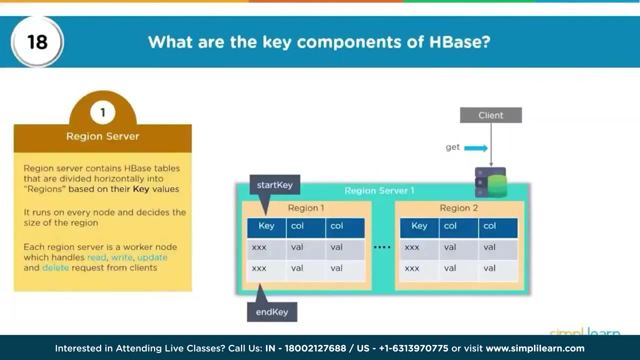 a very powerful NoSQL database. So let's learn on some of the important or critical questions on HBase which might be asked by the interviewer in an interview when you are applying for a big data admin or a developer position role. So what are the key components of HBase? 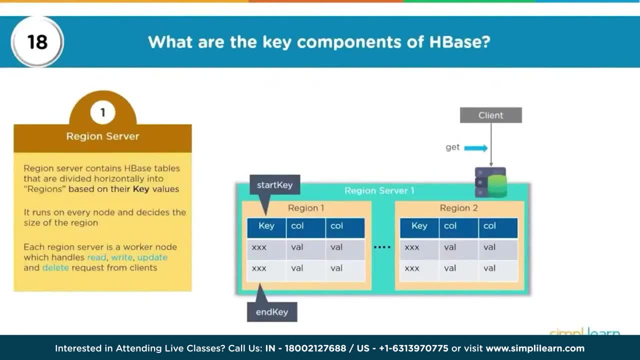 Now, as I said, this is one of the favorite questions of interviewers, where they would want to understand your knowledge on different components for a particular service. HBase, as I said, is a NoSQL database and that comes as a part of service with Cloudera or. 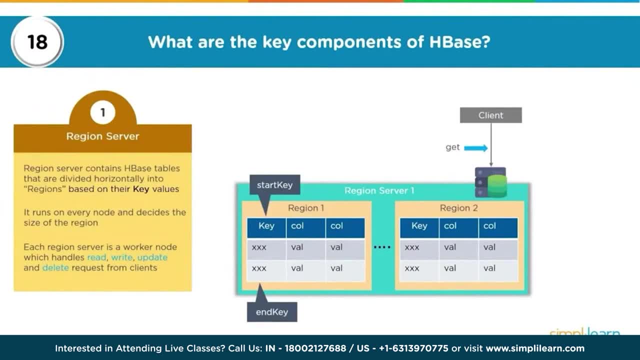 Hortonworks and with Apache Hadoop, you could also set up HBase as an independent package. So what are the key components of HBase? HBase has a region server. Now HBase follows the similar kind of topology, like Hadoop. Now Hadoop has a master process. 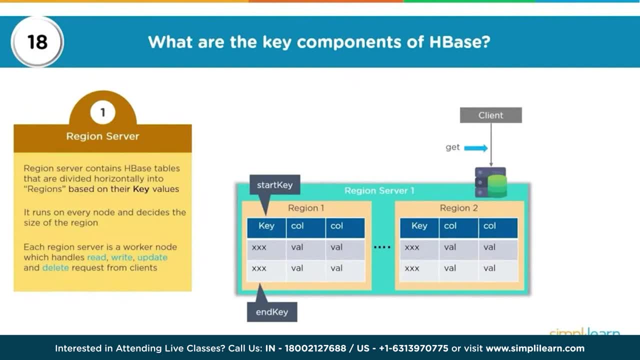 that is, name node, and slave processes such as data nodes and secondary name node. In the same way, HBase also has a master, which is H master, and the slave processes are called region servers. So these region servers are usually co-located with data nodes. 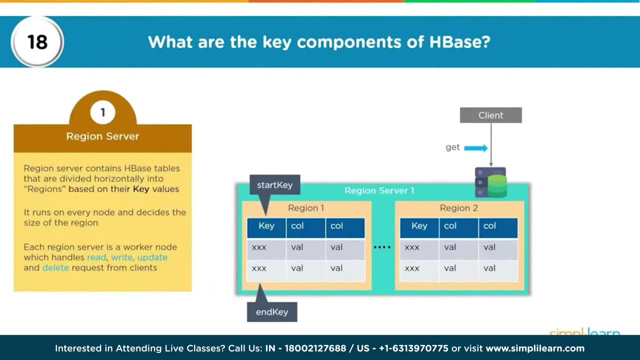 However, it is not mandatory that if you have 100 data nodes, you would have 100 region servers, So it purely depends on admin. So what does this region server contain? So region server contains HBase tables that are divided horizontally into regions, or you could. 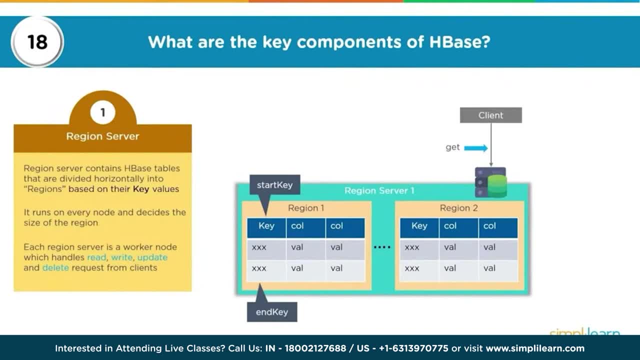 say group of rows, is called regions. So in HBase you have two aspects: One is group of columns which is called column family And one is group of rows which is called regions. Now these regions or these rows are grouped based on the key. 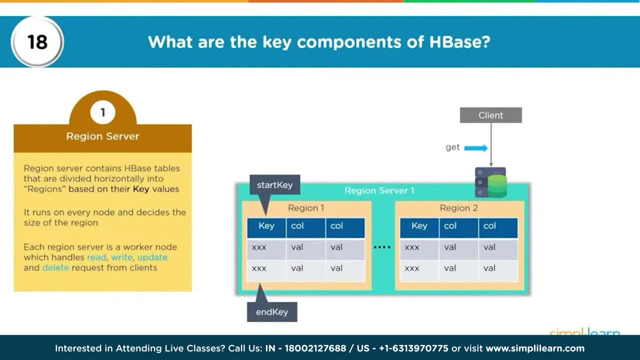 values, or I would say row keys, which are always unique. When you store your data in HBase, you would have data in the form of rows and columns, So group of rows are called regions, or you could say these are horizontal partitions of the table, So a region server. 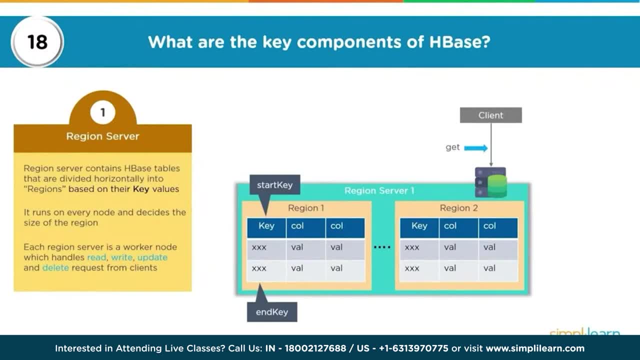 manages these regions on the node where a data node is running. A region server can have up to 1000 regions. It runs on every node and decides the size of region. So region server, as I said, is a slave process which is responsible for managing. 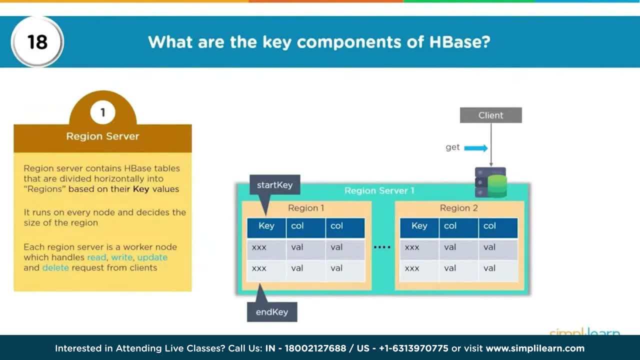 HBase data on the node. Each region server is a worker node or a worker process co-located with data node which will take care of your read, write, update, delete request from the clients. Now, when we talk about more components of HBase, as I said, 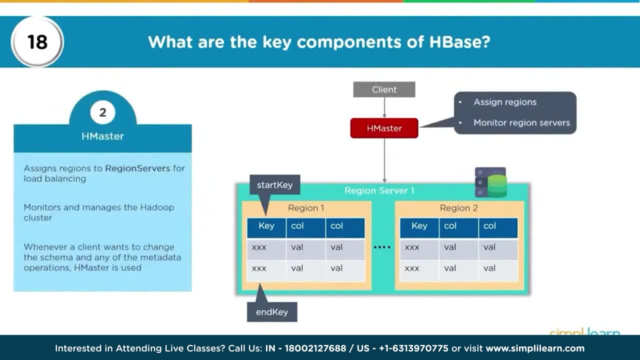 you have HMaster, so you would always have a connection coming in from a client or an application. What does HMaster do? It assigns regions, It monitors the region servers, It assigns regions to region servers for load balancing, and it cannot do that without the help of ZooKeeper. 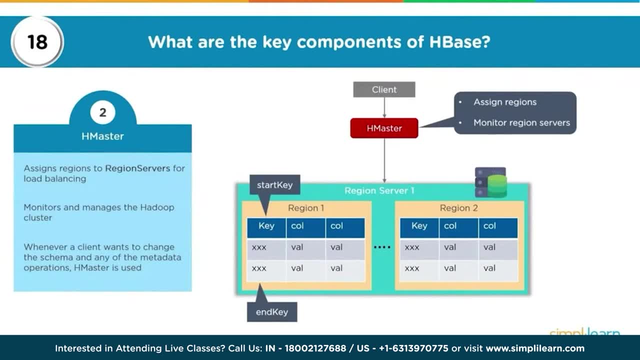 So, if we talk about components of HBase, there are three main components. You have ZooKeeper, you have HMaster and you have region server, Region server being the slave process, Your HMaster being the master process which takes care of all your table operations. 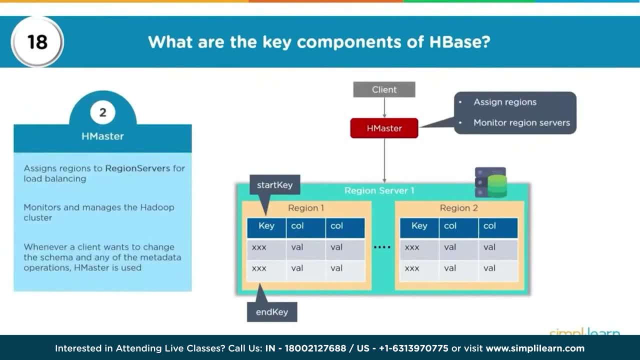 Assigning regions to the region servers, Taking care of read and write requests which come from client. and for all of this HMaster will take in help of ZooKeeper, which is a centralized coordination service. So whenever a client wants to read or write or change the schema or any other, 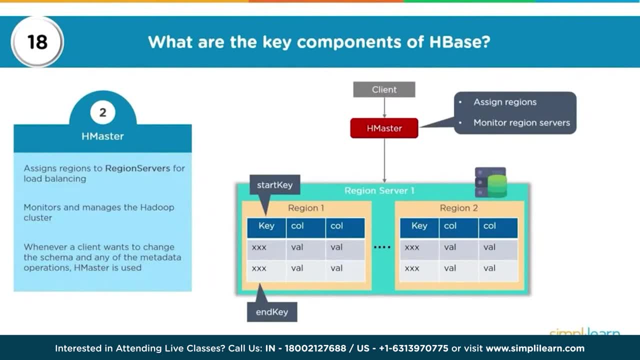 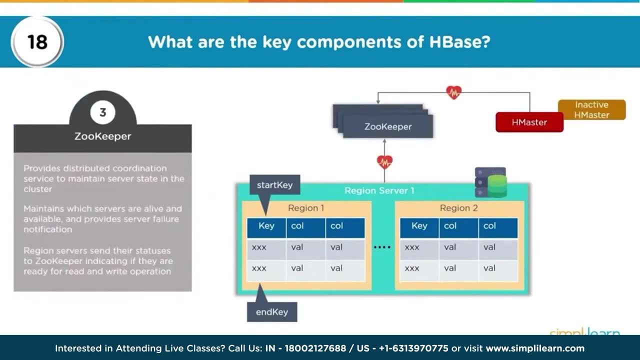 metadata operations. it will contact HMaster. HMaster internally will contact ZooKeeper So you could have HBase setup also in high availability mode where you could have an active HMaster and a backup HMaster. You would have a ZooKeeper quorum, which is the 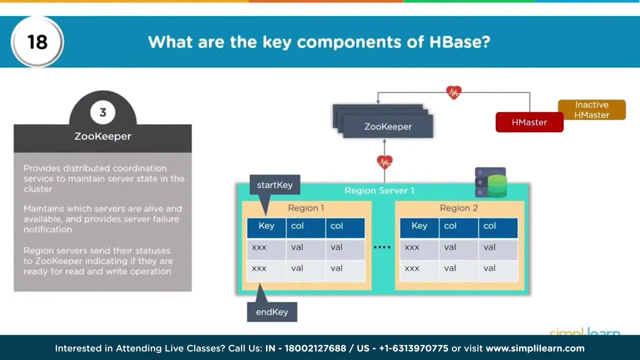 way ZooKeeper works. So ZooKeeper is a centralized coordination service which will always run with a quorum of processes. So ZooKeeper would always run with odd number of processes, such as 3,, 5 and 7, because ZooKeeper works on the concept of majority consensus. 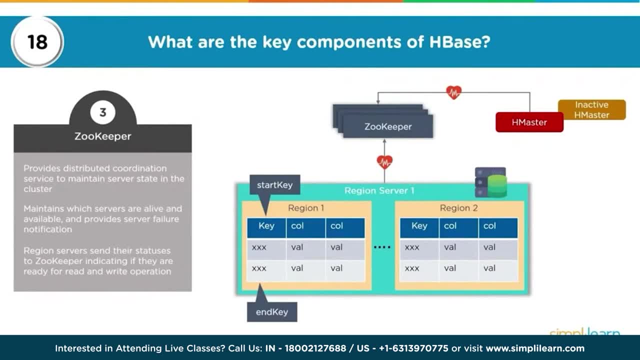 Now ZooKeeper, which is a centralized coordination service, is keeping a track of all the servers which are alive, available and also keeps a track of their status. For every server which ZooKeeper is monitoring, ZooKeeper keeps a session alive with that particular server. HMaster would always. 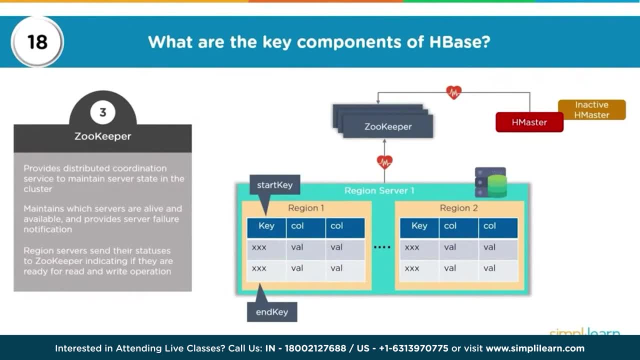 check with ZooKeeper which region servers are available alive so that region can be assigned to the region server. At one end you have region server which are sending their status to the ZooKeeper, indicating if they are ready for any kind of read or write operation, and at other end, HMaster is. 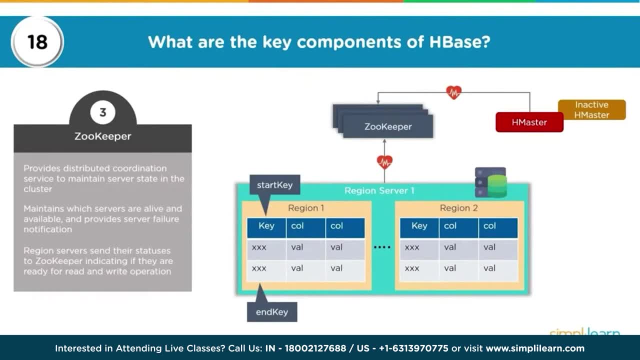 querying the ZooKeeper to check the status. Now ZooKeeper internally manages a meta table. Now that meta table will have information of which regions are residing on which region server and what row keys those regions contain. So in case of a read activity, HMaster will query ZooKeeper. 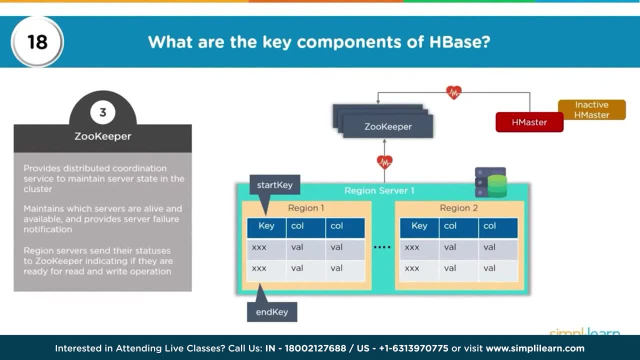 to find out the region server which contains that meta table. Once HMaster gets the information of meta table, it can look into the meta table to find out the row keys and the corresponding region servers which contain the regions for those row keys. Now, if we would want to, 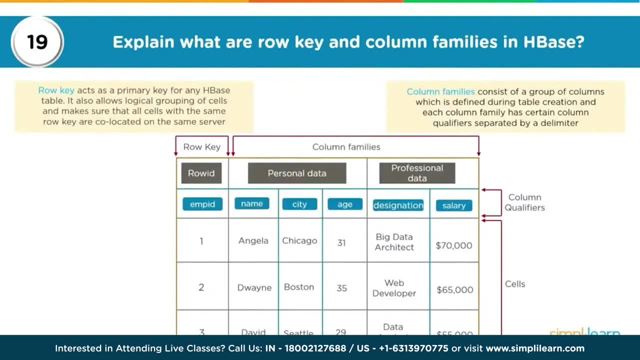 understand row key and column families in HBase. Let's look at this- and it would be good if we could look this on an excel sheet. So row key is always unique. It acts as a primary key for any HBase table. It allows logical grouping of. 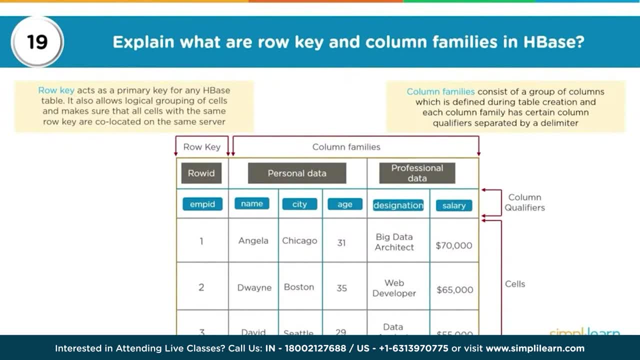 cells and makes sure that all cells with the same row key are co-located on the same server. So, as I said, you have four coordinates for HBase. You have a row key which is always unique. You have column families, which is nothing but. 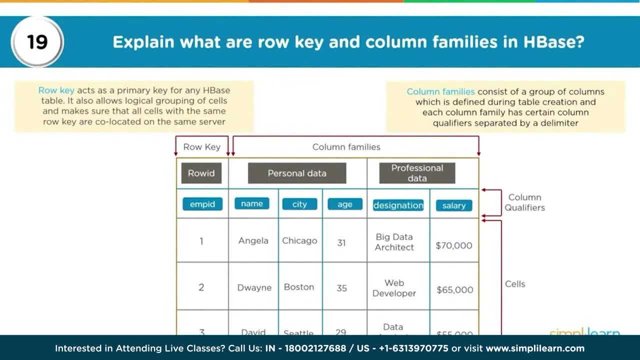 group of columns And when I say column families, one column family can have any number of columns. So when I talk about HBase, HBase is four dimensional and in terms of HBase it is also called as a column oriented database, Which basically means that every 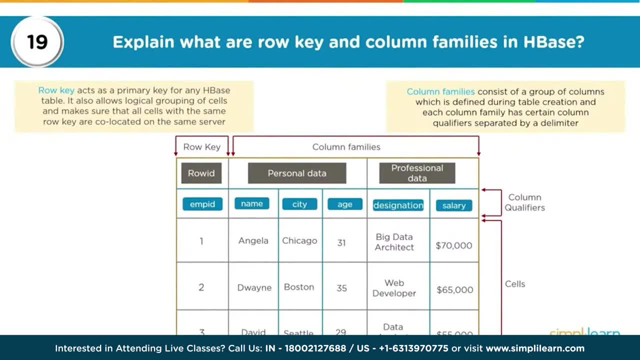 row in one column could have a different data type. Now you have a row key which uniquely identifies the row. You have column families, which could be one or many depending on how the table has been defined, And a column family can have any number of. columns. Or I could say for every row within a column family you could have different number of columns. So I could say for my row one I could just have two columns, such as name and city, within the column family. For my row two, I could have name city. 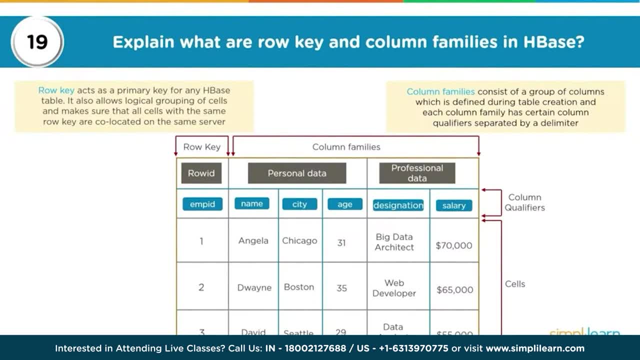 age designation, salary. For my third row I could have thousand columns And all that could belong to one column family. So this is a horizontally scalable database. So column family consists of group of columns which is defined during table creation, And each column 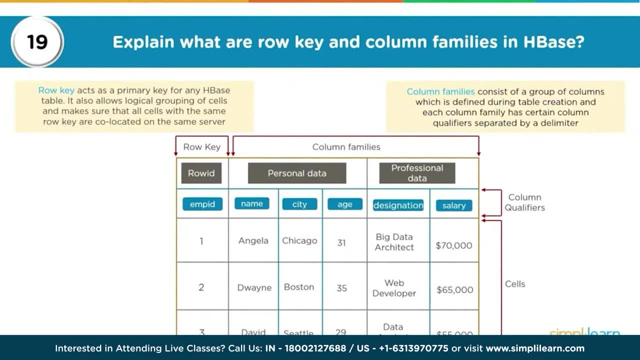 family can have any number of column qualifiers separated by a delimiter. Now a combination of row, key column, family, column qualifier such as name, city, age and the value within the cell is makes the HBase a unique four dimensional database. For more information, if you 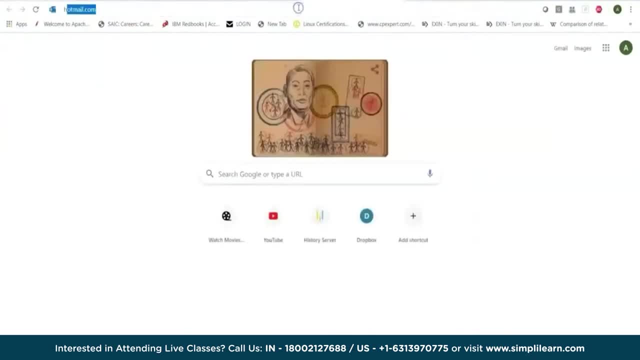 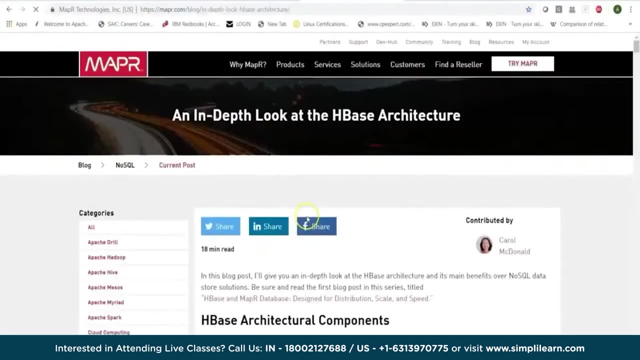 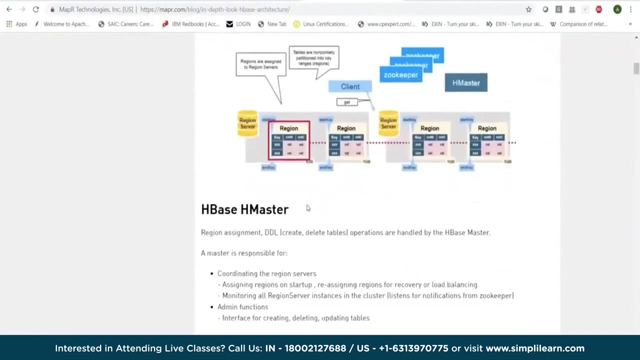 would want to learn on HBase. please refer this link, which is HBase Mapper, And this gives a complete HBase architecture. that is, three components of name node. Three components, that is, name node, region servers and zookeeper- how it works. 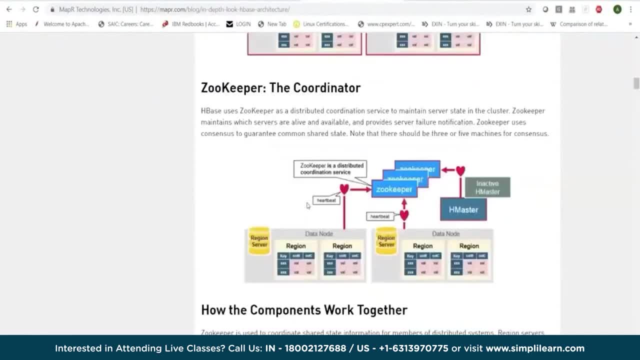 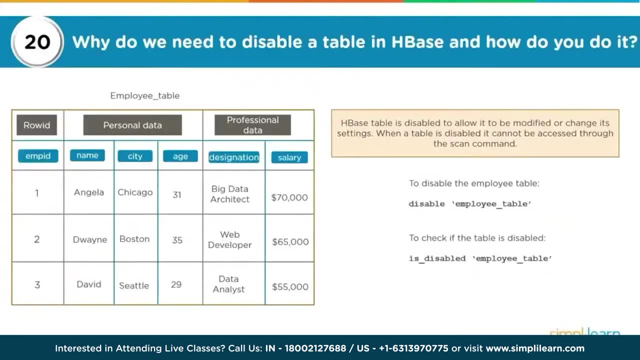 how HBase HMaster interacts with zookeeper, what zookeeper does in coordination, how are the components working together and how does HBase take care of read and write, Coming back and continuing? why do we need to disable a table? So there are different. 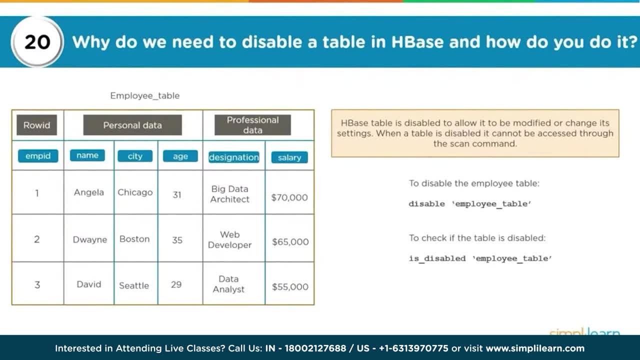 table operations, what you can do in HBase, and one of them is disabling a table. Now, if you would want to check the status of table, you could check that by is disabled and giving the table name or is enabled and the table name. So the question: 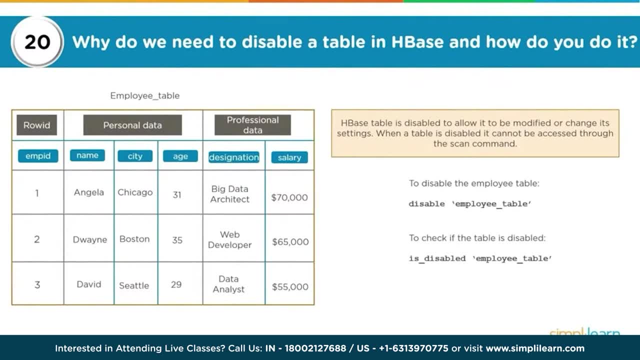 is why do we need to disable a table Now, if we would want to modify a table or we are doing some kind of maintenance activity, in that case we can disable the table so that we can modify or change its settings. When a table is disabled, it cannot. 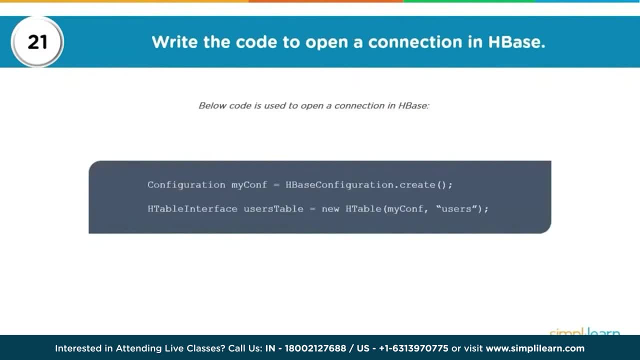 be accessed through the scan command. Now, if we have to write a code to open a connection in HBase. now, to interact with HBase, one could either use a graphical user interface such as Hue, or you could be using the command line HBase shell or you. 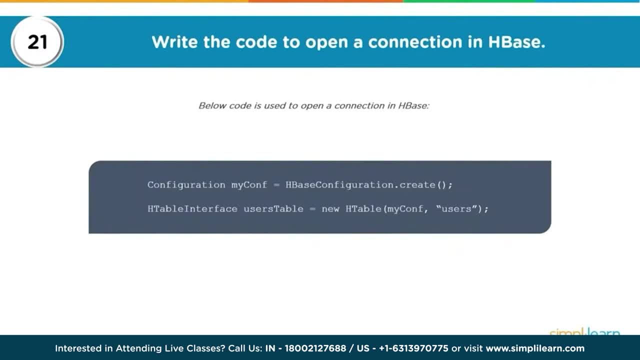 could be using HBase admin API if you are working with Java, or, say, HappyBase if you are working with Python, where you may want to open a connection with HBase so that you can work with HBase programmatically. In that case, we have to create 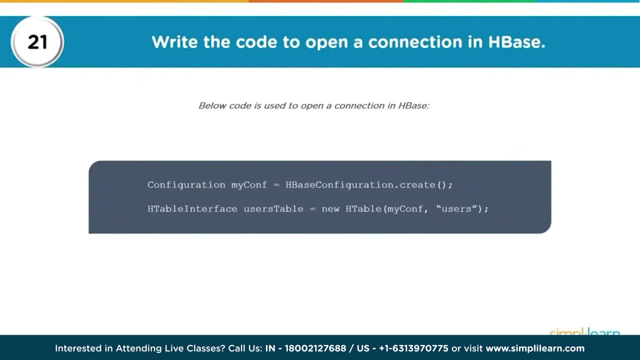 a configuration object, that is, configuration myconf, and then create a configuration object and then you can use different classes like H table interface. to work on a new table, You could use H column qualifier and many other classes which are available in HBase admin API. 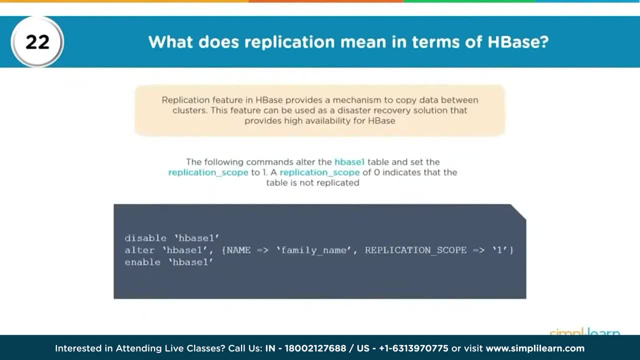 What does replication mean in terms of HBase? So HBase, as I said, works in a cluster way and when you talk about cluster you could always set up a replication from one HBase cluster to other HBase cluster. So this replication feature in HBase. 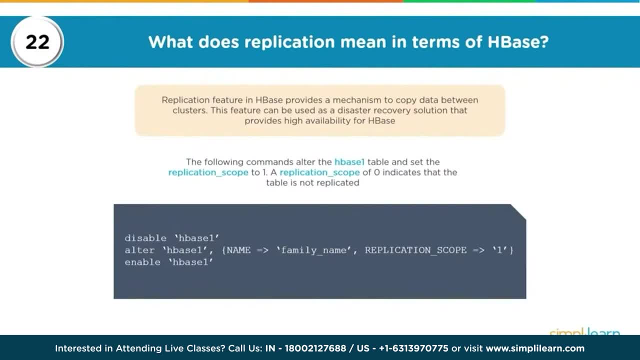 provides a mechanism to copy data between clusters or sync the data between different clusters. This feature can be used as a disaster recovery solution that provides high availability for HBase. So if I have HBase cluster one where I have one master and multiple region servers, 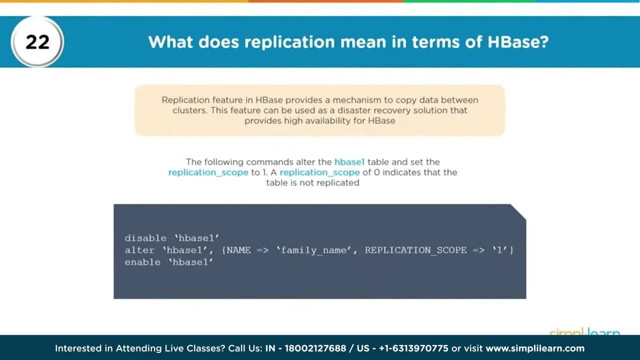 running in a Hadoop cluster. I could use the same Hadoop cluster to create a HBase replica cluster. or I could have a totally different HBase replica cluster where my intention is that if things are changing in a particular table in cluster one, I would want them to be replicated. 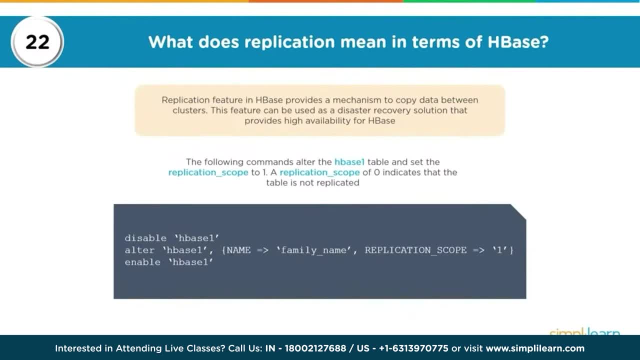 across different clusters. So I could alter the HBase table and set the replication scope to one. Now a replication scope of zero indicates that table is not replicated, but if we set the replication to one, we basically will have to set up a HBase cluster. 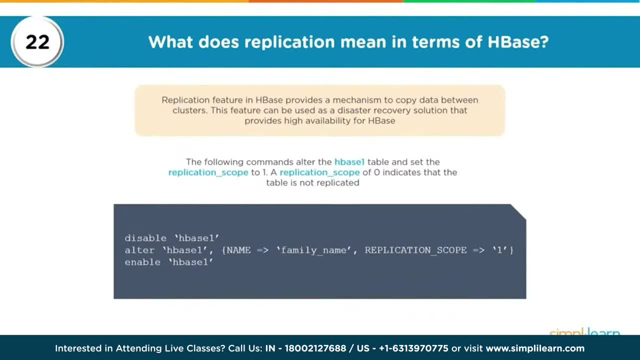 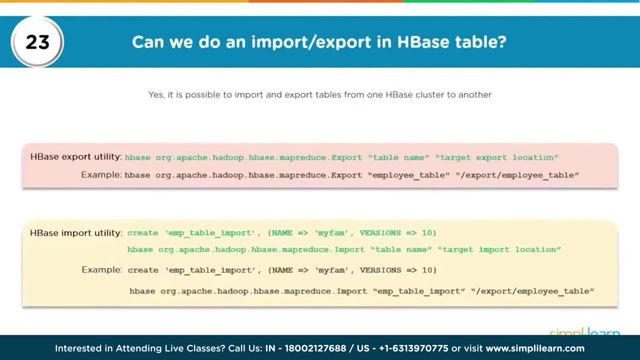 where we can replicate HBase tables data from cluster one to cluster. So these are the commands which can be used to enable replication and then replicate the data of table across clusters. Can we import and export in HBase? Of course we can. It is possible to import and export. 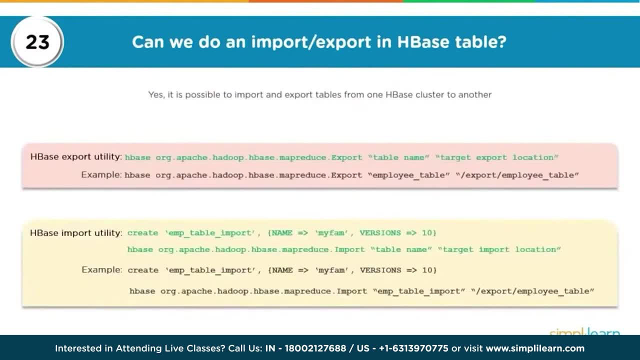 tables from one HBase cluster to other HBase cluster or even within a cluster. So we can use the HBase export utility which comes in this particular package. give a table name and then a target location so that will export the data of HBase table into. 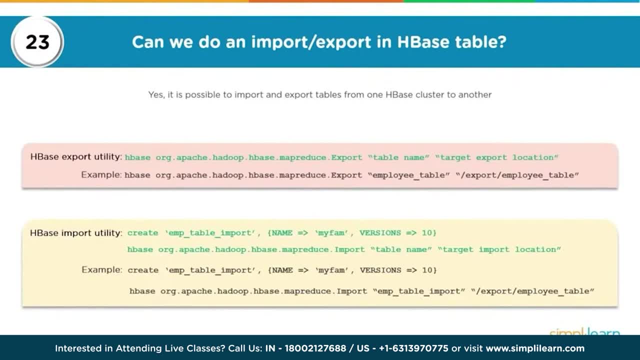 a directory on SDFS, Then I could create a different table which would follow some kind of same definition as the table which was exported, and then I could use import to import the data from the directory on SDFS to my table, If you would want. 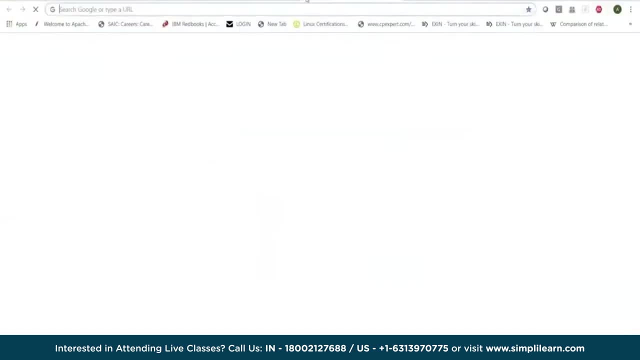 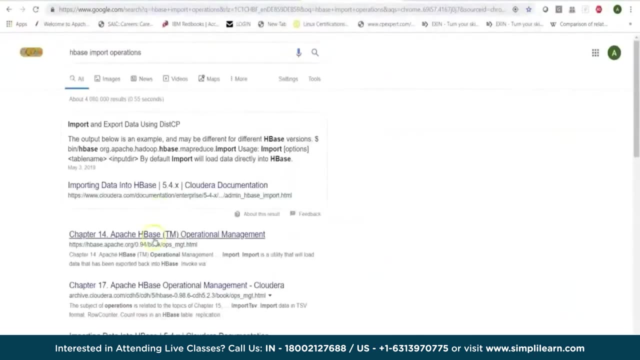 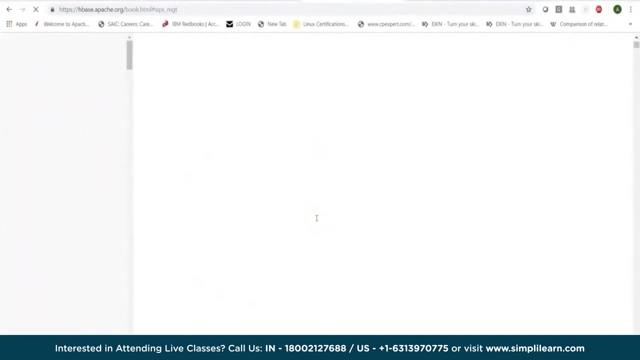 to learn more on HBase import and export, you could look at HBase import operations. Let's search for the link- and this is the link where you could learn more about HBase import export utilities, how you could do a bulk import, bulk export which internally. 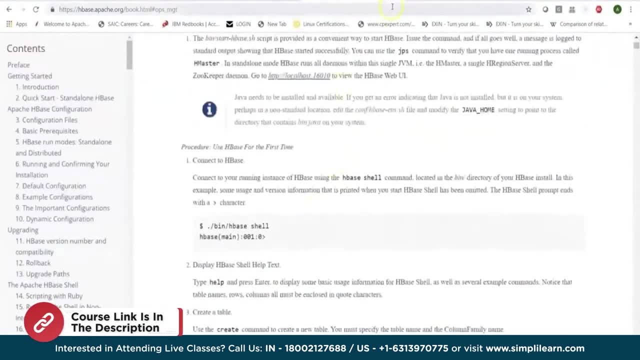 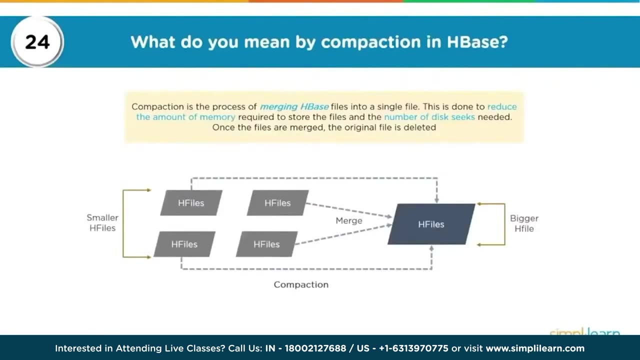 uses MapReduce, and then you could do a import and export into HBase tables. Moving further, what do we mean by compaction in HBase? Now, we all know that HBase is a NoSQL database which can be used to store huge amount of data. 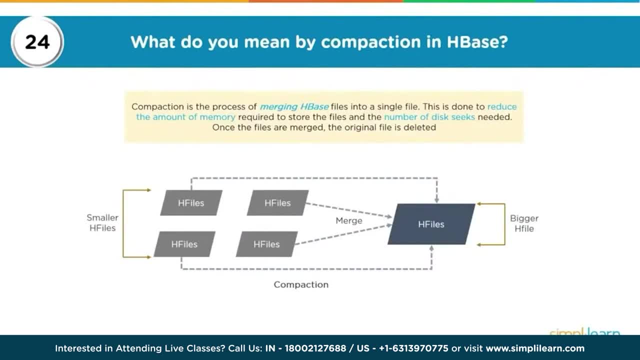 However, whenever a data is written in HBase, it is first written to what we call as write ahead log and also to mem store, which is write cache. Now, once the data is written in wall and your mem store, it is offloaded to form an internal HBase. 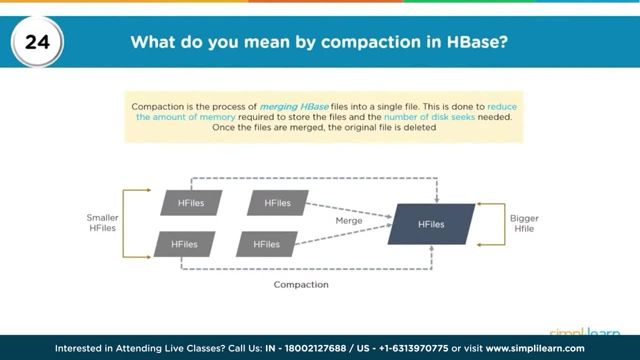 format file, which is called H file, and usually these H files are very small in nature. So we also know that SDFS is good when we talk about few number of larger files in comparison to large number of smaller files, Due to the limitation of name nodes. 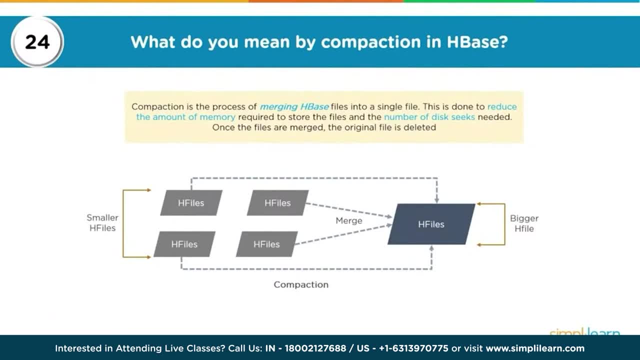 memory Compaction is process of merging HBase files, that is, these smaller H files, into a single large file. This is done to reduce the amount of memory required to store the files and number of disk seeks needed. So we could have lot of H files which get created. 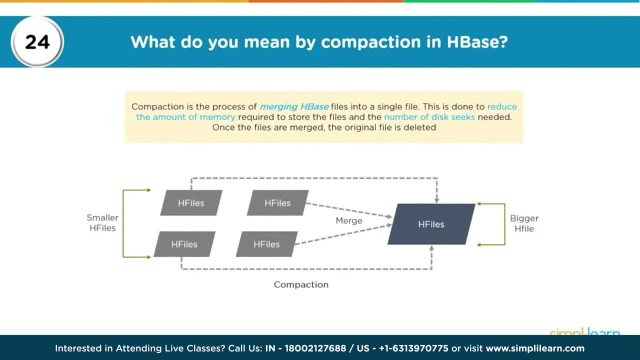 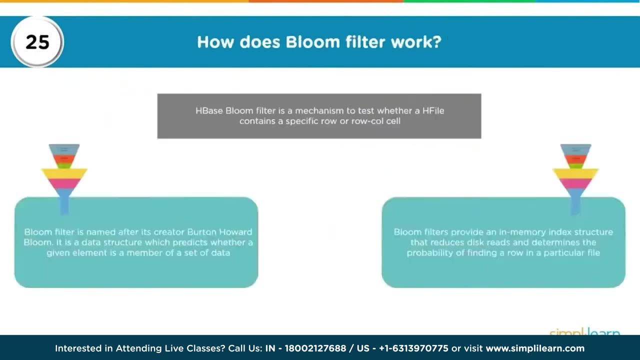 when the data is written to HBase, and these smaller files can then be compacted through a major or minor compaction, creating one big H file which internally would then be written to SDFS and SDFS format of blocks. That is the benefit of compaction. There is also a feature called 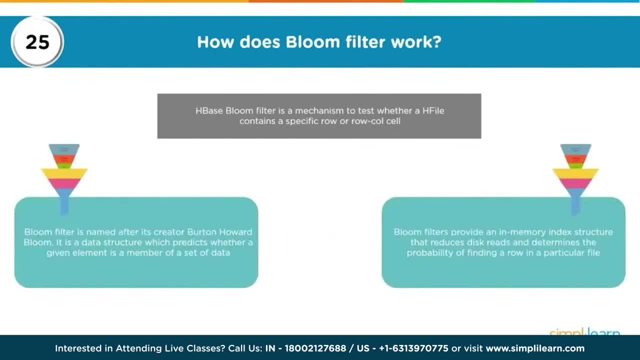 bloom filter. So how does bloom filter work? So bloom filter, or HBase bloom filter, is a mechanism to test whether a H file contains a specific row or a row column cell. Bloom filter is named after its creator, Burton Howard Bloom. It is a 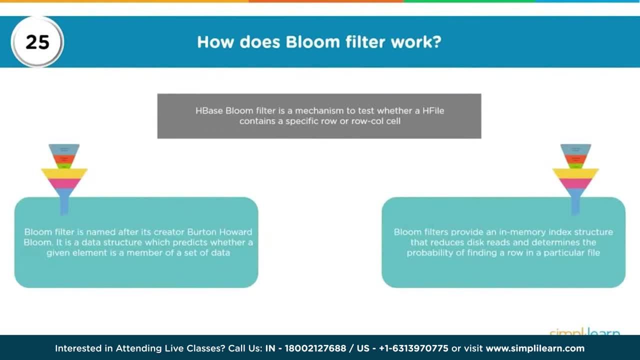 data structure which predicts whether a given element is a member of a set of data. It provides an in-memory index structure that reduces the disk reads and determines the probability of finding a row in a particular file. This is one of very useful features of HBase, which allows for. 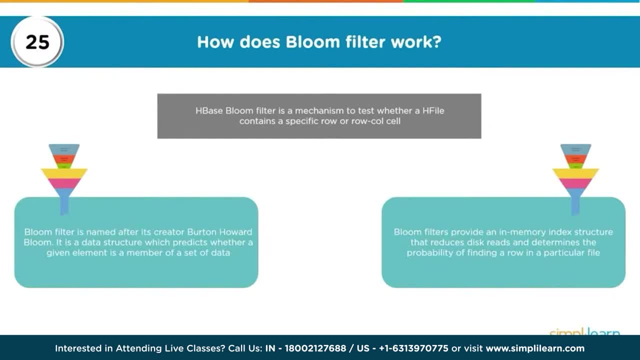 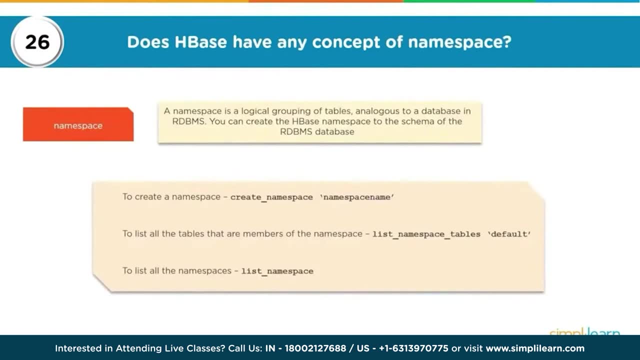 faster access and avoids disk seeks. Does HBase have any concept of namespace? So namespace is when you have similar elements grouped together. So namespace, yes, HBase supports such namespace. So namespace is a logical grouping of tables analogous to a database in RDBMS, So you can. 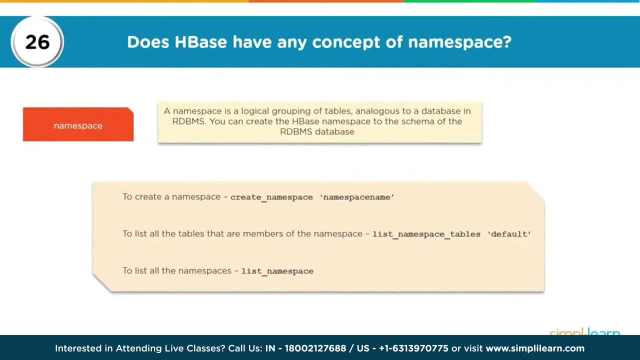 create HBase namespace to the schema of RDBMS database. So you could create a namespace by saying create namespace and giving it a name, And then you could also list the tables within a namespace. You could create tables within a specific namespace. Now this is usually done. 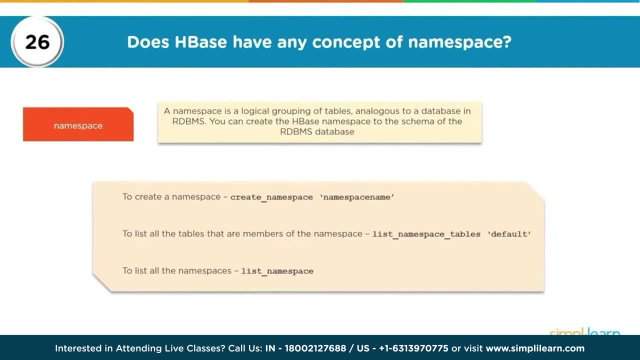 in production environment where a cluster might be multi tenant cluster and there might be different users of the same NoSQL database. In that case, admin would create specific namespace and for specific namespace you would have different directories on HDFS and users of a particular business unit. 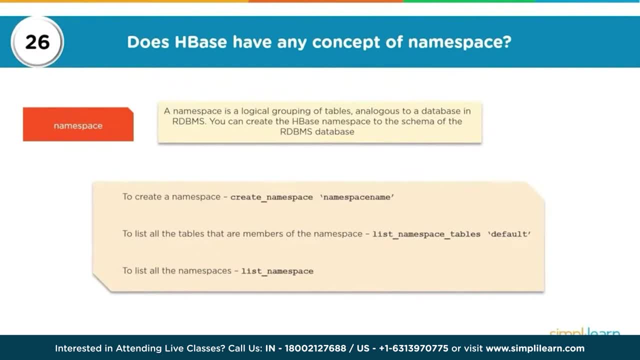 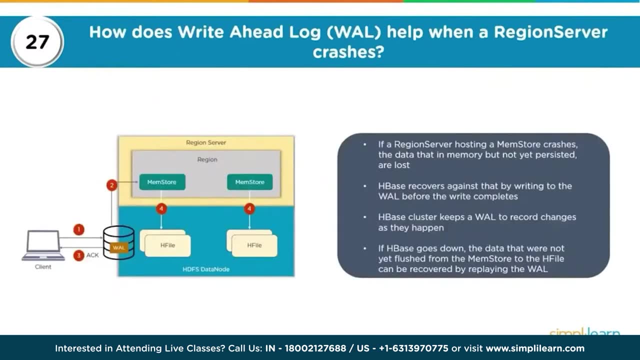 or a team can work on their HBase objects within a specific namespace. This is a question which is again very important to understand about the writes or reads. So how does write ahead log wall help when a region server crashes? Now, as I said, when a write happens, 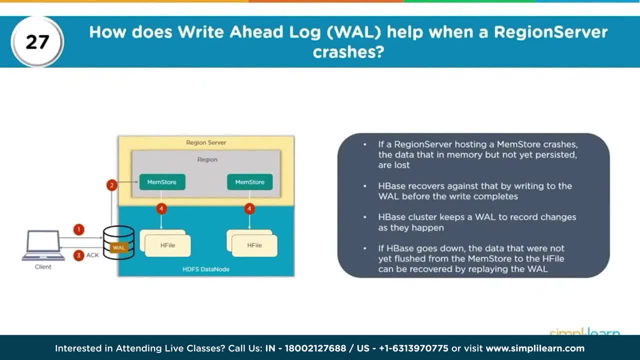 it will happen into memstore and wall. that is your edit log, or write ahead log. So whenever a write happens, it will happen in two places: Memstore, which is the write cache, and wall, which is a edit log Only when the data is written. 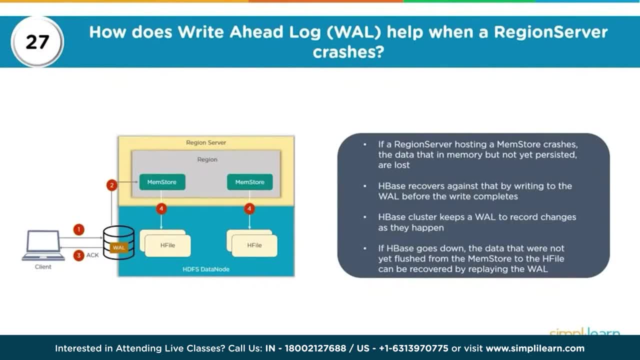 in both these places and based on the limitation of memstore, the data will be flushed to create an HBase format file called H file. These files are then compacted and created into one bigger file, which will then be stored on HDFS and HDFS data, as we know. 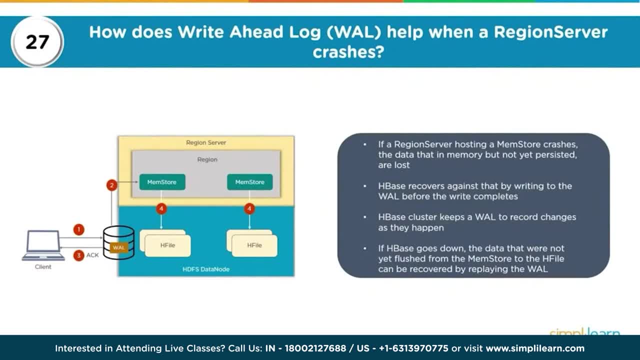 is stored in the form of blocks on the underlying data nodes. So if a region server hosting a memstore crashes, Now where is region server running? That would be co-located with data node. So if a data node crashes, or if a region server, 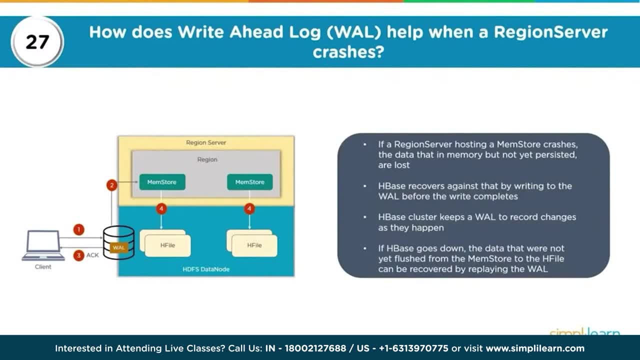 which was hosting the memstore. write cache crashes data in memory. the data that was in memory which was not persisted is lost. Now how does HBase recover from this? As I said, your data is written into wall and memstore at the same. 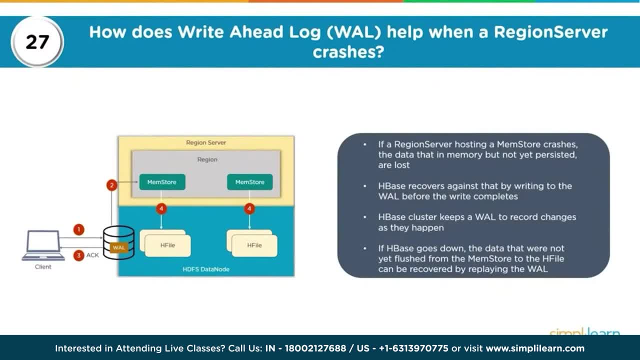 time. HBase recovers against that by writing to wall before the write completes. So whenever a write happens, it happens in memstore and wall at the same time. HBase cluster keeps a wall to record changes as they happen and that's why we. 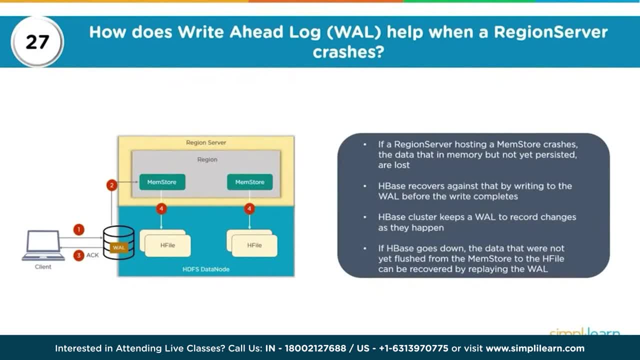 call it as also an edit log. If HBase goes down or the node that goes down, the data that was not flushed from memstore to H file can be recovered by replaying the write ahead log and that's the benefit of your edit log or write ahead log. 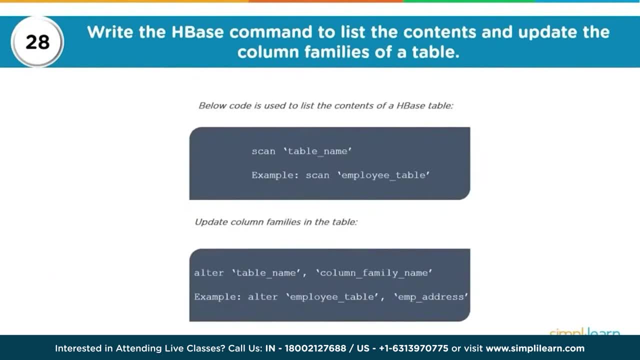 Now, if we would have to write HBase command to list the contents and update the column families of a table, I could just do a scan and that would give me complete data of a table. If you are very specific and if you would want to look at, 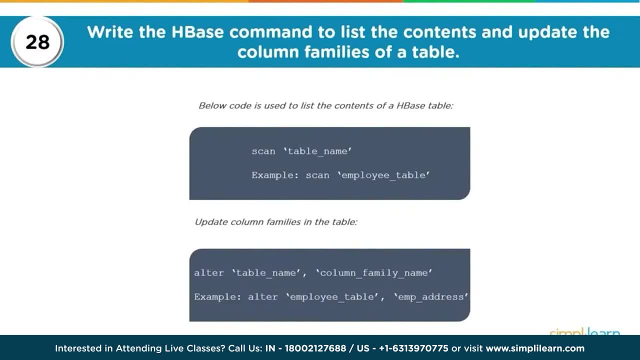 a particular row, then you could do a get table name and then give the row key. However, you could do a scan to get the complete data of a particular table. You could also do a describe to see what are the different column families and, if you would want to, 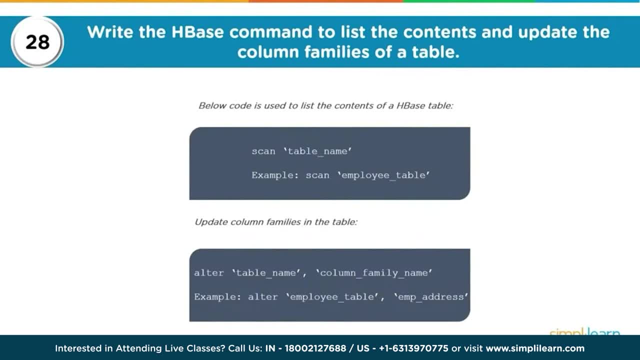 alter the table and add a new column family. it is very simple. you can just say alter, give the HBase table name and then give you a new column family name which will then be added to the table. What are catalog tables in HBase? So, as I mentioned, 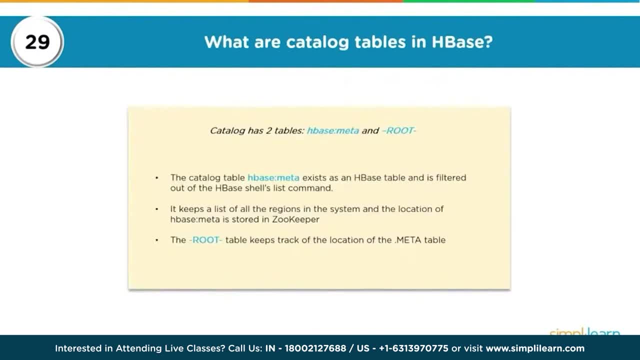 your zookeeper knows the location of this internal catalog table, or what we call as the meta table. Now, catalog tables in HBase have two tables. One is HBase meta table and one is hyphen root. The catalog table HBase meta exists as an HBase table. 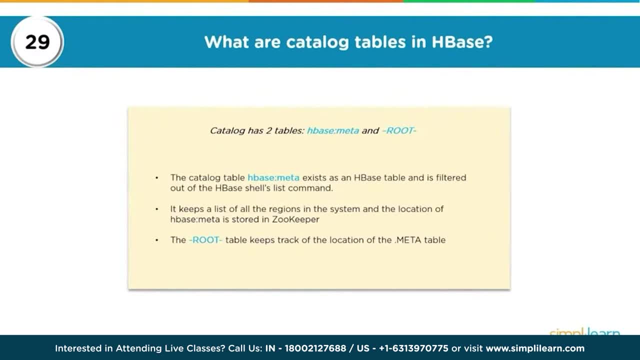 and is filtered out of HBase shell's list command. So if I give a list command on HBase, it would list all the tables which HBase contains, but not the meta table. It is an internal table. This meta table keeps a list of all regions in the 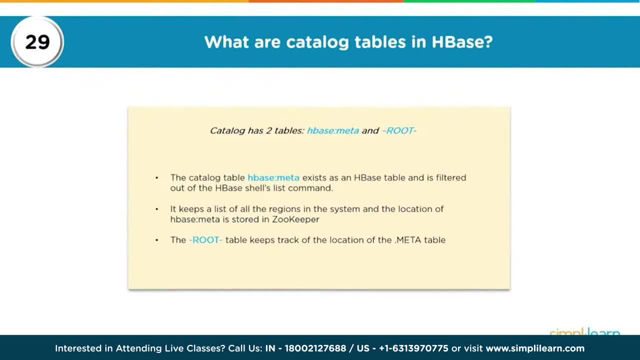 system and location of HBase meta stored in zookeeper. So if somebody wants to find out or look for particular rows, they need to know the regions which contain that data, and those regions are located on region server. To get all this information one has to look. 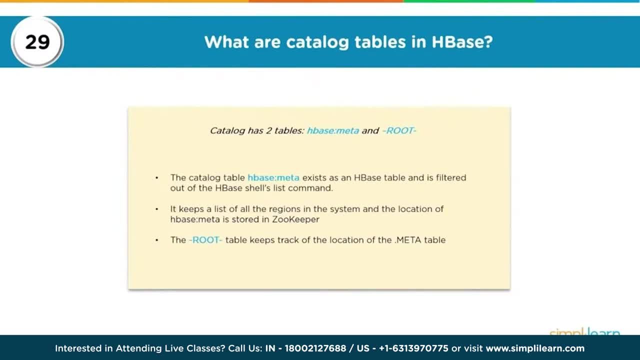 into this meta table. However, we will not be looking into meta table directly. we would just be giving a write or a read operation. internally, your HBase master queries the zookeeper. Zookeeper has the information of where the meta table exists and that meta table which. 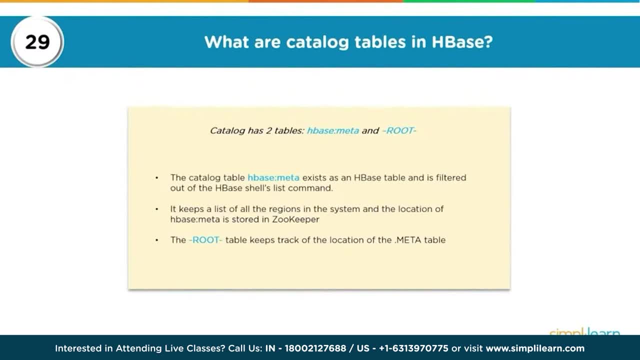 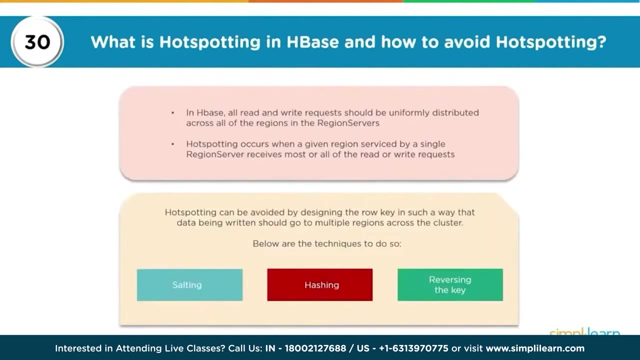 is existing on region server contains information of row keys and the region servers where those rows can be found. Your root table keeps a track of location of the meta table. What is hotspotting in HBase and how to avoid hotspotting? Now, this is a common problem. 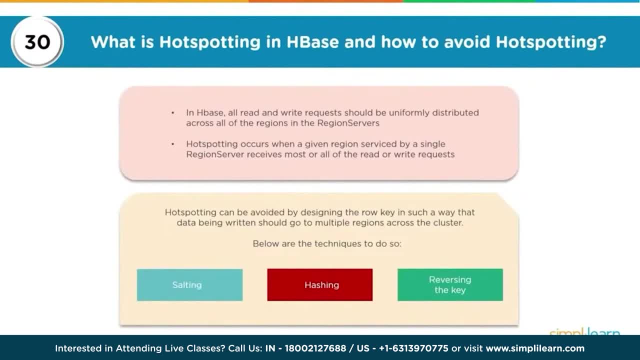 and always admin guys or guys who are managing the infrastructure would think about it. So one of the main idea is that HBase would be leveraging the benefit of SDFS. Your all read and write request should be uniformly distributed across all of the regions and region servers. Otherwise, 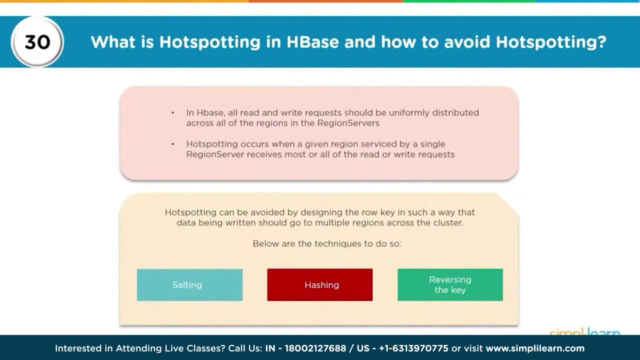 what's the benefit of having a distributed cluster? So you would have your data stored across region servers in the form of regions, which are horizontal partitions of the table, and whenever read and write request happen, they should be uniformly distributed across all the regions in the region. 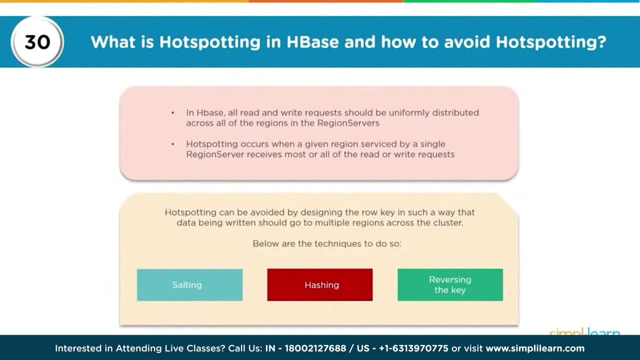 servers. Now hotspotting occurs when a given region serviced by a region server receives most or all of read and write request, which is basically a unbalanced way of read write operations. Now hotspot can be avoided by designing the row key in such a way that data 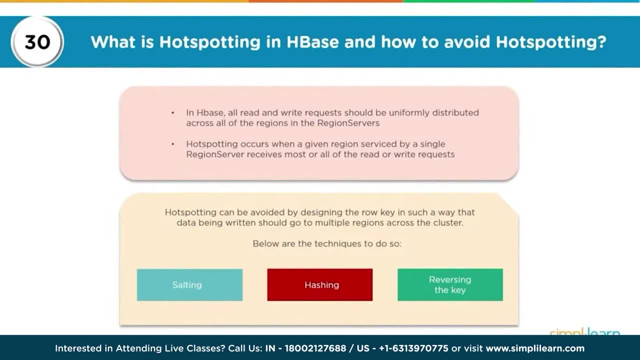 being written should go to multiple regions across the cluster, So you could do techniques such as salting, hashing, reversing the key and many other techniques which are employed by users of HBase. We need to just make sure that when the regions are distributed, 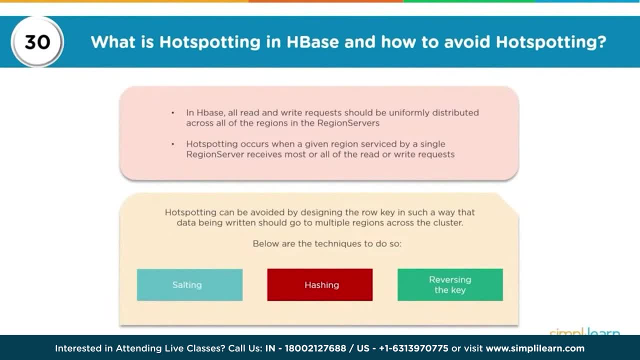 across region servers. they should be spread across region servers so that your read and write request can be satisfied from different region servers in parallel, rather than all read and write request hitting the same region server, overloading the region server, which may also lead to the crashing of a particular. 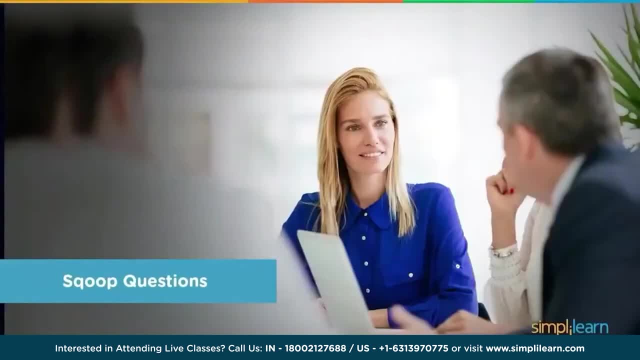 region server. So these were some of the important questions of HBase, and then there are many more. Please refer to the link which I specified during my discussion and that gives you a detailed explanation of how HBase works. You can also look into HBase definitive guide. 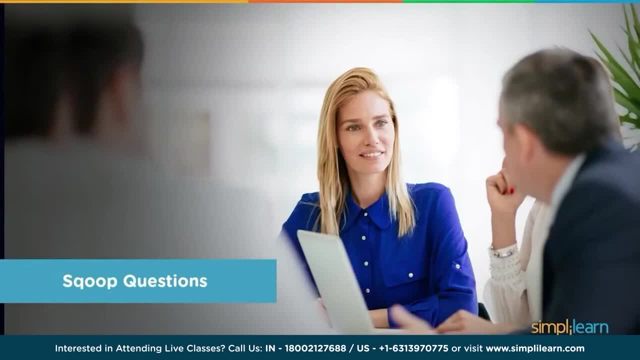 by O'Reilly or HBase in action, and these are really good books to understand about HBase internals and how it works. Now that we have learnt on Hive, which is a data warehousing package, we have learnt on PIG, which is a scripting or a. 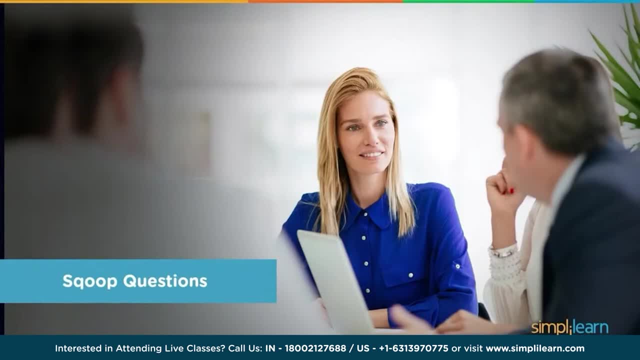 scripting language which allows you to do data analysis, and we have learnt some questions on a NoSQL database. Just note it that there are more than 225 NoSQL databases existing in market and if you would want to learn and know about more NoSQL databases, 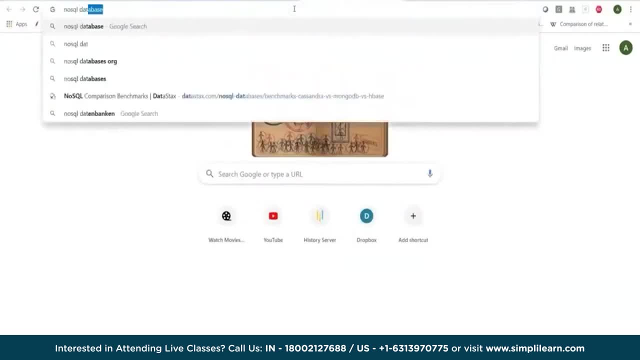 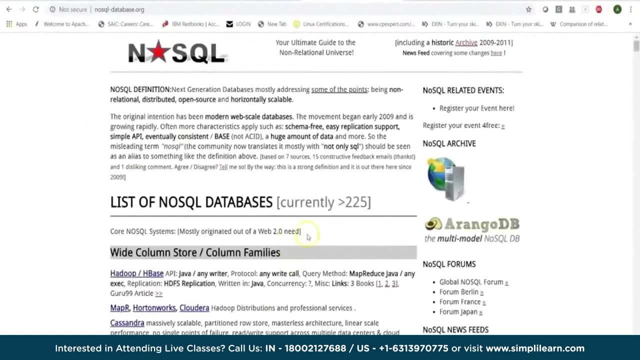 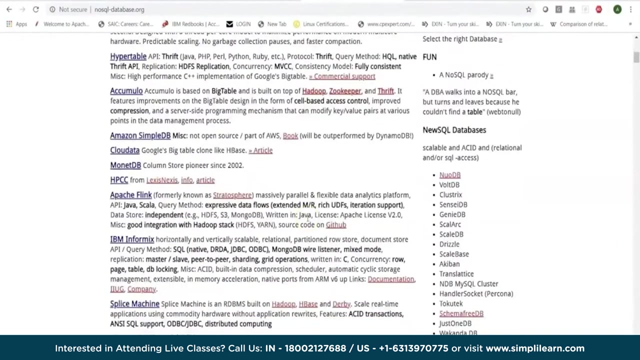 you can just go to Google and type NoSQL databases, org and that will take you to the link which is for NoSQL databases, and this shows there are more than 225 NoSQL databases existing in market and these are for different use cases used by different users and 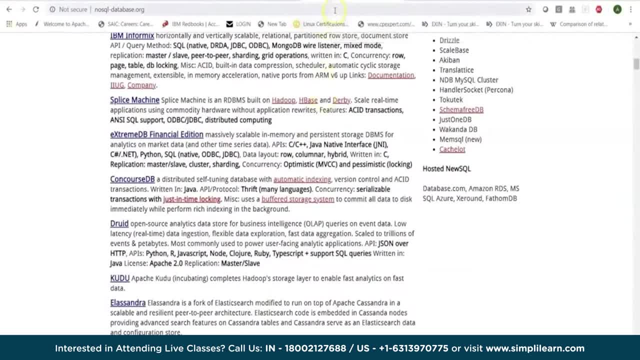 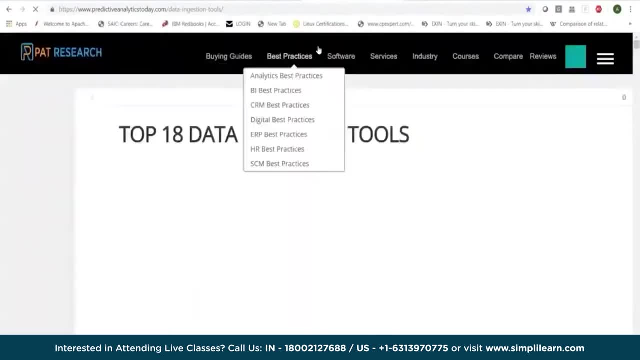 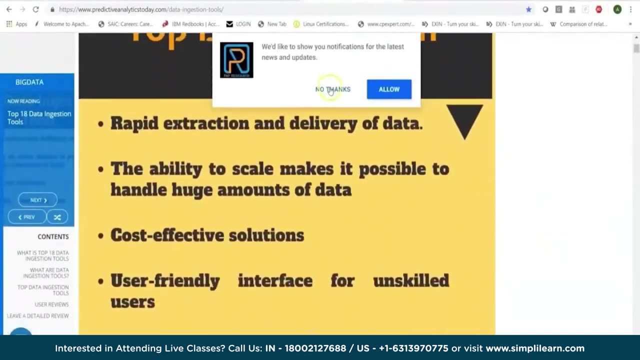 for with different features. So have a look at this link. Now, when you talk about data ingestion, so let's look at data ingestion, and this is one good link which I would suggest to have a look at, which lists down around 18 different ingestion tools. So, when you talk about 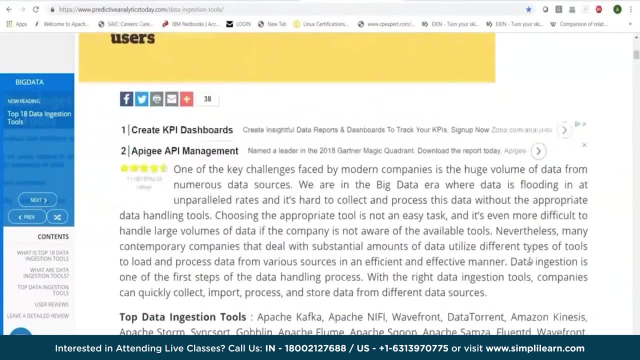 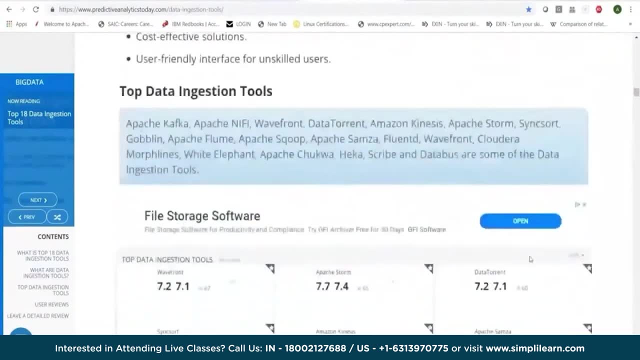 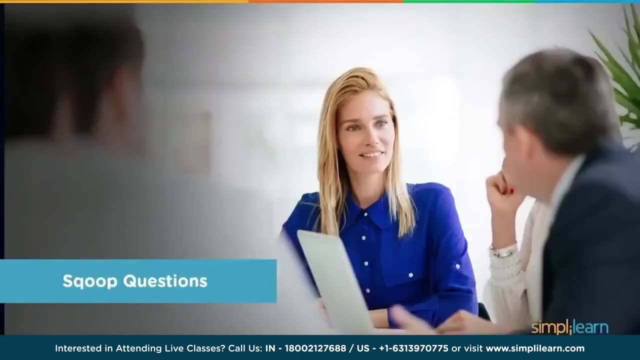 different data ingestion tools. some are for structured data, some are for streaming data, some are for data governance, some are for data ingestion and transformation, and so on. So have a look at this link, which also gives you a comparison of different data ingestion tools. So here, 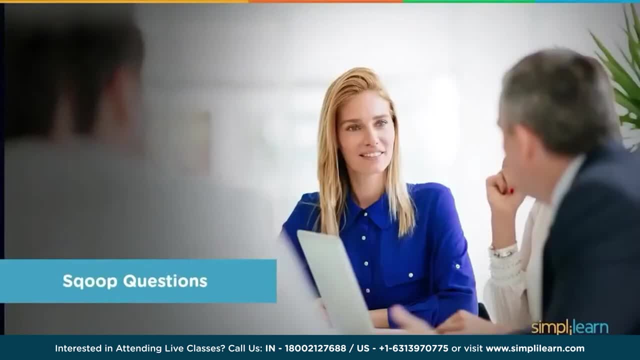 let's learn about some questions on Scoop, which is one of the data ingestion tools mainly used for structured data, or you could say data which is coming in from RDBMS, or data which is already structured and you would want to ingest that, you would want to store that on. 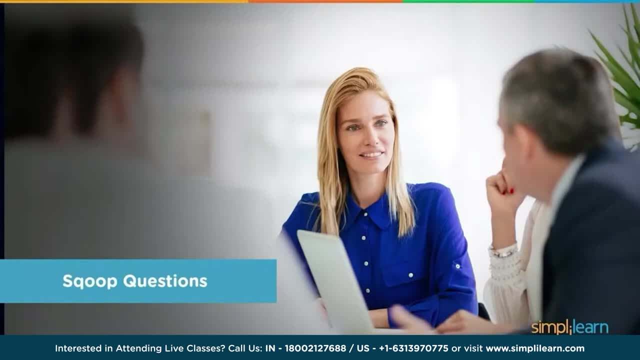 HDFS, which could then be used for Hive, which could be used for any kind of processing using MapReduce or Hive or Pig or Spark or any other processing frameworks, or you would want to load that data into, say, Hive or HBase tables. Scoop is: 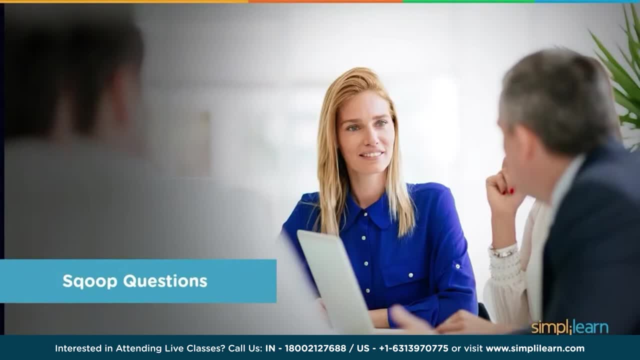 mainly for structured data. it is extensively used when organizations are migrating from RDBMS to a big data platform and they would be interested in ingesting the data. that is doing import and export of data from RDBMS to HDFS or vice versa. So let's learn about some. 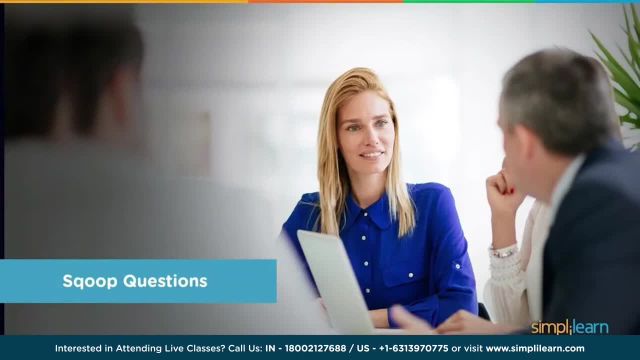 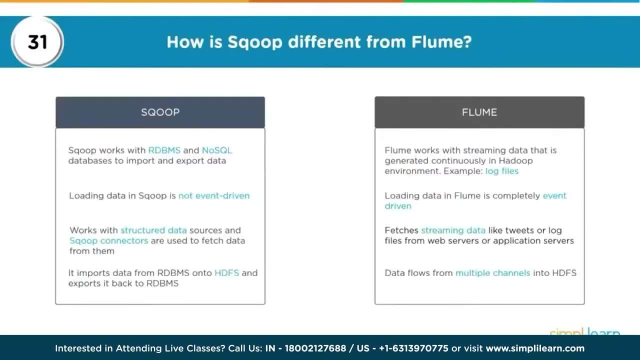 important questions on Scoop which you may be asked by an interviewer when you apply for a big data related position. How is Scoop different from Flume? So this is a very common question which is asked. Scoop, which is mainly for structured data, So Scoop works with. 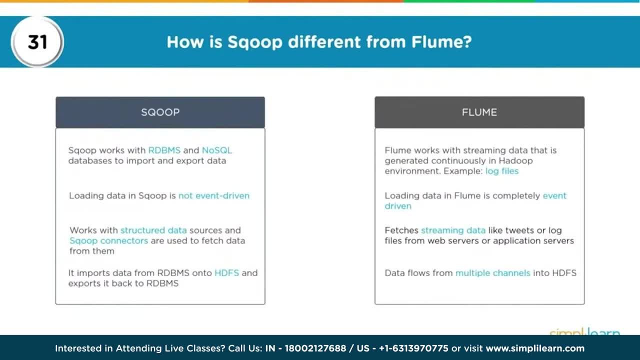 RDBMS. It also works with NoSQL databases to import and export data. So you can import data into SDFS, you can import data into data warehousing packets such as Hive directly or also in HBase, and you could also export data from Hadoop ecosystem to your. 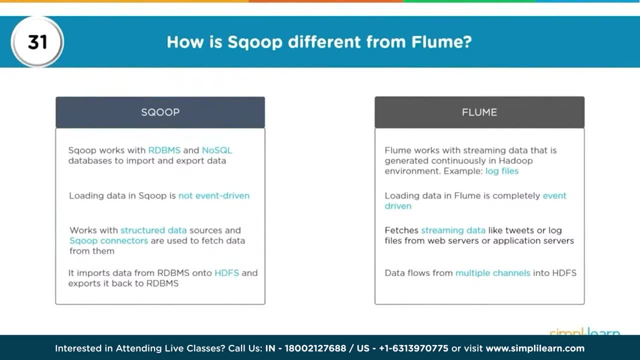 RDBMS. However, when it comes to Flume, Flume is more of a data ingestion tool which works with streaming data or unstructured data, So data which is constantly getting generated, for example, log files or metrics from server or some chat messenger and so on. So, if you 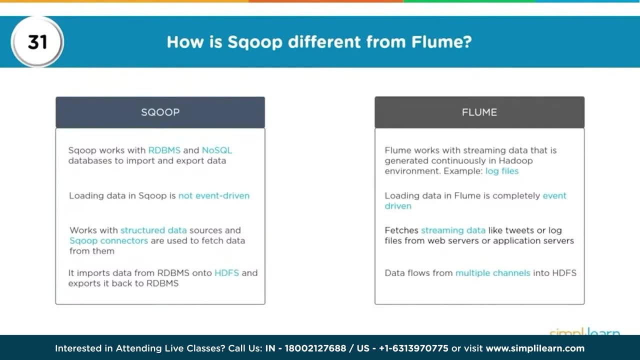 are interested in working on capturing and storing the streaming data in a storage layer such as SDFS or HBase. you could be using Flume. There could be other tools also, like Kafka or Storm or Chukwa or Samza, NiFi and so on. Scoop, however, is mainly 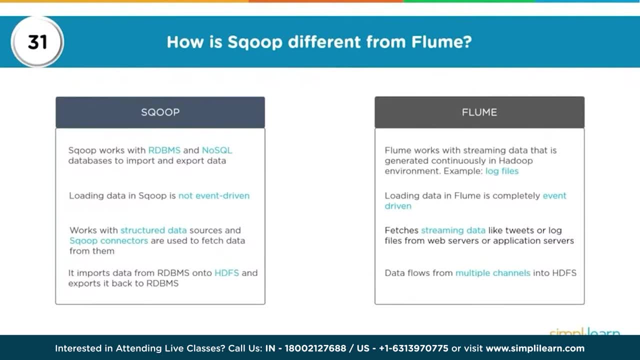 for structured data. Your loading data in Scoop is not event driven, so it is not based on event. It basically works on data which is already stored in RDBMS. In terms of Flume, it is completely event driven. That is as the messages, or as: 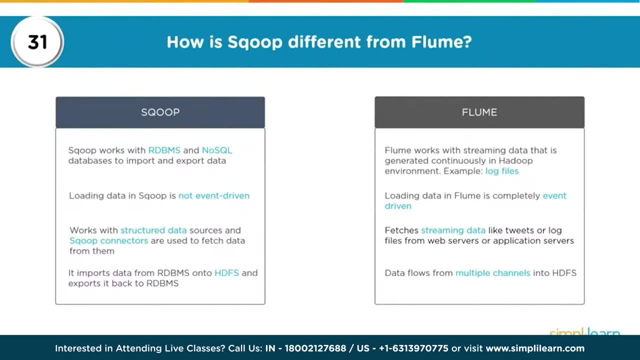 the events happen as the data is getting generated. you can have that data ingested using Flume. Scoop works with structured data sources, and you have various Scoop connectors which are used to fetch data from external data structures or RDBMS. So, for every RDBMS- 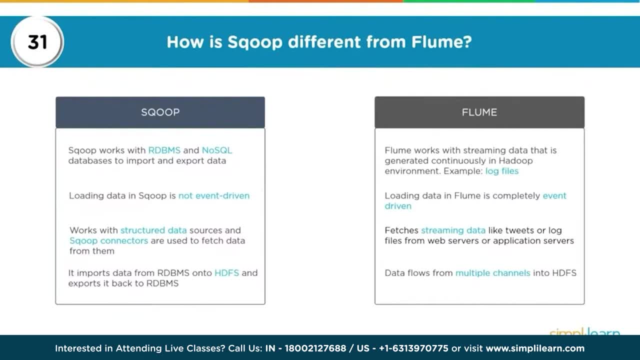 such as MySQL, Oracle, TV2, Microsoft SQL Server. you have different connectors which are available. Flume: it works on fetching streaming data, such as tweets or log files or server metrics, from your different sources where the data is getting generated and if you are interested. 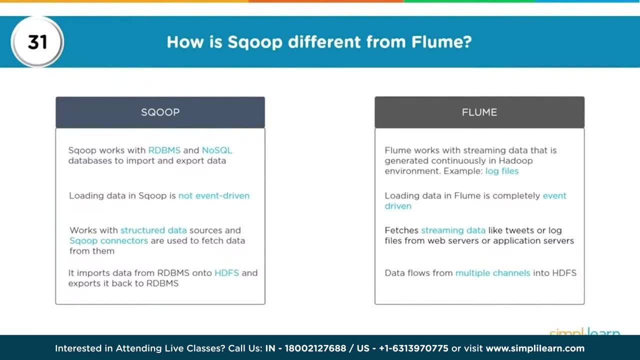 in not only ingesting that data, which is getting generated in a streaming fashion, but if you would be interested in processing the data as it arrives. Scoop can import data from RDBMS onto SDFS and also export it back to RDBMS. 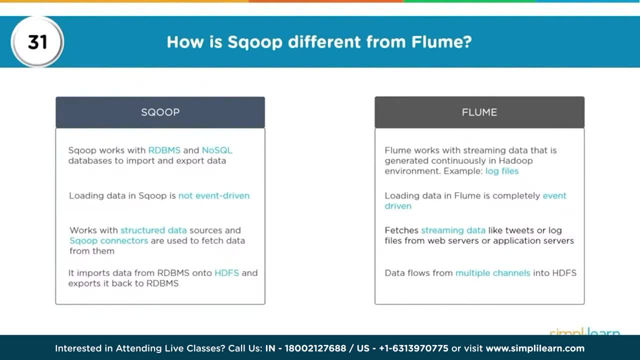 Flume is then used for streaming data. Now you could have one to one, one to many or many to one kind of relation. so, in terms of Flume, you have components such as your source, sync and channel. That's the main difference between. 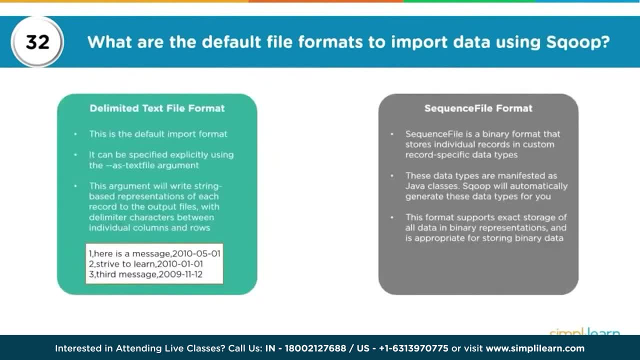 your Scoop and Flume. What are the different file formats to import data using Scoop? Well, there are lots and lots of formats in which you can import data into Scoop. When you talk about Scoop, you can have delimited text file format. 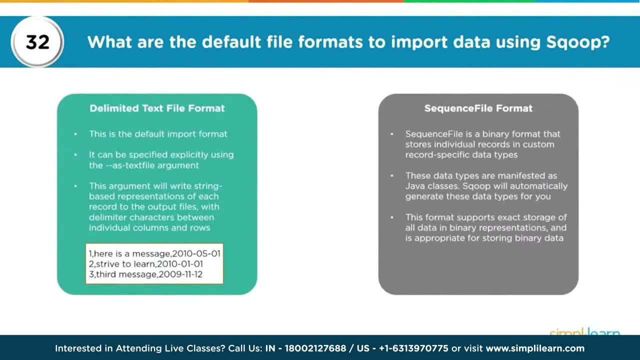 now that's the default import format. It can be specified explicitly using as text file argument. So when I want to import data from an RDBMS, I could get that data in SDFS using different compression schemes or in different formats using the specific arguments. So 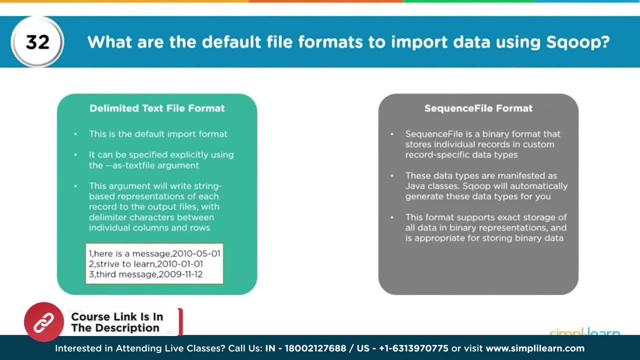 I could specify an argument which will write string based representation of each record to output files with delimiters between individual columns and rows. So that is the default format which is used to import data using Scoop. So to learn more about your Scoop and different. 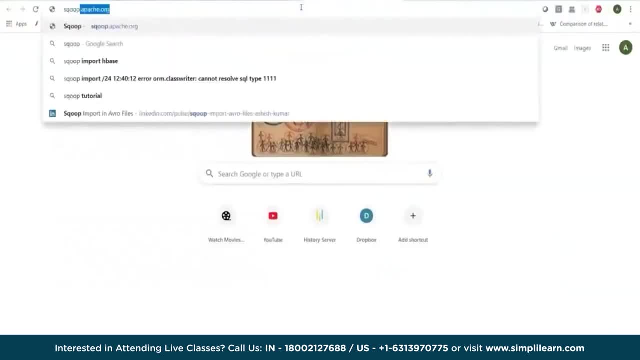 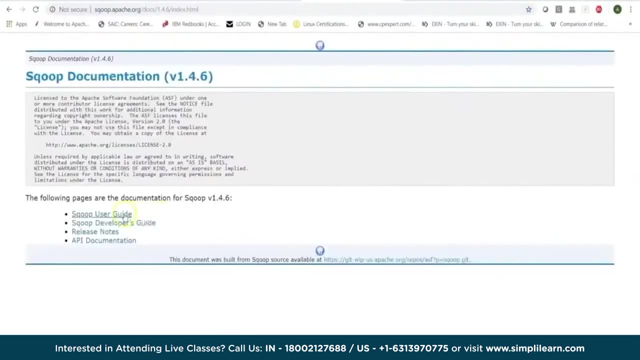 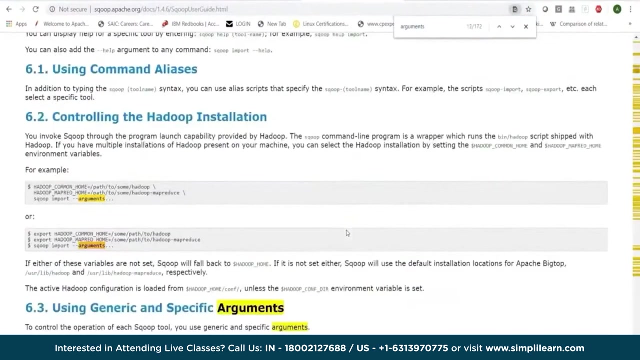 arguments which are available, you can click on scoopapacheorg, You can look into the documentation- and I would suggest choosing one of the versions and looking into the user guide, and here you can search for arguments and look for specific control arguments which show how you can import data using 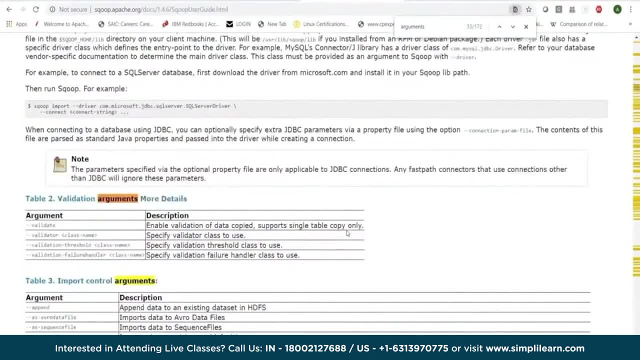 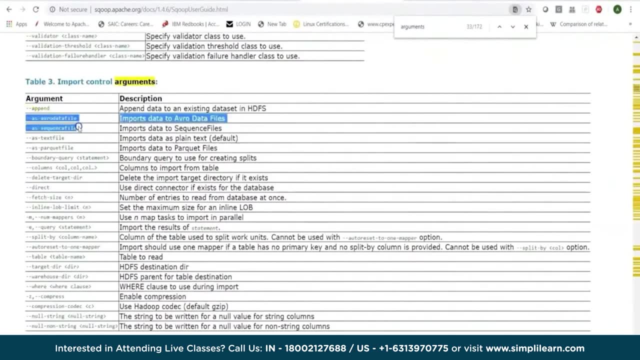 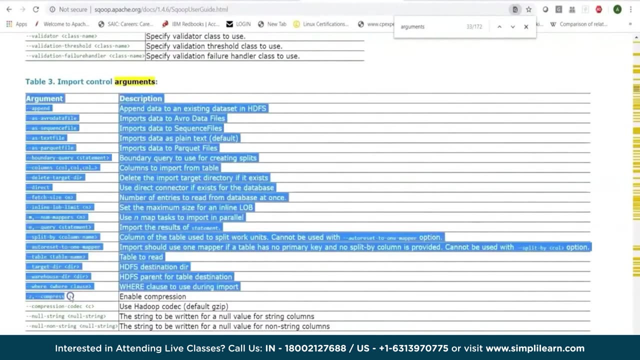 Scoop. So here we have common arguments, and then you also have import control arguments, wherein we have different options, like getting data as app row, as sequence file, as text file or parquet file. These are different formats. You can also get data in default compression. 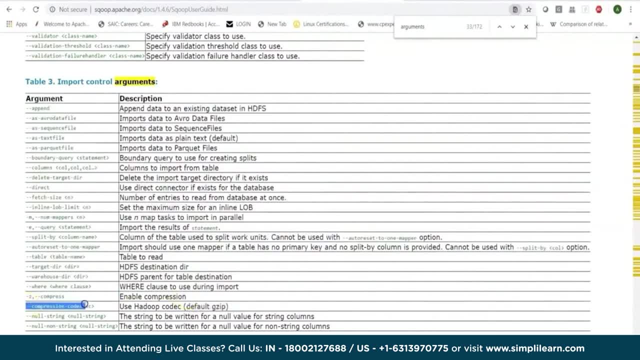 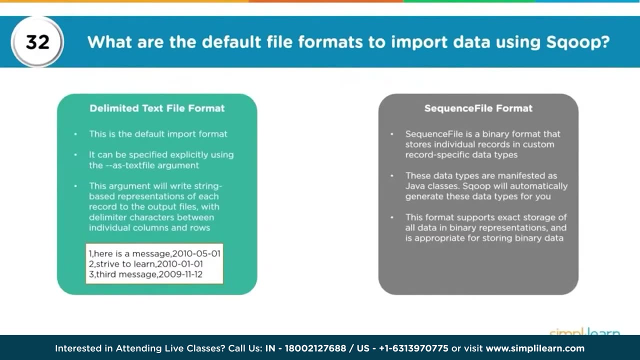 scheme, that is, gzip, or you can specify compression codec and then you can specify what compression mechanism you would want to use when you are importing your data using Scoop. When it comes to default format for flume, we could say sequence file, which is a binary format that stores. 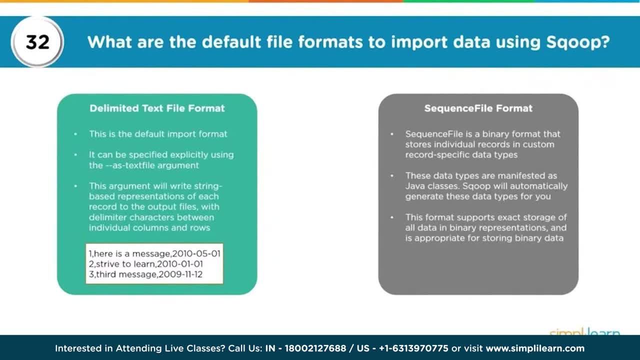 individual records in record, specific data types. So these data types are manifested as Java classes and Scoop will automatically generate these data types for you. So Scoop does that. when we talk about your sequence file format, in terms of your Scoop you could be extracting storage. 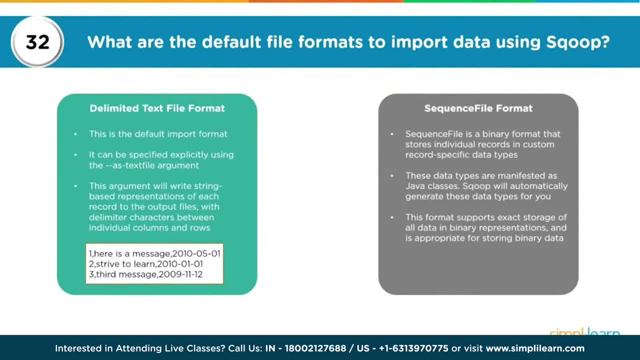 of all data in binary representation. So, as I mentioned, you can import data in different formats, such as app row, parquet sequence file, that is, binary format, or machine readable format, and then you could also have data in different compression schemes. Let me just show you some quick. 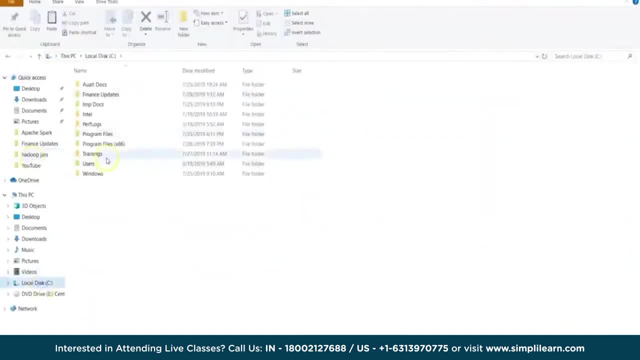 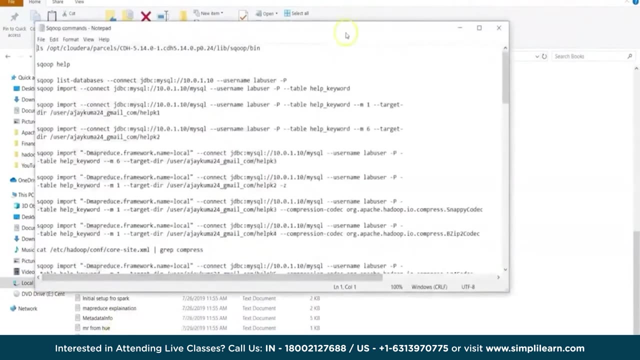 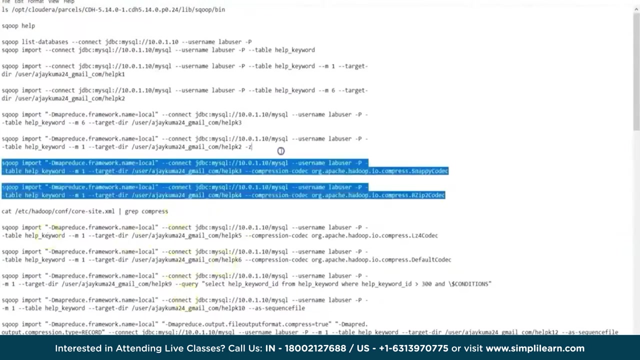 examples here. So if I look in the content and here I could search for a Scoop based file where I have listed down some examples. So if I would want to use different compression schemes, here are some examples. Have a look at these. So I am. 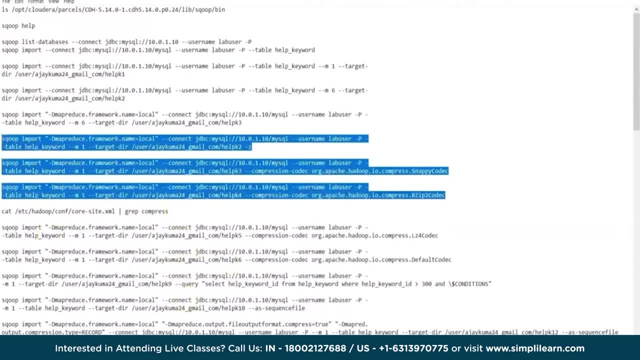 doing a Scoop import, I am also giving an argument so that Scoop, which also triggers a map, reduce job or I would say map only job. So when you run a Scoop import, it triggers a map only job. No reduce happens here and you could. 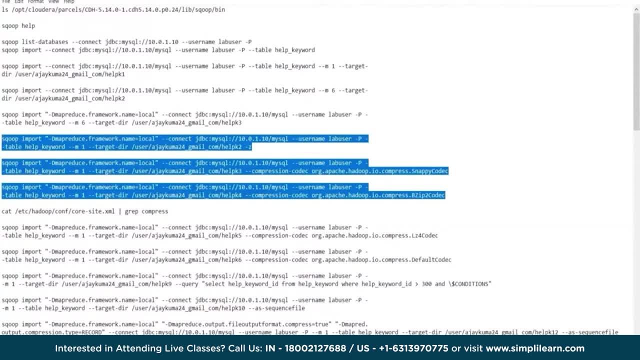 specify this parameter or this argument on the command line map: reduce dot framework, dot name so that you could run your map only job in a local mode to save time, or that would interact with yarn and run a full fledged map only job. We can give the connection. 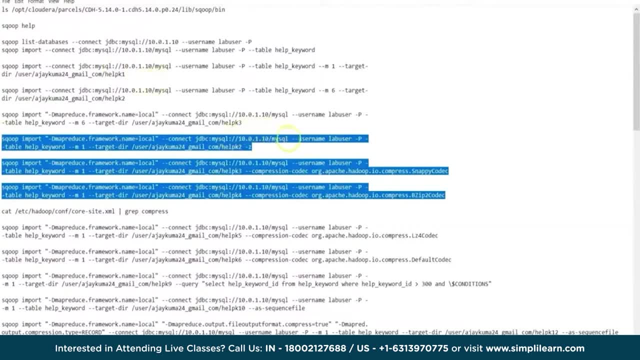 and then connect to whatever RDBMS we are connecting, mentioning the database name. give your user name and password, give the table name, give a target directory, or it would create a directory same as the table name, which would work only once, and then I could say: minus z. 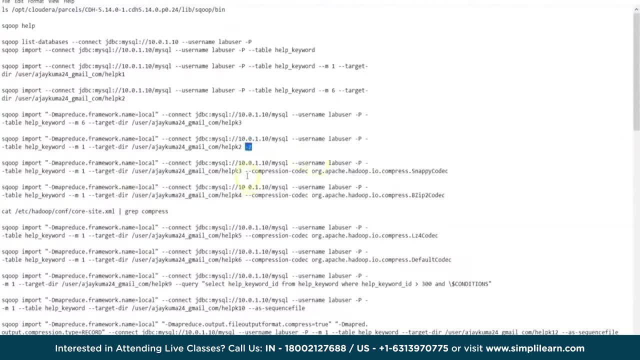 to get data in a compressed format, that is, gzip, or I could be specifying compression codec and then I could specify what compression codec I would want to use, say snappy, bzip, lz4, default. I could also run a query by giving a Scoop import. 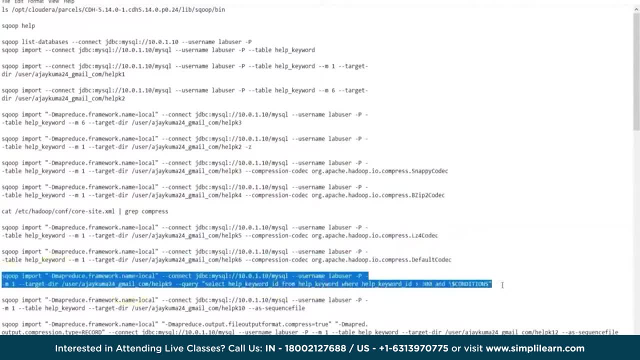 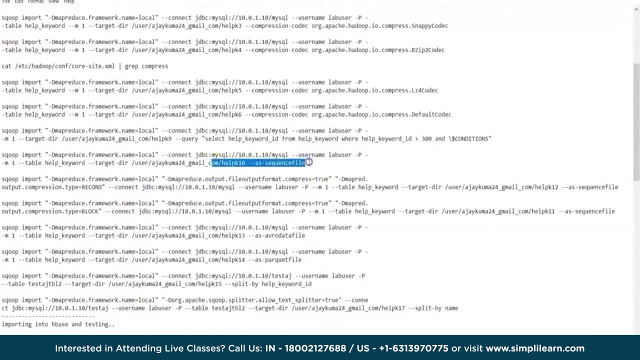 and when I am specifying a query. if you notice, I have not given any table name because that would be included in the query. I can get my data as a sequence file format, which is a binary format, which will create a huge file, so we could also have compression. 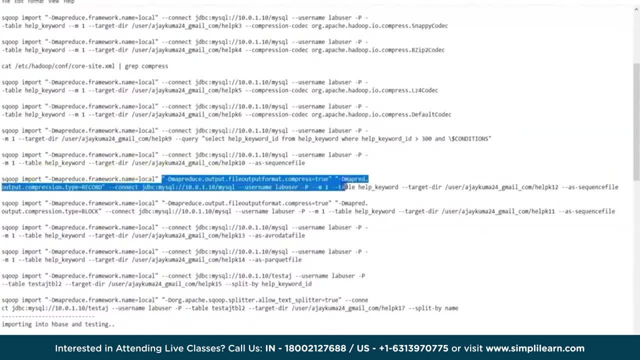 enabled and then I could say the output of my map job should use a compression at record level for my data coming in sequence file. So sequence file or a binary format supports compression at record level or at block level. I could get my data in a Avro file. 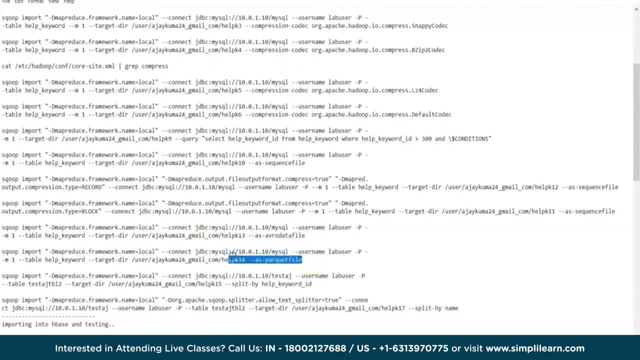 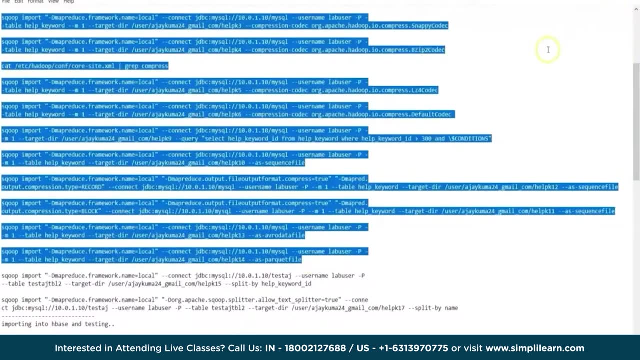 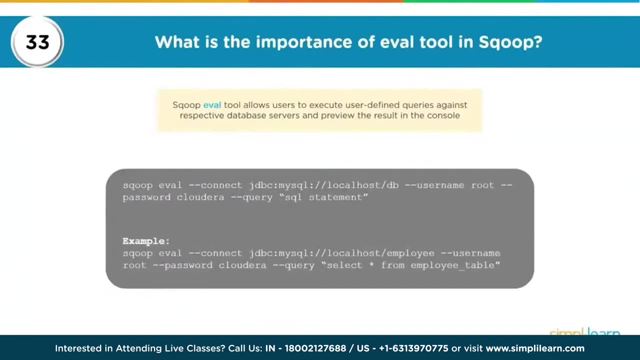 where data has embedded schema within the file, or a Parquet file also. So these are different ways in which you can set up different compression schemes, or you can even get data in different formats and you could be doing a simple Scoop import for these. Looking further, 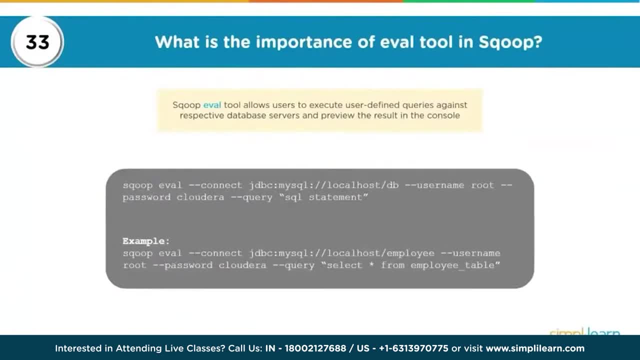 what is the importance of eval tool? in Scoop So there is something called as eval tool. So Scoop eval tool allows users to execute user defined queries against respective database servers and preview the result in the console. So either I could be running a straight. 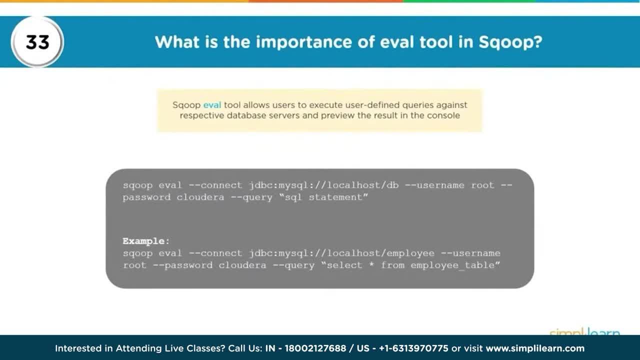 away query to import the data into my SDFS, or I could just use Scoop eval, connect to my external RDBMS, specify my username and password and then I could be giving in a query to see what would be the result of the query which we intend. 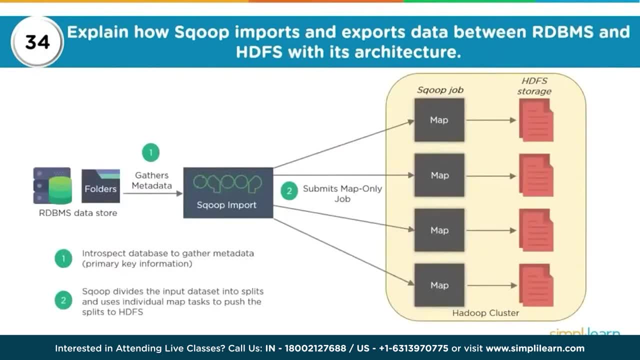 to import. Now let's learn about how Scoop imports and exports data between RDBMS and SDFS with its architecture. So RDBMS, as we know, has your database structures, your tables, which all of them are logical, and internally there is always. 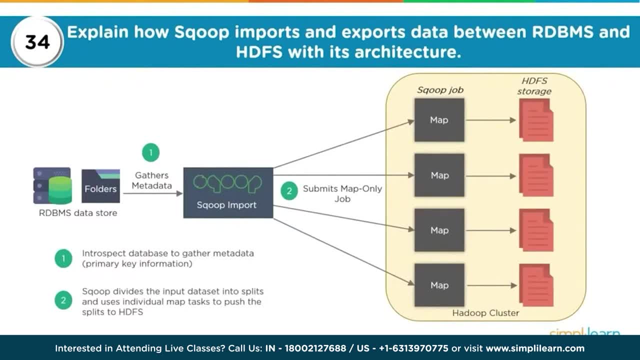 metadata which is stored. Your Scoop import connects to an external RDBMS and for this connection it uses an internal connector jar file which has a driver class. So that's something which needs to be set up by admin, but they need to make sure. 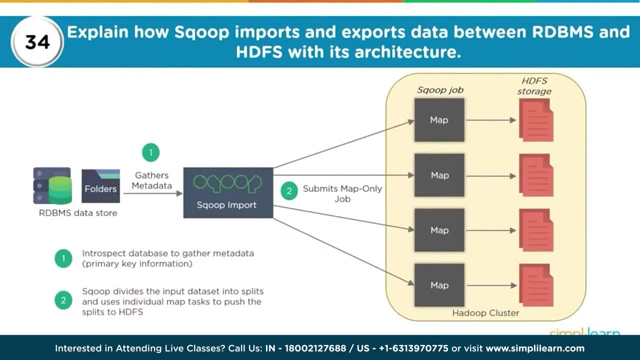 that whichever RDBMS you intend to connect to, they need to have the JDBC connector for that particular RDBMS stored within the Scoop lib folder. So Scoop import gets the metadata and then for your Scoop command it converts that into a map. only job. 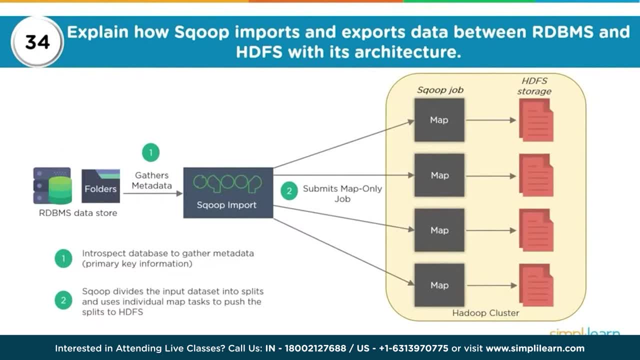 which might have one or multiple map tasks. Now, that depends on your Scoop command. you could be specifying that you would want to do a import only in one task or in multiple tasks. These multiple map tasks will then run on a section of data from RDBMS and. 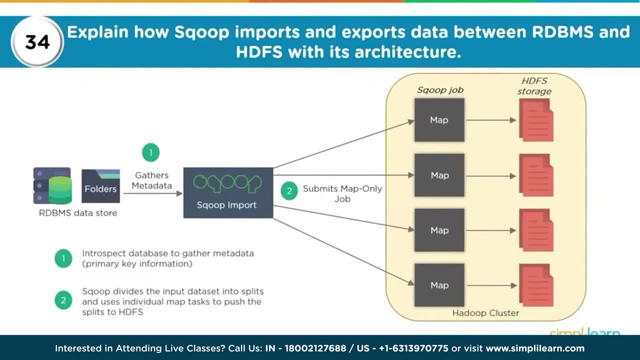 then store it in SDFS. So at high level we could say: Scoop will introspect database to gather the metadata. it divides the input data set into splits and this division of data into splits mainly happens on primary key column of the table. Now, if somebody might ask, 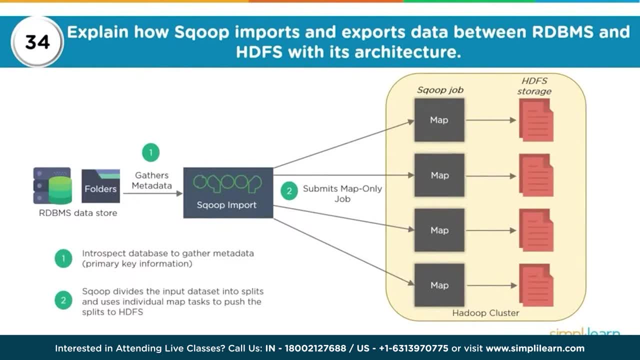 what if my table in RDBMS does not have a primary key column? then when you are doing a Scoop import, either you will have to import it using one mapper task by specifying hyphen- hyphen m equals one- or you would have to say split by parameter to specify. 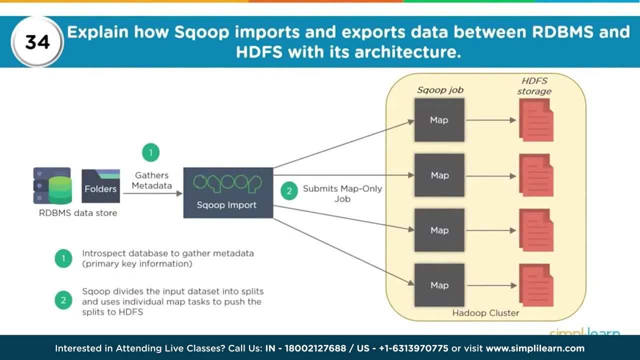 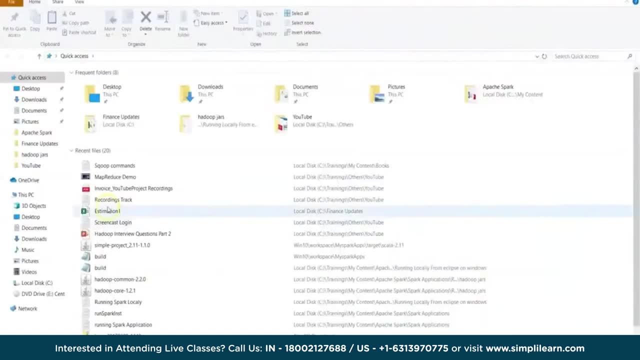 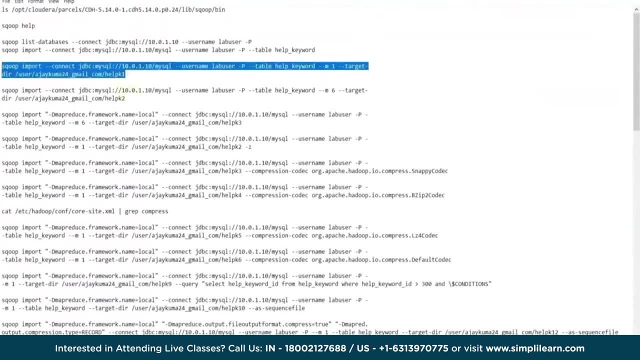 a numeric column from RDBMS and that's how you can import the data. Let me just show you a quick example on this, so I could just look in again into the Scoop command file and here we could be looking at an example. so if you see this one here, 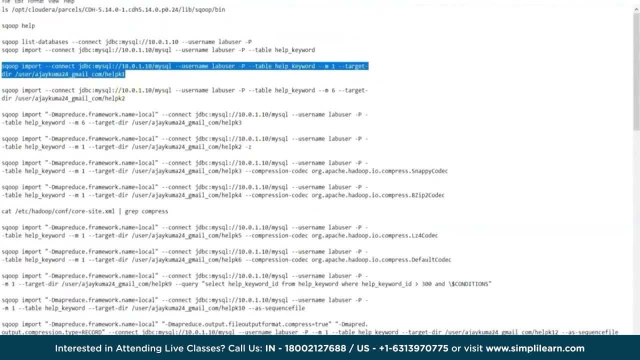 we are specifying, minus minus m equals one, which basically means I would want to import the data using one map task. now, in this case, whether the table has a primary key column or does not have a primary key column will not matter, but if I say a minus minus m is, 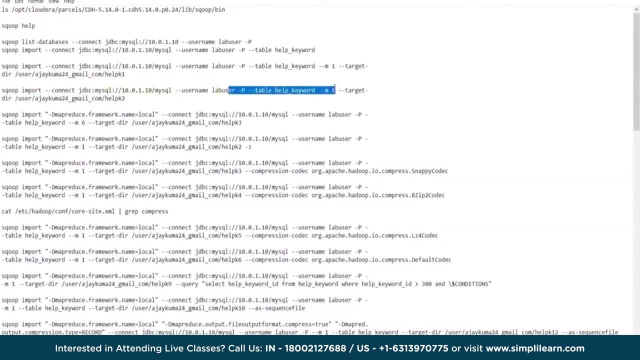 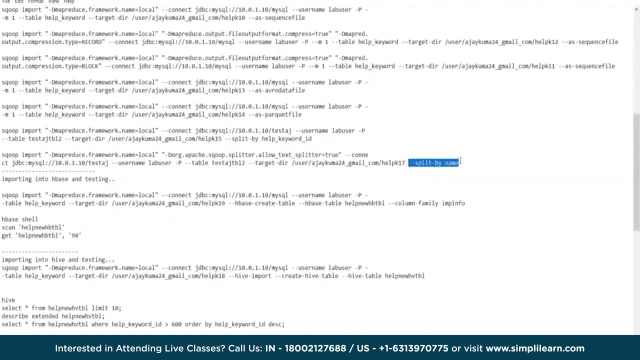 six, where I am specifying multiple map tasks to be imported, then this will look for a primary key column in the table which you are importing Now. if the table does not have a primary key column, then I could be specifying a split by and then specify the column. so 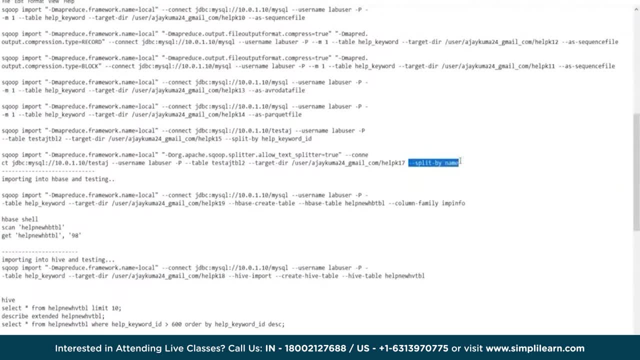 that the data could be split into multiple chunks and multiple map tasks could take it. Now, if the second scenario is your table does not have a primary key column and it does not have a numeric column on which you could do a split by in that case, and 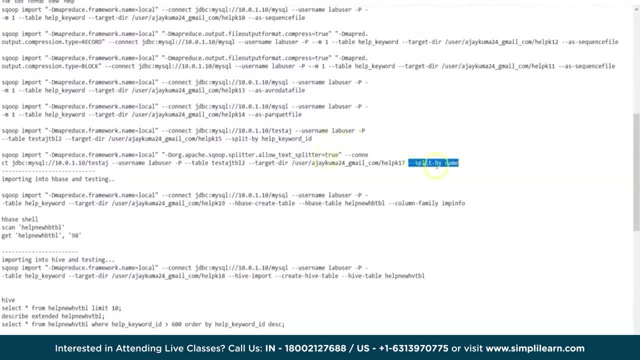 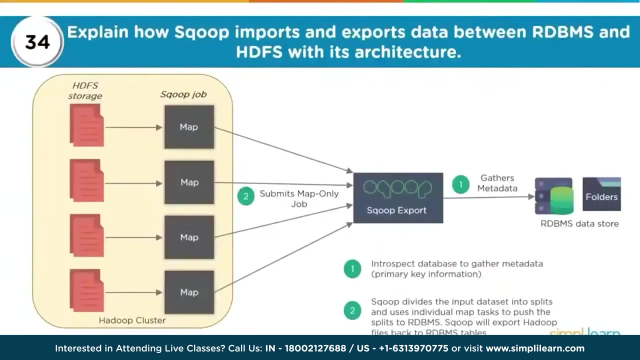 if you would want to use multiple mappers, you could still say split by on a textual column, but you will have to add this property so that it allows splitting the data which is non numeric. All of these options are given in the scoop: apache dot org. link Going further. 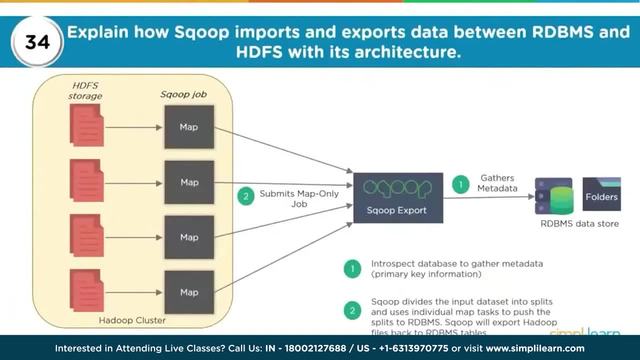 how scoop imports and exports data between RDBMS and SDFS with its architecture. so, as I said, it submits the map only job to the cluster and then it basically does a import or export. So if we are exporting the data from SDFS, in that case again, 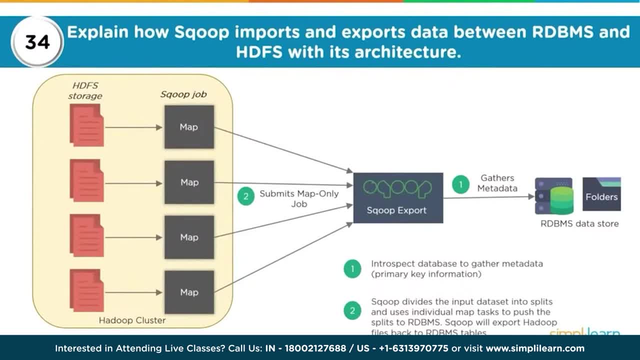 there would be a map only job. It would look at multiple splits of the data which is existing, which your map only job would process through one or multiple map tasks and then export it to RDBMS. Suppose you have a database- testdb- in MySQL. 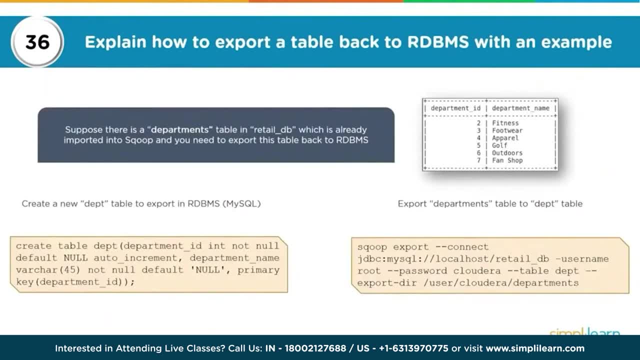 if somebody asked you to write a command to connect this database and import tables to scoop. So here is a quick example, as I showed you in the command file, so you could say: scoop, import. this is what we would want to do. You connect using JDBC. Now this will. 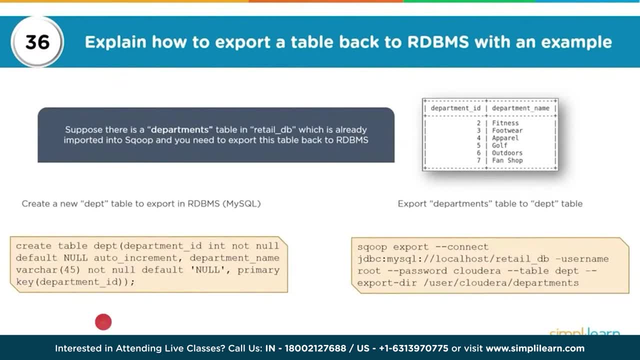 only work if the JDBC connector already exists within your scoop. lib directory. Admin has to set up that so you can connect to your RDBMS. You can point to the database. so here our database name is test, underscore db. I could give username and then either I could give password. 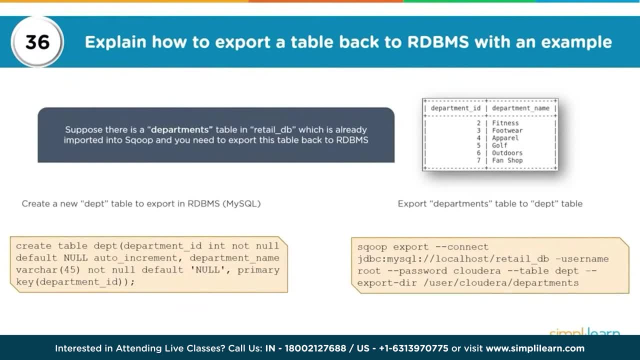 on the command line or just say capital P, so that I could be prompt it for the password and then I could give the table name which I would want to import. I could also be specifying minus minus m and specify how many map tasks do I want to use for this import. 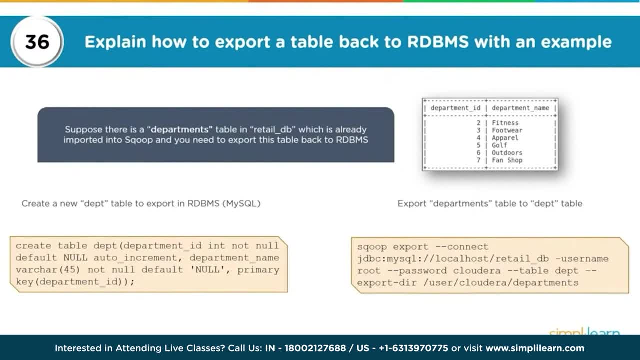 as I showed in previous screen, How to export a table back to RDBMS. now, for this we need the data in a directory on HDFS. So, for example, there is a departments table in retail database which is already imported into scoop and you need to export this table back. 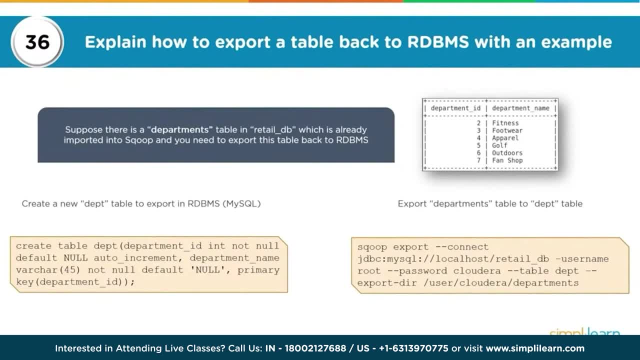 to RDBMS. So this is the content of the table. now create a new department table in RDBMS so I could create a table specifying the column names, whether that supports null or no, if that has a primary key column, which is always recommended, and then I can do a scoop. 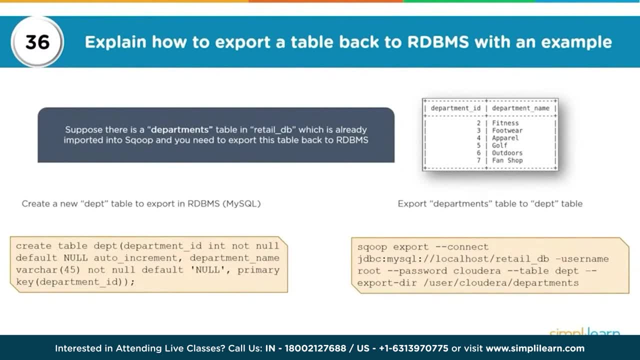 export. I can connect to the RDBMS specifying my username and password, specify the table into which you want to export the data and then you give export directory, pointing to a directory on HDFS which contains the data. This is how you can export data into table. 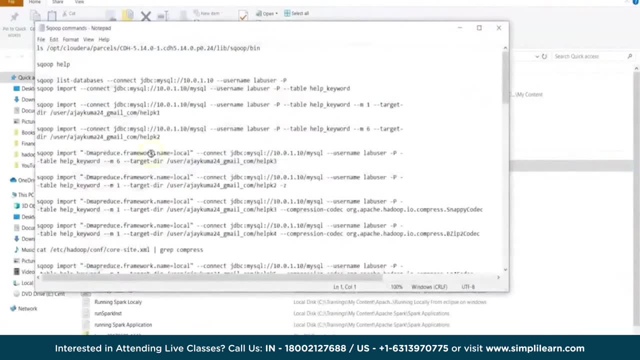 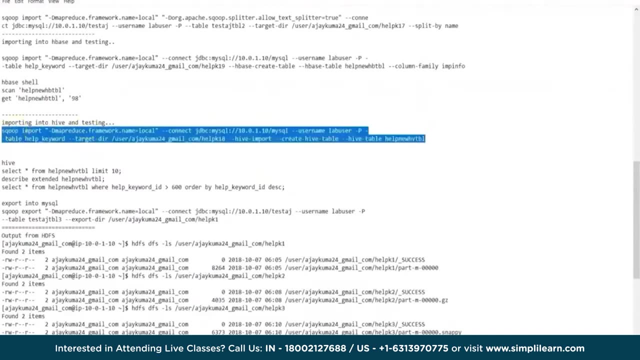 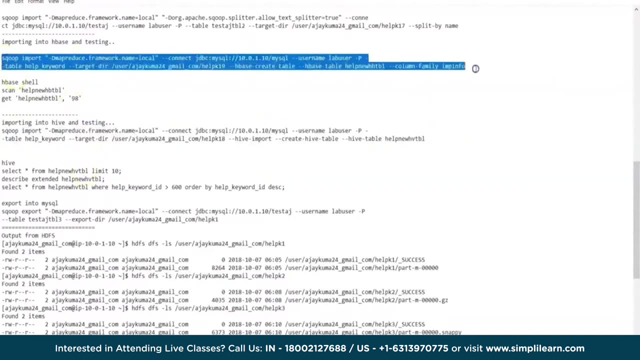 seeing example on this so I could again look into my file, and here I have an example of import. this is where you are importing data directly into HIF and you have scoop import, where you are importing data directly into HBase table and you can then query your HBase table to. 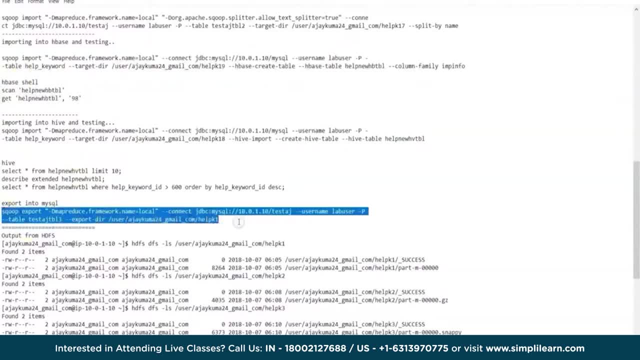 look at the data. you could also do a export by running your map only job in a local mode, connecting to the RDBMS, specifying your username, specifying the table where you would want to export and the directory on HDFS where you have kept the relevant data. this is: 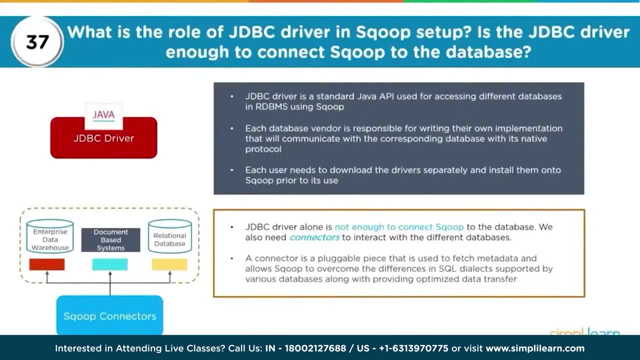 a simple example of export. looking further, what is the role of JDBC driver in scoop setup? so, as I said, if you would want to use scoop to connect to an external RDBMS, we need the JDBC ODBC connector jar file. now one or admin could download the JDBC connector jar. 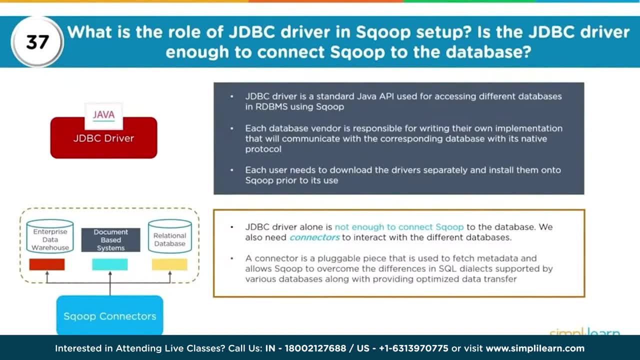 file and then place the jar file within the scoop lib directory wherever scoop is installed, and this JDBC connector jar file contains a driver. now, JDBC driver is a standard Java API which is used for accessing different databases in RDBMS, so this connector jar file is very much required. 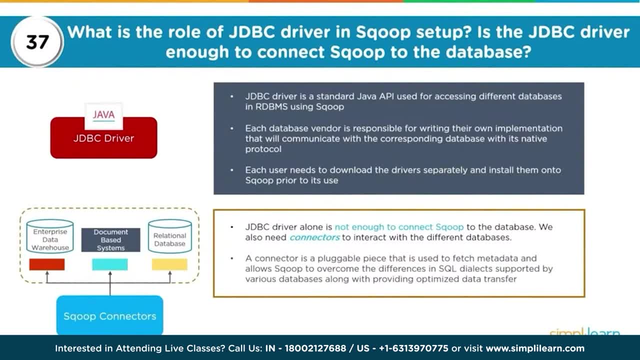 and this connector jar file has a driver class, and this driver class enables the connection between your RDBMS and your Hadoop structure. each database vendor is responsible for writing their own implementation that will allow communication with the corresponding database, and we need to download the drivers. 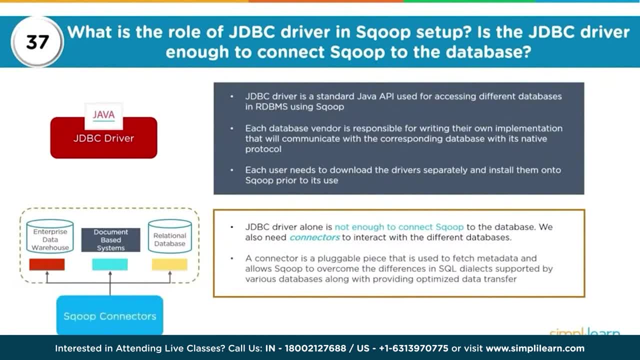 which allow our scoop to connect to external RDBMS. so your JDBC driver alone is not enough to connect to scoop. we also need connectors to interact with different database. so a connector is a pluggable piece that is used to fetch metadata and allows scoop to 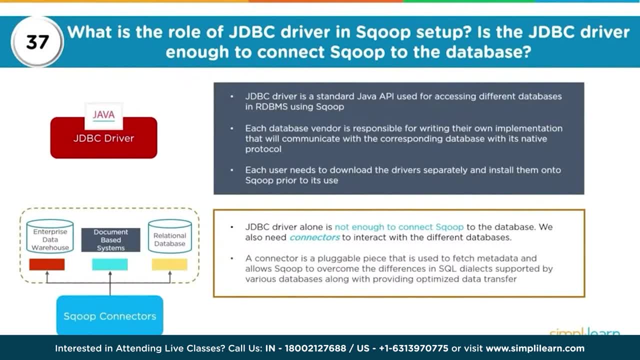 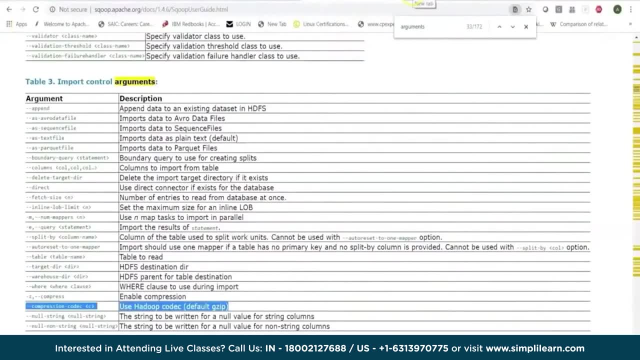 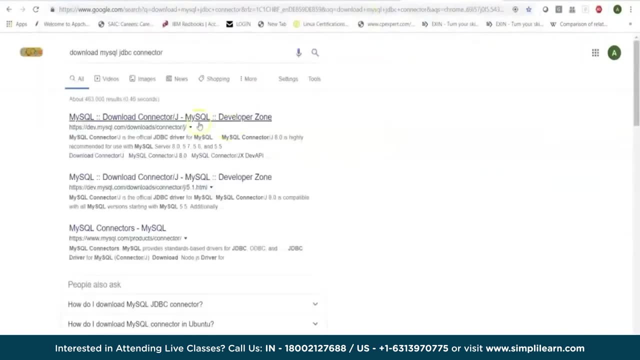 overcome the differences in SQL dialects. so this is how connection can be established. so normally your admins would, when they are setting up scoop and Hadoop, they would download, say, MySQL JDBC connector and this is how they would go to MySQL connectors. if you are connecting to MySQL similarly, 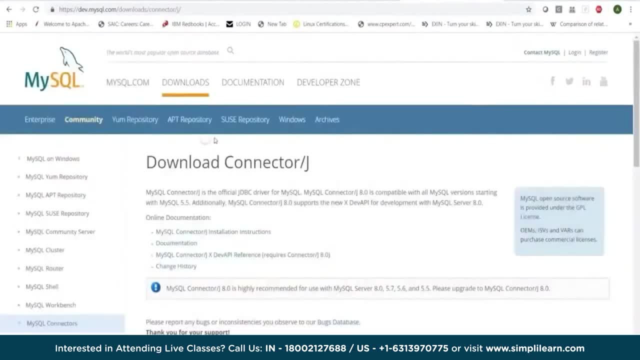 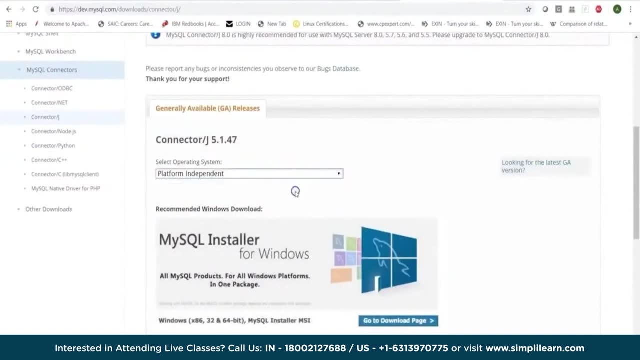 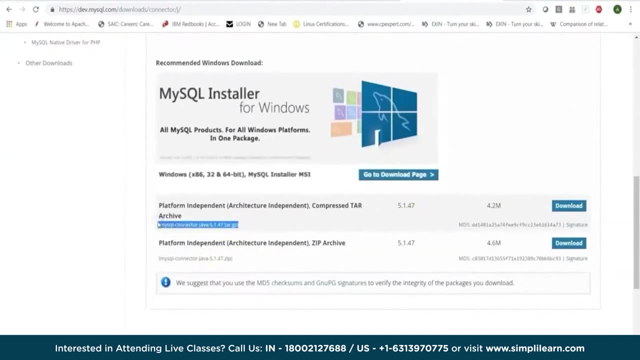 for your other RDBMS. you could be say, going in here you could be looking for a previous version, depending. you could be going for platform independent and then you could be downloading the connector jar file. now, if you untar this jar file, you would see a MySQL connector. 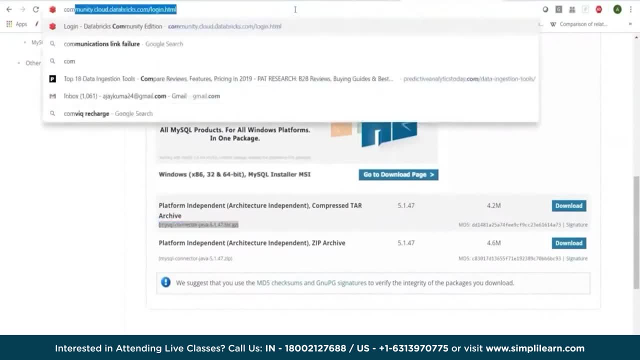 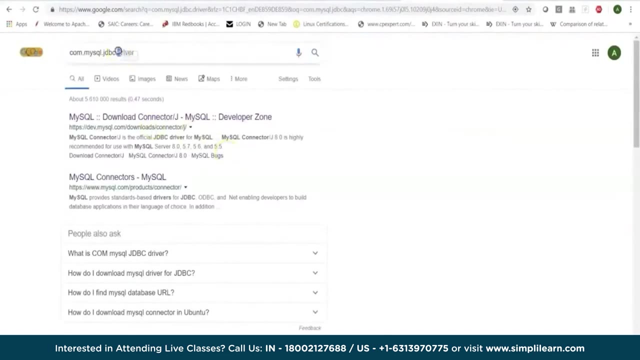 jar and if we look in, com dot MySQL dot. JDBC, com dot MySQL dot. JDBC dot, driver, so this is the package which is within the connector jar file and this has the driver class which allows the connection of your scoop with your RDBMS. so these things will have to be. 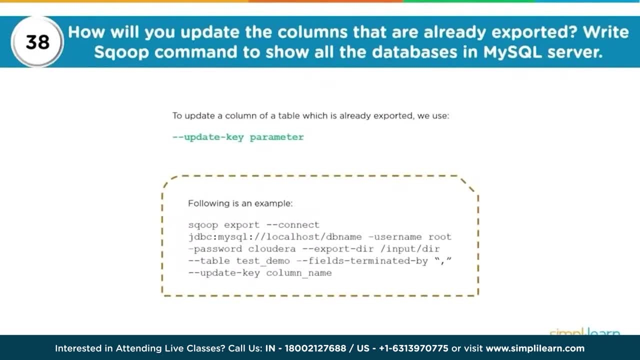 done by your admin so that you can have your scoop connecting to an external RDBMS. now how do you update the columns that are already exported? so if I do a export and I put my data in RDBMS, can I really update the columns that are already exported? yes, I 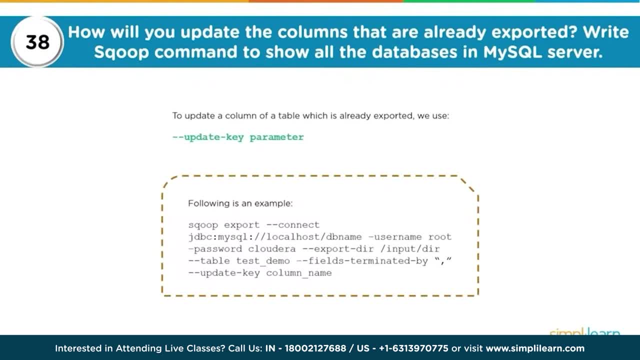 can using a update key parameter. so scoop export command remains the same. the only thing I will have to specify now is the table name, your fields terminated by- if you have a specific delimiter, and then you can say update key and then the column name. so this allows us to update. 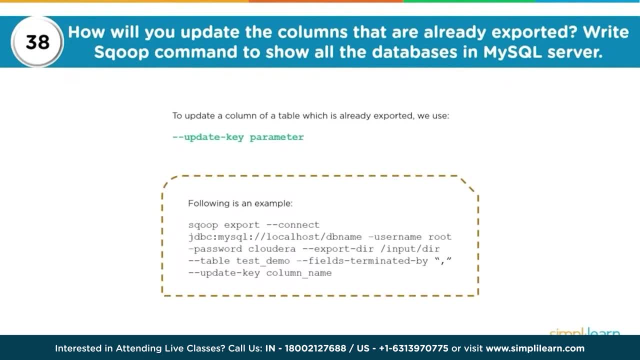 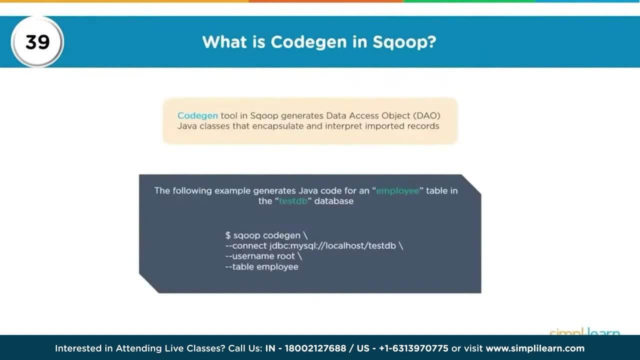 the columns that are already exported in RDBMS. what is code gen? so scoop commands translate into your map: reduce job or map only job. so code gen is basically a tool in scoop that generates data access objects, DAO, java classes that encapsulate and interpret imported records. so if I do a 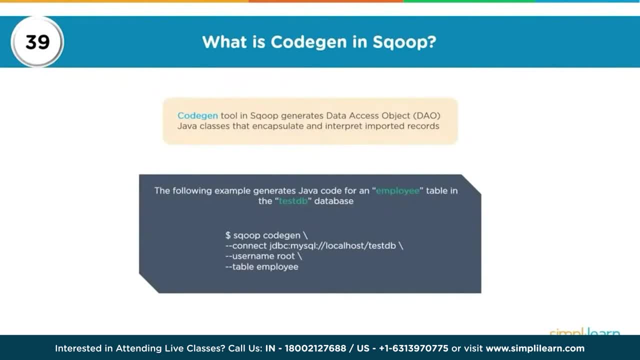 scoop code gen. connect to an RDBMS using my username and give a table. this will generate a java code for employee table in the test database. so this code gen can be useful for us to understand what data we have in this particular table. finally, can scoop be used to? 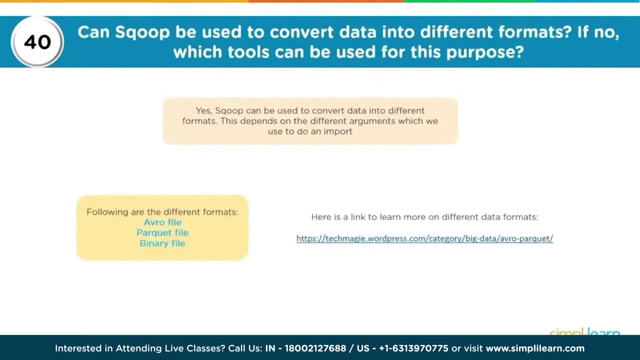 convert data in different formats? I think I already answered that right. if no, which tools can be used for this purpose? so scoop can be used to convert data in different formats, and that depends on the different arguments which you use when you do a import, such as Avro file. 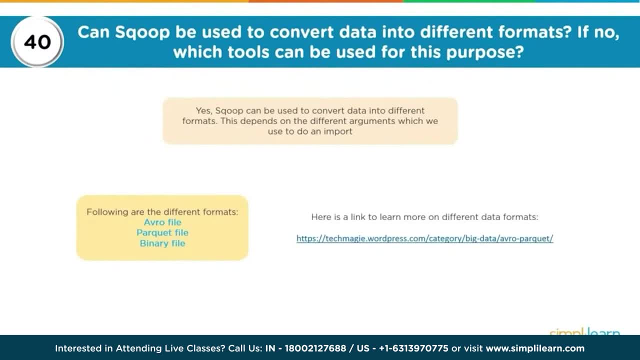 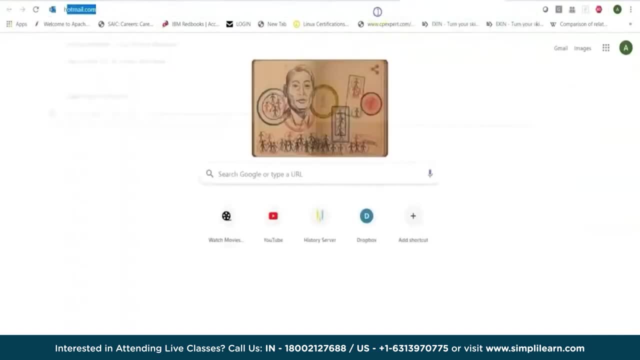 Parquet file binary format with record or block level compression. so if you are interested in knowing more on different data formats, then I think I can suggest a link for that and we can say Hadoop formats. I think it is tech, Maggie Avro Parquet, let's see. we can find out the. 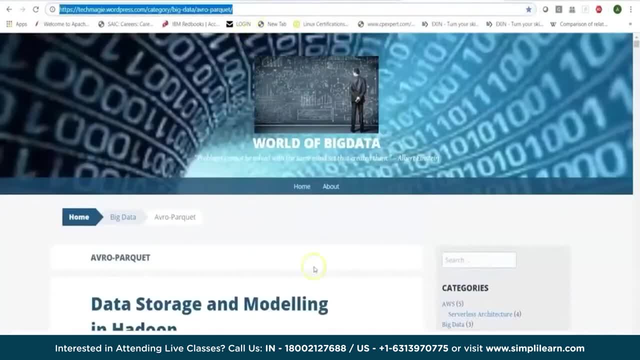 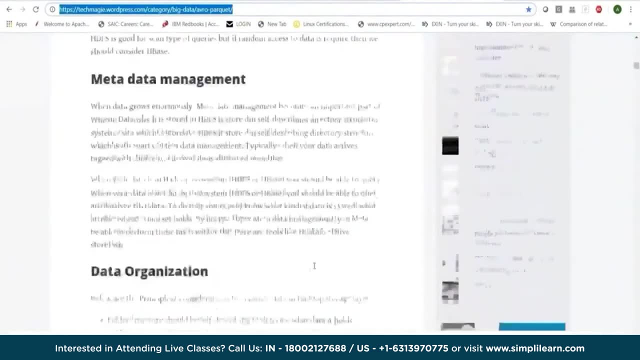 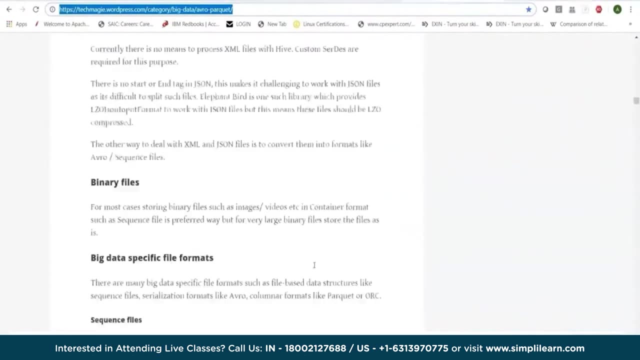 link tech. Maggie, this is a very good link which specifies or talks about different data formats which you should know, such as your text file format, different compression schemes. how is data organization? what are the common formats? what do you have in text file structure? binary sequence, files with compression without 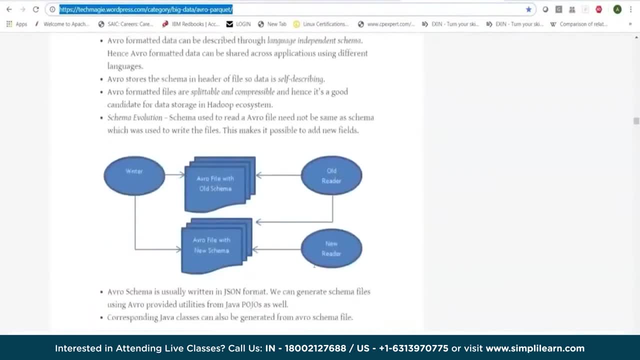 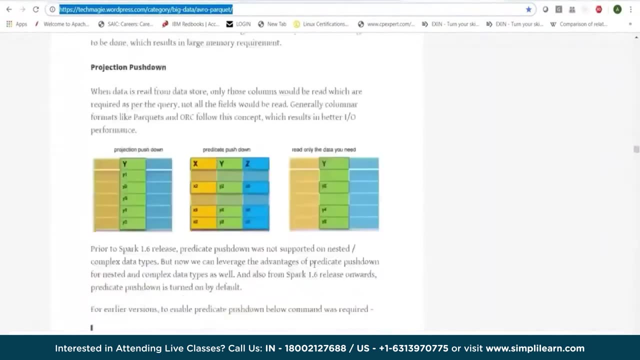 compression? what is record level? what is block level? what is a Avro data file? what is a? what is a Parquet file data file or a columnar format and other formats like ORC, RC and so on. so please have a look at this. so with this we have. 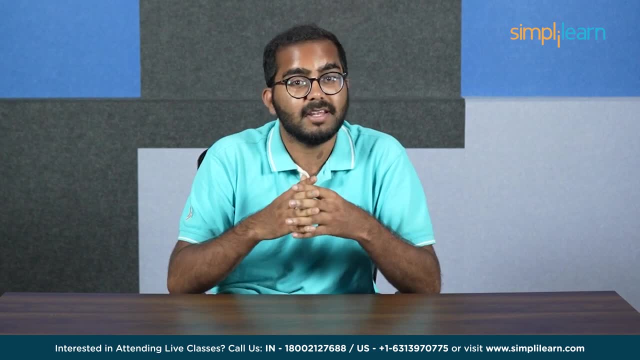 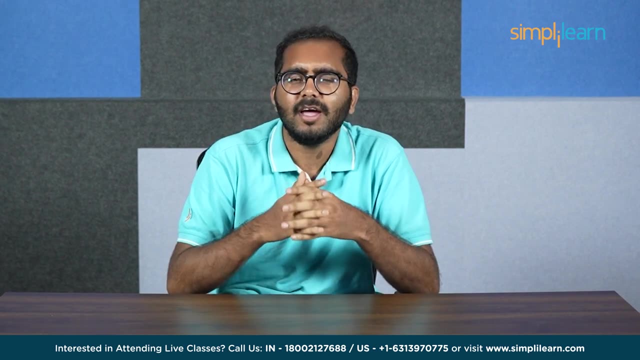 come to the end of this advanced big data full course. if you have found this session informative and interesting, please consider subscribing to YouTube channel. let us know our queries in the comment section below and our team of experts will be more than happy to resolve all your queries.